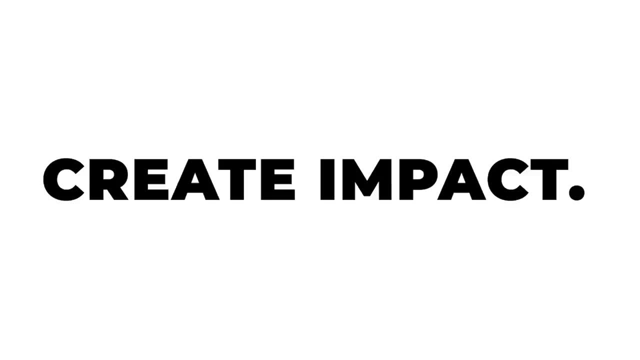 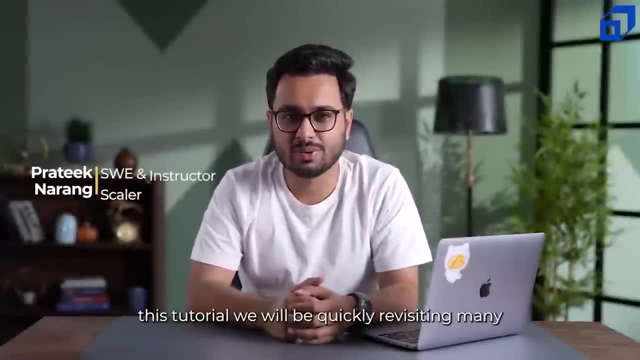 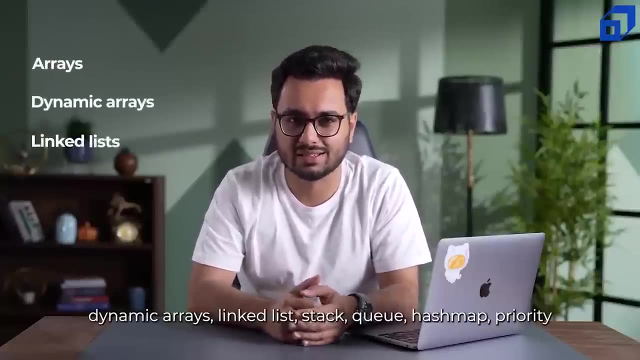 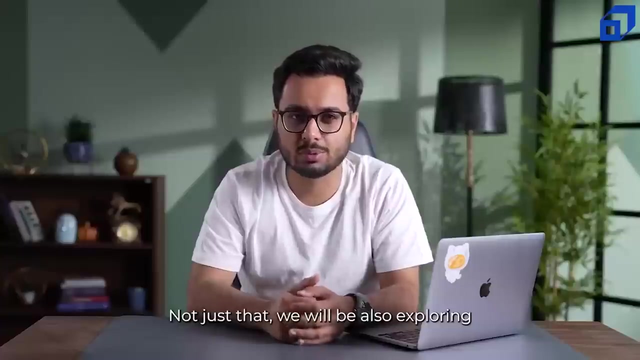 Hi, my name is Prateek Narayan, and in this tutorial, we will be quickly revisiting many fundamental concepts associated with data structures like arrays, dynamic arrays, link list, stack queue, hash map, priority queue and much more. Not just that, we will be also exploring Java's collection framework to use these data structures. 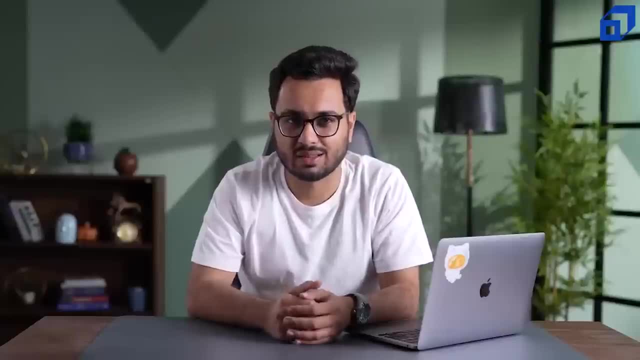 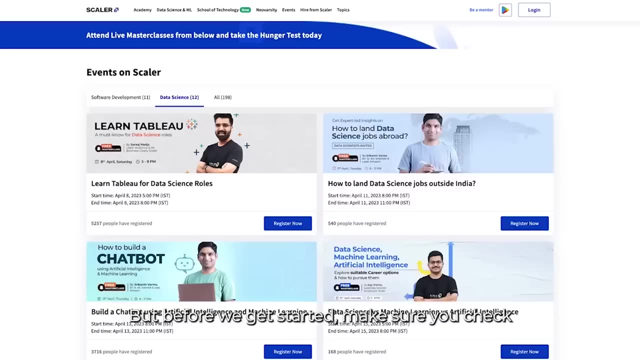 in solving problems and building real software. We will do many hands-on examples that will solidify your understanding of these concepts. But before we get started, make sure to check out free masterclasses on Scalar's event page to learn from the best industry-leading. 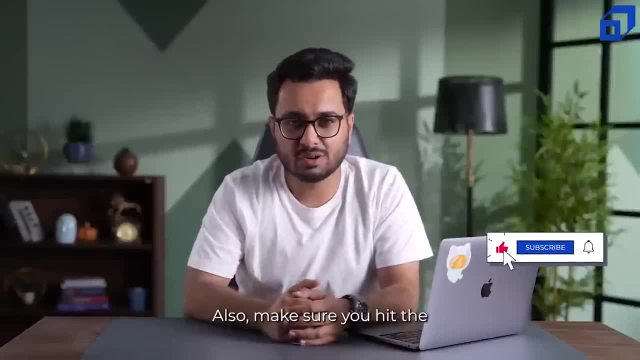 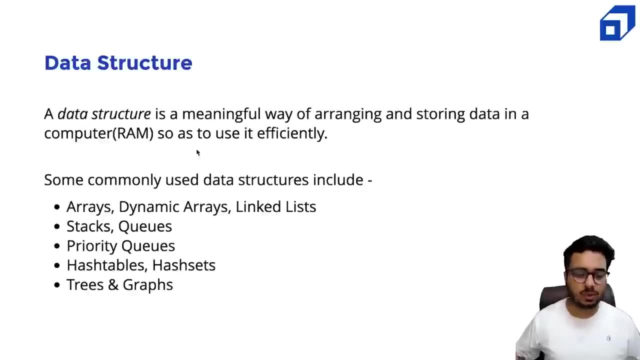 experts. The link is in the description below. Also, make sure you hit the subscribe button if you haven't already. Alright, so let's begin with the tutorial. Let us start by revisiting the concept of a data structure. A data structure is a meaningful 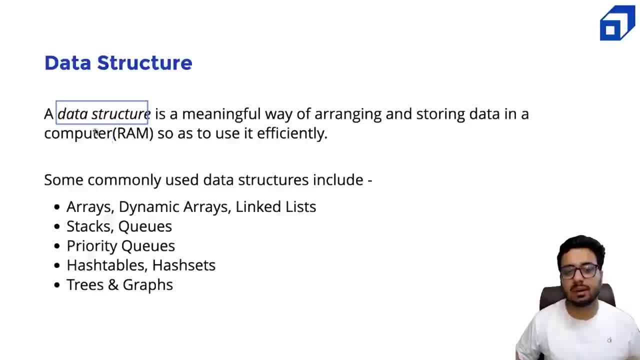 way of solving problems and building real software. A data structure is a way of solving problems and building real software. A data structure is a way of solving problems and building real software. A data structure is a way of solving problems and building real software. The first concept is data structure: A network of complex networked parts and 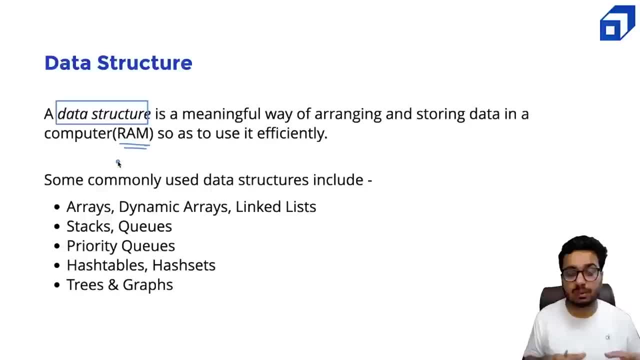 all the last, like fractional blocks. It is a way of gathering arrays, stacks, queues, hash tables, trees and graphs. Every data structure has its own properties, own way of ordering data, own way of implementing these operations. We'll try to understand how these data structures are different and 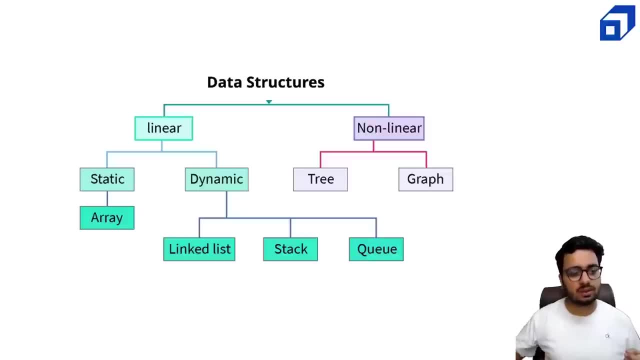 how we can use them in Java as well. Broadly speaking, they are divided into two categories. We have linear data structures. we have nonlinear data structures. There is one more category, I would say. we have associative data structures, in which we store data in the form of key value pairs, For example your. 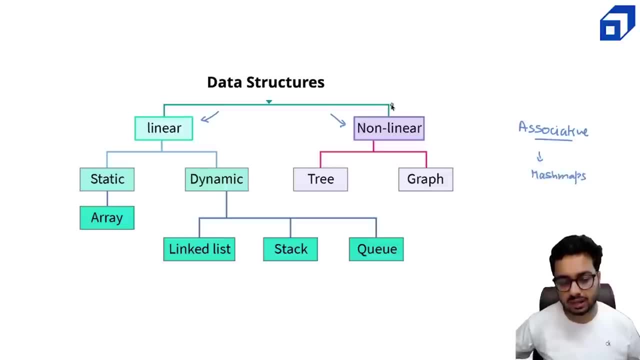 hash maps. We will talk about hash maps later in this course. Those linear data structures: they can be of fixed size, like a fixed size array, or they can be dynamic. that means they can grow and shrink in size. For example, your array list, your linked list, your stack, your queue In nonlinear. 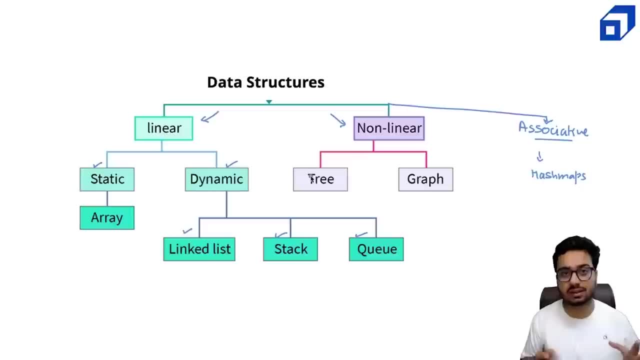 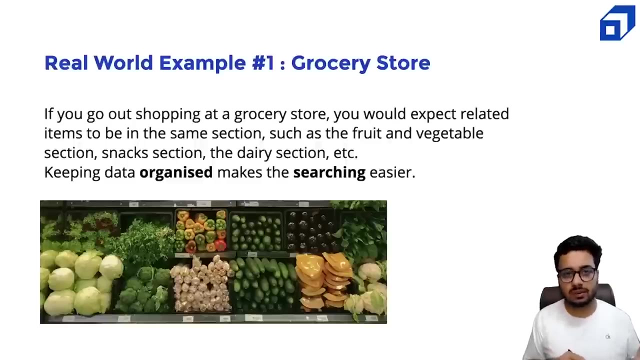 data structures. we might have data structures which have a hierarchical structure, for example, your trees Also have data structures which have network like data structure, for example. This is a very high level overview of how data structures are classified. But let us start by revisiting the importance of 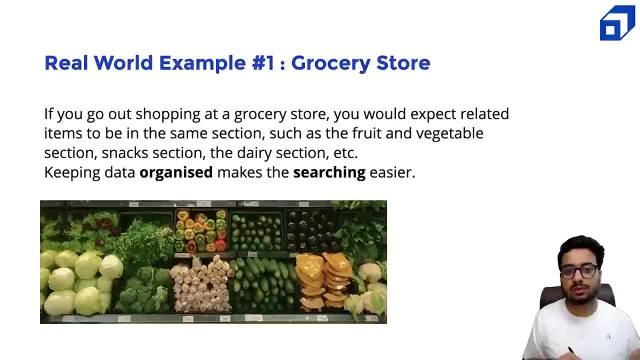 data structures in our real life. So suppose you go to a grocery store and you find everything is disorganized. Then it would become very difficult for you to search for a given item. But if your items are organized across racks and categories, you will easily find a particular item that you 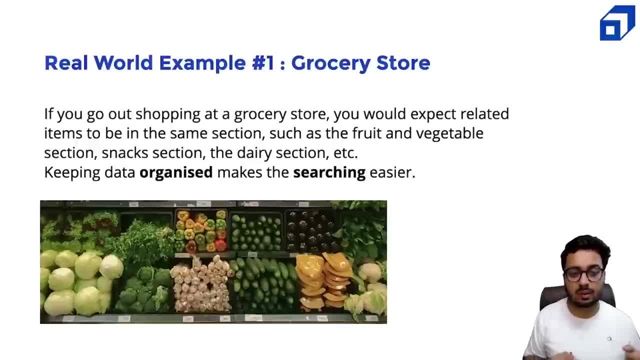 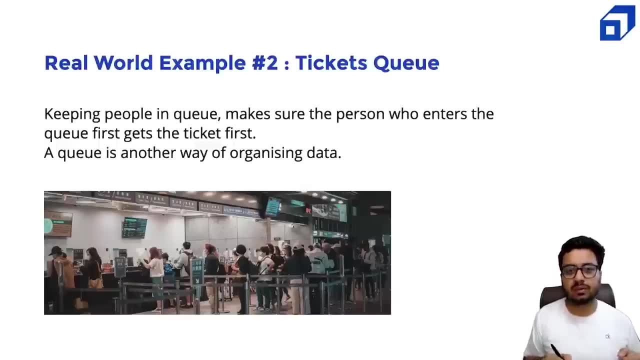 are looking for. So keeping data organized makes certain operations like your searching, faster. Similarly, if you go to tickets and if there is no queue, then it would be very unfair for the people to wait randomly. But if people are organized on the basis of their priority- the person who is coming- 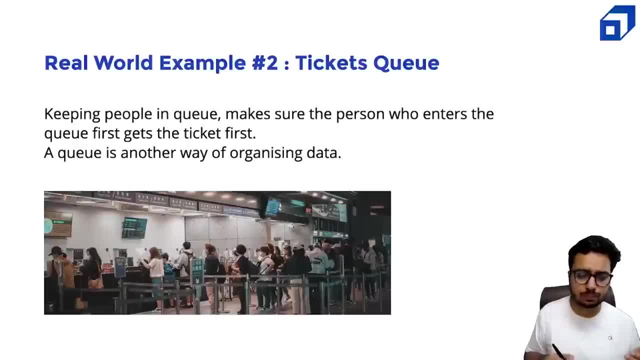 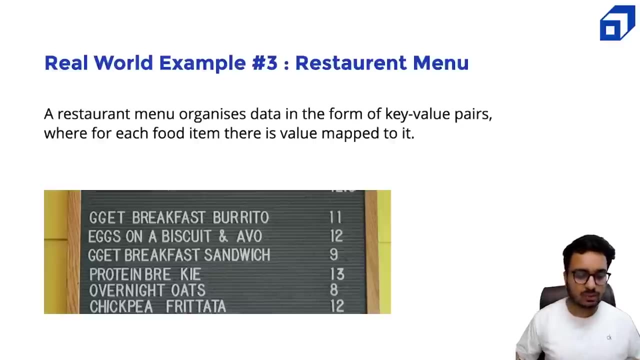 first and he is getting the queue ticket first. then it is called as FIFO ordering. Similarly, in data we might require FIFO ordering. So queue is a data structure that provides us with this kind of ordering. And let us look at one more example. Sometimes I go to a restaurant and I say I want to order a burger. Then I quickly. 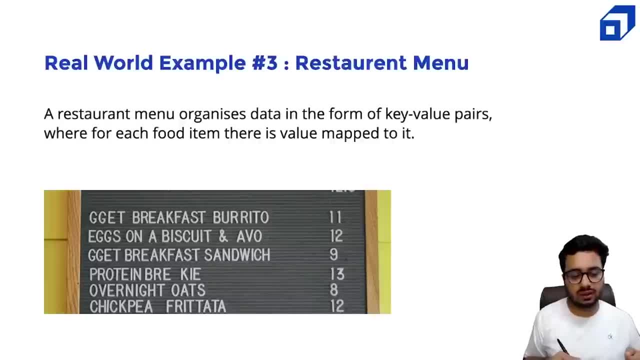 get an answer that the burger cost is rupees 100.. What is happening? For every item, there is a value attached to it, So for every key there is a value. So the data can might be stored in the form of key value pairs. And this is where some 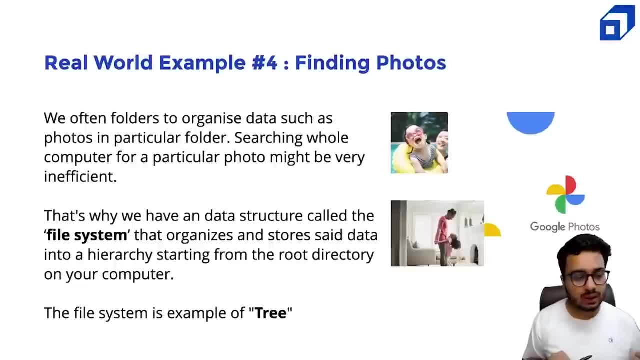 other data structures like queue order, order order order order order order- hash maps, come into the picture. Another example could be that if I am on my system and I am locating certain files, I know that in this folder I have kept this kind of a data. in this folder I have kept my PDFs in. 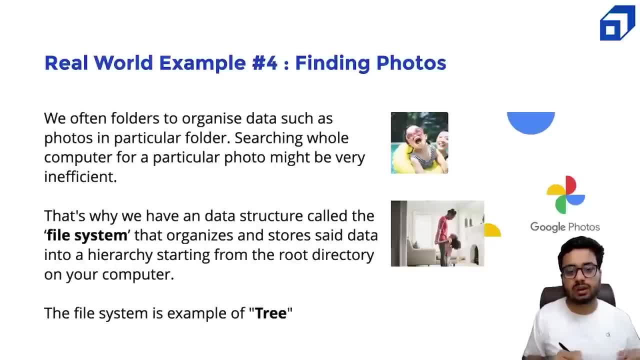 this folder. in this drive I have kept my pictures. What is your file system? The file system is a tree like structure. You start with your- my computer, you go to your drive, then you go to certain folders and you find the files that. 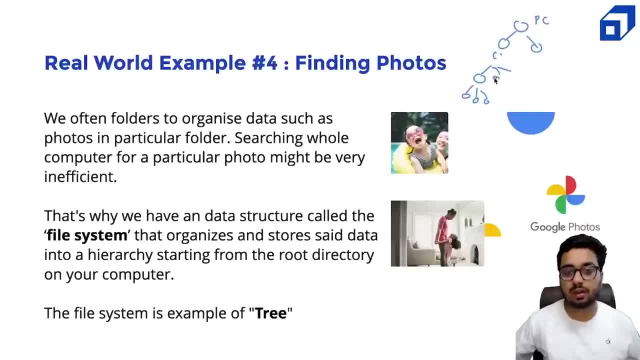 you are looking for. You do not organize this data in the form of a hierarchy, and if so, I will search the whole computer. It would be very inefficient for you and you will spend a lot of time searching for a given file. The file system is also an example of a tree like data structure. That 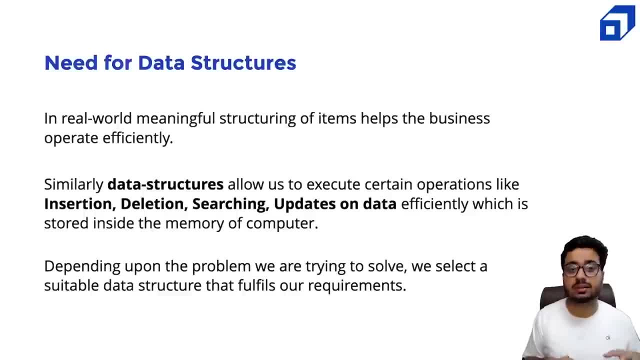 means we use data structures a lot in our daily life, in building software applications. In real world also, the meaningful structuring of items helps businesses operate efficiently. We saw the example of grocery store, So similarly, data structures allow us to execute certain operations like insertion, deletion, searching, updates on the data very efficiently. and then 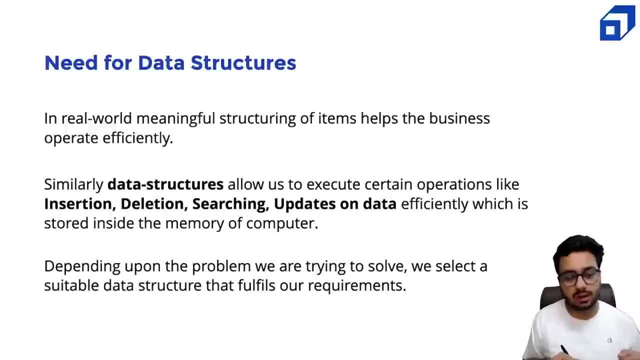 this data is stored inside the memory of the computer. Depending on the problem that we are trying to solve, we select a suitable data structure that fulfills our requirements. This is the goal of this video. In this lecture, we are going to understand how, according to different requirements, what data structure we will. 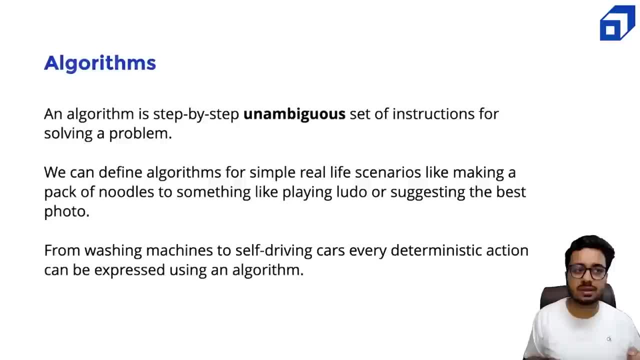 use and we will look at its implementation using Java collections framework. You might ask: okay, that's data structure. what is an algorithm then? Algorithm is the main logic. It is the step-by-step, unambiguous set of instructions for solving a problem. right, We can define algorithms for real-life. 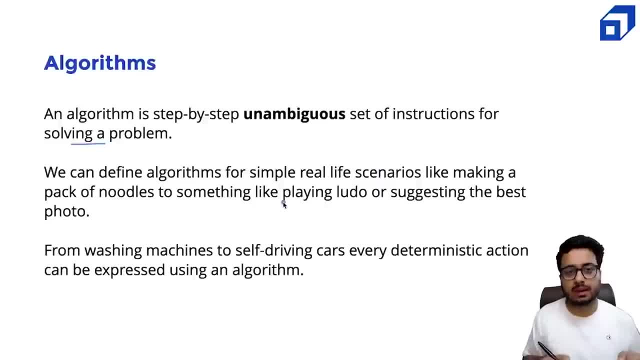 scenarios like making a pack of noodles, You might say, okay, take a pan, put two cups of water inside it, boil something, something. That list of instructions is an algorithm to make a pack of noodles. or maybe something complex, like if we want to play a Ludo game, or if I want to make an algorithm that suggests the best. 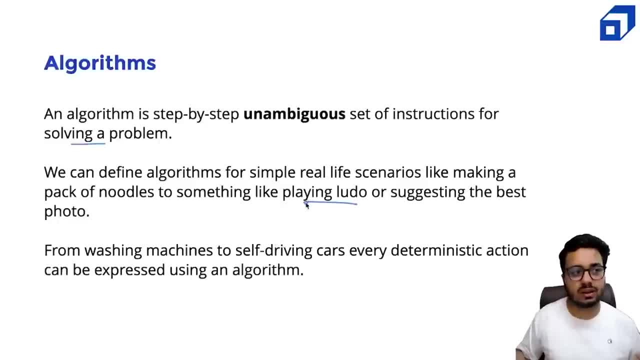 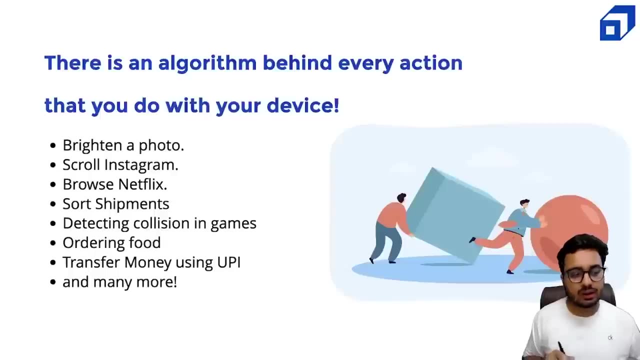 photo, out of a set of photos, We can devise an algorithm for that. So in real world, from every every deterministic action, for example, your washing machine, a self-driving car, all the actions your machines are taking- that can also be expressed using an algorithm In the software world, all the apps that you are using photo editing. 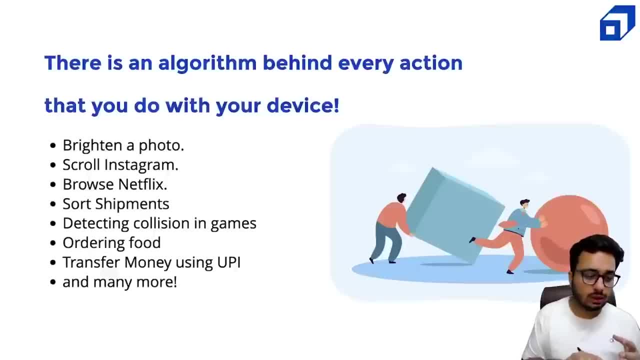 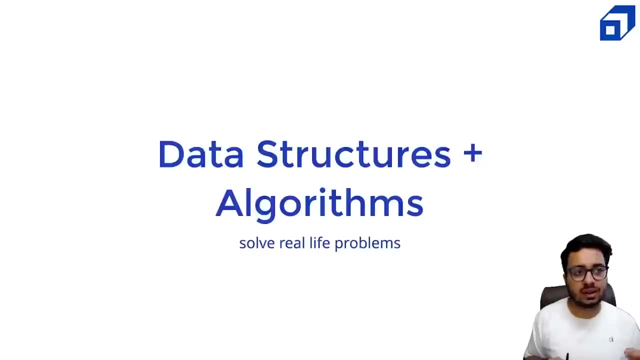 app scrolling, Instagram browsing, Netflix in a cargo hub, sorting of shipments, detecting collisions in games, transferring money through UAPI, ordering food. There is an algorithm behind every action that we perform, So that is why it is very important for us to learn data structures and algorithm right And when. 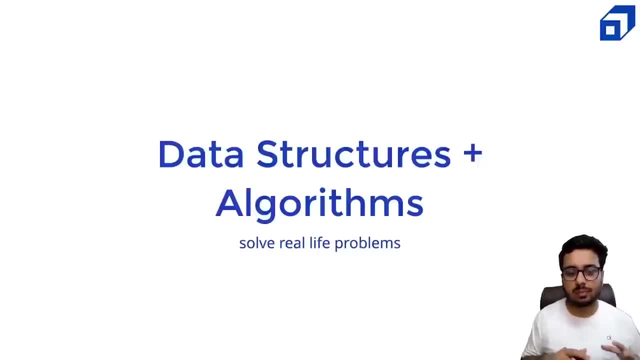 we combine data structures along with the algorithms, we build products that can solve real-life problems. That is an importance of data structures and algorithms. I will start with arrays. Let us start with the array, which is the simplest and the most widely used data structure. I am hoping most of you have. 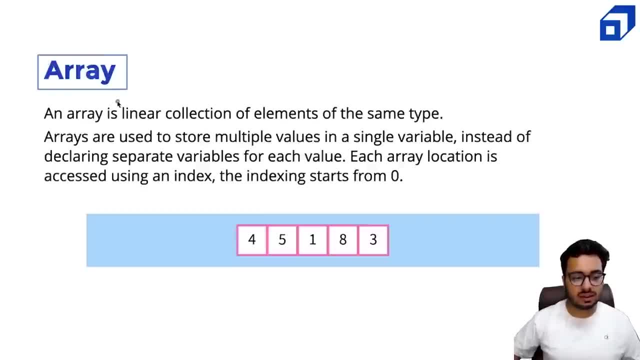 must have worked with an array. What is an array? Array is a linear collection of elements of the same string. If you want to learn about the string, you need to of the same type. so this is true for Java. other languages like Python, they. 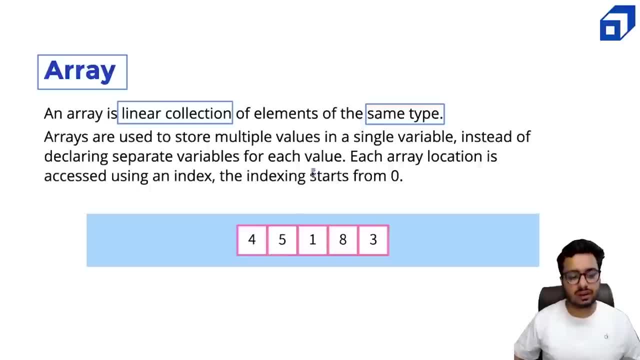 also support heterogeneous arrays. that means you can put different number, different types of data- for example integer string float- inside one array. arrays are used to store multiple values in a single variable. so let's say this is a container which is linear. that means it will occupy linear block of. 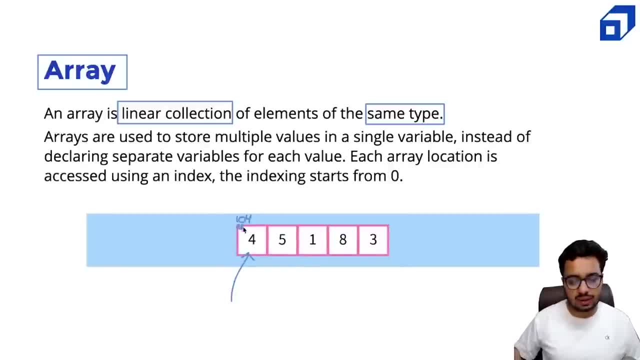 memory. for example, if this address is 104 and this bucket takes 4 bytes, the next address will be 108, next address will be 112 right, so it is a linear block of memory and this whole block of memory has a single name right and each element if I want to access it can be accessed using an index: the 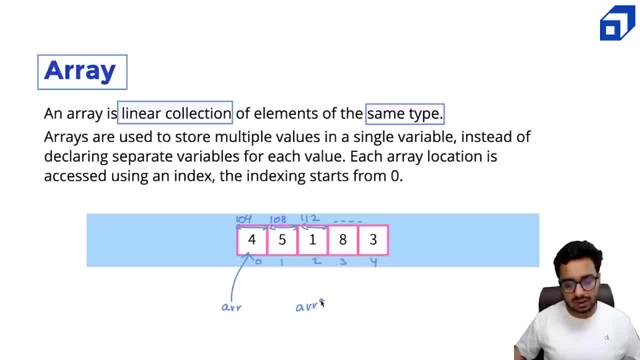 indexing starts with 0. so I can say, okay, I want to put something at area of 0. then I will say, area of 0, it is 4, I want to overwrite it. I will say, okay, area of 3, it's going to be 20, so I can. 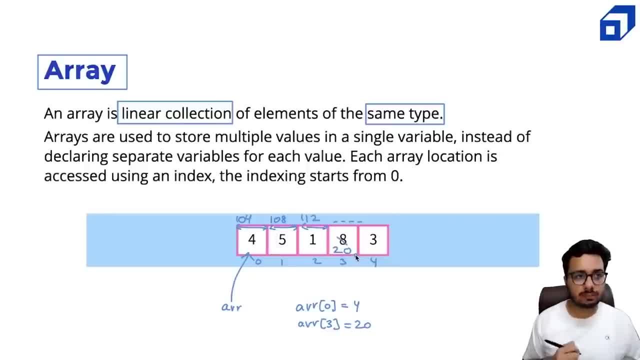 just overwrite this data and it will keep 20 right. each array location is accessed using an index. the indexing starts from 0. that is what we have just seen it, so we have the array name followed by the index. this is how you access the ith location inside an array. right now, let us look at some examples. 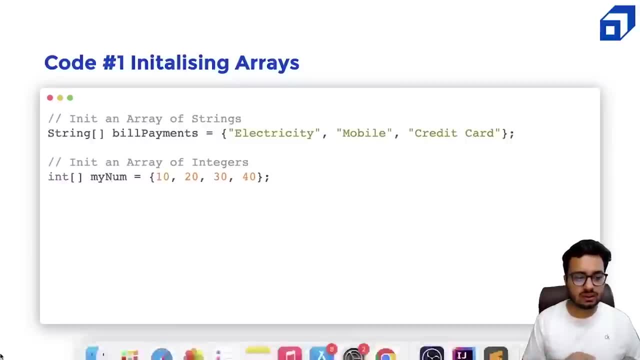 of an arrays. for example, if I want to create an array of strings in which I'm calling the variable as bill payments, I have defined three strings- electricity, mobile and credit card right- and I have an array of numbers. I have defined four numbers here. I have int, followed by 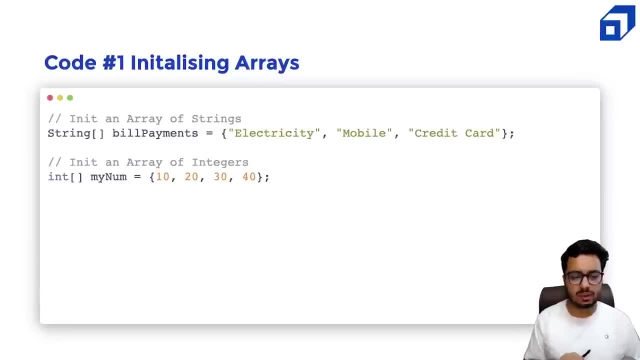 square brackets followed by name of the array. this is a very simple way of creating an array, but you can also create an array of fixed size where you have not given your data right. in the previous scenario, we have not defined the size. size will depend upon how many items we have initialized in this list. 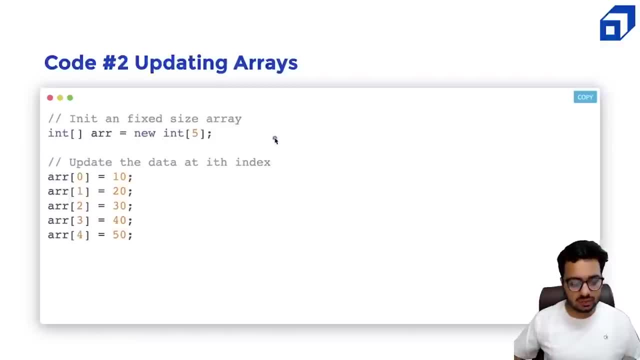 right, so you can directly initialize or you can first create a fixed size block. you can joke. I want an error that is able to hold five integers will use the new keyword, followed by the data type and followed by the size. what happens? it creates an array. so if I talk, 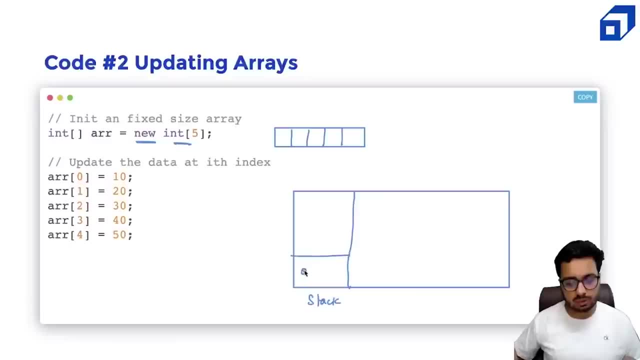 about Java, the variable ARR it most likely it goes into your back memory and the actual array that we have this. this is created in the keep memory line error we call as a object. reference error is holding the address of this array. error is going to hold 104. error is in the stack, whereas this: 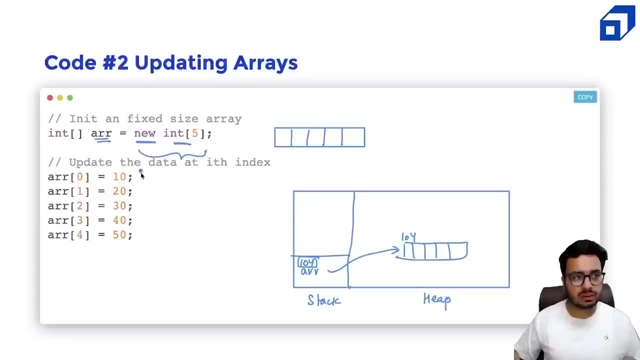 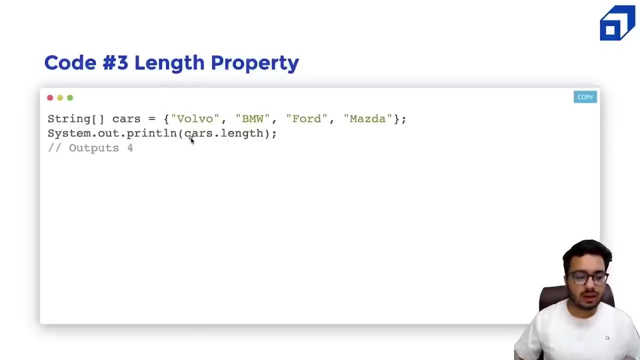 actual object. it is in the keep memory. now we are updating the data at the iith index. we are actually storing 10, 20, 30, 40 and 50 here. this is how you create an array and all the array objects. they have length property added to it. so if you say okay, 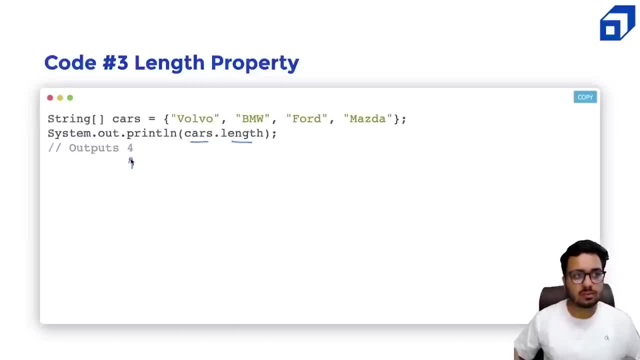 this is a length property and added to it. so if you say, okay, this is a cars area and i want to say cars dot length, this will give me, okay, how many objects are stored in this array or what is the size of this array. this will give me four. right, the size of this. 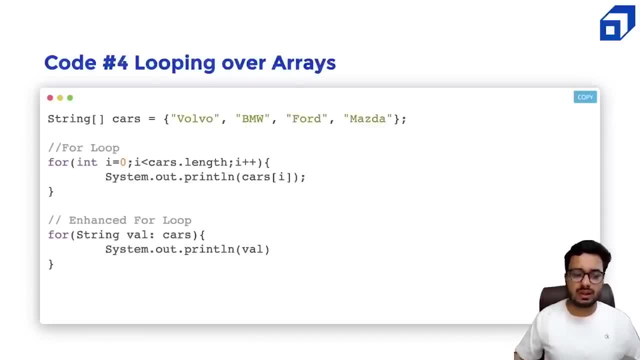 array and using the length property, i can also iterate over the arrays. right, so i can. okay, let me go over every index, from zero till cars dot length. that means i'm iterating from zero, one, two, three. the length is four. so i'm iterating over these indices and else, okay, let me print. 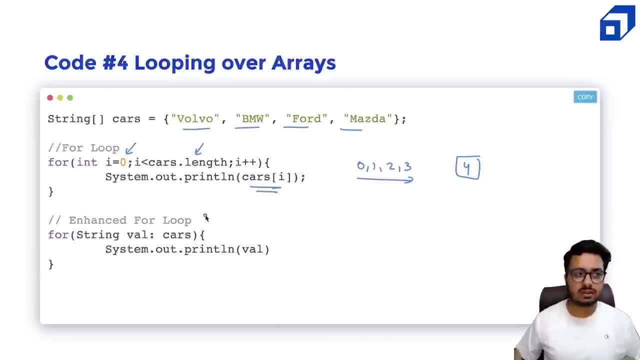 every car. i will print the ith object right, that is one way of iterating. using the length property you can get the size. other ways you can use a for each loop, or also called as enhanced for loop. you can okay for every string value that is there inside my um cars array. i want to go over that. 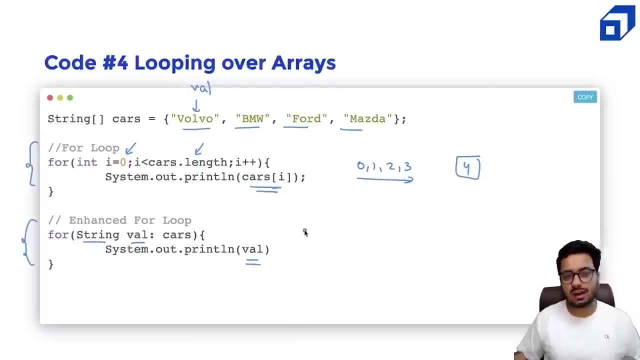 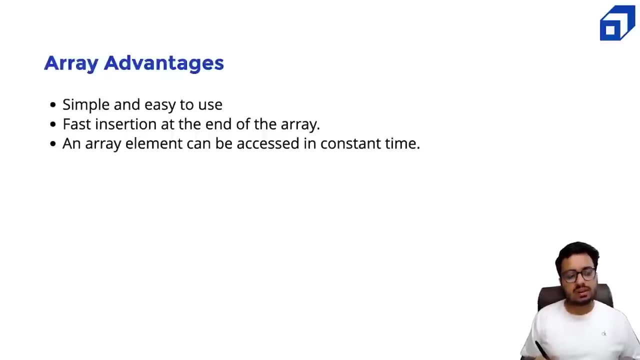 value and i want to print it. that is another way of iterating over the complete array object. then let's talk about the advantages of arrays. they are very simple and they are very easy to use. the insertion is really fast at the end of the array because if you keep a variable, that okay, these positions are filled. i want to put something here you can. 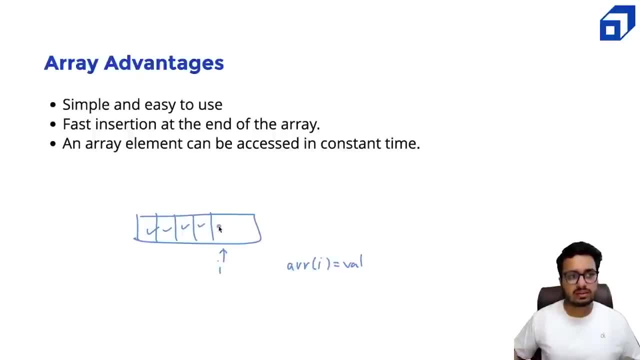 simply say: array of i equal to value, so that value will get stored here. you can insert at the end of the array very fast and array element can be accessed in a constant time. so if you want to get this element, you can simply say: okay, give me the jth element so you can access any random element, any random. 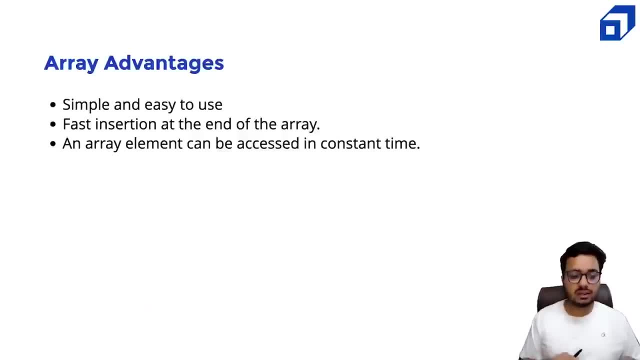 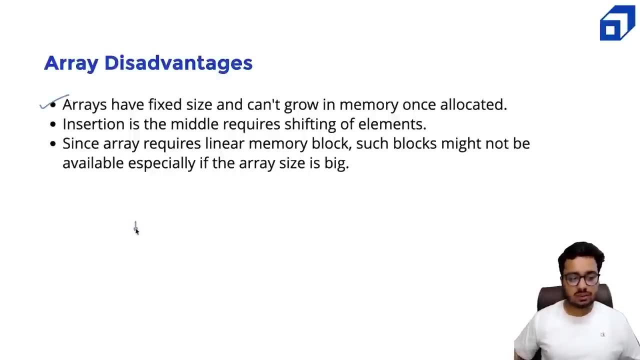 index and just order one time. that is an advantage of an array, but they also have certain disadvantages. the thing is, arrays have fixed size. so once you create an array- okay, new int of some size 10, you cannot say i will make it 15 or i will make it 20.. they have a fixed size. they cannot grow. 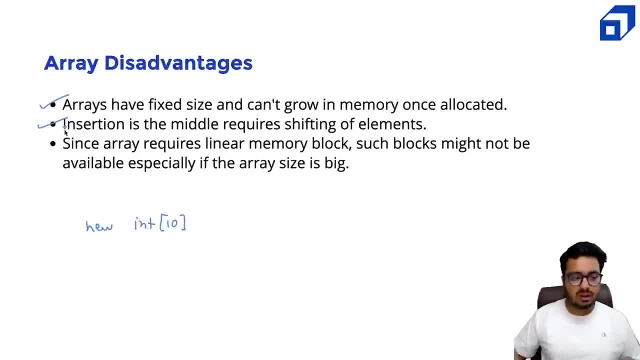 in memory once they are allocated. insertion in the middle requires shifting of the elements. if you have inserted something- let's say one, two, four, six, eight- and you say, okay, i want to insert three, what you will have to do? you will have to shift these elements to the right. then you can insert three in the middle. so it's going to take order of end time. 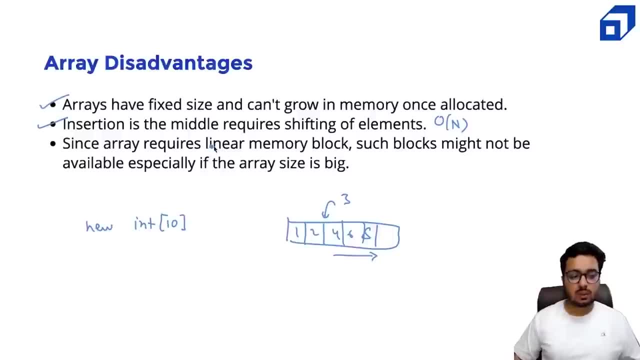 for doing the insertion. and second thing is, since array requires a linear memory block, such blocks might not be available if the array size is big. suppose this is your heap memory and suppose certain portions of the heap memory, they are already used up. right, and suppose if you. 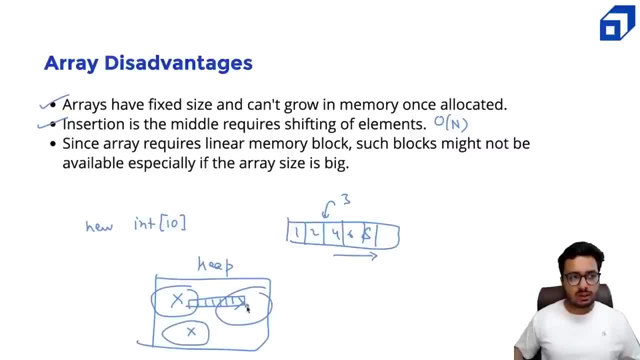 want to create a very big array which might go like this. now it is possible that such a linear block of memory is not available, but this amount of memory is available in the heap in chunks, right? so you might say, okay, some memory is available here, some memory is available here, some memory. 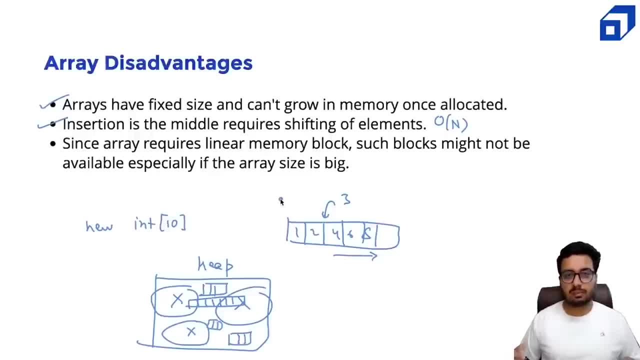 is available here. that is where linked list might perform better, because linked list does not need big linear chunk of the memory, whereas error requires a big linear chunk of the memory. right that such a linear block could not be present in the memory. now, arrays are used a lot in the real. 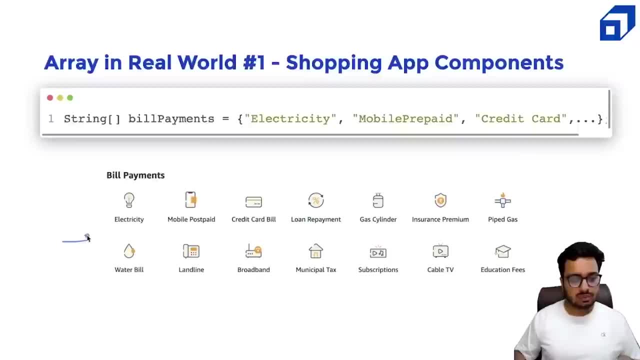 world. for example, this is a ui from a shopping website where i have to display these components right, the type of bill payments. i can say, okay, each bill payment is a string. so i have a fixed size array of bill payments in which i have defined all the categories. right now you might 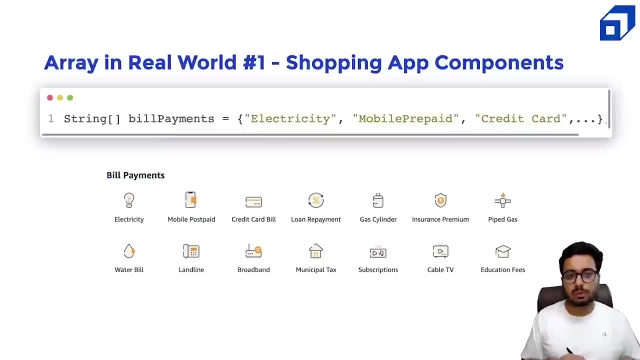 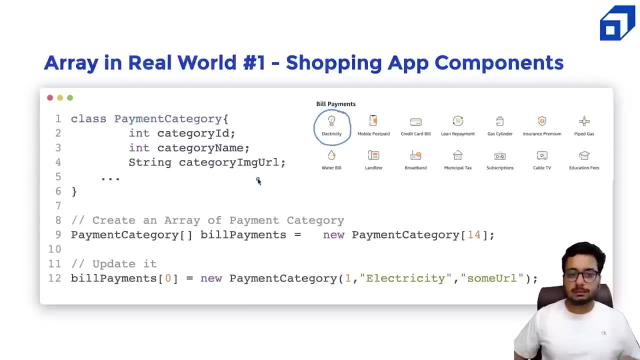 say: okay, this looks very simple. in actual world, it might be a bit more complicated. yes, it can be. what may happen is that each item is not just a string, but it is a- um, something more complex. let me call this as a payment category. what i can do? i can define a class called as payment. 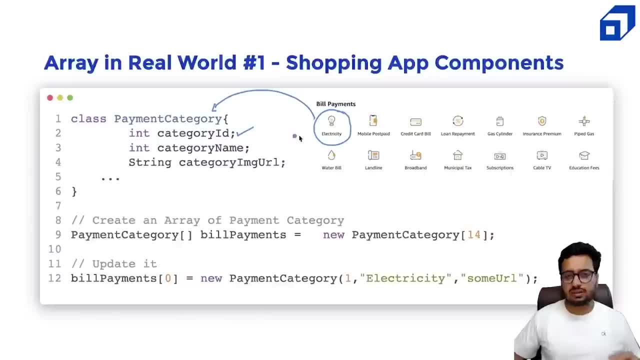 category which hold three things: maybe the category id, which is not displayed, the category name and the image of the category, right, the url of the image of the category. so i can hold all these things inside a class and then i can create an array of the following class. i can. 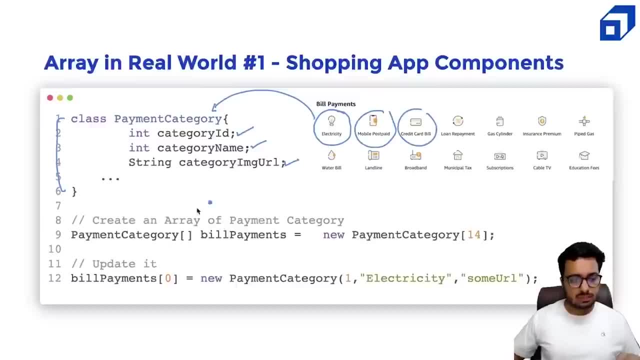 say: okay, i'm creating an array where each item is of the type payment category, right, so i'm creating an array of objects of the type payment category. i have initialized this array that is going to contain 14 items and i i need to create these objects as well. i need to say okay. 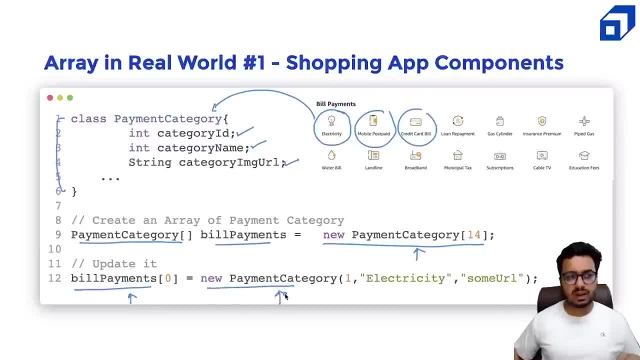 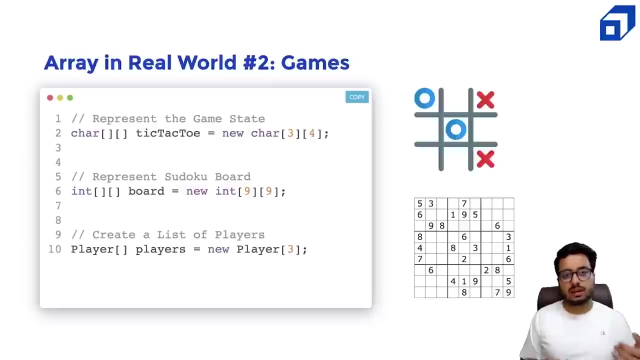 the bill payments of zero. it is going to hold new payment category and, using the constructor, i have initialized these values. okay, the payment category is one, the name is electricity. instead of creating an array of primitive data types such as integer or float, we can also create an array of complex data types such as payment categories, in this example right. secondly, there 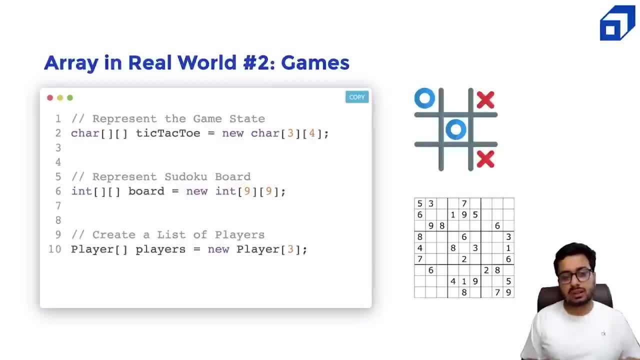 are two-dimensional errors as well, which are also used a lot, especially in games and puzzles. right here is an example of tic-tac-toe, where we might need a board, or here is an example of produco game, where might we might need a two-dimensional array to represent the 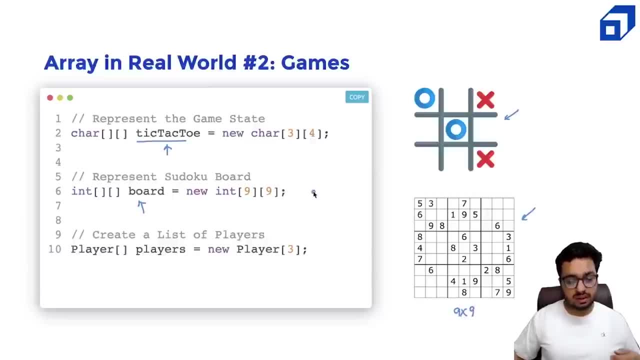 of the game, right. so it's a nine cross nine array. so i've created this array right, and i can also create a list of players. it's going to be a 1d array, but the data type is now a player, right. each player might have a name, it might have a score, might have certain methods associated with. 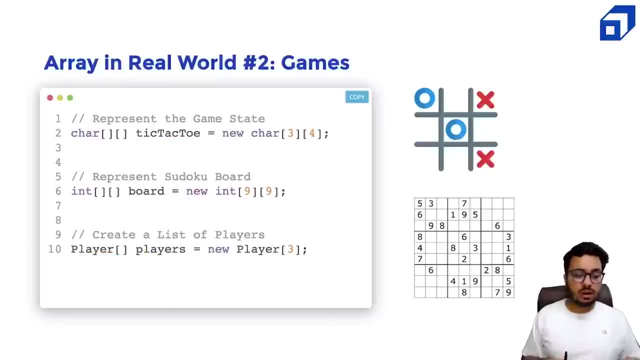 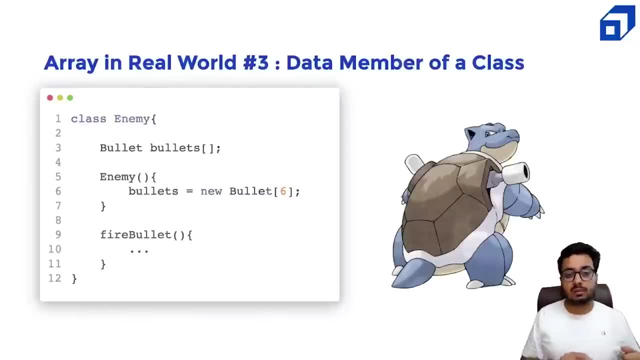 it right, it's an array of players, right? that is also how arrays can be used. another use case could be that array can also be part of a data member of a class. for example, you have a any week object. the enemy has certain bullets inside it. like certain number of bullets, the enemy can. 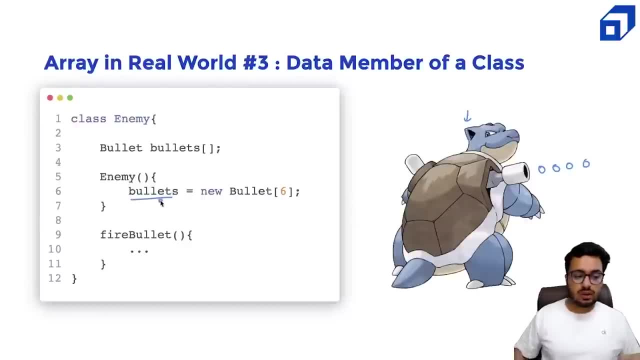 fire. i can create an array of bullets where each bullet is of the type bullet and i have created it when the enemy is created. for example, i want this enemy to have exactly six, six bullets. when this enemy is created, i can do something like this: okay, and when you're firing the bullet, maybe a? 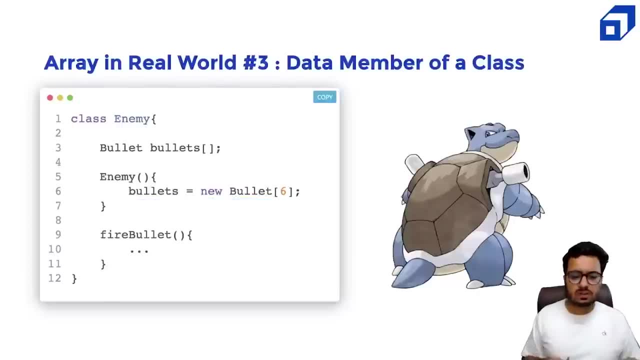 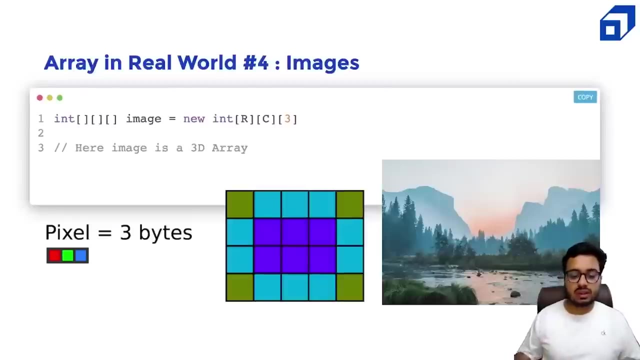 particular bullet might get deactivated. it. something like this can also be possible where your array is a data member of a particular class. this can also happen. another example could be the your images. so when you deal with images, you know each image is made up of a matrix of pixels. okay, of the size rows into columns so you might have. 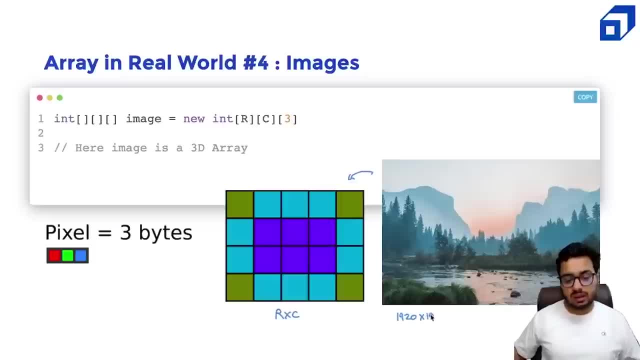 heard about an hd image, so that is 1920 by 1080. that simply means that we have these many pixels in this image and each pixel is actually made up of three numbers: a component of red, component of green and a component of blue. so that means each pixel itself is an array of three numbers, right? 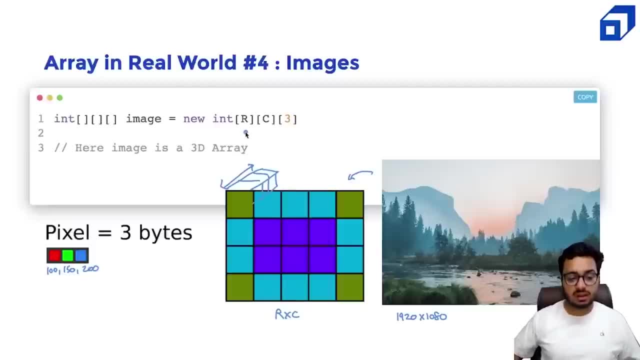 if i look at an image, the image is actually a three-dimensional array of rows, comma columns, into three right, where each pixel is actually going to store three numbers. when we do with work with images in python, you often see the arrays are three-dimensional, okay. another example: that when you're building uh software components, for example, a tool like 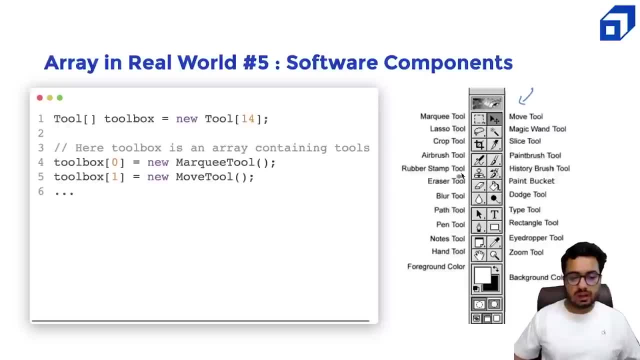 photoshop, right, you will say: okay, there is this grid where every item is a tool, so i can say: okay, tool toolbox, this is new tool, and in every index i'm creating a new tool. right, marquee tool is a type of a tool, movetool is a type of a tool like i can also do something like this. they. 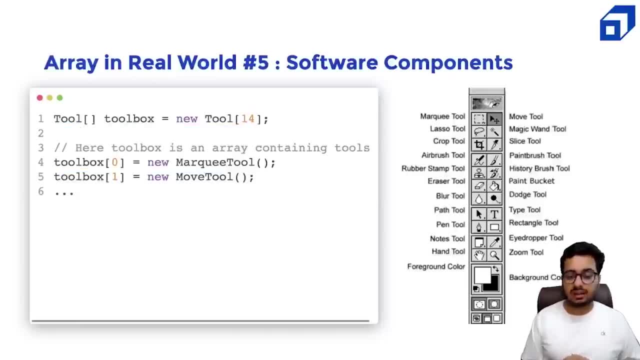 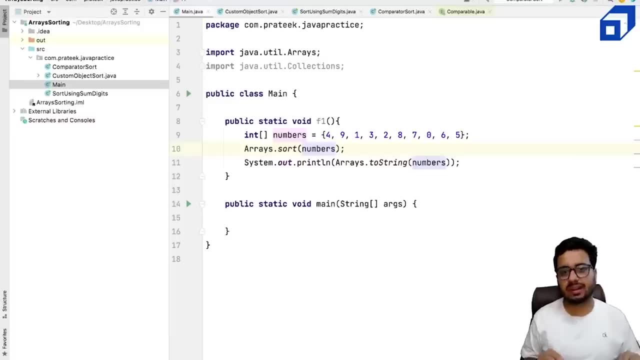 a lot in building real life software and that is the importance of arrays. right now we'll look at some code demo to work with arrays. now we are going to look at some code of an arrays, especially how do we perform an operation like sorting on arrays, which comes very handy in solving a lot. 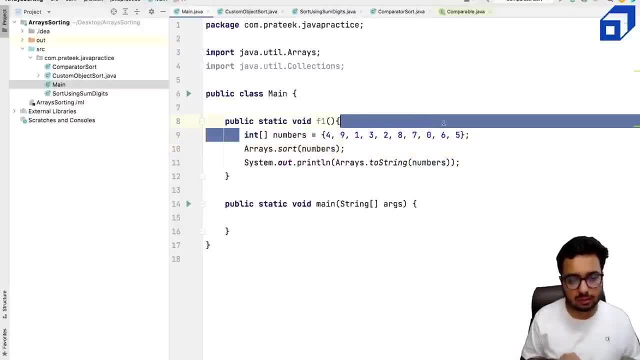 of problems. okay, so i have an array of numbers and i want to use a method called as sort right. so in java dot util package there is a class called arrays right. this class contains methods that will work on a array that we have created right. arrays dot sort is one such method. 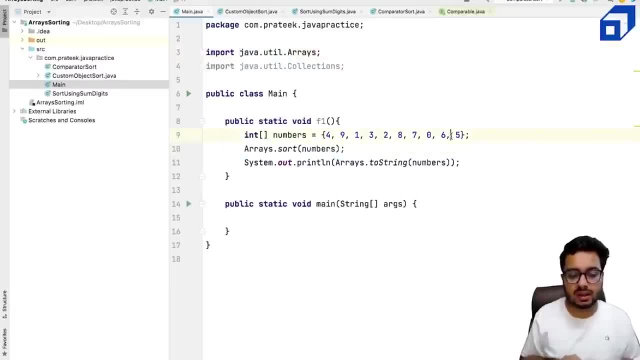 we want to use this method to sort our numbers array. let's see if i uh go and run this code. so i just need to call this function f1 so my array is created, the array will get sorted and we are going to output this array, right? 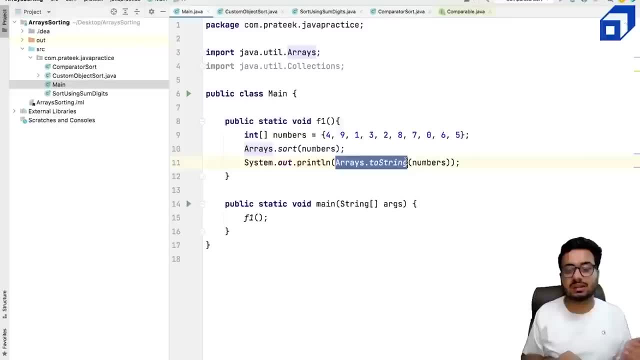 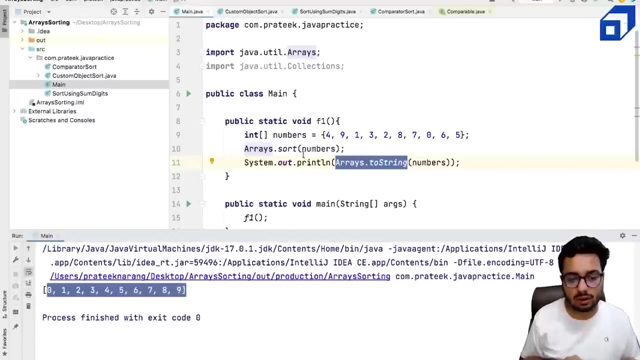 in a such method is arrays dot to string. i can convert this array into a string like representation that i can print directly. so let us just go and run this main method. so now you see, the data that you are getting is in a sorted order. let us look at one more example. let's say i have an array of 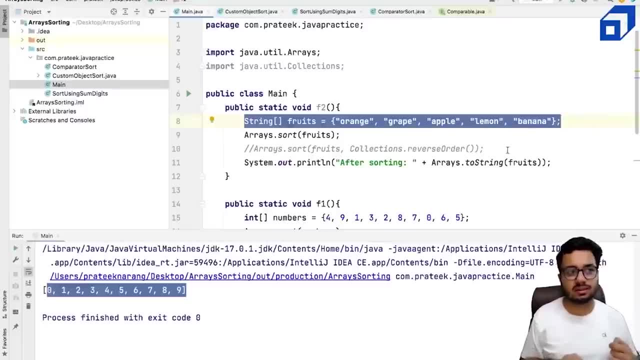 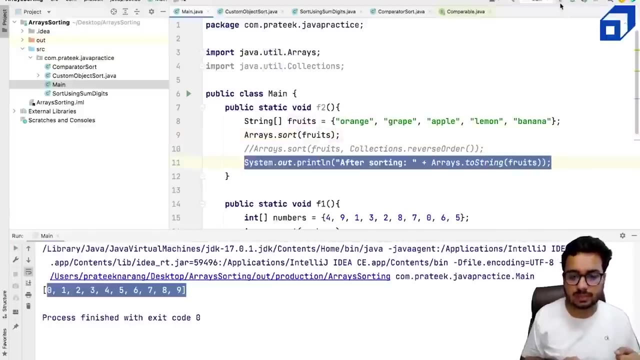 strings and i want to sort these strings again. what i can do? i can use arrayssort method, which is again an inbuilt method inside javautil, and i just need to pass the array object to this method. it's going to sort these objects and let us call our function f2 and let us run this code. now what? 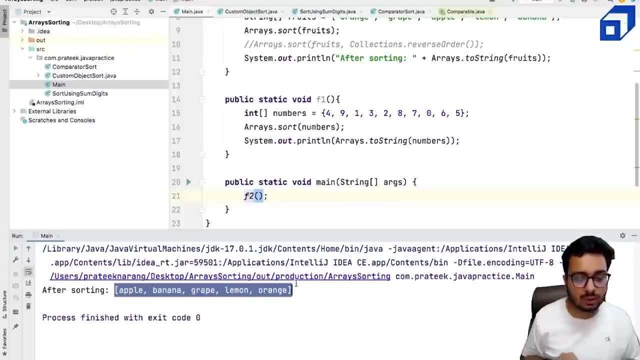 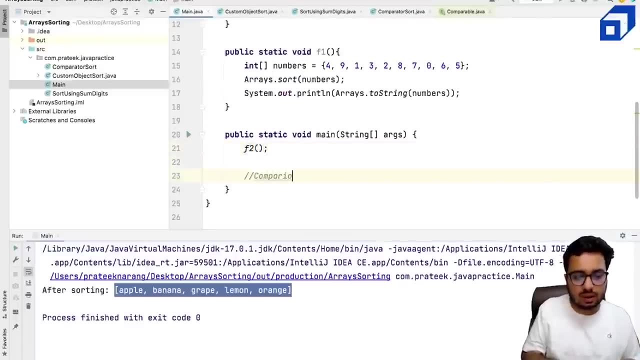 do i see, i see output- apple, banana, grape, lemon, orange- right now, how two strings are compared. let us talk a little bit about comparisons as well. now, comparing numbers is easy. i can compare is 5, 13.. is, yes, right? but if i have a string called, as, let's say, s1, that is abc, and i have string s2. 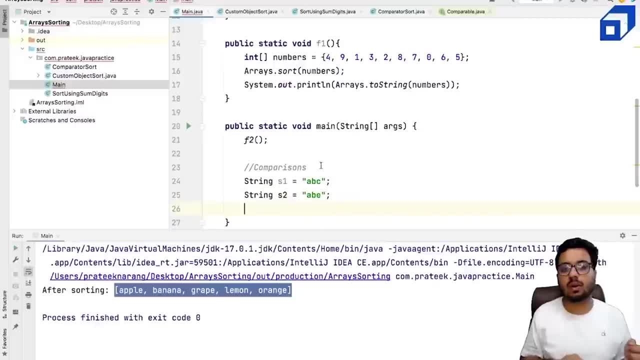 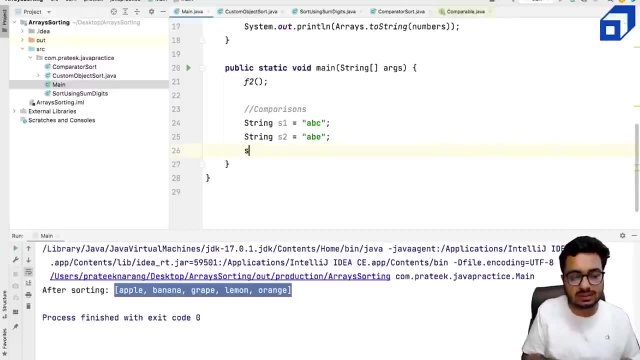 let's say i call it as a, b, e. now are they equal or are they naughty? how do we compare? by default, inside the string class there is a method called as compare to. if i say s1, dot, compare to, you see, there is a suggestion coming out and i say, okay, let me compare it with the string s2. 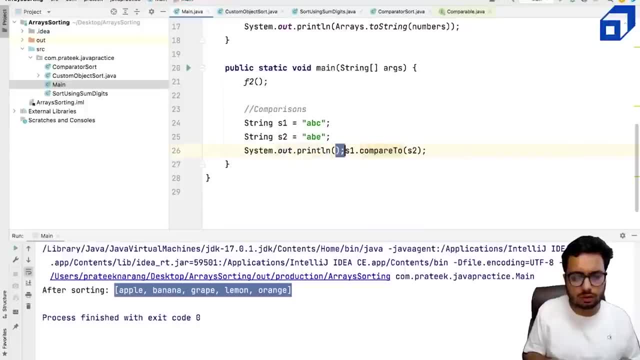 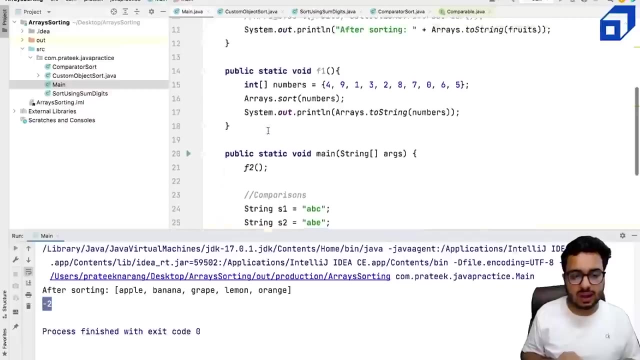 and let me uh show you the output of what this comparison function is going to return. now. why i'm teaching you is: this is very important because we also want to write custom comparisons for our object. i'm getting an output that is mine. basically, how sorting function works is. 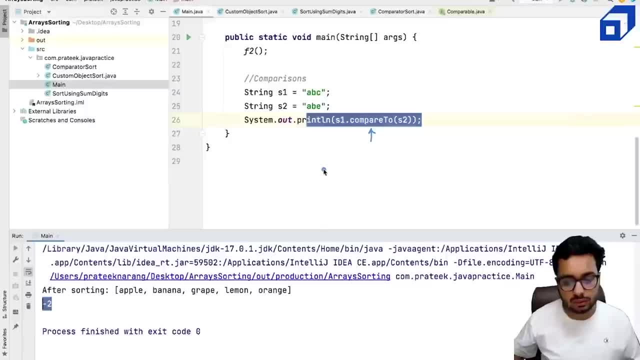 internally calls the compare to method. when you use arrays, dot, sort, and you give some array of objects to sort, right, so what it does, it calls the compare to method of that object. so string, basically, it is calling the compared to method of this object. so i'm saying s1. 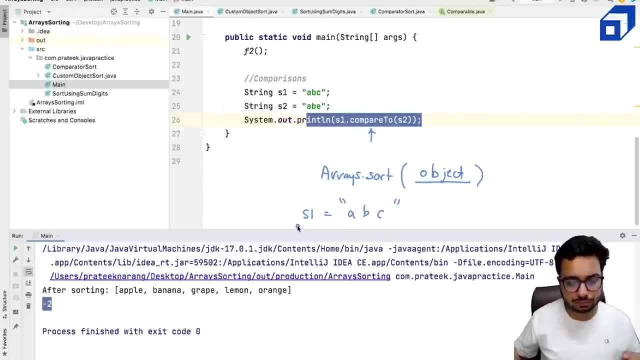 which is abc. i want to compare it with another string: a, b, e. now this compare to method. it's going to produce three types of outputs: 1 is a negative output, 1 is 0 and another is positive. so negative output simply means what? if we compare this again with a string avc, that is a, A, q, it's next to the first right string of the object. this. 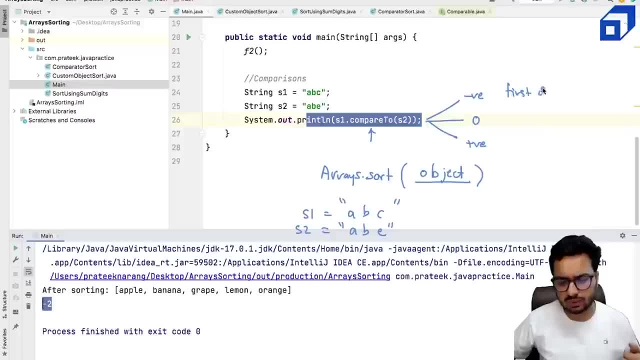 means that my first number is smaller. first object is smaller, that means it will come first in the list. positive number means my second object is smaller. that means it will come first in the list. and zero means the two objects. they are actually equal if i get a negative output. 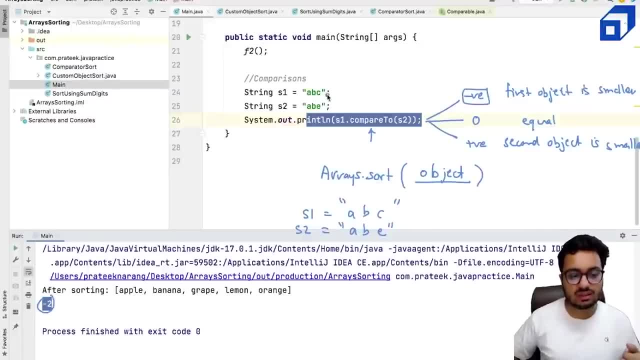 which i'm getting. in this case, that means a b c is smaller than a b e. let us also see how this minus 2 is actually coming right. so when you compare a b c with a b e, right. so you compare a with a, they are equal. so you move to the next position. you go with b, b and b: they are equal. you. 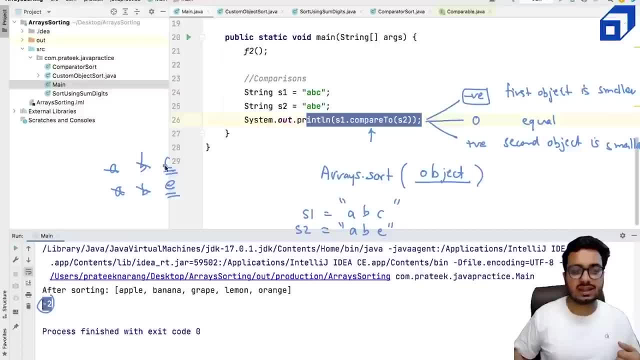 move to the next position. now you compare c and d right now. suppose c has some maski value, right? so maybe this is: uh, this was 97 98, 99, right and this is 97 98, and this is 97 98, 99 right, and this is 97 98, 99 right, and this is 97 98, 99, right and this is 97 98. 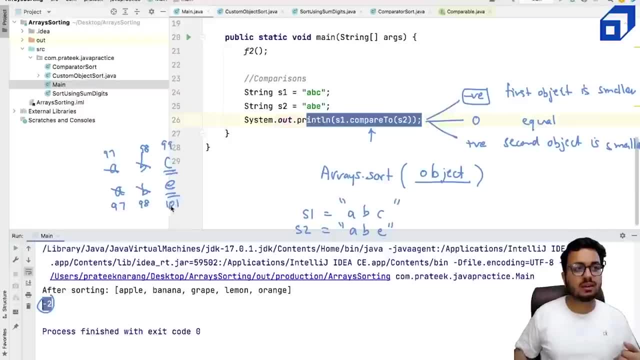 99, 100, 101. right, the ascii value of e could be 101. so when you take this difference, i think a, a is actually 90 not 97. so whatever the ascii value is right, you will take the difference. if you subtract c from e, you will get a difference of mine. that basically tells the sorting function. 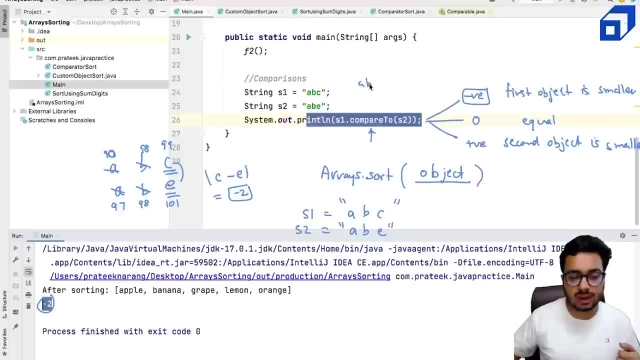 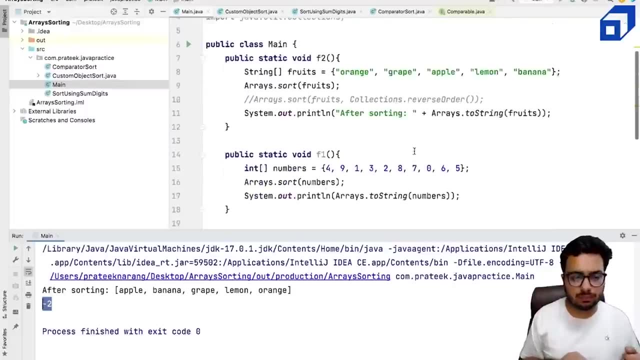 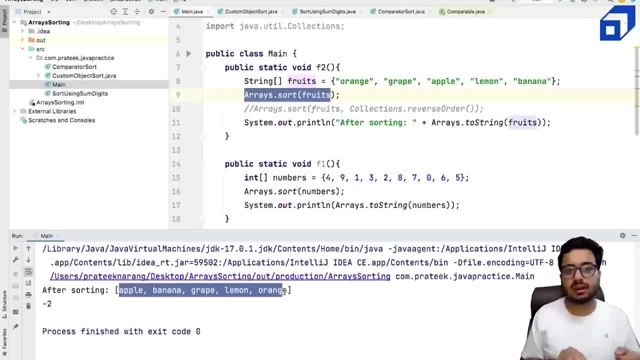 banana, grape, lemon and orange. they are coming in their dictionary order right, because a string knows a compared to function is present inside it, right. then i say: okay, i want to, i want to reverse this order, right. what you can do is one simple way of doing it is that you apply a custom. 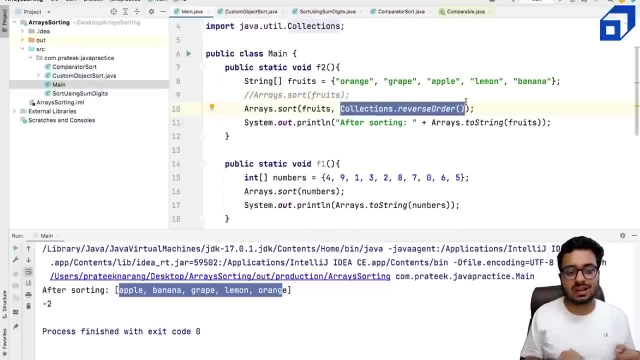 comparator called as collections or reverse order. that is exactly going to reverse this order. right to reverse the default output. okay, by default you're getting this output. if you specify this, it's going to reverse the default output. i run this code now we'll see. i will get orange first. 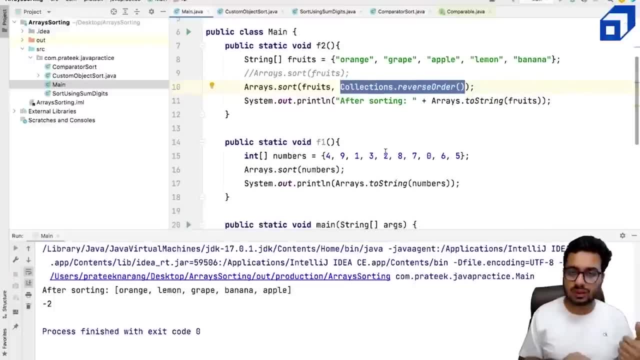 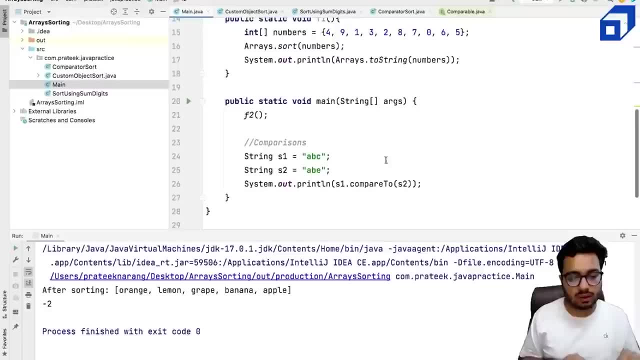 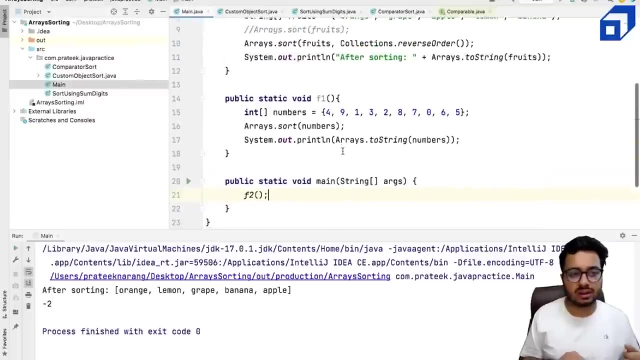 followed by lemon, grape, banana and apple. that is one thing that you can use to convert your ascending array into a descending. that is one way of doing it. so now you might ask, then, why we are studying this compared to method, or where do we need it? let us try to understand. 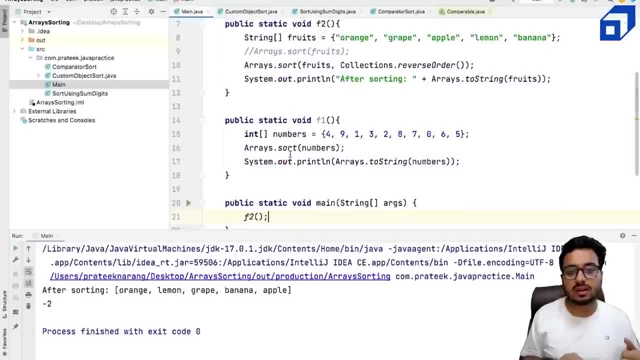 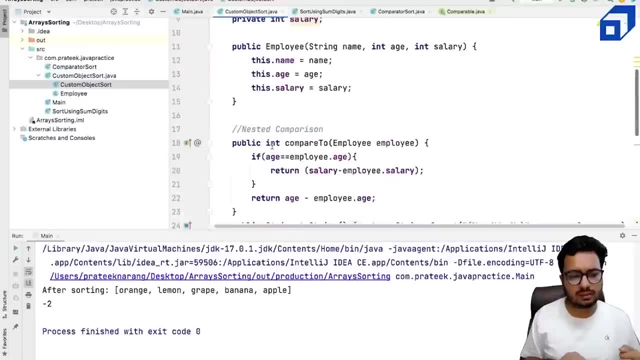 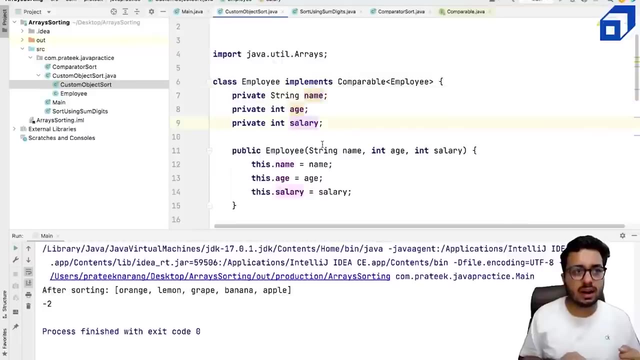 that as well. this was very simple. this was an array of integers or an array of strings. right, you might say that i have a custom object. i. i have, let's say, a class called as employee, where my employee has a name- agent, salary, right- and i want to create an array of employees. i have a array of employees, the array of custom objects. 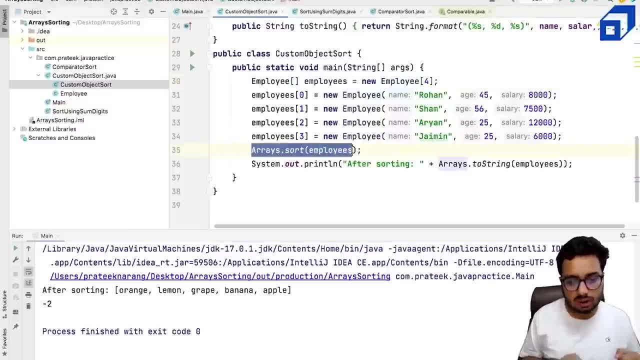 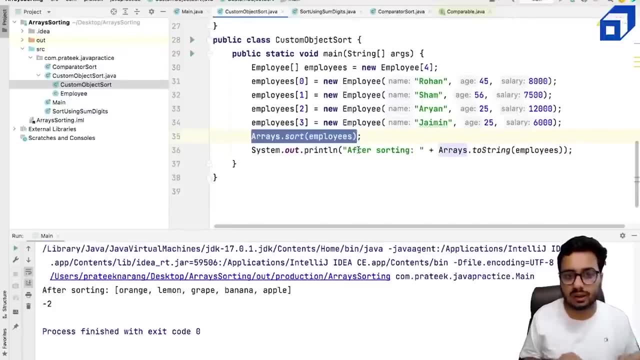 and i want to sort them. if you, uh, sort them right and if you do not tell java that, okay, i do not know. how do we? how do i compare to employees? most likely you're going to get an error right now. errors dot sort can also accept employees, but given that you define a method called as 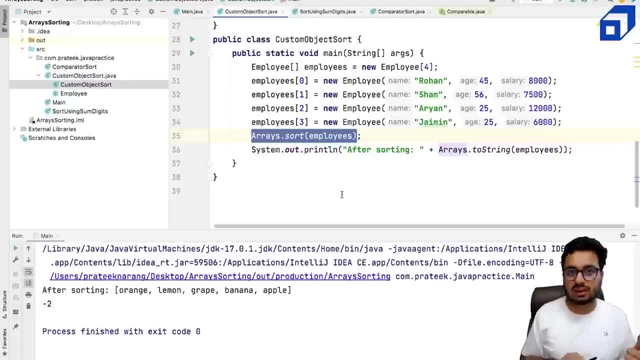 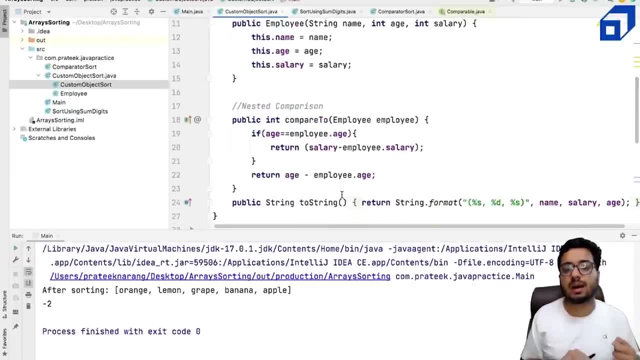 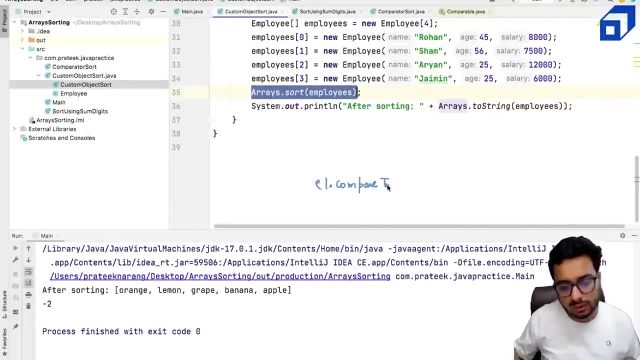 compare to inside the employee class if in the string class it is an inbuilt method, but in the employee class which we have written, we have to define. how do i compare two employees? for example, i have an employee e1. i want to call the compare to method and supply it some another employee e2, right? so when you say okay, 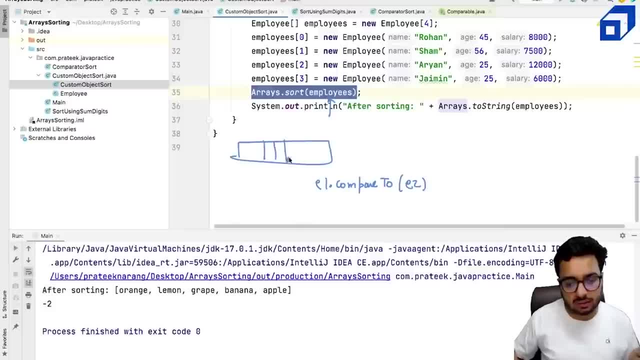 i am sorting a list of employees, right, this is an array of employees. so it will say: okay, i'm going to compare this employee with some other employee. so i will say employee i dot compare to some other employee, that is employee j, right, so the sort function is internally going to call this method, called compare to right now this. 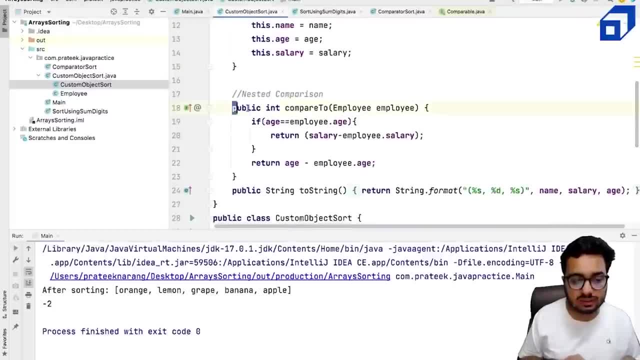 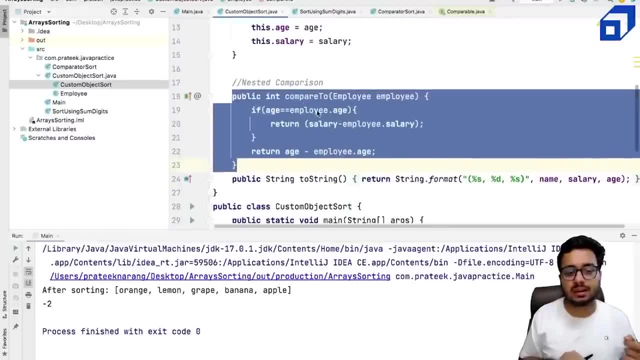 method is not there. what we have to do, we have to define this method inside our employee. i have my employee class and here i'm going to define my compare to method, how it will get called. it will get called internally employee i getting compared to with some other employee: j. right now it is up. 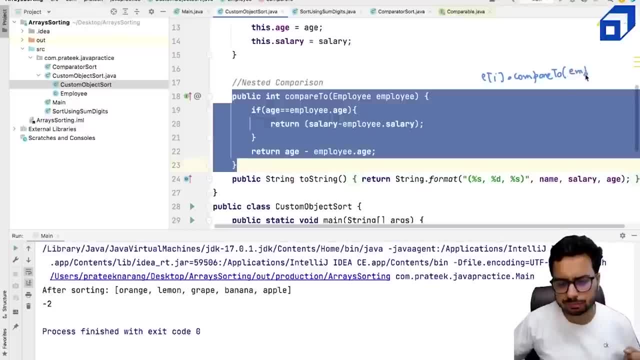 to you. how do you compare to employees, right? some other employee j right tmpe. now look at this. how do i write this method? basically what i'm doing. i'm saying if the two employers have the same age, i will compare them according to their salary. i'm saying salary 1 minus salary 2. so if the 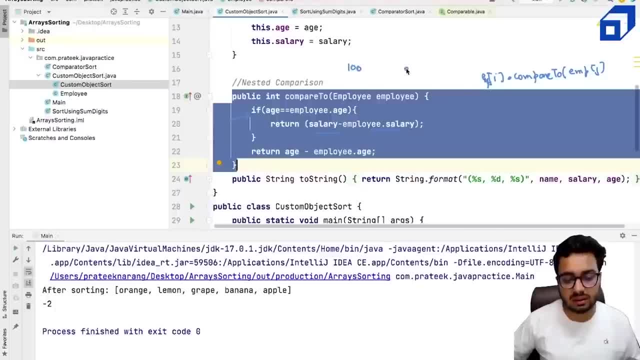 first employee salary is 100 and second employee salary is, let's say, 60. 100 minus 60 it's going to produce a salary of 100. so if the first employee salary is 100 and second employee salary is, let's, a positive number, that means the second employee will come first, the person with the lesser salary. 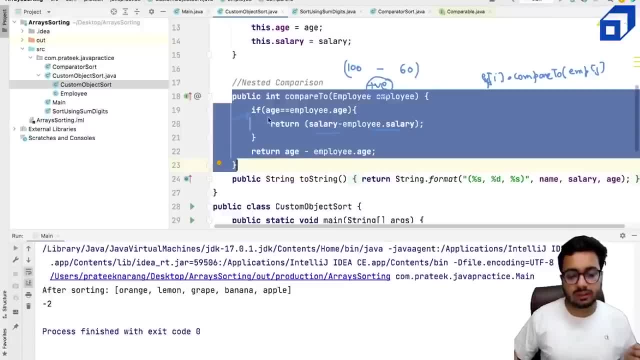 will come first, or if the age is not equal- i'm saying age minus employee dot age. this is the age of the first employee and this is the age of the second employee. for example, if the first employee is 50 years old, the second employee is 40 years old. 50 minus 40 it's also going to produce a 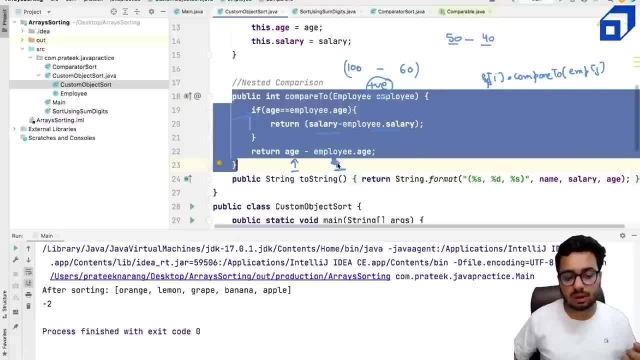 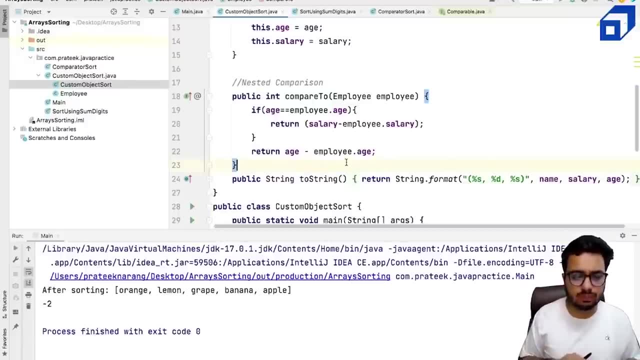 positive number. that means the second employee. it is smaller in age. so if the first employee is right, what this sort function is going to do, what this compare function is going to do? it's simply going to compare the two employees based on their age. if their ages are equal, it's going to compare. 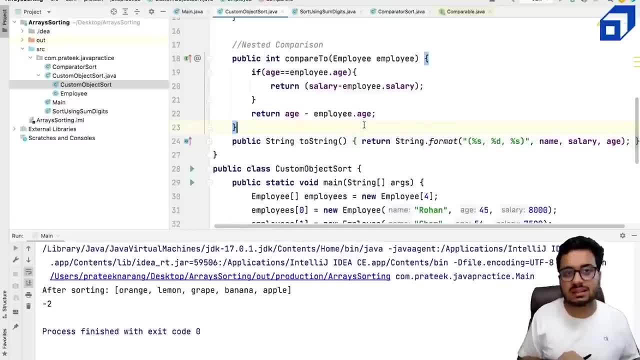 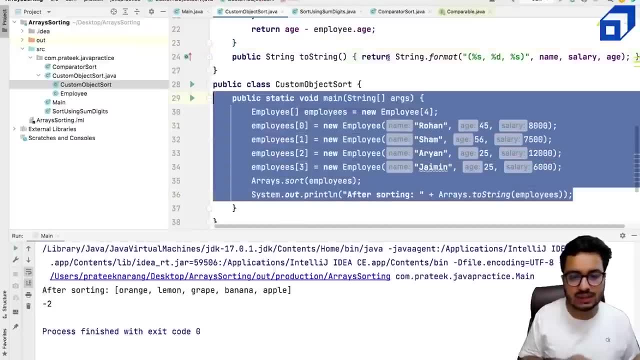 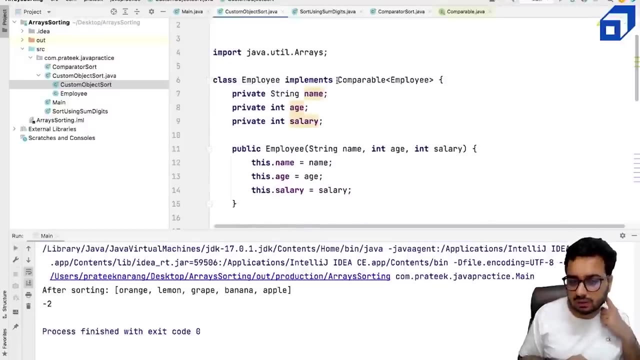 according to their salary- people with the less age and less salary. they are given priority. they will come first in the output. so let us run this code and see what do we really get right? okay, one more thing is that we have to: whenever you're creating this class, you have to tell that it implements the comparable interface. 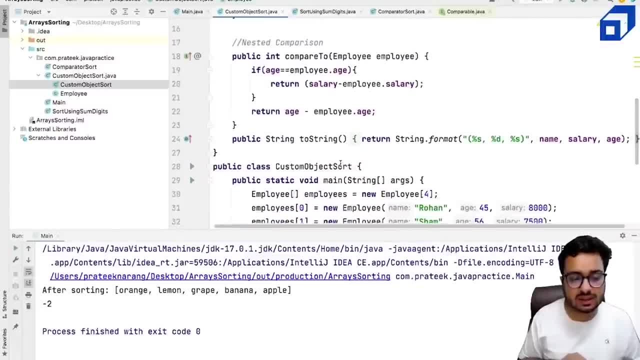 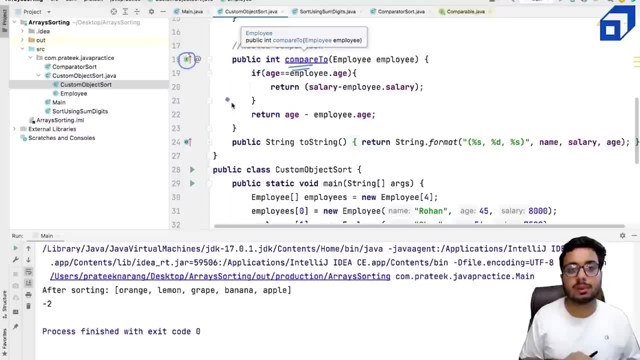 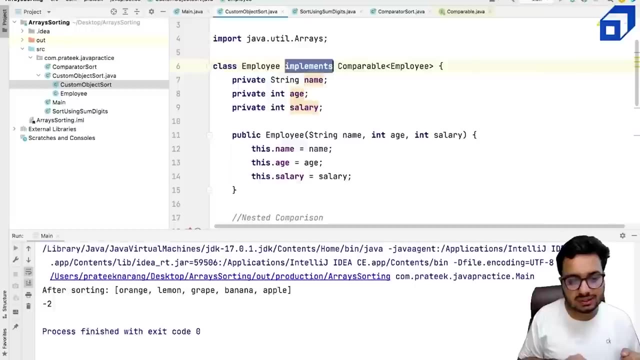 right. why? because the sort function expects that you will implement a compare to method. this compare to method is coming from the comparable interface. right, we'll discuss the concept of interface very shortly, but you should know that you have to say: this class implements the comparable interface for the employee in which we have a 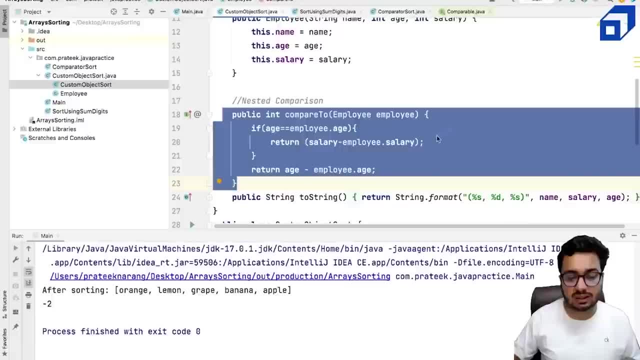 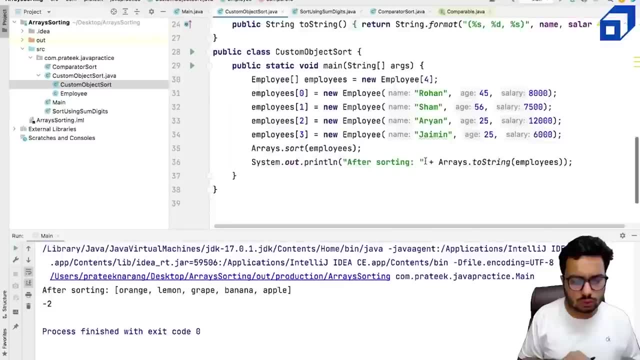 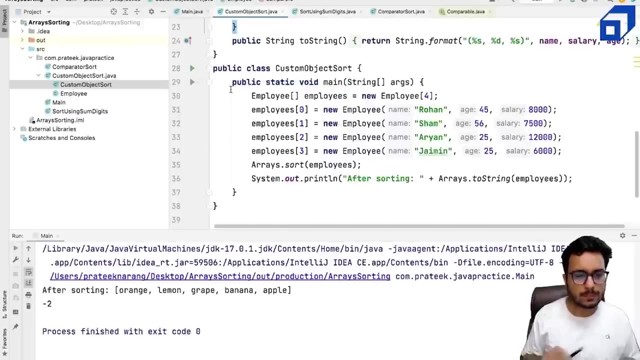 abstract method compared to- and we have defined this method in the current employee class. right, the body must be given here. so what? what is happening now? let me show you the output. let's run this one. we are sorting an array of objects, right? so I'm saying: let me print employees. so now I'm getting. 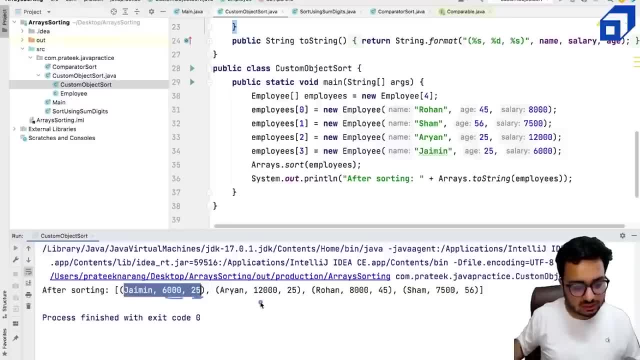 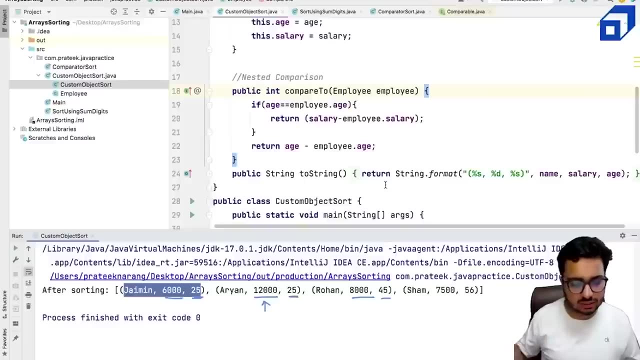 six thousand and twenty five. this is salary and age. I'm getting twelve thousand and twenty five. that means higher salary, same age, and I'm getting eight thousand and forty five. according to my logic, the first preference is on age. employees are sorted first on their age- 25, 25, 45 and 56- then they are sorted on their salary. if the age is same, the jam. 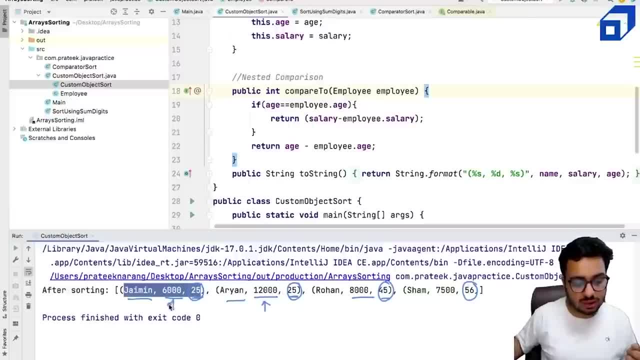 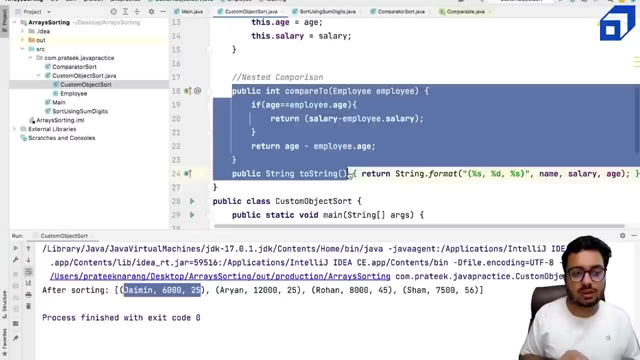 jam in and are in. they have the same age. so the person with less salary it's going to come first. so you can do. you can make any logic like: depending upon the situation, and this compare to method will tell the sort function. how do I actually sort? So I am hoping. 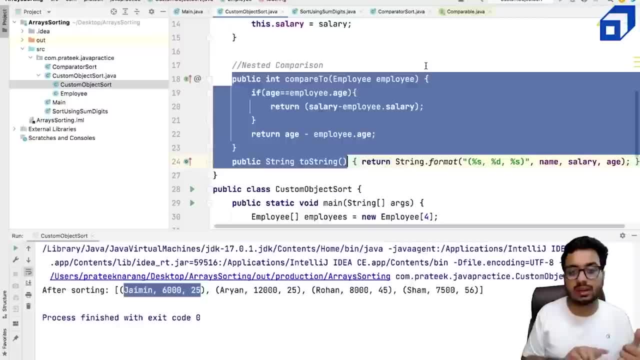 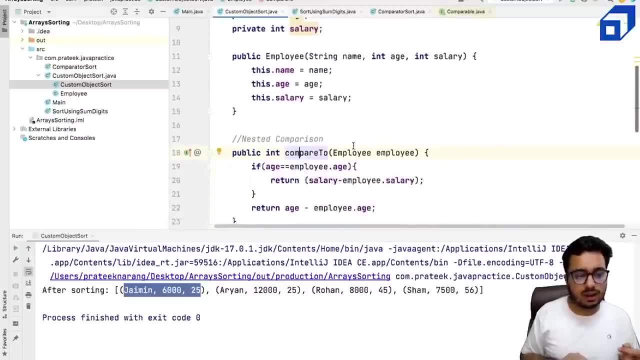 that this is clear. So one way is use the default sort function, but it does not work for the custom object. Then what you can do, You can write the compare to method. and now there is one more scenario in which might not want to go this way. You might. 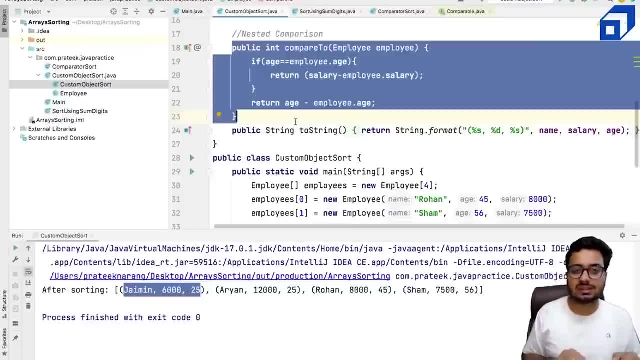 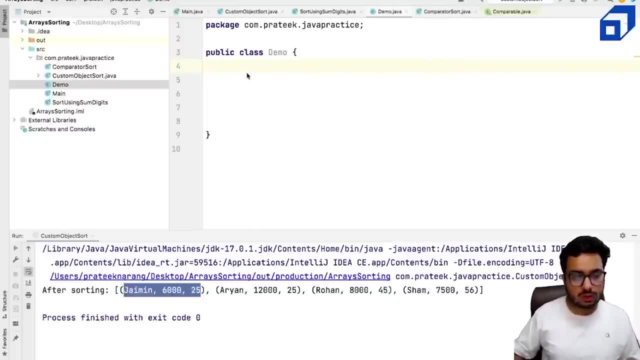 want to go with the comparator way. Let me discuss that as well. So let us discuss one more way of sorting using comparator. Now I am going to tell you why it could be important. Now suppose you have maybe a list of strings. if let's say: 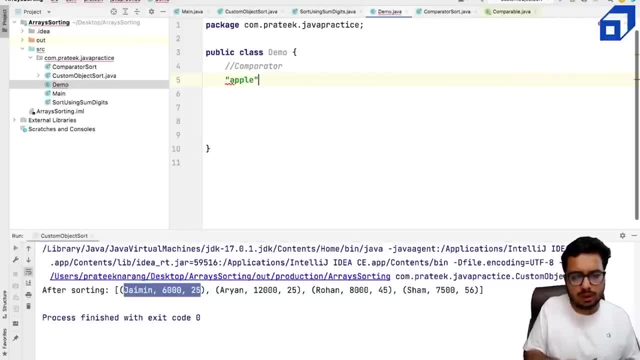 ABC. or let's say some fruits- Apple, mango, guava and orange- and you want to say, okay, I want to sort my fruits. I want to say, okay, erase dot, sort, I want to sort fruits. but I want to sort fruits maybe according to the dictionary. 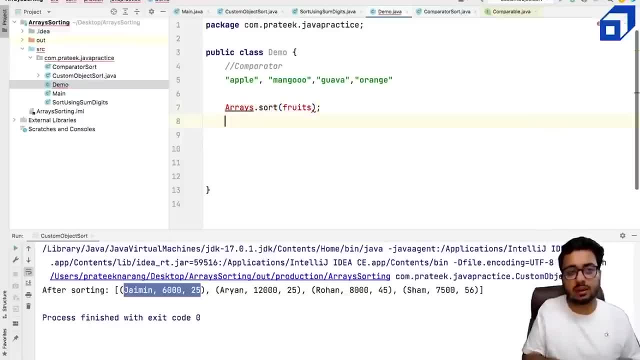 order. I want to use the default comparison, or maybe I want to sort fruits according to their length. I am not writing the proper code, but what I am trying to tell you is that if I want to sort fruits according to their length, I will have to go in. 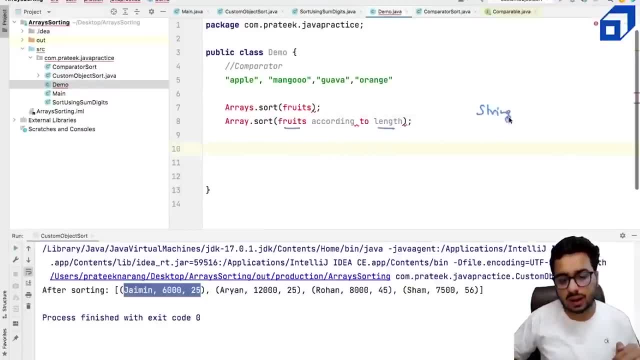 inside the string class, and inside the string class I will have to change the compare to method. Do you think changing the compare to method inside the string class, which is implemented in the java library, will be a good thing? The answer is no. We cannot go and 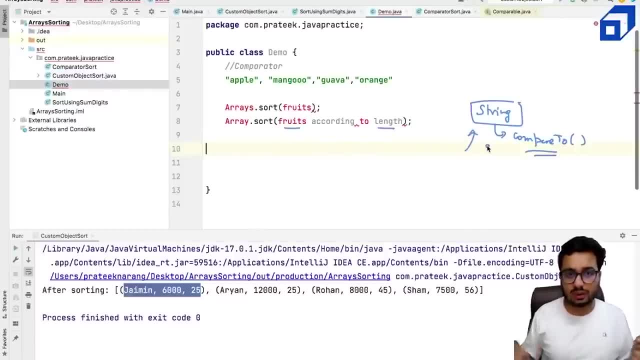 make changes in the library. That is one reason we will not use the default compare to method or we need some other way to do the sorting so that we have the flexibility. Another reason could be that I might have an if else like this: If the condition is this, I want to. 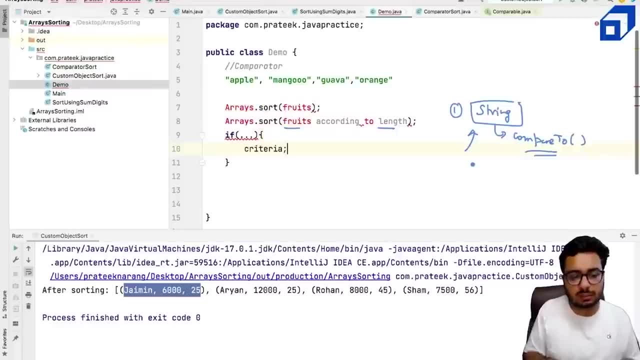 sort according to some criteria. if there is some other condition, then I have to use some other criteria for sorting. I might have something like this. Then also I will have to say that okay, go with the first way if your if condition is true. go with the second way if. 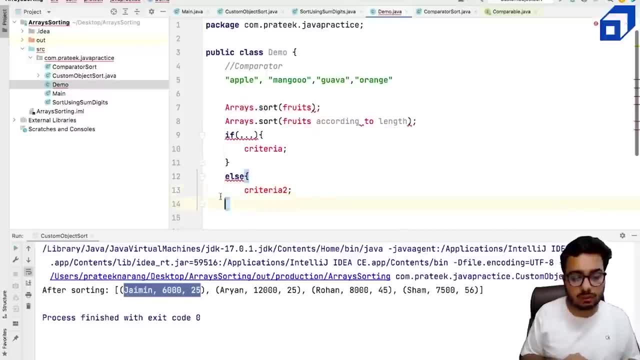 your second condition is true, Something of this sort. What I am going to tell you is that in such scenarios, where either you have conditional sorting or you will have to use your, you cannot go and change the library. compare to method for that particular class. there is third way of doing the sorting. 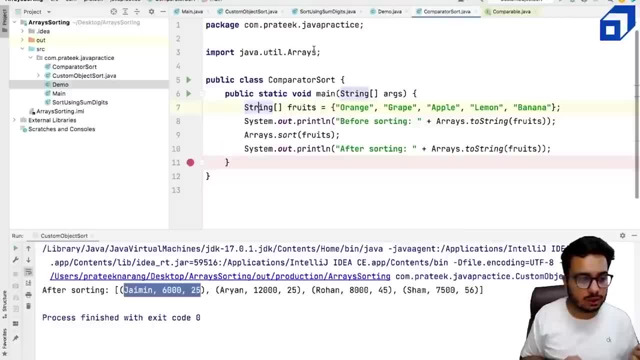 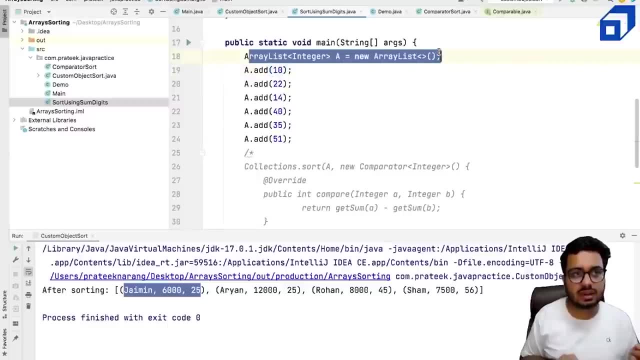 That way is called as comparator. I will show you an example of using a comparator. In this case I am creating an ArrayList of integers, ArrayList we will study very shortly. It is just like an array, but it is dynamic inside. It can grow and shrink. 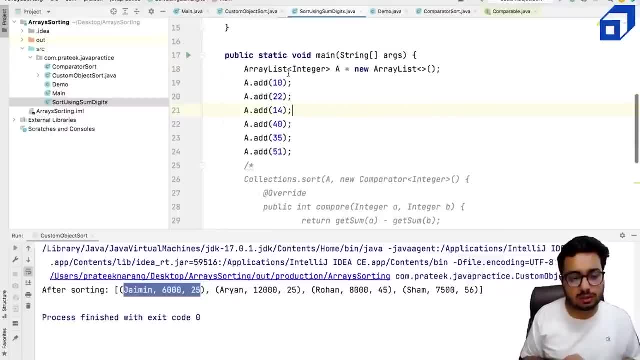 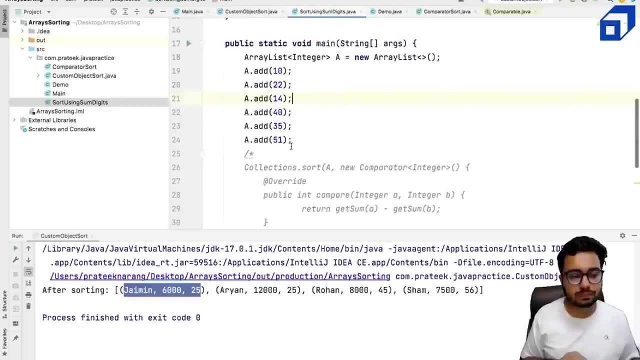 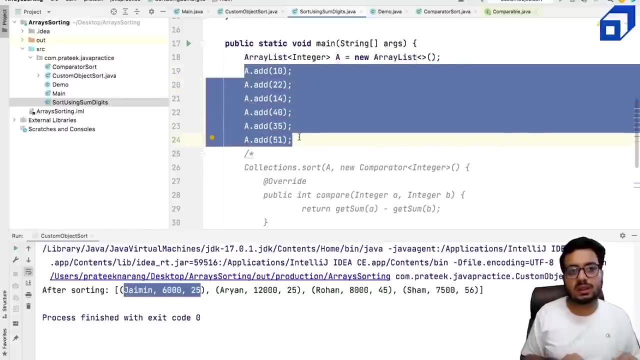 It is part of collections framework. we will study. The demo that I am going to do here is also applicable for ArraysSort method. What we have done is we have created a dynamic array in which I have added few numbers. What I want to do is: 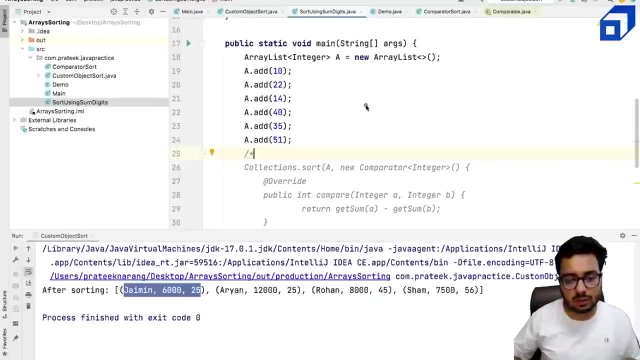 instead of sorting these numbers directly. I know 10 is less than 22, that's okay, But what I want to do is I want to sort these numbers based upon their sum of their digits. You might say: okay, how do I override such a comparison? 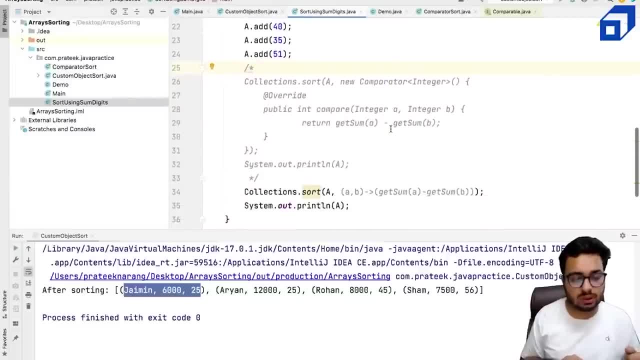 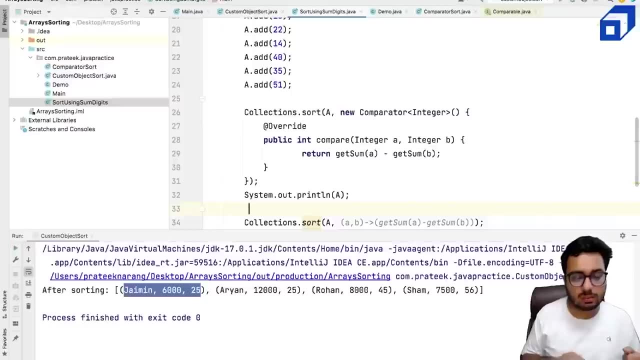 In such scenario, there is this third way that I am going to teach you. It is called as sorting using comparator. What we can do. we still need to call the sort method. If it is an array object, you will use arrayssort, but if it is an 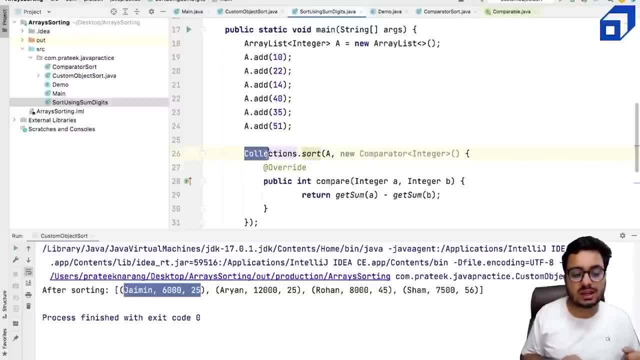 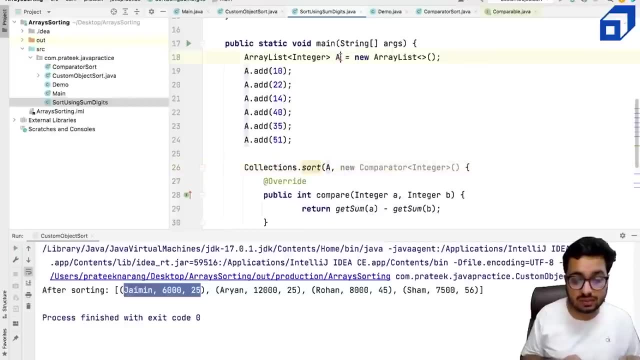 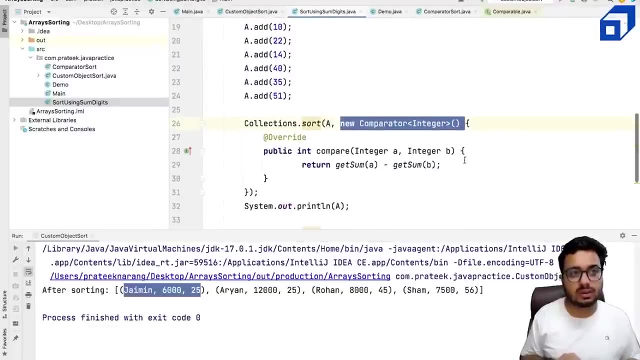 ArrayList, which is part of your collections framework. you will use collectionssort In this sort method. you need to give your ArrayList object. that is a that we have given And now we have to say that, okay, I am creating a new comparator object. It is an. 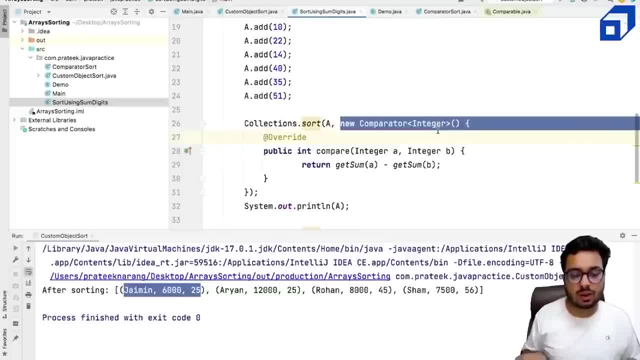 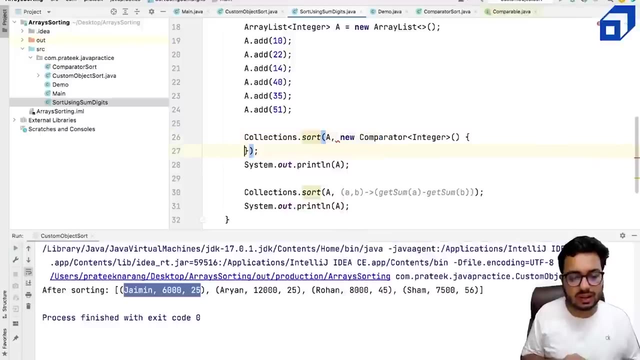 anonymous object. we are not giving it any And in this object we have to override the compare method. So I will just write this part again. once You will see, if you are using IntelliJ it will come using the auto complete feature. I create a new comparator object. 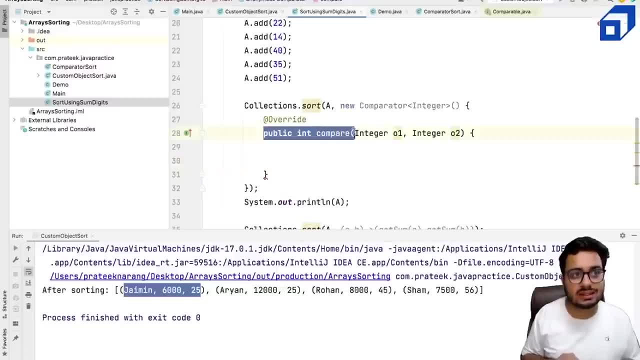 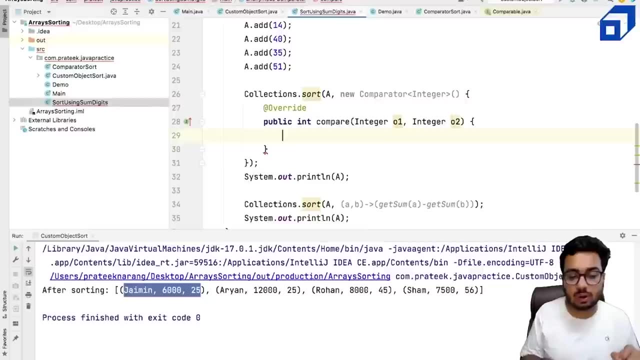 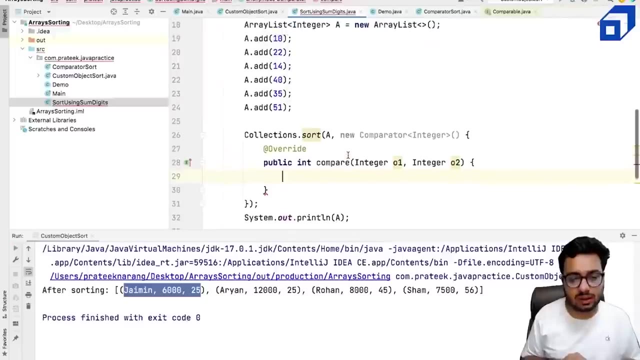 And in this it automatically creates a method called as public int compare. Note that it is not compared to this method. It is going to accept two objects that you want to compare And you want to tell how do I compare these two objects If there are simple strings, so integer. 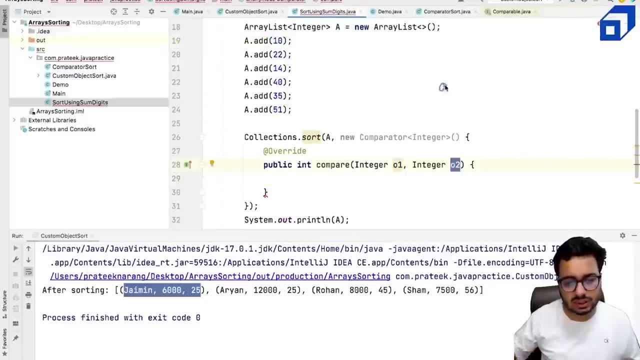 o1, integer o2. let's say first object: a is 10, b is 20.. If you simply return a minus b, that will simply compare these strings based upon their values. That means, okay, 10 minus 20, sorry, o1 minus o2. first object: 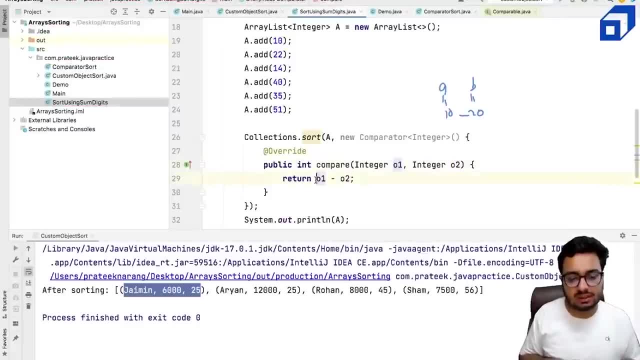 minus second object. I can do that. That will say okay, 10 minus 20 it is a negative number. that means 10 will come first. But if I do it other way, if I say I will negate this entire comparison, that means I am doing. 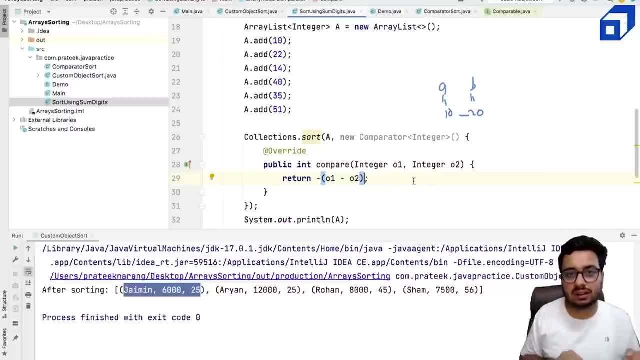 o2 minus o1. that means this list will be sorted in the descending order, But suppose, if I want to do based upon the sum of their digits. For example, this is 10.. So sum is 1 plus 0, that is 1.. 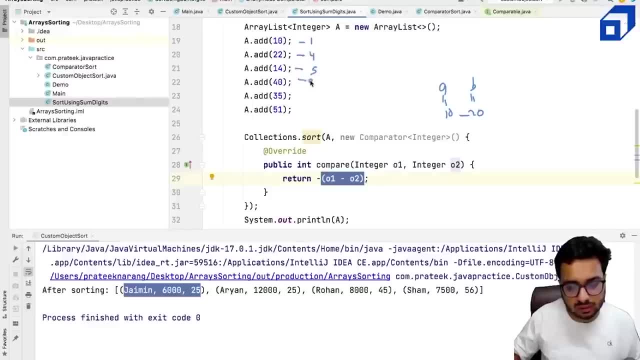 2 plus 2, that is 4.. 4 plus 1, 5. 4 plus 0, that is 4.. 35.. 3 plus 5: 8. 5 plus 1, that is 6.. I want to sort according to. 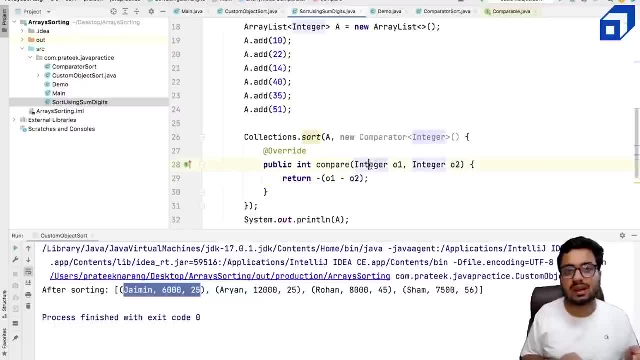 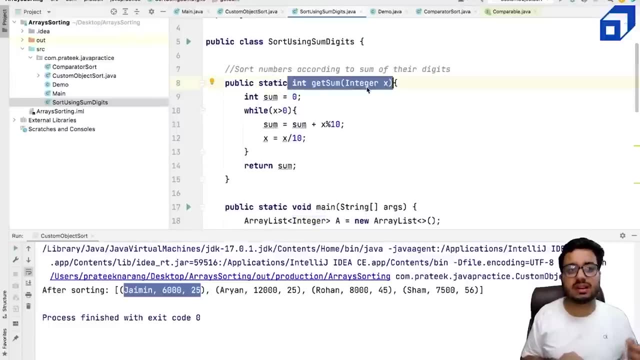 this What I can do. I can convert an integer into its sum. What I have done? I have written a function called as getSum. Given an integer x, I want to get the sum. So this is very easy. You know how to find the sum of an integer. 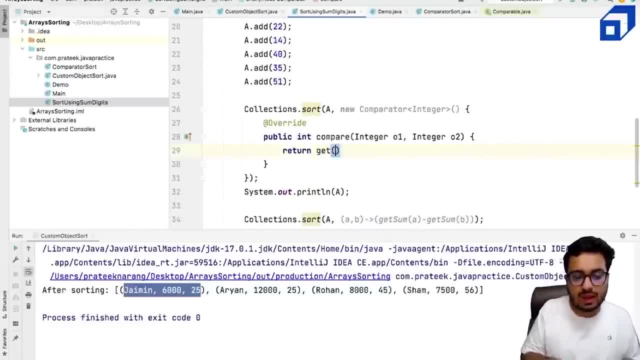 When I am making a comparison, what I will do is I will get the sum of first integer object, I will say getSum of a, and I will subtract: getSum of a is my object o1 and b is my object o2.. If I do this, 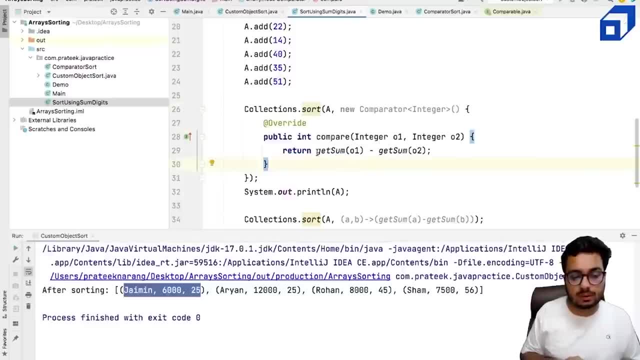 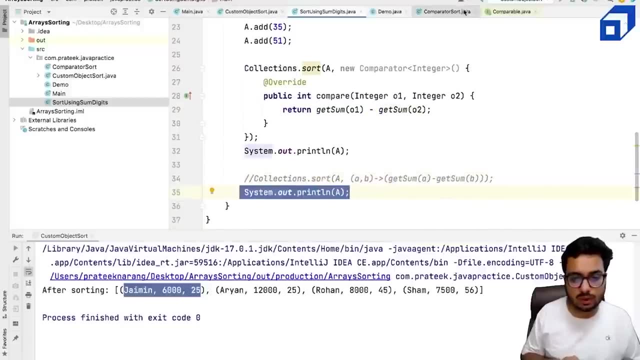 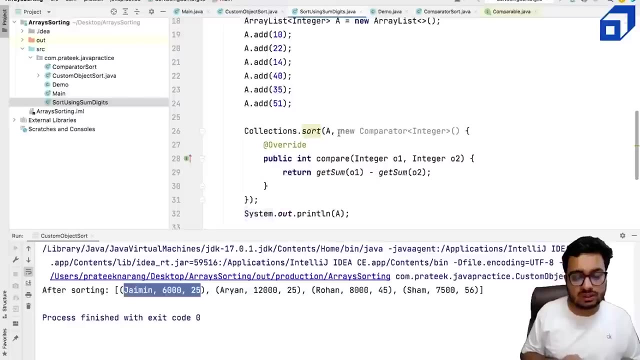 what is going to happen? So numbers whose sum is lesser. I will just comment this code out. I will show you the output. I will show you the output. Let us turn this code once. This comparator is telling the sort function that now you have to compare. 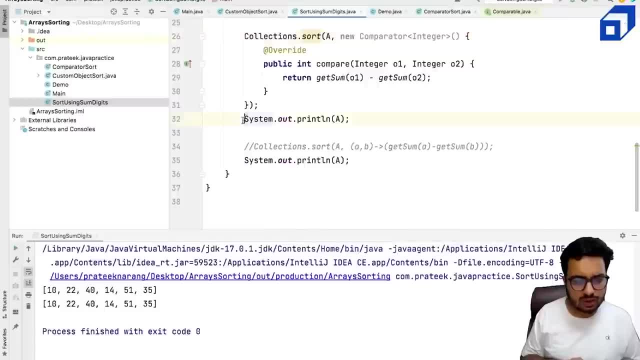 objects using the following criteria: Okay, so I have printed it twice Now, if you look carefully, 1 plus 0 is 1.. This is 4.. This is 4.. This is 5.. This is 6 and this is 8.. Now you look carefully at. 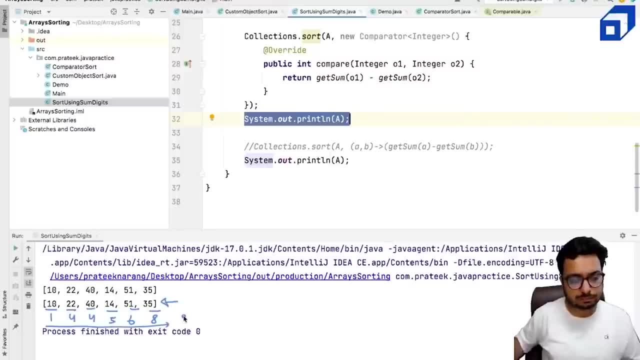 these numbers. they are sorted according to their sum. That is something that you can do. You can do the same thing with strings as well. You can do the same thing with employee as well. You do not want to implement the compareTo method inside the employee class. 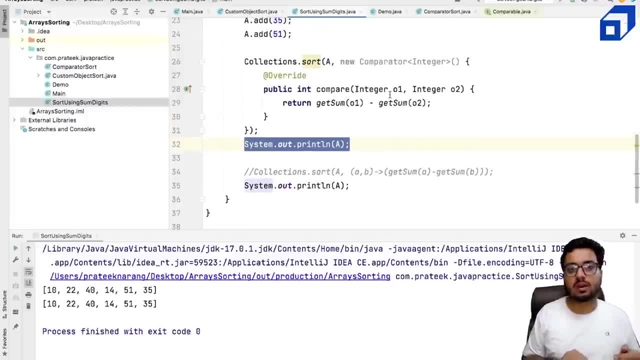 You can use a comparator, Or you want that on the top of it. I need another comparison based upon certain condition. If employees are near their performance period, I want to compare according to their salaries, not according to their age. So you can have that. 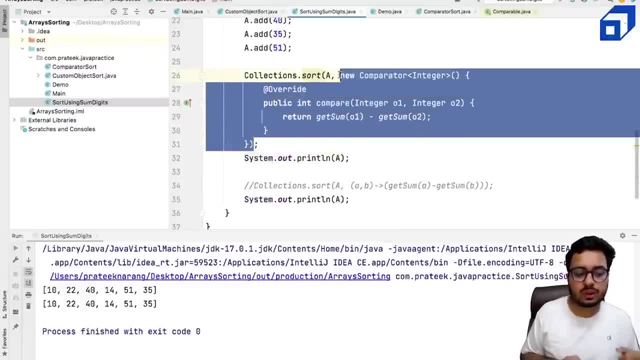 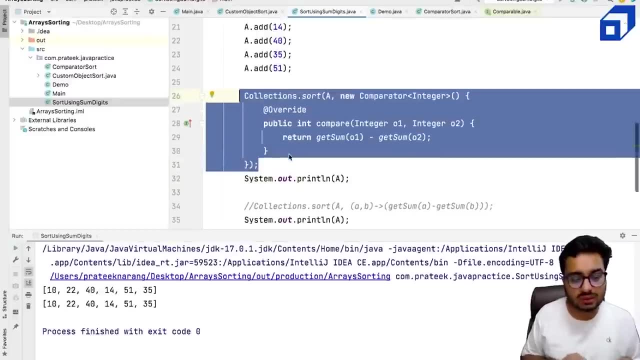 Comparator gives you another option to do the sorting. like You might say: okay, this looks little tricky, is there a shorter, easier way to do it? The answer is yes. So what we can do, we can use something called as a lambda function as well. 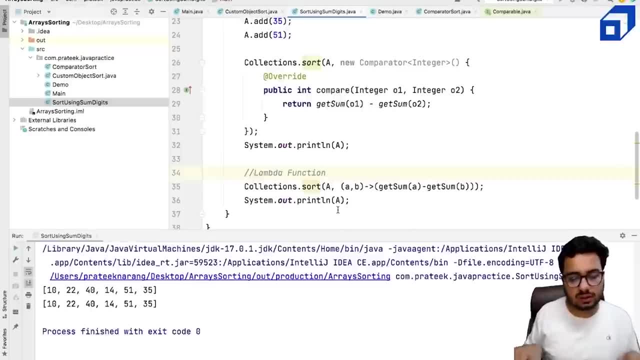 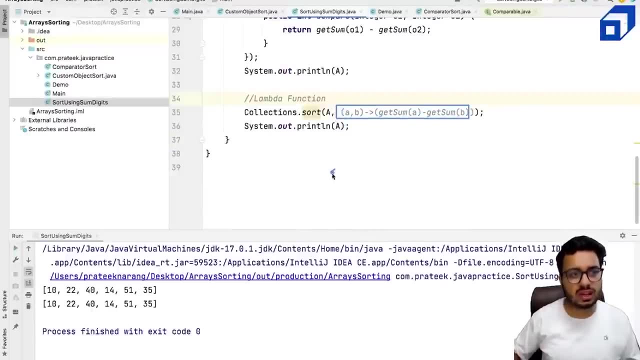 I will just tell you in a very short way what is a lambda function? It is a one line function, It is an anonymous function. So in Java, what you have to do, you have to write the inputs that you need to compare in these round brackets, For example, if I am comparing 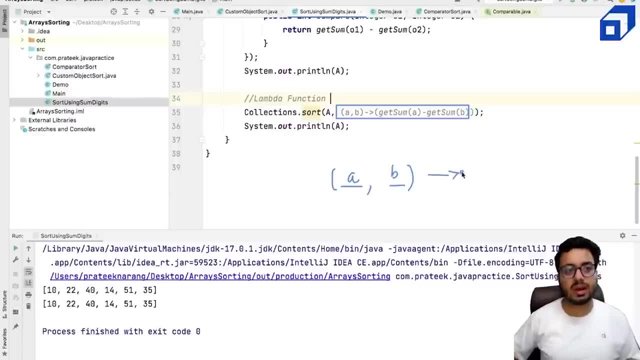 two objects, A and B, and with an arrow, you have to write the output of the comparison. Now, if you want to compare A and B, in this case, what is the output? I am saying, okay, getSum of A minus getSum of B. That is what we are. 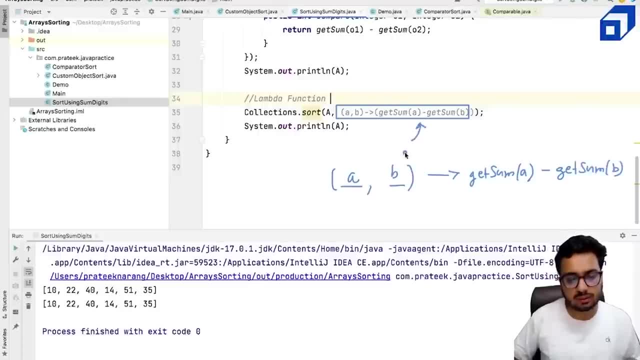 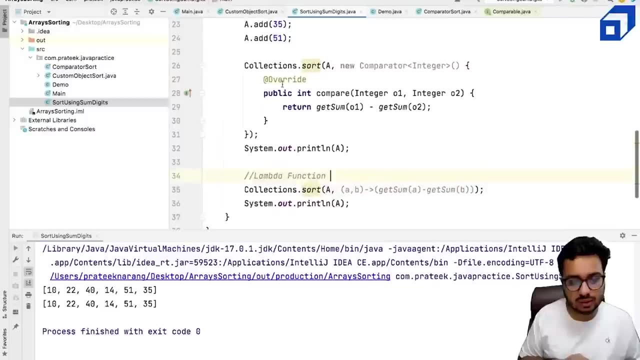 doing in the compare function as well. That thing. you put it here and this becomes a lambda function and it will do the trick for you. So you can just say that, okay, I don't want to write the compare method, I just want to use this value, that is. 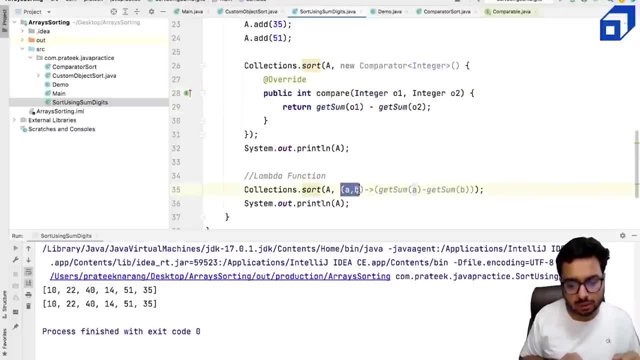 the output and use these numbers. that are my inputs. Given these two inputs, I want to return this output from the comparison. This will also work and if I show you, if I comment this code out, this lambda function will also do the same sorting thing that we want to. 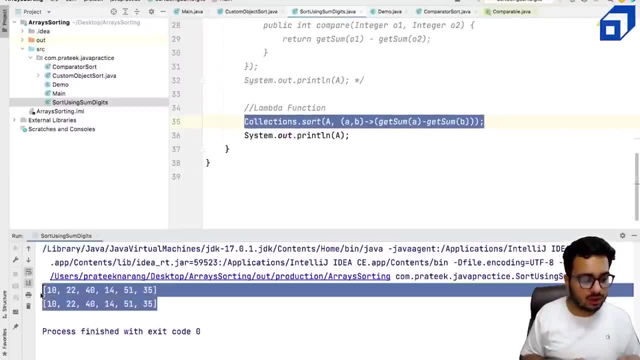 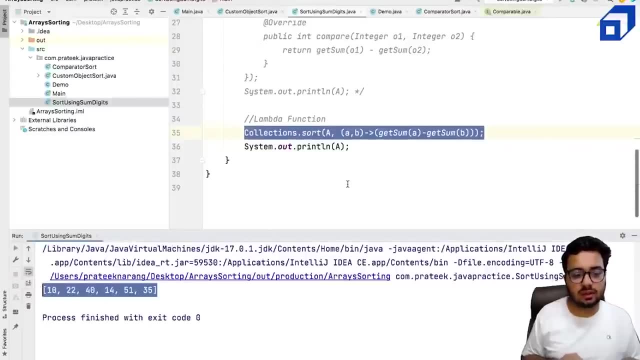 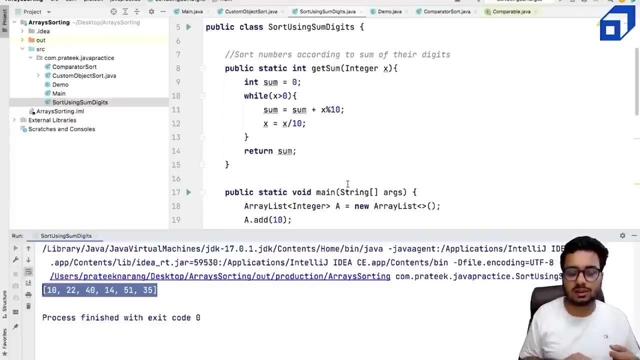 do. Let us sort them and let's see what do we get? We are still getting the same output. That is another way of doing the sort. Hopefully now you have understood the three different ways of doing sort. and that's all for sorting and we will start with the. 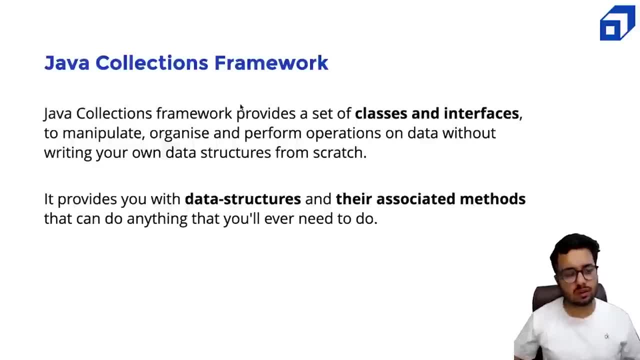 collections framework. next, Let's talk about Java collections framework now. Java collections framework is a framework in Java that provides us with set of classes, interfaces to manipulate, organize and perform operations on data without writing your own data structures from scrum. It provides you with library implementation. 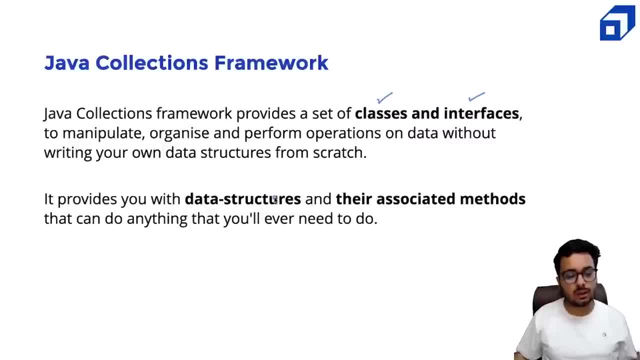 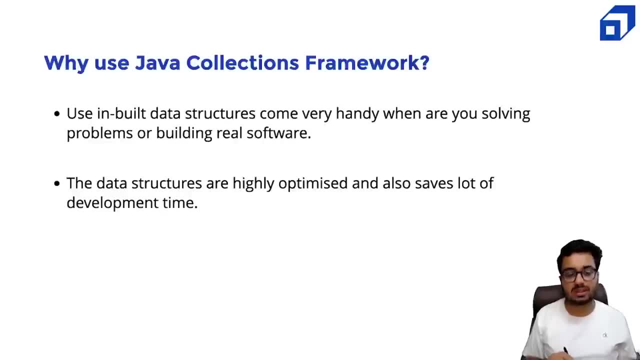 of data structures and their associated methods that can do anything that you will ever need to do. right. That means you will be using inbuilt data structures, because they come very handy when you are solving problems or you are building real life software. These data structures are also highly optimized. 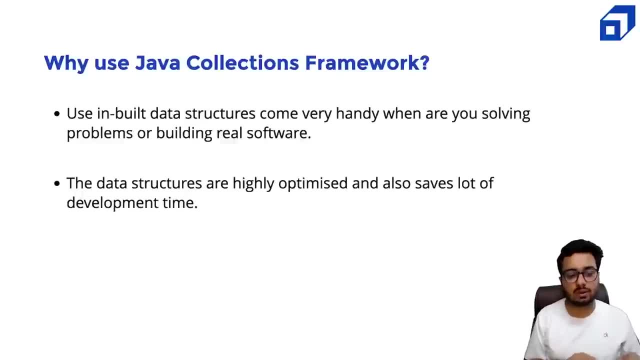 and they will, of course, save a lot of development time. So you don't need to write your own hash table, You don't need to write your own link list. This is what is standard practice. Most of the times, we would be using the library implement. 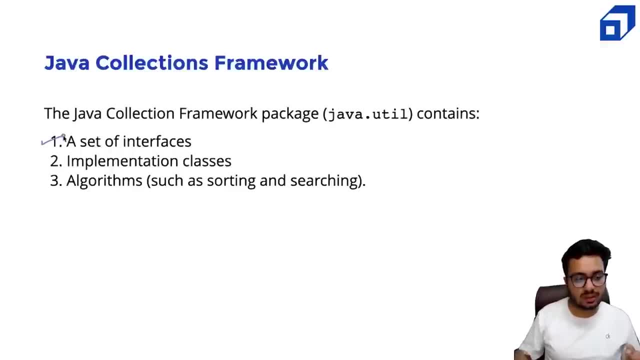 Just to summarize once again, what do we have? We have set of interfaces. we will see. We have implementation classes, The classes that actually implement those interfaces. We have also algorithms. I showed you the examples of arrayssort method, collectionssort method. Similarly, we have methods. 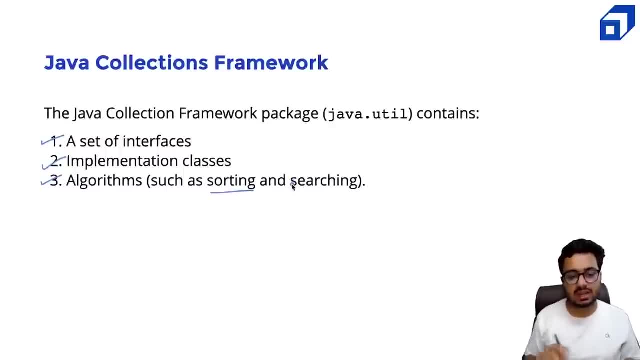 for searching, like binary search, available in the java collections, So you can just go and look at what all those methods are. But for now, what I will be doing, I will be doing a quick demo of interface versus a class so that you can really understand. 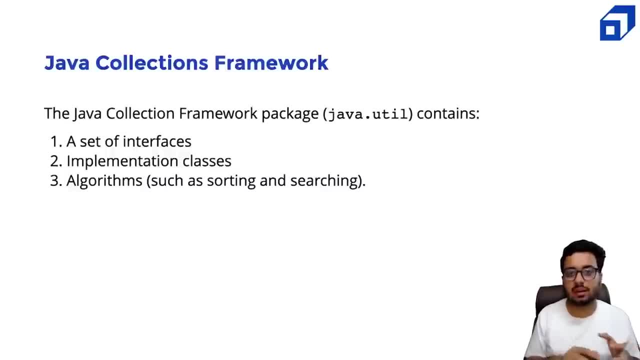 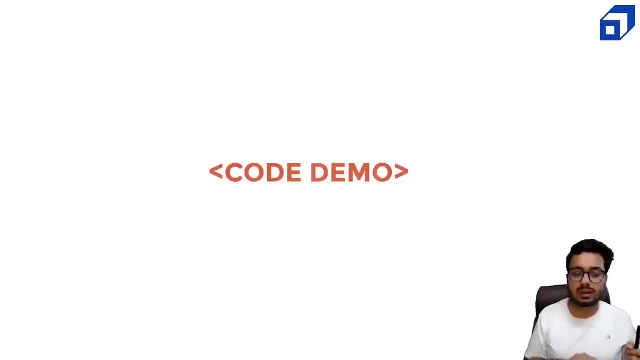 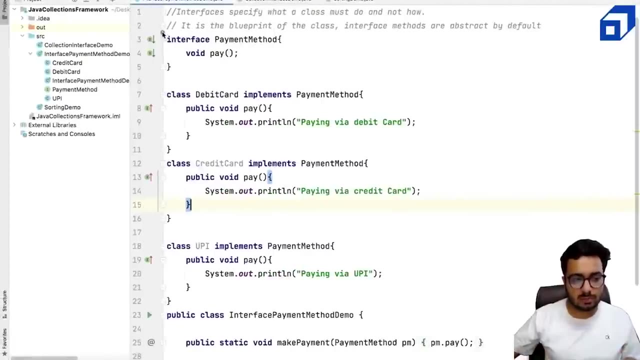 how these interfaces and classes are being organized inside the java collections. Let us jump into a small code demo to understand the concept of interface versus a class. In this example, what I have done, I have defined an interface called as a payment method. What is an interface? 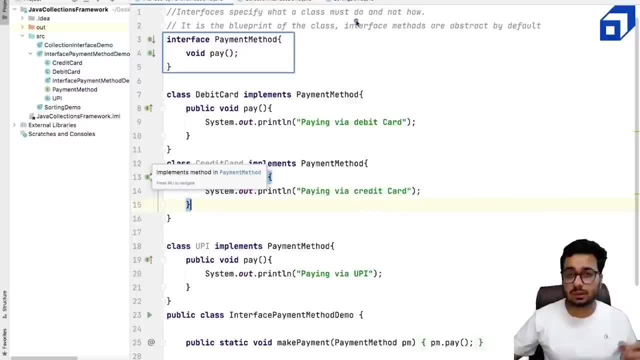 An interface specifies what a class must do and not how. That means we do not have the implementation of the pay method. We do not know how to make the payment, but we are saying there must be something called as a pay if it is a payment method, Any payment method. 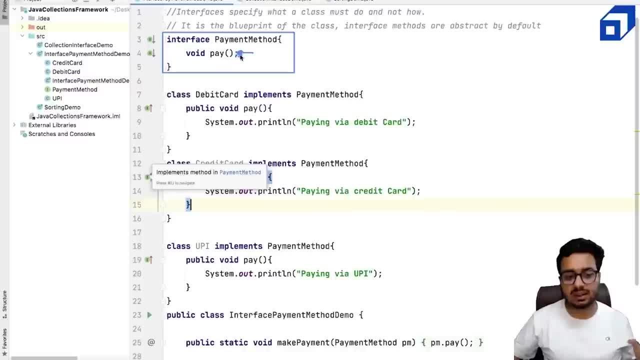 that we have must implement a pay method inside it. It is a blueprint for the class. Interface methods are abstract by default, so they do not have any code inside. Now suppose I have. I am going to create payment method called as debit card. Debit card is a class. 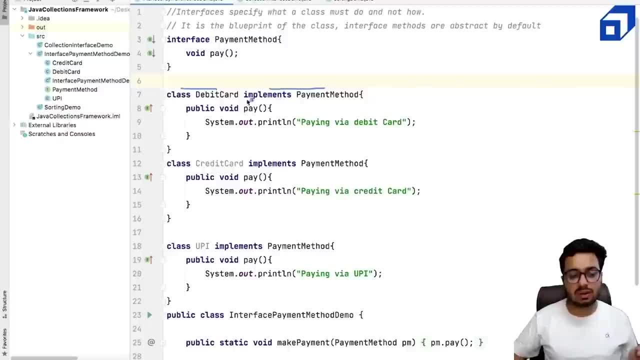 which implements payment method. That means now debit card must define a pay method. So for now I am just saying that debit card pay method prints paying via debit card. Similarly, I have one more class called credit card, which also implements the payment method I have. 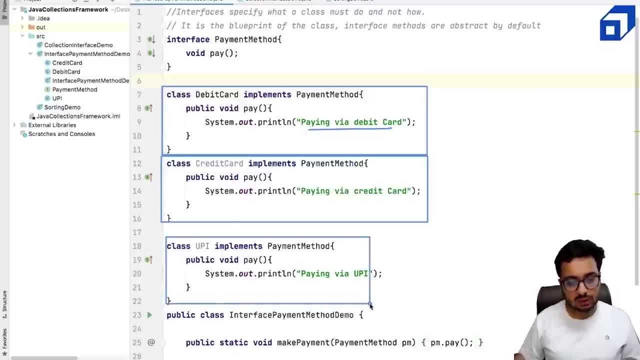 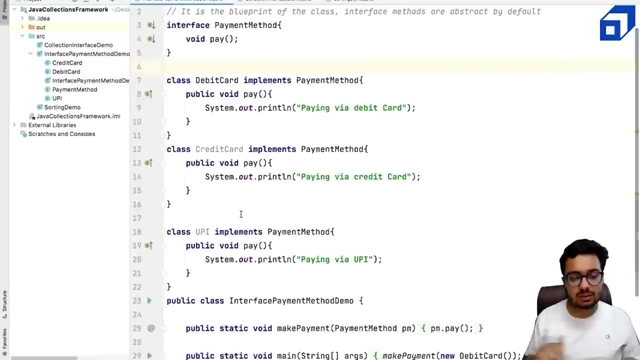 one more class called UPI, which also implements the payment method. All these classes, they have the pay method and they are implementing the payment method. There are different ways of creating the payment method. Execution of each payment method would be different. Credit card might have a different. 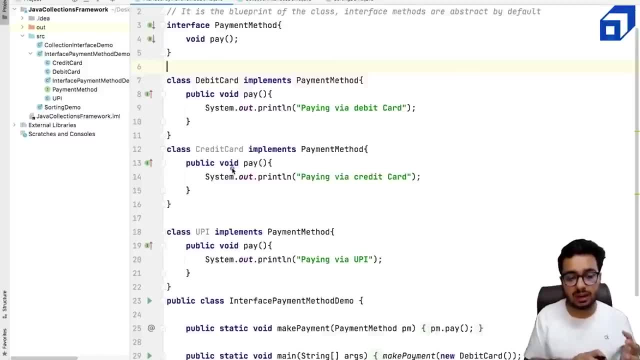 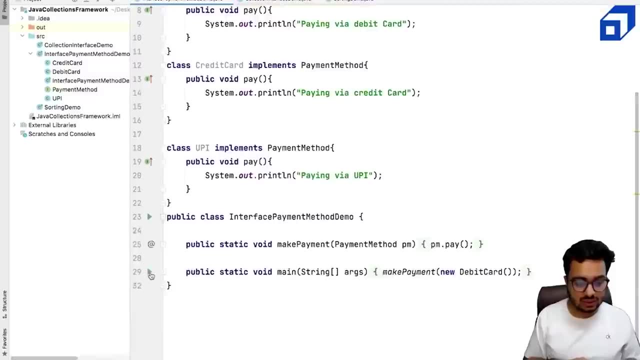 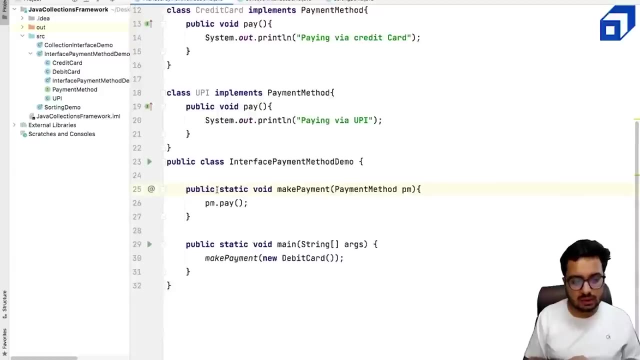 mechanism. UPI might have a different mechanism of making the payment. Debit card will have a different mechanism of making the payment. Why we are doing this? let us try to understand. Now suppose we have method called as make payment and this method can accept. 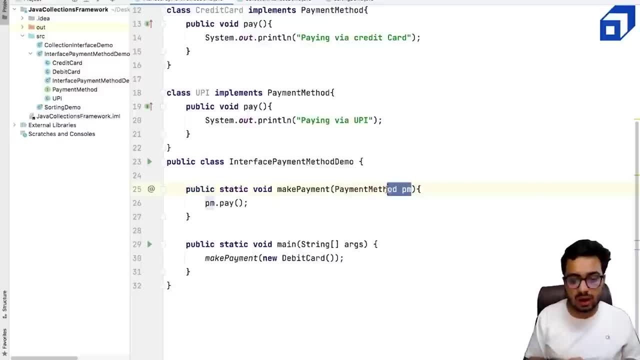 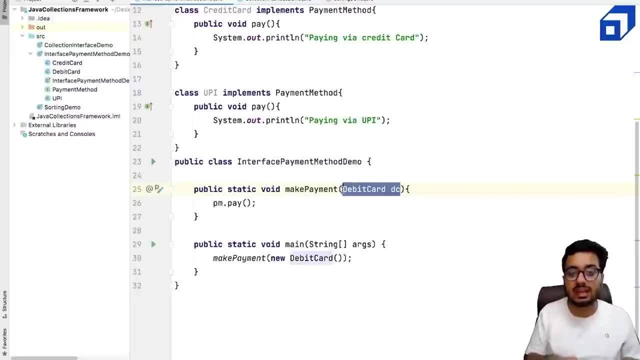 any payment method. I am not hard coding here. I am not saying that I will only accept debit card DC. I will not accept debit card. I can accept any payment method. One thing is: we need a general structure. We need a general data type. 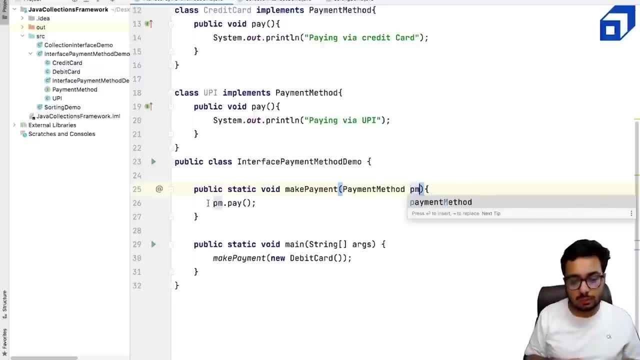 that can hold all payment method, And here I am going to call PMpay. Now why this method will work. Let me show you how do you create objects of it. I can say: debit card, DC, this is equal to new debit card, and I say: 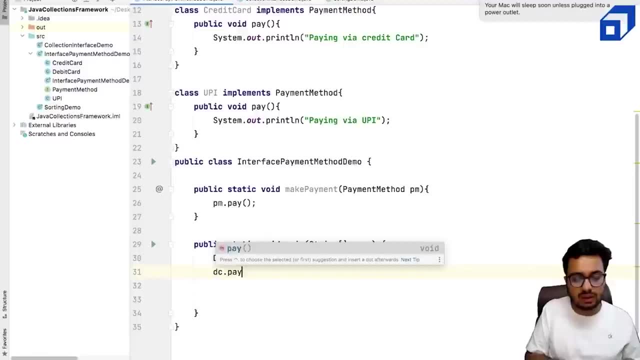 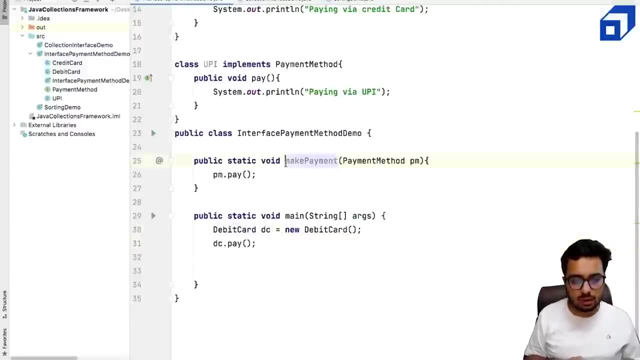 I am creating a debit card, Then I can call DCpay. This will work. I am creating a debit card. object: DCpay will actually work. right, I am not calling this method as of now, But what I can do is I can call the. 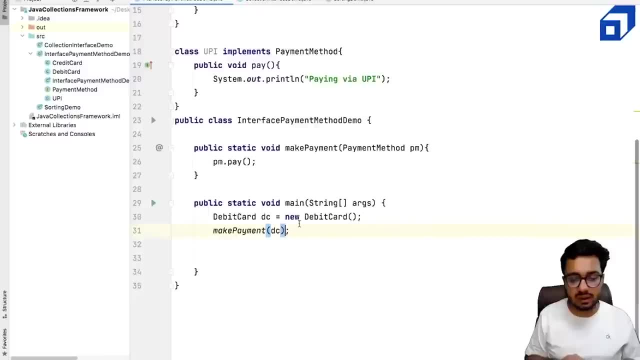 make payment method and I can pass it the debit card object. Why? Because debit card object demands the payment method interface. A better way to do it is suppose you have some code here. You say DCpay. Suppose your debit card is not working or the debit card service is down or there is. 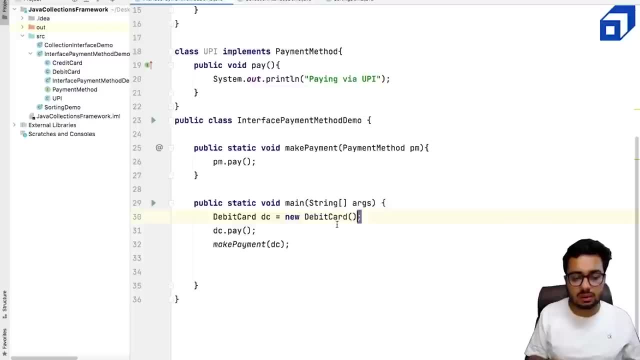 some issue and you want to make it change it to the credit card. You want to say: I want to try credit card. If you do this, this is going to give you a problem Because a debit card data type cannot hold a credit card. 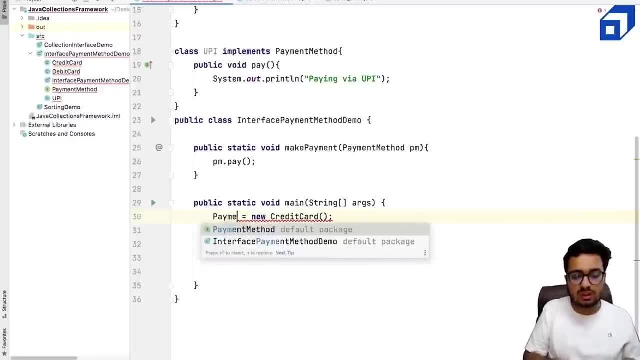 But what we can do is we can use more general data type. that is payment method. Payment method is PM. I can say, on the left side, I will have a payment method which is implemented by a credit card. Payment method is a more general data type. This is a good 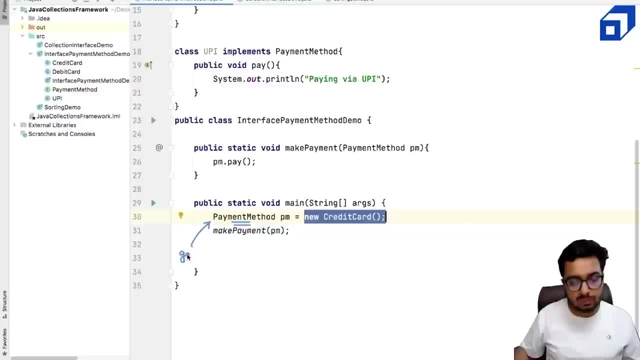 design practice as well. This data type, we will keep it more generic. This is a specific class that provides implementation of methods defined in this class. This is a specific class. This could be credit card. This could be debit card. This could be UPI- I can pass. 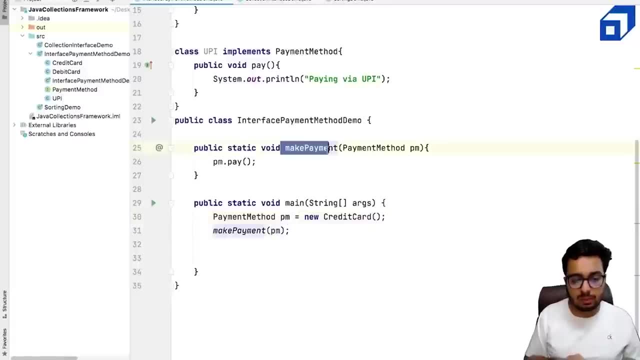 this object PM to any method make payment. It does not care whether I am going to call the pay method of debit card, credit card, UPI. Whatever is the object passed, it will call the pay method of that object. That means, with minimum change in code we can. 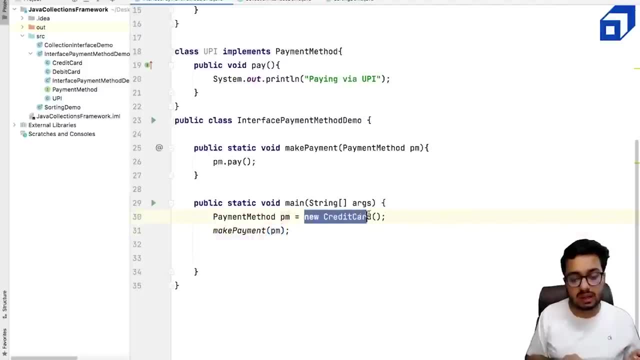 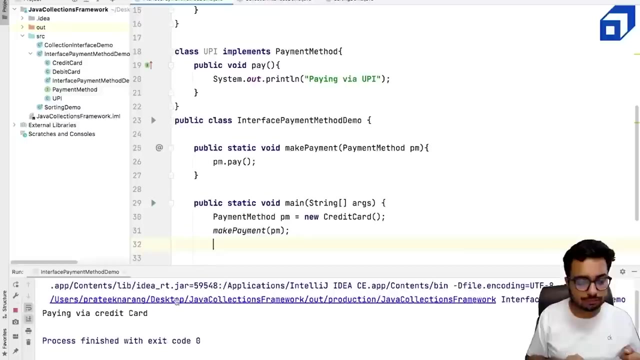 achieve this general behavior. Any payment method object will work inside the make payment method. If I go and run this code, I will show you what is going to happen. It will say: I am going to make a payment using a credit card. Paying via credit card. 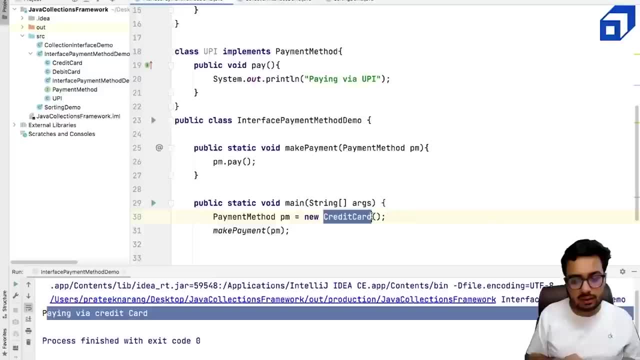 If I say no, I will make it UPI Without changing your make payment method. you have just changed this object. It will pay via UPI. I am going to run this code now: Paying via UPI, That means this object reference. 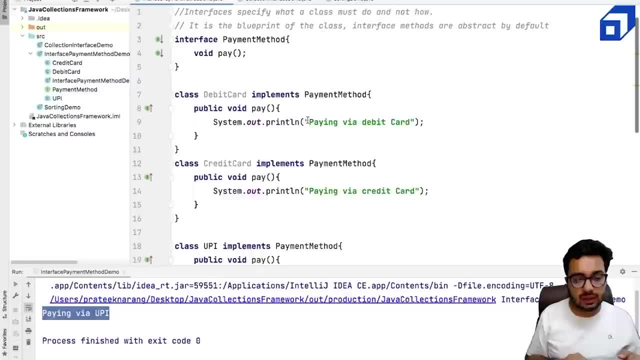 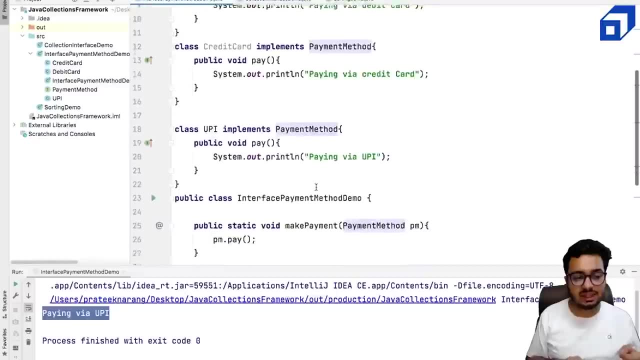 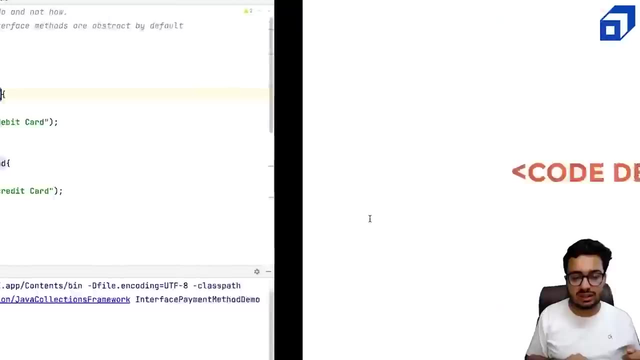 can hold any object, Any object which implements the payment method interface. That is a quick revision about interfaces and classes in java, and collections framework heavily uses this concept of interfaces and classes a lot. Let us look at how this is implemented in the collections framework as well. 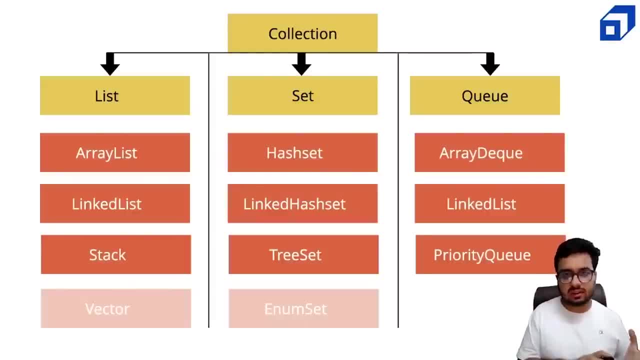 There are so many components inside collection framework. There are interfaces, there are classes, there are child interfaces, there are child classes, and the hierarchy is bit complex. What I have done is I have drawn a simplified diagram so that you can understand how these components are. 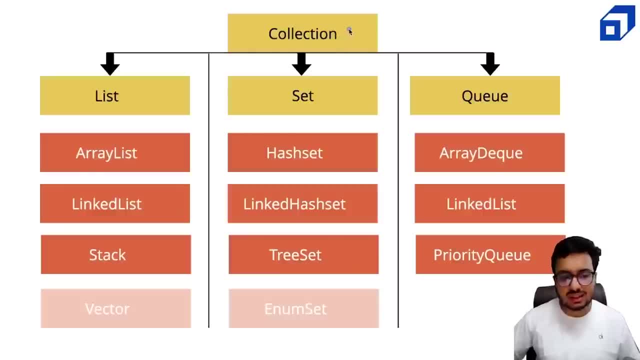 related. On the top we have something called as a collection interface. Collection is an interface inside collections framework. There are three more interfaces which are child interfaces of the collection interface. They are list set and queue. They all extend the collection interface Queue. 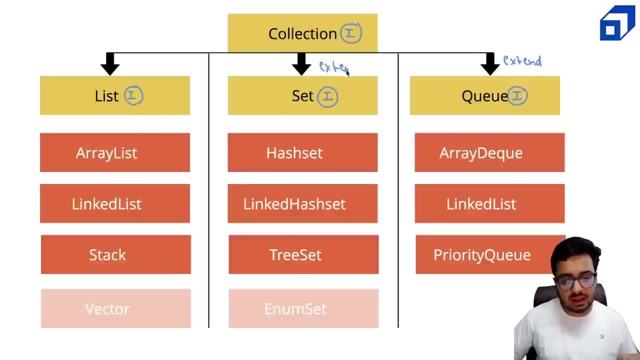 extends collection. set extends collection and list also extends collection. That means some methods are there in collection and list adds some additional methods which are specific to the list. Set adds more methods which are specific to the set. Queue adds more methods which are specific for the. 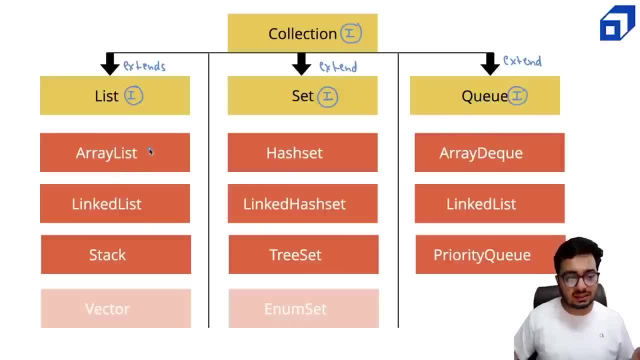 queue like behavior. And then there are implementation classes which actually implement a list. So ArrayList implements a list. the other way: The ArrayList is going to implement a list, LinkList is also going to implement a list, Stack is also going to implement a list. 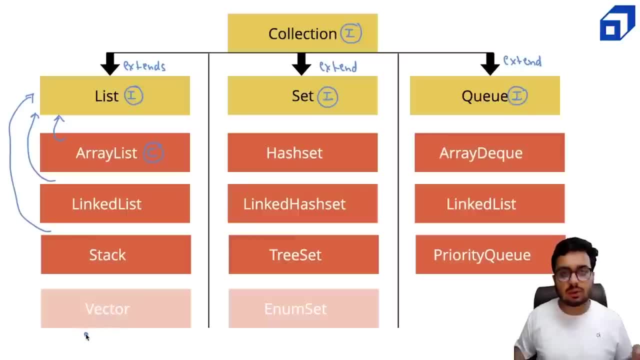 Vector is also going to implement a list. So a vector is a concurrent data structure. That means if you need to work, if you need to share this data structure across multiple threads, then vector is the synchronized data structure. So we are not going to do concurrent. 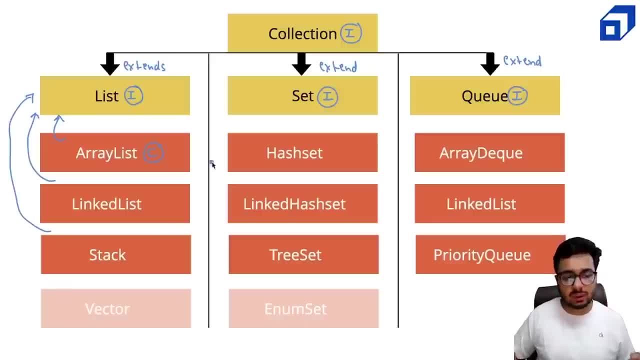 data structures in this tutorial, So I will leave vector at the moment. Similarly, HashSet implements the methods of the set, LinkList implements LinkedHashSet implements methods of the set And TreeSet also implements methods of the set. Now, what is the difference? 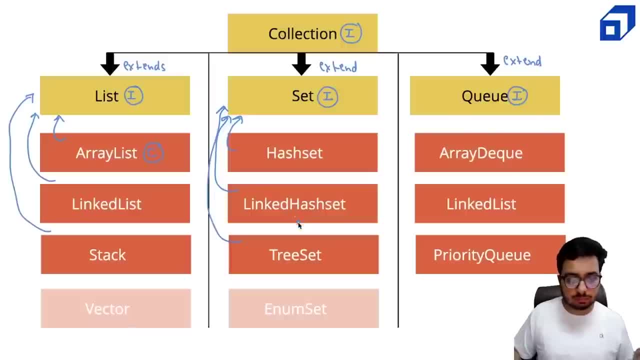 The way these methods internally work, that is different. TreeSet might use something like a self-balancing binary search tree, whereas HashSet might use the concept of a hash table to store the data. So the implementation of methods is different, and their time complexities they are also. 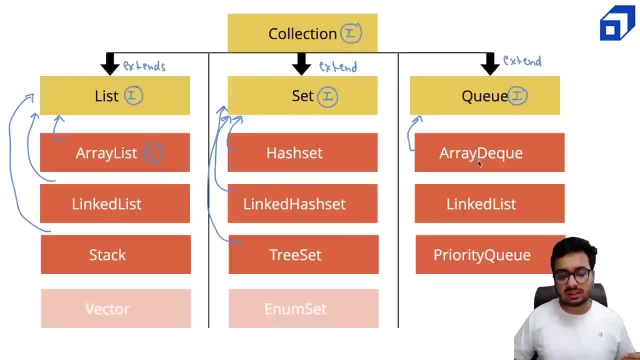 different. So for queue, we have three implementations. We have ArrayDeck, which is a double ended queue, we have a link list which is like your, which serves as your FIFO link list, and there is a priority queue which again internally uses a heap-like data structure to give. 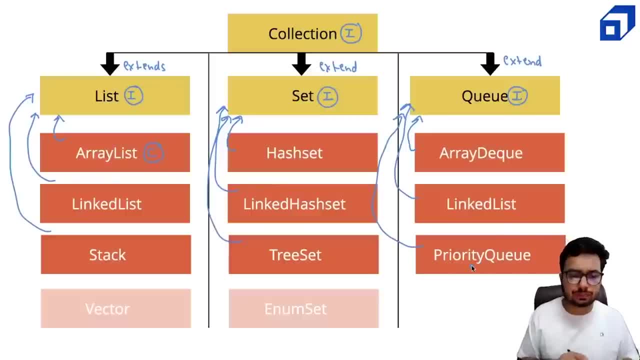 priority to the elements which should come first, right? So we have interfaces and we have classes that implement those interfaces. The ones that are in the orange, they are the classes. the ones which are in yellow, they are the interfaces, right? So I hope you understood this simple hierarchy. Now you might. 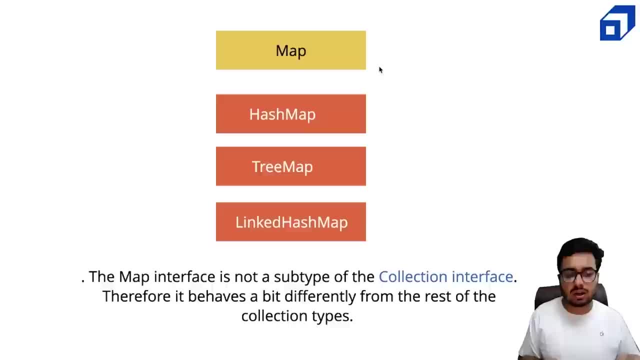 be wondering: where is HashMap? HashMap is not a part of collection interface. It is not a subtype of a collection interface. It has been kept separately and it behaves differently from rest of the collection types, So that means the map will be treated differently. So map is an interface. 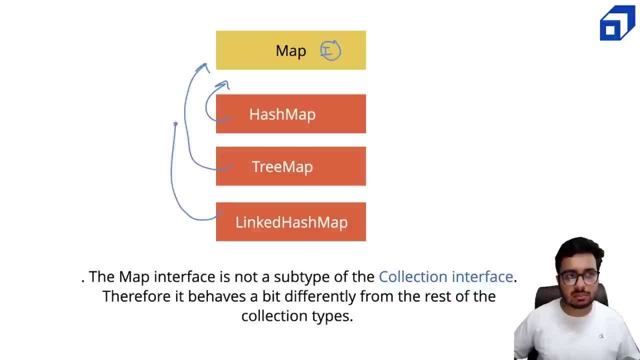 that we will look and HashMap, TreeMap and LinkedHashMap. they are the implementations for the map interface. right? We will use one of these implementations if you want to build something like a map which can store key value pairs. So we will understand the differences between these implementations as we go. 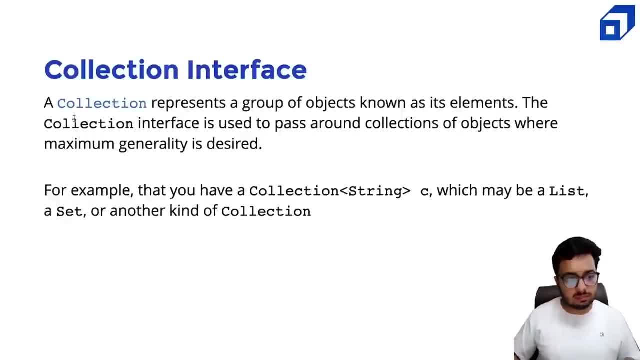 through this tutorial, right? So let me tell you little more about collection interface. The collection interface. it is a general interface. it represents a group of objects which are known as elements. It is simply grouping different objects and it is used to pass around collections of objects. 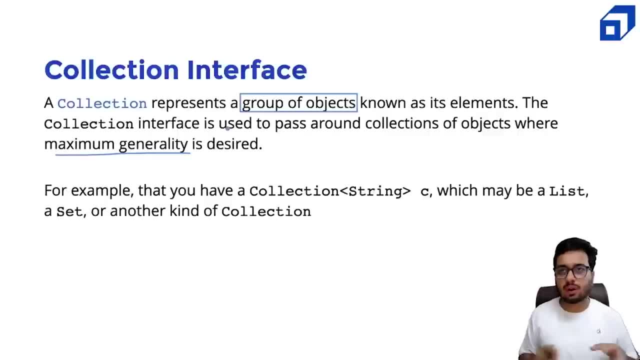 where maximum generality is required. okay, You just want a group of objects. you don't want to use specific priority queue method or specific queue method, or you don't want to use specific HashMap method, right? So you just want some general methods that I should be able to add into the collection. 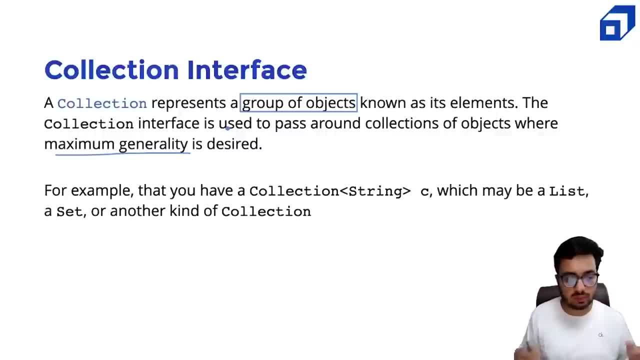 I should be able to remove from the collection. I should be able to delete from the collection, right? For example, you have a collection of string of this collection. again, it might be implemented using a linked list. It might be implemented using a set. It might be implemented. 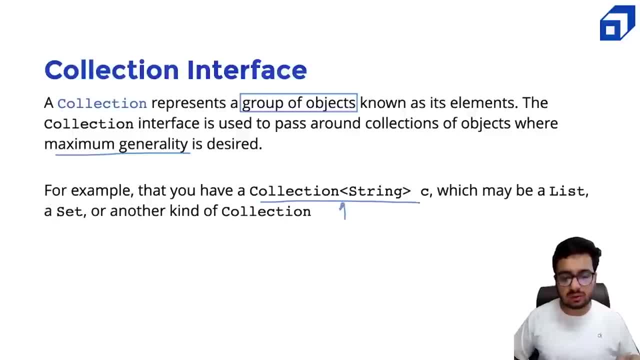 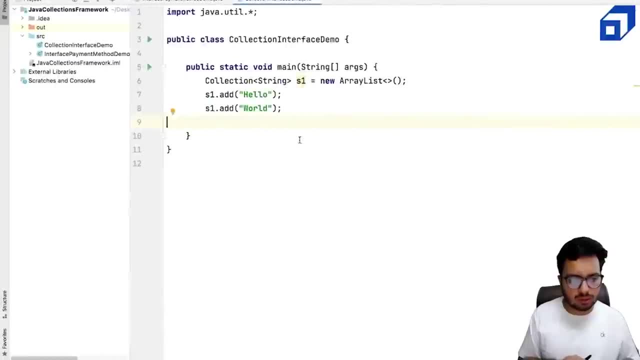 using a ArrayList We don't know, right? So we have to provide one way, implement or represent this group of strings, right? So let me show you a code demo here. So I have collection of string s1 now this interface collection is an interface. 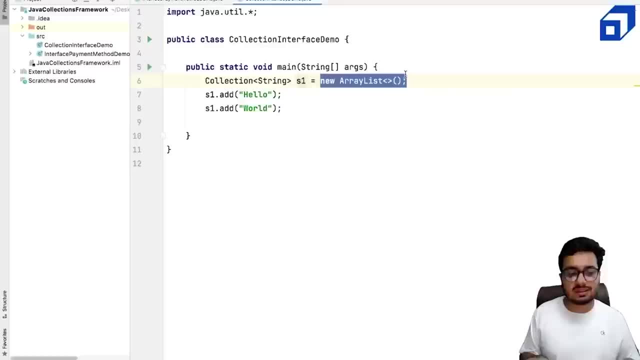 so I need a class to implement it. So I say, okay, this collection will be stored using a ArrayList. So I am adding something into the ArrayList, right, I am saying s1.add- hello, s1.add world. right Now you might ask: where is this add method defined? 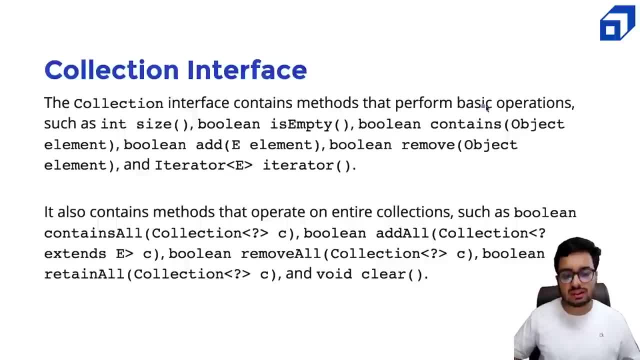 So I will tell you. the collection interface contains method that performs basic operation, So such as size. every data structure, you need to get its size. Every data structure should know whether it is empty or not. Every data structure should know whether a particular object is present inside it or not. 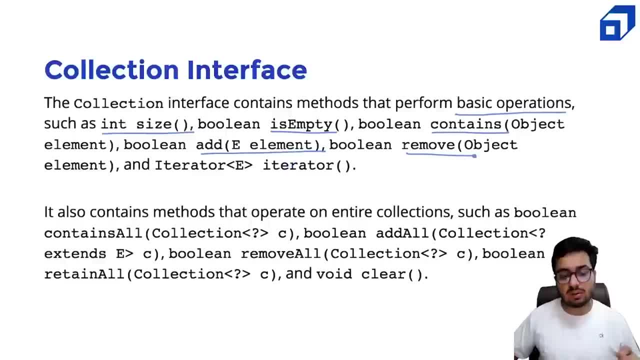 Every data structure should support that. I want to add some element. I want to remove some element. I need a iterator. It also contains methods that operate on entire collections, such as add all Given another collection. can I add all the elements of this collection into the current collection? 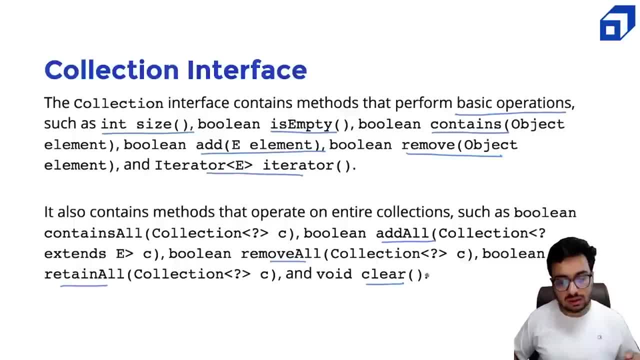 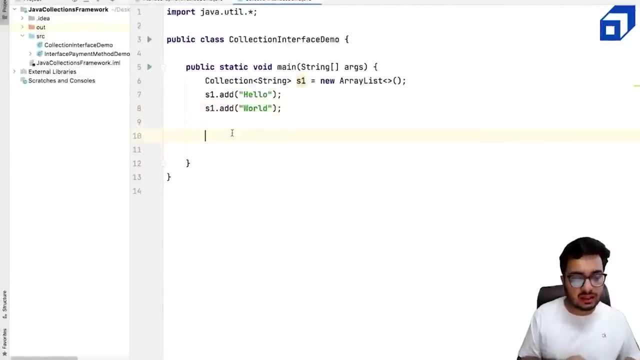 Yes, I can Remove all, retain all Clear. These are general methods that are defined in the collection interface. that means all the implementation classes will have to define these methods. Let me show you something here. So let us say I create one more collection. 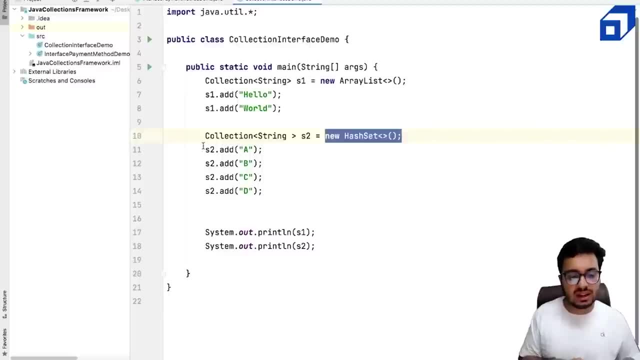 and this collection is implemented using a hashSet. In this hashSet, I am adding two strings: a, b, c and d. Now this add function is going to behave differently from this add function, because this add function is implemented by the ArrayList, But this: 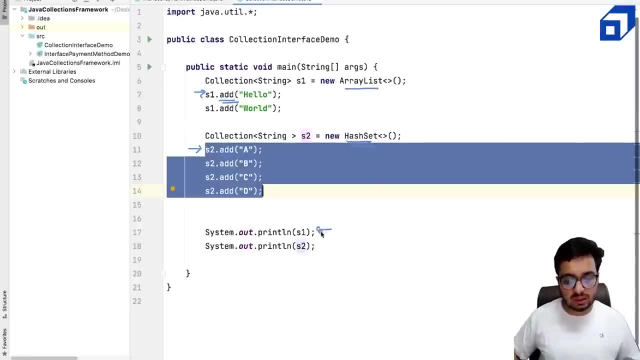 add function is implemented by the hashSet. So if I print s1 and s2, I would be able to see there are two group of elements. If I just run this code I will see I have collection s1 and I have a collection s2.. 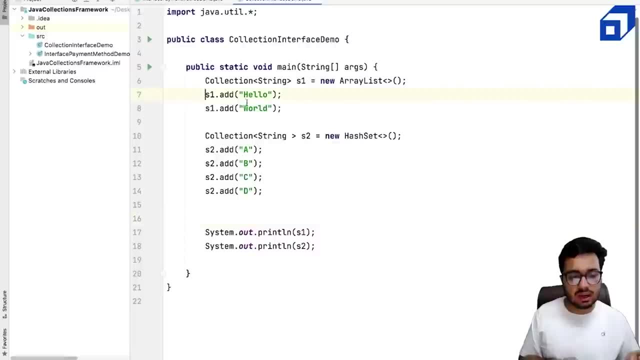 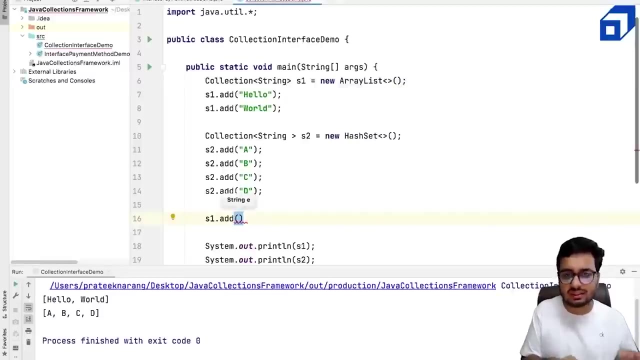 Now suppose I want to add all elements of s1 into s2.. Can we do that? Of course I can do that because the collection interface gives me methods like addAll, So s1.add. I can give any collection here. I can give list, I can. 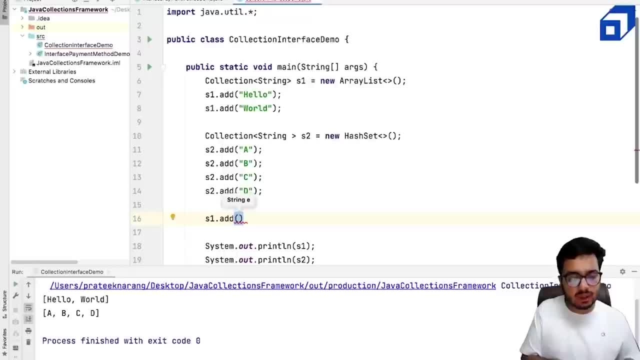 give ArrayList. I can give queue. I can say okay in my hashSet I want to add all elements of ArrayList. That is s1.. I can pass another collection into my addAll method. Method is addAll. It's a general method. 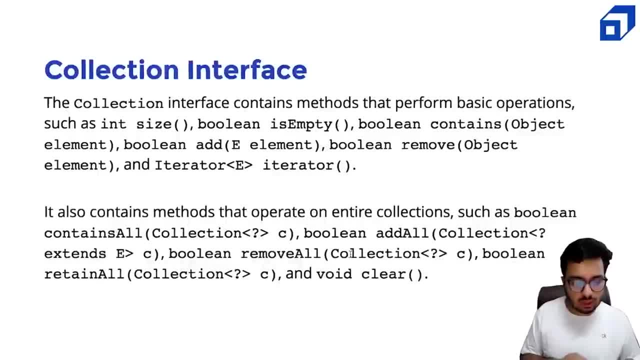 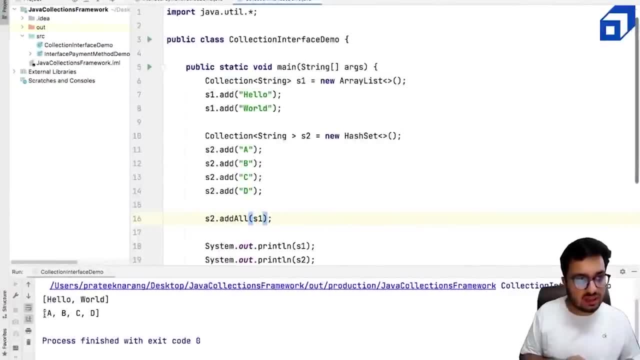 Any collection can be passed. This is what it means. Method is addAll That's correct. So let's go and run this code Now. if I see a, b, c, d it's here, I will also see: helloWorld is also there. 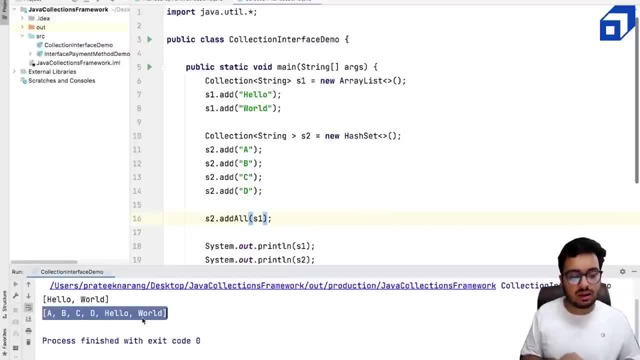 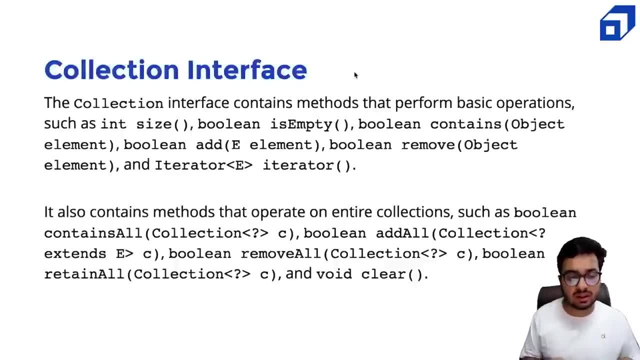 You can see all elements of s1. they got added into s2.. All these general methods, they are defined in the collection interface. I hope you are understanding it. So that is at the top right Now. why we are learning this? Because we want to use these data. 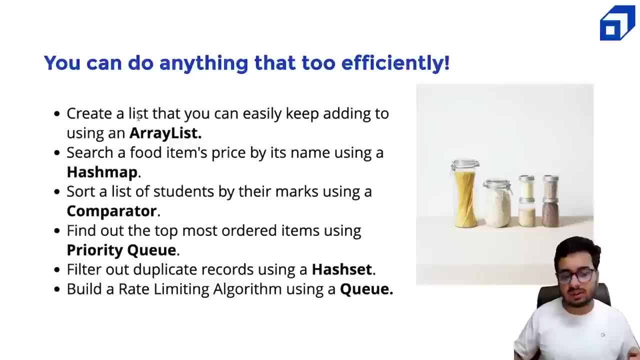 structures to solve problems efficiently. It is so powerful that we can do lot of things. For example, we can create a list in which we can keep adding to. We just saw an example of ArrayList. We can search items very quickly inside a HashMap. 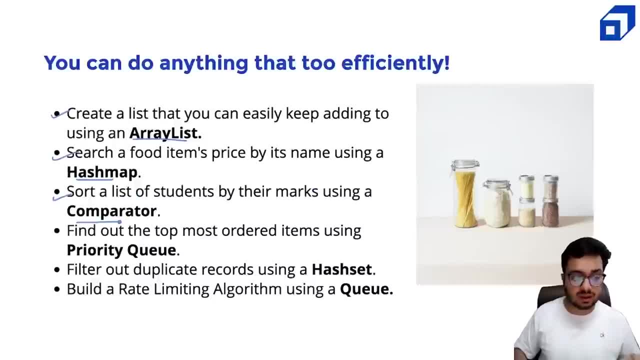 We can sort a list of students by using a comparator. We have just seen comparators. We can also find top most ordered items using a priority queue. We can filter out duplicate elements using a HashSet. We can build a rate limiting algorithm using a queue. We can do. 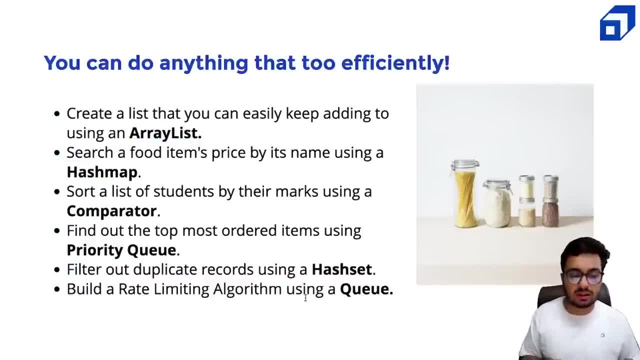 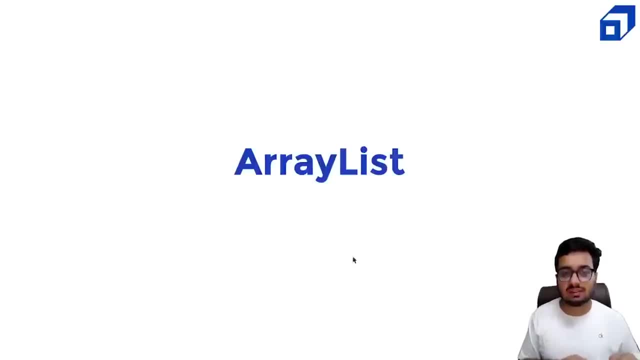 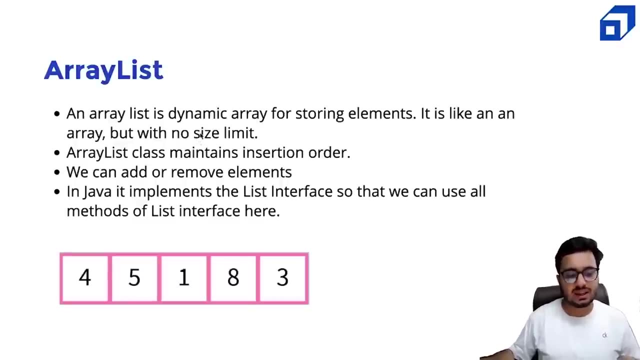 lot of stuff using the collection framework, and that is why we are learning it Now. next we will dive into specific classes, and the first class that we will start is ArrayList. Let us talk about ArrayList. ArrayList is like a dynamic array for storing elements. It's an array, but 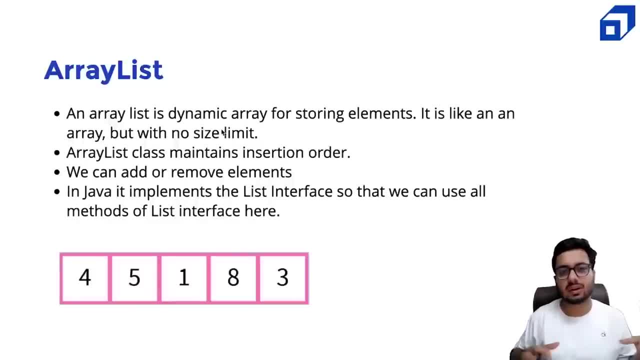 with no size limit. That means if an array gets full it will grow in size and it can accommodate more elements till you have memory available inside your heap. ArrayList class is a dynamic array. It maintains the relative insertion order. If you add element, it will always. 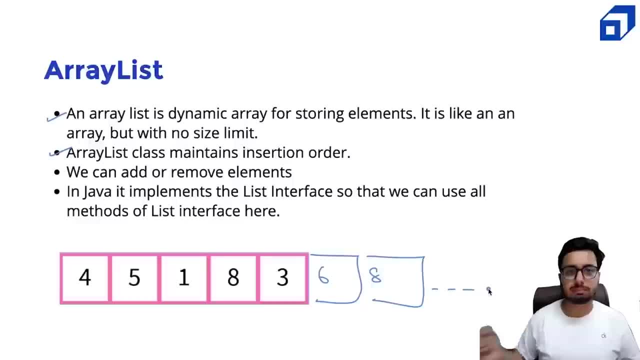 get added at the end. That means we will get the same order as insertion. We can add or remove elements. Even we can search for elements, and it implements linear search. That means it will take linear time to search it In Java. it implements the list interface. 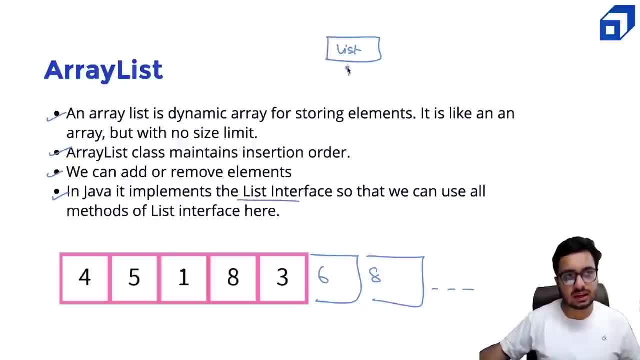 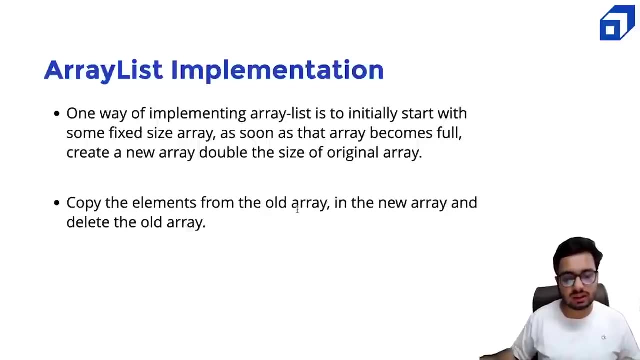 so we saw that list is an interface and ArrayList is an implementation of list interface. All the methods that are available in the list interface are implemented by ArrayList. Now how it is going to work internally, I will give you a quick idea. Internally it 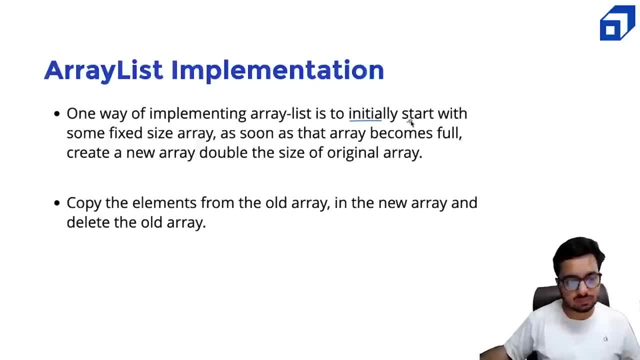 uses a fixed size array only. It starts with some fixed size array In Java. the default size is 10.. By default it will create a new array of size 10 and as soon as the array gets full it will double the size of the original. 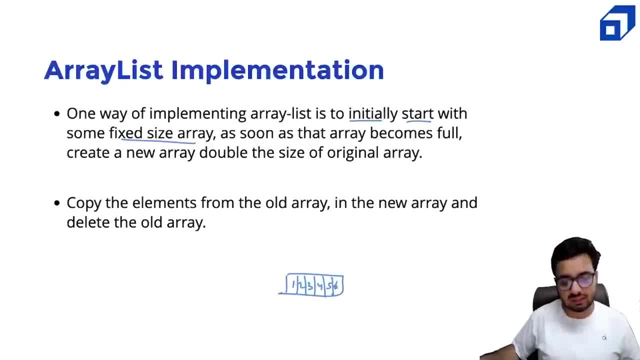 Now that doubling cannot happen in the same place. Suppose this array was full. What it will do? It will create a new linear array. Suppose this size was 10.. It will create a new array of size 20 and it will copy all these elements into. 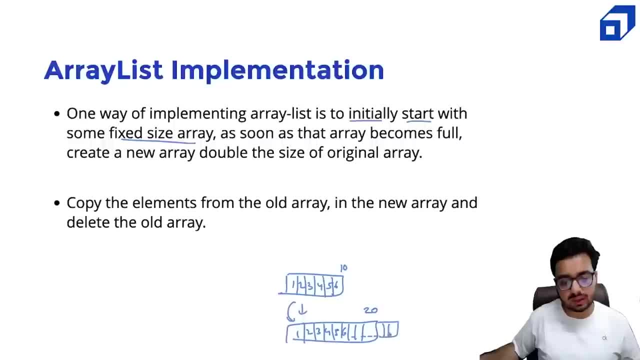 the new array And then you will have some extra buckets for new elements. Once this gets full, it will again delete the previous array. It will create a new array of double the size Copy elements here and delete this array as well. This is how it happens. 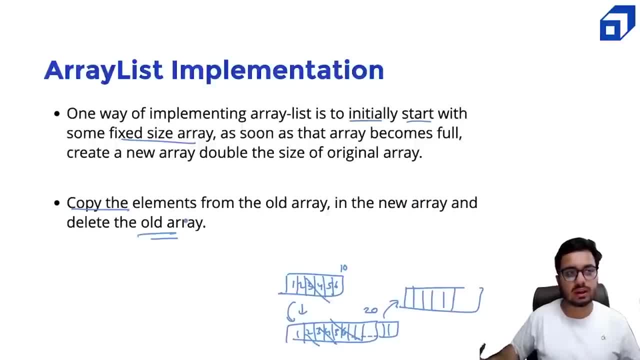 Copy the elements from the old array in the new array and delete the old. This is how this array actually works. That means the doubling of the ArrayList is an expensive operation and we should reduce the frequency of this doubling. How do we do that, If you know? 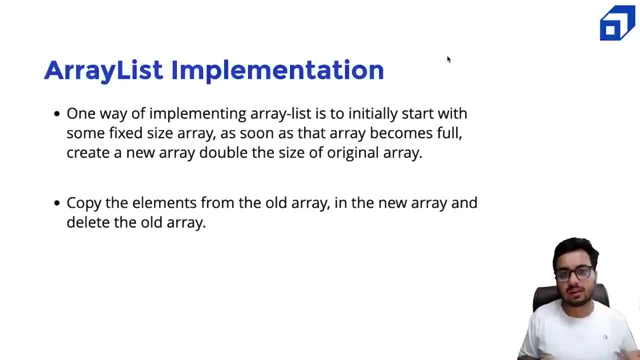 you are going to store 1000 elements, create an ArrayList of initial size 1000.. If you by chance exceed 1000, the doubling will happen. The array size will become 2000.. It is a good idea to start with some initial size that is equal to. 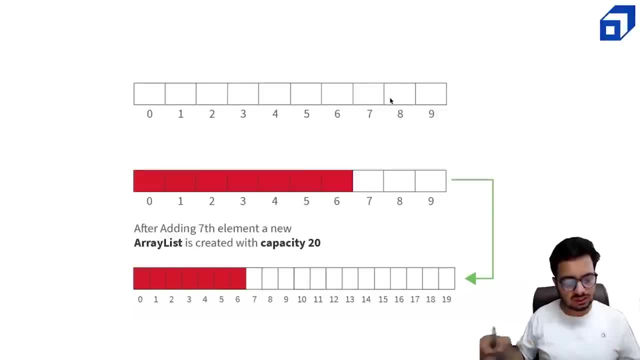 your requirement. In Java, this doubling procedure is little different. It says: okay, I will maintain something called as a load factor. This load factor is, I think, around 0.7.. That means if 70% of your array is full, the doubling will get triggered. 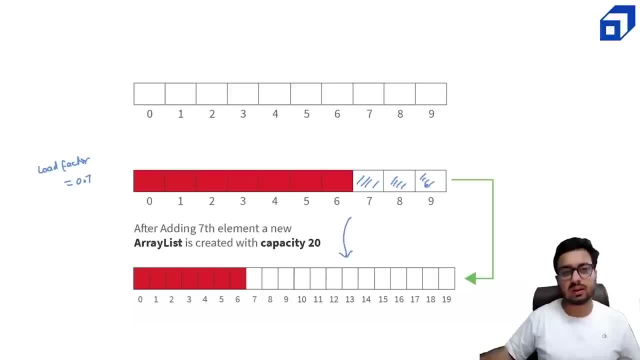 So we will not wait till filling of 100% of the array. If 70% of the array gets full, the doubling function gets triggered After adding the 7th element. if the initial size was 10, new array is created with a capacity of 20.. 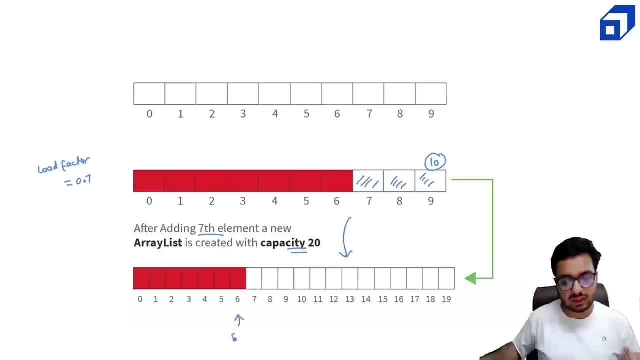 There are two things. When you talk about size of the ArrayList, it tells you how many elements are currently stored in the ArrayList. If you use the size method, it is not. the capacity Capacity is generally more than the size. Capacity is how much space has been. 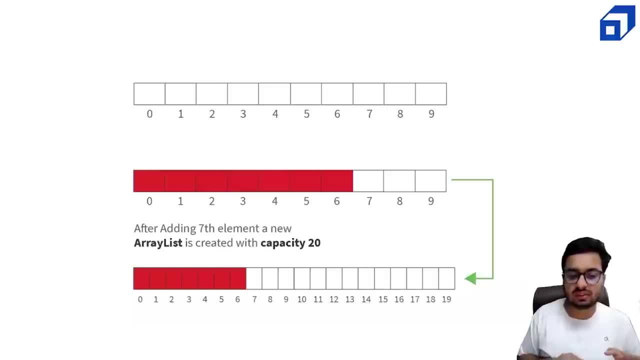 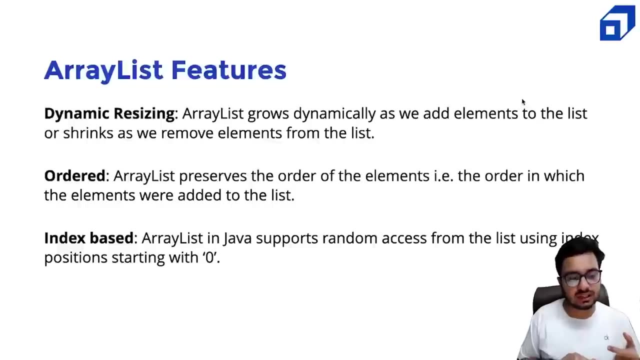 allocated internally, Whereas size is the number of elements that we have stored in the ArrayList. So what are the features? It is dynamic in size. It can grow and shrink in size. Secondly, it is ordered. It preserves the order of elements. Third, it is index space. 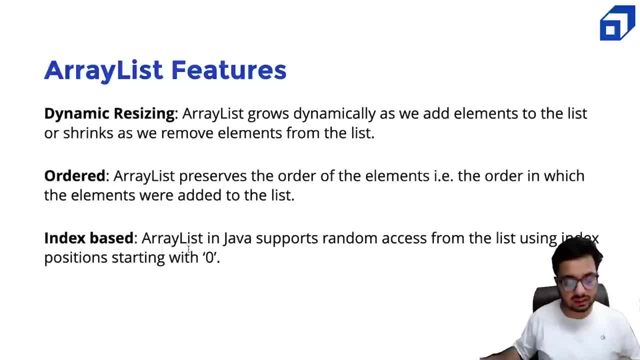 Just like an array, you have indices. ArrayList also have indices. If you want to access a particular element, Okay, I want to get this ith element. You do not write array of i. Instead, you write ArrayList dot get. i Give me the ith. 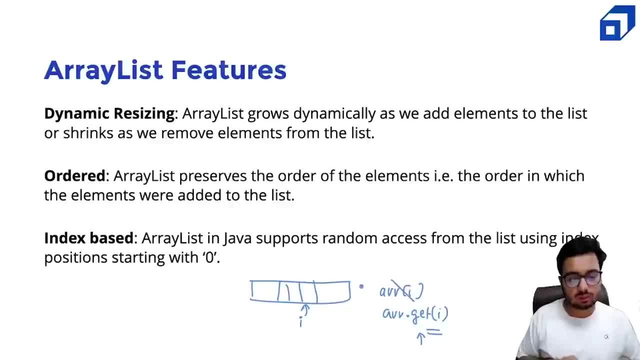 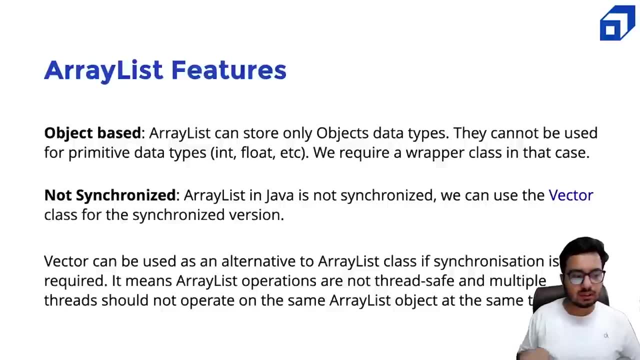 element. Get is a method that you will use to access any ith element, So this also works in order. one type Indexing is zero based, So another property you need to know is it is object based. ArrayList can only store object data types. 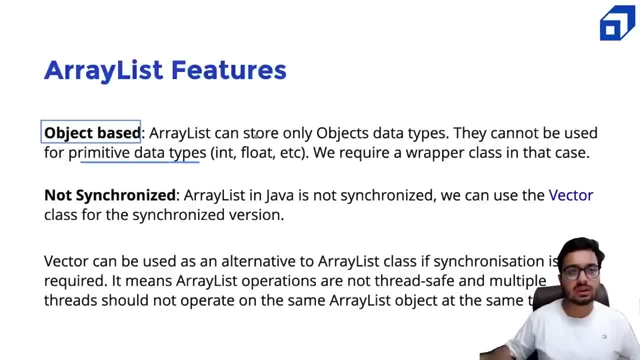 That means it cannot be used with primitive data types. You cannot create an ArrayList of int, float, etc. Then you might be wondering: how do we create an ArrayList of integers? For that you have to use wrapper classes. In Java, the wrapper class for int is called as: 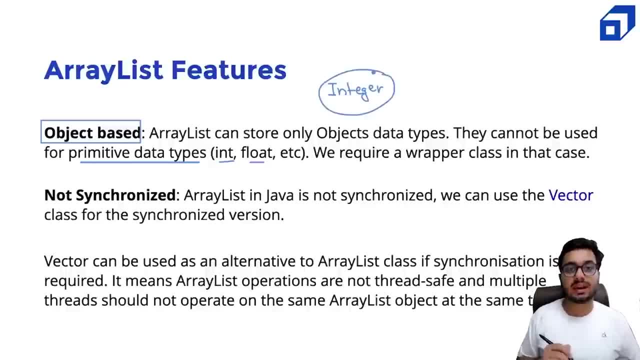 integer. So you will always create an ArrayList of the data type integer, not as int. And secondly, it is not synchronized. That means it is not a concurrent data structure. If you need, if concurrence is important for your application, you have to use. 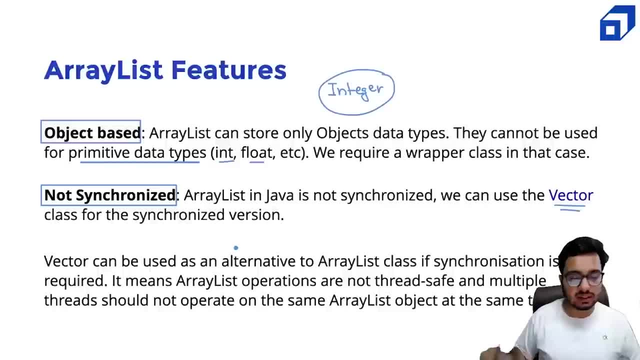 vector, which is the synchronized version of ArrayList. So ArrayList operations are not thread safe and multiple threads should not operate on the same ArrayList. So this is a basic data success tutorial. If you want to learn about advanced concepts, we will cover it in some other video. 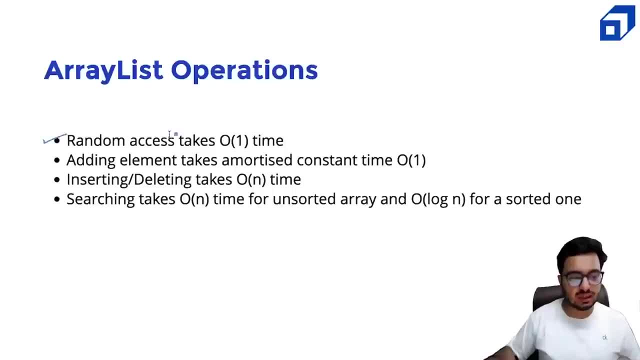 So what are the operations? We can get any element using the get function. We can add any element using the add function. We can also add more elements using the add all function. So I give you a list. I want to add it. I can use add all. 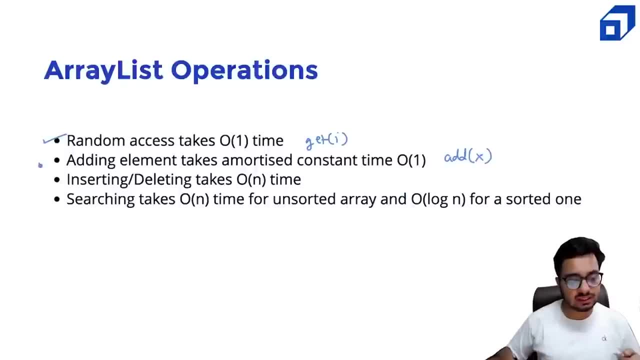 I can give some element x that can be added. Insertion and deletion In the middle. it is going to take order of end time. So if you insert something in the middle, right, So it is okay. I want to add something in between. it will require shifting of remaining. 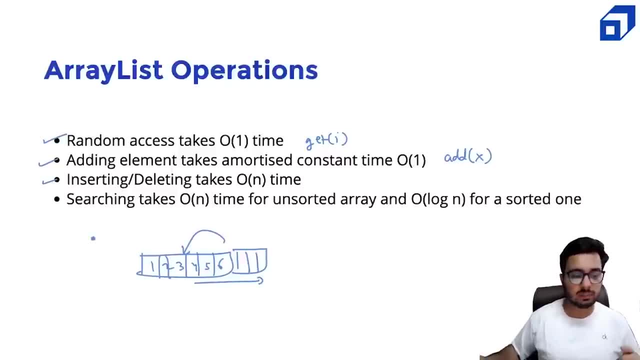 elements. That means that will take order of end time. Searching takes order end time By default. if you use the contains method it is going to do linear search, But if you know the ArrayList is sorted then you can use your own binary search method or 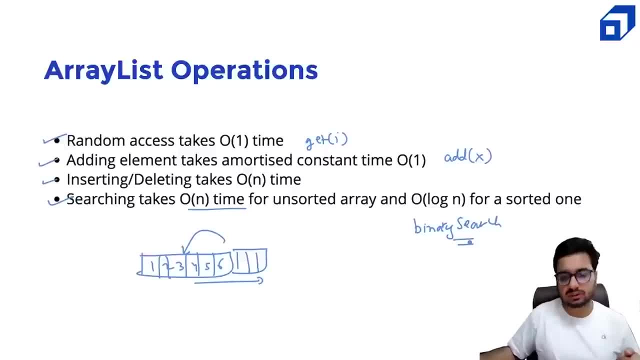 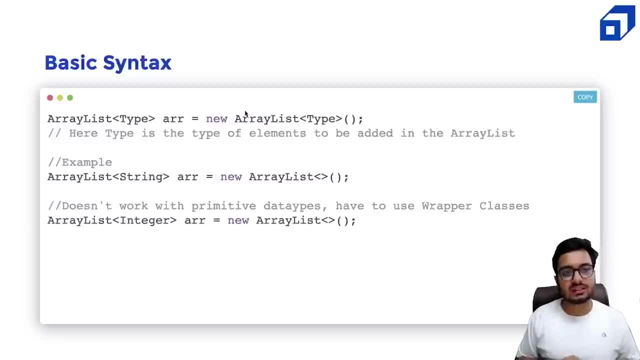 the binary search provided by the library function. You can use that as well. That searching will take log end time if your ArrayList is already sorted. Now let us look at basic syntax: How we can create an ArrayList. ArrayList- this is you have to define. 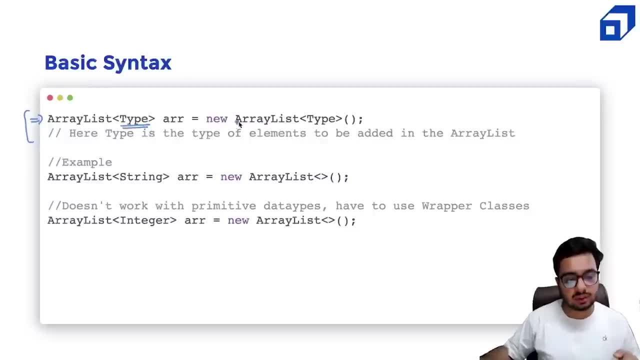 what kind of object you want to store here, And then you say, okay, I want to create a new ArrayList object. So this is how we do it. For example, you can create an ArrayList of strings And you say it is a new ArrayList. You can create an ArrayList of. 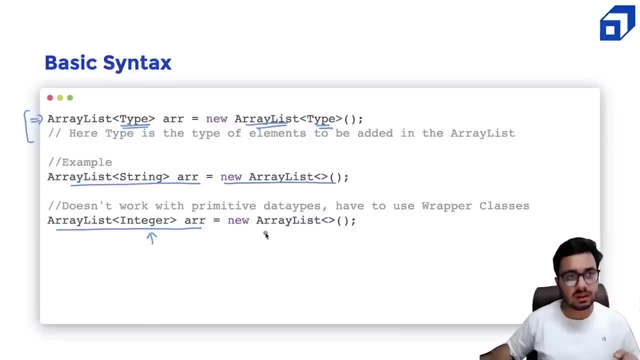 integer. I told you it does not work with primitive data type. You have to use other upper classes. In general, I would make this left data type to be of the list type, because ArrayList is a type of a list And as a good design. 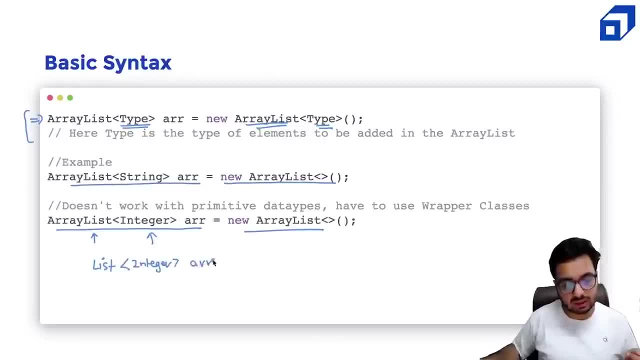 principle, it is preferred that we make this data type more general as possible. So we can say, okay, the list we are creating an object of the type list Implementation is given by new ArrayList. This is a more recommended thing to do than doing ArrayList This. 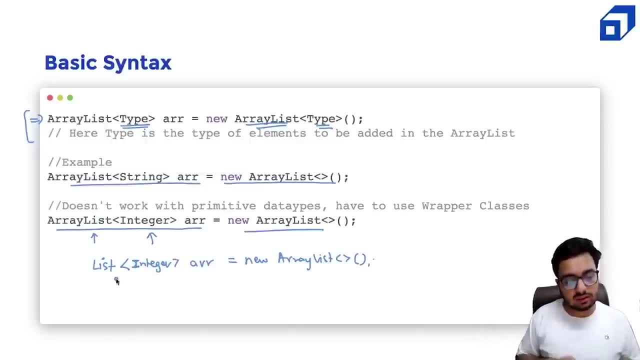 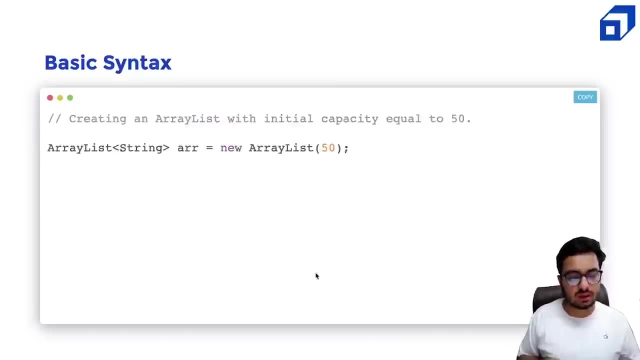 you will learn in the design principle. So we will create an object of the type list, which is implemented using the ArrayList class. This is what we will do. So we can also use the constructor to give an initial capacity, So you can pass a number. 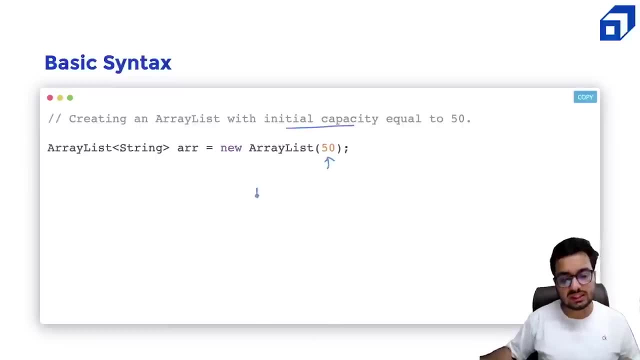 here that will tell me. okay. I want an ArrayList whose initial size is 50. it is not going to be 10. So by default the initial capacity of the ArrayList would be 50. That means until this ArrayList is not full or it is not 70% full. 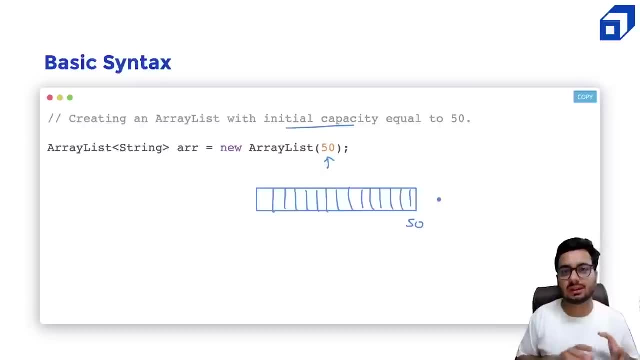 the doubling will not execute. If you know that you are going to work with 10,000 elements, create an ArrayList of size 10,000 or 11,000 so that your doubling does not happen again and again Because it is an expensive operation. 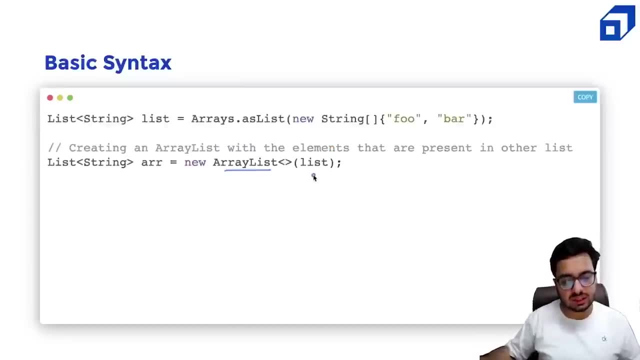 We can also initialize ArrayList using another list, So you can give another list. for example, here we have a list of strings which is storing foo and bar, And I am going to initialize an ArrayList with another list. That is also possible. So we have seen three ways. 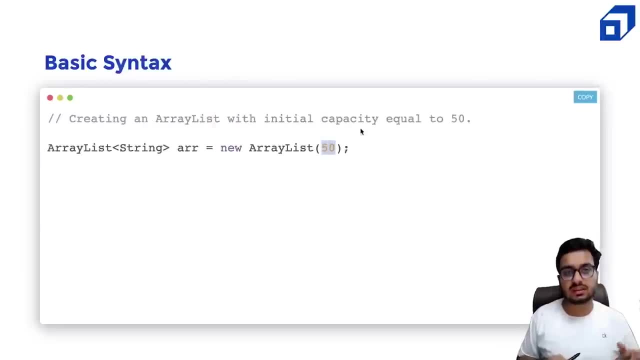 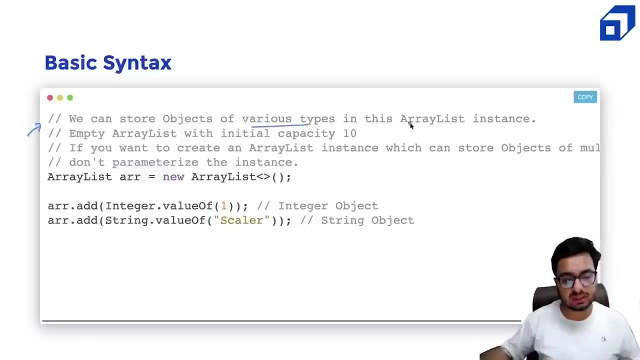 Default constructor, a constructor with the initial capacity and a constructor that accepts another list collection to initialize this ArrayList. Now, one more cool thing about ArrayList is we can also store objects of various types in this ArrayList. Why So, if you want to create an ArrayList which can store 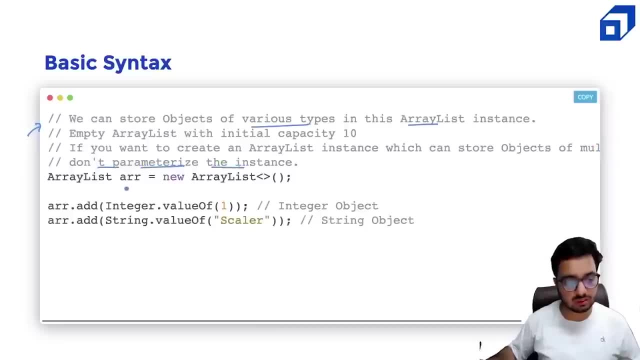 objects of multiple different data types, then don't parameterize the instance. If you see, here I have not specified any specific data type. here That means, this ArrayList can store different object data types. So I can add an integer. So I am saying: ArrayList dot add. 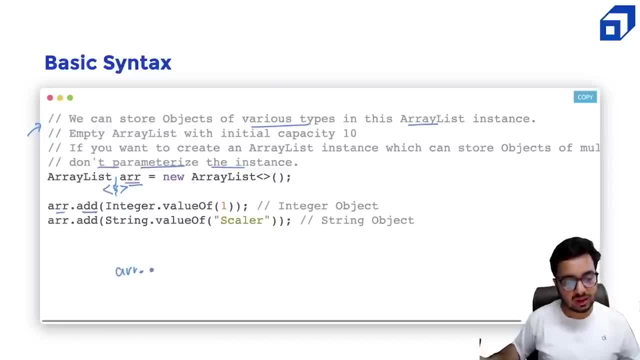 integer dot value of 1.. Now you might ask why I cannot do this: ArrayList dot add 1.. Because it is of the type int, So I need to type cast this into integer data type: Integer dot value of is a method that creates: 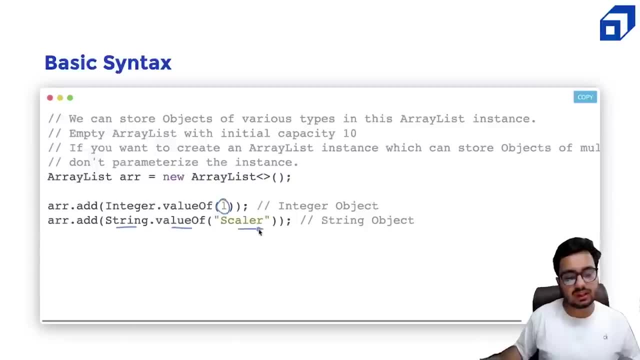 an integer object out of this one String dot- value of scalar. So this is optional. We can simply say ArrayList dot add scalar. So it is going to add a string object inside my ArrayList. If I show you in the demo, I have created an ArrayList here. 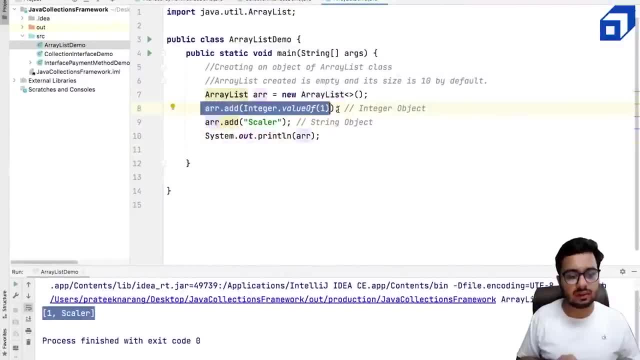 I say okay, ArrayList dot add integer dot. value of 1. This is going to add an integer. and then ArrayList dot add scalar. So I am storing an integer object and a string object inside the same ArrayList. So this is also possible. So you see the output here. 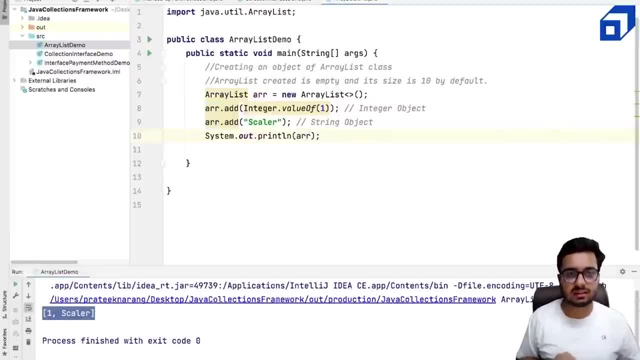 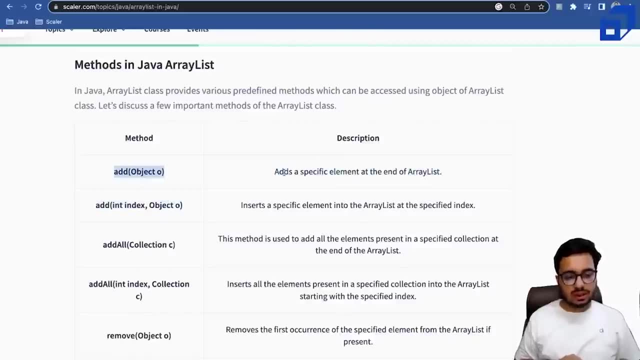 Let us talk about some more methods of ArrayList. So predefined methods include lot of methods. So there are methods for adding objects. If I simply call the add method, it will add at the end of the list There is a add method which also accepts an index and an object. 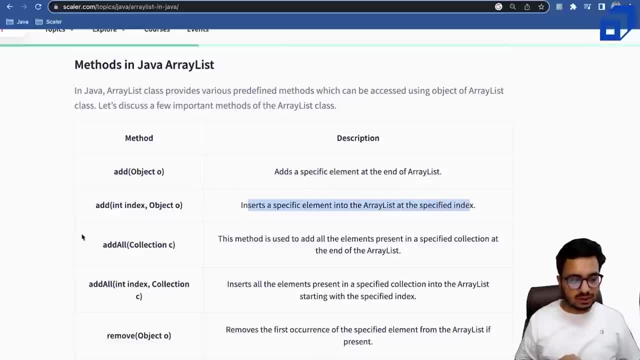 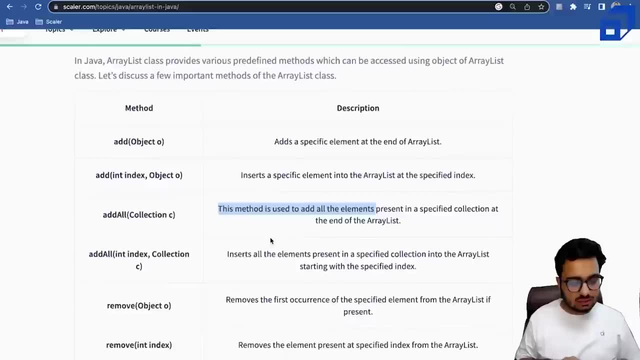 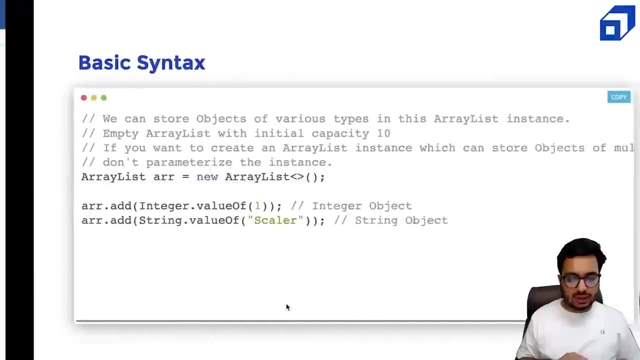 It will insert into a specific index of the list. There is a add all method. It will add another list, another collection into this list. So we can also add another collection at a particular index in this list. Let us look at the add methods first. 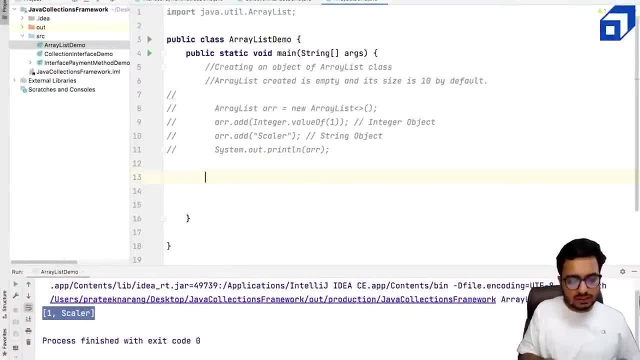 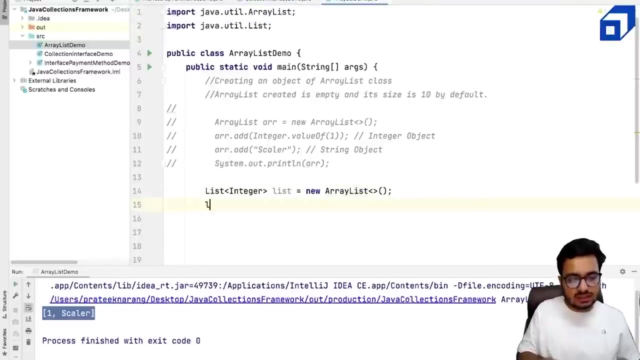 I can say I want to create an ArrayList, So list of its integers. I call it as list And this is equal to new ArrayList. You can see we have imported the list interface and we have imported the ArrayList class Inside this list. I need to add some numbers. 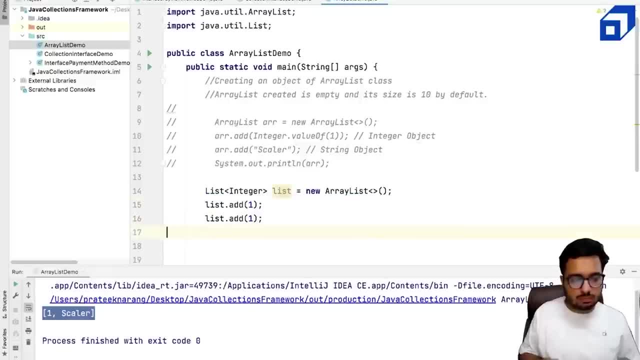 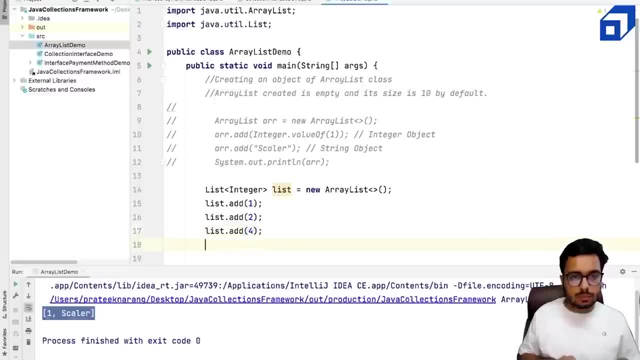 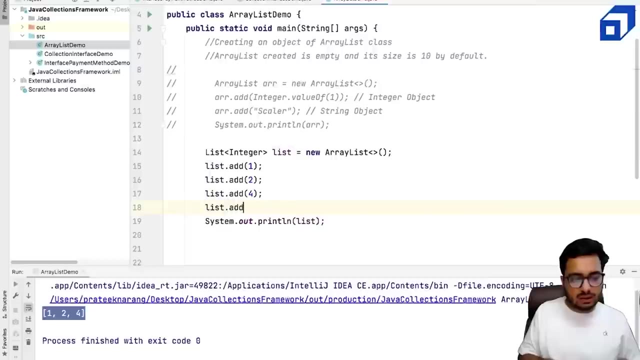 I can say add 1, add 2,, add 4. So let me show you And if I print this list I see I get 1 to 4.. I have added these numbers. Now, what I can do, I can add at a particular index as well. 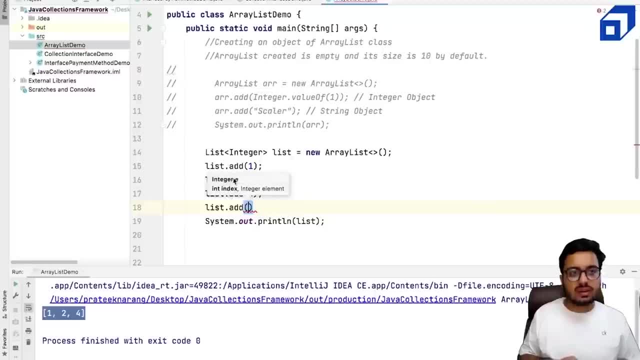 I can say I want to add at a certain index. So either I give an integer or I give an int followed by an integer. I can say: add at index 2.. The element is 15.. If I do it, it will do insertion in the middle of the. 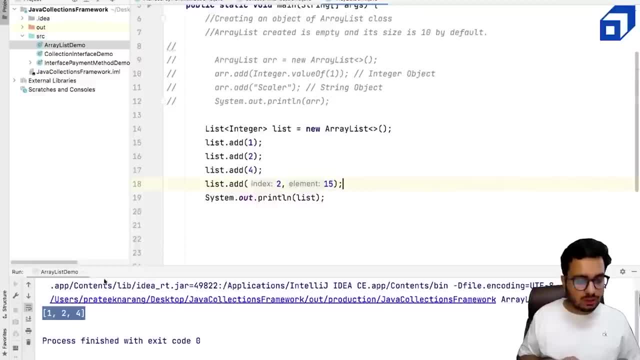 list. That is also possible. So you can see, I get 15, which is now present at index 2.. So by default it is like the first parameter is the index, The second parameter is the value that I am going to insert, That is, the add function. 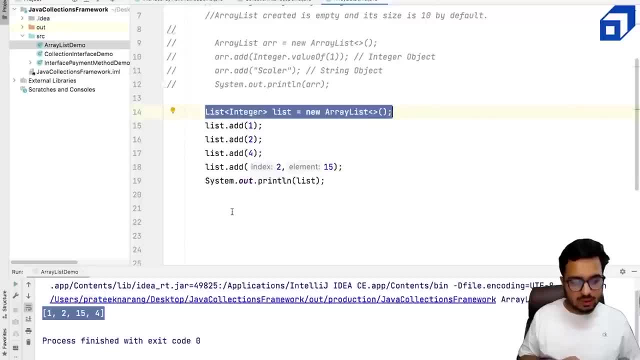 I can create another list as well. I can say, okay, I need another list, List 2.. And I can say list 2.add 15.. And I can, or let's say, this is 25.. I can also add all elements of list 1. 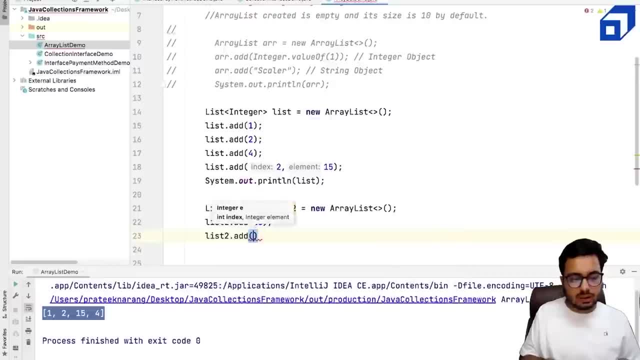 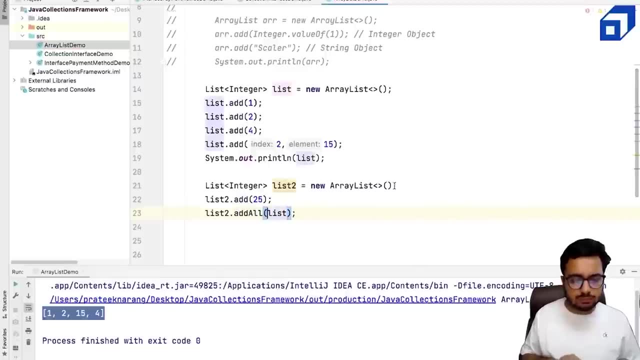 in list 2.. I can say list 2.add list, So I can pass another collection here, So add all. I need to call the add all method And this will also work, And I can print list 2 as well. 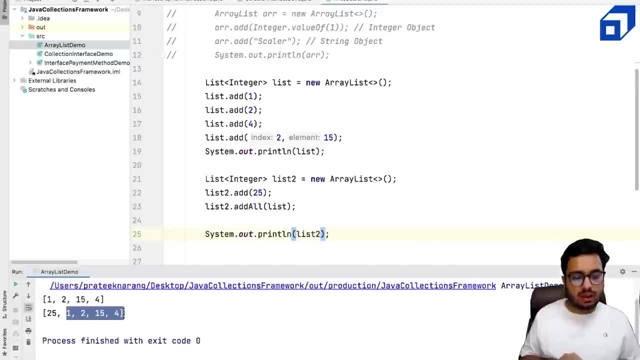 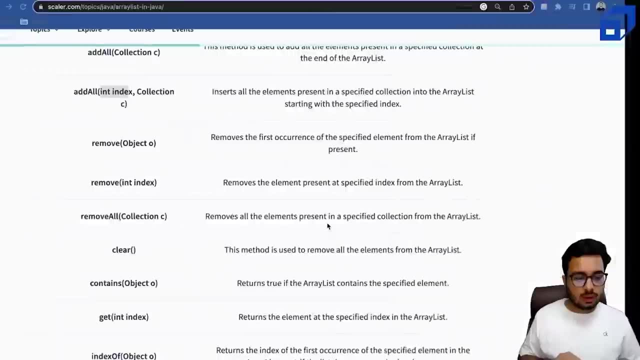 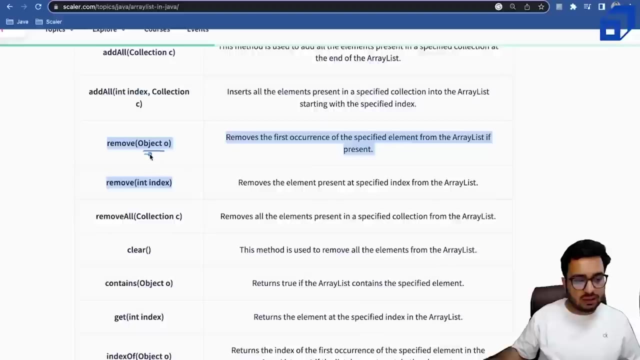 You can see I am having 25 here, followed by all elements of list 1.. That is how do we use the add method. Next we will look at, look at the remove method. So now remove method is actually a overloaded method. If you look at, we can pass. 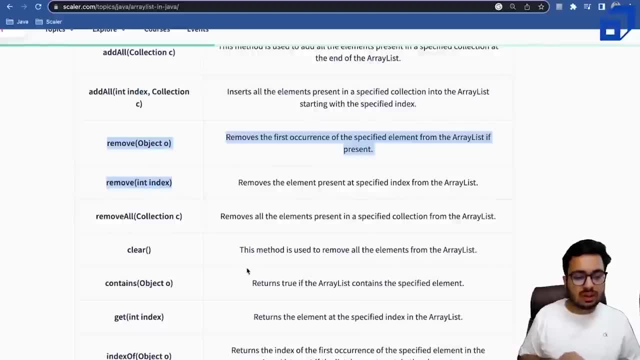 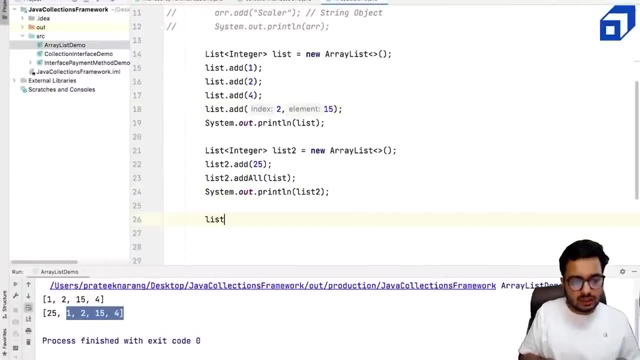 an object, We can also pass an index. Now this becomes tricky, especially if you are working with integers. If I say, okay, I want to remove something, I want to say list, 2., remove, 1. What does it mean? Am I removing the index or 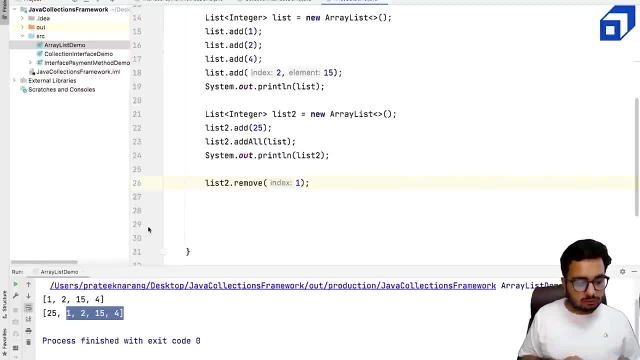 am I removing the value 1?? So, or let me just say list, remove 1.. If I talk about first list and I want to remove 1 from it, Let me show you it will actually remove the index, Because when you are passing, 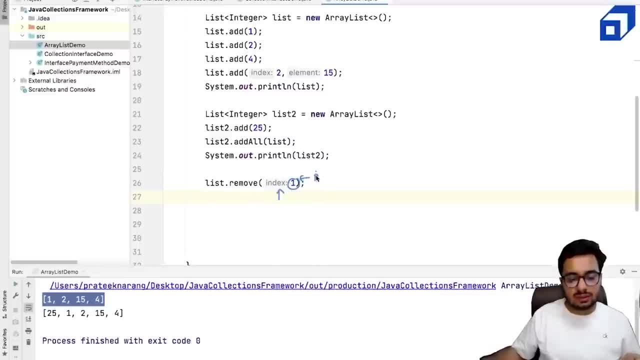 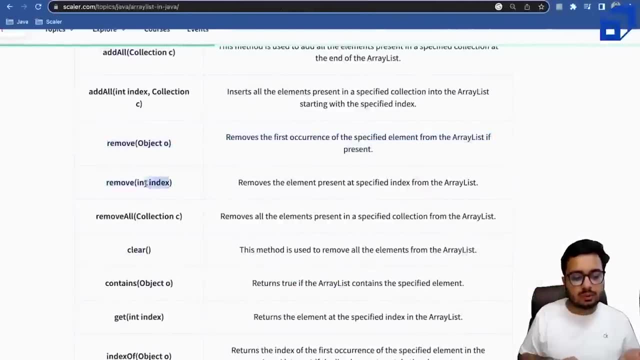 1. simply like this: it is going to assume it is of the data type int. So if you look here, So when I pass int data type it removes the index at the at the following index it will remove. That means it will remove the element. 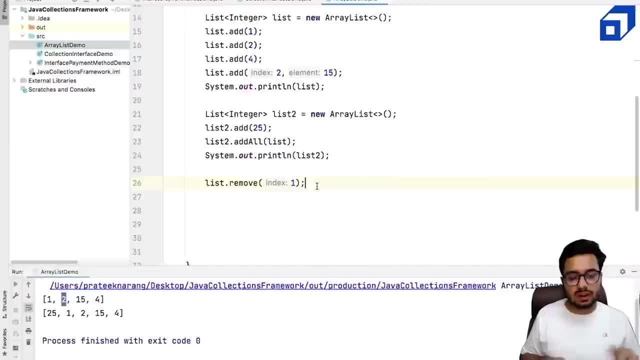 2 from list 1.. But if I want to remove the value that is 1, what will I have to do? I have to convert that into an integer object. So I have to say listremove integervalue of 1.. That means: 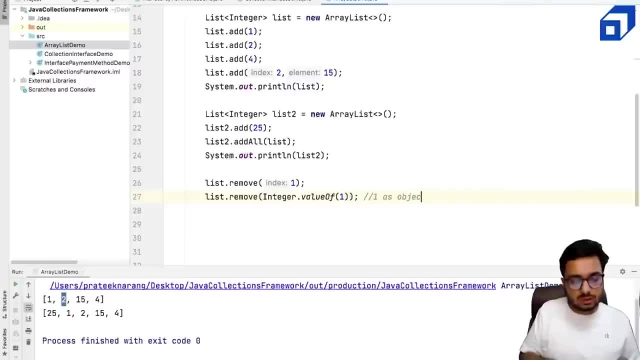 remove 1 as a object. So if I remove both, Let's say that means 1 and 2- both will get removed. Let me show you the output. I will print: system sout list. Show me what you are going to remove. Now you can see. 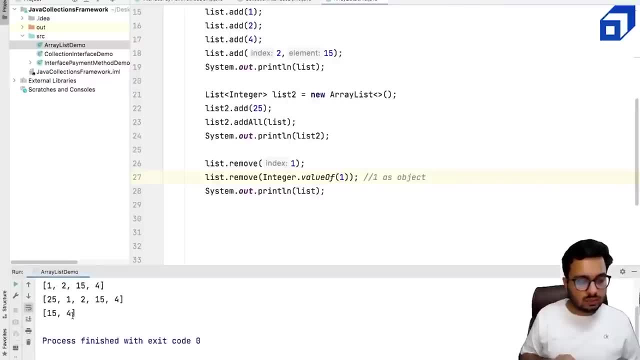 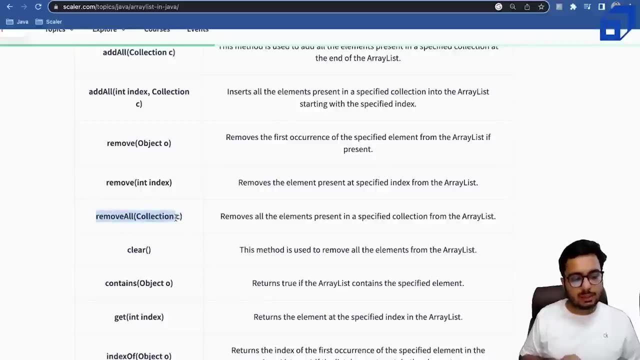 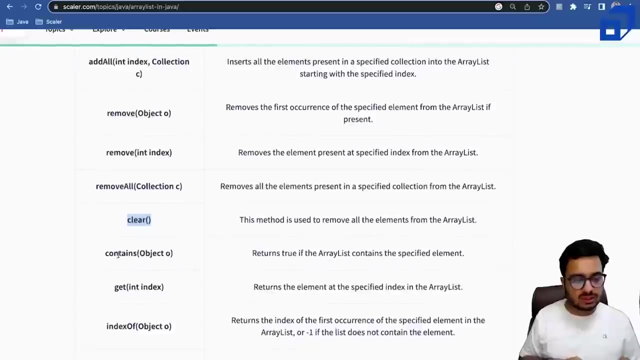 the output that both 1 and 2 they got removed and we got 15 and 4.. Similarly, you have a remove all method which will accept another collection. It will remove all elements from that collection. from the given collection. Clear will remove all elements from the list. 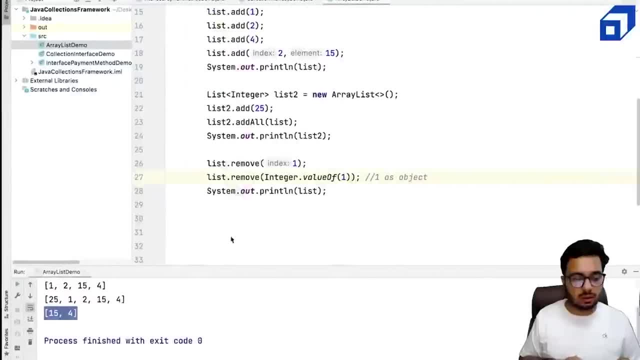 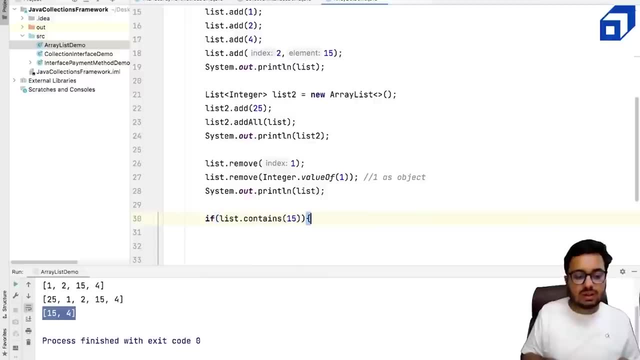 Contains will tell me whether a particular element is present or not, So I can check that. okay, if list contains 15, do something. Contains is your linear search, So sout. yes, 15 is present, Something like this, So you can use the contains method. 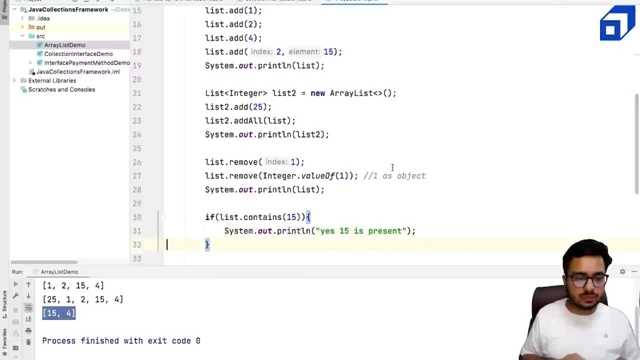 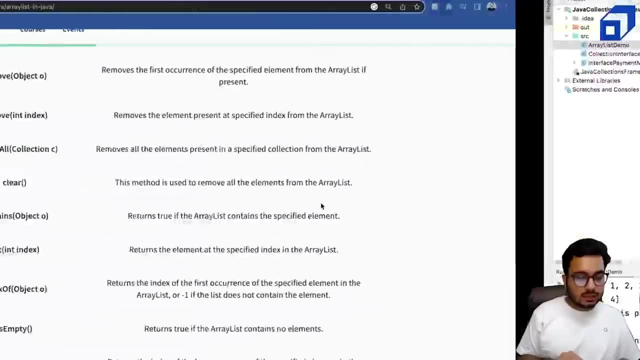 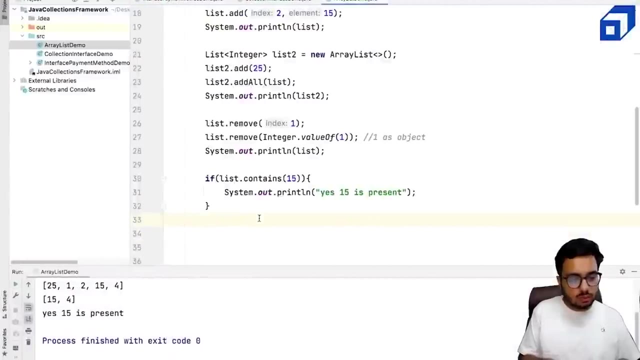 with almost every collection. Let me run this and you can see that we are getting. 15 is present. Okay, so there are more methods. there is a get method. So if you want to read a particular index, you want to say, okay, show me what is. 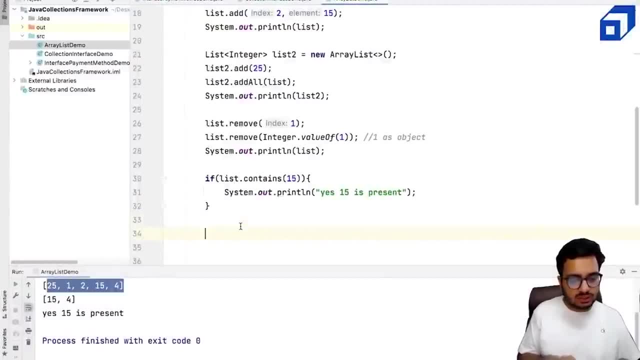 present at the 0th index. You can say sout or you can maybe you want to iterate over the entire array list. You can say for int i equal to 0, i less than list dot size or list to dot size, i plus plus I want to get. 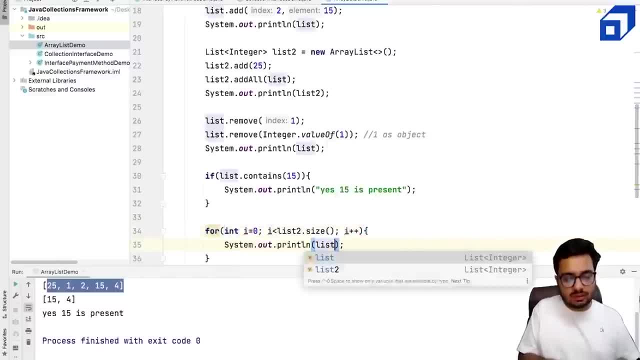 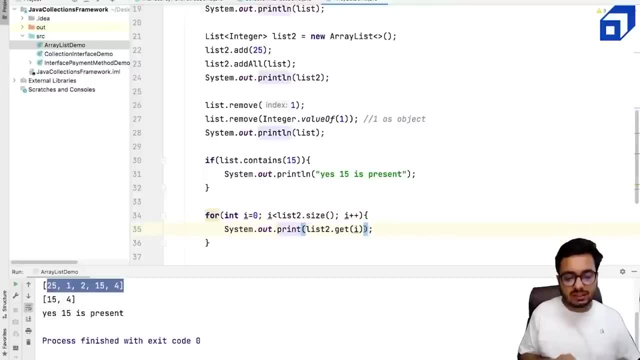 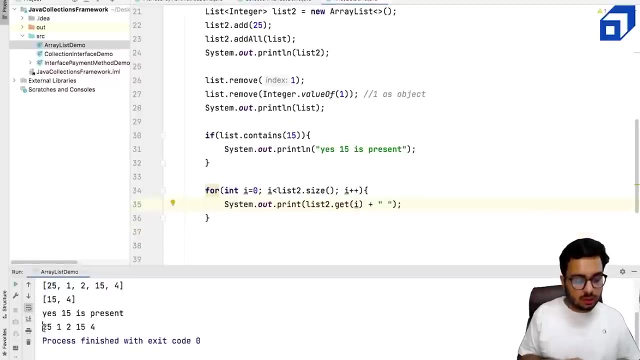 the elements at each index. You can say sout list to dot get i. This will give you the elements at given ith index. So get function is used to access the ith element. So let me run this and you can see we are able to iterate over all. 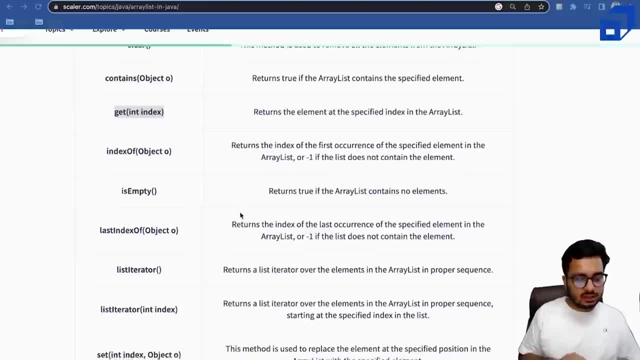 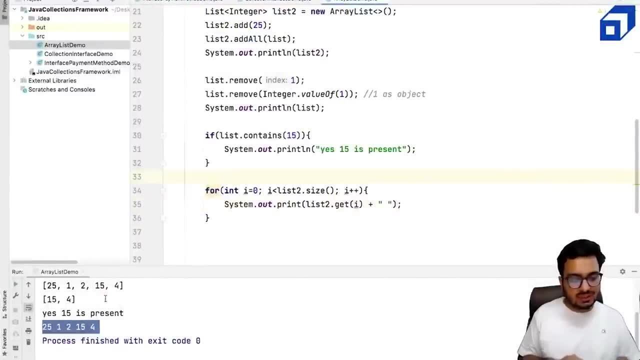 the elements in this list. So just like get. there is another method that is called set. So if you want to update a particular index, you want to say okay, I want to make this 0th element as 50. So you can say okay, list. 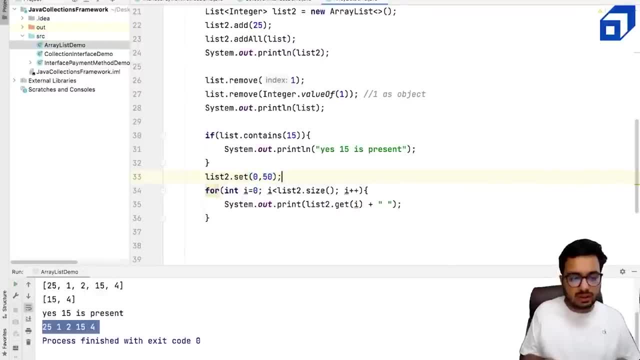 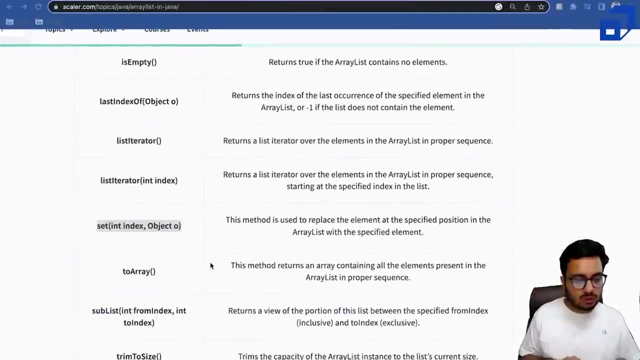 to dot set 0th element, make it 50. This will work and now your 0th element will be 50. You need to give the index and the object that you need to store here. This is the set function. There are more methods. I won't be able to cover all. 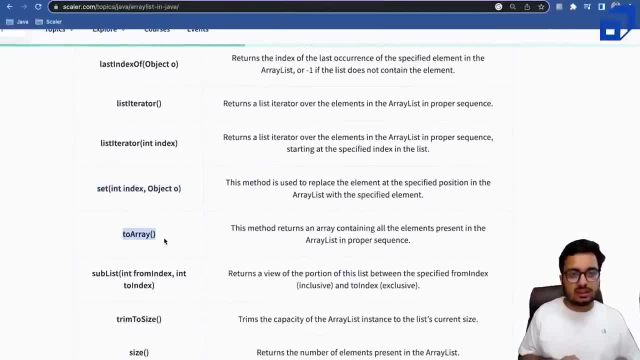 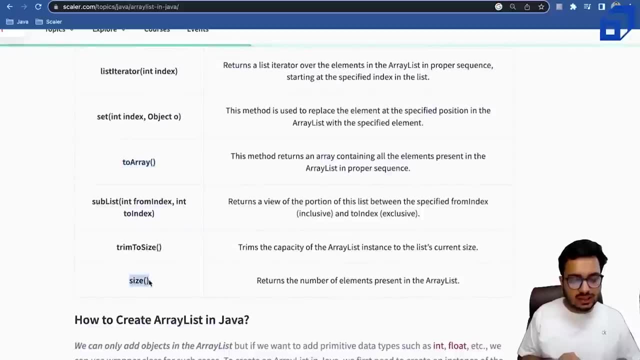 the methods, but we have covered most of the important methods. There is a method called toArray- If you want to get an array from an ArrayList, you can use this- and there is a method called as size, which we have just seen. There is also method called trimToSize. that means 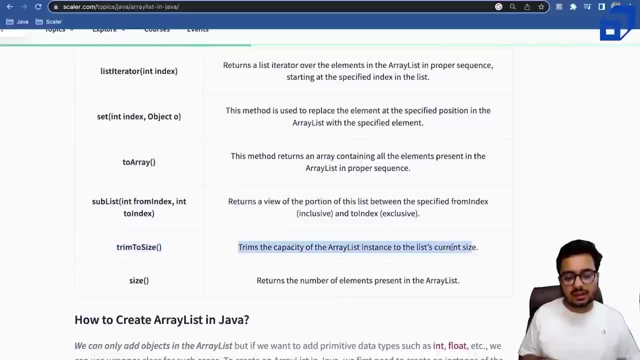 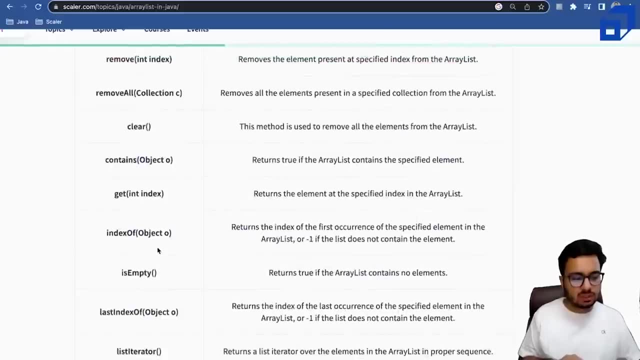 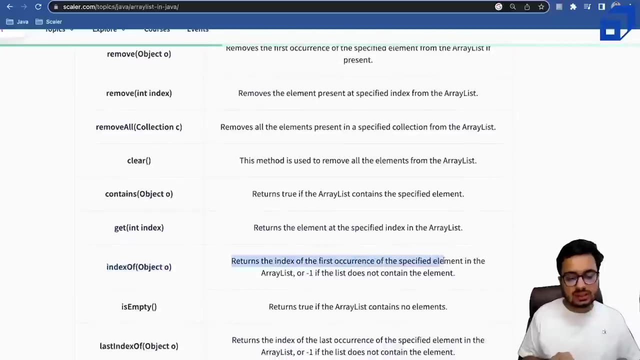 if we want to reduce the current size, like if we want to reduce the capacity to the current size, we can use this method: trimToSize. These are some of the important methods associated with ArrayList. There is also indexOf returns, the index of the first occurrence. 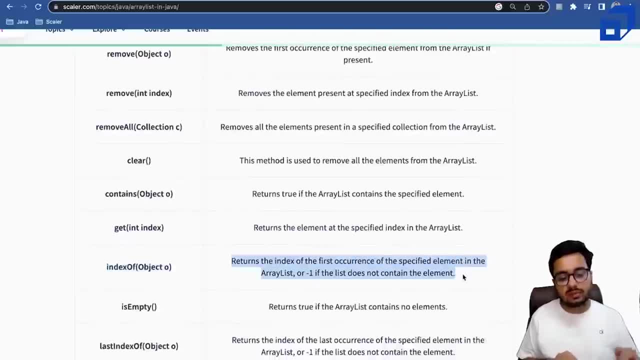 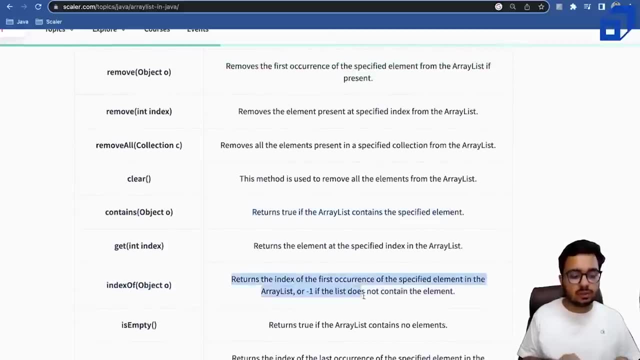 of the specified element in the ArrayList, or minus 1 if it does not contain the element. So contains: is going to give you Boolean present or not. IndexOf is going to give you at what index it is present or not. Now we will look at some more ways to. 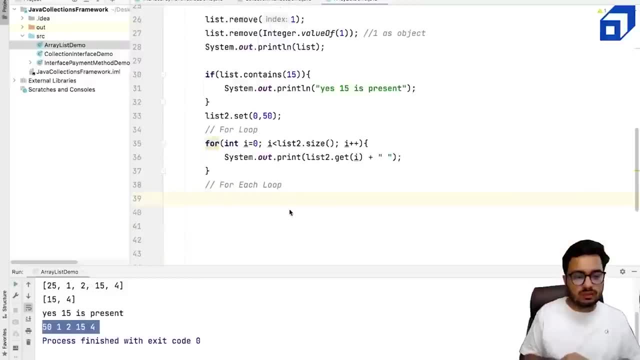 iterate on the ArrayList, Let's do a quick demo. We have seen for loop. We can also use a for each loop. So I can say: for every integer x in my list2, I want to access it and I want to print it. So I can say: 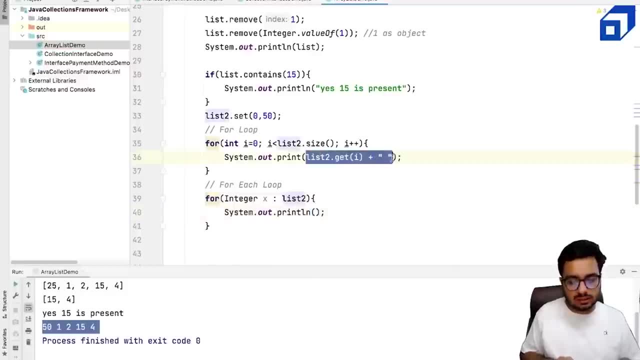 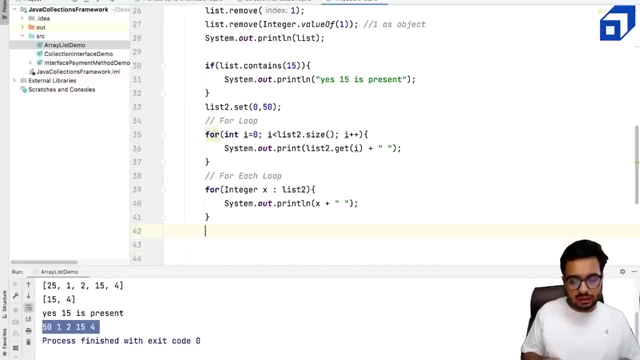 soutList2.getI. soutList2.getI. that is my another way of iterating and printing. Sorry, I will not do this. Let me print this number x. Let me run this code. There is one more way that I can also iterate on the list using an. 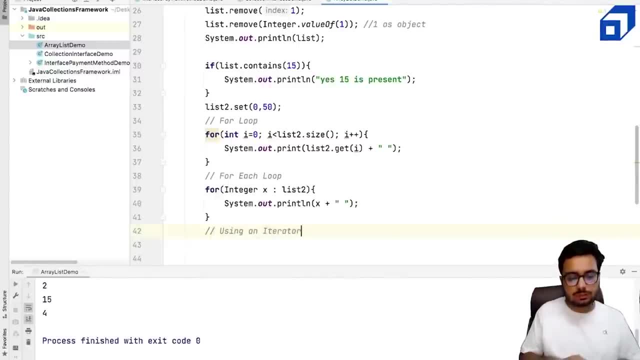 iterator. So you can see we are getting all the elements, That is, 1,, 2,, 15,, 4, and 50 is also there. So we are starting from 50 here We are getting all these elements. So iterator. 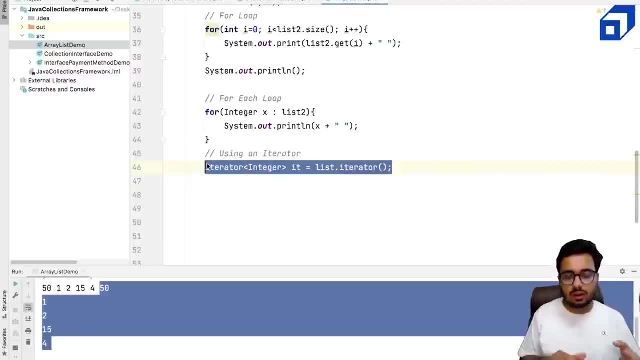 is one more way to traverse on a java collection, All java collections. they support iterators. So what you can do, You can create a iterator object by calling list dot iterator. This iterator has a method called as hasNext, which tells me whether I can access the next element. 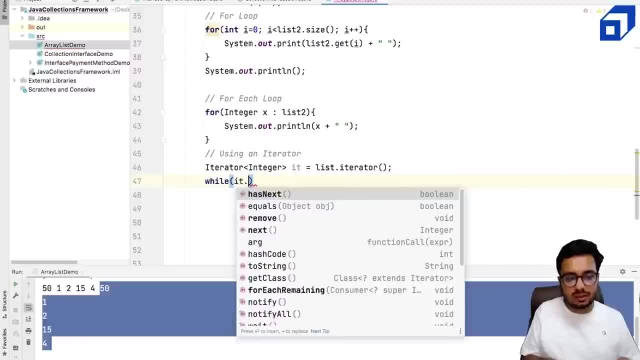 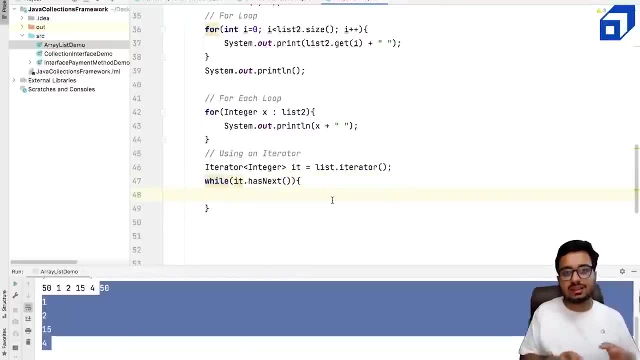 in the collection or not. If your collection has finished, your hasNext will give you. there is no other element, So I can say: while ithasNext, if there is an element present, I can access it. So I can say: sout itnext. This will give me the next element in the 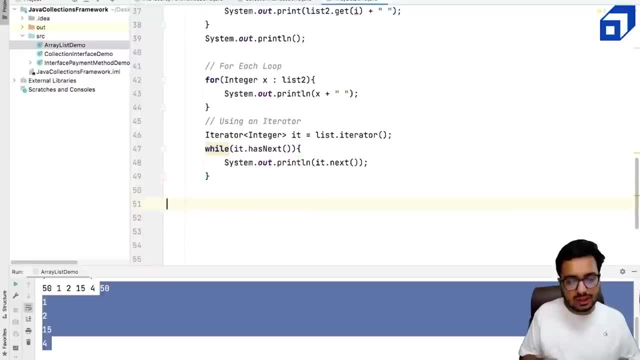 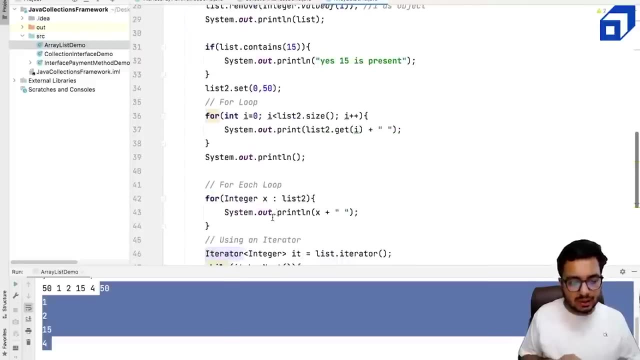 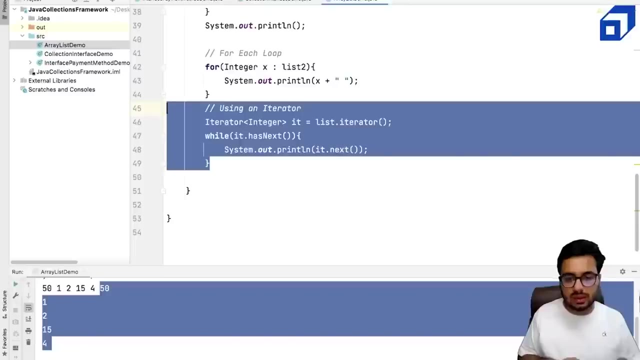 collection. This is another way using which I can iterate on given collection. So iterator is coming from the javautil package only, So this will also print all the elements present in this list. Let us quickly run the code and see We are getting the. 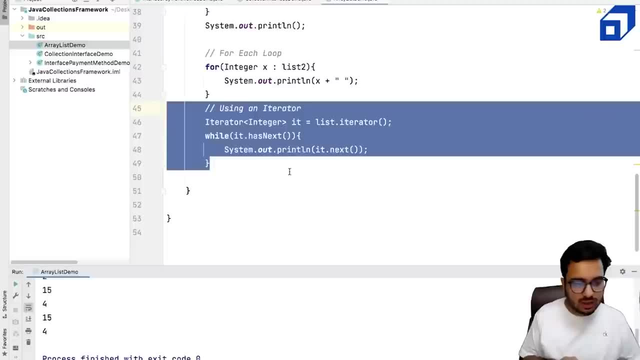 same output using iterator as well. So I iterated on list 1, which is 15, and 4.. Again, I iterated using iterator, which is 15 comma 4.. That is what I am getting by iterating on my list. That's all for. 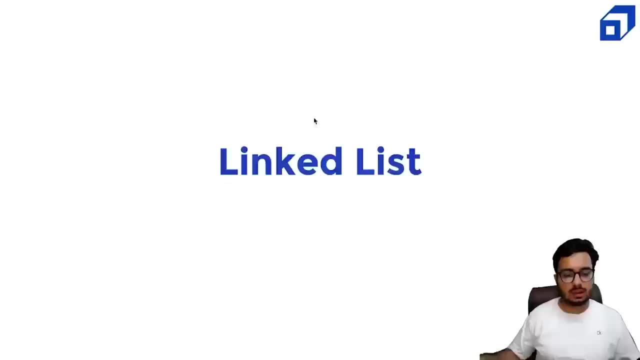 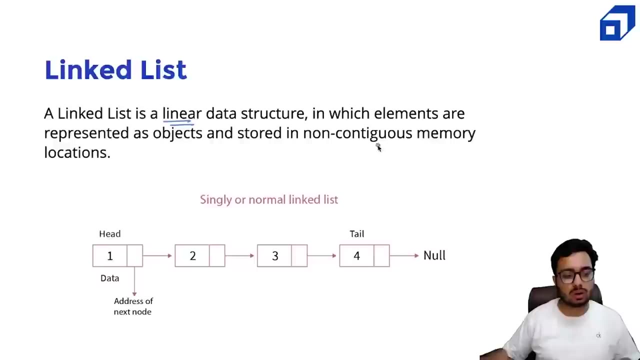 ArrayList. I hope you understood the methods of ArrayList and how it works. Now let us jump into LinkList. So LinkList is also a linear data structure in which elements are represented as objects stored in non-continuous memory. For example, if this is your heap memory, 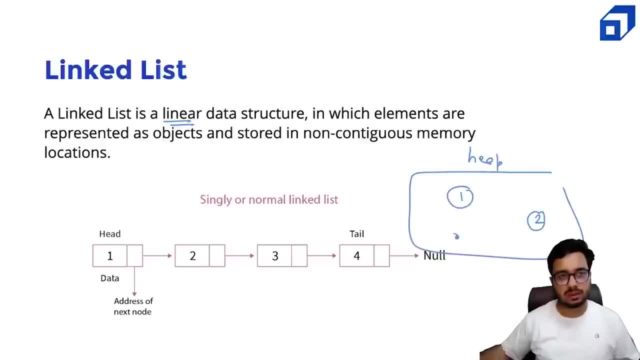 and you have some data. maybe 1 is stored here, 2 is stored here, 3 is stored here, 4 is stored here. They might form a chain like structure, and where each object is referring to, the is holding the address of the next object in the. 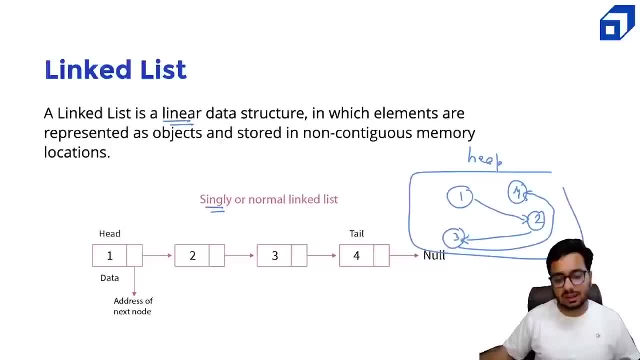 chain. This is called as a singly LinkList, where each object knows the address of the next node but it does not know anything about the previous node. So if you arrive at 3, you can only go to 4.. If you arrive at 4, you can only 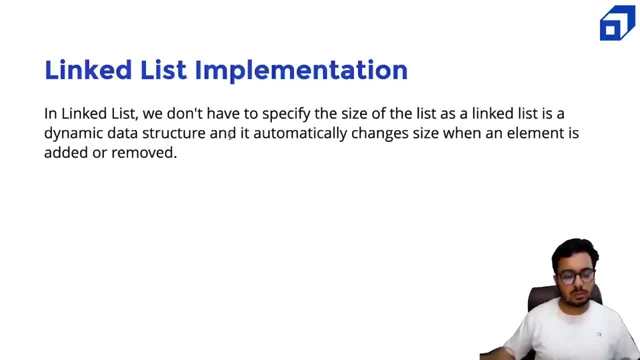 go in the forward direction. Let us talk about LinkList little more. So we don't have to specify the size of the LinkList. It's a dynamic data structure. As you add more data, more objects get created in the memory and they become part of the chain. 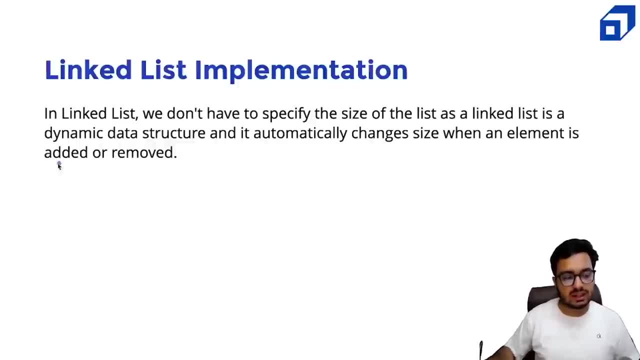 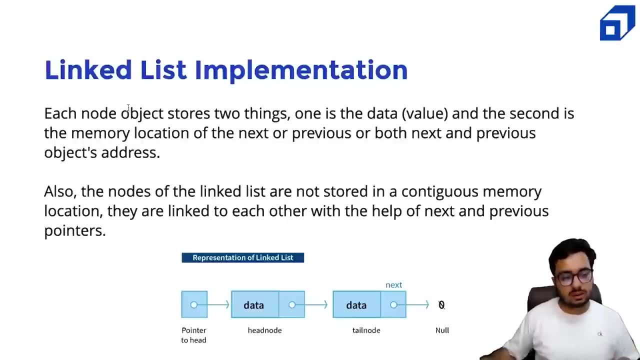 And size is changing automatically as the data is added or removed, So you don't need any fixed size array to initialize it. Now let's talk about the implementation, As I just talked about each node in a LinkList. it's going to hold data. It is also going to hold 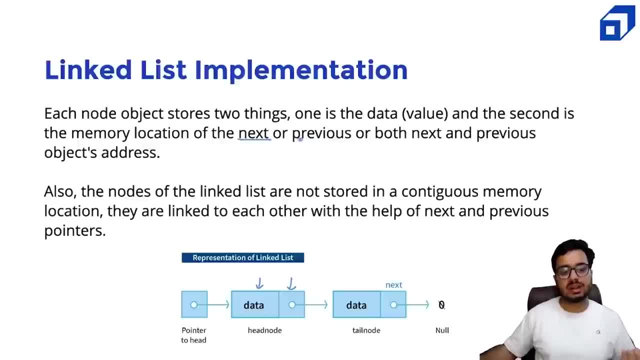 the address of the next node And if it is a doubly LinkList, it is also going to hold the address of the previous node. Nodes are not stored in a continuous memory location. They are linked to each other with the help of next and previous pointers. 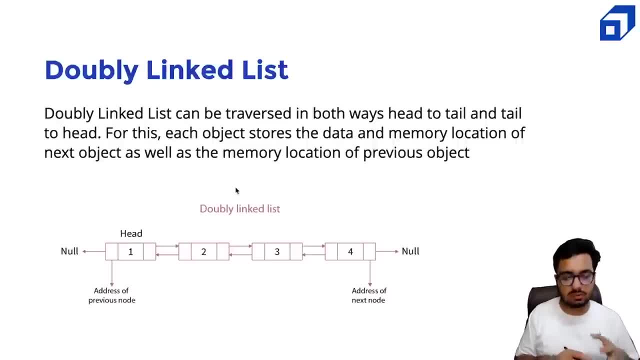 So this is something we will go into detail when we talk about, when we do a tutorial on LinkList, But for now we just want to see how to use the inbuilt LinkList class and understand its advantages and when to use it. So in Java, the default. 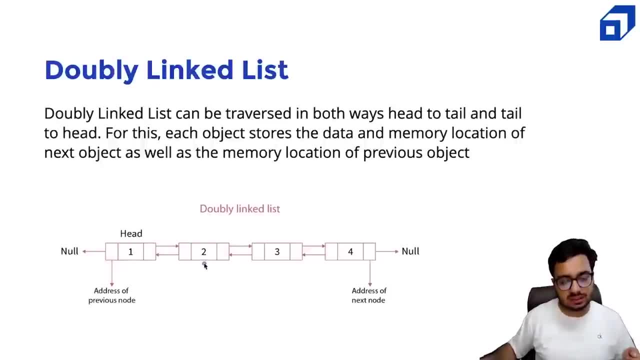 implementation provides us with a doubly LinkList. So a doubly LinkList. each node stores three things: The object or the data, the next node's address and the previous node's address. So at 2 you know where is the next node located. and 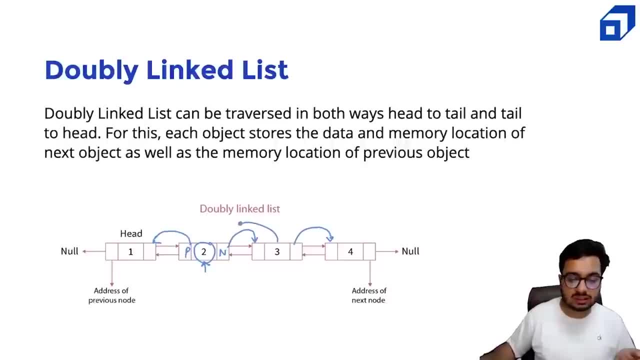 where is the previous node located. At 3, you know where is the next node located and where is the previous node located. So you know all the three things at each node inside a LinkList. That is what a doubly LinkList is, And creating a doubly LinkList is fairly. 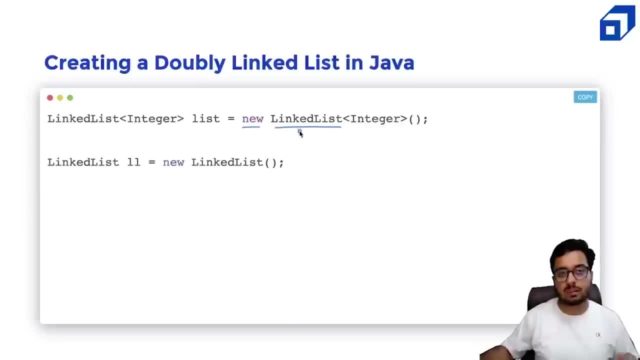 simple, So you just need to use the LinkList class provided by the javautil package and the data type- What kind of data you want to store in this LinkList- and it will create a LinkList for you. Now let's talk about the features of. 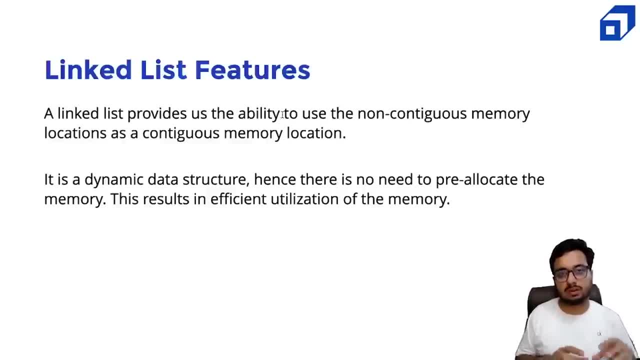 the LinkList. The biggest feature is we can use the non-continuous memory. So if you don't have a linear block available, we can still create a big chain by utilizing the non-continuous blocks of the memory. It is a dynamic data structure. 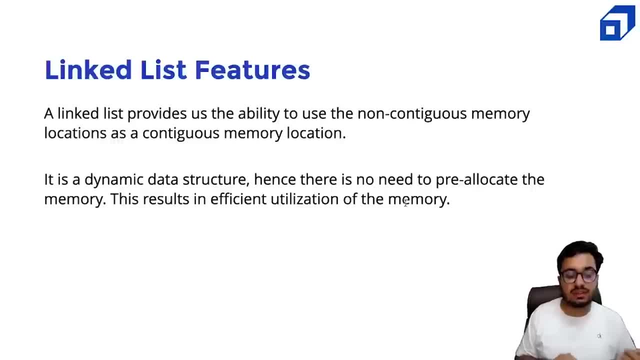 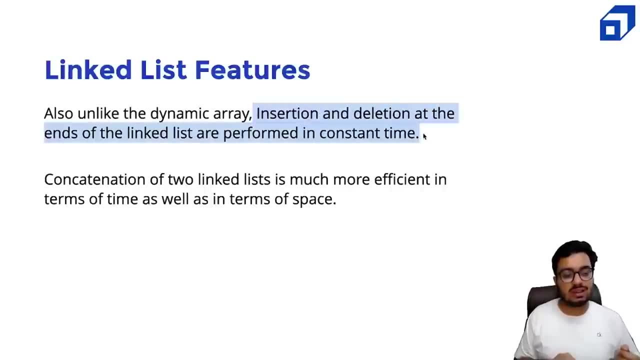 there is no need to pre-allocate the memory, and hence it results in efficient utilization of the memory as well, And insertion and deletion at the ends of the LinkList are performed in constant time. Now, this is a very big advantage. So if you have an array and you want, 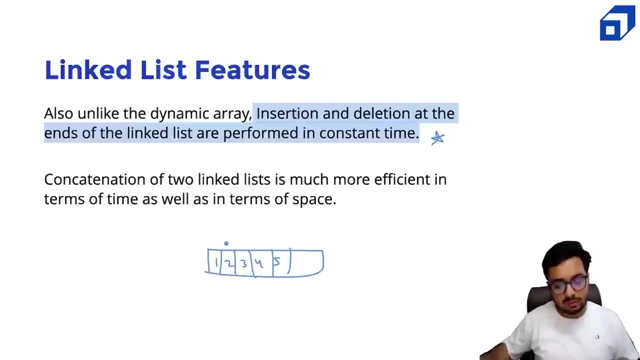 to insert something at the beginning, you would see that I will have to shift the entire array. then I can insert a zero here. But in case of a LinkList, this time which is order n in an array inserting at the beginning, It's going to be: 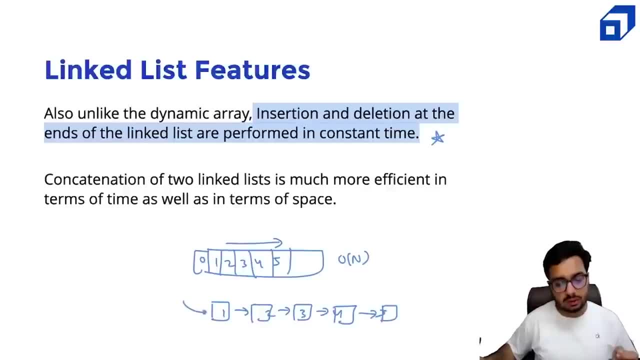 very fast. Suppose you have 1,2,3,4,5, you already know this node and you say I want to insert a zero here. So you create a new node and you say head should point here and zero should point here. This 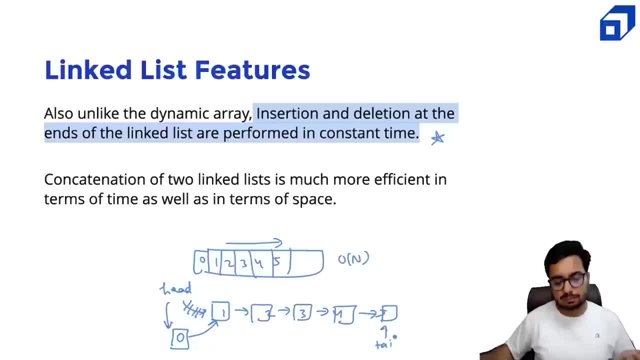 can be done in order one time. Similarly, the last node is referred by a tail pointer. If you want to create something at tail, you can simply add six here and your tail will move here. So if it is a doubly LinkList, insertion and deletion both. 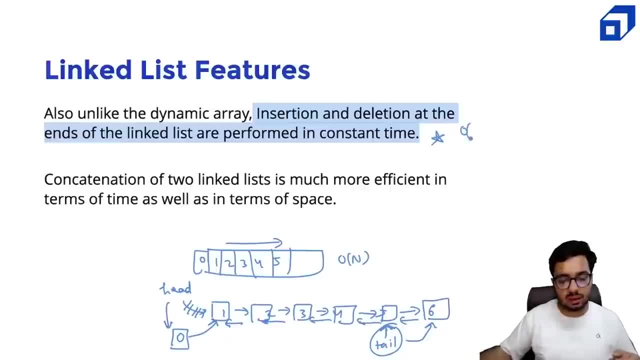 at the both ends can be just done in order one time. This is a very, very big advantage of LinkList and concatenation of two LinkList is much more efficient in terms of space and time. So if you want to merge two array lists, you will have to copy. 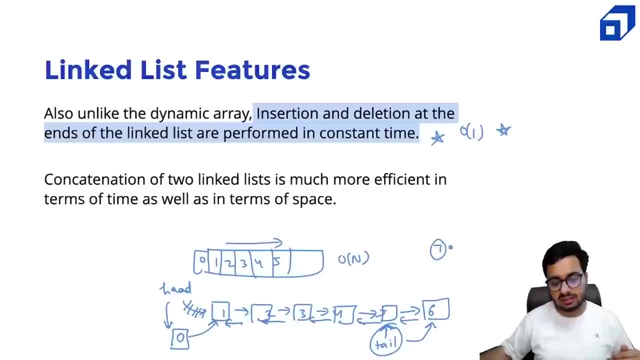 all the data. But if you want to merge two lists- let's say I have another list- seven, eight and nine- In that case merging is also very easy. You just need to connect this node with this one, which is again going to take order one time. 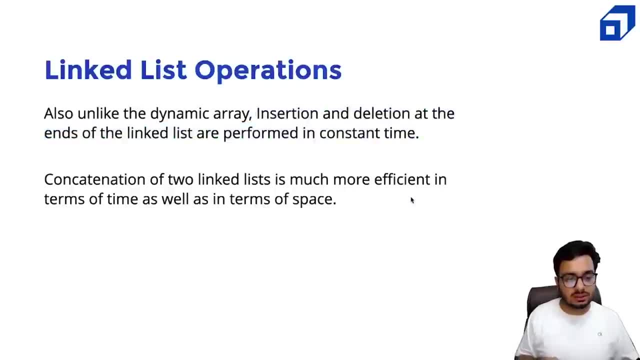 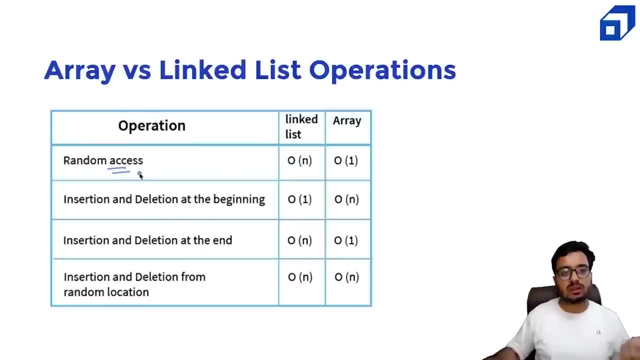 Concatenation is also very fast in case of a LinkList. So let's talk about the differences between the operations. So random access that means if I want to get any ith element, This is very fast in array So I know I can get. 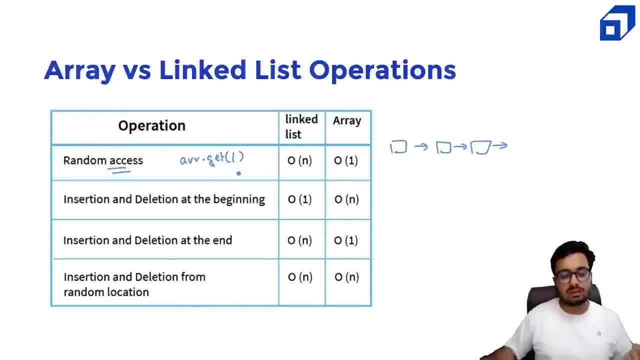 I can do arraygetI. This works in order one. But if you want to get some ith element inside a LinkList, there is no direct way. You have to iterate it. It's in the worst case. it will be order of n Insertion. 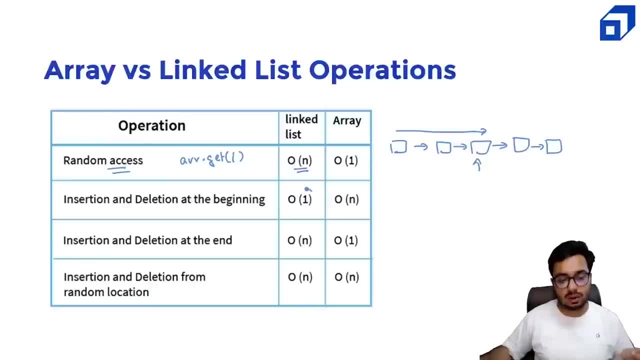 and deletion at the beginning. In case of LinkList, as I told you, it's order one. In an array, it's going to be order n because you have to do the shifting, Insertion and deletion at the end. So if it is a, 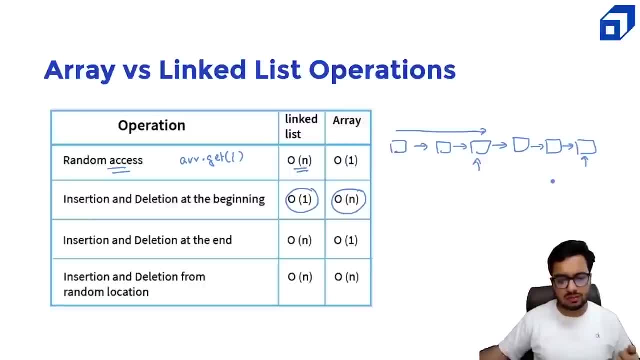 doubly LinkList and we are maintaining the tail pointer. You can do it in order one time as well, And in array it is also order one, So this can be made order one. It depends upon the implementation: Insertion and deletion from the random. 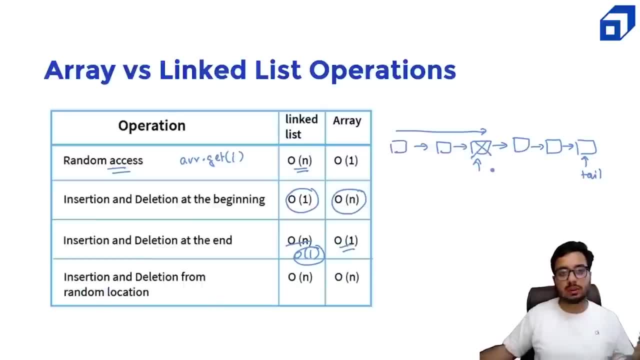 location. So of course, this deleting something from the middle, both in array and a LinkList, will take order of n time. So I hope you understood the basics of a LinkList. Now let's look at the implementation. So I have this code in which we said we are creating a list. 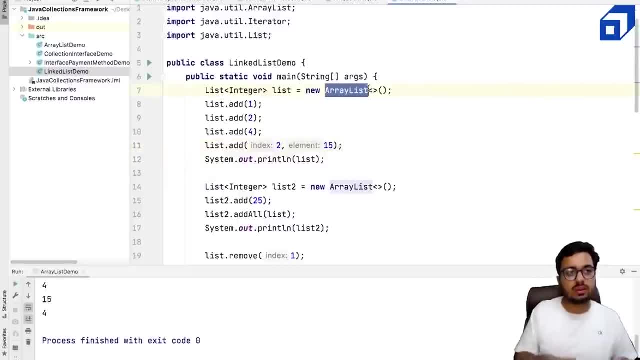 which is using a new ArrayList object. So instead of now using ArrayList, I can simply replace it with LinkList, And since both ArrayList and LinkList implement the list interface- So all the methods that we saw with this list- they will also work with LinkList. 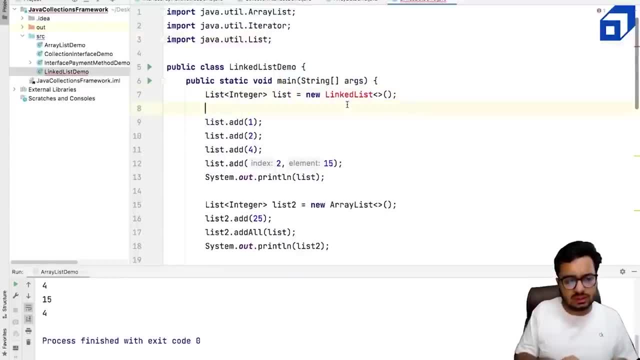 as well. If I need to import this class, let me just type LinkList and this will get imported. So import javautilLinkList. So this is also there. If I run this code, as it is the same ArrayList code, it will work. All the methods that we used. 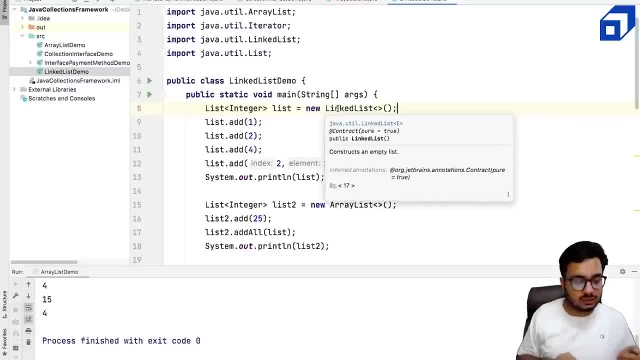 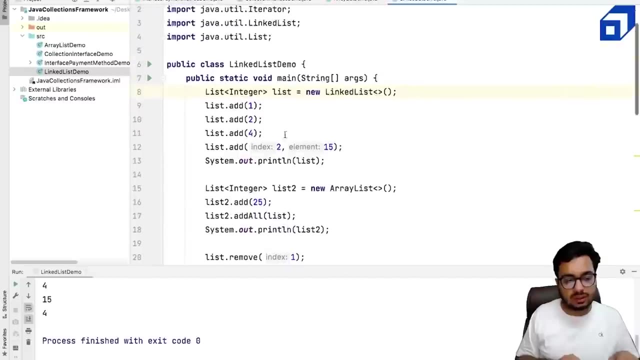 on ArrayList will also work on LinkList as well. Now, apart from it, there are some additional methods as well which are provided by LinkList, For example, adding something at the beginning of the list. So that method is not there in ArrayList, We can use that method. 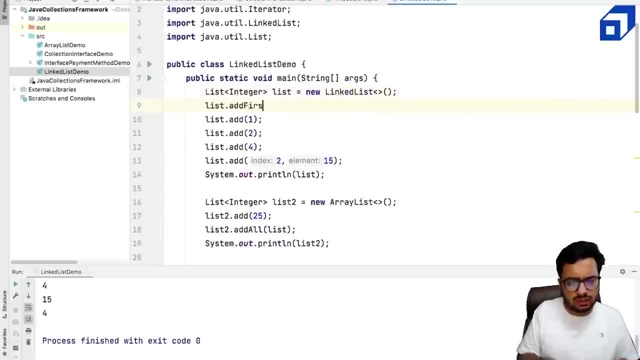 For example, I can say listadd first. I can say in the beginning: you add an element that is 0.. You might be saying we are getting an error here. At first, there is nothing like this. Now why we are getting this error? because add first is not a method. 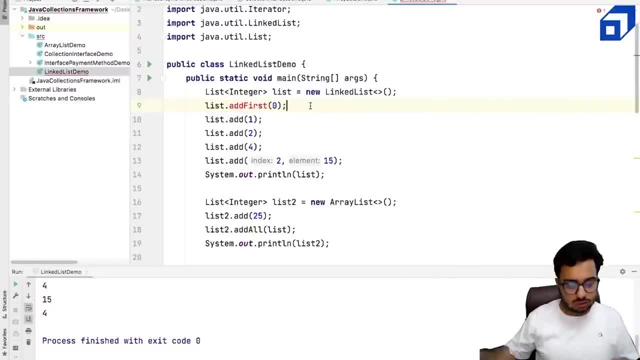 inside the list. So what happens is your list says that you must implement an add method, Whereas your LinkList class, which implements your list interface, it says: I will implement the add method, I will also implement the add first method. That means you cannot call. 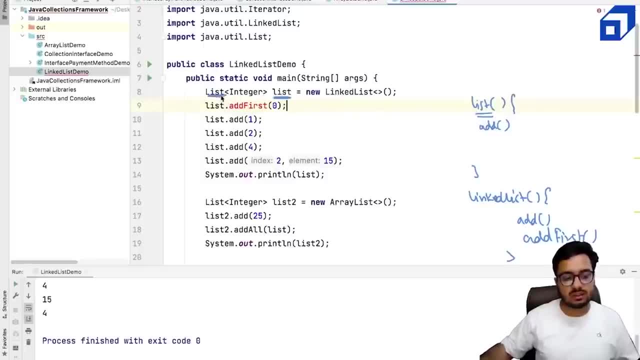 add first method on a list kind of a variable. It is of the type list. What I need to do is the object that I am now creating is exactly a LinkList. If I make it LinkList, you can see add first will work because you can easily add. 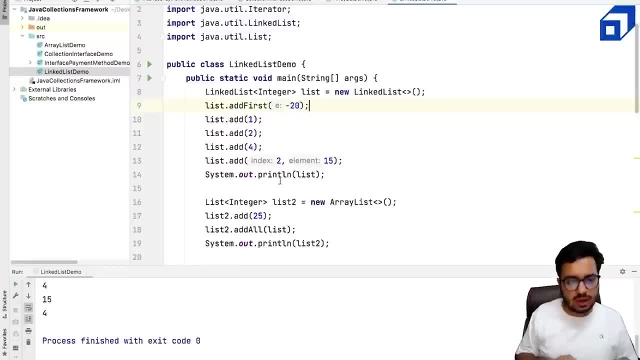 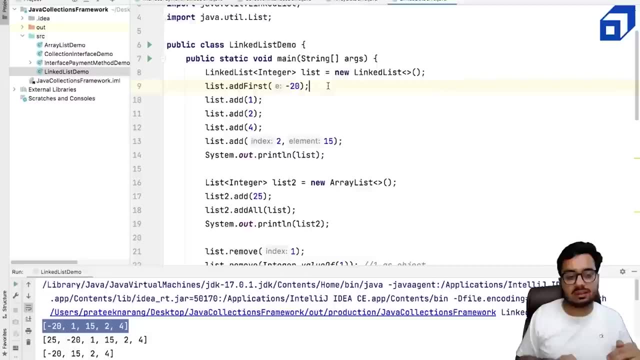 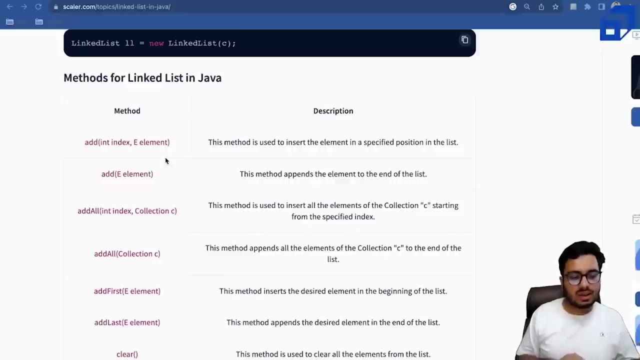 in the beginning of a LinkList. I can say, maybe add minus 20 here and show me this list. It is added in the beginning of the list. We have more methods. Let's look at some more methods. Just to save time, I will quickly. 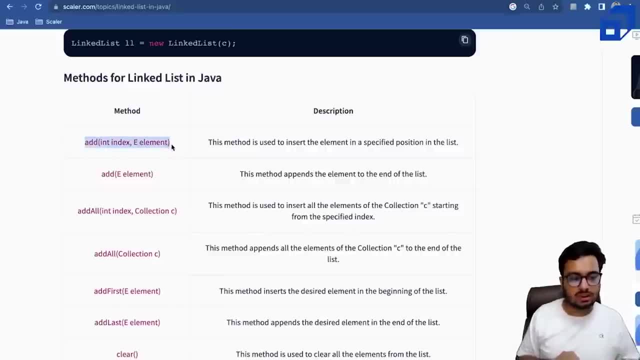 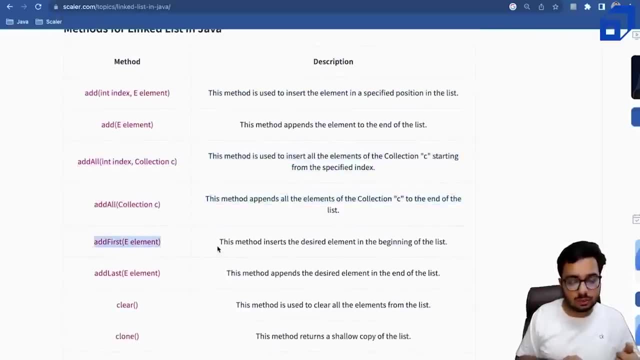 go through all of these methods. There is an add method which we saw on the list. This is also there. Add all is also there. Add first. I just showed you the demo. It adds the desired element in the beginning of the list. Similarly, 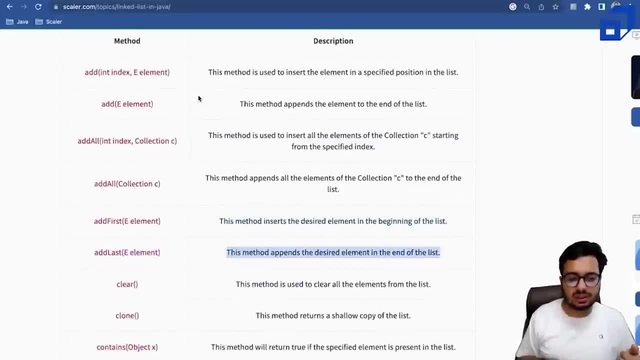 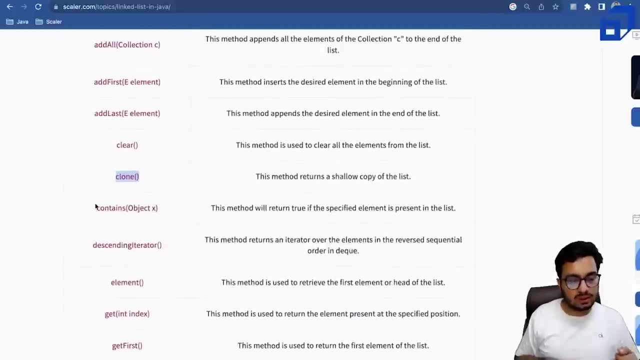 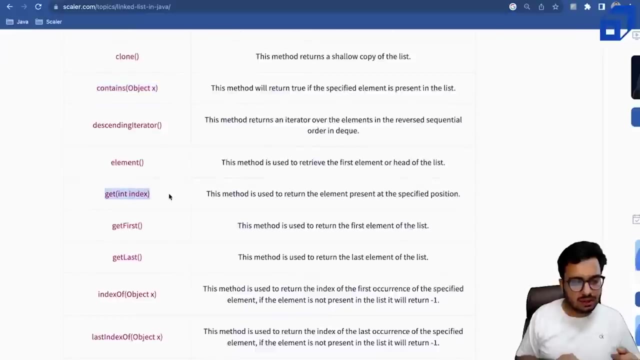 there is an add last method, It will add at the end of the list. There is a clear method which is fine. There is a clone method which creates a shallow copy. There is a contains method element present or not, Then popular methods are get. 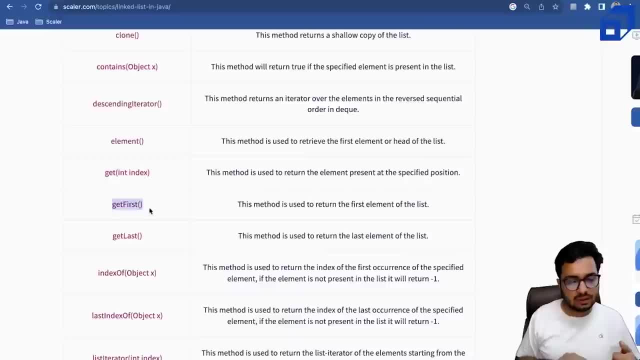 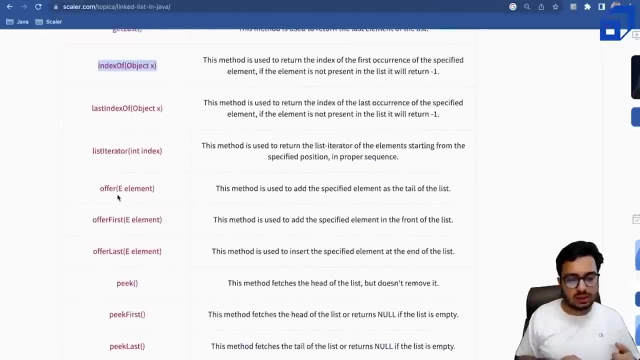 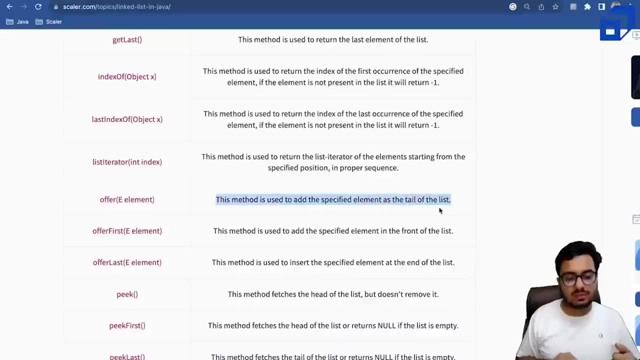 I want to get particular element. It works in a linear time: Get first, get the first element, Get last, get the last element. Index of you can use Now. there is also a method called as offer. This method is used to add at a specified element. 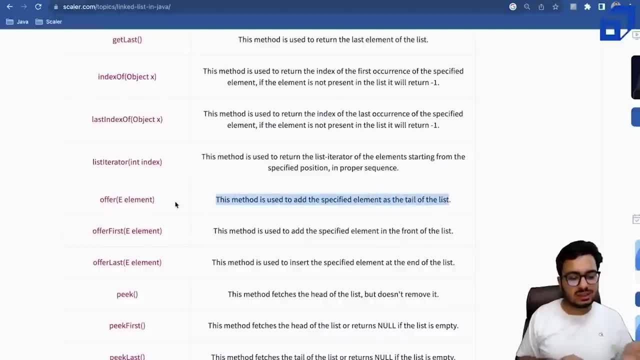 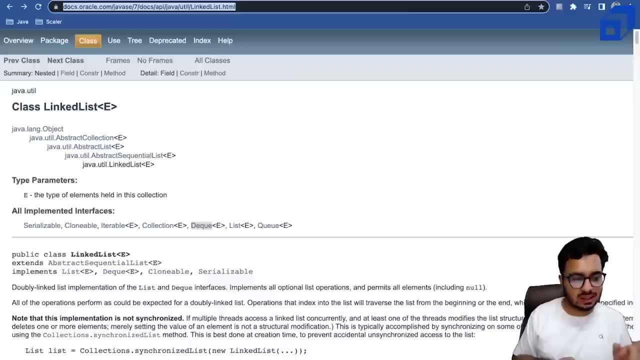 at the tail of the list. Now you might be asking: what is the difference between add versus offer? Let us discuss this as well. For that you need to go to the Java link list, class Java link list, the oracle docs. If I look here, 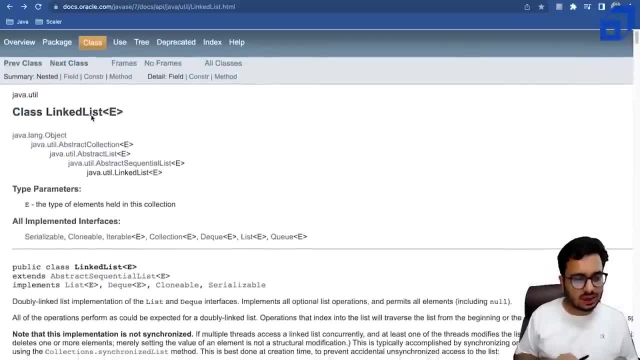 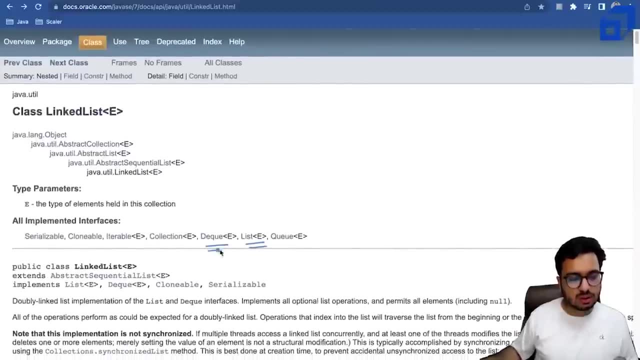 what is happening? the link list class. it actually implements not just your list interface, it also implements your tech interface. It also implements your queue interface. That means all the methods of the queue, all the methods of deck. they should be available as a part of link list. So what is deck? 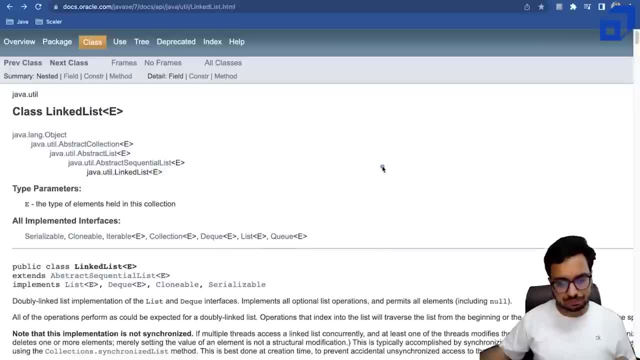 Deck is a doubly ended queue. That means you can do push and pop. That means you can add from the rear end, remove from the rear end. and you can also do push and pop. That means you can add from the front side and also remove from the. 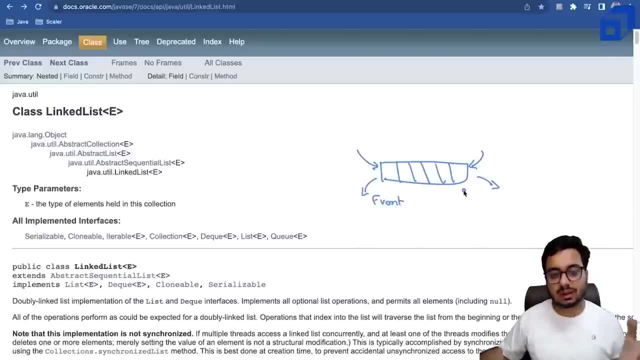 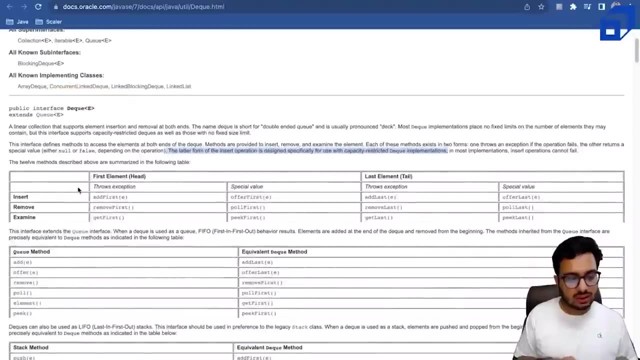 front side of the queue. That means in such a case you can do push and pop Now in order to implement this deck interface or the queue interface. let us look at what all methods are there in the deck interface. Inside the deck interface. you see there are methods. 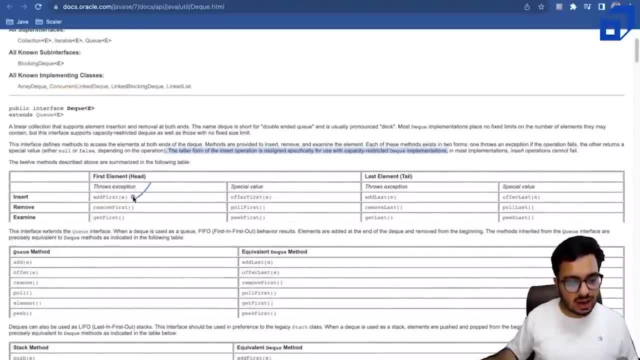 you want to insert something, at the beginning there is a add first method that should be implemented by that class. You want to remove something: remove first should be there. You want to get something: get first should be there. Similarly for the last element: add last, remove last and get last. 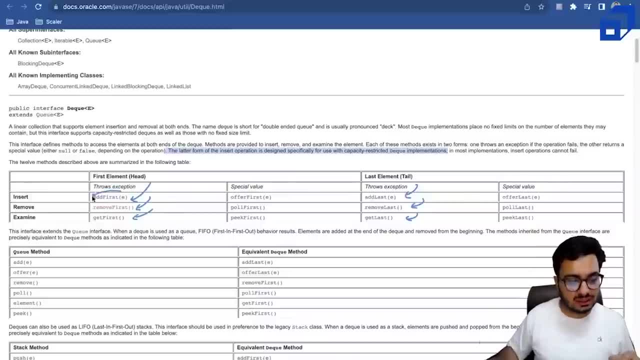 should be there. Now. there are two versions of the same method. One is add first, one is offer first. What is the difference between add first and offer first? The difference is written here. So what they are saying is that both methods are provided to insert, remove and examine. 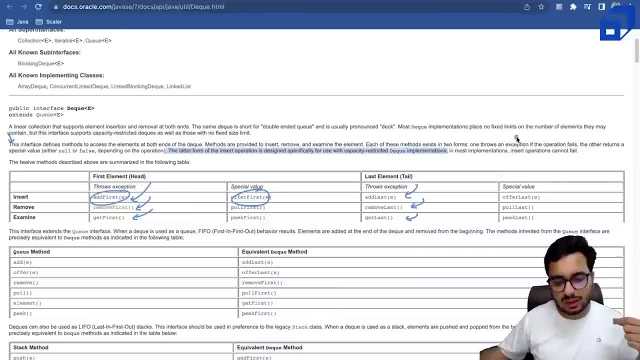 the element. Each of these methods exist in two forms. One throws an exception if the operation fails. The other returns a special value, Basically your offer method. it returns like true or false or null if your operation fails, Whereas add first will throw an exception. 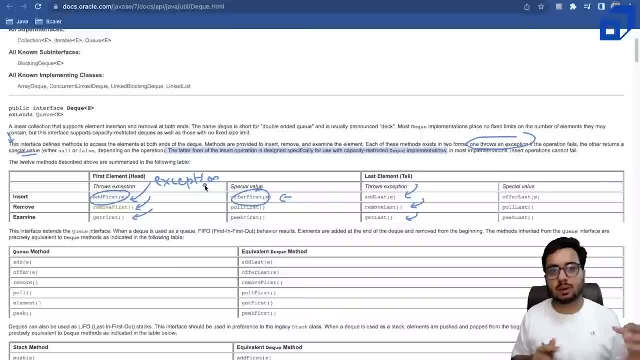 So it again depends upon your use case How you want to use this method. If you are working in an environment where your capacity of the data structure is restricted and you are trying to insert something and your data structure is already full, What do you want? Should it return false? 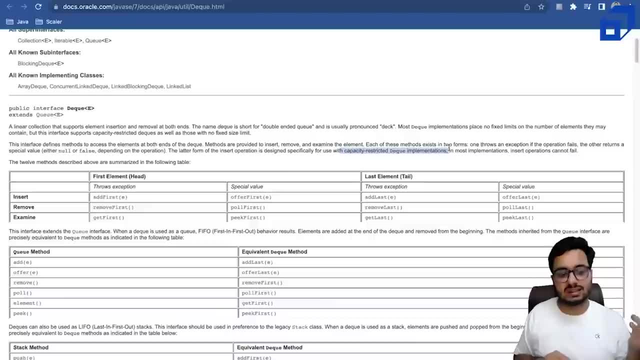 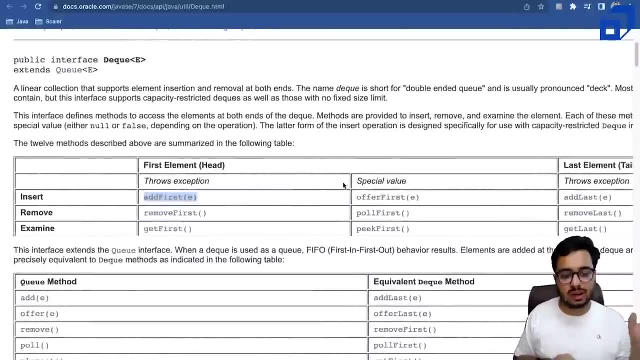 that I cannot execute this operation, or should it throw an exception? If you want to throw an exception, go with the add first method. If you want to handle it using a value like true, false or null, you will have to go with the offer first method. 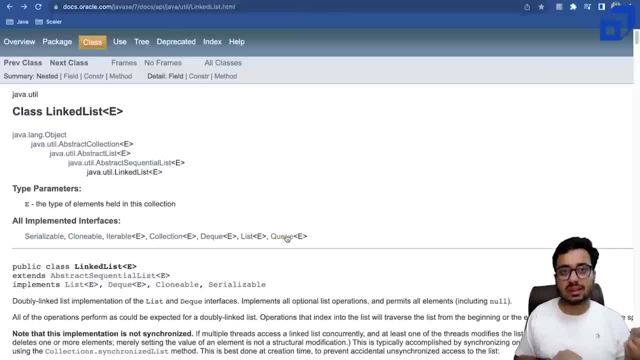 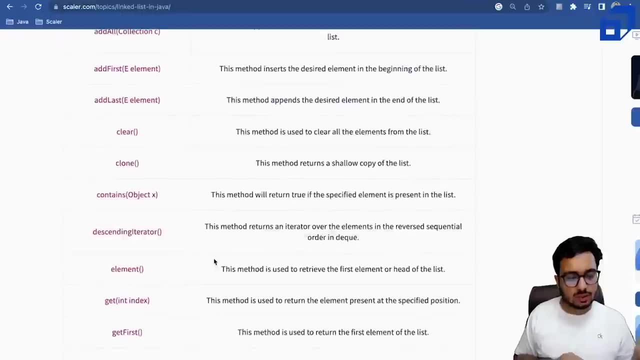 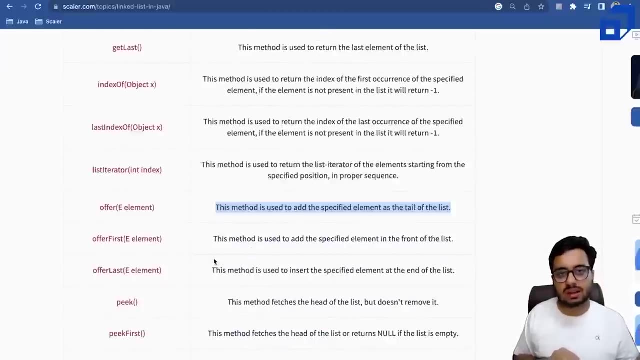 Because linkless implements the queue and the deck interface, which needs these methods. Hence, you will see there are many methods which are doing almost same work. Between add and offer, there is a difference of the return type. Should you not the return type? but how do you handle the failure case? 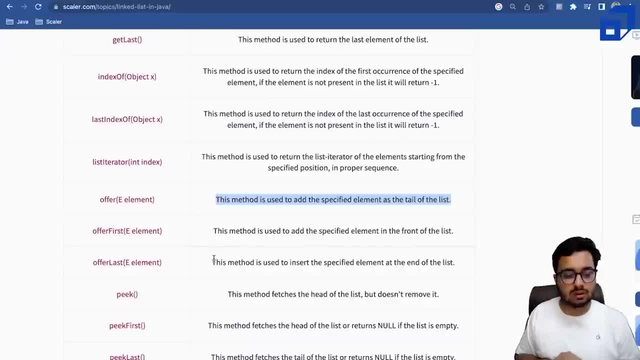 So you are going to return something like true, false, or should I throw an exception? So that is offer and we have offer first and we have offer last. Then there is a method: peek. So peek means look, I want to look at the element. 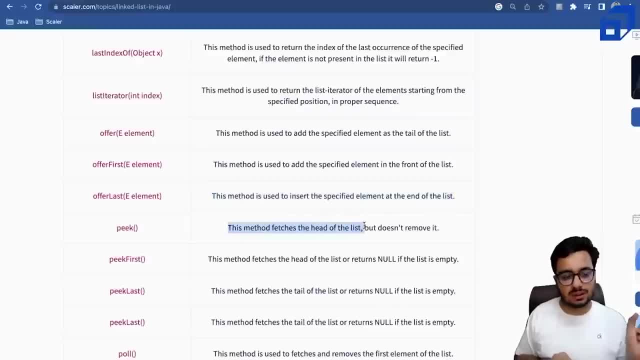 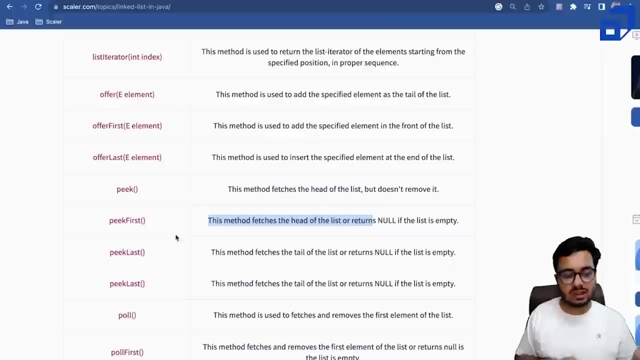 So if you simply call peek, it will show you the first element of the link list. The head of the link list Peek first fetches the head of the link list Peek and peek first. they are same, Peek last. show me the last element. 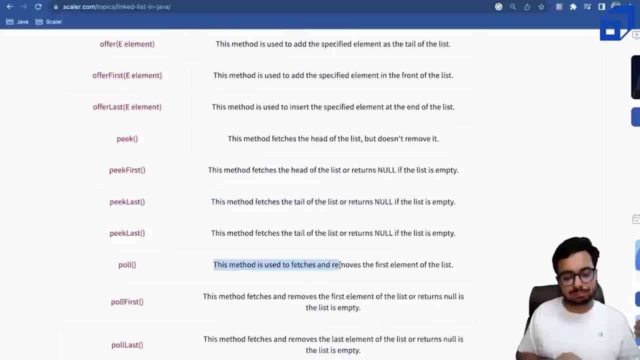 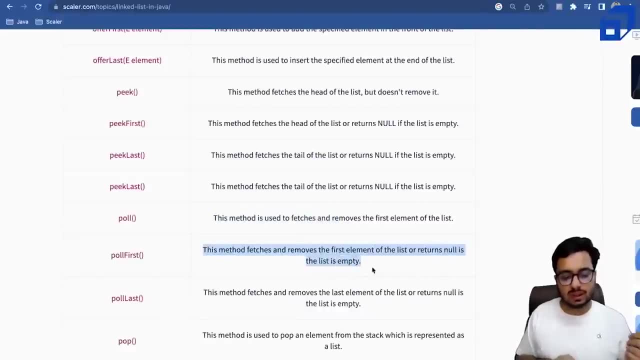 Then there is a method: poll. Poll means I want to fetch the first element of the link list. It will return the first element and remove it. Poll first is also same: Remove the first element or it is going to return null. if the list is empty, Then there is: 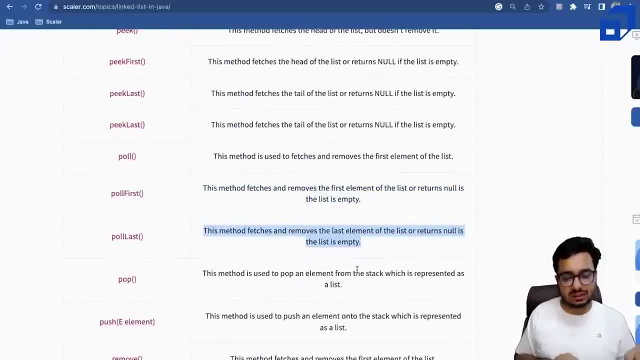 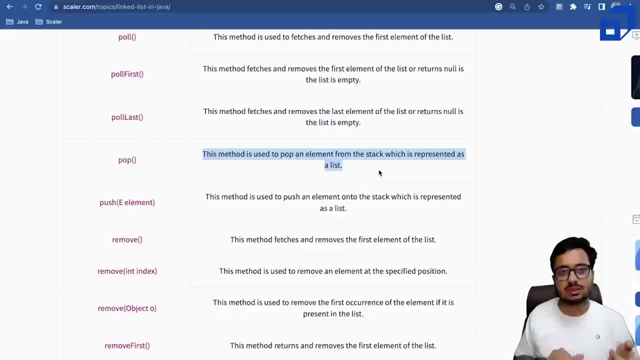 poll last. It will remove and give you the last element of the link list, or it will give you null. if the link list is empty, There is a method called pop as well. Link list can also be used as a stack, So in stack we generally call: 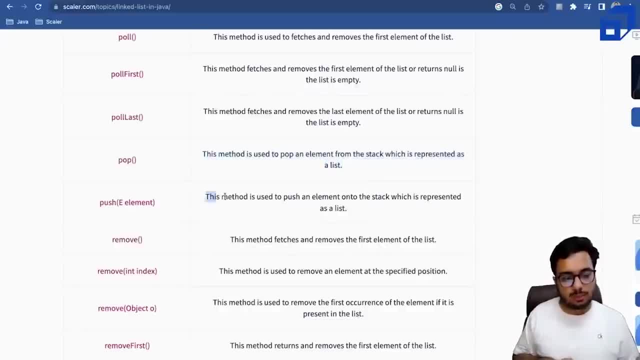 removing the last element as pop And push is also there. If you want to push something in the stack, I am pushing something, so it will push something into the link list. If I say pop, it will remove last inserted element from the link list. 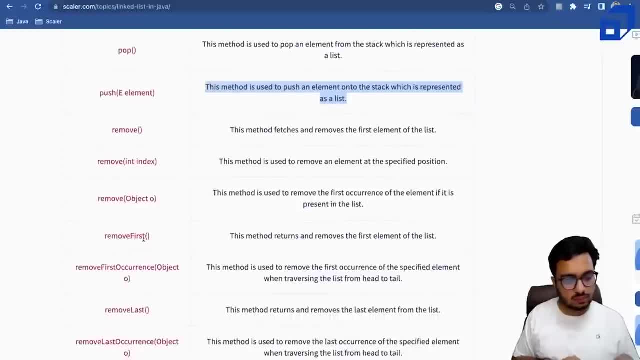 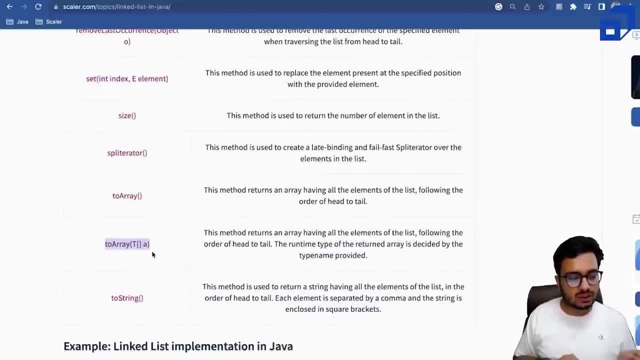 Similarly, the remove method is there. Remove first is there. Remove last is there. Set is there. You want to update a particular element and toString is there. That means, if I want to print a link list, it will call the toString method and each element is separated by a comma. 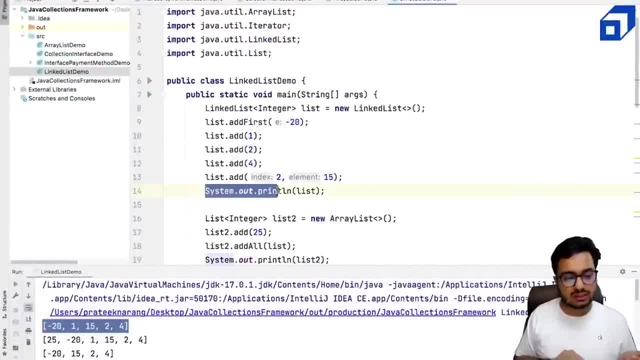 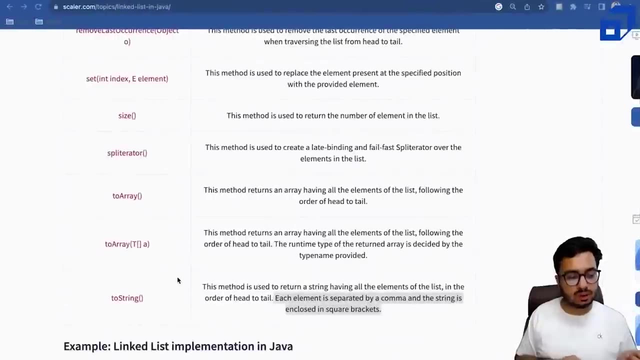 and it is enclosed in square bracket. Whenever we are printing this, whenever we are using systemoutprint list, what is happening internally? it is using the toString method of the list object to give us list which looks like this: This is coming from the toString method. 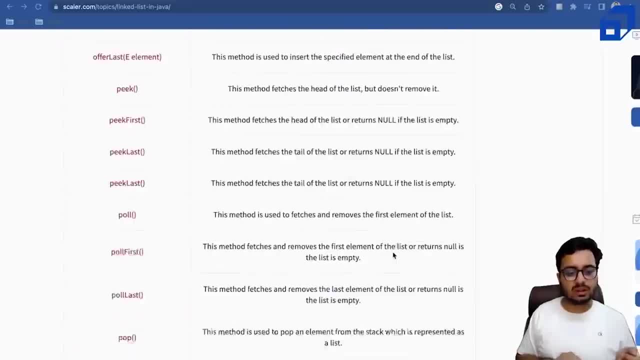 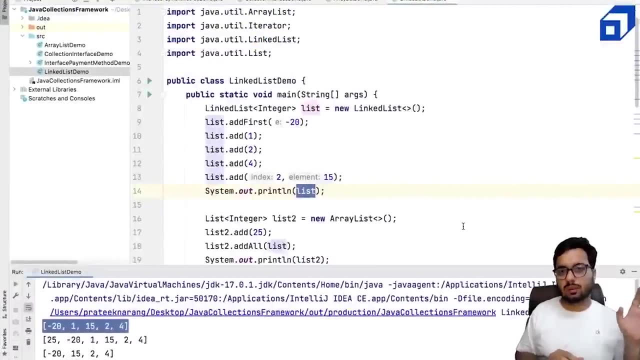 So I hope you really got an idea on what all methods you can use on a link list. So many methods are there. So mainly you need to remember that you can work on both ends. You can work on the front side, You can work on 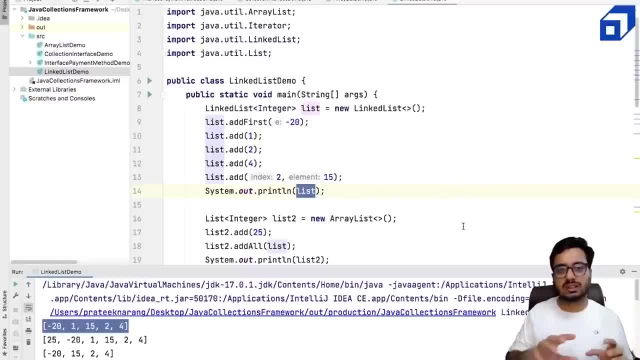 the rear end And you can also insert in the middle, search in the middle, But insertion and deletion at the ends. it is fast In the middle. it is difficult. Random access: it is difficult. It is going to take order of end time compared to. 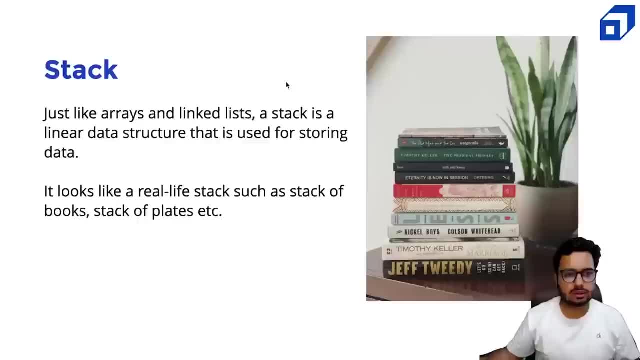 an array, So that's all. I will see you in the next data structure. Let's talk about stack. Stack is a very simple and easy to use data structure, So, just like arrays and linked list, It is also a linear data structure. 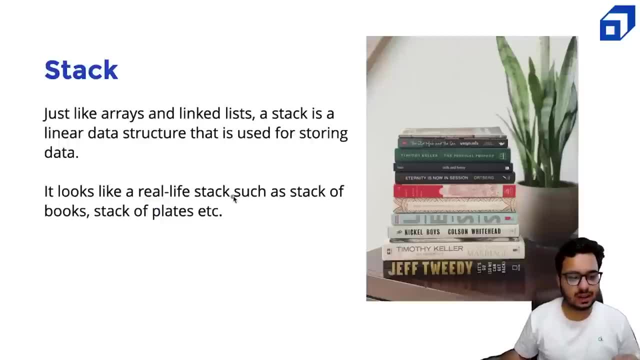 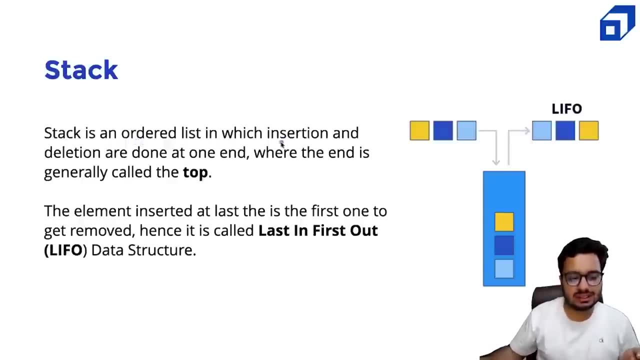 that is used for storing data And it looks very much like a real life stack, such as a stack of books, a stack of plates and let's see. So. it's kind of an ordered list in which insertion and deletion are done only at one end, For example, if you have items. 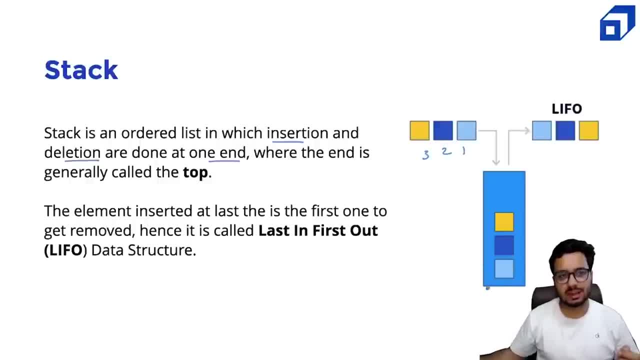 coming in 1,, 2,, 3 and you push them items into a stack. so 1 will go, then, on the top of it, 2 will go and 3 will go And if you start popping items, 3 will come first, then 2 will come. 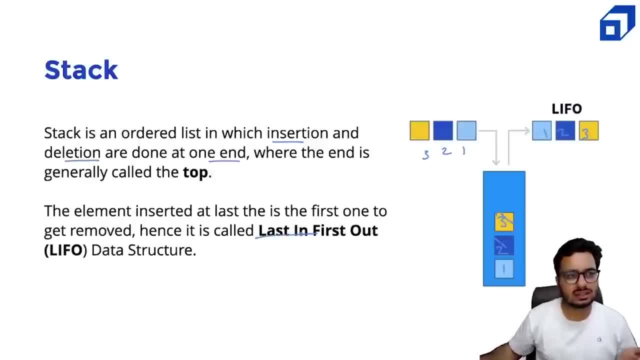 and then 1 will come. It's also called as last in, first out data structure. The element which is inserted at the last is the first one to get removed. For example, if you keep a stack of books, you put a C++ book, then you put a java book. 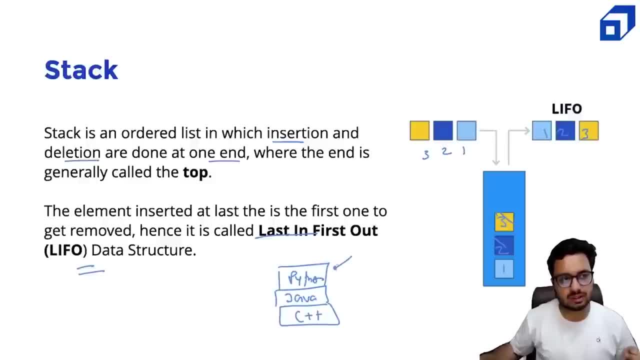 and then you put a python book- Python book is the one that you can pick first, followed by java book, followed by C++ book, Last in first out, property stackhacker. So internally, if you want to see how it is implemented, you can use a fixed size array. You can also 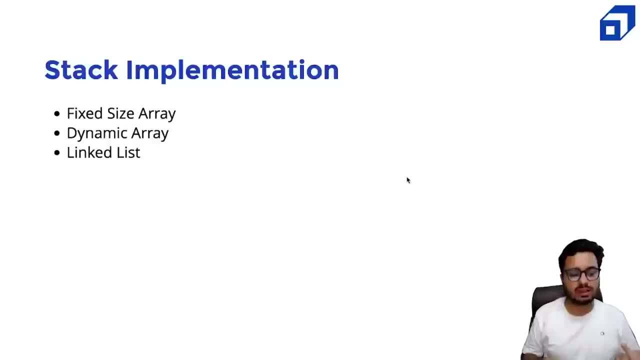 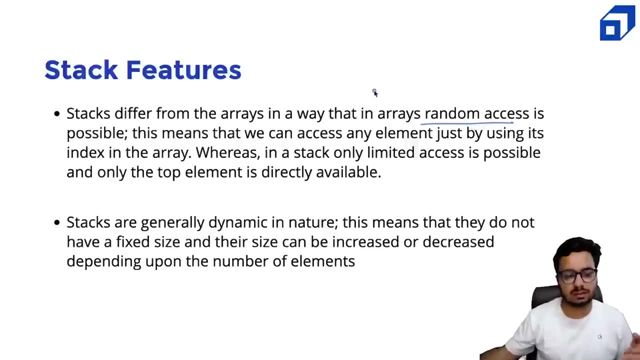 use a dynamic array. You can also use a linked list To implement a stack And how it is different from arrays. Arrays allows random access. You can get any ith element, but in case of stack of books, you can only access the top most element. 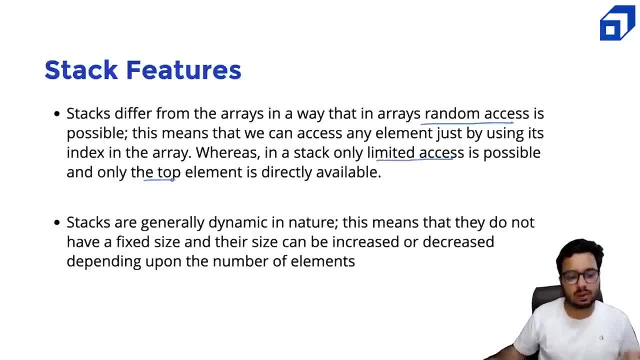 So in a way, there is a limited access possible and only top most element is directly available in case of a stack. Stacks are generally dynamic in nature. That means we don't have a fixed size and size can be increased or decreased depending upon the push and the pop operations. 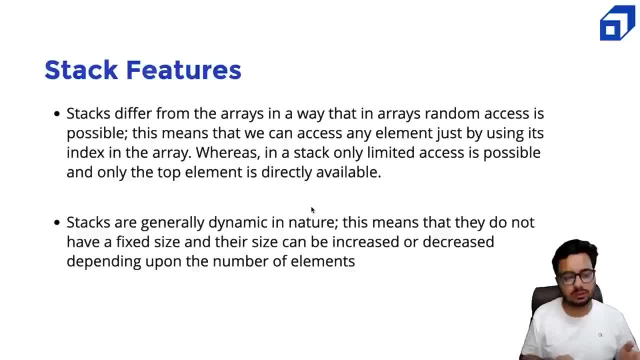 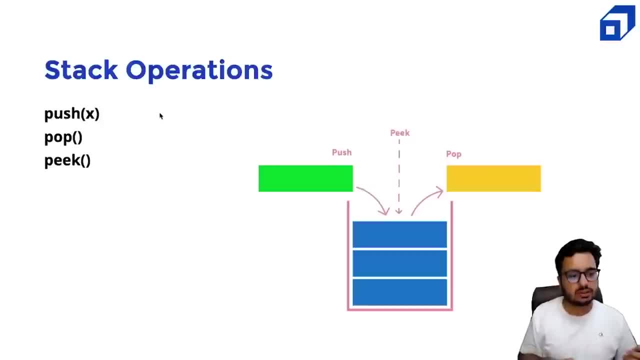 that we are doing right. So the container that you are using can be a fixed size array as well, but in general it would be dynamic, such as a dynamic array or a linked list. So the operations on stack, we are very simple. You can push an element. 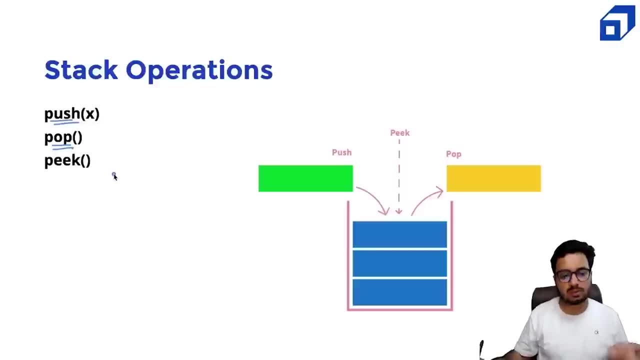 into the stack. You can pop something from the stack And you can peek. Peek means you can look at the top most element. Let us look at a code demo to understand these operations well. So in java we have a stack class which is: 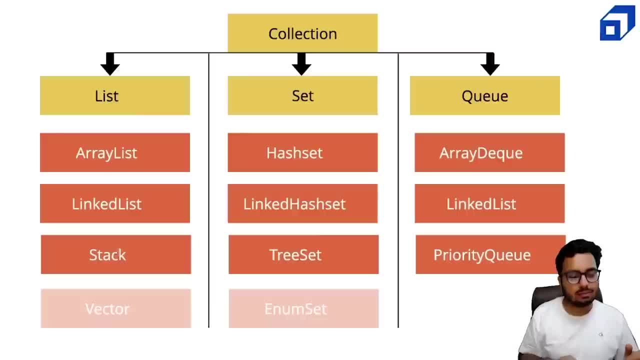 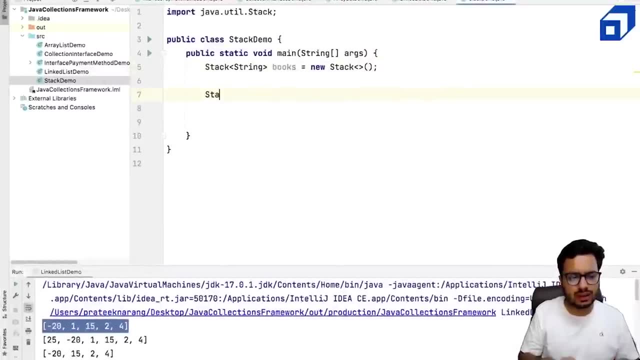 which also implements your list interface, but on the top of it, stack has its own methods as well. So let us look at a demo. So I have created a stack object, stack of string called books, and in this I can push something So I can say: books dot. 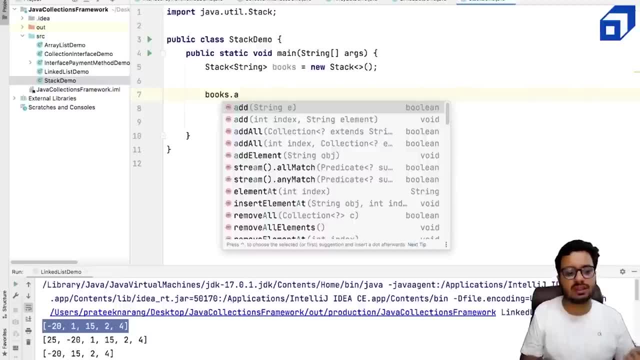 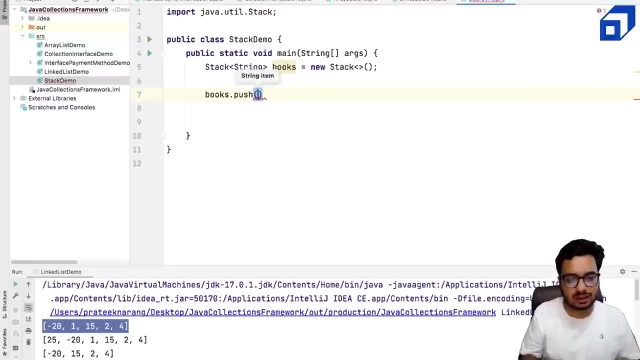 push. Now you see there is an add method as well. The add method is coming from the list interface, or I can simply call push method, which is specifically implemented by the stack class. So I can say, okay, let me push C++, let me push java. 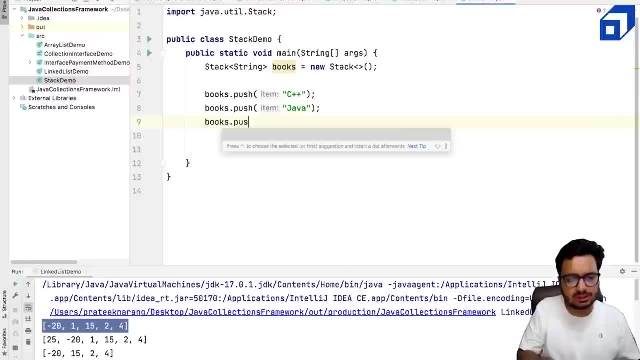 and let me push python. Let me just create three books and push it. Let us look at python. If I print the stack, it can show me what elements do we have. I call it as books. Let us run the code and suppose if I want to see the top most element. 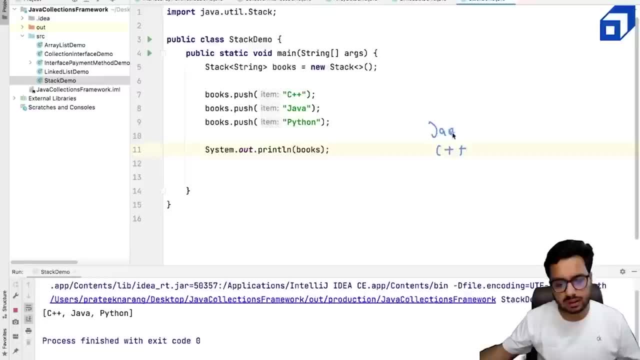 the top most element will be what It should be: pythonite. I want to look at the top most element so I can simply call peek right. So I can say, okay, sout books dot peek, that will give me python. and if I want to remove it, 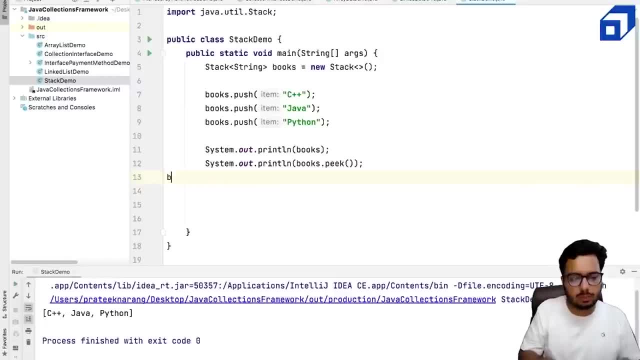 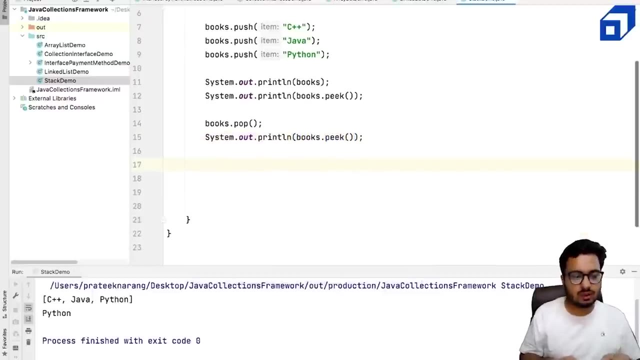 I can call the pop method. I can say books dot, pop, that is going to remove the top most element. and now, if I do peek I will see java next, sout, books dot. and apart from these methods, we can run a loop like we can say: okay. 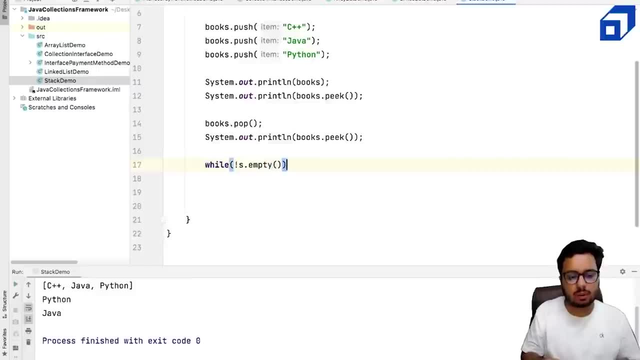 while the stack is not empty. I want to stack dot. sorry, books dot is empty. while this is not empty, I want to keep on popping elements. I want to remove them so I can say: sout, books dot peek, and I want to pop everything: books, dot. this is. 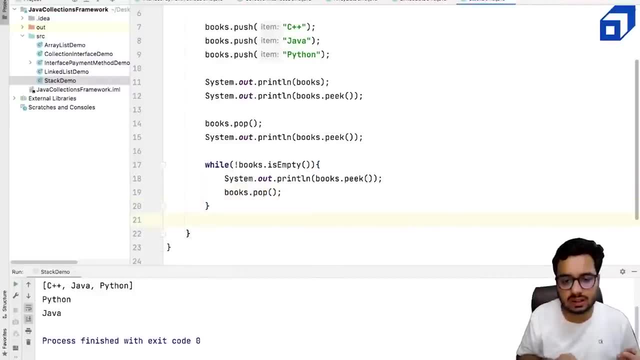 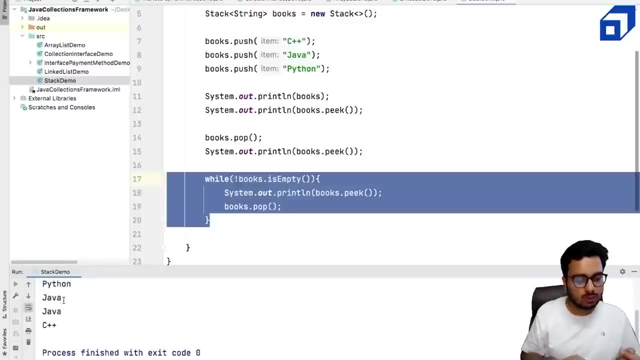 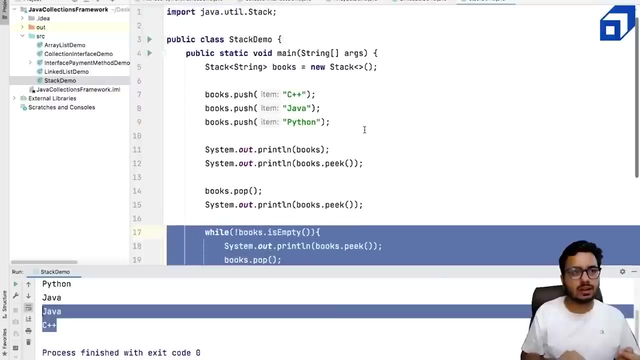 one way to iterate on the stack: you have to remove all the elements, and yeah, so I hope you are able to understand this example. so we are able to remove all elements. we first removed python, then we removed java and then we removed s plus s. that's all about stack, very simple. 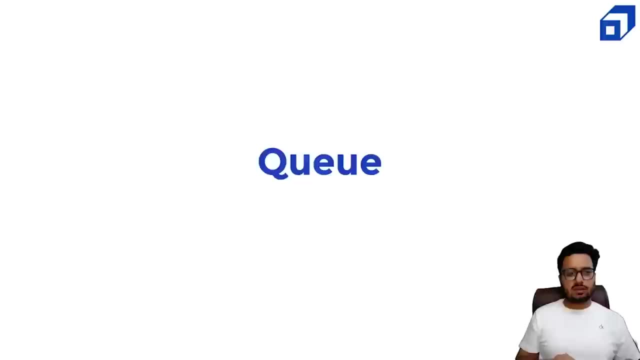 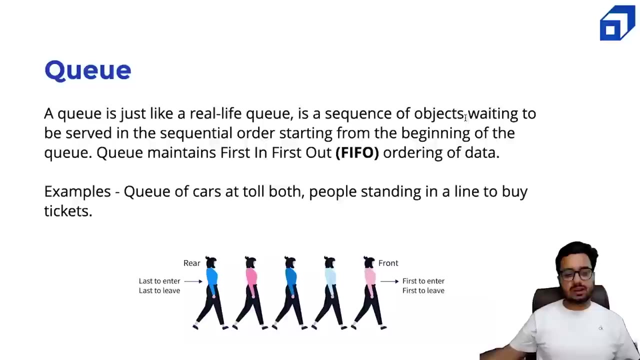 data structure and hopefully you will be able to use it. Let us talk about queue. A queue, again, is a very simple data structure. It's just like a real life queue. It's a sequence of objects waiting to be served in the sequential order, starting from the beginning of the queue. 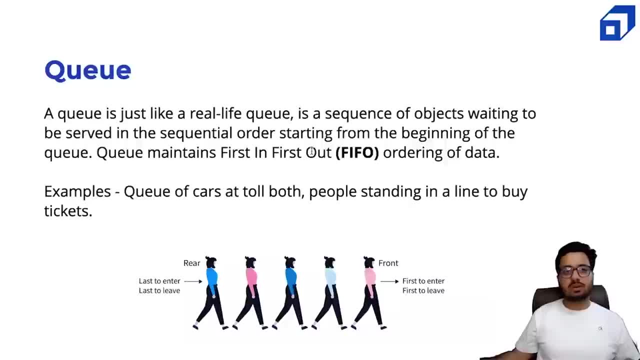 so in general, queue maintains a FIFO kind of ordering, but we also have something called as a priority queue, which is little different. For example, FIFO queue would mean a queue of cars at a toll booth. Cars are coming in to get their ticket or people are standing in. 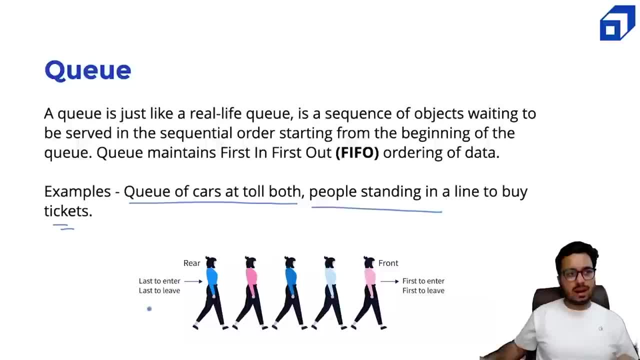 a line to buy their tickets. What happens in general? people enter from the rear end of the queue and they leave from the front side of the queue once they get the ticket. so adding some thing into the queue it's called as NQ. removing something from the queue is called as. 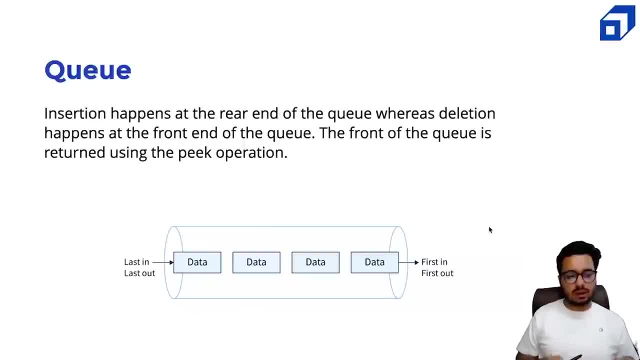 DQ. someone has been removed from the queue. So insertion, as I discussed, it, happens at the rear end of the queue, whereas deletion happens at the front end of the queue. last in, last out- the person who is entering in the last is the last one to come out, or you can say it's a. 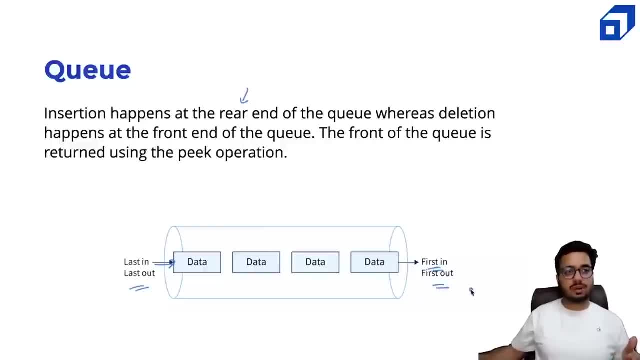 FIFO: first in, first out. the person who is coming first is the first one to come out. right The front of the queue is returned using a peak operation. so if you want to say, okay, I want to see who is at the front. the most libraries. they have a peak method like: 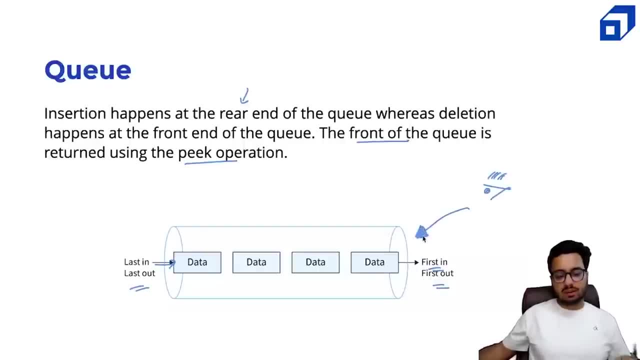 in java we have a peak method to see what element is at the front of the queue and similarly there are methods like offer to add something at the end of the queue and if you want to remove something from the front side, it's called as poll. we'll look at three methods. 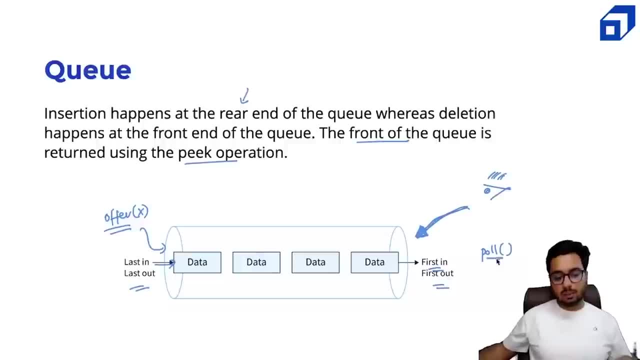 offer: adding something at the rear end, polling, removing something from the front side. and peaking means looking what is at the front, okay, so peak only gives you the element, whereas poll removes an element from the queue, right? so these are three methods that we will discuss if you want to implement a queue. 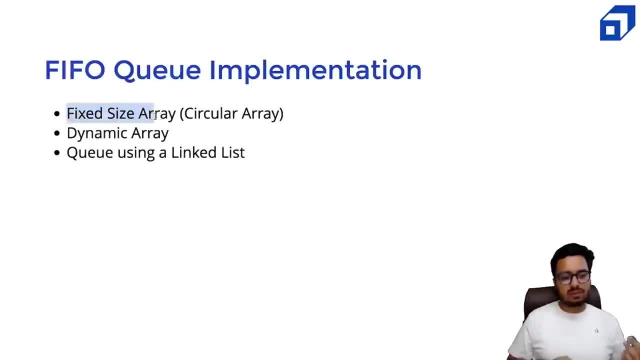 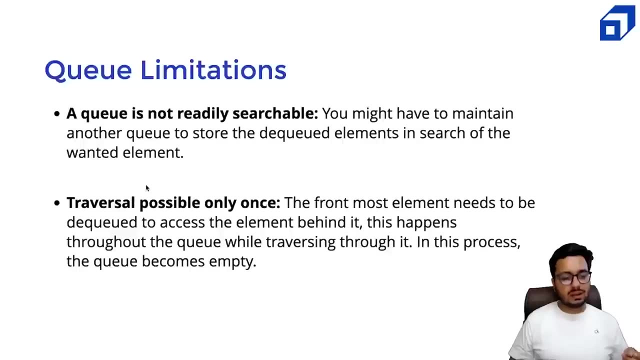 at your own end. you can use a fixed size array, also known as a circular array, to implement the queue. you can also use a dynamic array or also you can use a linked list. so there are limitations of queue. data such as queue is not readily searchable. you cannot. 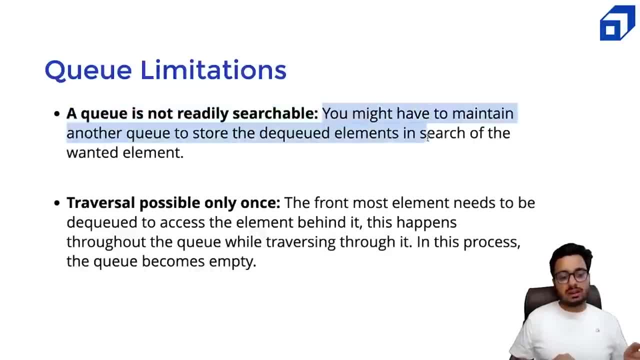 go inside the queue and search, so you might have to maintain another queue to store the dequeued elements. okay, so you have to empty the entire queue if you want to search for something and traversal- of course we cannot traverse, that is the same thing. so you have to. 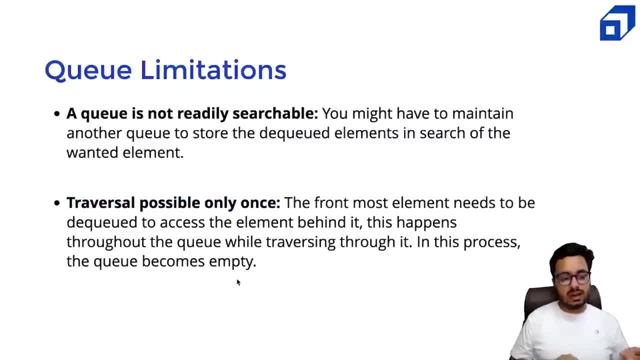 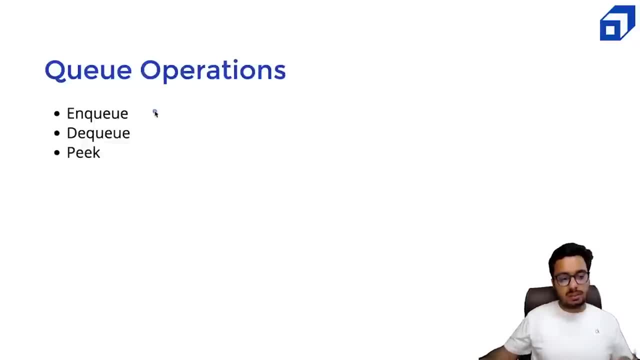 again remove all the elements to do the traversal and in this process queue becomes empty. so these are limitations of the queue. so operations: you want to add something? so the equivalent java method. it is called as offer. i want to add something into the queue, want to remove something? the java. 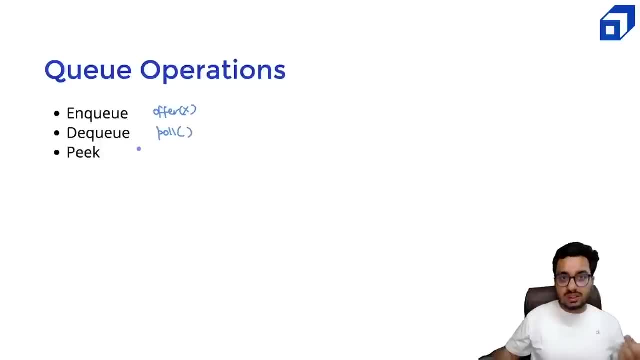 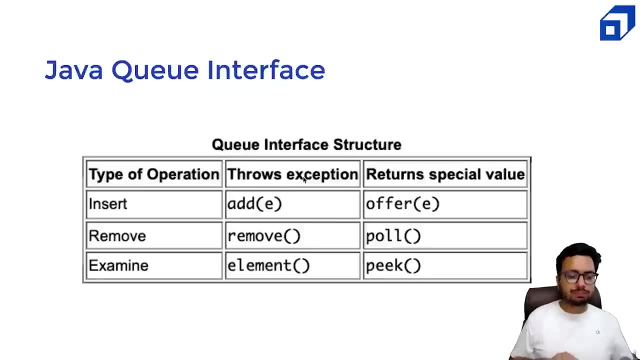 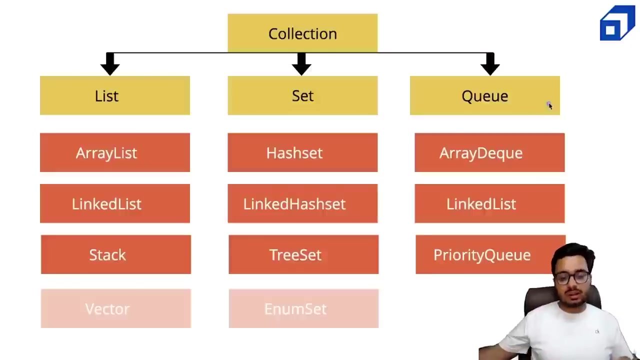 method, it is called as poll and if you want to look who is there standing at the front, the method is called as p. let us look at the queue methods in our code demo and if i talk about what are the methods there in java right? so if i told you that queue is 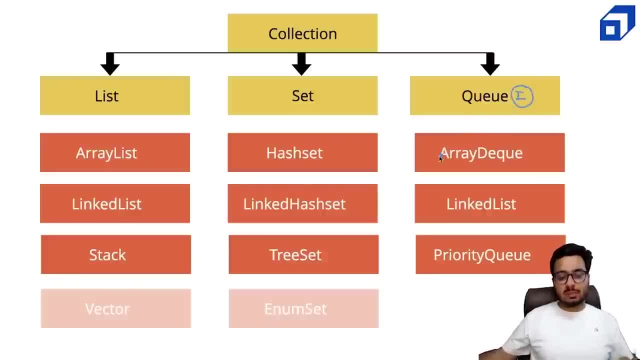 an interface in java right. so this interface is implemented by three different classes. one is called array deck, which stands for only ended queue. you can use link list, which we will be using to implement our before queue, and there is also something called as priority queue, which we will also 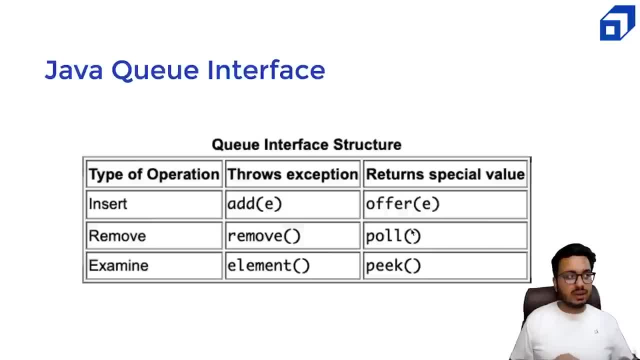 study very soon. right, we will go with the link list while implementation. right, the methods that i told you. they are insert, remove and examine. examine is like peak right now. again, i told you there are two, two versions that java provides one set of methods that throws exception. so 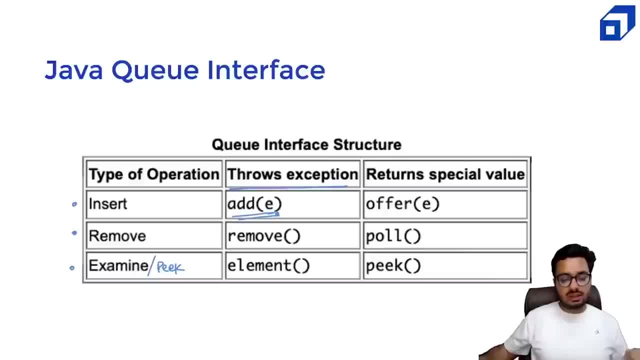 if you use- okay, i want to add something into the queue. there is a add method. or if you want to do the same functionality, you can also use the offer method. offer method returns a special value, whether your operation was successful or not. add method might throw an exception, if your 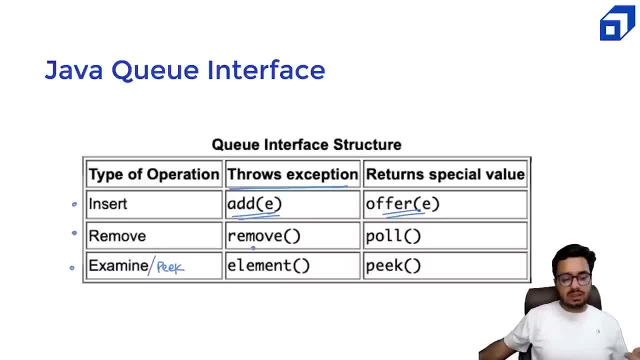 add: operation fails because of some reason. okay. similarly, remove throws an exception. if your operation fails, poll will not throw an exception element. you are looking for an element? maybe at the empty queue? right, it can throw an exception. peak will not throw an. this is how these methods are designed, so i will be. 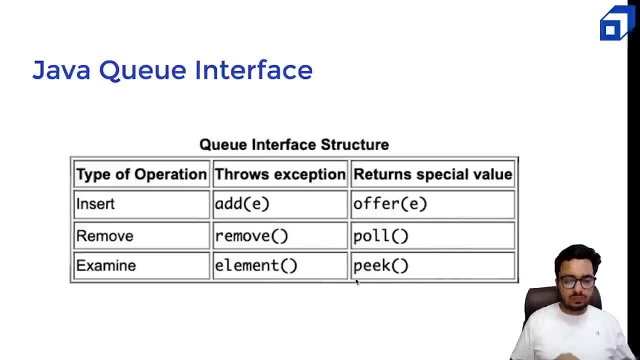 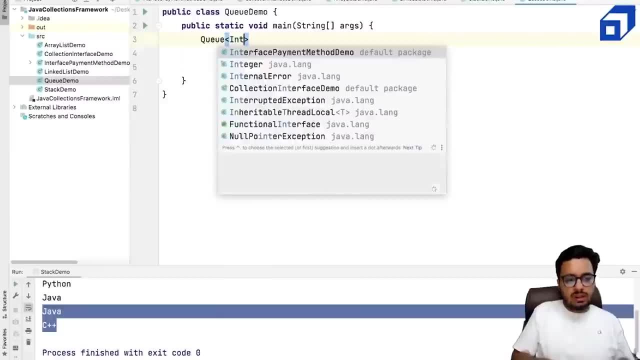 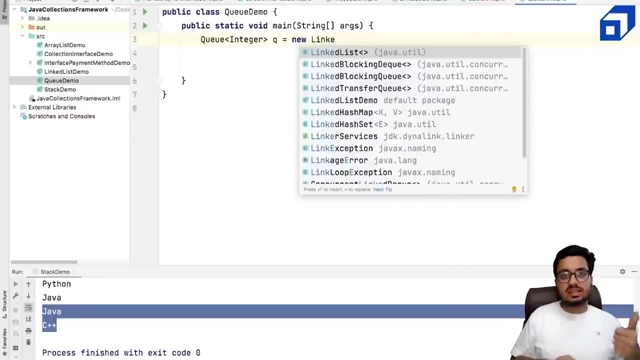 going with these methods. okay, in the implementation. let me jump into the code and let's quickly create a queue, right? well, it's okay. i want to create a queue of integers. i call it as queue and it's okay. the queue implementation. so queue is an interface. the 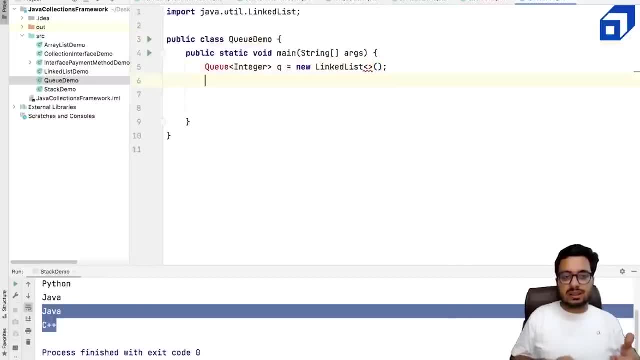 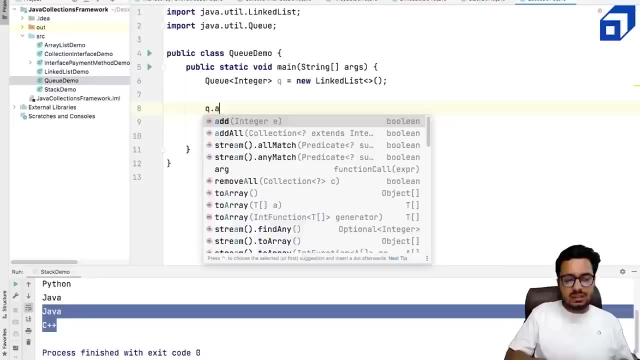 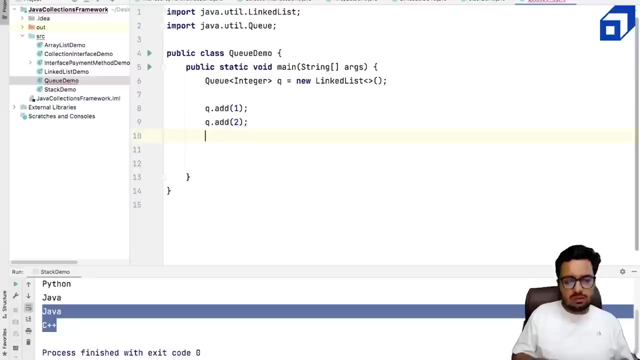 implementation is provided by the link list. we will be using link list for this queue right, so we also need to import it. now how do i do it? i can say queue dot, add some numbers. let's say one, two, three and four. let me just copy this. 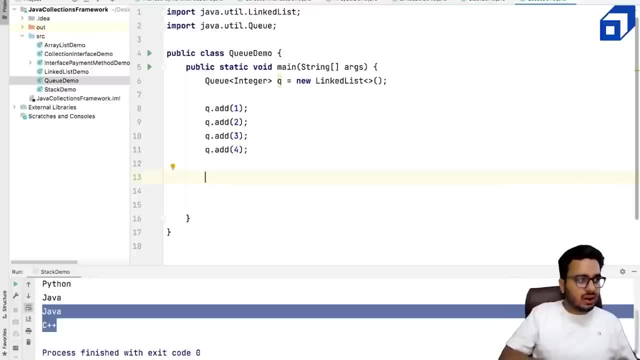 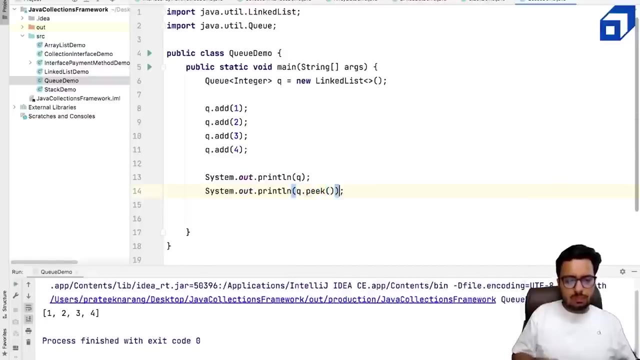 now, if i say, okay, i want to see who is at the front of the queue, or let's just print the entire queue, let's run this code and simultaneously let's see who is at the front of the queue so i can say, s out queue dot peak. 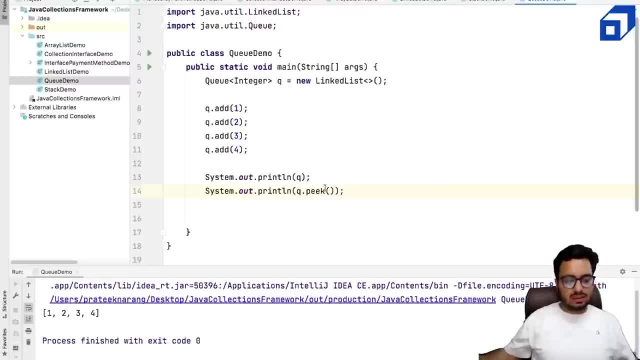 show me who is standing at the front, i will see one is standing at the front, so one came first. right now, if i remove this, it's okay. i want to remove one. i can say: queue dot um whole and then i can say: show me the entire queue and also. 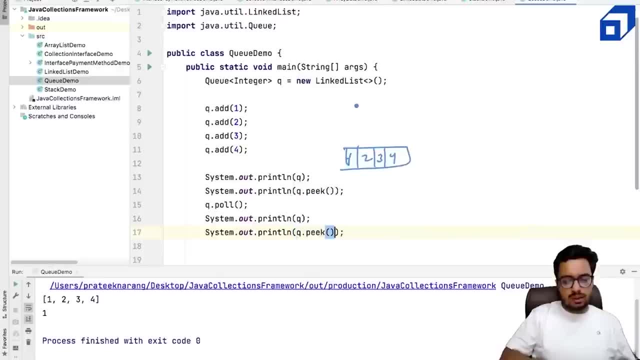 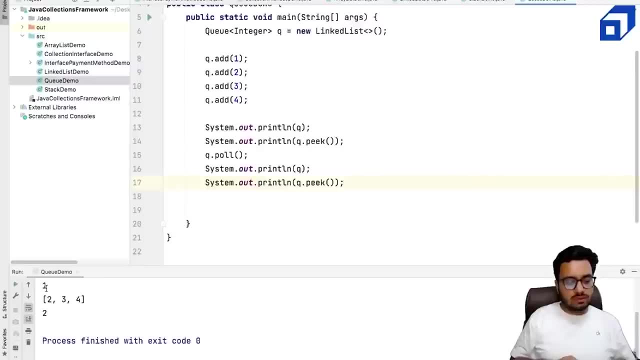 show me the front element. i can say queue dot, just like stack. you can also use a while loop to empty all the elements of the queue. so after removing one the queue is two, three, four. and if i look at the front element, the front element is now. so you can put a loop like: 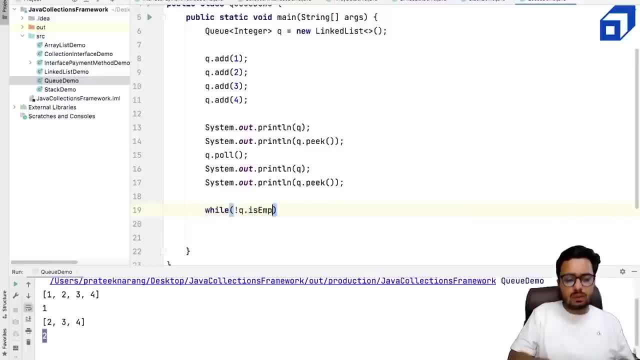 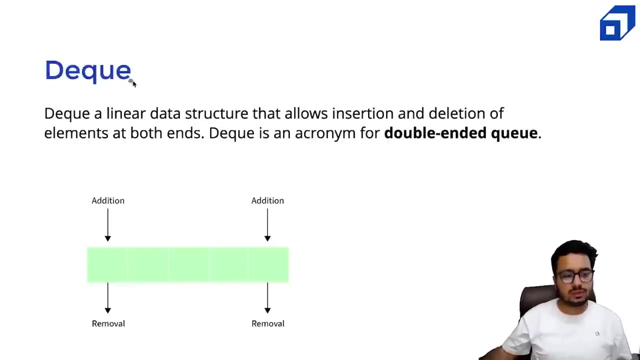 this: while your queue is not empty, you can keep on removing the elements from the queue. that is all about queue. i hope you really understood, uh, how to use queue in java. so next in line is the deck data structure. so it stands for doubly ended queue and it's pronounced: 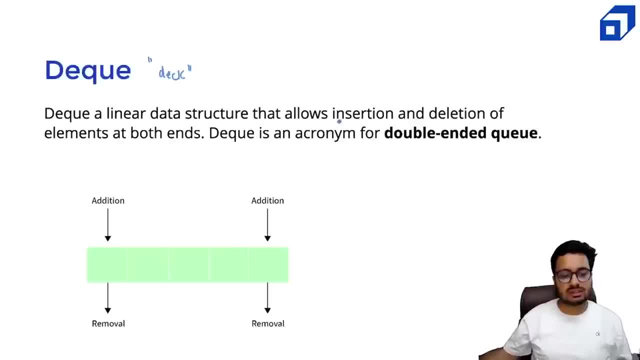 as deck, so it is again a linear data structure that allows insertion and deletion at the both ends. okay, so you, you can do insert here, you can. okay, i can expand in this side, or i can also expand in this side. maybe i insert five, maybe i insert twelve, or 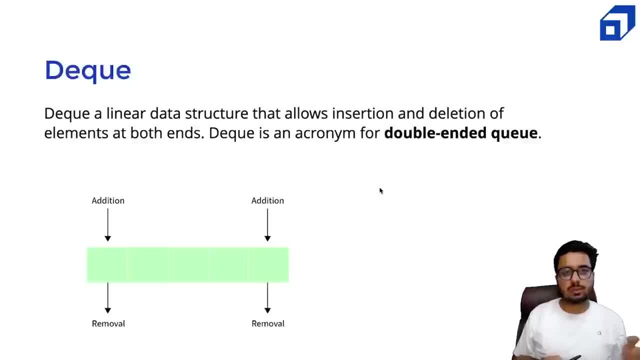 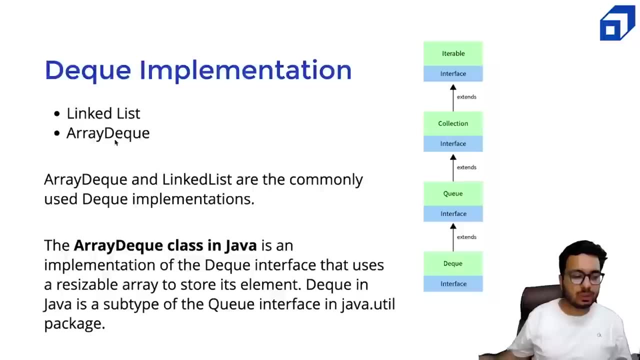 i can remove from both ends of the queue. it's a queue that supports insertion and deletion at both ends. so basically, internally we can use a link list to implement it, and java also provides a special class called as array deck, which implements the deck right. so if i look at, 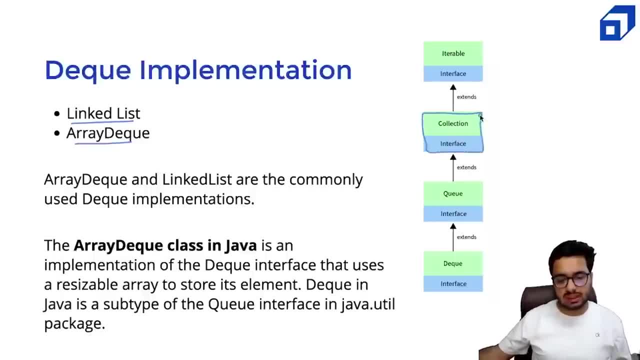 the hierarchy. so we start with the collection interface. we have seen the queue interface extends the collection interface. it adds some more methods into the collection. then there is also a deck interface which i have not shown earlier in the diagram, and the array deck is a implementation of the deck interface. 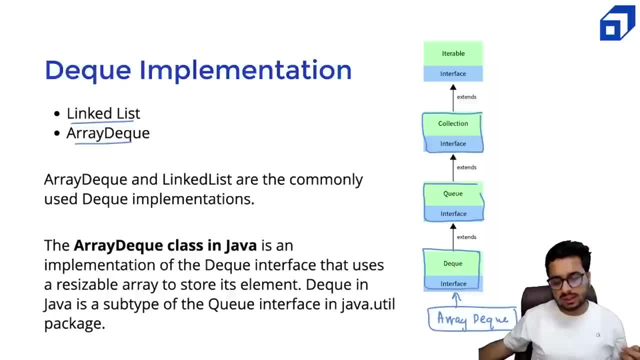 array deck is implementing the class that implements the deck interface, which is extending the queue interface. so this is what you- it's a good to know thing, not mandatory right. array, deck and link list are commonly used deck implementation. if it is a double link list, you can see it is. 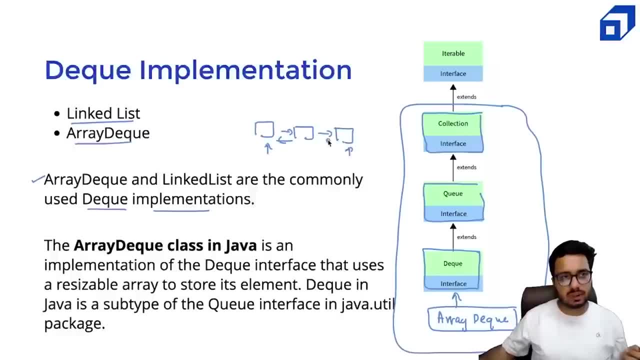 very easy to expand something on both the ends right, so you can simply add something here as well, and your tail will move right. you can add something here as well, your head will move right. so it's pretty easy to use link list. but array deck internal implementation is: 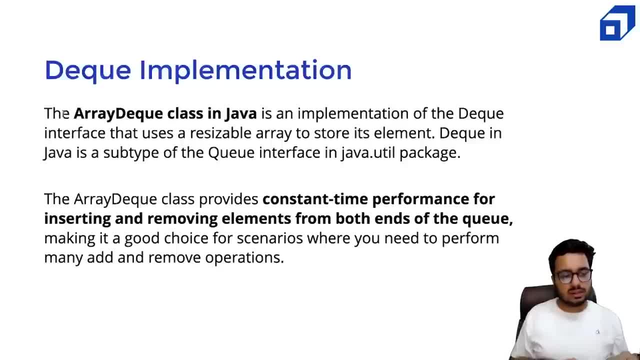 little more complicated. i'll discuss few more points about array deck. it is a implementation of the deck interface that uses a resizable array to store its element, and deck is a subtype of queue interface that we have just discussed. best thing about array deck class is it provides constant time performance. 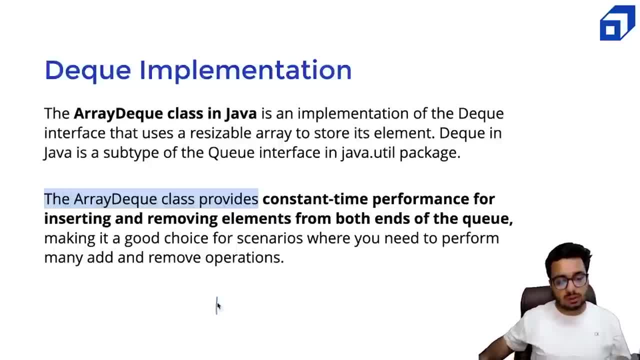 for inserting and removing elements from both the ends of the queue. now this is very tricky. right in an array we cannot do constant time insertion and deletion at both the ends. we can do only at one end, right. but in deck, in array deck it uses internally some. 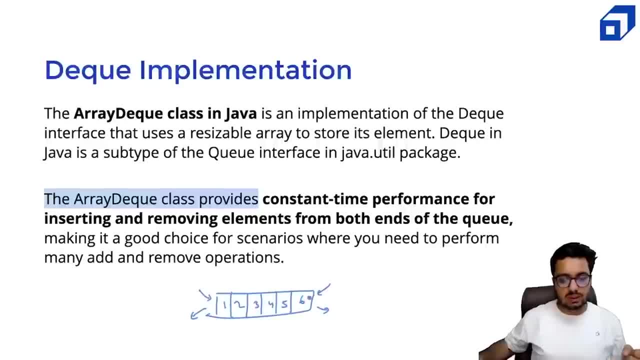 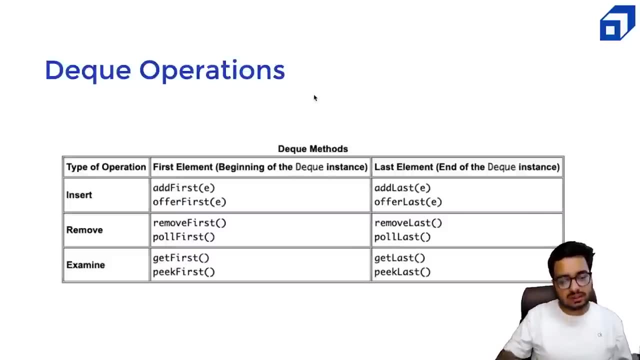 complicated mechanism so that we can remove and insert from both the ends of the queue and these operations can be done in order one time from both the ends, right. this is a very powerful feature of array deck that we must know. talking about the operations, right, if you want to add something. 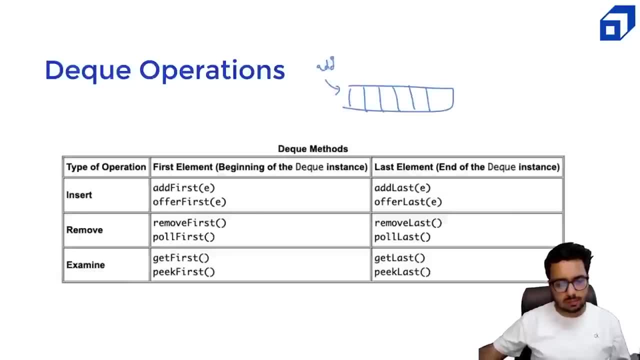 at the beginning. you can say: add first, okay. or you can use a method called as offer first. these are two methods which are doing the same work. there is a minute difference if, due to, let's say, capacity limitation, you don't have memory or you are restricting the size. 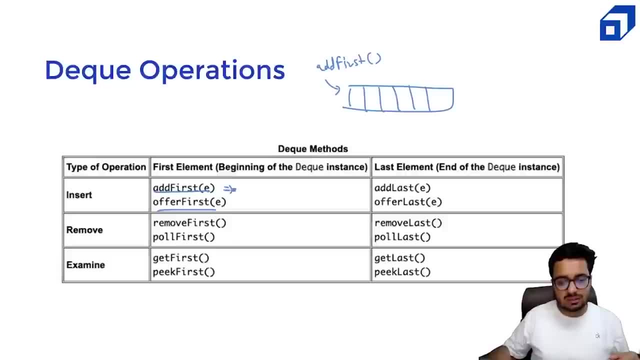 of the queue and you are trying to add some element, then add first will throw an exception. will throw an exception, just like other add method we have discussed. the offer method will return false at okay, i could not return this element. i could not add this element. similarly, 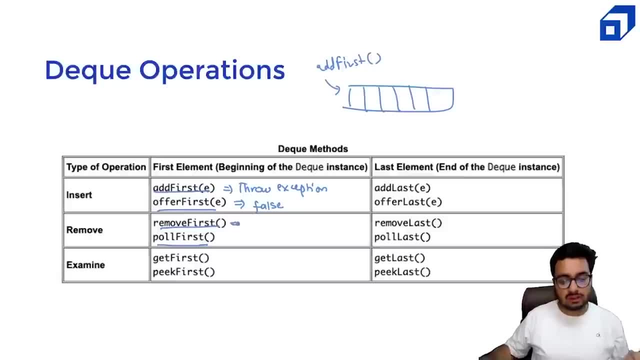 we have remove first and poll first methods. so remove will throw an exception. poll will return true or false. get first will throw an exception. peak will tell me whether the element like if i could not get that element, it will throw an exception. peak will tell me null, i could not remove that element. 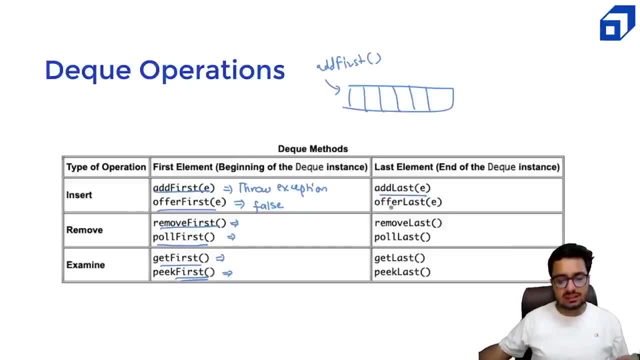 that might happen. right, there is add first. there is add last, offer last, remove last poll last, get last peak. if you ask me what method i would be using, i would be using offer first, poll first, peak first. so if you want to do operations at this end, 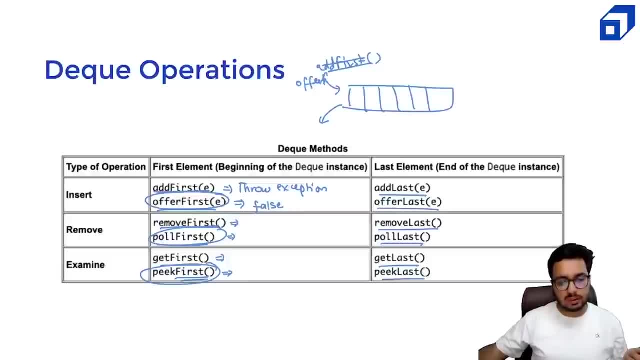 you want to add something, use offer first. you want to remove something from the front, use poll first. and if you want to look at what is this element, you can use peak first. same operations. if you want to do a this end, what you will do, you will say offer last. i want to. 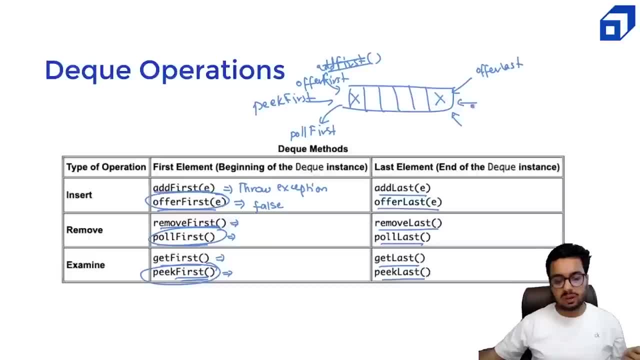 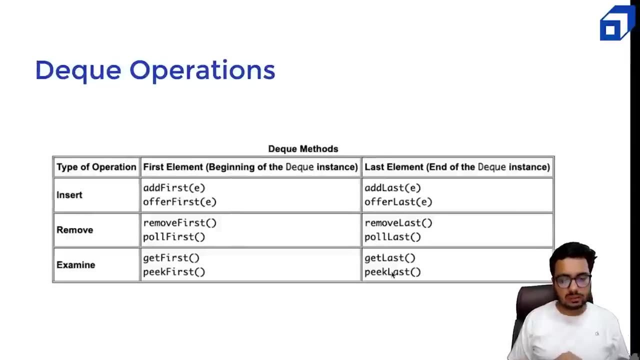 add something here, i want to remove something from here. i will say poll last and i want to see something. what is this last element? so i can say: peak, show me the last element, this tech. so that is about the operations of tech. now let us look at: 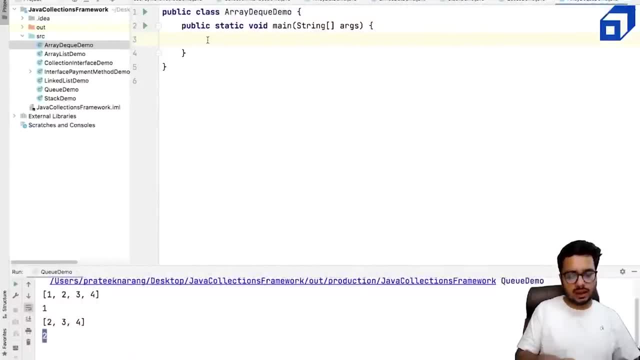 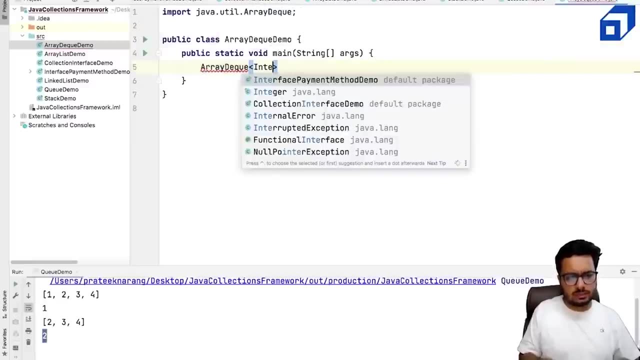 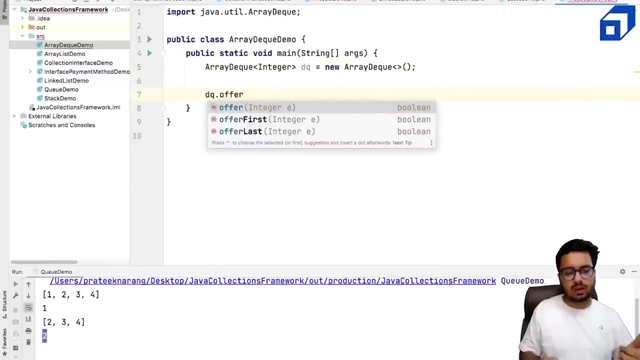 a code demo for tech. let us create a array deck object. you can say array deck object. you can say array deck of, let's say integer, integer, integer equals to, equals to, and in this deck i can add elements. i can say offer. so there is a offer method as well. 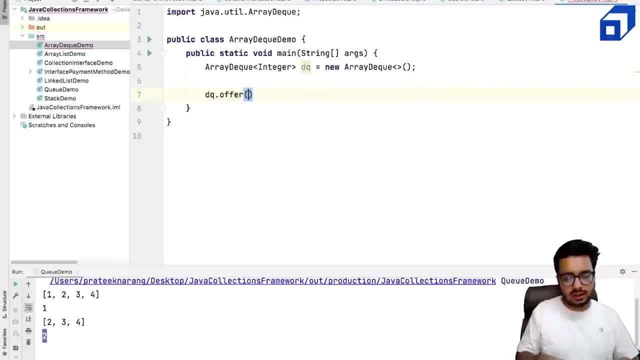 offer first is there, offer last is there. so i can say, okay, let me show you offer first, let's say 12 tech dot offer, let's say 15 tech dot offer, offer last: let's say 20 tech dot offer, let's say 30. let me show you what. 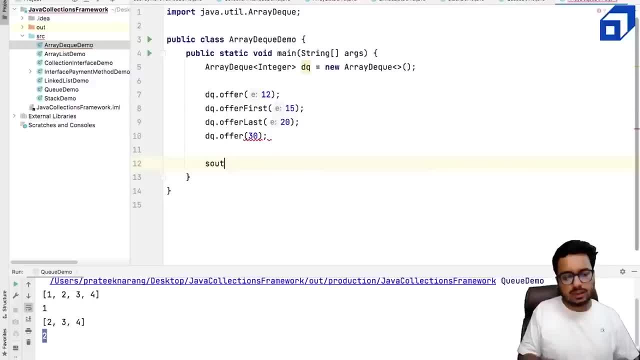 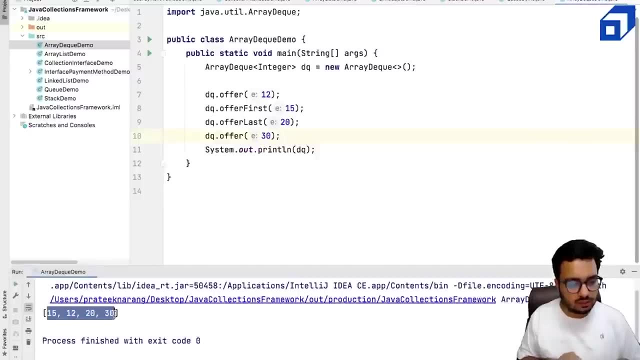 in what order the elements have been inserted s out. i will say deck and let's run this code. i am getting 15, 12, 20 and 30. so first i had 12 offer. first i said in the beginning i had i want to add something. 15 gets added here. 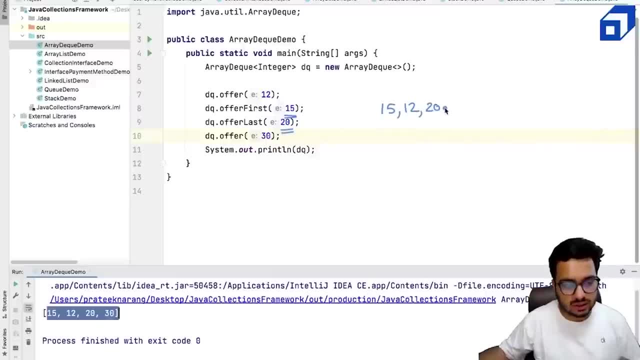 then i say offer last 20, so 20 gets added here. then i said offer 30. offer is actually behaving like offer last offer and offer last. they are doing the same work. this is how your deck is getting created. similarly, if you want to remove something, you can call the. 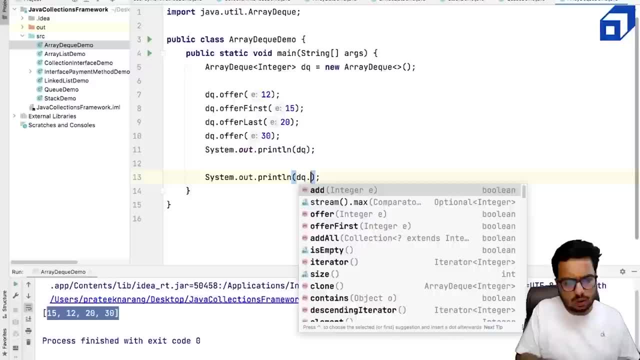 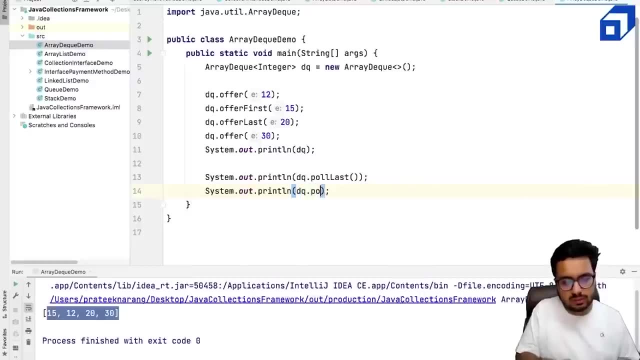 poll method. you can say: s out tech dot poll last. give me the last element, s out tech dot poll first. give me the first element: s out tech dot. and if you want to see now what is the new first element, you can just call pick s out tech dot. 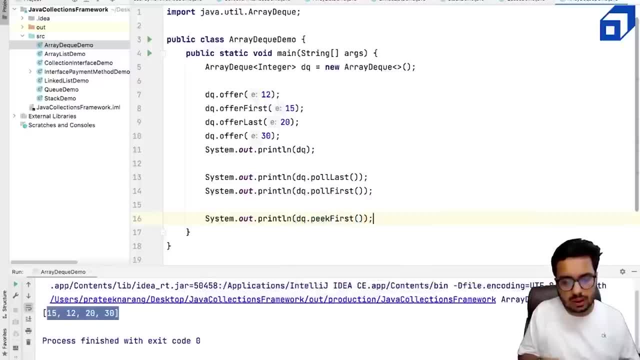 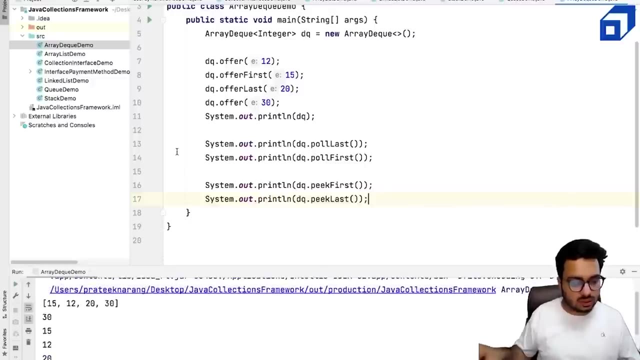 peak first. show me the new first element and s out: show me the new last element, peak last. let us run the code and see this is our deck. if i say give me the last element, so it removes 30, it's gone. give me the first element, it. 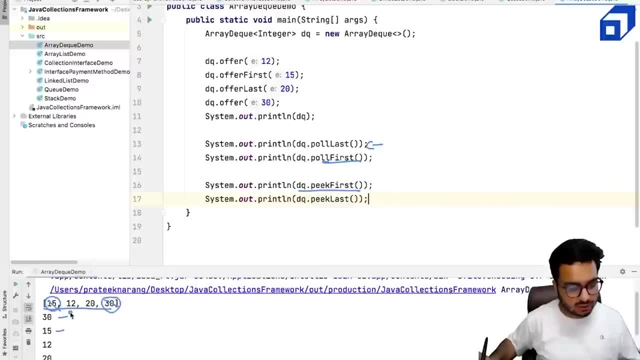 removes 15, it is gone. show me the first element. the first element is 12. show me the last element. the last element, that is how easy it is to work with deck, and i hope you understood the concept. let us talk about priority queues. priority queue is a special type. 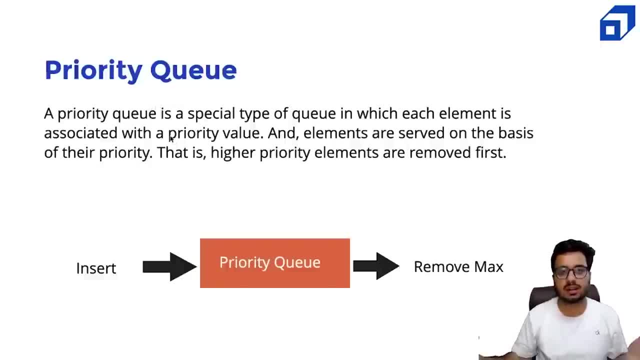 of queue in which each element is associated with the priority value. for example, if people are standing in a queue and you might want to give priority to the senior citizens, maybe age is a criteria in which people will get their tickets. okay, senior people will get their ticket first. young people will get their. 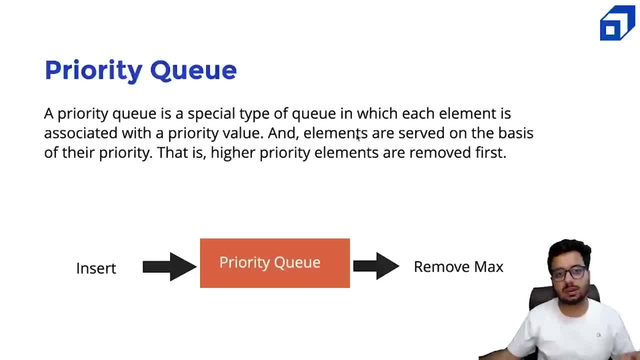 tickets later. so, basically, elements that we are going to serve in the queue, they will be served according to a certain priority. higher priority elements are going to be removed and it is up to you. how do you define the priority? okay, maybe a big number has a more priority. 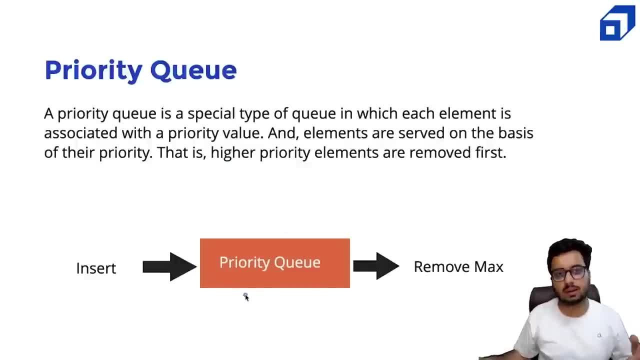 or maybe a lower number has a more priority. we can have a max priority queue. we have a min priority queue. we can insert like people can join the queue, right, but maybe this is 16 years, this is 20 years and this is maybe, uh, 4 years. 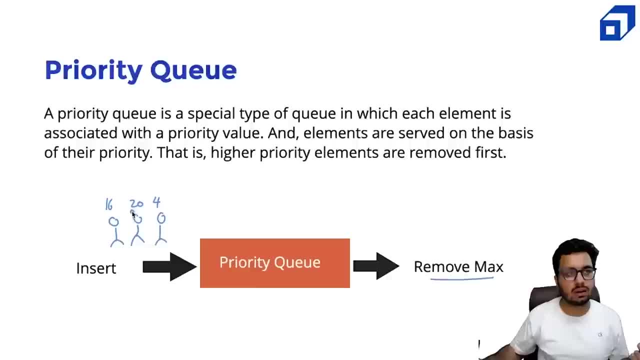 right now. if i say, okay, i want to remove someone, i will remove the person with the maximum. i will remove person 20, right, so this will get removed so people can join the queue. but when i am going to remove people, the people with the higher priority will get. 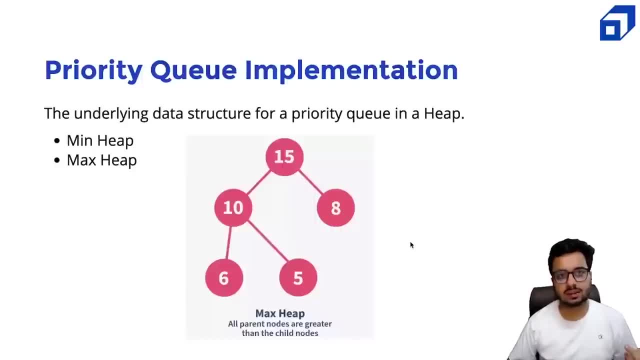 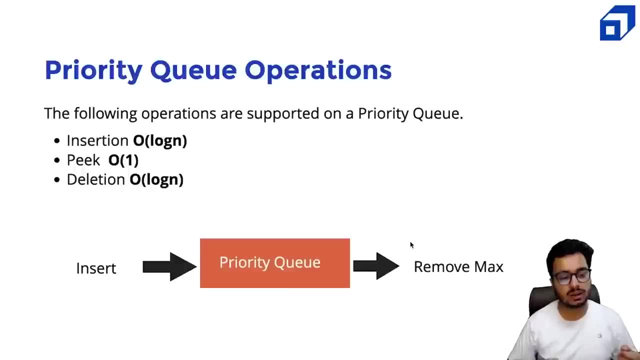 third, first right. so the underlying data structure for a priority queue. it's a heap. we can have a mini for a maxi. i will not be able to dive into the details of heap at this point. we'll be looking at how do we use the java priority. so 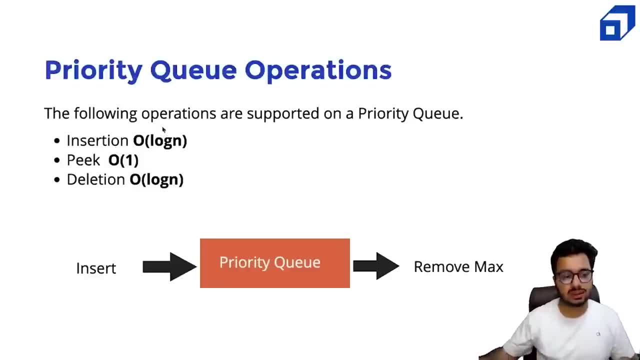 the operations that are supported. we can insert something. inserting in a queue it's called as a offer. i can offer some data inside a queue i can look at. i want to see who is standing at the front of the queue that is called as peak and if i want to. 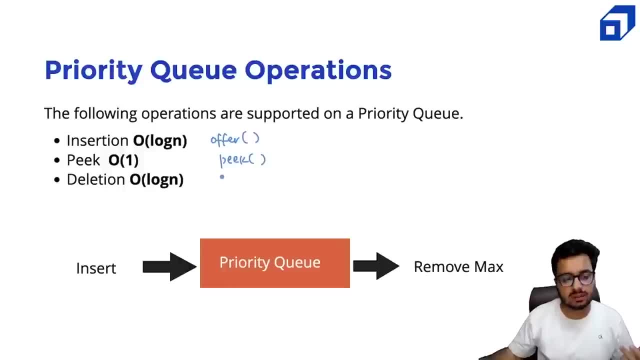 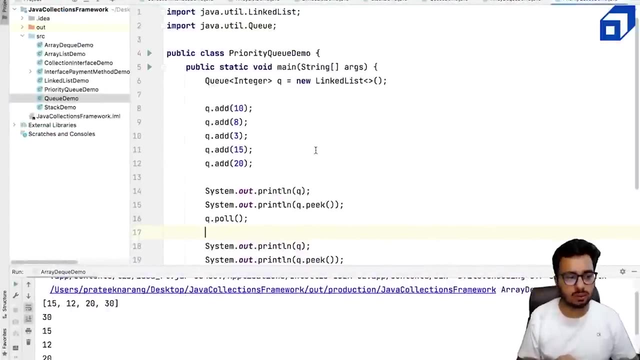 perform deletion. i want to remove someone right from the queue that that is called as pole. we'll be looking at these methods and insertion and deletion. they are login methods, looking who is at the front, the order, one method right. so let us do a quick code code demo as well. 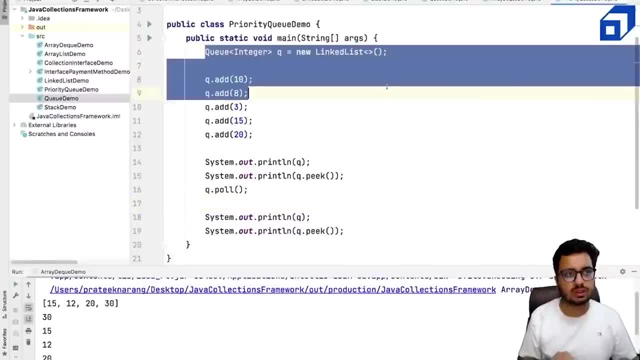 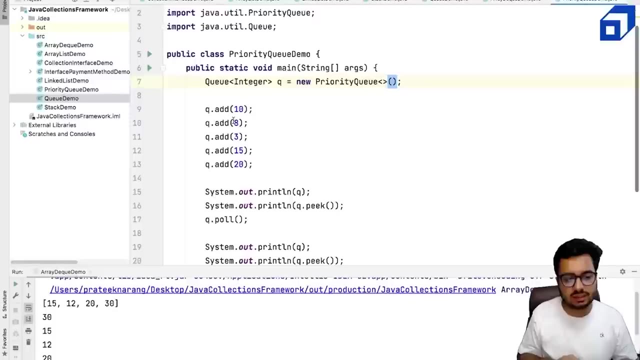 so we have seen how to work with the queue. this is the code for a queue. a priority queue is a class that implements the queue interface. okay, so right now. it was a feed flow queue. now i'm going to change it to a priority queue, right, so rest, everything will change. 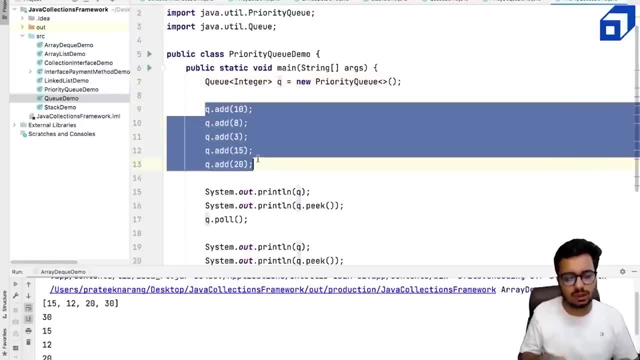 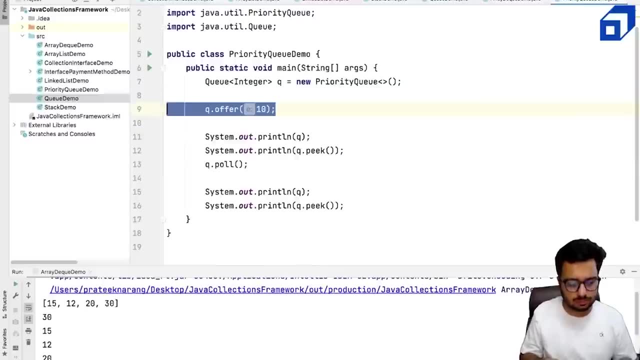 if you want to add, add method will also work. but if you want to use the offer method, i can use offer method as well. i can say queue dot. offer some numbers. 10 will change the data. like i have: 10, 0, 8, maybe 7. 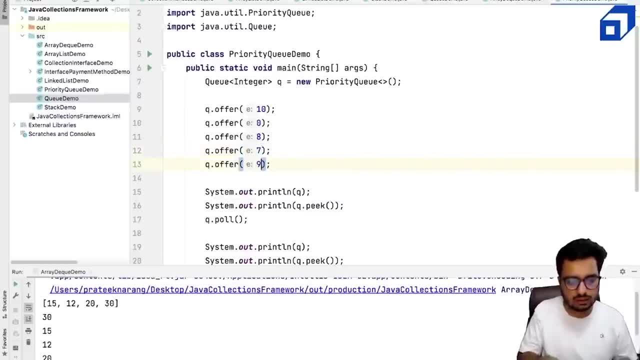 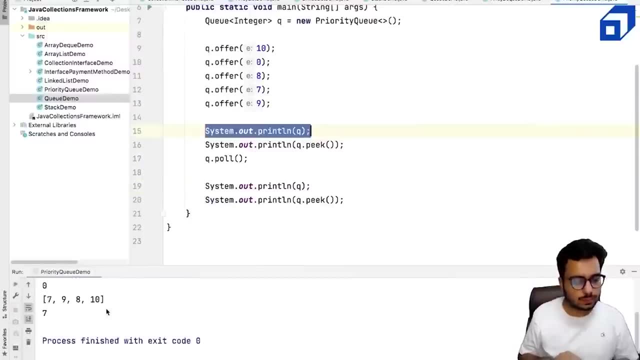 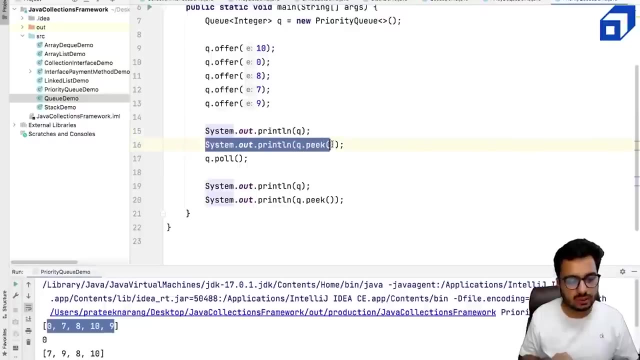 and let's say 9. now, if i say okay, i want to print the entire queue, let's see what output do we really get? okay, so i'm getting this output: 0, 7, 8, 10 and 9. i want to look at what is the first element. 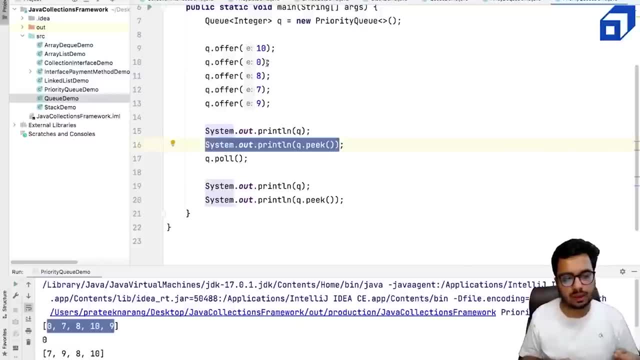 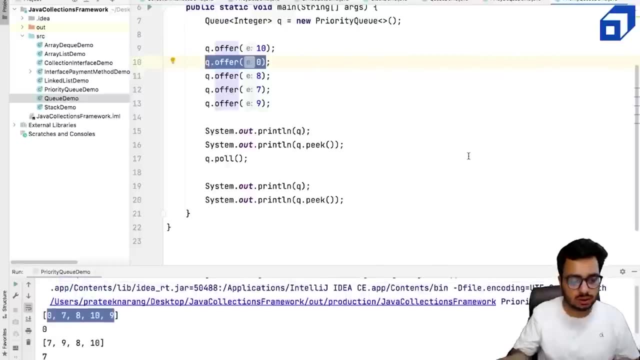 i'm, in this case, the lowest element. it's getting priority right. so you see 0 is coming at the front of the queue. rest of the queue is not actually sorted, only the priority element. it comes to the front of the queue, right? so 0 is there if i say okay. 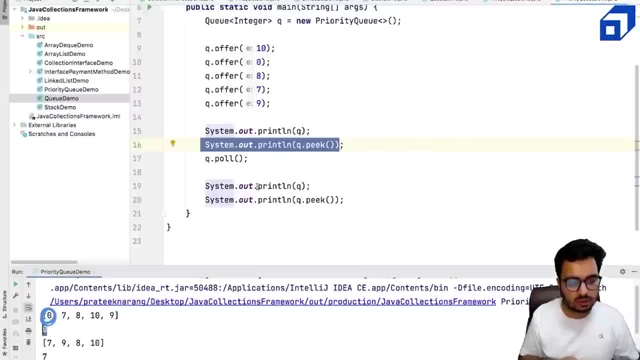 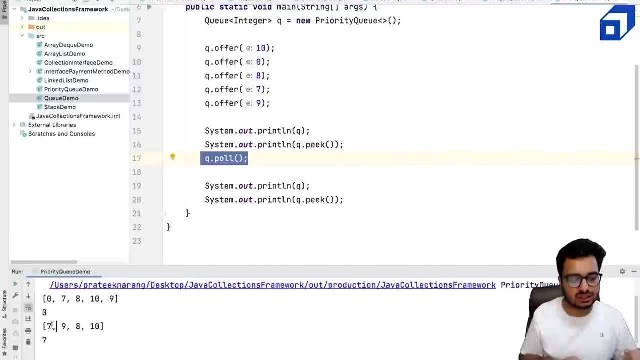 i want to look at this element, so this element is 0. and i want to remove this element, so it removes 0. and now what is the next lowest element in the queue? that is 7. so 7 comes to the front of queue, if i. 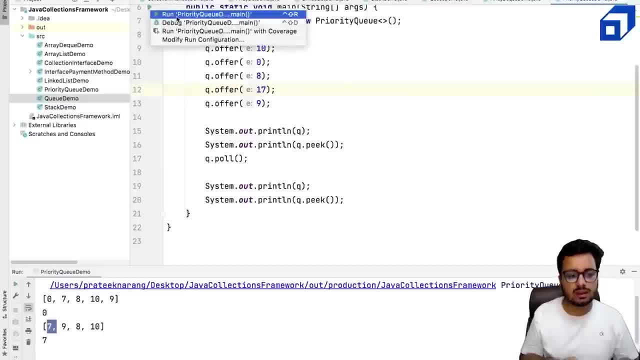 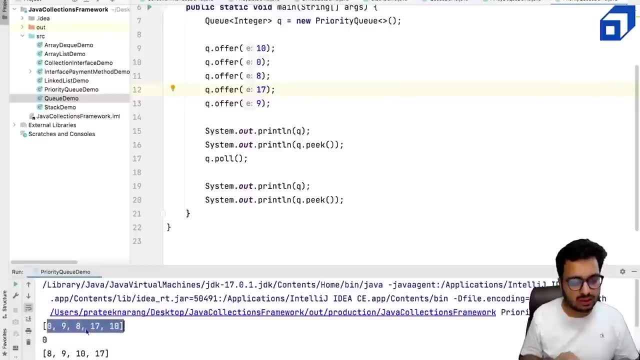 make it 17, then the next lowest would be 8. right, so let me run it once again. now i have 0, 9, 8, 17 and 10. the lowest element, it is at the front. then if i remove 0, the next lowest is actually. 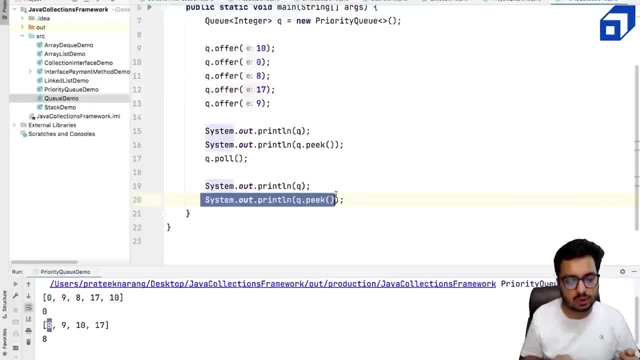 8. so that comes to the front. if i remove that element or if i look at what is that element, i get that element 8. using the peak operation, you can see the element. using the pole operation, you can remove the priority element. now you might ask if i 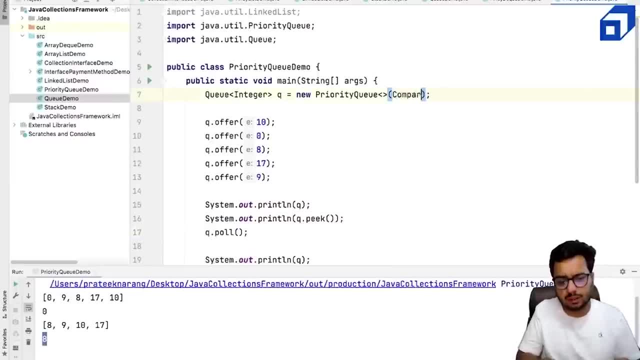 want to reverse the order? okay, so in that case you can pass one more comparator, so i can say: okay, comparator dot, reverse order. this is exactly going to reverse the comparison. the main priority queue becomes a max priority queue. in this case, the highest element, it's going to get a priority right. so now you. 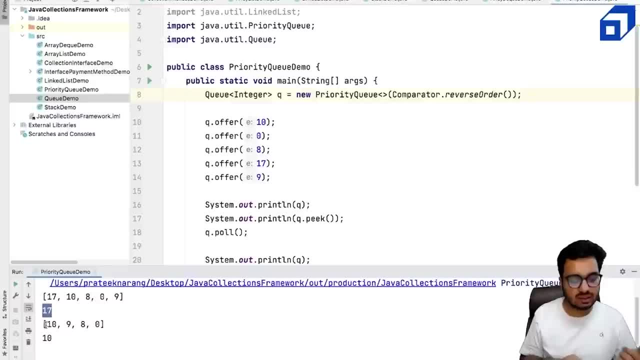 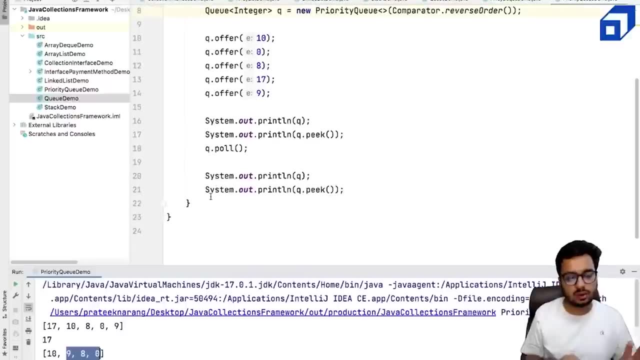 look at: 17 is standing at the front. if we remove 17, 10 is standing at the front and there is no specific order for rest of the elements. that is unpredictable. we are only worried about the element at the front should be either the main element or the. 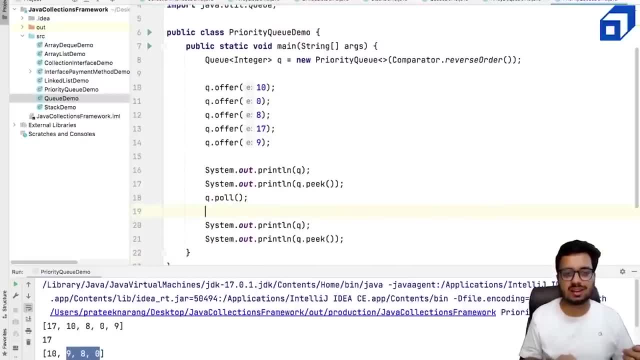 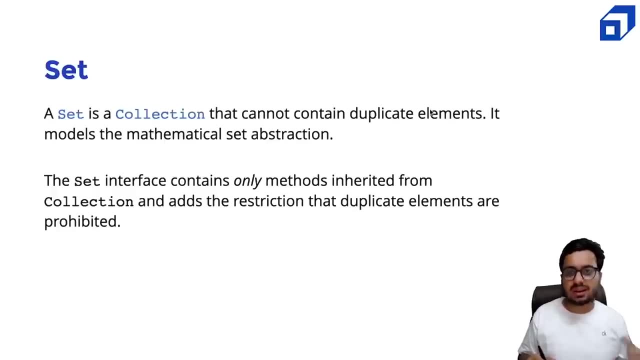 max element. this is about priority queue in java. let us talk about set interface now. so what is a set? mathematically, it has a collection of elements that cannot contain duplicate elements. okay, so set. in java it models the mathematical set abstraction. now the set interface that we have seen. 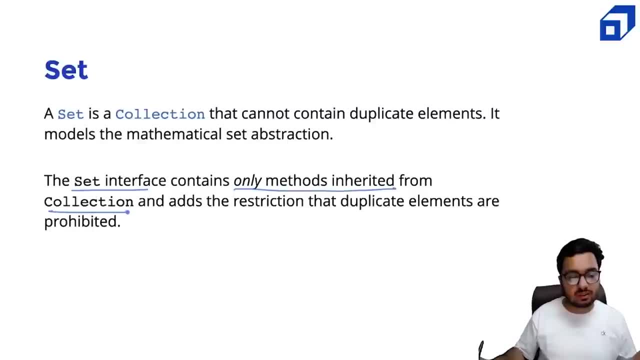 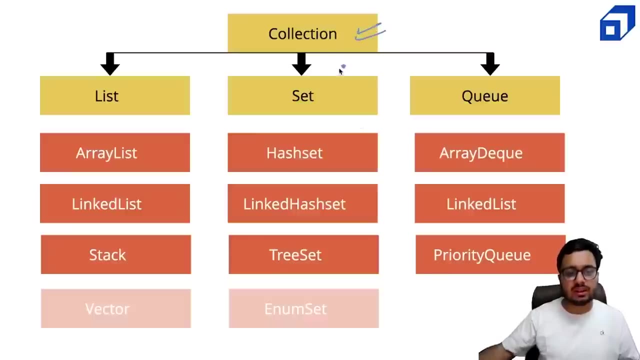 it contains only the methods inherited from the collection. that means there are no additional methods inside the set interface. all the methods are inherited from the collection. but it adds the restriction that the duplicate elements are prohibited. everything, all the methods which are there in collection, right the same methods are. 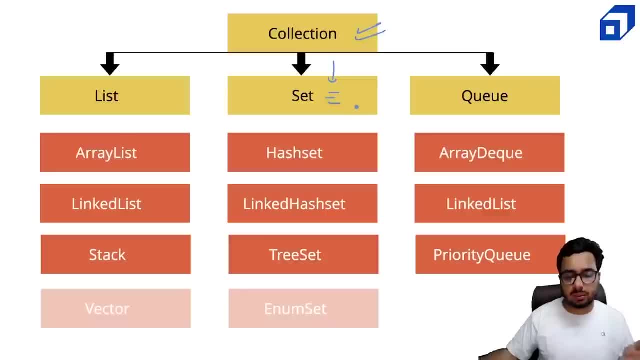 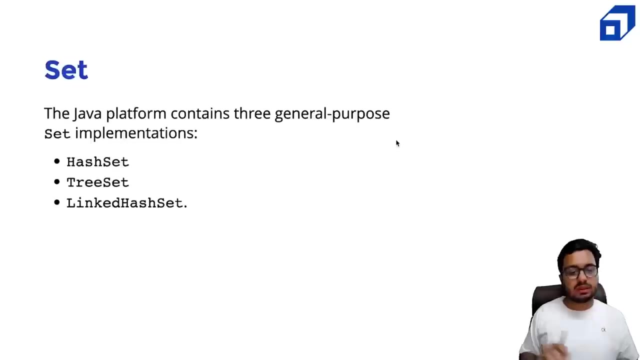 there in set, except the condition that duplicate elements cannot be present. there are three classes in java that provide the implementation of set: there is hash set, there is link set, linked hash set, and there is tree set. so let us try to understand the differences between the three implement. so, as i 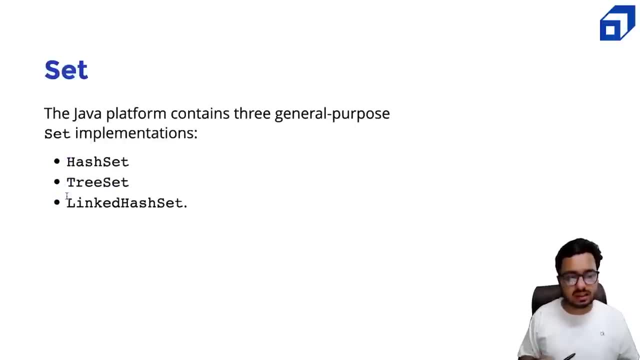 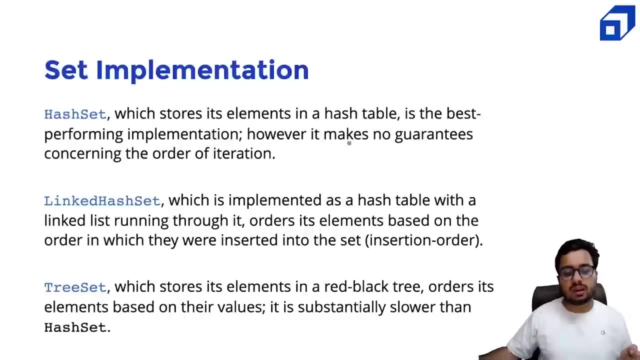 discussed. there is hash set, tree set and linked hash set. so hash set stores the elements inside a hash table. it is the best performing implementation. however, it makes no guarantees regarding the order of iteration. you say, okay, i inserted 10, 20, 15, 18 inside the set and if you start, 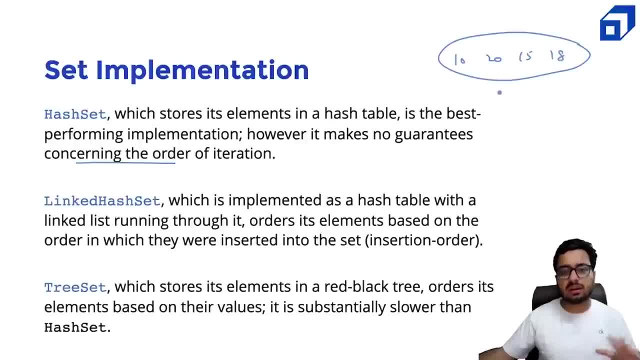 iterating over the elements. you are not guaranteed to get any order. you might get 20, 18, 10 and 15, so the elements will come out in any random order. so it does not ensure any kind of ordering on the hash set. the internal data structure is a hash table. 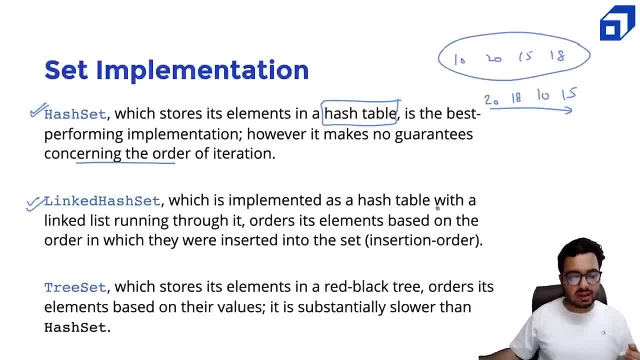 and there is a linked asset. so it is implemented again as a hash table and along with the hash table we maintain a linked list. so that means these elements are going inside the hash table, but also we chain them together so that we are able to maintain the order of insertion. 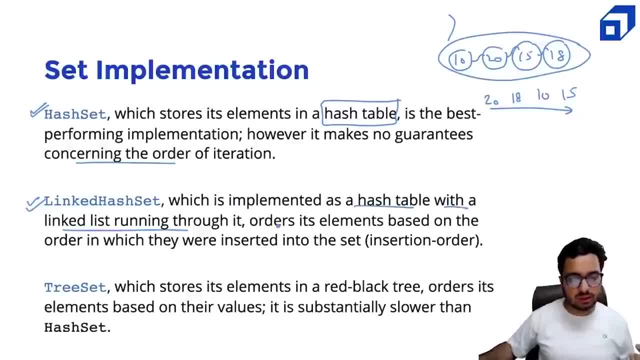 so it has implemented a hash table with a linked list running through it. it combines the features of hash table and a linked list and orders its elements based upon the order in which they were inserted. so, basically, it maintains the insertion order. okay, so it's going to give you the 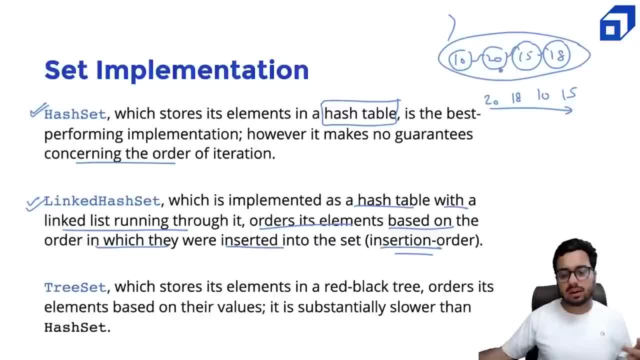 features of the hash set, along with the ordering that is maintained. there is one more thing that is called tree set. it stores elements in a red black tree. so red black tree is a self balancing binary search tree, which is a height balance tree, and it orders its elements based upon their values. 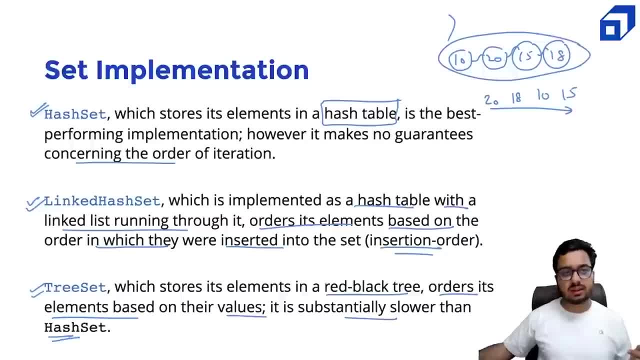 and it is subsequently slower than the hash set. basically, whenever we talk about BST, right, and it is a height balance BST, okay. so if you have to do an insertion, searching inside in such a tree where the tree height is log n, so it's going to take all the methods like. 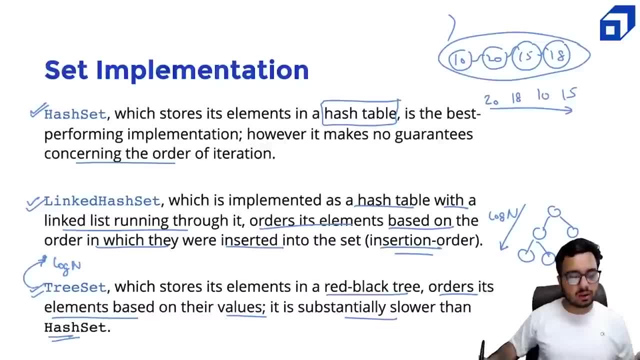 inserting data, finding data. they are going to take order of log n time inside a tree set, whereas on hash set and linked hash set the time complexity is going to be order 1 on average. basically, the advantage of tree set is it keeps your data sorted. linked hash set keeps. 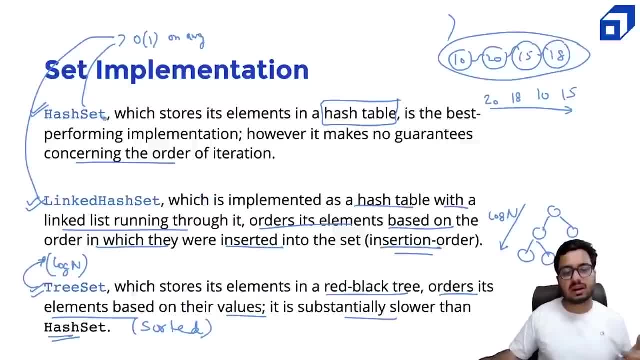 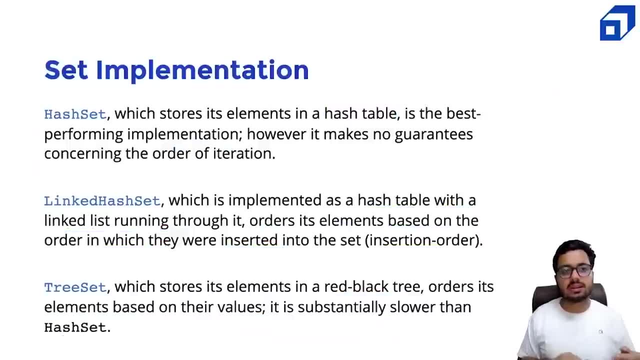 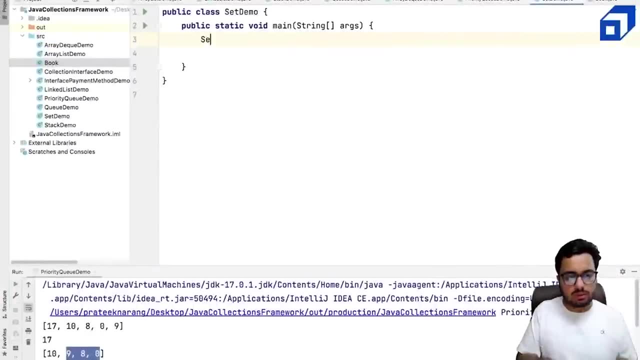 the same order as input hash set. it is the fastest and it is the, but it does not give us any guarantees on the order. so these are three different implementations of set in java. let us look at the code demo for a hash set. okay, if i want to create a? 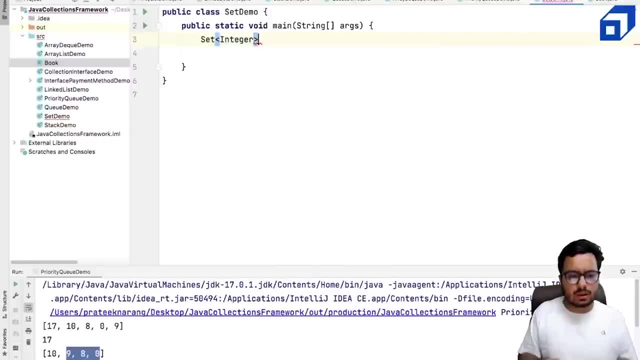 set, let's a set of integers. yes, this is equal to new hash set. right now i want to do something on this. let us import as well javautilset. import has been done. let us add few numbers into it. let's say: set dot add sorry s dot, add some. 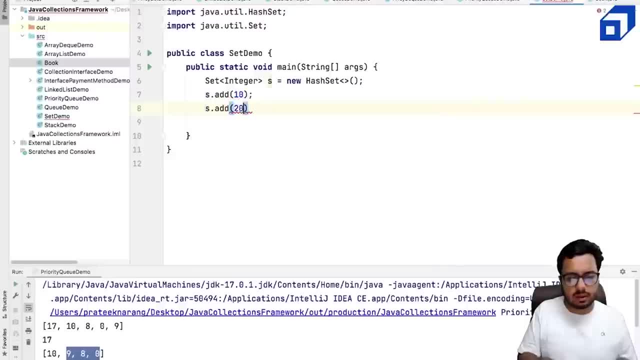 numbers. let's say 10 s dot add, 20 s dot add 18 and s dot add. let's say right and s dot add. i have added few numbers, so let me display s s out. let us run this code and see what do we get. 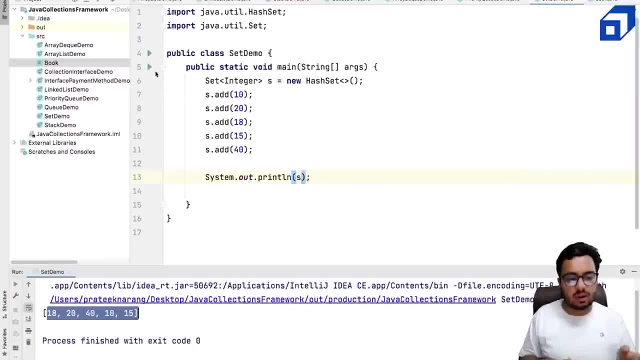 i am getting 18, 20 for 10, 10 and 15. you see the order is random, there is no fixed order: 18, 20, 40, 10, 15. it is kind of a random order if i want to add, like if i add a duplicate element once. 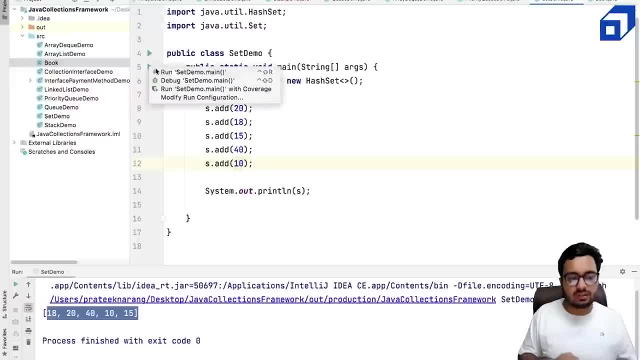 again. if i say, okay, add 10 once again, and if i run this code, you will see this: it will not store the duplicate elements. only one, 10, is stored, even if i added once again, the duplicates get filtered out. so no duplicates are allowed in the set. 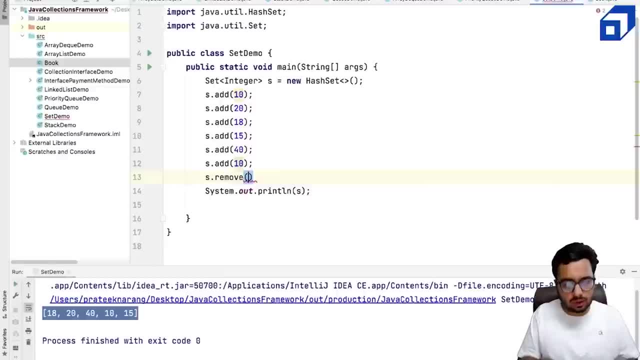 suppose i want to remove an element so i can say s dot remove 40, this will remove 40 from the set. and what is not there? and suppose if i want to check if a particular element is present or not, so if i can say s dot contains: 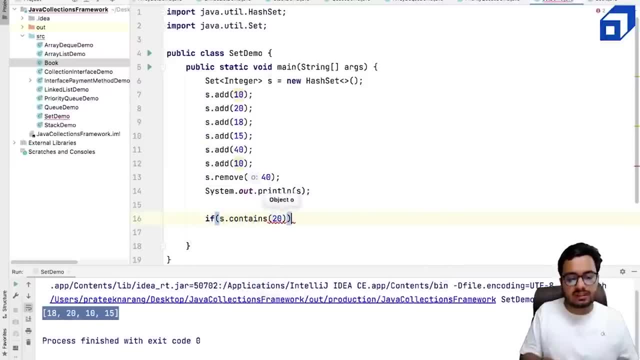 some number, 20, so you can say, yes, it is present. or i can simply say: just do s out whether 20 is present or not, so s out s dot contains. so it will give me true or false, whether this element is present or not, so i will get a true. 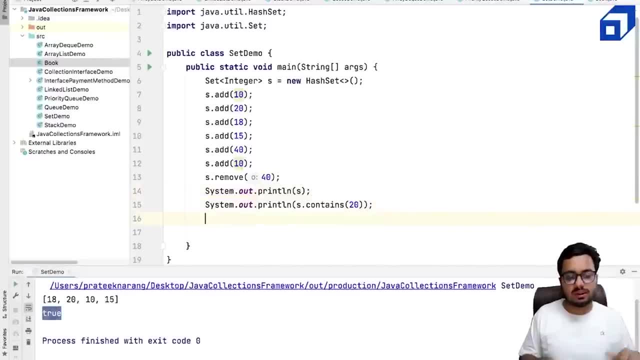 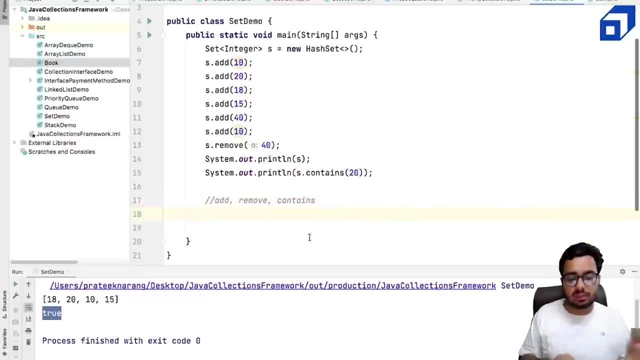 here right, so 20 is present. these are the three fundamental methods: add, remove and contains- and if you remember these are the methods. they were part of collection interface as well. we can use these methods on any, any data structure that we have seen so far. right, and all of them they inherit. 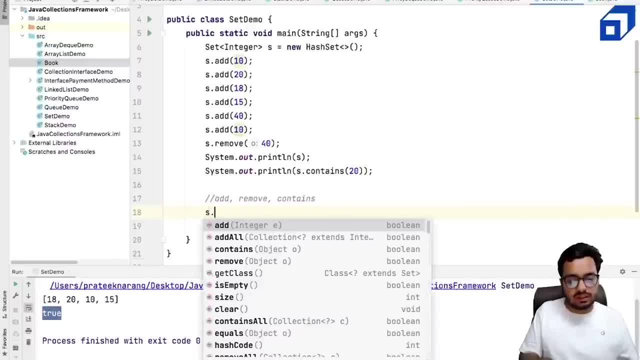 from the collection interface. there are few more methods which we have with. the collection interface is empty. we can check size, how many elements are there in the set? clear, remove all elements from the set and we will also see how do we use set with custom objects. so 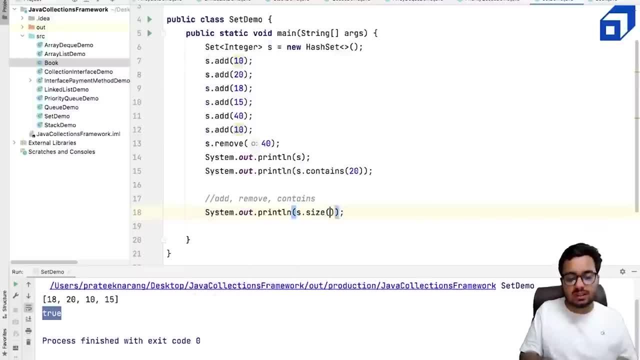 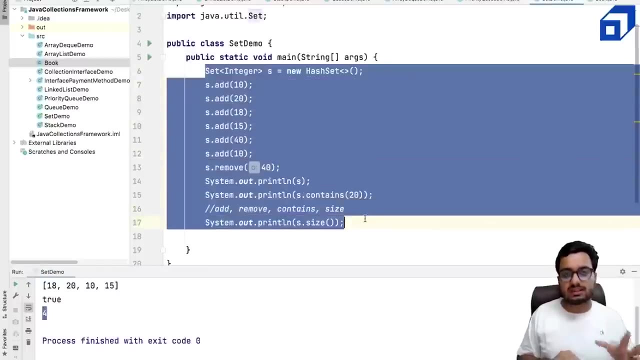 let me first show you the size method. how many elements are there in this set? so currently we have four elements. so this method will tell me. okay, there are four methods, so there are four elements inside it. now we have worked with a set of teachers. sometimes we might have to. 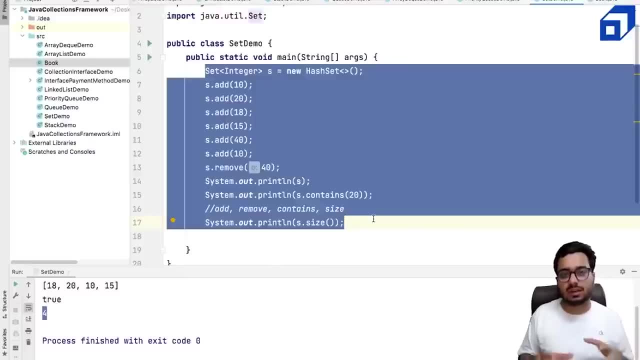 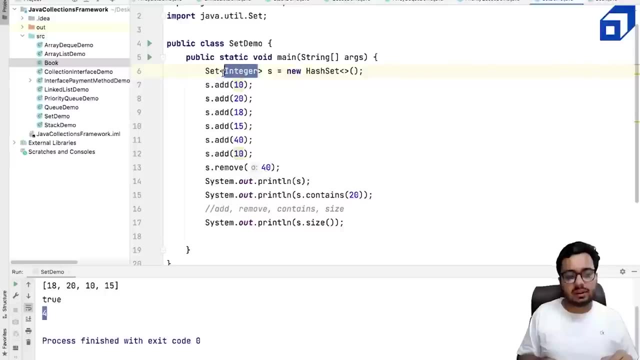 work with a set of a complex class, maybe a set of books, set of students, a set of uh payment ids or set of debit cards. right, anything, anything can come here. so data type can be anything. so let us see how do we implement set with a custom data type and what will change. 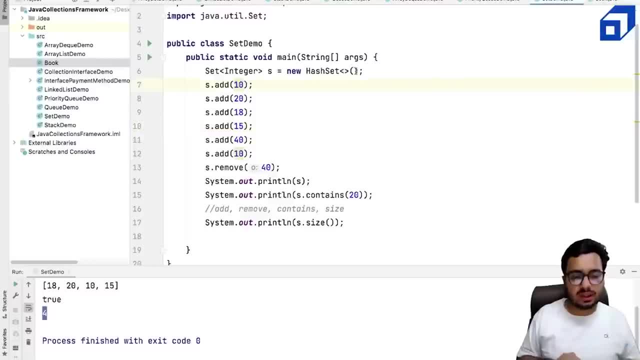 okay, before we uh discuss the custom set, there is one more thing. so we just discussed that. okay, we can use a hash set class in java, but we can also use linked hash set and we can also use preset. so i'll comment this out and i'll show you. 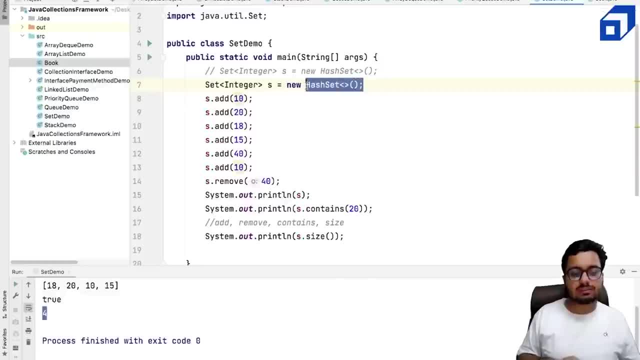 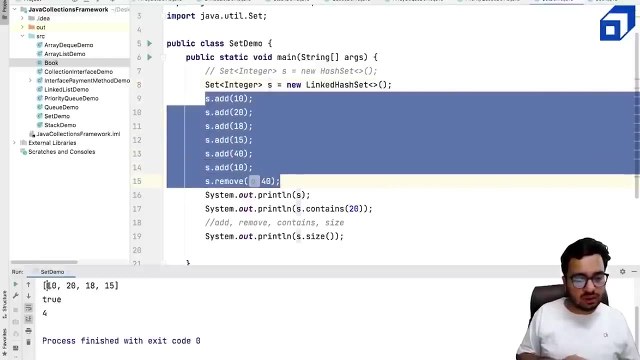 two more examples. instead of creating a asset, i can create linked i set in java and if i use this, you will see i will be able to maintain the same order as insertion in this set. if i remove 40, i will get 10, 20, 18 and 15. so this for this. 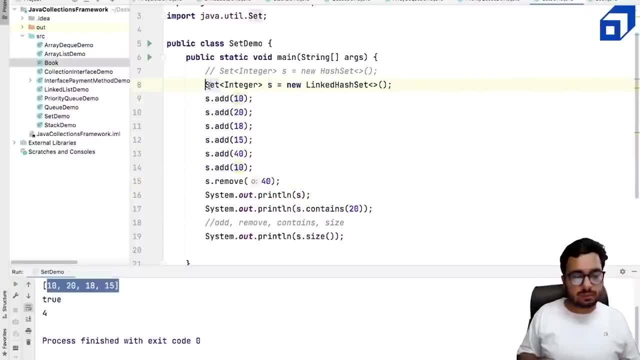 follows the order of insertion and if i use something like a tree set that is slower because it uses uh self balancing binary search trees doing add and remove, it's going to take login time on a tree set but it's going to maintain elements in a sorted order. so 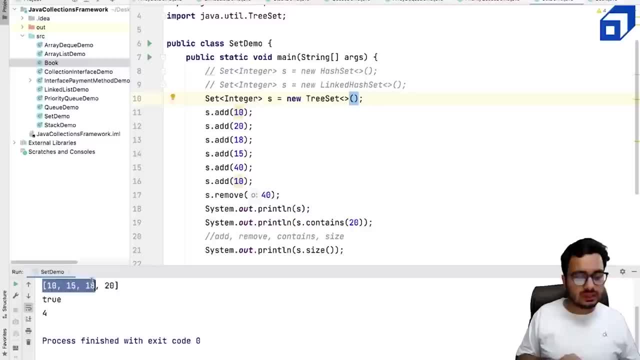 let's see that as well. now the elements are sorted in the set because we are using a tree, so i hope you are able to understand the differences between asset link set and tree set. now we will move into a set with a custom class, set of custom. 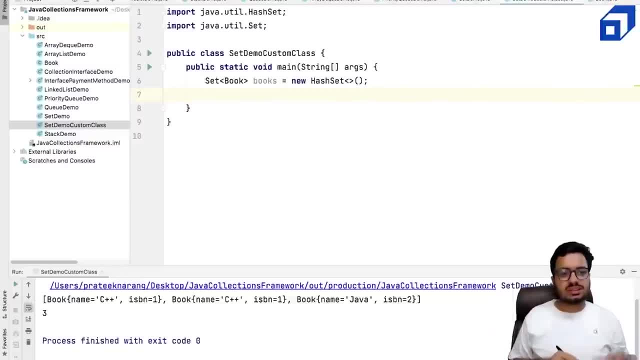 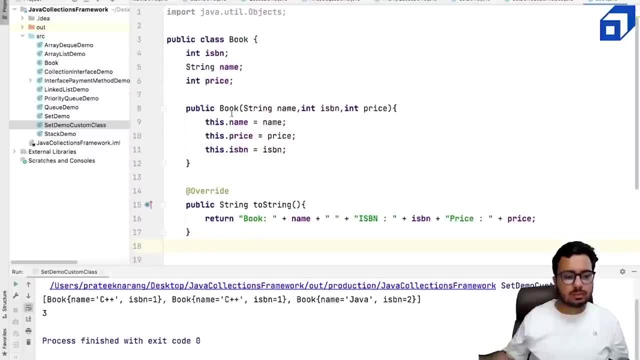 objects. let's see that. now let us discuss how do we use set with a custom class. suppose you want to create a set of books. what i have done- i have defined a book class in which book has three properties- has been name and price as the attributes of a book. 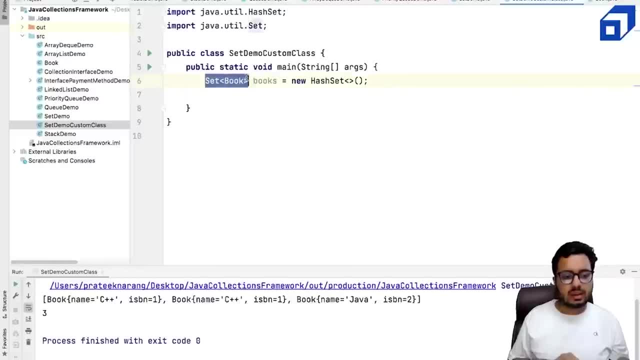 what i am doing. i want to create a set in which every item is of the type book. now let us insert few books into this hash set. i can say: books, dot add. let's say i want to create a new book. each book should have a name. 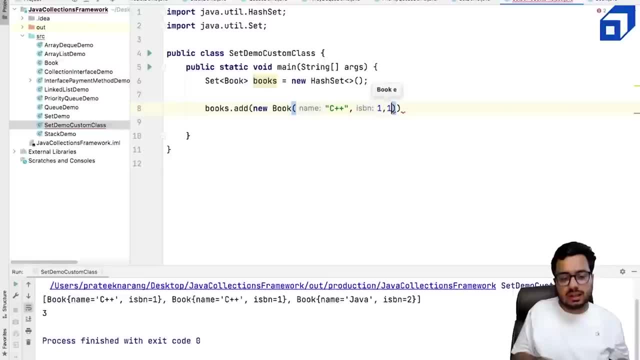 i has been, which is a unique code, and let's say the price of the book, and let me say, okay, i am going to add few more books, and here i make the name, as, let's say, java i has been is two, and let's say i change the price right now if 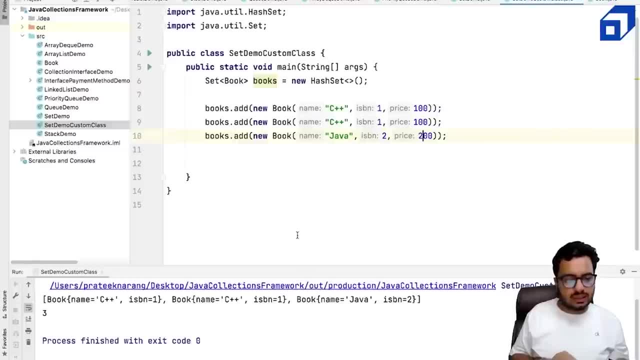 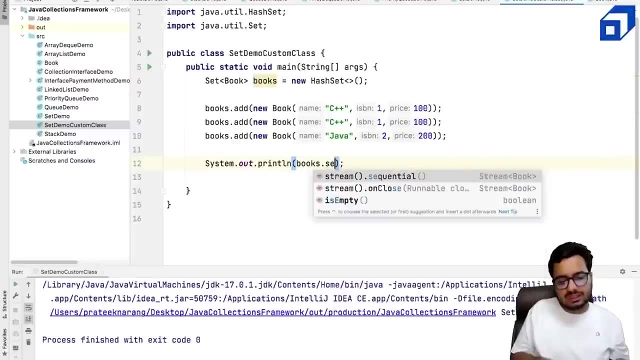 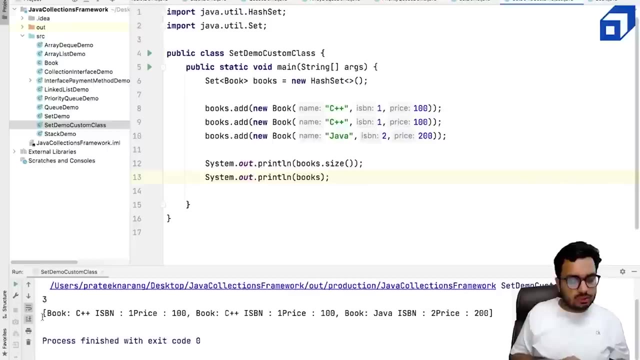 i, let's say, go and run this code, let us see how many books we will have. so s out books. dot size and let's say s out books. i also want to see what are the books that the set is storing. so i am storing three books and you can see c plus, plus. 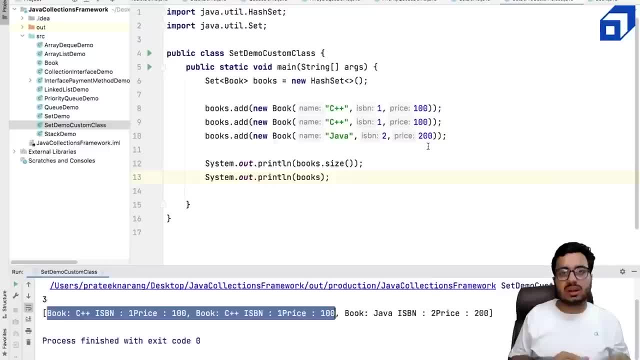 book is getting stored twice and java book is coming once now. why is this happening? why it is not able to filter out that these two books are really same. the reason is we are creating this object using new right so for the set to know whether these two objects are. 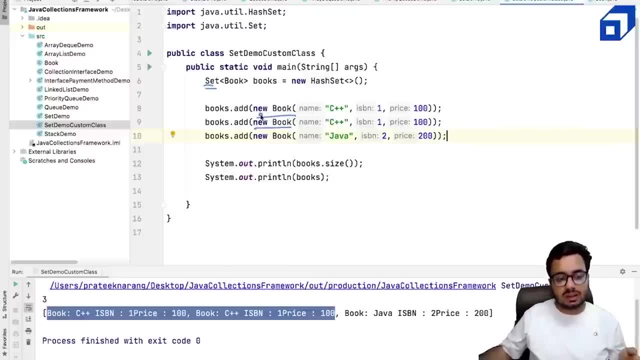 same or no? there is no way right. so we are creating a new object. set will treat that these. these are two different objects created at two different memory locations. maybe this is one zero five, six, two zero, eight zero. so for set, these two books are different because they 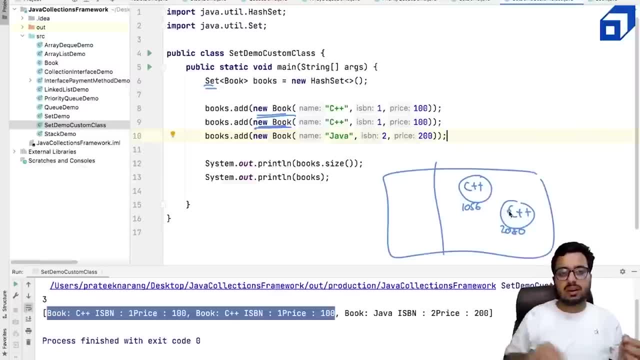 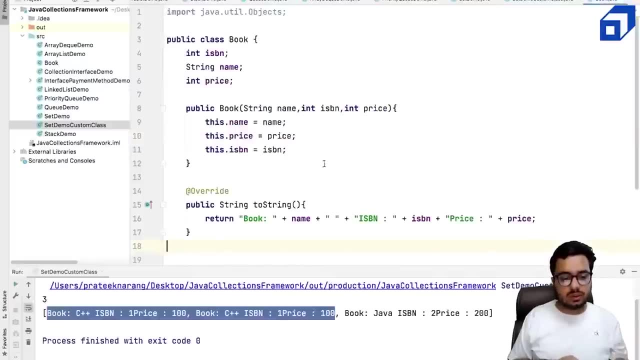 are two different objects in the memory right. we need a way to tell this set that, okay, you should consider these two objects as same. in order to do that, one thing we need to do is we need to define internally. it is using the concept of hashing right. it is going to compute. 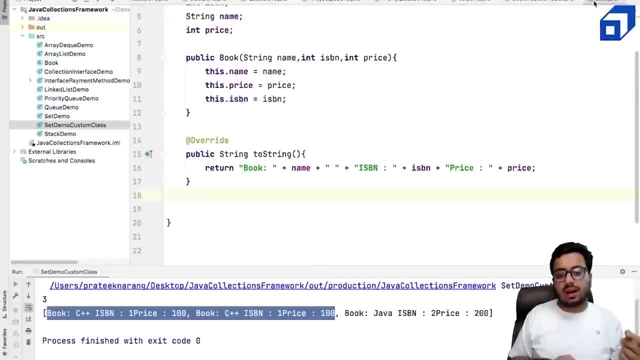 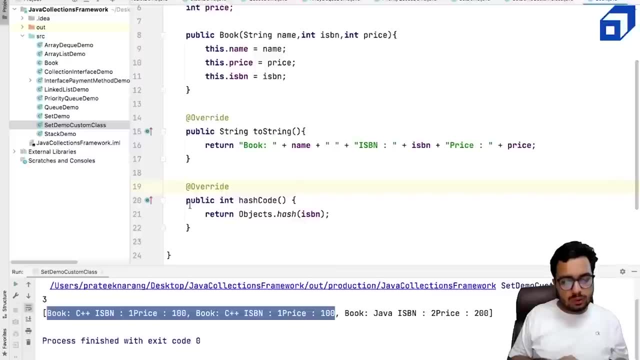 the hash code for an object. you have to tell me how do i compute the hash code. so for that, i need to uh, overwrite a method which is called as a hash code. what i'm going to do, i'm going to overwrite a method called as a hash code. in this case, 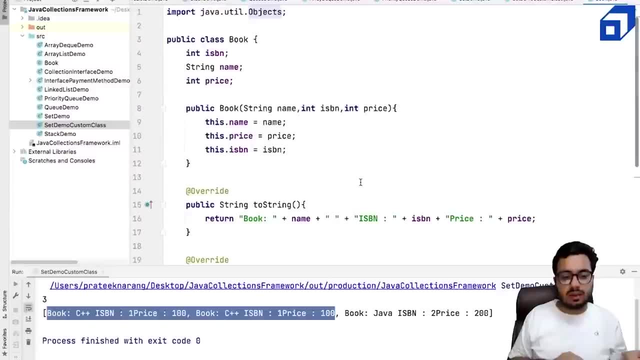 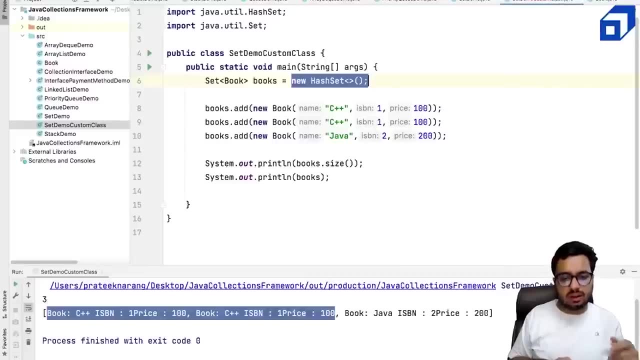 if i want to compute the hash code of a book, maybe i want to say: okay, compute it only on the basis of is been. is been is a unique number. so let me do it once again now. let's see if something changes or not. so again, it is not changing. 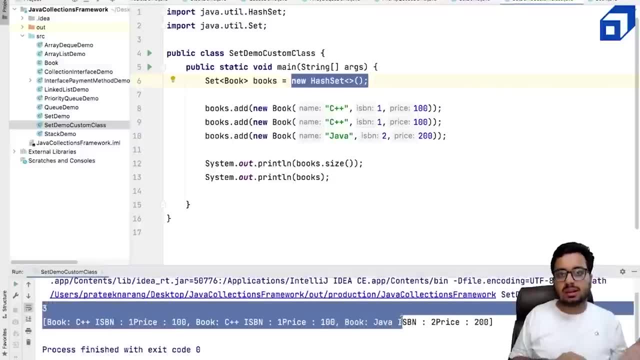 so when i'm hashing the books, although the books are getting hashed on, the basis of is been still the set does not know whether the two books are equal or not. so what happened? we, uh, computed the hash code for this book, inserted it into the set, this book. 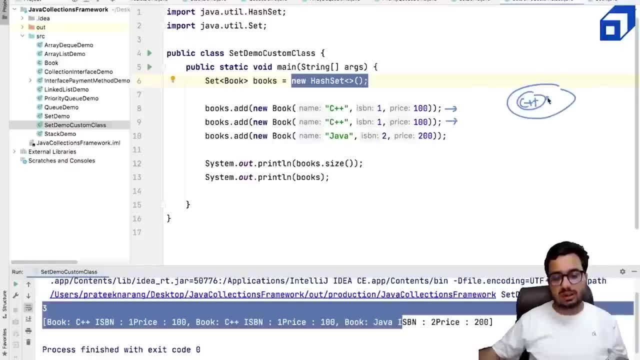 went into the set again computed a hash code for this book. it also went into the set two objects. they can have the same hash code. that is okay and uh. the thing is i need a way to tell the set consider: these two objects are equal, so maybe 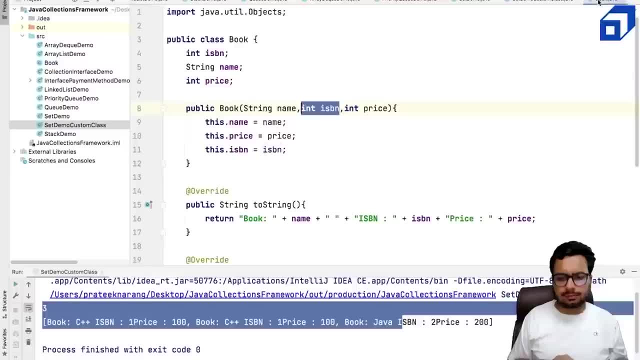 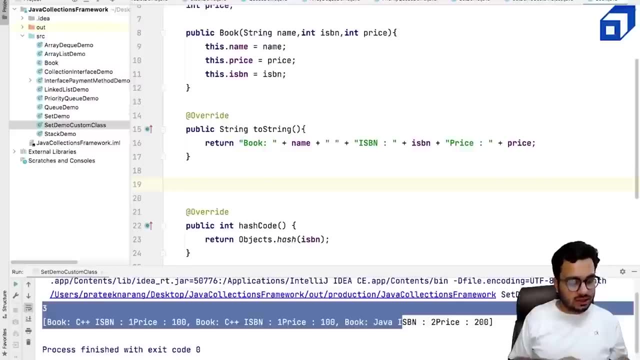 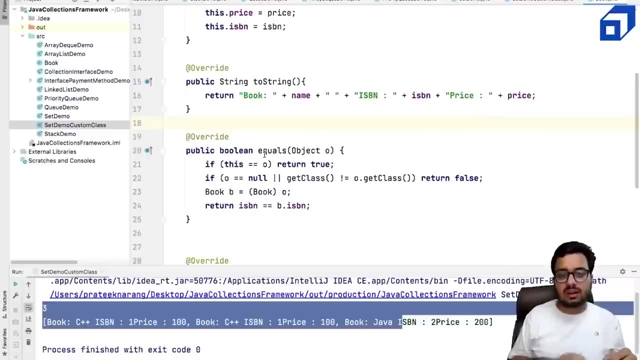 i want to say that, uh, so i need to uh, provide a method that is called as equals method. okay, so let's see how do we write this method. so there is a pretty standard template to do it. so, whether two objects are equal or not, so whenever you are, 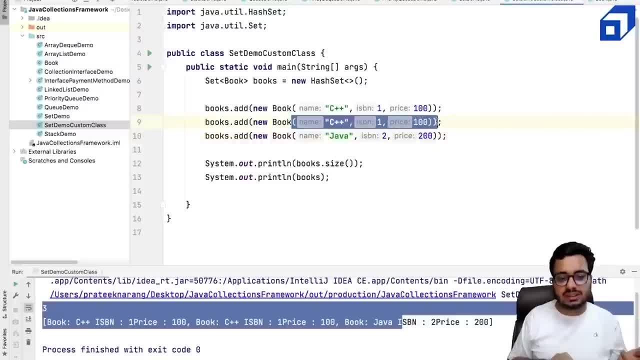 inserting a new object. let's say you are inserting this object into your headset. it's going to compare that, whether such a object is present or not. so why, at what location it's going to compare? it's going to compute the hash code and it's going to check whether we 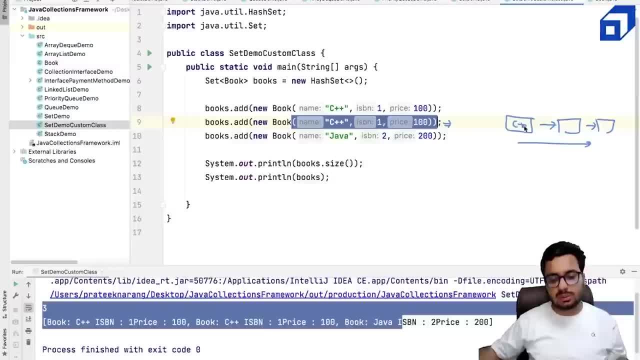 have uh, something at that location or not. so suppose c plus plus was there, some other book python was there. suppose they two had the same hash code. so it's going to compare whether these two are equal or not. whether these two are equal or not, this concept will be little more clear if you understand. 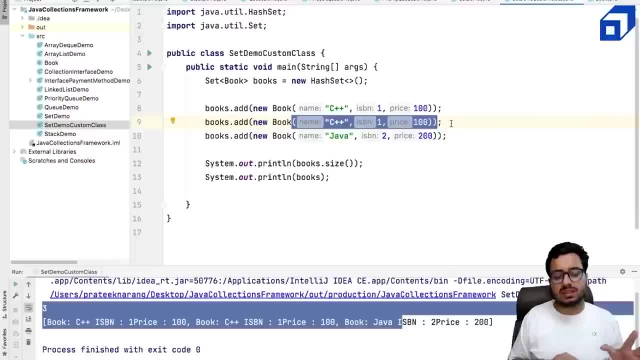 the technique of separate chaining. like different objects, they can have a same hash code if they have the same isbin or the hash function is producing the same value. for two different numbers as well, it can happen, right, but what we need to do is we need to tell that, okay, the two objects. 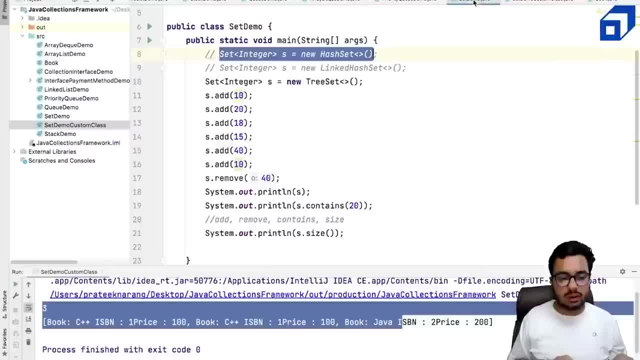 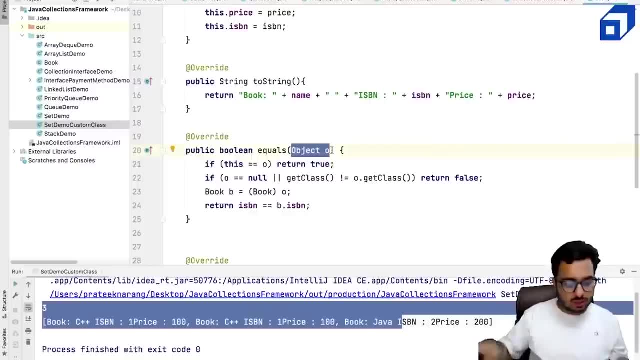 are equal if their isbn is same. so what i will do is: uh, what i have done here is i'm saying that okay, um, i'm giving you an object. so i say: okay, book b1, compare this object equal to b2. they do, these two objects are equal. 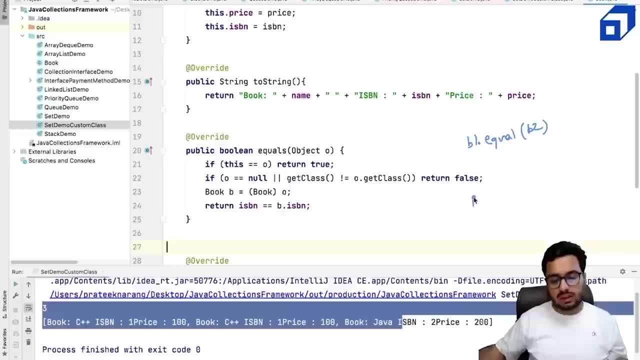 in like two, three scenarios. i'll discuss what are those scenarios. suppose i create a book- b1- which is equal to new book and i say, okay, b2 is a book which is equal to b1. so in this case, what is happening? i have just one book object. 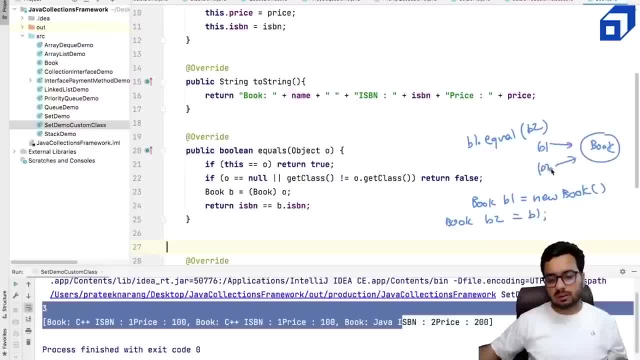 both b1 and b2. they are pointing to same right. if i make any change in b1, it will also affect in b2. so what i'm doing? that if this is equal to o, that means if the current object and the other objects they are referring to the same. 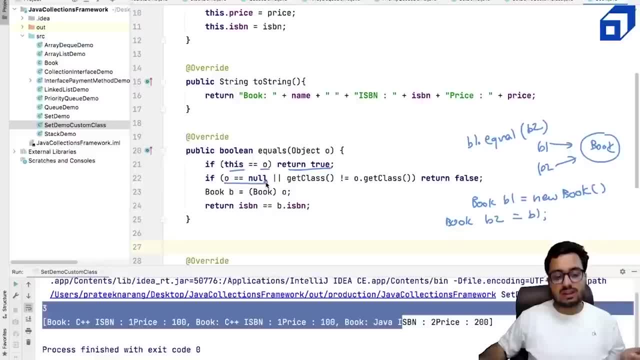 memory that means they are equal right if o is null, if one of the object is null, they cannot be equal, or if the two objects they belong to the different class. so suppose if i compare a book with a student they can never be equal. i am returning false, otherwise 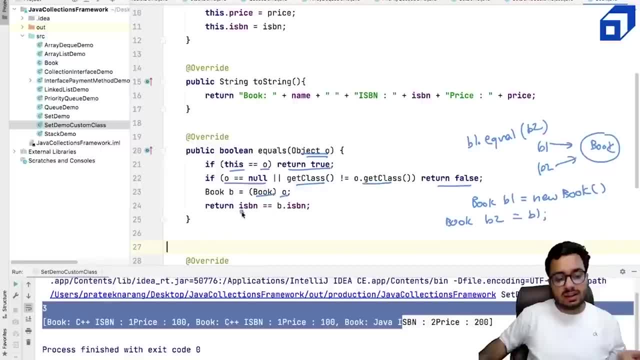 any given object. i type cast this into book loss and then i compare. that is, the isbin of my book is equal to the isbin of other book. if this is the case, consider the two book objects to be equal. if i add this, equals method, my 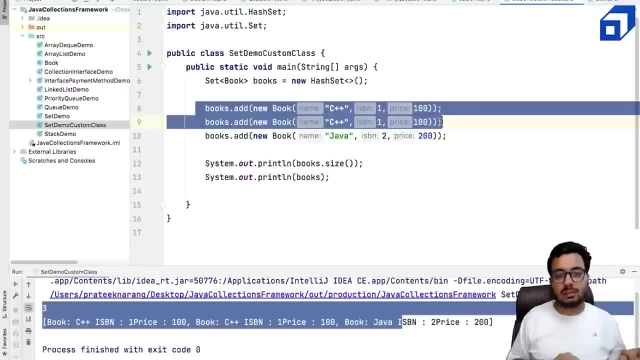 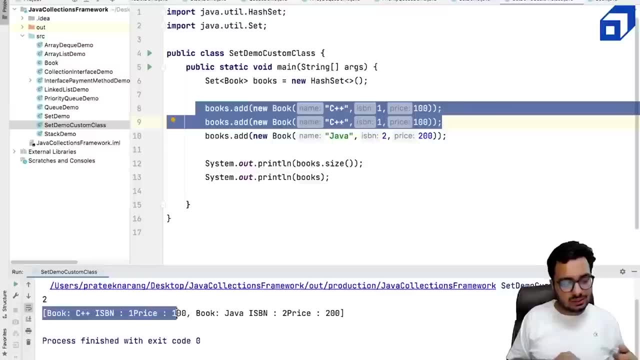 hash set will come to know that okay, these two books, they have the same isbin. i will not insert them again, even if i now look i have only two books. okay, and c++ is stored only once. now, even if i change the name of this book, i say okay. 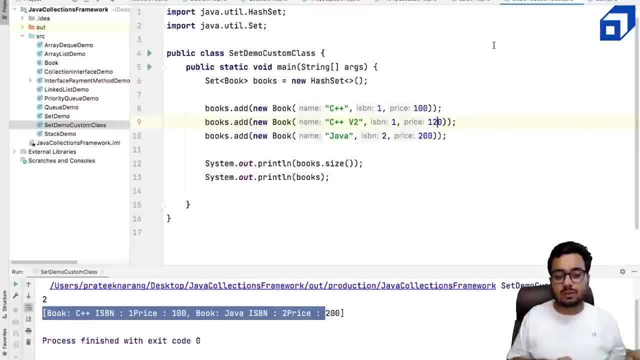 this is c++ version 2 and the price has been increased to 120. will hash set store this book? the answer is no, because it is only going to compare on the basis of isbin. if isbin is same, i will not again store this book, right, but if you want, okay. 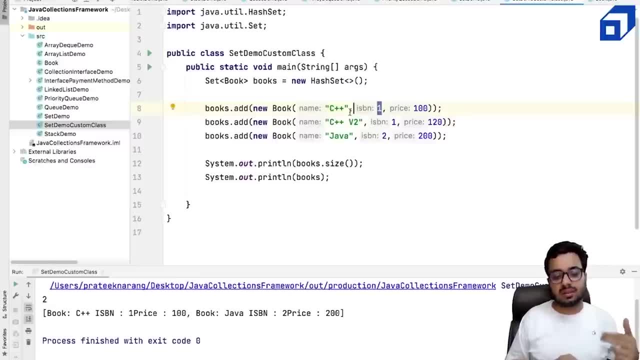 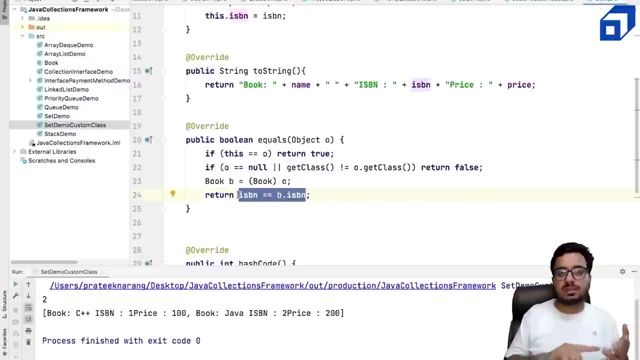 the two books are equal if they are name is same, if their price is same, if their isbin is same, then in the equals method you can have two more conditions along with the isbin that i should match, all the three parameters for the comparison. the equals method is important. 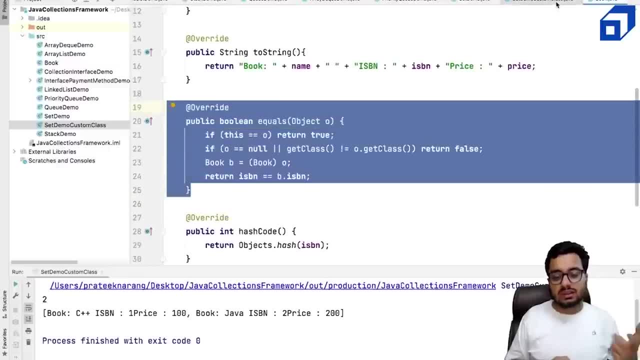 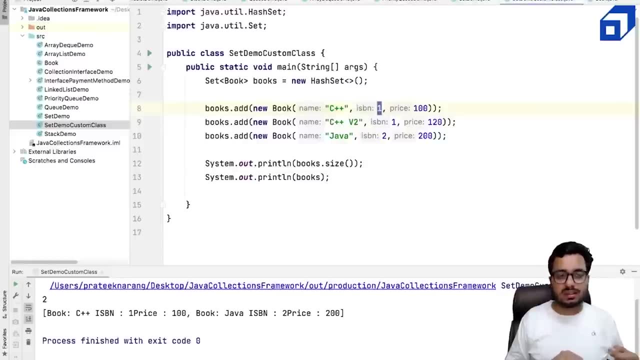 so you need to override this method to tell the set in what scenario you should consider two objects as equal. i hope you are getting it and that's all for this implement. let us talk about the final data structure. that is a map. a map contains values on the basis of. 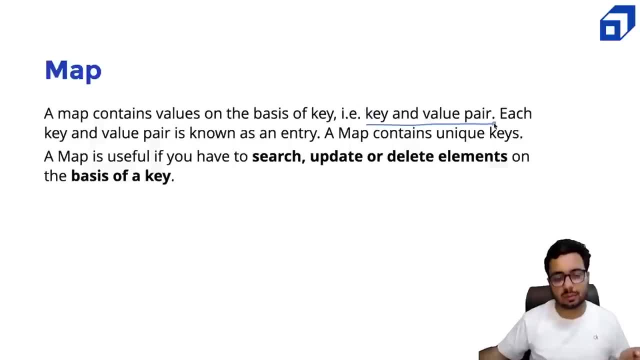 a key. that means it contains information in the form of key value pairs, just like a restaurant menu. whenever you go to a restaurant, you say, okay, i want to have a burger, and you immediately get to know: the burger is 50. i want to have a pizza? the pizza is. 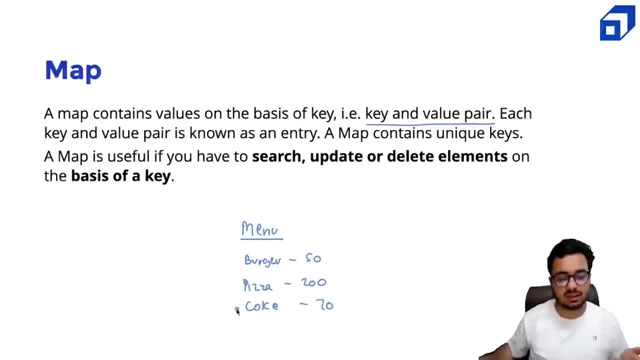 200. i want to have a coke. the coke is, let's say, 70. there is a key, there is a value associated. a map contains unique keys. that means i cannot have a burger twice in my menu. okay, a map is useful if you have to search. 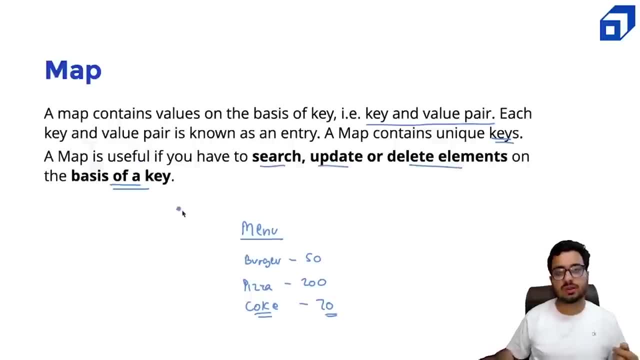 update or delete elements on the basis of key. so we do not ask, okay, what item is after burger or what item is coming before pizza. the ordering is not that important to us. what is important that, given a key, what is the value associated with that item? and i want. 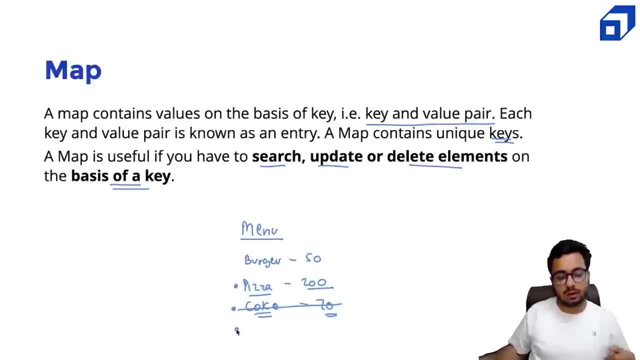 to: okay, coke is out of stock, so i want to delete this key value pair, or something new has come up. i want to insert that key value pair for operations like these. map is a very good, useful, powerful data structure and most of these operations they run in order. 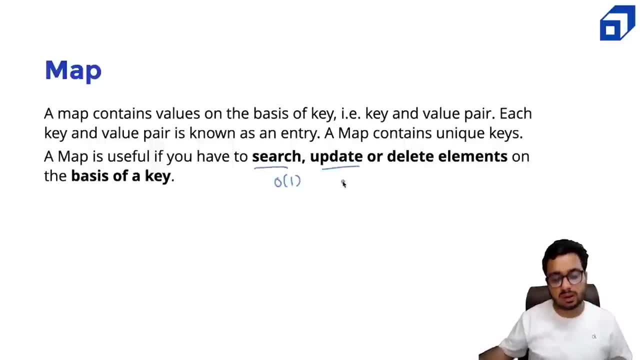 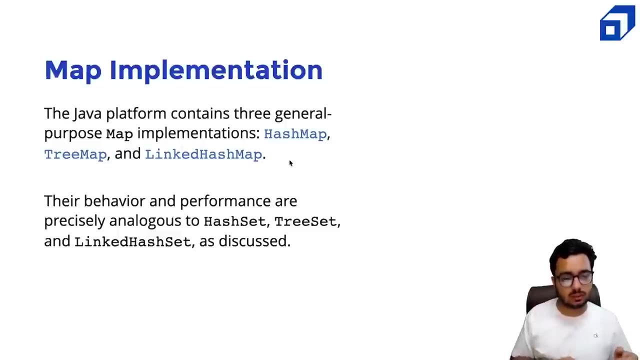 one on average. so search is order one on average, update is order one on average, delete is order one on average. so very powerful data structure. now let us talk bit more about map. java platform contains three general purpose implementations. one is your hash map, another is your tree map. 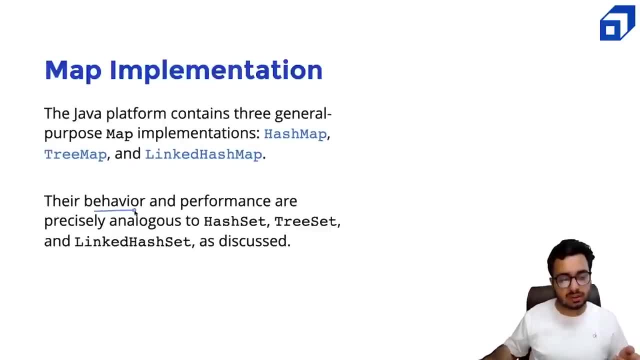 another is your linked hash map. so the behavior and the performance is same as the way hash set, tree set and link set work right. so hash map internally uses a hash table. it's the technique called separate chaining that is used to implement a hash map. so to understand hash map, 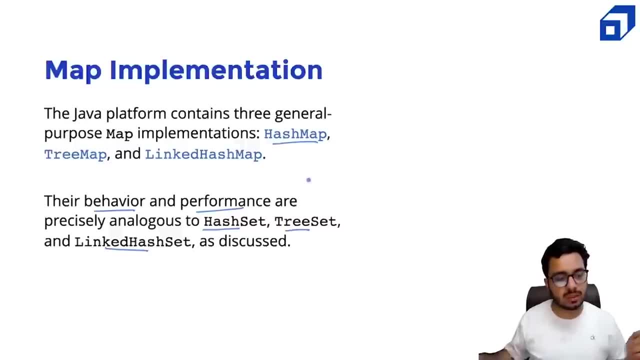 we'll do a separate video where we'll dive into the internals of a hash map. tree map is like a self balancing binary search tree and, linked hash map is your hash table and it also maintains a linked list of the elements in which, like, it chains the elements through the linked list as well. 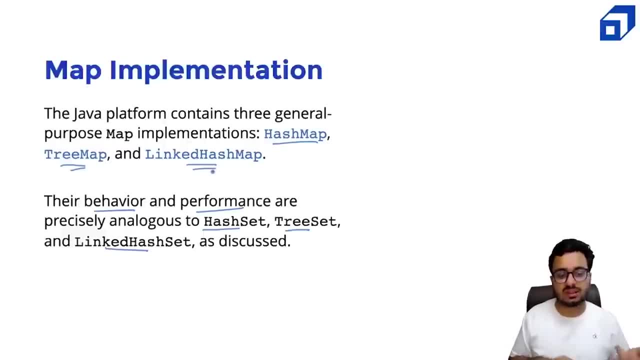 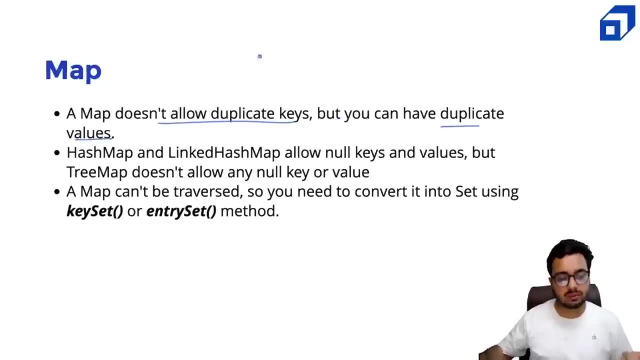 in the order in which they were inserted. so it's more complex than a hash map. map does not allow duplicate keys, just like a hash set. we cannot have duplicate elements, but we can have duplicate values. for example, burger can cost 50, noodles can also cost 50. the value can be. 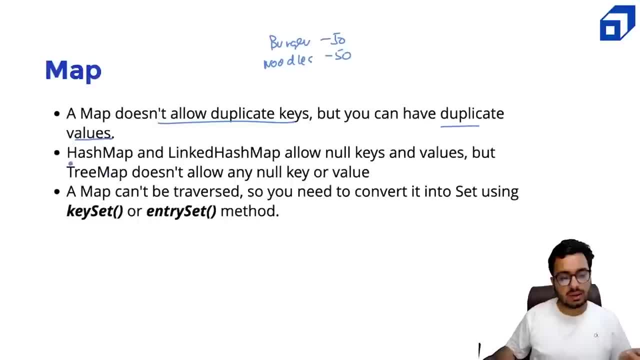 duplicated but the key must be different. right hash map and linked hash map. they allow null keys and values, but tree map does not allow null key or a value. right tree map you cannot store a null key. map cannot be traversed so you cannot directly iterate on the map, so you need to convert. 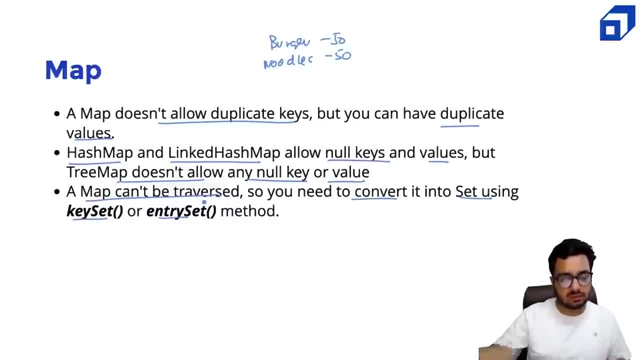 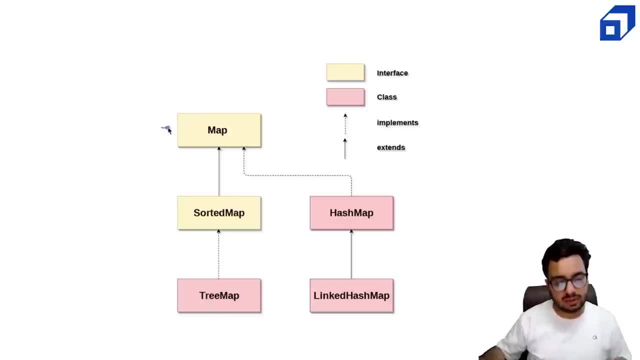 it into set using key set or entry. this we will look into the code demo. talking bit more about, uh, the hierarchy in java, there is a map interface, okay, and hash map is a implementation for the map interface. there is a linked hash map which builds on the top of 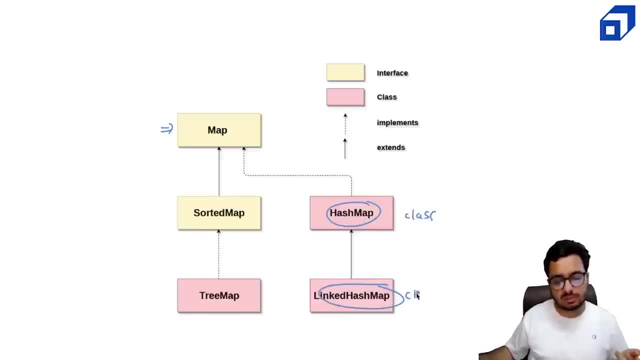 your hash map class right. hash map is a class linked. hash map is also a class. tree map is a class that implements your sorted map interface. sorted map interface is again in a child interface of map right it. it kind of extends that. here. ordering is important. you get the keys in a sorted 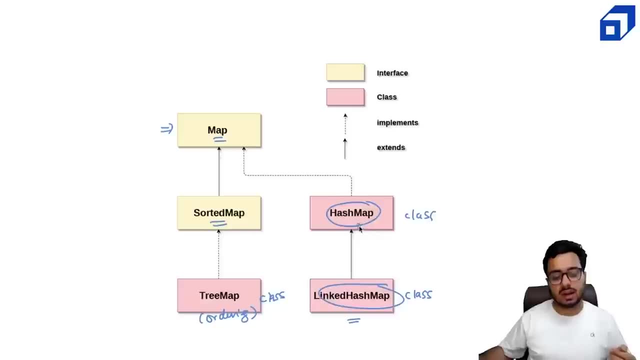 order: here you get keys in the order in which they were inserted and hash map. it is the fastest. here you don't get any ordering on the key. this is the difference between the implementation. also, the operations are order one here on average operations on tree map they are order of log. 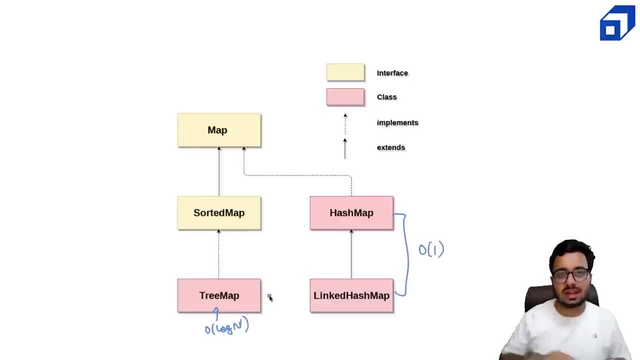 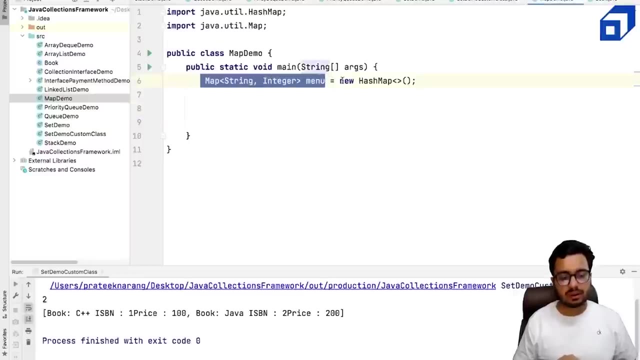 n on average. why? because it is using a self balancing binary search tree. okay, so here i have implemented a map object by using the hash map class right. i have created a map called as menu and i am going to add certain items. i can say menu, dot add. let's say: 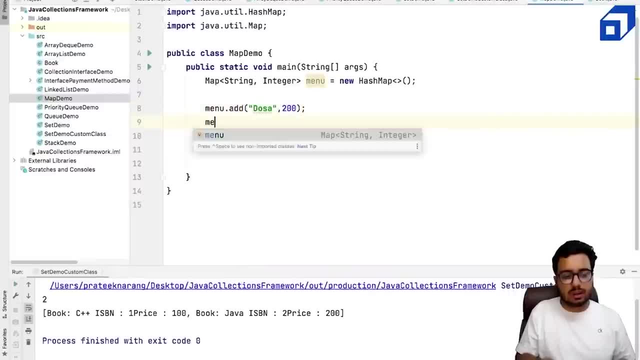 the item is dosa and the price is 200. menu dot add. let's say the item is burger, the price is 50. we are getting a error here, so the method is called, as put, hash map. we don't have the add method because it does not. 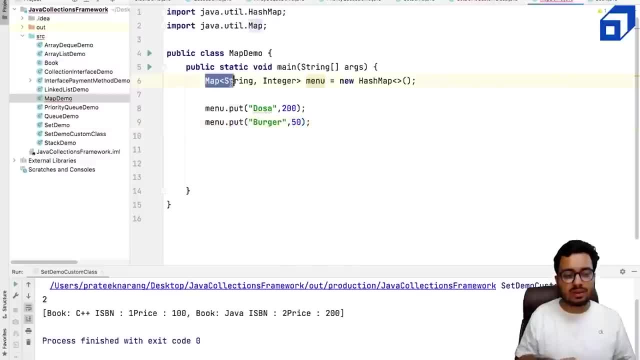 inherit the collection interface. okay, i told you, map is separate from um. map interface is not? uh, it's not a child interface for of collections interface. so it has method called put. it does not have a method called add. i can put key value pairs like this. i can say menu: 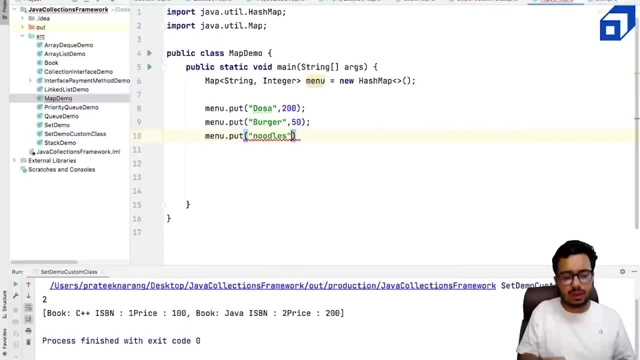 dot, put noodles and maybe some price, and here i can say: s out, show me the menu, let's see if we get something here. so let's see, what do we get if i run this code. in the meanwhile i will write down some more methods. i can see there are. i can see. 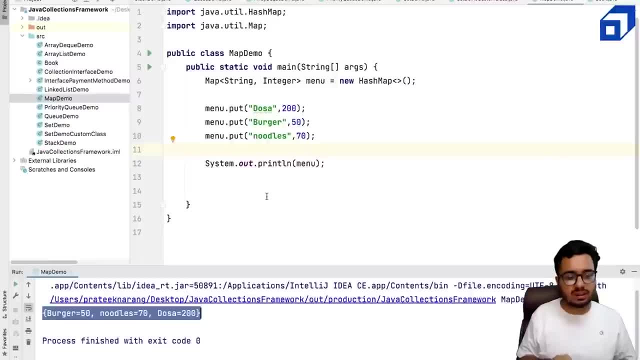 the uh list of key value pairs that are stored inside this map. i can also remove something. i can say menu dot remove. i give burger. i just need to give the key. burger will get removed from the map. i can also search that if my menu contains some item. 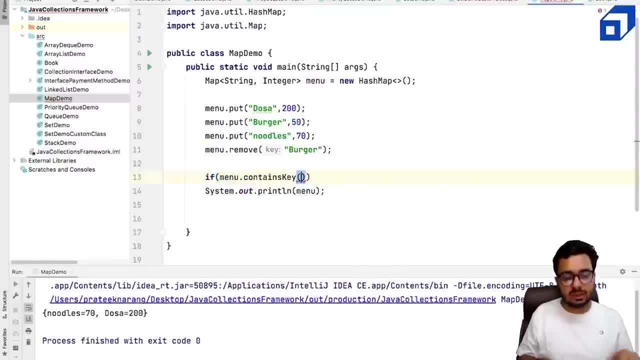 like dosa, i can say contains key. this is the method and i can check whether it is present so you can say: yes, out uh s out dosa found, so you can do this as well. but after removing burger, we have two items, noodles and dosa, in our map. 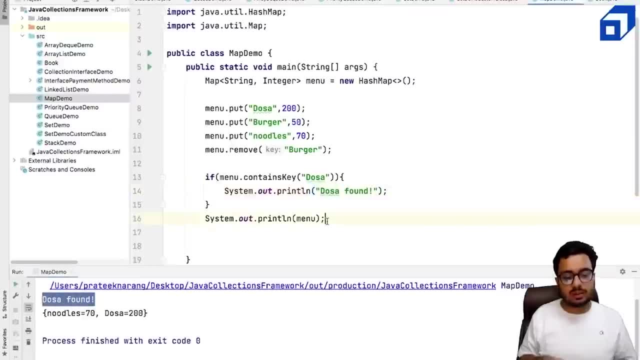 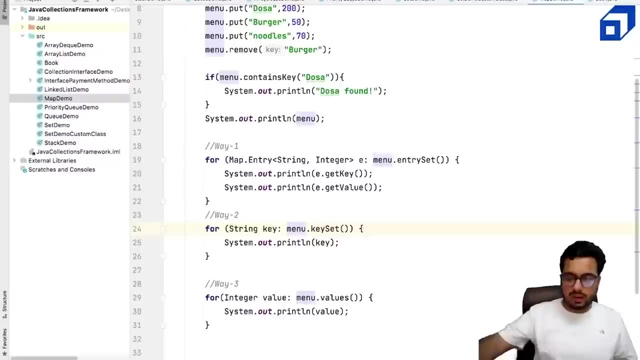 right, so dosa is there. so dosa found it's get. it gets printed. now let us also talk about how we can iterate on the map. there are multiple ways, right? so what we can do is: okay, i just written the three ways to iterate so that we can save some time. 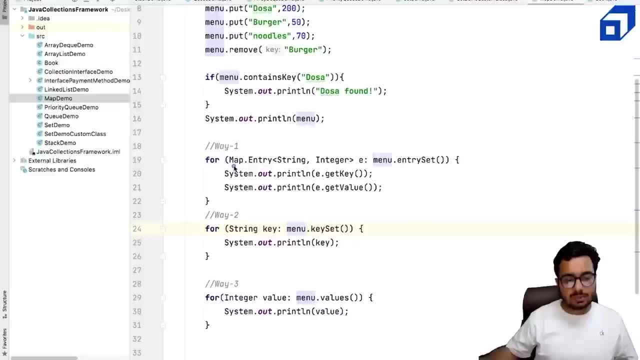 so the way one is i can do: i can create an object of the type map dot entry and this object is uh iterating over uh all. so map menu dot entries. it is a method that gives me the list of key value pairs, where each key value pair is. 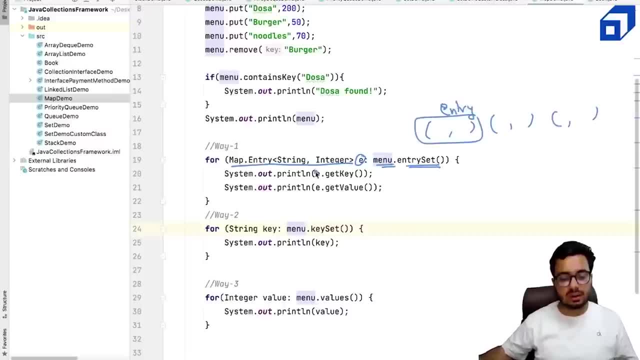 considered as a entry, right? i'm saying, okay, give me all the entries and, given any entry, i want to get the key and i want to get the value. so that is one way. so you are printing the first entry, the second entry and then the third entry. that is one way. 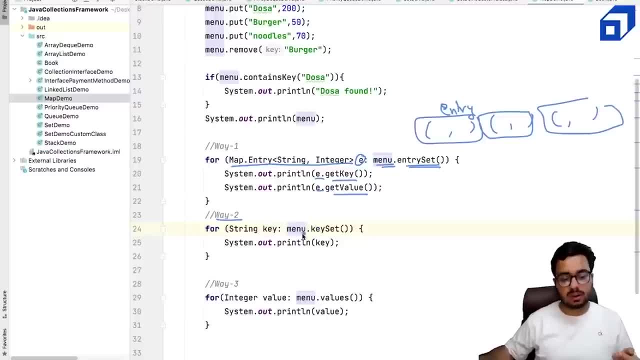 another way is, if you want to just get the keys of the map, you can say: okay, menu dot key set, so it will give me all the keys, like dosa, burger noodles, and you are iterating over these keys, those keys are strings. then you can say: okay, i want to iterate. 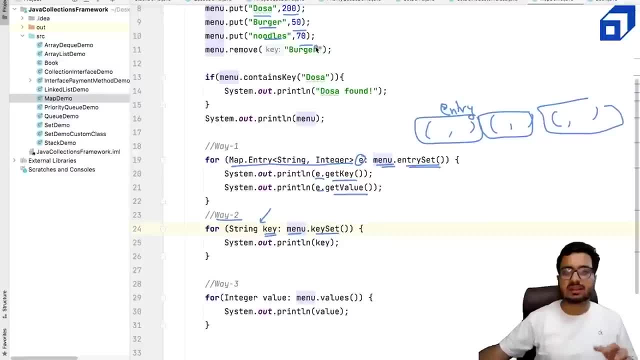 over the values that are 250- 70. i just want to iterate over these values so you can call the method called menu dot values and it will give you a set of values and you can iterate over this set using a for each loop and for every value. you can print it. 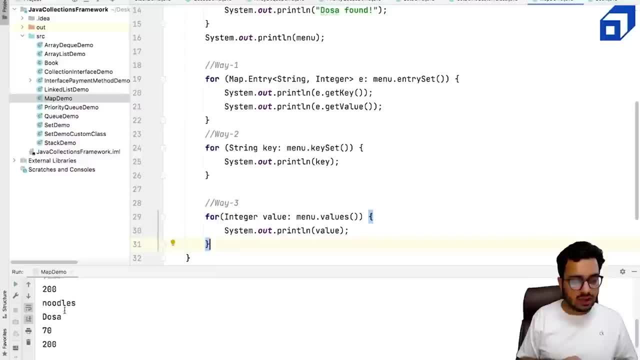 i'll just run this code and show you the output. you can see, i'm able to iterate over the keys, i'm able to iterate over the values and i'm also able to iterate over key value pairs. right, so this is coming from this loop and apart from it, there are some more. 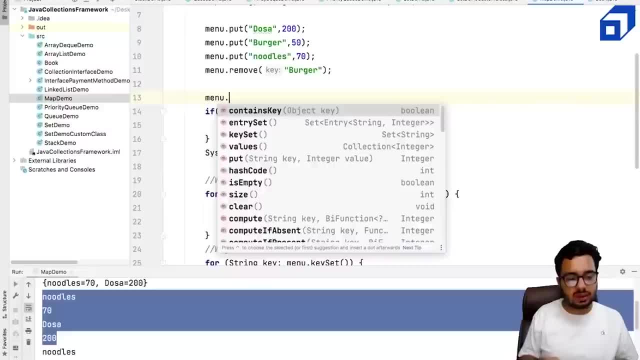 functions which can come handy. so you can, i would suggest and try those methods. is empty, whether the map is empty or not, size how many elements we have here. clear out everything in the map, right? this is clear. method is helpful if you are working with multiple test cases. 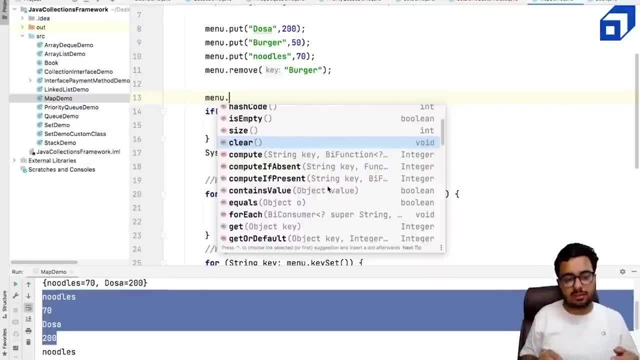 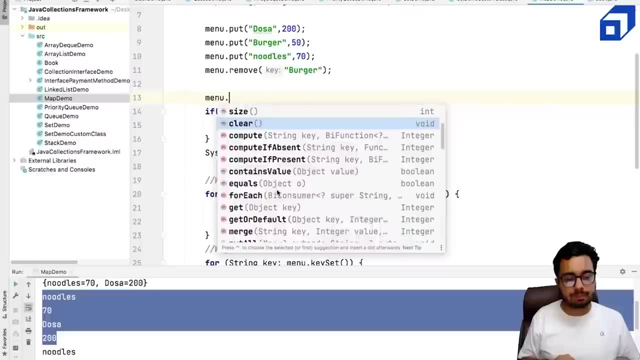 every time you have to load new items and discard the previous items from the hash map. instead of destroying the object and creating a new object, it's better to clear out everything from the previous map. so then there is get or default. if the key is found, you want to return. 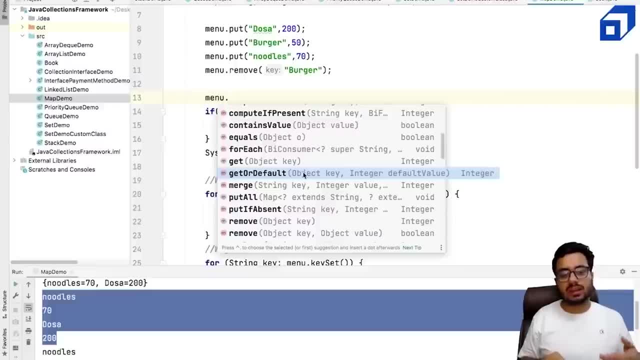 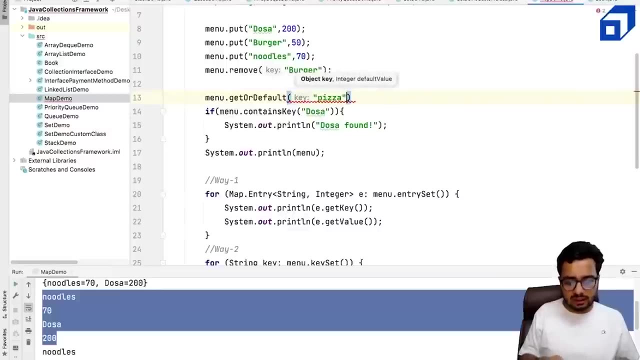 some value, you want to return the value. or if the key is not present, you want to return some default value. this is something you can use. so, for example, i can say menu dot get uh. let's say uh, pizza, so pizza. have not inserted if the pizza. 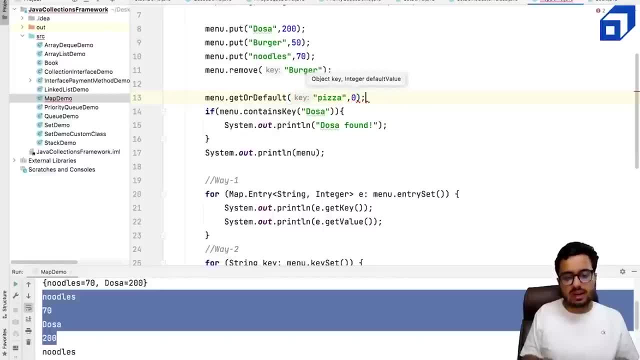 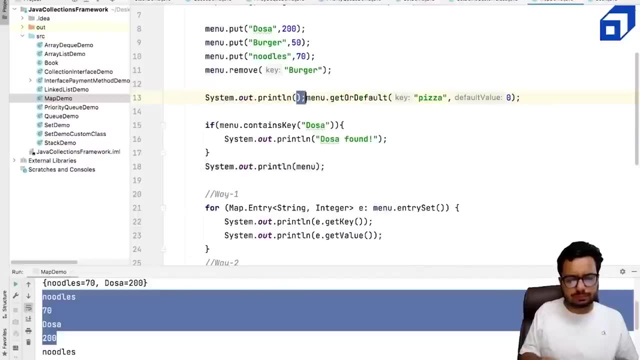 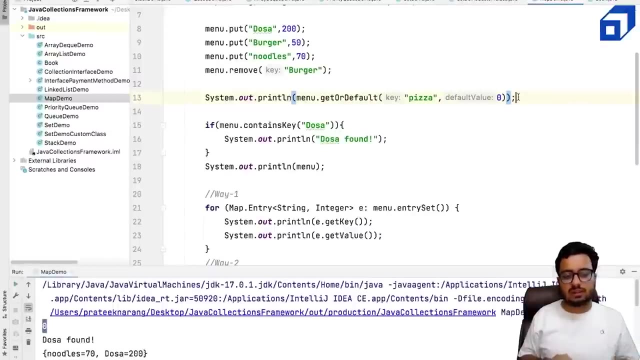 is not there. i can say: the default value is, let's say, zero. that means um, in this case, i will get an answer: that is zero, right? press out this value, right, what i'm getting? i'm getting zero. that means visa is not present. the default value 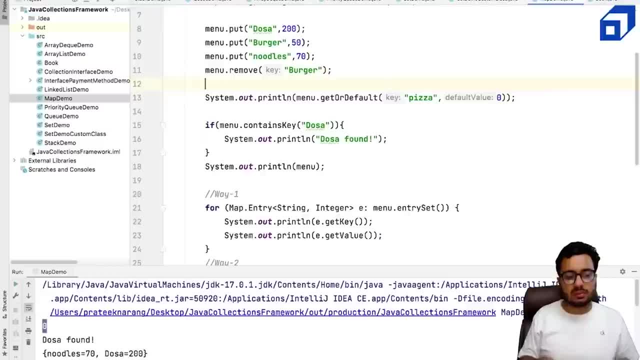 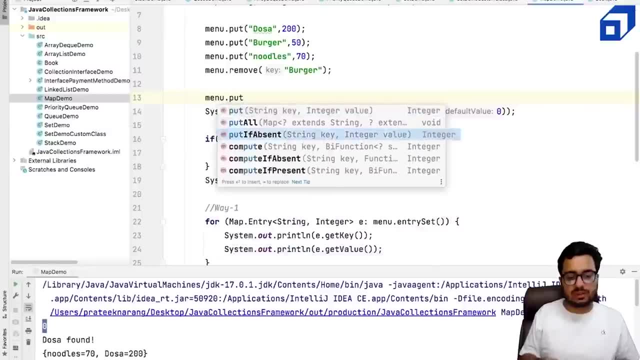 if the item is not present, i think the default value for that item is zero. i can also say: uh, i want to put pizza if it is not there, so menu dot put. if absent, i can say: okay, it will first check if the item is not there. if pizza is not there, 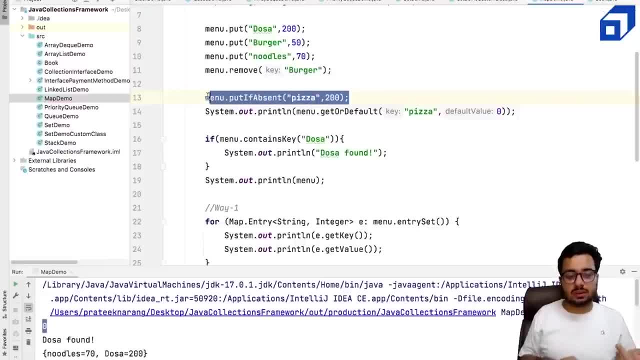 put pizza inside the map and put the value of pizza as 200. if i go and run this now, it will first insert pizza because it's not there. so it's basically using the put method with the condition and now, if, if i inquire about, give me the price. 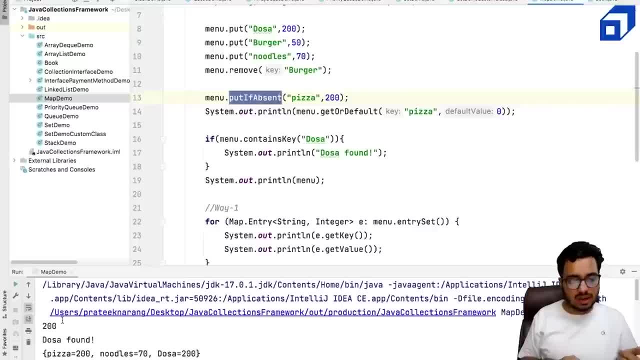 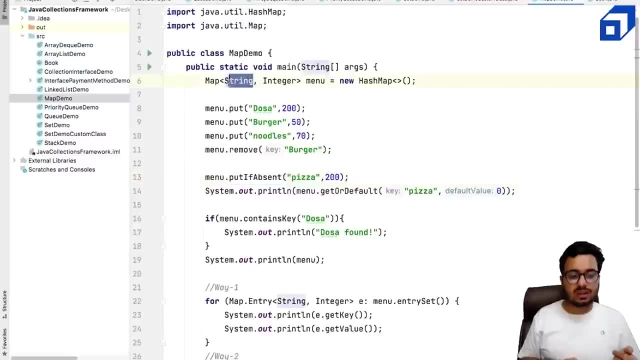 of pizza. now the pizza is present because we have added it and i'm getting the pizza price. as that's all for map, right and now? what you can do is you can also have a custom class here. you can also have something more complex here, for example: list of integers. 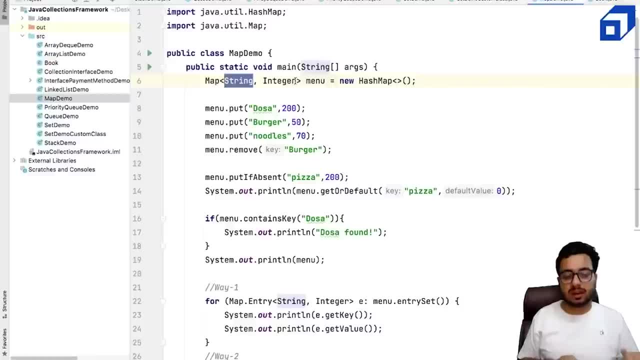 list of books. key can be of any type, value can be of any type, but if you are using a custom key, again you will have to overwrite your hash code method and the equals method, just we did in the case of hash set as well. one more thing we can. 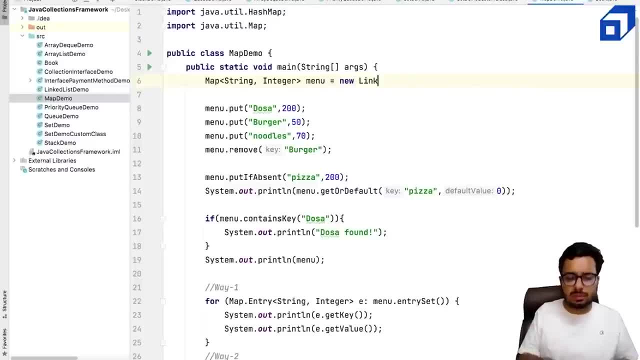 do is, if you um want to replace this with a linked hash map, you can do that. everything will remain same and your ordering will also be maintained. and you can also replace it with a tree map if you want. everything will remain same, except the internal structure will be now. 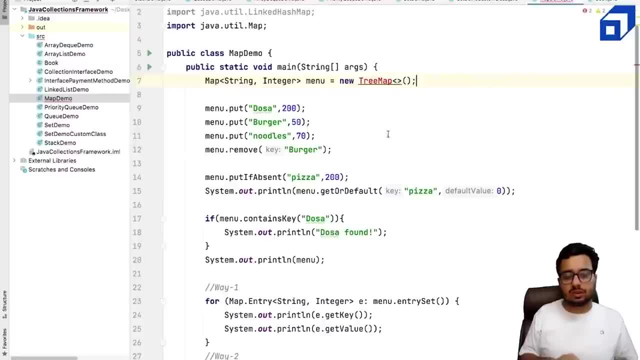 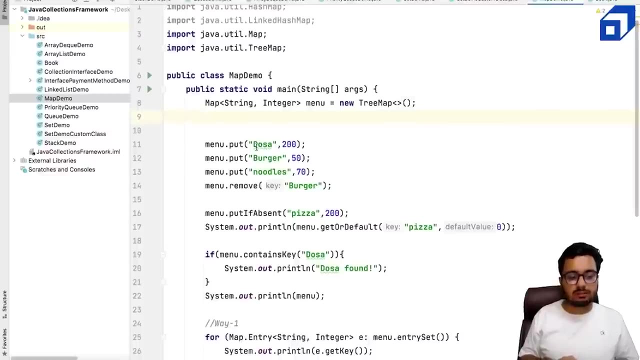 it will be using a self balancing um bst, right, so you can also do a tree map kind of a stuff here. we need to import it. uh, tree map, map is the code will work fine, except now the elements will be sorted according to their um keys, right? 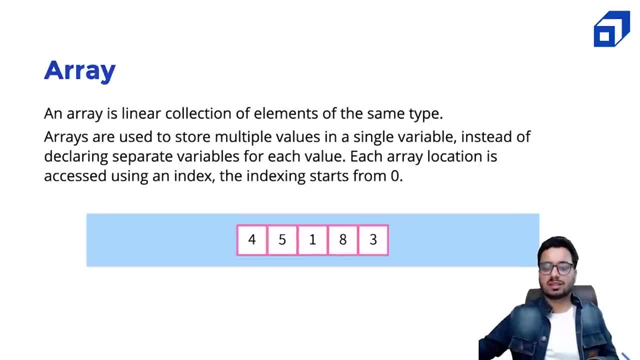 let us begin by revisiting the concept of an array. array is a very simple data structure that represents a linear collection of elements of the same type, right? so the concept of array is here in across all languages. in python it is called as list, in c++ and java: 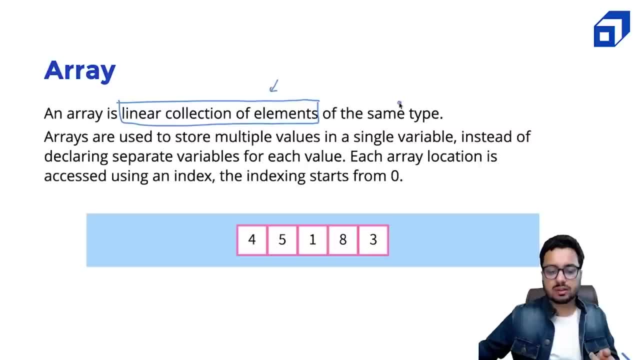 it is called as an array right, and most of the time it is of the same type. but in python the arrays can also store elements of the different type. so arrays are used to store multiple values inside a single variable. i say, okay, this is a container. the name of the container is just. 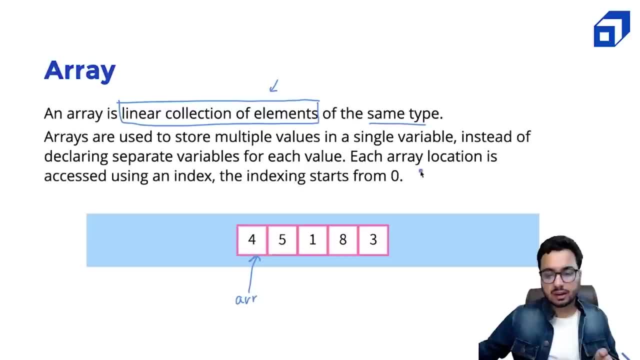 one variable, but it is going to hold multiple values, right. instead of declaring separate variables for each value, we just create one variable. now this helps us because, suppose you want to store 100 integers will not create 100 variables. instead, you will create one array and in this array, 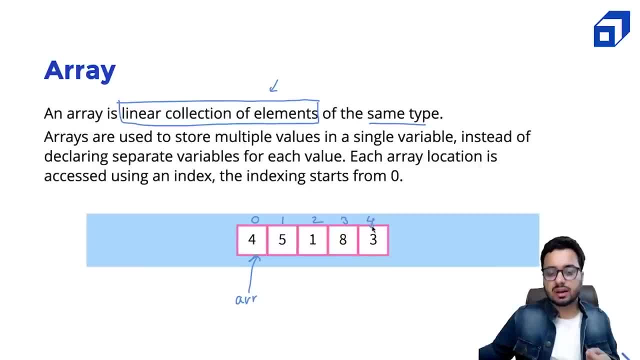 you will have multiple buckets. each bucket is referenced by an index. okay, if you want to store something at this position. indexing always starts from zero. right, you will take an array of zero. i want to store the number four at this position if i want to store something or i want to update. 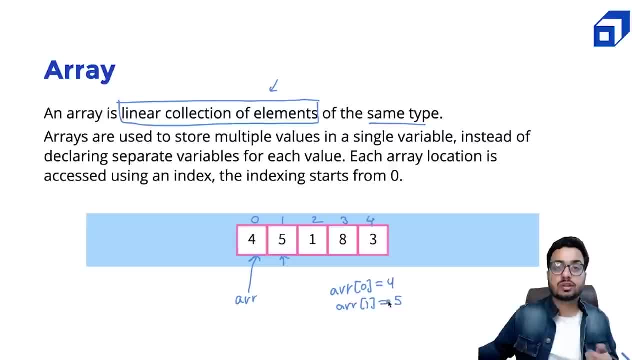 something i will take an array of. one should store five, or it should be fifteen, so i can update the value anytime i want, right? so this is the syntax, right? so the variable name is array, and how do i create it? so, if i want to create an array of integers, 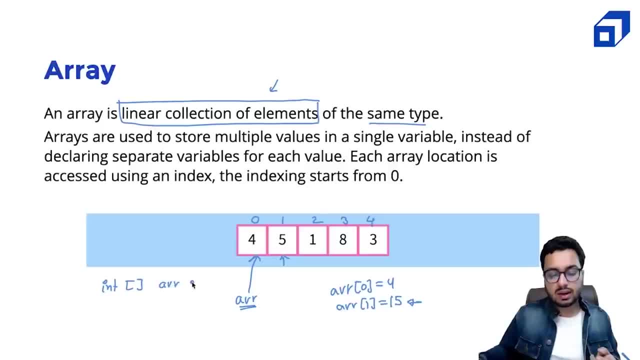 i will say int, followed by square brackets, followed by arr, followed by here we will see. there are a few different ways. one is we can use new keyword to allocate some memory, or we can directly give the values which which we want to initialize the array with right. let us jump. 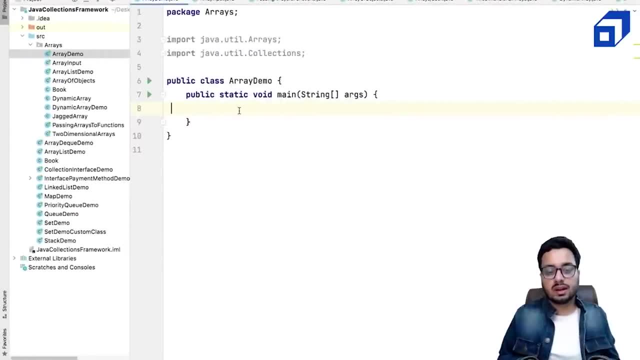 directly into the code and see various ways to create an array and work with them. so first of all i'll say: okay, i want to create an array, so this time i'm just initializing it with some random numbers. i'm not using the new syntax. we will do that as well. this: 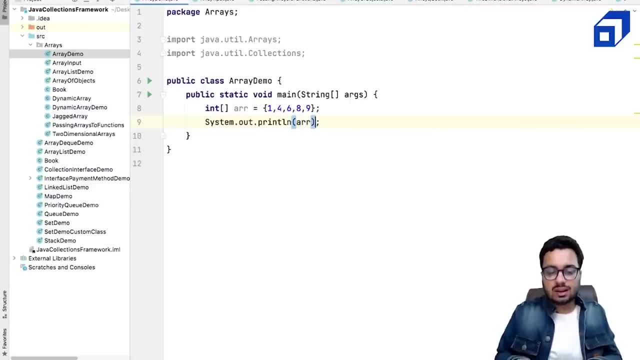 creates an array. if you do s out, here are let us understand what happens behind the scenes in the memory, if you do this right. so let me go and run this code. i will see some, some kind of address. in java it is called as object reference, so i see this number. 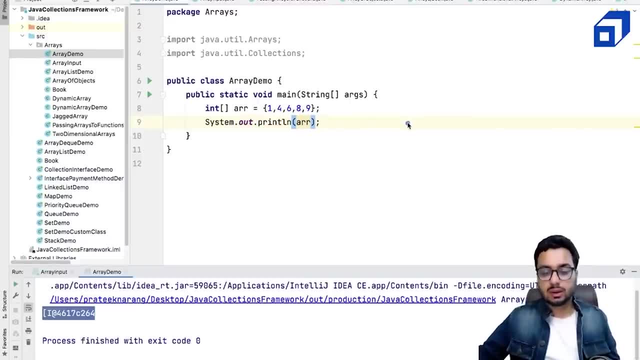 now what is happening if you dive little bit into what is happening in the memory right when your program is executing? your ram memory is divided into two parts. one is your stack memory and one is your heap memory. both of these memories have their different properties- any function that you're calling. 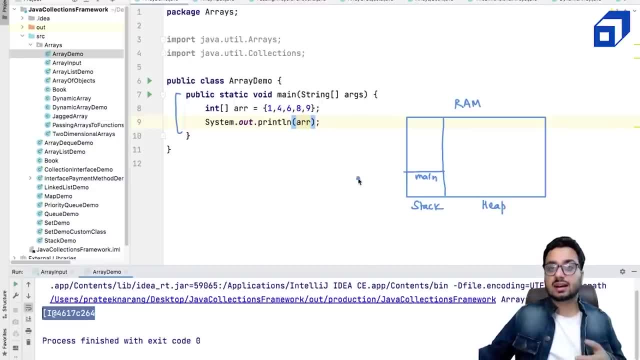 it goes into stack and it creates a stack frame out of it, right? and when you're creating this, something like this, you say, okay, uh, i'm doing index this. that is equal to 20.. when you create a primitive variable like this: x is a bucket, it is created here and it. 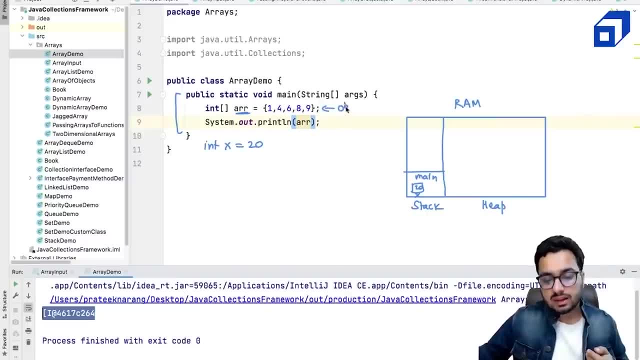 is storing 20.. but when you create an object, java is an object, the actual object, it is created in the heap. so you your one, four, six, eight, nine, it is created in the heap and the address of this object, whatever is this address? 264, right? so 264 is. 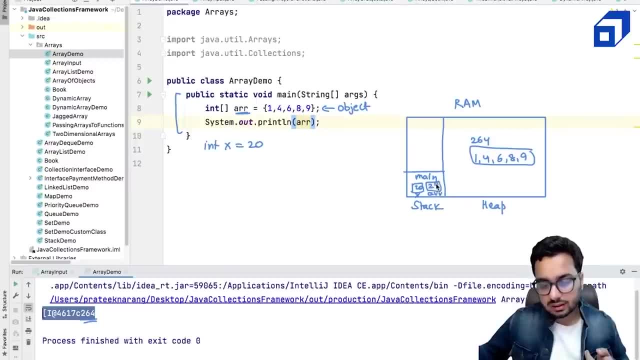 stored in a variable which is there in the stack, and this is storing 264. that means the variable in the stack frame is pointing to the array object. so we call this arr as a. this is a object reference. this arr is not the array itself. it is referring to the array right. 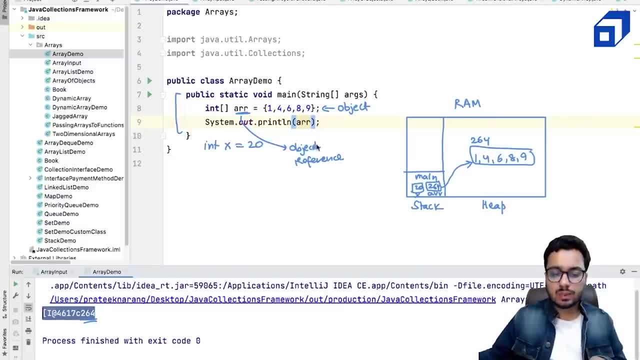 this is how it is created. uh, behind the memory, right now, when you're going to print arr, it's not going to print the contents of the array. instead, it is going to print, um, what is stored in arr, if you want. okay, i want to print the contents of this array, right? 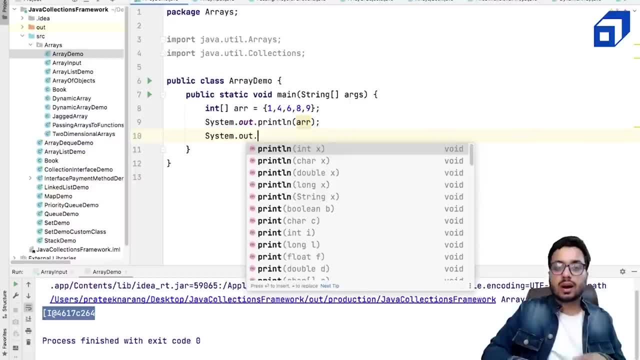 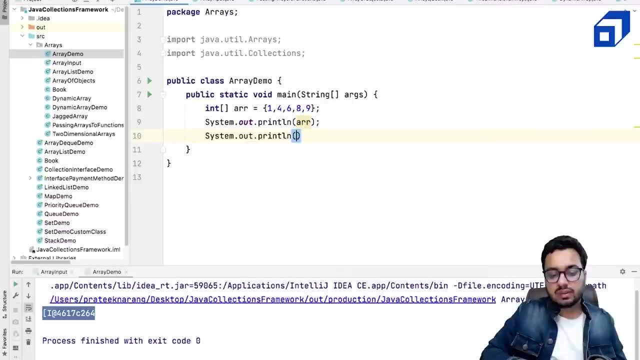 what i will do. i will say: okay, i need a way to iterate on this array and convert everything, uh, and print everything. right, there is a input function that we can use. so this: there is a different class. okay, it's. there is a class called as arrays. 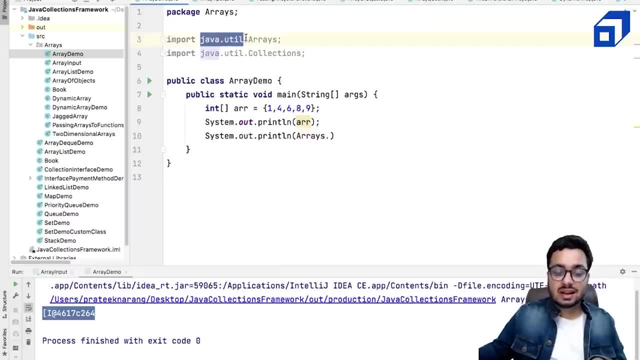 and it is part of javautil. so arrays class has certain helper methods to work with these kinds of arrays. these methods, we have to pass the array object and get our work done. so one such method is toString. i will give you some kind of array and i want you to convert. 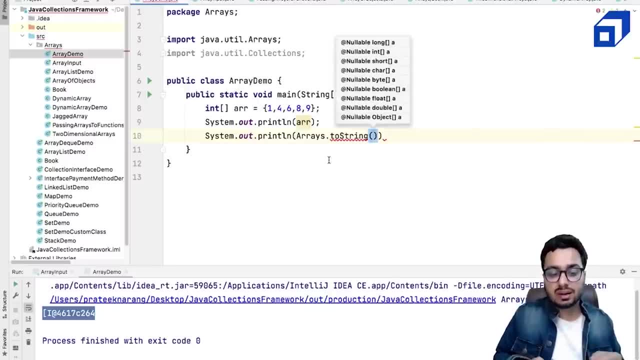 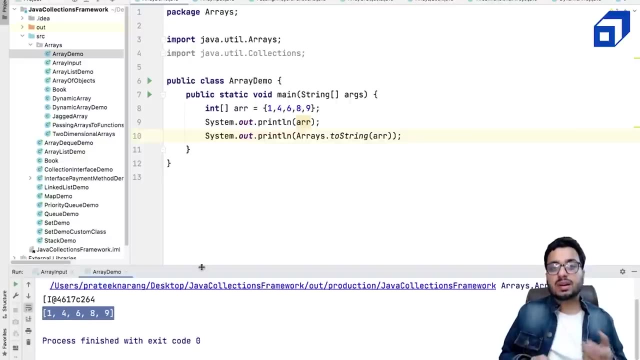 this into a string, like representation, that can be printed using systemoutprintl. so let me give this array and now, if i show you what is the output, let's see. now i am getting this array, so i am hoping that you are able to understand why this is working right. 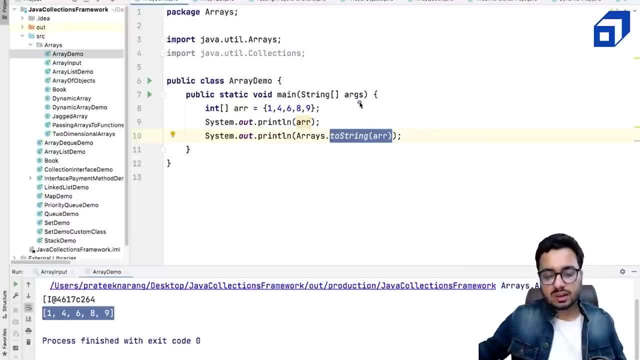 what could be the logic behind this toString? it is doing nothing, but it is doing a traversal on the array using a for loop and it is adding everything into a string. so it says, okay, i will start the string with a square brackets, then i will add the zeroth element, then i. 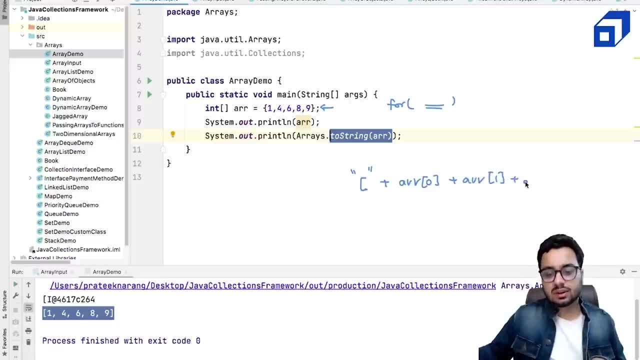 will append the first element, and so on. something like this it is doing. but what is happening? it is simply iterating over the array. so if i talk about how much time it will take, it will first take order of end time to iterate over all the elements of the 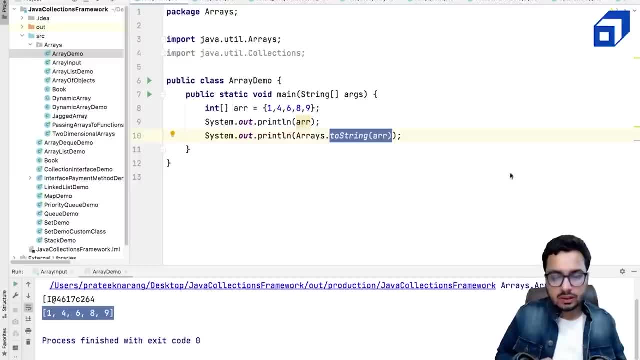 array. okay. so let us look at one more method in this array. so let me create one more array. let me call it as some array, let me call it as array2. this is equal to new int. so i am saying, okay, let me create an array. this time i am not. 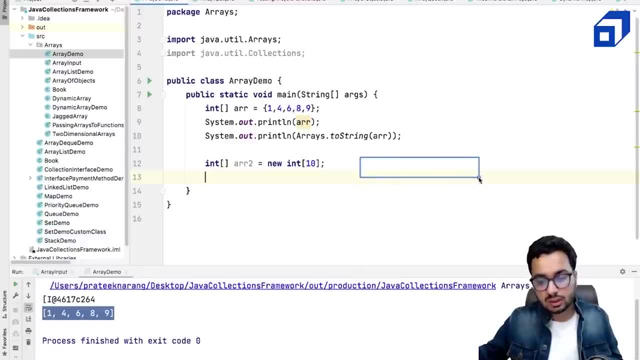 going to give you the data, but i am simply giving you size of the array. that okay. i want an array that should be able to hold 10 numbers. one thing you can do is you can manually initialize every index. you can say array of 0 should. 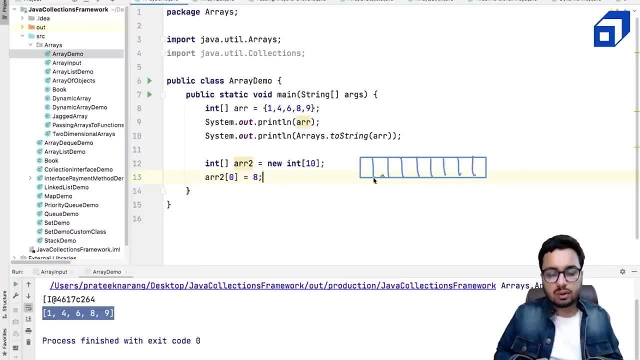 be 8, or let's say i want to fill 5 in every position, right? one way is you put a loop and update every index, or you read input. that we will see very soon. but there is one more method if you want to initialize an array. 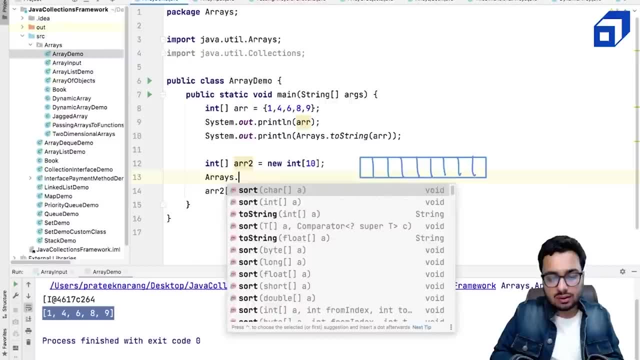 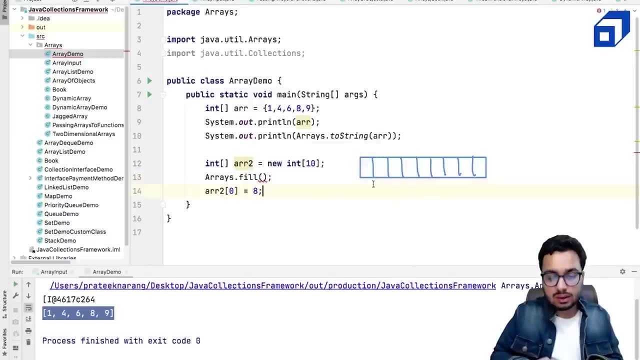 with a particular number. so that method is called as arraysfill. look at this. there is a fill method and you can say: okay, i want to fill this array with number that is, 12. you need to pass the array object, that is, array2, and maybe the value that you want to fill. 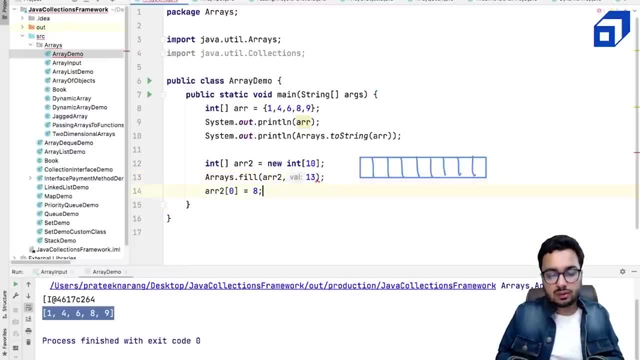 maybe i want to fill with the number 13. now, if i show you the output, i can say sout, array2. but i have to first convert it into a string so that i can print it as arraystoString. that is array2. okay, let me print the second array. can you guess what the output? 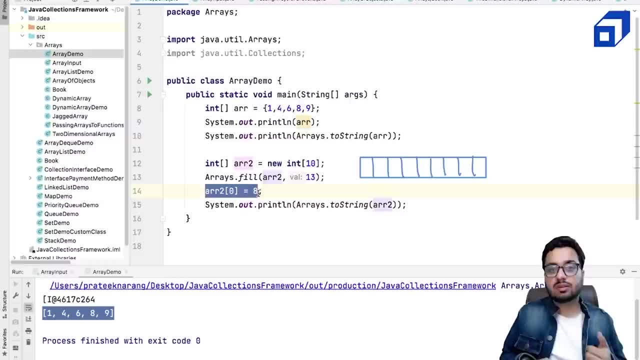 would be. the first element would be 8, which i have overwritten. okay, so this is updating the 0th element and rest all the elements will be 13. this is what we are getting right. so fill method is going to fill this array with 13 at each position. 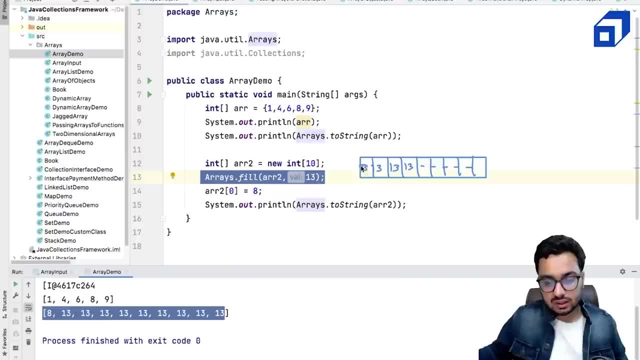 and so on. and first, 0th index i am updating as 8, so i get 8, followed by all 13's. that is another method present in arrays class. okay, arraystoString, arraysfill- one more method that is coming into my mind. it is very popular. 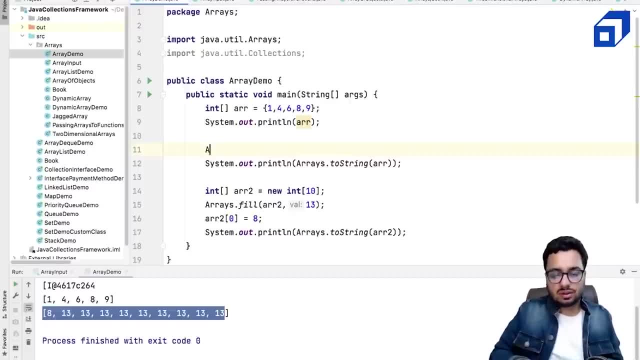 we need it often. this method is called as arrayssort. that is also present in this arrays class, so i can say, okay, let me sort this array. i want to put all these numbers into ascending order. so i say 1, 14 um 81, so i just randomize the numbers. 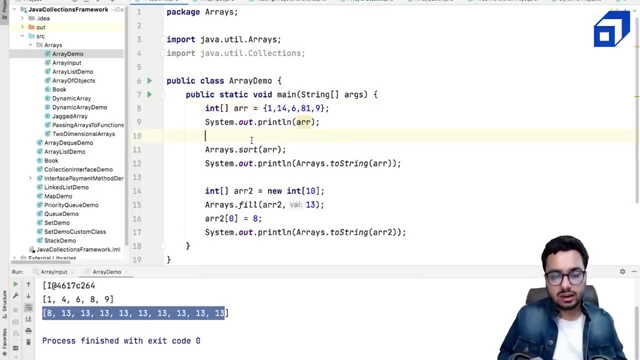 so that after sorting i can see they are actually in the sorted order. if i run this code now, you will see this array. it is going to be in the sorted order. see, the array is getting sorted. so internally it uses something like a quick sort kind of an algorithm and 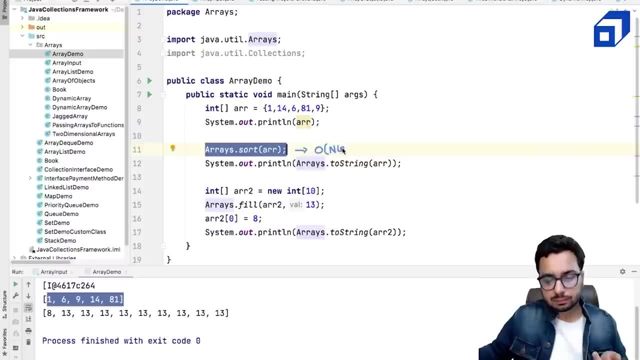 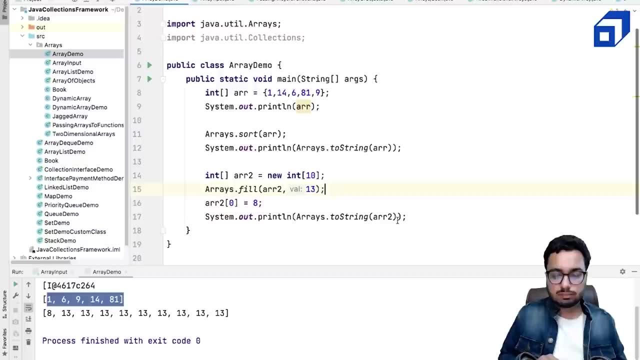 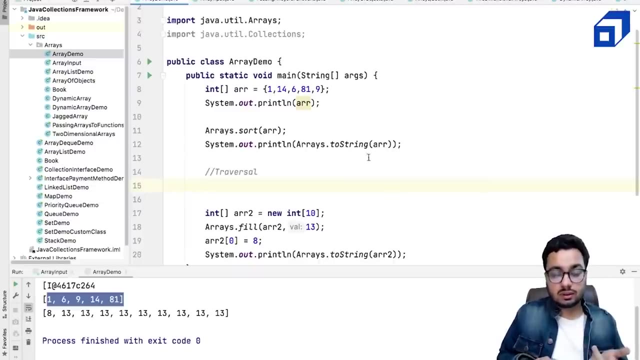 the running time, complexity of the sort method it is: order of nlogin. okay, so this is something that you should. okay, so let us look at one more fundamental thing in arrays, that is traversal. so there are three ways to two ways to traverse the array. one is: 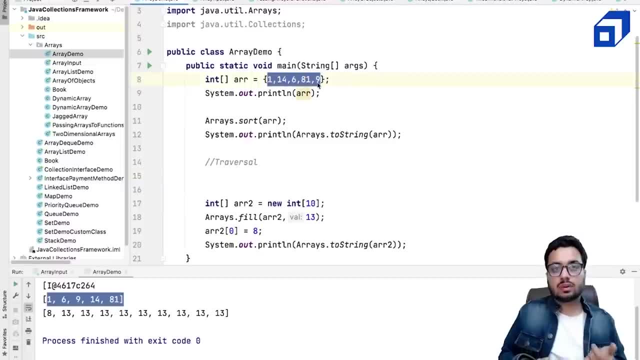 that i can find out the length of the array and then i can go over every index. if i talk about this array, i know there are five elements. so the indices are 0, 1, 2, 3. so array object has a property called as length. so if i say okay, 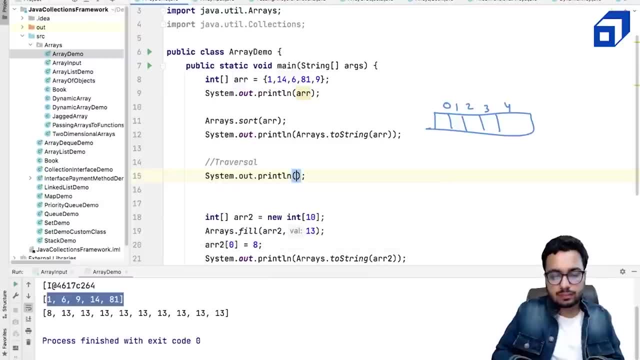 i want to see the length of the array, so sout array length. i can say this is given by length attribute of the array object. i can say array dot length. this will give me okay. this particular array has five elements. so and if i have to iterate i can say okay. 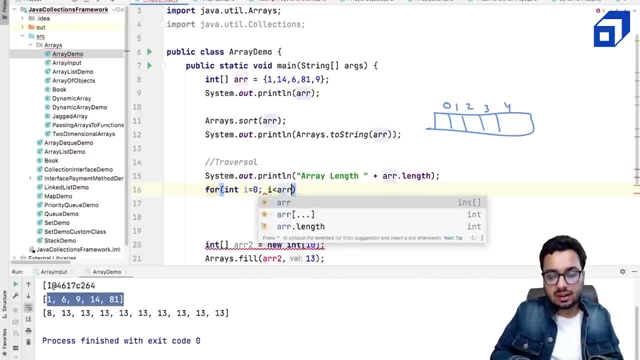 for i equal to 0, the index starting from 0. i less than array dot length: i++. and what i will do? i will say sout array of i. this is going to print the ith element of the array and we are doing it for all indices less than 5. 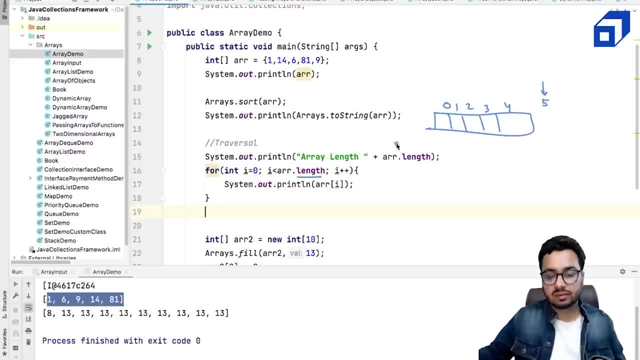 we do not go till 5, but we go till less than 5, because the indices start from 0 and they go till n minus 1. this is n. the last index will be n minus. the other way is: you can also use enhanced for loop. 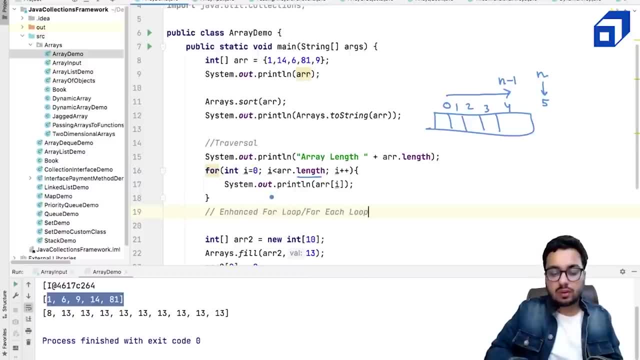 also known as for each loop, so you can take a for every integer x that is present in this array. i want to print that x, in this case x is not your index, but x is the value that is contained in this array. so if it is like 1, 6, 9, 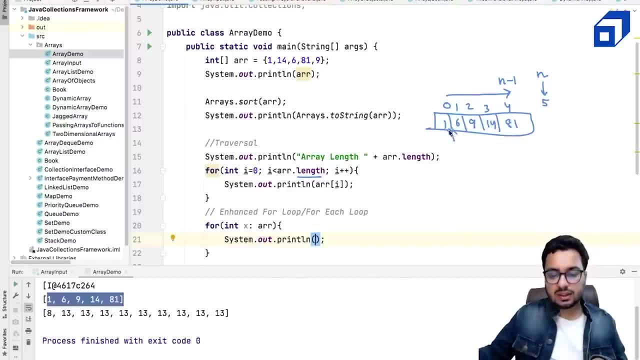 14 and 81. so in the first iteration x will take the value 1. the next iteration it will take the value 6, then it will take the value 9, then it will take 14 and then it will take 81, if i simply. 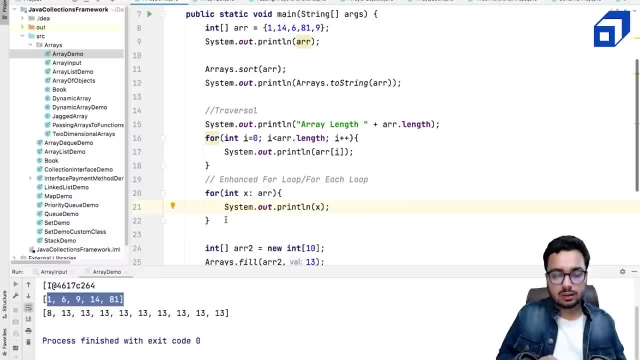 print the value of x. it will again give me the contents of these are two ways to iterate on the array. if you want to iterate on some part of the array, better go with the for loop, if you know that. okay, i want to iterate over all the values. 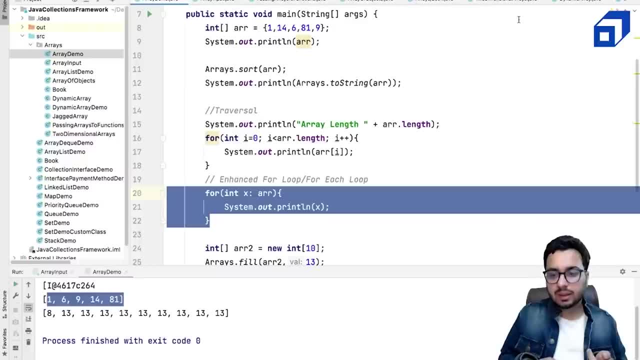 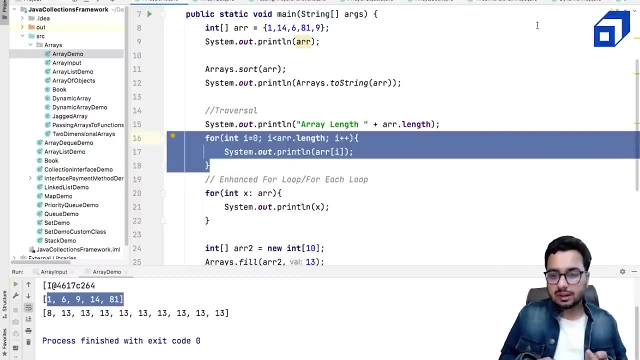 then the for each loop is a more simpler syntax, okay, but the first loop is more powerful because you can start at any point, start at any index and you can stop at any index. so let's run this code and see that we are able to iterate on this. okay, so? 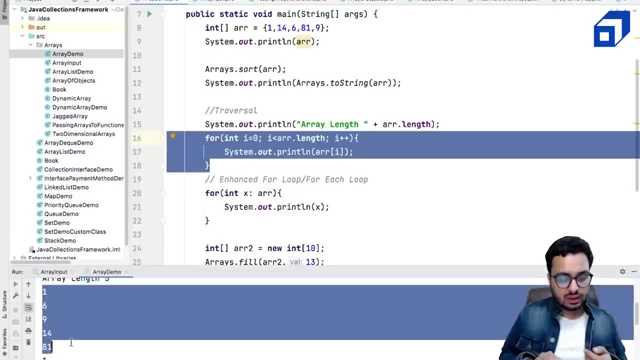 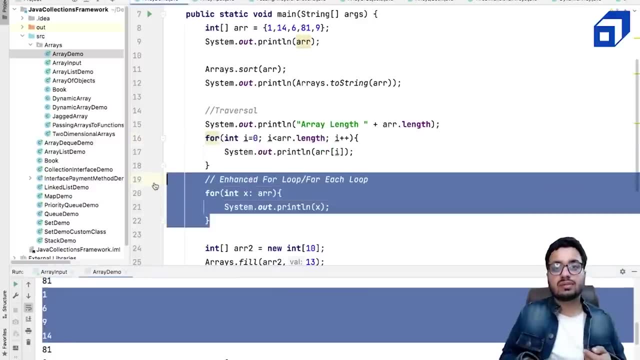 we can see. uh, we are able to iterate 1, 6, 9, 14 and 81. this is coming from the for loop, and 1, 6, 9, 14 and 81. this is coming from the for each loop that we have written let. 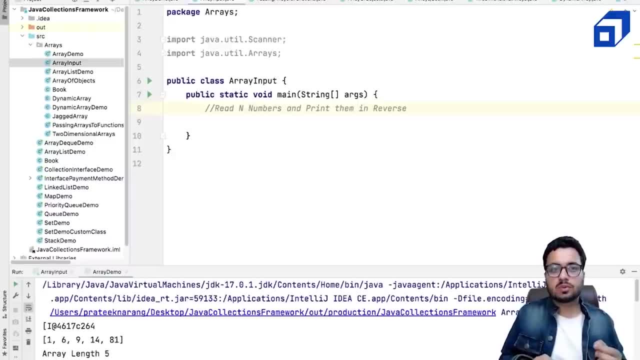 us look at another way of building an array. many problems will require you to reading n numbers and storing them and working with them. so, for example, a very simple use case is we have to read n numbers and we want to print them in reverse. without storing them, we cannot print them. 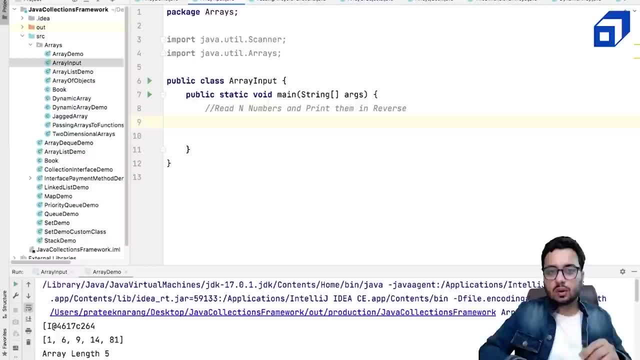 in reverse. that means we will need an array to do it. how do we read n numbers? so it's very simple. first of all we need a scanner java. so scanner is used to, uh, scanner object is used to read something from the command. okay, i can, okay, first tell me. 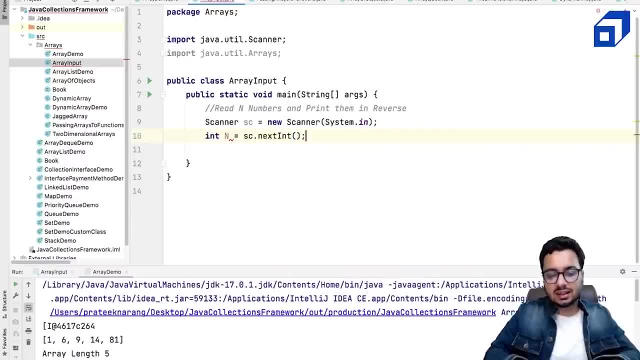 how many numbers are there? the method is called as next. once you know n, then okay, i'm going to create an array. how do we create an array? let's say i want an integer array and i can say- this is new here. i define: uh, what is the size of this? 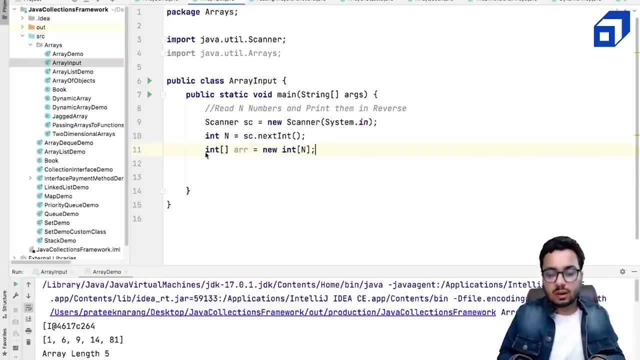 array. this will create an array of size n. now i want to read this array again. it is pretty simple. i will read the youth index, first index. second index, up to n minus one at the end it's okay, i less than n, i plus b, and in every iteration i can do. 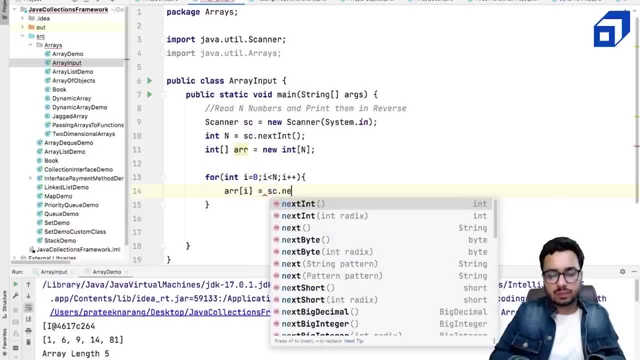 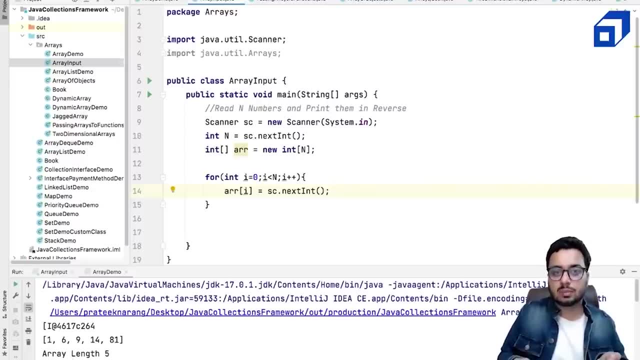 array of i is going to hold n value will read from the user. i can say scanner dot next, scanner dot next, and will pick one number from the command, put it in the ith bucket and once i am done i want to print them in. printing is easy, so how do we print it? 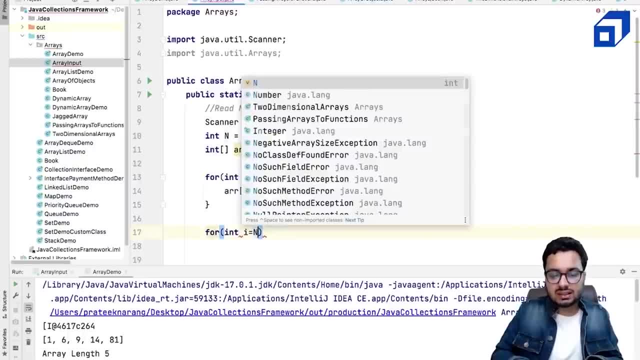 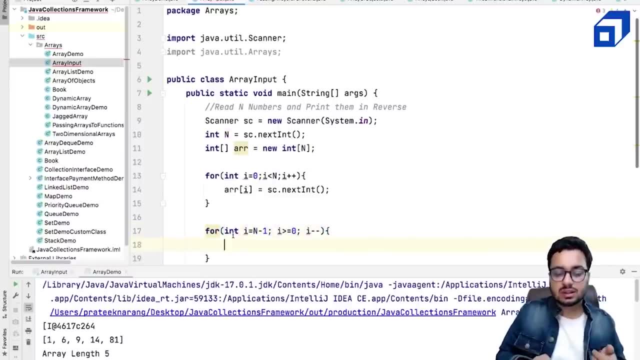 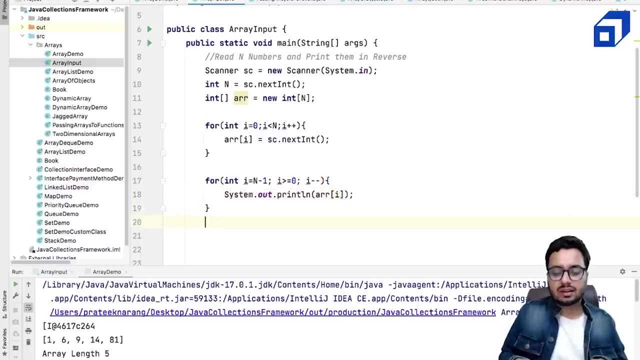 i can say: okay, i can start from the last index that is n minus. i can go till the first index that is 0 i minus. so i just need to reverse the loop that i'm using to iterate over the array and i can simply, uh, iterate in the reverse. 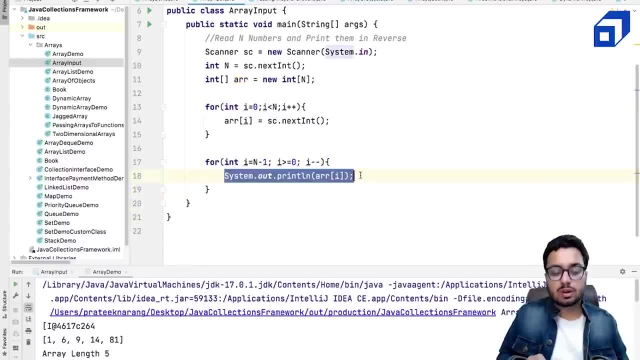 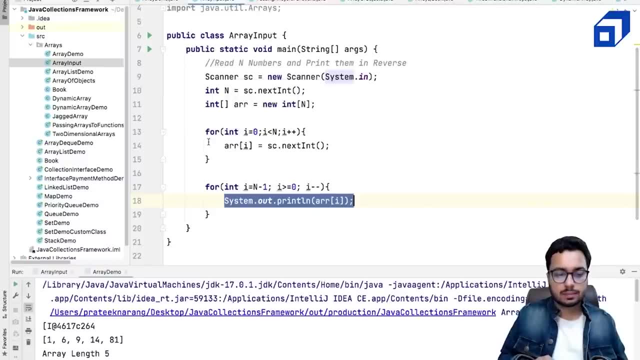 direction. so system dot out dot println array of i. let us go and run this. system dot out dot println array of i. let us go and run this code and see, suppose i want to, uh, read five numbers and print them. so let's say the numbers are: 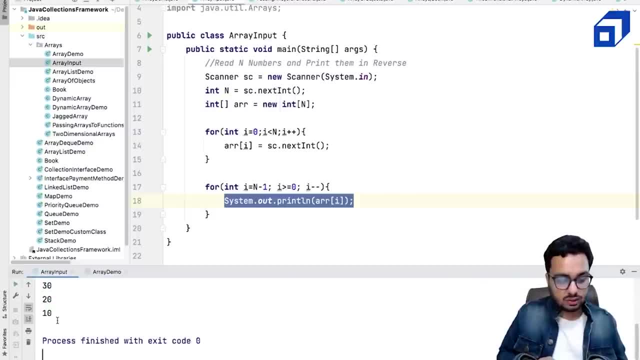 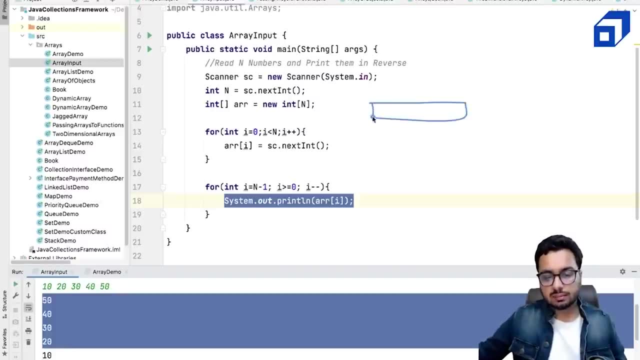 10, 20, 30, 40. so you can see, i'm able to print 50, 40, 30, 20, 10.. so what happened? i created an array of size n, then i stored numbers. i said, okay, go over index 0 and read one number from the command. 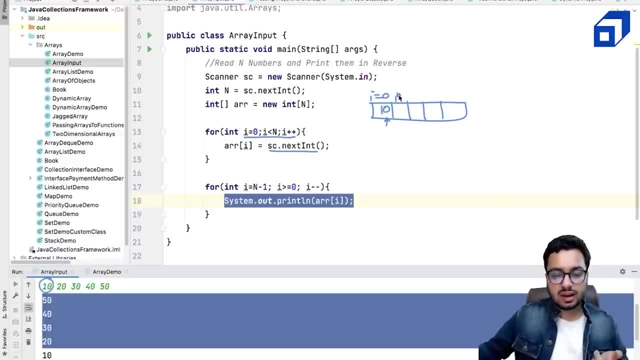 line. so it it read 10, it's quoted here, then i becomes one. it is reading one number again, scanner dot. next in the next integer in the line it is reading, it is storing it, and so on. so 30, 40, 50.. then what i did? i? 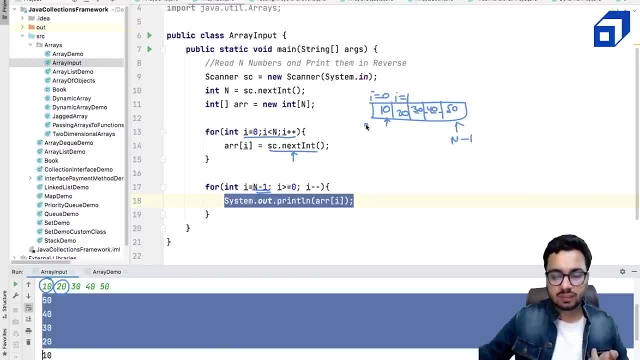 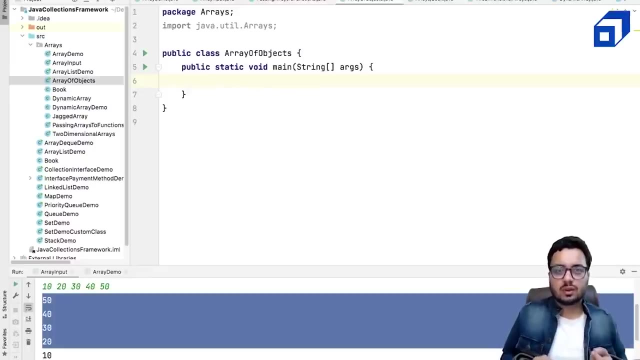 iterated from the last index, which is n minus 1, till 0 in this direction. i iterated and i printed array of five. this will print my array in the reverse order. the next thing i want to talk about arrays is array of objects. okay, we have seen how do we create an array. 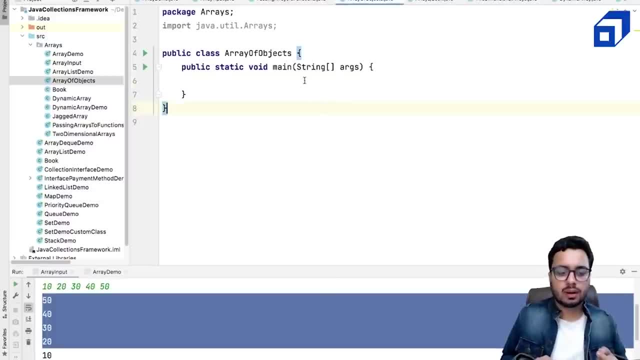 of primitive data types like integer. similarly, you can make a array of float area of boolean, like primitive data types you can work with. but what is an object? so complex data type like strings? string is an object. okay, you can also have a user defined class and you want to store objects of that. 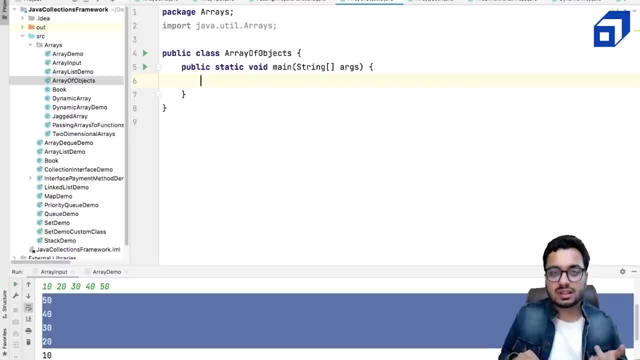 class in your array. let us see how that actually happens at the memory level and also at the syntax level, right? so suppose i have. i have a book class. i'll just delete the method in this book class. i have defined three attributes of the book. one is isbn. 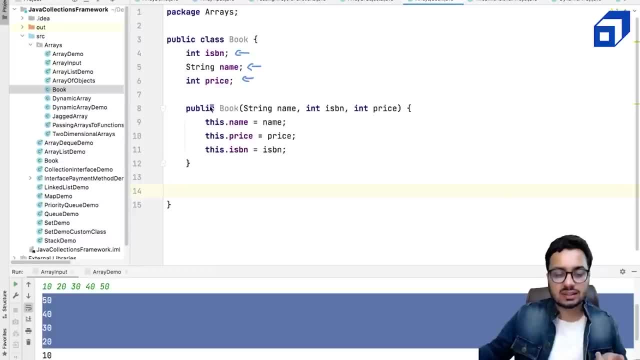 which is your unique book code, a name and a price. and i also have a constructor to create a book object. right, if i want to simply create one book object, how i will do it? i will say, okay, i want a book b. this is equal to new. 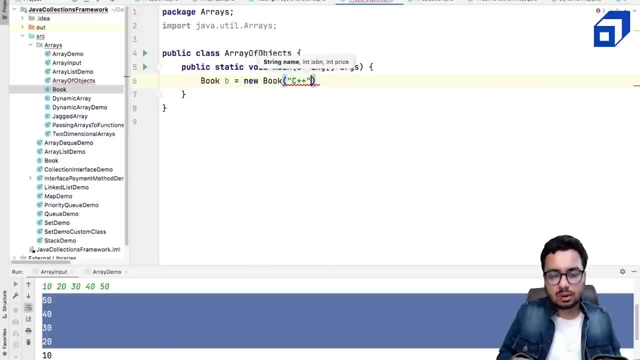 book. in this new book i want to pass the name of the book and isbn and the price. i say, okay, these are the three attribute or three values that i'm going to initialize this book with. this just creates one book object, but what we really want, we want to create an array of books. how? 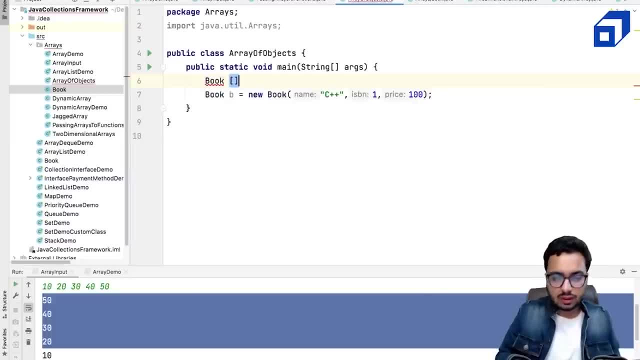 do we do it please? okay, book, followed by square brackets. that is the data type of the array. then you have to give a variable name. i say okay, the name of the array is called as books- let's keep it intuitive- and followed by new book, suppose i want to store. 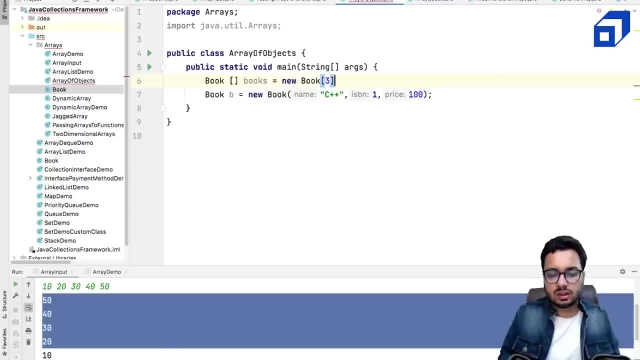 three books in an array. this is going to be three. now what it's going to do, right, as i discussed in an integer, your memory is going to get divided into two parts. one is your stack memory, which your main is getting called, and we have a variable called as books. 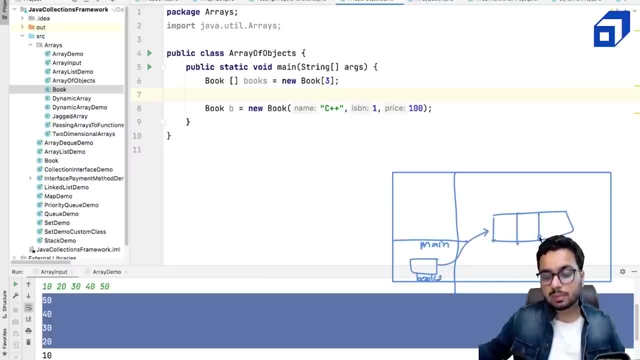 which is going to refer to an array that is capable of holding three. now, this is this position, is books of zero, this is books of one and this is books of now. how do i put a book here? so one option is that, okay, i have created a. 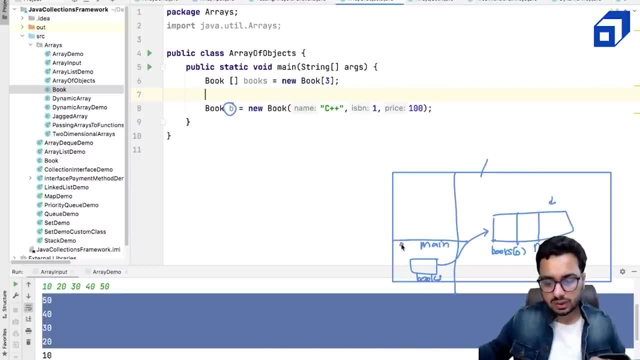 book. object b already, so b is a book, so b is also created here. b is pointing to book. that is a, c plus plus book. c plus plus book has some address, let's say 104. b is storing this value, 104. now i want to put this book inside this. 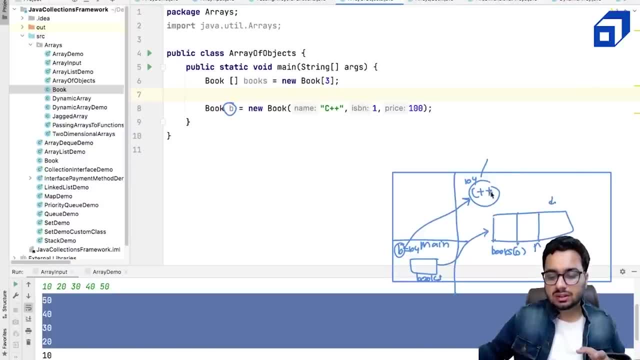 array. i cannot like, physically, i i cannot say, okay, this object will go inside this box in the heap. no, this is now not how it happens. the way to do it is: you will have to say that books of zero, it is going to hold b. books of zero is going to hold b. 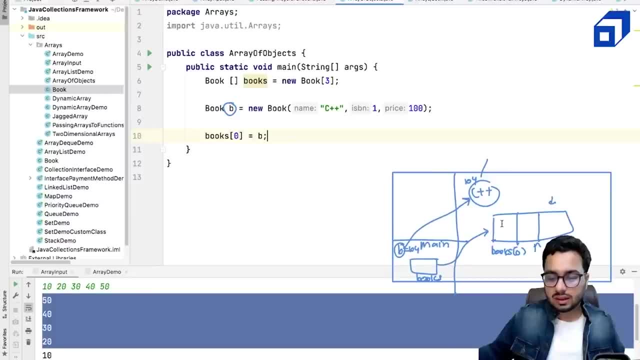 that simply means that whatever is the value in stored in b, it is also stored in here. this value is one zero. that what does it mean? so it simply means that books of zero is referring to the c plus plus object, c plus plus book object that is present. 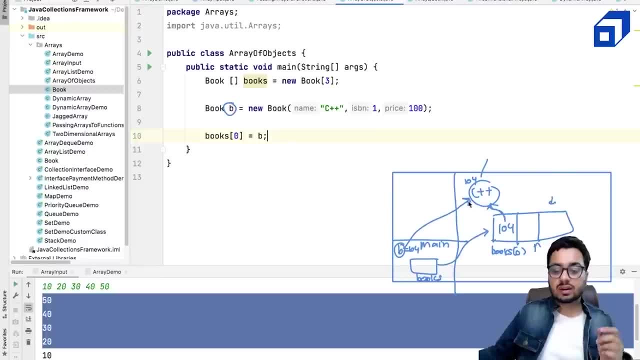 in the heap. this is how it is getting stored. in case of area of integers, it is different. case of array of integers you say, okay, uh, area of zero, this is equal to five. the number is directly stored here, right. but when you say books of zero, this is: 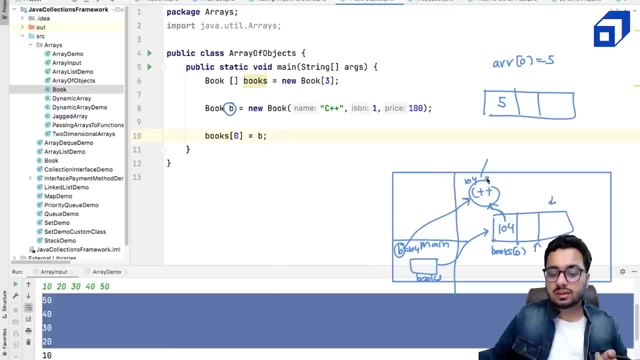 equal to b. uh, books of zero is holding the address of this book of. now you might say: okay, this, this might be the reason, um, because we have created a b reference variable and then we are copying that value. even if you do something like this, you say, okay, books of one should be equal to. 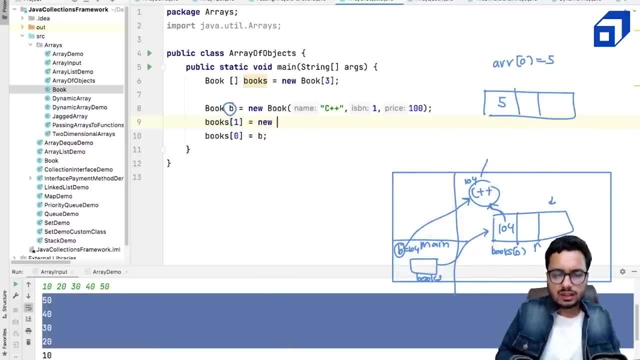 new book and let's say this is a java java book with code 2 and price is, let's say, 200. and let's say, books of 2 is a new book which is, let's say, a python book and code is, let's say, 3, price is, let's say, 100. 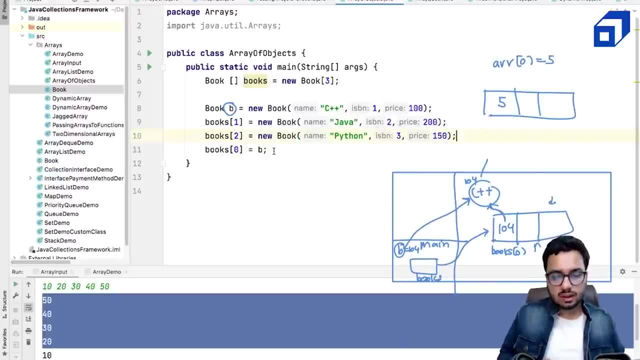 something like this: let's say we have now books of 0, books of 1, books of 2. what is happening when you're doing this statement? this is even doing the same work, just that this new book object is getting directly stored inside books of 1, so that simply means whenever you use new book, it creates. 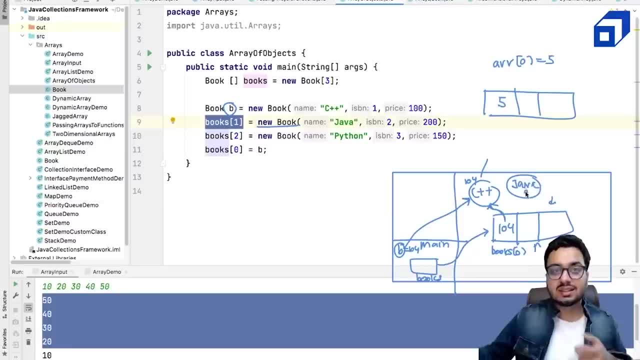 a book object in the heap memory right not going to create inside the array. java book is created somewhere in the heap. maybe this location is 216 and this address is getting copied here, so this is going to be 216. that means books of 1 is going to refer to this java object. and when i say books, 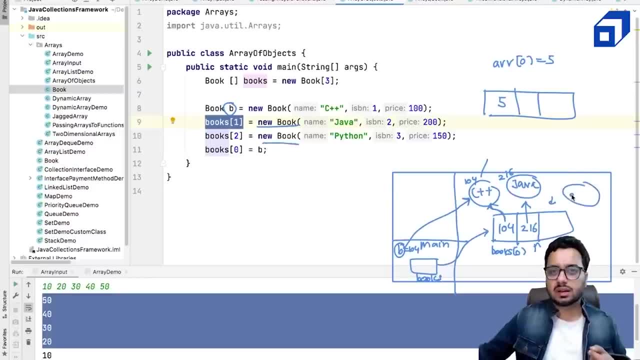 of 2, this is equal to new book. so again, a new book object will be created in the heap. let's say this is python and it has some address, let's say 780, so 780 will get copied here. now, you want this? okay, i want to. 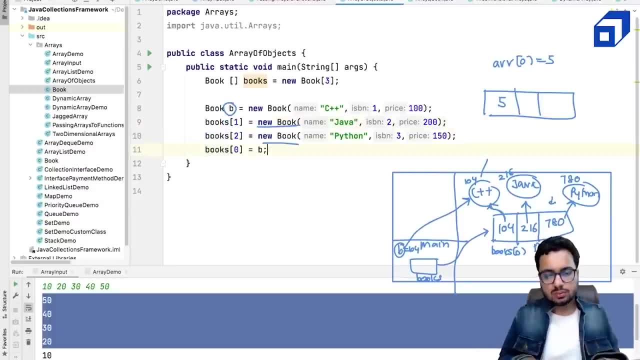 really verify. this is how it is stored. let me show you, um, by doing an sout right, if i say sout books, what i'm going to get. i'm going to get the address of the whole array. maybe this books array is created at a location that is. 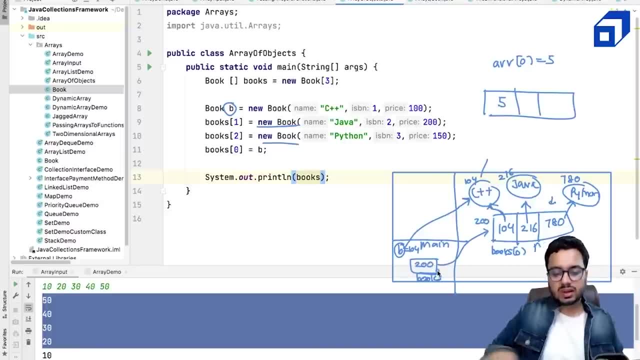 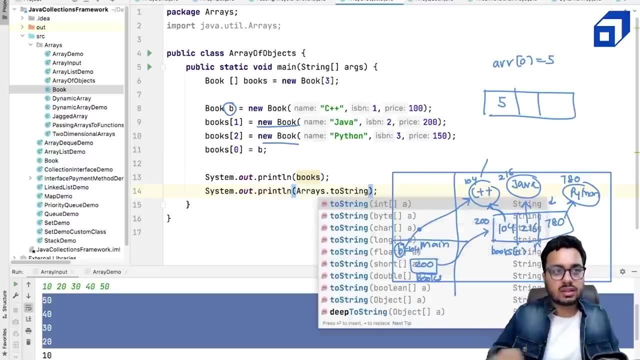 a book, object 200. I'm going to get this 200. but now you might say, okay, no, I don't want to print this. I want to print this entire array. if I say sout arrays, dot, toString, basically I want to. I traverse on this books array and I want to print it. let me show you this output: what? 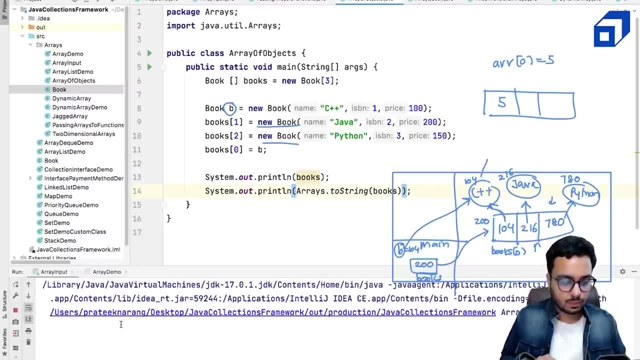 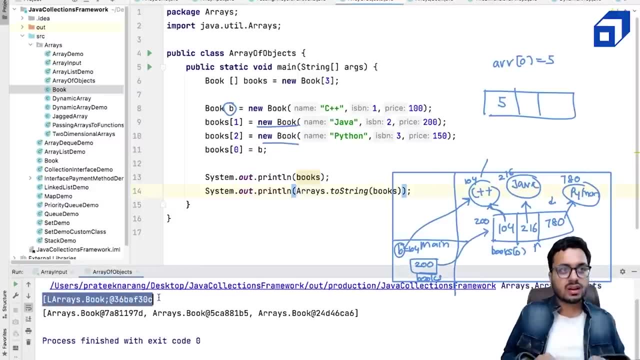 output and do we really get? let me run this one now you see, what we are getting here is the address, is the value that is stored in this book variable, and what we are getting here. these are the three addresses stored in this array, which are referring to the three. 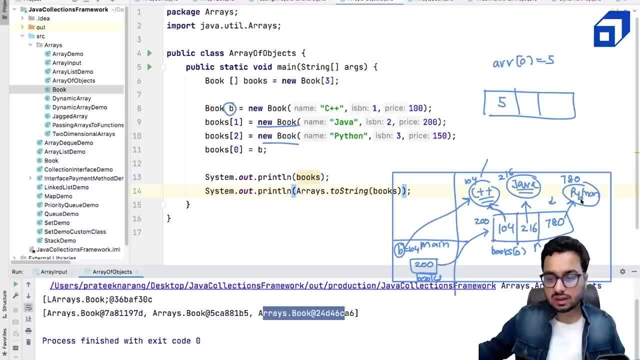 books that we have this- this is C++, Java and python- three objects. their addresses are stored in the books array and this is what we are getting right. you might say: I want to print the content, I actually want to print the object, I don't want to print the print an address. how do I do that right? 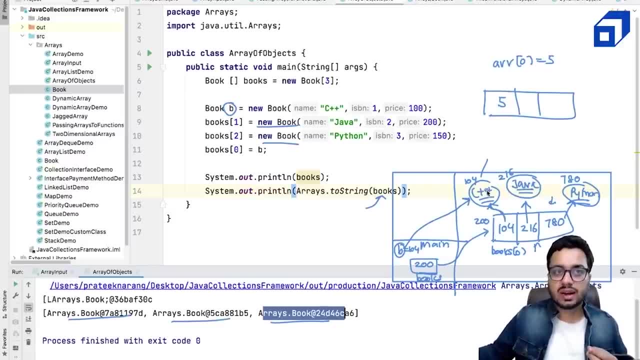 the reason is: Java does not know how do we print this book. okay, how do we actually go to a location and print that object? so, in order to do this, there is a method called as toString that is present in inbuilt classes. okay, for example, when you print strings, print. 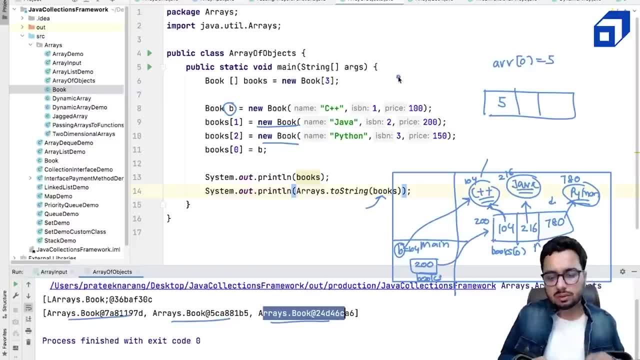 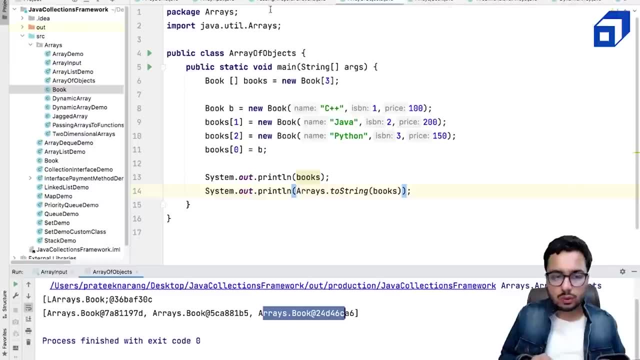 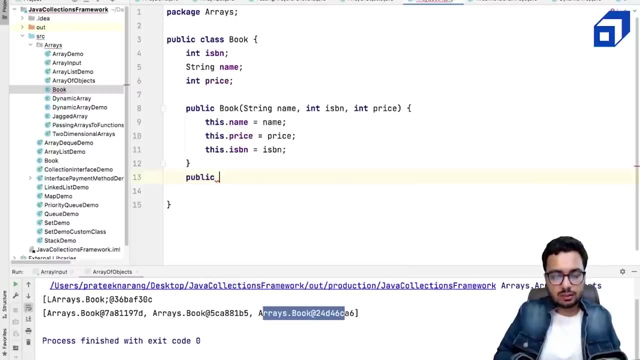 a string as a toString, or if you print, like some object, right, so many objects have their own toString method. what we have to do? we have to go inside the book class, which is this, and we have to say: okay, I want a toString method, public string toString, so this method. 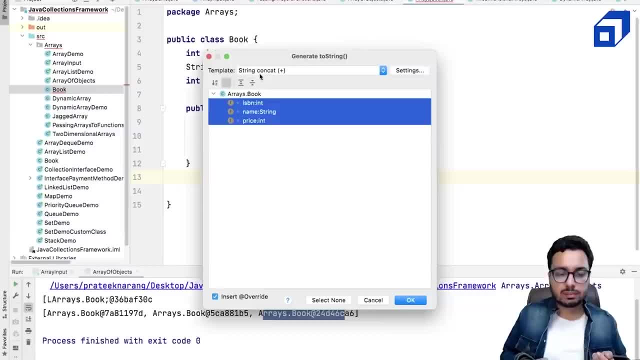 should return a string. it is automatically giving me a recommendation that there is a default template in which I will concatenate these three properties, Okay, of the book, which looks good to me, so i will just click ok and it will create a method for me, right? 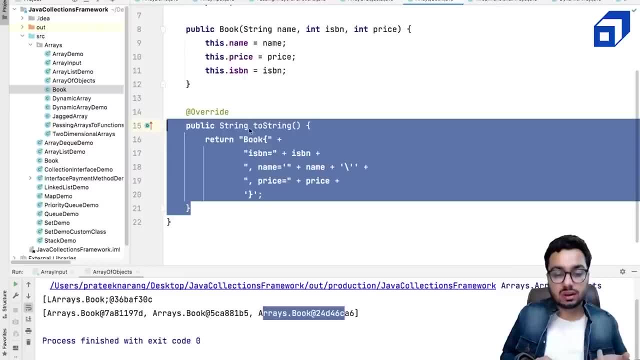 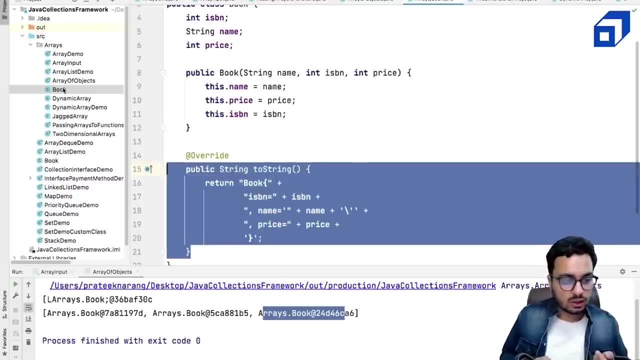 so when i want to say okay, i want to convert this book into a string, internally it is going to call uh, the two string method of book. right, which method i will tell you. right, let us go to area of objects. when are you saying errors? dot to string. it is going to iterate on each book. 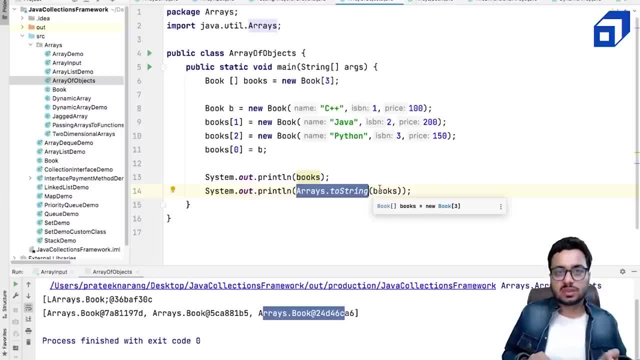 and it is going to convert that book object into the string like representation, if the two string method is overwritten. right, we have overwritten that method, so what we will get, we will get the contents of the book. let's run this code now once again and see what do we get now. now you can see. 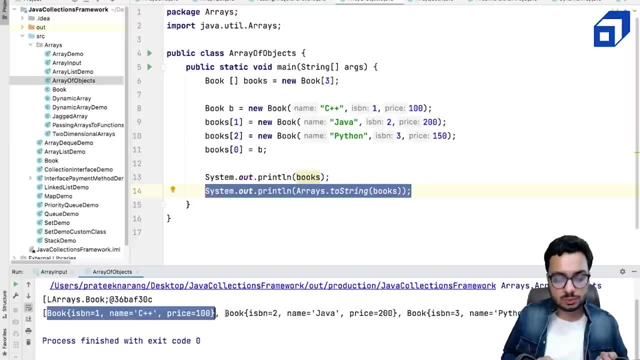 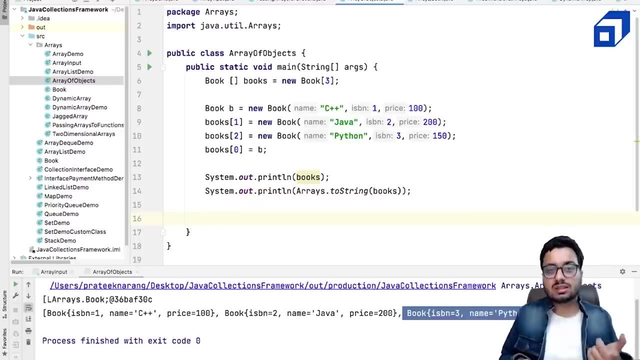 i'm getting a book that is the c++ book, then the java book and then the python book. you might ask: okay, can we do something on this object? the answer is yes. maybe you want to, uh, start this array of books, right. so do you think erase dot sort will work? i want to sort this array of books, will it work? 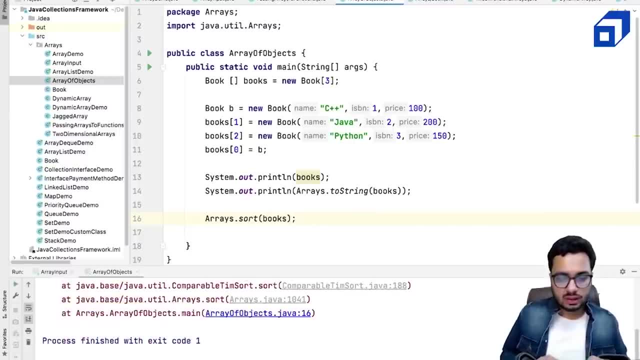 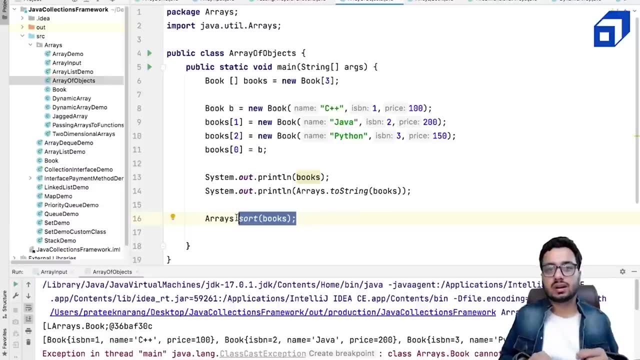 i might get an error. okay, i'm really uh getting an error here. why? because the sort function does not know how do i compare two book objects? okay, so how do i do it? uh, this book object, i don't know how do i compare it to the soundness object? okay, so how do i do it? uh. 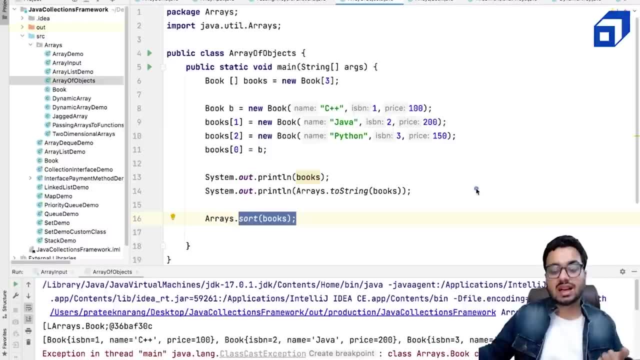 this book object. okay, so how do i do it? uh, are three ways that i have discussed in my previous video in which i have discussed java collections. one is using a compare to method, one is using a comparator and one is using lambda function. i'll give you a quick, uh way to do it which is using the lambda function in this video. 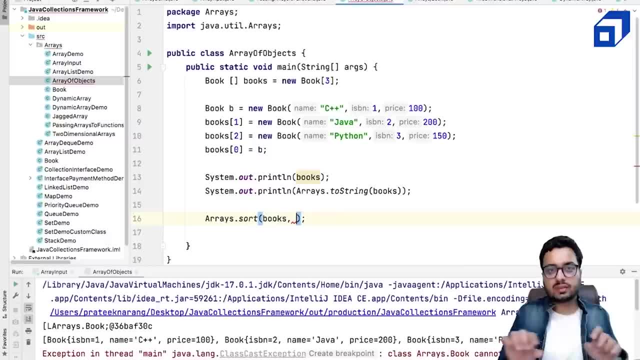 i what i need to do. i need to define one line function in which i will say: okay, how do i compare two book objects, the two inputs, let's say book b1 and b2, so they can be any two books. the sorting algorithm is going to pass book objects to this function, followed by an arrow. 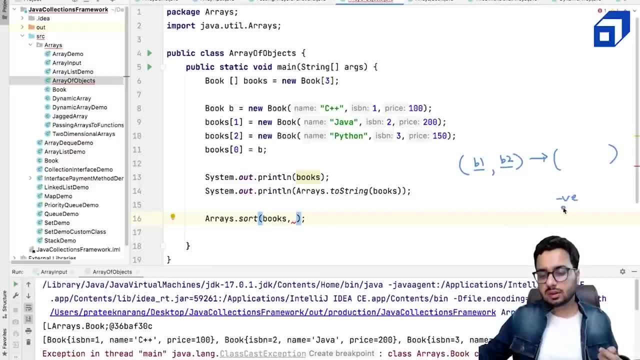 followed by: i should return a number which is negative, zero or positive. so if i return a number that is negative, it simply means that my first book is smaller, right, okay. and if i return a number that is positive, that means my um first book is bigger, right i? i need some way to convert these two books into the numeric values, for example i. 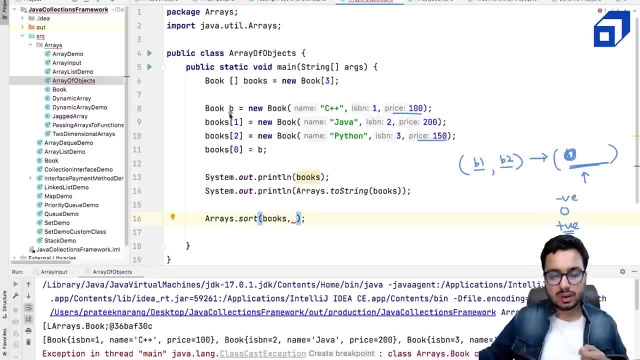 want to sort these books according to their price. let's say i'm comparing uh, c plus plus and java. if i return 100 minus 150, what? what does it return? it returns a negative number. that means the c plus plus book is smaller than the python book, something like that. let me show you. if i say uh, 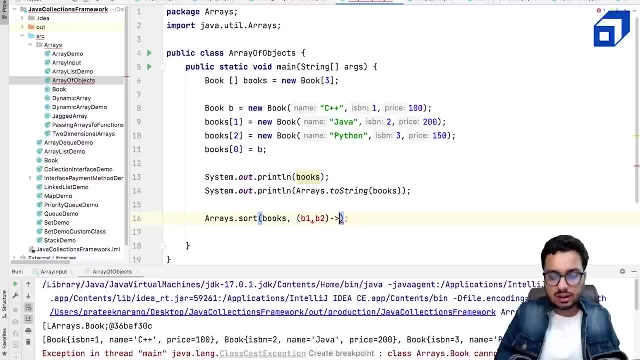 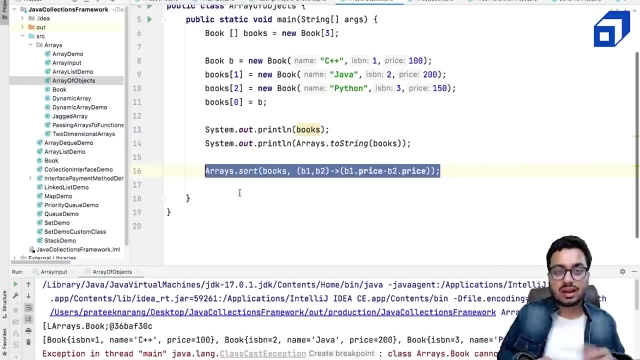 i want to compare two book objects, b1 and b2, and in return i will say that compare on basis, on the basis of their price. so i will return a number: b1 dot price minus b2 dot prime. this is a shortcut way of writing a comparator right using a lambda function. i'm comparing two books. if the first book 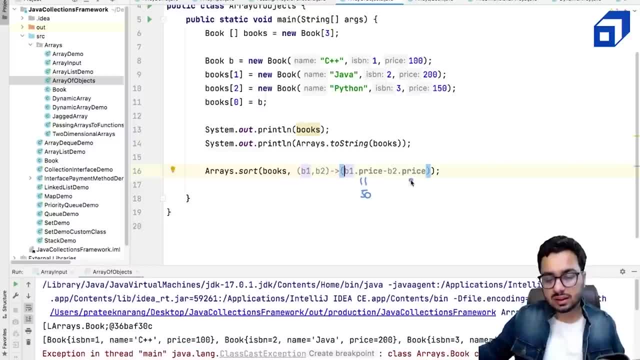 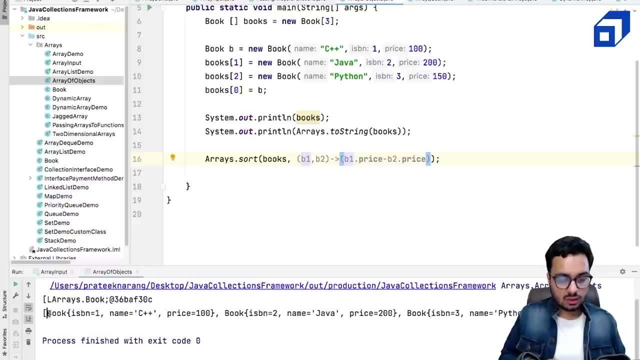 price is, let's say, 50 and second book price is 100. this expression will return a negative number. that means the first book is smaller and hence it will be placed first in the list. right, let me go and run this and we will see what happens. so i'm getting now the c plus plus book, followed by: okay, i forgot. 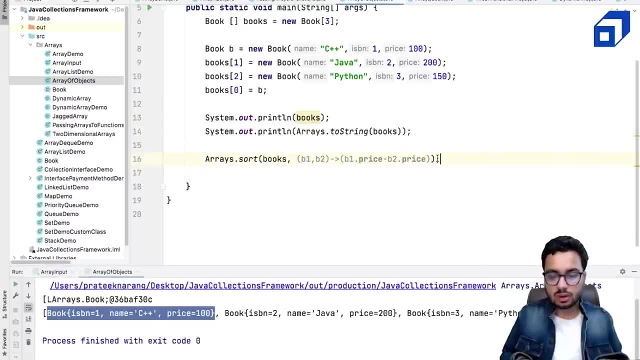 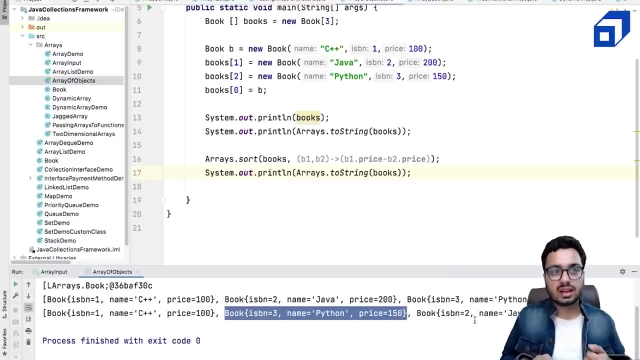 to print this after sorting right. before sorting, it is c plus plus java and python. let us see what happens after doing the sorting right. i'm getting c plus plus the least price, then i'm getting the python book which is 150 price, and then i'm getting the java book which is having a. 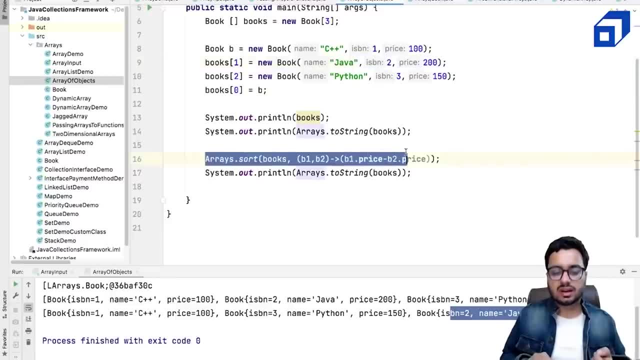 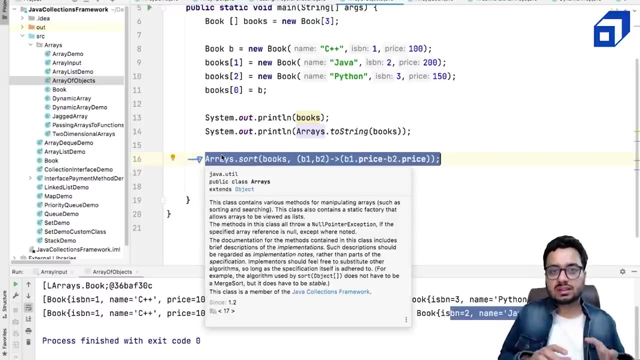 price of 200. okay, so i hope you are really understanding how we are doing the comparison and we can tell the sort function. this is the parameter on which i want to do the sorting right. if you want to write more complex comparisons, like multiple, if else conditions, 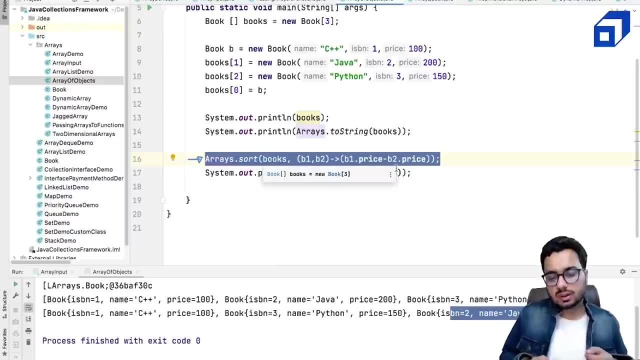 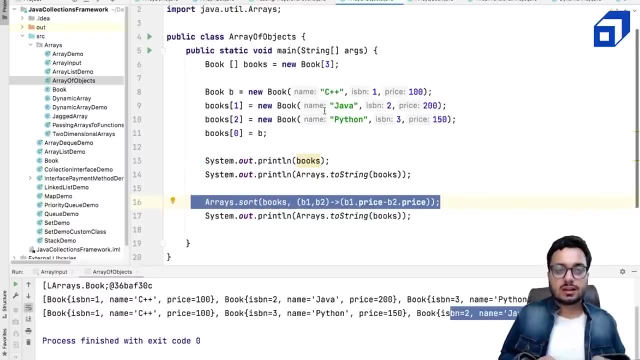 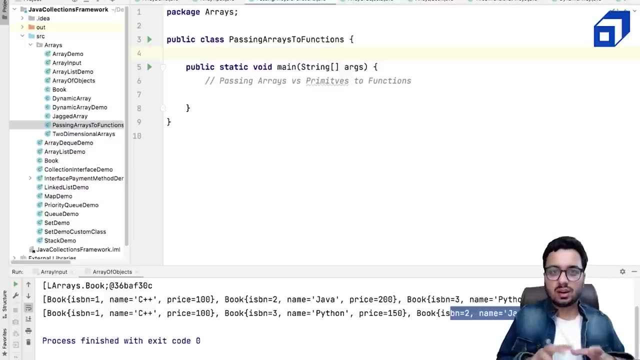 then you have to go with the comparator way of uh, comparing the two books. okay, so that is how you work with array of objects, and i hope these concepts are clear. let us move on to the next concept, that is, how do we pass arrays to functions and what happens internally in the 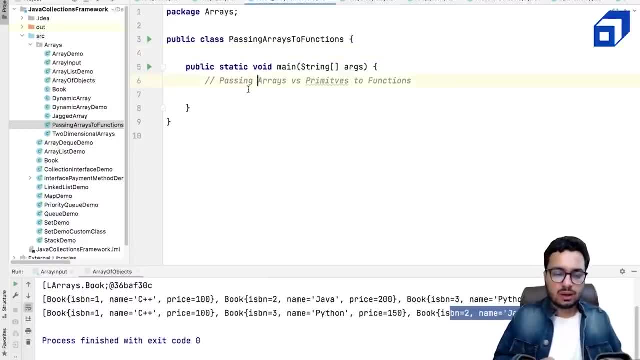 memory. so let us discuss this concept for example. uh, let's say i have a variable called as uh money, which is, let's say, i have 100 rupees, and let's say i have a function called as uh double money. right, so is okay, i will get some money and i want to double it so i can joke. money equals to: 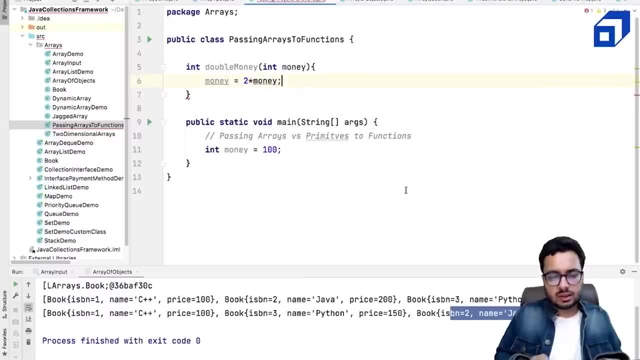 twice of money and that's it. now i call this method, i call the method called as double money, and i give it money right, and now i can say, okay, let me, so let me call it as public void. i'm not going to return anything, public, static void, double money i've just. i have, i have a single variable right. so basically what i'm. 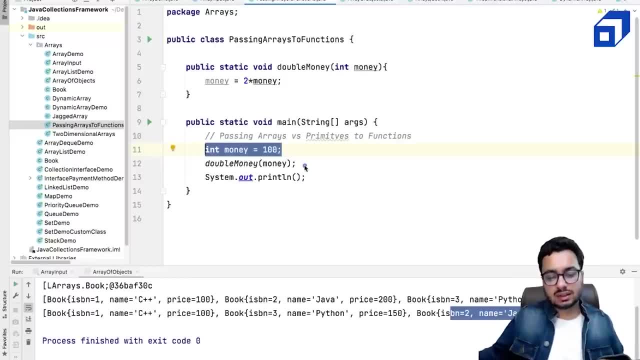 trying to tell you is: i have this money variable. i pass it to a method called as double money, which should which people might think that it's going to double it. but let's see what do we really get. if i print money here, what do you think what output you can expect here? 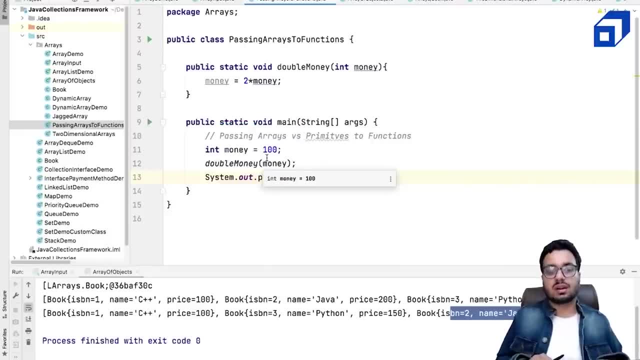 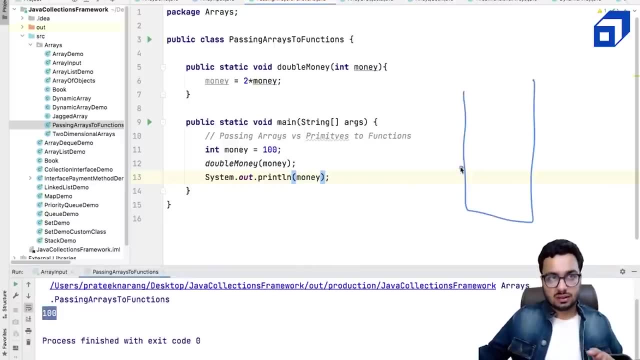 let me go and run this code. the output will be still 100. the money is not going to change, so i'm still getting 100. so let us understand what is happening behind the scenes. this main function is created in your stock memory. this is your stock memory, and there is a variable called as money. 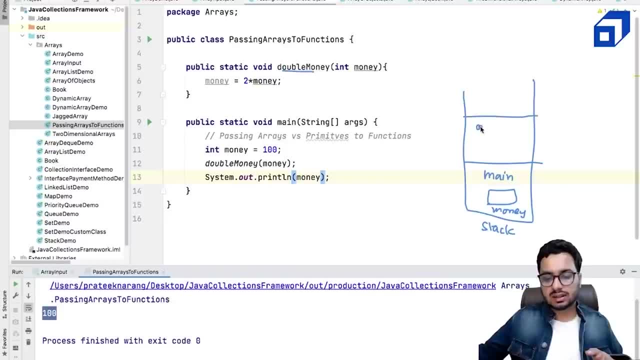 and when you make a function call, another function is called. that is your double money. and in this function you have another variable called as money. it exists in a different scope, in a different part of the memory. this money was 100. so when you call this function, this money is. 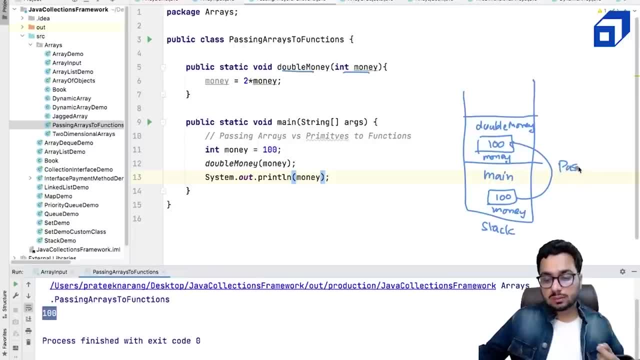 getting copied here, right copy, right, passed by value. it is getting passed here. we are passing this value 100, and here you say money equal to twice of one. you say: okay, i'll make it double, i will make it 200. now this function call is over it. 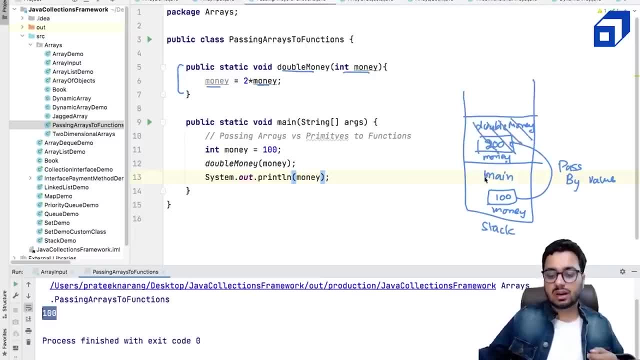 does not return anything. this stack frame is destroyed and you are back here now. when you print this money, what you are going to get? you are going to get just 100.. now let us repeat this experiment in, in in a case. instead of having one variable, let's have a array object. 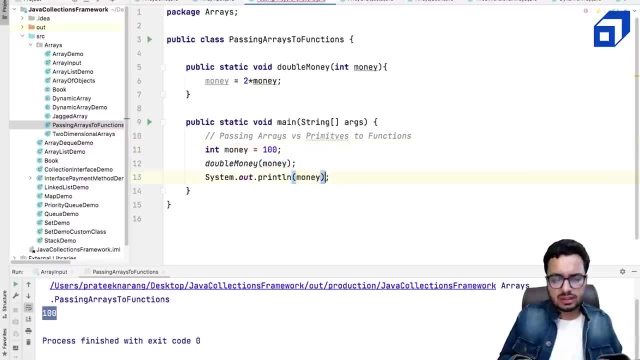 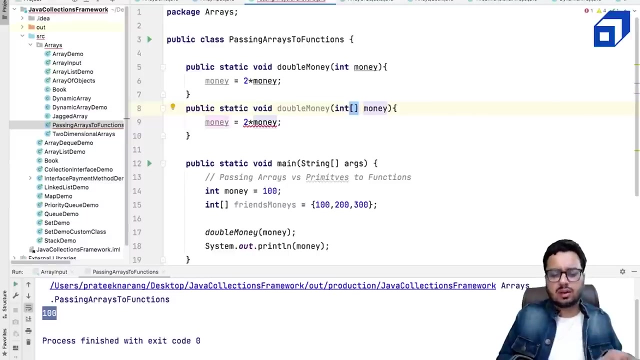 is okay. i have, uh, multiple friends and they have some money. so i say friends money, it's a integer array and let's say a friend has 200 and 300 and i create one more function called double money, which is going to accept money array or friends money, right, whatever you want to call it in this. 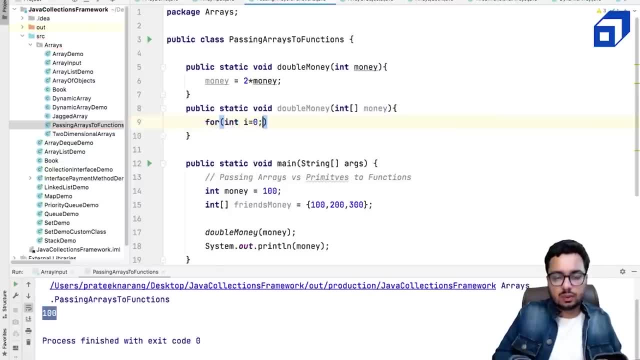 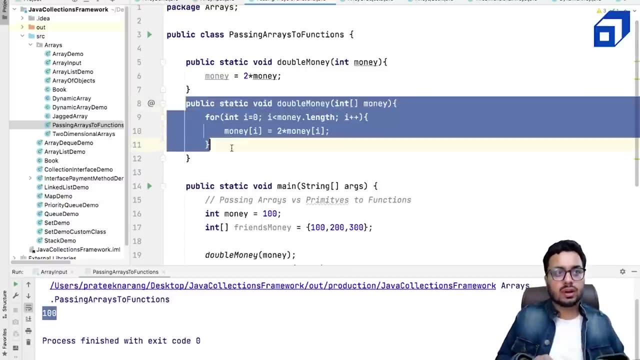 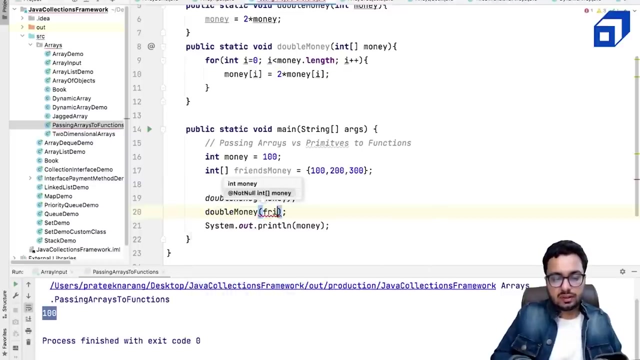 case i iterate over this array: for int i equal to zero, i less than money, dot length i plus plus and i say money of i should be twice of uh money off, and again i do not do anything, i do not return anything. now i again call this function, i call double money and i give friends money which is 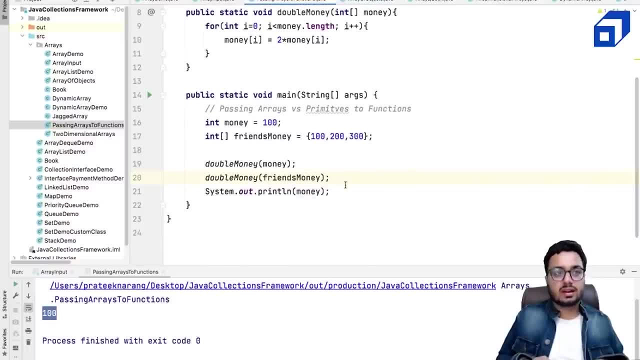 an array right now. what do you think? will my array get doubled? will my money in this array? will it get doubled? the answer is yes, it will. so let us see how and why it's going to happen. so if i print friends money and if i show you the output now, okay, i have to use the 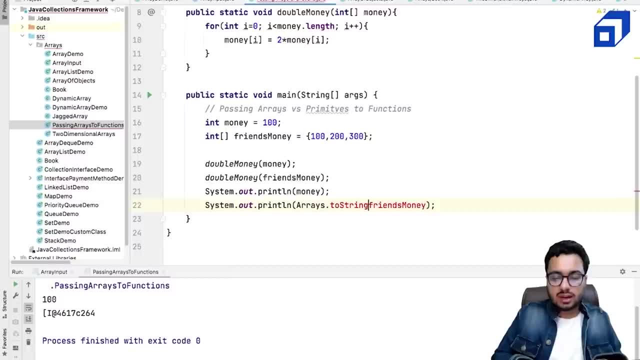 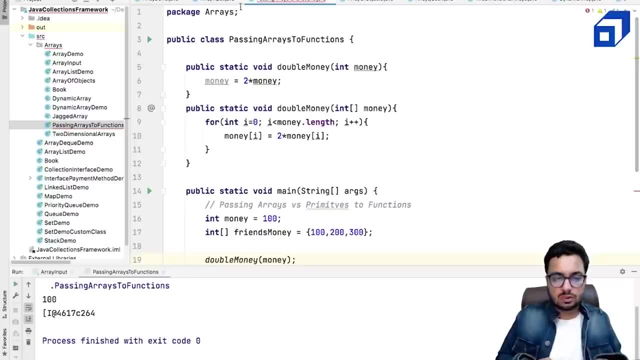 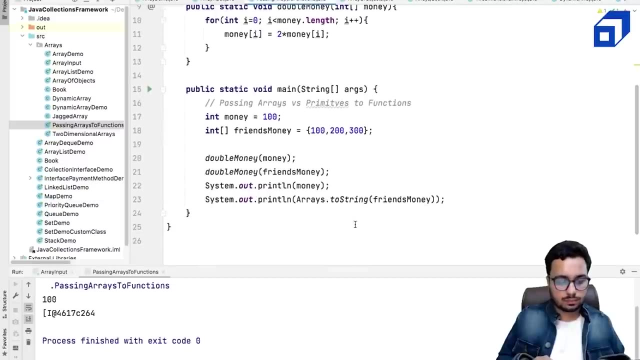 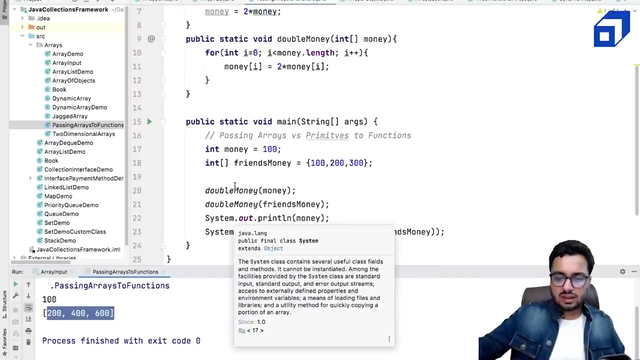 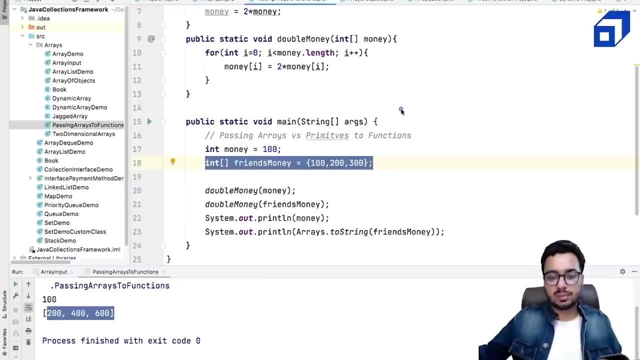 method arrays dot to string so that i can actually print the contents of the array. so now this money is actually getting 200, 400. so you might think it is not doubling for the primitive data type, but it is doubling for the array primitive. behind the scenes, what is happening? 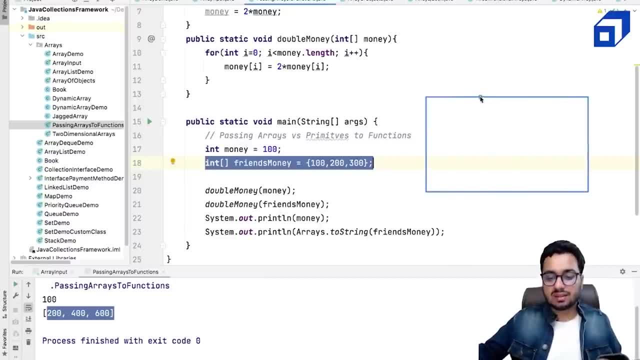 we have already seen. now let us see what is happening when you are passing an array. so you have your stack memory. i told you the array is created in the heap memory. you are 100, 200 and 300. they are created here, right, and they have some address. let's say the address is: 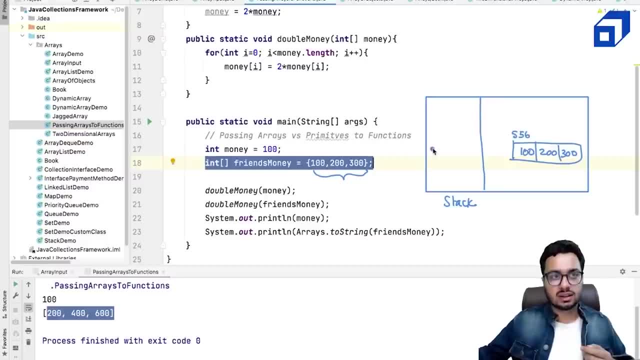 556. this is the location at which the array is created. when you called your main function, it got created in the stock, your variable friends money. it is also created here. what is this variable holding? it is holding the address of the array, so it is holding five, five, six. now, when you call this function, double money, you're passing the variable. 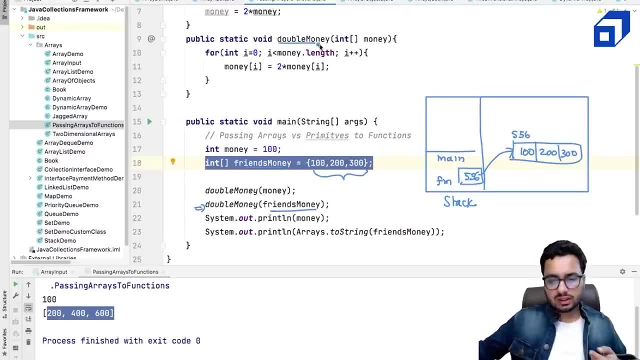 object: reference friends money to it. okay, so we are calling this function double money and it has a variable called as money, in which what is the value that is getting copied? it is not the array that is getting copied, it is the value inside this uh function variable friends. 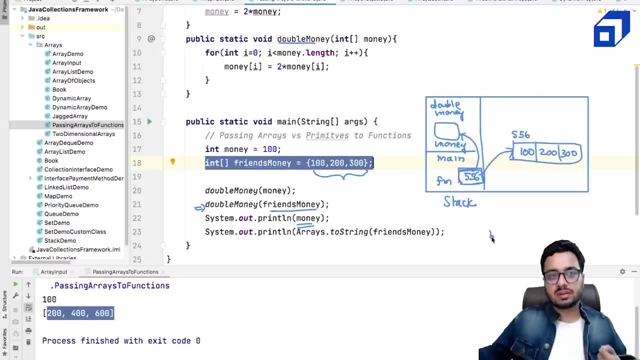 money. it is getting copied right. so in java everything is passed by value. okay, but in case of array, what is the value that is getting passed? it is not the array object, it is the address that is getting passed. you have five, five, six getting copied here. when you say, okay money, i equal to twice of money. so this money is also referring to the 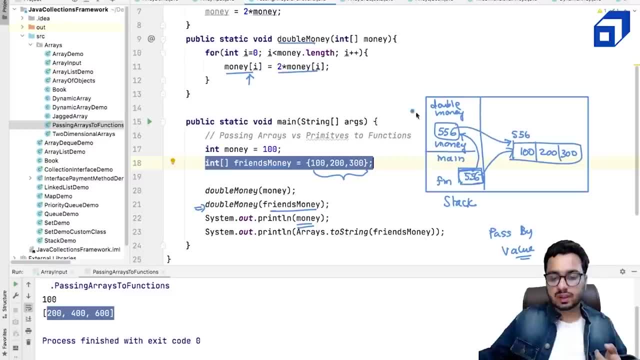 same array. when you access the ith location using this address, you eventually end up here. it's okay, money of i should be twice of money. you make it double, make it 400, you make it 600.. now this function is over. this is uh. this call is gone. this link is also gone, and when you come back, 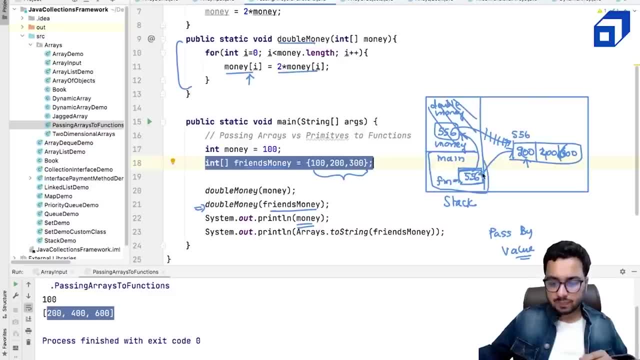 again here and you try to access the friends money array. the actual array has been changed, right. okay, so, although it appears like a pass by reference, but the concept is still called as pass by value in java. okay, but for the objects that are stored in the heap: okay so, objects in the heap. 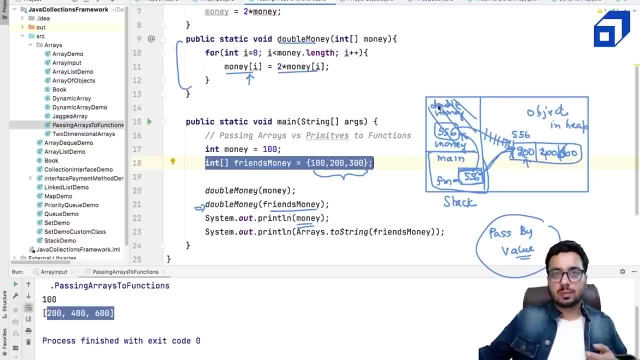 when you pass them to a function, their address is being passed. okay, that is something that you should know, and now i hope you are able to understand what happens when you pass an error, a function to change the array. the actual array will get changed if if you want to create a copy. 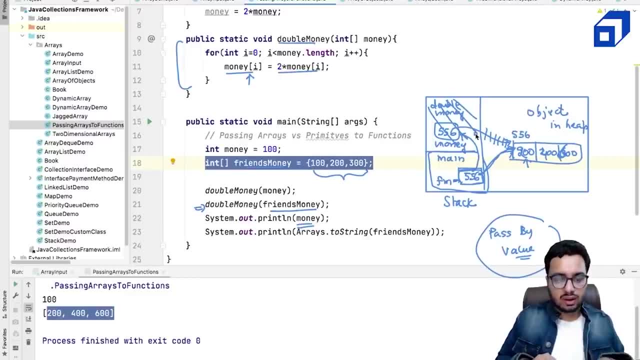 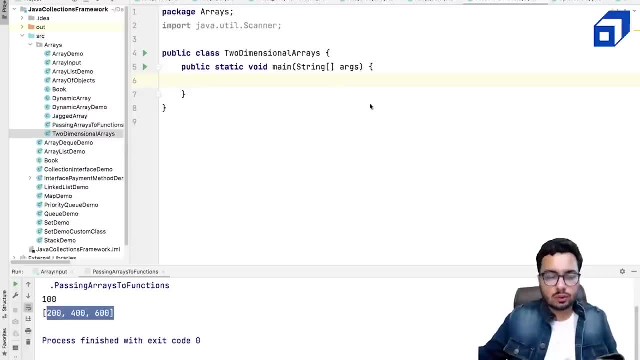 of the array. you have to use some methods like clone or what right, so that is how it is. are passed to a function. now let us move on to two dimensional arrays. okay, so many real life problems. for example, games and puzzles like tic tac toe. they might require you to store data in the form. 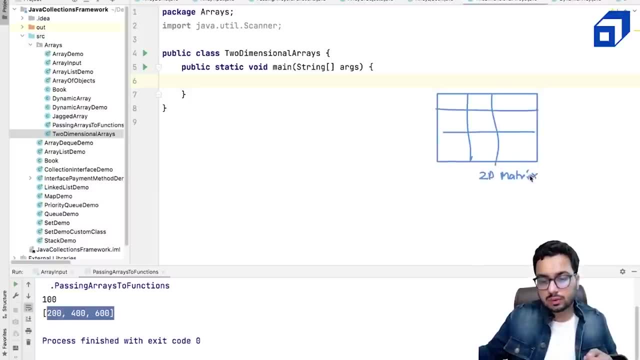 of a 2d matrix. now, if you want to store data in the form of a 2d matrix, you need a two dimensional array, right? you can also have a three dimensional, four dimensional, n dimensional array, right? how do we create such an array? i'll show you few ways to create these kind of arrays. so first i 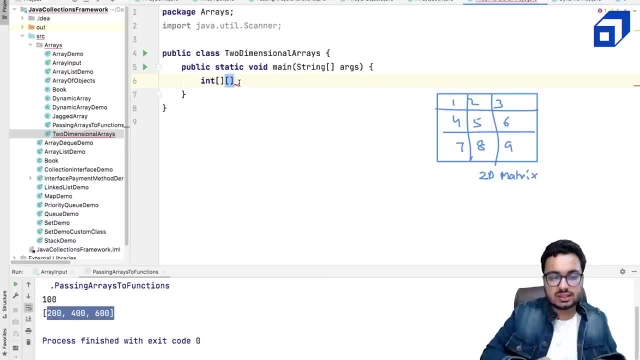 need to define the data type, and in this case it's a 2d array, so i will have to use these square brackets two times. i'll tell you the reason why, then. one ways i can directly give the data right now. if you look at data, 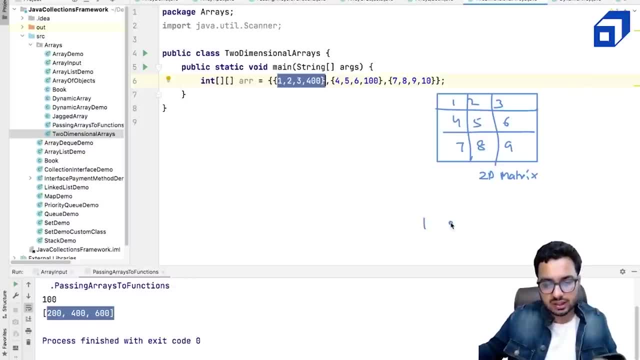 array. it has three rows and four columns. it is like one, two, three and four hundred. this is like one object. then i have four, five, six and hundred. this is like another object. and then i have seven, eight, nine and hundred. seven, eight, nine, hundred. this is like another one. now, 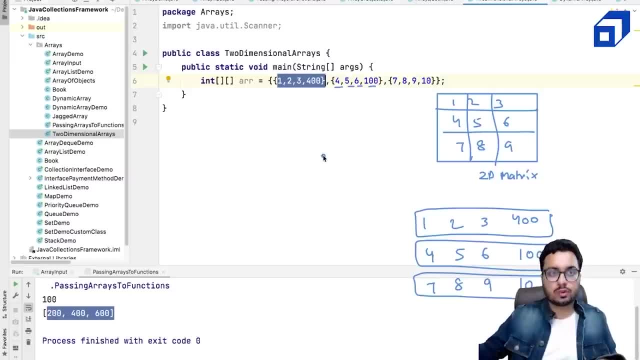 how they are stored internally, the memory. let us discover. for java, 2d array is nothing, but it's a 1d array in which each, each row, or each, uh, each row is like one object, right? so can i say it's a 1d array in? 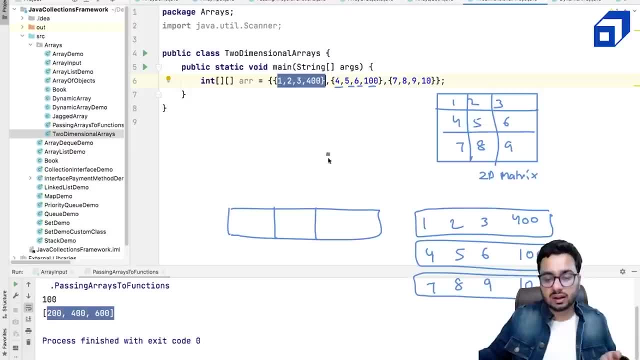 of objects where each object itself is a one dimension. so in the memory there is no 2d array created internally. it's going to use a 1d array where i can say: the 0 throw this. this element is my array of 0.. array of 0 itself is an array. that is what i'm trying to tell here. array of 0 is of. 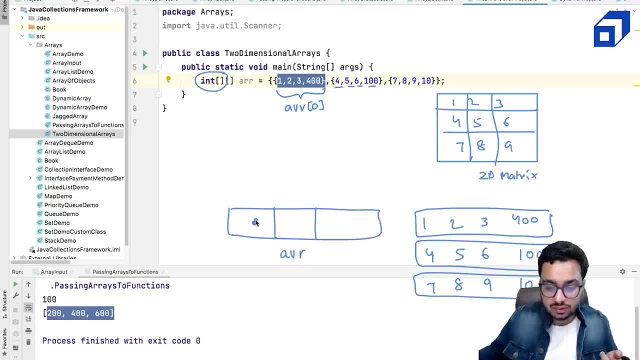 the type intr square brackets. that means array of 0 represents 1d array. array of 0 is going to hold the address of another 1d array. let's say this address is some something. that address will be present here. specify area of one that is also going to hold. 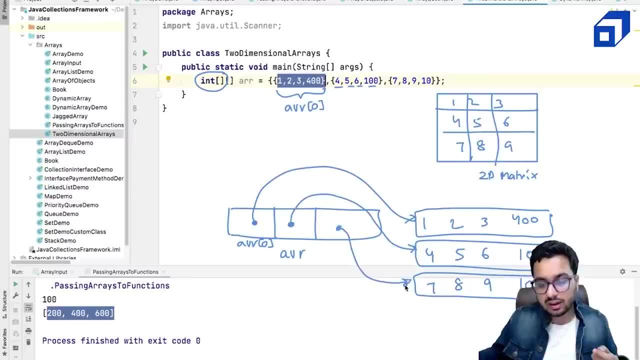 the address of another array and area of 2 it's also going to hold the address of another. this is area of 1 and this is exactly how it is stored. and where is your error? error is here this variable, it is in the stack memory. and these arrays, these four arrays, they are in the 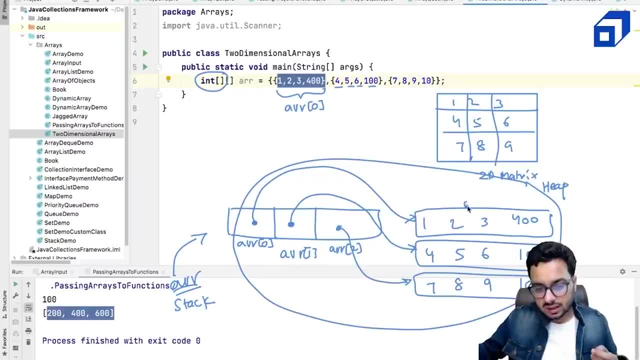 okay, this. i am saying this is a object. a 2d array is nothing, but it's a 1d array of object, 1d array of objects, where each object is also an array. this treated like this way, right? so treat it like this is one book. this is another book. this is another book, right? each row is one. 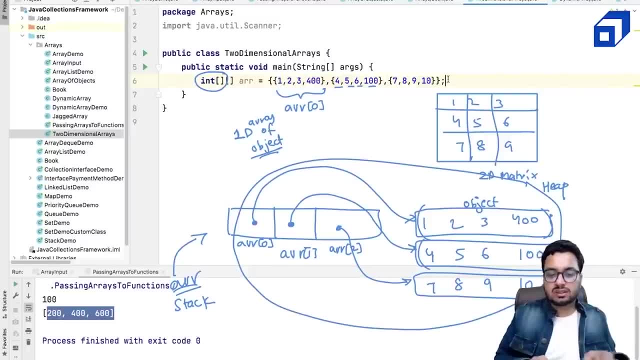 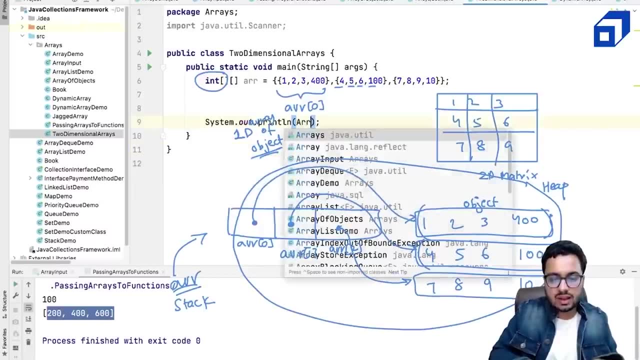 object. now you might say: okay, prove me, this is how it is told. so let us uh go and do s out. let me show you. um, i can say arrays, dot to string. i want to to print this array, i give arr and again i will import java dot, util dot if i make this import. 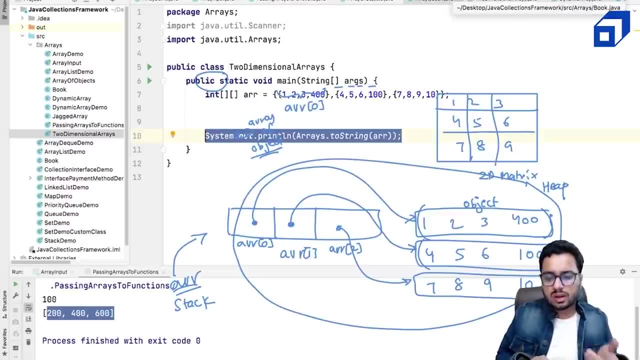 and i call this method: arrays- dot to string. now what i am hoping to get. will i get the contents of the array or will i get these addresses? let us see what do we really get. i need to run this. look at this. i am getting three addresses. what are these three addresses? these are the three. 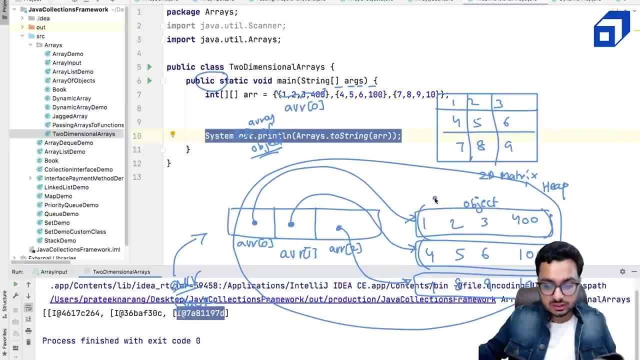 addresses of these three row objects that we have created. this is two, six, four. this is stored here. this is 30c. this is this is the address 30c and this is one nine seven. one one nine seven. this is the address of enough. then you might ask: okay, if i want to print a 2d array. 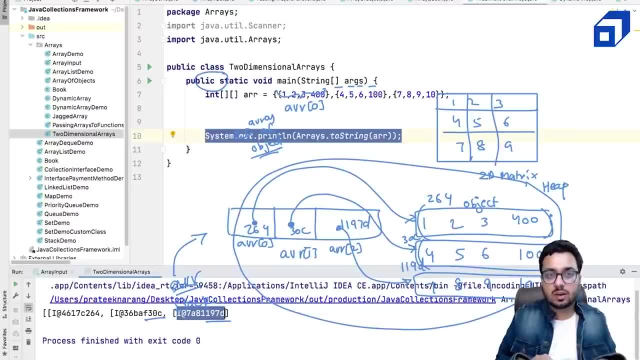 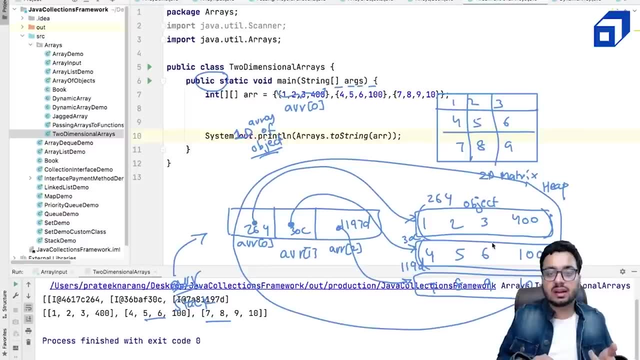 using a true two string method. can i do that or should i iterate over this array? i will tell you: you can do both, please. you can use an inbuilt method to print this entire array. you can also iterate over this array. let us first look at a inbuilt 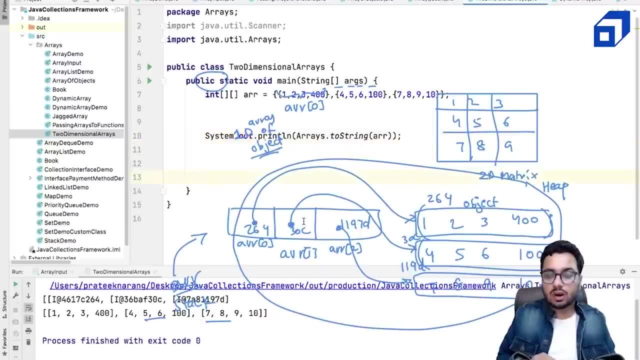 method. if, if you have a structure like this, it's so you have to. you just don't need to iterate over these values, but instead you need to say, okay, i also need to iterate the objects they're referring to, right? so basically it's kind of a recursive structure, right? so this is referring to some. 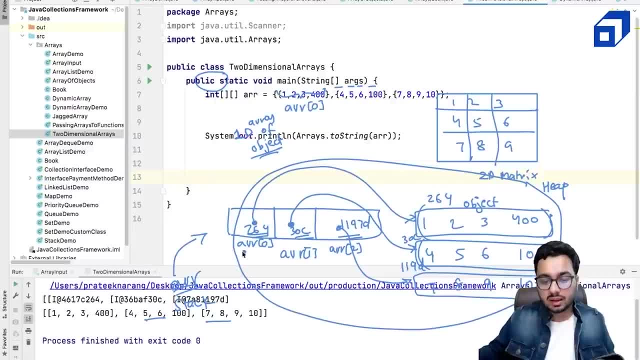 object. this might also be referring to some some other object. so i want to go deep inside this, all the values, right. in order to do an iteration like this, what i have to do i have to use a method called, as it is, dot, deep to string. i iterate deeply inside these structures and then print. 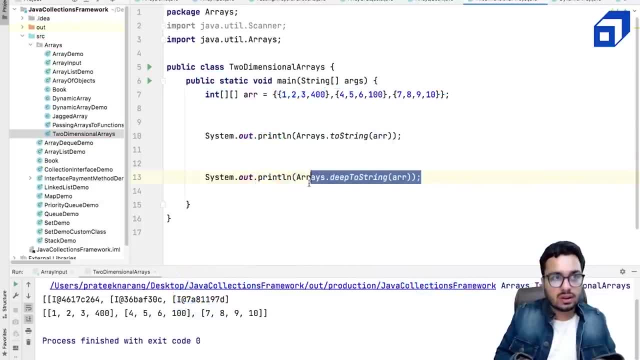 this array. if i call this method right, there is dot deep to string. what will happen? it will go inside those arrays, those rows as well, and it will print them right. if i go and run this code, you can see this is the output that i'm getting right, so i hope you are able to understand the 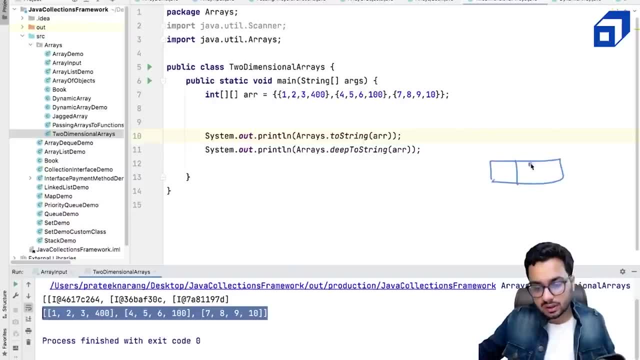 difference. okay, now how this 2dr is dot. just a quick recap: this array, this arr, is a 1d array which is holding three rows in it. so three rows. each row is a 1d array object containing four numbers. so now let us do one more thing. let us write a method. 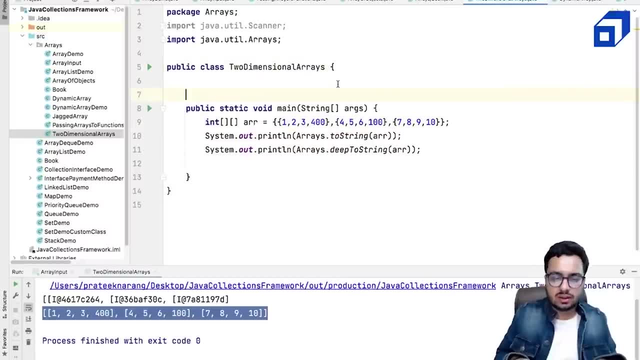 called zero in the blueprint for that array so i'm gonna add a keymaxAdject entered here. i will called as print that is going to iterate on this 2d. Sometimes we have to manually use a for loop to iterate over a 2d array. Let's see how we can do it. So public void: public. 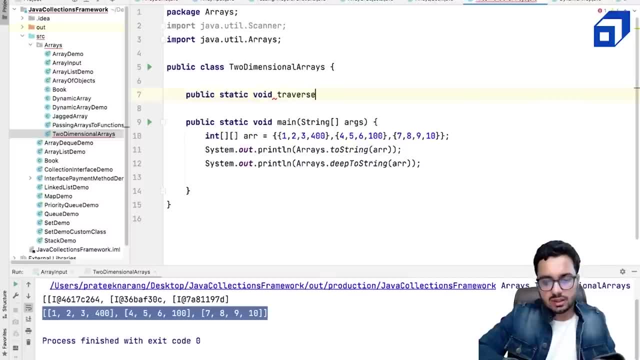 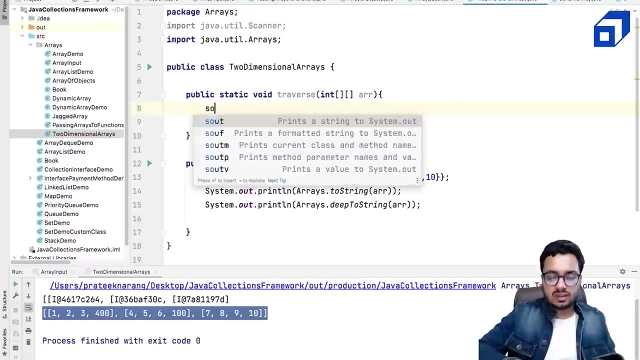 static void, etc. verse input is a 2d array, So I will create a reference variable, ARR. How do I iterate If I simply say see s out error dot length. can you guess what is this length going to be? What is the length of this array? this array is holding three items. 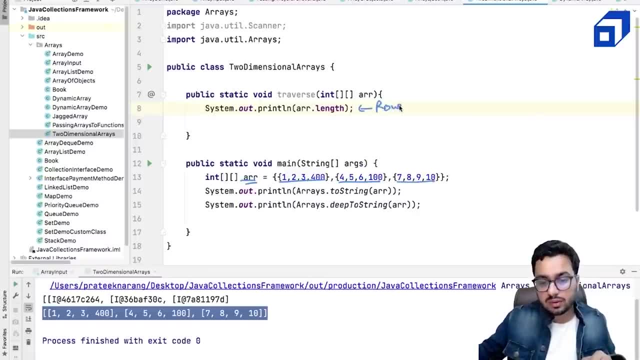 this length is giving me the number of rows I have. if you want to figure out how many rows I have in this array, these are the number of rows, how many columns I have in this. that is nothing, but the number of elements in each array is the number of columns I. 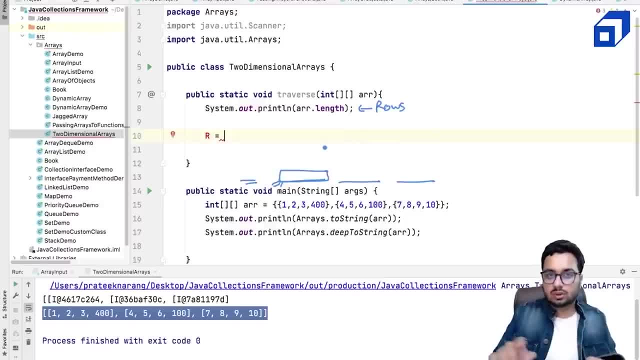 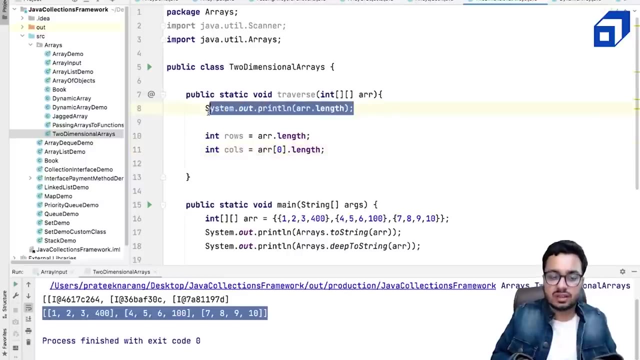 can say if it is a big size array- rows cross columns- the rows will be nothing but number. of rows will be nothing but array. Now, length, how many columns i will have? that is nothing but array of zero dot. length: the number of elements in the first array. if this is same across like all the arrays. 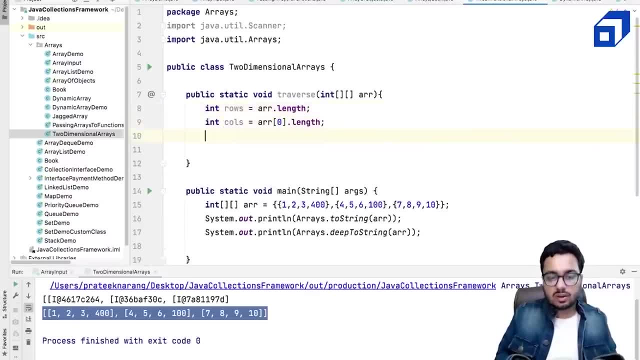 the number of columns. i don't like. how do i iterate? iteration is pretty easy. i can say i equal to zero, i less than the number of rows, i plus plus. and then i can say: okay for j equal to zero, j less than the number of columns, j plus plus s out array of i, j. so let's see, uh what? 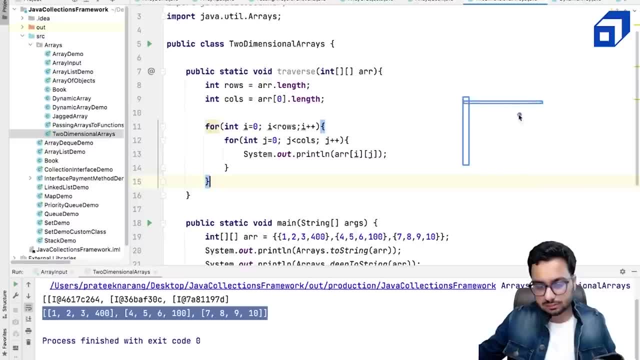 does it really mean? so if i have an array like this, let's say 1, 2, 3, 4, 5, 6, 7, 8, 9, this is one object. another object: this is array of zero. i iterate over rows. i is zero, so array of zero is fixed. 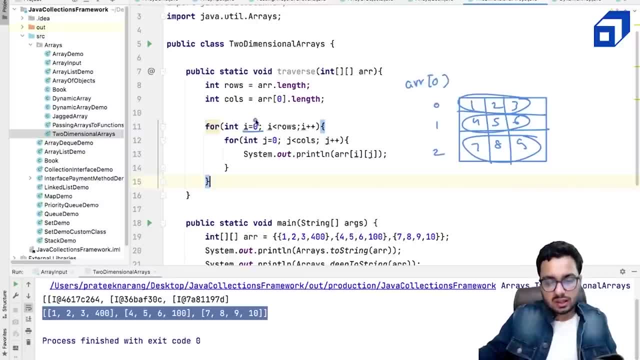 if i go over 0, 1, 2, these are the row numbers. for each row number, i say: okay, i trade over the columns. array of: i gives me this. then, using this, j gives me the column. so, array of zero: zero gives me one. array of zero: one gives me two. array of zero: two gives me this number. so j is going along. 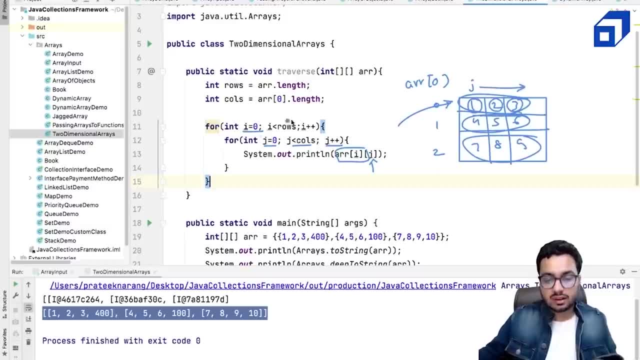 this direction. i is changing across row right. so what i'm doing i'm going over each ith object and then i'm using a j to traverse the elements of that particular row. this is how we generally do the traversal right. you can also do it other way around, so i'm iterating across the rows. 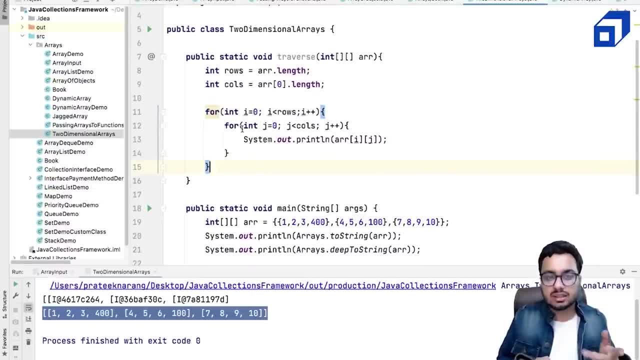 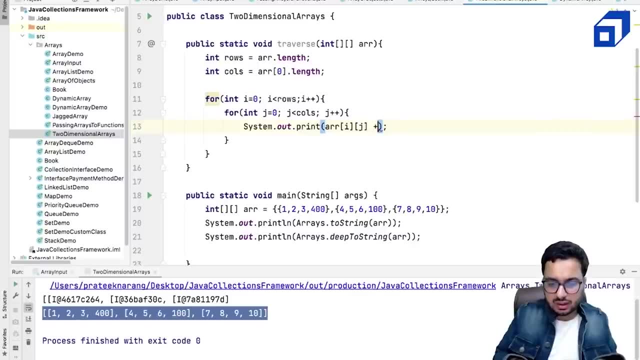 you can also iterate across the columns by changing the order of these. if i show you the output, it's okay. i'm going to print them in the same line and after my row is finished i'm going to give a new line so i can say s out. 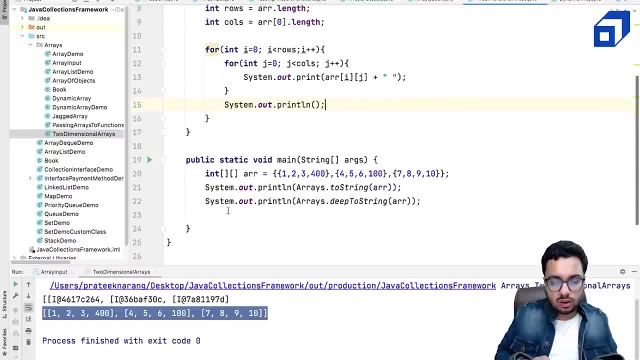 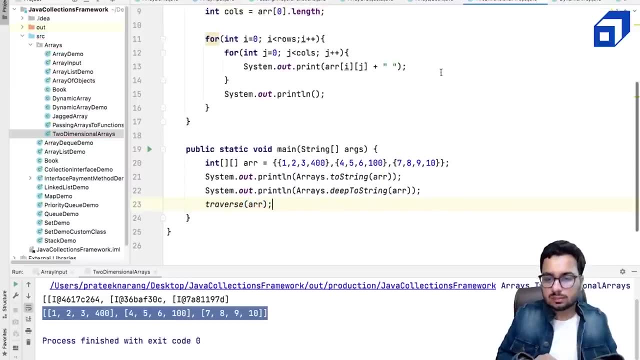 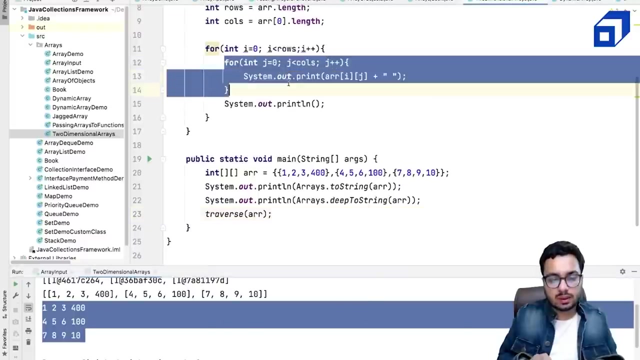 and ln. so now, if i call this method that is going to be traverse, and i give this array, i will see an output which looks like a 2d array. right, let us go and run this code and you can see it. so i'm able to iterate over all the rows and for each row, i'm able to iterate over all the columns of that. 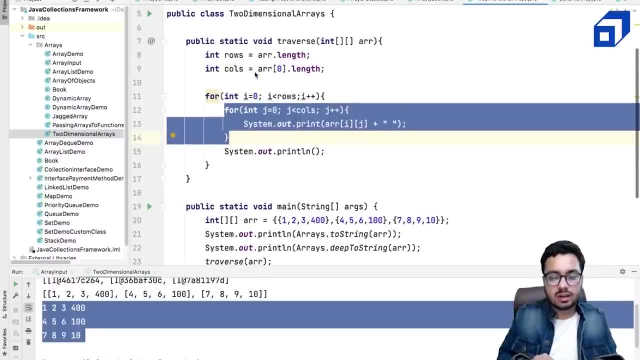 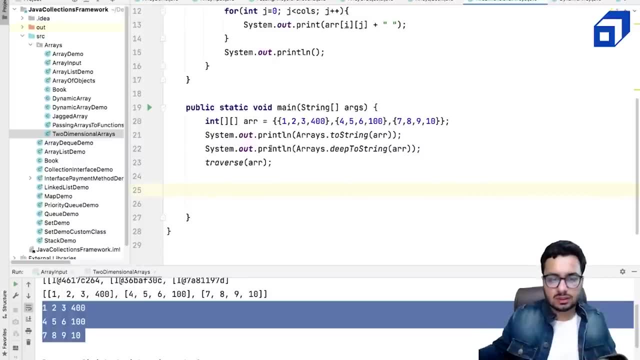 particular row or all the numbers in that particular. so i hope you guys have learned. traversal is clear to you. now some of you might ask that, okay, can we do, uh, some kind of sorting on this 2d array? maybe i want to compare each row with some other row. okay, so i want to do sorting. 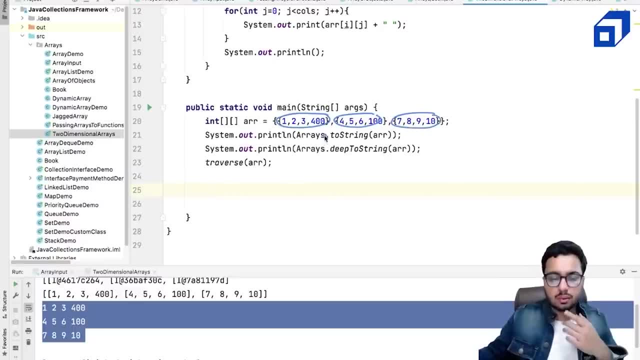 uh, across the rows. i want to sort rows and you might have a different criteria. you might say, okay, i want to sort on the basis of first element, or i might want to consider the sum of all elements, right? so how do i do that? so it's very easy. so, consider each row as one object and i want to. 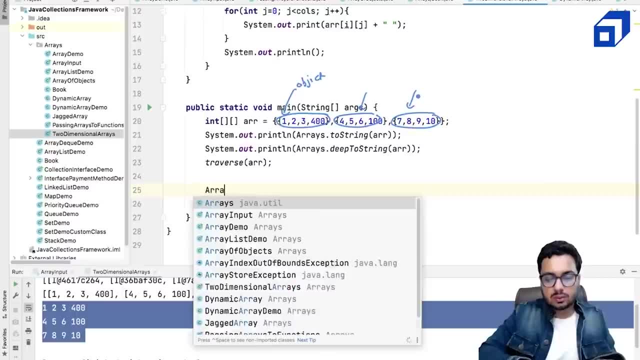 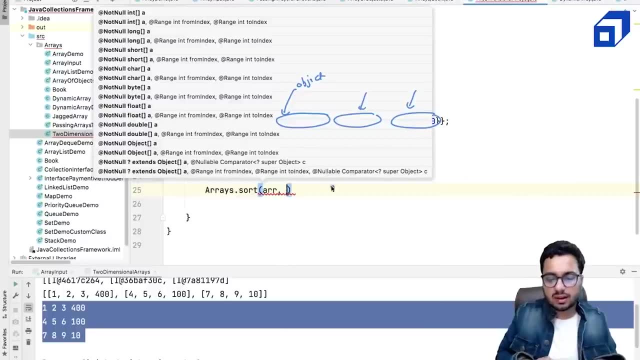 compare this with other elements, objects. What I can do, I can use errors dot sort method. it will assume that I'm going to give you a 1d array. That's okay, So it's going to. and this: this is actually a 1d, Okay. 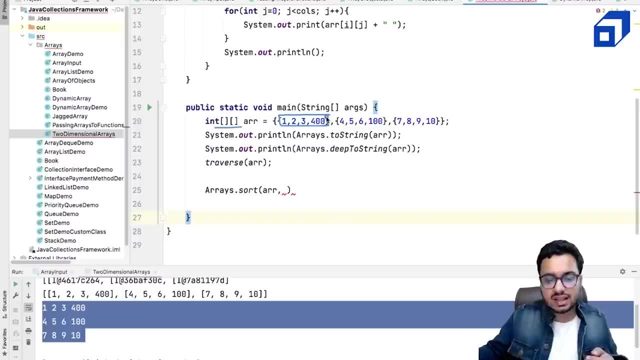 although the syntax is 2d array, but Java considers this as one element of the array. This has another element of the array and this has another element, Suppose, if I want to sort according to their sum, right, What I have to do is okay, fine, I will give you. 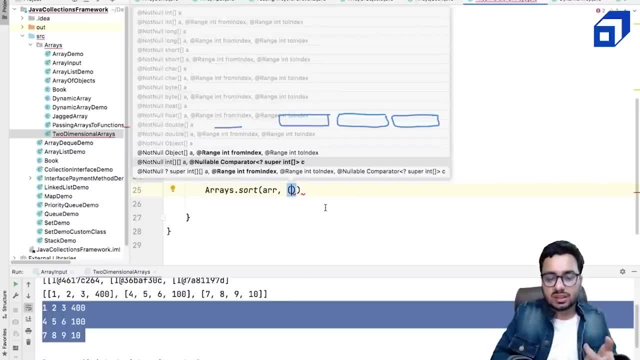 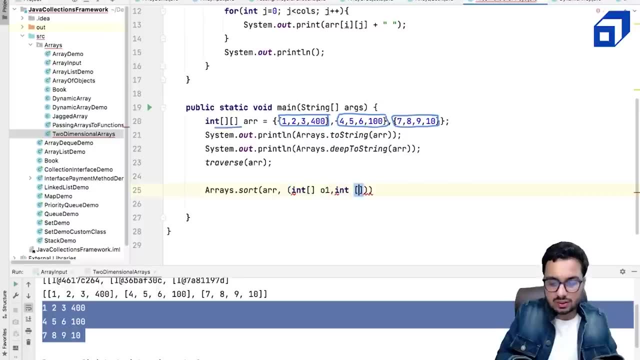 two objects. What are the data types of these two objects? these two objects are arrays. I have int square brackets, object one, int square brackets, object two, And in return I want to get their sum. So I can joke, I can create some method called as get some in public. 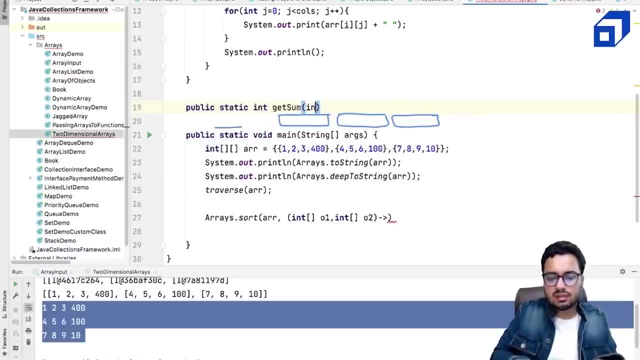 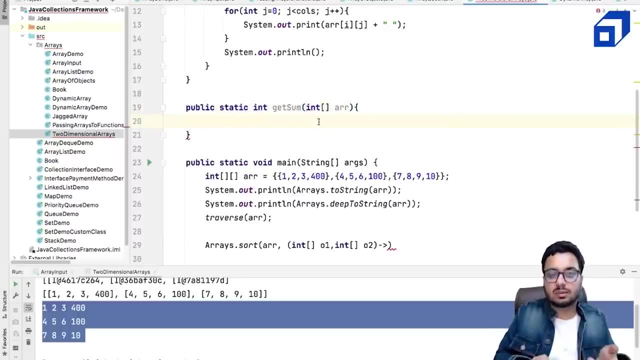 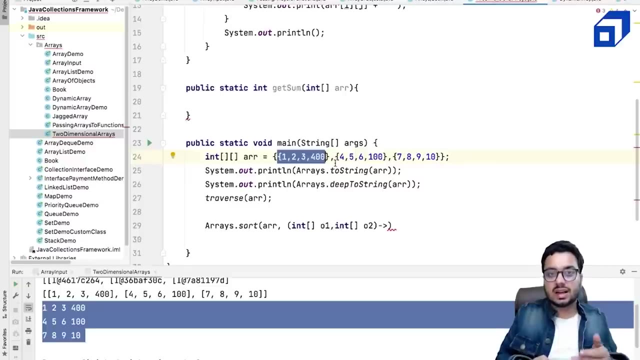 static int get some, even a 1d array. I want to find the sum of that array. I give some array. I want to find the sum of that. I want to sort these rows according to their sum. Basically, the row which has a higher sum should come at the end of this array. How do I do it? 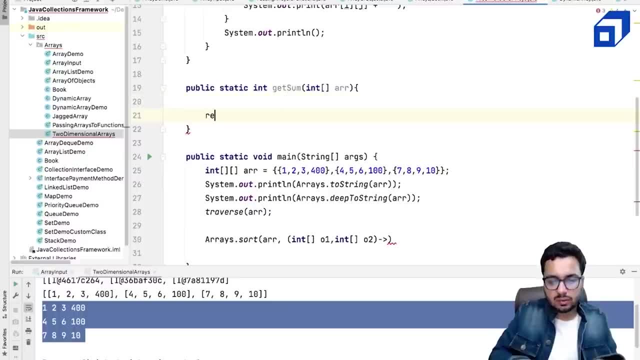 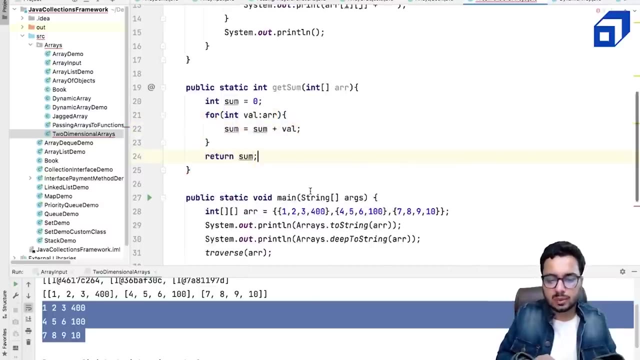 First let's write a helper function to get the sum. So for now I can say: int sum equals to zero or int value inside this array, I can sum equal to sum plus value And I can return. This is pretty easy. Now here in my lambda expression, I can say: okay, I'm going to compare. 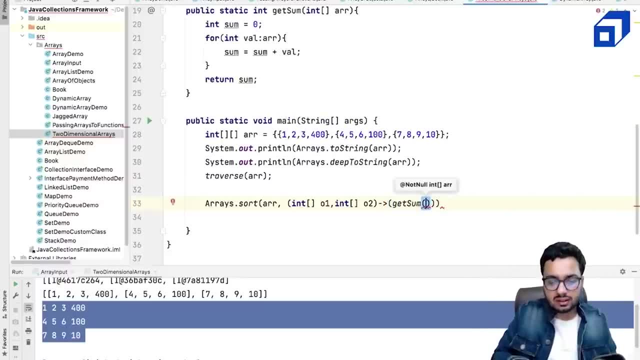 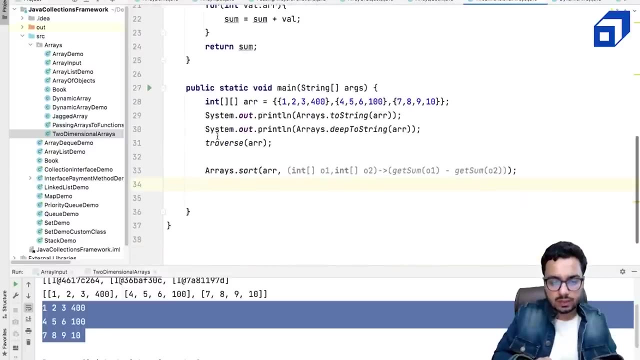 on the basis of sum of these arrays. So array one, which is my object one, minus get sum of array two, which is my object two. That's it. And if I do this- and now I want to show you the output- I can again print this array after doing the sorting, And let us see what. 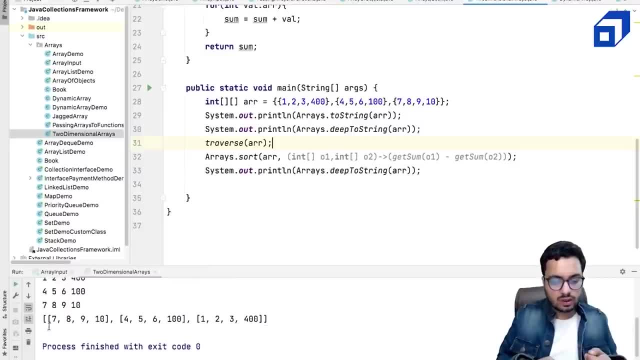 do we really get? Now, if you look carefully, I'm getting this array first, which has the least sum. this array has a higher sum And this array has even the highest sum by because I'm I have a very big element- 400,. you can verify what I have done. I have written a lambda function. 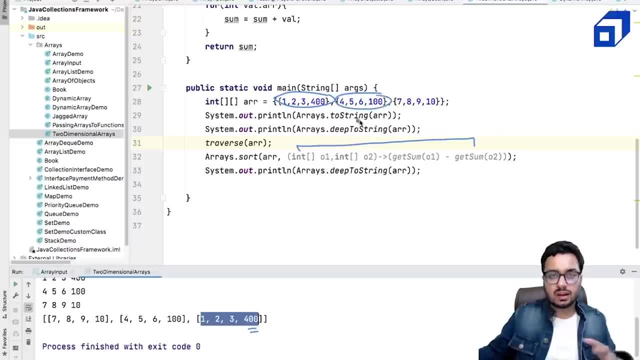 that is comparing two rows any like internally. it will call some logic to compare two rows. okay, It is comparing two rows According to their sum. if you want to compare on the basis of first element or the last element, that that that can also be done by do this once again. here I can do okay, one. 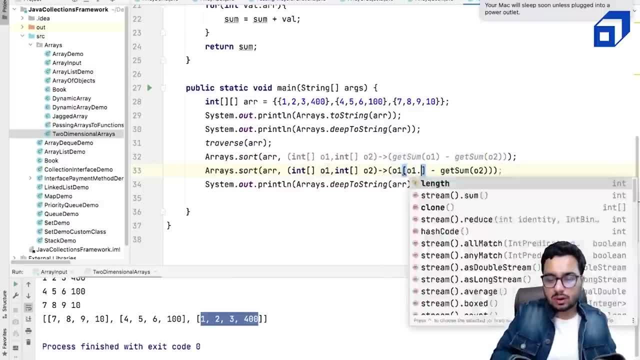 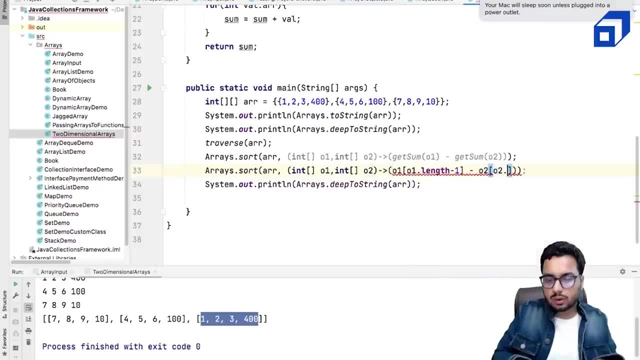 dot get last element. how do I get it into? okay over and dot n minus one, that is giving me the last element and O two of O two dot length. I'm saying, okay, Let us compare On the basis of last element. in that case this array will come first and this array. 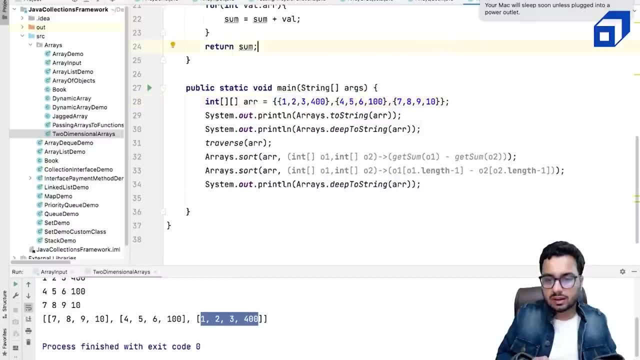 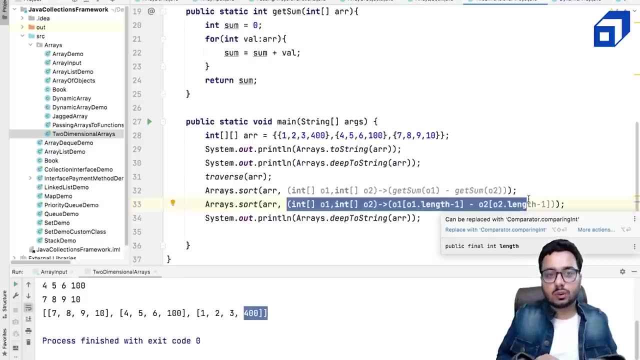 will come, and then this array will come. If I go and run the code once again, let's see what do we really get. Okay, so I'm getting n, red and 400.. That is how powerful these lambda functions are. They can also work with 2d arrays. 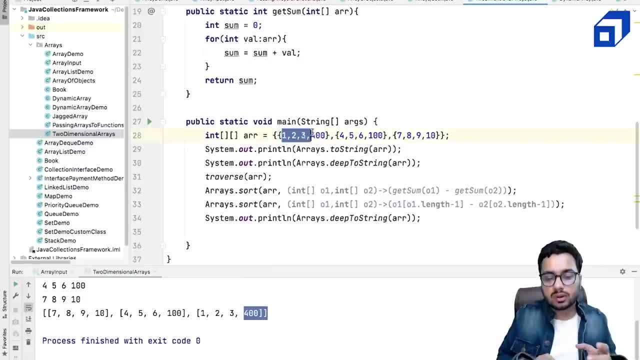 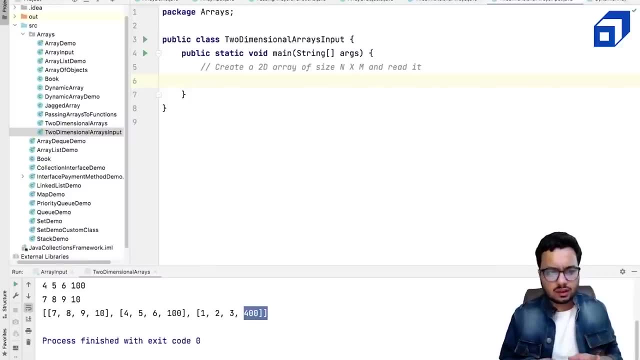 But now you're not going to compare, you're going to come, you're going to treat each row as one object. That is something that you must learn. We have seen how do we work with a 2d array, but we have not seen how do we take input. 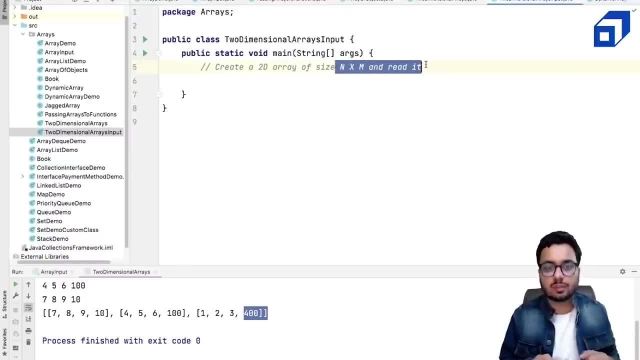 a 2d array of size n, cross m and read it from the user. Okay, Let us do that as well. First of all, I'll create a scanner so that we can read numbers from the user. So scanner SC- this is equal to use scanner. 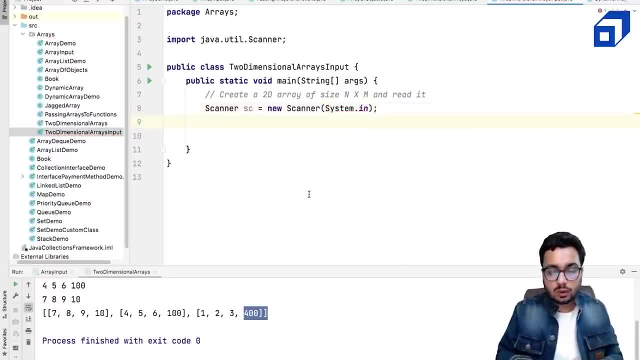 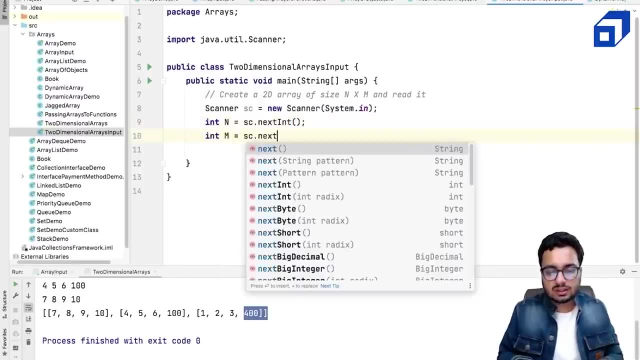 And let's read: Okay, Let's see how many rows we want to create. number of rows is scanner dot next, and number of columns is also going to be standard. So I'm going to create a 2d array of size n cross m. how do I do it? pretty simple. 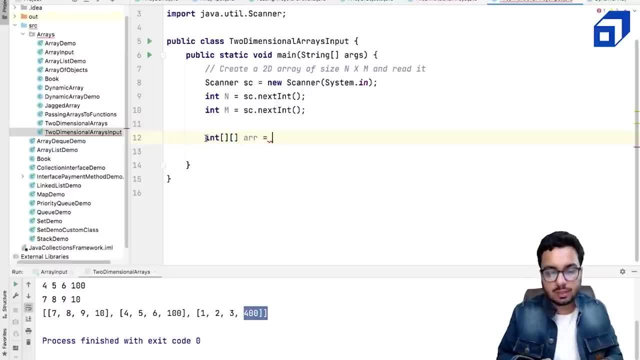 So I define variable. ARR is of the type int- square bracket- square bracket. this is equal to new int, And here I define the number of rows is n and the number of columns, which is m. Once I do this, Java will create an array. 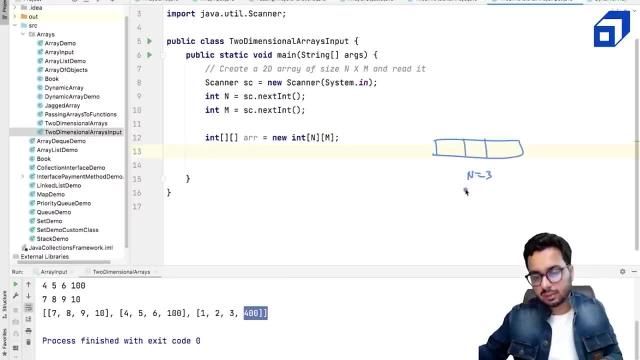 In which I have, let's say, n equal to three and Ms, for it's going to link these like that internally. This is how they will get hated. Now, what I want to do, I want to read numbers and put put them here. I want to show: the 123 is the first row. 5678 is the another row. 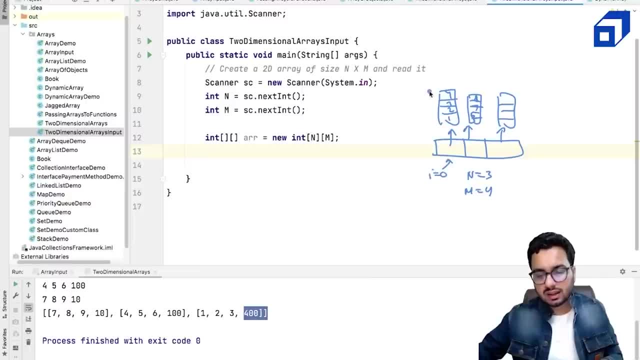 How do I do it? I have to go to the zeros index. then I have to iterate over from j equal to zero till j equal to 3012.. Okay, Then I have to go to this index. read this array. I have to go to this index. read this: 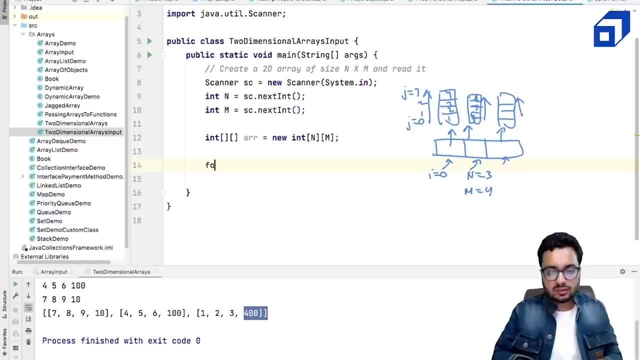 array. Let's see how we can do it. I can say for int: i equal to zero, i less than n, i plus plus. then for each row I need to read the elements: j equal to zero, j less than m, j plus plus, and array of i comma j. 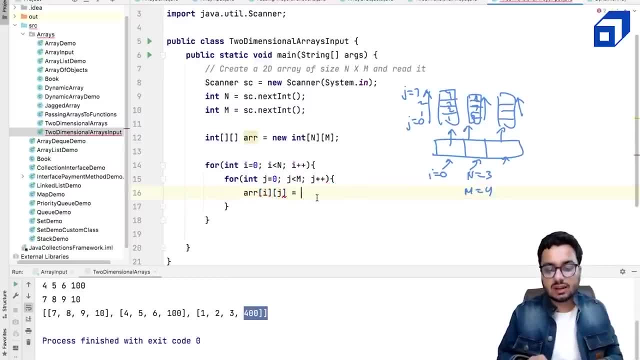 In the ith row, The jth. Well, I want to read a number and a dot extent. fine, This is it. It's. once this is done, I have read all the elements and what I need to do. I need to print. 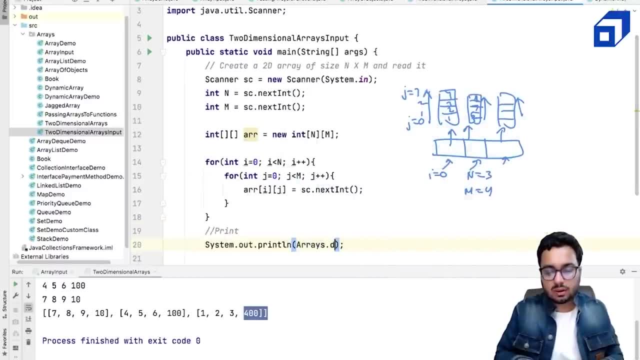 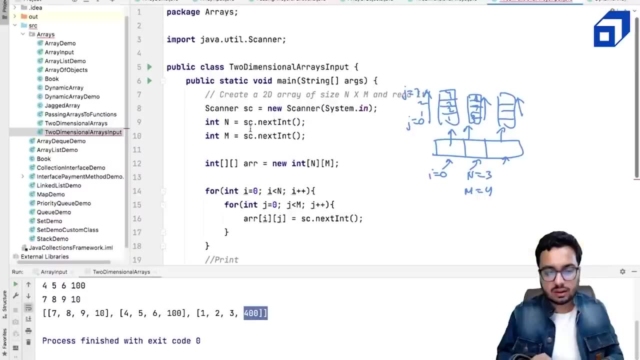 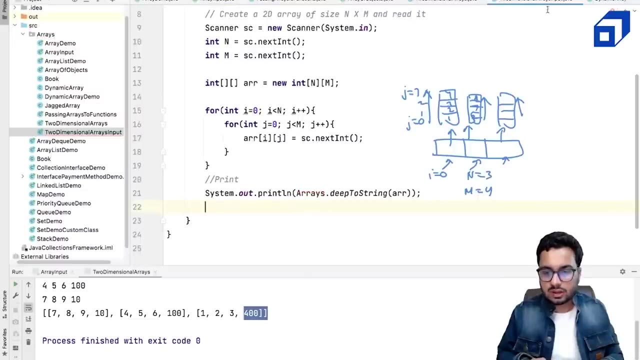 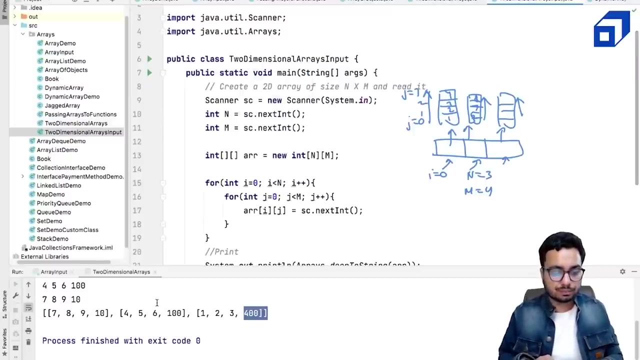 so I can say: okay s out, it is dot deep to string and I will give it. I need to import Java dot. So let us run this code and see are we able to read an array from the user or not. Let's say I want to have three rows and four columns. 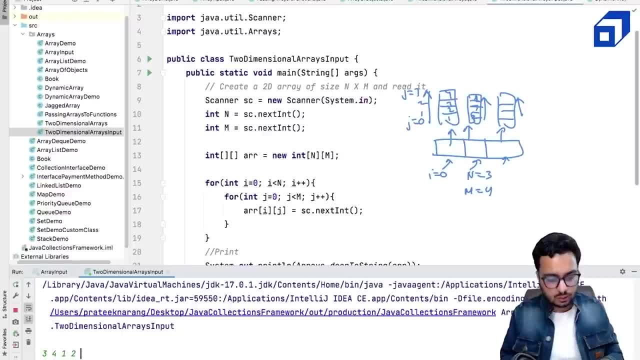 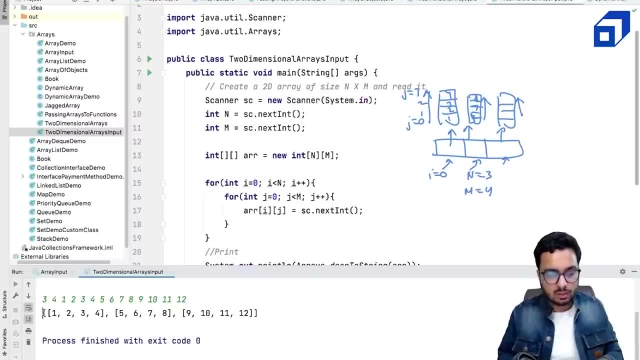 I need to give data. Let's say I'll give 12 elements: 123456789, 1011.. So, yes, I'm able to create an array with three rows and four columns and you can see: first row, Second row and the third. 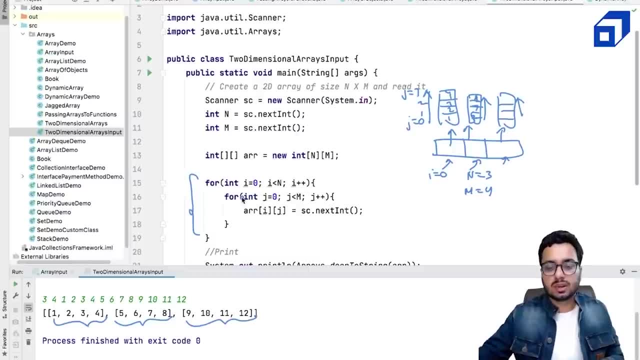 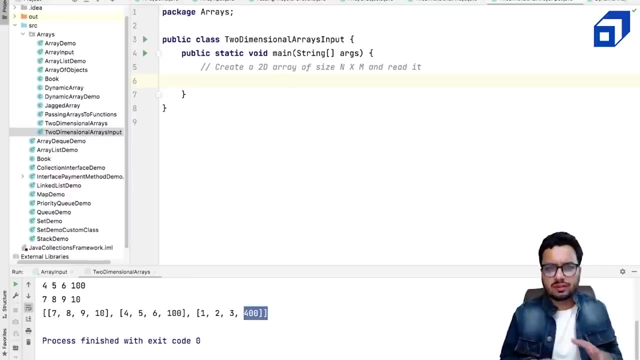 So this is how exactly we get a two dimensional array, And this is how the memory representation of 2d array looks like. This is my variable, ARR. Okay, so let's move on to jagged array. next, we have seen how do we work with a 2d array. 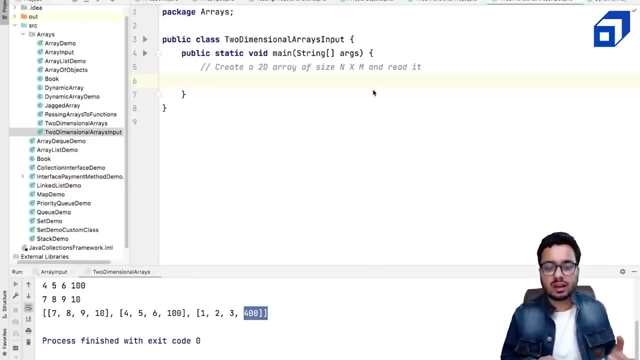 but we have not seen how do we take input- a 2d array of size n, cross m and read it from the user. Okay, let us do that as well. First of all, I'll create a scanner so that we can read numbers from the user. 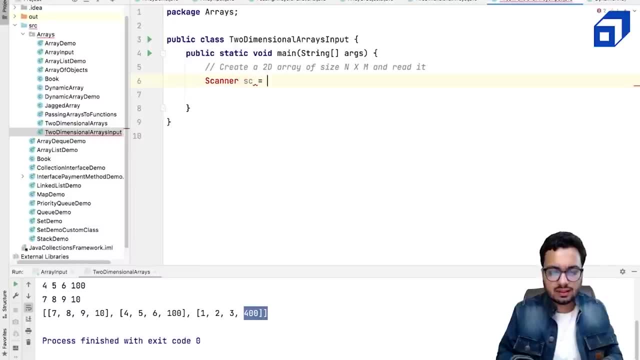 So scanner SC, this is equal to use scanner, And let's read how many rows we want to create. number of rows is scanner dot next, and number of columns is also going to be standard. So I'm going to create a 2d array of size and cross them. 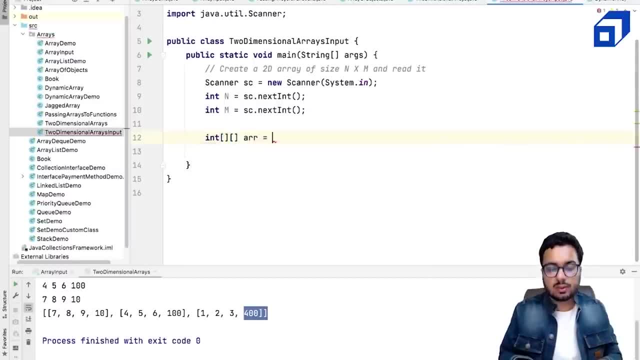 How do I do it? Pretty simple, So I define variable. ARR is of the type int- square bracket, square bracket. this is equal to new int, And here I define the number of rows is n and the number of columns, which is m. Once I do this, Java will create an array in which I have, let's say, n equal to three. 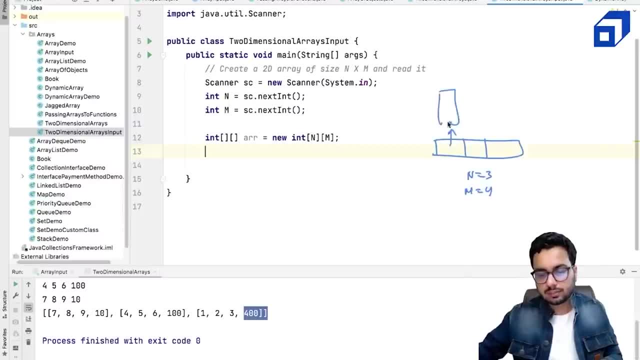 and m is four. It's going to link these like that internally. this is how they will get created. Now, What I want to do, I want to read numbers and put, put them here. I want to show: the 123 is the first row, 5678 is the another row. how do I do it? I have 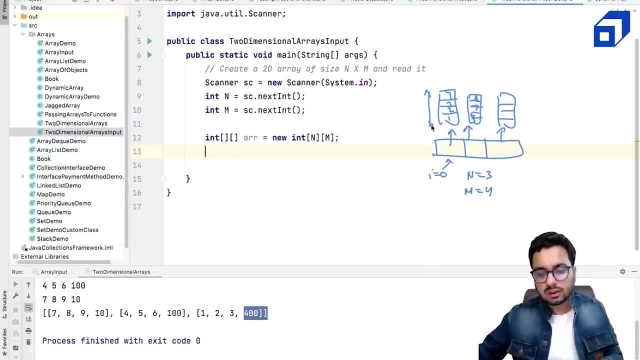 to go to the zeros index. then I have to iterate over from j equal to zero till j equal to 3012.. Then I have to go to this index. read this array. I have to go to this index. read this array. 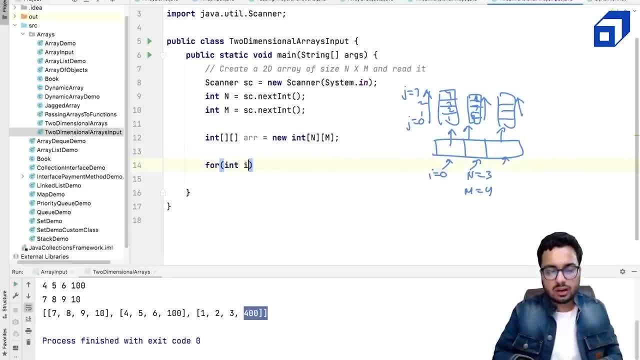 Let's see how we can do it. I can say for int: i. equal to zero, i less than n, i plus four. Then for each row I need to read the elements: equal to zero, j less than m, a plus plus, and array of i comma j. 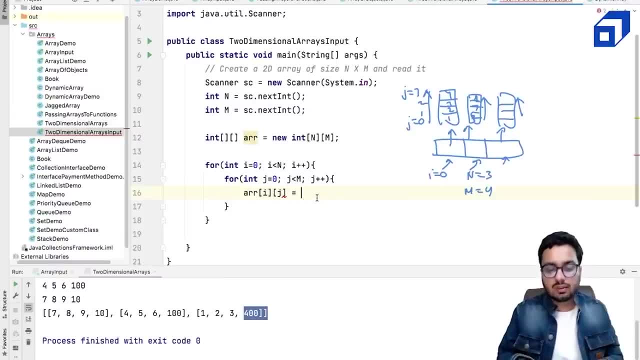 In the ith row, the jth cell. I want to read a number and a dot extent. fine, This is it. It's once this is done, I have read all the elements and what I need to do. I need to print. 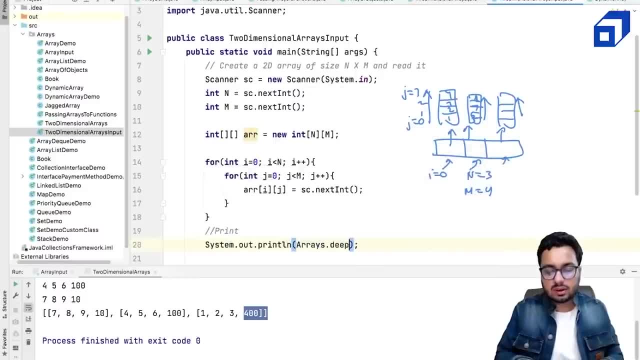 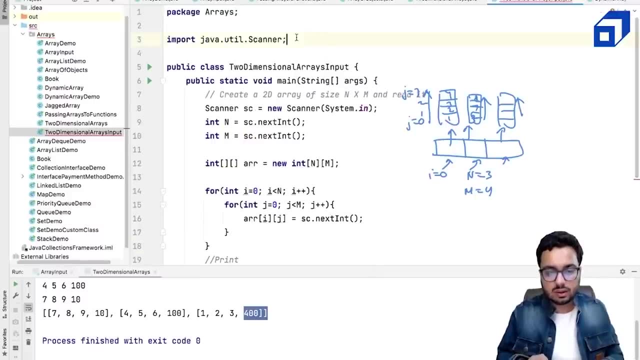 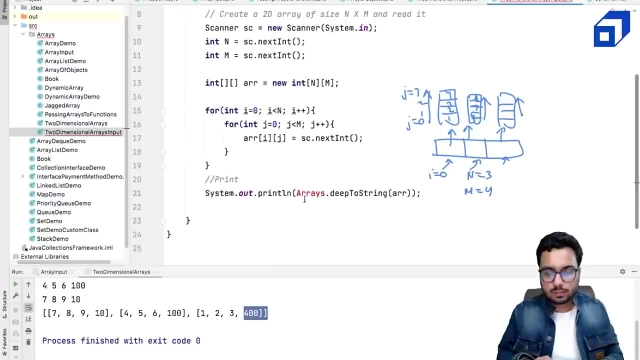 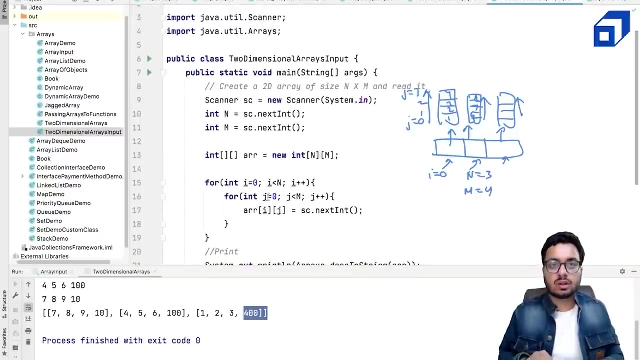 So I can say: okay, S out, it is dot deep to string And I will give it. I need to import Java dot to tilde. So let us run this code and see are we able to read an array from the user or not. 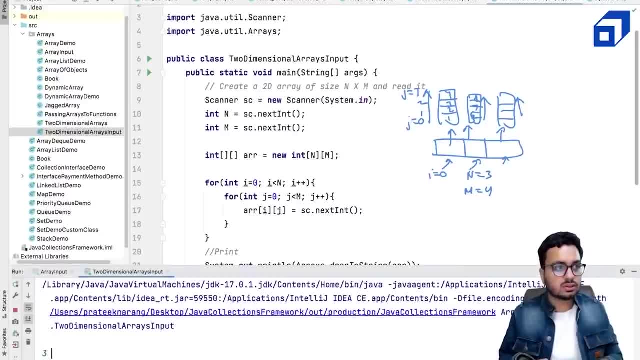 Let's say I want to have three rows And four columns. I need to give data. let's say I'll give 12 elements: 1, 2, 3, 4, 1, 2, 3, 4, 5, 6, 7, 8, 9,, 10, 11.. 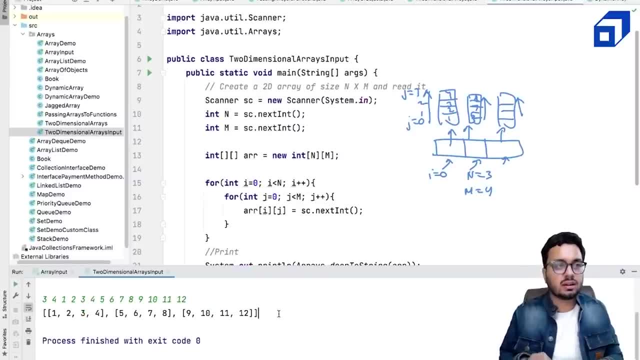 So, yes, I'm able to create an array with three rows and four columns, And you can see first row, second row and the third. So this is how exactly we get a two dimensional array And this is how The memory representation of 2d array looks like. 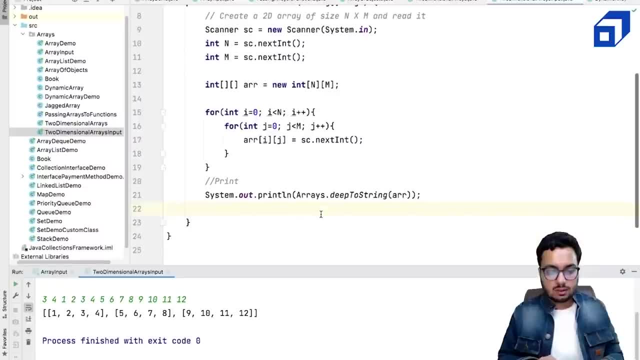 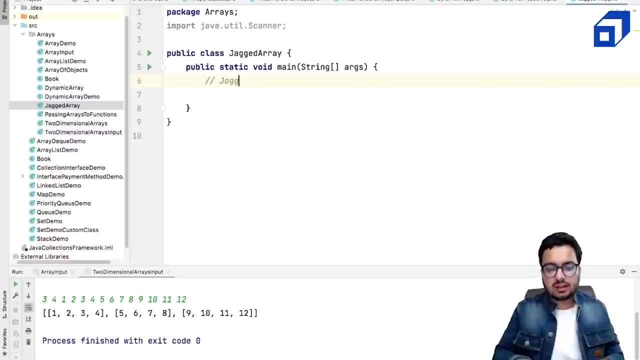 This is my variable ARR. Okay, so let's move on to jagged array. next let us discuss what is a jagged array. A jagged array is an array with variable number of columns. variable number of columns. How this is possible, let's see. it's an example. let's say I have three columns in one row. 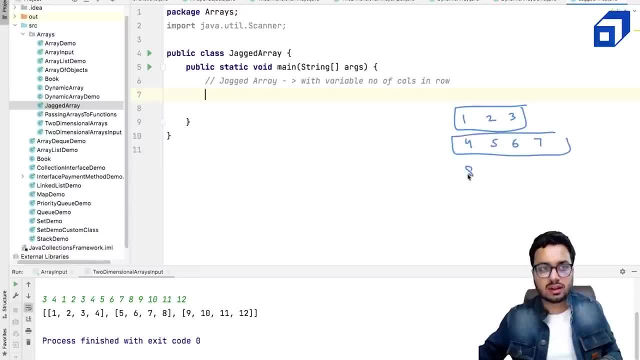 In another row I have, let's say, four columns, And in another row I have just two columns. Can we create such an array? The answer is yes. Why? Because when you create a 2d array in Java, each bucket is referring to an array object. 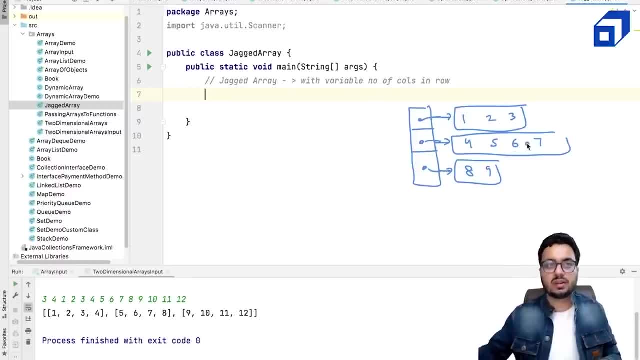 Each array object is independent of the previous object that we have created. What I'm saying is we are creating three different objects for three different rows And each object can have its different length. for example, this length is two. this length is four. 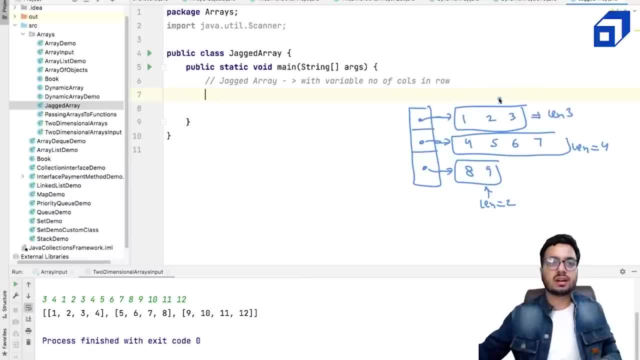 And this length is: let's see how we can create an array like this. Now it's again a 2d array which looks like this: 123456789.. In this case we don't have a fixed number of columns. we need to. number of columns are. 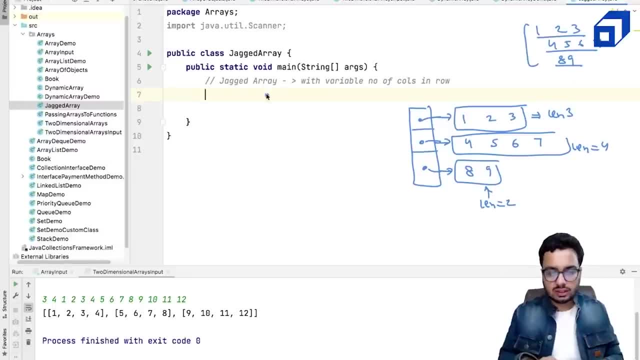 variable in each row. How do I do it? So let's see, I'll start by creating a scanner. equal to new scanners is important. Oh, I'm just going to read the number of rows from: the user Is a scanner. 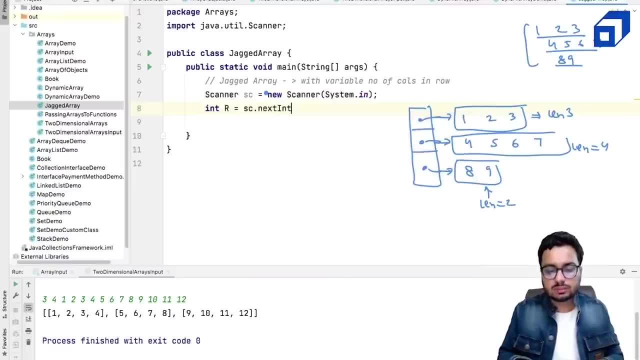 Next, Once I know the number of rows, I can initialize my array. I can say int, square bracket, square bracket, ARR. this is equal to new, and, and here I just define the number of rows is okay, I need our number of rows. how many columns are there? I will tell you later. 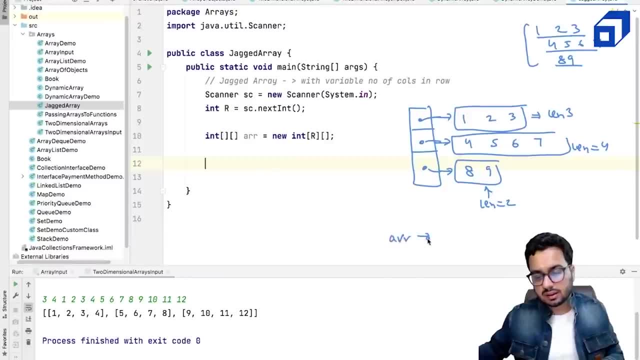 What does this code do? it creates an ARR that points to an array that is going that will hold. that will hold these array objects, but they will be created later. it's only going to create an array with our number of buckets inside these. these will be created. 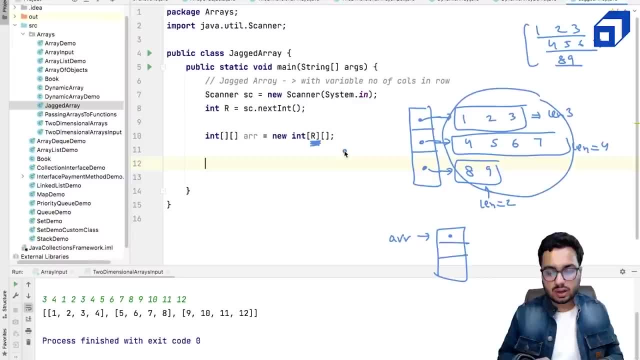 later. this part we will do next. right now, what I need to do, I need to iterate over each bucket: I equal to zero, I less than R, I plus. Now I'm going to ask: okay, tell me how many columns you're going to have in this row. 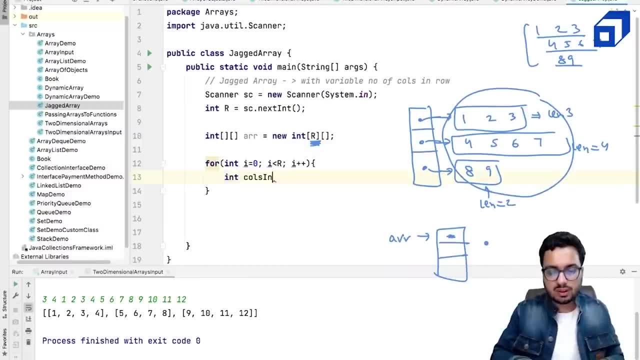 I'll ask the user I can accept a columns in the current row, how many columns. I'll ask the user to tell me number of columns in the current row. can also output here s out columns in the current row. tell me how many columns will have in the current row. 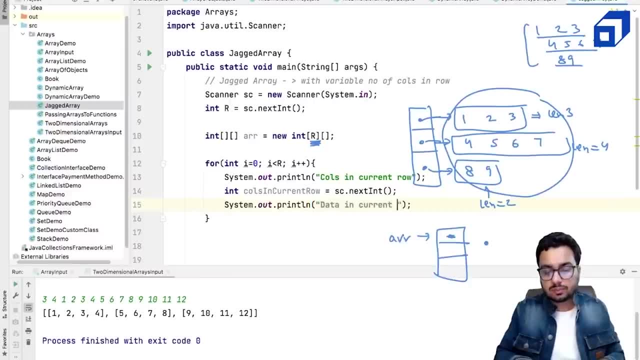 And then you can say: s out data in the current row. Maybe if I said I have two or three columns, then I will run a loop three times to read those numbers. This is okay for int i equal or int j equal to zero, a less than columns in the current. 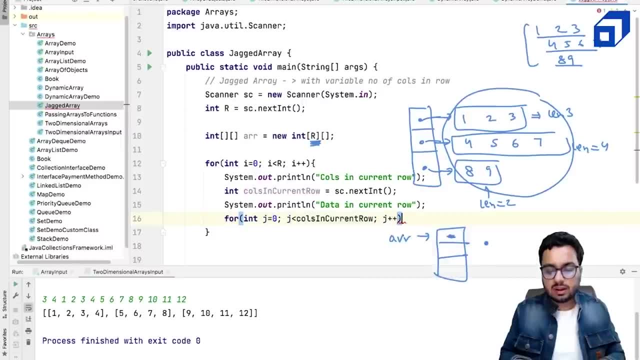 row A plus plus. now the thing is, where should I store this data? this array object is not yet created. First, I have to create an array object here in which I should be able to store data. How do I do it? 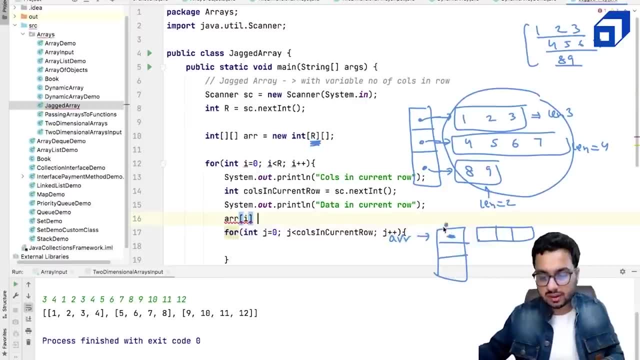 I said, fine, this array of, I array of, is this bucket. It should be a point to a new one day in which I can hold these many, of these many numbers that is equal to columns in the current. this line of code will actually create this array. 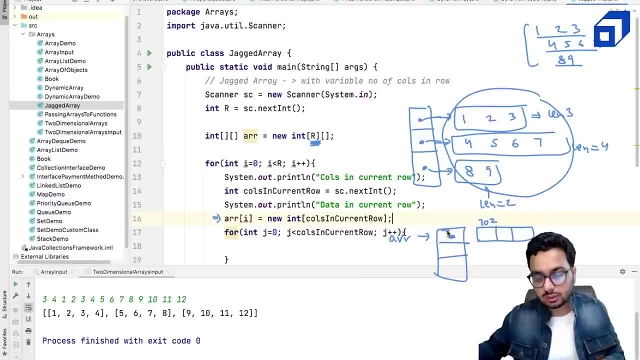 And suppose this address is now 702.. This is stored here. seven And this link is established. Now I can read data and I can store it. This thing we will repeat for every row. I'm iterating over These buckets now and I'm going to say, okay, read the next number and store it here. 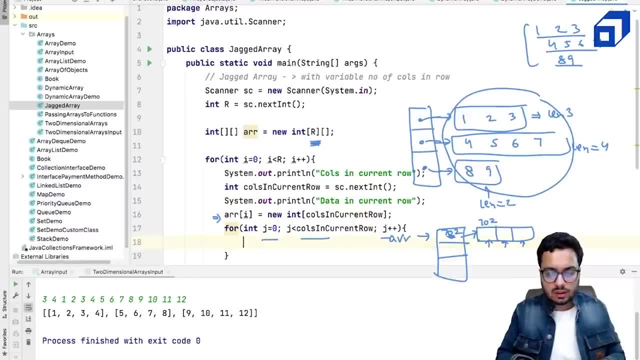 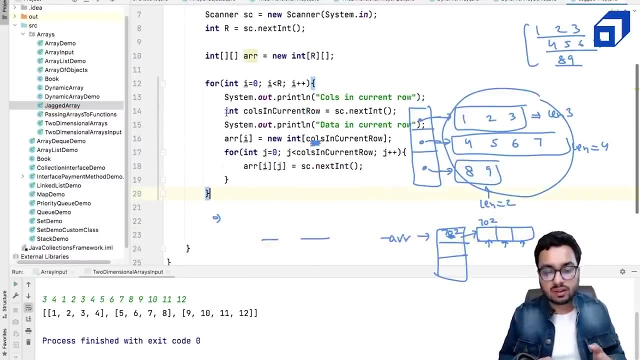 I can say array of i, j. this is equal to can a dot. That's it. And in the next iteration we move on to the next row And we do the same work And we ask how many columns you have in the next row. it says, okay, I have four columns. 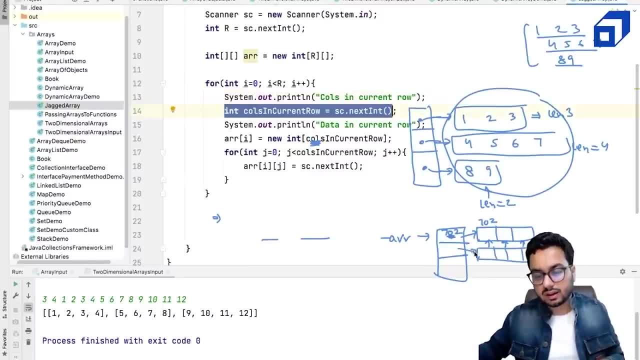 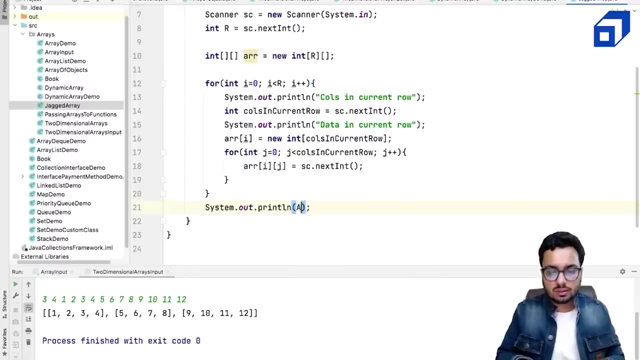 I create an array of size four And I link it here using this line, And then I again read it. I read these: let me show you by running this code that we can actually create a jagged array s out. there is dot deep to string. 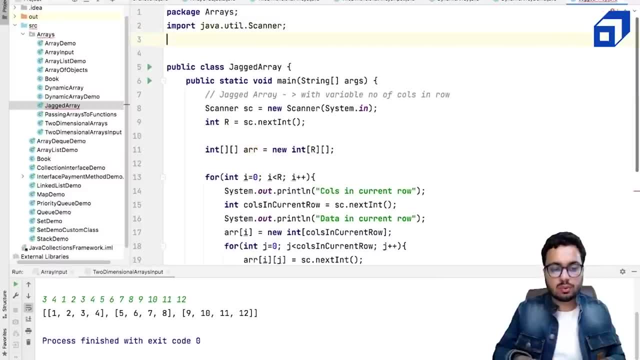 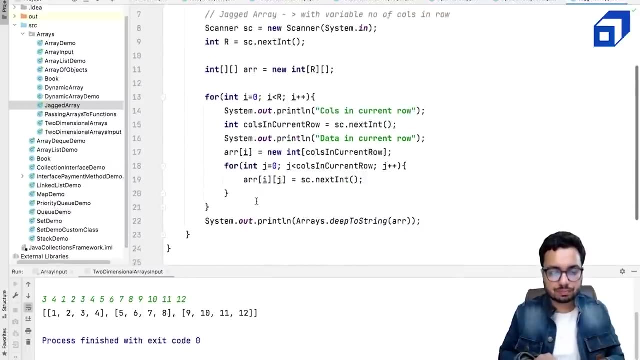 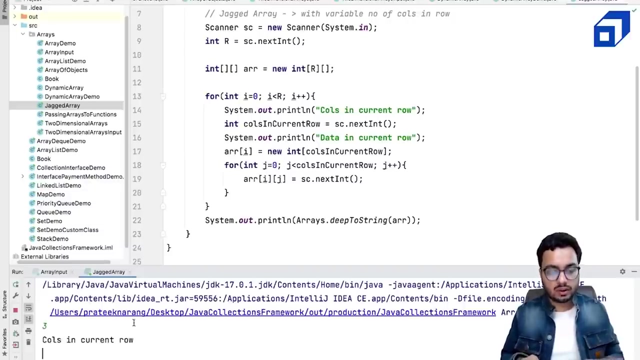 And I can give here And again I have to import java dot utp. So let's go and I want to create an array with three rows. I have to tell me how many columns in the current row is okay- four columns. 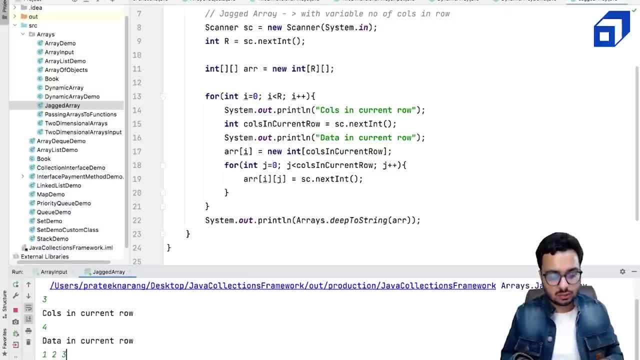 And then I have to tell me what are the four numbers, in that it's a one, two, four. then the next row: how many columns? maybe just three columns, and the numbers are 789.. Then in the next row, let's say two columns, the numbers are, let's say, 10 and 20.. 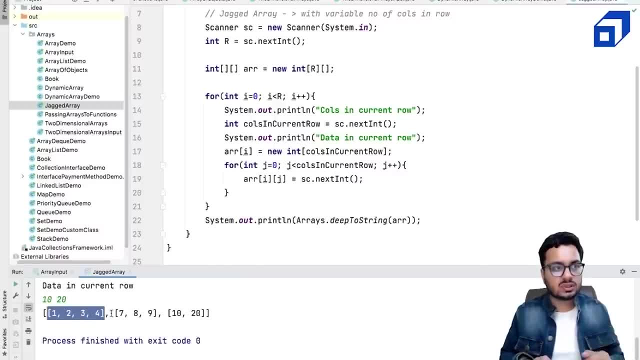 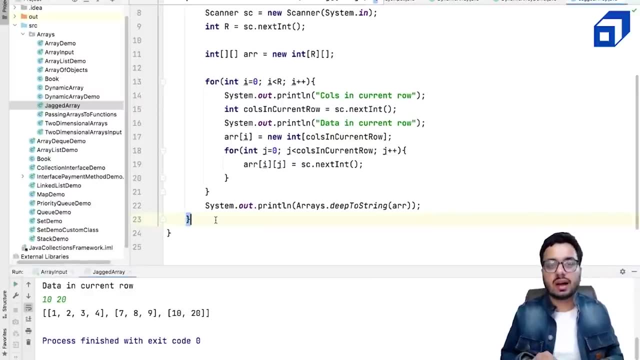 What do I see? I see a jagged array: four columns, three columns and two columns. This is how we can create an array in which every row has variable number of elements, And this is called as a jagged array. Now we are going to look at dynamic arrays. 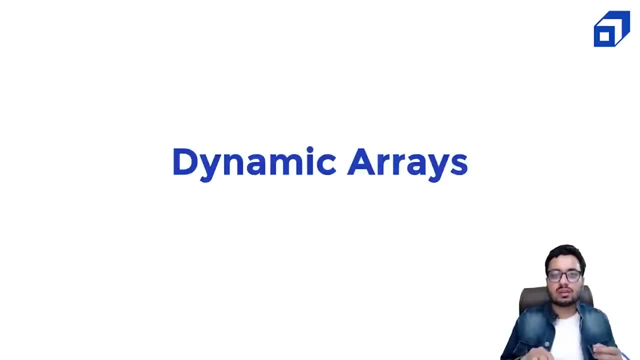 So far the arrays we have created, they had a fixed size. once you create an array of size n, you cannot add more than n elements into it. That is where dynamic arrays come into picture. For example, you're building a to do list where you can keep on adding tasks every day. 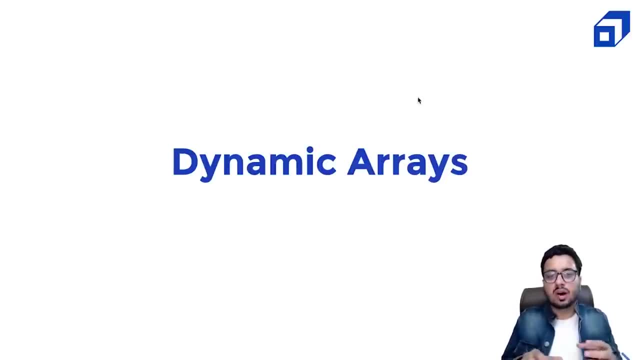 And you might be removing some old tasks as well, So you do not know how many elements you would be storing in your list, So you need something like a dynamic array in that case. in Java, dynamic array is provided by the library As a part of Java collections framework. the class is called as ArrayList. you will also. 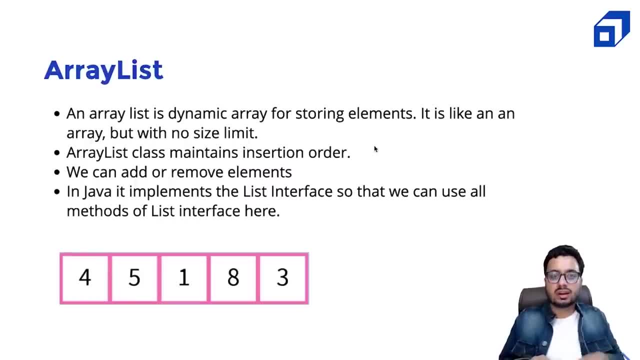 see how this class internally works, But before that we will look at a demo, A demo of using ArrayList. if an ArrayList is a dynamic array for storing elements, it's like an array, but with no size limit. It also maintains the insertion order that we keep on adding elements and they will. 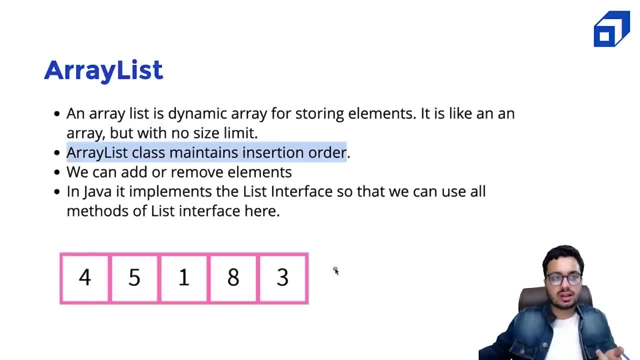 get added at the end of this array, right? So if I say, okay, I want to add six, I want to add seven, I want to add 12, they will keep on adding in this, at the end of the array, we can add elements. we can also remove elements. 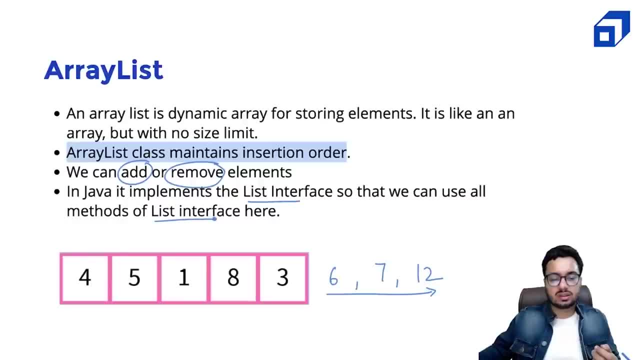 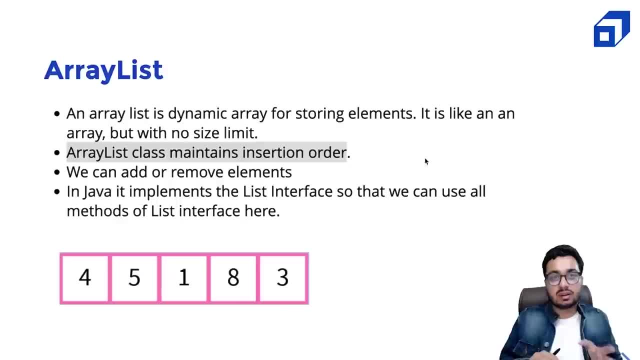 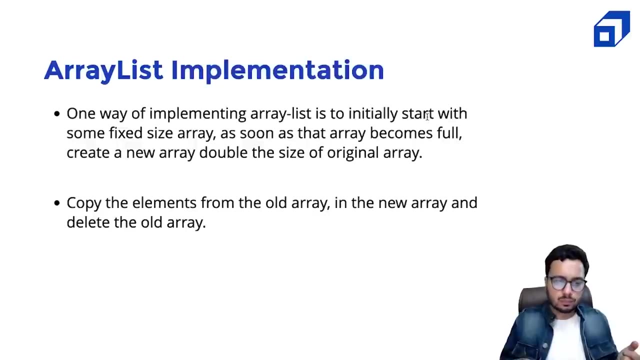 And list interface here. So list interface is part of collections framework And I've done a detailed video on collections framework link you can find in the description of. you can watch that video if you want to learn about what about the collections framework and various data structures present inside the Java collections framework. 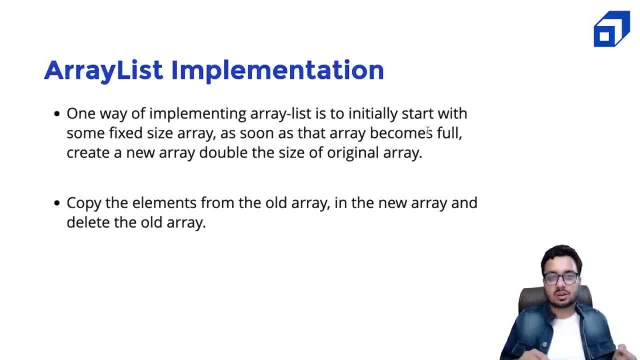 Now how this ArrayList is implemented. let us talk about how this array is actually dynamic. how does it grow and shrink? One way of implementing the ArrayList is Start with some fixed size array. So I guess in Java, this fixed size array is having a default size of 10.. 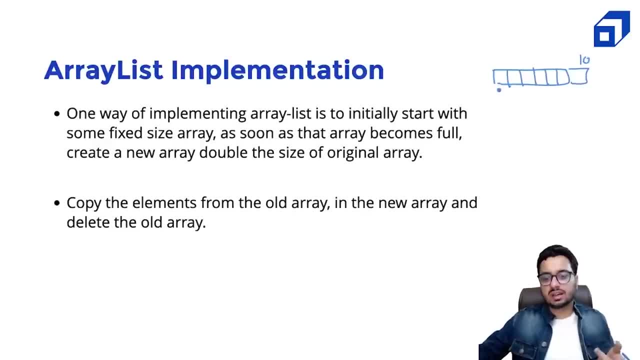 So whenever you say, okay, I want to create an ArrayList, it will give you space for 10 elements, But as soon as this gets full right, you say, okay, I've used all the elements, right. What it will do? it will double itself. 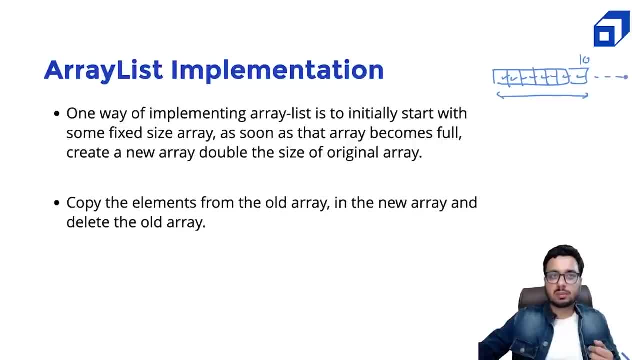 Now, you cannot double in the same memory, because this memory might be occupied by some other data sector or some other part of the program. What it does, It looks for New memory in the heap, where it creates an array of the double size, and it's going to. 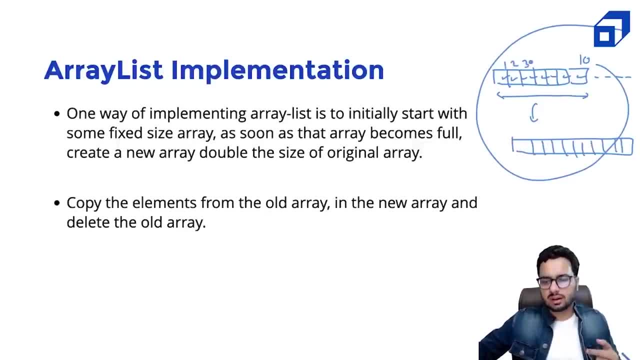 copy the old data into the new array. Let's say this data was 1,, 2,, 3,, 4, up to 10, it's going to copy all this data in the new array And then the remaining elements. the remaining 10 boxes are available for putting some new. 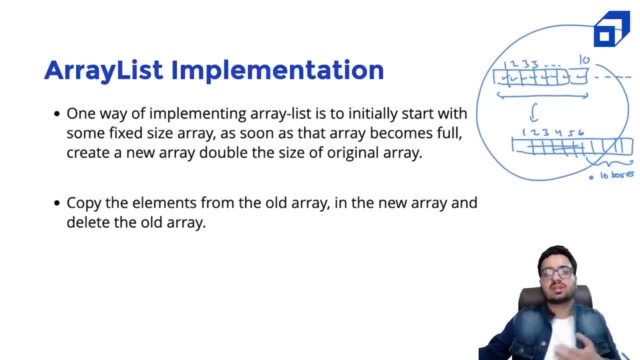 data right. Once this gets full again, you have to do the same thing again: double the old array by creating a new array, copy the data from the old array And you have to delete the old array. So in Java the deletion is done by the garbage collector. 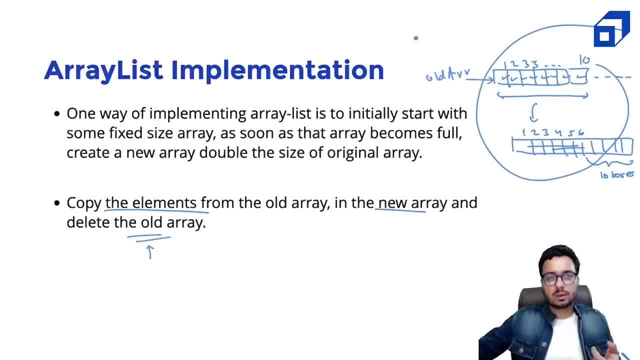 For example, if this is my old array and I say old ARR equal to null, what does it mean? No one is referring to this array. This object becomes eligible for garbage collection. Okay, So in other languages like C++, you have to use the delete keyword. 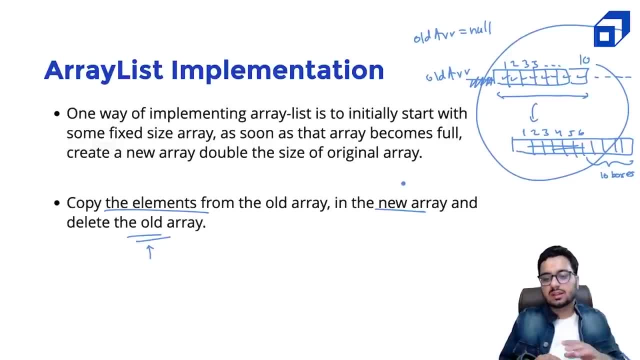 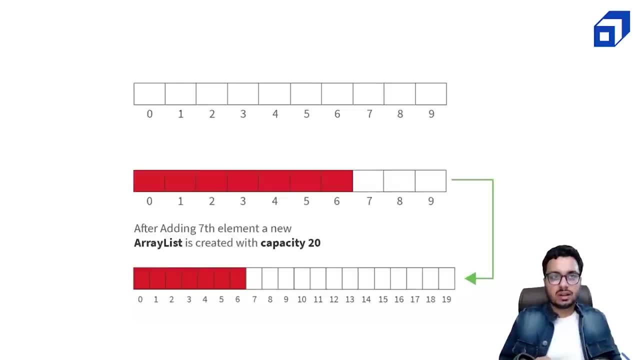 But in Java, the garbage collector takes care of objects that no one is referring to. So first, let us first look at the demo, right? So to be precise, in Java, Java maintains something called as a load vector. Load vector is what percentage of your array is currently filled, right? 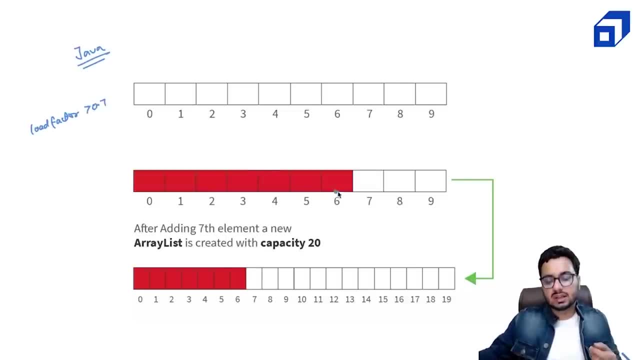 So if I say, okay, if my load vector goes more than point seven, that means if I have space for 10 elements and I put eight elements in this array right, that means it is the time to double the array, right. 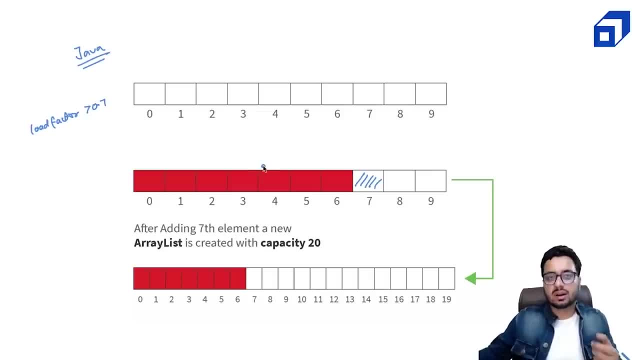 So right now I was doing it full capacity, But you can also do it early. If you're, 70% of the array is full, right. so that is your current size upon your capacity. If this percentage exceeds point seven, the Java triggers this function that doubles this. 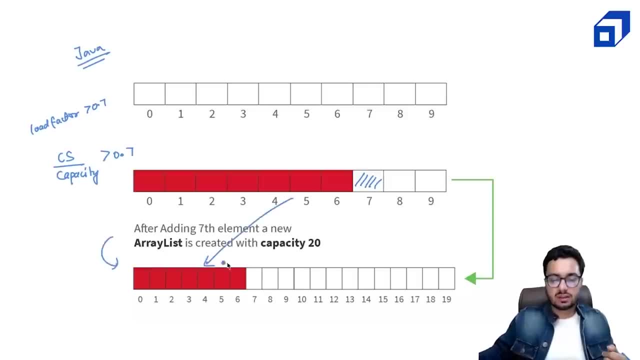 array, So it creates a new array, copies the data here and you have more space available for storing new elements. okay, ideally, if you know that. okay, I'm building the application in which I will require space For around 1000 elements. it is better to initialize your array list with the initial 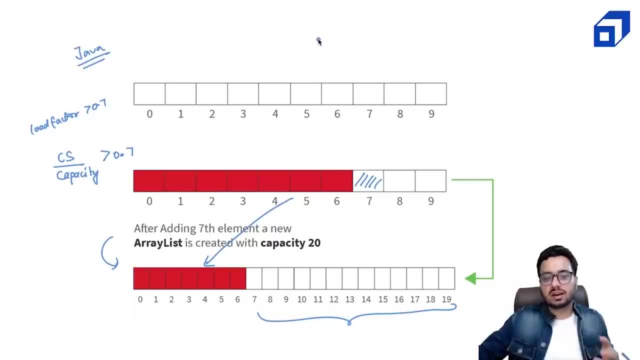 capacity of 1000 so that your doubling does not happen again and again. And if you look, I need maybe 1100 elements to take a safer limit. okay, and you took, Okay, I created an array with 1000 elements. that is fine. it will double one time. 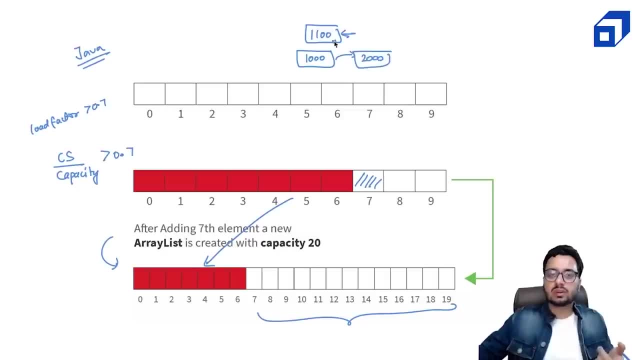 So from 1000, it will become 2000,. right, In 2000, you can easily store 1100 elements. So basically, you should have a rough idea of the range, how many elements you would be needed, And accordingly you can initialize the array list so that your repeated doubling operation. 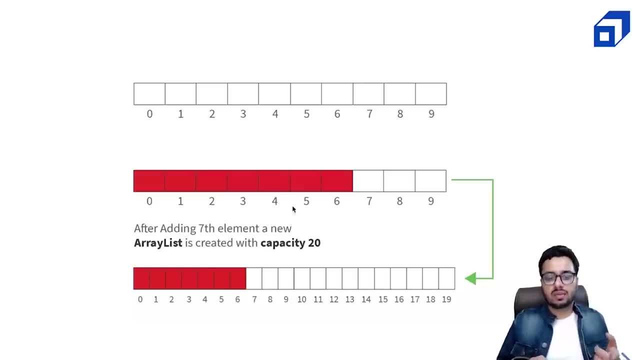 can be minimized. And doubling is an expensive operation by because it copies all your data into the new array, which is going to take linear time. right? That is how the internals of the array list work, right? So let us also talk about features. 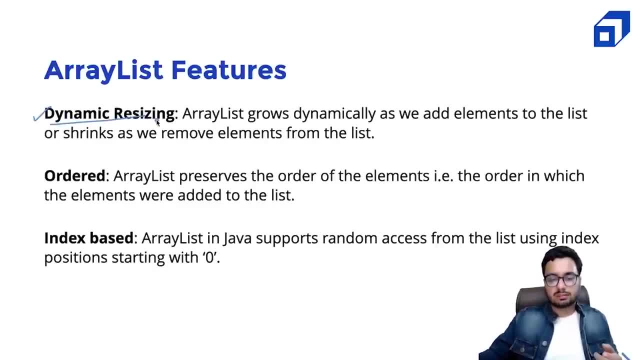 ArrayList is a dynamic data structure. Okay, And it can grow dynamically. it can also shrink as we remove elements from the list. So, again, there is certain criteria. okay, when 20% of the list is occupied, I might shrink it to the half, something like this. we can have a conditional condition on shrinking. 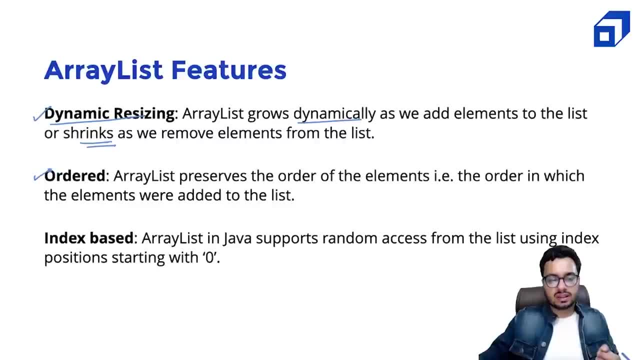 as well, just like we have a condition on growing. Second thing is it is ordered. it preserves order in which the elements were added to the list. it is index base, does it's? it's an error internally, right? so it also has. 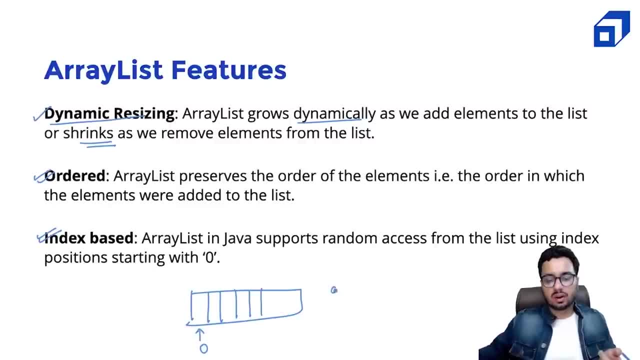 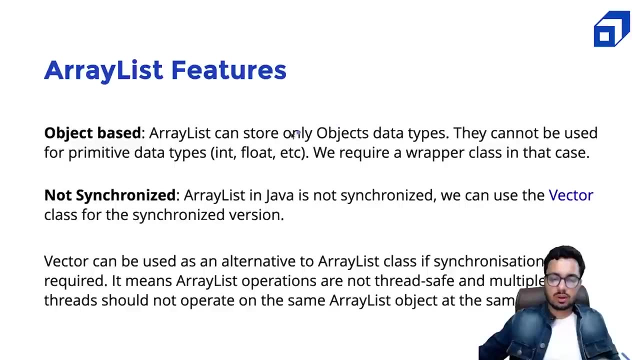 indexing. So when we add an element, we will say okay, array dot get zero. it provides us with a get method And I need to allocate. this is the index I need to access. right And okay. and ArrayList can also store. 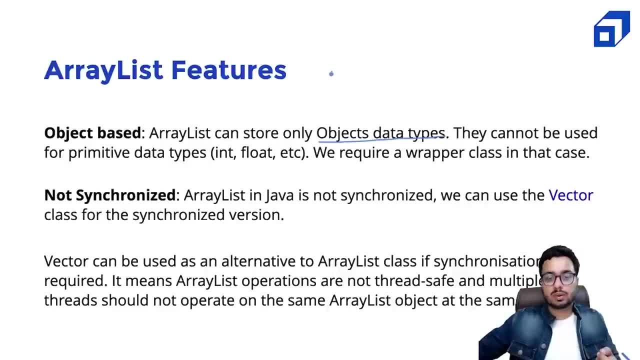 It can only store object data types. that means it cannot store primitive data types like int. if you want to create an ArrayList of ints, you will have to use the corresponding wrapper classes. Okay, So for that you need to have some idea about wrapper classes. I can create an ArrayList. 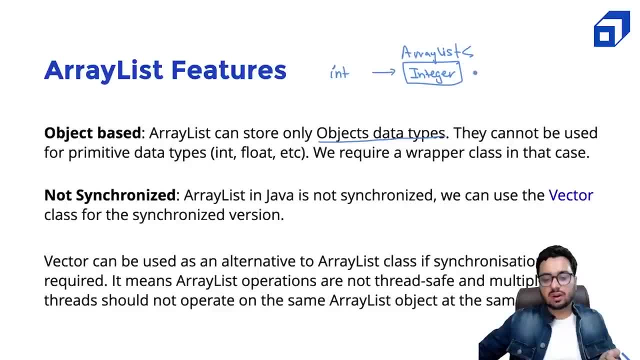 of integer. where integer is a wrapper class for int data type, it cannot be used for primitive data types require a wrapper class in that, And another thing is it is not synchronized, So you need a concurrent data structure. then there is a something called as vector, which 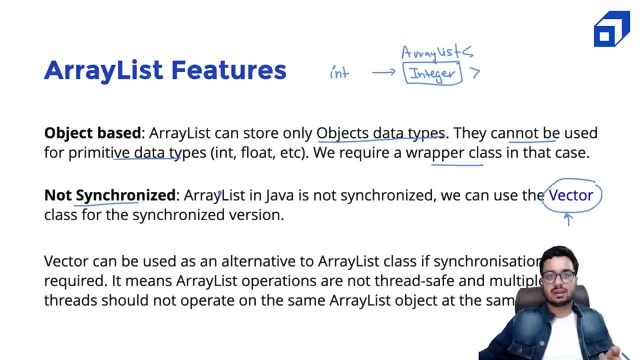 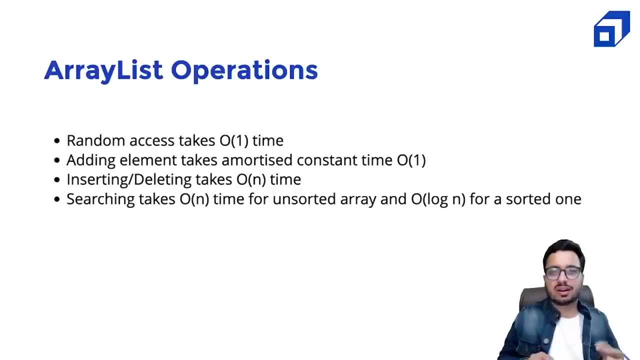 is a synchronized implementation of ArrayList. Okay, This concept is pretty advanced. If you're working with multiple threads and stuff, then you might be using vector. So let us look at a demo of using ArrayList Before we jump into the code. let us talk a little bit about the kind of operations. 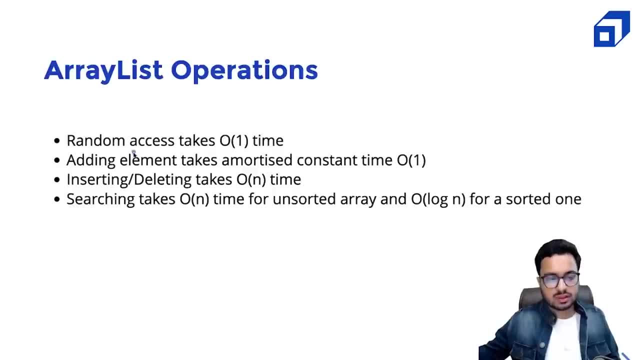 we can do on an ArrayList. So one common operation that we do is we want to access an element, so it is called as random access. that is done using the get function. I can get any random element in order of one time, which is pretty obvious because internally it is accessing the array. 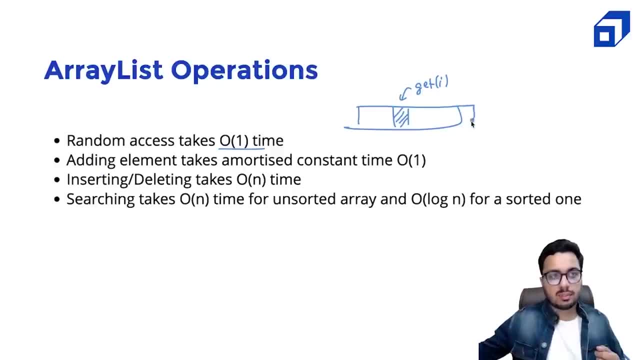 Okay, then I can add elements. I can add elements at the end of the ArrayList, which will take order of one time, But you can also add elements in the middle of ArrayList, which will require shifting of elements. Okay, inserting elements in the middle. it's going to take order of n time. 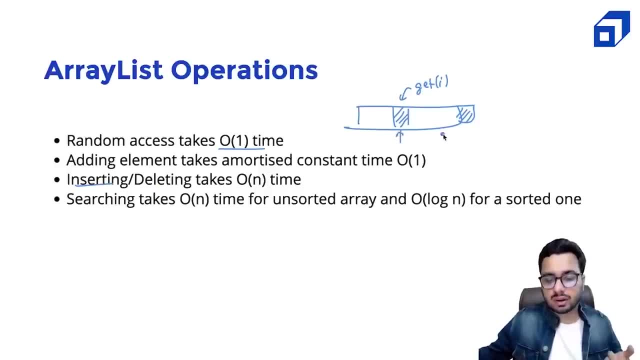 Similarly, deleting something from the middle is also going to take order of n time because the remaining elements will have to get shipped. searching in general. it takes order of n time because it's going to use a linear search Right. But if you have a sorted ArrayList you can use your own binary search method or you. 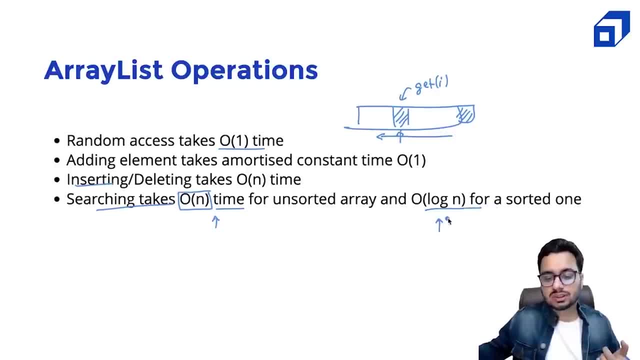 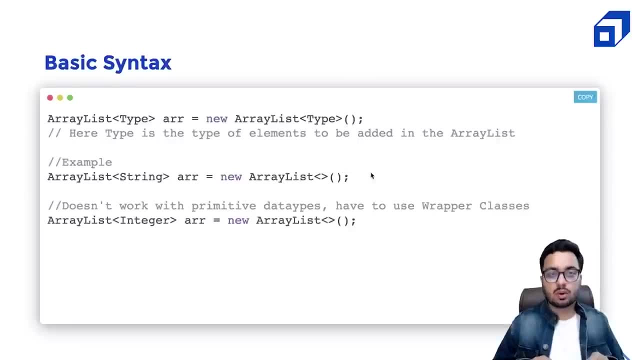 can use collections dot binary search method to search in order of login, in order of login time, if your ArrayList is sorted. Okay. So how do we create an ArrayList? It's a predefined class in Java collections. I can say: okay, ArrayList of a following type: 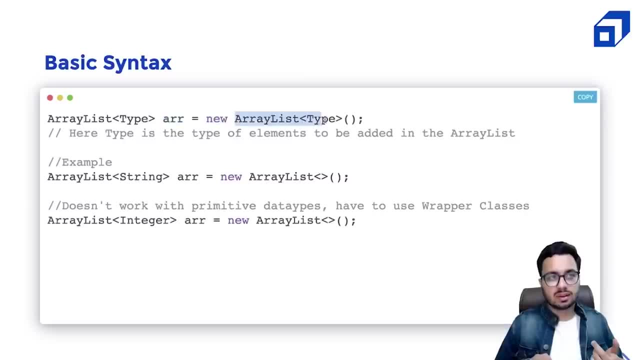 followed by name of the variable, followed by new ArrayList, and this will create an ArrayList in Java. Okay, So what is the default size? Default size in Java? it is 10.. Right. For example, an ArrayList of strings can be created like this: 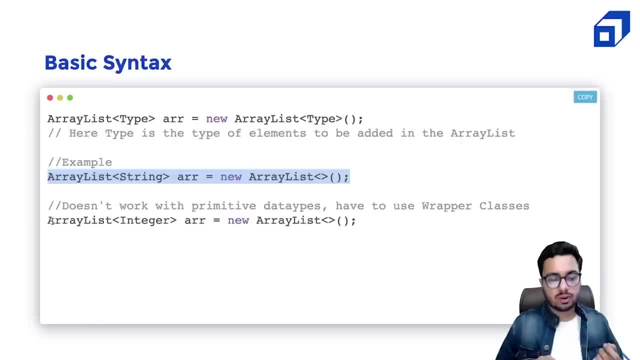 And it does not work with primitive data types. Okay, so I told you that we have to use wrapper classes. we will have to say ArrayList of integer. if you say ArrayList of int, it will not work. So you will have to say ArrayList of integer, right? 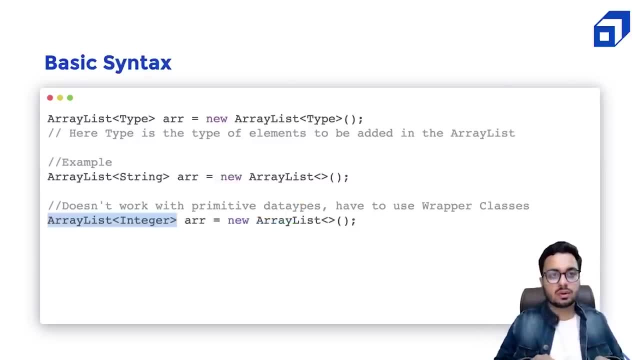 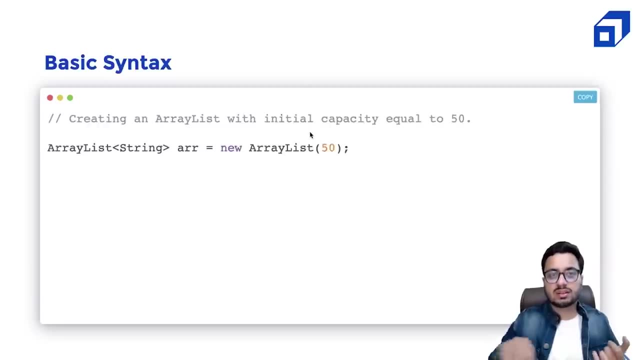 This is equal to new ArrayList. That is how you will create an ArrayList object in Java. Next thing is you can also give some default size. So basically, the ArrayList class has three constructors In one constructor. you don't give anything, So it uses a default size of 10.. 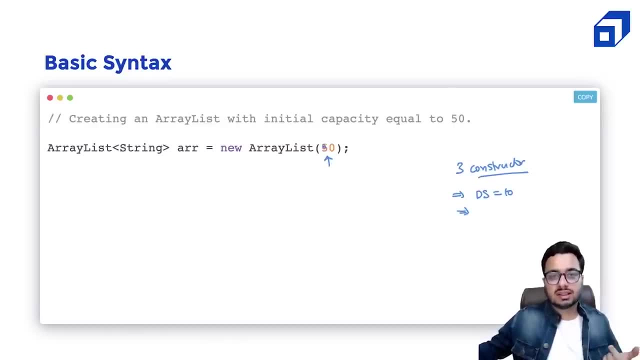 In another constructor it accepts. you give me the default size and I will create an ArrayList of that capacity. So I'm saying 50. That means it is able to hold 50 objects in this ArrayList, And once you reach 50 capacity it will double itself. 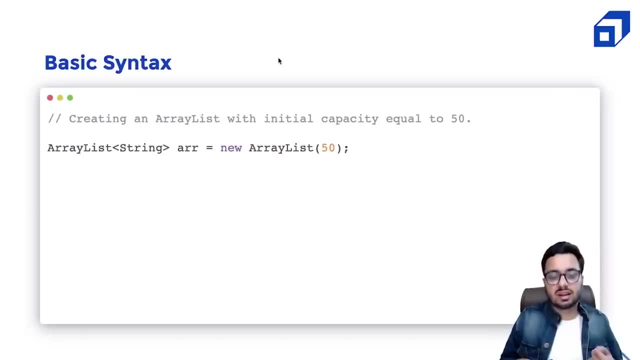 And there is a third constructor as well, in which you can initialize an ArrayList from some other list or from from some other collection as well. That can also be done. For example, in this case we have a list of strings And we are initializing the ArrayList using this list. 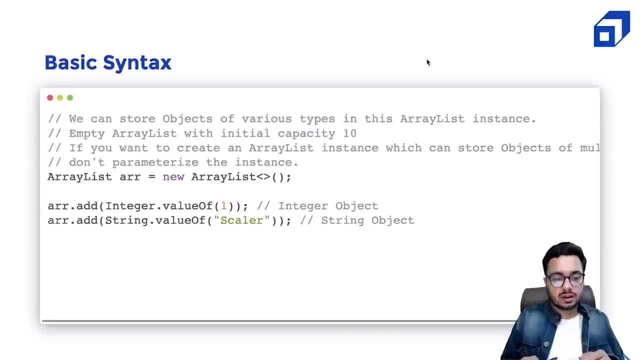 That is the third constructor call. that is being done right. So one more point to note about ArrayList is it allows us to store heterogeneous elements as well. For example, I can- I can- add an integer into it. I can also add a string object into it. 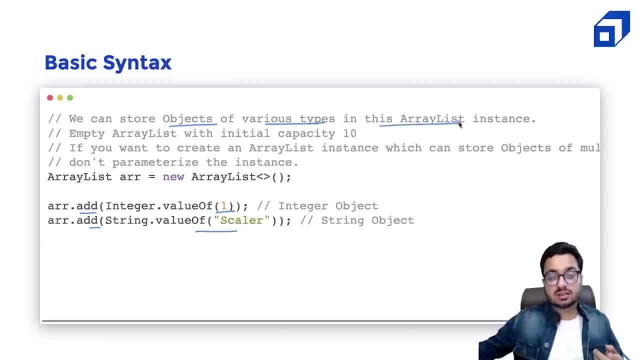 We can store objects with various types in an ArrayList instance. also, in this case, when you're creating this ArrayList object, you don't need to parameterize the instance. you didn't don't need to define what kind of data it is going to hold. it will hold all types. 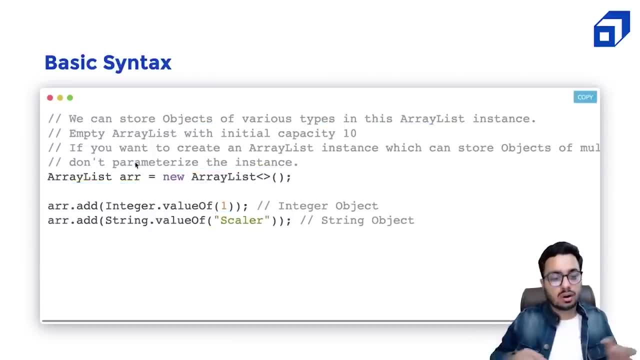 of objects in it, right, So you can put a string, you can put a book, you can put a dog- anything will work in the same ArrayList. So that is about it. Now let's talk about how do we create an ArrayList. 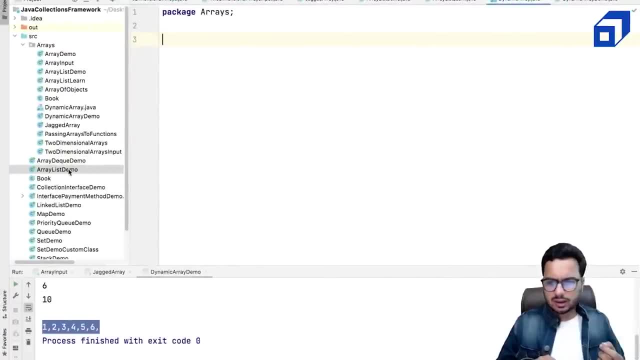 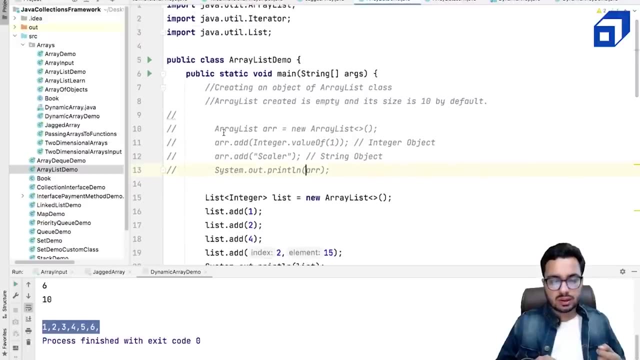 Now I will show you a quick demo as well. So I did this demo. in Java collections video that I have already done, I have shown you that you can create an ArrayList. So the first four lines I show you. we are creating an ArrayList in which we have not 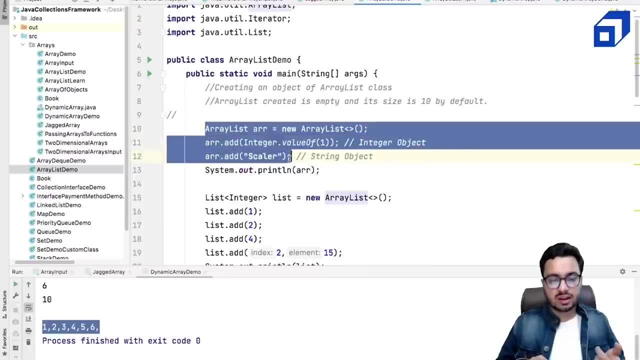 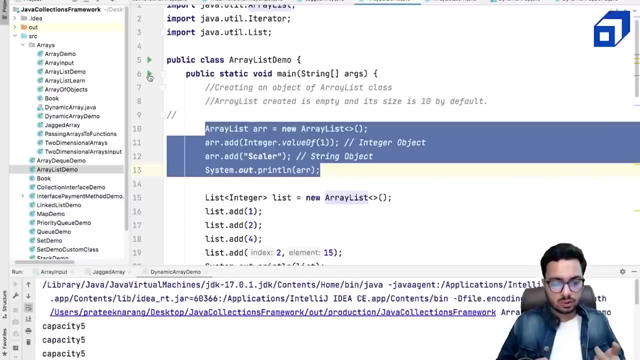 defined the data type, then we are pushing an integer, then we are adding a string and then we are going to print it. Let me just run this code And let me show you- Okay, Let me show you- the output. I need to run this. 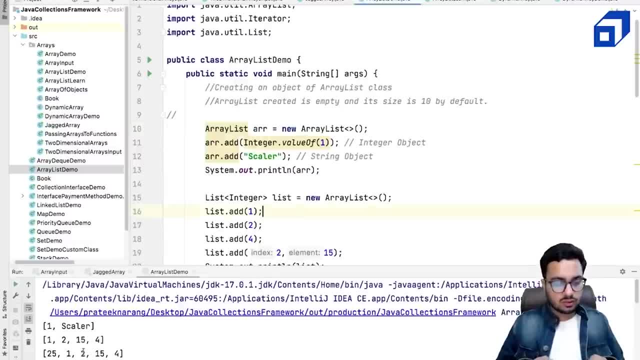 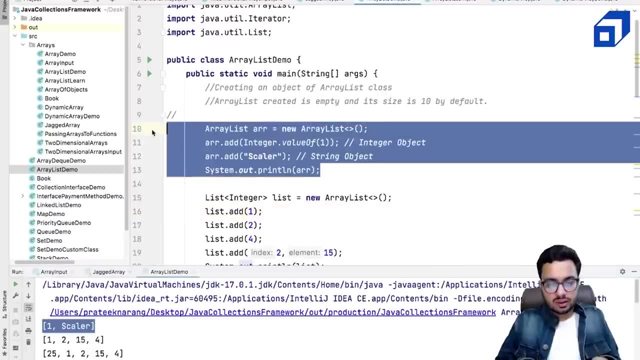 Yeah, So if you see, here I'm getting an ArrayList in which one item is an integer object, the other item is a string object. So we can definitely do this. I'll comment it out, then I can say: okay, create an ArrayList. 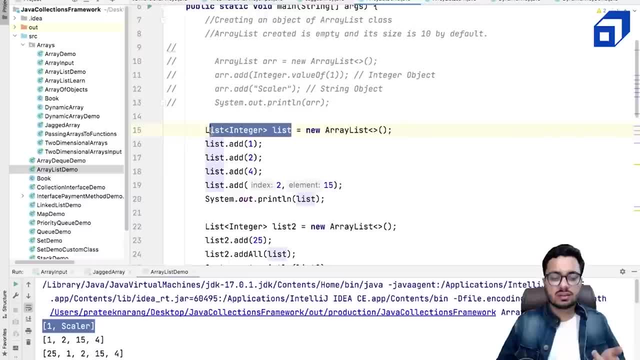 Because ArrayList implements an interface. So I can say this: Left and right data dip can be created. So I can say, okay, create an ArrayList. It can be more generic, it can be. it can have list as the data type. that is perfectly. 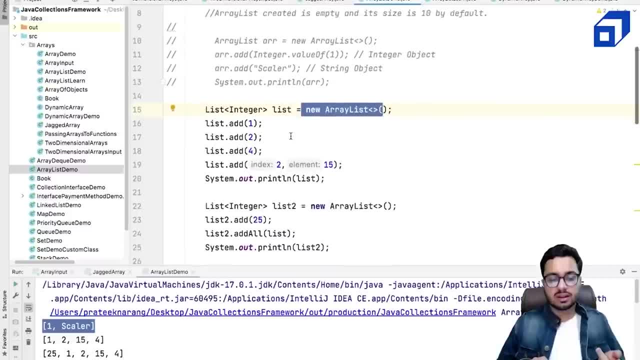 fine, because an ArrayList is an implementation of a list. So I can call the add method to add something at the end. I'm saying: add one, add two, add four. then I can also use this add method by specifying the index, So the add method is overloaded. there are two add methods: one which adds at the end. 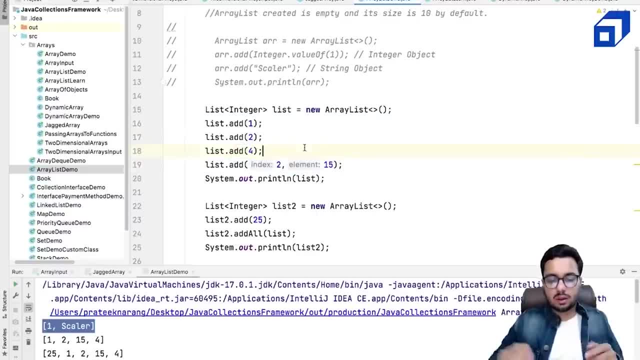 and one which adds at a particular index. I'm saying, okay, add the second index, You should add 15.. So it becomes like this: 124,. then add the second index, which is 012.. I want to add 15 here. it will become 1,, 2,, 15 and 4.. 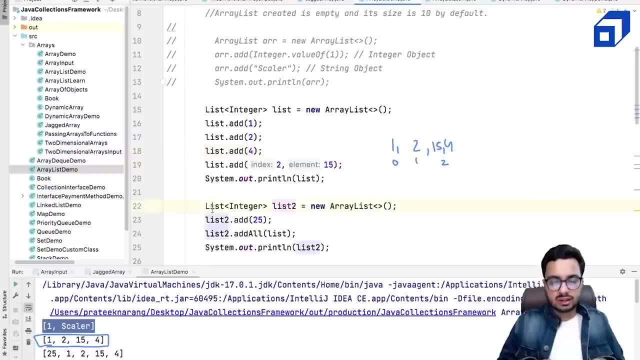 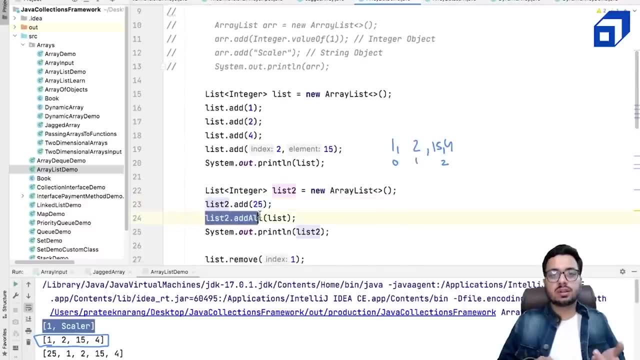 This is the output that we get. Then I've created another list in which I have added 25.. And then I'm using a method called as add all. add all is used if you want to add all items present in one list into another list. 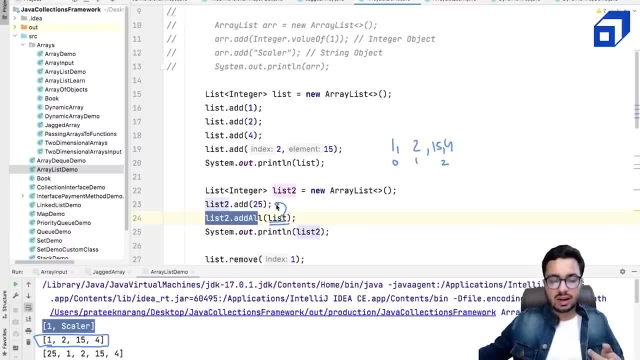 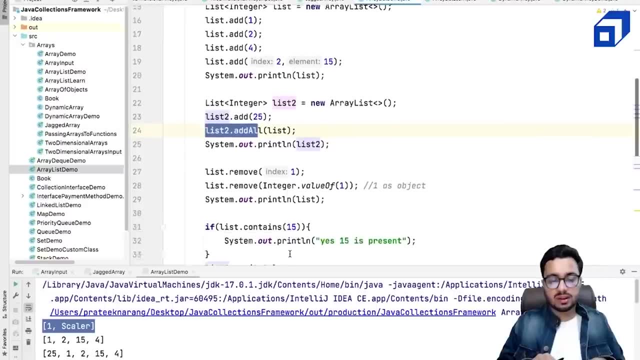 Add all will iterate over all items In list one and it will add them into list two. you will see 25, followed by all items that are present in list one are now present in list two. Just like add, we have a remove method. 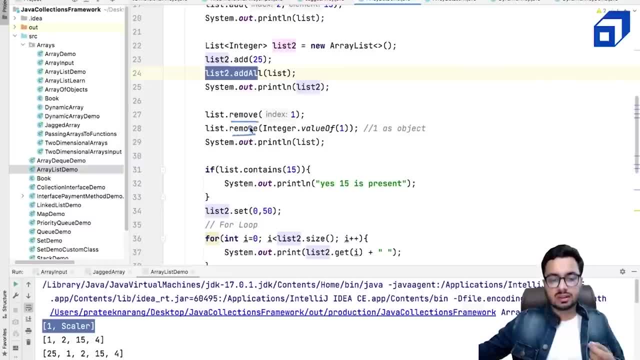 Remove method is also. there are two remove methods. the one remove method, which accepts an integer. So if I show you something like this, this dot remove, you can see. one remove method accepts the index And second, remove method accepts the object. If you have. 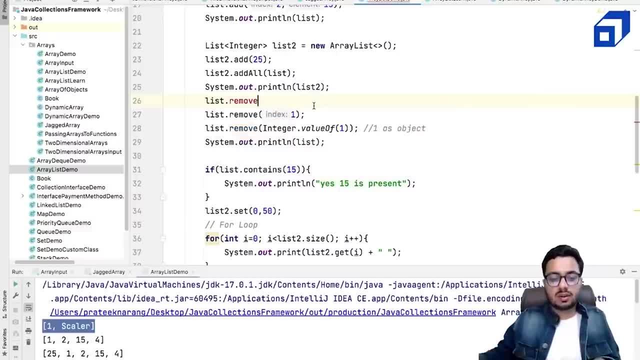 So if you have to give the object of the type integer, you have to typecast into the integer data type So I can say, okay, integer, dot value of one. it will mean that I'm I want to remove one from this list. But if I simply pass one, it would mean that I want to remove the element at index one. 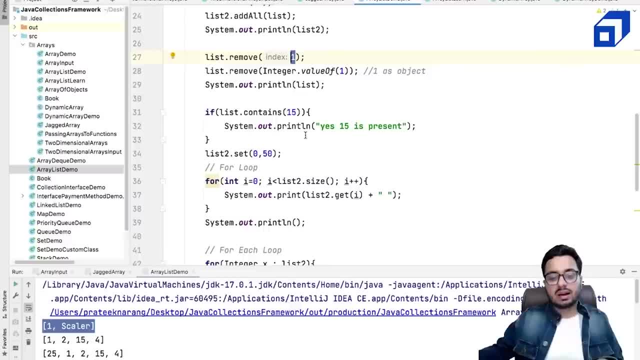 right, That is how the remove method works, right. And if you want to search something, then there is a contains method will tell you, okay, whether the following integer or following object is present inside the list, This list or not. That is your searching method. 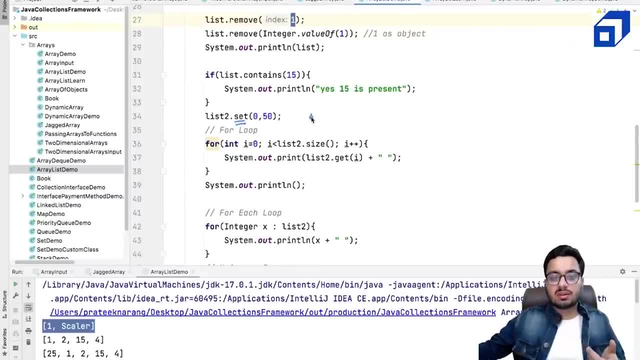 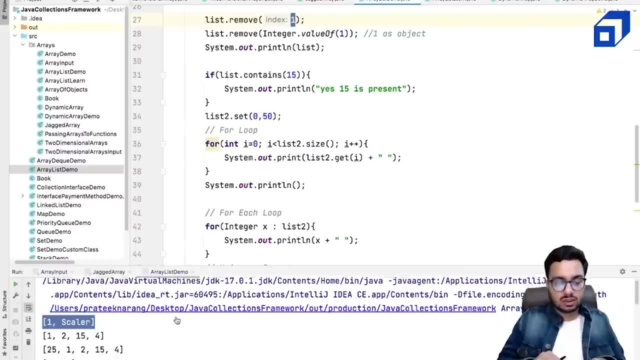 There is one more method that is called as set. That means I want to update something. So if I want to say, okay, I want to update the zeroth index, And this is the object that I want to store at the zeroth index. 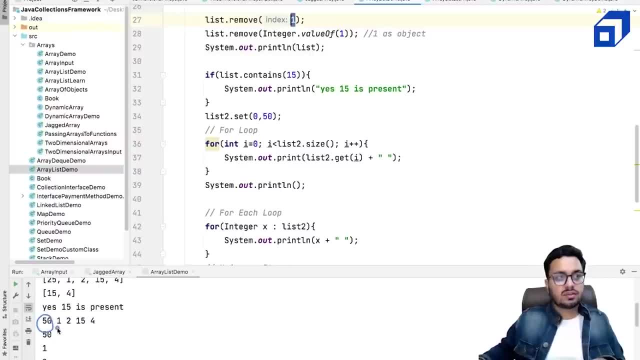 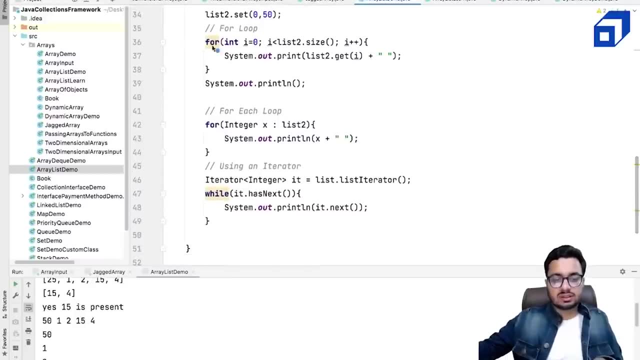 If I do this, you will see at the zeroth index, instead of 25, now the new element that I have stored, it's going to be 50. And apart from it we can iterate over the list. So list dot size gives me how many elements are there. 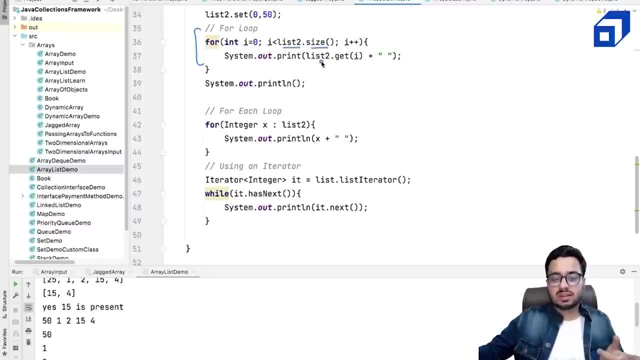 It's not the capacity, but how many elements are currently present. that will give me and I can use the get function to get the ith element from this list. That is one way of iterating over an array list. can also use a for each loop, if you want. 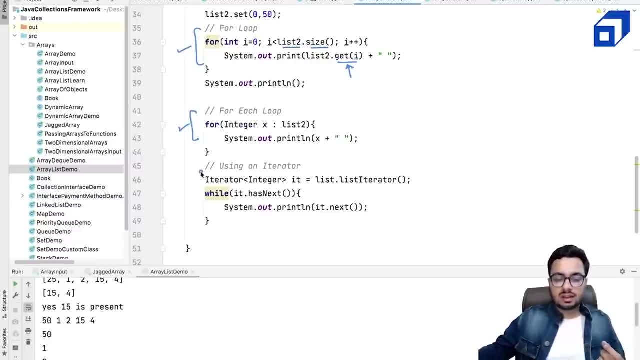 to iterate over the entire list. And third ways, you can also create an iterator object And while iterator dot has next, so has next tells me whether the next element is present in the list or not, While it has elements, Keep on iterating and you access the next element using the next method. 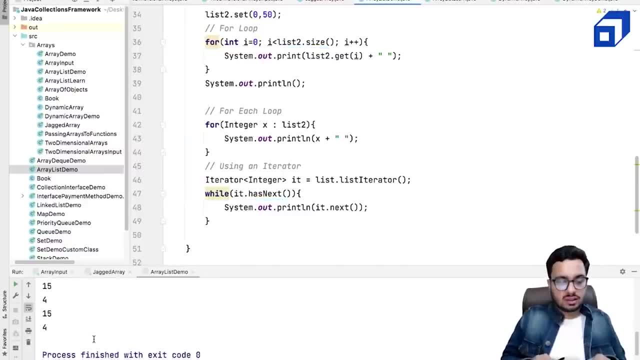 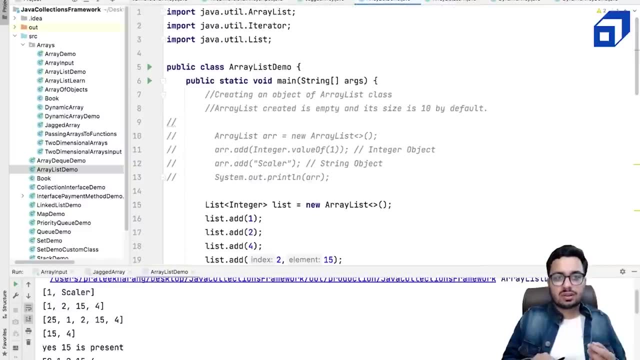 So that is another way of iterating over the error list. So you can use this methods and you can work with error list while solving a lot of problems. Okay, So that is about error list And, if needed, you can also refer the Java oracle docs to go in more details of these. 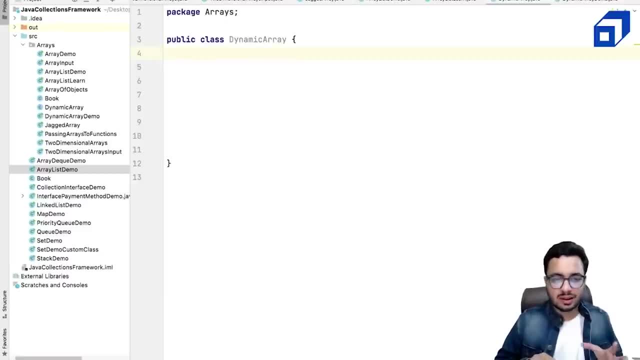 methods. Let us come to the final part of this tutorial. So you so far you have worked with arrays, You have worked with error list, And now I want to show you, if you want to build your own dynamic array class, just for your better understanding of error list, was you're asked to implement an error list at? 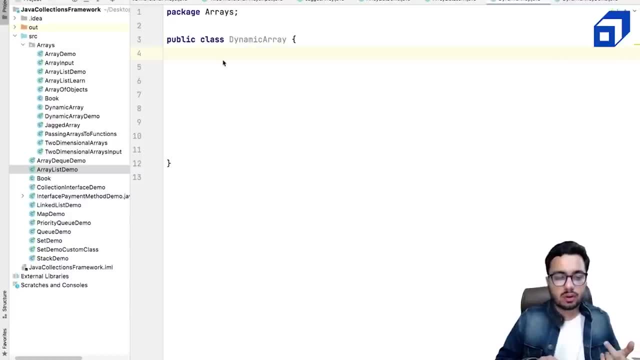 your own how you would do it. What we want to do? we want to implement a class called as dynamic array. What thing we learned? First thing is it internally uses an array. That means one data member of this class would be an array and this array would have some. 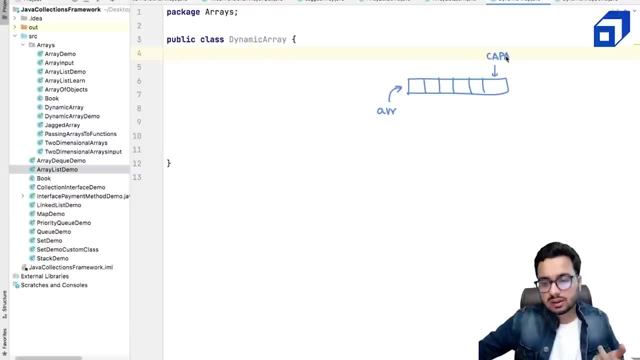 size also. So it's okay. It has some default capacity. right This capacity and be provided by the user, or we can have some default value as well. We will look at that And then, if you start putting elements, start adding in elements in this area, you also. 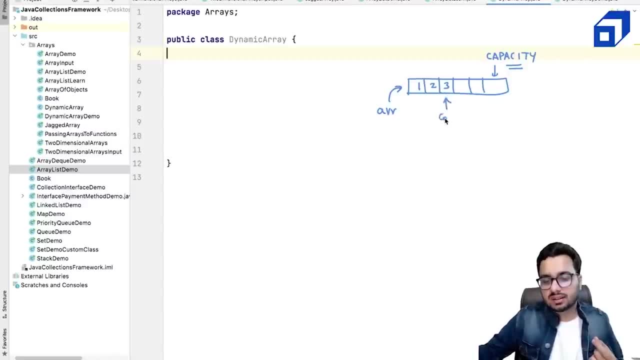 need to maintain how much errors fold. maybe current size. maybe the current size is 3012.. If the next element comes, can I insert it at the current size index? Can I insert it at the current size index? Yes, I will insert it at the third index. 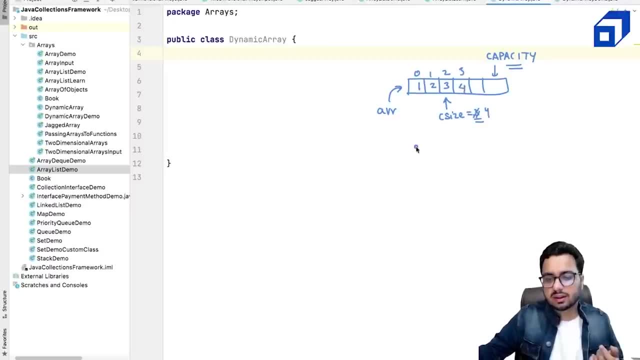 It's an element, is four, and I will increment the current size right. So it is clear that I need one data member that is array, one data member that is current size, one data member that is capacity and maybe one constant where in which is going. 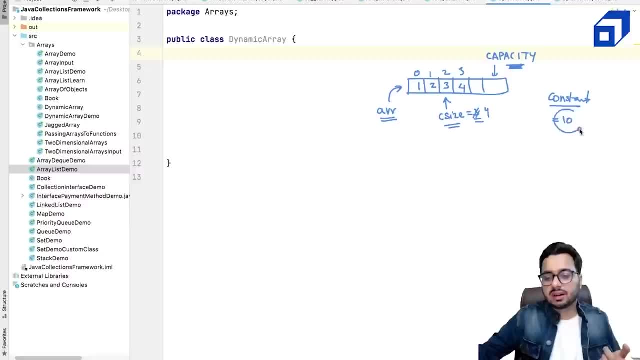 to store how much would be my default capacity, that I can call it as default, So by default, the capacity of this. So let us create these data members. I've created an array, right, I've created a capacity, I've created current size and I've created a default for which the value is 10.. 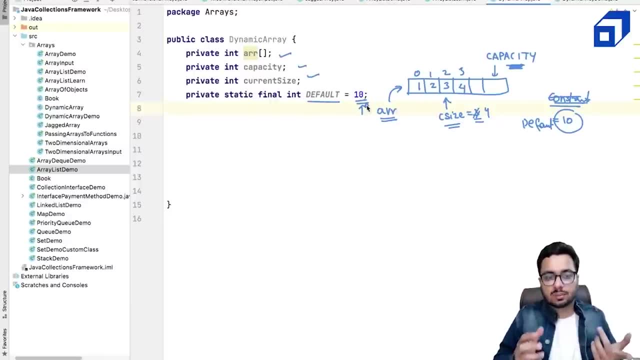 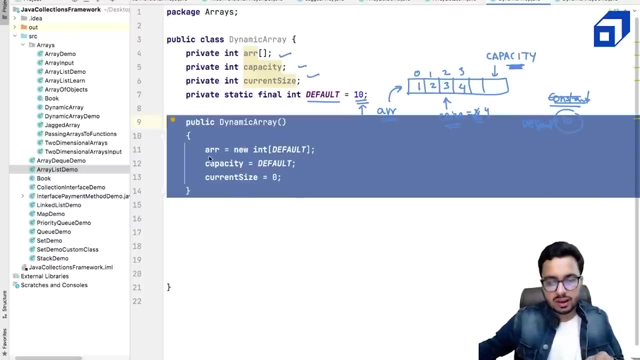 Now user says: okay, I want to create a new dynamic array object. how you're going to initialize these variables? okay, Suppose I do not give you any default capacity, I will need a constructor. right and in the constructor What I will do: I will initialize my array equal to the default size. default of size. 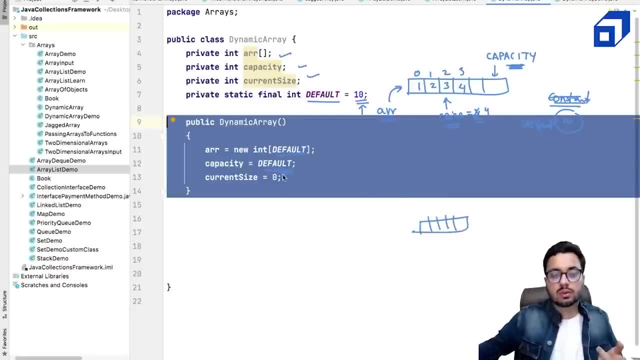 10.. I was okay. the capacity variable is also equal to default right. Why I need this capacity? because capacity can keep on changing. If n size 10 gets full, I will make it print. if 20 gets full, I will make it 40.. 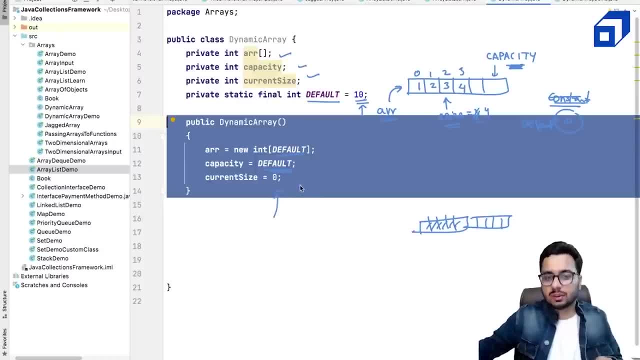 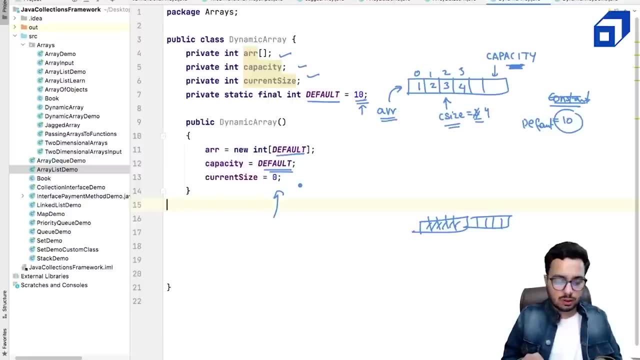 The capacity will keep on doubling and current size that is going to be zero, right, Because I have not added anything. But suppose if the user says, okay, no, I'm going to give you a default size of the nary, then how do I do it? 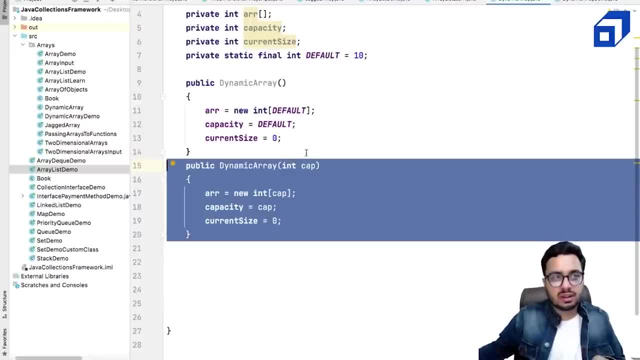 In the constructor. I will accept. Okay, you tell me the capacity. I will initialize my capacity equal to that capacity and I will create an array of that capacity. right, And current size is still zero. Okay, so that is how the constructor is getting created. 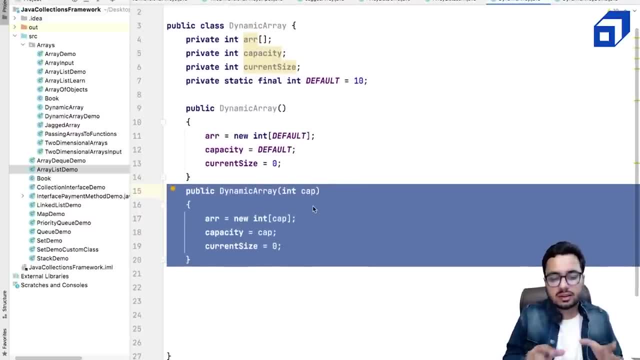 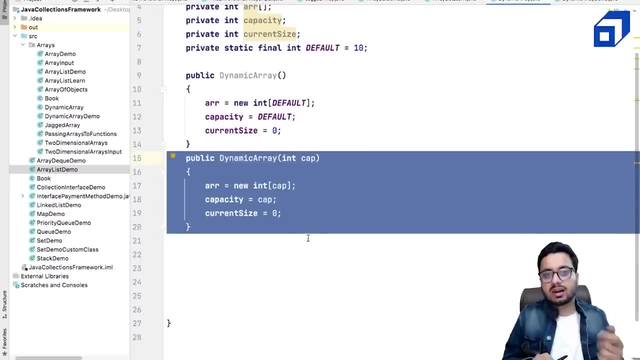 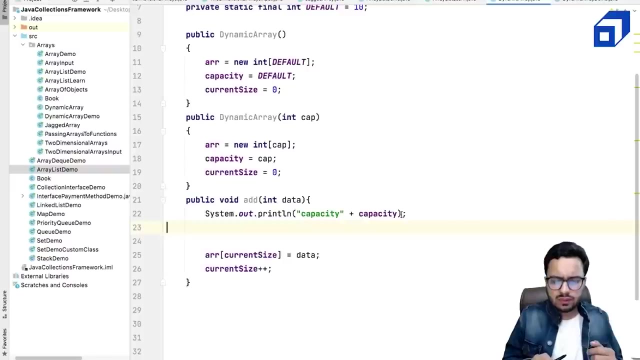 The third constructor, in which I get another list and then I create this. I'm not creating that. I'm writing a simplified version of an array list right now. suppose I want to add something into my array list. how should I do it? very simple, I will define a method called as art. 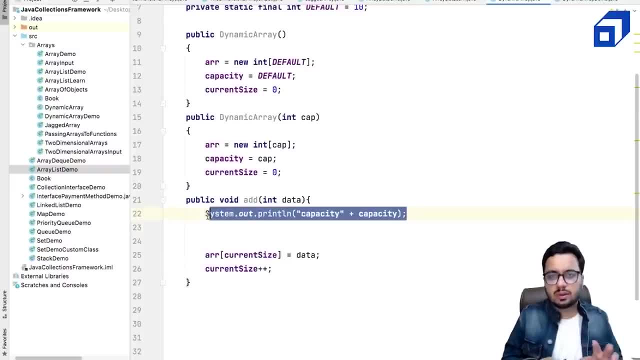 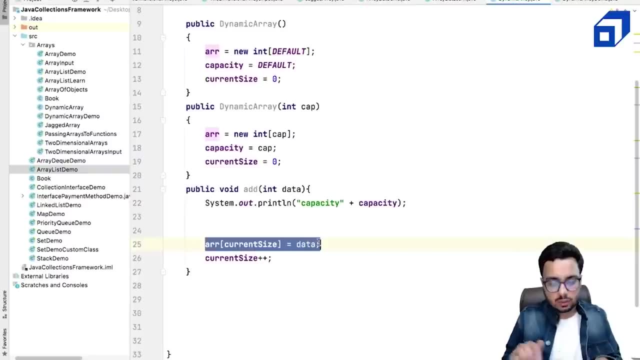 And I will. I'm just printing the capacity as of now, but I will remove this statement so that we can see, while running the code I can, the area of current size. this is equal to data Basically. in the beginning my current size, it is zero. 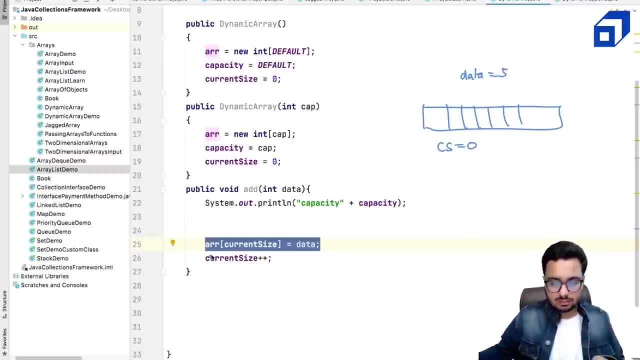 And I get some data. This should be equal to five. I said fine, array of zero, this should be equal to five. And I say current size plus plus, so my current size becomes one. So that means next time I will do insertion here again. I get a data that is six. 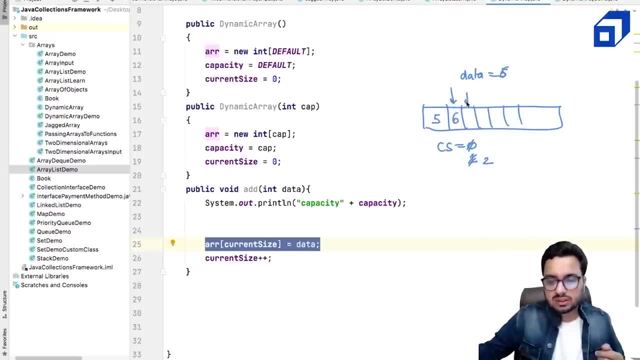 What I do. I put it here and I increment the current size to the next time. my insertion will go here. or suppose I keep on adding elements And after some time my current size becomes equal to the capacity. So my capacity was 10.. 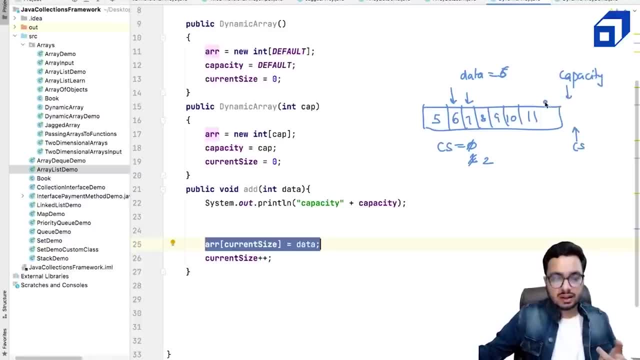 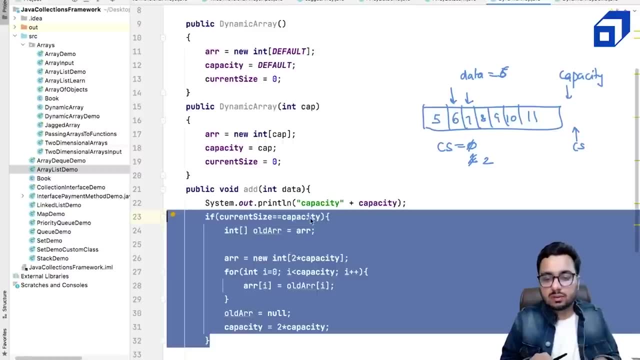 And my current size is also 10.. That means I have already inserted 10 elements. If something like this happens- okay, my current size, it's going to be equal to the capacity- what should I do? I need to double my array. how I am doing it. let us try to understand. 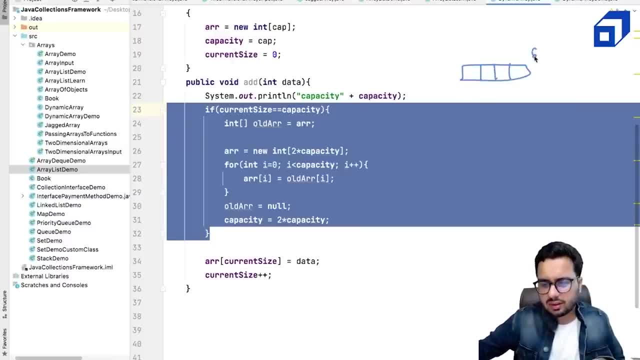 that. So let's say I have an array of size of capacity for. I insert one element, current size becomes one. I insert one more element, current size becomes two. I insert one more element, current size becomes three. I insert one more element, a current size becomes four. current size is. 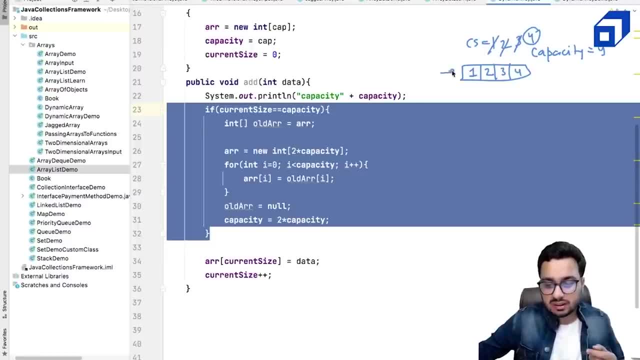 equal to capacity. If this happens- and this is my error- what do I do? I create a variable called as old array. I say okay, old array, pointing to this error, the old array. then I say error, which is the data member of the class. it should refer to a new array which has a double. 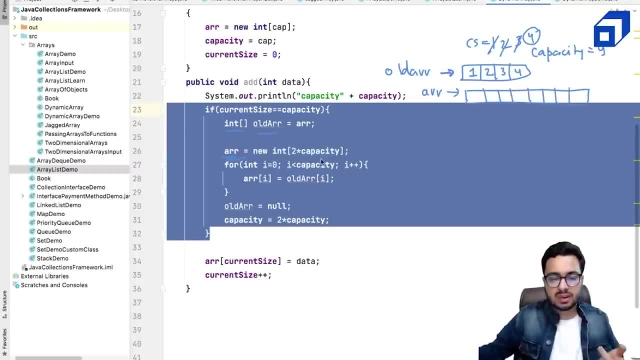 capacity. it should have double capacity. So that is what I do here. then I iterate over the old array, I iterate over these elements And I say: array of five. this is equal to old array of five. I copy all these elements. 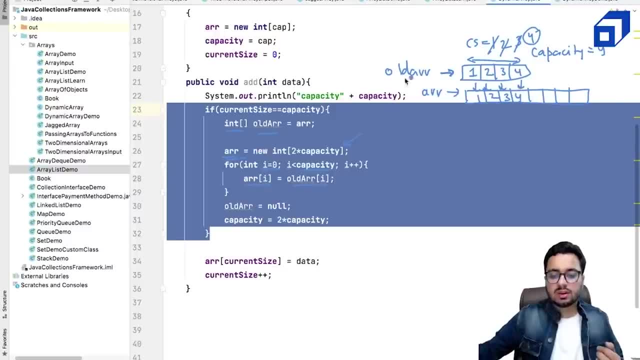 here. Fine, I do it. What should I do? I say old array. this is equal to null, So I break this connection. That means no one is pointing to this array. Now the garbage collector will delete it. here the garbage collector will get invoked. 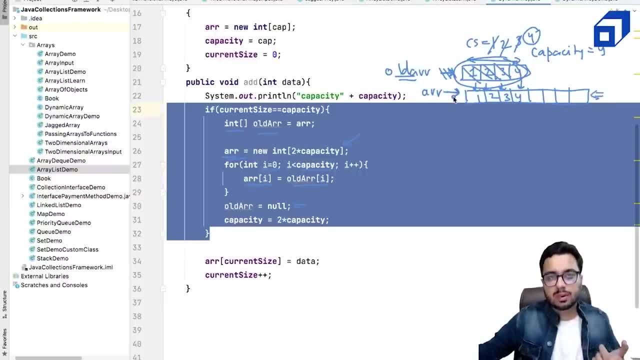 And, of course, for the new array, We have updated the array property, but we have not updated the capacity property. The capacity was still four, But now the capacity should be- I'm saying, capacity equal to twice of capacities, but what do I do? 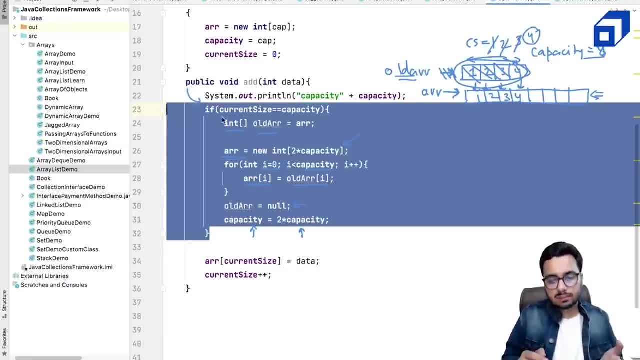 I first check if my error is full, I double it And then I can insert data into. I say: array of current size, array of current sizes still four, zero, one, two, three, four. at the fourth index I can put the new data, maybe the data. 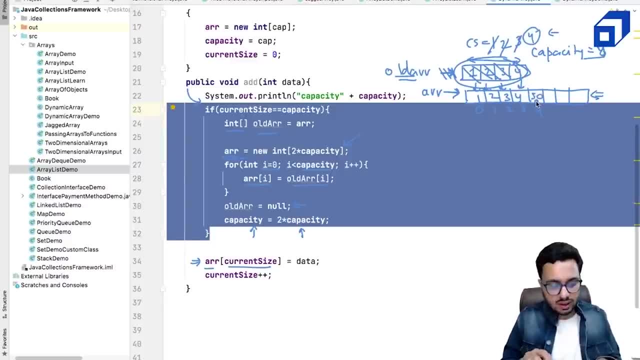 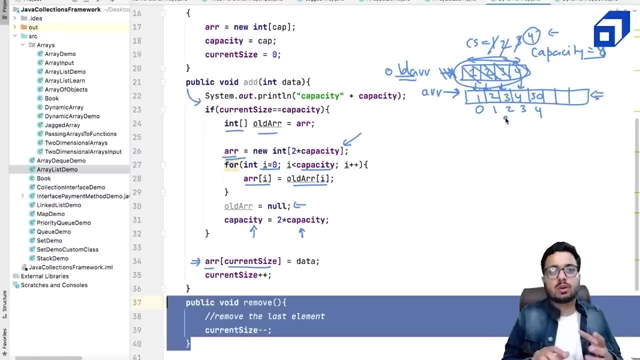 is I put it? That is how I implement the doubling operation inside my array. or suppose I want to remove something, So removing is easy. right, I'm not removing from an empty array. So that check you have to. either you do not, either you put some conditions here, or you. 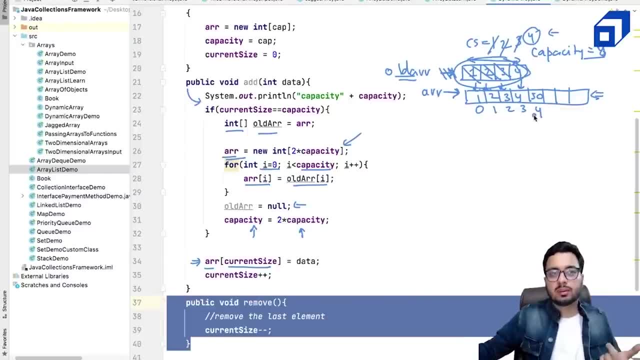 throw an exception, right? I'm simply saying, okay, I want to remove an element. I'm simply removing the last, last element. So this is my current size. I said, okay, I'll reduce the current size, And it means okay. 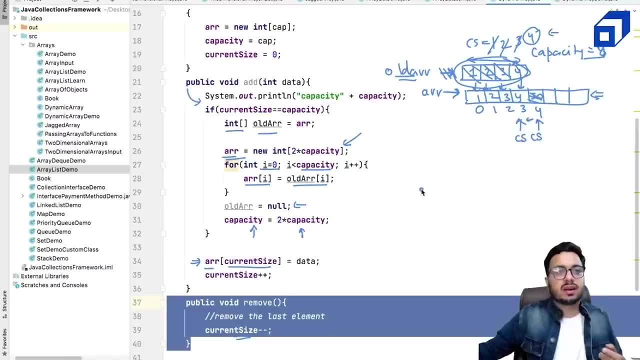 I am going one step back. current size minus minus. I'm removing one element from the array. The element will stay here, But next time you add something it will get overwritten. Okay, And if you have to iterate, you will only iterate on on this range, doing current size. 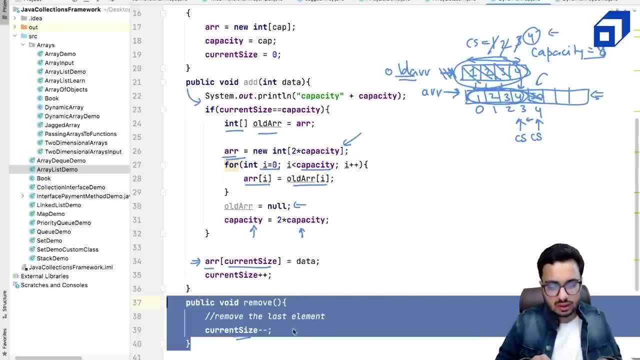 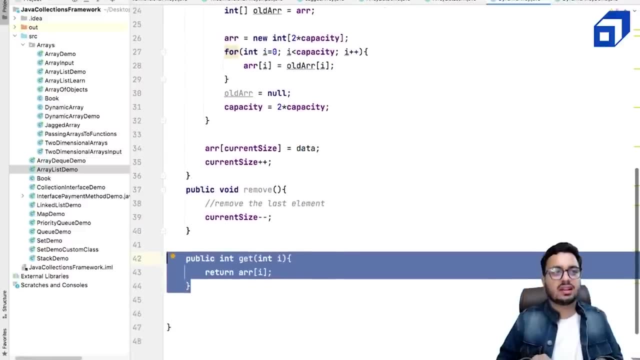 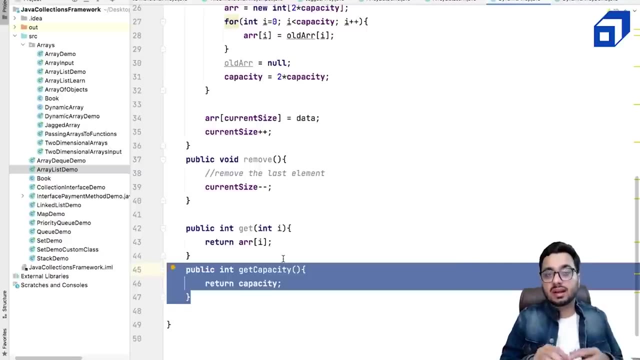 minus. minus will remove last element as well. There are some more methods we can implement. For example, if I want to Get the ith element, that is pretty easy. you simply return array of I. if I want to get the capacity- how many elements my array list can hold- I can return the current capacity. 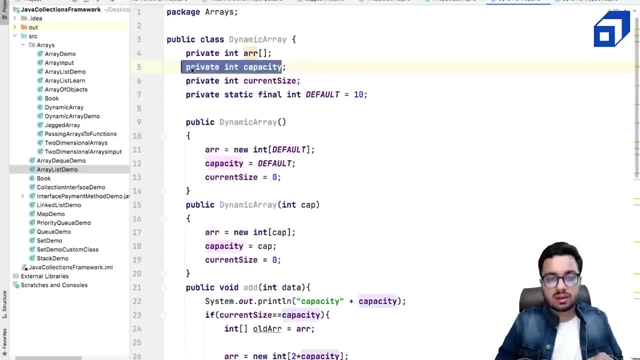 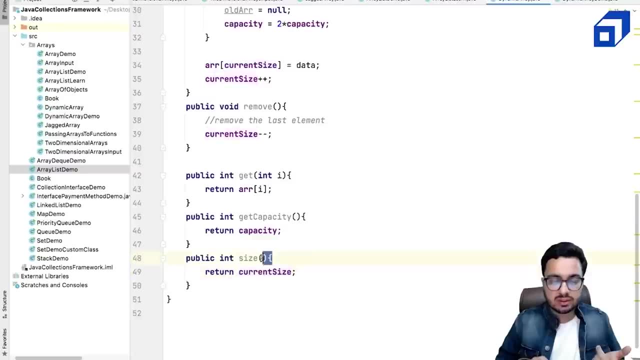 I cannot do XSS directly because it is a private variable, So I've created a getter to return it. then if I want to get how many elements I currently have, I say: okay, there is a function called size that I've implemented. it is going to. 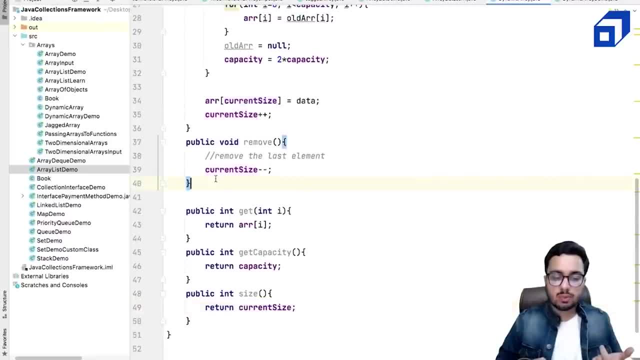 return the current size. Now you can create more methods. you can create a method called contains, in which you will implement linear search And you will tell whether that element is present or not. if you can implement a method called as index of, in which you will return the index of the element where it is present. 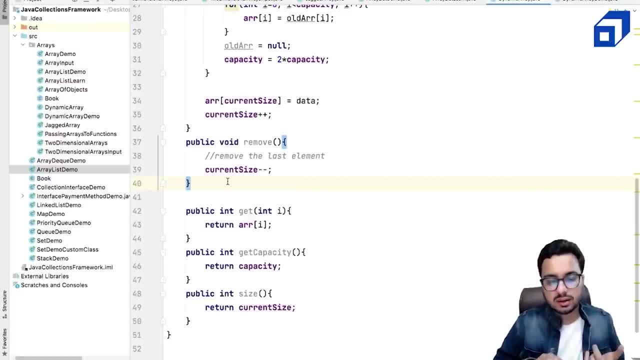 So instead of returning a Boolean, you can return an integer index as well. you can also overload the remove method, where you will get an integer value. So either you remove the element at that index Or you can remove the element at that index. 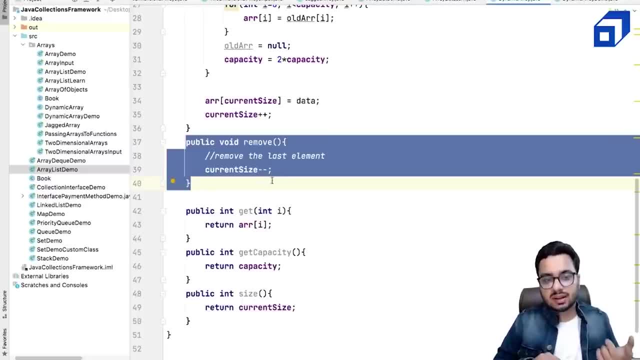 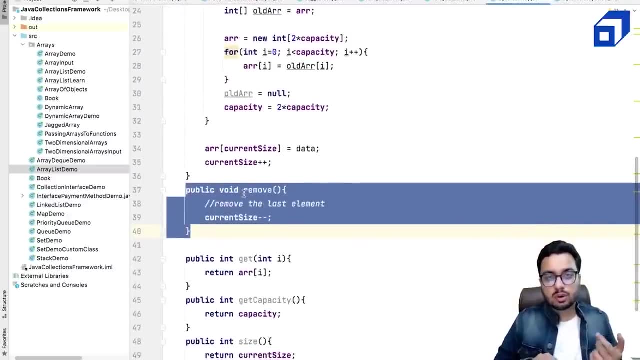 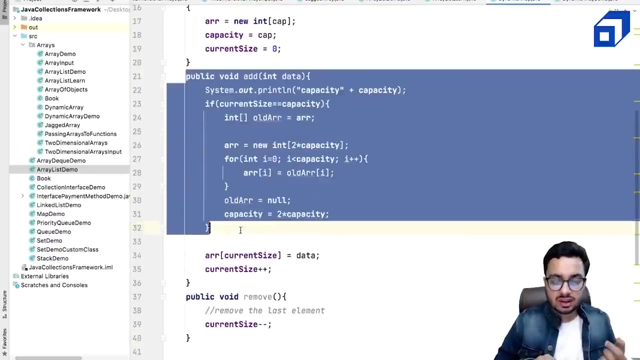 Or you remove that value right so you can do something like that as well. So the internal implementation is bit more. I would say it's more robust, it is more powerful. But this implementation we did so that you get an idea how the doubling operation in 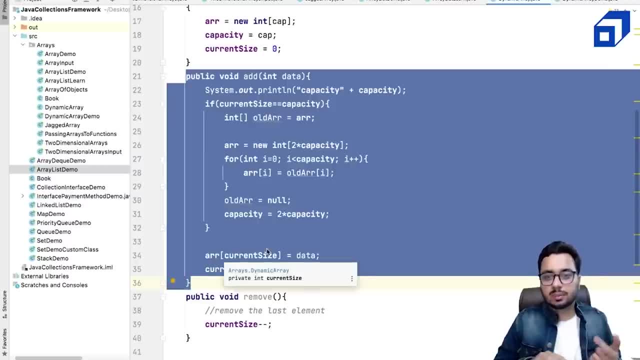 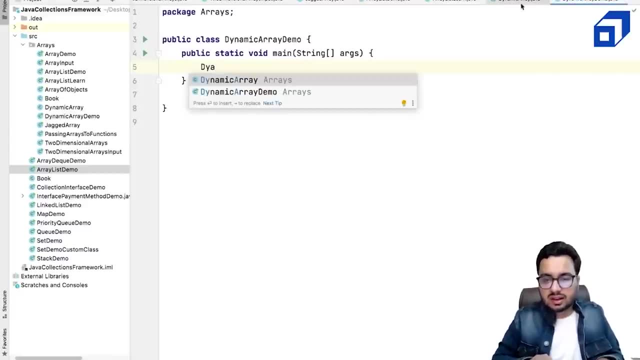 an array list is actually working. okay, how things are happening behind the scenes. Let us test our class by creating a dynamic array object. in my class that I have defined it is called as dynamic. I can say dynamic array, da this is equal to dynamic array. 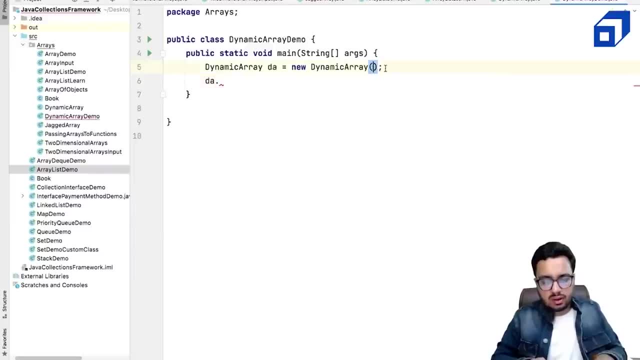 And I want to use some methods inside it. Let me say default size is five instead of 10.. So default to as it is five, da dot add one. let me just add five elements. Let me say one, two, Three, four, five. 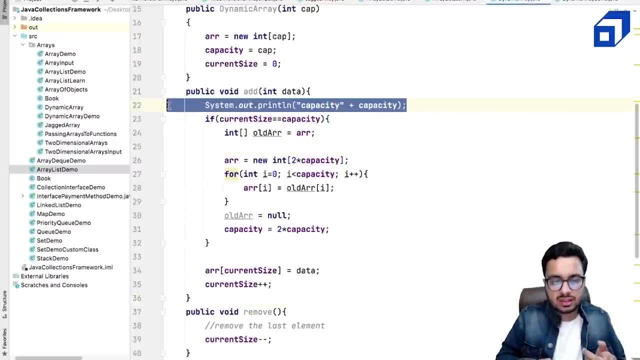 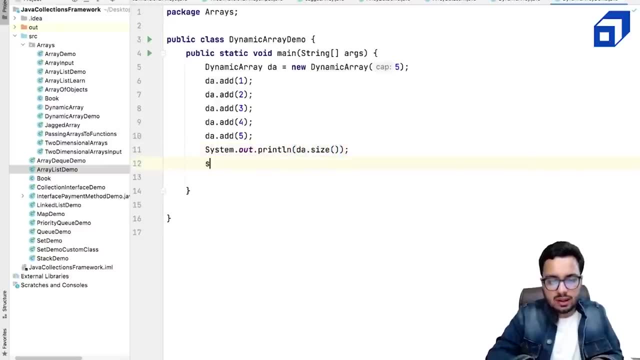 At this point I want to see what is the size of the array And what is the capacity of the array. Let us see s out da dot size and s out da dot capacity. Both should be five at this moment, But as soon as I insert the sixth element, the size should be six. 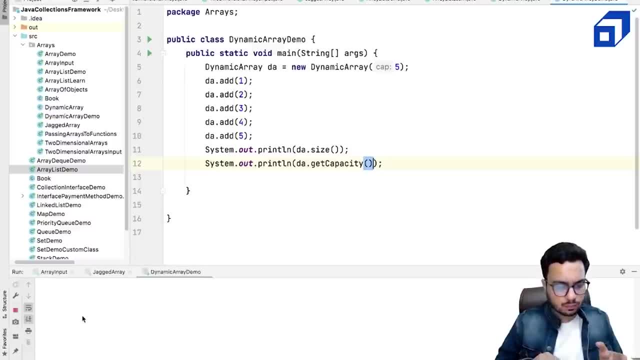 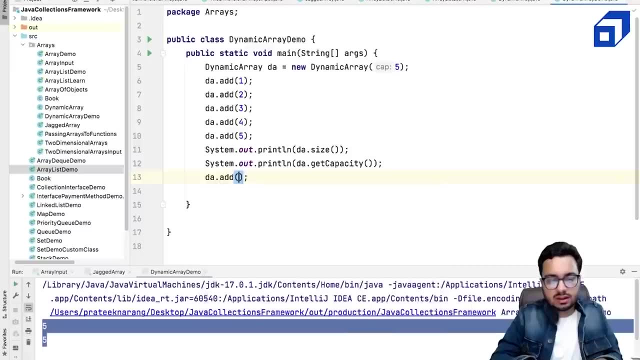 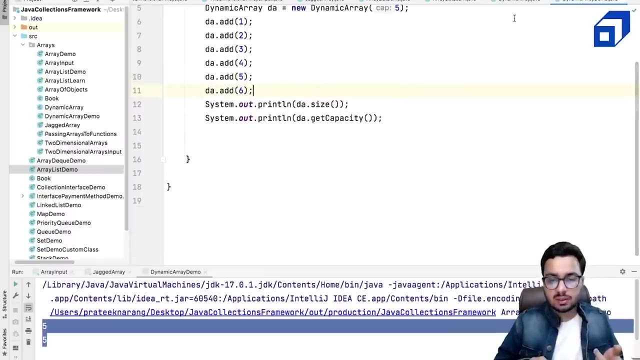 And the capacity should be Okay. so both are five at this moment. Let me insert one more element. it means a da dot art six. And now, if I add this element, you will see the doubling operation will get triggered, right. 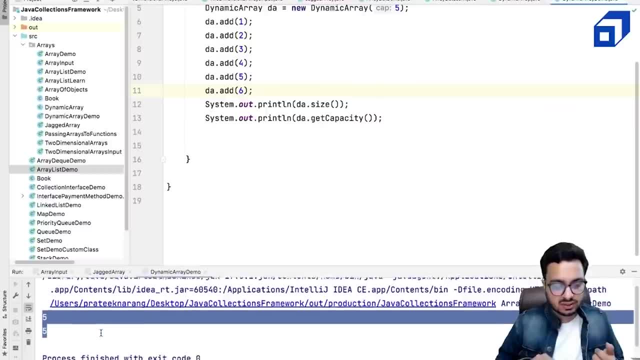 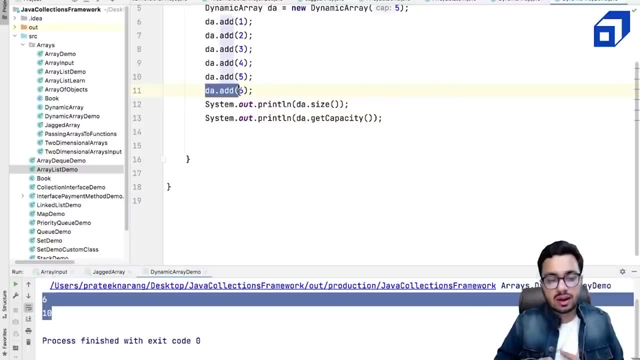 That means the capacity should be now 10.. The size should be six. Yes, that is happening. it shows your array of size. five: it got full And as soon as you add sixth element, it doubled itself. that doubling thing is happening. 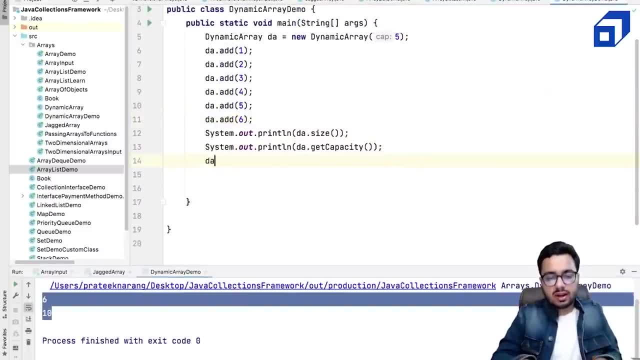 right. You can see here Now I can also say: okay, I want to add seven, I want to remove the last element, And then I want to add it. That means I added seven, I removed one element, I added it to seven will get overwritten by. 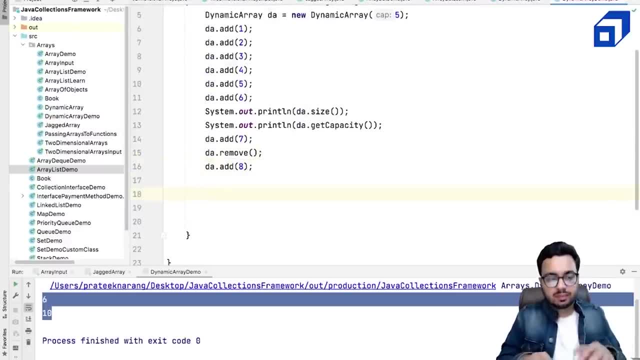 eight, And if I want to iterate on this area and see what all elements are there, so I can say for int, i equal to zero, I less than n, what is n? the number of, basically da dot size, the number of elements present. 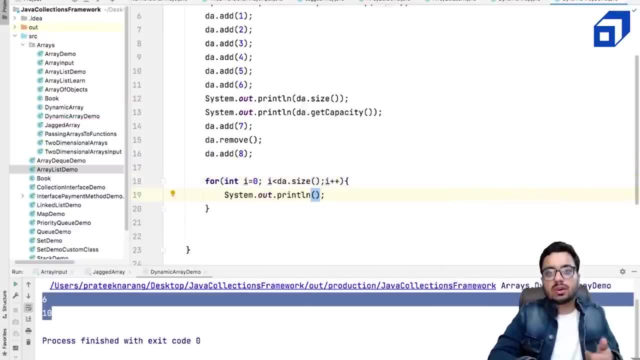 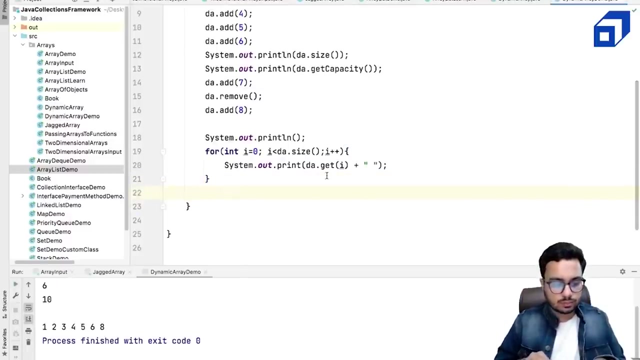 I plus plus And I can say: s out, I want to get the ith element. I can say, da dot get ith element. I want to show them in a straight line. I'll do s out here And like this: oh you can see, like 12345678.. 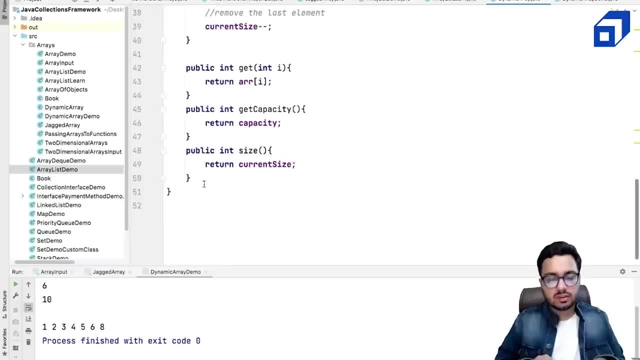 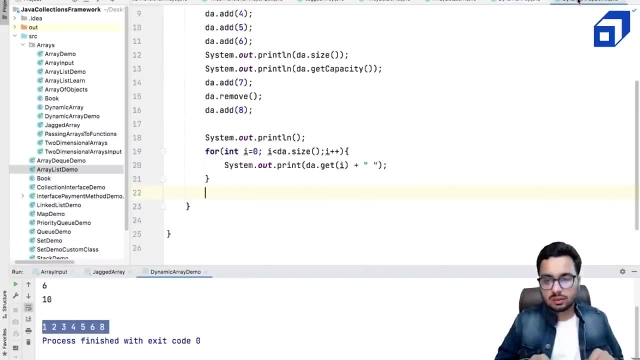 You can also implement a method called as to string, Which will simply iterate over the array and join all these numbers inside a string. So you can use the two string method also to print your dynamic array right. So instead of traversing, you can give this as a method inside the dynamic array classes. 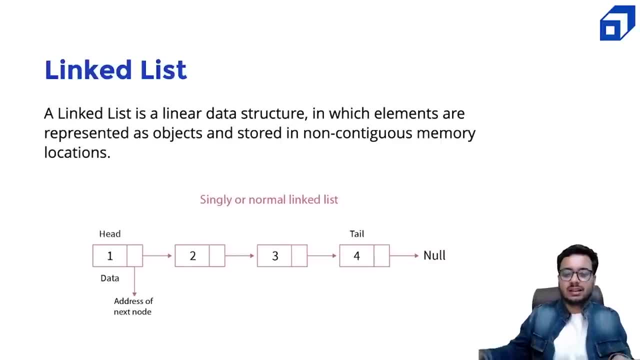 Let us begin with linked list. What is a linked list? A linked list is a linear data structure in which the elements are represented as objects and they are stored in non continuous. So let's start with linked list. So linked list is a continuous memory location. 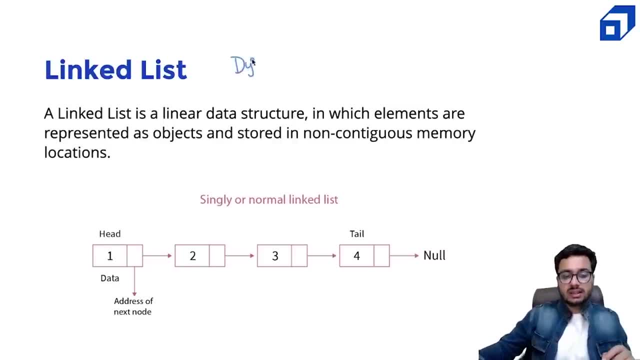 Okay. so one thing that you need to note about linked list is it's a dynamic data structure, right? Unlike an array, where you need to tell: okay, I want an array of size n. you don't need to specify the size of the linked list. 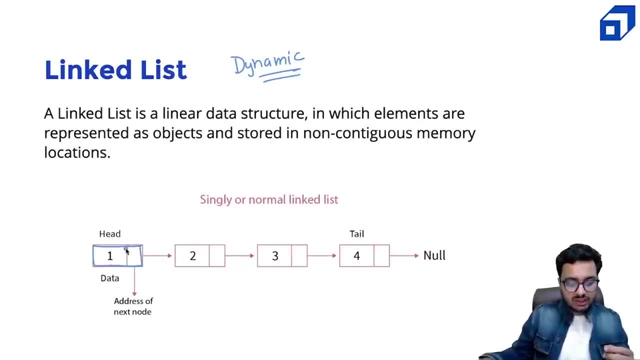 Every time you get a data, you create an object, you put the data inside it and you put it in the form of a chain or in the form of a linked list, right? So why the name linked list? because we have a lot of nodes. okay, each node is an object. 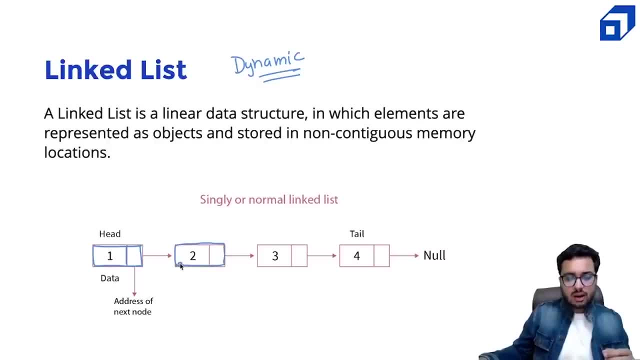 in a heap And these nodes are connected with each other. Right How they are connected. So each node is created at some memory. let's say, this address is 205.. The previous node knows that the next node is present at this address. it to will know. 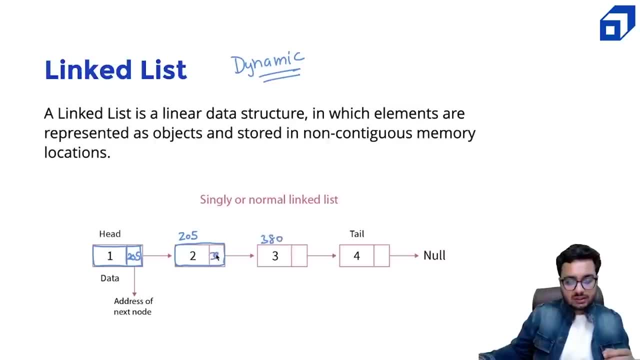 the next node is present at some address that is also going to store data, right? So each node is going to store two things: One is your data And one is the address of next node, right? So if you know the address of next node, you can easily traverse the data structure. 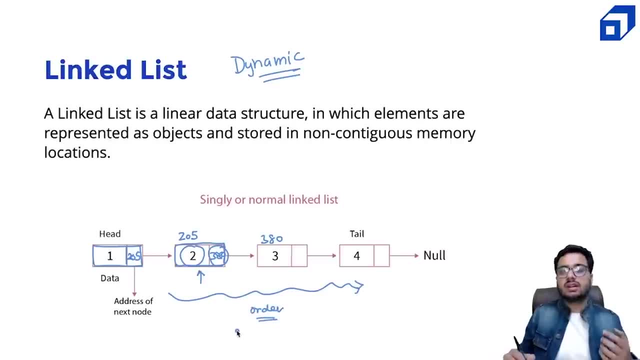 And you can also put things in Store, things in an ordered way, right? So every time you get a new data, we can insert at the beginning, we can insert at the end. we can also insert in the middle, right? So it's up to you how you want to maintain the ordering inside a linked list, right? 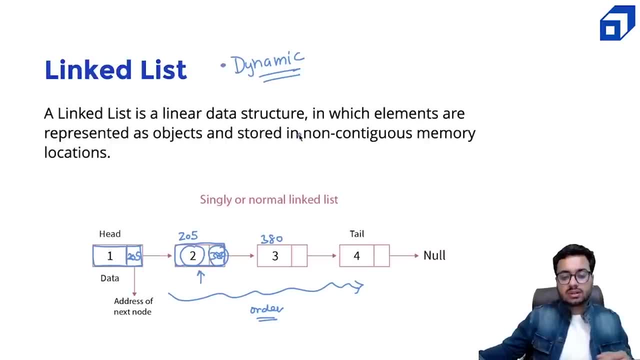 One thing to note is it's a dynamic data structure And the nodes in which the data is getting stored, they are stored in non contiguous memory locations, unlike an array right. So that is what linked list looks like right now. in linked list, we do not specify the 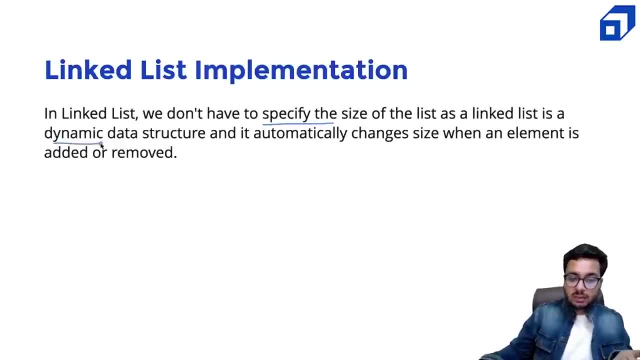 size, As I have already discussed with you, and it is a dynamic data structure. It automatically changes size when an element is added or removed. So we'll go into the internals of how addition and deletions are performed on a linked list in this tutorial. 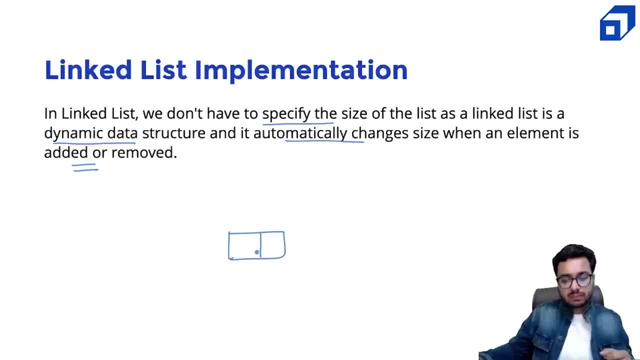 So, while doing the implementation, I will show you that. okay, if there is a node, how do I connect the next node? How do I add something in the beginning? How do I add something in the middle? How do I delete something right? 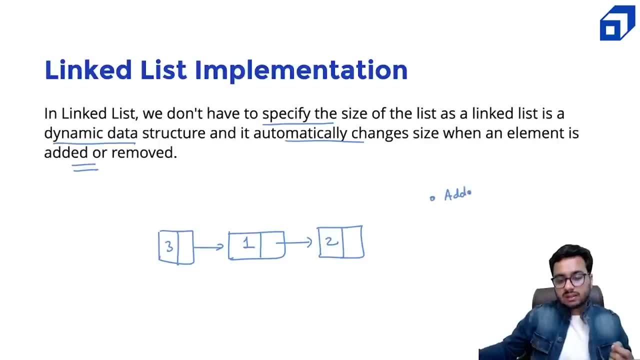 So the fundamental operations that we will be learning would be addition- Okay, Removal right And getting a node right. So I want to get a particular node. I can. how do I get that node right? So, given an index, I can iterate to that index right. 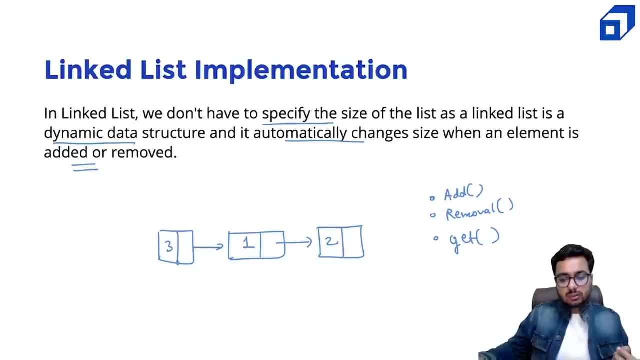 One thing that is bad about linked list is if you suppose want to get the middle node right In array, you can say, okay, give me the ith element. So this, this property, is called as random access. The linked list is a bad data structure. if you need to access ith element, why? 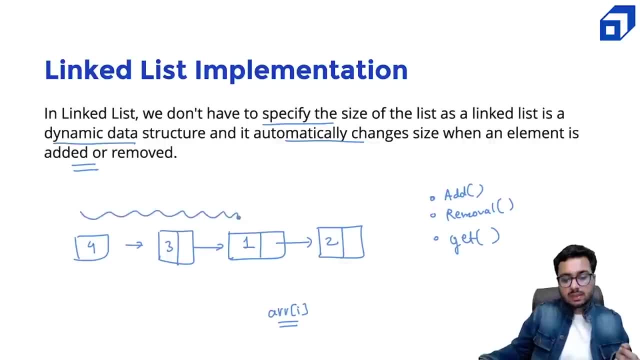 Because you cannot directly get this element. You have to traverse a lie positions to get this element right. So it's it's bad at getting nodes, It's bad at random access, but it is good at certain things that we will see. 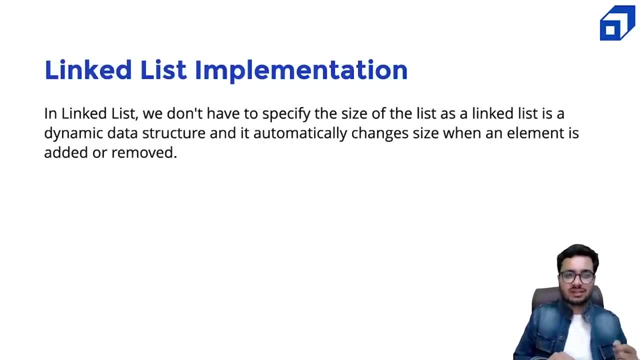 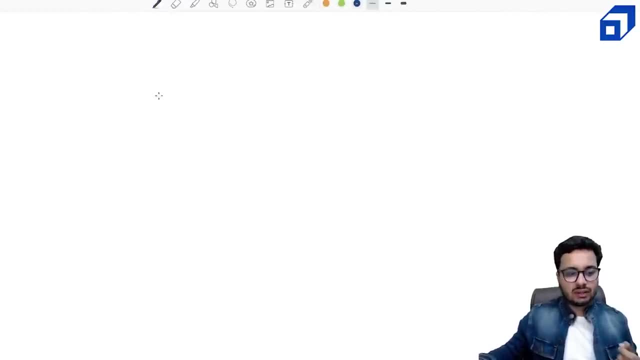 All right. So, that being said, let us jump into the implementation of linked list. Now let us dive into the implementation of linked list. So far, what we have learned is that linked list is a chain of nodes in which every node is connected to the next node. 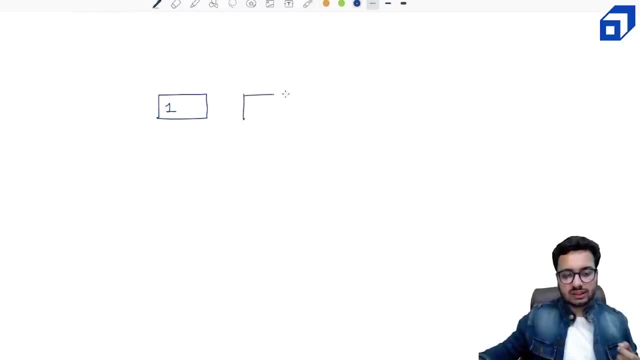 Okay, If there is a node one, it must be connected to the second node, Let's say node two. Right, So the way to do it is that in every node we also store the reference of the next node. Okay, For example, if this node is created at some memory location. let's say two zero six. then. 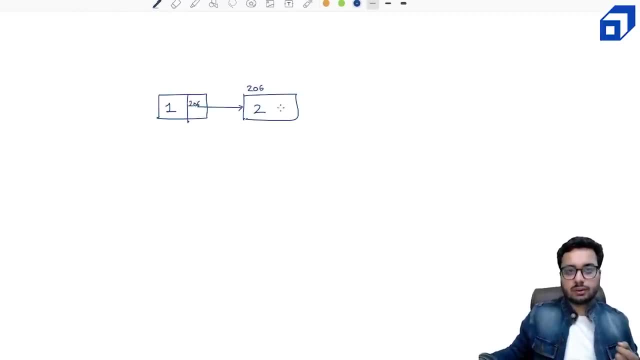 this node must store, what is the reference of this node, where it is created, right And for the first node, what we need to do. for example, if this node is created at some some location- one, one, five- then we need to store this location one, one, five in a. 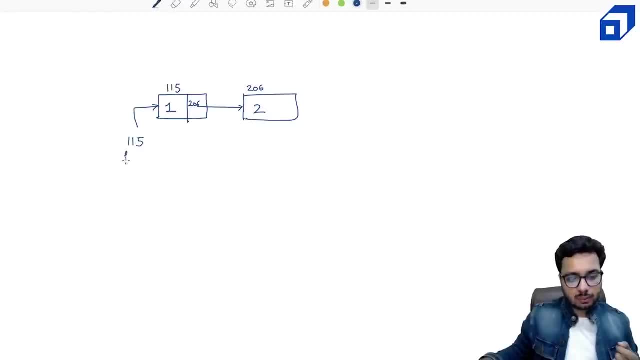 special variable. Okay, We generally call this special variable As Head. Right, Okay, And second node will store the reference to the third node and so on. Right, So, third node. maybe it might be at 480.. So I might be storing 480 here. 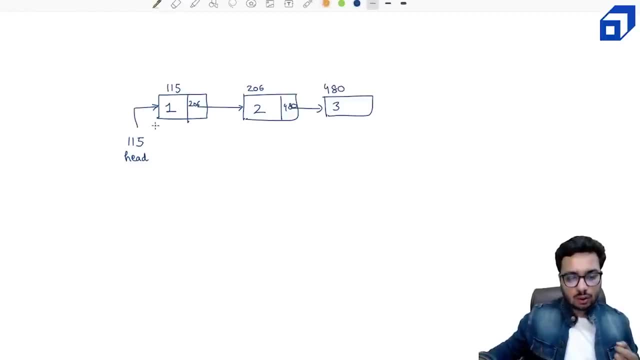 Right Now, the first step in the implementation is that: how do we implement this structure, Okay, This uh object that we see here. So we are calling this object as a node object. Right, What I will do? I will say, okay, I will define a node class and this is capable of folding. 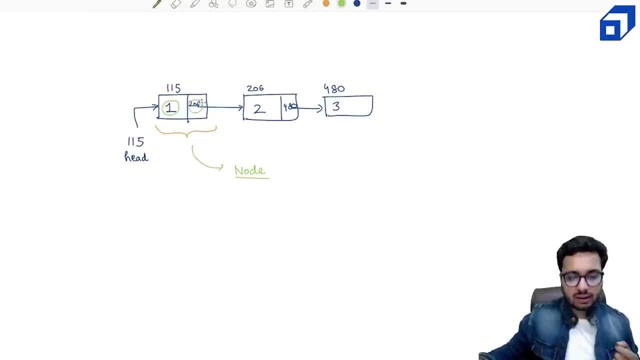 two things: One is my data and one is my reference, Right, So each of these boxes is a node, right? So each uh node is going to hold a data. Now, a data can be of a different type as well. 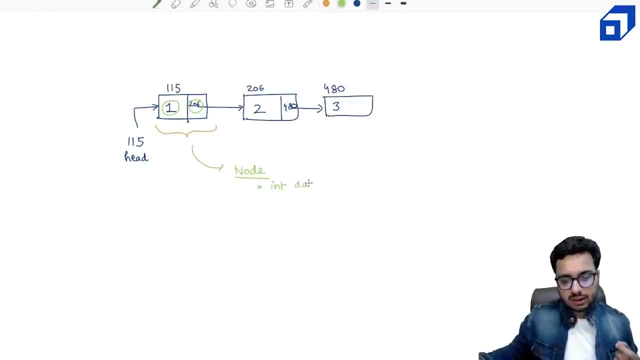 So, just for the sake of simplicity, I'm treating it to be a integer. but it can be an image, It could be a book, It could be any object. Right, And the second thing I have is a reference to the next node. 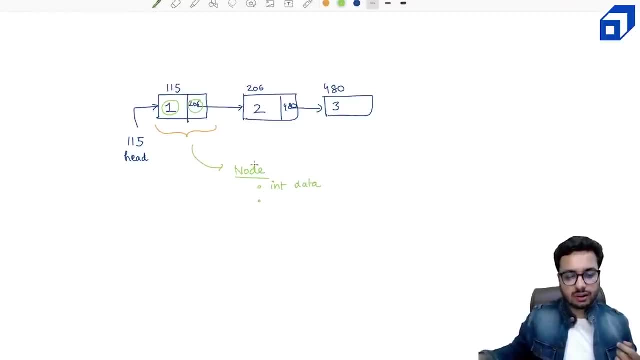 Right, So how do we uh, store a reference to the next node, Right? So I say okay, uh, this will be of the type node and let's call this variable as next. Right, We have data and we have next. 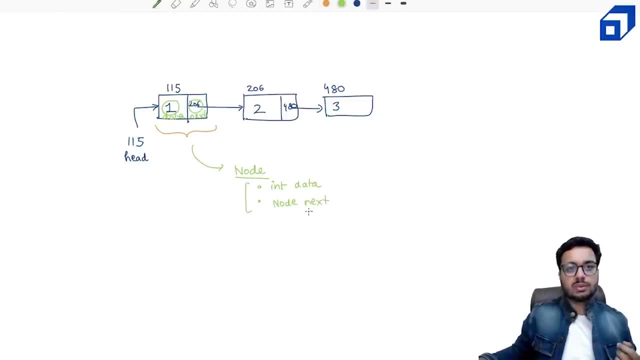 If you're confused, I will explain you. uh, what is this concept? So let us first start with the code. Let us create this structure and let us try to understand that. Okay, Inside the node class, you can have an object reference which is holding the address of: 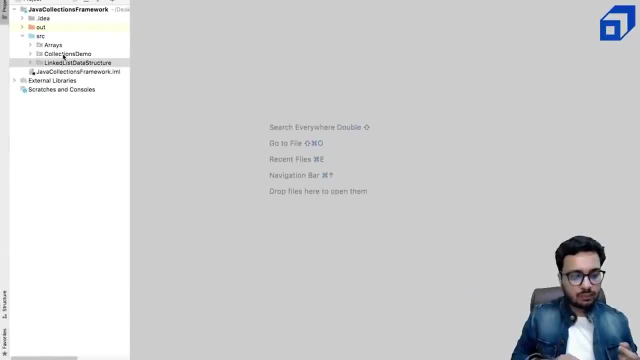 the next node, Right? So let us go into IntelliJ, And I have created a package called link list data structure, And here I'm going to create a Java class called as let's node dot- Java. Right Now it automatically creates a class for me, but it does not have data members. 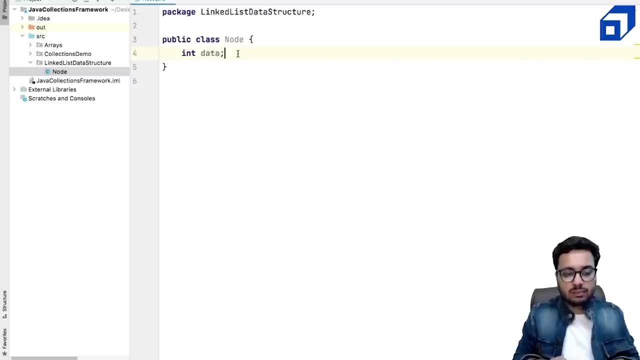 So how do I add data members? I can say, okay, I want data and I also want something called as next, So that will be of the type node Right Now. this does not mean that there is. there will be an object inside an object. 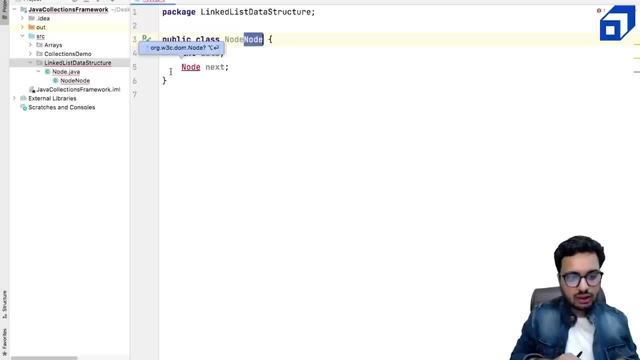 No, this is only a way, This node Right, It's only a way to hold the address of the next node Right. This is of the type object reference. I will tell you Right. And let me do one more thing. 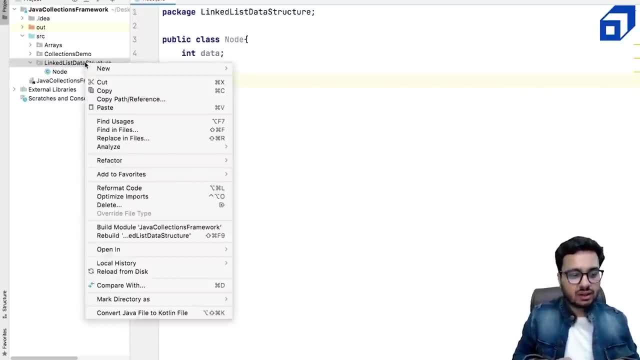 Let me add a constructor here as well, So you will see why we need a contractor. Let's do one thing: Let's create main Right. Let's create a link, list, demo and other class in which I'm going to test my functionality. 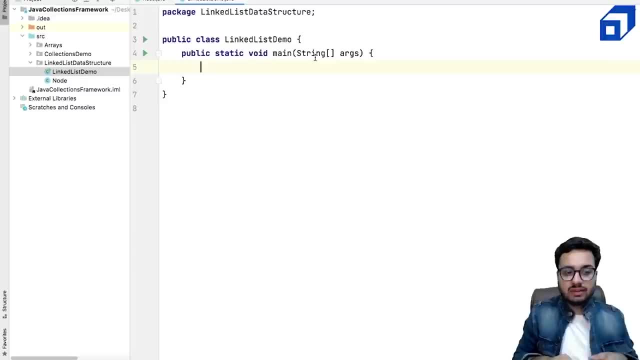 In this class I will create my main method where I'm going to test my functionality, Right? So let's create a node, object, Right? Okay, No day. This is equal to new node right now. This? no, this does not hold any data, right? 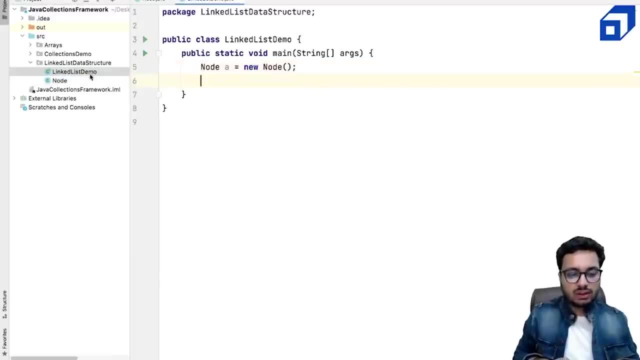 So a a is not going to contain any data by default. The value of integer is a zero Right, And next would be none Right. So what I can do, I can joke. Okay, A dot data equals to five. 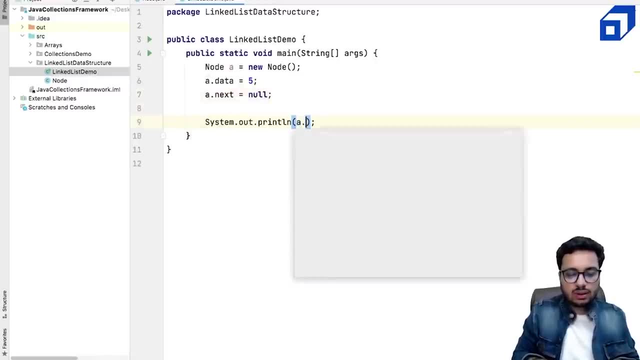 A dot next equals to null, And if I say, okay, as out a dot data, what I'm going to get, Let us see, Right. So I'm getting this uh value as five, which is absolutely correct, Right. 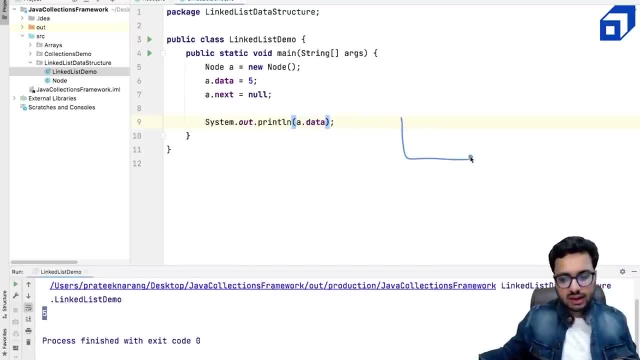 Now why this is happening. Let's see what it did Writing this code. it created a node Right, And what is a? a is referring to this node, So a is a address right, A is a object reference. 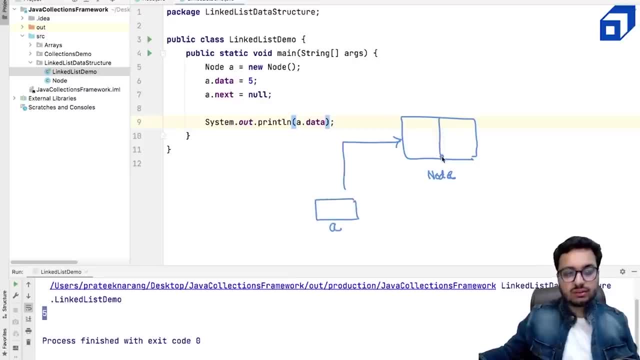 So a is another bucket which is holding the address of this node. So this node has two things: One is my data and one is minor. So this is your data and this is your next. And this node has been created at some memory location in the heap. 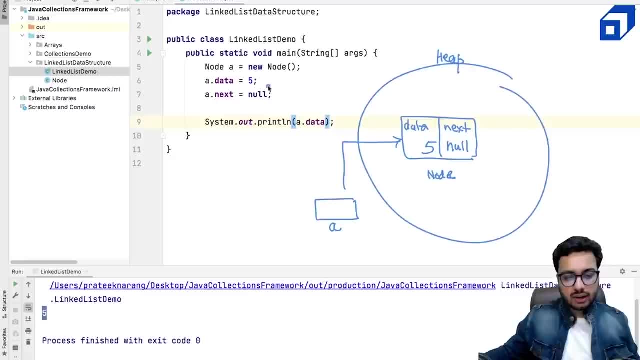 Right. This is my heap memory. So a- uh, this address might be, let's say, five zero eight, Right? What is a holding A is holding five zero eight. This is what is exactly happening behind the scenes. So in this case, this a is also an object reference right. 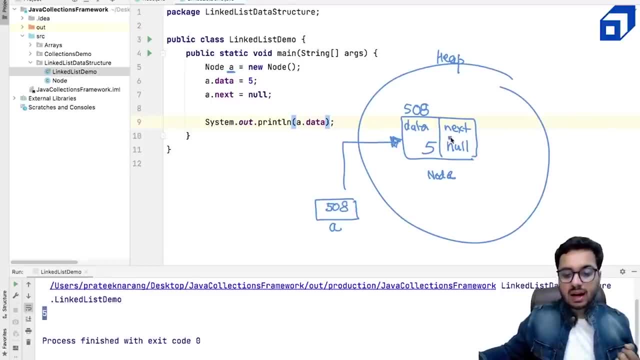 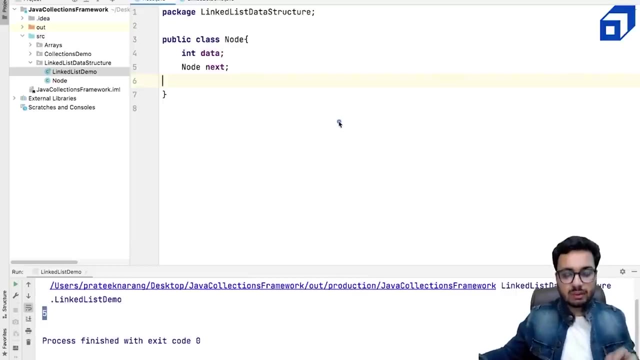 And it is referring to an object inside that object. I have one more reference. Okay, How do I access this value? I access this value by a dot. next, So this is what is happening when you're creating this node: Right, It is giving you- uh, it's wrapping up- two data members inside one bucket, inside node. 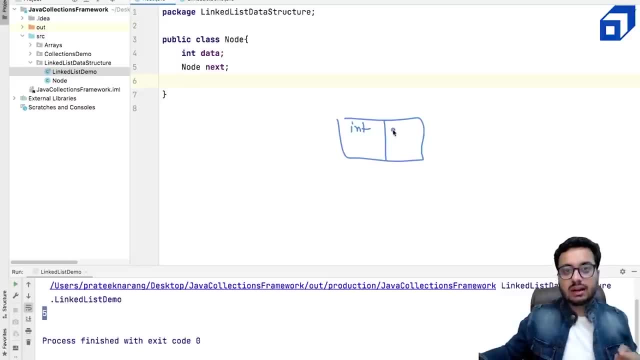 You have an integer value and a reference to the next node Right. If I say, okay, there is one more node Right, It's a node B equals to new node Right. And I say, okay, Next should refer to B. So if I print out what is a dot next to a dot, next is nothing. 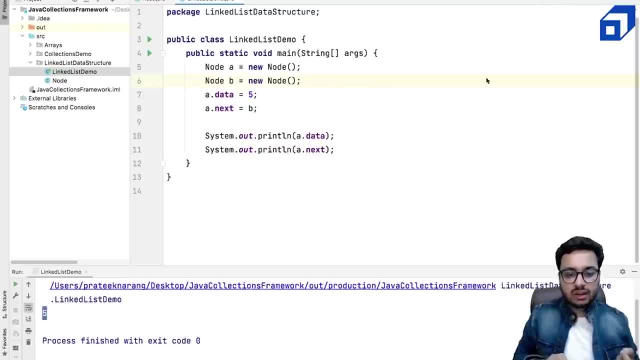 but it is the address of the B node that we have created, or the value that is getting stored inside B right now. if you see, this is the reference of the next node, right? So let me show you through a memory diagram. So a is referring to a node. 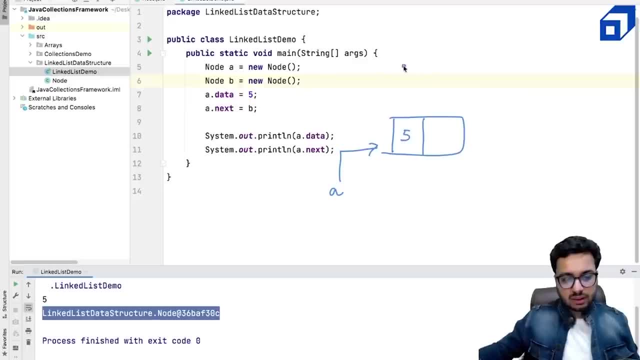 Okay, A is five, B's some other nodes. So let me do it like this. So a is a variable that is holding this address. Let's say one zero eight. This value is five and B is 30, C Right. So B is some other node. 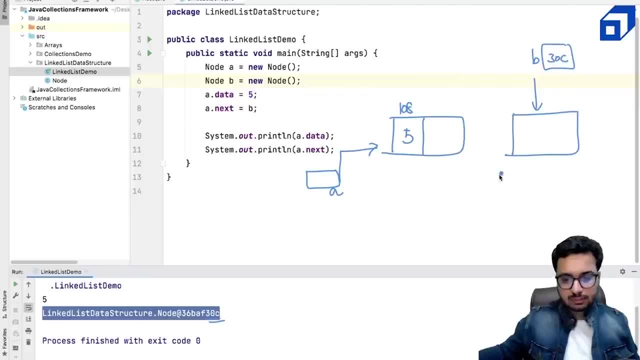 B is another variable that is holding this value. 30 C. Right, And this is the address of next node. I don't have any data and null value, So it will be the default value of integer and uh, next right. 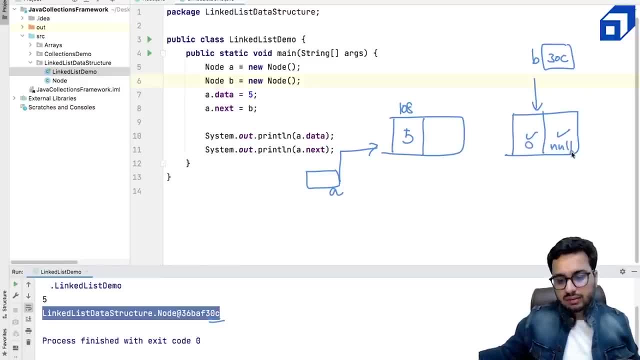 So that will be zero and null Right. So I have zero and I have none. Now B is referring to this. So when I say a dot next equal to B, so inside a dot next, which is this field, I'm copying. 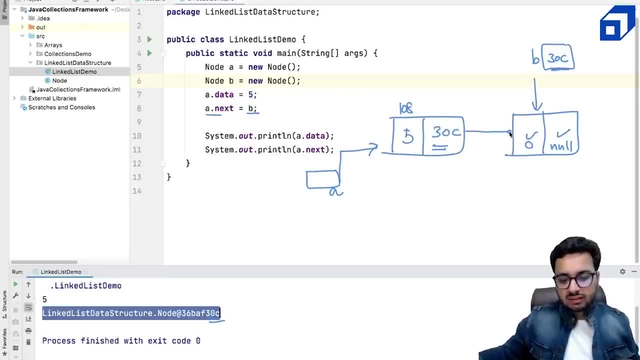 whatever is present in B. So I'm copying 30 C. It means, in a way, this B got connected with it Right Now. even if I lose this variable B, this chain is still connected, right. So this is how we are going to work with nodes. 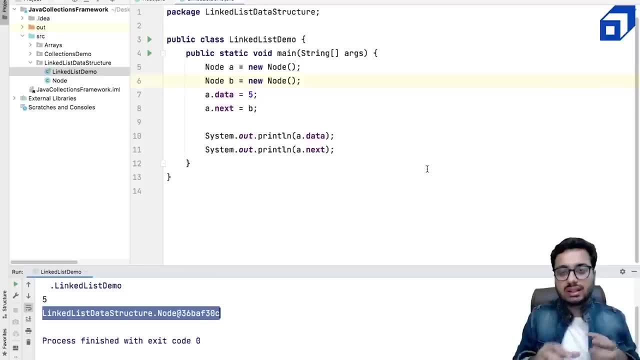 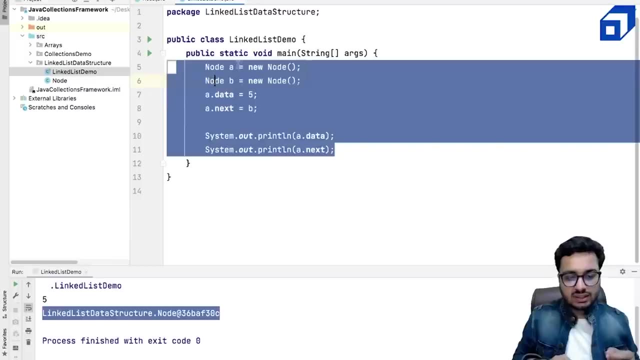 And we will write one more class that does all this manipulation of nodes. We'll call that as a linkless class, Right? So I hope this node concept is clear. What is a? what is new node? The new node is getting created in heap. 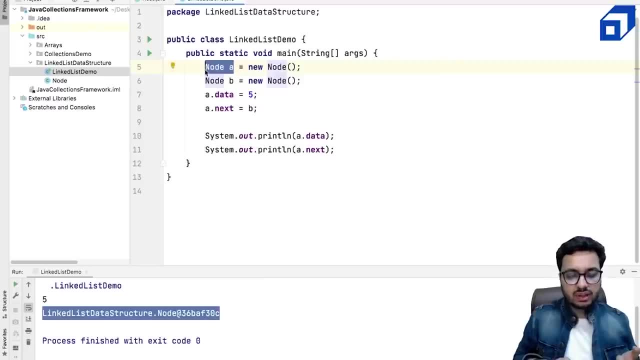 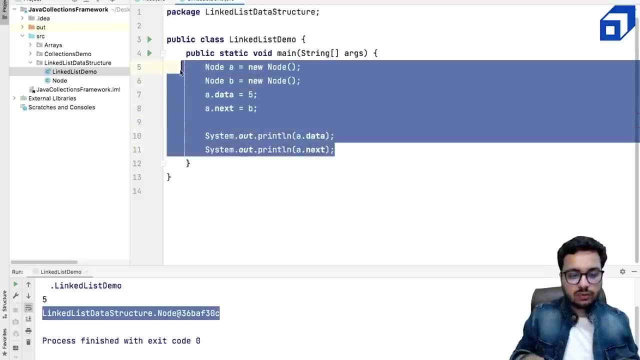 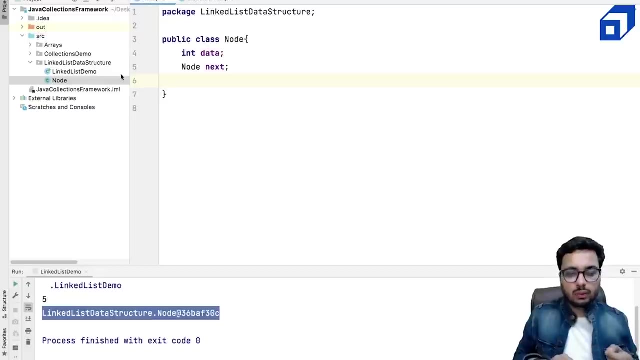 In this case, this is a reference variable here, And this variable is created inside stock at this point, Right? So what I will do? I'll remove all this code and I will do one more thing, Instead of, like every time, doing a dot data equal to something, a dot next equal to something. 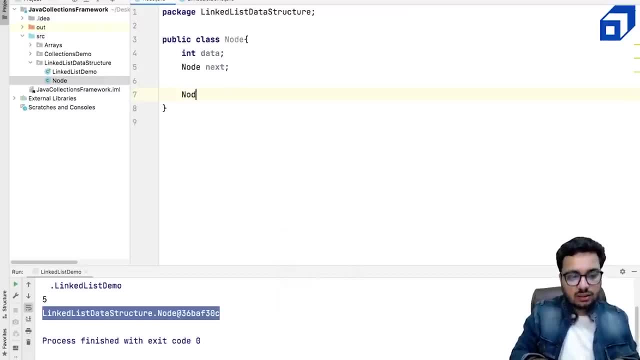 I will define a constructor inside this class. I call it as node. It will accept some integer, Let's say data. It will accept some value of next, but in general we will not know that value of next. Okay, So whenever you creating a new node, you know the data is okay. 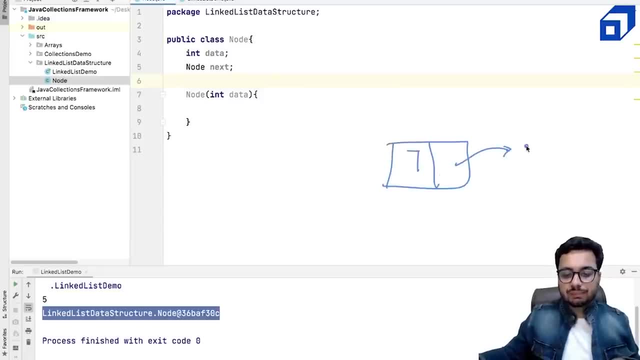 I want to create a new node with data seven. What will be connected in the next node, We do not know at the moment. Right, So what we can do, we can leave this variable initialized with the default value. Right, So I can say this: dot data equals to data. 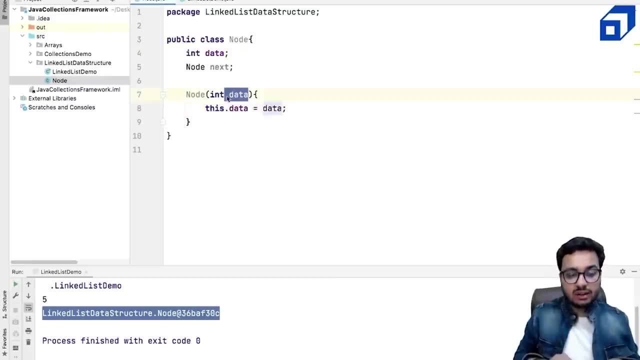 I'm initializing this variable with the data that I'm getting Right. So, since the two variable names are same, writing this here is important, so that compiler knows that we are talking about this data member as an attribute. Right And next. what about next? 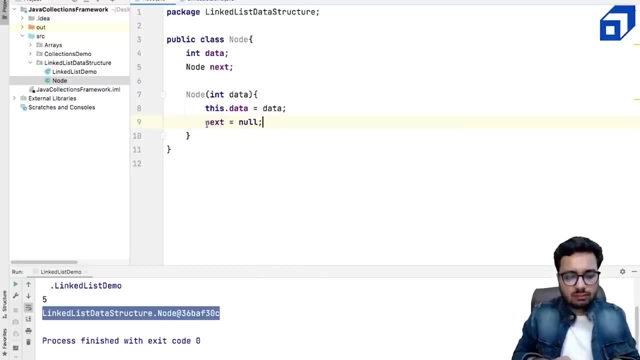 So you can say next is null. or you can do this dot: next is null. Both are fine, Both will work Right. This is the constructor for the node class Right Now. if you want to create a node A now, you will say okay, node A equals to new node. 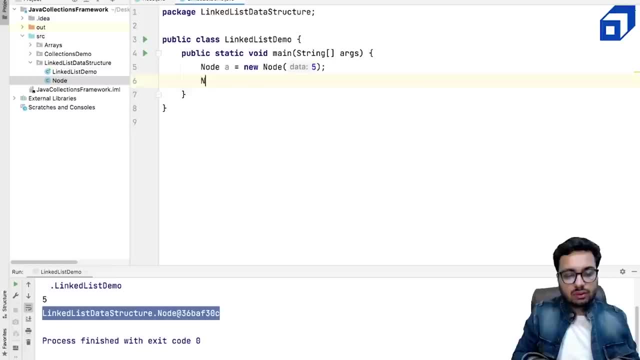 You just give the data as five and you say node B equal to new node, You will say data is six and A dot next equal to B. This creates a very simple linked list in which we have two nodes. Okay, If I say sout A dot data and show me what is the data in the next of A. 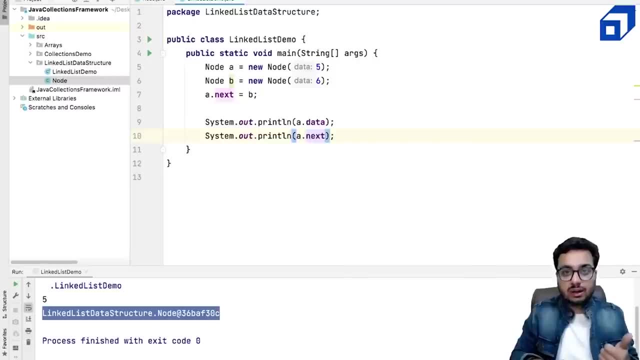 So how do I do it? A dot next gives me the address of B, The address of B dot data. So I will say five followed by six. Right? So I will see this. So I see five followed by six. So what we did? we simply created a linked list in which we have just two nodes. 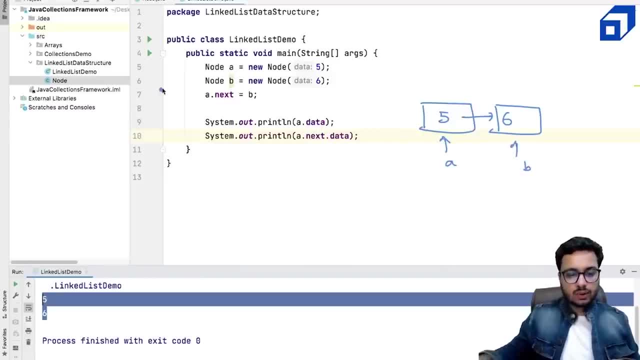 This is A, This is B, Right, Okay, And A dot next is storing B. So A dot next is storing Right Now. you might say, okay, this looks very easy. I have to add ten nodes, twenty nodes, hundred nodes, thousand nodes. 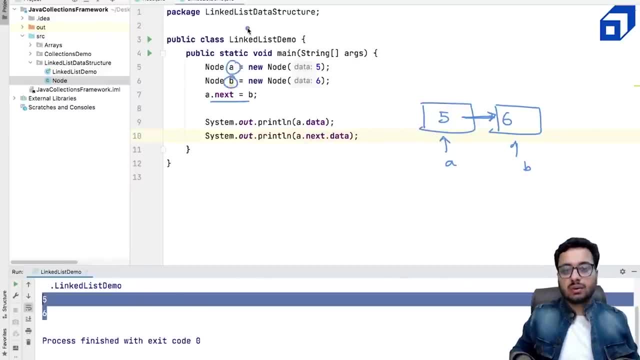 Will we create so many variables and attach them manually? The answer is, of course, no. We will write an algorithm that does insertion in the linked list, deletion in the linked list, And it helps me to get the nodes in the middle of the linked list or at the end of the linked 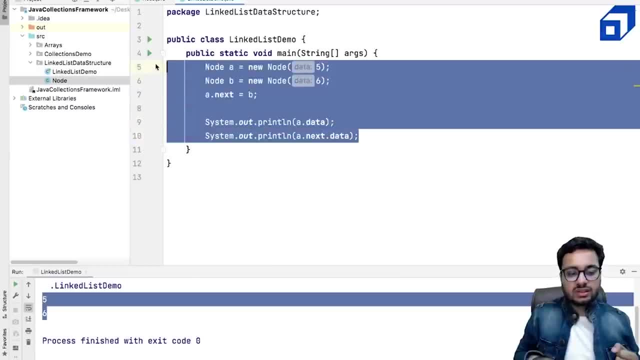 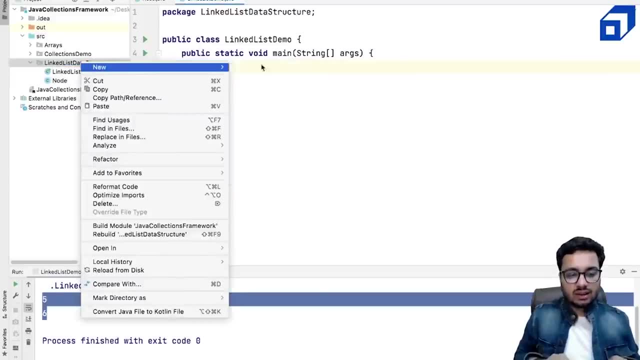 list or at the beginning of the linked list Right To do all these operations. what we will be doing, we will be writing our own linked list class. So what I will do, I will create a new Java class and I will call it as linked list dot. 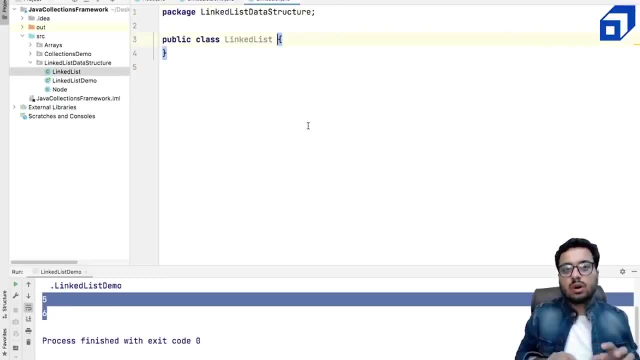 Java, in which all these operations involving these nodes will be done. Right, Let's see the implementation of linked list. So let us see the implementation of linked list. Suppose you want a data structure that is like in the form of a chain- Right, 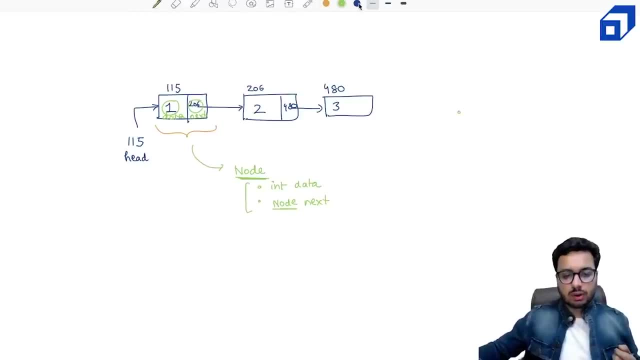 And you want to build certain methods. You want to say, okay, I want to do addition in this linked list. That means I should be able to add more nodes inside it. I should be able to remove nodes from this linked list And I should be able to get the nodes from this linked list. 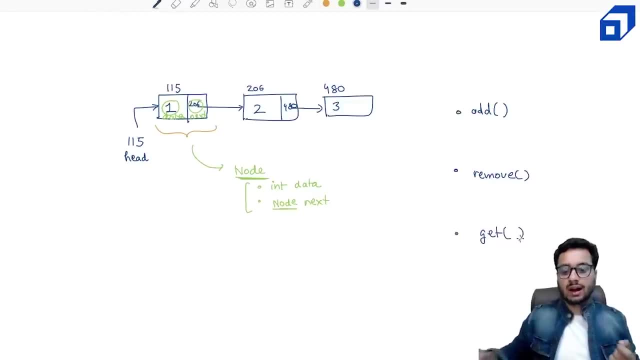 That means I want to read nodes from the linked list Right Now, the add operation. it can happen at three places, Right? Maybe if there is a linked list like this, you can say: okay, I want to add something in the beginning of the linked list. 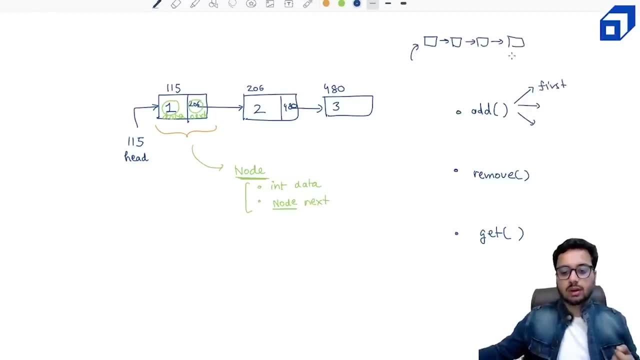 I can say, okay, add at the first position. Or you might say, okay, I want to add something, Add something after the last node, Right? So you might say, okay, I want to add at the last node. Or I might want to say that I want to insert something in the middle. 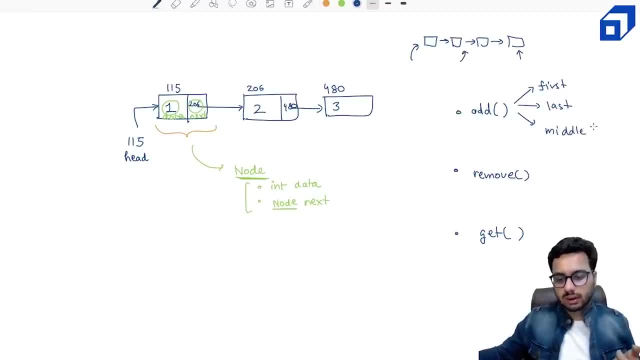 So I might be doing something in the middle or at a given location- Okay, At a given position inside this linked list Right. Similarly, remove can happen at the beginning. So I will say: remove first would be an operation, Remove last would be an operation. 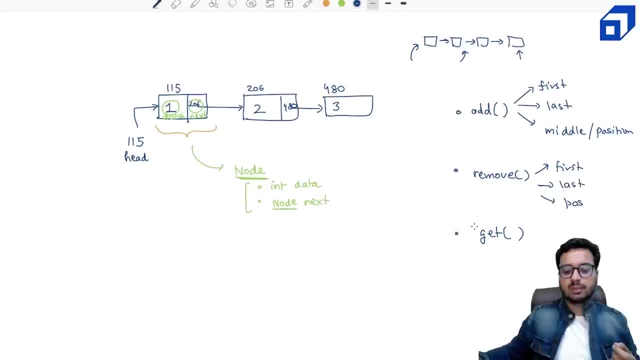 And remove at a particular position can be an operation. Similarly, get me in the. okay, I want to read something. I want to get the first element, I want to get the last element, Or I want to get the middle element. Right. 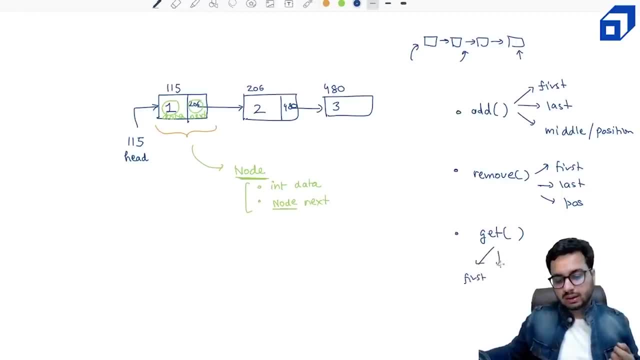 So I will say: I want to get first element, last element and element at a given position, Right. So what we will be doing, we will be implementing these operations Right Now in order to implement these operations Right. What is important. 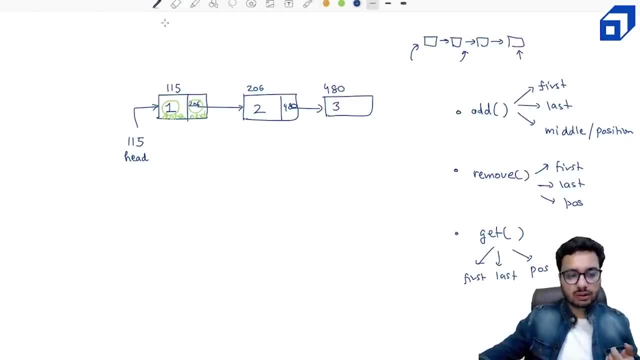 Let us start by understanding how my add operation will work, Right? So whenever you want to add something, So one thing you need to know is what is the starting point of the linked list, Right? So suppose you want to add something in the beginning, you must know the starting point. 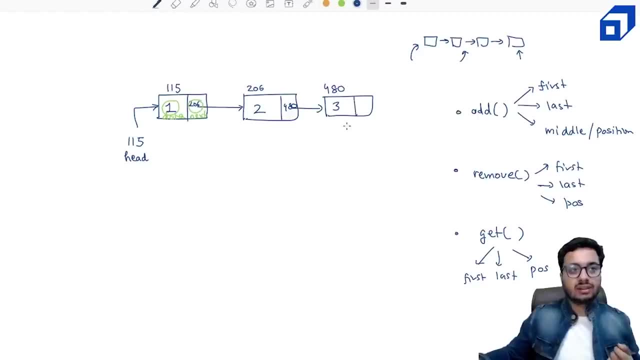 Or you want to add something at the end Right. One way is: if you are adding something at the end Right, That means, if you are creating a node here, you must access this node and update the next variable of this node Right. 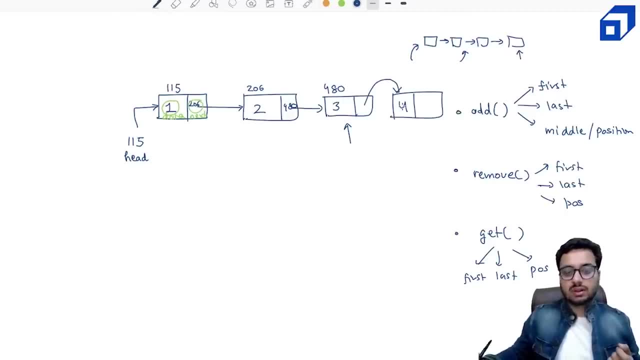 You would say, okay, in the ending of this node, I will attach this node. One way is you always iterate till this point, Starting from the head, And this will actually take order of end time. If you iterate from here to here, it will take order of end time. 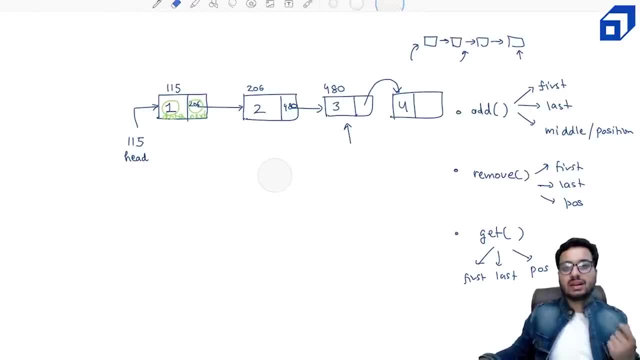 So I don't want to do that. What I will do, I will say okay, every linked list will at least know what is my head and what is my tail. I will keep another reference that always point to the last node of the linked list. 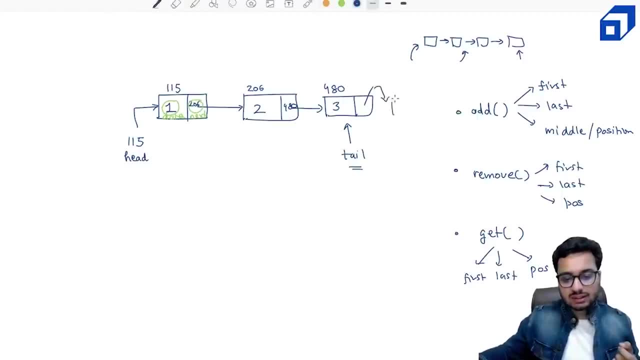 Whenever you will add a new node at the ending of the linked list, I will say okay, I will modify the tail node, I will attach the node and I will update my tail variable to go here Right? So let us see how these operations are implemented. 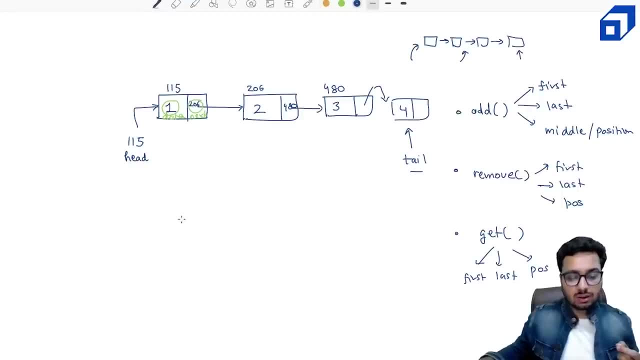 So what I'm trying to tell you is that, if you're implementing a class called linked list, this linked list will have data members- Okay, Something that the linked list should know, Okay- And some operations that the linked list will does- Right. 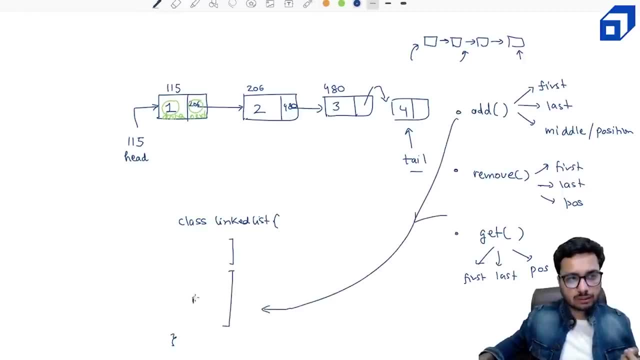 So here are the operations. They will be part of the methods Right, And we will have some data members or attributes. What are the data members? What are the things that the linked list must know? One is head. What is my starting address? 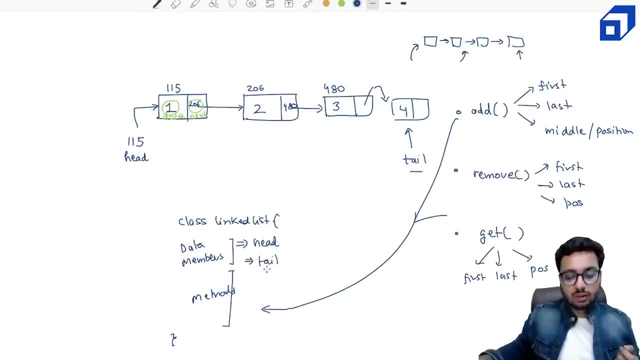 One is the tail. What is my ending address? So again, keeping this is optional, but I want to optimize certain operations. For example, add at last should not be an order n operation, It should be an order one operation. I need to keep the tail variable as well. 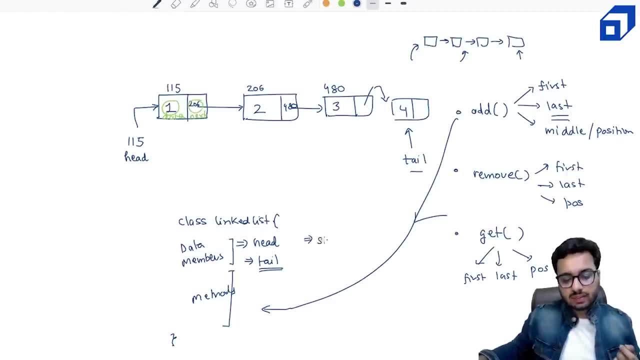 Right, And maybe some optional information like size- How many nodes I have in the linked list? Okay, So maybe I want to implement a method like get size- How many items are already inserted in this linked list? This is a useful operation. 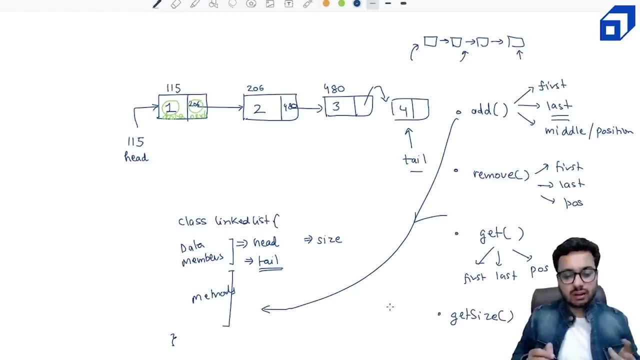 We want to check. Okay, If the size is zero, that means linked list is empty, Right. Otherwise, you can check: if the head is null, That also means linked list is empty, Right. So we will also implement this operation like get size, and maybe we'll implement operation. 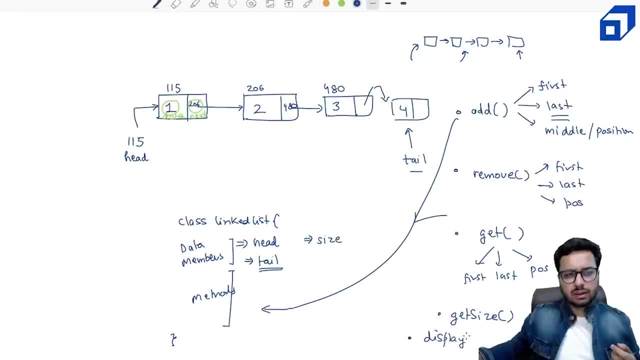 like display. I want to show the entire linked list. Okay, Or you can implement a method like to string. I trade on this linked list and convert it into a string. So that is just like a display method. I want to show the entire linked list to the user. 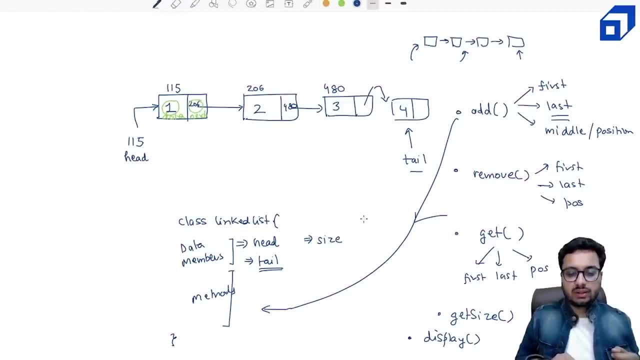 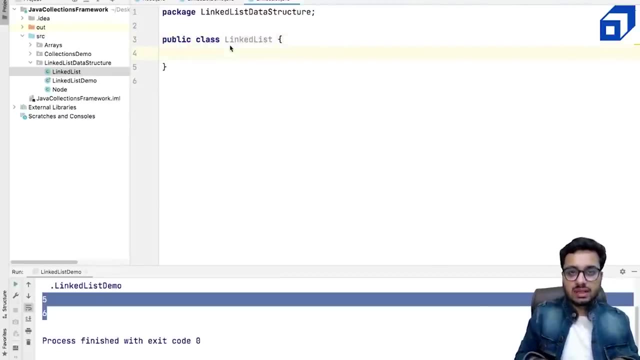 Right, So let us start by implementing these operations one by one. This is my linked list class. So, first of all, what I will do, I will add some data members and I will add a constructor to it. That's okay. I want to create a head. 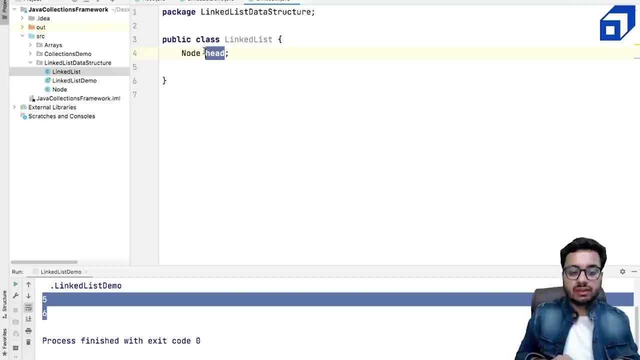 So node head. Again, head is a object reference. It has a data type called as node. Then I will have node tail And one thing I can do is I can make them private. So private node head and private node tail. I don't want people outside the linked list class to know where is the head node where? 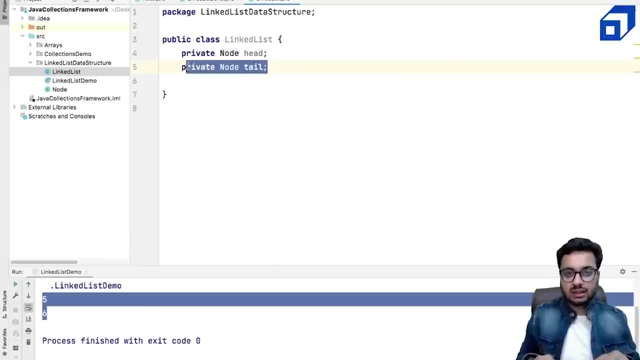 is the tail node, So I will not expose this data outside the linked list. class Right And I can also say private int size. I'm not making it public because I don't want this size to be changed by someone outside. The size should change automatically. 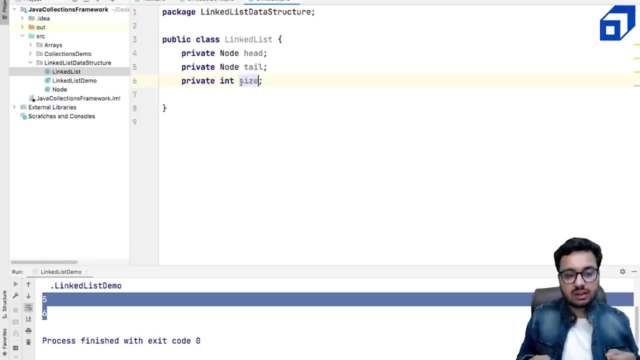 When something is inserted or something is removed from the linked list. So it should be a private variable only changed by the linked list class, Right? Next thing I want to do is I need to initialize a constructor. Okay, When, whenever user says, okay, give me a new linked list. 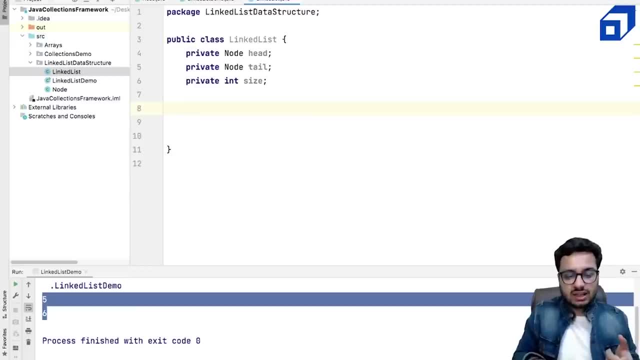 What should I do So that linked list will have zero nodes inside it, So I need to initialize these three data members as well. That is okay, Linked list. There is a constructor here, And what I want to do? I want to say head and tail. 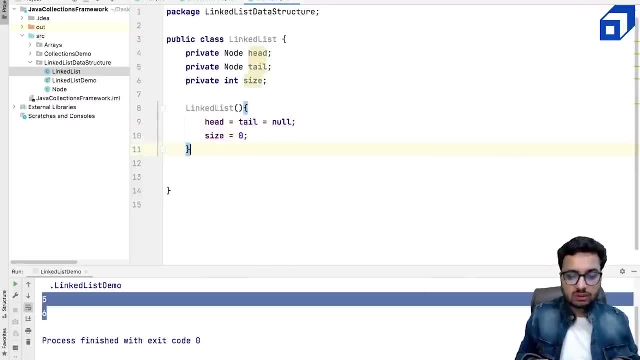 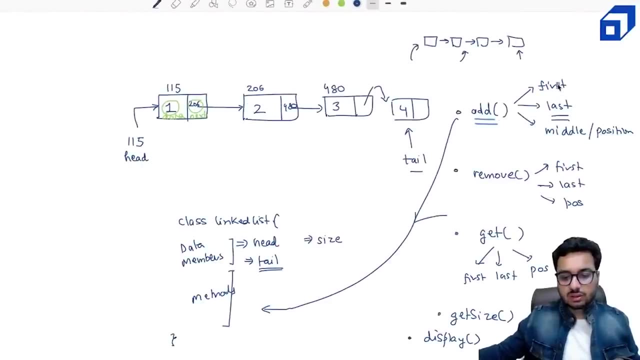 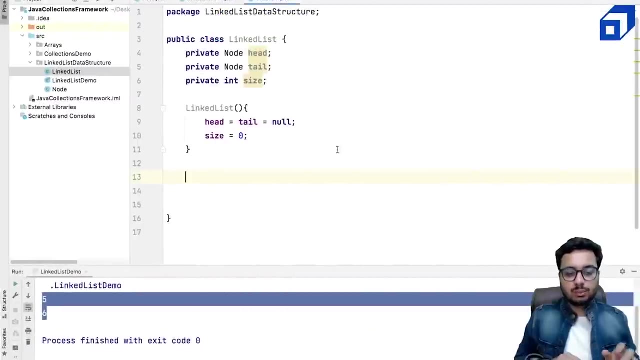 They will be null and the size would be zero. Okay, So this is my constructor And what is the first thing I will do? I was okay, I want to do an insertion. I will add: I'll write three methods: One to add something at the beginning, something at the end and something at a given position. 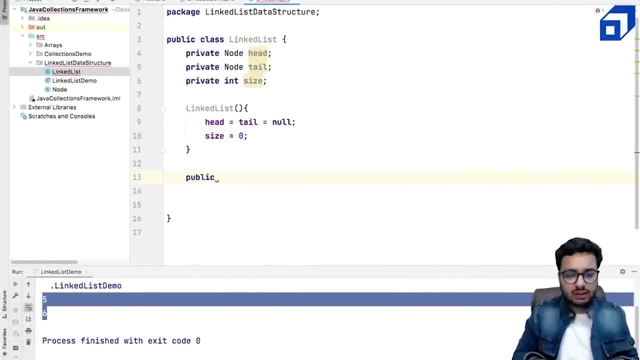 in the linked list. That's okay, Public method, And the method is of the type void Add, And let me call it as: add first, Okay, And public void at last, And public void Add at a particular position. So add at. 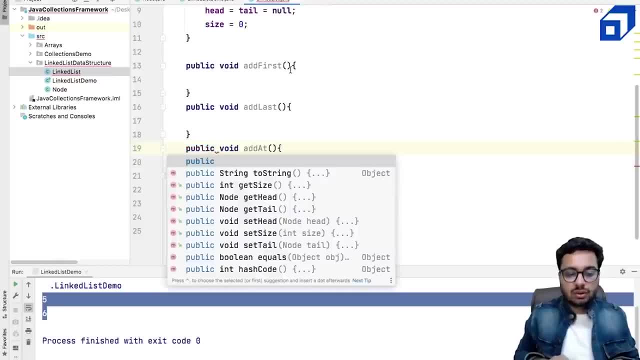 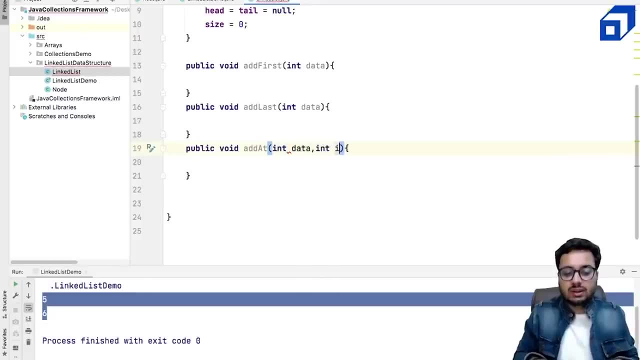 In all the three methods, I should know what is the data that I need to add, And in the third method, I should also know at what index I need to add. Now take a pause and think how you will implement these methods. Okay. 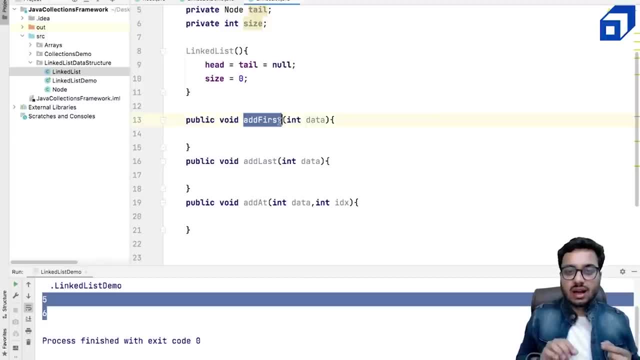 If you're given a linked list and you want to add something at the beginning of the linked list, how you would add in: Okay, So what will be the code behind this method? Take a pause and think about it, Okay. So let us discuss the first method. 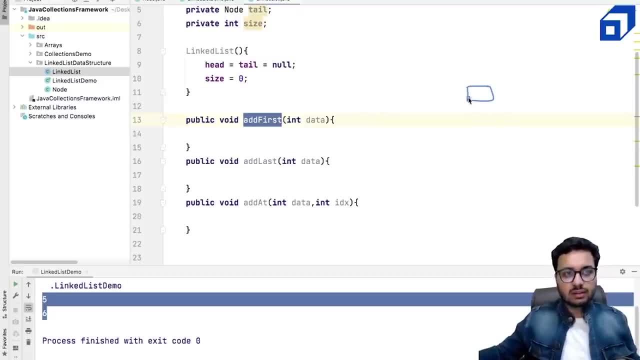 Add first. Now suppose you have a linked list, right? Let's say this is a, this is B, this is C, This is already there and head is referring to this node. I want to say, okay, I want to add another, node D, which is at the beginning of the linked. 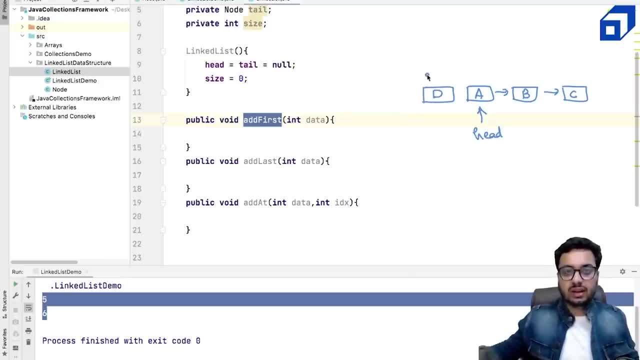 list right How I will do it. The first thing is I need to create this node. So how do I create a node object? Very easy, I simply say: let me create a node called as N. This is equal to new node. 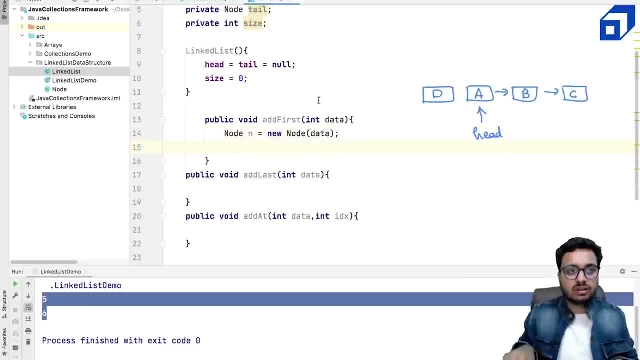 And the data of this node is same as this data that I've given. So this creates a new node and N is referring to this node. right, N is an object reference, local reference created inside this function, which is referring to this particular node. 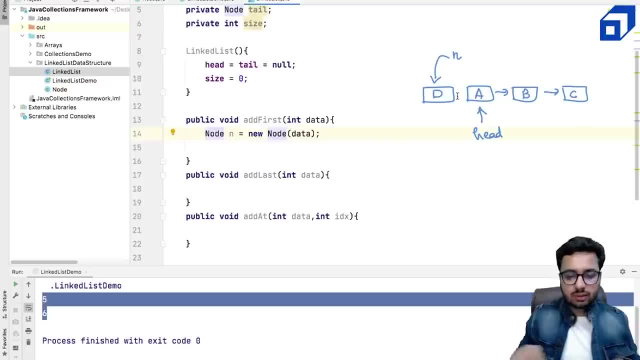 What should I do? How do I connect this? I would say, okay, N dot next should refer to the head. So if head is already there, N dot next should connect to head. So it makes this connection right. One thing I need to do is I need to say, okay, this head, it should move here. right, 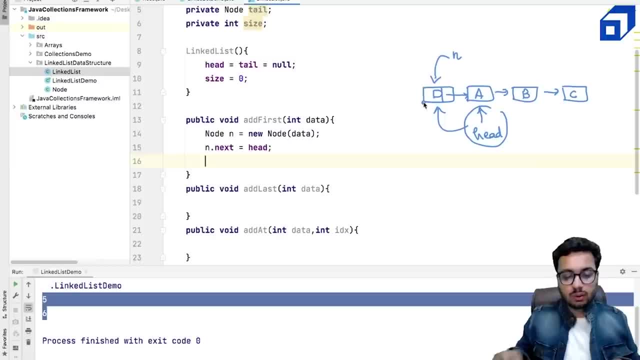 This head should not refer to A. instead, this head should refer to, now, D. I can say head is equal to N. This will work really well. And one more thing I will do is size++. Every insertion will increment the size of the link. 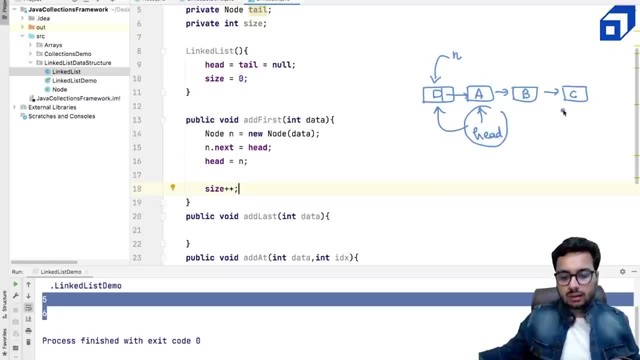 So this will work really well if the link list is already there, right? But suppose you are creating the link list for the first time and you call the add first method. So head and tail, both were null, right, And you said: okay, I want to create a new node. 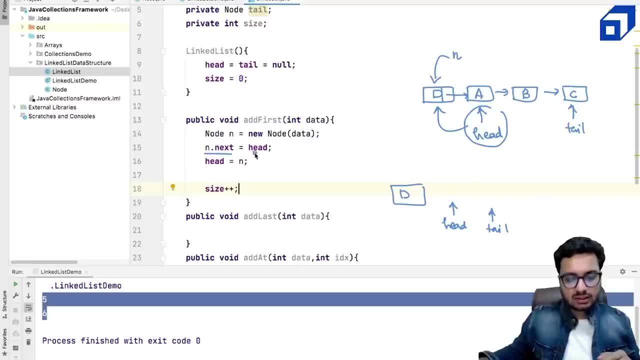 So you created a new node called D and N. dot next is equal to head, So head was null. So D is next is also null, which is fine, right. And then you say head is equal to N. This head refers to this node, which is also fine, right. 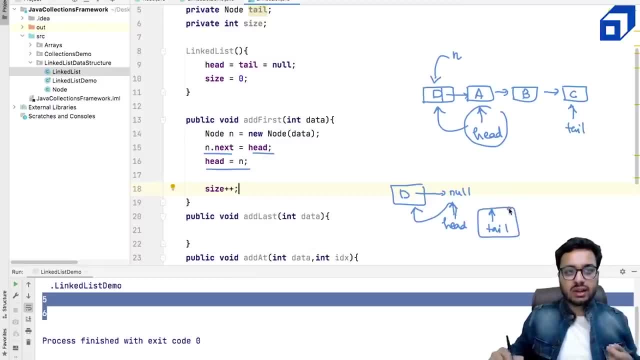 But the thing is, the tail is not getting updated right Whenever the first node is inserted, right. Let's say the first node is A, both head and tail should refer to this node. right, What I can do, I need to add a separate condition that if. what if the size was zero before? 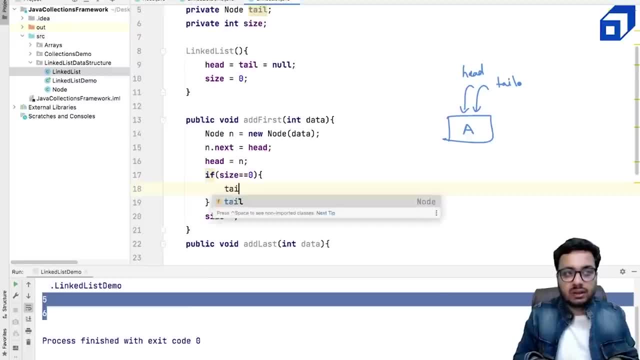 adding this node. in that case, my tail will also get updated. So tail should also point to head, or tail should also refer to N, right? This is a special case when you have zero nodes. In that case, you also need to update the tail, right? 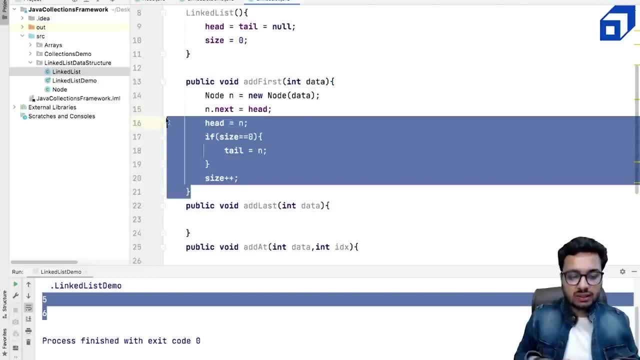 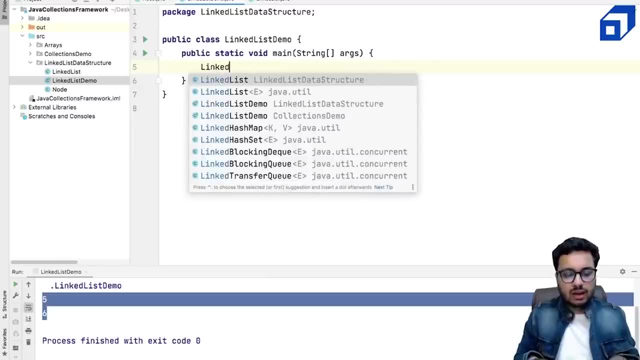 This is my add first method. Let us test the functionality of add first method. So what I will do? I will go in link list demo. It's okay. I want to create a link list L. this is equal to new link list. 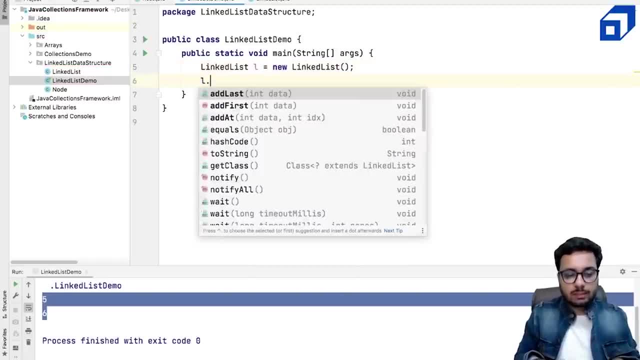 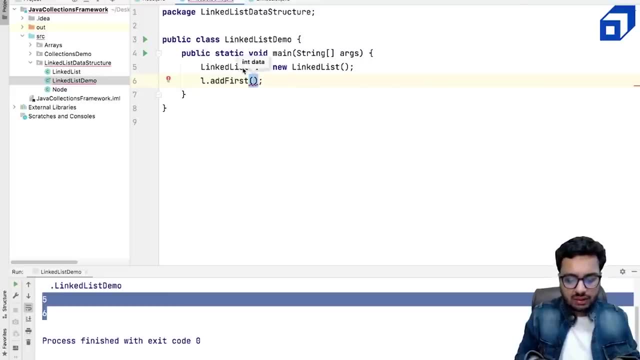 And now in this I can say: okay, End L dot add first, And I will give some data, let's say 10. And say L dot add first, I will add 20.. And then L dot add first, I will add 30, right. 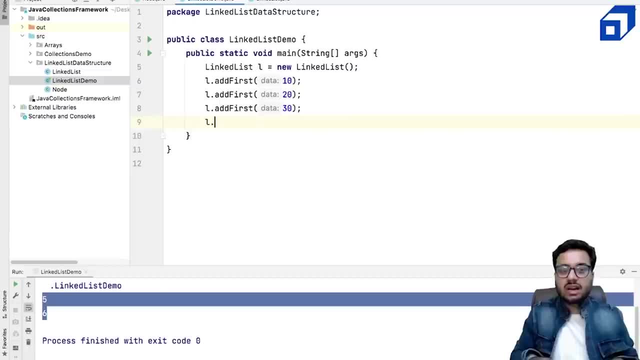 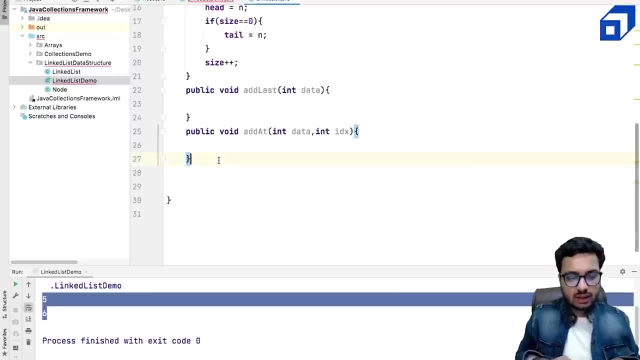 So I want to see this link list, So I will call the display method, which I have not implemented, So I will. we will implement the display method as well. right, Let us go back into the link list class And let us add one more method. 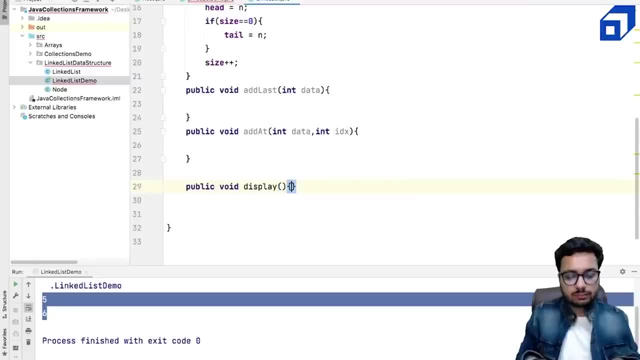 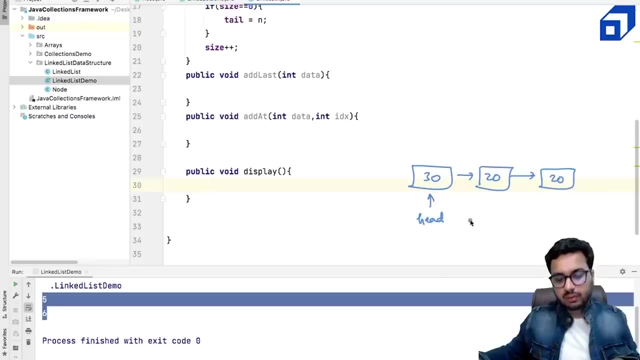 Click void- display right. So how do I display the link list? Now it's going to be pretty easy. Suppose the link list is 30,, followed by 20,, followed by 10, right, And head is referring to this node, okay. 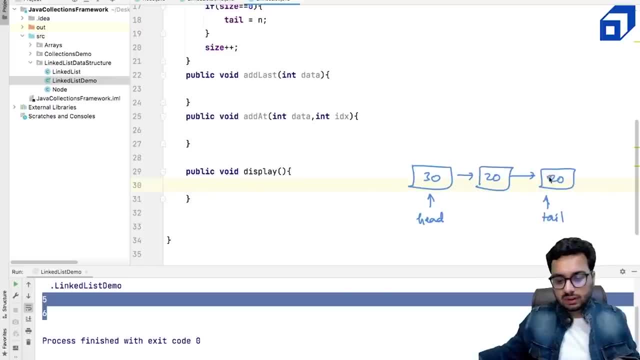 Tail is referring to this node. This is 10, right. So tail is referring to this node. So what I need to do, I need to start iterating from head till the end. So it's okay, I will take a temp variable. 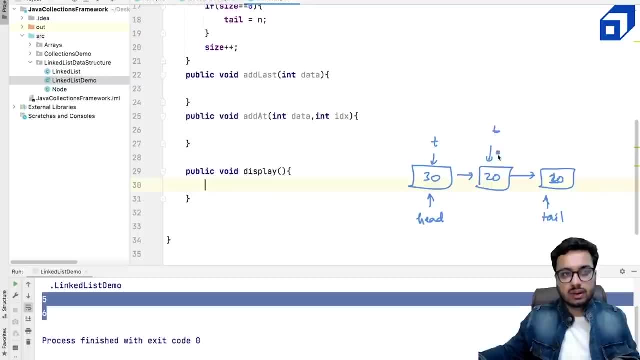 I will print it And I will take temp here. I will print it. I will take temp here. I will print it. I will take temp here, right? So what is happening? So, once my temp reaches null, I will stop. 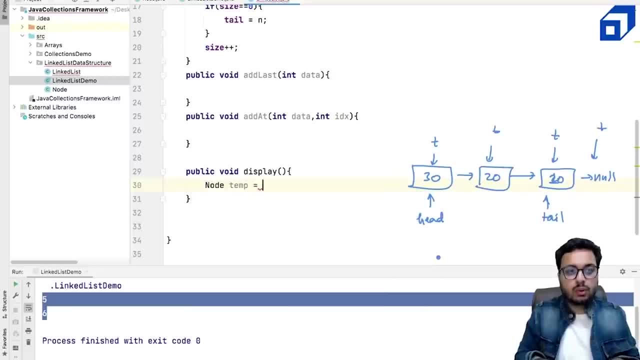 So what I can do? I can say: node temp. this is equal to null. So temp is again a reference, It's not a node, right? So sorry, it's equal to head, It starts from head, And while this temp is not equal to null, what do I do? 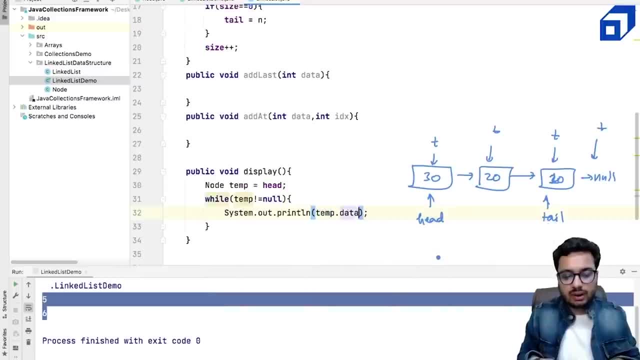 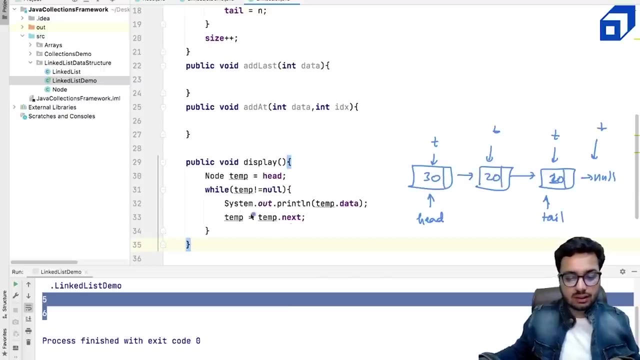 I print the node, So I say sout tempdata and take this temp to the next node. Temp equals to tempnext. Temp goes to the next node. This while loop will help me to iterate on the entire link list. right, So temp starts from head. 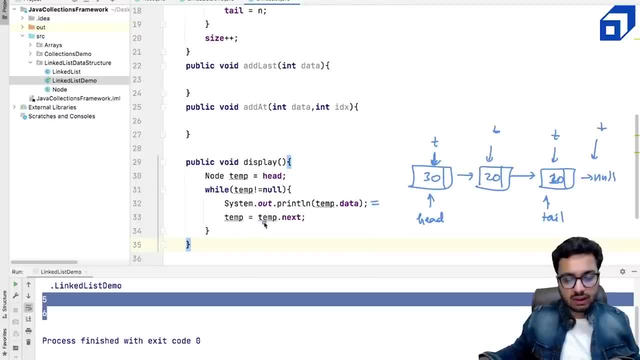 Temp is referring to this node. I print out 30. Temp equal to tempnext. So tempnext means this value. So this value means this node. So temp goes here Again. tempnext means this value, which is this node. 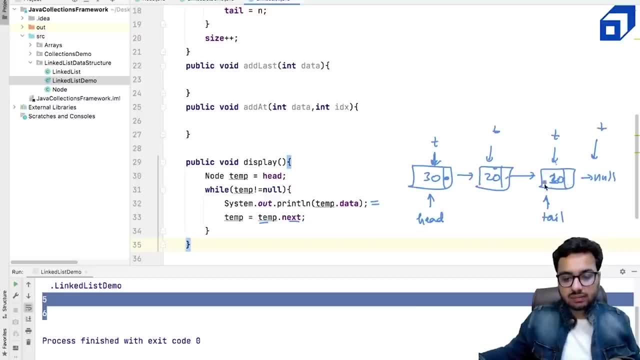 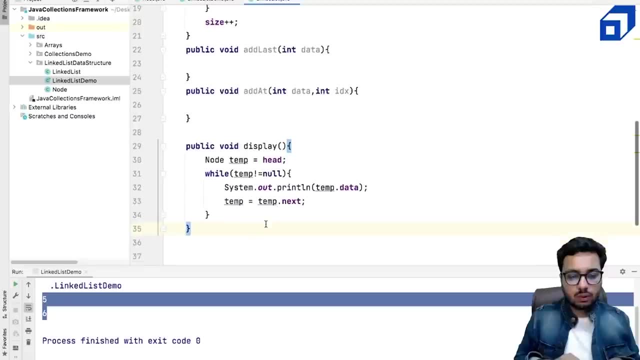 Temp goes here. Again, this is not null, This node is not null. So I say tempnext, which is this value, which is null. So temp actually becomes null And my loop stops right Now. the display method is there. 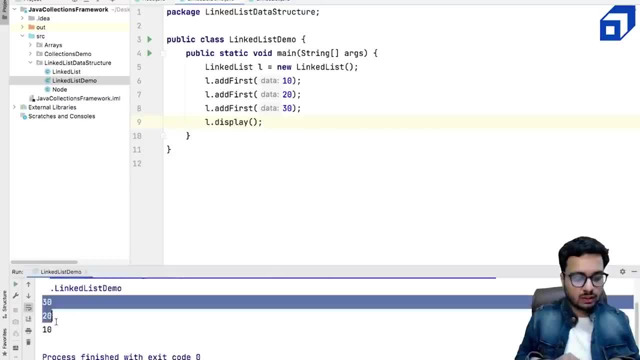 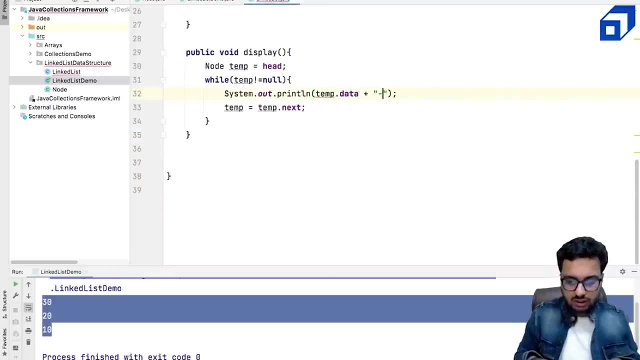 And we can run this code. Okay, so I see 30,, 20, and 10,, which is okay. That means my link list is getting created. But to show you in a linear fashion what I can do, I can put an arrow here. 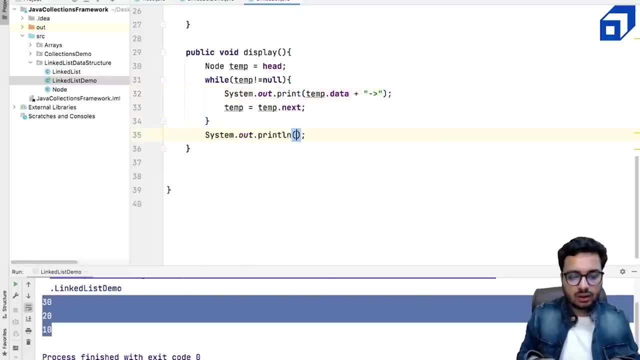 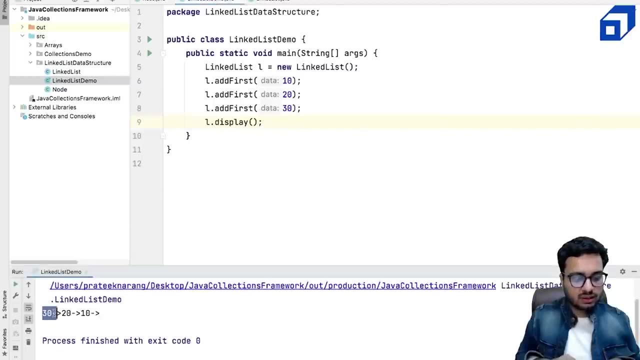 And I can put a new line here. right, This will make the representation look little better. right, I'm getting 30,, 20,, 10.. If you look carefully, I added 10 in the beginning, So 10 got added. 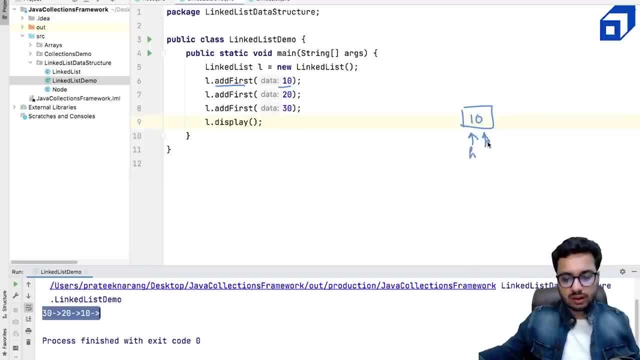 That means my head and tail. both were here. right Then I added 20, in which 20 got added here And my head moved here right Then 30 got added. A new node was created. It got connected here. 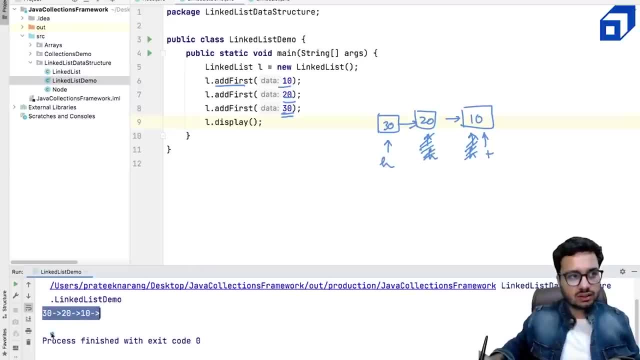 And then my head moved here right. This is how the link list is going to look like: 30,, 20, and 10.. I hope you are able to understand the addFirst method right Now, on the similar lines, what we will do. 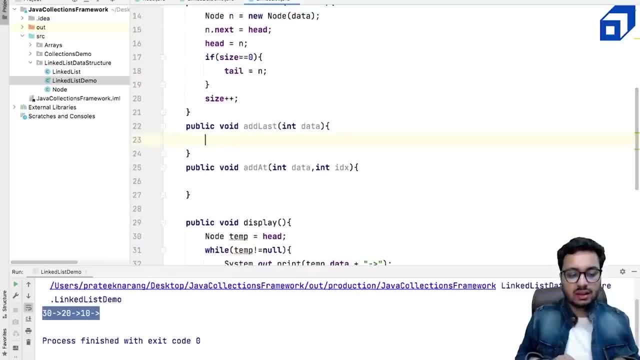 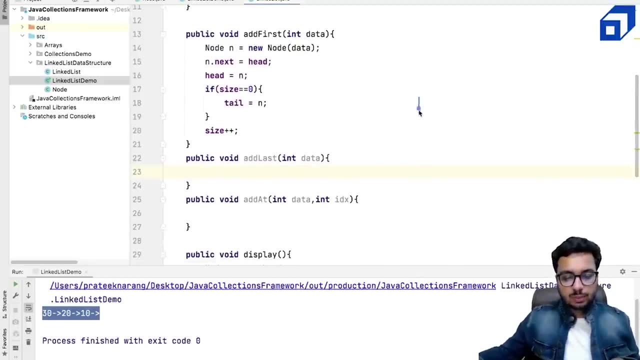 We will implement the method called as addLast. Now take a pause and think how you will implement the addLast method. Alright, let us see right Now. suppose you already have a link: list A, B, C, right, And I want to add a new node D, which is at the end of the list. 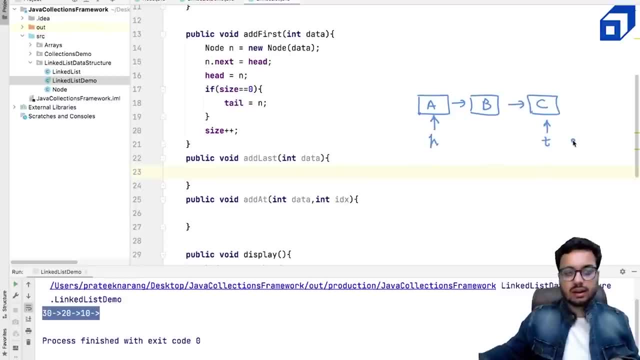 So this is my head And this is my tail, right. So how do I add a new node here? First of all, I need to create this new node. So how do I do it? I can say, okay, fine. 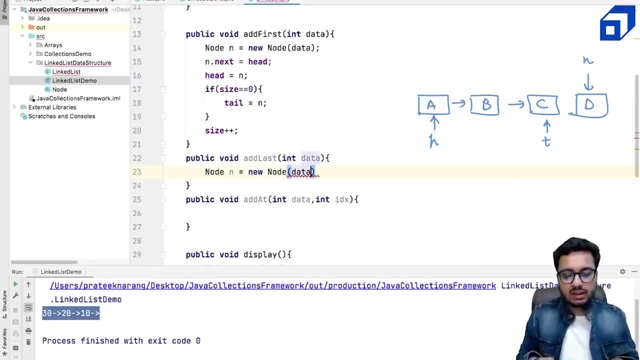 NodeN. this is equal to newNode And I give the data to this node that I'm getting right Now. how do I connect this tail node with the new node? That connection is pretty easy. So what I need to do, I need to update this value and give it the reference of this node. 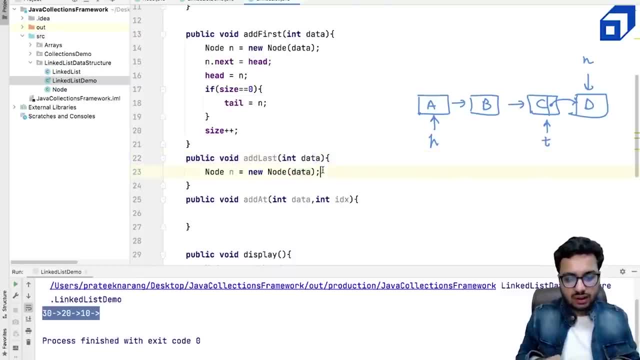 which is stored in N, right. So I need to say that: fine, tailnext, this is equal to the new node that we have created, right. So this makes the connection, And I also need to say, okay, this tail should be here. 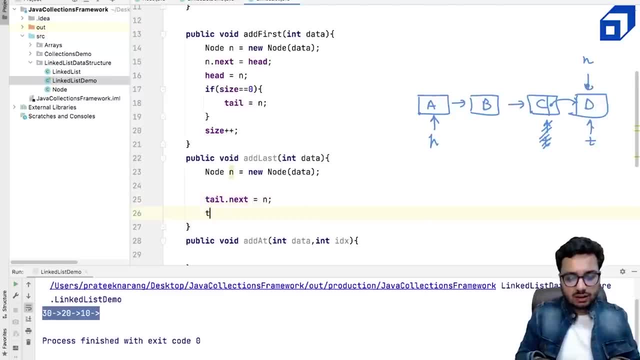 Because this node is now the new tail, So I can say tail equal to tailnext, Or you can say tail equal to N, Both are fine. right Now this tail has also moved, And one more thing we will do is we will just size++. 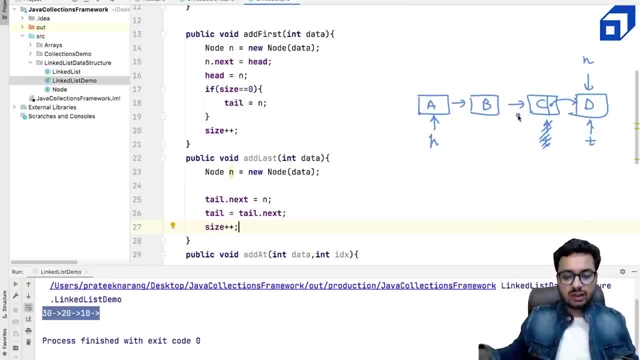 Now, this will work fine when the linked list is already there, right, But think of a case when your linked list is not created. That means both head and tail they were null And you inserted the first node by calling the addLast function. 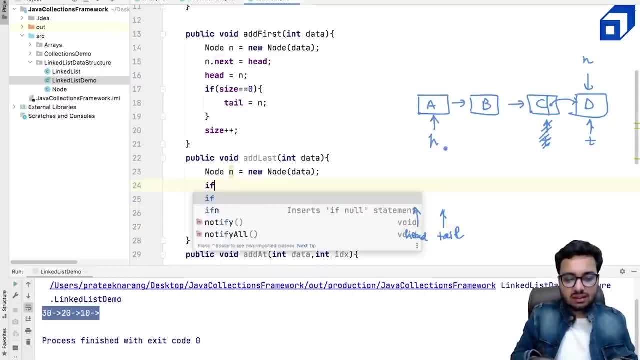 You say: okay, I don't have a linked list. That means if the size is 0, and you are adding the first node in the linked list, then how should the update should happen, right. So you still created this new node, N, right? 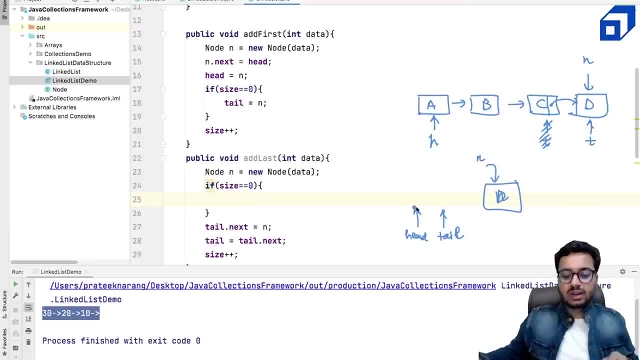 With the data D, N is referring to this node. So in this case, both head and tail should get updated. They should point to this node, right? What I can do, I can say: okay, head and tail, they will refer to N, right? 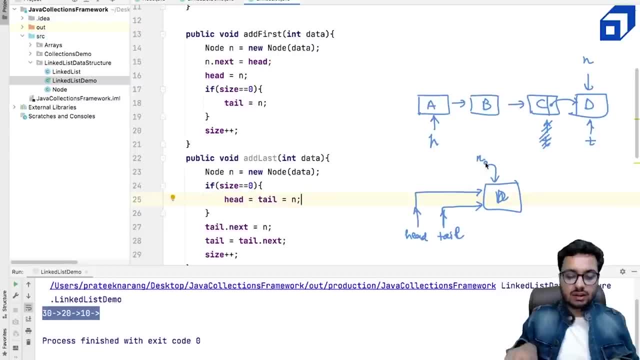 They will also store the address that is stored in N. right Now you might ask: okay, what happens to this N? So N is a local variable. It will get destroyed after this function call is over. But head and tail, they are the data members of the class. 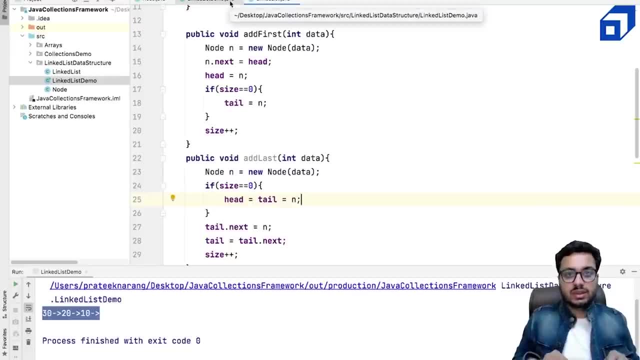 They will exist till you have the linked list object in your memory, right, So they are not going to get destroyed, right. So N is a local variable, It will be over right And anything that is allocated using new will not get destroyed. 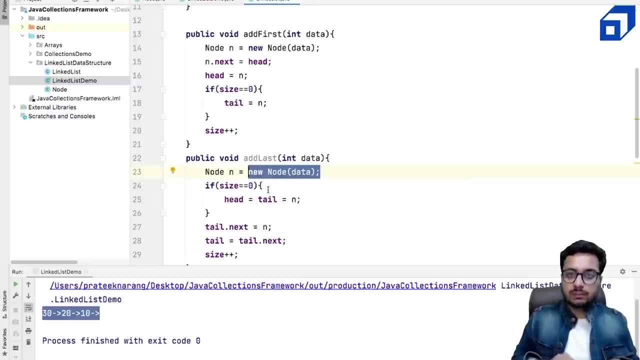 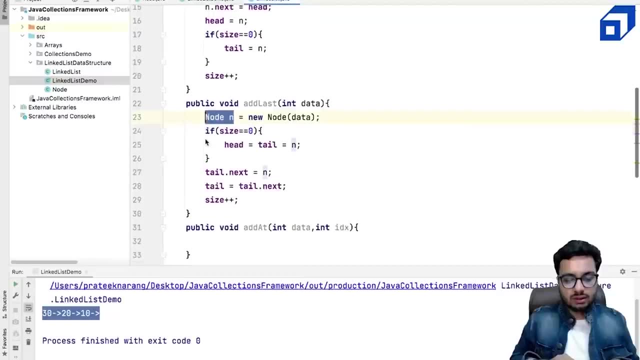 Why? Because if someone is referring to this memory, that memory will not be garbage collected, right. So head and tail, they are referring to this. node N is a local variable. It will get destroyed, right. So this way, add last will work. 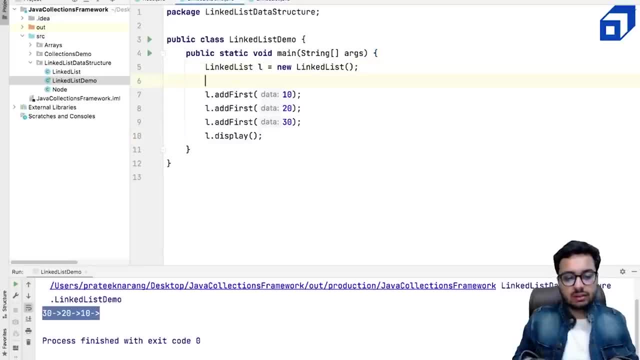 So now let us test our functionality right. So I say okay, L dot add last, Maybe this is 40 this time. And again I say okay, L dot add last, This is 50,. right Now, if you look carefully. 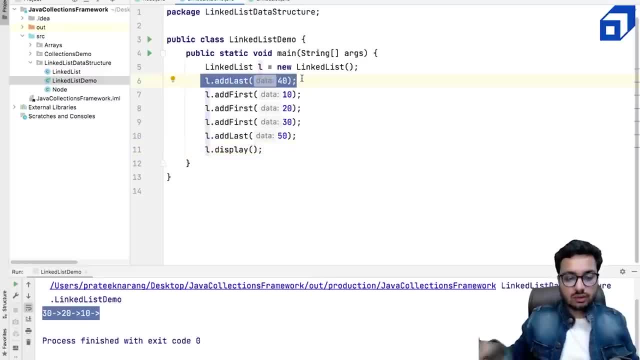 I'm adding the first node by calling add last function. First 40 was added, Add first 10.. So 10 was added, Then 20 was added, Then 30 was added. Now again I'm calling the add first method on a linked list. 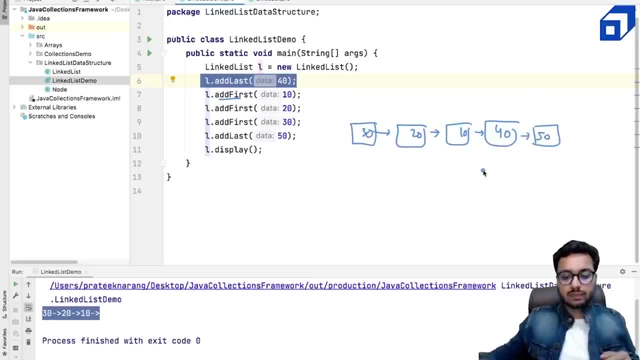 which is already built. So 50 should get added right. So if I say L dot display right, It will give me this linked list. Let us see the output. We are getting this linked list: 30, 20,, 10,, 40,, 50.. 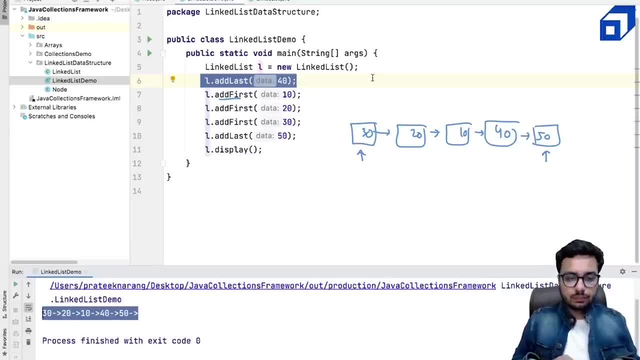 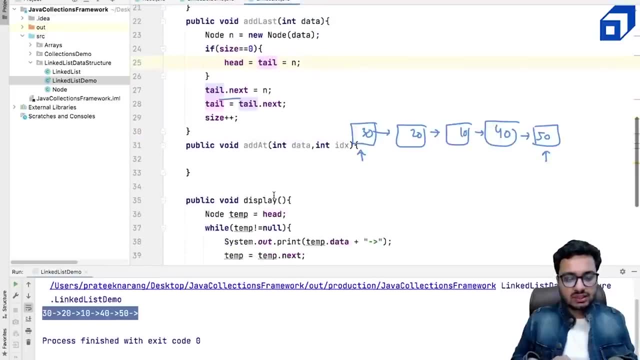 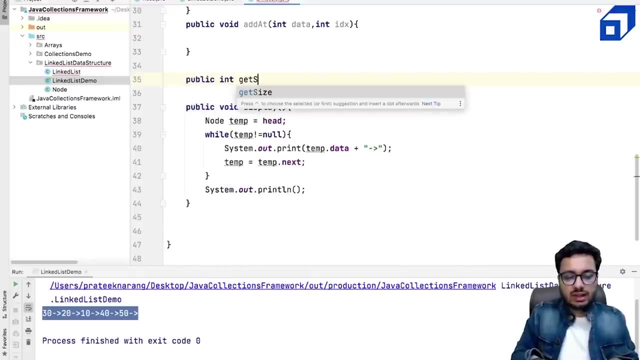 That means this is working really fine, right? Okay, Let us go back here and let us implement one more method. That is okay. Give me the size right. How many nodes we have? That's going to be easy. Public int get size. 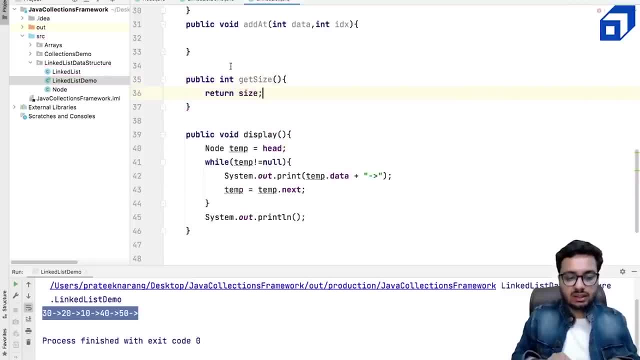 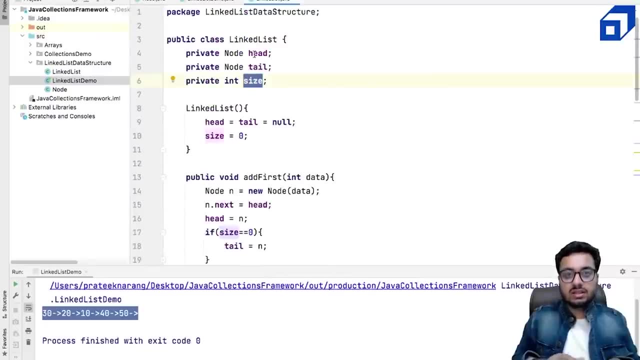 And what we are going to do. we are going to return the size of the linked list. right, We are doing it this way because if you make this size public, anyone can change it. right, I'm only giving the getter to access the size. 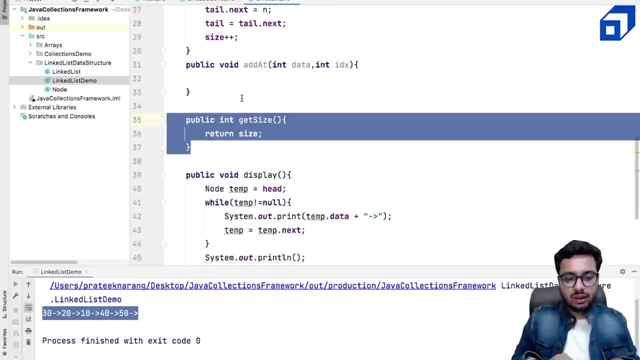 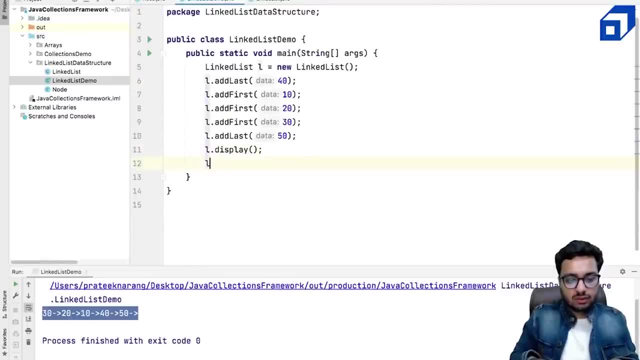 I'm not giving any method to set the size of the linked list. Okay, So that size should be updated only through the add and the remove methods. So this is also fine. So I can say L dot, get size, And I want to display how many nodes I have in this linked list. 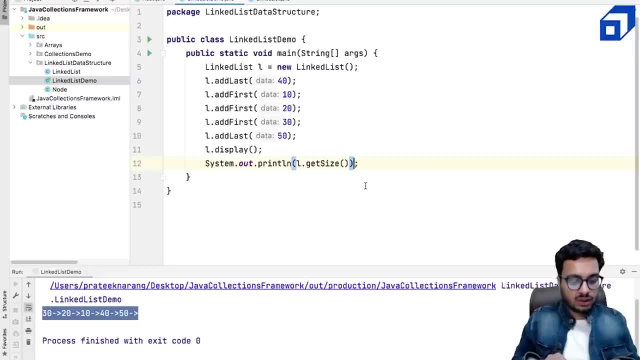 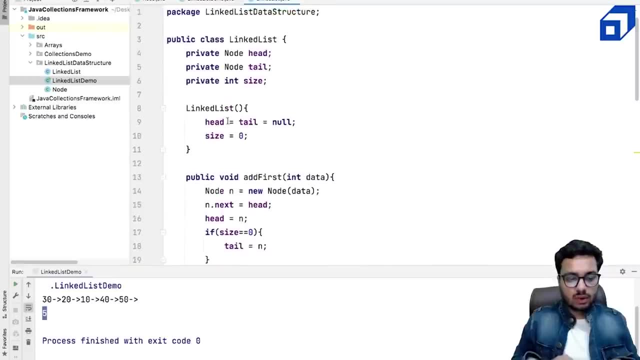 This is again a order one operation. right, I can say: okay, there are five nodes, Let us talk a little bit about the complexity. So your constructor is doing order one work At first. it is also doing order one work. 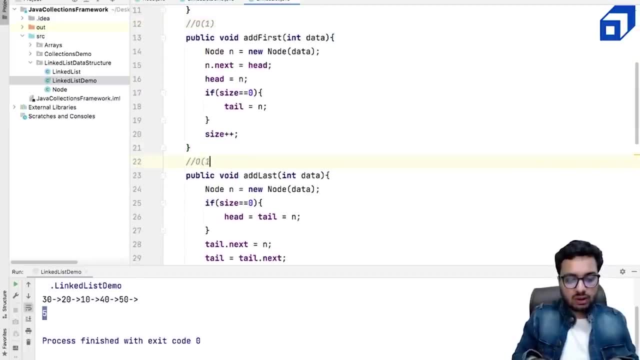 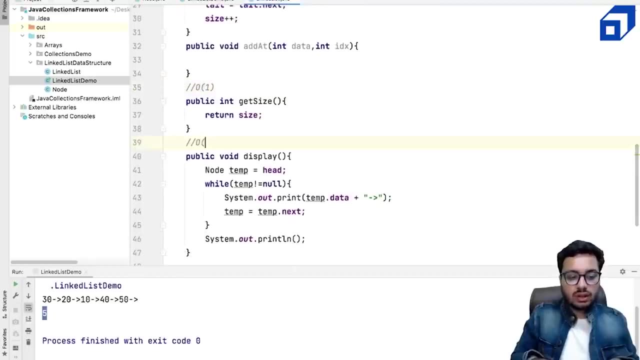 No loops involved Here also. we are doing order one work- Get size. we are doing order one work- Display. we are iterating over all the end nodes. We are doing order of end work right Now. the next method is add- add right. 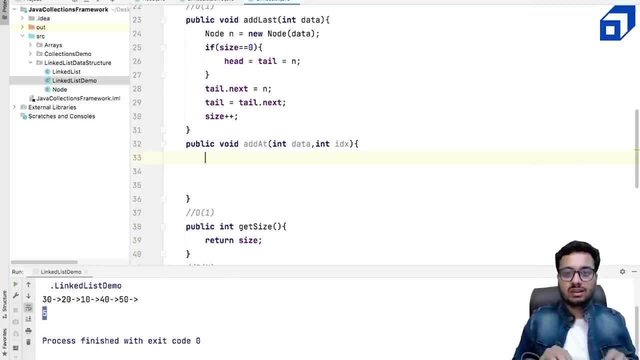 So take a pause and think how you will implement add add method. And if you want to insert something in the middle of a linked list at a particular index, okay, So let us see it next. So we are discussing how do we implement the add add method, okay, 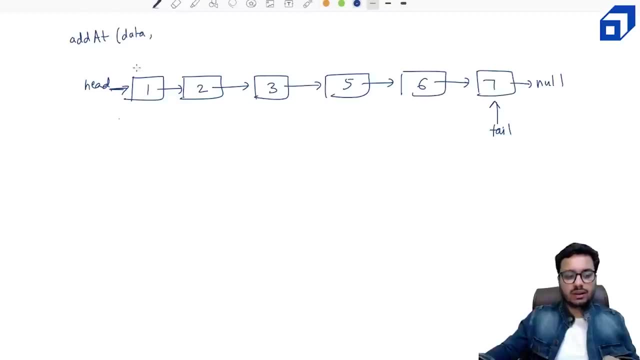 So we are given: okay, this is the data that you need to add And you have a particular index at which you want to do this insertion right Now, suppose my data is four And my index is three. That means okay, zeroth index, first index, second index. 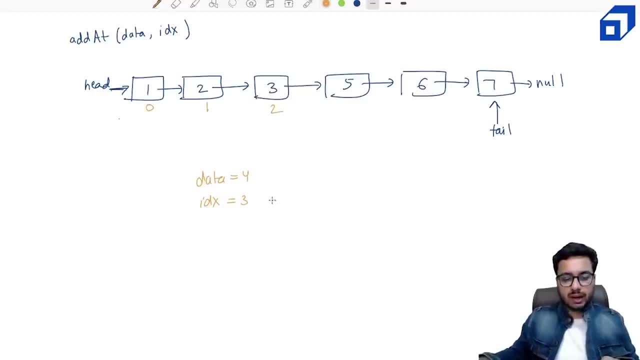 Here I want to add Third index. the new node should come right. Or you can say: okay, after three nodes I want to insert the fourth node. So this is my fourth node that I want to insert somewhere here, right? 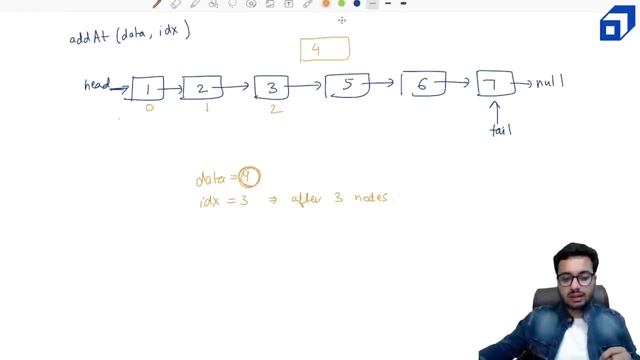 So how I will do it right. So one way is okay: I will create a new node, And n is referring to this node, four, right? But how do I connect three with four and four with five, right? So this is going to be easy. 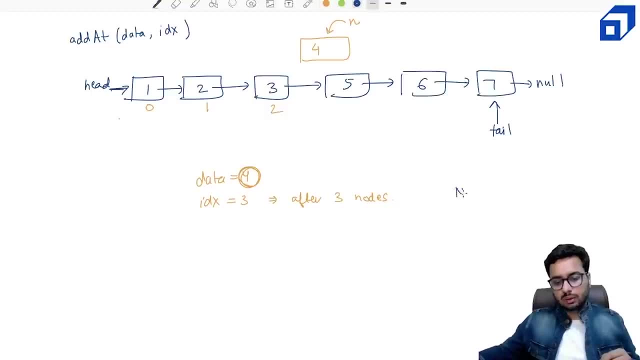 How You can say: okay, let me create this new node n. So node n this is equal to new node with my data four. right Now one way is okay. I can say: I need to reach this node right. 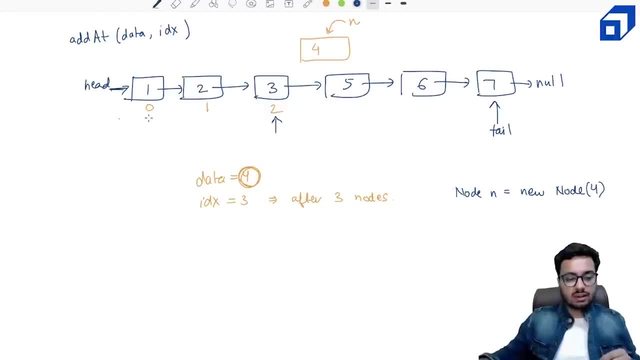 How do I reach this node? That means if I start from this node and I want to reach the third node right After three nodes, I have to insert. That means I have to reach the third node. If I take one jump here, I reach two. 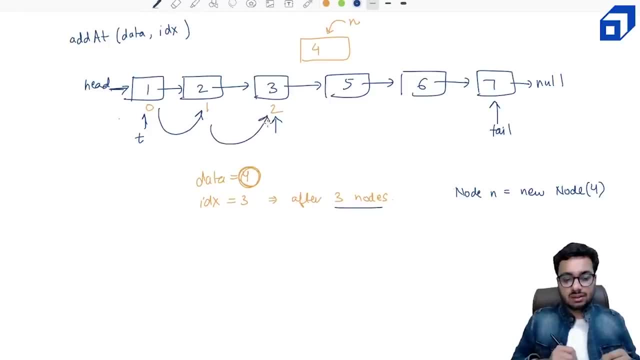 If I take one more jump here, I will reach this node right? That means, in order to reach three, I need to take two jumps, right? Okay, So if my index is some p right, I need to take p minus one jumps, right. 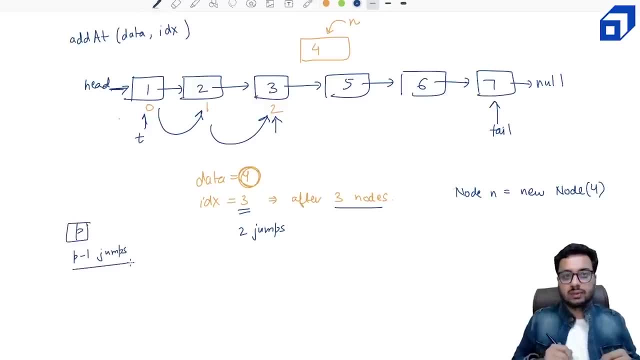 For a particular position, p, I need to take p minus one jumps. This we will do it using a loop right? Let's say I've reached this node and I'm holding this address in a variable called temp right. Now how I will do it right. 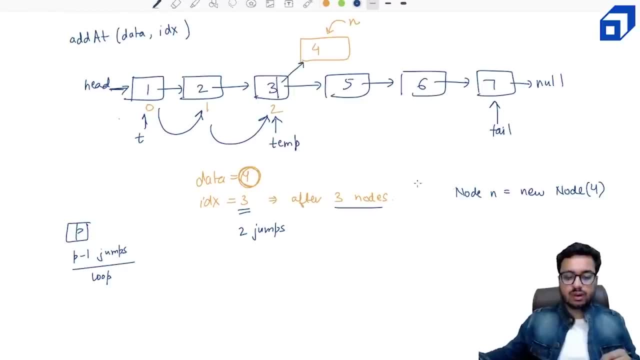 I can say okay, temps next should point to four. If I do this, temp dot next should refer to n. What loss I will have? I will lose the address of five. I don't want to do that right. How should I do it? 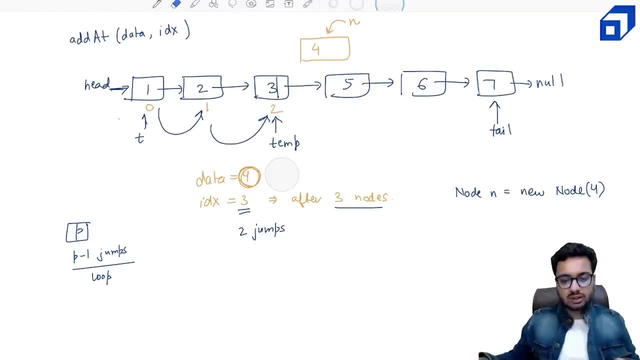 I will say that, before doing this operation, let me say that four should store the address of five. Can I do that? Of course, yes. How do I do that? I can say n dot next. That is the next of four. 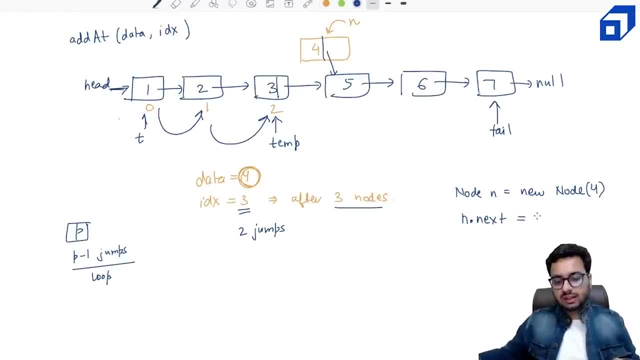 Should refer to five. So what is the address of five? It is nothing, but it is the next of temp. It is temp dot next, right. Once it is done, can I update the address? the next of three, Of course, yes. 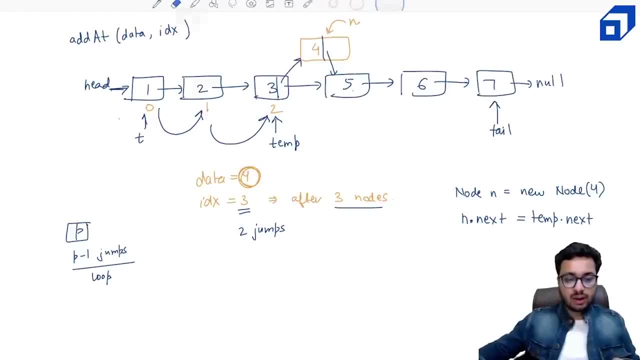 I can say: okay, three is next. Now it should point to four and this link will automatically get broken. So I can say: three is my temp. Temp dot next should be equal to n. In just these three steps I will be able to insert n. 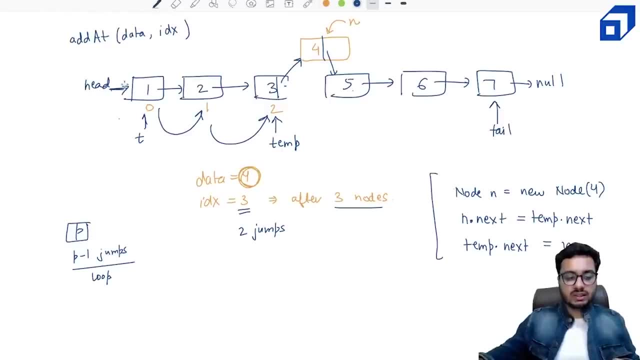 I will be able to insert a node in the middle right Now. we might have a special case where we might need to insert a node in the beginning or at the end, or we are getting an index which is out of bounds. Let us see how we will handle those cases. 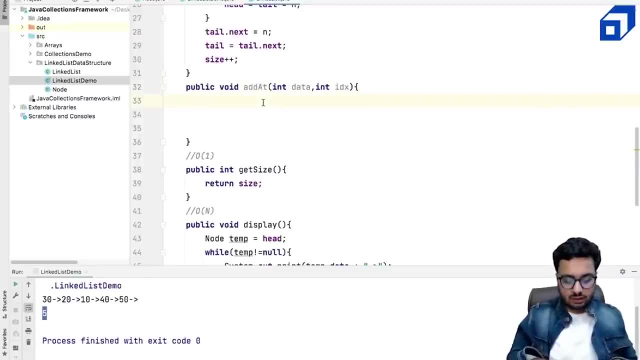 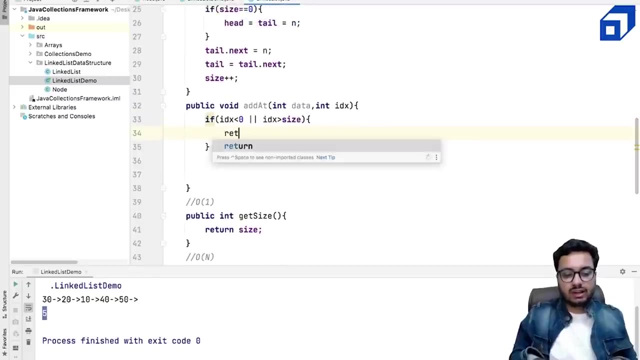 So first of all, I'm going to check if this index is out of bounds, right? So if my index is less than zero or my index is greater than the size of the linked list, that means I cannot insert this node. So in this case, what we can do is either we simply return right. 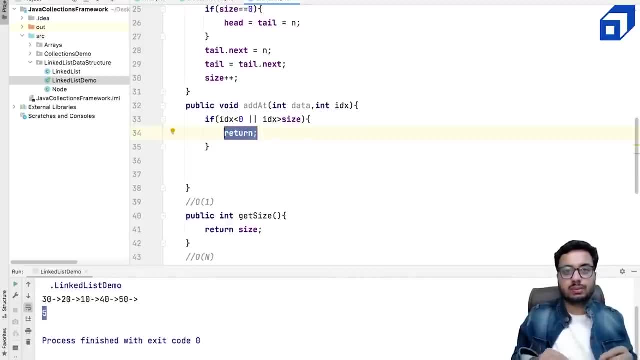 But that's not a good idea. We should tell the user that you are doing something wrong, right. One way to do it is we can throw a new exception and we can say: okay, index out of bounds that you're using the incorrect index. 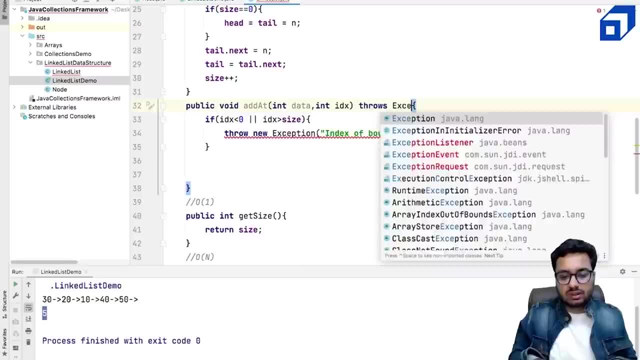 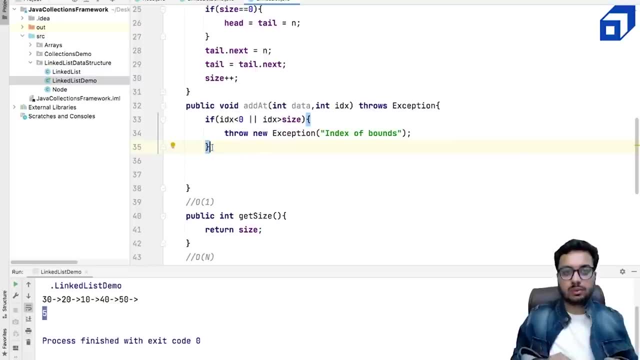 And here I have to say, okay, this method throws an exception. right, I can throw an exception in this case, and an error will come in the middle, In the main, when this program is executed, right. And now, if my index is zero, that becomes a special case. 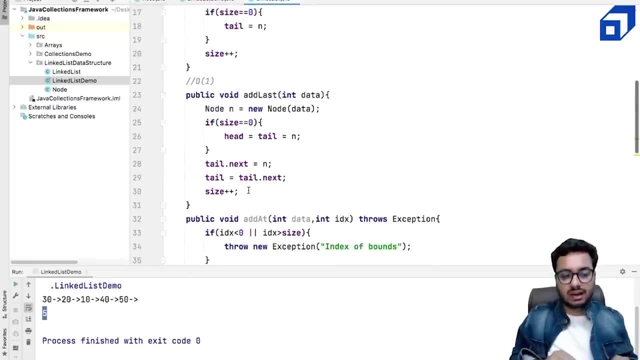 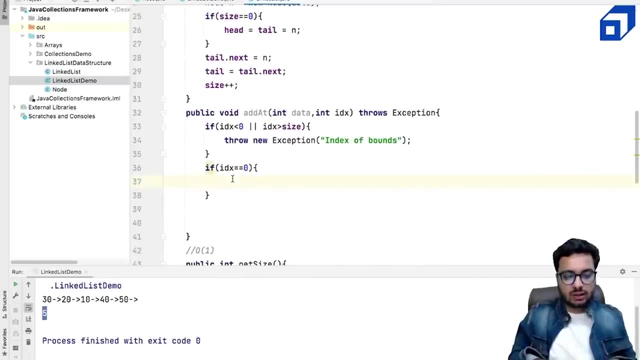 That means: okay, I'm trying to add something at the beginning that I have already handled. We can just call the add first method with the data, right? So I can say you call the add first and you give the data. That's it. 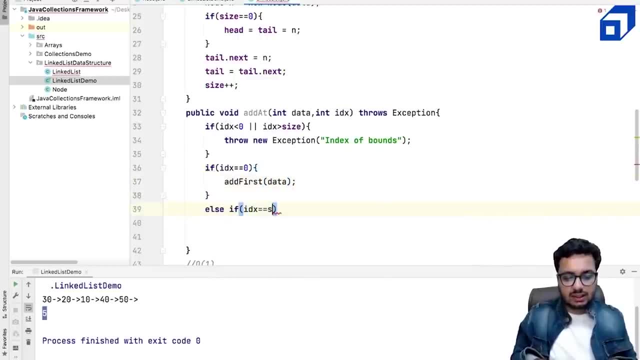 Else, if your index is equal to size, that means if the linked list has Three nodes and you want to insert something at index three, that means you're inserting something here, right, Which is again at the ending of the linked list. In that case you can call the method at last and you can give the data right. 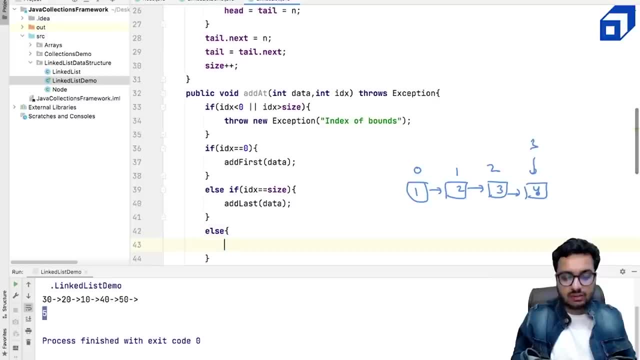 In the else block we have to write the exact logic that we are talking about, right? So let's see how we will do it. Suppose your linked list is like this: One, two, three right, And I have five, six, seven, right. 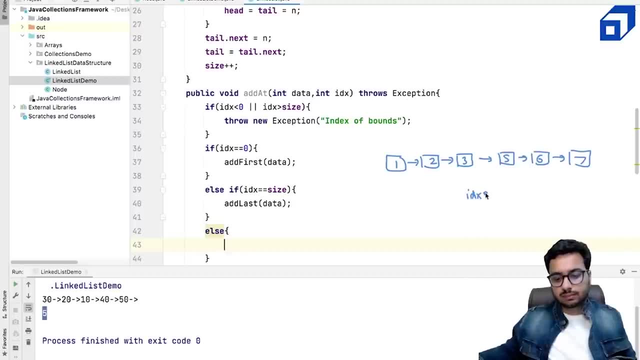 So I'm telling you that, okay, after three nodes you have to insert a data that is four, right? So how do I do it? First, I need to reach the third node, right? So I need to take a temp and reach this node. 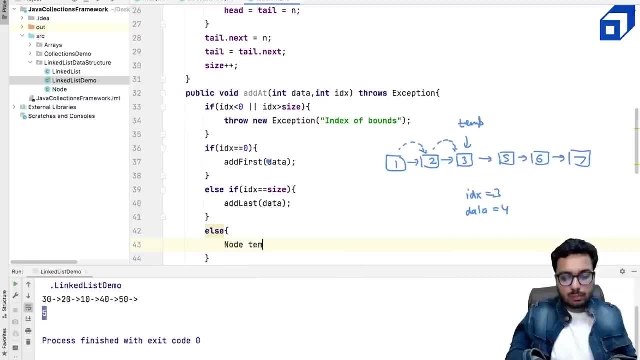 So temp will start from head. So I can say node temp, this is equal to head. How many jumps I have to take? I have to take index minus one jumps. So I can say okay, for int jump equal to one. 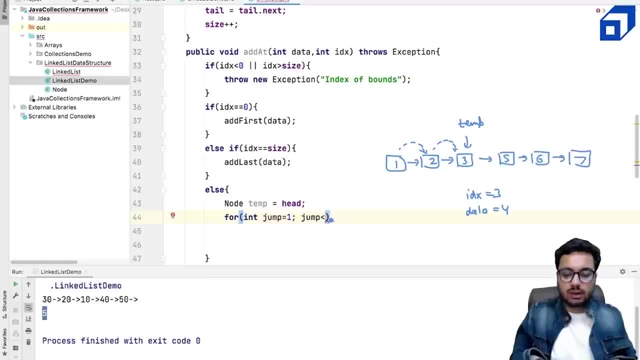 Jump less than equal to index right. Jump plus plus right. Or, if it is sounding confusing to you, you can say: less than equal to index minus one right. These many jumps, as I told you, we have to take right. 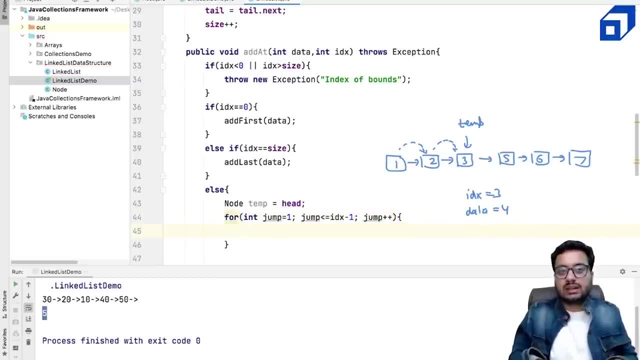 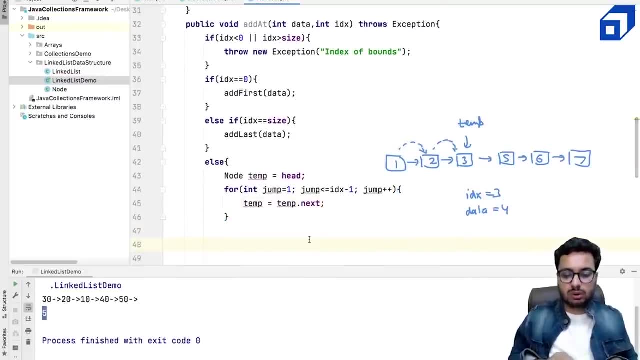 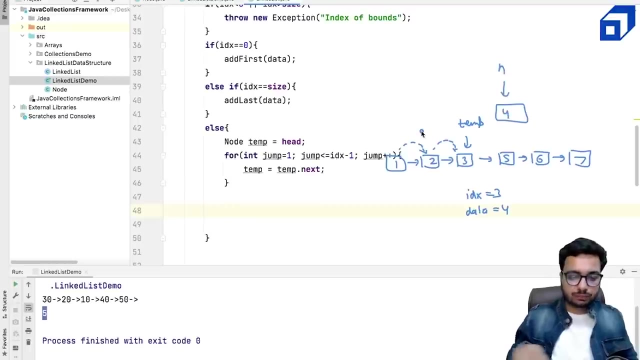 In each jump what we should do. temp will take a step, So temp will go to the next node, Temp equal to temp. dot next. Now I'm in a good position to do some insertion here, right? What I will do is: okay, let me create a new node n, whose data is four. 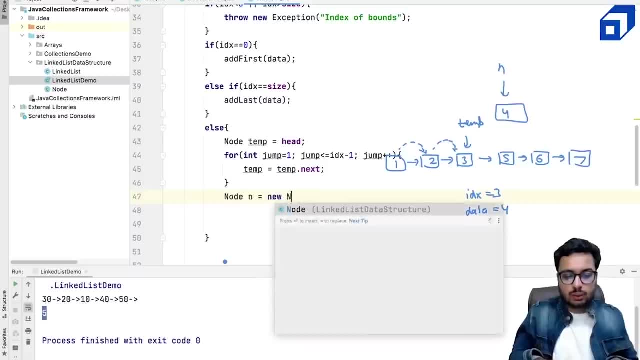 I can say node n. this is equal to new node with the given data. And n dot next should refer to temp dot next, as we have just discussed here as well. right, So four should get connected with five. That is the first step. 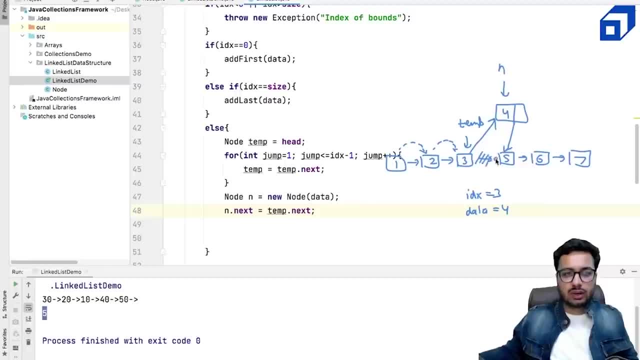 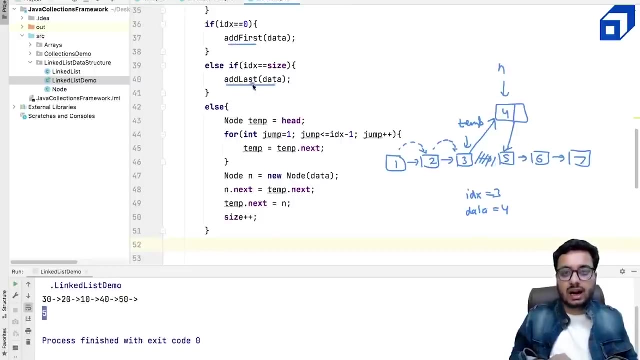 Then I need to connect three with four, right? So how do I do it? So three is my temp dot. next should point to four. So four is n, That's it. And size plus plus Size we will update here. So here we are not doing size plus plus because at first and at last will automatically increment the size, right? 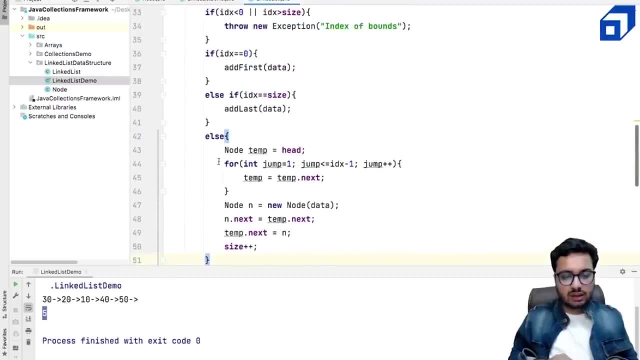 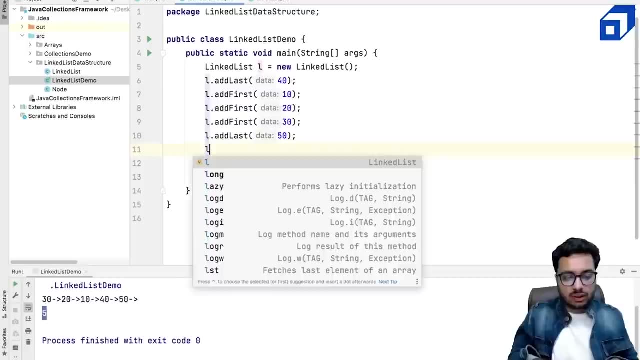 That's it. So that is my insertion in the middle. Now let us run this code in main and see if it works really well or not. right Now I can say: okay, this was my original linked list. L dot add at index. 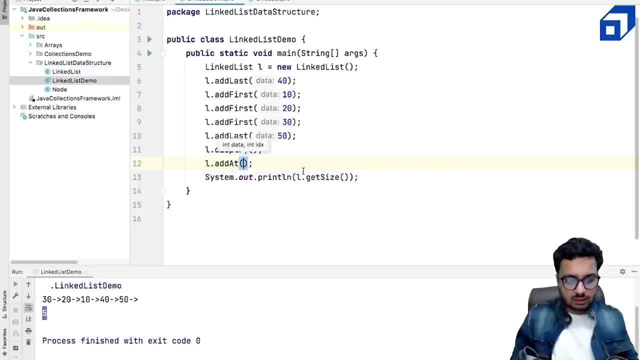 Let's say I want to add at some index zero. Let's say the data is zero. right, L dot add at index. I want to add something at the last index, So L dot get size. Okay, Now I'm getting a getting not add last, but I can say add at. 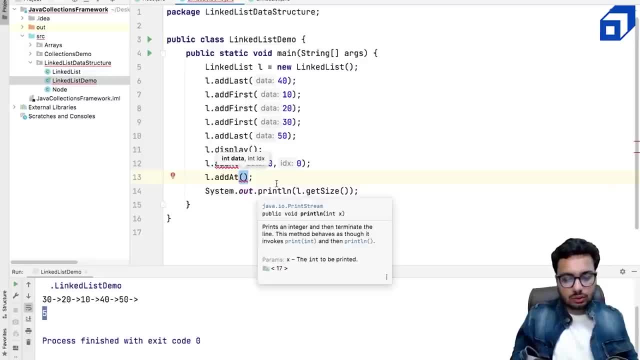 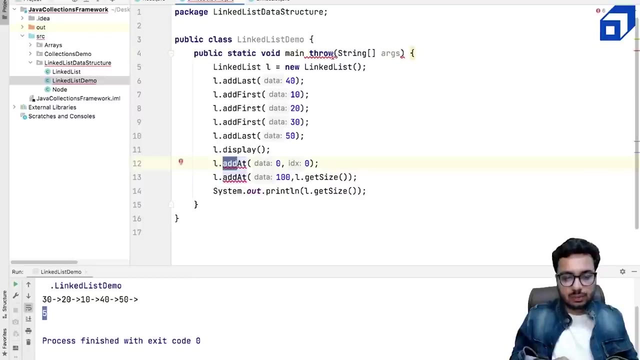 So index will be, let's say, the last index. So data is, let's say, 100.. L dot get size. Now again here- I'm getting this because I'm not written- throws exception. So main can also throw an exception because it is calling a method that throws exception. 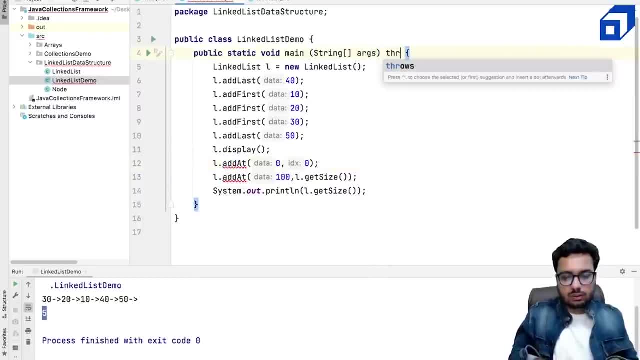 So main can also throw exception right. So we have to write this here, right, And let's add something in the middle as well. So L dot display And I also okay, L dot add at index four. Sorry, data is four. 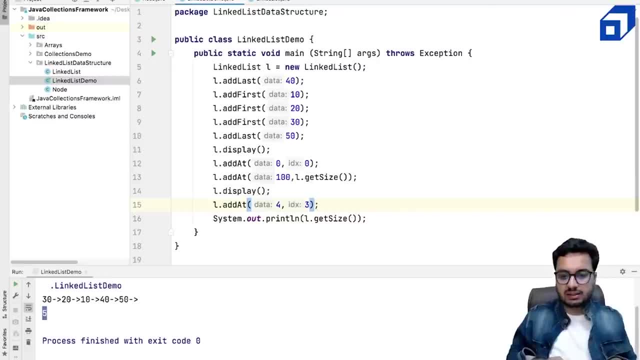 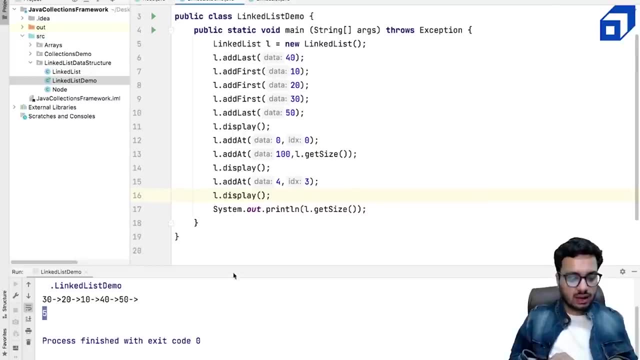 At some index. let's say three, something like this, And again let me say L dot display. So this will test over all the three cases and we should be seeing that they should work fine, right? So in the first case I added zero in the beginning. 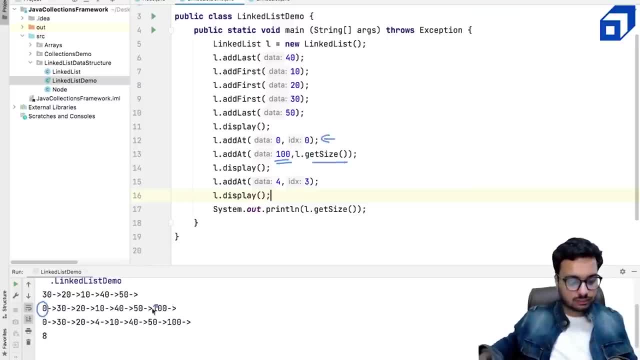 Fine, I added hundred at the end. Fine Working fine. Then in this linked list I said: okay, at index three, I should insert four, So zero, 30,, 20.. This is the third index before 10, I will insert a four. 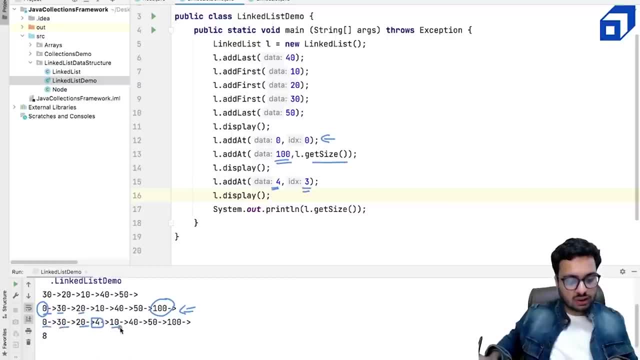 So zero, 30,, 20,- I'm getting a four here- Then 10,, 40,, 50 and a hundred. That means in the middle it is also working fine And I display this list right. And finally I have eight elements. 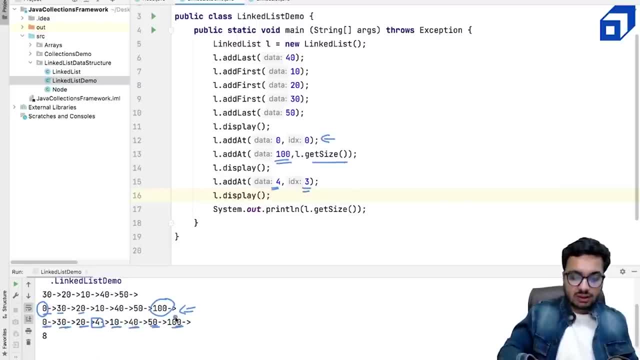 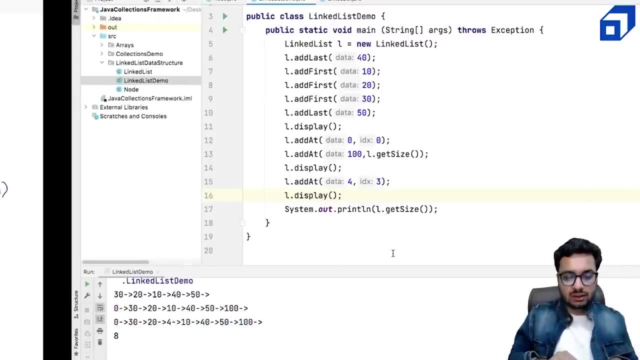 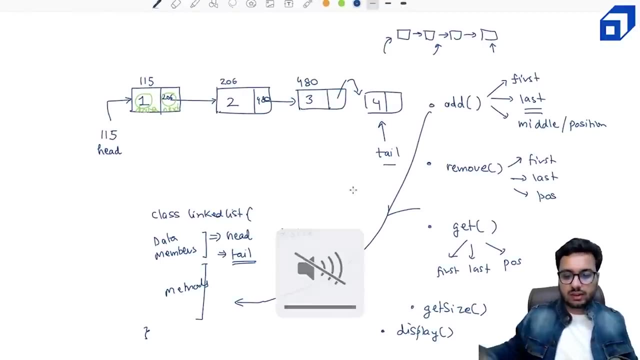 One, two, three, four, five, six, seven, eight. That means that size update is also working fine in all the three cases right? So that completes part one. That means we are able to add nodes In the linked list in all the three cases. we have seen at first. we have seen at last. 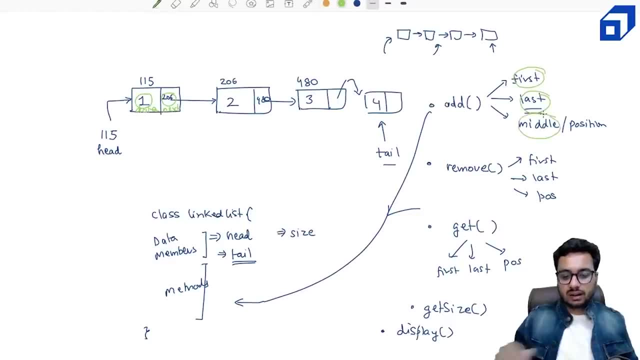 and we have seen art in the middle right. Next we will move on to get, And after that we will move on to remove. So take a pause and think how you can implement these methods: Get first, get last and get an element at a particular position. 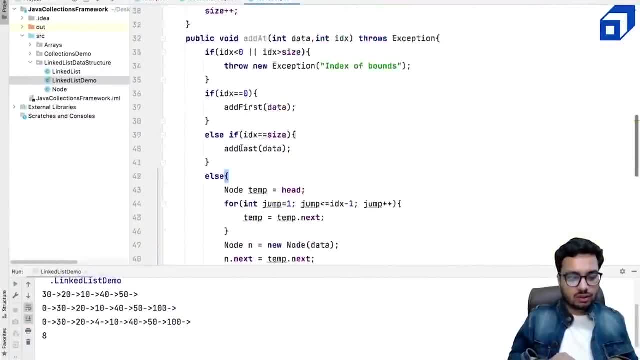 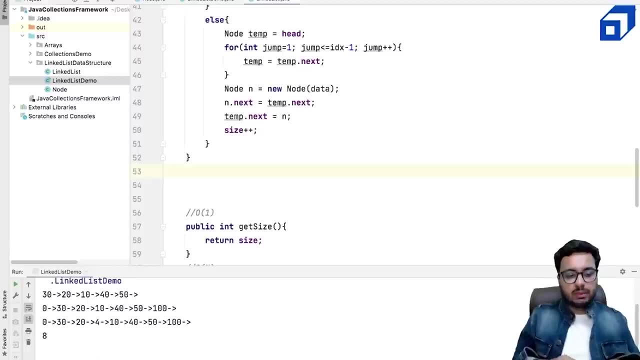 It's your time to code And I'll just show you the art art method. So pause this video here And try to implement these three methods. Let us implement the get method right. So I need to write a method called public int- get first. 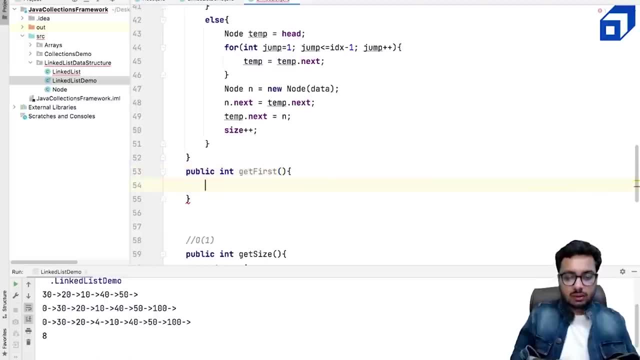 That means I want to get the first element of the linked list, But what if the size of the linked list is zero? I do not have any such elements, So I will have a special case. If size is zero, I can throw a new exception that the linked list is empty, right? 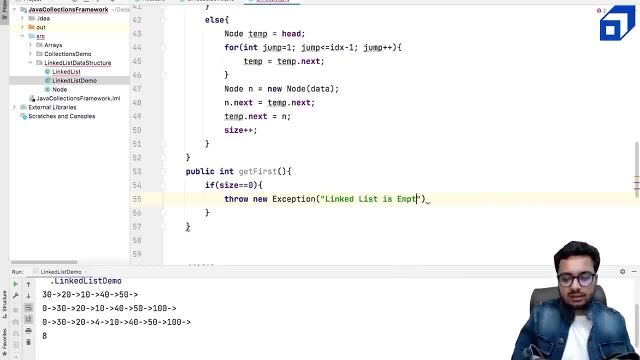 So linked list is empty. That is the error that I'm trying to make. I'm trying to show to the user right, And here I have to tell that. okay, this method also can also throw exception right, So throws exception. 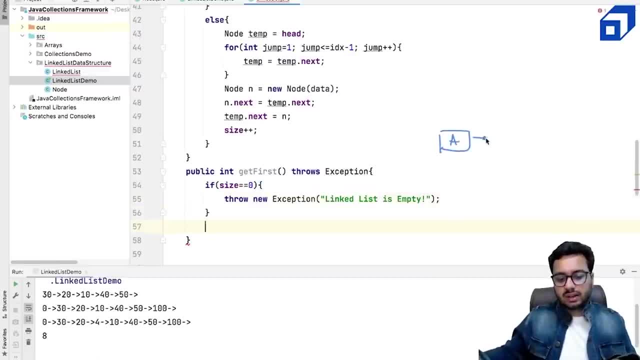 But if the size is not zero- the linked list is there- then it is pretty easy. We just need to return the data present in the head node- So head is referring to this node- Access the data and return it. Return head dot data. 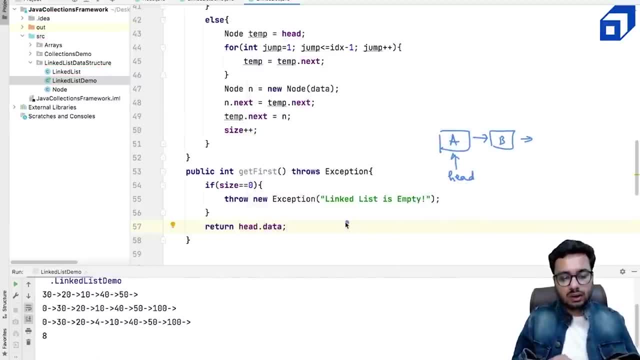 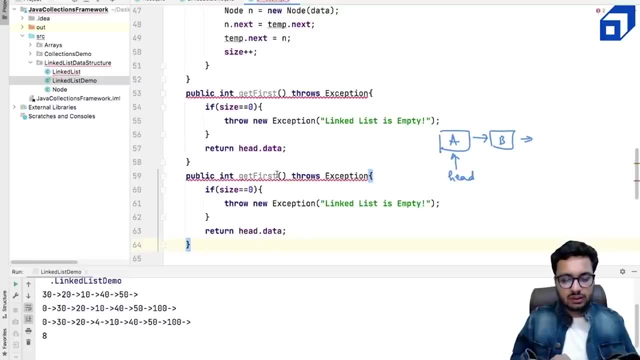 That's it. Size will not change And this is what you will do. So, similar to this, you can also write: get last. So again, if the linked list is having size zero, then there is no last element. You will throw an exception. 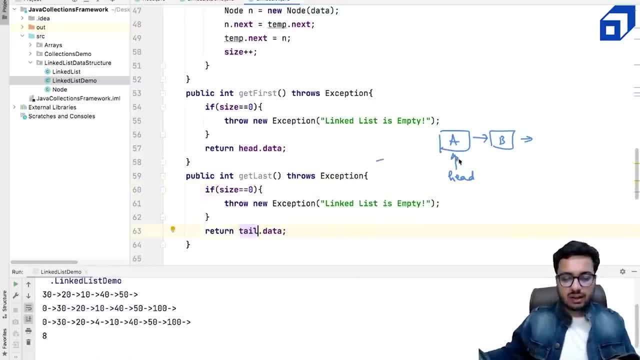 And in that case the last data will be at the tail node. You can say: return tail dot data. That's it. If you want to get something in the middle, that is going to take one more step because you will have to loop through it. 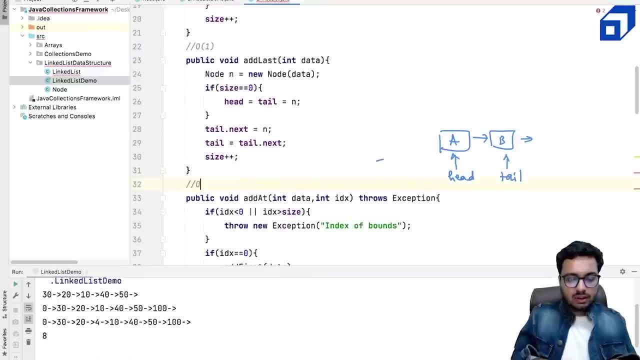 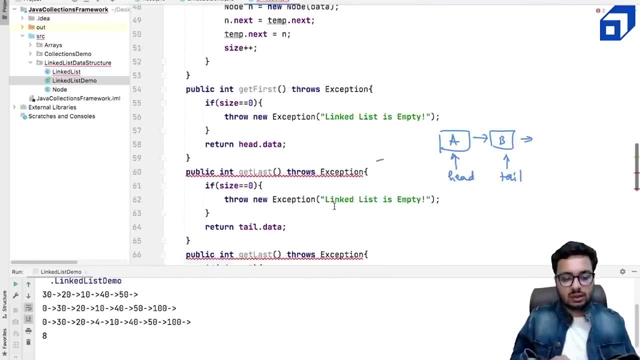 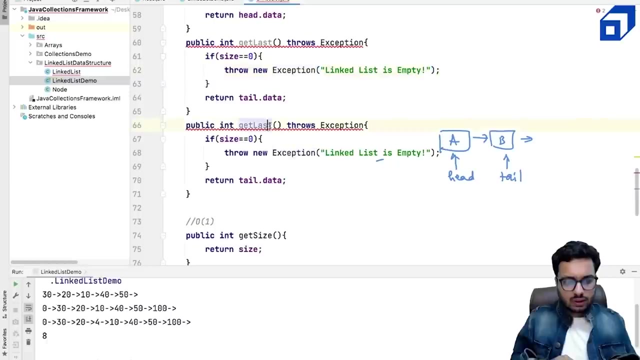 Right, Okay, So are that we did not discuss? It's going to take order and time because you are the worst case. You might have to loop till the second last or the last one. So get last. we have done Now this. this will be get at a particular index. 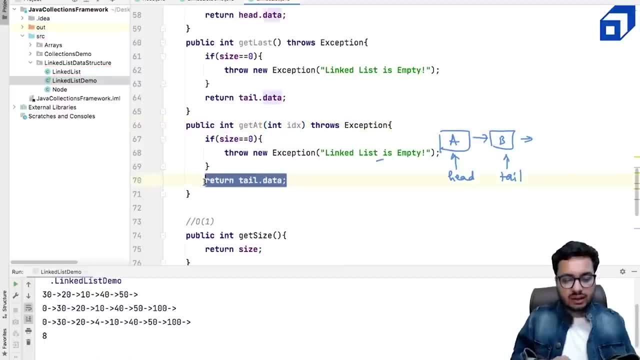 If I give you an index and I want to get an element at that how it will work out. take a pause and think how you will do it. This is also easy. right Now, user is giving you an index. Now it is possible that this index is also out of bounds. 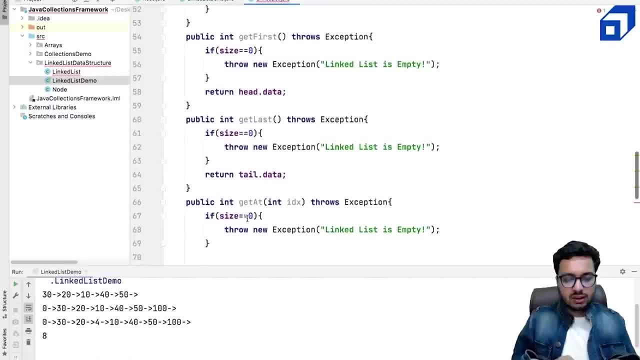 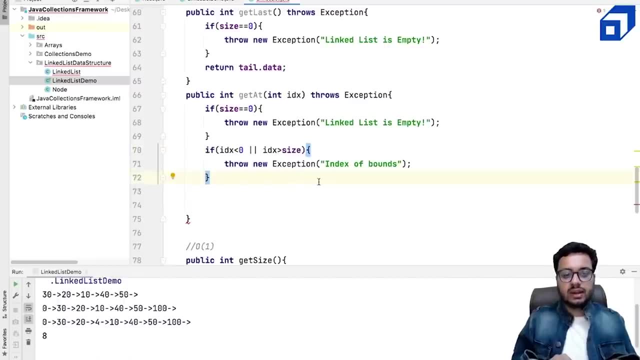 Like we saw here, right, Like in the case of addition, it is also possible that this index is out of bounds. So if index is less than zero or it is greater than size, I can throw an exception index out of bounds. Then if this is not the case, right? 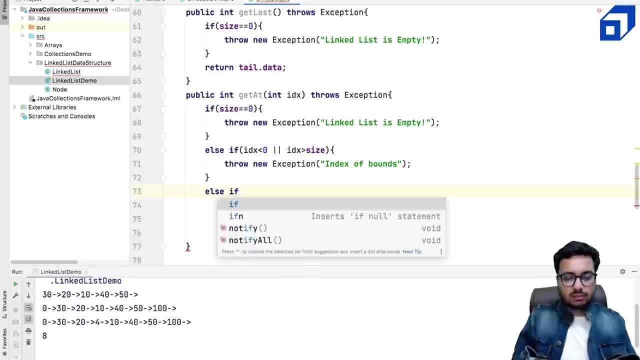 So if this is not the case, if the user is really giving you a valid index right, As if it is possible- You're talking about index zero. If that is the case, you can say return: get first. This can happen, as if index is equal to size. 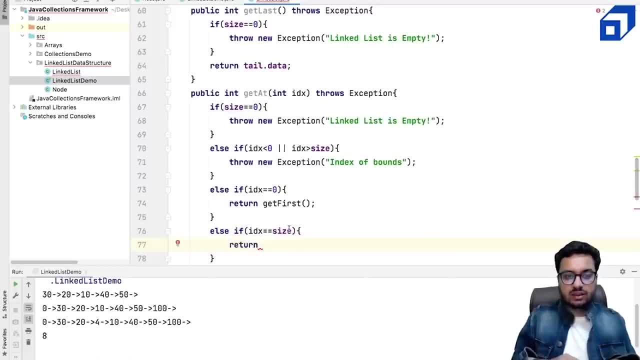 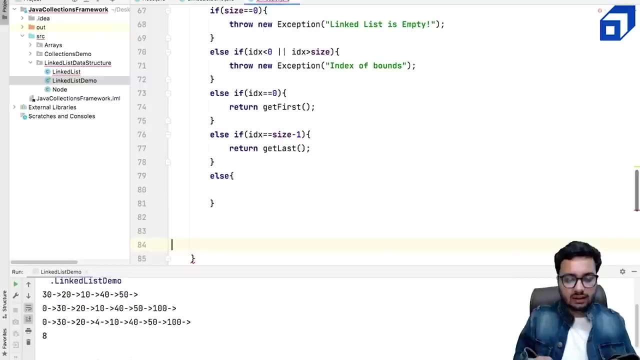 You can say return size or size minus one. It will be size minus one because the last element will have an index size minus one. You can say: return: get last. Otherwise what do you need to do? You need to iterate on the linked list, right? 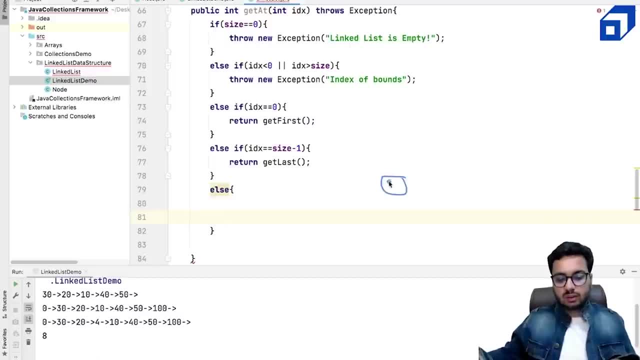 So that iteration part is easy. What we will do, we'll have, let's say, A, B, C, D and so on. right, This is index zero, one, two, three, four. right, I want to get something at the second index. 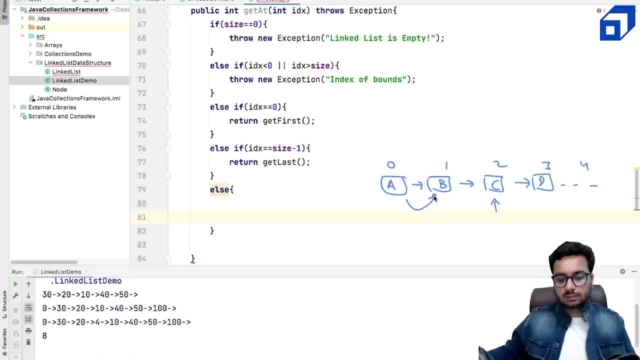 What I need to do. I need to take one jump, one more jump, two jumps to reach this particular index right. So that means take the number of jumps equal to that index. I can find node temp that is equal to head. 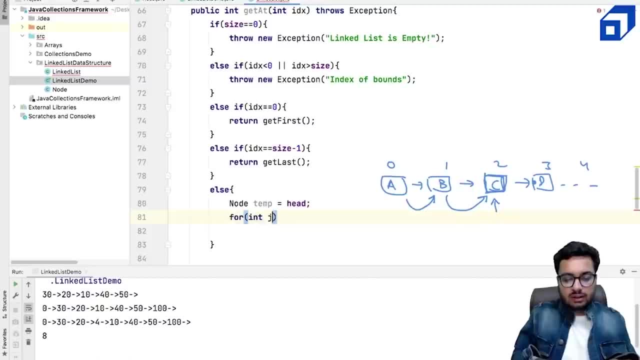 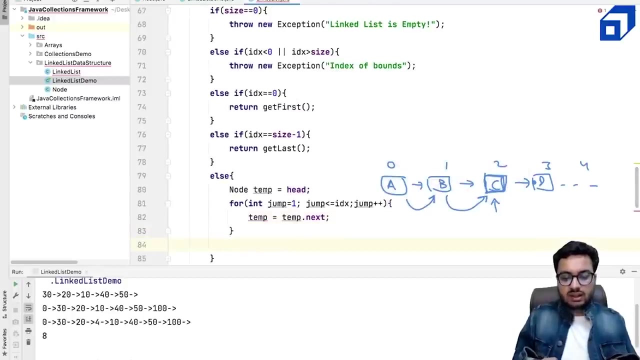 And for int jump equal to one jump less than equal to index Jump plus plus. What do I do? I take my temp to the next node, Temp equal to temp dot. next, Once I reach this node, I need to return the data of that node. 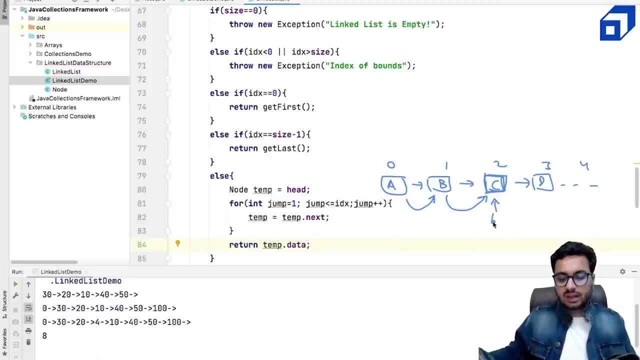 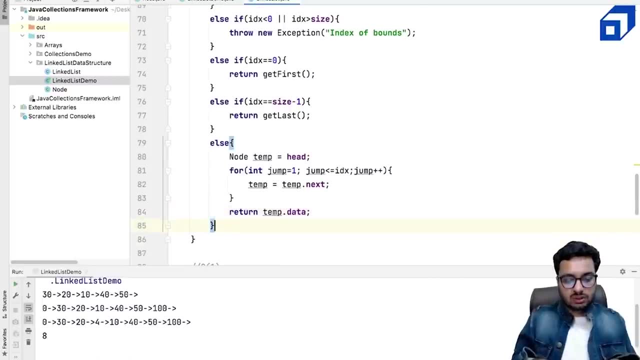 Return temp dot data. That's it. I take my temp here And I return this data. right, This will give me the data at a given position. So that is my get at particular index. Now let us test this code. 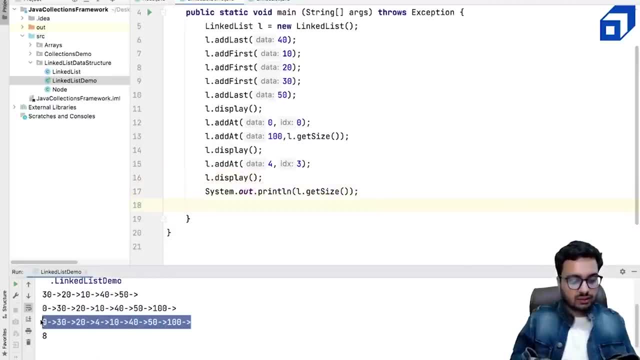 So I want to say, okay, fine, In this linked list that we have, I want to get the zeroth element: S out L dot get first, S out L dot get last And S out L dot get last. S out L dot get at index four. 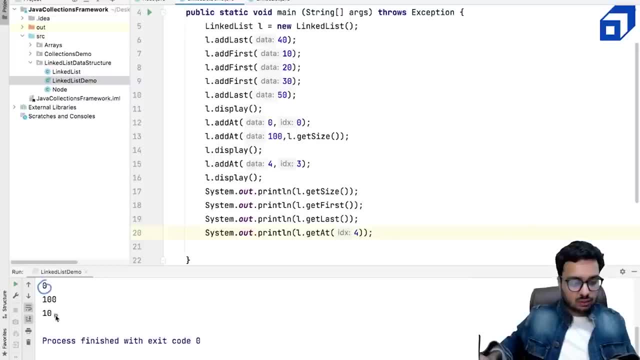 Let's go and run this code: The first element is zero, Last element is 100.. The fourth element is 10.. Let us verify. So zeroth index, first index, second index, third index, fourth index. So fourth index is really 10.. 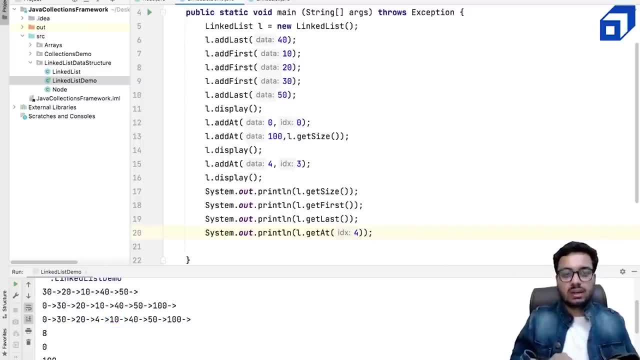 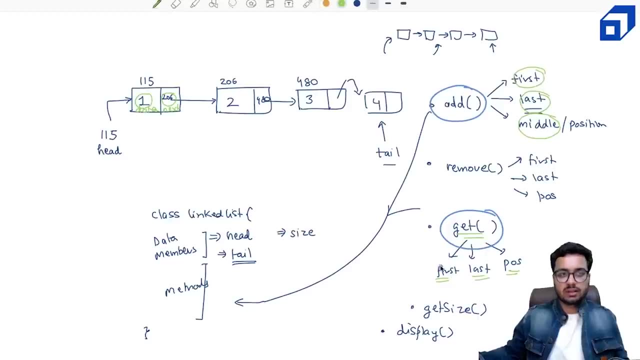 That means my output is correct. That is how we build the get at methods in the linked list. So far we have seen the add method and the get method. Okay, all the three versions. So getting first, adding first. they all take order one time. 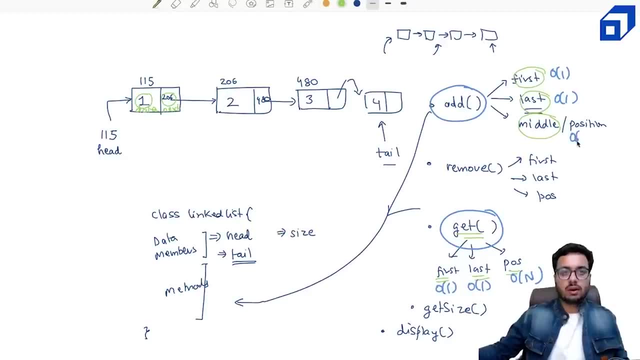 But doing some work at a particular position. they take order of n time, So other methods are all one. Now we have the remove method. We want to remove first, remove last and remove at a particular position. Let us see how we will write these methods. 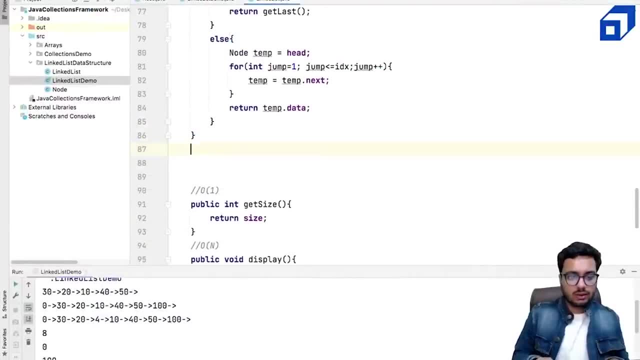 So what I will do? I will create remove methods, public int, So remove. I will also get the data that has been removed From that particular index. So return type would be int, So remove first. You might think it should be very simple. 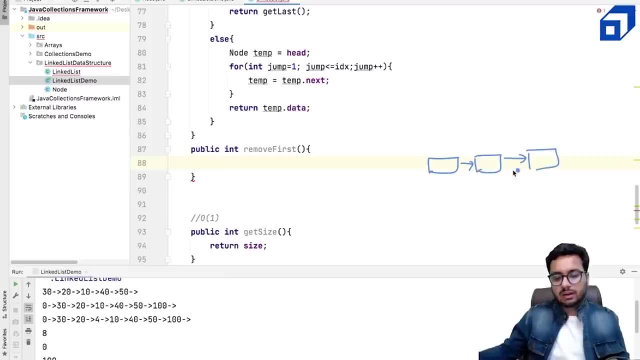 Whatever is at the head, I will return that. So I want to remove this. let's say, 10, is there 20 and 30. And this is my head. How do I remove this node? So one way is okay: you can store the output. 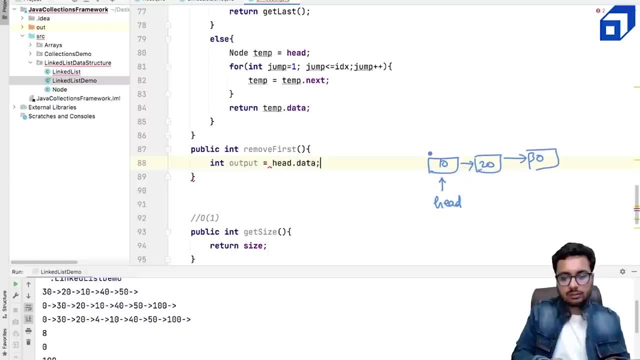 That is going to be headdata, And then you can say: okay, this head Will move to the next node, So head will go here, So head is going to be at headnext. So doing this, will it remove this node? 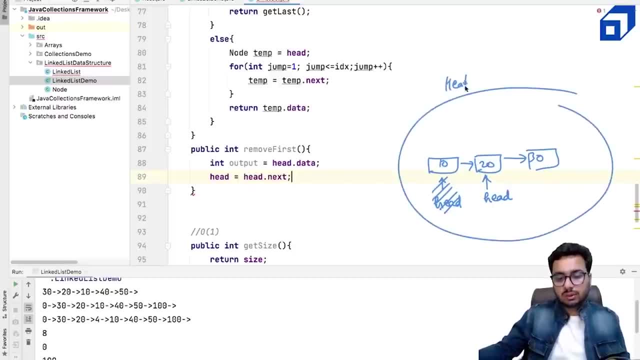 The answer is yes. So in heap, this node is a node that no one is referring to. What will happen? It becomes eligible for garbage collection, So garbage collector will come And it's going to sweep away this memory. That means now your linked list will be only this. 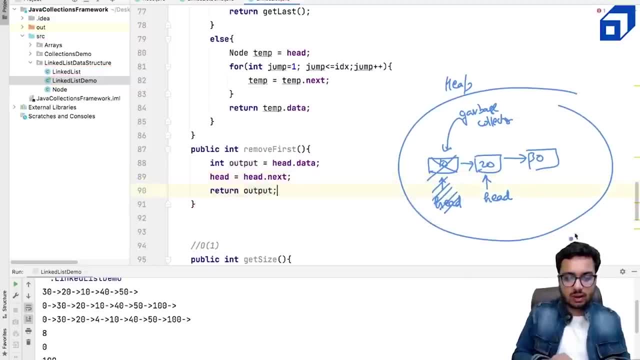 But there are few special cases. I can say: output will be returned. That's okay. You also need to reduce the size. This dot size minus minus. This is something we need to do, But what is the special case If the linked list is empty? can you remove the first element? 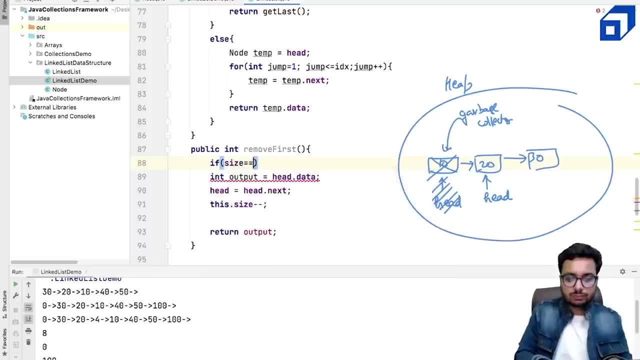 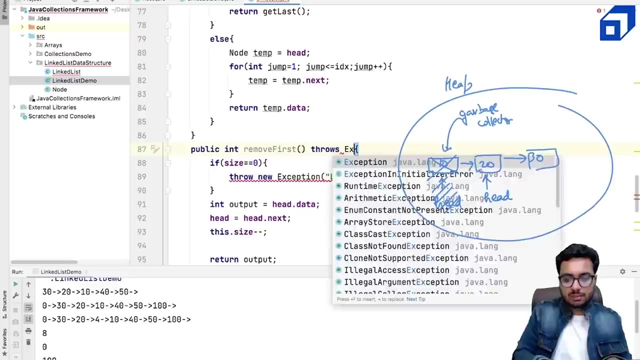 The answer is no. We have to check if the size is 0.. What we will do? We will throw an exception. We will throw new exception. that linked list is empty, Fine, And we need to tell that this method throws exception. 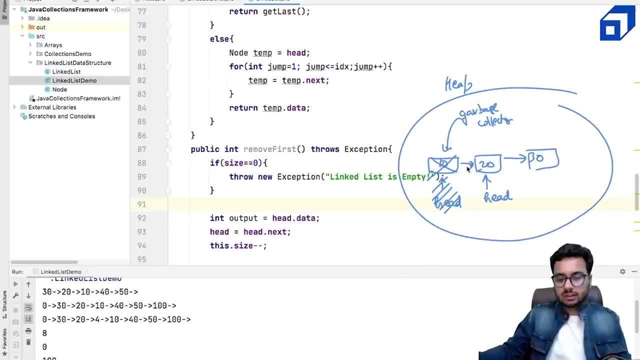 Now what about if the size is 1?? So head will get updated, fine, But if you have just one node and both head and tail- they were pointing to this node- Will it form a special case? Of course, yes. If this node is getting removed, what will happen to head and tail? 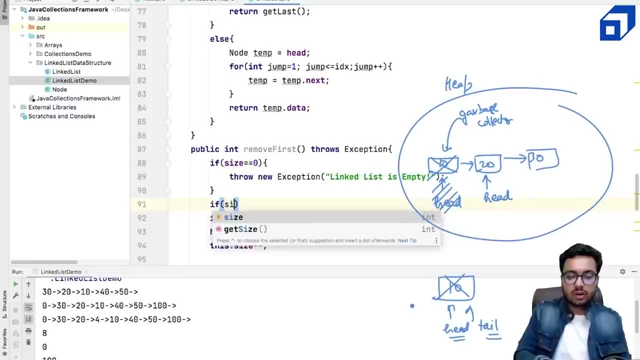 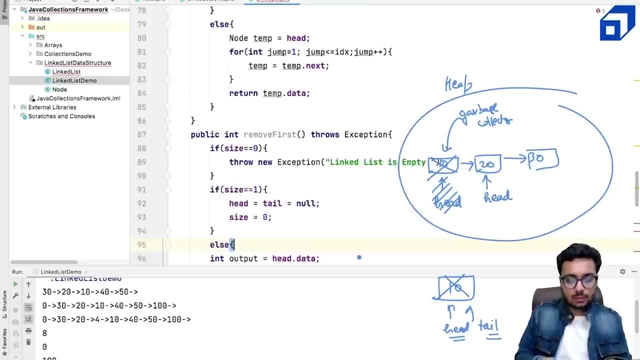 They will be reset to null. If your original size was 1,, how do you remove it? You will set your head And tail equal to null. Size will become 0.. Okay And else Sorry. Yeah, So one thing we can do is. 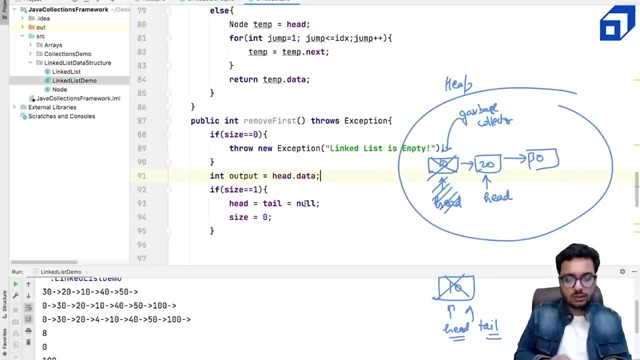 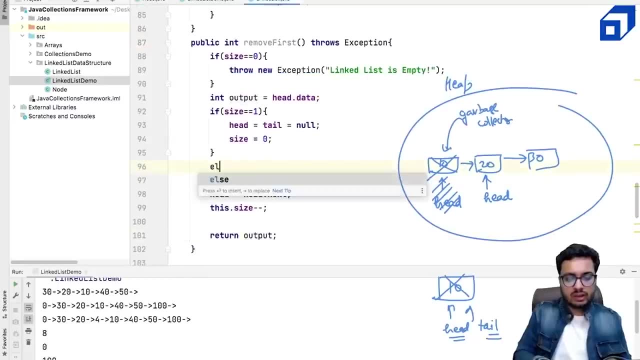 This code we can move here. Output is equal to head dot data. Okay, And we will of course return output. This code we can move in else case. That means if there are, like, At least 2 nodes. In that case, 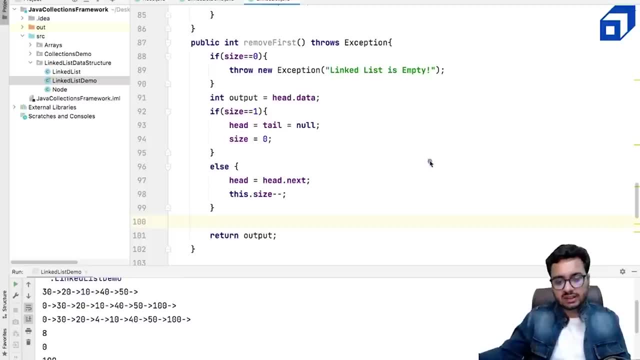 Tail will not be affected, Right? So what about this case, Else case, If there is 10.. There is 20. And there is 30.. So this is my head, This is my tail, Even if my move Remove this node. 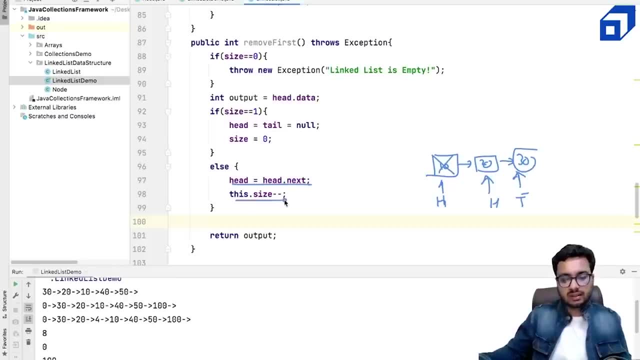 Head comes here, Right. So head goes to the next place. Size gets reduced, So tail is not affected, Right? But if I have just one node And I remove that node, In that case Head and tail both will be affected. 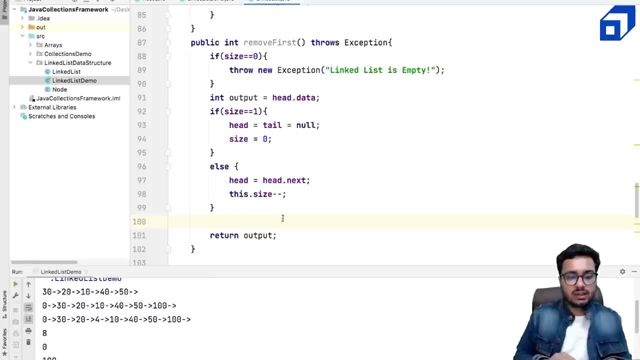 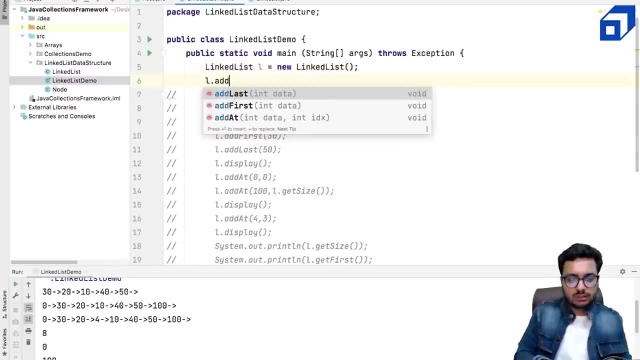 So they are reset to null And the size becomes 0. So that is how the remove first method should work. Now let us test this method. Let me create a new linked list. Let's say I add At the first position: 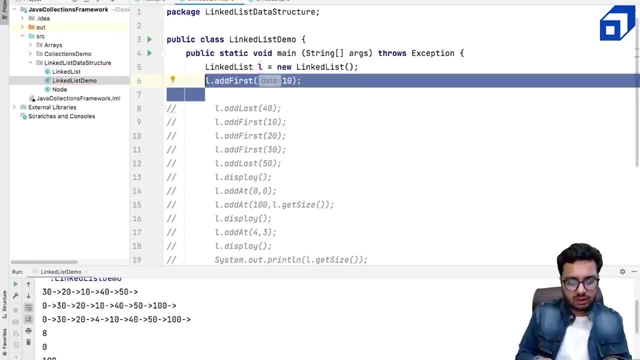 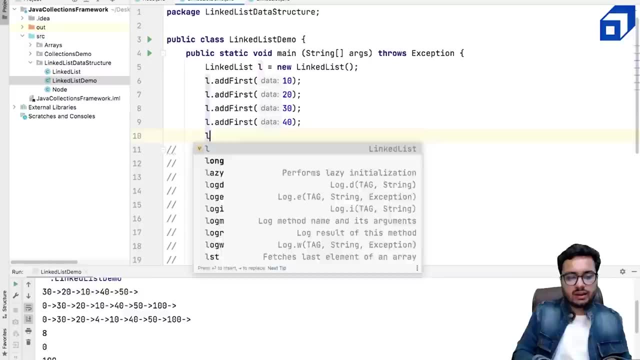 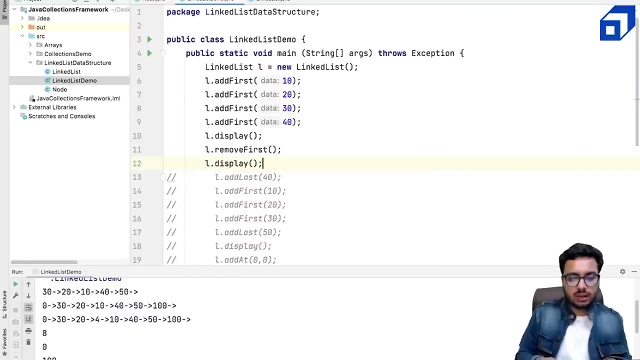 Let's say 10.. Then I add 20,, 30,, 40.. 20,, 30,, 40. And I can say L Display. Then I can say L Remove first And L Display. 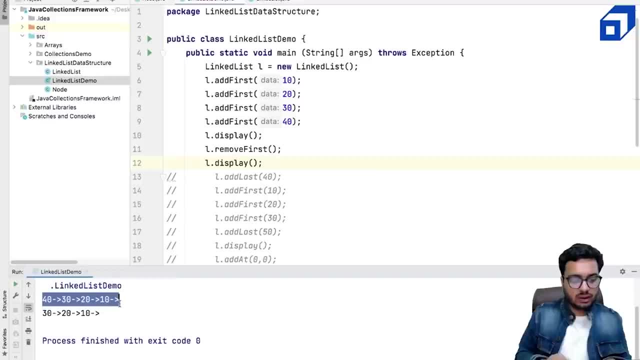 Right, So I am getting 40, 30,, 20, 10.. Fine, And if I remove the first element, 40. My linked list is 30, 20, 10. Which is fine, Okay. 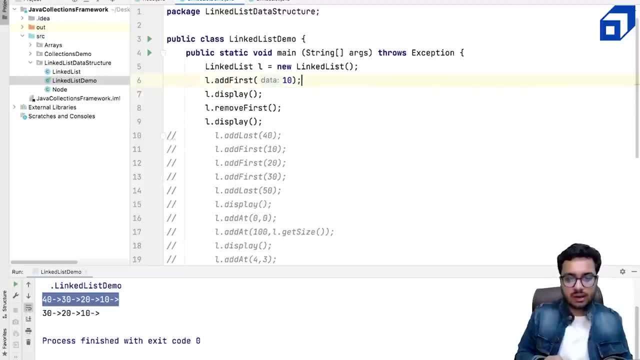 If I have just One element in the linked list And let me see if it works well. So I have one element, I removed that One element, My linked list is empty. Fine, That also works well. Right, And I can say: 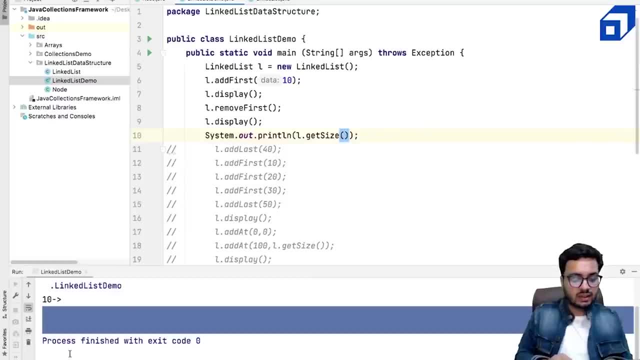 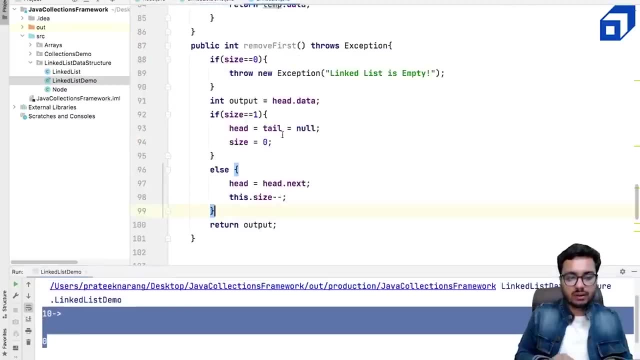 Sout L Size. I want to see if my size is getting updated properly. Yes, The size is zero and I don't see any output here. That is how I will implement Remove first method. Now on the similar lines: 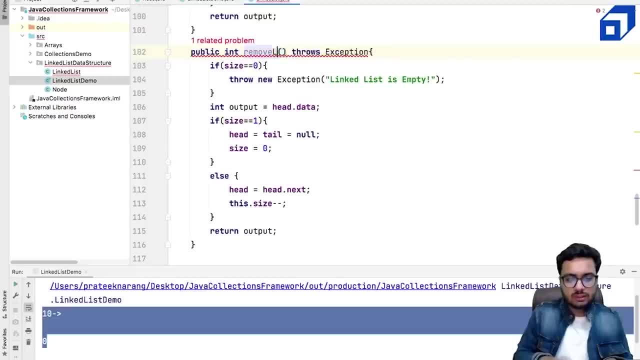 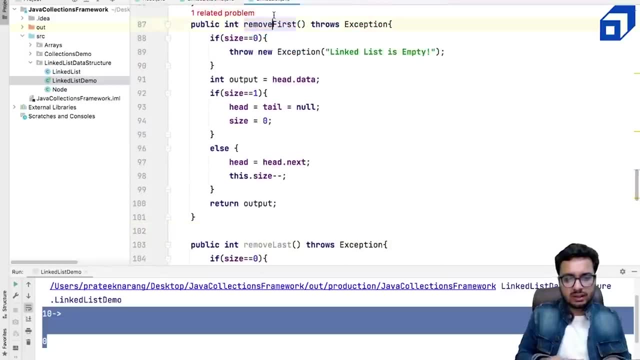 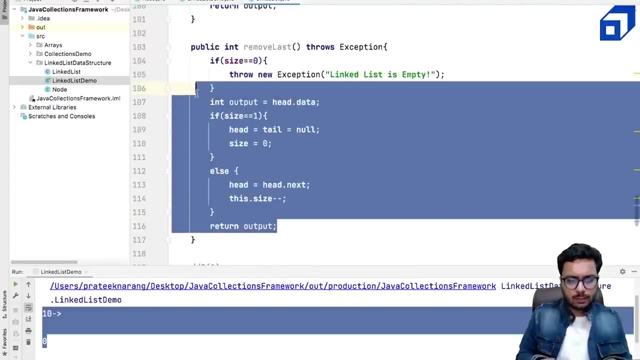 Can you implement the remove last method? Okay, Just need to think What will change, What will happen to head and tail, How much time it will take This method. It's going to take Order one time, Right, Remove first. 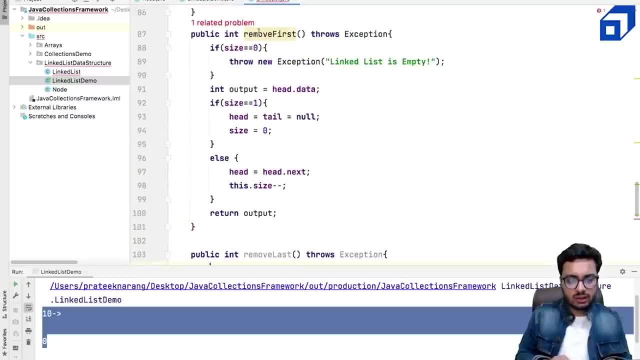 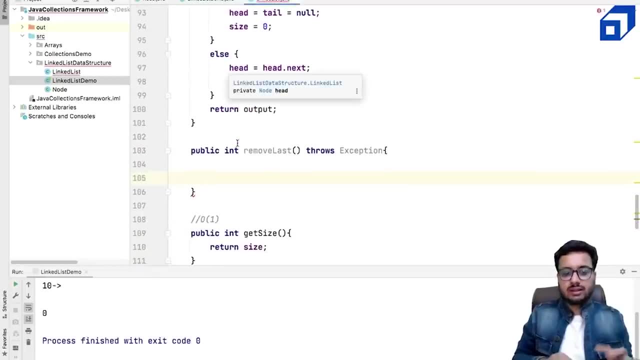 But you have to think How much time remove last will take. Okay, So let's see: Remove last. Okay, So First case is Okay. If your linked list is empty, You cannot throw anything. You cannot Remove anything. 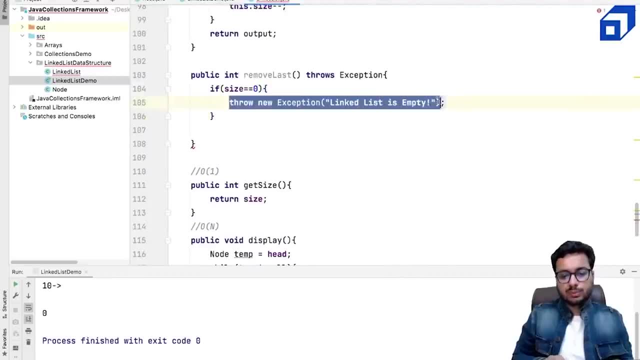 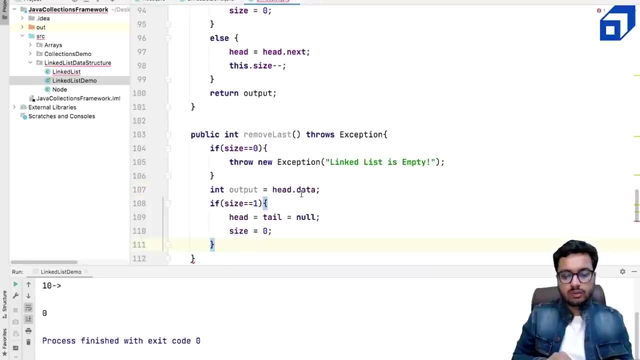 So if Your size is zero, You will throw a new exception. Okay, So, Similar to this one, Your output In this case will be what Your output will be now: tail dot data. You know, the last node Is: 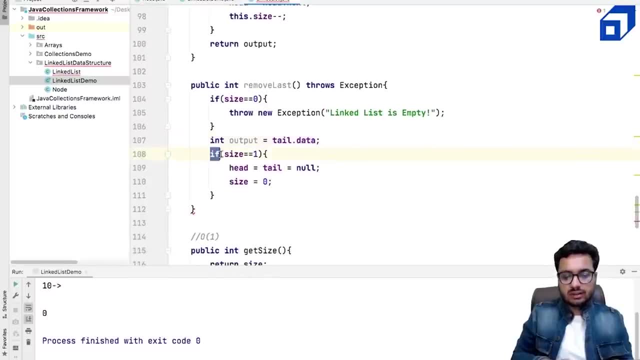 Tail, And that data is your output Right. So if your size is one, What you will do? You will Reset your head and tail to null, And you will The size is zero If this is only one node, Both head and tail are referring to this node. 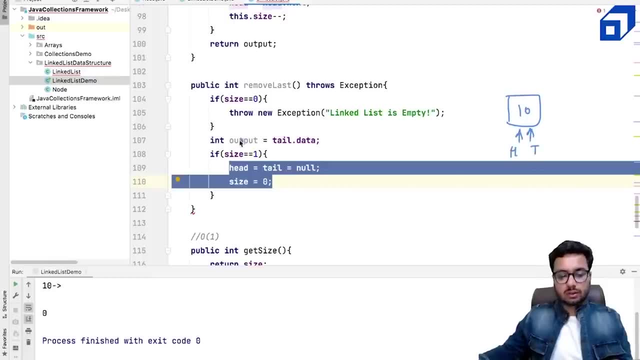 You want to get this data. You store this data in a variable called output, That is tail dot data. Original size was one. If this is removed, Then You can Remove This Node. If this is removed, Head and tail. 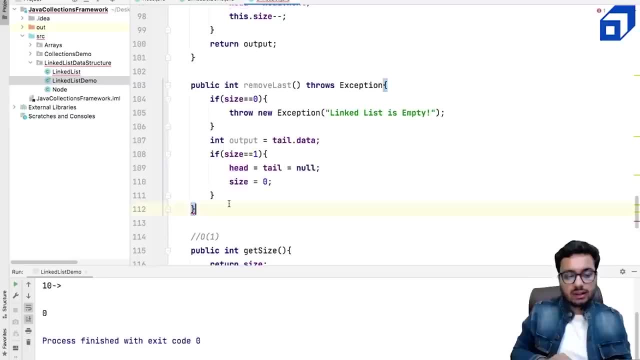 They are reset to null And size becomes zero, Which is correct, Right? Otherwise, If you really want to Remove something, Right? So you will have to check That, If your index is in the bounds Or is it zero. 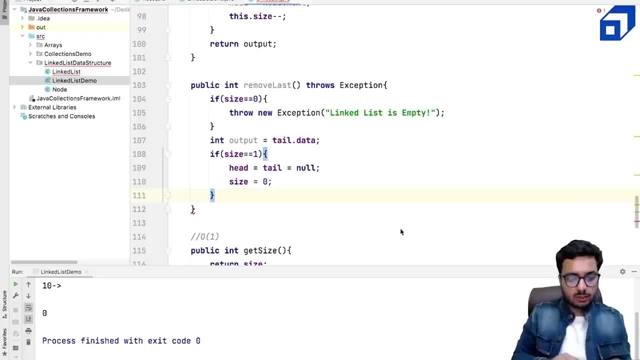 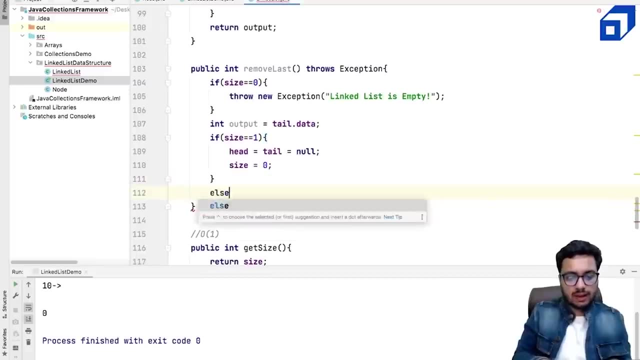 Or is it the last index? Sorry, You don't need to check here, Because we are Talking about remove last Right. So you just need to Remove the last node Right. So what I will do, I will say: 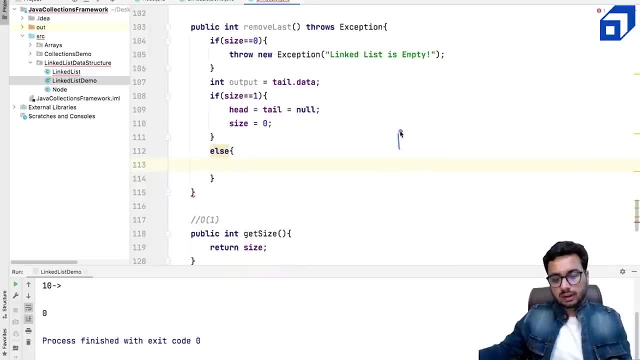 Okay, Else, There are more nodes, Right. There is One tricky Thing here: That If it is a singly linked list, Right, And This is your tail node- You are saying: I want to remove this node. 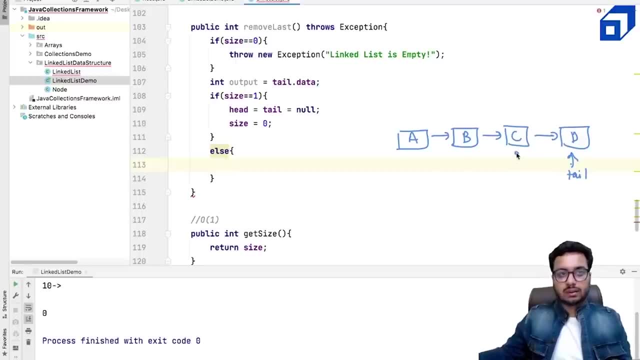 Right, That means Tail should be updated. Tail should come here. The new tail Should Come here Right After removing this node. I have stored this d In a variable called output, So output is tail dot data, So output is d. 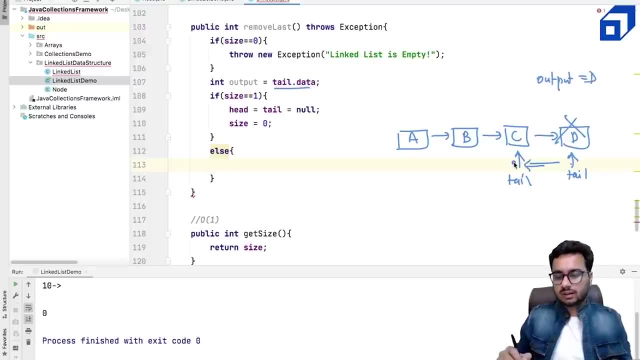 Right, How do I bring it back? There is no way to do it Right, So I will do it Right, Even if you maintain, Okay, I will maintain previous of tail for every node. Suppose This was the previous. 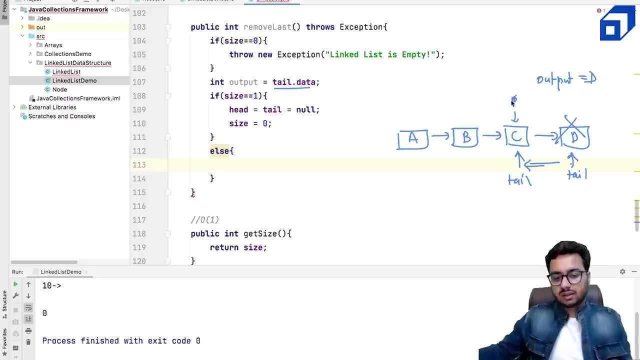 But when you remove, See How you will get the previous. The answer is: We don't have an Any Order One way Of Coming to the previous node. We have to iterate from the beginning To reach this node. 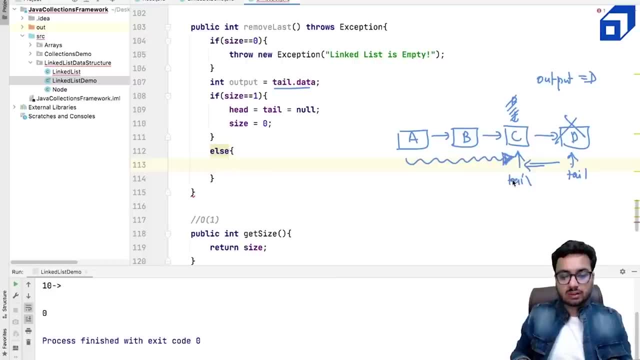 Right, So that I can update my Tail variable. Right, So this is going to take time, Right? Or The other option is You maintain a doubly linked list In which, If you do that, Your Remove last. 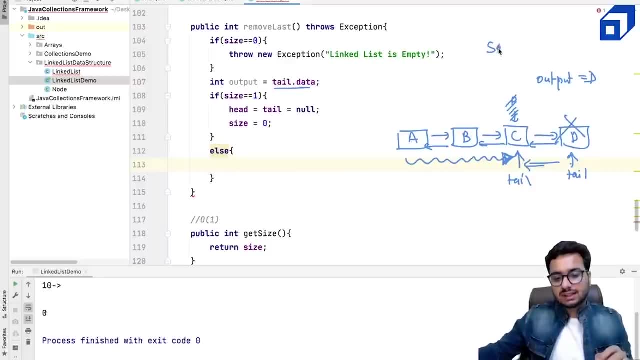 Will work in order one time, But for now We have a Singly linked list. That means We have Only the next Address, Right Singly linked list. In that case We have only one option: Start from the head node. 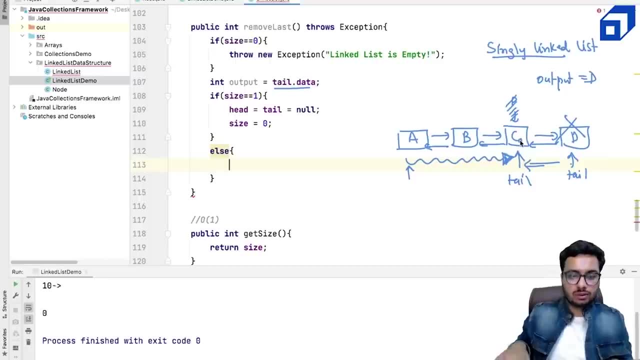 And try to reach The second, last node. So how do I do it? So I take a variable Called Temp, Which starts from head. I can say: While Temp Next Is not equal to Tail Right. 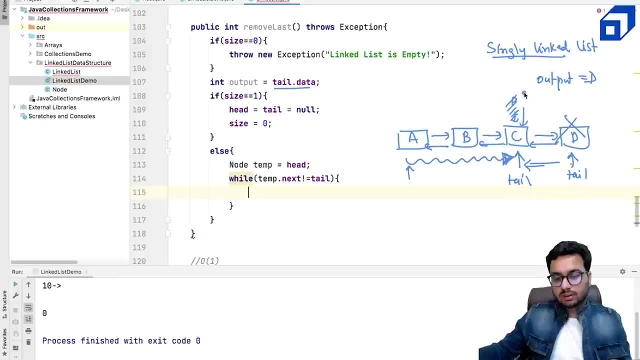 So what is the stopping Condition? So when I reach This node, Temp Dot Next, This is equal to Tail Right. So this is the Tail node Right. Suppose this is my C, This is my. 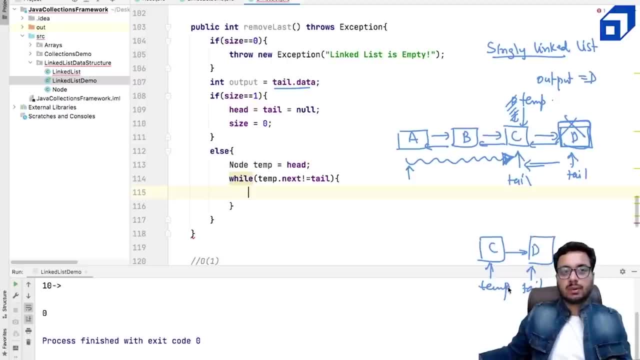 Temp, And this is my Tail node, This is my D Right. So I am saying: While Temp, Dot Next Is not equal to Tail Which starts from here, It goes here, It stops here. 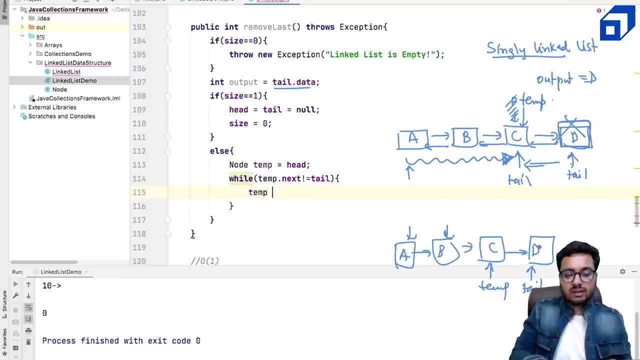 Right, Because C Is next Is equal to Tail, So Temp Will stop at C, So I can say: Temp Equals to Temp Dot. Next, My Temp Stops At The. 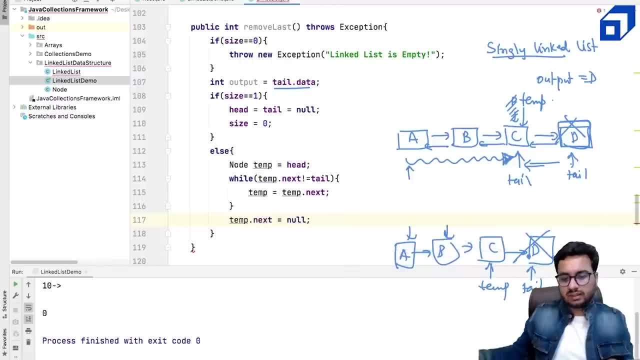 Second, Last Node Right Now, If This Is Equal To Null, What Will Happen? This Object Becomes Eligible For Garbage Collection Because No One. 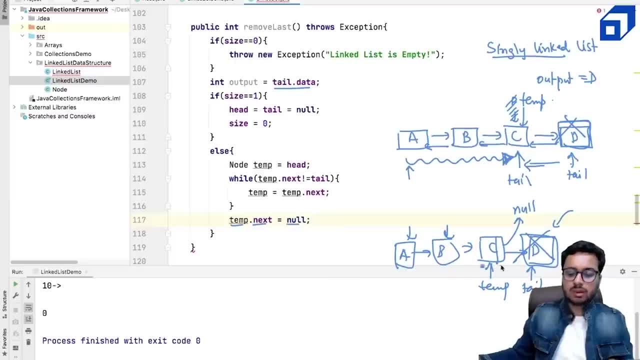 Is Referring To This Object Right. So Garbage Collector Will Stop At Temp. So Once This Is Done, What Should I Do So Temps? 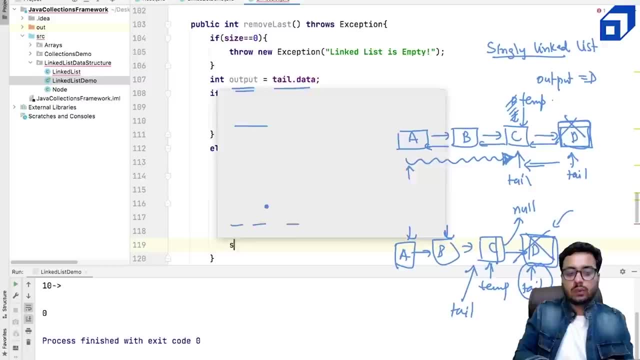 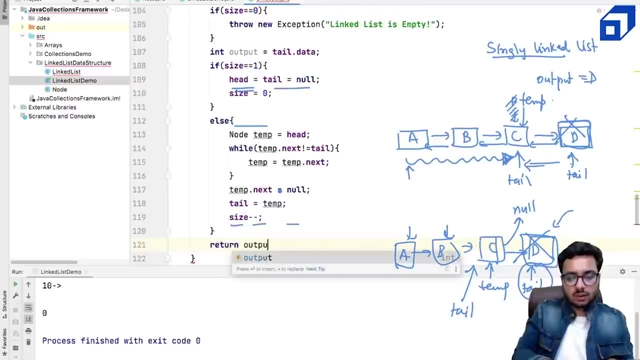 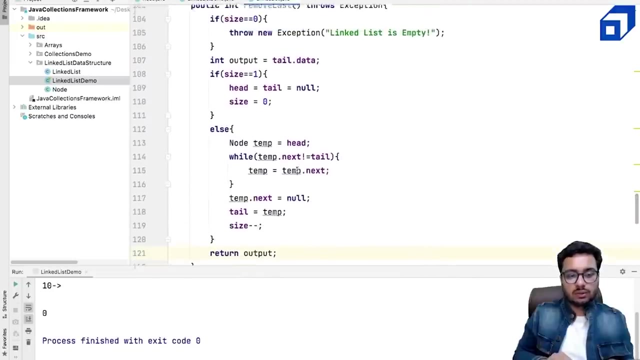 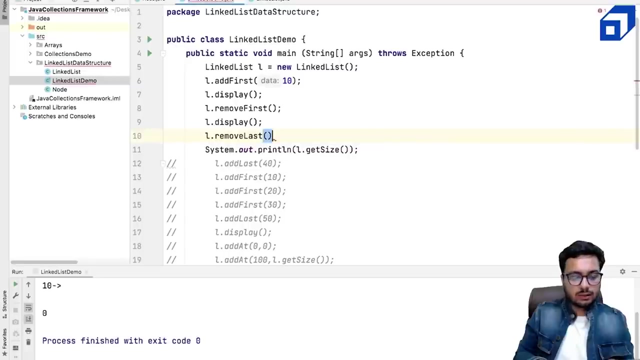 Next Is Now Null. This Tail Should Be Updated, So This Tail Should Come Here To The Output. That Is How Remove Last Will Work And 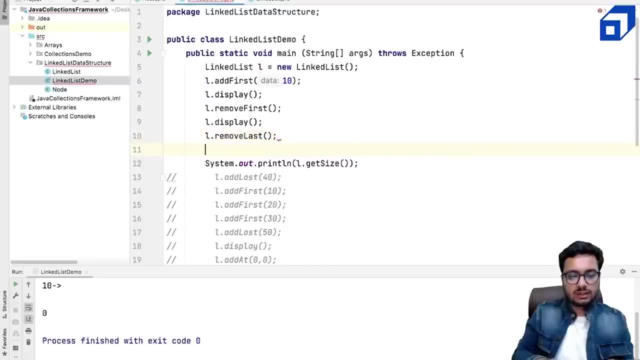 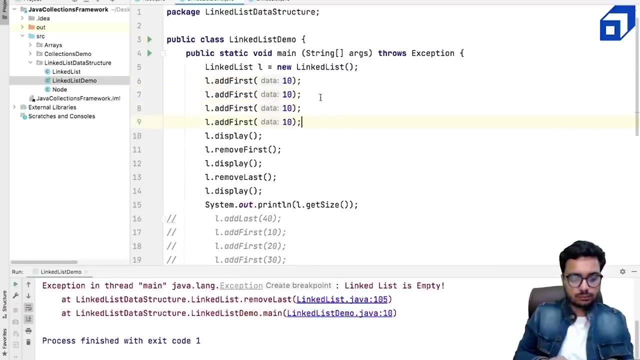 If I Now Show You L Remove Last, And Maybe If You Want To Output, That's Okay. We Have 20.. 30., 40. So Right, 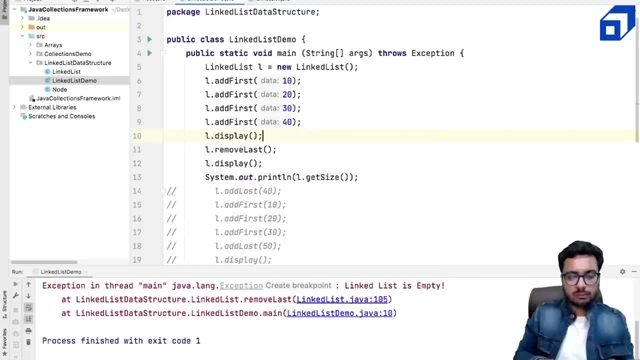 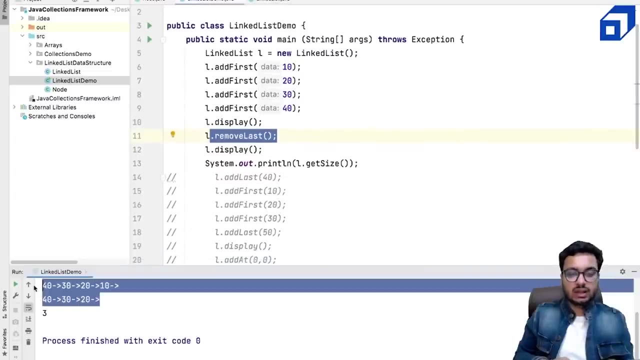 Now I'm Getting An Exception Because You Know It's An Empty Link List. So 10., 20., 30., 40. L Display, And Then I 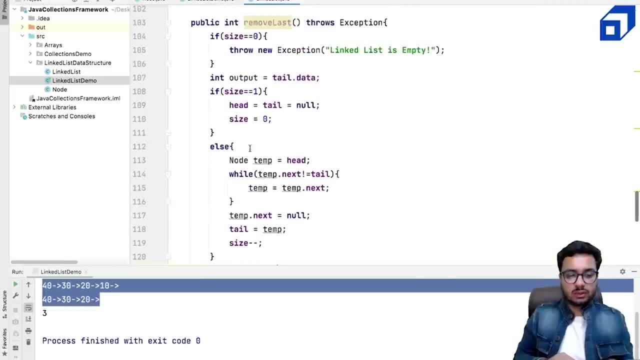 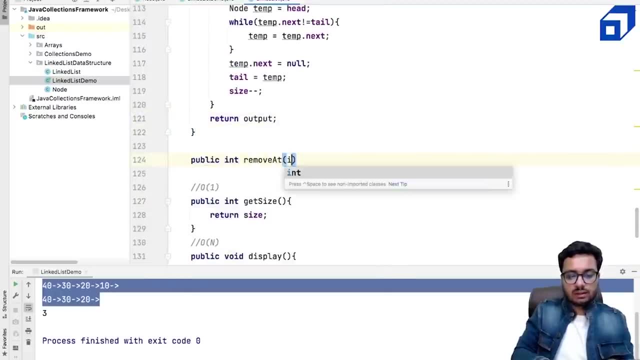 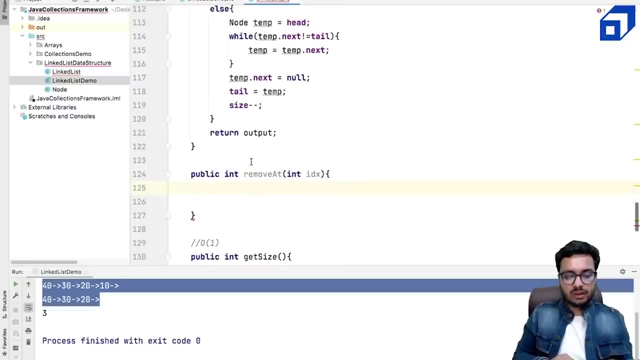 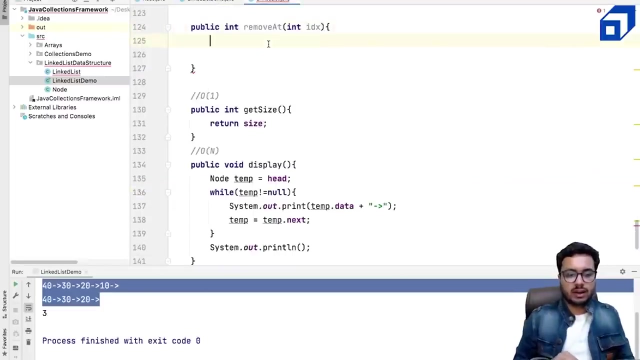 Of Course It's Going To Be Removed At A Particular Index. We Want To Write One More Method: Public Int. Remove Art Given Index Again. 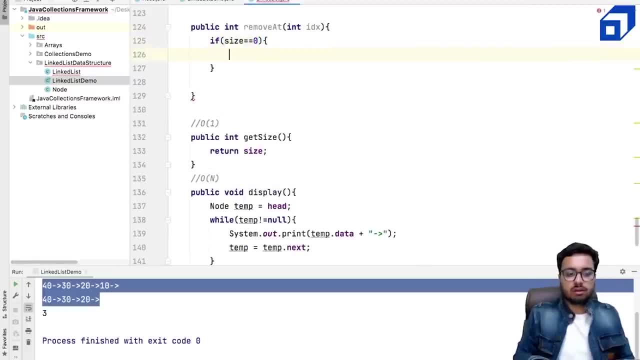 Before I Write The, You Will Throw A New Exception. So Throw Exception, Throw A New Exception And You Will. Okay, Link List Is Empty. You. 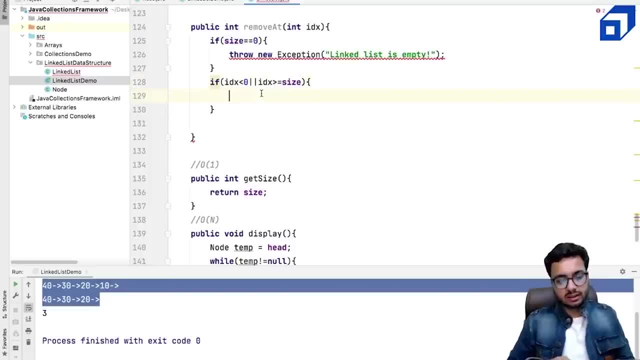 Cannot Remove It Or You Can Check. This Is The Case. I Have To Throw New Exception. I Will Throw A New Exception And Will Tell. 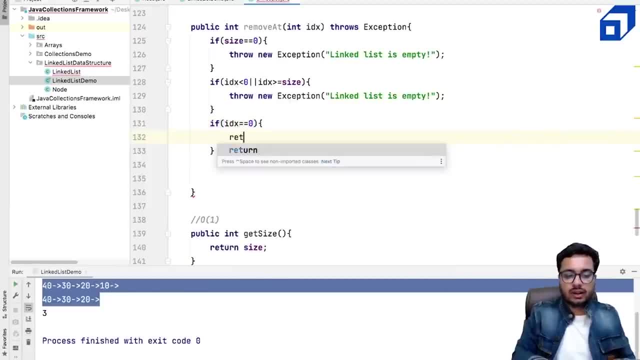 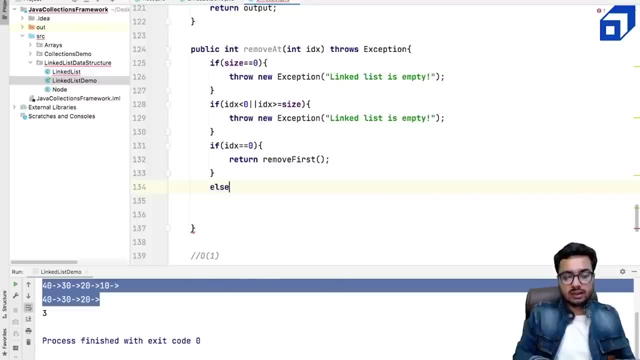 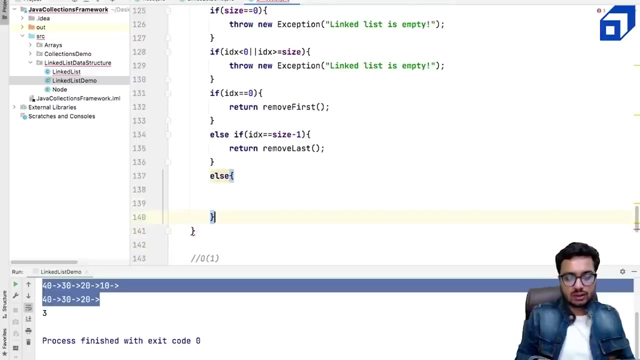 That This Method Can Throw An Exception. All Right, So Let's Start. As If Index Is Equal To The Last, Which Is Size Minus One. 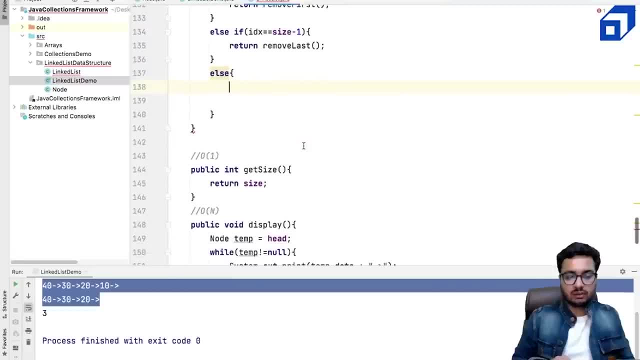 Will Return Whatever Is Removed By Remove Last Method. And Now Is The Time And Is Okay. I Want To Remove Something From Index To 012.. 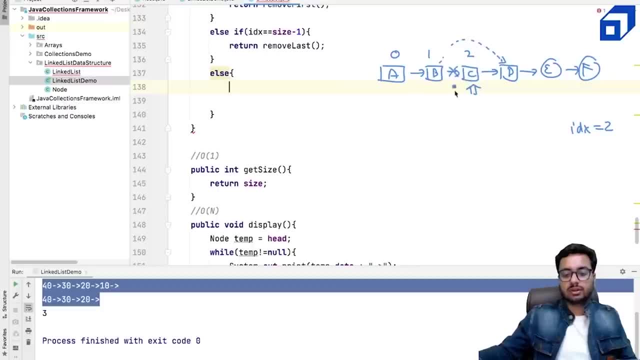 I Want To Remove This Element. If I Want To Remove This Element, That Means We Should. That Is B. So If My Index Is To 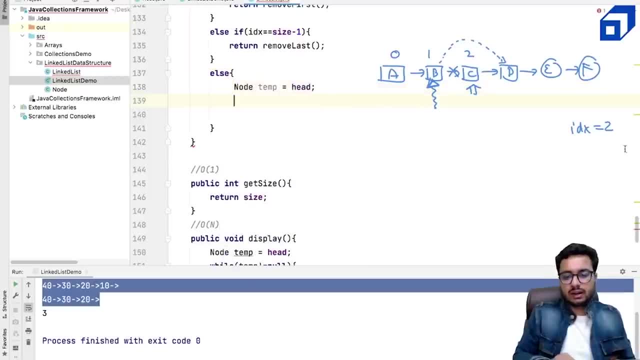 I Need To Reach One Node Behind That Index. How Do We Start Node Again? Fairly Easy, I Can Say Here And At This Node: 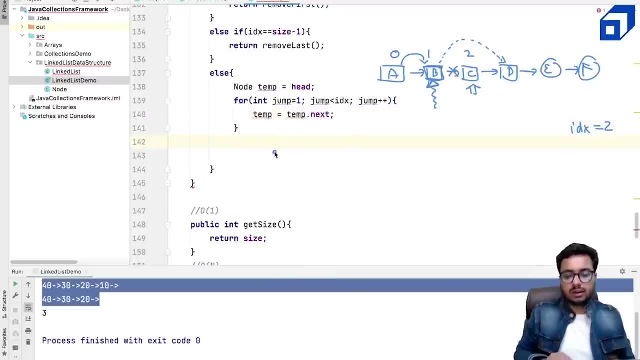 I Will Start Doing Certain Operations To. First Of All, Let Me Take Them To That Particular Node. Now I'm Standing At This Node And 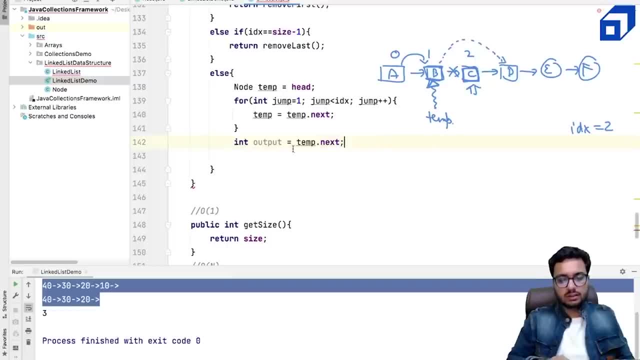 I Want To Return That Output. Or Let's Say This Is My Node, Which Is Okay. Either Way We Can Do It. Node Called Output. 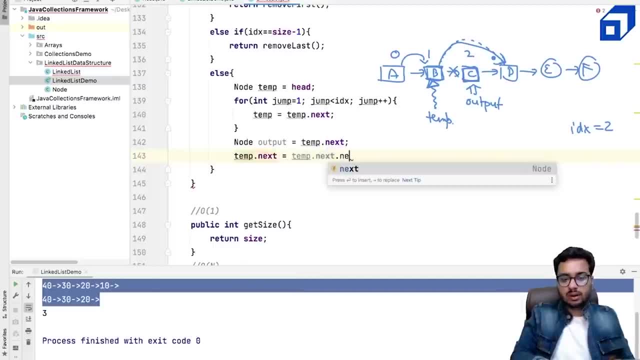 So This Node Is Output Next. So That Is My D, Or You Can Say Output Next. Again, I'm Connecting B With D, Now No. 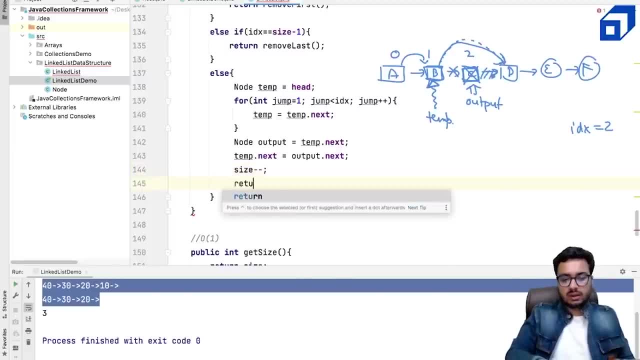 One Is Pointing To See It Will Output Dot Data. This Output Is A Local Variable Right. It Is There Only In This Function Once. 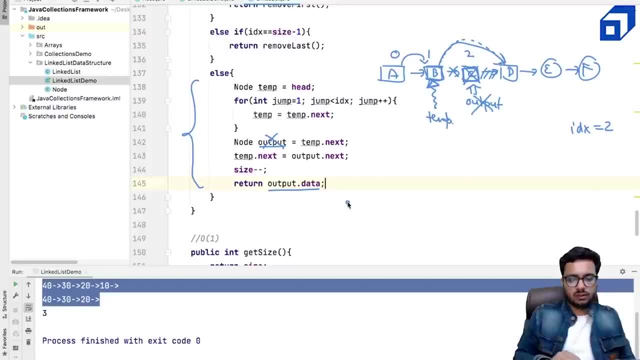 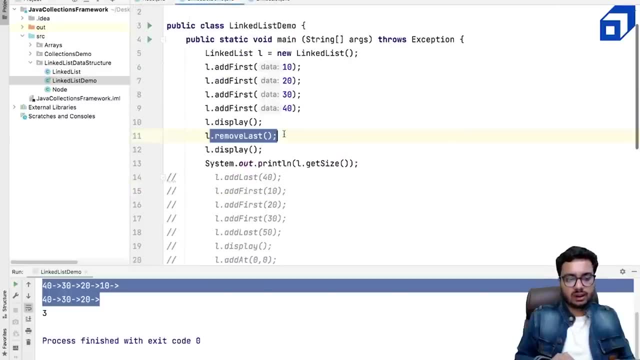 I Return Output Dot Data. There Is This Function: Call Is Over My Code. I Can Say L Dot Remove At Index. Let's Say One. 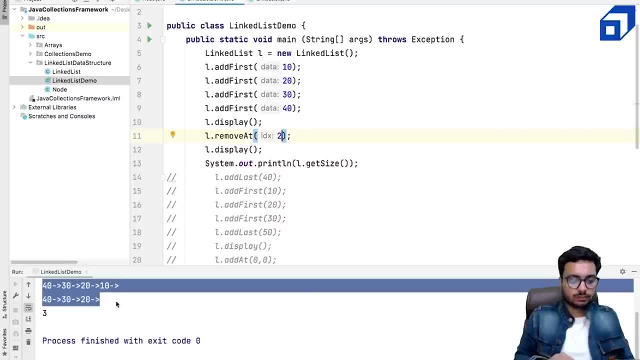 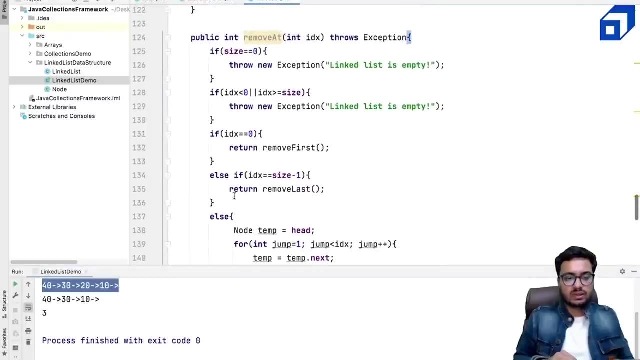 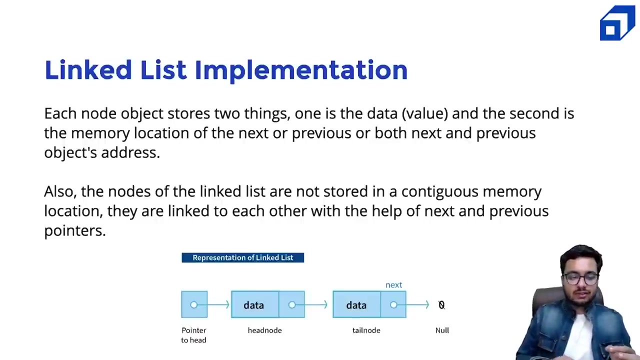 Given This Link List, Let's Say Remove At Index 2. Which Is Okay. Show Me What Is How We Can Remove Something From The Middle. 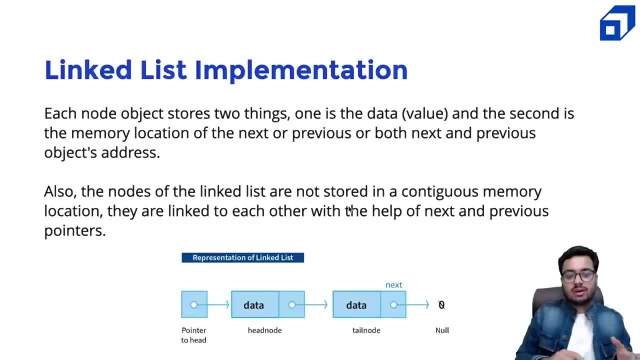 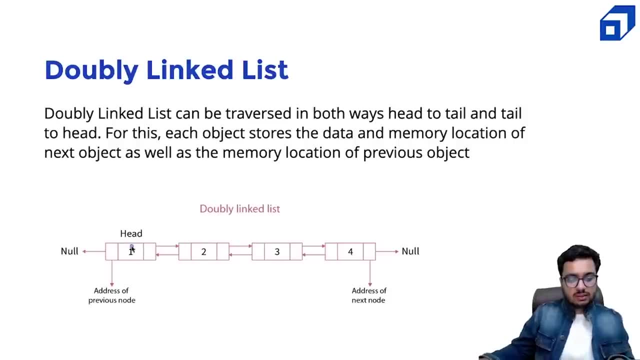 Of Link List. So Far We Have Seen The Implementation Of Single Link List Right So, In Which We Said Previous Reference To Will Hold The 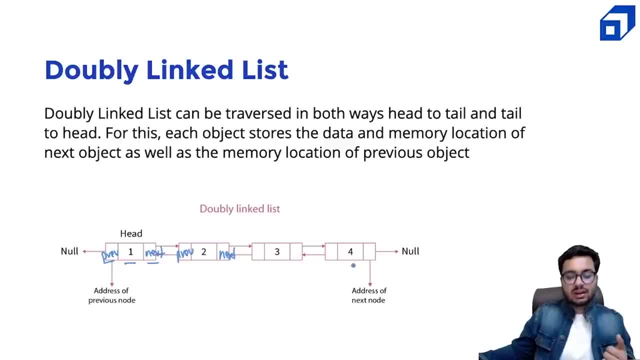 Address Of Three, Who Will Also Hold The Address Of One Right Now. The Advantage Of Double Link List Is That You Can For A Double. 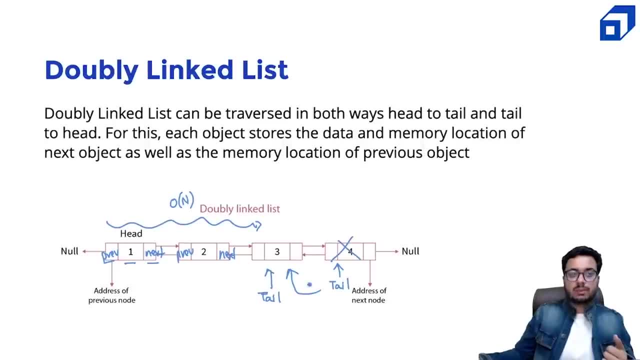 Link List. I Can Just Come Back To The Previous Note. Okay, Because Four Knows The Address Of Three, So I Can Update My Tail. 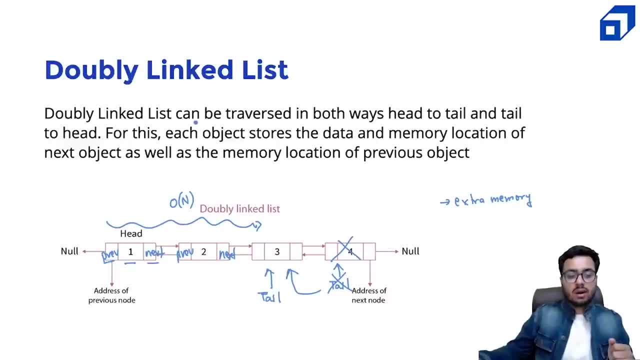 Pointer So You Can Do Insertion And Deletion In Order One Time Right. So Each Object Stores Data And Memory Location Of Next As Well. 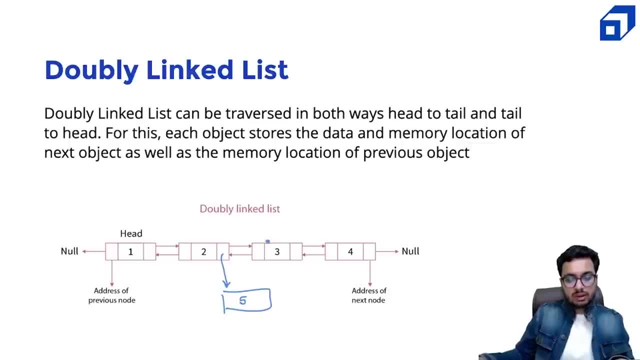 As The Previous Object. Right, So What I Will Do Is As Okay, Let Me Create This New Note Five And Let Say This Is My 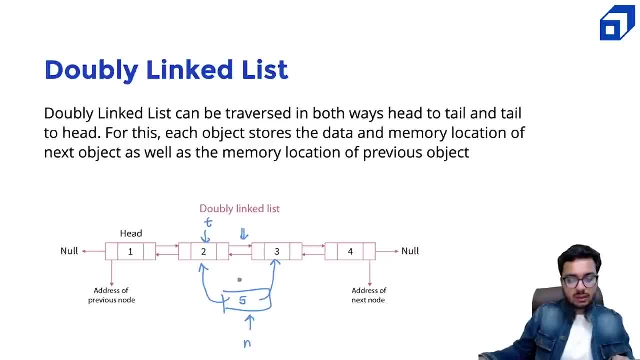 Temp Here. I Want To Insert It The Right, And I Also Need To Say Three's Previous Right, Or We Can Do It Other Way. 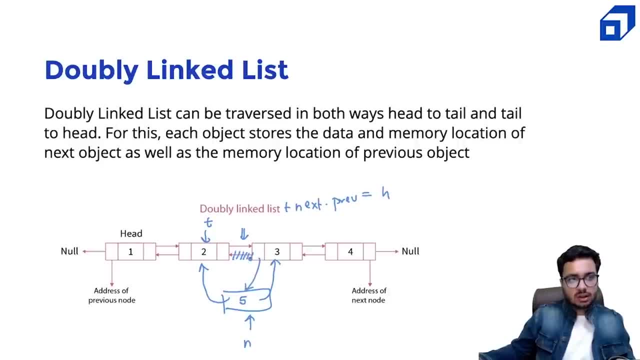 Right. We Can First Say That This Node, Which Is The Next T Dot, Next, This Is Equal To And Right. So Again, You Just Need. 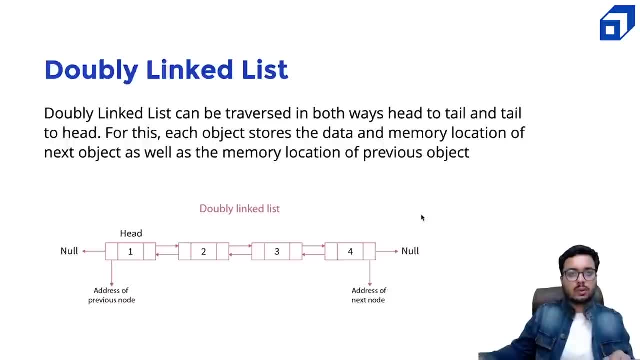 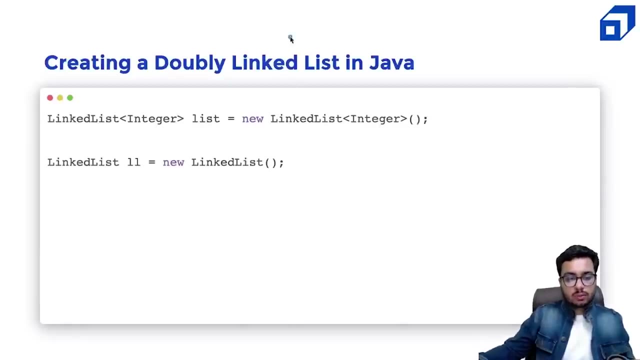 To Think Logically And You Need To Execute These Instructions In A Particular Order. So What Happens In Java, Right? So If You Want, 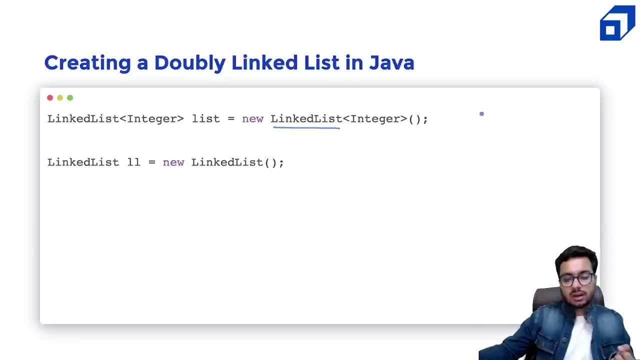 To Use This Class Inside Your Collection Framework, Then This Class Is Already Implemented. So There Is A Class Called. I Have Covered Collections In My 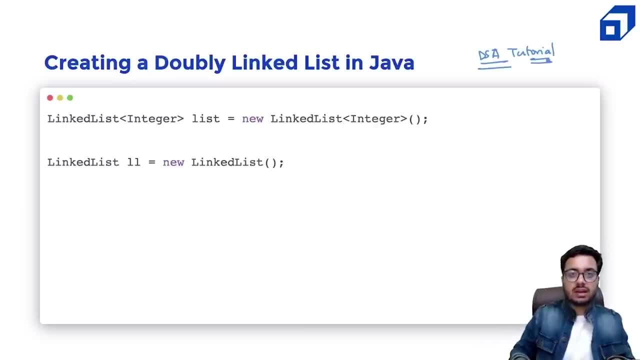 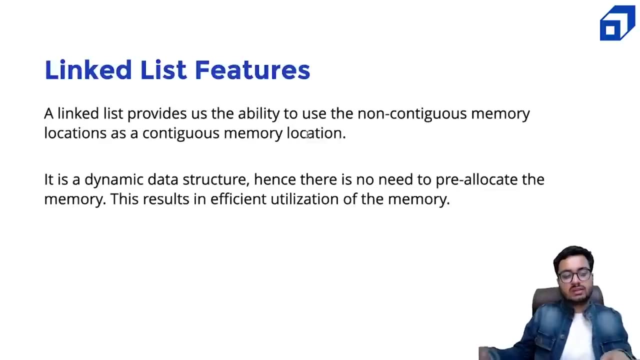 DSA Tutorial On The Channel. You Can Watch That And Learn How Do We Use The Inbuilt Double Linkless Or Inbuilt Linkless Class. 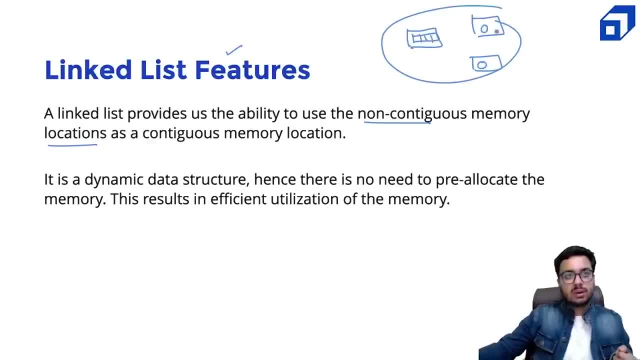 You Cannot Create A Big Array, But What You Can Do Is You Can Use Some Memory Here, Some Memory Here, Some Memory Here, And You 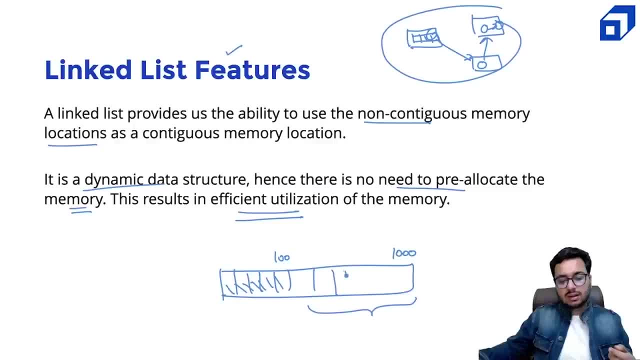 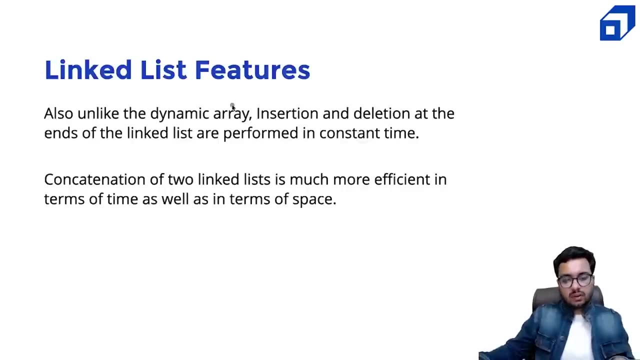 Can Just Connect To A. It's A Waste Of Memory, It's Not Efficient Utilization Of Memory. So, Linkless, You Create Memory On Demand And 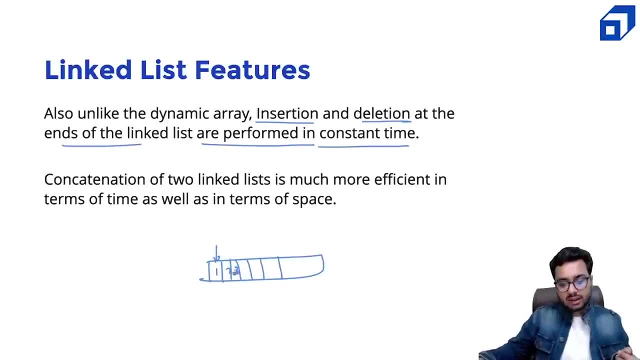 Hence You Only Use That Much Memory. That Is Something. If I Insert Something Or If I Delete Something Again, I Have To Shift All The 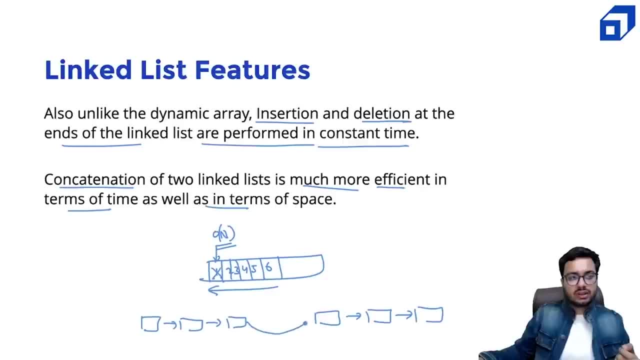 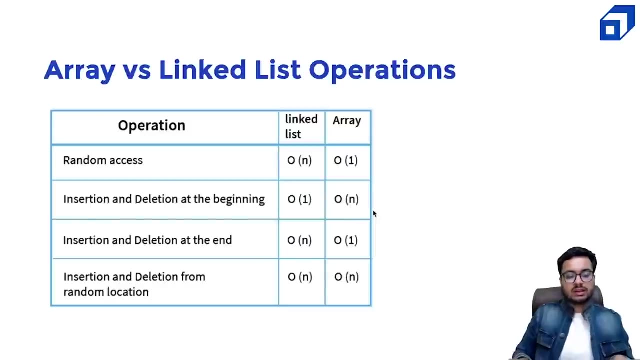 Elements Right And Joining To Linkless Is Much More Efficient. In Again An Order One Operation, So It Saves Both Your Space And Time Right. 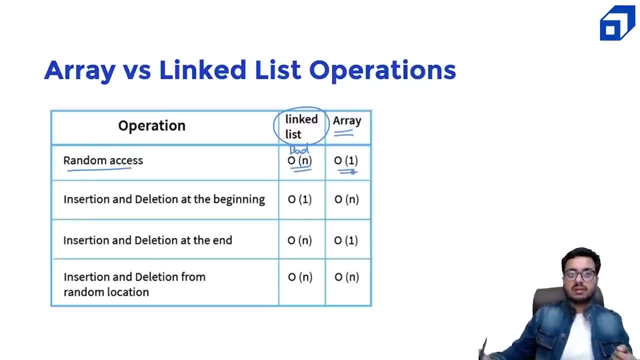 So That Is All About Linkless. So A Quick Revision On The Operations Random Access. If It Is A Double Link List, It Be It. 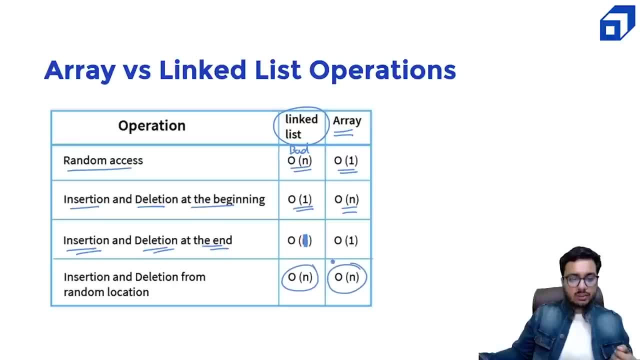 Can Be Done In Order. One Time Right In An Array. Also, It Can Be Done In Order. One Sector Has Its Own Pros And Cons. 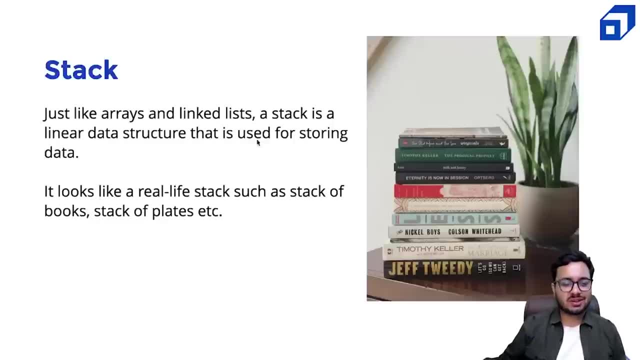 Depending On The Problem, You Have To Decide Whether You Will Go With A Link List Or An Array. Let Us Talk If You Want To. 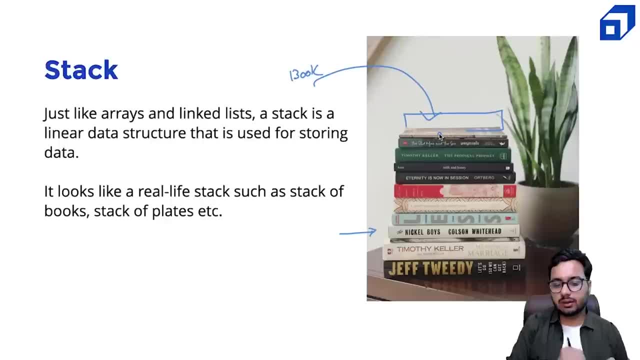 Put A Book, That Book Must Be Inserted From The Top Right. You Cannot Insert Books Directly In The Middle Right. You Cannot Insert A. 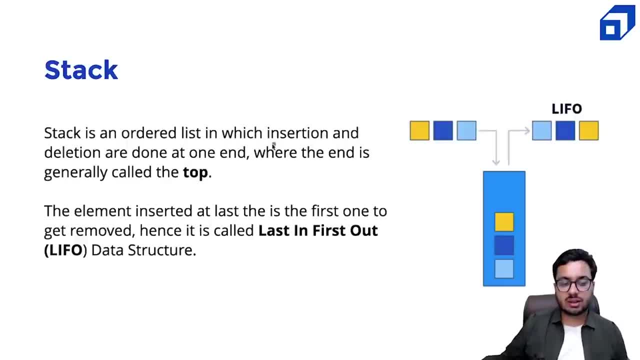 Book. Basically, It's A Data Sector In Which Insertion And Deletion They Are Done Only At The One End, Where End Is Called As. 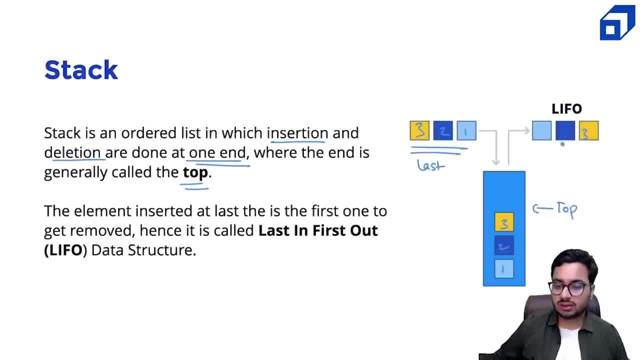 The Top Of The Stack, The Last Item Is The First One To Come Out, So Hence This Behavior Is Also Called As Last In First. 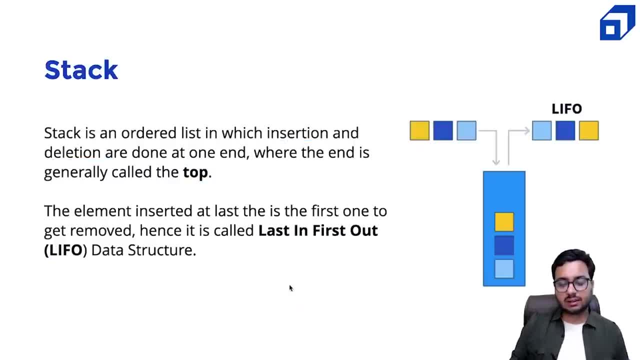 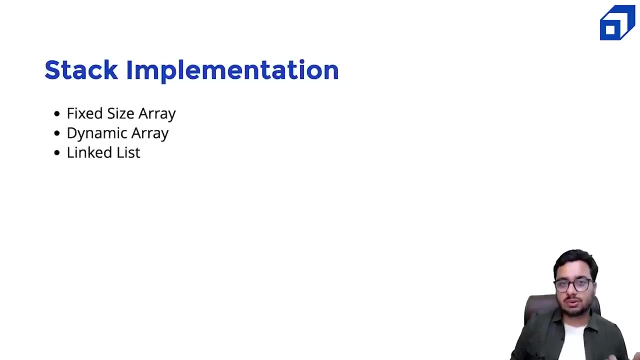 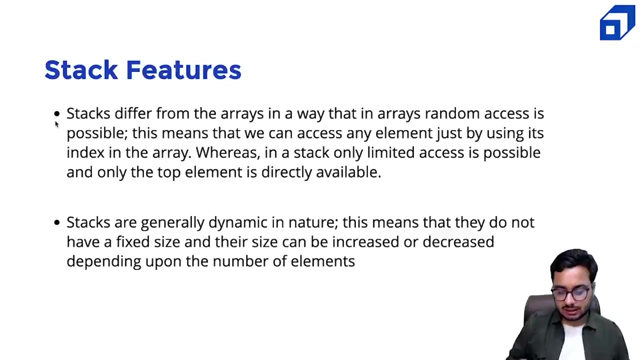 Up Right When You Do Execute These Operations With Something Like An Undo Redo Stack. You Can Do That Right, And Problems Where This Last. 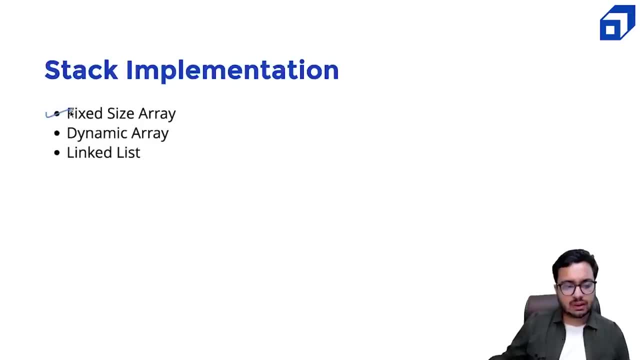 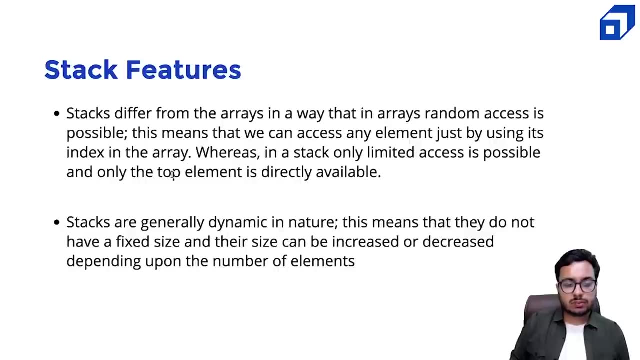 In First Out Behavior Is Important. Stack Can Be Used Here Right. So The Implementation Details Very Soon. But Before That Let Us Also Talk About 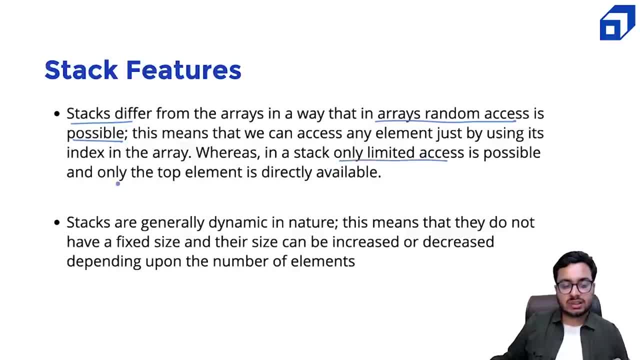 Features Of The Stack. Right: The Stacks Are Different From Arrays In A Way That Top Elements, So The Size Of The Stack Can Keep. 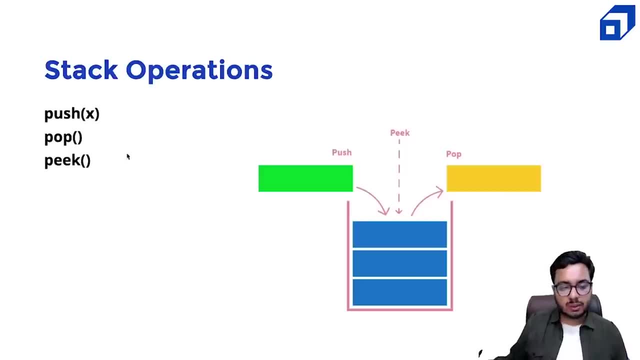 On Changing Right. So Generally We Do Not Say It's Going To Have Any Fix Size Right If You Are Looking For The Element. So 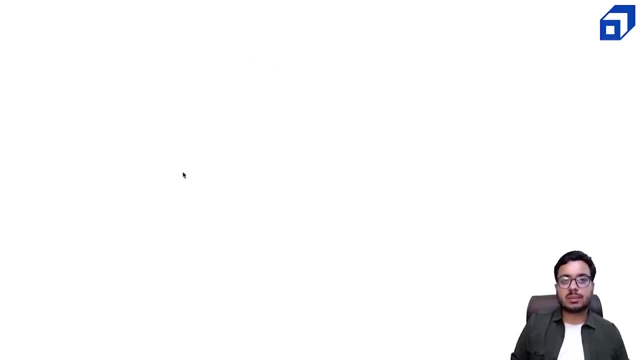 We Call It As Peak, Sometimes Also Called As A Top Right. We Want To Seek The Top Most Element That Is About, Which Can Use. 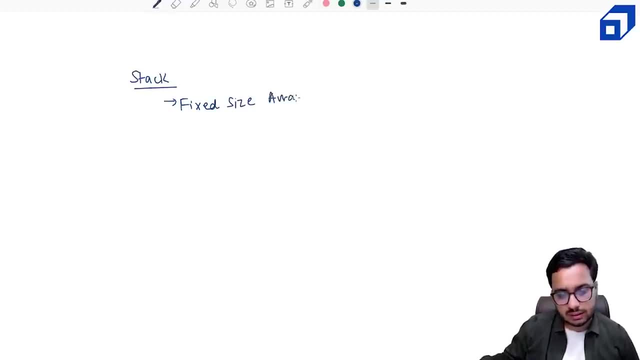 A List Or A Link List. Okay, So We Will Discuss A Fixed Size At Implementation And Another Implementation Using Dynamic Array, Which Is Called As. 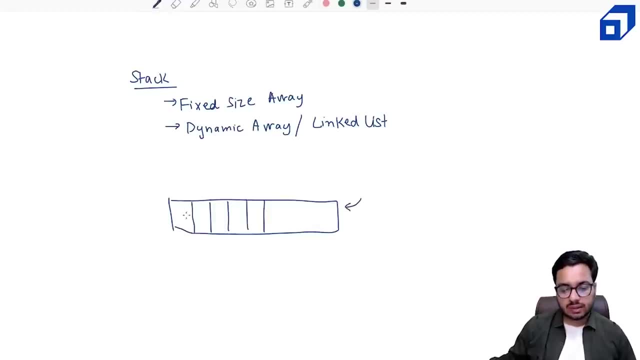 Only From One End. Right? That Means, If Is Okay, Every Insertion Will Go From Here. So One, Two, Three, Four, Five, If I Want. 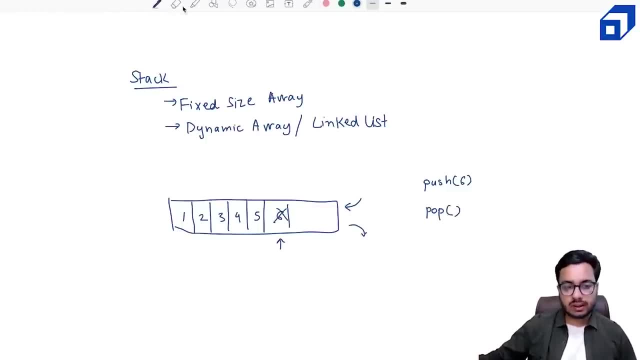 To Insert Six. I Would Like To Implement That. Okay, I Want To See What Element Is At The Top Of The Stack. So If You 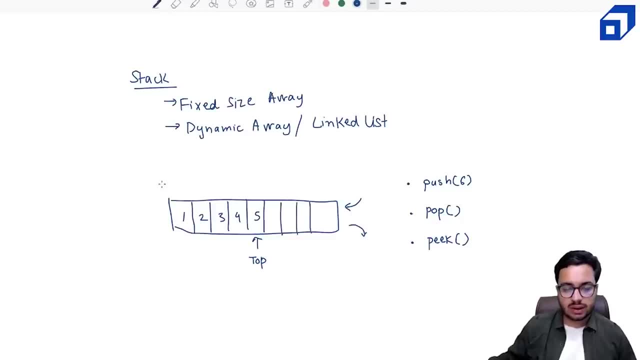 Remove Six, And We Call This Method Fix Size, And We Can Add Elements From This End Of The Array. So Let Us See How We 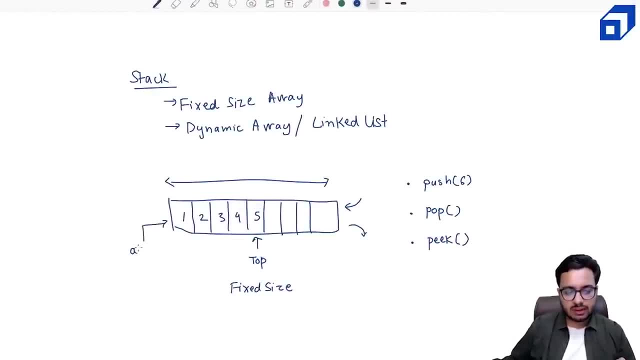 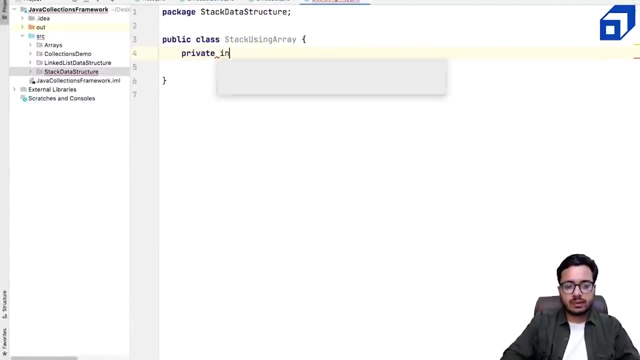 Can Implement A Stack Class In Our Code. Let Us See What Is The Maximum Capacity Of The Stack. Right. What I Will Do, I Will. 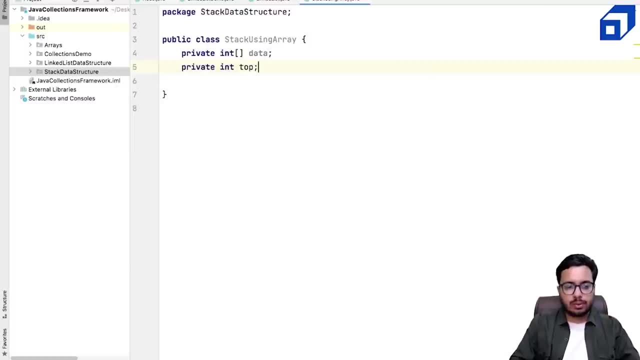 Define These Three Attributes As Data Members Of The Class. First Thing I Need To Define The Default Capacity Right, And This Is Equal To 10.. 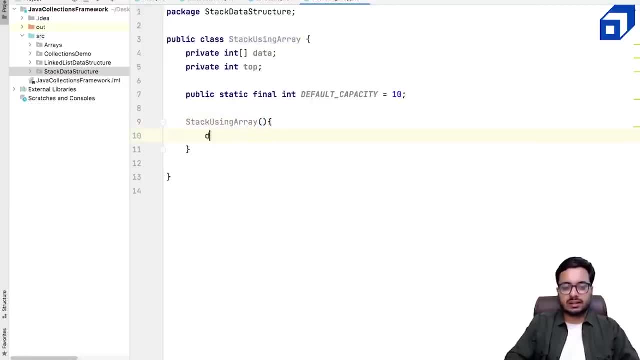 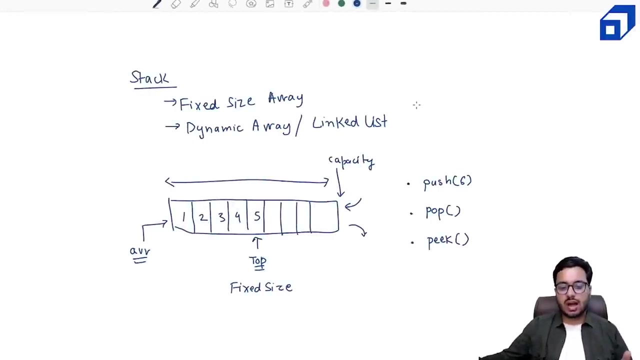 Right Now I Need To Define A Constructor. I Can, Okay, Start Using An Array. There Is At Which I'm Going To Store The Element. 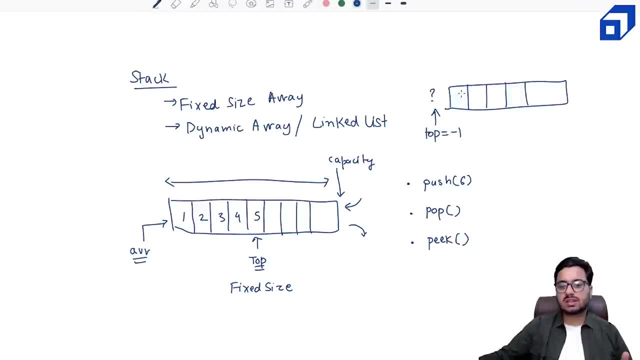 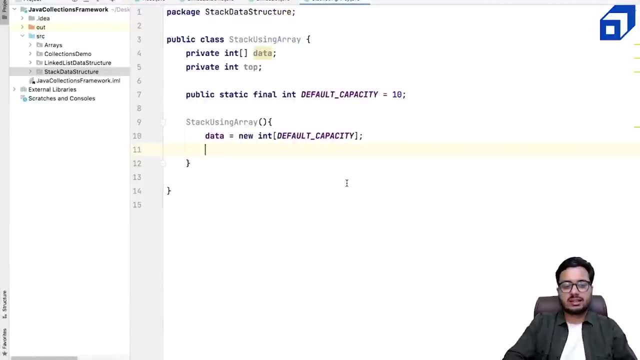 At Which I'm Stored, The Last Element. So In The Beginning I Can See My Top Is At Minus One User Input, So I Can. 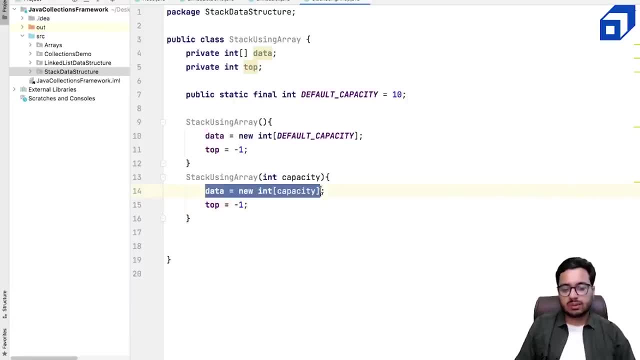 Define, I'm Getting Some Capacity. So In This Case I Can Say: Okay, The Array That I'm Creating, It Has This Particular Capacity Right. 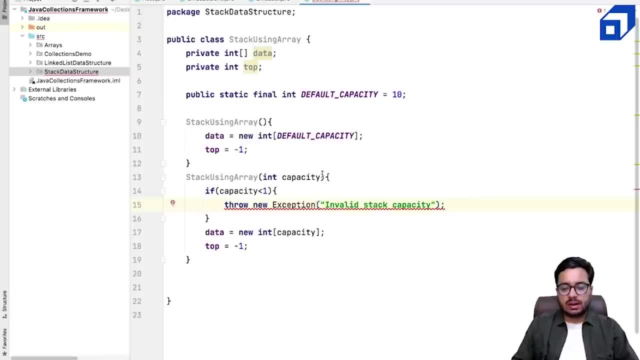 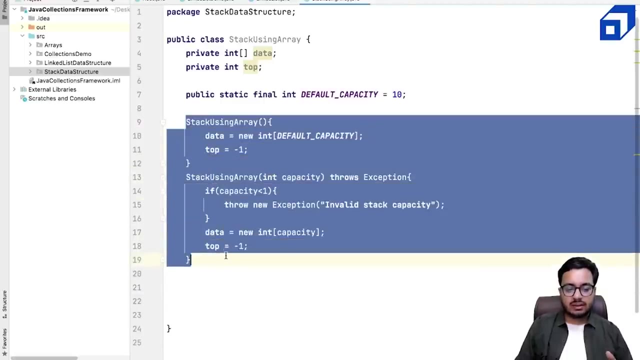 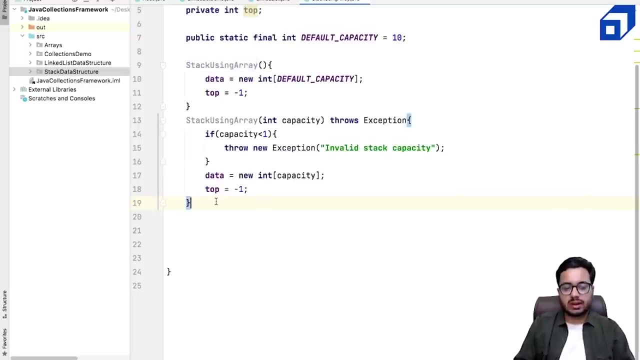 Or We Can Do, And Here We Can Say: Okay, This Function Can Throw An Exception, Those Exception. This Is How We Will Create The Contractor. 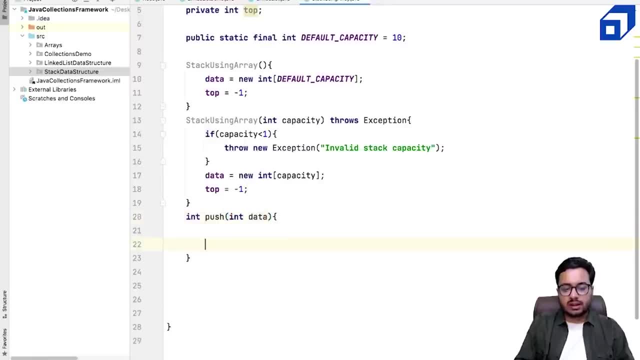 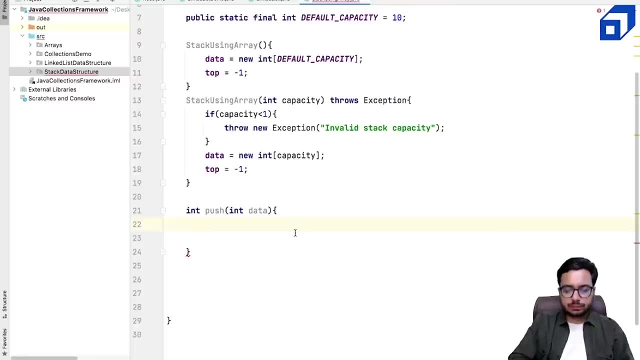 For The Stack Class Right, Whether My Stack Is Full Or Not. Only I Can Push Right. How Do I Check? How Do I Check Right? 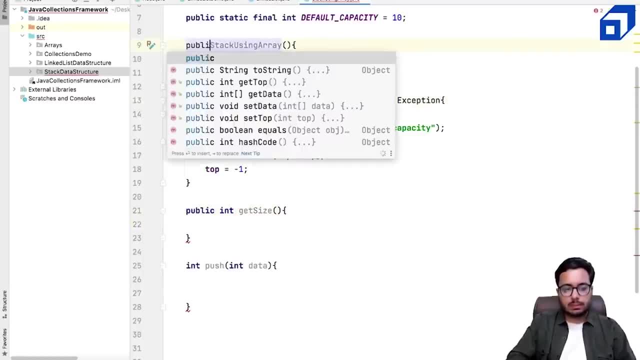 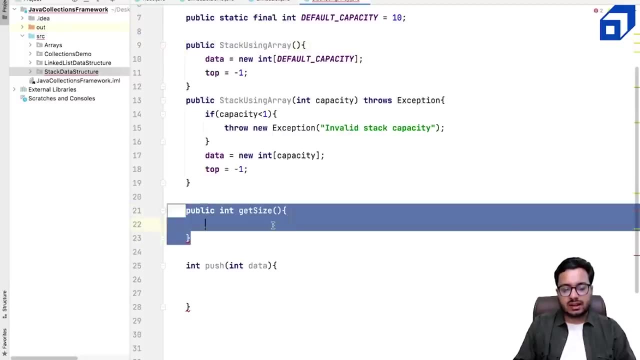 Let Me Do One More Thing. Let Me See What Is The Current Size Of The Stack. Can I Say The Current Size Is Nothing But. 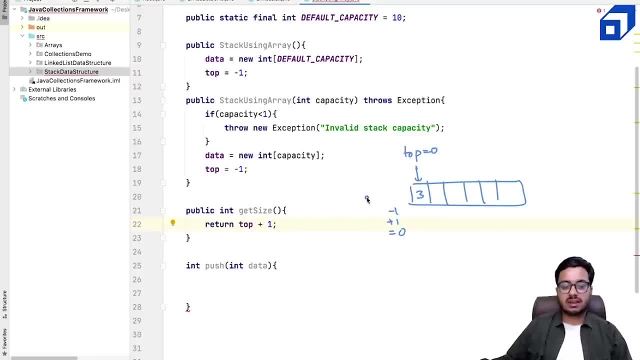 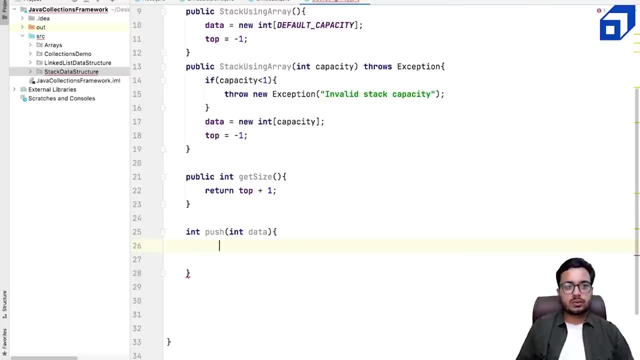 The Value Of Top Plus One. So In The Beginning Top, Let Do Just Think About It. Okay, So What We Can Do Is We Can. 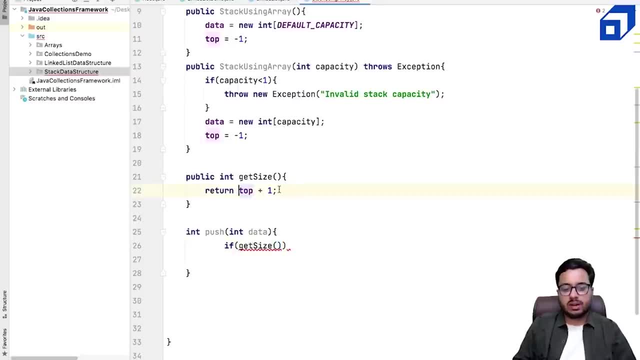 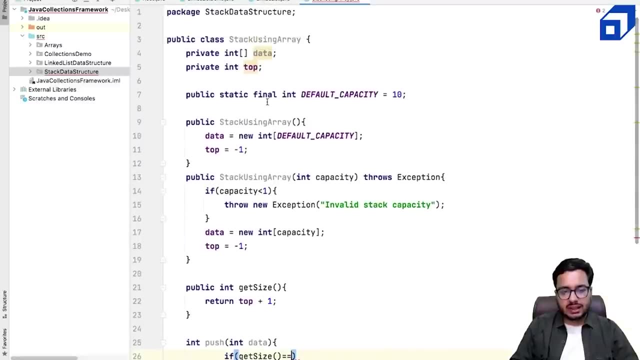 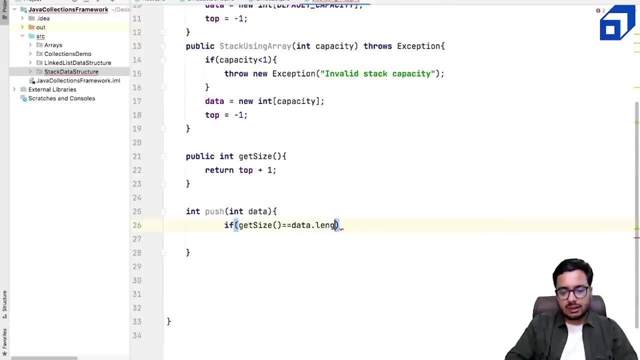 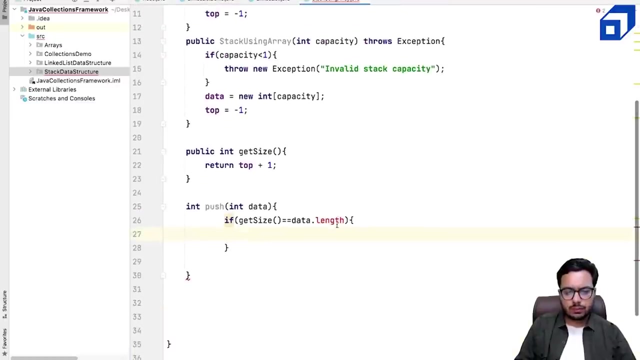 Check That. Whatever Is The Current Size Of The Stack, Is It Equal To Length, Right? So Array Has A Property Called As Length, If These 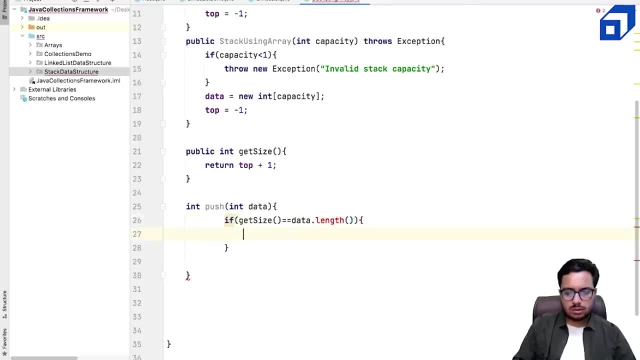 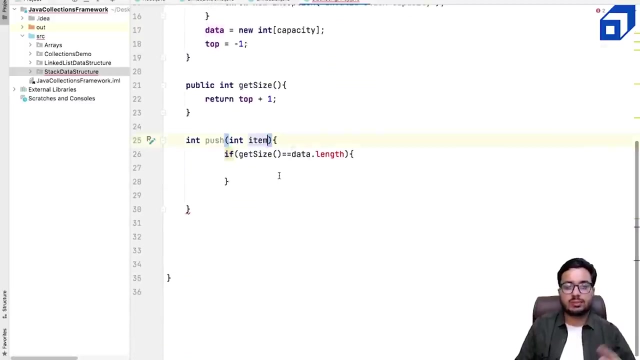 Two Are Equal. That Means My Array Is Already Pulled, Okay, So We Are Getting An Error Here And Data Is Also An Array Here. 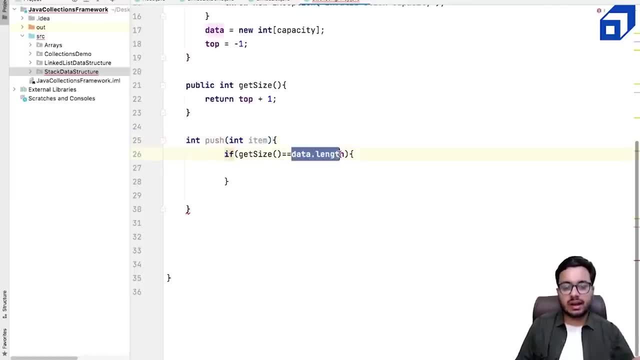 Right, I Need To Make It Something Different. I Need To Say: This Is Some Item That I'm Pushing Into The Stack Exception, All Right. 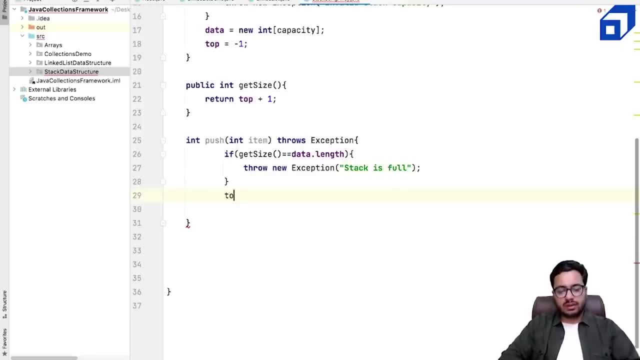 But If This Is Not The Case, So What I Will Do? I Will Increment My Top Also Define: Increment The Signature. Now What Is Happening? 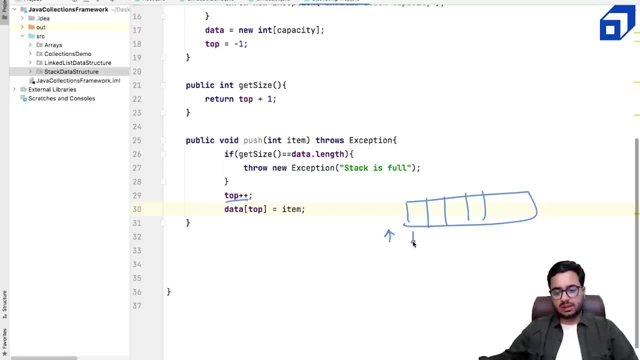 That Your Top Was Here, I Said: Push 3.. To My Top Comes Here And I Put The Item. I Said: Push For My it's a six, seven and the capacity of there is also five. so if it is there so i can say stack. 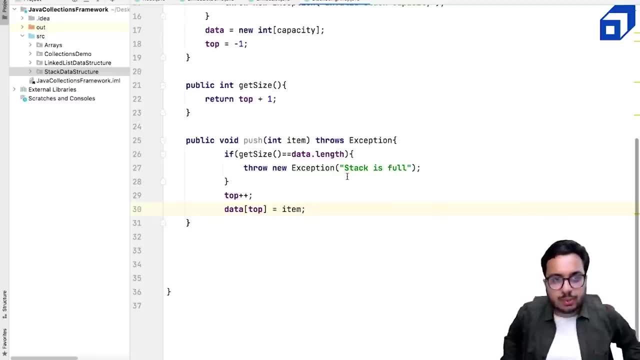 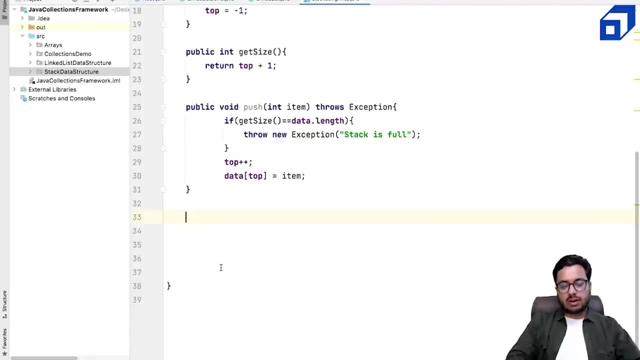 is full right. so that is how we can perform the push operation on the stack. right now. let us talk about how do we remove something from the stack. right now i can say, uh, i will have public int pop. okay, i want to remove the topmost item. so again here what you can do. you can make a check. 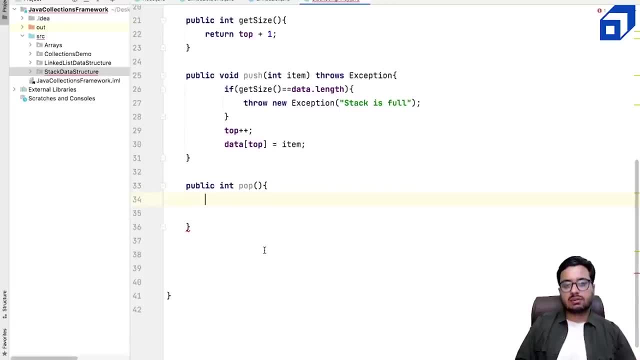 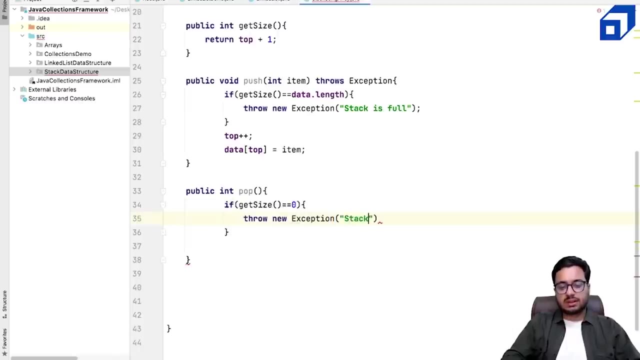 that if my stack is empty right, then i have to throw an exception. i cannot uh pop from an empty stack. so if get size tells me, okay, this size is zero, there are, there is no data in the stack, so you can say, uh, throw new exception. stack is empty, right, and here we can say this method: 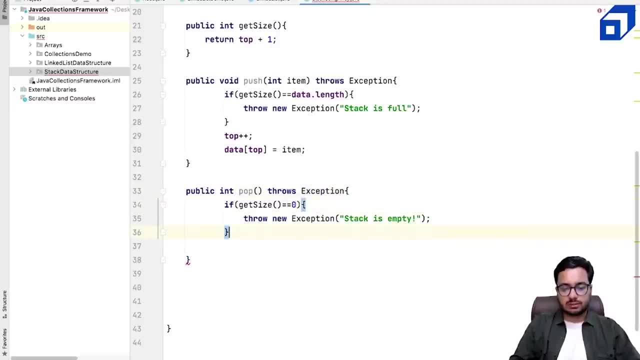 throws exception right? okay, if this is not the case, i can easily remove something from the stack. i will store my answer, so i answer that i want to return. it will be a data of top right. what i can do: i can reduce top top minus minus and i can return. 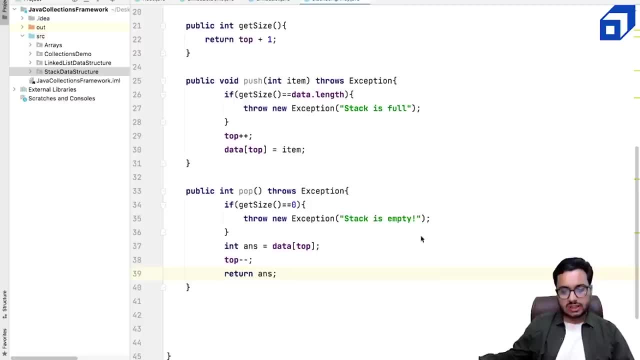 the answer that i have. let's see what we are really doing. so we are saying, okay, one, two, three, four, this is my top, right? i want to remove this. so i can simply say, okay, this top will come here and i will copy this four in a variable called answer and i will return it. right, you might say: 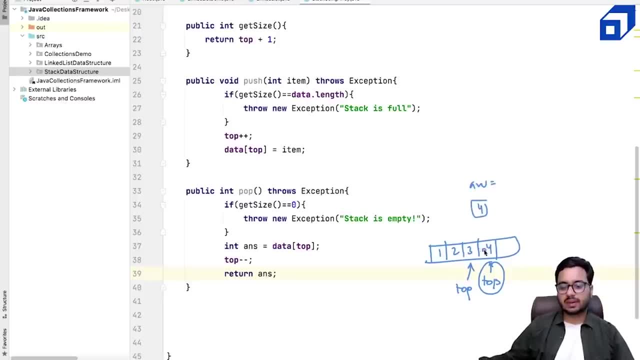 okay, if i print the stack i might see four. that's not going to be true because we will only print up to one, two, three, right up to top right this data. if you want, you can make it zero or you can keep it as it is right. so just to make it little more more clear, i can say: answer of top, i'm making it. 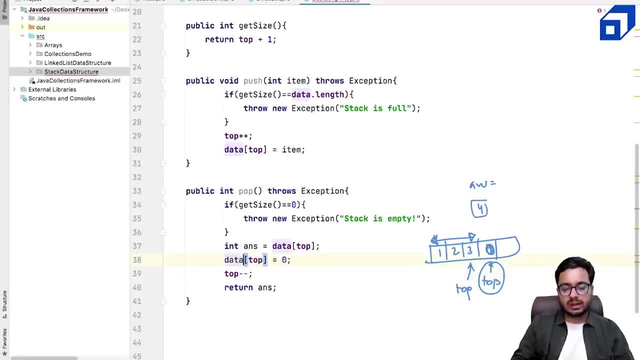 zero, so that, oh sorry, rate of top. i'm going to make it zero so that it looks good when you try to uh, look at the entire array. right, so i'll. so in general, you are not going to look at the whole array, but only the array delta top. but that's okay. so this is. 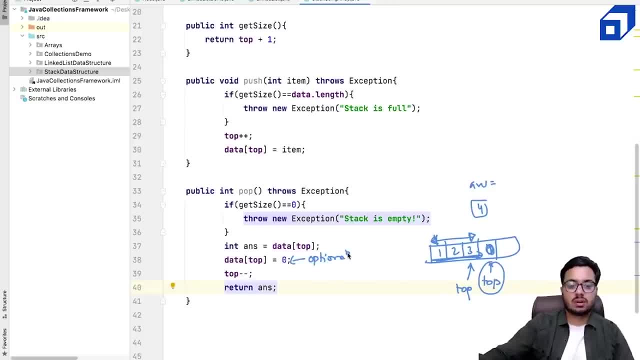 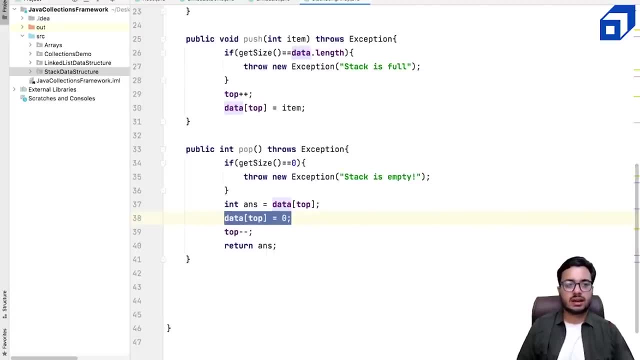 an optional step if you would like to do right, because data can be zero, also right. so, again, this is an optional thing if you want to. that is how you will remove something from the tank. right now we have the method to look at the topmost element, right? so sometimes this method is called: 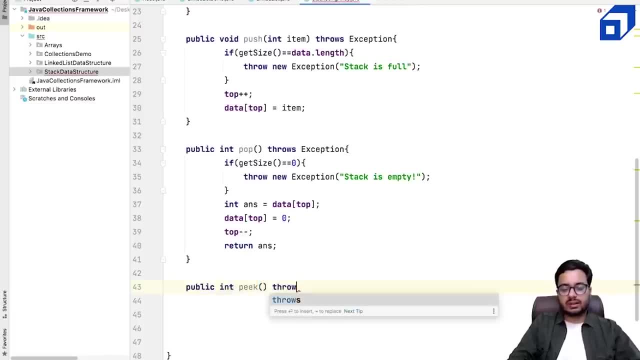 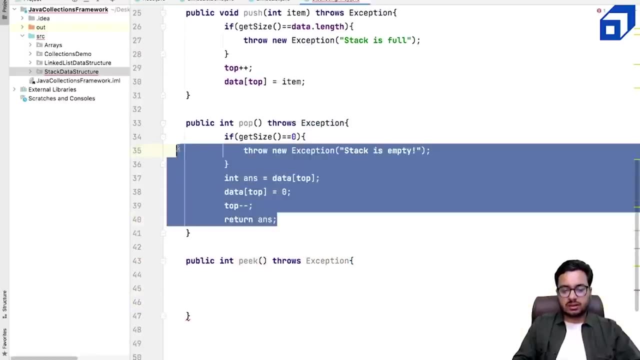 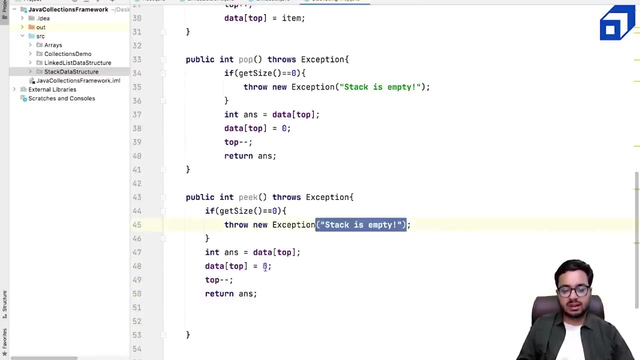 sometime it is called as peak, right? if you want to look at the peak method? uh, it's pretty easy. you just need to do the similar thing, right? so it's okay. if the array is empty, then you can throw a new exception. that stack is empty. otherwise, 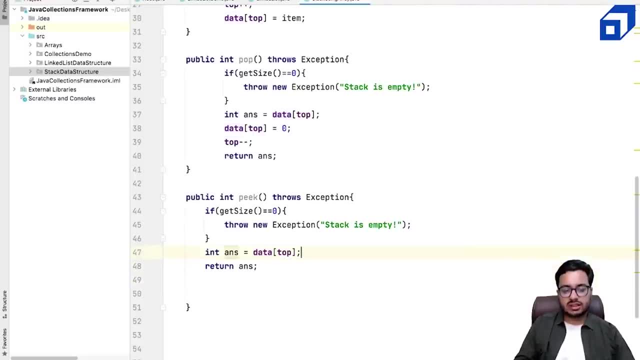 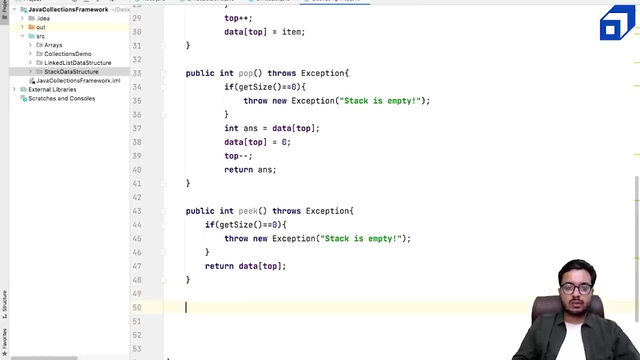 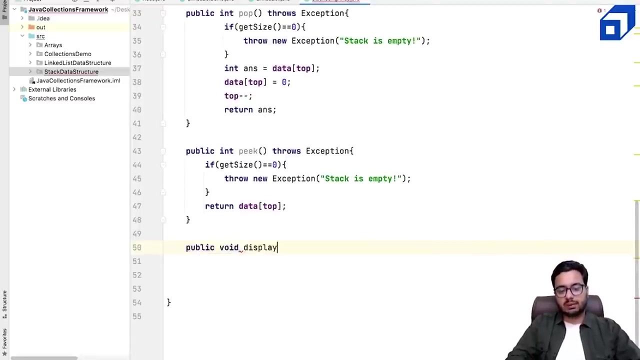 you get the data but you don't remove it. so that's it. you can, or you can, simply return data off top. okay, the topmost element you can return directly. so that is your peak method. right, let us add some more methods. if you want to print the stack, so i will print everything up to top right. public void display. 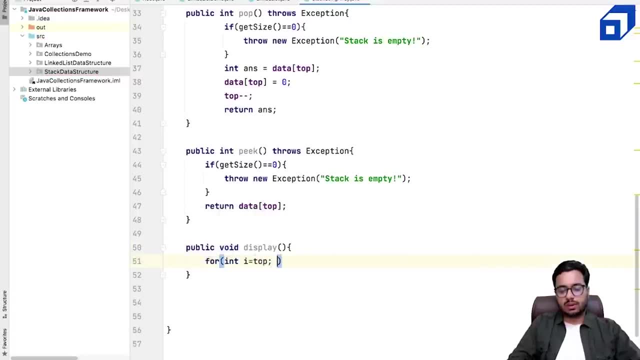 so i can say: for int, i equal to top, i greater than equal to zero, i minus minus. so i will iterate on the items in the reverse order. so if it is like one, two, three, four, i will first. okay, i'm going to print from top to the bottom right like this. so 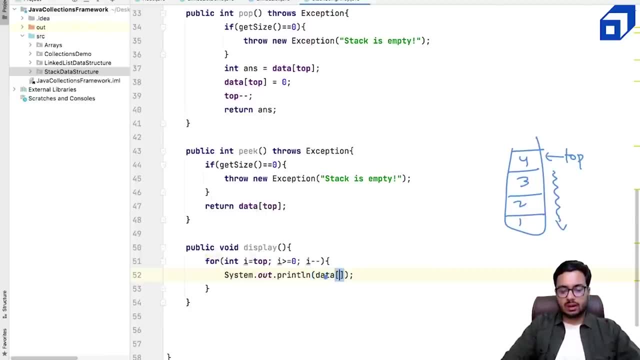 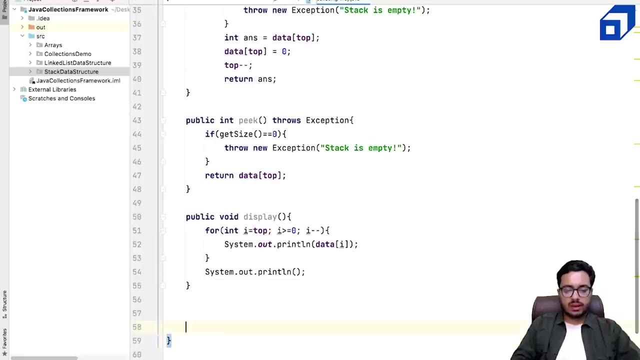 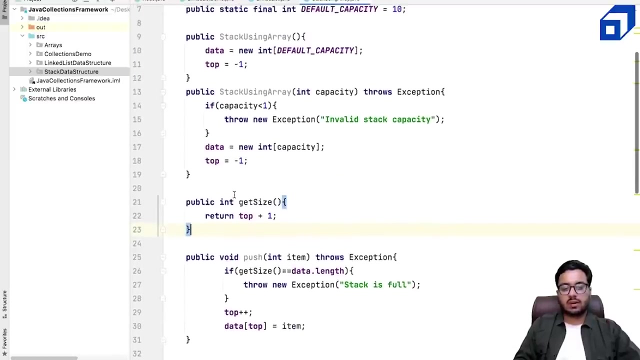 what i will do is okay s out data of i. that's it right. so that is my display method and i can give a new line here. okay, so any other methods if we would like to write. so maybe we want to write a method called as is empty or is full, so we can write those method as well. 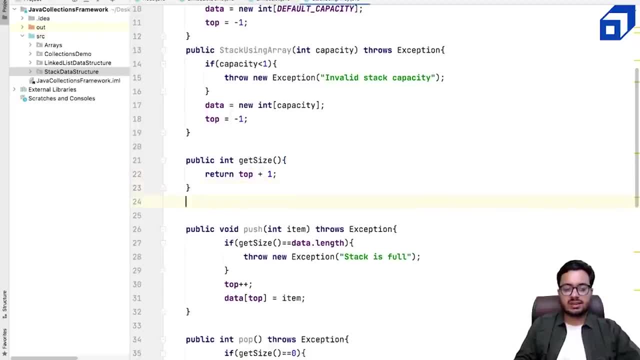 so i i can. i will write is empty method whether the stack is empty or not. so i can say: public int, public boolean is empty. so this is helpful when you want to continuously remove elements from the stack until the stack is not empty. so this method can be used right now. i can return if my get 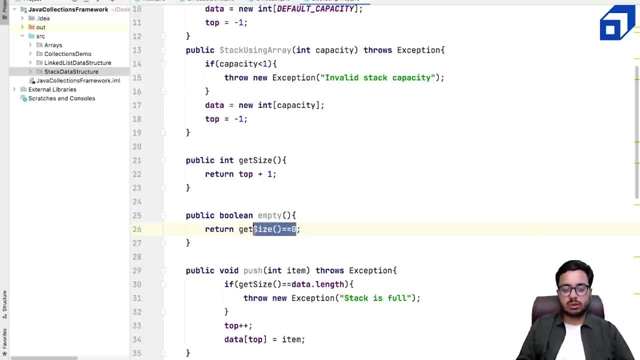 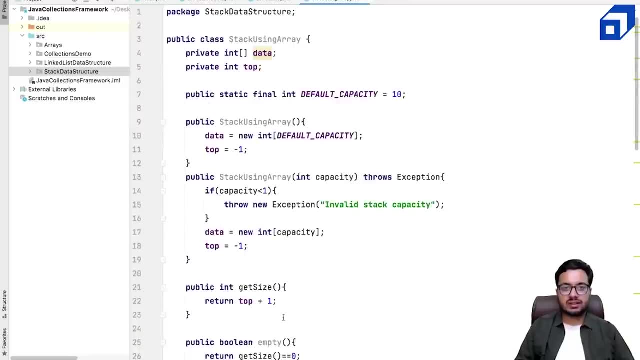 size is equal to zero, so this expression will evaluate to true or false. so i think this looks good. next, we will test the functionality of this stack that we have created. now let us write one more class so that we can test the functionality of this stack class. 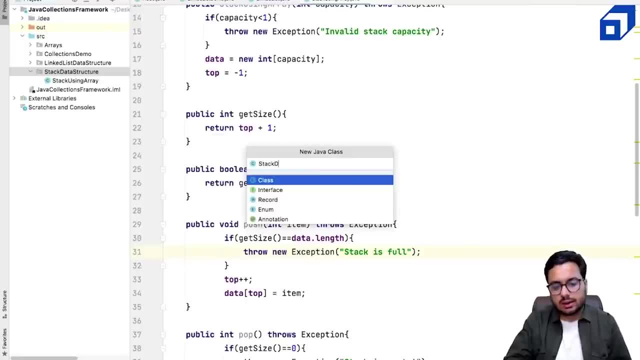 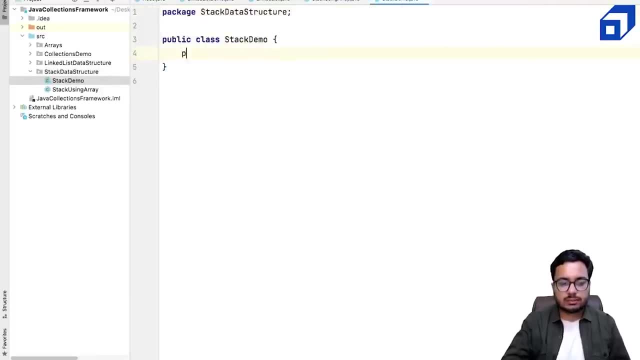 so i'll call it as a stack demo. dot java right. so in this start demo we will create a stack object. so main method is there. i can just stack s. sorry, this should be dark. using an array right tag. using an array, i call it as stock. this is equal to new stack. new stack using an array right. 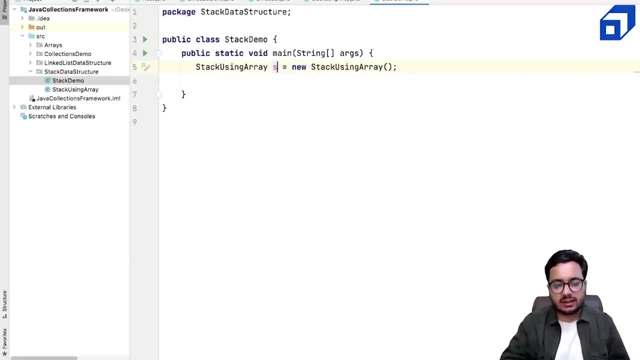 so i've created the stack object, or just call it as s. let us push some numbers into it so i can say: s dot push one, s dot push two, uh, s dot push three. so we have to push. method can throw an exception so i can say: 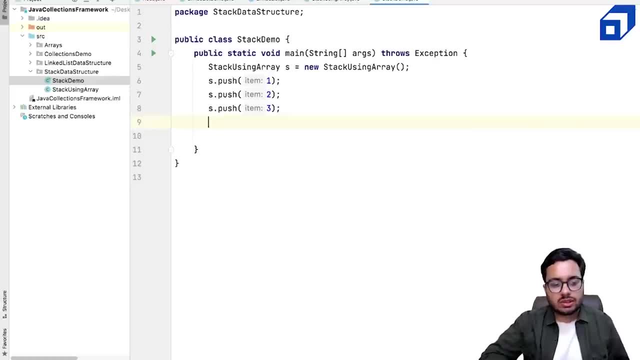 main can also throw an exception. so s dot push three, four, five, whatever it is right, and then we can try to extract items from the stack. so four, five, six, i've added six items. i can say, okay s dot display, show me, uh, the stack height. let us run this. 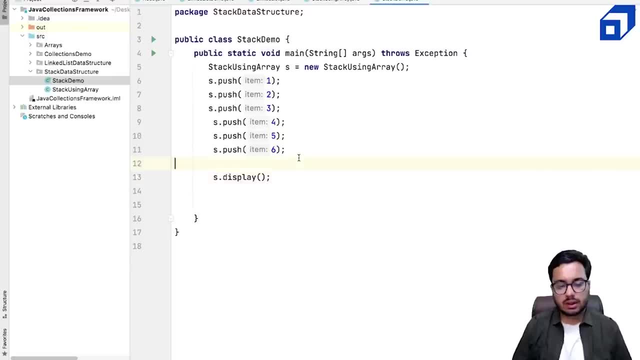 and see what do we get right. and at the same time, i will do one more thing: i will pop items from the stack until the stack is not empty. so, while the stack is not empty, what i will do? i will give me the topmost element so i can say: s dot, peak, print the topmost element, so s out, uh, topmost element. 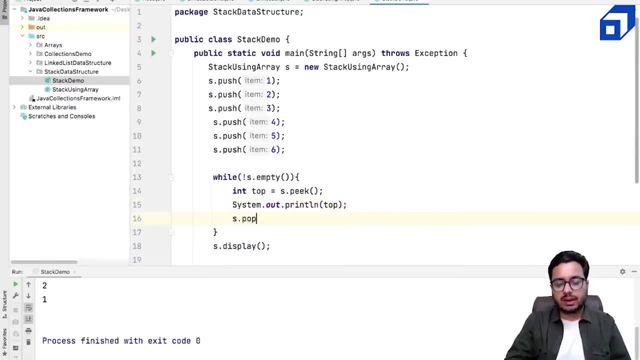 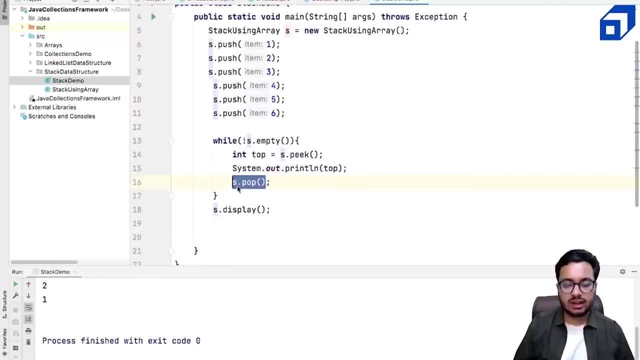 and remove it. so i can say s dot pop, right, a pop function you can also use, uh, because it also gives you the element, and remove it right. but here we are not reading the value from the pop, we are just reading the value from the peak function. so when we are printing it, you see six is at the top. then 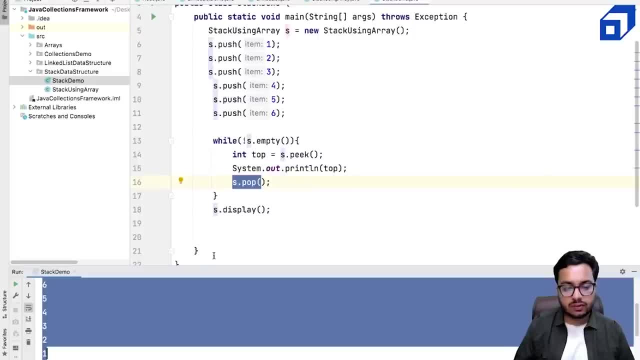 five, then four, then three, then two and then one. right, if? if i do not call the display method, instead i use this while loop, what is the first element that will get removed? that will be six, and then i will remove it, so i can say s dot, pop, and then i will remove it so i can say s dot. 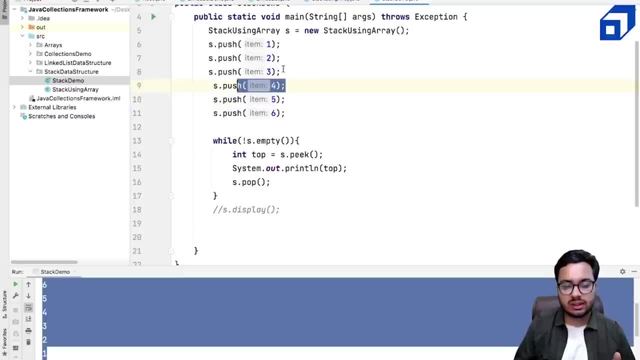 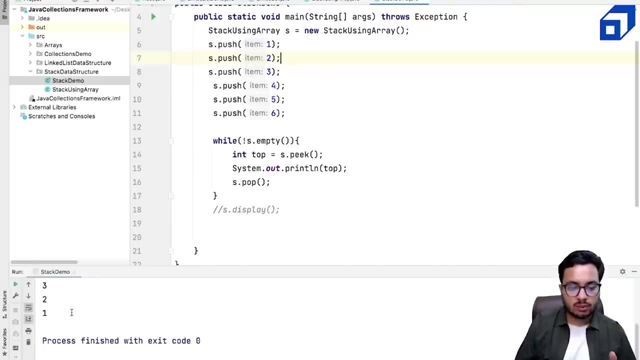 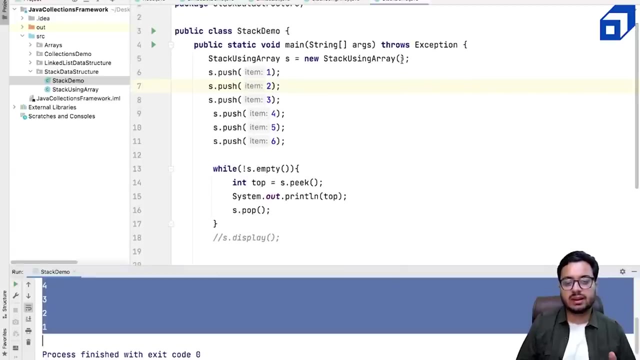 last in, first out, then five, then four, then three, then two and then one. let us go and run this code and we will get a same output by removing all elements from the stack as well. right, so you can see. that means our class is working perfectly fine. by default, the capacity is 10. 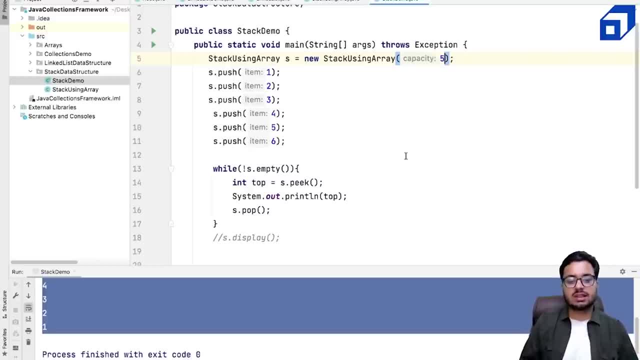 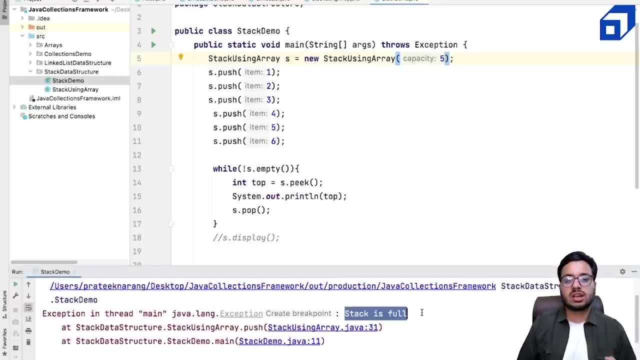 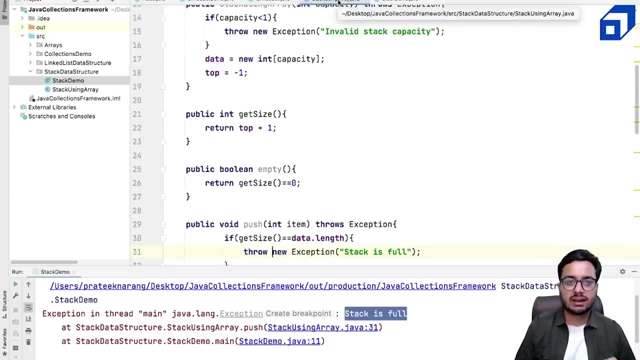 if i show the capacity is five and i try to insert six elements, then this code is going to throw an exception that the stack is already full and i can not push any more elements into the stack. the next implementation of stack we will see using a dynamic array and a linked list. let us talk about dynamic stack. 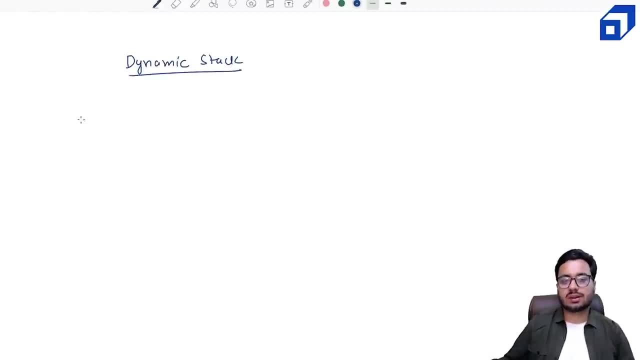 now there are two options to implement it. one is you can use an array, or one is you can use a linked list. so when i say array, we can use a dynamic array, right? so suppose you are implementing the stack using an array and at some point your array got full, okay? your array got full, so you can use a dynamic array. and at some point your array got full, okay, your your array got full, so you can use a dynamic array. and at some point your array got full. okay, your current size is equal to capacity, right? current size is equal to capacity, right. 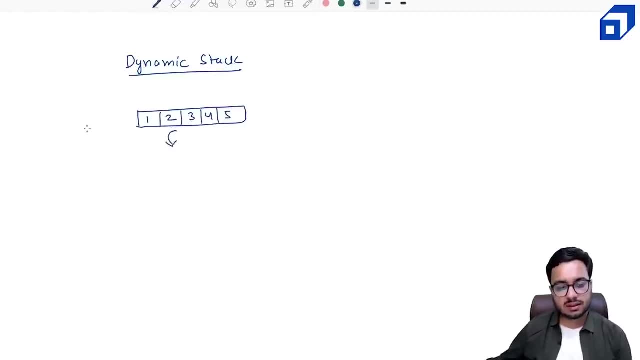 current size is equal to capacity. right, what you can do is using the same logic as. what you can do is using the same logic as. what you can do is using the same logic as array list, array list, array list inside your push method. what you will do: you. 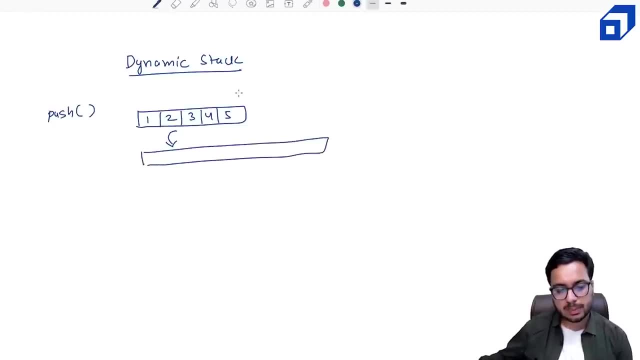 inside your push method, what you will do, you, inside your push method, what you will do, you will define. i will create a new array, will define, i will create a new array, will define, i will create a new array of double the capacity, if this is c. of double the capacity, if this is c. 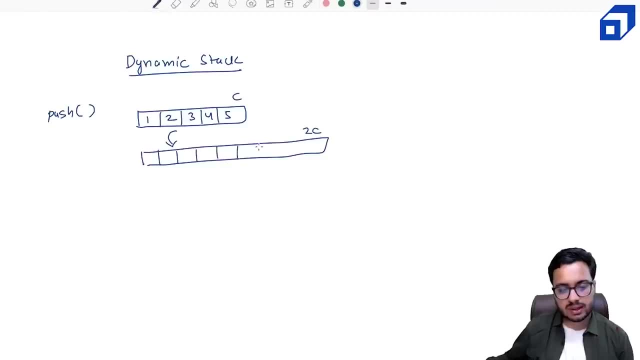 of double the capacity. if this is c, i will create an array of. i will create an array of. i will create an array of 2x of my capacity, 2x of my capacity, 2x of my capacity, and i will copy the elements here. 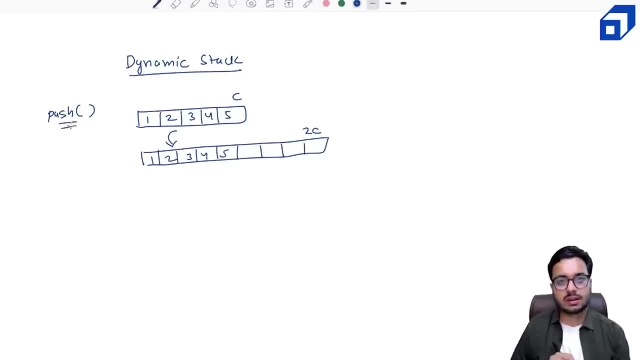 and i will copy the elements here. and i will copy the elements here: right, right, right. that is how my push method will. that is how my push method will. that is how my push method will get changed right and pop will remain. get changed right and pop will remain. 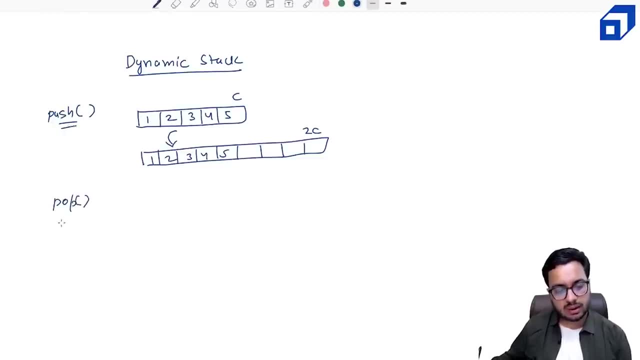 get changed right and pop will remain same. i am not going to shrink anything so same. i am not going to shrink anything so same. i am not going to shrink anything, so pop will remain same. pop will remain same. pop will remain same. even the top method will remain same. no, 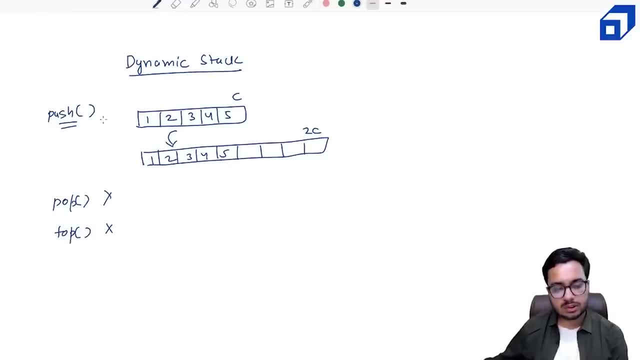 even the top method will remain same. no, even the top method will remain same. no changes changes, changes right. nothing changes here, only in the right. nothing changes here, only in the right. nothing changes here, only in the push method. we are going to change push method. we are going to change. 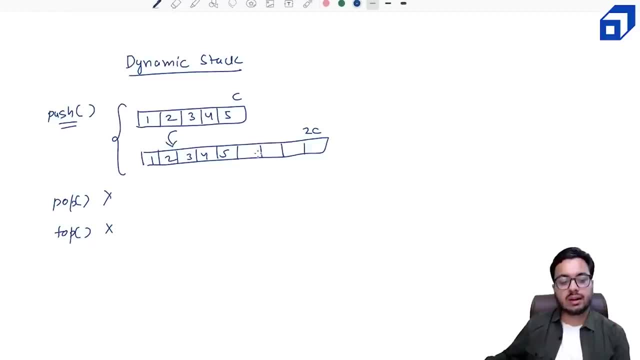 push method we are going to change. error will not overflow, instead it will. error will not overflow, instead it will. error will not overflow, instead it will get, get, get a doubled right. and again this copying, a doubled right, and again this copying a doubled right, and again this copying is an expensive operation, right? so we? 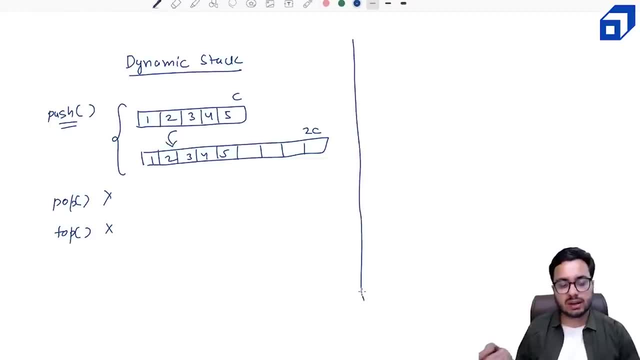 is an expensive operation, right, so we is an expensive operation, right, so we should make sure that this is not, should make sure that this is not, should make sure that this is not happening. happening too frequently right happening. happening too frequently right happening happening too frequently right. that is why initial capacity is. 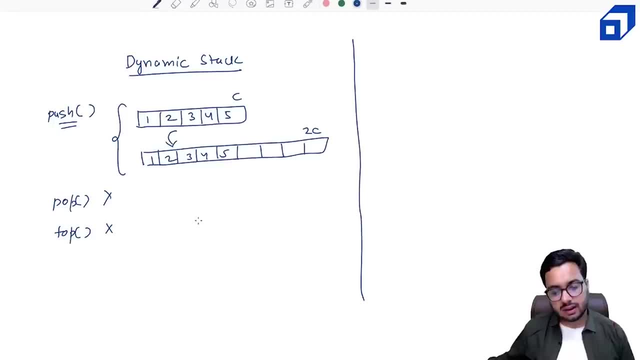 that is why initial capacity is. that is why initial capacity is important, right so that is important, right so that is important, right. so that is using an error list right now, if you using an error list right now, if you using an error list right now if you want to discuss it in the code, so you 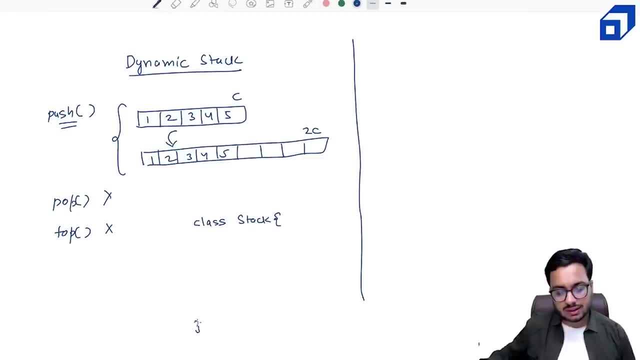 want to discuss it in the code. so you want to discuss it in the code, so you can. okay, i have a class called stack can. okay, i have a class called stack can. okay, i have a class called stack. so either you can keep a error list so, either you can keep a error list. 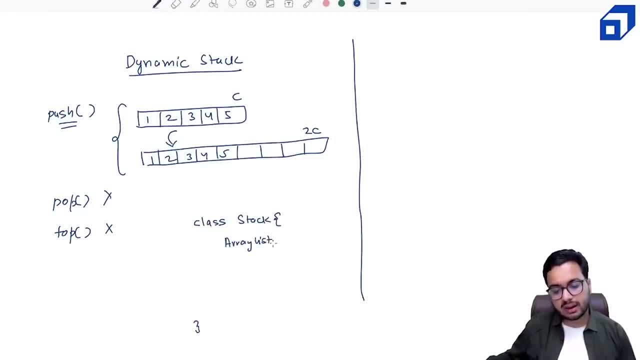 so either you can keep a error list- object here right, object here right. object here right- because we have already implemented, because we have already implemented, because we have already implemented error list. it can be your error list. it can be your error list, it can be your implementation. it can be library based. 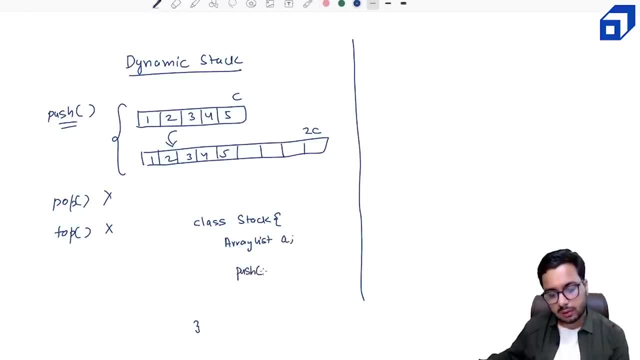 implementation. it can be library based implementation. it can be library based implementation as well. whenever you go implementation as well, whenever you go implementation as well. whenever you go get a call for push, get a call for push. get a call for push, some item i, you can simply say: okay, a dot. 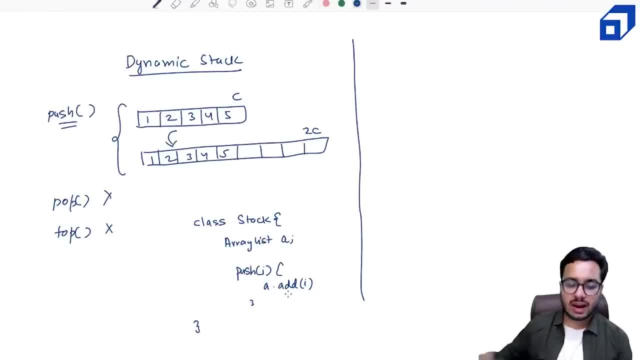 some item i. you can simply say, okay, a dot, some item i. you can simply say, okay, a dot, add item. i so add function. we know it add item. i so add function. we know it add item. i so add function. we know it adds. at the end of the array list the. 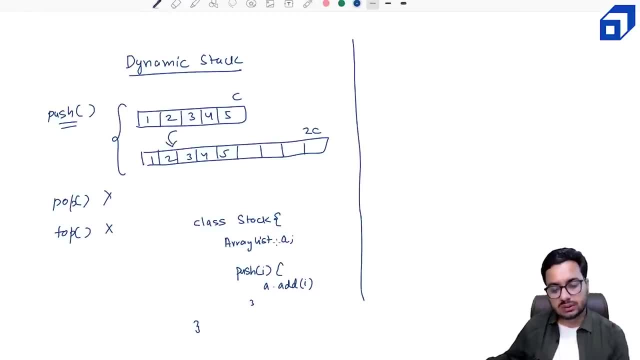 adds at the end of the array list, the adds at the end of the array list, the code becomes even simpler right, or if code becomes even simpler right, or if code becomes even simpler right, or if you don't want to use. you don't want to use. 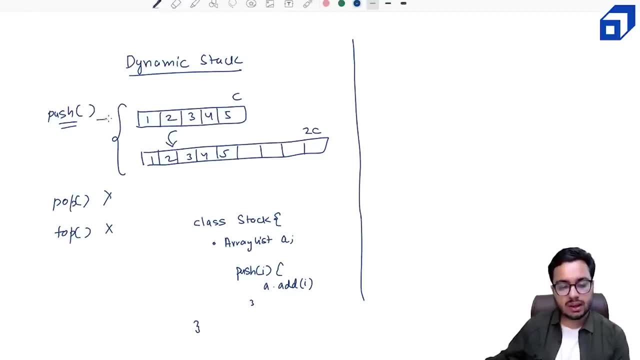 you don't want to use the inbuilt class, right. what you can do- the inbuilt class right. what you can do the inbuilt class right. what you can do. you can take the manual array like we. you can take the manual array like we. you can take the manual array like we did in the previous example. 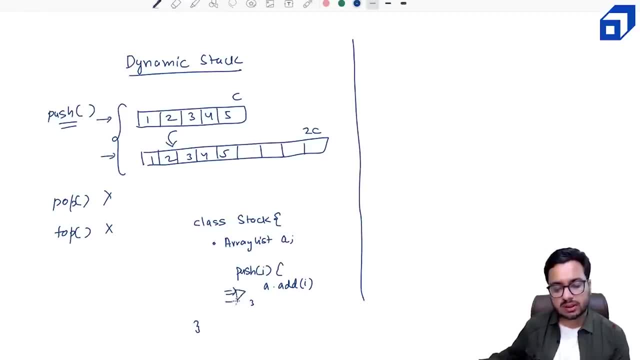 did in the previous example, did in the previous example and write the doubling logic inside the and write the doubling logic inside the and write the doubling logic inside the push method. so i'm hopeful that you will push method. so i'm hopeful that you will push method. so i'm hopeful that you will be able to do that part right. 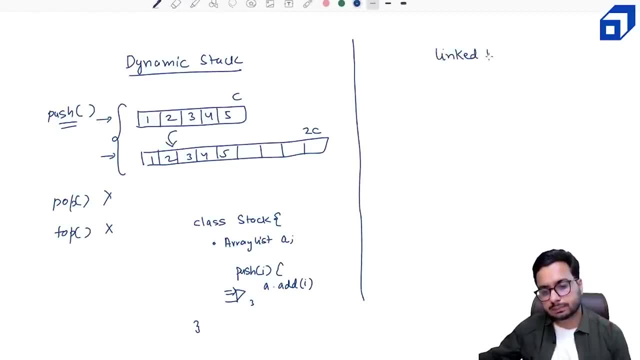 be able to do that part right, be able to do that part right. another option is you can use a link list. another option is you can use a link list. another option is you can use a link list. also right, also right, also right. i suppose we are building a stack i got. 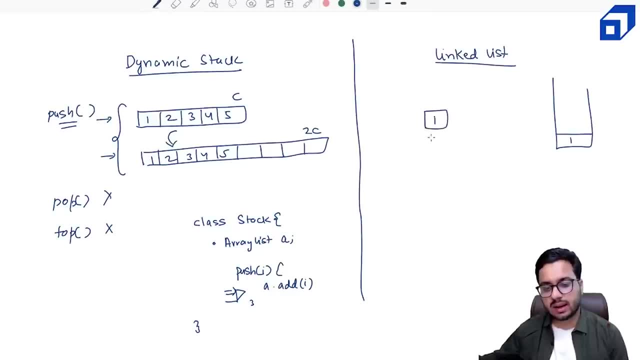 i suppose we are building a stack i got. i suppose we are building a stack. i got one one one. so i insert that node into the link list. so i insert that node into the link list. so i insert that node into the link list. my head is updated. 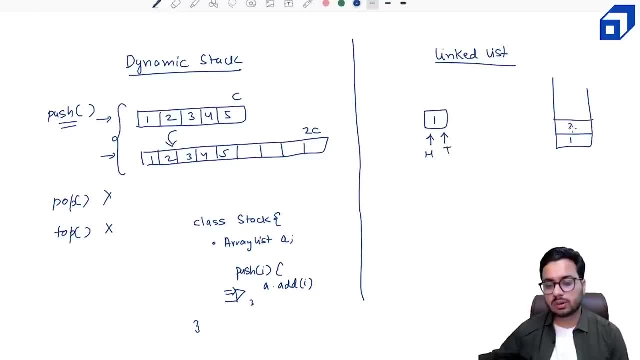 my head is updated. my head is updated. tail is also updated right now. suppose you, tail is also updated right now. suppose you tail is also updated right now. suppose you you got two now. the question is: where you got two now. the question is where you got two now. the question is: where should i insert two? should it? should it? 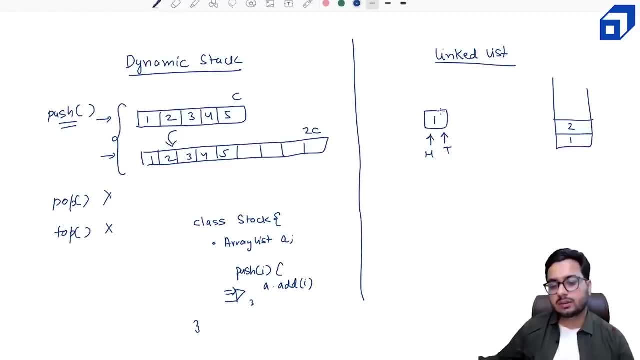 should i insert two? should it should it? should i insert two? should it? should it go at head or should it go at go at head? or should it go at go at head or should it go at tail right? one option is okay if i put tail right. one option is okay if i put. 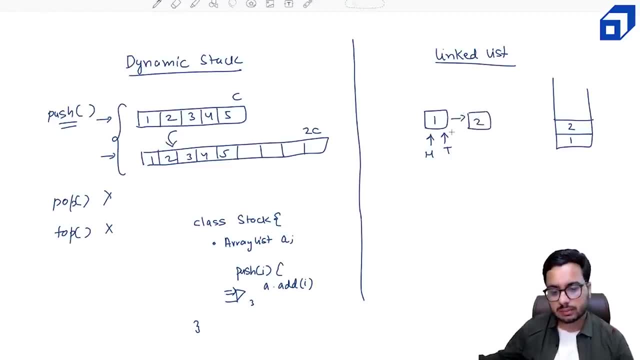 tail right. one option is okay: if i put it at tail, it at tail, it at tail, insert at tail. if i do it, insert at tail. if i do it, insert at tail. if i do it, this tail will go here. right, this tail will go here right. 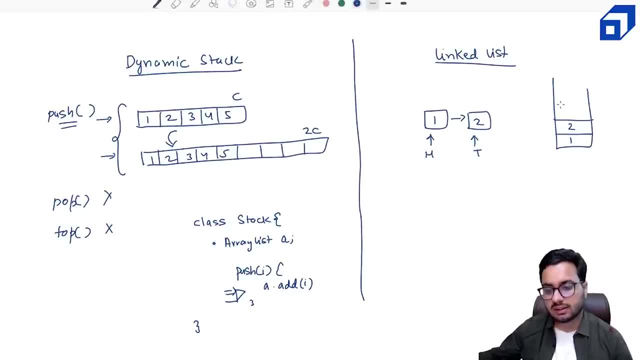 this tail will go here, right, okay, and suppose i got three, then you okay, and suppose i got three, then you okay, and suppose i got three, then you can again insert, can again insert, can again insert. it at tail, this tail will go. it at tail, this tail will go. 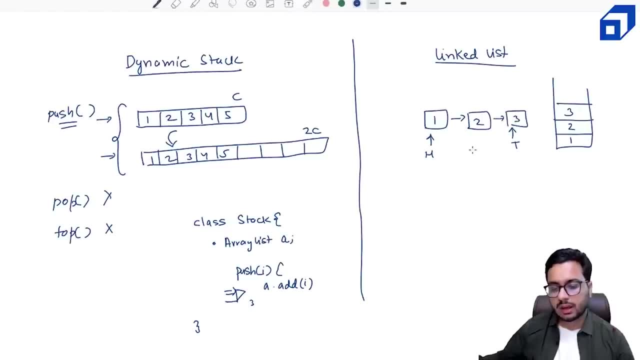 it at tail, this tail will go here, and three is also inserted right here, and three is also inserted right here, and three is also inserted right now. the question is if i want to remove now. the question is if i want to remove now. the question is if i want to remove something, if i want to pop out three. 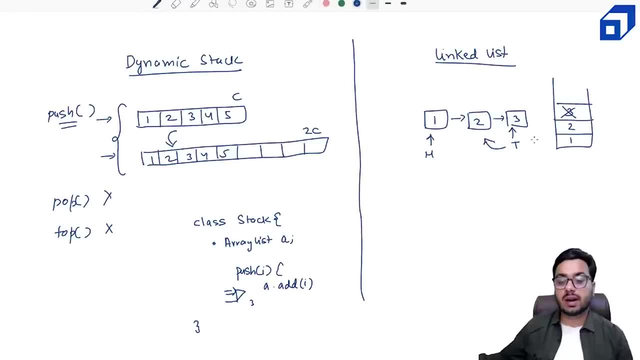 something. if i want to pop out three something if i want to pop out three, right, how do i move this tail back right? right, how do i move this tail back right? right, how do i move this tail back right? i cannot move it back in order one time. 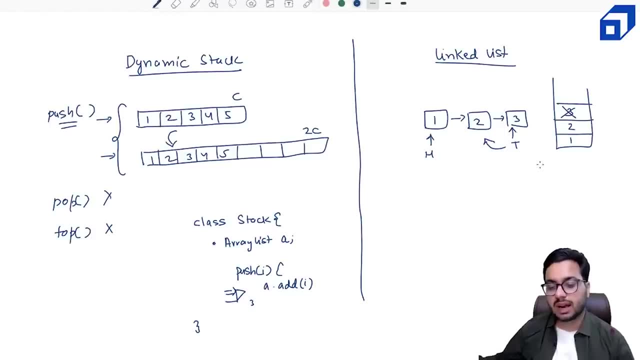 i cannot move it back in order one time. i cannot move it back in order one time. right, i have to traverse from the right. i have to traverse from the right. i have to traverse from the beginning, beginning, beginning. this is going to be time taking, so push. 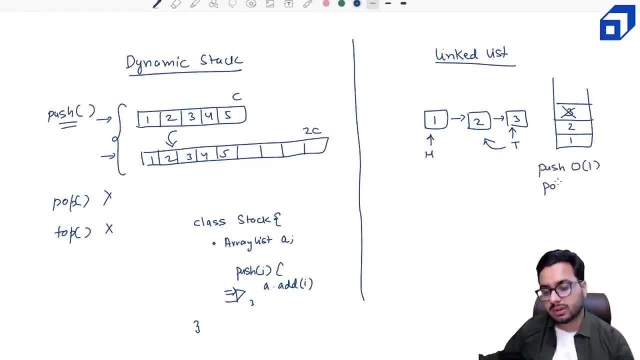 this is going to be time taking, so push. this is going to be time taking, so push is going to be order one, but my pop is is going to be order one, but my pop is is going to be order one, but my pop is going to be order of n. 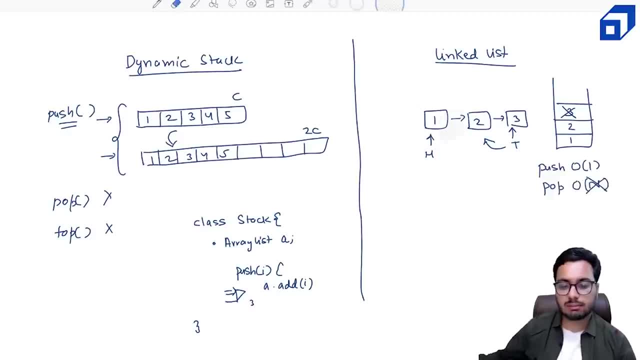 going to be order of n, going to be order of n, which is not acceptable here, right so, which is not acceptable here, right so which is not acceptable here, right. so. hence i need a better implementation, hence i need a better implementation, hence i need a better implementation using a linked list. 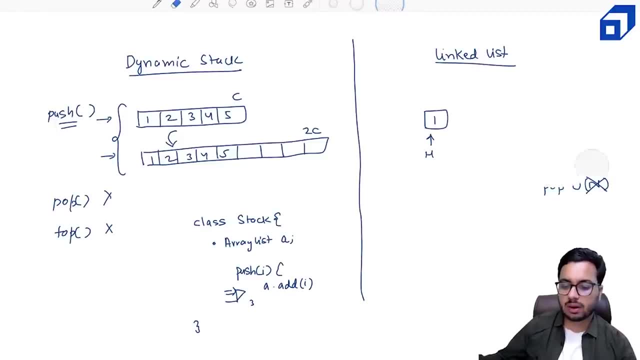 using a linked list. using a linked list, let us do one more try, suppose i got. let us do one more. try, suppose i got. let us do one more try, suppose i got. one, one one, and both hadn't till they got updated and both hadn't till they got updated. 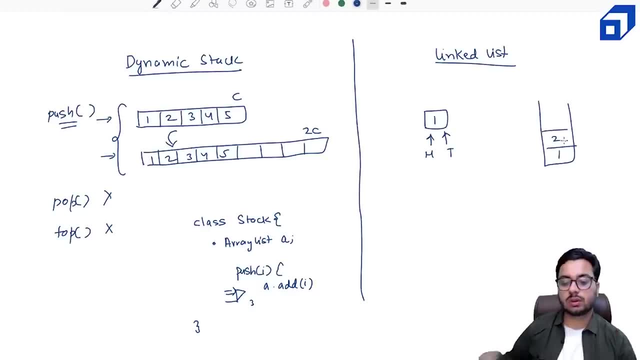 and both hadn't till they got updated right, right, right. if i want to insert two, right. if i want to insert two, right. if i want to insert two, two will go here. two will go here, two will go here. i will create a new node. i will create a new node. 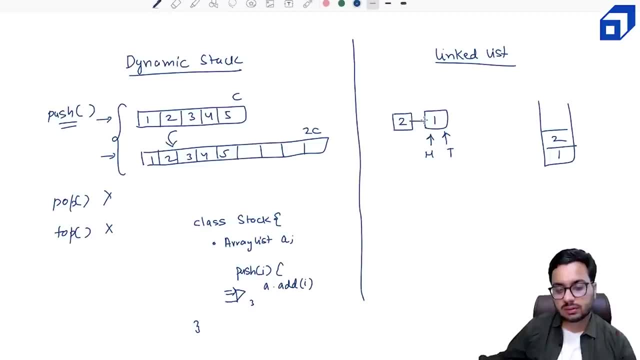 i will create a new node, okay, okay, okay, and i will connect this node and i will connect this node and i will connect this node with the head. so basically i'm inserting with the head. so basically i'm inserting with the head. so basically i'm inserting at the 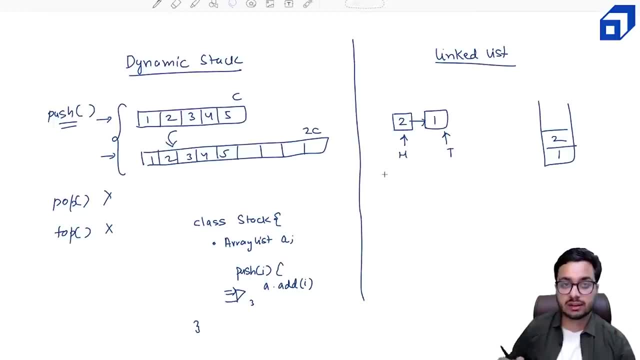 at the, at the head, only this head head, only this head head, only this head will move here, fine right will move here, fine, right will move here, fine right. because that that we have seen how to, because that that we have seen how to, because that that we have seen how to insert: at it. 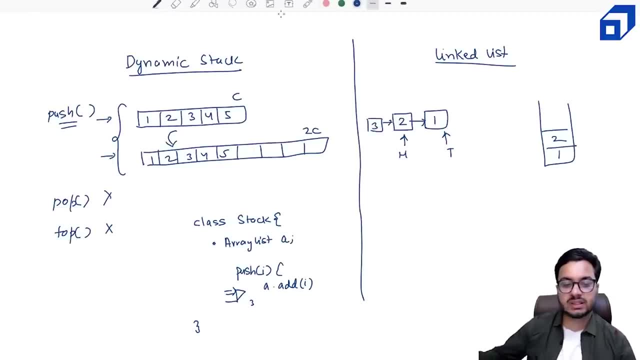 insert at it. insert at it, then i insert three. i create a new node, then i insert three. i create a new node, then i insert three. i create a new node connected with the previous head, connected with the previous head, connected with the previous head, and i update this head right, this head. 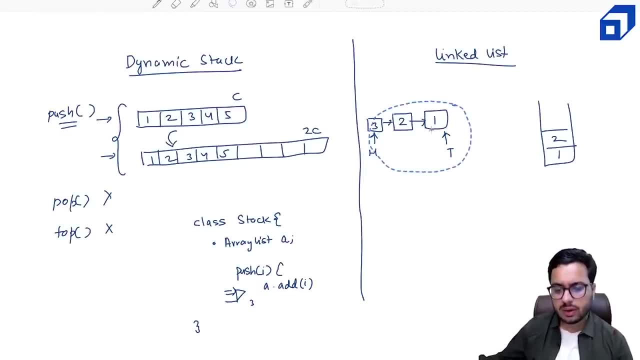 and i update this head right, this head, and i update this head right, this head: can, can, can, come here right now. if i want to remove, come here right now. if i want to remove, come here right now. if i want to remove something, i can say, okay, i want to. 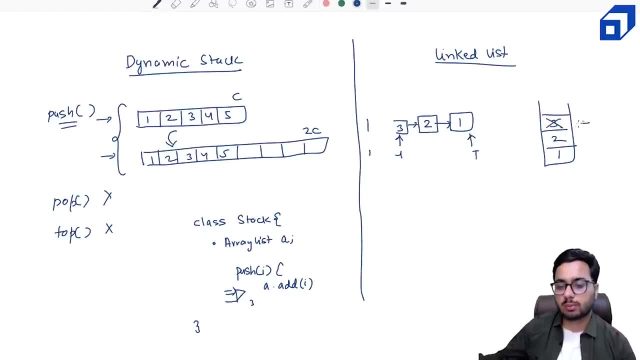 something i can say, okay, i want to something i can say, okay, i want to remove, remove, remove the topmost node. i want to pop this the topmost node. i want to pop this the topmost node. i want to pop this node. right, how do i remove it? 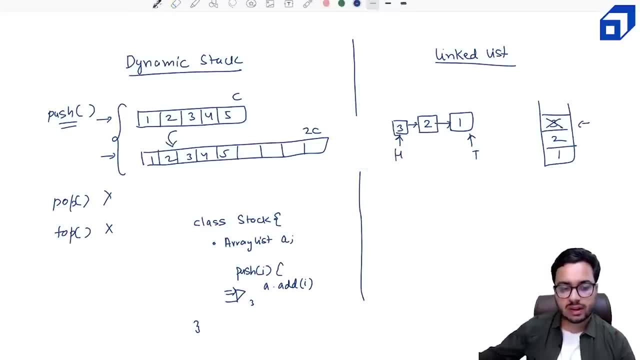 node right- how do i remove it? node right, how do i remove it. this is now pretty easy. how we can say: this is now pretty easy. how we can say: this is now pretty easy. how we can say: okay, fine, let me move the head from here. okay, fine, let me move the head from here. 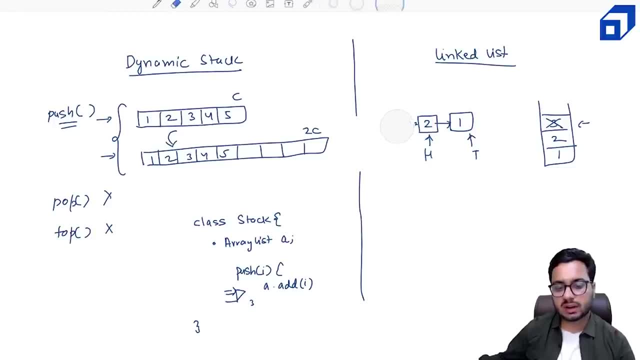 okay, fine, let me move the head from here to here. and this node now becomes to here. and this node now becomes to here. and this node now becomes eligible for garbage collection right. eligible for garbage collection right. eligible for garbage collection right. that means popping is very easy, even. 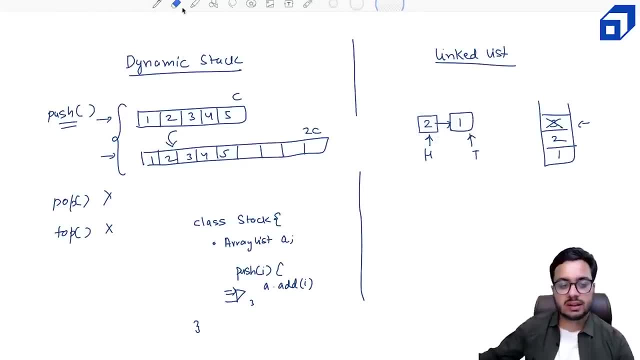 that means popping is very easy. even that means popping is very easy. even looking at the topmost element is very. looking at the topmost element is very. looking at the topmost element is very easy. so the element at the head: easy, so the element at the head. 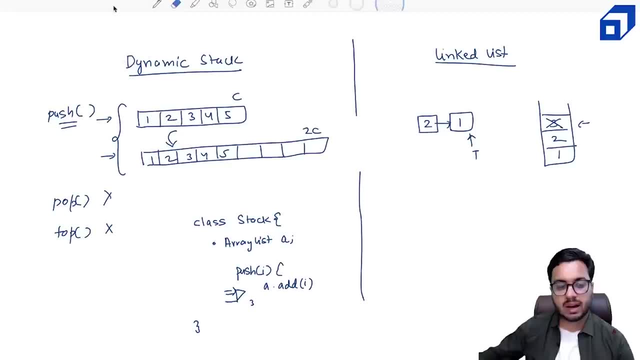 easy. so the element at the head is the element at the top. so again, if i is the element at the top, so again, if i is the element at the top, so again, if i want to remove this thing, my head will want to remove this thing. my head will. 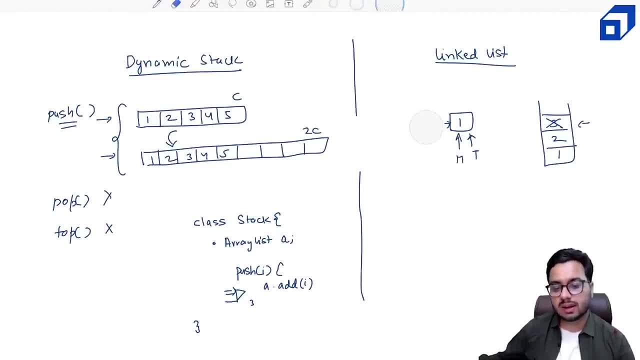 want to remove this thing, my head will go here, go here, go here and the node 2: it will become garbage and the node 2: it will become garbage and the node 2: it will become garbage. collected, so using linked list, also collected, so using linked list also. 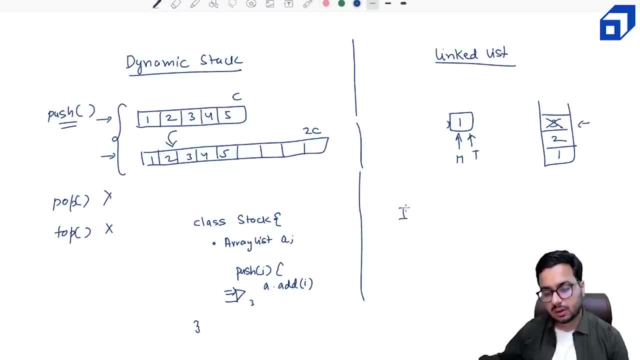 collected. so using linked list also, building a stack is very easy. if you building a stack is very easy, if you building a stack is very easy if you want to insert something or you want to want to insert something. or you want to want to insert something or you want to push something. 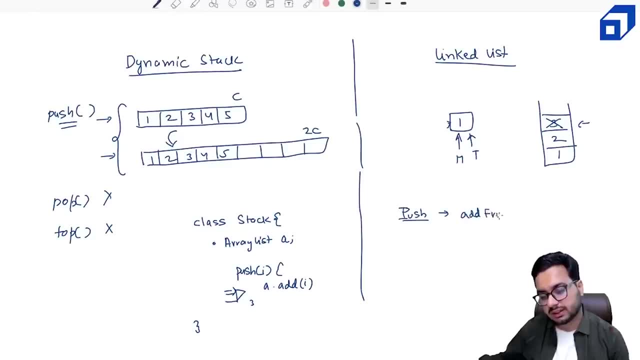 push something. push something. you can say, okay, i will call the add. you can say, okay, i will call the add. you can say, okay, i will call the add. front method of the linked list. front method of the linked list. front method of the linked list it it. 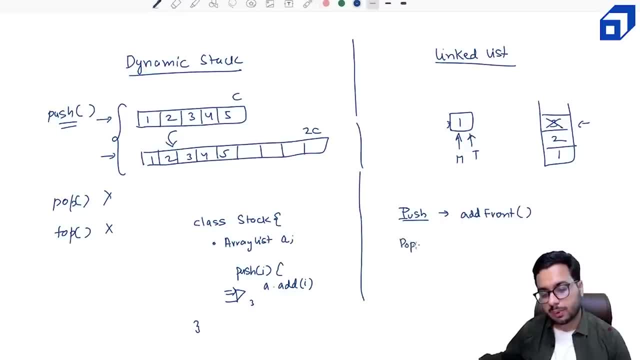 it or insert front, whatever it is. and if i or insert front, whatever it is, and if i or insert front, whatever it is, and if i want to pop something, i will say remove. want to pop something? i will say remove. want to pop something? i will say remove from the front. okay, i think, add first. 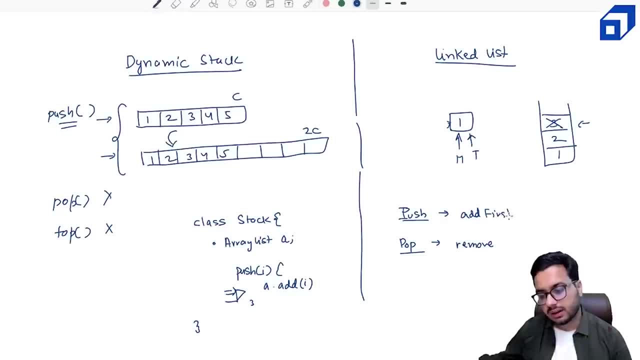 from the front. okay, i think add first. from the front. okay, i think add first. we call called it as add first. we call called it as add first. we call called it as add first. i need to add at the first position and i. i need to add at the first position and i. 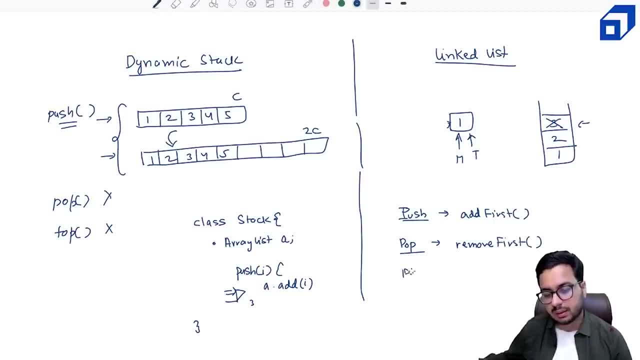 i need to add at the first position and i need to remove at the first position. need to remove at the first position, need to remove at the first position. and peak is nothing but it is the get and peak is nothing but it is the get and peak is nothing but it is the get. first i want to get the first element of 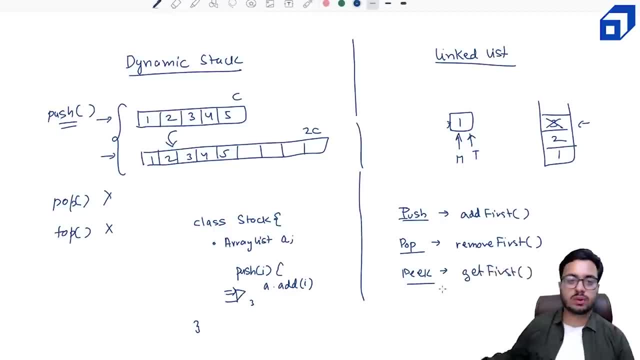 first, i want to get the first element of first. i want to get the first element of the, the- the linked list right. that is how it's linked list right. that is how it's linked list right. that is how it's going to work, right. so, regarding the, 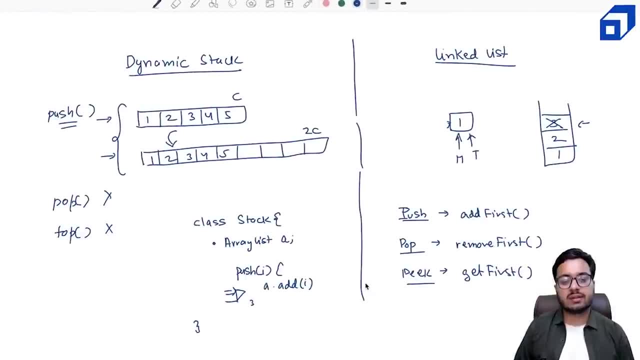 going to work right. so, regarding the going to work right. so, regarding the implementation, i think it's now pretty implementation. i think it's now pretty implementation. i think it's now pretty easy, given that we have implemented easy, given that we have implemented easy, given that we have implemented arraylist, we have implemented linked list. 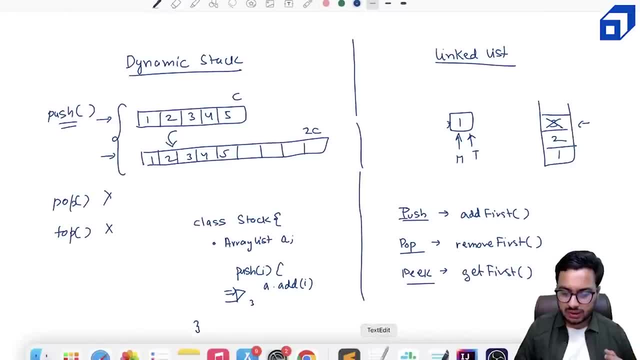 arraylist- we have implemented linked list. arraylist- we have implemented linked list. what you can do. you can also what you can do. you can also what you can do. you can also put that code inside your. put that code inside your. put that code inside your dynamic. 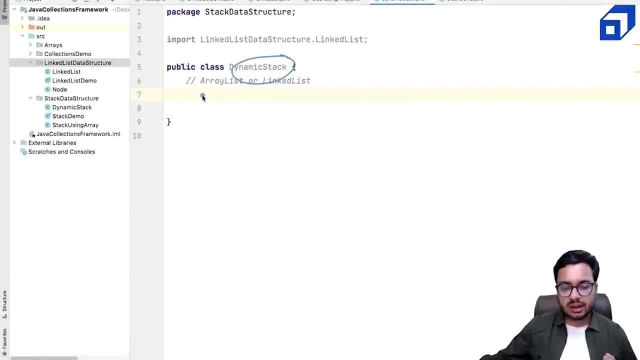 dynamic dynamic tag class as well. right now. three options tag class as well. right now. three options tag class as well. right now three options: either you write entire code, either you write entire code, either you write entire code. that is option number one. you define the. that is option number one. you define the. 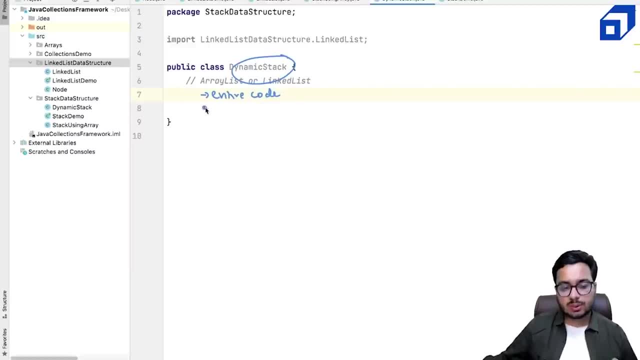 that is option number one. you define the node. you write how do we insert at node. you write how do we insert at node. you write how do we insert at front. second option is: you can use uh front. second option is: you can use uh front. second option is you can use uh, the linked list class that we have. 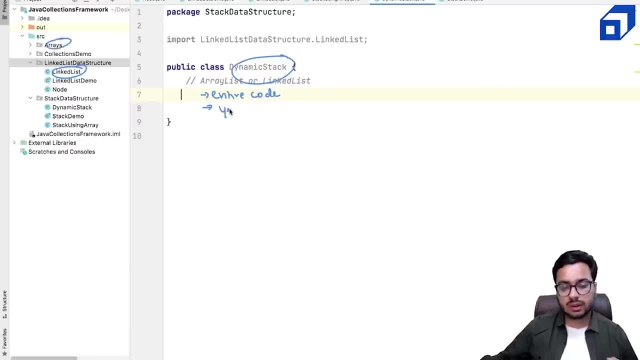 the linked list class that we have, the linked list class that we have created or created or created, or the arraylist class we have created, so the arraylist class we have created, so the arraylist class we have created, so you can use, you can use, you can use your library version. okay, if you don't. 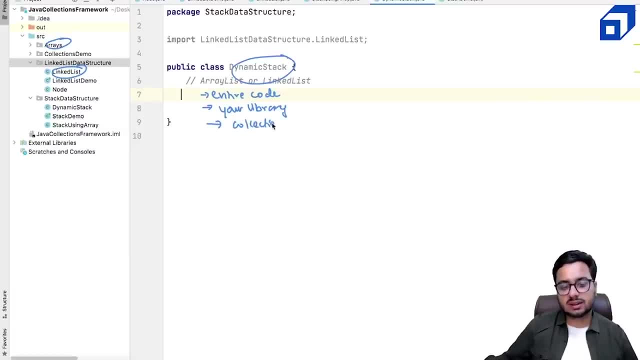 your library version, okay. if you don't, your library version, okay. if you don't want to do that, you can also use. want to do that. you can also use want to do that. you can also use the collections um, the collections um the collections um arraylist or the collections linked list. 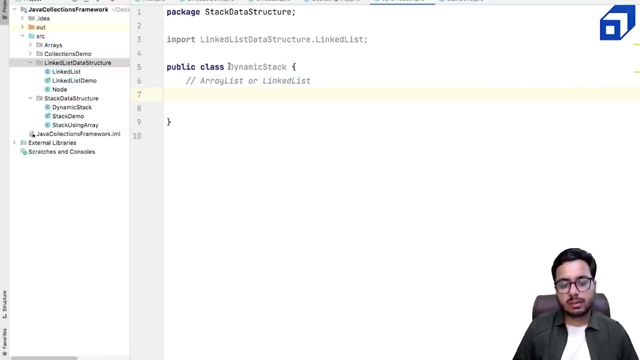 arraylist or the collections linked list. arraylist or the collections linked list- right any. any code you can use to right any. any code you can use to right any. any code you can use to build your own version of dynamic stack. build your own version of dynamic stack. 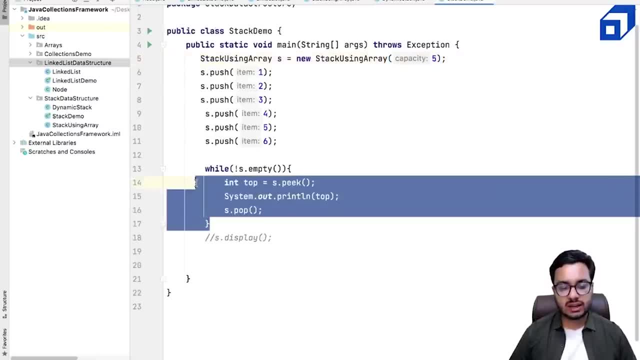 build your own version of dynamic stack: right, right, right. and the behavior wise, it will have same. and the behavior wise, it will have same. and the behavior wise, it will have same functionality, except that it will not functionality, except that it will not functionality, except that it will not get full. 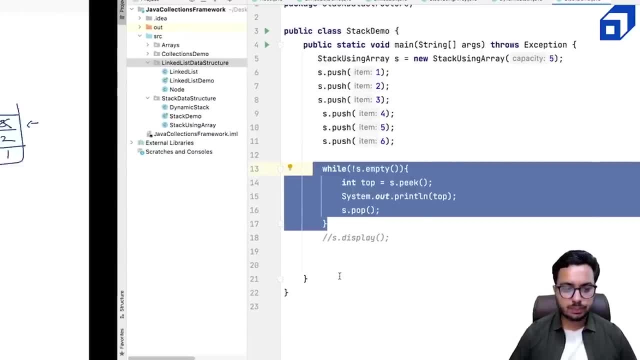 get full, get full, unless your system memory is not full, unless your system memory is not full, unless your system memory is not full. right, right, right. so that's all for dynamic stack. hope you so. that's all for dynamic stack. hope you so. that's all for dynamic stack. hope you understood the functionality of dynamic. 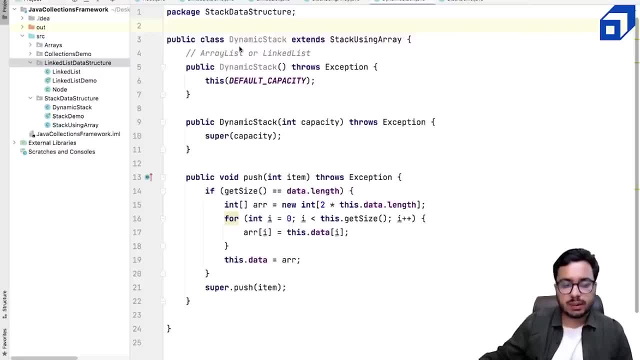 understood the functionality of dynamic, understood the functionality of dynamic stack. okay, i'll show you one more stack. okay, i'll show you one more stack. okay, i'll show you one more: implementation of implementation of implementation of implementing dynamic stack. using the implementing dynamic stack, using the implementing dynamic stack, using the stack, using array class. so this class, we 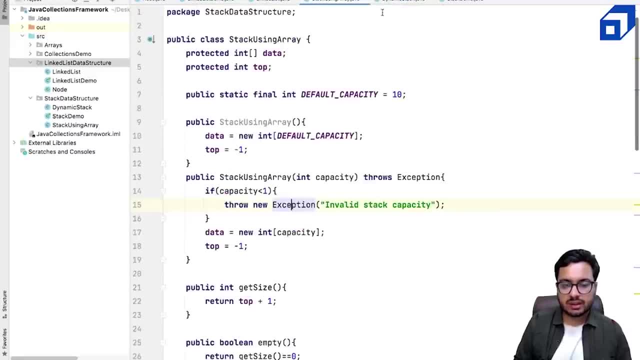 stack using array class, so this class. we stack using array class, so this class we have have have just written so what i'm doing. i have just written so what i'm doing. i have just written so what i'm doing. i have created one child class called dynamic. 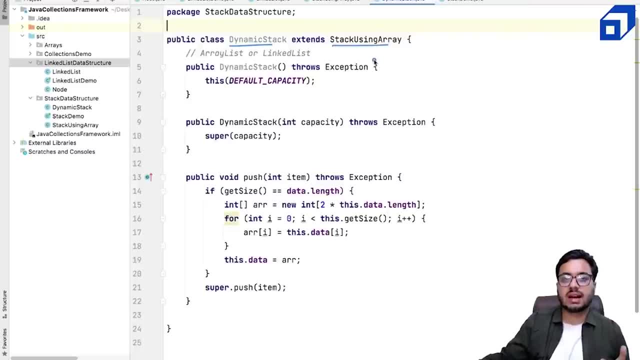 created one child class called dynamic, created one child class called dynamic stack, stack, stack and it is extending the stock using and it is extending the stock using and it is extending the stock using array class that we have just written inside this class. i have only updated inside this class. i have only updated. 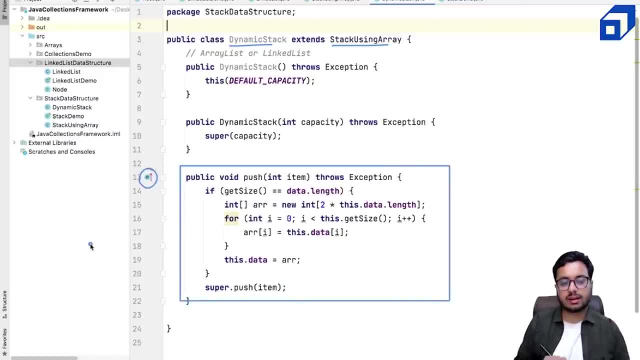 inside this class. i have only updated the push method. so basically i have the push method, so basically i have the push method. so basically, i have overwritten this method right, overwritten this method right, overwritten this method right, and i have provided two constructors. so, and i have provided two constructors so, 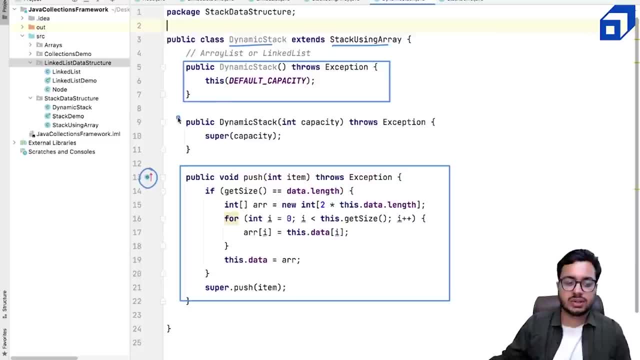 and i have provided two constructors so that i can provide a build: the dynamic that i can provide a build, the dynamic that i can provide a build. the dynamic- stack object right. stack object right. stack object right. so the first constructor does not accept. so the first constructor does not accept. 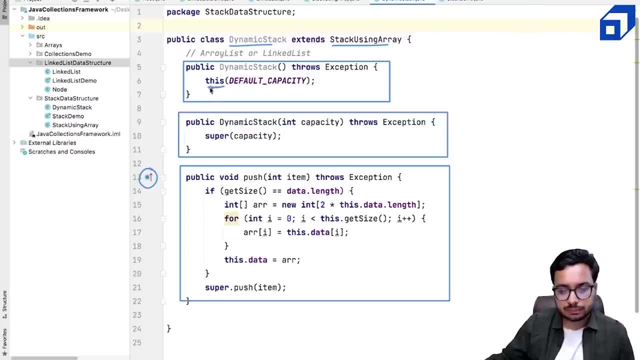 so the first constructor does not accept any capacity. so i call any capacity. so i call any capacity, so i call the constructor, the constructor, the constructor. so this is basically calling this method. so this is basically calling this method. so this is basically calling this method with the default capacity. so i say okay. 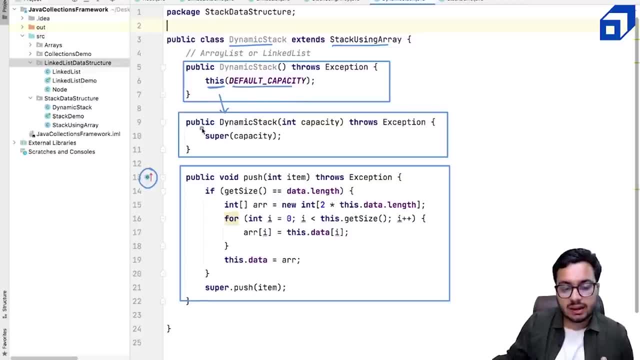 with the default capacity. so i say okay with the default capacity. so i say okay, go and create a start with the default. go and create a start with the default. go and create a start with the default capacity. right, capacity, right, capacity, right. and if i get a capacity from user, then 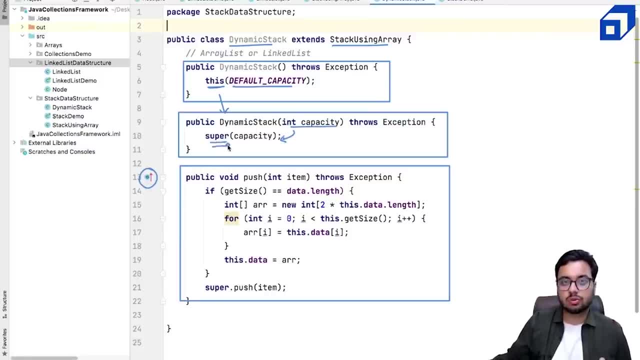 and if i get a capacity from user, then, and if i get a capacity from user, then also i can i call the constructor of the. also i can i call the constructor of the. also i can i call the constructor of the parent class. so super is for calling the. 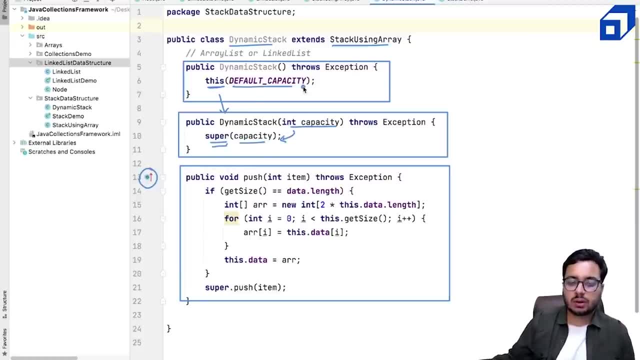 parent class. so super is for calling the parent class, so super is for calling the parent class, parent class, parent class. and i give the capacity. okay, you go and and i give the capacity. okay, you go and and i give the capacity. okay, you go and call the constructor. 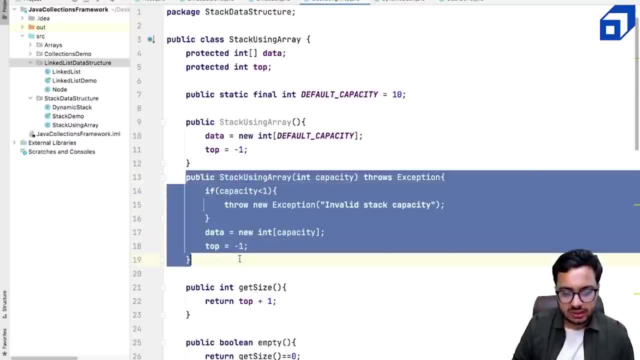 call the constructor. call the constructor that is here right. so that is here right. so that is here right. so this constructor is getting called right. this constructor is getting called right. this constructor is getting called right and i pass in the capacity. so either i and i pass in the capacity, so either i. 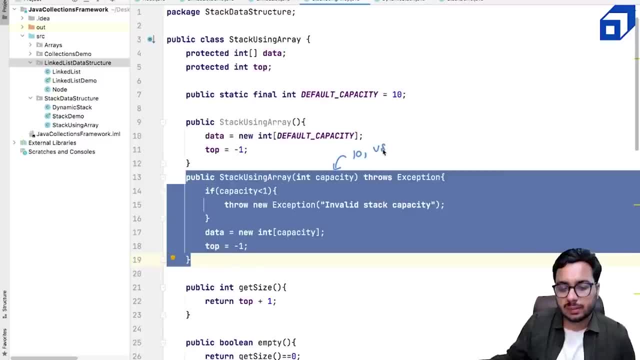 and i pass in the capacity. so either i pass in the default capacity that is 10, pass in the default capacity that is 10, pass in the default capacity that is 10, or i give the user defined capacity or i give the user defined capacity or i give the user defined capacity right. 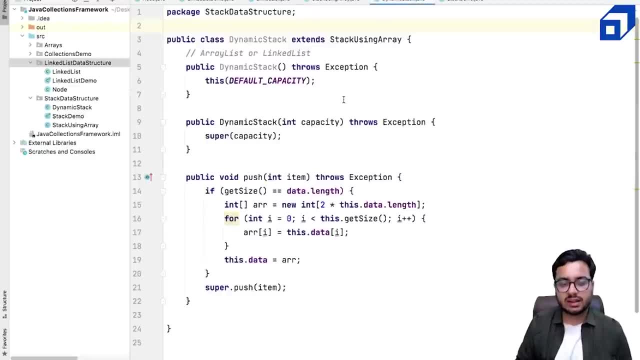 right, right, so i give that, so this, so i give that, so this, so i give that, so this calls the parent constructor and calls the parent constructor and calls the parent constructor and initializes that array right. initializes that array right. initializes that array right of that particular size, right, the pop. of that particular size. right, the pop of that particular size. right, the pop method. i told you it's not going to method. i told you it's not going to method. i told you it's not going to change the peak method. it's not going to change the peak method, it's not going to. 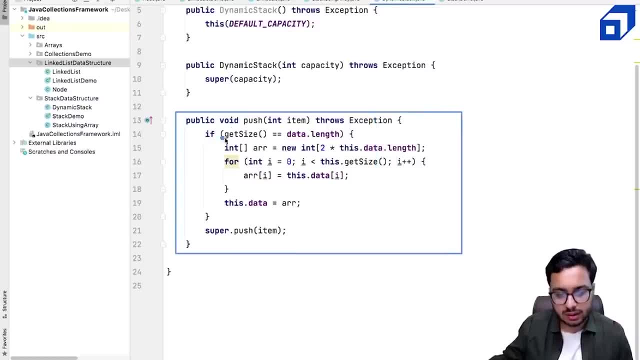 change the peak method. it's not going to change. change the peak method. it's not going to in the push method. if my array is full in the push method. if my array is full in the push method. if my array is full, right. so if get size is equal to data, 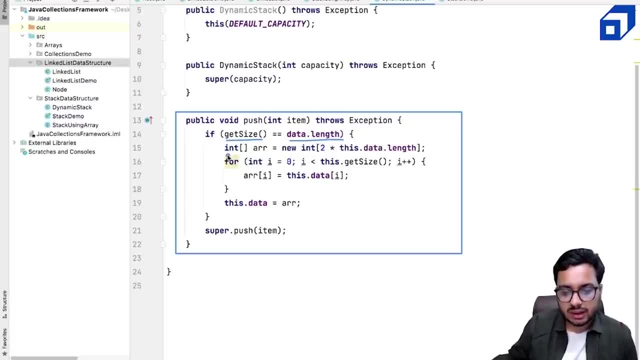 right. so if get size is equal to data, right. so if get size is equal to data, dot length, dot length, dot length- right and what i will do: i create a new right and what i will do. i create a new right and what i will do. i create a new array. 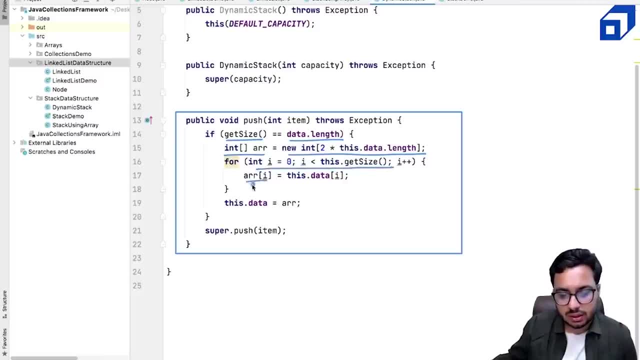 array. array of twice the size. i copy all the of twice the size. i copy all the elements into the new array. okay, and i say okay, this dot data should, uh, now point to this area. right, what happens? so data was pointing to the old array. right now data is pointing to the new array. 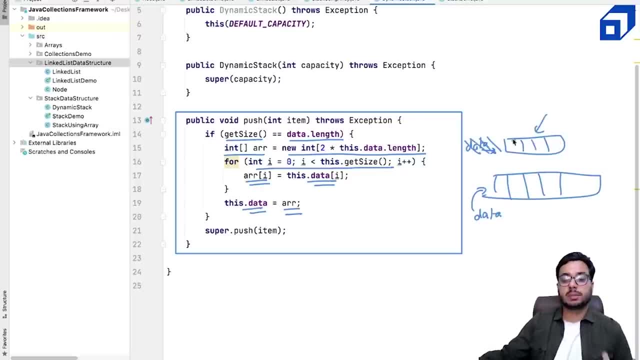 so this reference is gone. that means this array will be garbage collected, right. so this is error. error is a local variable. it will be destroyed, but data is a class member, so it will not get destroyed. so using the this keyword is optional. it is for more clarity that we are talking about. 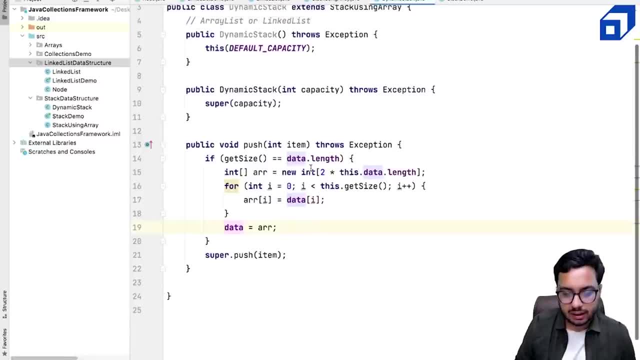 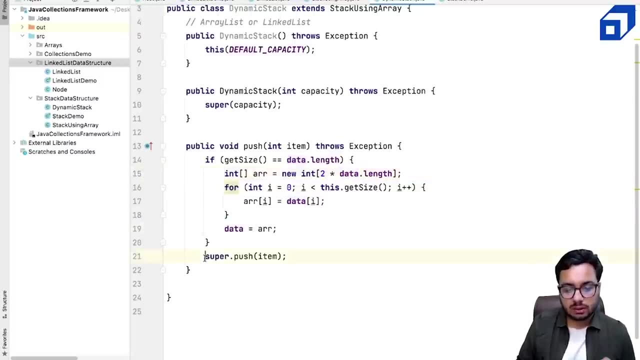 the data member, very, not any local variable, right? so that is what we are doing here, and then, after we expanded the array, we call the push method of the parent class in the parent class. now, if, if your array has already expanded, you will never get this condition. this condition will never be met. 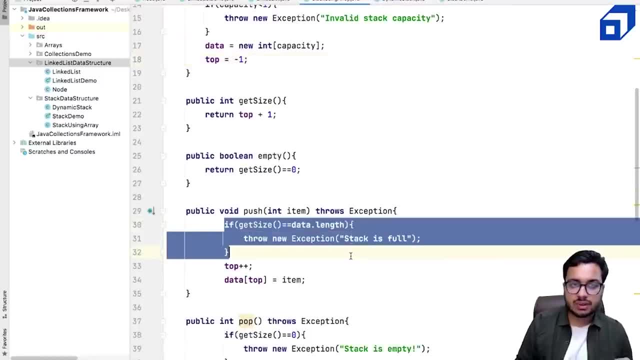 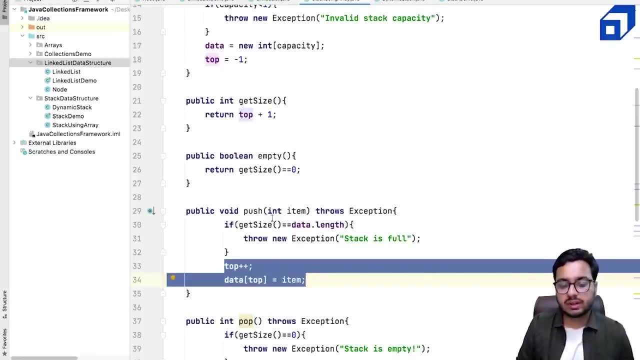 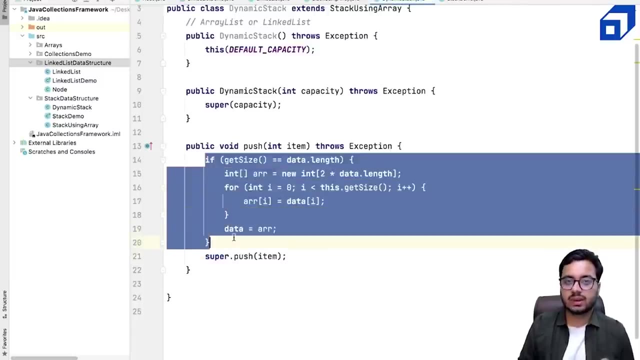 which condition? uh, data dot length is equal. so exception will not be thrown. and what will happen? top plus plus. and data are of top equal to item, so this code will actually execute. if condition will not be true, before calling the push method of parent function, i simply expand the array in case of a dynamic. 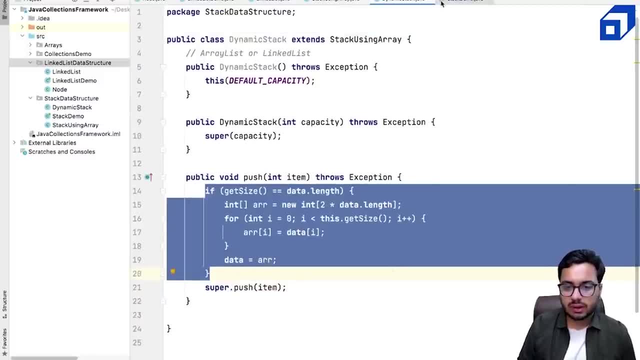 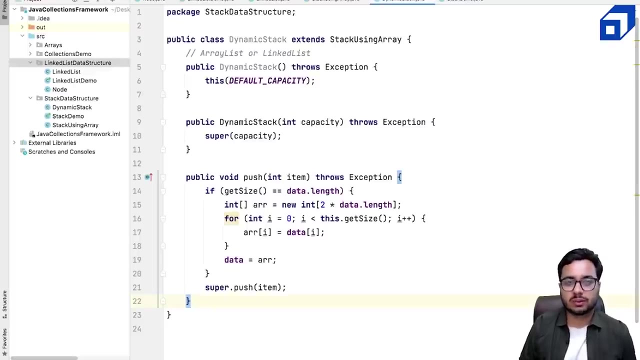 array. this is what i rarely do and it will work. so what you need to do, you need to replace this stack with the dynamic stack. you can try it out and it will work right. so that is another way of using inheritance and creating a dynamic stack object for you. one small change i wanted to. 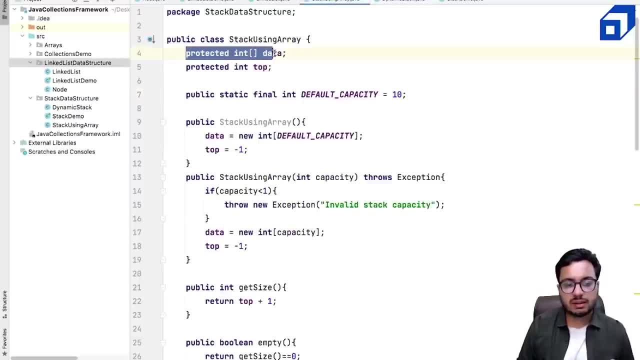 discuss was i did a change that i made these data members, which were earlier private, i made them as protected. now, right, why? because i want to use these data members in the child class as well. right, so that is the only change i have done in the class called stack, using an array. 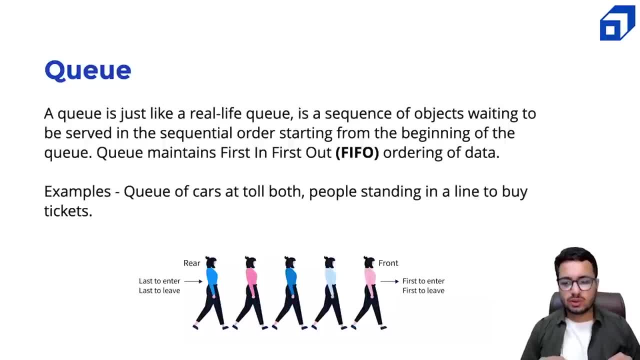 so let us start by understanding the fundamentals of a queue. what is a queue? a queue is just like a real life queue. so, in most general terms, a queue represents a sequence of objects waiting to be served in a sequential order. okay, so one thing you need to remember is q is also a linear data structure, like other linear data structures you have seen. 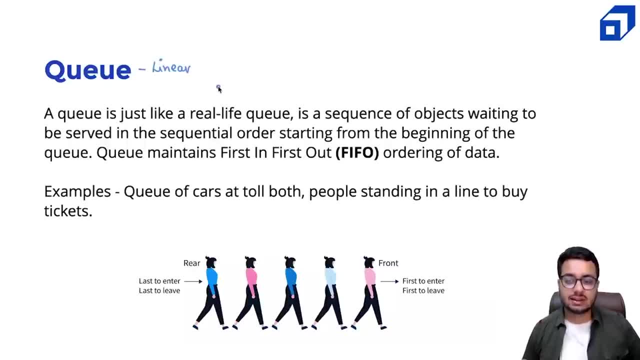 so far. arrays, array, list tags, linked list q. q is also a linear data structure that stores the data in the sequential order, starting from the beginning of the queue, right, for example, let's say, if you see on the screen the person who enters the queue first if you go to a bank right, the person who enters the queue first, it is at the front of the. 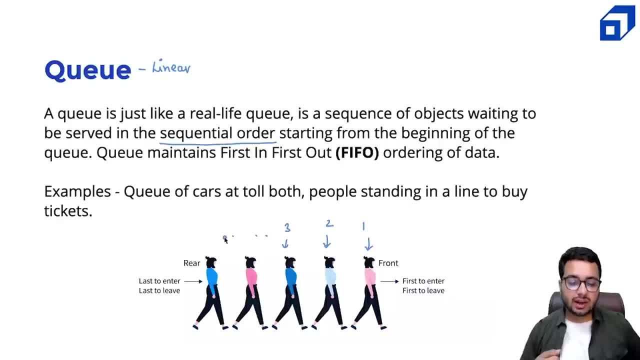 queue, second person is behind it, third person is behind the second person, and so on, right. so, in general, q has two ends. one is called as front, from where the people will be served, right, and one is the rear end, from where people will join the queue right. basically, insertion of data. 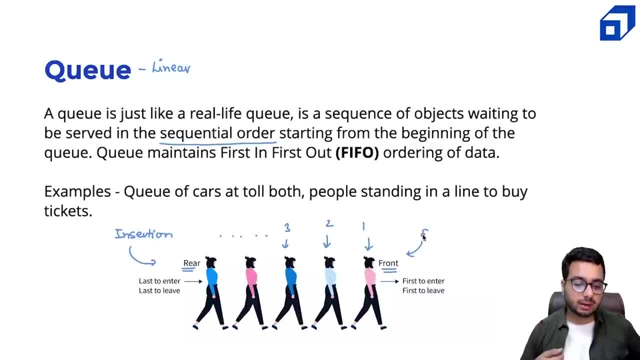 And removal of data will happen from the front side right People at the front. once they are served, they will get removed from the queue. right Now. this queue can also be seen as queue of cars at a toll booth right. 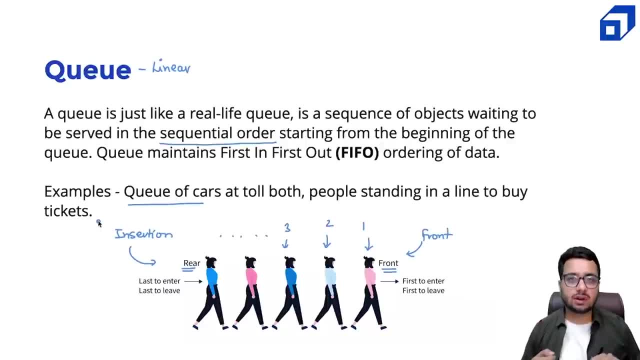 People standing in a line to buy tickets- right. And in the world of computer science, we use queues a lot, right. For example, many people are uploading videos on YouTube and YouTube has maintained a queue so that people who have uploaded videos first- their videos will be processed right. 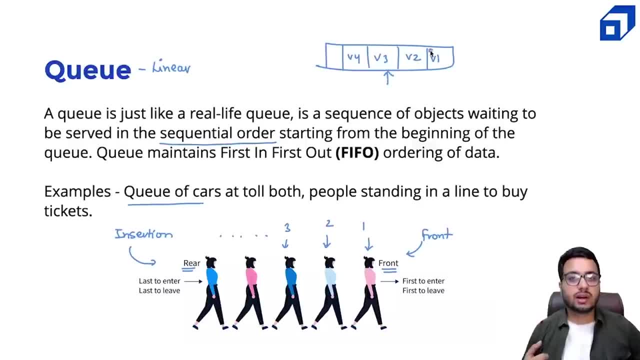 We might maintain a queue of videos on the server waiting to be processed right. Similarly, in software applications, for example, an application has to perform several tasks, It might maintain a queue of the task that it needs to perform so that our work gets done right. 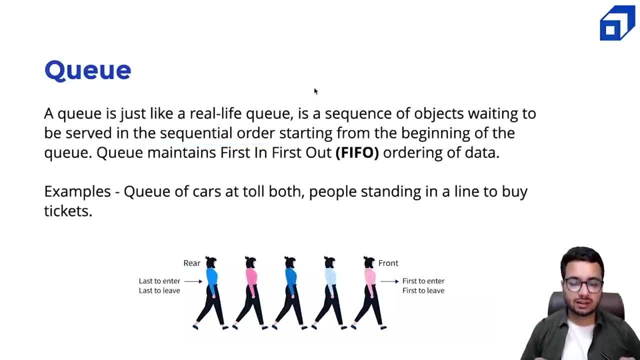 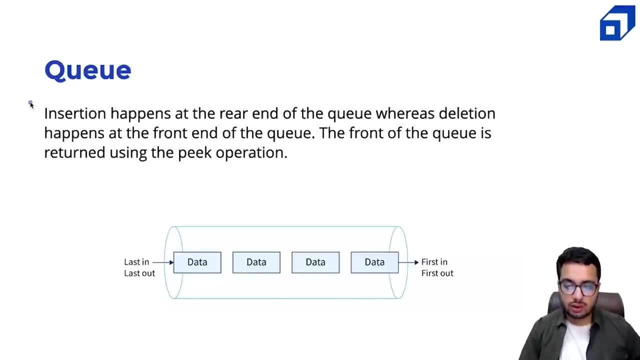 So queue is again a very important, very interesting data structure. right Now let us talk a little bit more about the operations. So, as I discussed, one fundamental operation on the queue is insertion. right, I want to insert something. 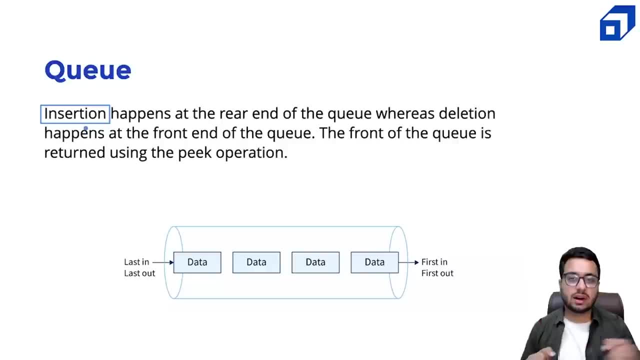 I want to insert something into the queue, right? So the kind of queue that we are discussing, current now it is called as FIFO queue- First in, first out queue- Why? Because the person who joins the queue first is the first one to get served, right. 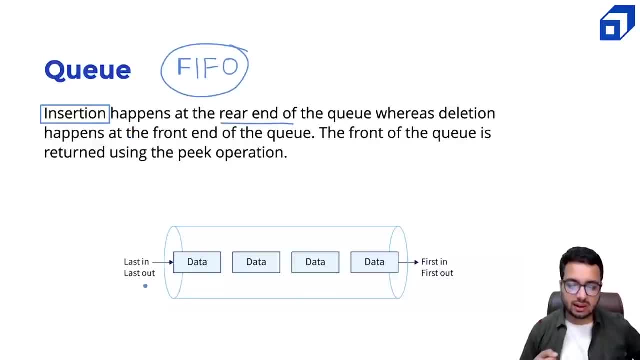 In a FIFO queue, insertion happens at the rear end of the queue, So this is your, let's say, rear end right, Whereas deletion happens at the front end of the queue. So this is your front side right. 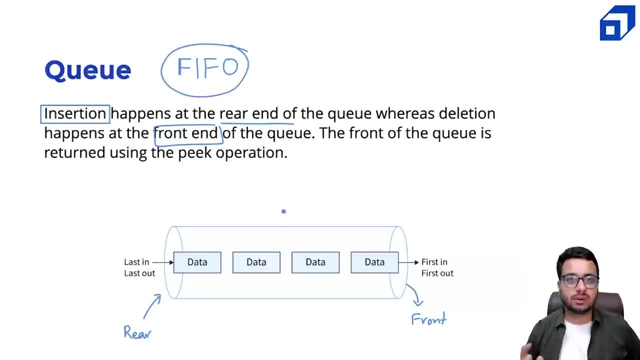 So anything you cannot show? okay, I want to remove something from the, From the middle of the queue. That is not possible. Only the data which is at the front of the queue will be removed. right, There is one more operation. 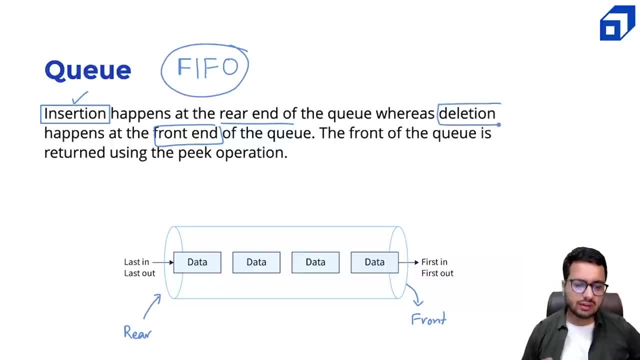 So we have seen insertion, We have seen deletion- right. We will discuss how these operations are implemented using other data structures- right? There is one more operation that is called peak, So I want to look what is the front element? okay? 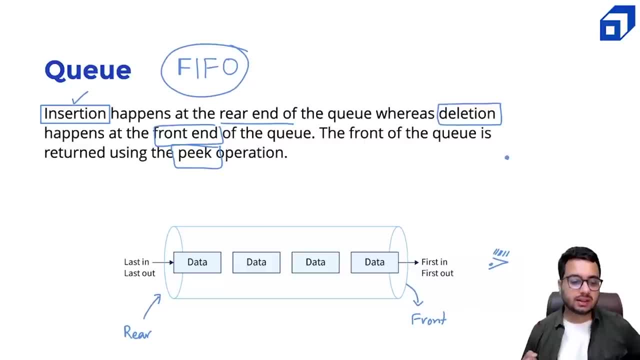 Who is standing at the front, We call that operation as peak. So just in case of stack, if you remember, the peak operation returns the top of the Top element of the stack In a queue. peak operation should return the front element of the queue right. 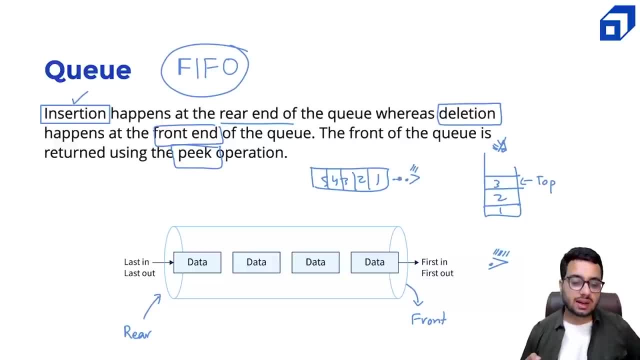 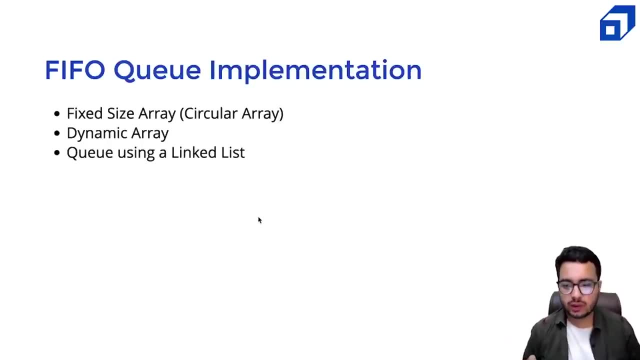 The person who is standing at the front of the queue. So that is what peak operation will do, right? So, as a next step, we will look at the implementation of a FIFO queue, right? So there are three common ways to implement a queue. 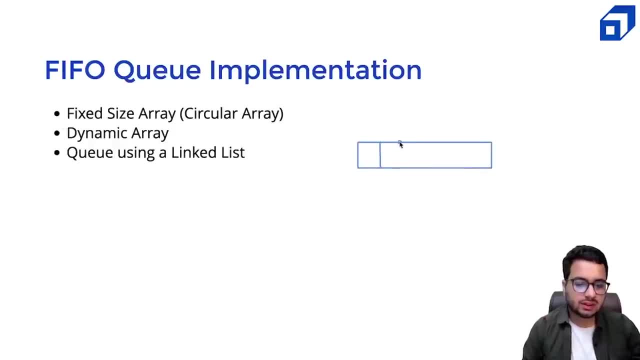 We can use a fixed size array, right, And we will see how this array will behave as a circular array When we are going to implement it. Okay, So in this case, queue will have a limited capacity because the array size is fixed. 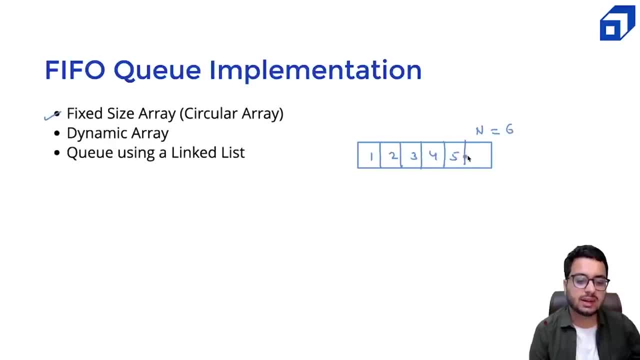 Suppose n is 6.. I cannot have more than 6 elements in this queue at any given point right. Second is: I can use a dynamic array. I can write my own logic for creating a dynamic array. For example, if my queue gets full, I will define I will double the array. 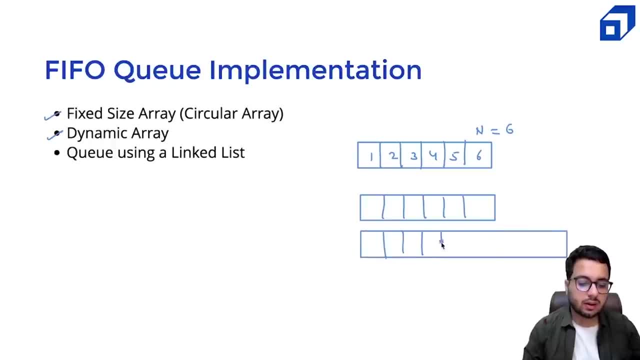 I will create a new array of double the capacity of the given size Right Now. if again the queue gets full, I will again do the same thing. right, This is called as implementation using a dynamic array. The other option is, if you do not want to write the functionality of doubling, it is already implemented inside your array list class. 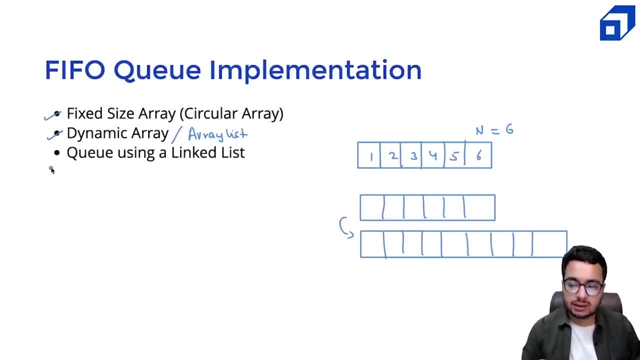 You can also implement queue using the array list, right? Third is, we can use build a queue using linked list as well. right, You know, linked list is a dynamic data structure, So we will look at how a linked list can be used to implement a queue as well. 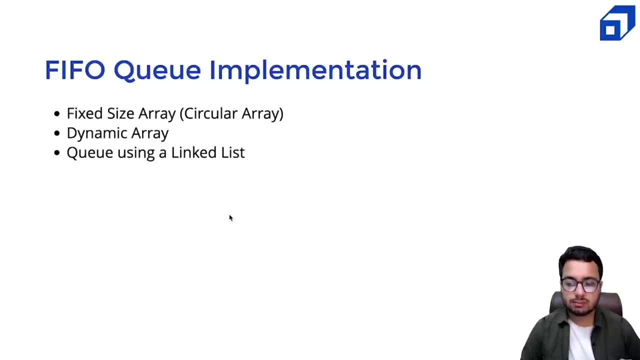 So we will look at how a linked list can be used to implement a queue as well. So let us start with the first implementation, that is, implementing a queue using fixed size array. Now let us talk about how we can implement operations on a queue using a fixed size array. 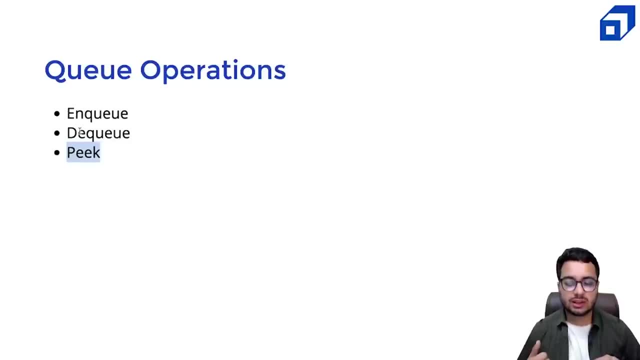 So the three operations that we need to build are enqueue, dequeue and peek. So enqueue means I want to insert something into the queue, Dequeue means I want to remove the element at the front And peek means I want to get the element at the front. 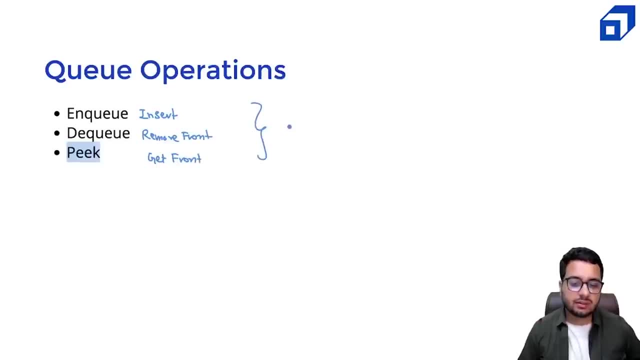 These are the three things That we will have in a C4 queue: First in, first out. right Now let us see how we can use a fixed size array to create these operations on the queue right. So in the beginning I should know if something is coming at what index. I will insert it into the queue. 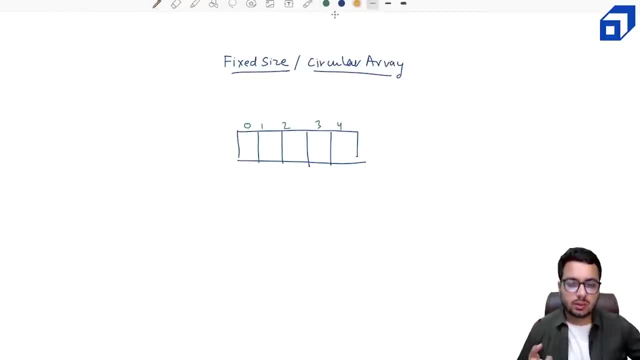 And at what index. I will remove it from the queue, right? So what I will do? it is okay. Let us take a variable called front And it is here. right, We can also take another variable here, But again, that is optional if you are maintaining the size of the queue. 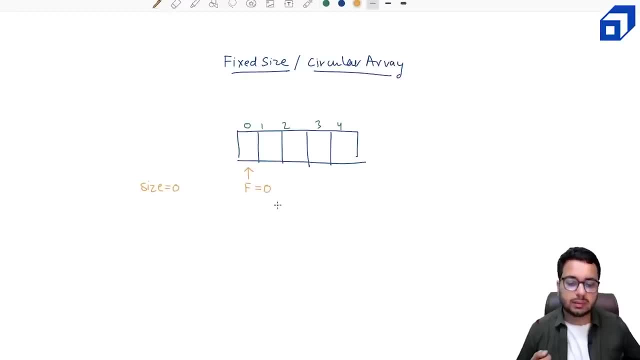 In the beginning. size is 0. Front is also at 0. That means nothing is inserted in the queue yet. right Now someone says: okay, person 1 is going to join the queue And I will insert it right. 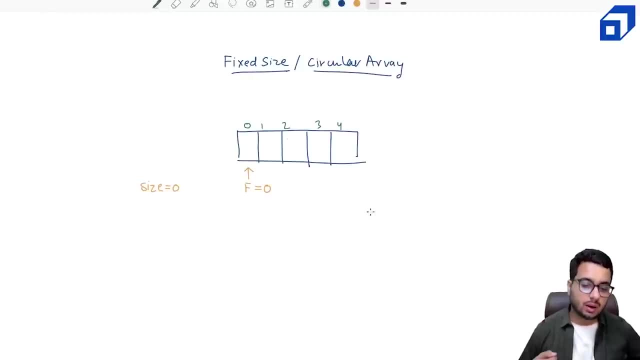 What I will do. I will insert it at the rear end. okay, So how do I compute the rear end? Let us see, The rear end can be said as front plus size. I will tell you why, right, So what is front? 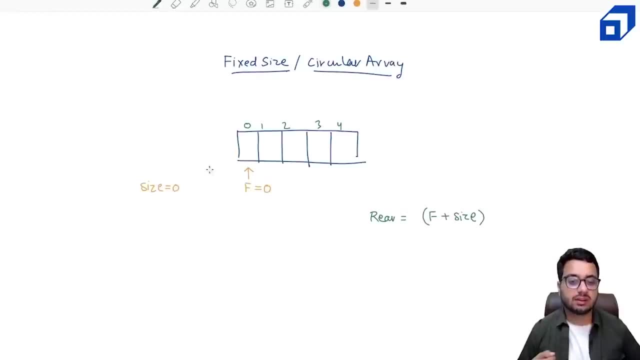 Front is 0.. What is size? Size is 0.. So 0 plus 0.. So 0 is 0.. So I can insert person 1 here in the queue right And I will increment the size. 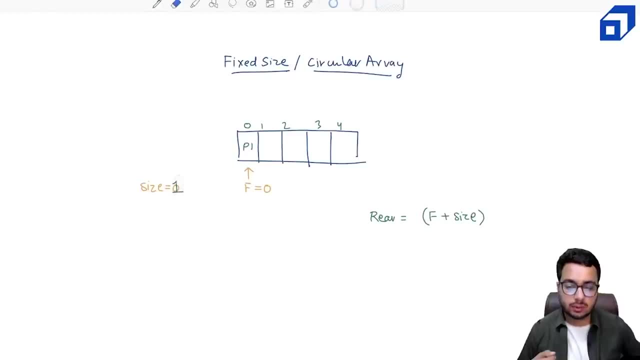 The size will become 1, right. Size is going to become 1, right, So I am not going to change the front. Look carefully, I am not going to change the front right Now. it was 0 plus 0.. 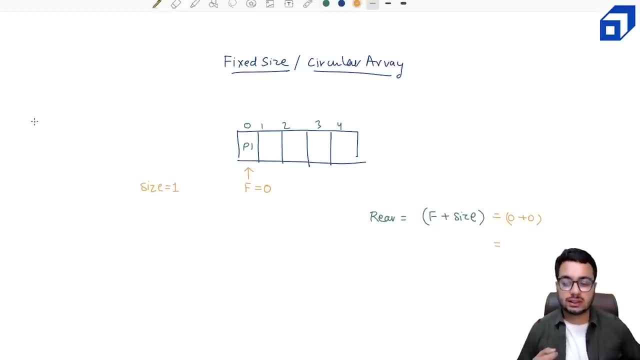 That is fine. right Now I can say again: I want to insert person 2,. okay, I want to insert person 2.. At what index I will insert? I will insert it. I will insert it at the rear end, right. 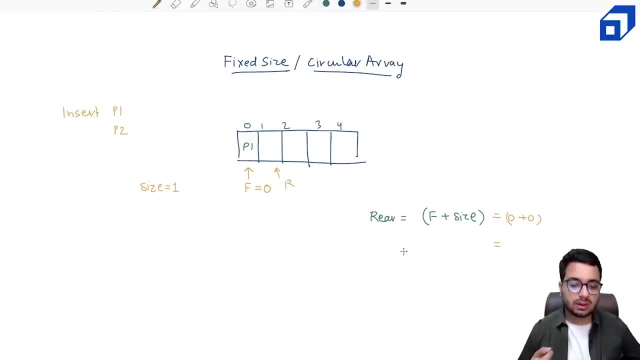 So what will be the rear my? What will be the rear value now? It will be f plus size. So f is 0.. Fine, Size is 1.. It is going to be 1.. I can insert person 2 at this index. 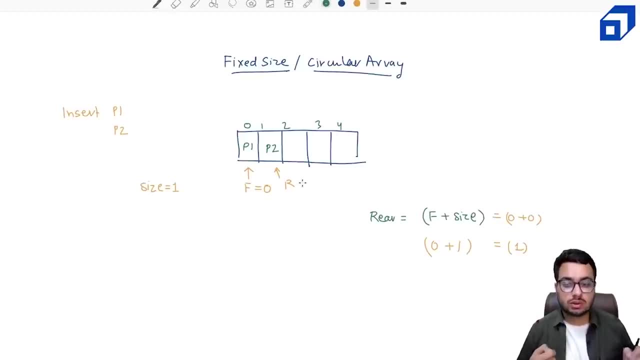 Very good right Now. let's say one more person wants to join the queue, So I want to insert person 3, right Size is already 2, right. I have inserted 2 elements, But what index I will insert? 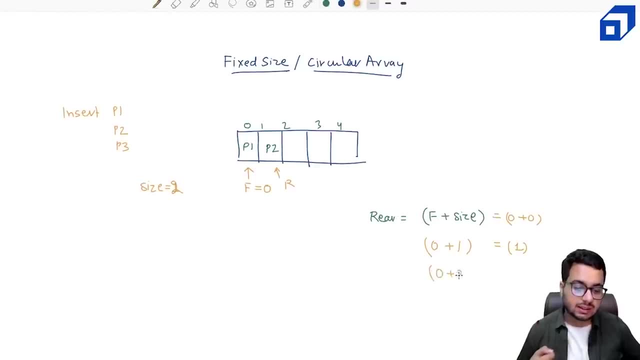 I will insert it at the rear index. What will be the rear index? 0 plus 2, that is going to be 2.. That means person 3 will be inserted here And this is the new rear. The front is not changing. 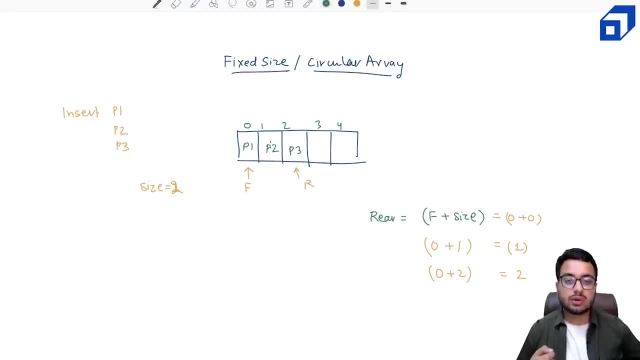 Rear is changing. in this case, Again, I want to insert person 4.. Let's insert person 4.. So size is already 3. now right Size is already 3.. What will be the new index? 0 plus 3, it's going to be 3.. 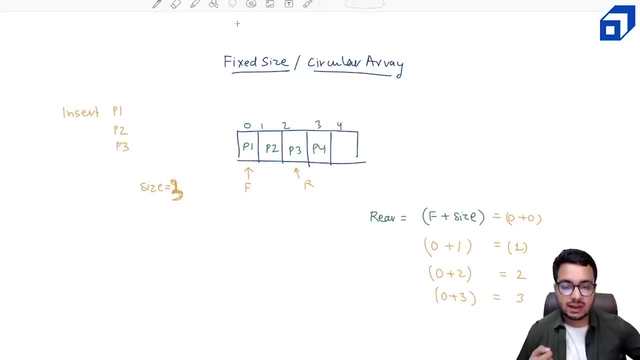 I can insert person 4.. At this index- And my rear is already here right Now- suppose I have done a lot of insertions. I want to remove something right. So I have inserted till person 4 also. 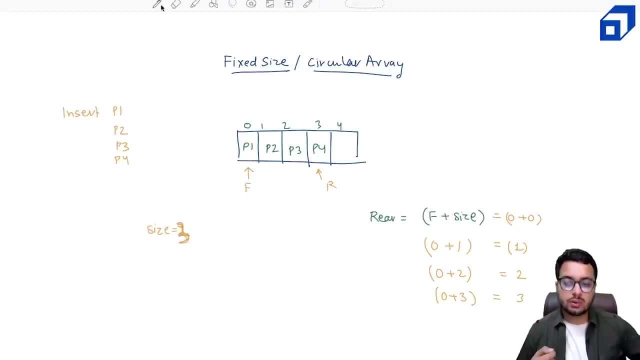 And I want to see how my front is going to change right Now. suppose I want to remove something. I want to perform dequeue right. So that means I got a query to remove the front element. The front element will get removed, right. 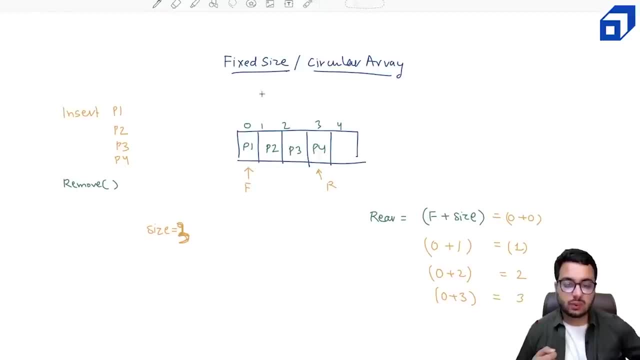 Now how do I remove it? If I move this F one step forward right And I will have to reduce the size. Right now the size was 4.. Because 4 elements are there in the queue right, My size becomes 4.. 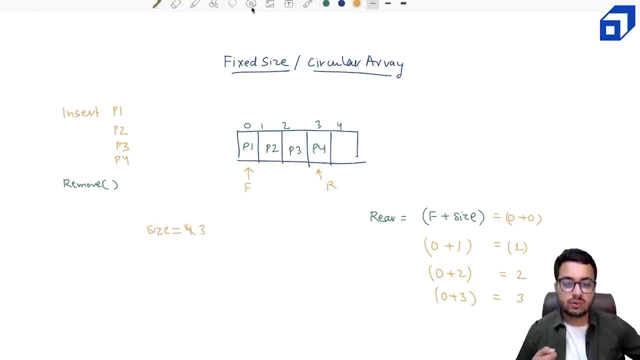 From 4, it becomes 3. And I say, okay, F should move one step ahead. So I will say, okay, I will take this front one step ahead. That means this P1 is it's kind of removed. 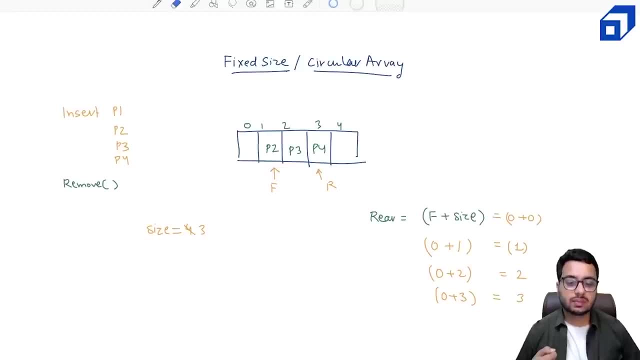 It's not there, right? So the area between front and rear, it is the content of the queue. Now suppose I want to insert something more, right? So what I will do, I will again do front, which is at 1, okay. 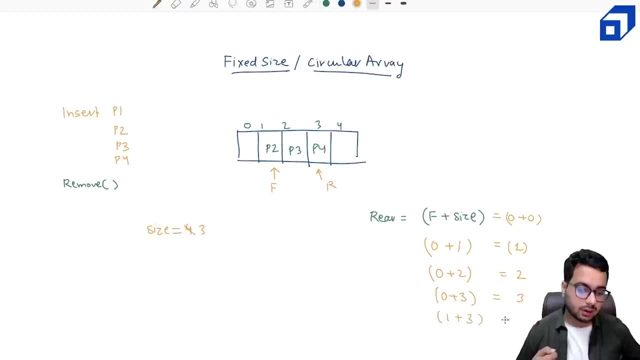 Plus size, which is at 3.. Look carefully. So 1 plus 3, I get an index 4.. That means the next insertion will happen at this index. Can I insert something? Of course I can insert something, because queue is not yet full. 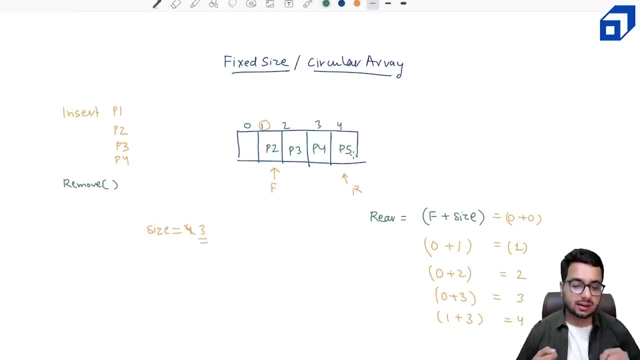 I insert something at this index Now suppose I want to do one more insertion Again. what is the value of size? now, Size is still 4.. Size is 4, right. So what will be the value of rear? 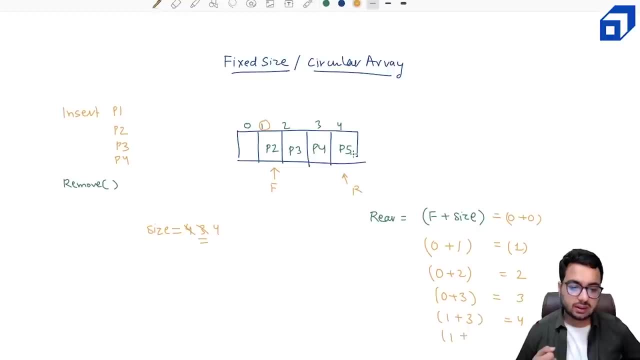 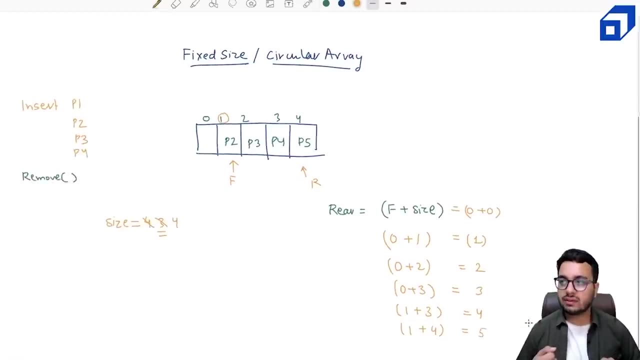 So it will be front, which is 1,, plus rear, which is at, which is plus size, which is 4,. right, It is going to get 5.. Now, is this 5 a valid index? Is this 5 a valid index? 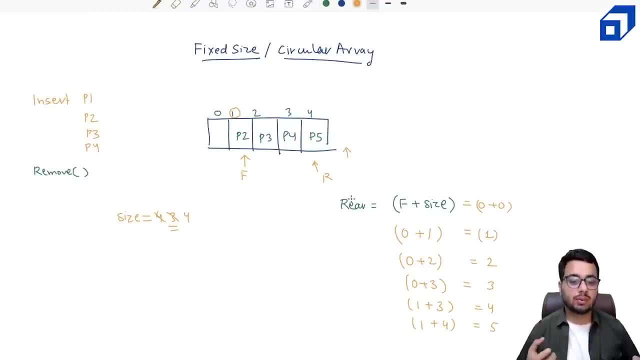 The answer is no, right. Now I will get a problem that it will give me index out of bounds exception, But queue is not yet full. Queue is not yet full, So how should I handle this case? right? The way to handle this case is by treating this array as a circular array, right? 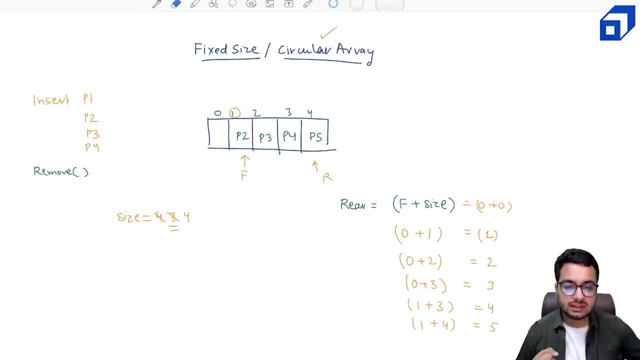 If you exceed 4, you should come back to this index. You should kind of rotate And you should come back here right Now. how do I achieve this? I have to say: take a mod with 5.. Every time you hit a 5,. 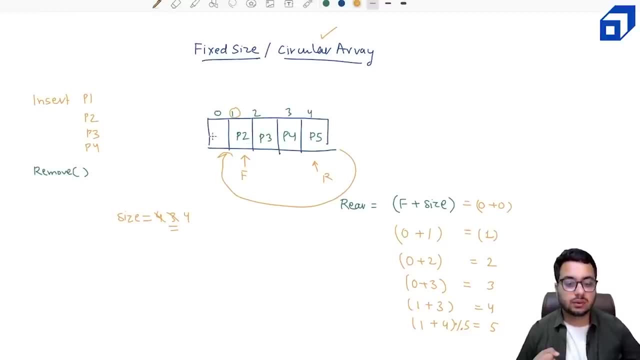 you go back to 0. Again you start filling the queue from this index. Now suppose I got this P5. I have already got. I want to insert P6, right, This P6 will get inserted here, right? What I am saying is the rear will not be updated using this formula. 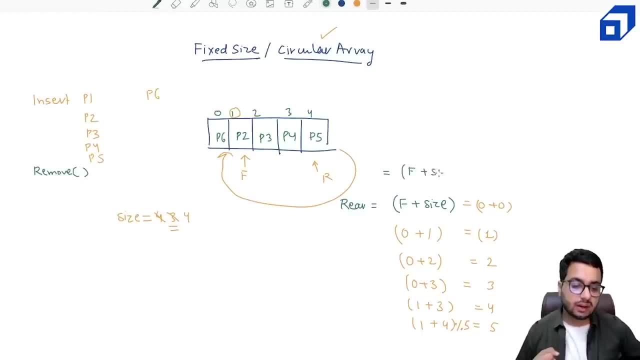 The rear will be updated by using front plus size mod of the capacity of the queue. The capacity is 5,. right, I have to take a mod with capacity. So that means if you hit the capacity, if the rear index hits its capacity. 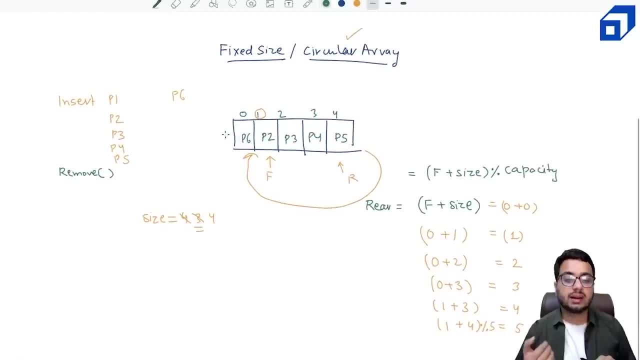 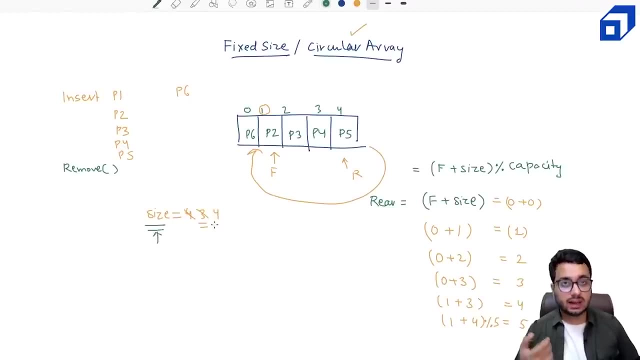 it will be again shifted back to 0.. So why did? your queue is not full. You have to check that. okay, if my size is 5 and I have only 4 elements, then I can add more. The size is 5 and I have already added. if the capacity is 5 and the size is also 5.. 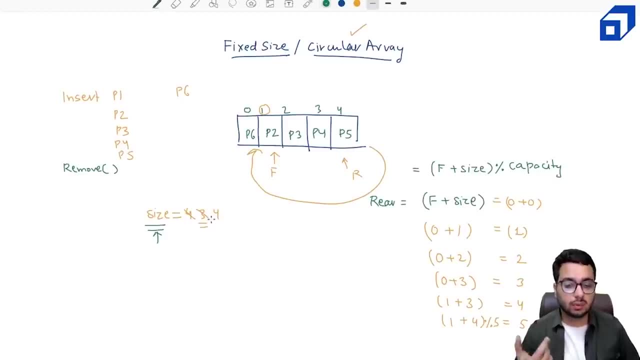 In that case I will throw that. the queue is full. I cannot insert anything more, right, So I will insert. So I will insert it here right Now. my front is still at P2, right Front is still at P2, but my rear is here, right? 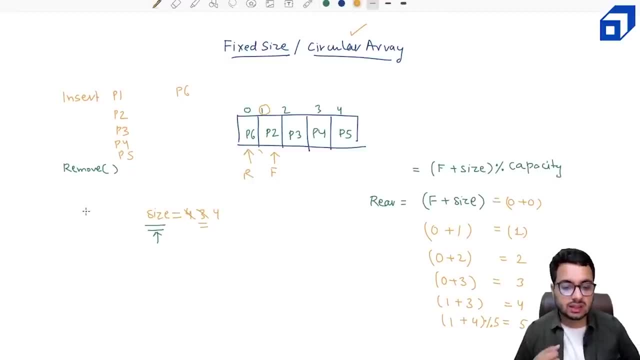 Now someone says, okay, I want to remove something. or let's say, I want to insert something right Now. what is the size? The size is 5.. Can I insert something more? The answer is no right. So what? you will check that if your size is equal to the maximum capacity that we have allocated. 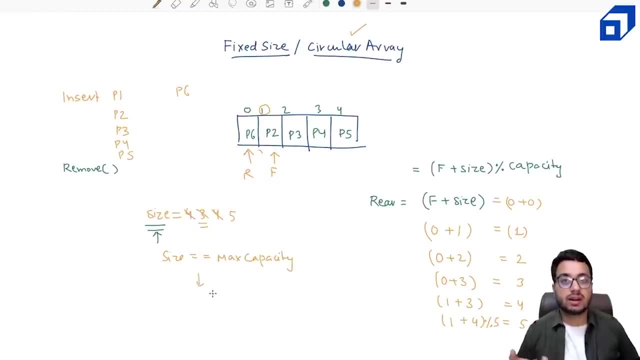 I cannot insert anything into the queue, So I have to throw some kind of error. that queue is full, right. Now again, let's say I want to insert, perform the remove operation, right. So how I will do it. 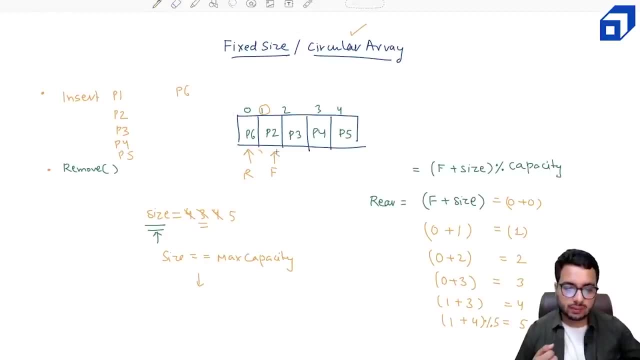 I will just find I will move this front from here to here. I will reduce down the size from 5 to 4 and this makes that P2 is not there, right? So P2 is not there. I will either make it 0 or I will just keep it like this, right. 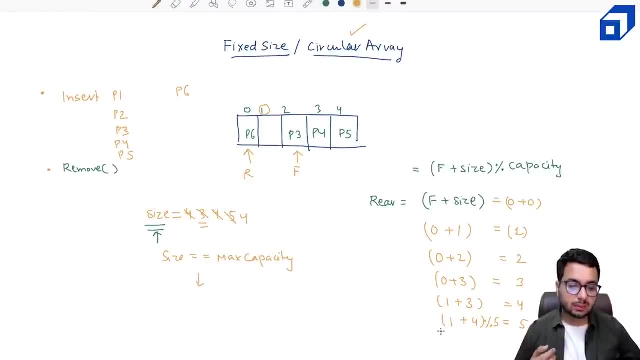 Now I can insert something. right, I want to insert something. So what is my front? Front is at 2.. What is my rear? Sorry, what is my size? The size is 5.. So 2 plus 5 mod 5.. 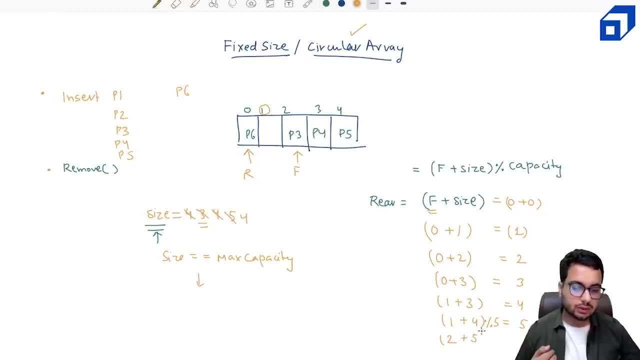 It gives me 2.. Oh sorry, The size is actually 4.. The size is 4.. So 2 plus 4, that is 6 mod 5.. It gives me 1.. 2 plus 4 mod 5, it's 1.. 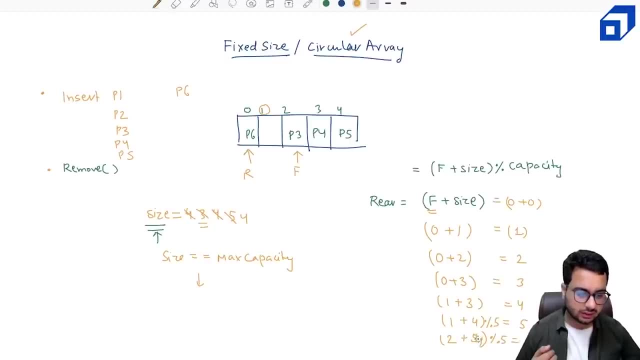 That means the rear should come here and the next insertion will happen at this index. So if this is the case, I will insert something. So what is the size? The size is 5.. The size is 1.. So what is the size? 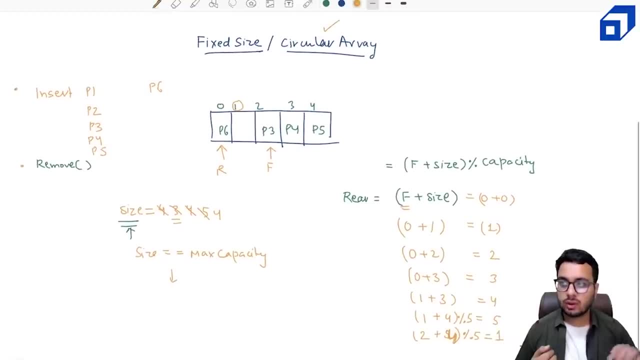 The size is 2.. So what is the size? The size is 1.. So what is the size? The size is 2.. So that means the rear should come here and the next insertion will happen at this index. 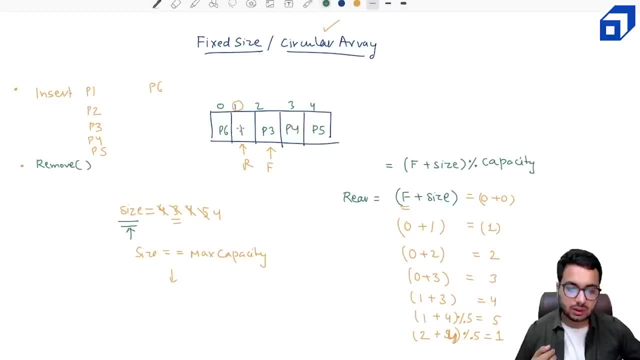 So if P7 comes, that person 7 will be stored at this place. Again, if you want to remove something, you will remove from the front. So the front is P3.. So you will read the elements in this order. 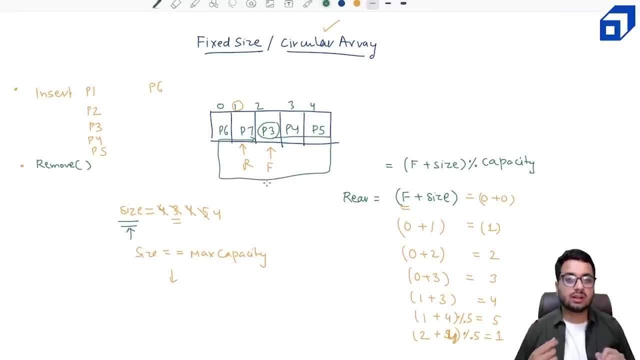 The elements will be removed in this order. One thing you have to notice when you are moving your front: your front will also go like this: It will go to P3., P4., P5. And again it should come here. 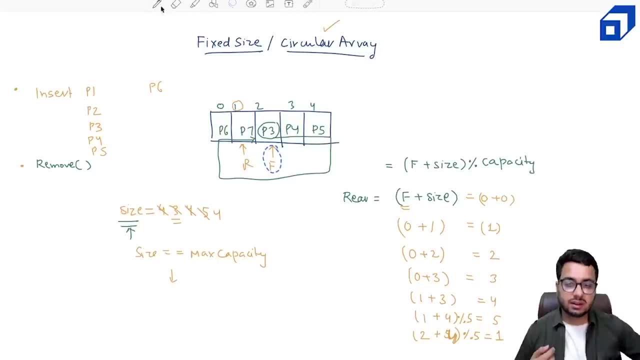 P6., P7. Basically, what I am trying to say is that when you are doing this operation that front will move like F equal to F plus 1.. Here also we should do mod with the capacity so that both front and rear move in a circular. 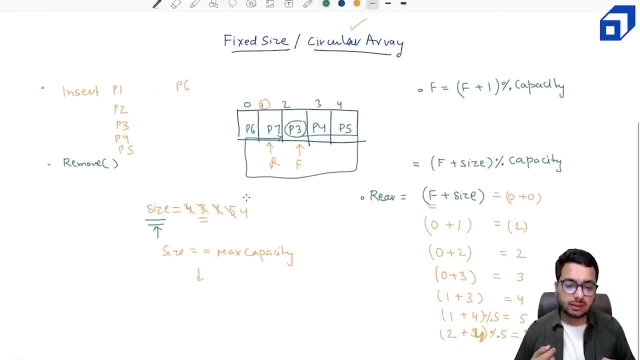 fashion inside there At any given point I have to check: if the queue is full, I cannot insert something. If the queue is empty, I cannot remove something. So we have to handle two cases that if size equal to maximum capacity, I cannot insert. 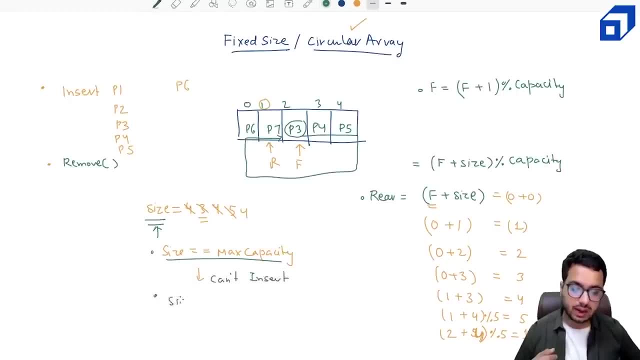 And if the size is 0, I cannot remove. So these will become our special cases in the code. So I cannot remove. So I hope you understood the logic for the fixed size queue. and now we will jump into the implementation. 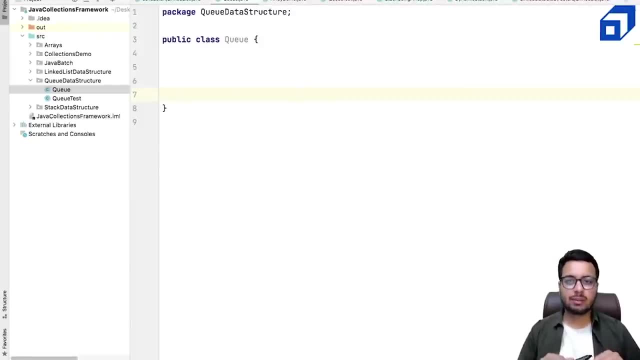 Let us start implementing queue using a fixed size array. I will be using Java, but you can use any language of your choice for the implementation. Let's begin. The first thing I will need to do is I need to create a class queue and I need to define. 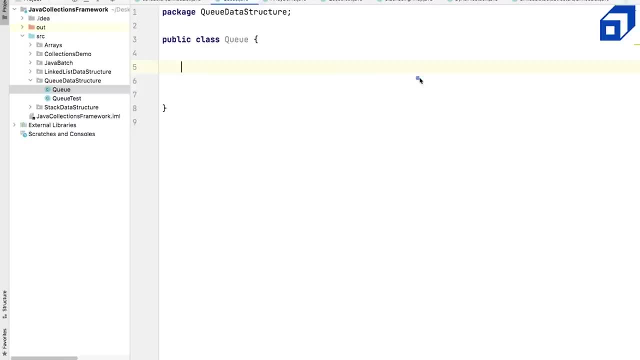 few data members. So, as we have discussed earlier that if you are using a fixed size array, we will need an object reference to store this array. So you can call it anything, I am just going to call it as ARR. 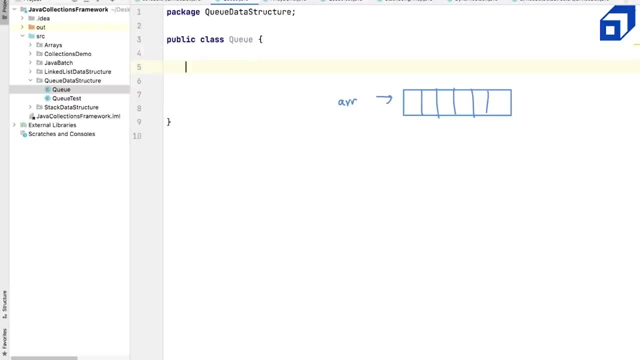 So let's create this variable data member, So I will simply call it ARR. Okay, This is private, It's an integer array and I need to define what is the maximum capacity of this queue, So that I will define using a constant, because I am taking a fixed size array. 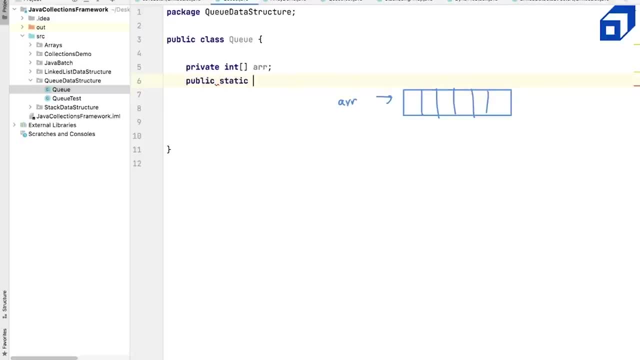 Well, it's okay. Fine, This constant will be a public static final int, called as default capacity, and this is equal to 10.. Now one thing: I need to notice that if someone is inserting data into this queue, what is the current size of the queue? 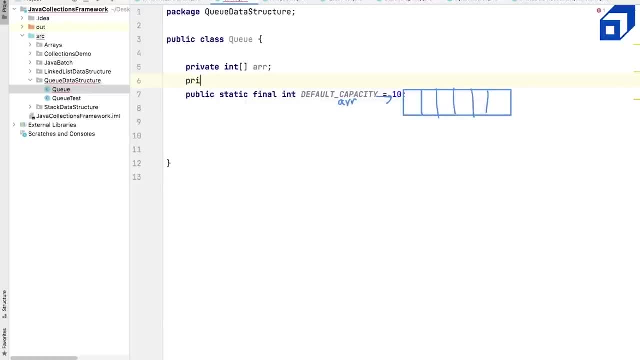 So I will take another private variable to denote the size of the queue. Now, in order to perform operations like insertion and deletion, I must know the front of the queue. So I will create another variable that is private int, and I call it as front. 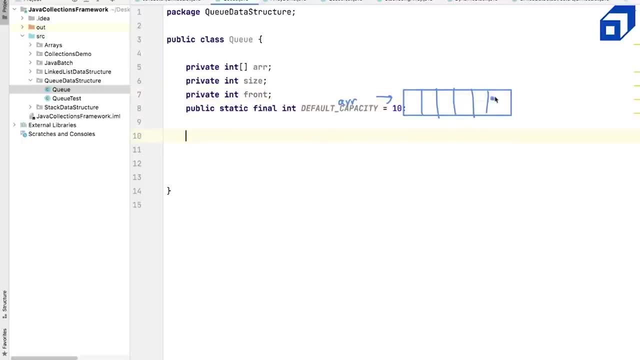 These are the four data members that we will need. So one is your capacity. Let's say that is 10.. Then there is your front, which is initially at zero, And there is size, which will be also at zero. Now we need to initialize these data members. 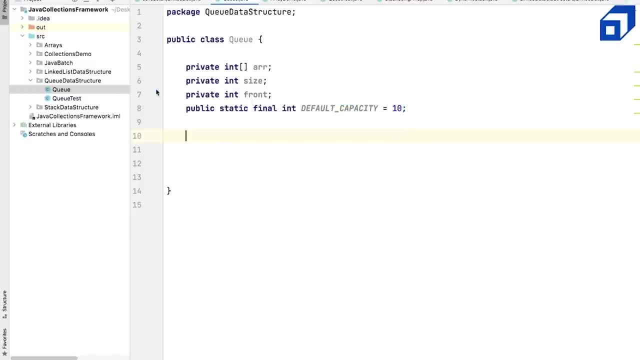 So that part we will do in the constructor for the queue. So I will define: Let's create a constructor and in this constructor I am going to create a queue, So maybe I am going to get some capacity as input. 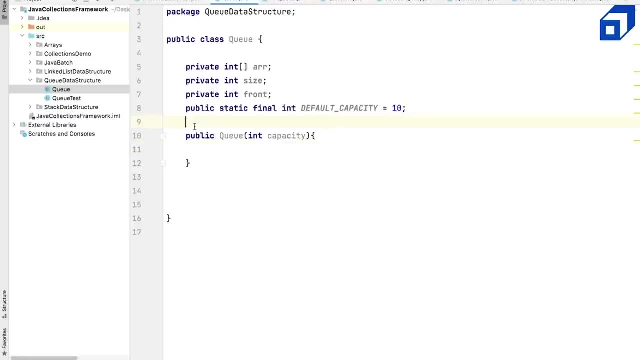 If nothing is given, I will use the default capacity. So I will create actually two constructors: One is the parameterized accepting Capacity and other one does not accept any capacity from the user. So in this case we will use the default capacity. 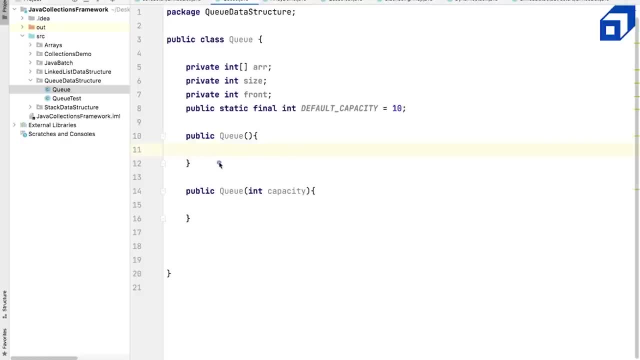 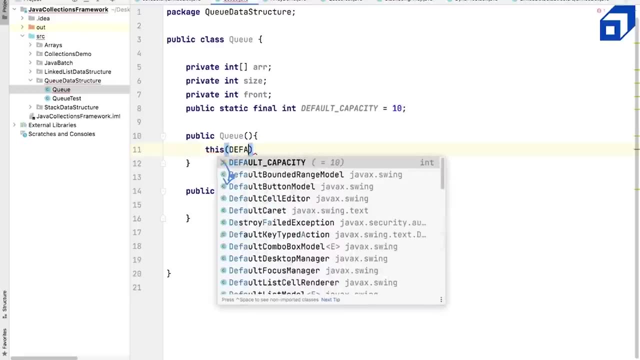 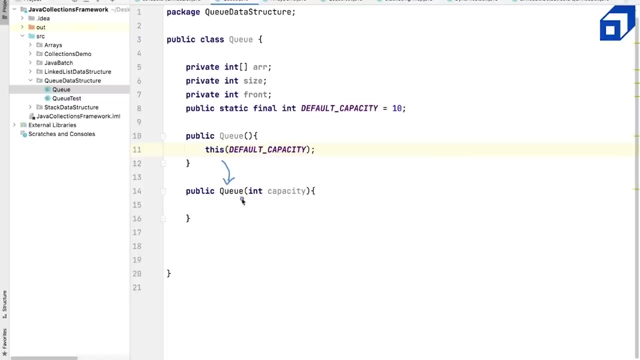 So one thing we can do is from this constructor we can directly call this and we can say: fine, You can call this constructor and give default capacity as a parameter to it. So that will help me to avoid creating an array here, and that part I can do directly. 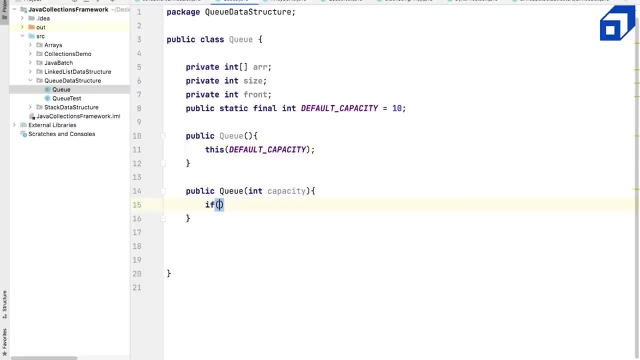 here. So let's see how we can do it. Now, if my capacity is less than one, if someone gives a wrong argument, maybe a negative capacity, In that case my code should throw an exception. So I can say: throw new exception, that invalid capacity you are giving it to me. 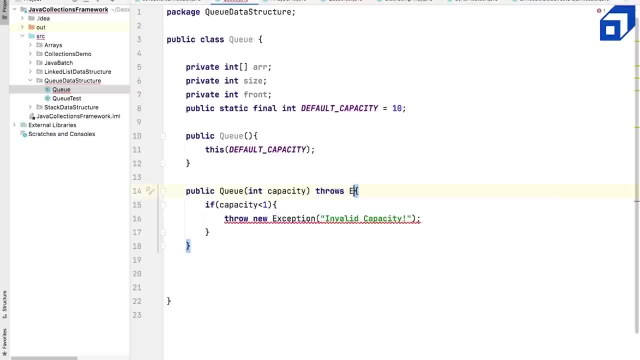 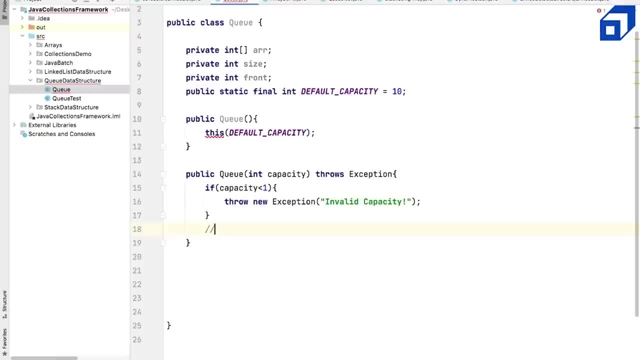 And also we need to define that this throws an exception. All right, So let's do the actual work. Actual work is that we need to initialize this array. So I need to say that fine, This array that I have. 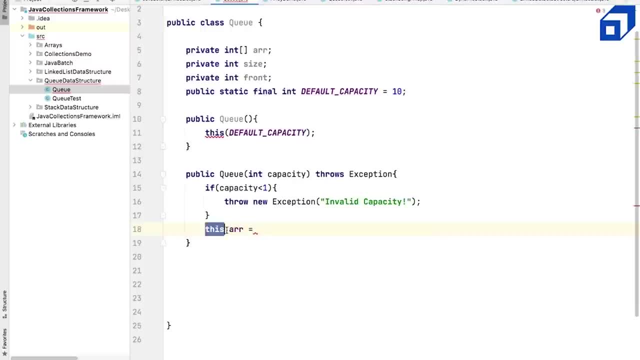 Again, I'm using this, which is optional here, But it's a good thing to do, because you are clearly referring to the data member of the class. So this dot array should be a new array of capacity. Now this capacity can come as an argument from the user directly. 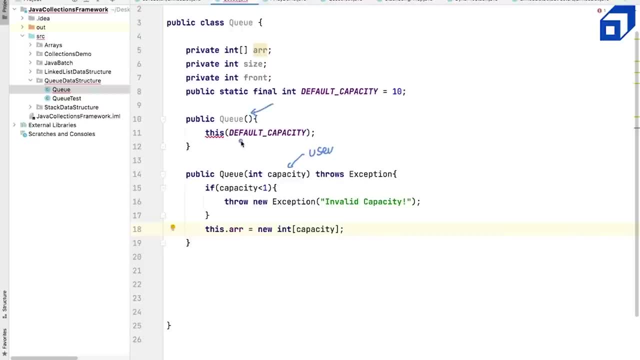 Or if the user does not give, then this constructor will be called and this capacity will come from here. That will be your 10.. And here also we need to say that this method can also throw an exception. So this is how we have initialized our array. 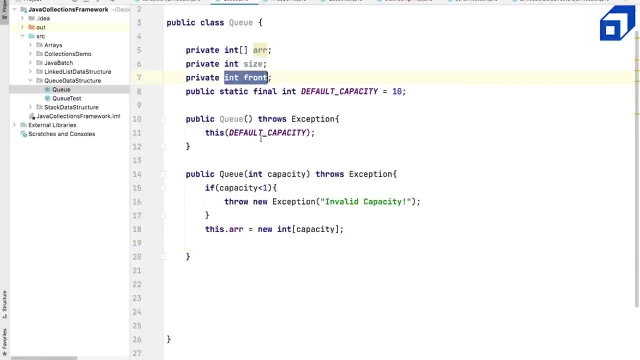 Now we need to initialize the size and the front variables. Initializing them is pretty easy. So I can say: this dot size, it is 0.. And this dot front, that is also 0.. All right, So I hope this is clear. 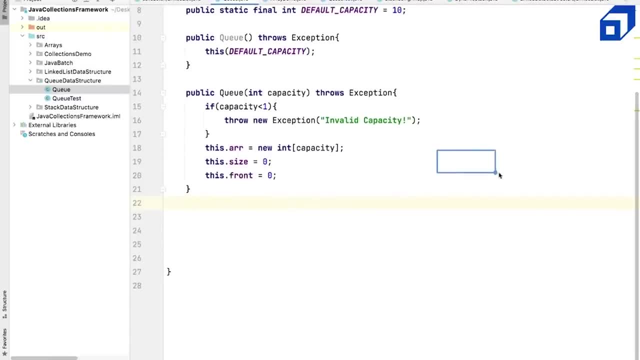 So we have created a new queue of given capacity. It can be fixed size, It can be given by the user as well. Right, So we have a capacity. right, Let's say capacity in this case is 1,, 2,, 3,, 4,, 5,, 6.. 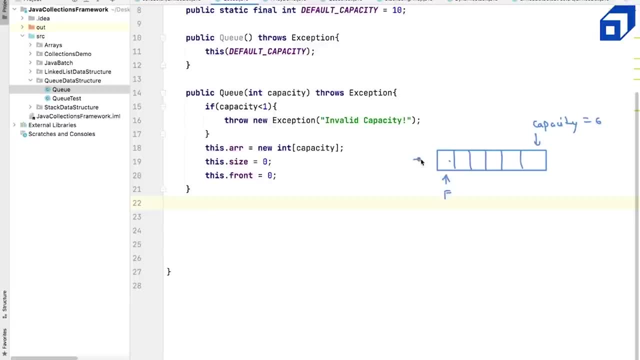 So capacity is 6.. Front is 0. Error is referring here And the current size of the queue is also 0. So the queue has been initialized correctly. Now the next operation that we need to build On this queue is NQ. 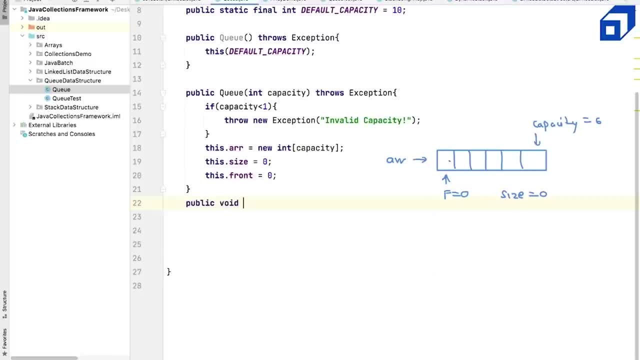 I want to push something into it So I can say public void NQ, And I am going to get some data or value to add into this queue Now, since it is a fixed size queue and it is possible that queue is already full. 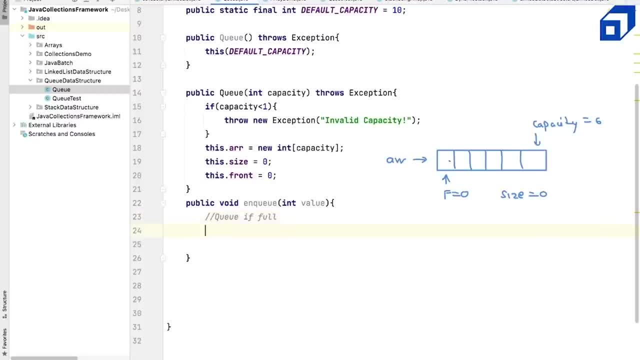 So how do I check if the queue is full? I can simply say that, fine, If the current size, if this dot size, that is my data member, It is equal to the capacity of the queue. So what is the capacity? 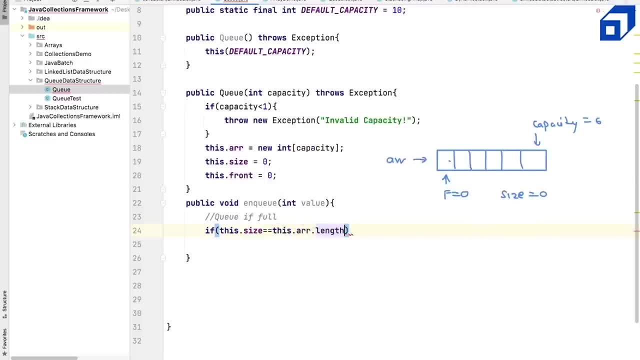 This dot array, dot length, Length of the given array, Then I can say: throw new exception. That my queue is. And here I can say that this method also throws a exception, But if the queue is not full So we can insert it. 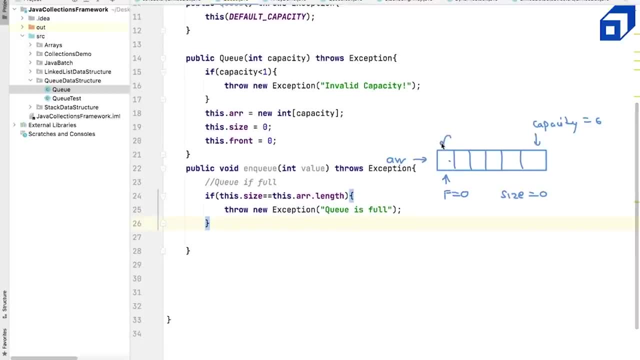 Right. So if the queue is not full We can say, okay, fine, We will push something at a rear index. So we will need to compute that rear index. Let's see how we can compute that So I can say the rear index. 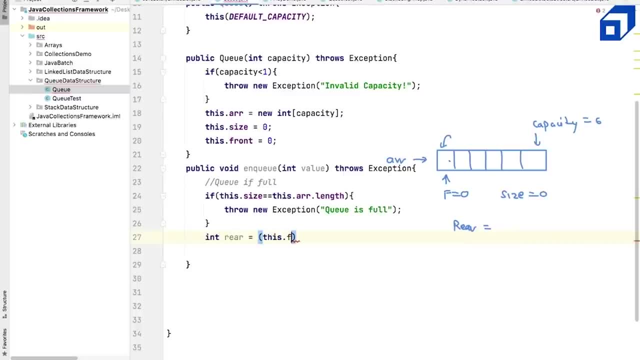 According to the formula, is the front index plus the size, And then we have to take the mod with the capacity, So that capacity is nothing but this dot array, dot length. That is the capacity Now. in this case, rear will be 0 plus 0.. 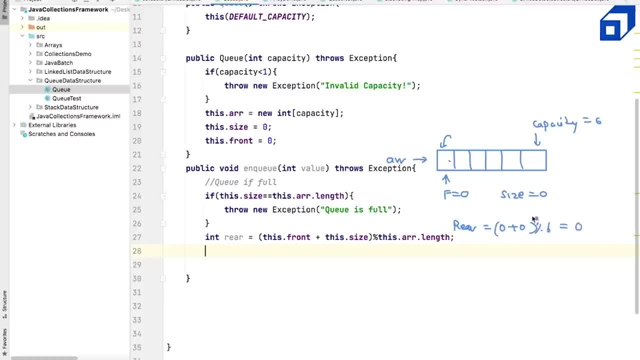 Mod with 6.. In that case it will be 0.. So I will insert something here, And then again size will also increment. So we will put the data, So we will say this dot array- at the rear index. 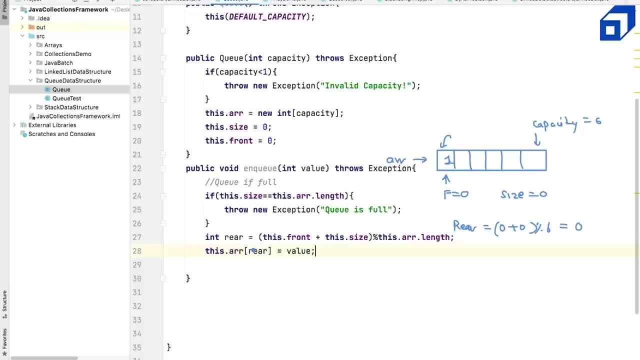 I want to put the value I am storing 1.. And I need to upgrade the size. I need to say the size is now 1.. So next time the rear would be 0 plus 1 mod 6.. Next time the insertion will happen here. 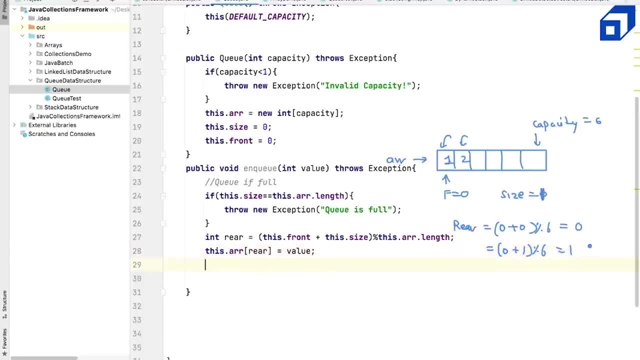 So maybe I push 2. So I will do the insertion at this index. So in order to achieve that, I have to say this: dot size plus, plus. So I need to increment the size as well. That's how the enqueue operation will work. 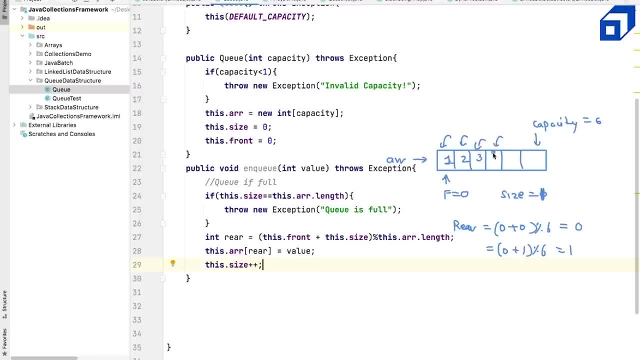 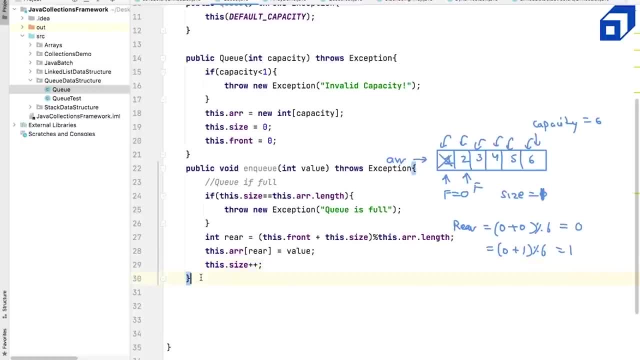 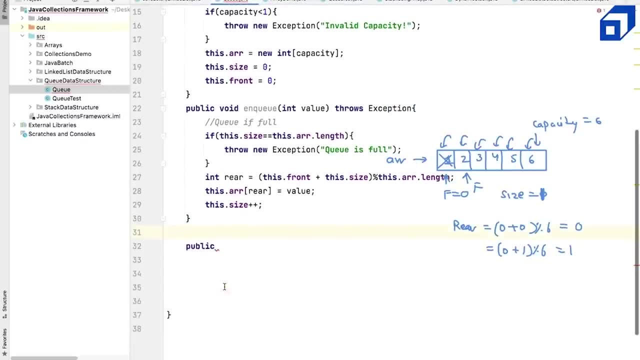 Now let us look at the remove method as well. So in that case We can call the method as public. Now, either you can make it as void or you can make it as int. So you also want to return what has been extracted from the queue. 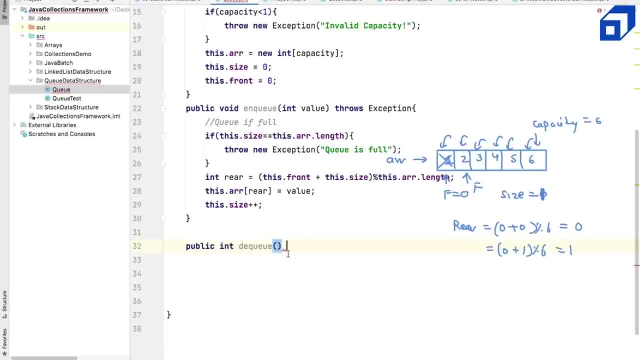 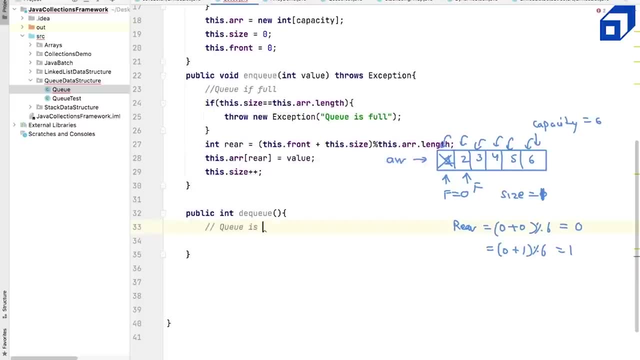 So in that case you can make the return type as int. Now this method can also throw an exception If your size is 0. That means queue is empty. You cannot remove anything from this queue If this dot is empty. 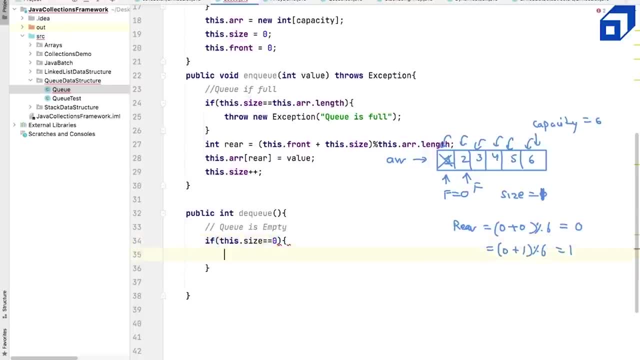 That size is 0. What you should do. You will say, okay, Throw new exception, that queue is empty. But if this is not the case, I can say: throws new exception here. Sorry, throws exception. But if this is not the case, 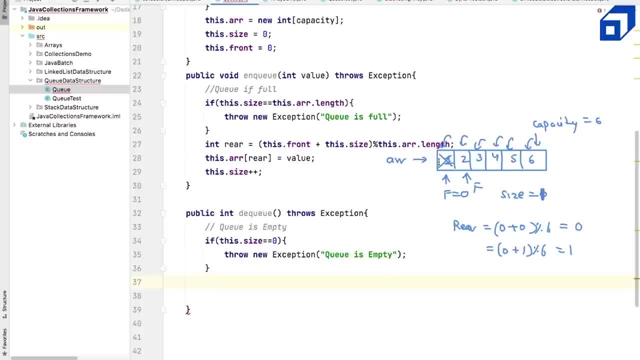 What we discussed, What we will do. So we will store maybe this data one, We will store this one here. We can say: okay, Our output, The answer that we want to return, Is present at this dot array of front. 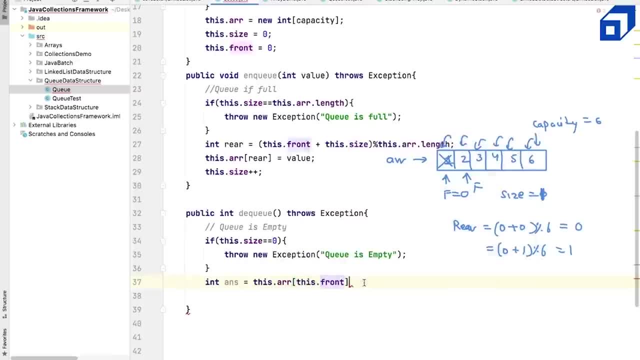 Right, Or this dot front, Whatever. Right. So you can definitely return this answer, But you have to update your front And you have to update your size as well. Right? So I can say, fine, This dot front will move. 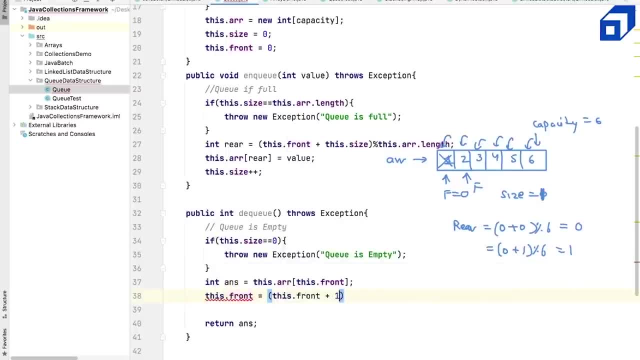 This dot front equal to this dot front Plus 1 mod capacity. So capacity is this dot array, dot length Right And the size will reduce This dot size minus 1.. If you remember from the diagram, This is what we discussed earlier also. 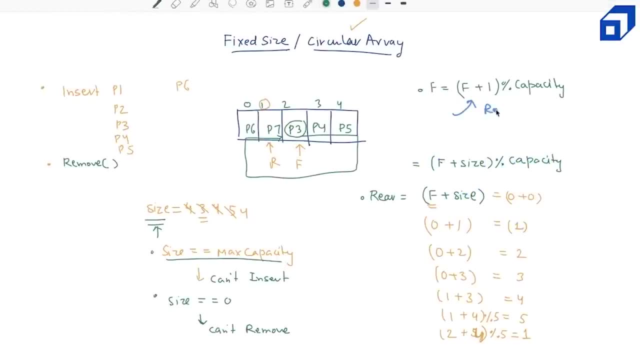 That this is how my front will change In case of removal Right. Okay, And this is how I will compute rear Right In the case of insertion Right. We have already discussed how it's going to work, So I am changing the front. 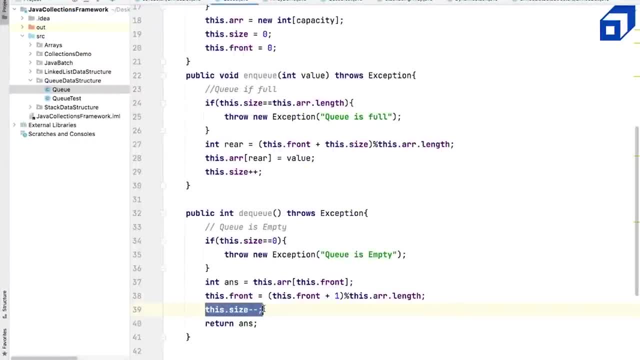 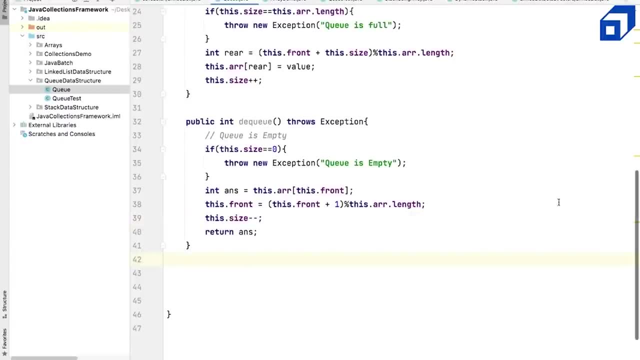 So I am changing the front And I am changing the size as well. So this is my DQ method Right Now. let us write some more methods that would be helpful. So one method would be peak If I want to look at the front element. 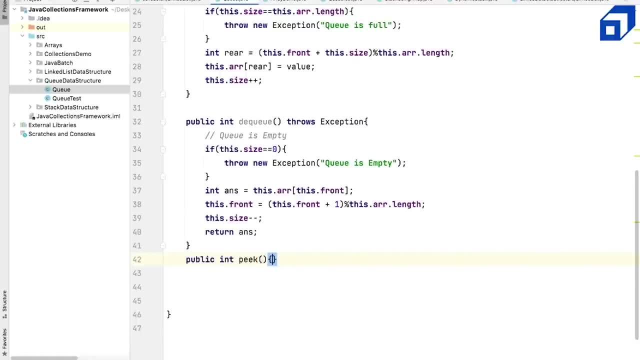 I can say, fine, Public int peak. Now, if again the queue is empty, I cannot look at the front element. So if this dot size is 0. I can say, fine, Show new exception. The queue is empty. Cue is empty. 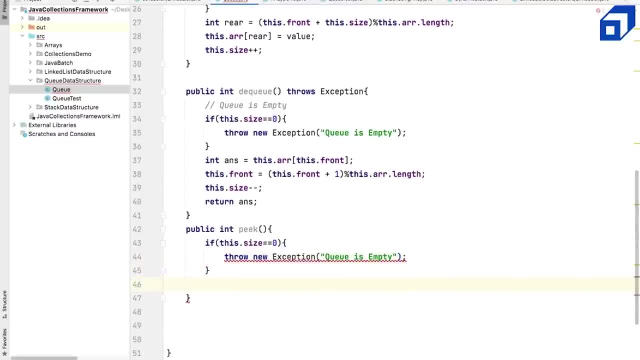 That means I cannot remove anything from this queue Otherwise. Okay, Let us just fix the error. Otherwise I can say: return The front element, this dot array of the Index, which is this dot front. Okay, That is my peak method. 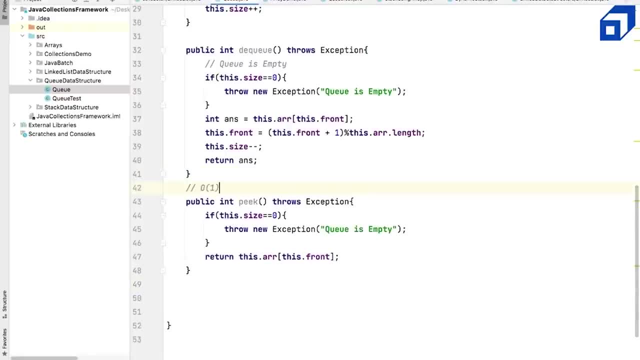 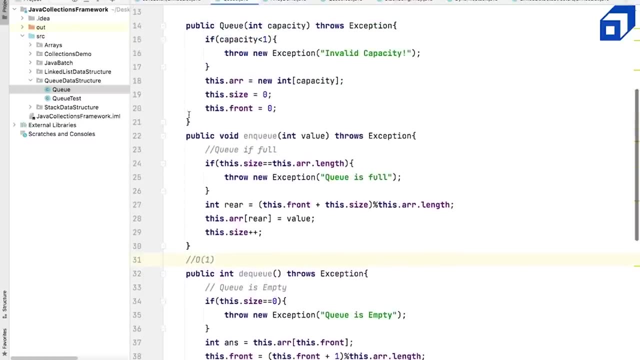 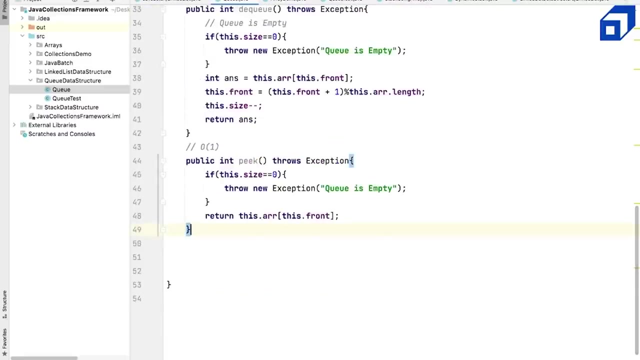 Return the front element. So the complexity of this method would be would be order one here also DQ method, it will be also order one. the insert method, that is also going to be order one. the constructors are also order one part from it. we can make two, three more methods. one is to check if the queue is 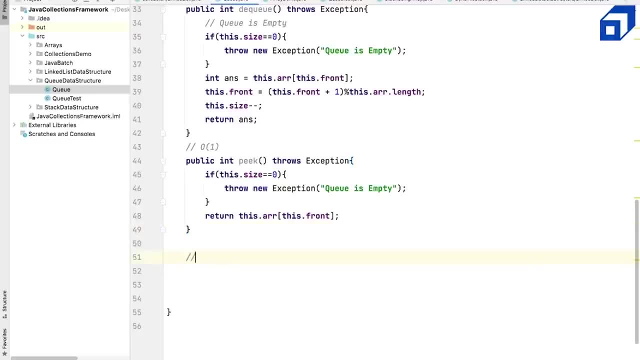 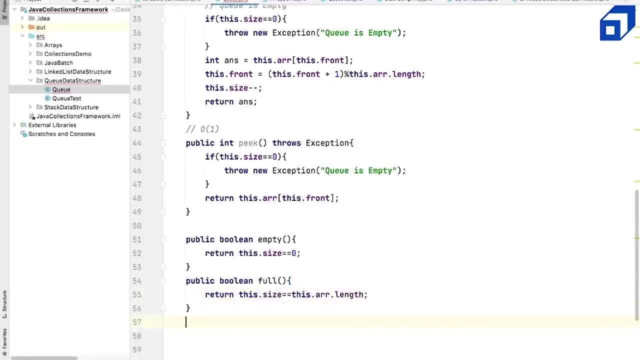 empty or not. that can be a boolean method. I can say public boolean is empty or just empty, right, I can return true, if this dot size is equal to zero. I can make a method called public boolean full so I can return if this dot size equals this dot array, dot length it. that will tell me if the queue is full. 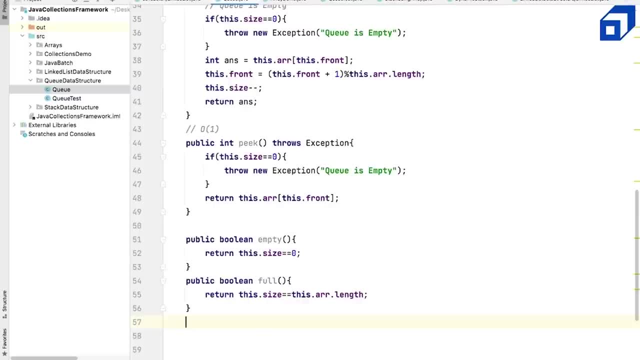 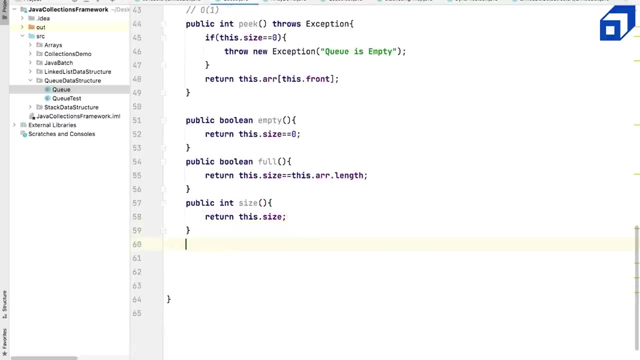 what else I can also make a method to get the size public int size. I can return this dot size from this method. anything else that you think would be helpful? maybe just a method to print the entire queue right? so maybe I want to display the entire queue right in Java and this method is called as to string which is present in. 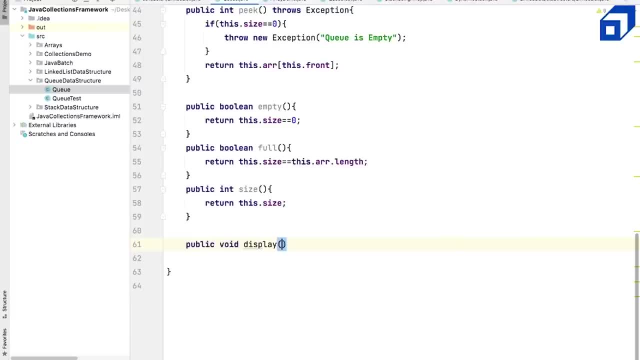 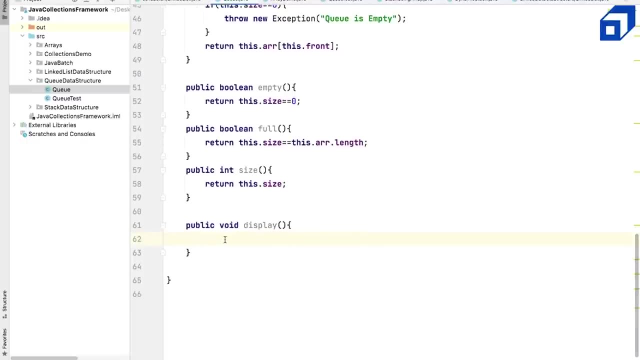 the default class. I need a way to look at all the elements of the queue, right you? so right now I'm not going to iterate from front to rear, I will just display the array. so it's more of a method for debugging, not for doing anything else. 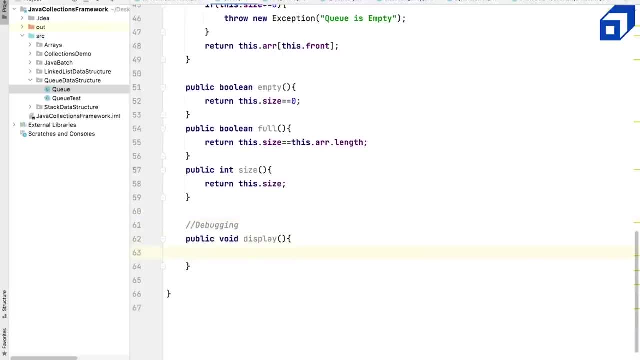 okay, I'm just going to print my array. or we can say: we can print. one simple way: you can do it s out arrays, dot to string and you can to this dot error, right. but now, instead of doing this, you can also say that, fine, I would print. 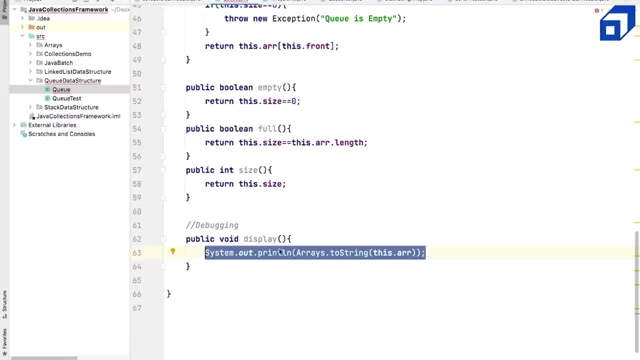 elements from rear to front. suppose this diagram is your queue, so maybe I want to print the elements from rear to front, right, or front to rear. so how I can do it right now, suppose if my front is at 2, right, I want to print, let's say, 1, 2, 3, 4, 5, 6. so I want to print all the elements from front to rear of the queue. I want to display all these elements. so my output should be 1, 2, 3, 4, 5, 6. so how I can do it? very easy, I can. I know this index, I can compute this. I can compute this. I can compute this. so this is f plus 0. this is f plus 1. this is f plus 2. this is f plus 3. this is f plus 4, right. so I want to print all the elements from front to rear of the queue. I want to display all these elements. so my output should be 1, 2, 3, 4, 5, 6. so I want to print all the elements from front to rear of the queue. I want to display all these elements. so my output should be 1, 2, 3, 4, 5, 6. so I want to print all the elements from front to rear of the queue. I want to display all these elements. so my output should be 1, 2, 3, 4, 5, 6. so I want to print all the elements from front to rear of 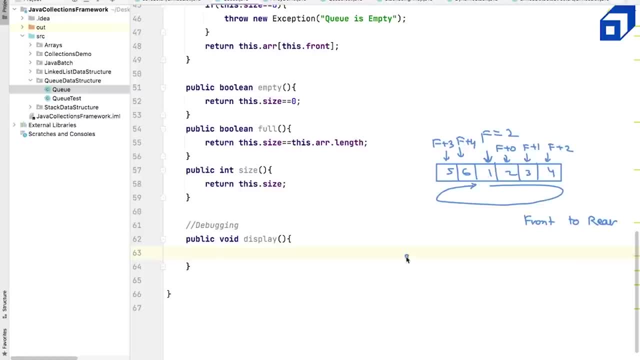 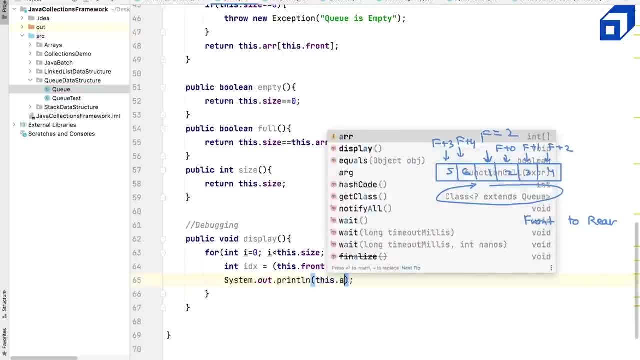 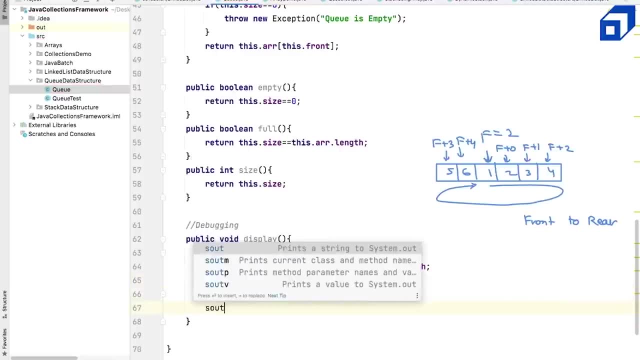 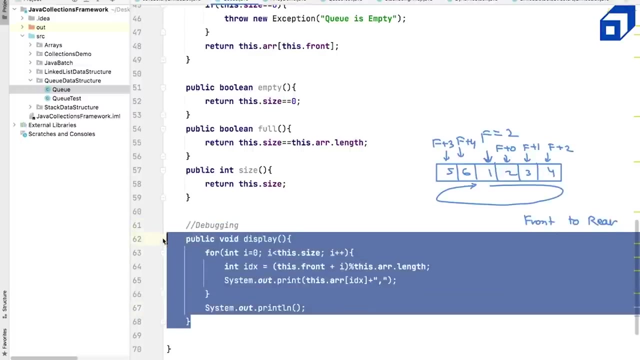 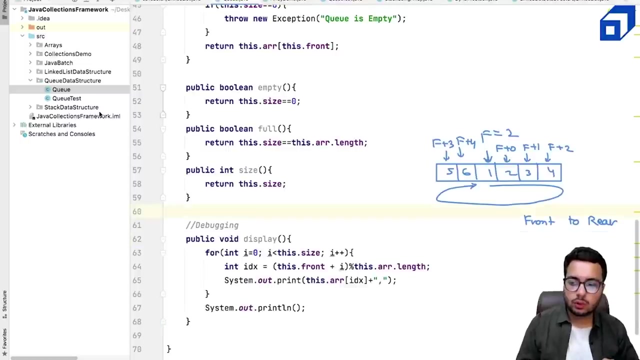 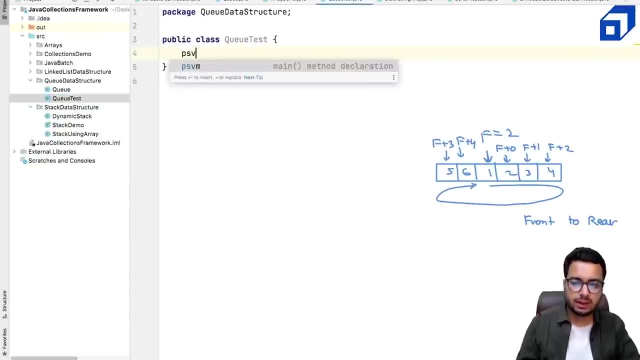 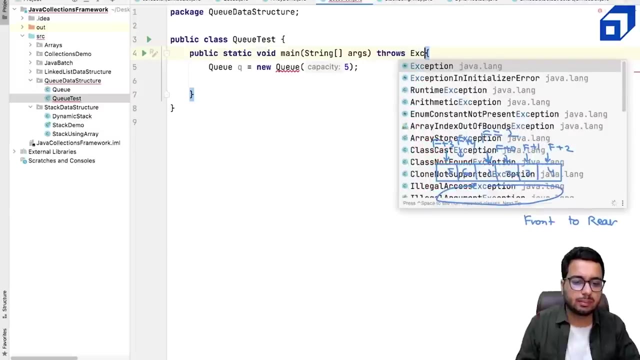 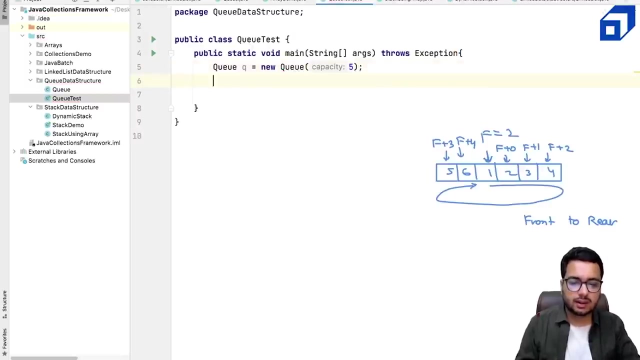 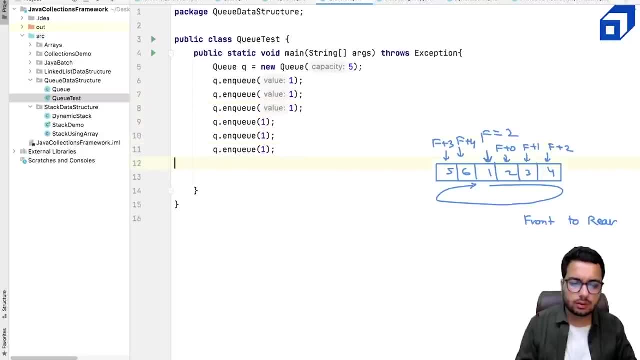 it's a two, three, four, five, then i remove something. let's say q dot eq, q dot eq, and then i can say seven and eight, and then i can say q dot display. right now let's see how this q should look like. let's go and run the code. 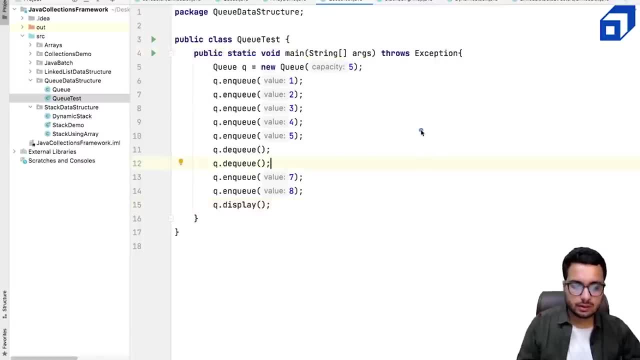 so i inserted one, two, three, four, five, so q was full. then i removed something right, so i removed this, i removed this, my front is here, and then i enqueued seven and eight. so seven and eight, they will come here right. so if i now print my q it should be like this: three, four, five and. 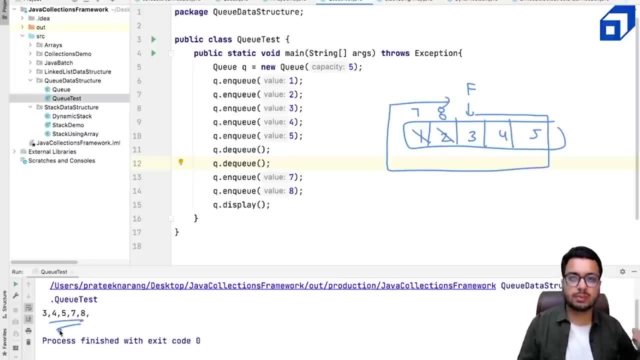 seven, eight, yes, that is what i am getting right. that means you can see that i have a q dot display right now, and then i can say: q dot display, right now, my q is behaving in a correct manner. the front element would be this. next front would be this: 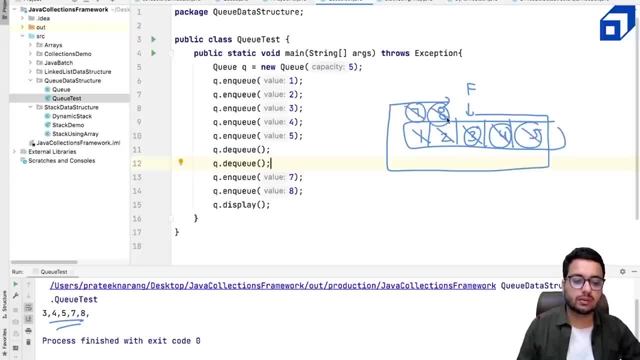 next front would be this, next one would be this. next one would be this. so i hope you understood the implementation of q using a fixed size array. next we will jump into the dynamic array implementation of the q. let us now discuss the implementation of a dynamic q right now, there. 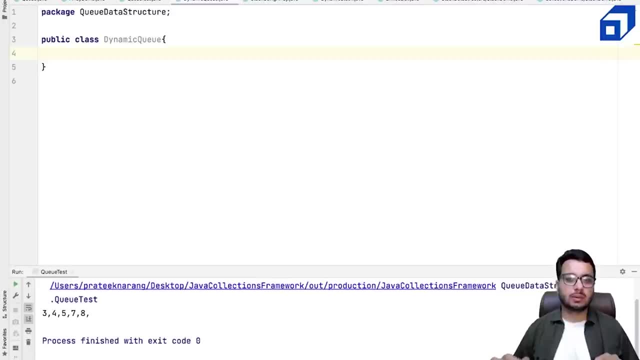 are two ways. one, you can use a link list or you can use a dynamic array as well. right so, in this implementation, i am going to show you how to implement a dynamic array as well. right now, i am going to show you how we can use a dynamic array functionality and we are going to extend the 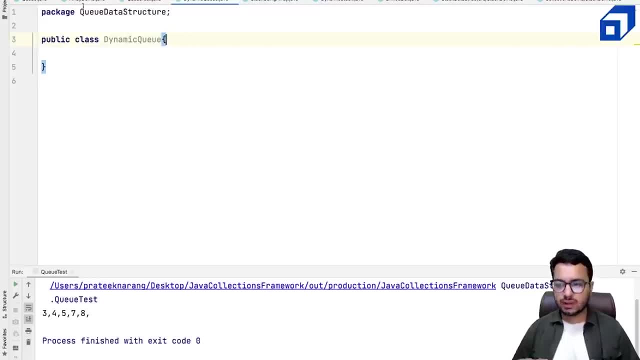 implementation of the q class by adding this functionality. okay, so q. we have already written what i'm going to do. i'm going to create a class called dynamic q, which will be the child class of the parent class. so dynamic q extends the q class. right now, one thing to notice: that this dynamic q 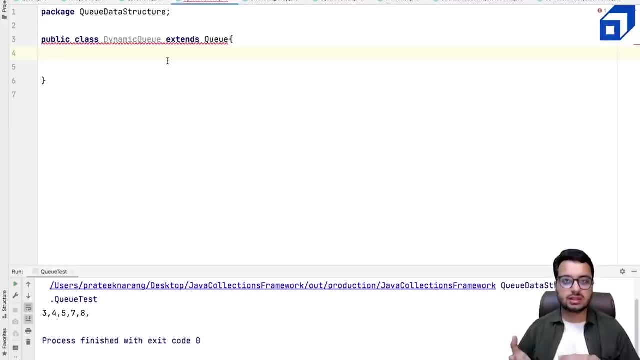 it's going to behave in a similar way, the operations nq, dq, peak. they will remain same. the only thing is the logic in the insertion operation, that is nq operation. it's going to change right. so first of all, let us start by creating the constructors for this class. so i 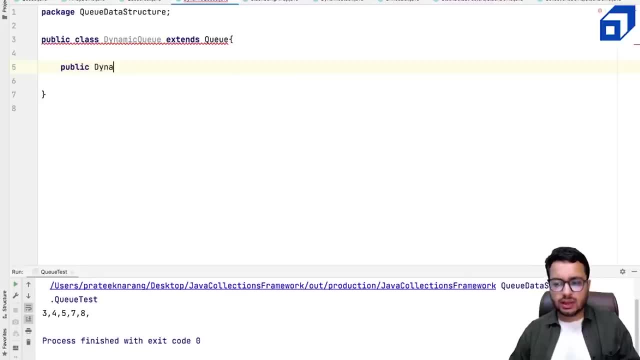 can say public dynamic q. again, there can be two types of constructors: one without the capacity and one with the capacity, right so, public dynamic q, where i'm going to accept some capacity right now, in this case in the first constructor, what i'm going to do, i'm going to simply call the second constructor with default capacity. so i can say this and call: 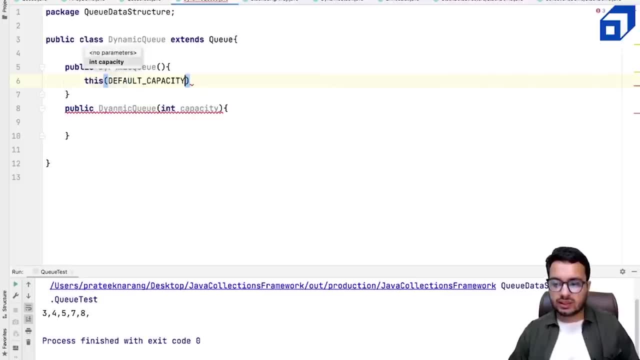 it with the default capacity. basically what is happening: if i want to create a dynamic q object in which i'm not getting any capacity, so i make a call here. if i get a call here, it again what i can do. i already know how to create an array of a given capacity. that i'm doing in the parent. 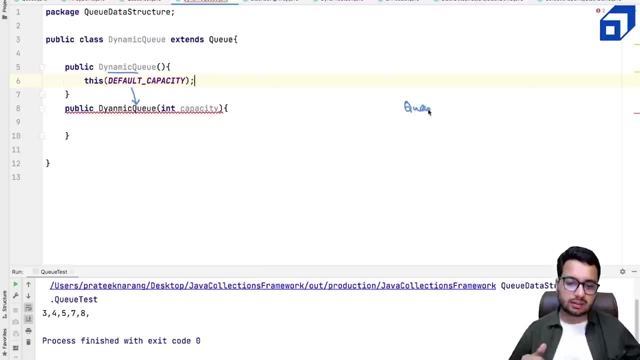 class, right. so q is my parent class, dynamic q is my child class. if i want to create a fixed size, error in both. so if i get a call here to create a dynamic q, i can redirect the call to the parent constructor. so i can say super and i can pass in the given capacity that i'm. 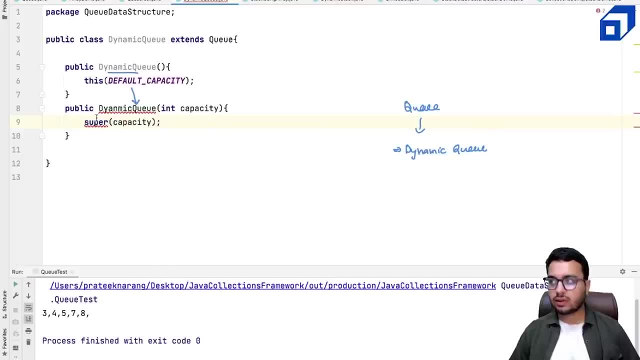 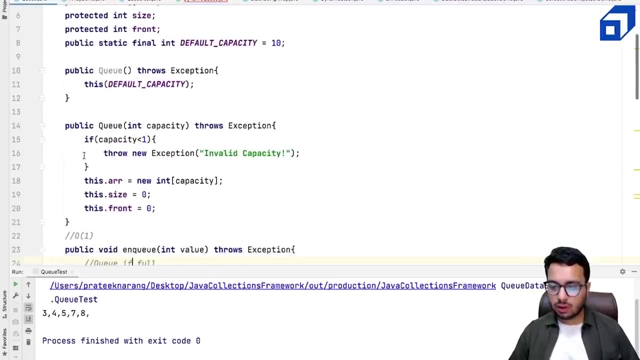 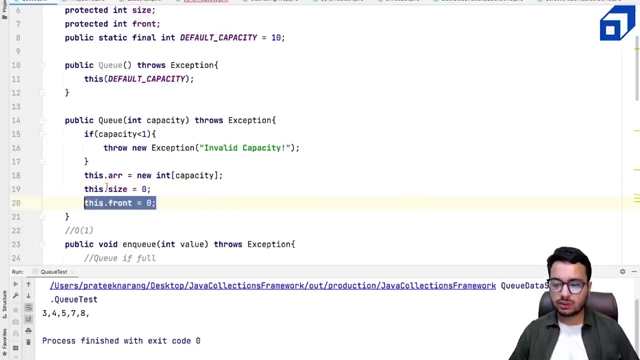 getting right. basically, i'm calling the constructor of the parent class. right now. this is a spelling mistake. dynamic now the parent class, constructor, if we look carefully here, right. so basically, what is happening? the call is going to come here to this constructor. so we are already initializing the array correctly: size is reset to 0, front is set to 0 and we are 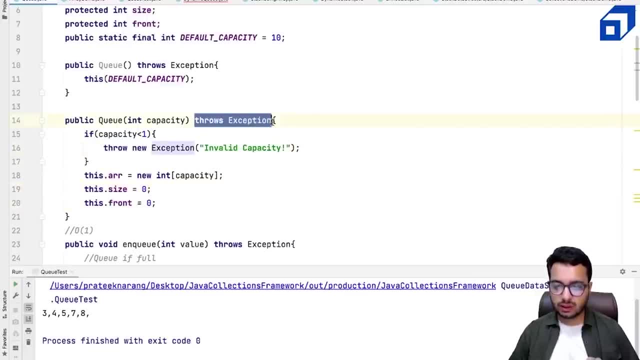 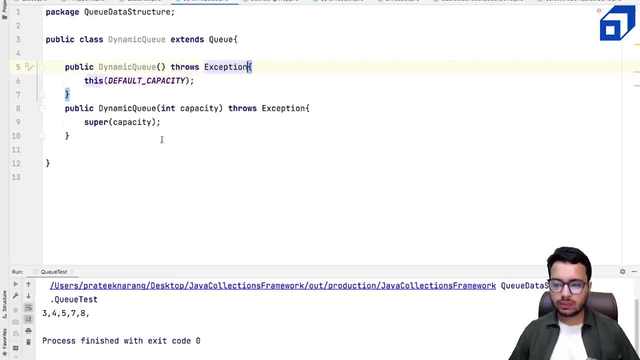 also throwing the exception. we can also say that our dynamic q can also throw an exception. this can also throw an except now the errors are resolved right. so constructor part is in now. there won't be any change in other methods except nq. let us see if i want to enqueue. 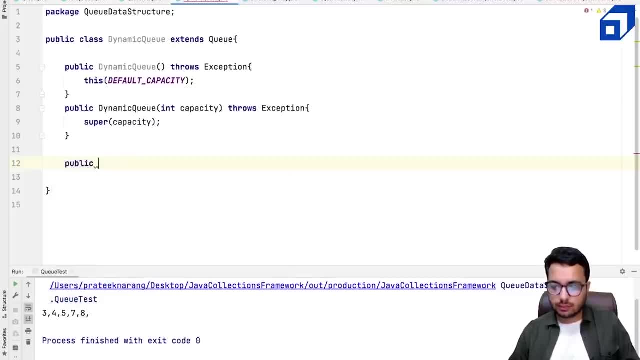 something. uh, let's say public void. thank you, so i'm going to overwrite the method that i have written for insertion. you can see we are overriding this method right. there are two things we have to do. we have to expand the array right and then we have to put the element. if the queue is full, okay, put the element right. expand if q is. 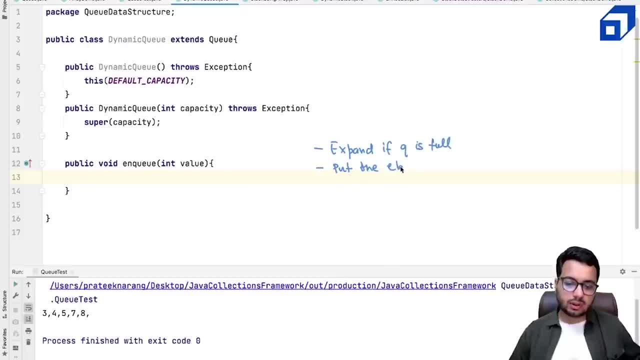 full. and then we have to put the element right now. this functionality we were not doing in the previous uh implementation. now we have to do the same functionality right now. assume that your q looks like this. so suppose q is like this: one, two, three, four, five, six, right. 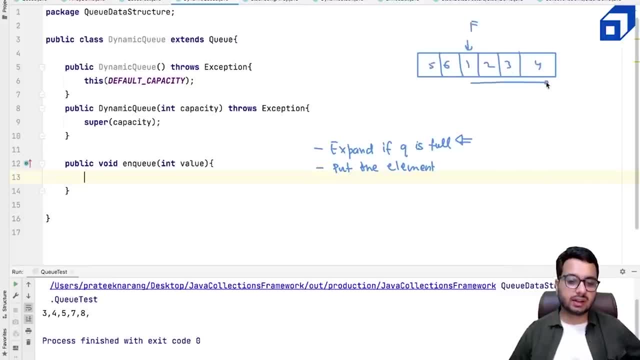 and suppose my front is here. that means if i want to read data, i will read the data in this manner, right? so my capacity was six, size is also six. that means my q is full right and i want to create a new queue, a new array, basically with double the capacity, right? let's just say that this is going to be. 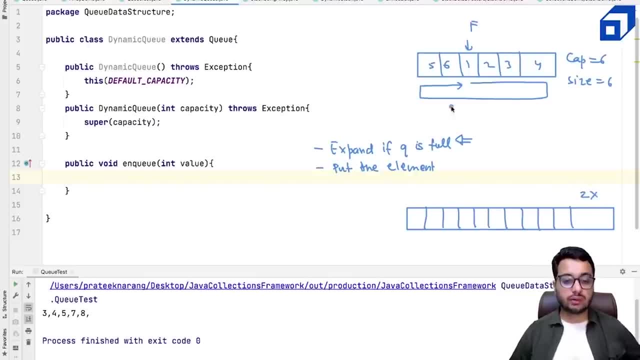 2x twice of the original capacity. now, if i want to copy this data, can i copy it directly? can i say i'll copy 5, 6, 1, 2, 3, 4? will that be correct? the answer is no. why? because if i want to do a next, 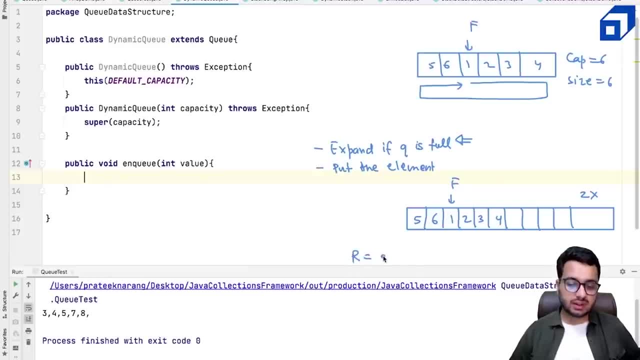 insertion, right. so at what index the next insertion happens? it happens at front plus size, right? so in this case front is at 2, fine, size is 6.. next insertion will happen at the 8th index. that means i will start filling from this index. but is it correct? the answer is no, right, because 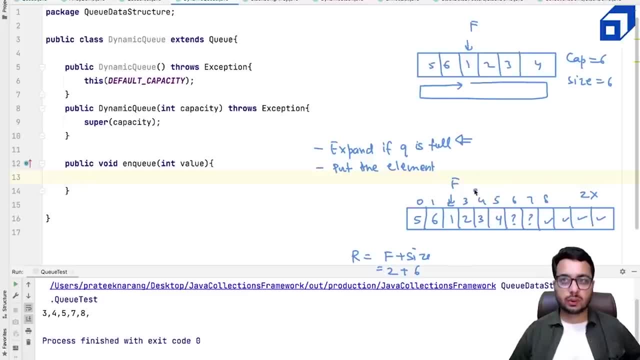 what happens at these places, we don't know right. so the correct way of doing the copy is: you create a queue of double the capacity, right? you iterate over this part. let me change the color. you iterate over this part in a circular way and you copy the elements here. 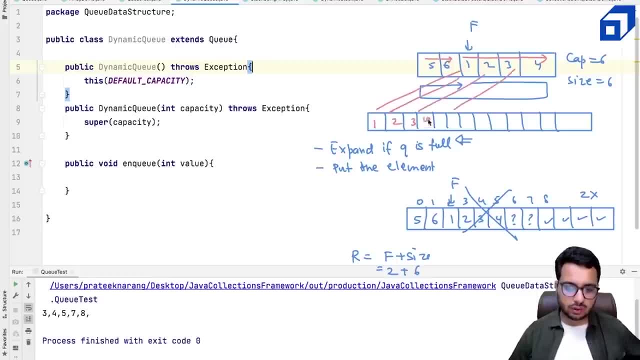 so you copy one, two, three, four, then you copy five, six. this is my front, this is my front now, if i want to do an insertion, so my rear would be front plus size. front is zero, fine, size is six. i'll start copying from the sixth index: 0, 1, 2, 3, 4, 5, 6. that is correct. so if i want to push something that, 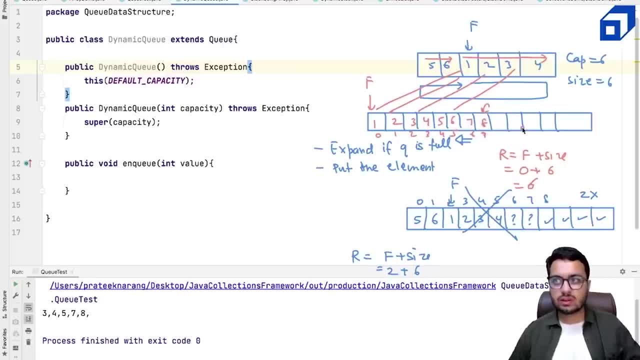 insertion should happen at these places. right, see how we can do this, right. so let's say: this is my original array, this is my temporary, in which i'm going to perform a copy. i will say if what? how do i check the size? if this dot size is equal to, 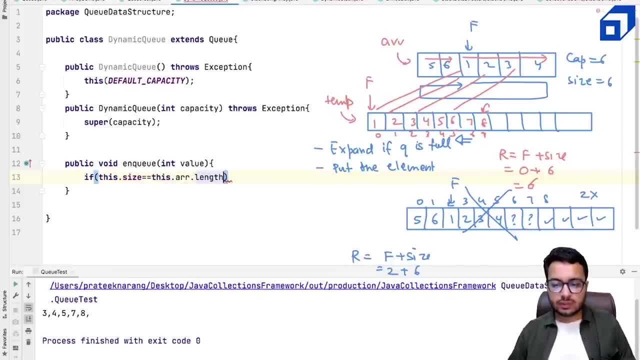 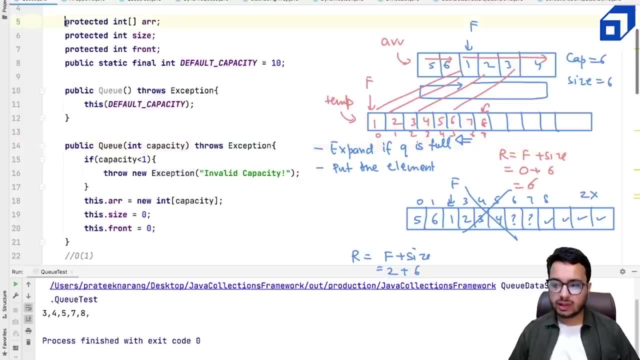 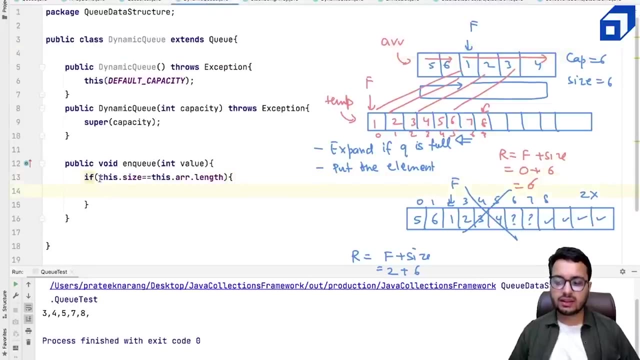 this dot array: dot length right now. one thing: you will notice that these members were earlier private. i've just made them protected. now, right, i've made them protected so that i can use them in the child class, right coming back here, so i can access the data. members of the parent class. 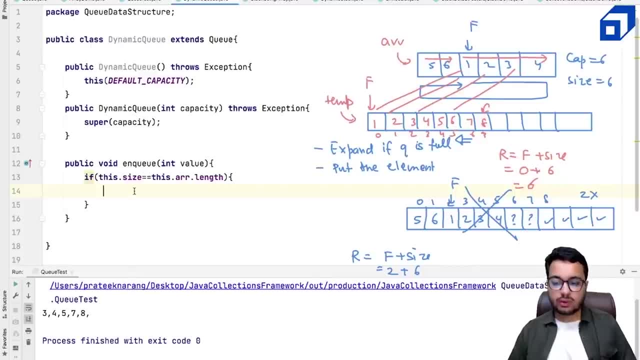 because they are now protected, right? so what i have to do? i have to create a new array of double size. so let's say there is a new array called temp that is equal to new end of size twice of this dot array, dot length. so this is created. now i have to copy the data. 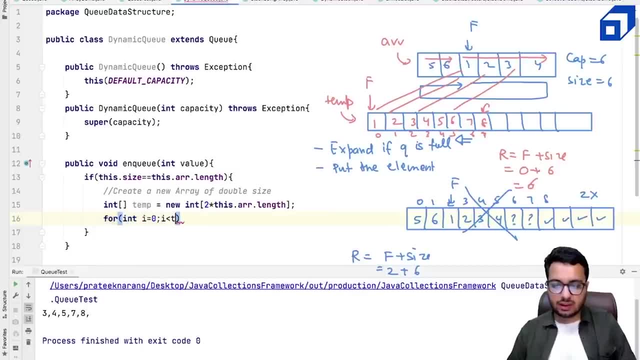 so i can default for int. i equal to 0, i less than this dot array, dot length. that is the size, right? or you can say this: dot size, both of them, they are equal. i plus plus, right? i'm going to run a loop these many times, right? okay, so i'm going to iterate over these positions. 7, 8 will come later, right, i need. 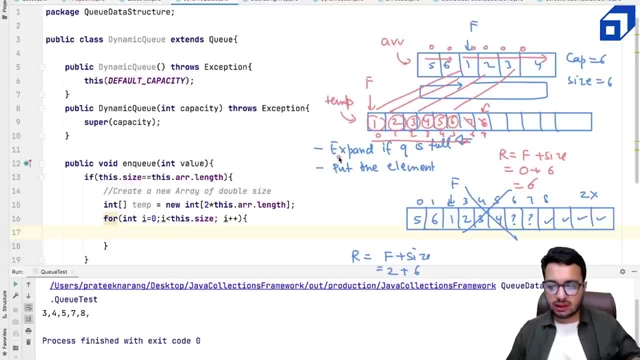 to copy these values right, so i can say temp of i. and at the ith index in the temp, what should i copy? at this index? what should i copy? i should copy the element from the front, so this is f plus 0. then at the next index i should copy this value: this is f plus 1. then this is f plus 2. 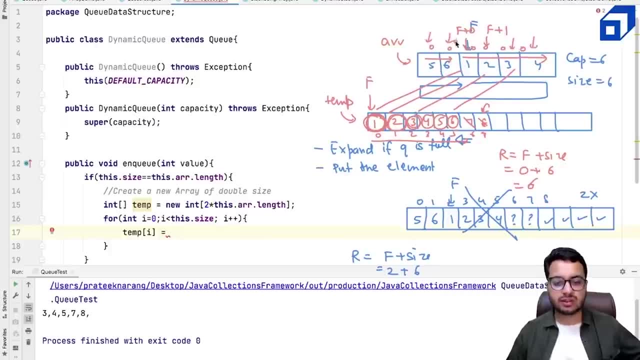 f plus 3, f plus 4, f plus 5 and so on. right, so i can say this is going to be equal to this dot array of- let's uh, find the old index. so this is going to be this dot original front plus the original size with the original capacity mod. right, so the elements are at the um at this. 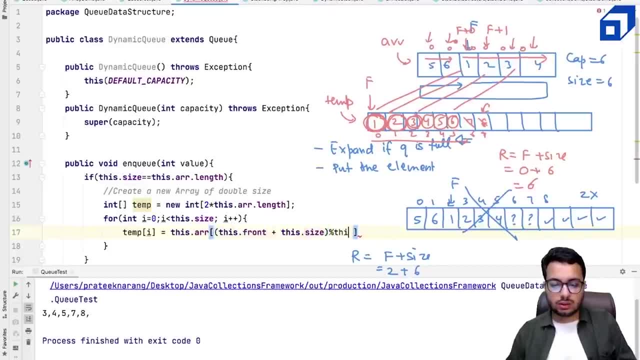 particular index right mod. this dot array dot length. this is what i need to do, right? sorry, this dot front plus this dot a plus i- sorry, that's a mistake- f plus 0, f plus 1, f plus 2, f plus 3, basically the ith element. 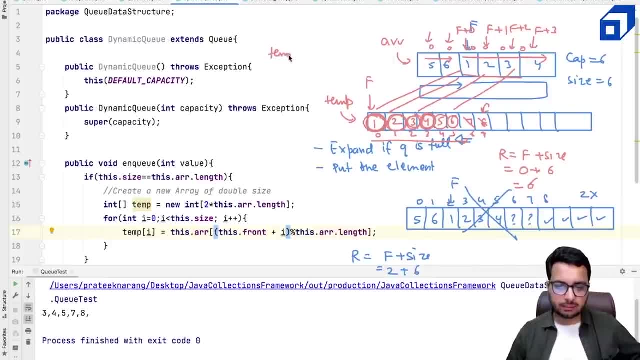 okay, so the element at, let's say, temp of 3 will be equal to array of f, which was, let's say, 0, 1, 2 plus i. i is 3 mod 6. it will be array of 5. the fifth index: 0, 1, 2, 3, 4, 5. so that element is 4, that's. 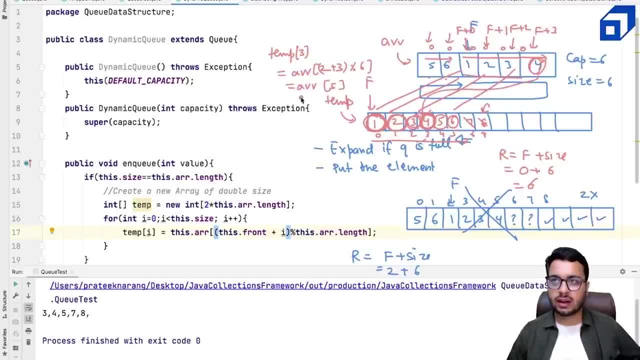 correct. so at the third position i'm putting the value, that is, 4, right arrow 5. this is what i need to do, right. so, just like we did in the display method in the queue, that is the same logic we are using here. right once this is done. 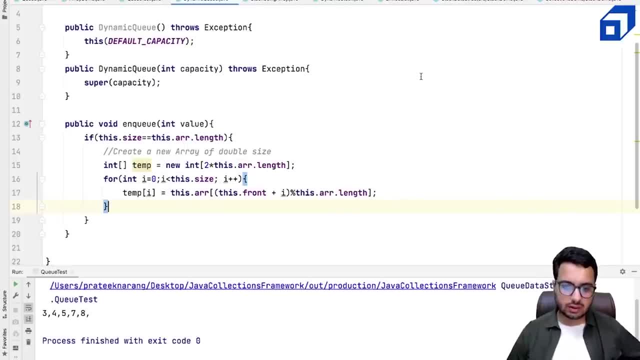 temp array has been created, right, so i've erased all of it. i'll just do it once again. it was like: 1, 2, 3, 4, 5, 6, right, this is my front now i've copied this data like this: 1, 2, 3, 4, 5, 6, so i have to reset the front here. right, this should be the new front. 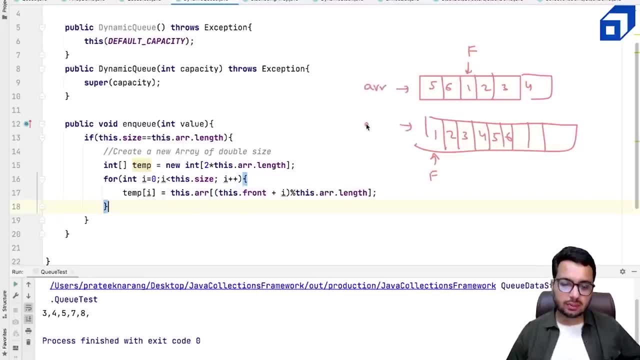 okay, and this was my array. this was my temp right. one thing i need to change is that this error should refer to this memory. this connection should get broken. i can see this dot error. this will be now referring to temp object and now doing this, no one is referring to this memory. 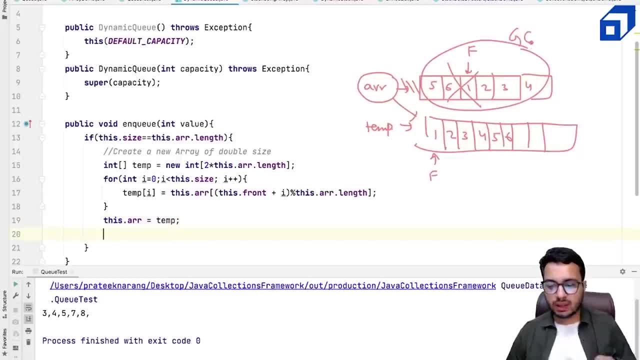 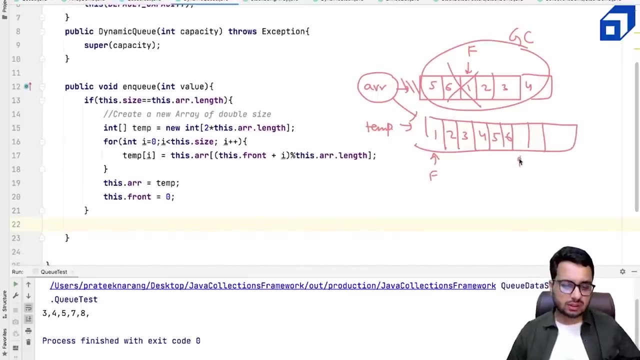 so garbage collector will clean up this memory and this dot front will be set to 0, right. but have i really done insertion? as of now? the answer is no. we have still not done the insertion part right. so how do i insert? i can say, fine, so what i've gotta do is estrogen. 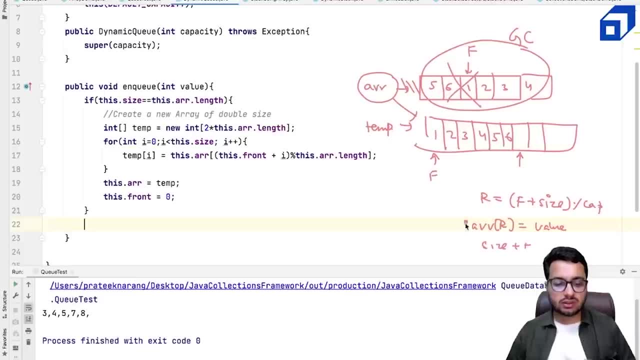 because i've not already done this null ending yet what sorry. i had left something for future, so i will ever do the anyway. sorry message. output time is open right now. i'llhoo a machine Vaad now. this method will get to know that the array has been changed because error is now referring. 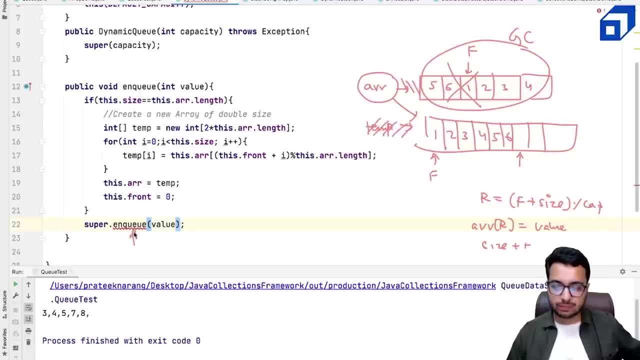 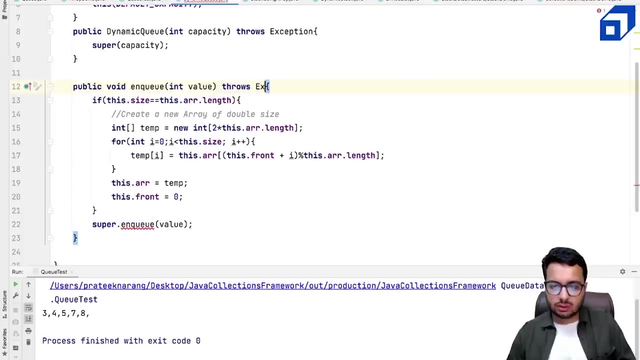 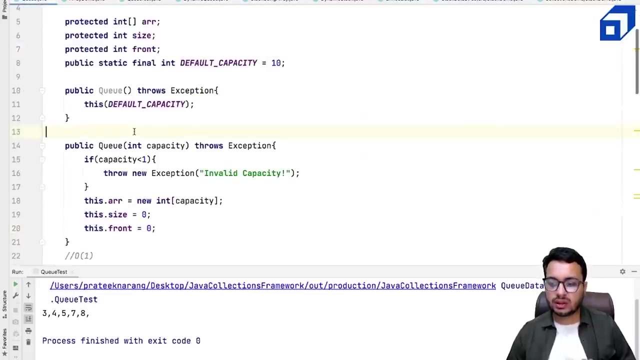 to this memory, right, and it will try to push something into this method, uh, something into the new array, because we have changed arr, which is now referring to the new array, right? so i can say this method can also throw an exception, shows exception. this error should get resolved. let us look at the nq method of the parent class. so here what is happening? this is: 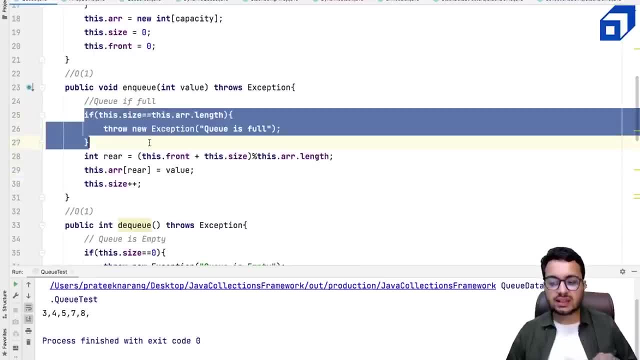 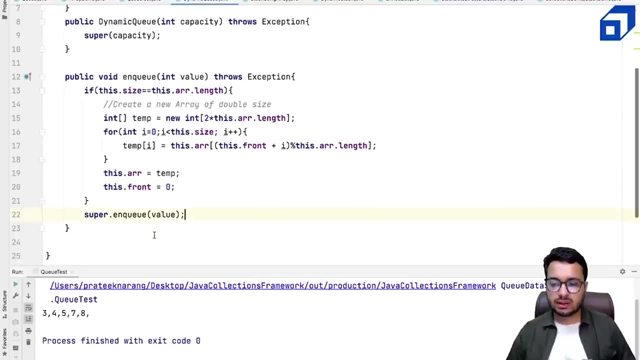 what we are doing right now. this condition is handled in the child class. if q is full, double it. when you come back into the parent method, this condition will not be true. what code will execute? this code will execute. right, that is how we have implemented dynamic queue using a dynamic array. 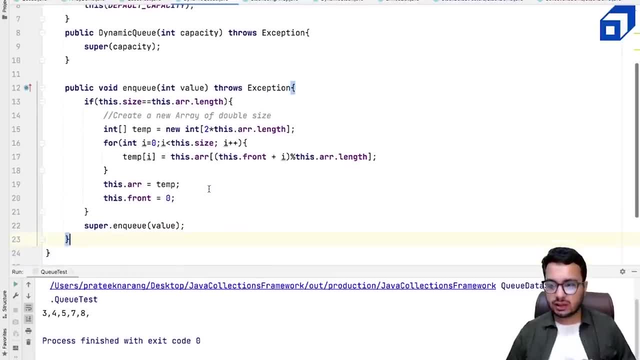 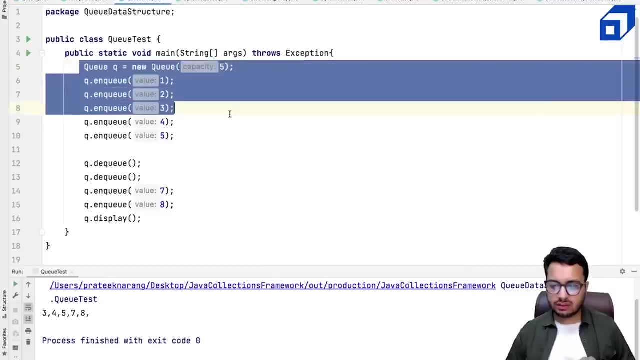 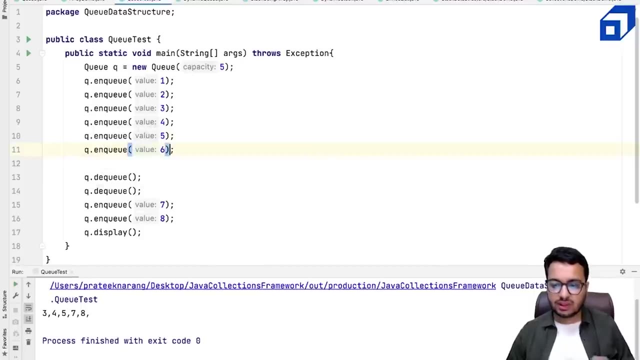 right now. let us test down, a test our functionality. let us go back into qtestjava, right? so earlier i was creating a queue of fixed size. if i try to- uh, let's say, push six elements in a queue of size five, i will get a exception. right, i'm using the fixed size queue. let's see. 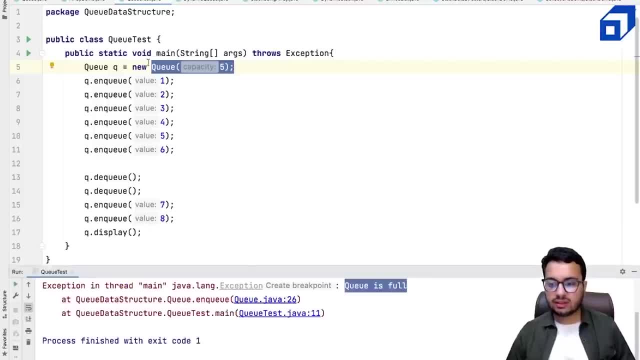 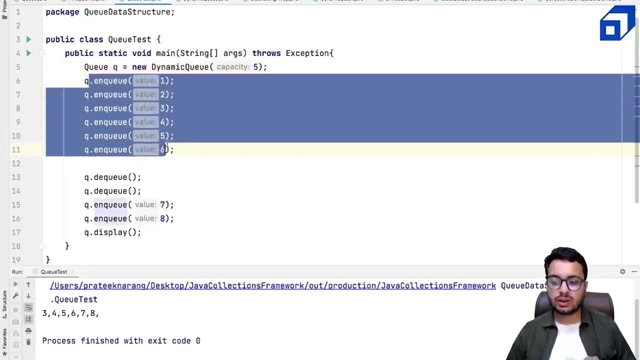 so i'm getting an exception that q is full right now if i replace this q object with the dynamic q object. let me show you if i do this, i should be able to hold it right. yes, i'm able to hold it. i do not get any exception. 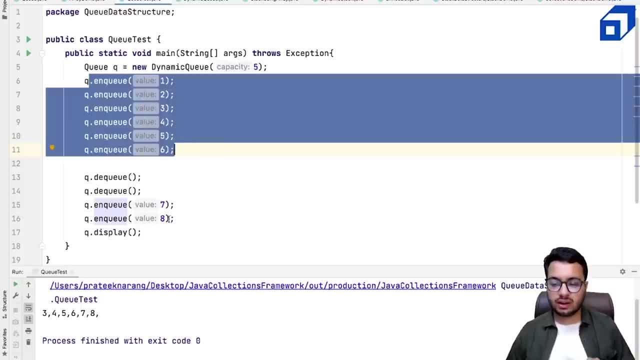 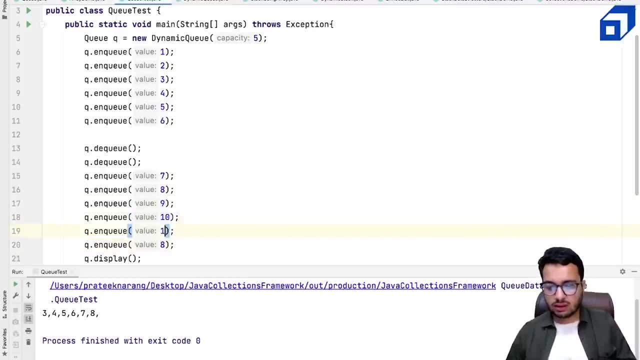 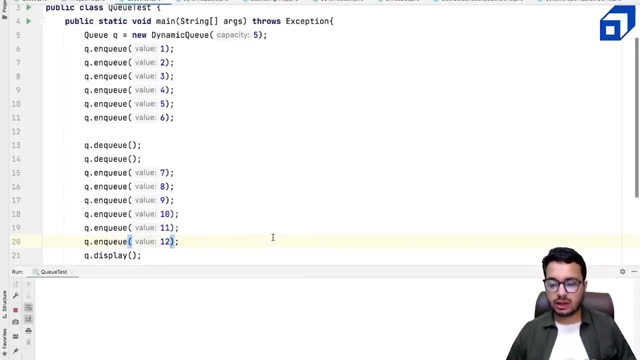 because q, q is getting expanded right and even i can put more elements i can define. let me put 9, 10, 11, 12, right and so on. so let's see what output we really get. i'm getting everything from 3 to 12, which is correct, right. so you inserted 1- 2. 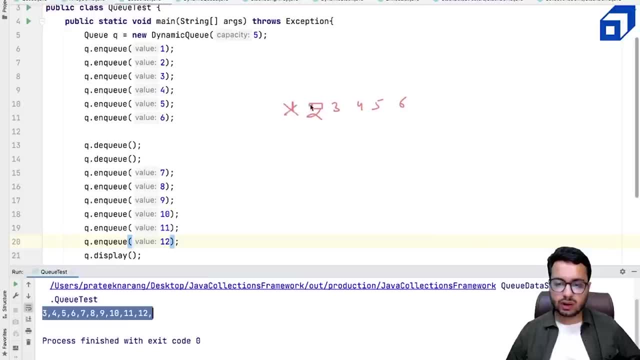 3, 4, 5, 6. then you removed 1, 2, the elements at the front. then you inserted 7, 8, 9, 10, 11, 12. okay, irrespective of the initial capacity, which was 5, you are able to hold more elements because 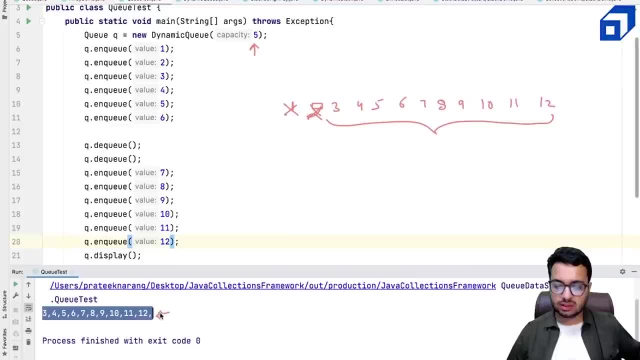 your array is getting expanded during the insertion process, right? so in this case you will never get it. q is full exception, unless you run out of your uh deep memory or something like that, right? that is uh dynamic queue using a dynamic array, right? so next we will discuss. 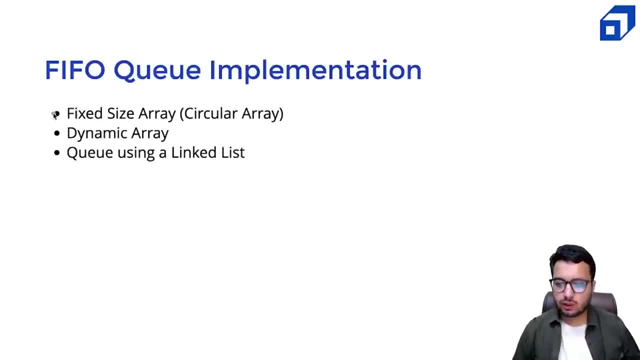 dynamic queue using a linked list. so so far we have seen uh two implementation: fixed size error implementation and dynamic error implementation. we have seen right. you can also use a error list object, uh, if you want. right now. third kind of implementation by will involve a linked list because linked list is also a linear data structure. right now you might ask. 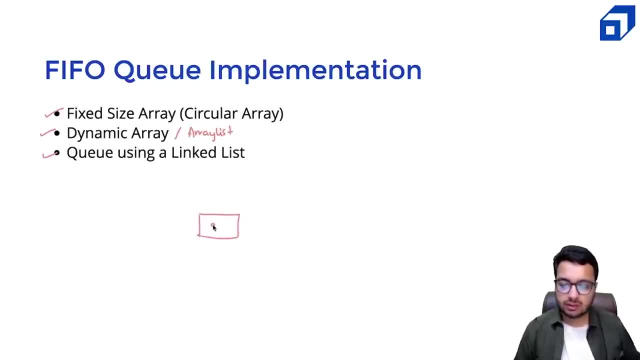 how we can use a linked list. it's pretty simple and very intuitive as well. now suppose you are inserting something, so one is at the beginning, then you insert two, then you insert three, then you insert fourth. right now, if i ask you, uh, this is, let's say, head and this is tail, right? 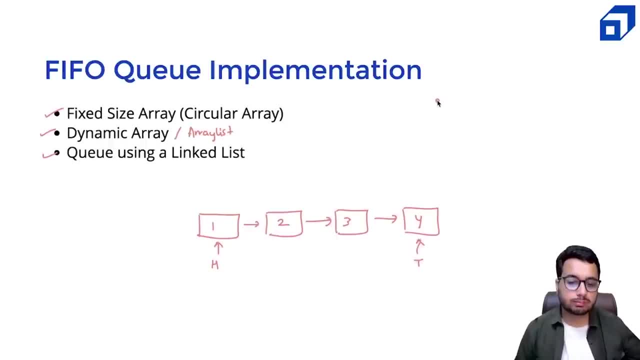 if i ask you where is the front element? right, so i want to get the front element. so that is one. if i want to remove this element, can you remove it? of course, yes, you can say, okay, i will move this head here and that means this element will be removed. if i want to read the front element, 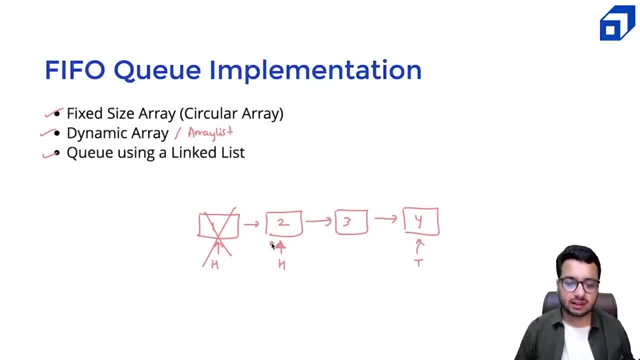 again. that element is at present at the end of the link list. if i want to insert something, it should go at the rear end. so where is the rear end? the rear end is at the tail right, so you can easily insert something here and your tail will come here right. so your head and tail, uh data. 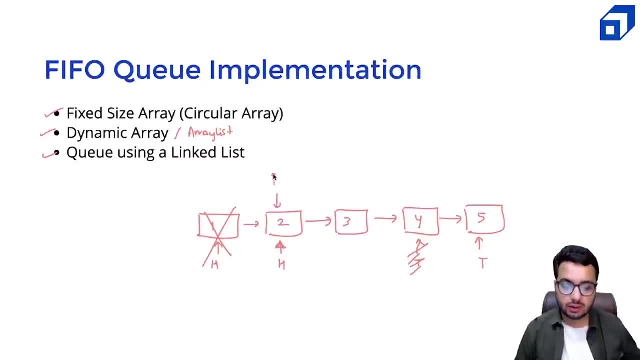 behave as front and rear for the link list. so this will be your front, this will be your rear. you can always insert at the rear end, which is insertion at tail, and it will be a order, one operation, and you can always remove from the front end, which is again going to be a 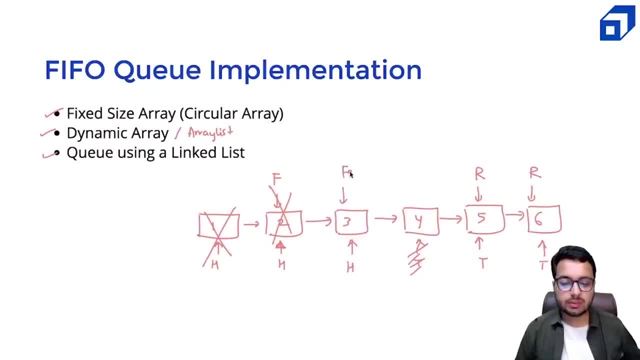 order, one operation right. so very simple implementation. and we have already covered linked list. i will not write the code using linked list. once again, you can either use the same class, so in your queue class you can say: fine, i'm going to create a linkless object. linked list l. 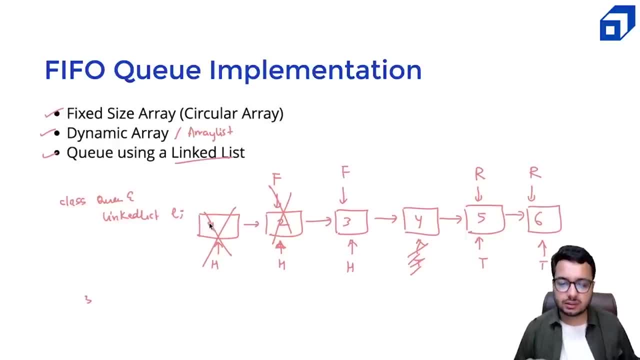 and whenever you want to enqueue, you add it to the linked list, and whenever you want to remove, you remove the first element of the linked list. okay, so those methods can be implemented, or you can implement all those methods from scratch as well. right, so that is about uh, implementation. 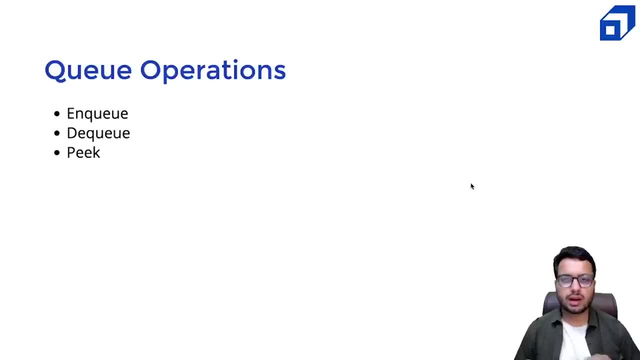 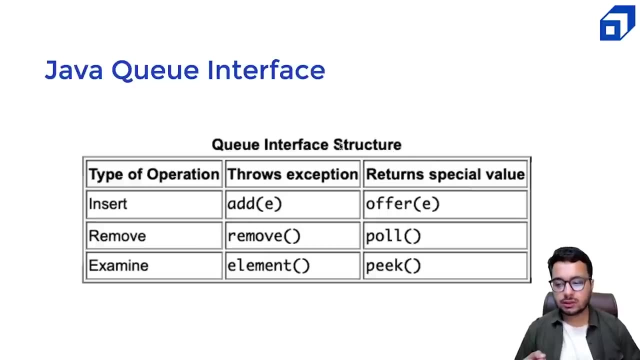 using a linked list. now, before we wind up this tutorial, i want to talk a little bit about the java queue. that is part of collections framework, right? so the java queue supports, uh, three types of operations. so one is your insert, remove and examine. right, so examine is like getting the. 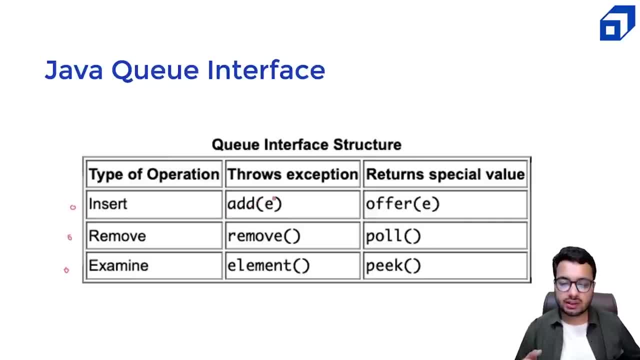 front element. right now there are two variants of the methods that are provided. so in one variant the methods throws an exception. like the variant that we have coded, those methods throw an exception. if you want to add something, the method is called as add instead of enqueue, right, so you? 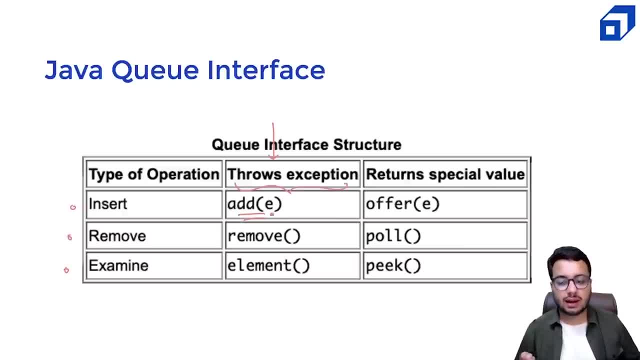 will create a queue object and i will call the library method add, right? if i want to remove the front element, the method is called as remove instead of dq, and if you want to get the front element, it is called as element, right? if the queue is empty, it will throw an exception, right, and the 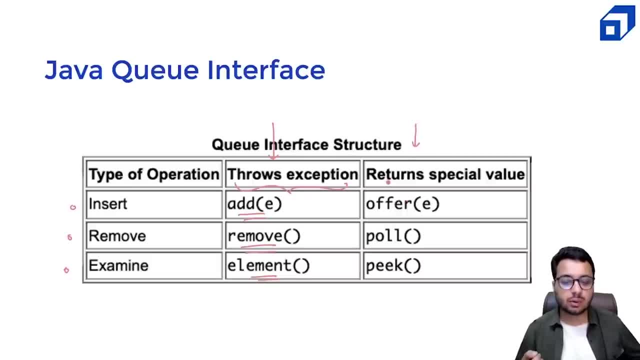 second set of methods. they are also same, but instead of throwing an exception, they will return a special value, maybe a boolean value, whether the operation was successful or not right. so add and offer: they are equivalent methods. remove and pull: they are equivalent methods. element and peak: they are equivalent methods. okay, so i have discussed. 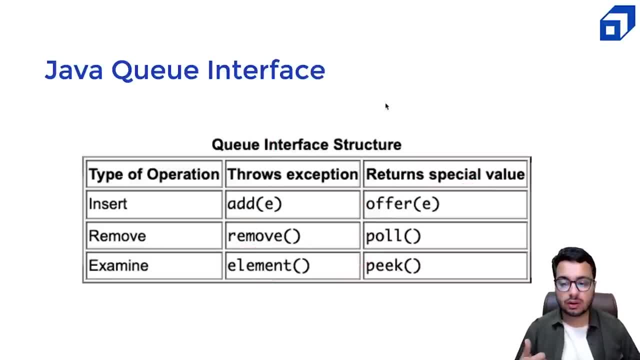 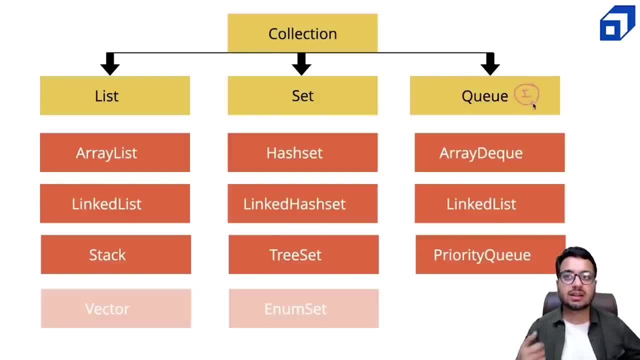 about queue interface in my java collections tutorial on the channel right. so what we talked about is that in java, queue is actually your interface, okay, and there are three implementations. there are three classes that implement this cube. so your linked list class- it implements your fifo queue that we have just seen, that we can build a queue using a linked list. okay, and there is. 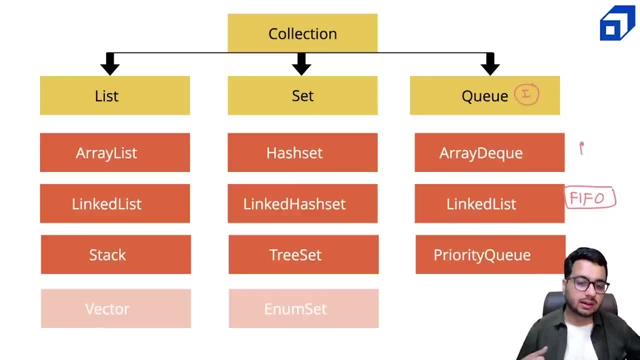 something. there is a class called as array deck, so array deck is a class called array deck class is a class that implements another kind of queue in which you can insert and remove from both ends right. so it is called as a doubly ended queue. so in this case the behavior would be different. 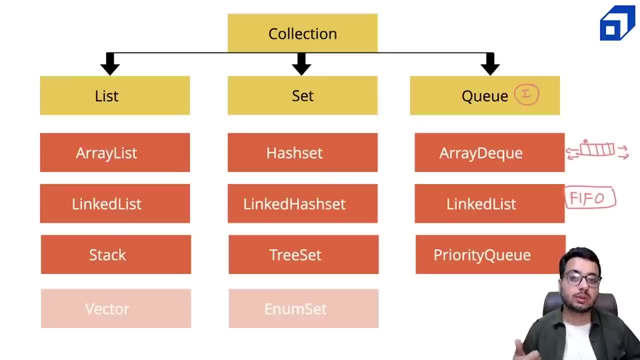 you. you can add at first position, you can add at last position, you can remove at first position, you can also remove at last position. so it starts. it is a doubly ended queue. it's called as deck right. it's not dq, it's called as deck right. it's a different type of queue and third type of queue. 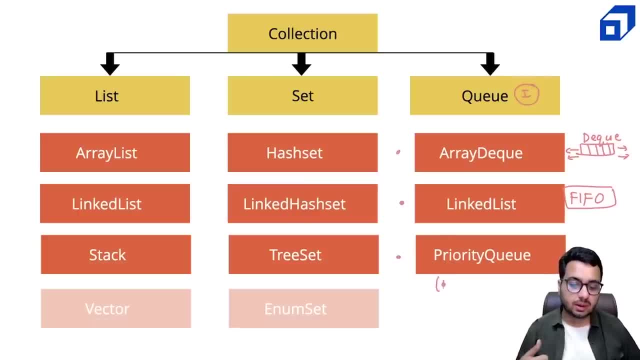 is called as a priority queue, which we will of course discuss. it is based on the concept of keep data structure. in this case, the elements don't maintain a fifa ordering, but they maintain a priority ordering. so, again, it's a big topic. we will discuss it separately. but if you want to see, 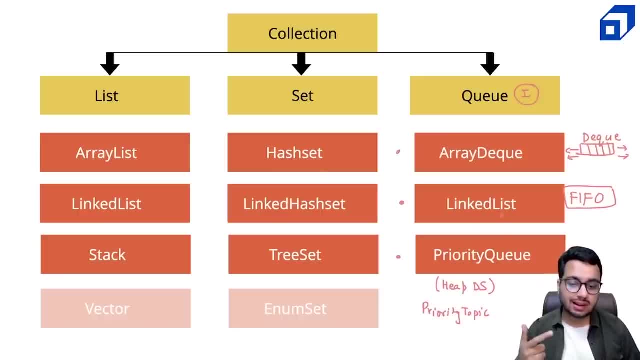 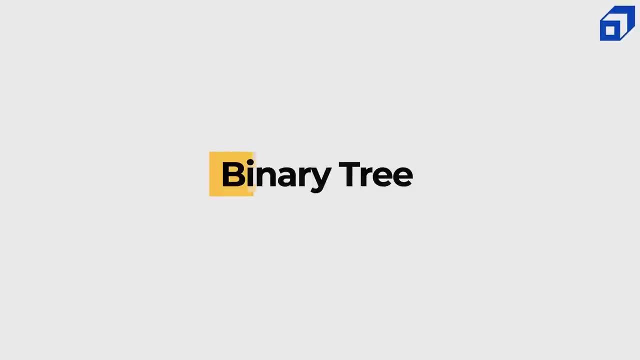 the code demo how these different cues are, how these classes are different in behavior. check out my video on data structures and in which i have discussed the complete collections framework as well as different implementations of queue, as a part of that video. let us start the topic by understanding what is tree data structure in computer science? a? 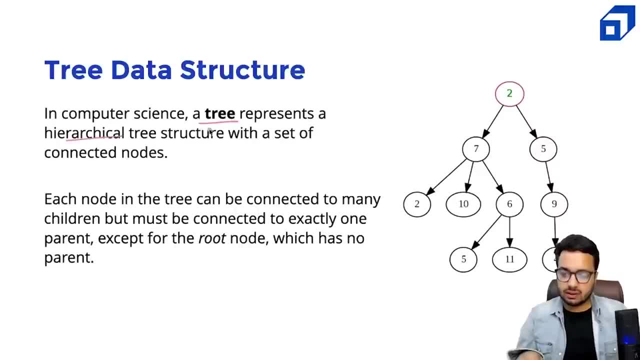 tree represents a hierarchical structure with a set of connected nodes, right? so, for example, if you look at this diagram, this actually represents a tree and this node, it is the starting of the tree. it is called as a root node, right? we will discuss where it can be useful. so 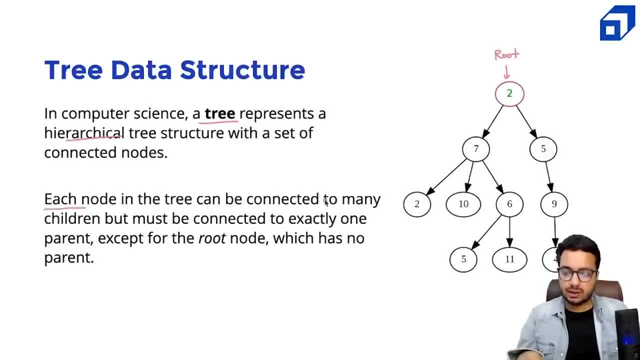 in this structure, each node in the tree can be connected to many children, so this is a non-linear data structure. the first non-linear data structure that we are covering is a tree. so far, we have talked about array, we have talked about linked list. all of those data structures were linear. 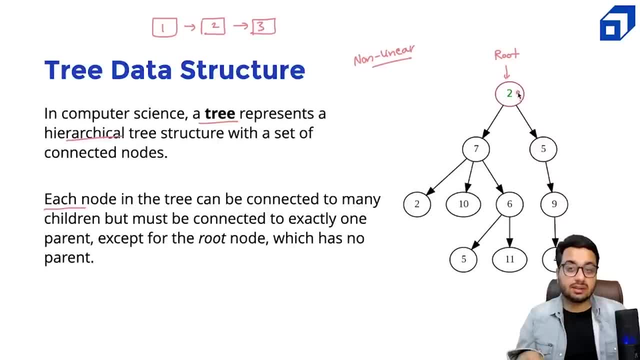 data structures because they were following a sequence here. there is no sequence here. there is a hierarchy right. so each node can be connected to many children. so 2 is connected with 7 and 5.. it is connected with 2 children, so 7 and 5. they are children of 2 but must be connected to exactly one parent. so 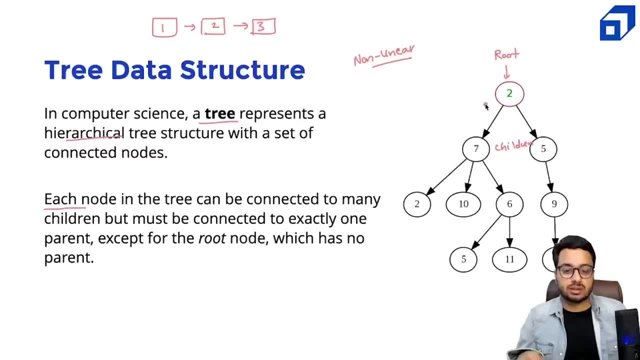 each node must have one parent. i cannot say: 7 will have two parents. no, 7 will have only one parent, that is 2.. 5 has only one parent, that is 2.. 2 has only one parent, that is 7.. 10 has only one parent. 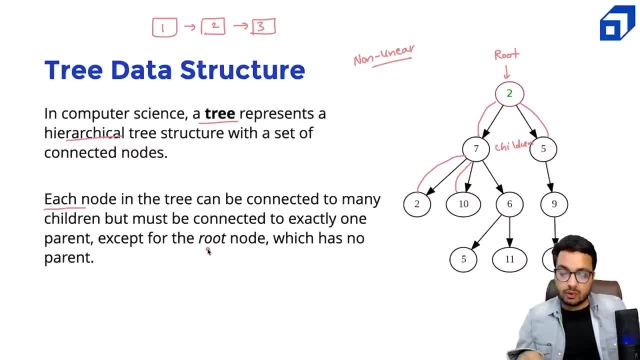 that is also 7, right? so except for the root node, which has no parent, so root node has no parent, rest all the nodes. they have one one parent right now, because of this property, there will be an interesting observation. suppose you are creating a tree in which you are going to have 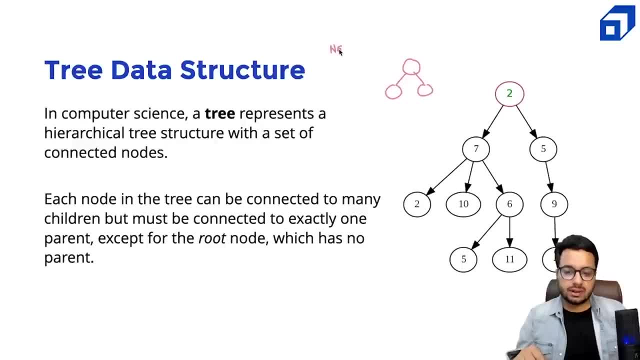 n nodes. okay, for example, i have three nodes here. how many edges you will have, except for the root node? for every node that you will have that you will add, there will be an edge. so there will be, of course, n minus one edges in the tree. so in any tree that you are going to create, irrespective of is it a binary tree or not, 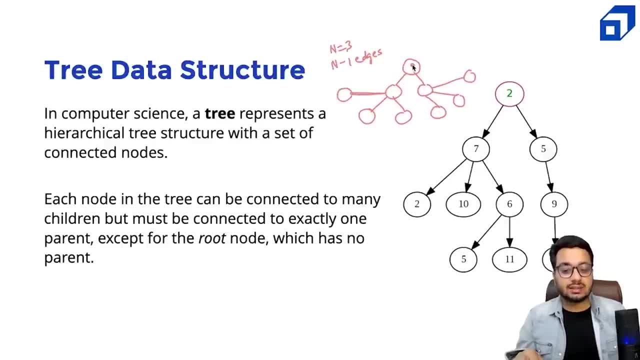 each node that you add will add an edge in the tree except the root node. okay, so root node does not add any edge in the tree except the root node. if there are n nodes in the tree, there are, there would be n minus one edges. okay, because root node has. 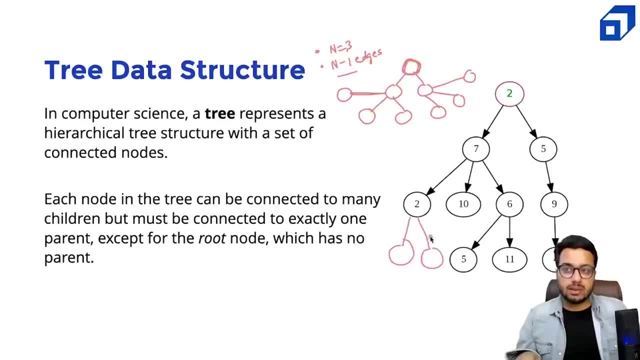 no parent rest. all the nodes that you add, they must be connected to a parent through an edge right. so this is an interesting observation. you can note. so in n every tree there will be n nodes and there would be n minus one edges in the tree right. 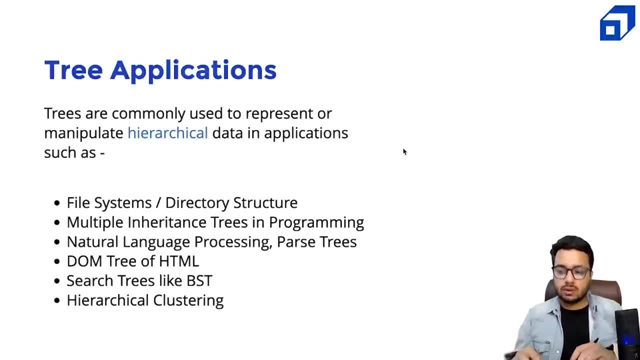 so that is tree data sector. now let us talk about where this data sector can be used, how it can be helpful in computer science. okay, basically, trees are used to represent or manipulate hierarchical data in applications such as file systems or directory structure. right, so all of you have worked with the file system. 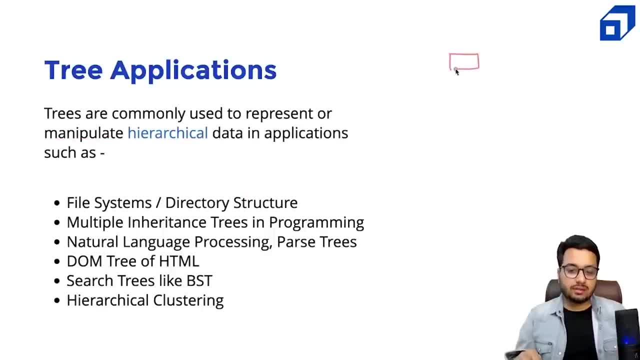 so what happens in a file system? you say, okay, i have my pc in this, i have certain drives- t drive, d drive, e drive- and then inside this i have folders f1, f2, f3, f4, and here also i have folders. then i have sub folders, right? maybe i have photos here, maybe i have some documents here, right? 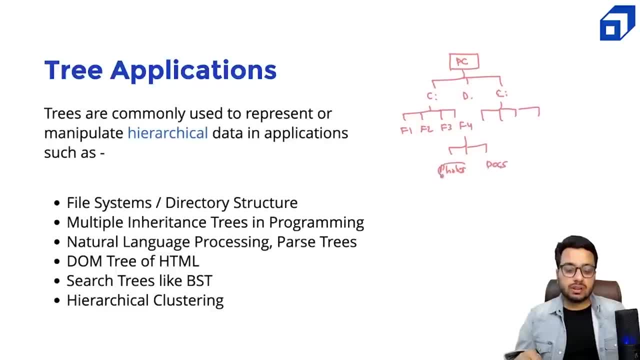 now we often do operations like that: okay, i want to move these photos from here to here, right? so what is going to happen? you're not going to copy this data. you're going to say, okay, i'll cut and paste. so if you simply want to move this photos from here to here, what do you need to do? you do. 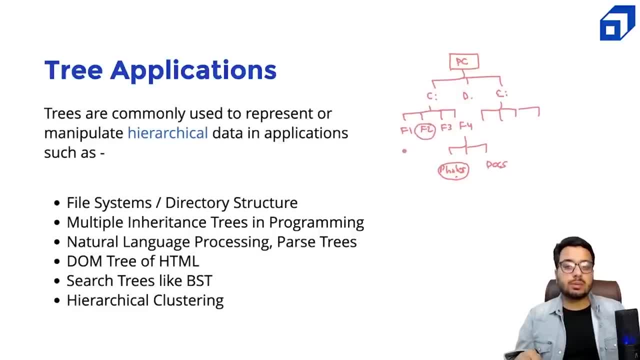 not need to copy this information to some other part of the disk. you only need to change the reference right. that, okay. earlier this reference was stored by f 4, now this reference is stored by f2. basically, the links right, the links to the folders and subfolders. they can be easily changed if the data structure is implemented using a tree right. 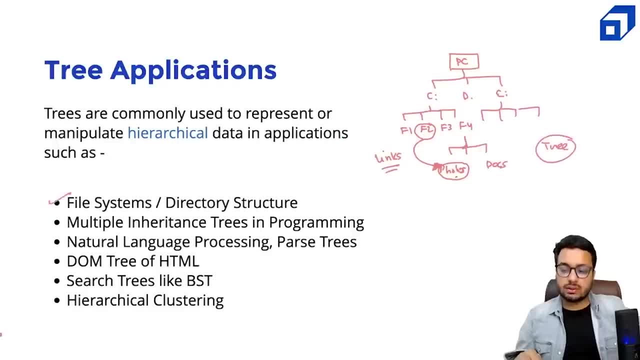 this is something we will discuss. right, the file system is a good example of a tree data structure. right, multiple inheritance trees in programming. so this is used when you're using object-oriented programming concepts and you have a class c which is going to inherit from a class c which is going to inherit from a class c which is going to inherit from a class c which is 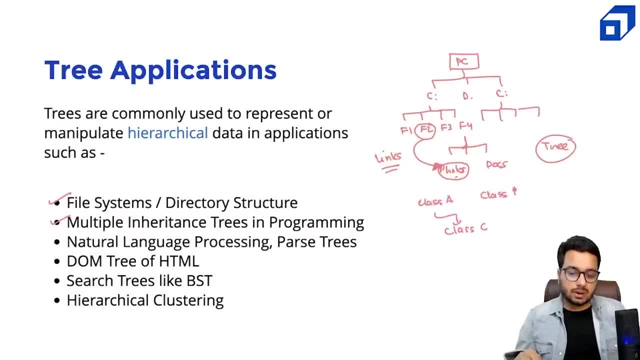 class c, which is going to inherit from a class a. it is also going to inherit some methods from a class b, right? so this is a, not exactly a tree, i would say, because this node, this is inheriting from two different classes. irrespective of that fact, basically, 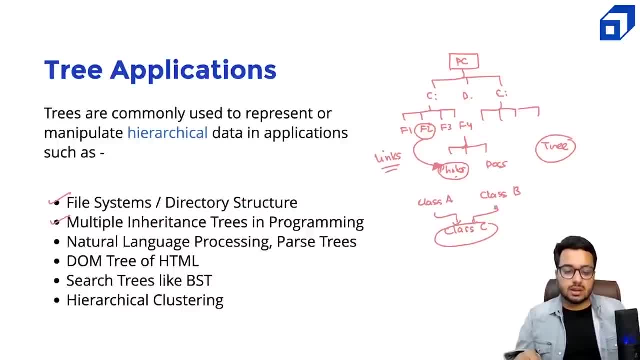 uh, the trees are internally used by the compilers to see what methods would be part of the class that you have implemented using inheritance. okay, then again in natural language processing. basically, whenever you have a sentence- for example, i am going for a party right now- this sentence can be broken down into: 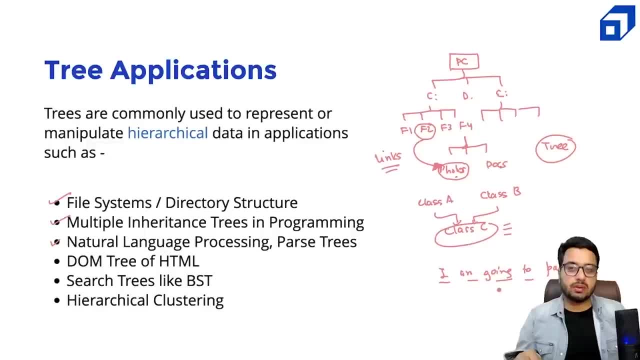 certain components, maybe you have a verb, maybe you have a subject, maybe you have a predicate or you have even for language parsers, okay, so what are your parsers? whenever you write code, it goes through a language parser so that compiler can figure out if there is any error in the code. 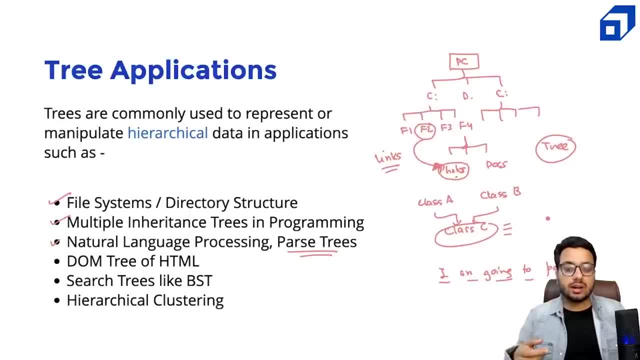 it is having the correct syntax or not. so they again form a parse tree of that code, right? so, again, it's an interesting concept that you will learn in compilers. right again, they are used a lot in understanding of the language. okay then, in html there is a dom tree, so whenever you open, 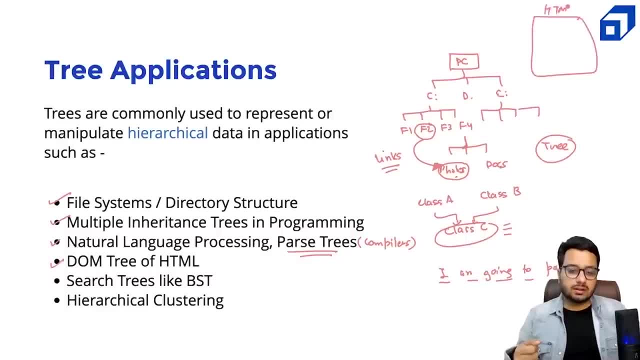 up a website, right, you see, there is a html code. right inside html code there are a lot of tags, there is head, there is uh body. right inside body there is a paragraph, there is a div, there is a image. right, if you look carefully, this whole document. 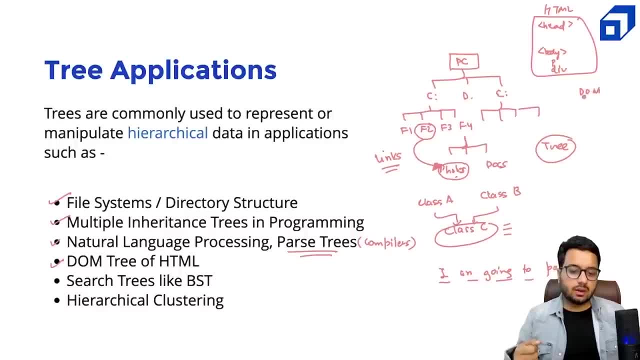 forms a dom tree. so inside dom tree you have head, you have body. right then you have certain elements, you have div, you have paragraph here, you might have image, you might have some text. right, what is happening? you want to say, okay, i want to click this particular button. and on clicking this, 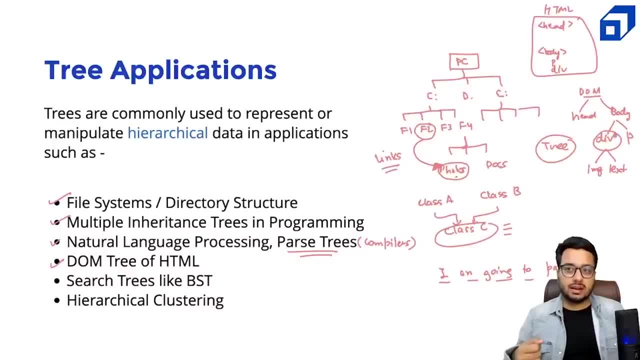 button this div uh will change its color right. so how do you fetch elements from this huge web page? so there are methods like document dot- get element by id. document dot- get element by tag name. what it is doing it is traversing this dom tree. it is a tree of objects. okay, it is a tree of objects. 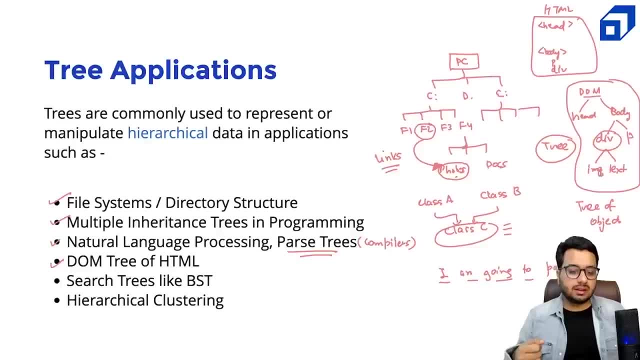 in your web browser. again, it's behind the scenes, so it is doing some kind of search operation on this tree and it is trying to manipulate this tree, right? for example, you scroll your web page and a new item is added from the bottom, so maybe it is adding something in in the list, right? so your tree is getting. 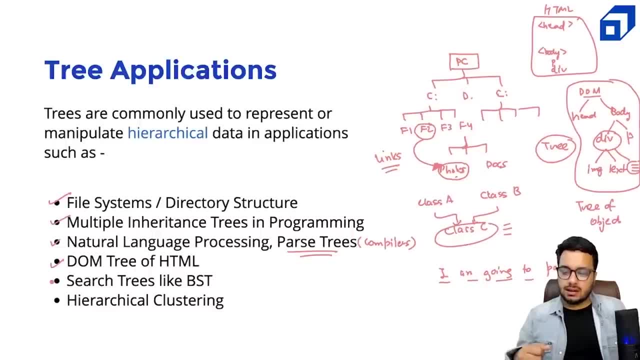 modified. right then, of course, there are uh trees which are used in search operations, like binary search tree. there are trees which are used to implement data such as like map self-balancing trees. okay, so they are used to implement data such as like map self-balancing trees. okay, so they are. 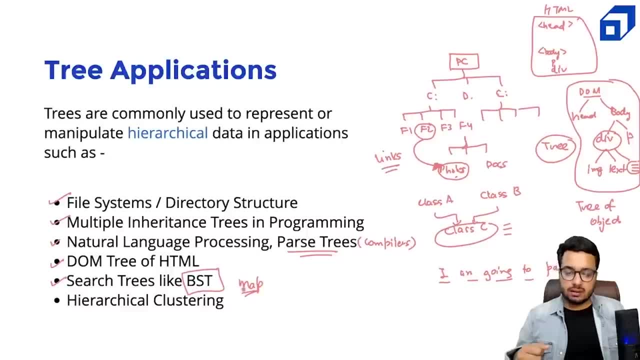 to performは'ster searches and keeping data ordered. we will talk about bsts in the coming class. in machine learning there is a concept called as hierarchical clustering, so it is a part of, uh, a clustering technique, okay, where i want to group together similar items, so it comes under. 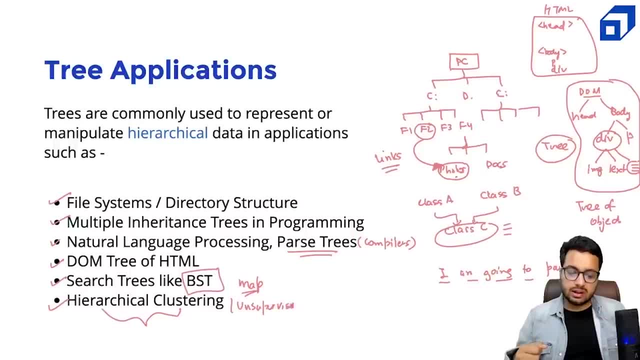 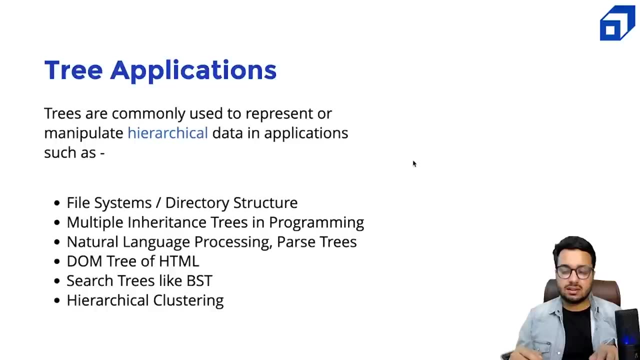 part of unsupervised learning. so there also, the tree data sector is used, right. so you we see a lot of applications are there and that becomes uh very important for us to understand uh the tree data sector. so in this video we will be uh talking more about binary trees in general. 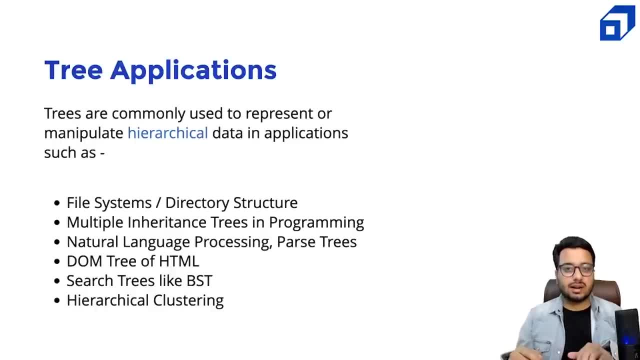 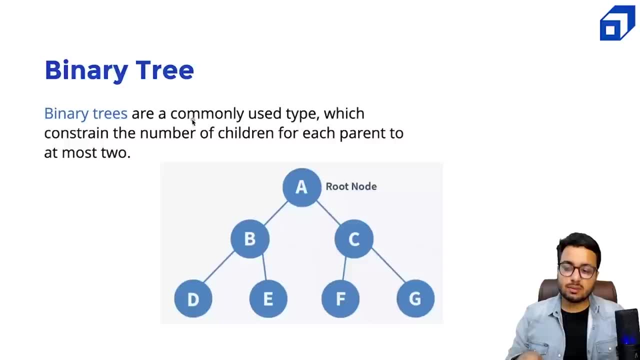 because that they are the most common ones, uh, that are widely used. okay, so let us start with binary trees. so let us start by understanding what is a binary tree. so, as i discussed, it is the most commonly used, uh, tree structure in which you can have at max two children. okay, so it constrains. 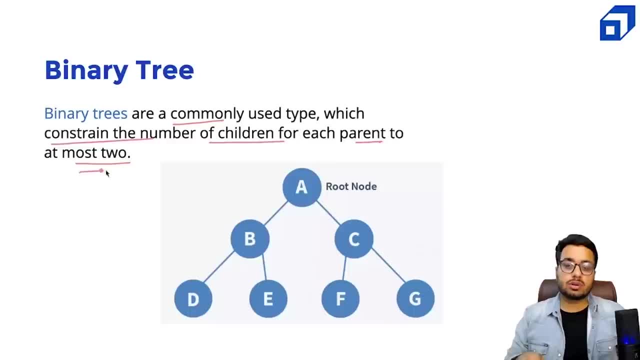 the number of children for each parent to at most two. that means a node can have zero children. for example, in this case the nodes d, e, f, g. they don't have any children. they are also called as leaf nodes. the nodes which don't have any children, they are called as leaf nodes. node can also have. 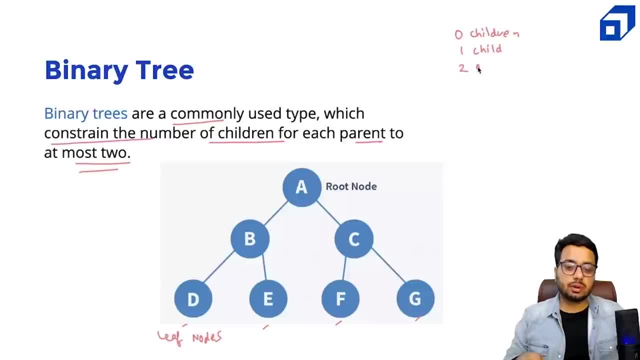 one child right. or it can have two children- right. it cannot have more than two children. for example, if i draw a few structures, you have to tell me whether it is a binary tree or not. is it a binary tree? the answer is yes. each node has zero child. one child or two children right? okay, is this a? 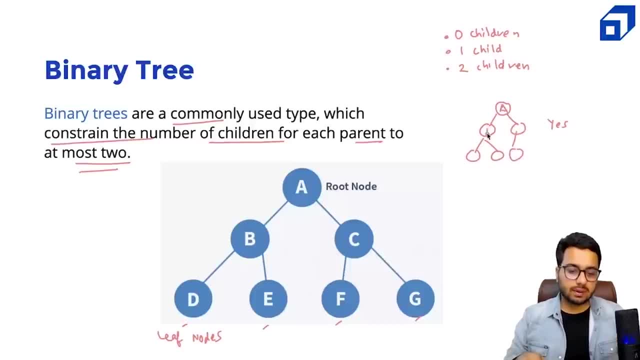 binary tree? the answer is yes. so this node, the node c, it has one child. a and b, they have two children. and d, e, f, they have, they don't have any children. hence, in this case, we have three leaf nodes. so this is again an example of a binary tree. right now, what we are going to learn in this tutorial, we 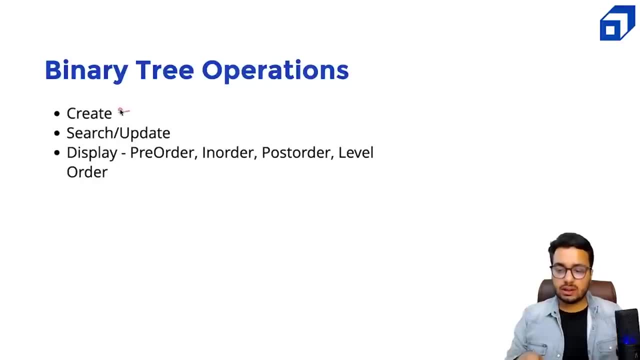 are going to learn about different operations. how do we create a binary tree? how does the node structure look like? how do we perform search or update operation on a binary tree? how do we display a binary tree? and there are four popular ways to do it: pre-order traversal. in order traversal. 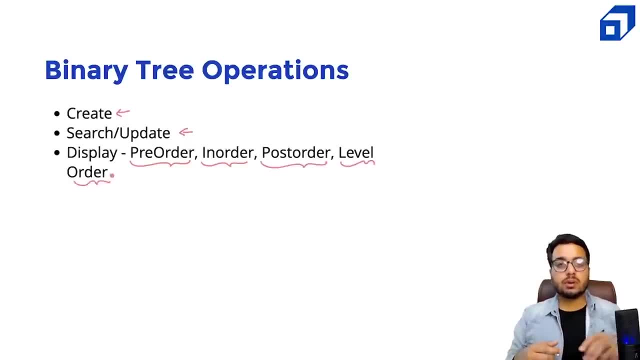 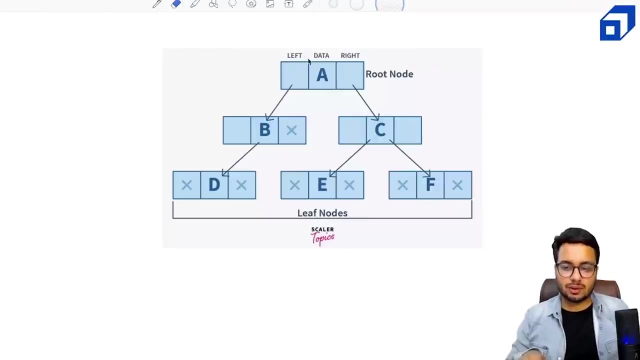 post order, traversal, level, audit, reversal, okay, so we are going to look at all those, all these things one by one, and we'll be starting with creation of tree first. let's begin with that. let us talk about creating the tree. so first of all, we need to understand the structure of the node, that is. 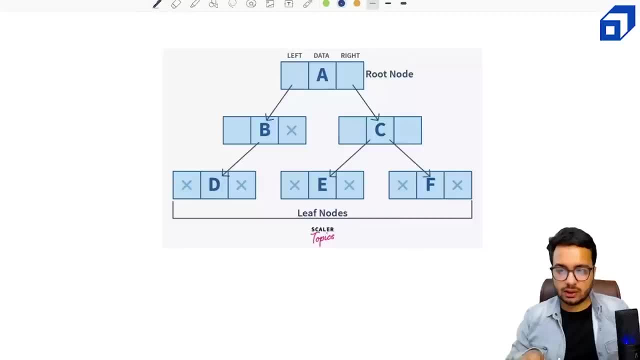 going to create the tree, right? so in this tree, if you look carefully, there are so many nodes and this box represents one particular node. okay, that is the root node, right? so i have the root node. now, what is this root node going to contain, or any node going to contain? it is going to store? 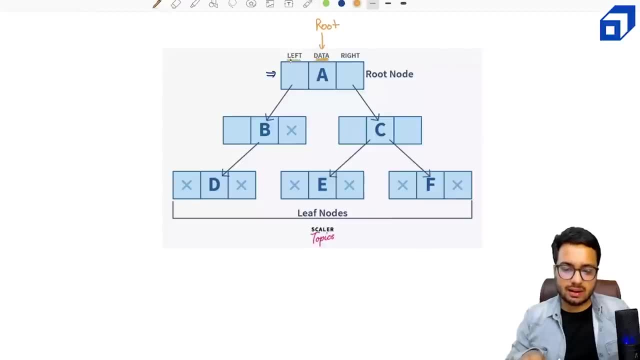 three things. one is your data, one is the address of the left node, one is the address of the right. okay, in java we also call it as the reference. right now, suppose this object b, it is created at some memory address, let's say 250. right, this is the location of b in the heap, where it is. 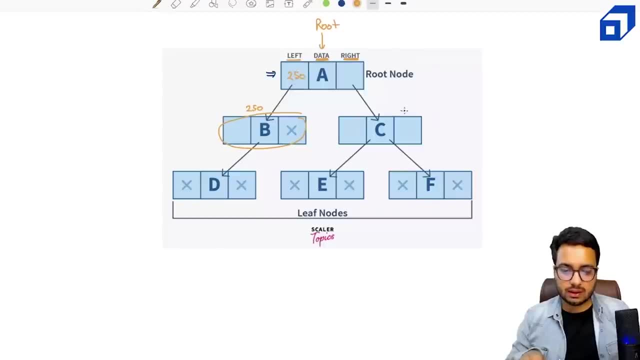 created. so a is left is going to store 250. let's say this is created at some location- 380. so a is right, is going to store 380. right, a itself is created at some some location. let's say 400. the root is going to store 400. okay, so root is not a node. 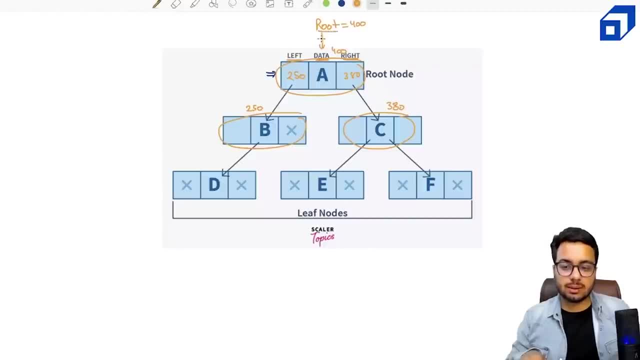 root is just a reference to the root node. okay, so root variable is holding the address of the root node. right now. b is left, is referring to d, so d is created at some location, let's say 560, so here we will have 560. now d is left and right. they are, they are null, they don't refer to anyone. 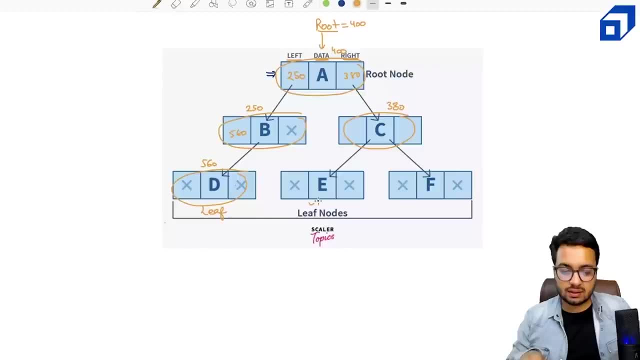 because d is a leaf node right, so d is a leaf node. e is a leaf node. f is also a leaf node. so they are left and right, they are null. a, b is a node with a single child, right because it does not have any right child. hence this value is also null. and here i will store the address of e, here. 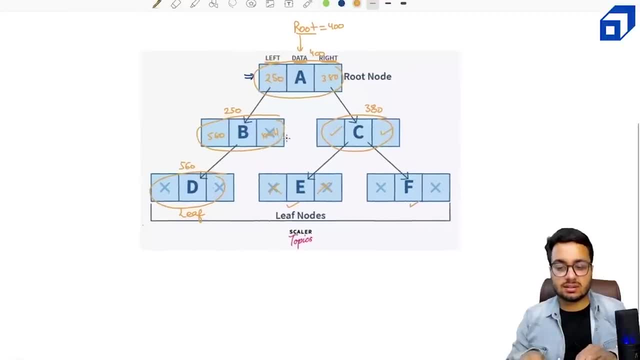 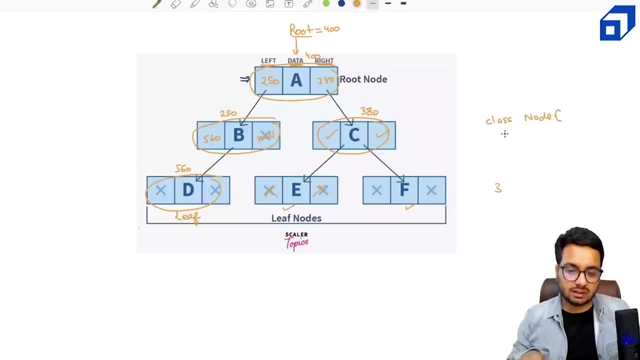 i will store the address of f right, so i hope you are understanding the structure of the node. so i need to implement a class called node, in which i will have three things. one is my integer data. data can take any type. just to keep it simple, i'm taking it as a integer. one will be my node left. 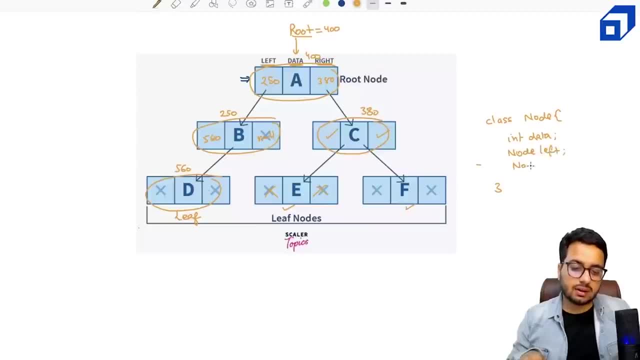 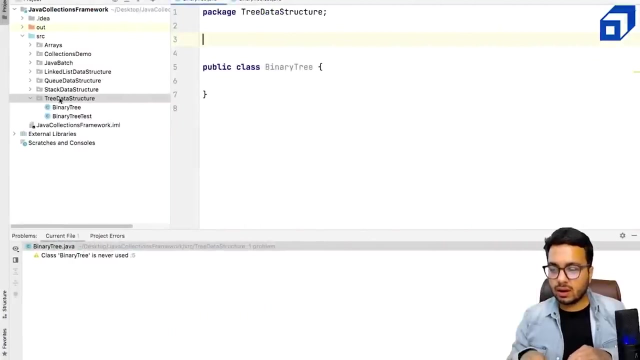 a reference of the next left node and node right a reference to the right node. if the left and right node does not exist, then i will set this value to null right now. let us see in the code how can i implement this node class. let us go to intellij. now i am going to implement the tree. 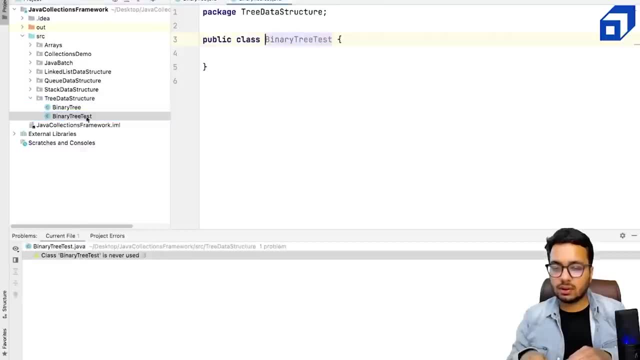 data structure. i have a class called binary tree. i have a class called binary tree test. both are empty classes as of now. in order to build binary tree class, i need to define that. what is node right? so node will have three things: one is my data, one is my left and one is 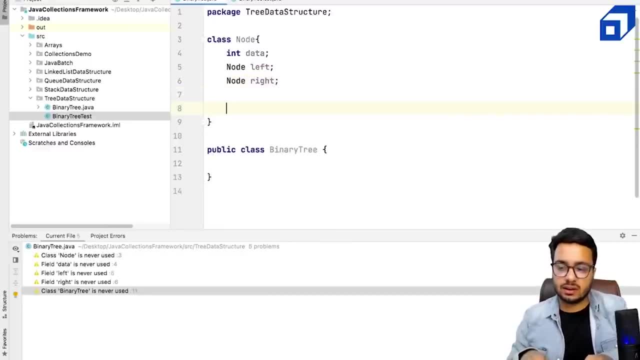 my right. apart from it, i also need to give a constructor here that whenever a new node is constructed, what data it should take. so it's okay, data i will know, but at the time of construction of new node i do not know what node will go into the left, what node will go into the right. so i will. 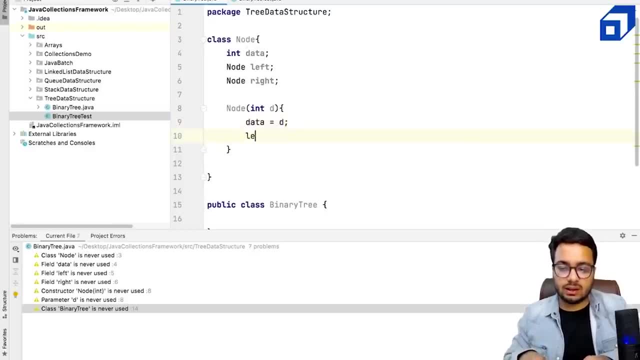 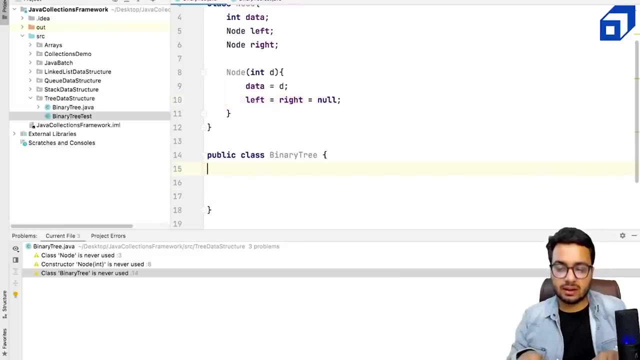 simply say that my data this is equal to d and left and right they will be set to null by default. so whenever you are creating a new node, you do not know the left and right, uh nodes, so these will be set later. right now comes the binary tree class. now suppose we want to create a tree like this. 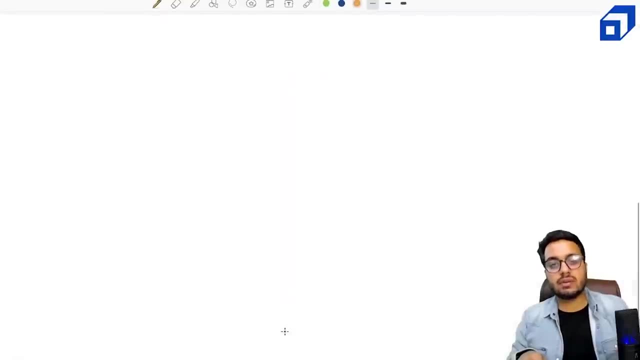 okay, or let me take up another example in which i have numeric data. i can say, okay, let me create a tree like this, one connected with another node like this. so i will just create a tree like this. ok, let me take up another example in which i have numeric data. i can say, okay, let me create a tree. 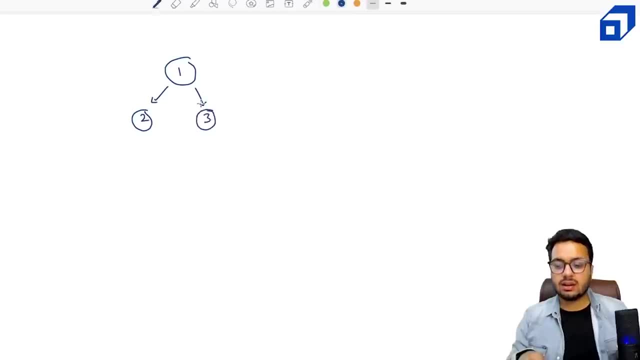 with two and then it is connected with three. right, let's say very simple tree, three nodes. now, how you will read this tree? the first thing is: how do i read this tree? right, so the first input i will get is the root node. okay, user will enter one. i will say: fine, input is one. let me read this. 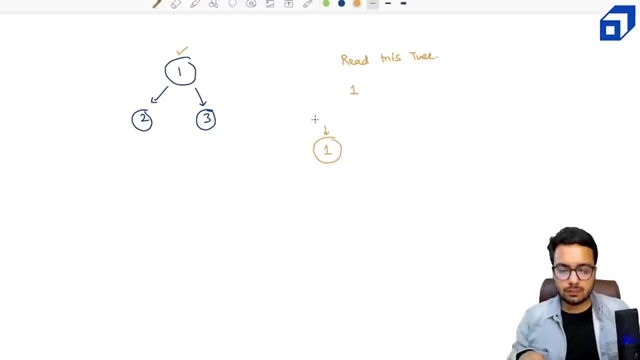 create a node called a root node, and root node is going to point to this node right and in the left of this. i will again read from the user. right, the user says, okay, fine, the next node is two. so i'll define, i'll create a node called two. i will attach it in the left of one. 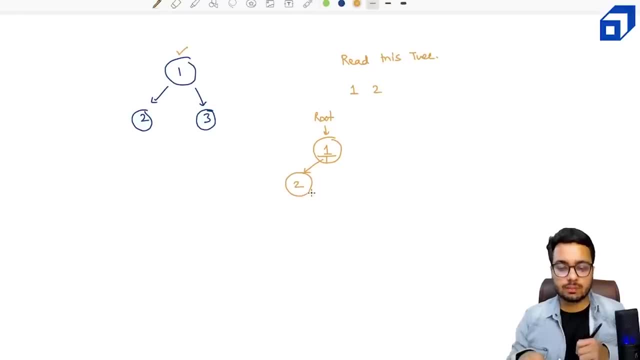 like this: okay, and now what is the next node? i will read right now: it can happen that i have something in the left of two, or i have something in the right of two, or i have something in the right of one right, so i do not know. 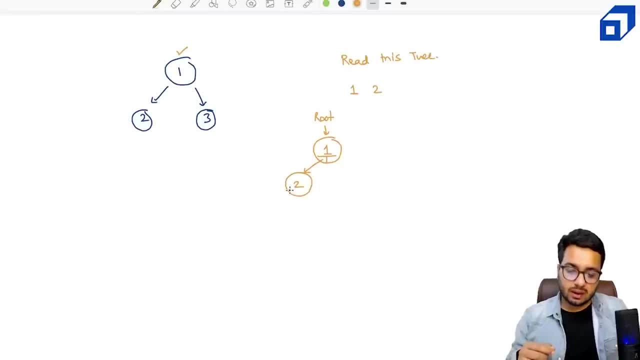 you. the way we are going to do it is we are going to read now what is there in the left of two. okay, so if the left of two is null, right, i will input minus one. so minus one in the input will denote that near is nothing here. so i will simply set this value to be null right. what is right of? 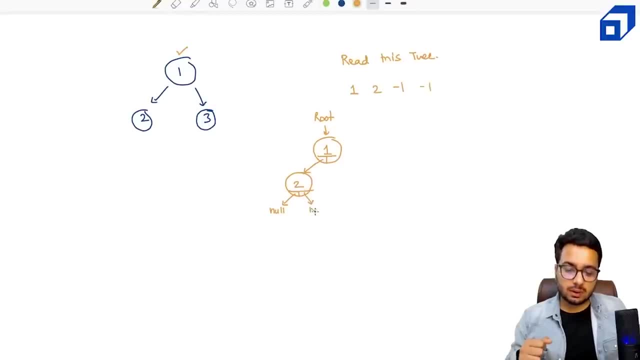 two. i'm again going to say it is minus one, so i will set this value to null right now. this option is gone. i've read it. this option is gone now i can only read this. i will come back here i will say: fine, this two is done. now try to read what is there in the right of 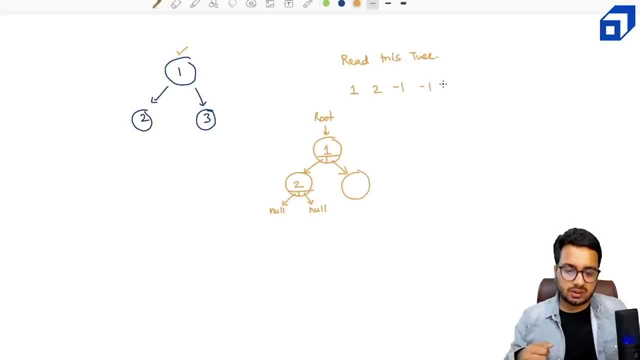 one right, so it's okay. the next input is three. i will create a new node and i will attach it, of course, here, but before that i will read what is in the left of three. right, so attach part will happen a little later. right, i'll read what is in the left of three, so this value would be minus one. 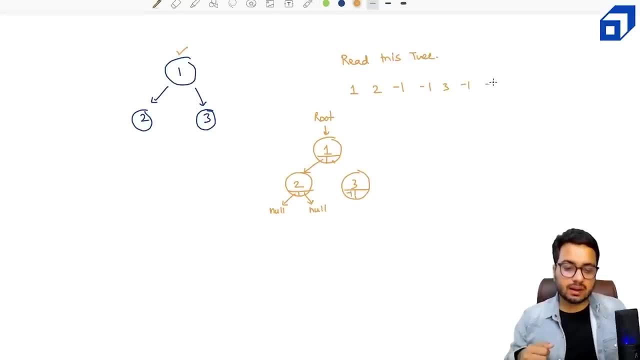 minus one. what is there in the right of three? again i say minus one. now this node is constructed, or in a way i can say this subtree has been constructed. so once it is constructed i will return it back to the parent. so the parent is one, it will get connected here, right? so this will become more clear once i 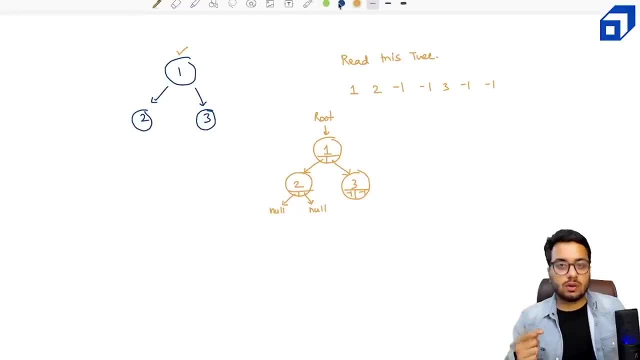 write the code. the idea is: i will, of course, do it for a bigger tree as well. this is little tricky, right? so what the idea is? we are going to build a tree recursively. we are going to build recursively right now how we are going to build a tree recursively. we are going to build a tree. 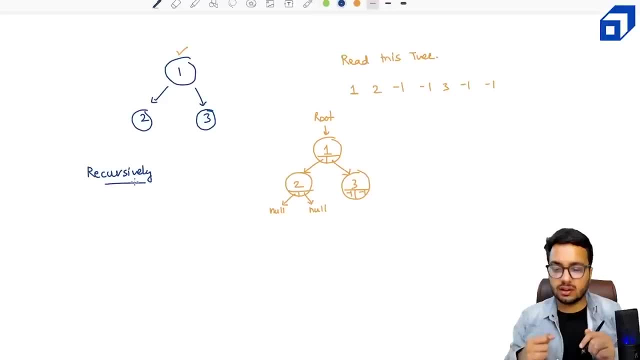 recursively many tree operations. they are recursive in nature, right, so it's okay. fine, i will build the root node. that is one. then i will build the complete left subtree. in the above example, the left subtree has only one node, so it looks easy. right, i will build the complete right subtree. 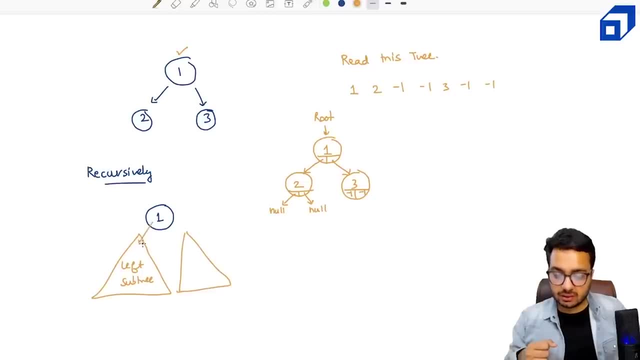 right. okay, i will build the complete left subtree and i will attach it here. that is part one. i will build the complete right subtree and then i will attach it in the right of one 8, so we will do it for a bigger tree as well. so let us jump into the code first and try to see. 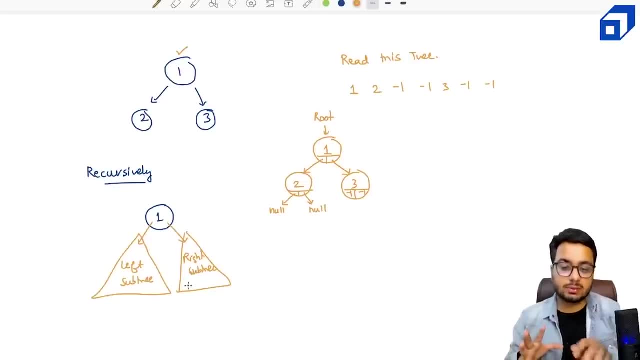 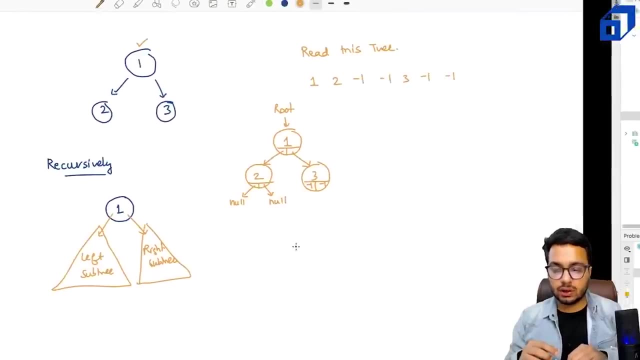 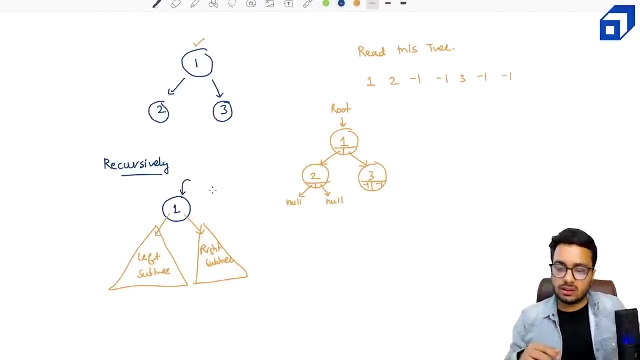 how this can be written. of course, i will do a arrive and explain you how you can build a more complicated tree like this with the same code. okay, let us go into the binary tree class. one thing is for sure: that every tree must know what is the root node. what is the root node? 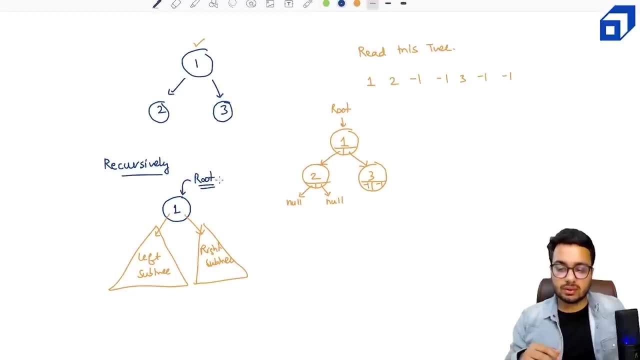 this is something that will be the property of the tree. every tree must know what is the root node, just like in a link list. every link list knows what is the head of the link list, what is the tail of the link list. so in in case of three, you must know that what. 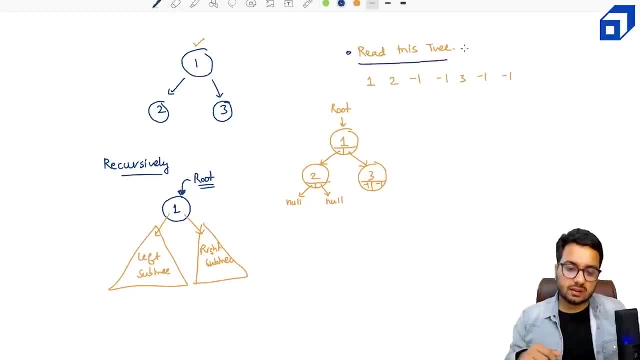 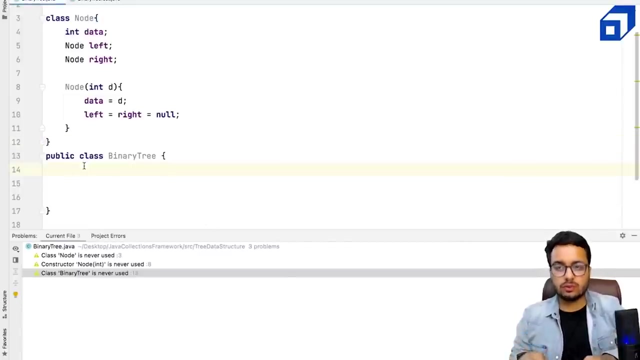 is the root node, right? so one thing is there. i am going to read this tree. so user will, input will come through the user, right? so let us see the tree construction part. so in this binary tree class, what i am going to do, i am going to first define the data members. 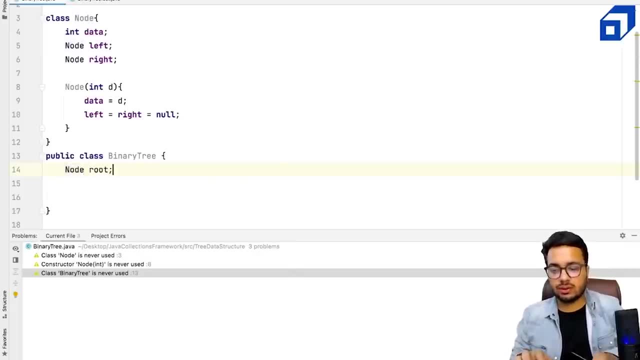 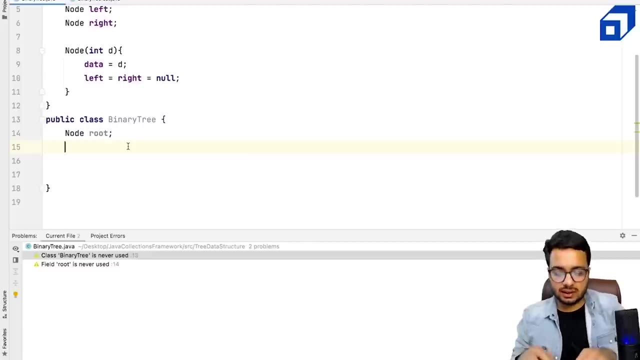 of the tree. so i have only one data member. that is the root of the tree right now. this root should be initialized where it should be initialized, of course, when the tree is created. so when the tree is created, it is created, then the constructor is called. i need to define a constructor called. 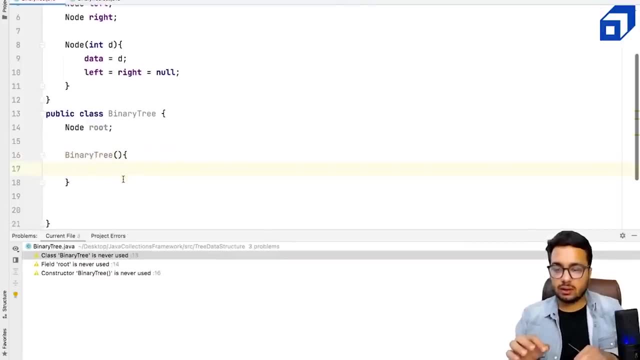 binary tree. right now in this constructor, what i need to do? i need to take input from the user. so in order to take input i will need a scanner object. i will say scanner se. this is equal to new scanner system dot in. so scanner object is used in java to read inputs. 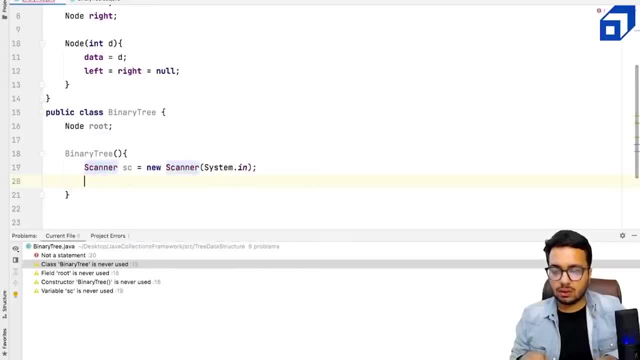 so i have imported the scanner. right now. the building of the tree is recursive in nature, so i will create a helper function to do it, so i can define node, let's say create tree, and to this create tree method i am going to supply the scanner object so that 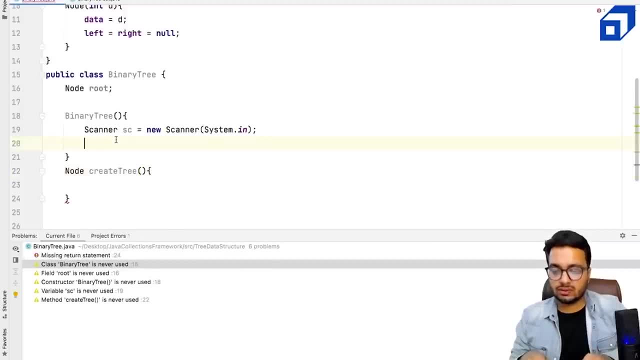 this method will actually read from the user. okay, so i will define. the root should be initialized by calling the create tree method. so create tree is a helper method getting called in the constructor that will read the tree from the command line. right now i'm going to pass the scanner object here so that i can use it to read data from the user, right? 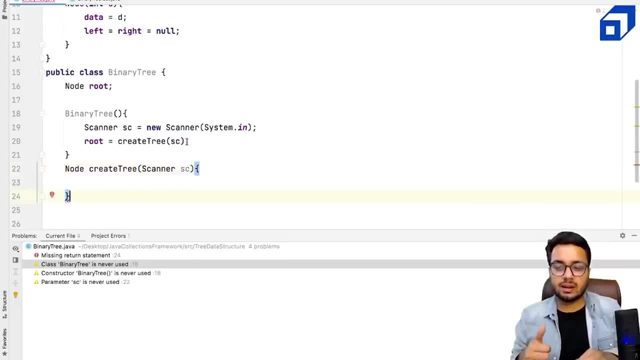 i'm no, i don't want to create this object again and again. uh, inside this method. okay, so i am creating it once and that object is being circulated across all the recursive function calls that are going to happen right now. suppose i read something i can say: okay, 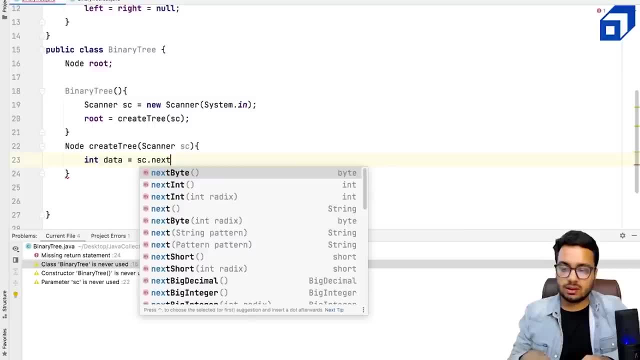 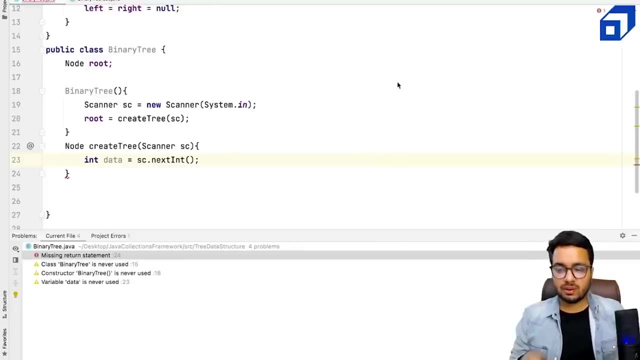 uh, data that i'm going to read is scanner dot, next stent, so i'm going to read something. all right. now i have read something from the user. let's say, this data is one right what i want to do. okay, this data can also be minus one, right, i'm asking. okay, tell me what is the 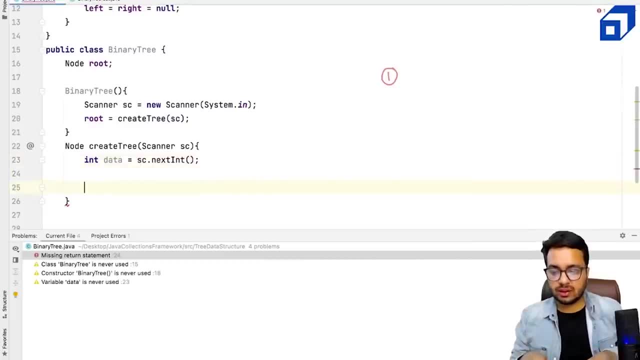 next data. so i will actually have a two, two types of case. one will be my base case. if my data is minus one, then what should i return? i will return a null. that means okay, i don't want to attach any node here, start sub trace, just null. 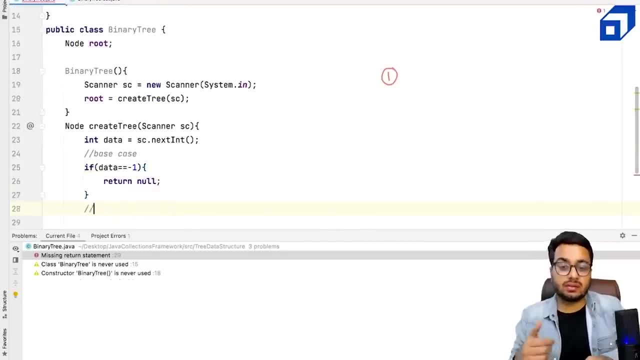 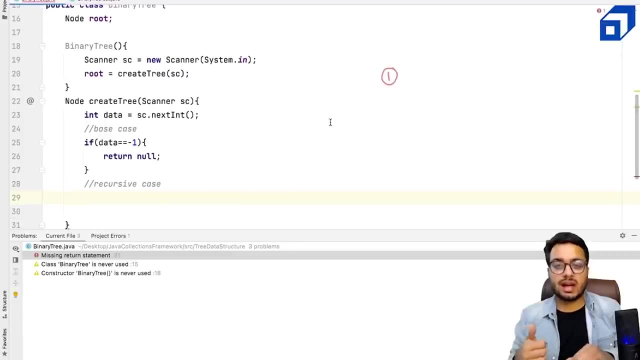 i will return null. but if it is not, minus one. if it is something else- basically i'm talking about the recursive case. for example, if my input is one, what i will do? i will create a new node. i'll say i'll call a node root. this is equal to new node and i give it the value data, right, if root is. 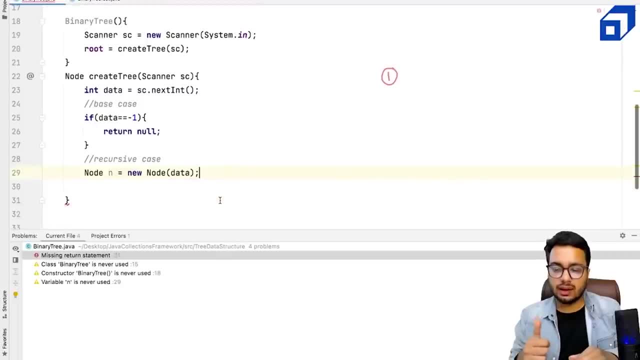 confusing to you. just call it as n, right? i create a node called n which is initialized with this data. so suppose my input is one, right? so i say: okay, n is a new node. now what should i do? i need to read the left sub tree. basically, i need to create a left sub tree here and attach it here. 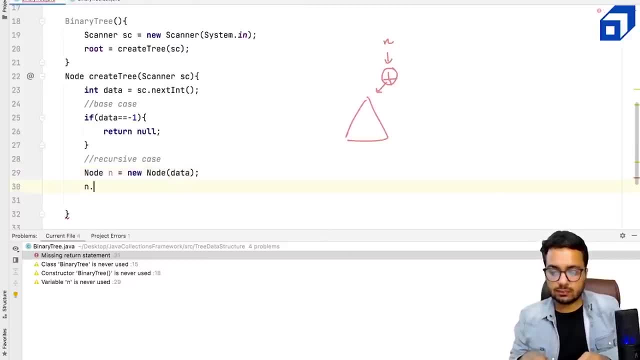 What I can say, that in the left of n, nleft should refer to a new tree which is equal to createTree. Again, scanner will get passed. What should nright point to? nright should also refer to a new tree called create that is returned by the createTree method. 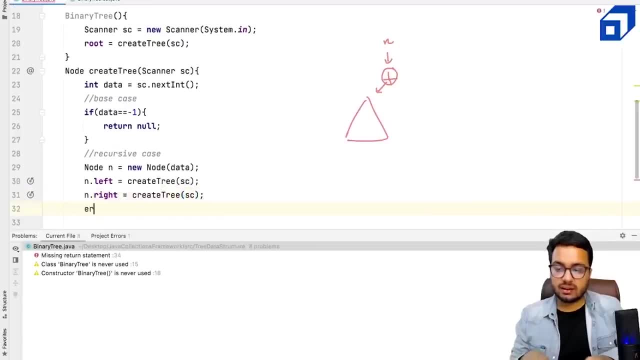 And again, the scanner is going to get passed And then I can return n. So what? I am saying that nright should also point to a new tree. So left subtree, right subtree, This is the recursive way of constructing the tree. Now you might ask: how does this method will actually work? 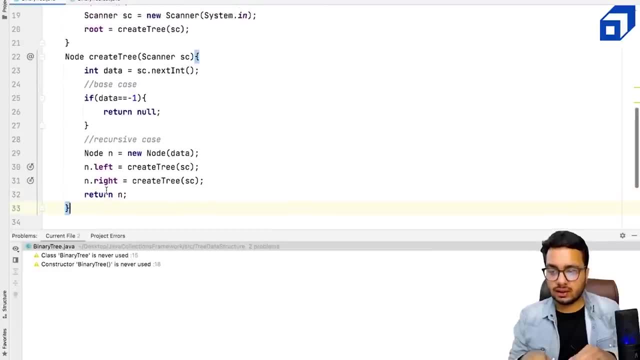 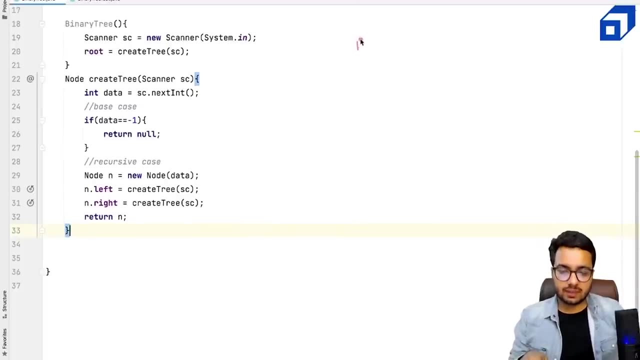 I will show you it will actually work. Let's see how it's going to work. So let us take an example of a more complicated tree. Let's first start with a simple tree. Let's say I have a tree like this 1, 2.. 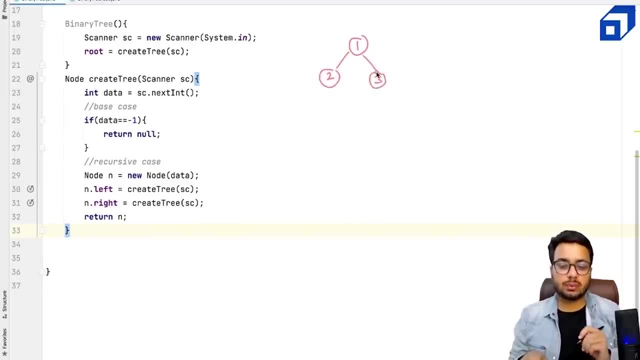 3. For this tree, what is my input going to look like? So input will be 1.. Then it will be 2.. Then it will be left and right of 2, which is minus 1 minus 1.. Then it will be 3 and left and right of 3, which will be minus 1 minus. 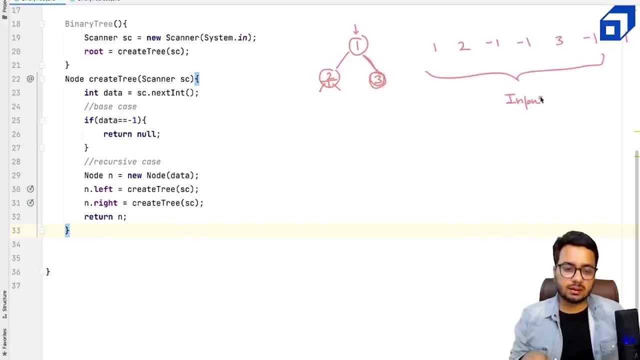 Given this input, I actually want to create this kind of a structure. Let's see how it's going to happen. So I said, fine, Root is equal to createTree. I call this method createTree. It reads something from the user, So 1 integer, it's going to read. 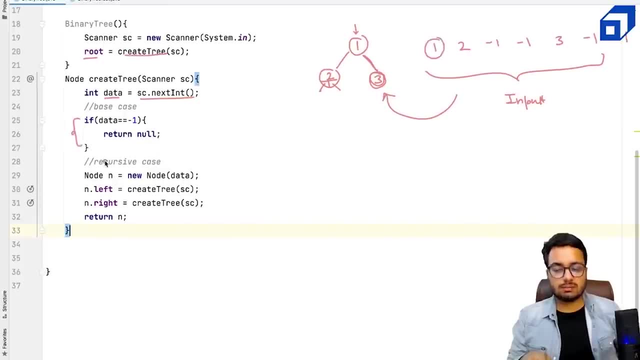 So it's going to read 1.. So data is not minus 1.. Fine, I come here. Node n: this is equal to newNode. So basically I have a stack call In which n is going to say n is a newNode Where the data is 1. fine, 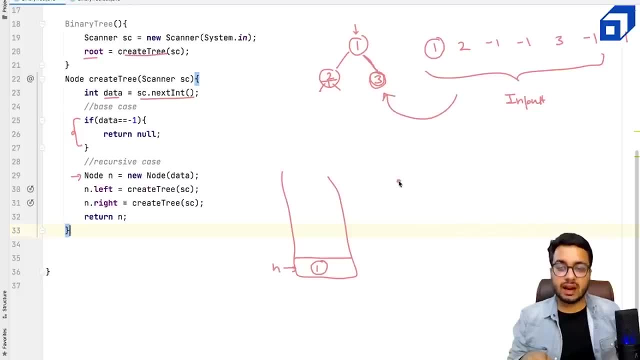 Now nleft. it makes a new call, nleft right. So I said fine In the left of 1.. I want to createTree, So again, createTree is called. If you come again in this function you read something from the user. 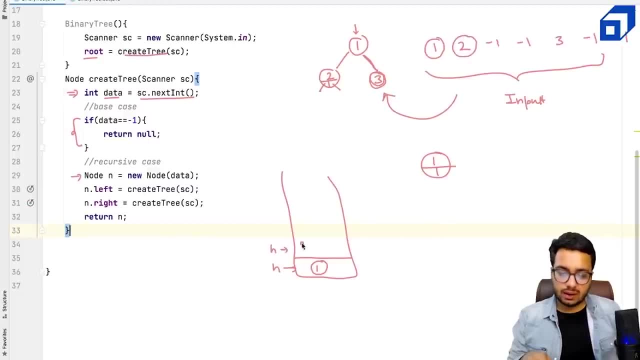 So you read 2.. Fine, You said fine, I create a newNode n. Okay, a newNode n is created. So earlier n was here, Now the new n is here. Right, It's a local variable. It is created in every stack call. 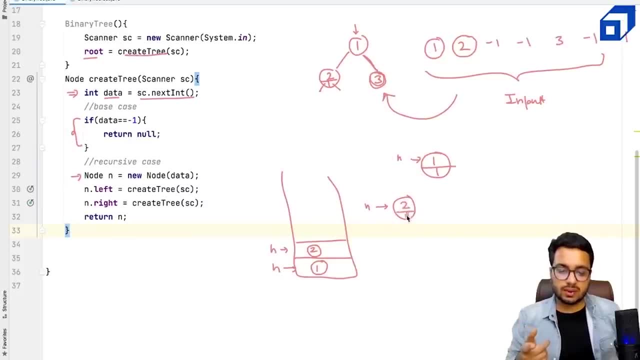 It is here. This is equal to newNode, Where the data is 2.. Fine, Now nleft, this is equal to createTree, Right. So again, I call, I make a function, call CreateTree, Go and do something, Right. 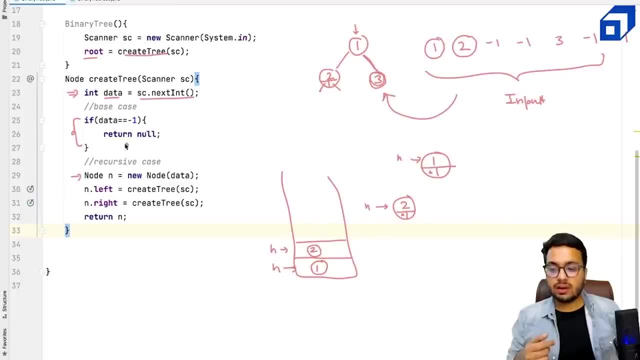 So I have made a call for here. Right Now, if I go and read what is the next number, It is minus 1.. So I return null. Basically, what happens? So 2's left made a call And it got a value that is null. 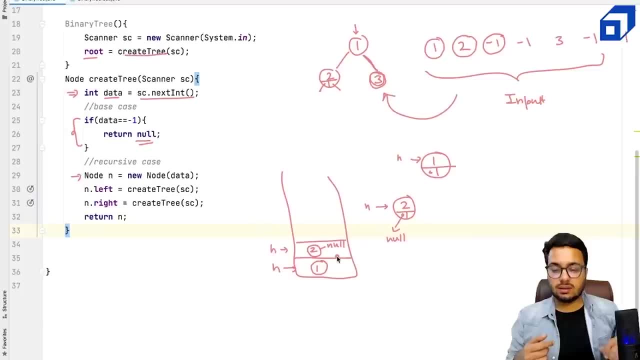 So 2's left starts pointing to null. Now, what is the next number? Now, what is the next call that is going to happen? We are in this stack And I make a call that 2's right This is equal to createTree. 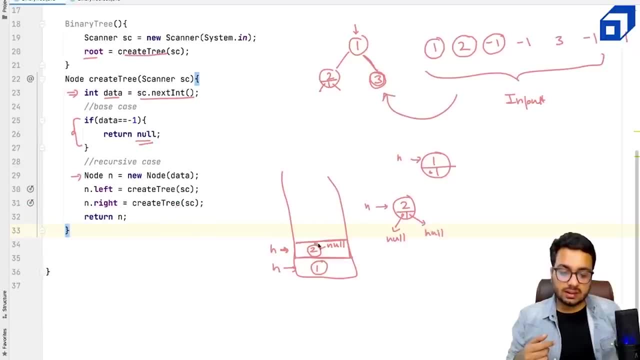 So I make another call Here And this value is also null Right. Once these two calls are over- This one and this one- I return n. So I return this n back Where. I return it to the place from where it was called. 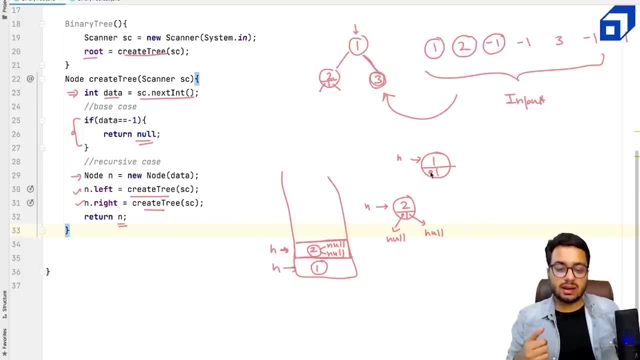 So who called it? One called it, So one gets to know that my left should refer to this node. So by returning this n, This answer goes back to the previous function And one's left is now connected with. Now what is the next call we are going to make? 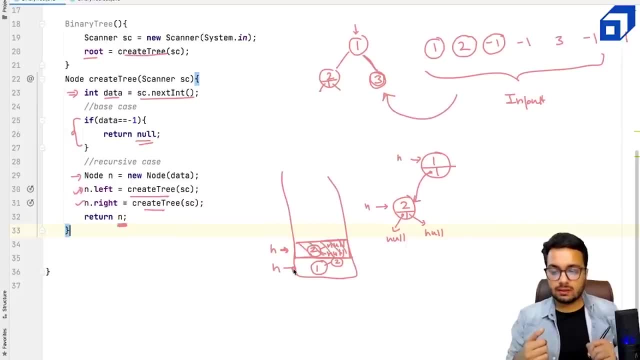 So one's left is now created. So this call is over. One's left is now created. Right Now one says, okay, fine, My left is created. I am pointing to 2.. I will make a call to update my right. 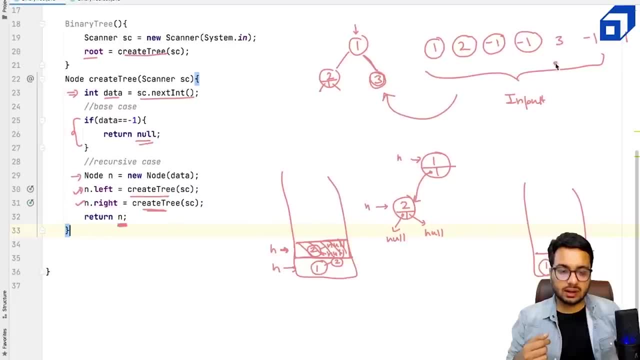 So n dot right? this is equal to createTree, Right? I have already read Again. a new function call is made. You read the next number, That is 3.. You create a new node From line number 29.. You say the new node is 3.. 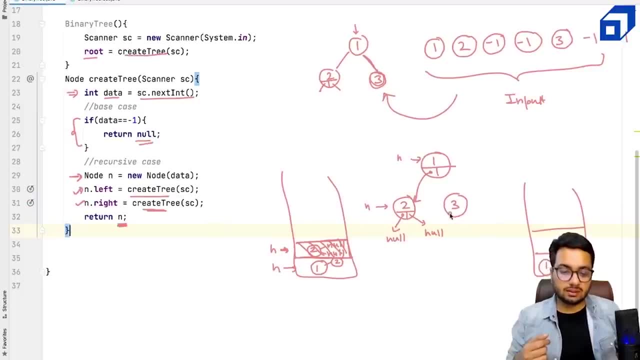 n dot left. This is equal to createTree. So 3's left makes a call to createTree, Which again reads the data That is minus 1.. So you return a null. So 3's left says: okay, make a call. 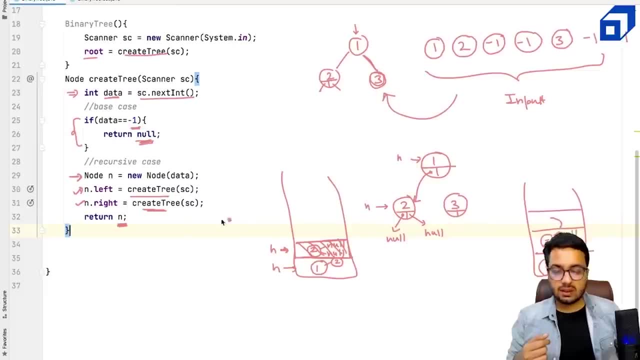 That call says I will return null. Now 3's right says: make a call to createTree. It goes and reads a number that is minus 1.. Again it returns a null, And then you return n. So now n is this: 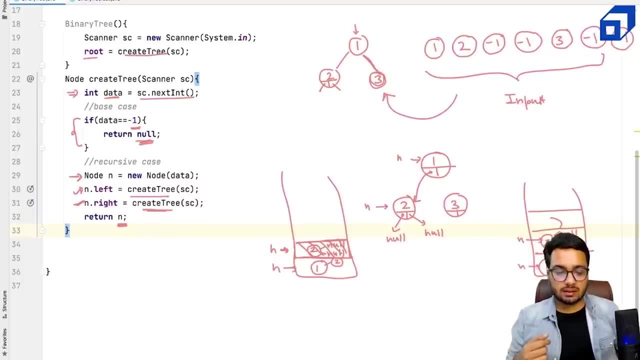 So it returns 3 back. When you return 3 back, what happens? Who called 3?? So 1's right made a call to create this tree, So 1's right is now going to store the address of 3.. So it gets connected here. 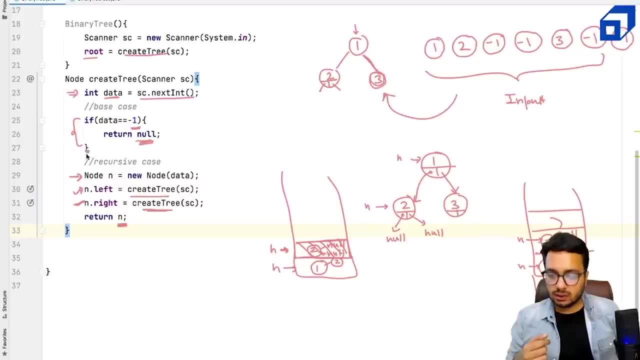 From here. if you return n, Where does it go? It goes back to the constructor, Because this made a call to createTree. Finally, root is referring to the address of 1.. Okay, I will hide myself So that you can see. 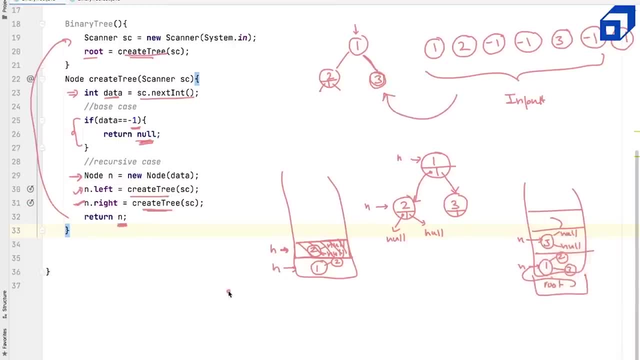 The root is referring to this 1.. So this is how it is happening. So this is a small example Demonstrating how this small tree is constructed using this code. Now I will run this code on a bigger example as well. Now, some of you might not be convinced that whether this code will work for a bigger tree or not, 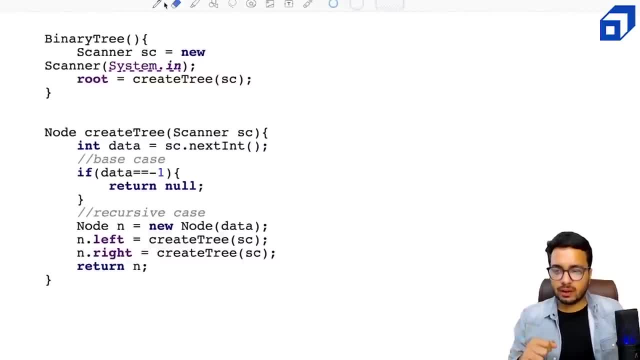 So let us rerun this code on a bigger example. So this is the method: createTree. That again I am explaining with a big example. Let's say I have a tree which should be built like this. Let's say I have 1.. 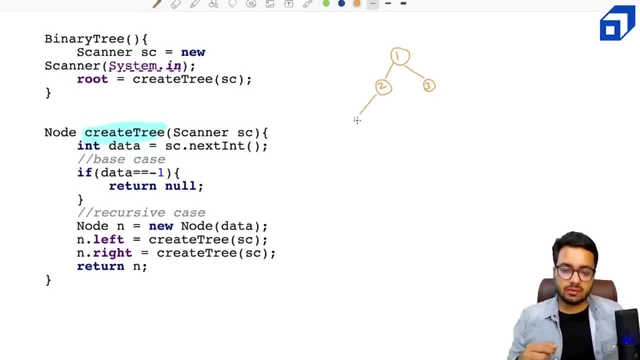 I have 2., I have 3., I have 4., I have 5. And maybe I have 6.. Now what input should I give? So first of all, I will give the root node. So input will be 1.. 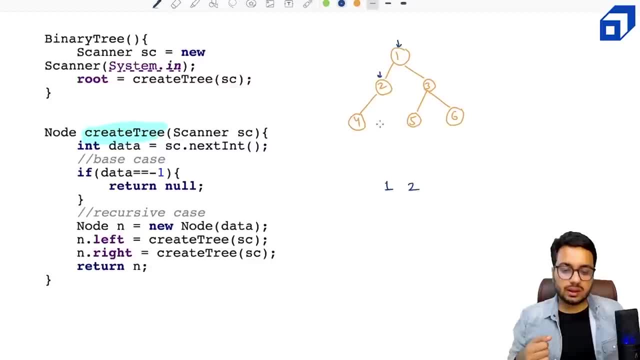 Then I will go left, Input will be 2.. Then again I will go left, Input will be 4.. Then I will go left of 4., Which is minus 1.. I will go right of 4., Which is also minus 1.. 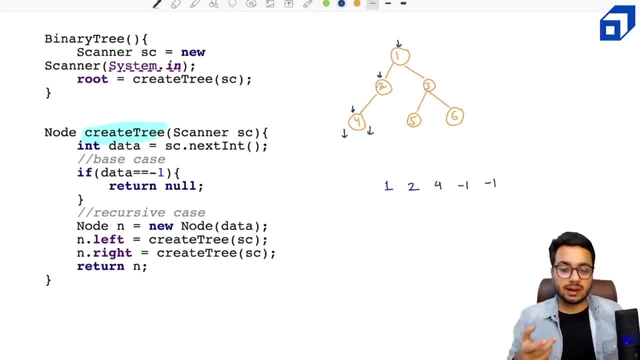 Then I will come back, Because 4 is done. I will come back. I will go in the right of 2.. So right of 2 is again minus 1.. Then I will go back. 2's left is done. 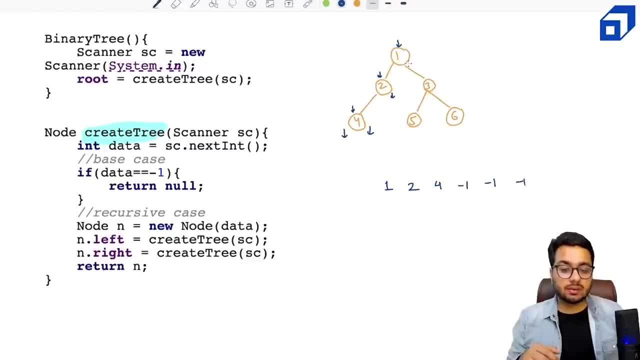 2's right is done. So I will go in the right of 1.. So right of 1 is 3.. Then I will go in the left of 3., Which is 5.. I will go in the left of 5.. 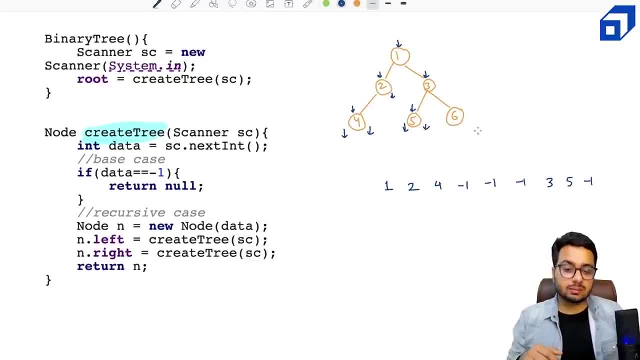 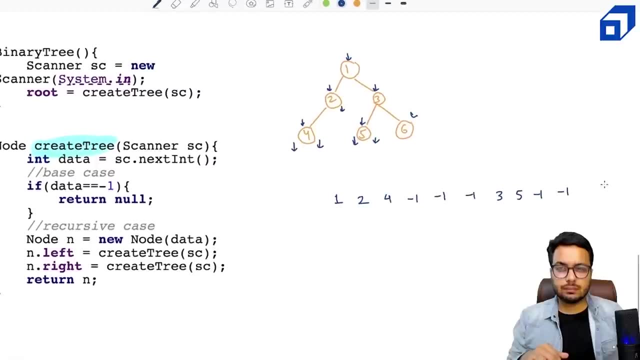 Which is minus 1.. Right of 5., Which is also minus 1.. Then I will go back. I will go in the right of 3., Which is 6.. Then left of 6., Right of 6. Minus 1.. 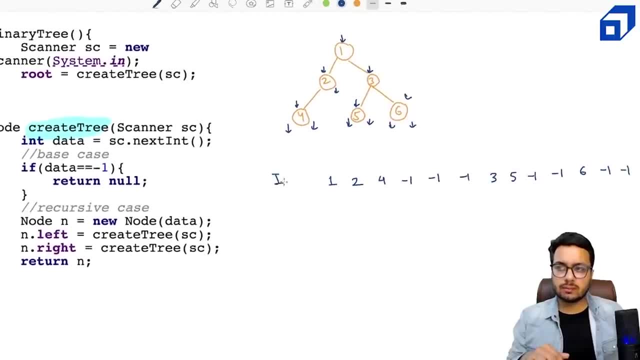 Minus 1.. So the goal is: Given this input, I want to create this tree structure in the output. From this input, I want to create This tree structure. Now let us see how we are going to do it. So, again, I am going to read some data. 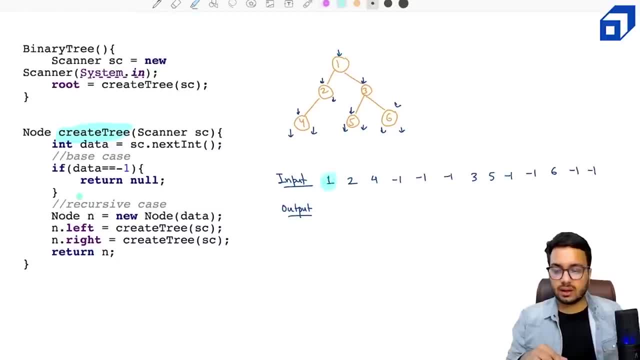 So I will read The first number, That is 1.. I will say: fine, Data is equal to scanner dot. next end, It's not minus 1.. So I create a new node. n Right, So Fine, Let's create a new node. 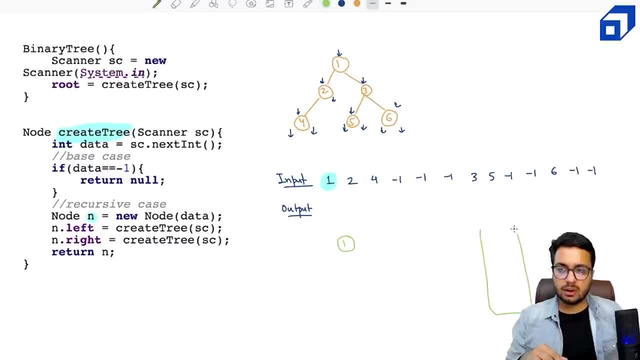 N, that is having data 1.. Let me draw the stack as well. Side by side. So n is referring here Right Now. what? So, if you want to learn Key, What is the function that is currently executing? So that is. 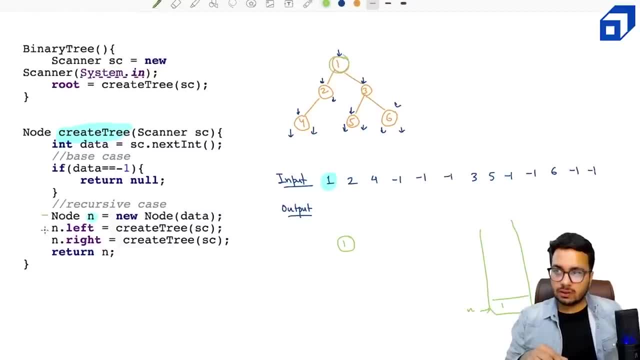 At the top of the stack, So n is created. Now you make a call N dot left equal to create tree. So you are making a call to create something in the left of 1.. Right, So 1 makes a call for the. 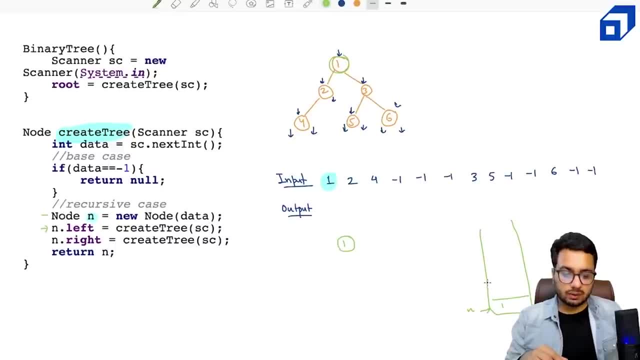 Left part. So again You go Call this function. You read data. So data is the next number, That is 2.. Fine, You again create a new node. Now this Function is paused. This function is paused here. 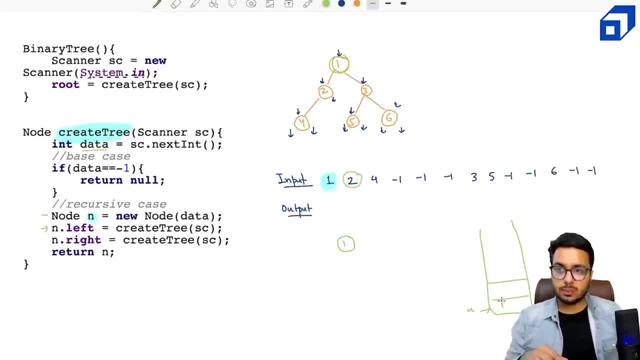 You said Fine, So you create a new node. Now this Function is paused. This function is paused here. You said Fine, I am going to create a new node, And That node is 2.. That node is 2.. 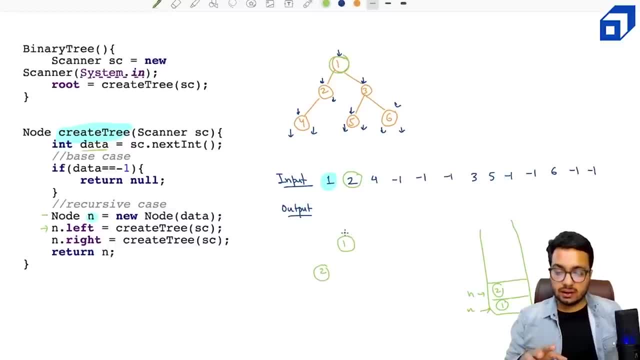 Right Now it is not connected. It is not connected with 1. Right. And again You say: I want to connect something in the left of 2. What will be that something? Again, You make a function called to create tree. 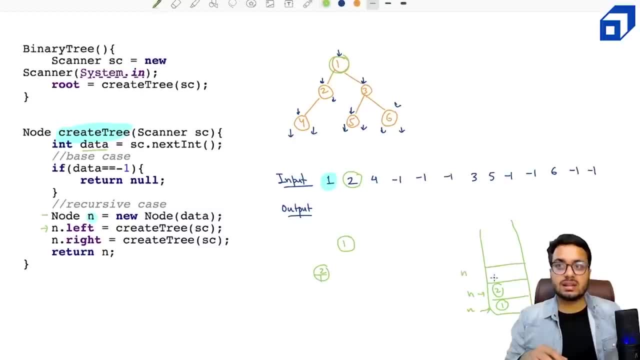 So again This is paused And it is expecting to build its left tree. So you again Call the function create tree. You read the data. So now you are going to read 4.. So you read: 4. You read. 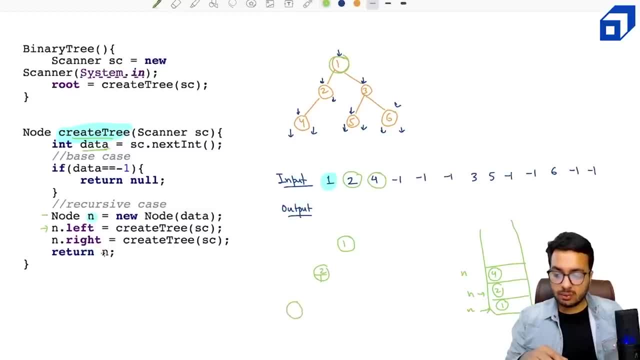 4. Now 4 says Okay, I am. I am a new node And I will create something in my left. A 4's left Makes a call To create tree. The 4's left Again makes a call. 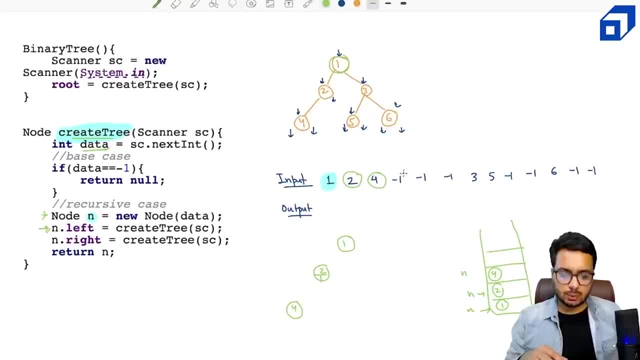 To create tree And in this case You read data. The data comes out to be minus 1.. And if the data is minus 1. You return null. The 4's left Gets to know that My value is. 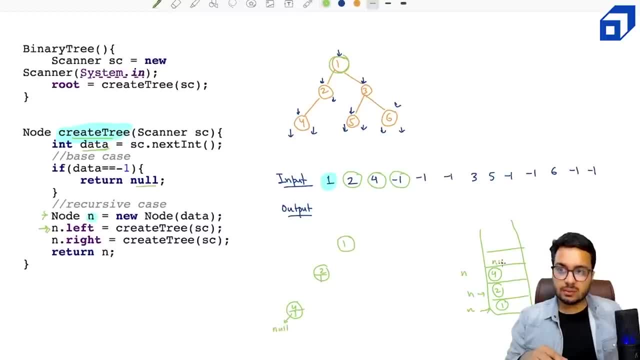 Null Right. So a null is returned from this function Which is attached with Left of 4. Then Then you hit this line for the first time In this function: call Right N dot right. This is equal to create tree. 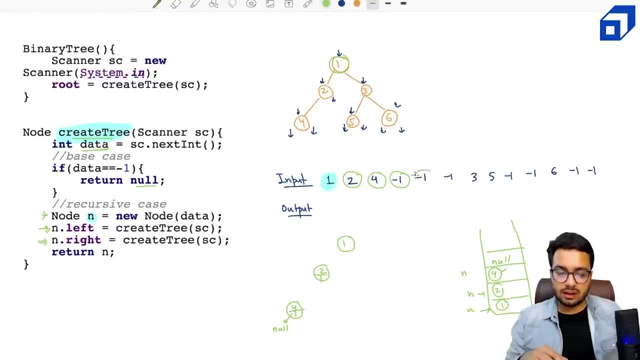 Now you say, Okay, I will again call create tree. I will Read this number. This number is again minus 1.. It returns a Null in the right, also 4's left and right. They are null. That means 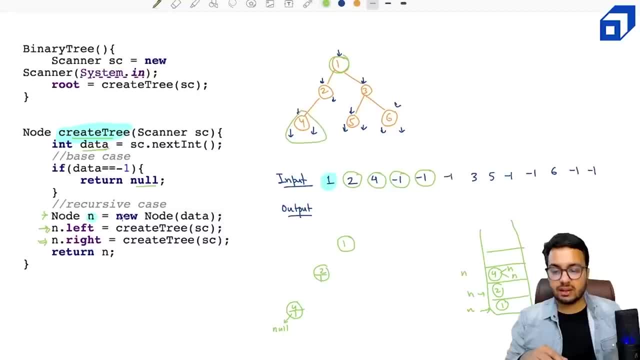 The subtree of 4 has been created. This subtree is finished. I will return N. This is null And I will return N. N. is this Now where this return value will go? It will go back to the place From where it was called. 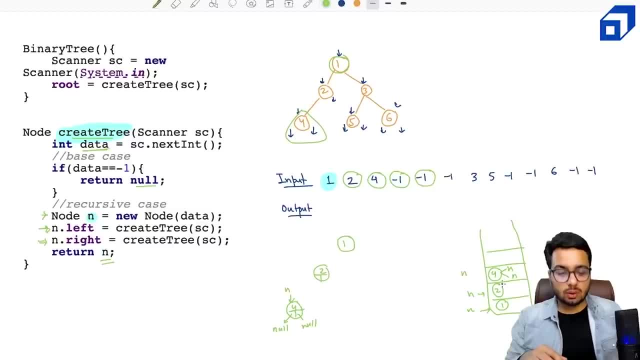 So who called it? 2's left called it. So 2's left is now connected with 4.. And this function call is Over, Right. So 2's left Is connected with 4. Right Now. this is the point. 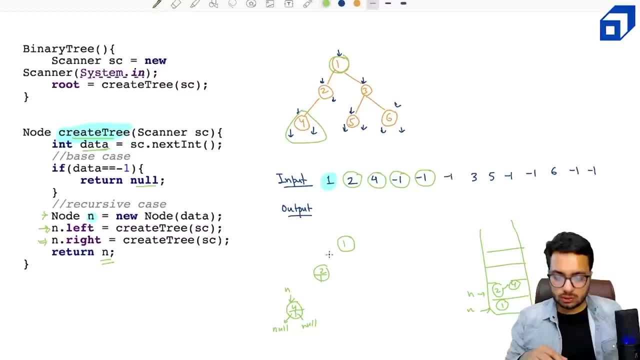 Where this connection has been established Right. 2 made a call to 4.. 4 said Okay, I will build myself. Right So. 2. Made a call to 4.. 4 said Okay, I will build myself. 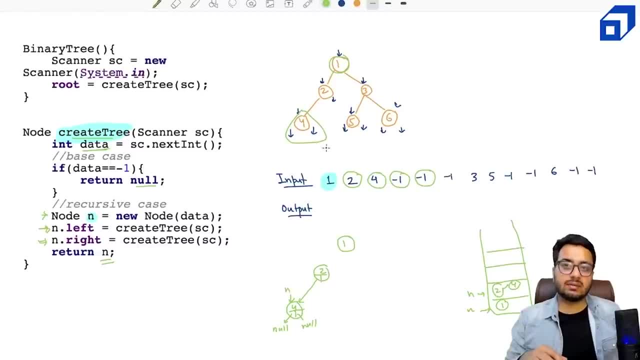 Right. 4 said: Okay, I will build myself. I will build my left and right, Which are null, And now I will return myself Right. So 2's left is over. Now what will happen? 2 will make a call on the right. 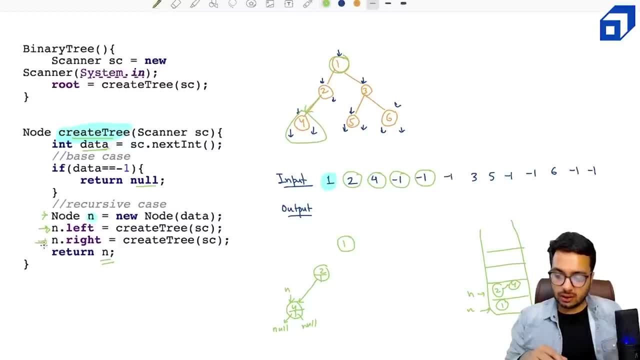 The right subtree. So 2 makes a call here. N dot right, This is equal to create tree. Now what do I read Next? Again, It is minus 1.. So I return a null. I return a null from here. 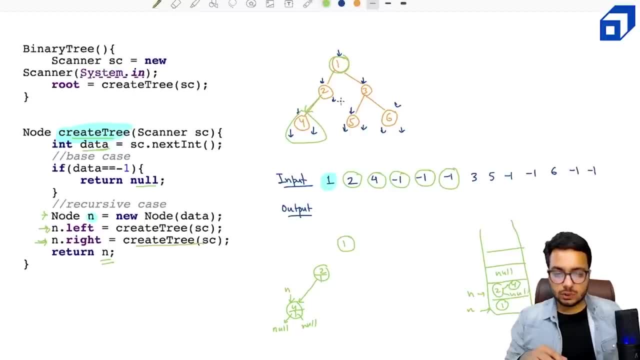 So 2's right Is null. So 2's right Is null. It's not referring to Anything, Right? So this value is N Null. Now 2's left Is done, 2's right. 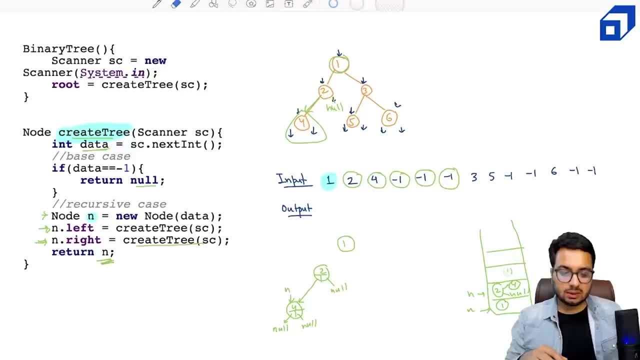 Is done. I read I say return n. So return n means What is the function That is at the top? At the top, I have this function. I'm going to return This subtree, This whole subtree, Back. 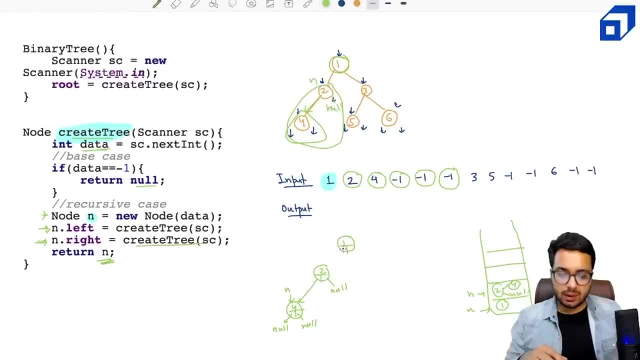 To 1.. So basically, 1 will get to know That my left Points to this n And hence The left subtree Of 1. Has been built. Now I will build The right subtree, Right, Okay? 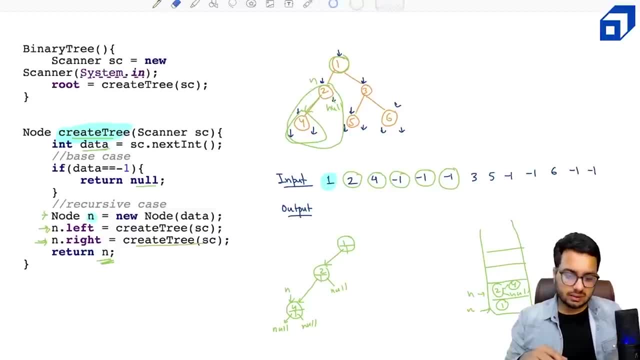 So 1 will say: Okay, Fine, My left subtree Has been built. This is over From the call stack Once. 1 is now connected With 2. And 4. Right This tree. A 1 will say: 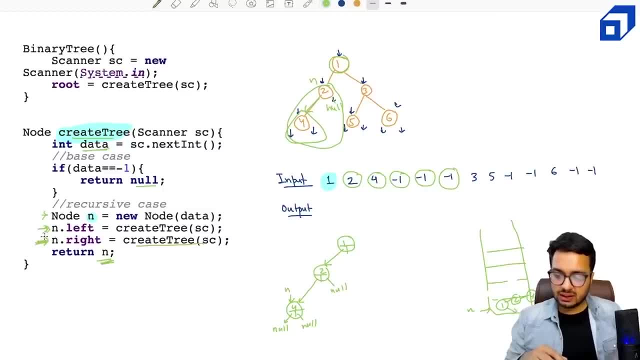 Okay, Now It is my turn To call the right. So once Left is done, It will execute This line And dot Right. This is equal To create a tree. Now, This is the new node. So 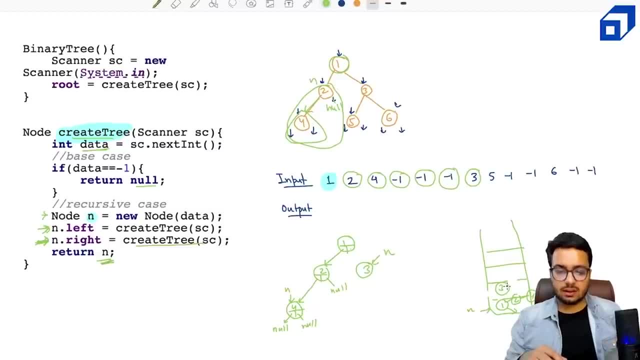 3 is created, And then You Again Make a call To the left. You read a number: 5 is created, This is new node. And you again Make a call To the left, Minus 1.. 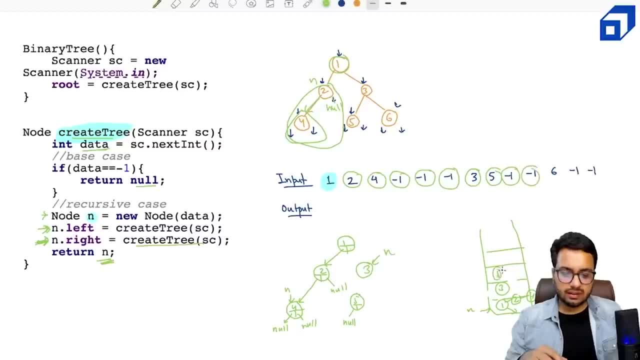 So 5 left Is null Again. You make a call On the right. 5 left Is null Again You read Minus 1.. So 5 gets attached In the left Of 3.. 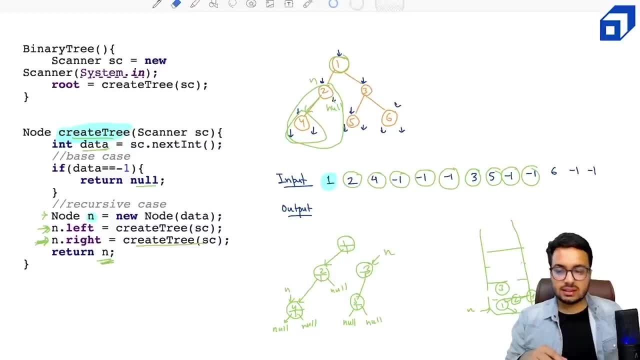 So 5 is returned, It Gets attached In the Left Of 3.. So 5 goes here. Then Again, What is going to happen? You will say, Okay, I want to build something On the right. 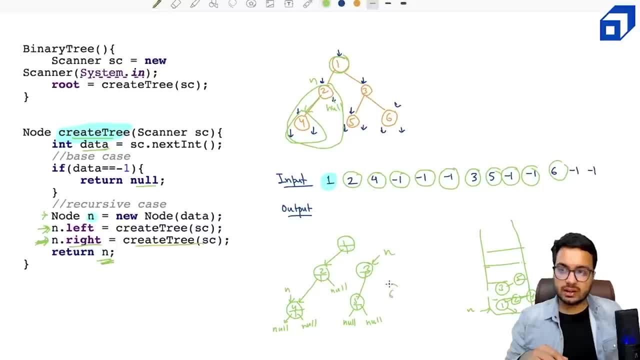 Of 3.. So 3 is left Is done, 3 is right Is done, So I will again Make a call. It will read 6. A new node. I will read the right, Which is also. 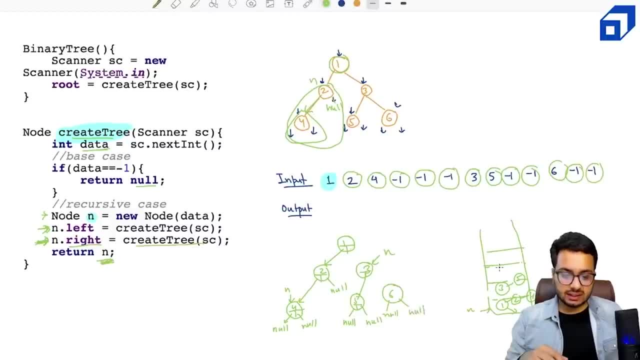 Minus 1.. And then I will return n. So When you return n, This 6. Is returned back To the right of 3.. So This 6 is Being attached here. And then You say: 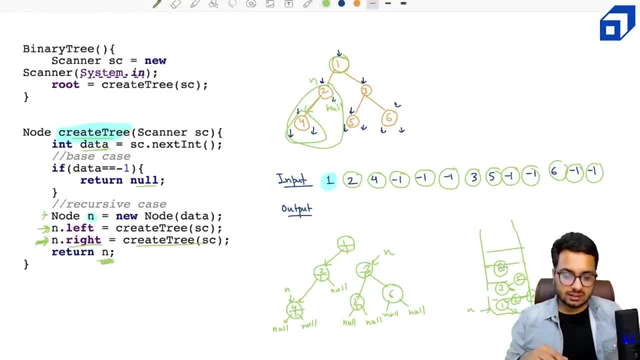 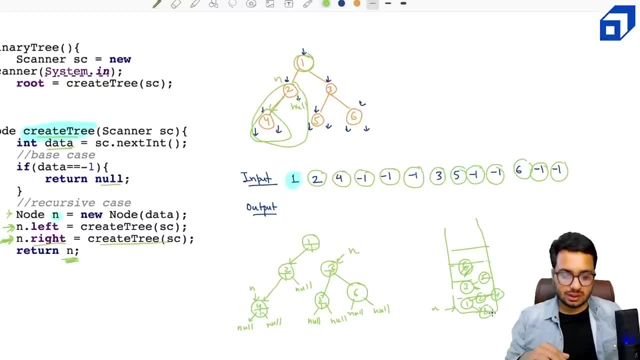 Okay, I am going to return n. So When you return n, You return this 3.. Back to 1.. So Once, Once Right Is going to point To This Subtree 3.. 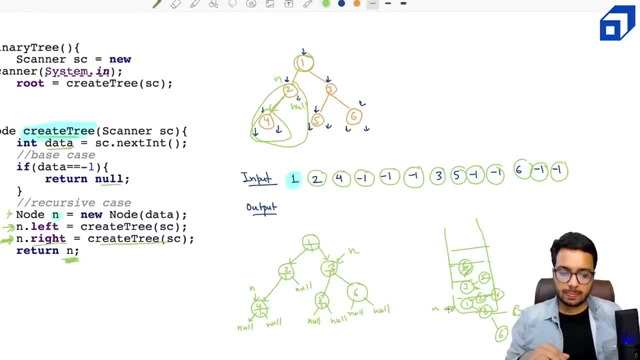 Is attached With 1.. Finally, When you are here, This call is over, Right, You will return n, So n will be This node, And it is returned Back Here. Root Equal To. 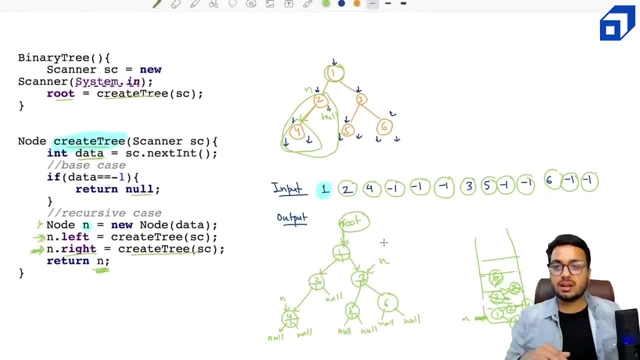 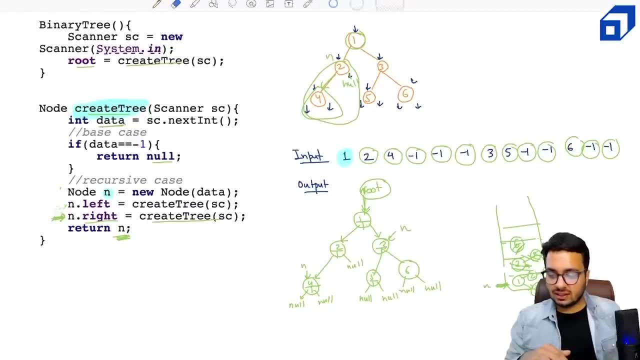 Create Tree. This, This Becomes The Root Of The Tree. So Root With This Recursive Function. Okay, This Way Of Building The Tree, It Is. 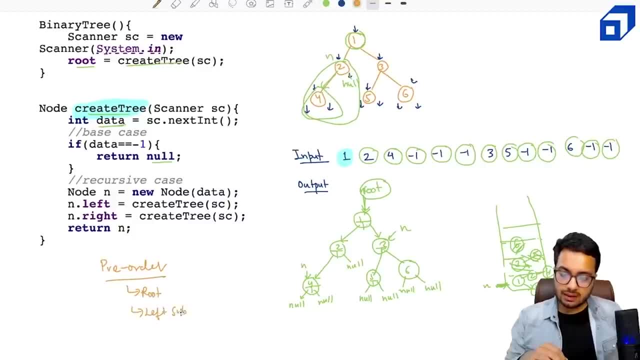 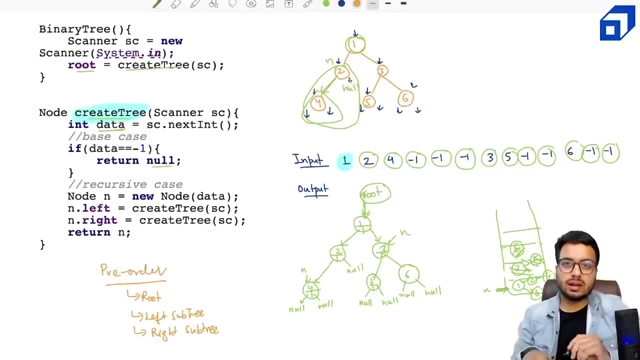 Called As Preorder. Preorder Means First We Are Building The Root Node, Then We Are Building The Tree Function Right, Or Create Tree Function Right. 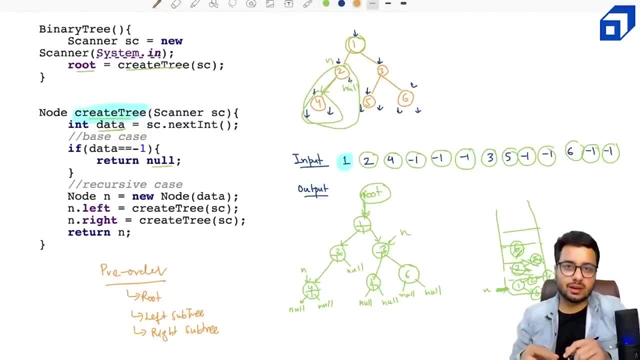 Next, We Will Look At How We Can Print This Tree In A Similar Way. Now Let Us Talk About The Root Node Of The Tree. 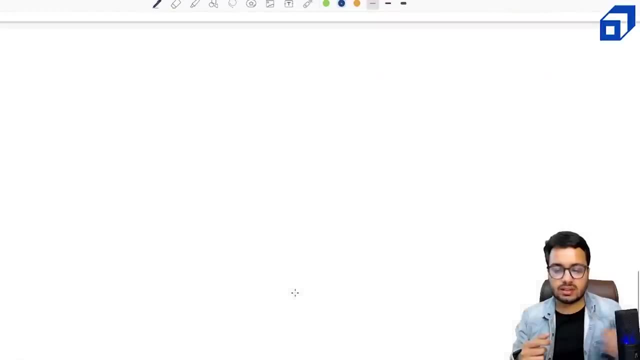 Right So. A Tree Has Been Built, A Tree Has Been Created. We Want A Way To Go To Each And Every Node, Right So We. 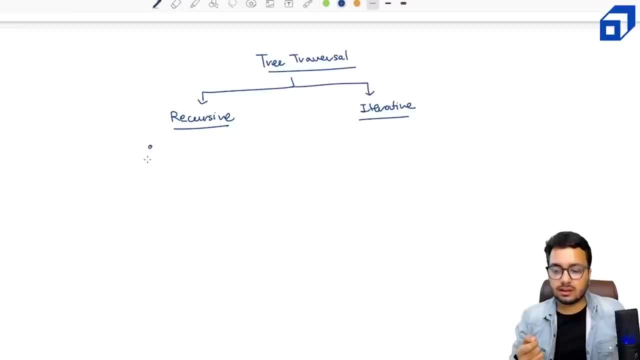 Will Discuss All These Ways Now, Right In Recursive Way. Again, There Are, It Depends Upon The Ordering. Okay, The Way Is Same. We Basically Recursively. 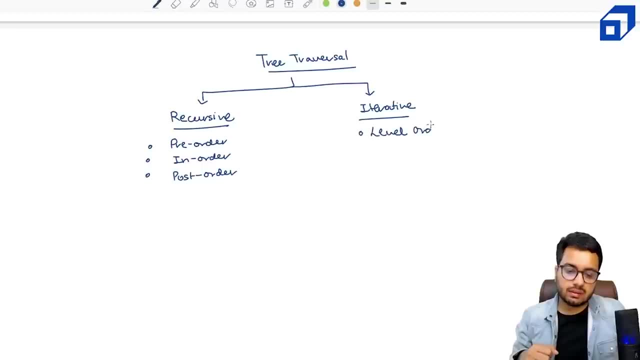 I Was Only One Way That Is Called As Level Order Reversal Right. So All Of These Traversals, They Are Going To Travel All 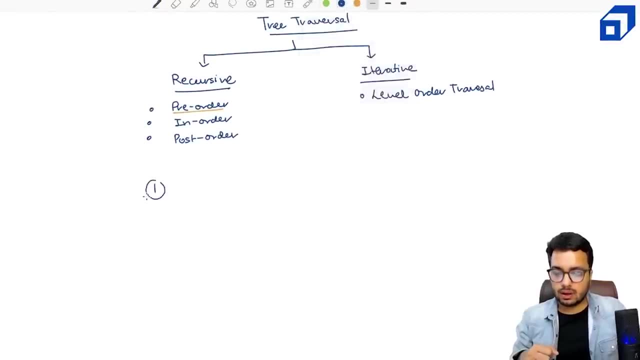 The Nodes, But The Order In Which? Or Five? What Is This Pre Order? Traversal Says That. Fine, What I Will Do, I Will Travel. 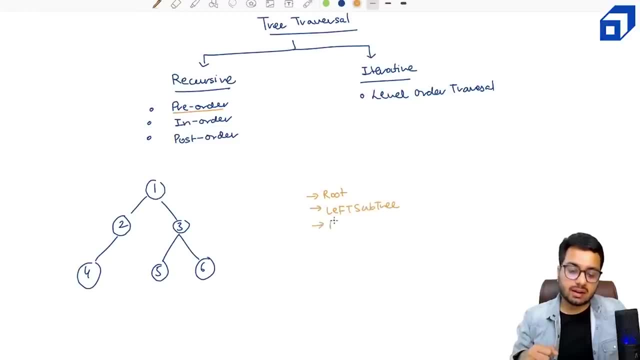 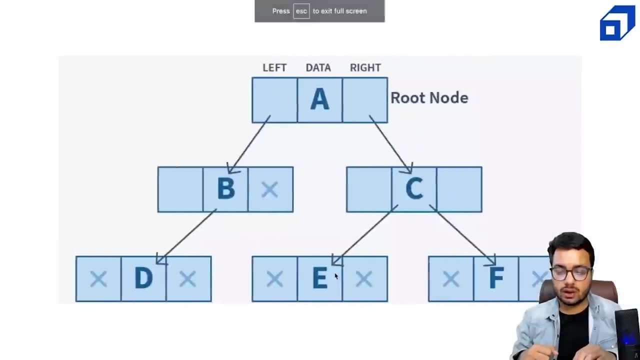 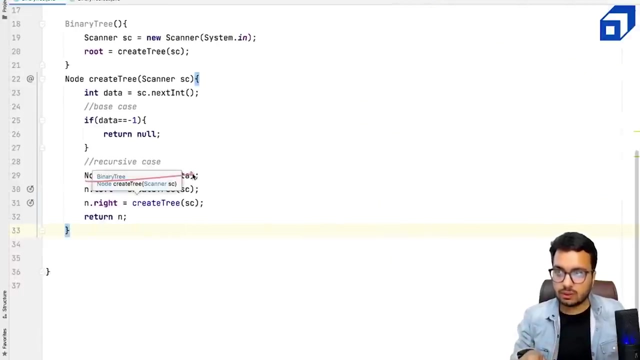 The Route Note, Then I Will Recursively Traverse The Left Subtree. If You Look Carefully, We Are First Building The Route Note And Then 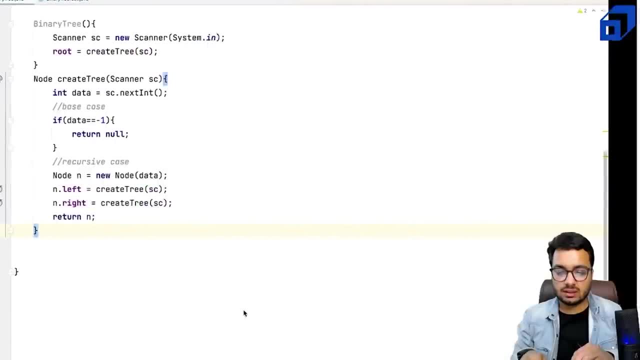 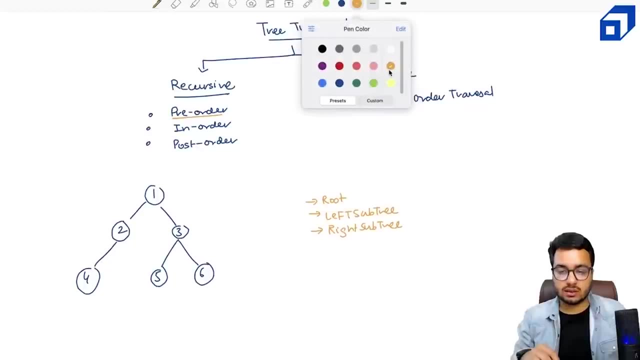 We Are Recursively Building The Left Tree. If You See, In This Case The Output Will Subtree. So This Whole Is My Left Subtree. 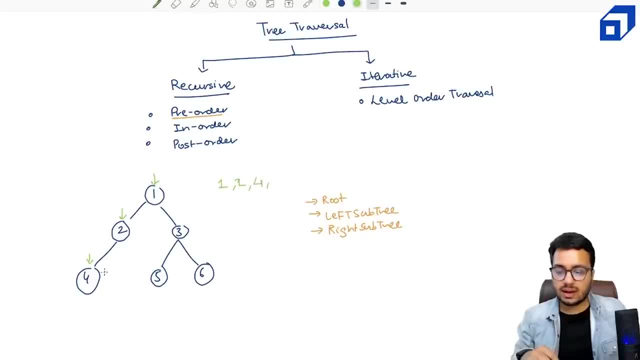 So I Will Print The Route Note That Is To. Then I Will Go To The Left Subtree. So Left Is Has Been Printed, So 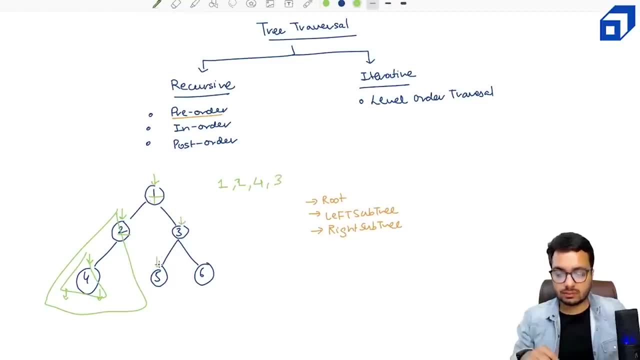 I Go To The Right Of One, So I Come To Three. I Will Print Three. I Will Go Left. I Will Go Left. I Has 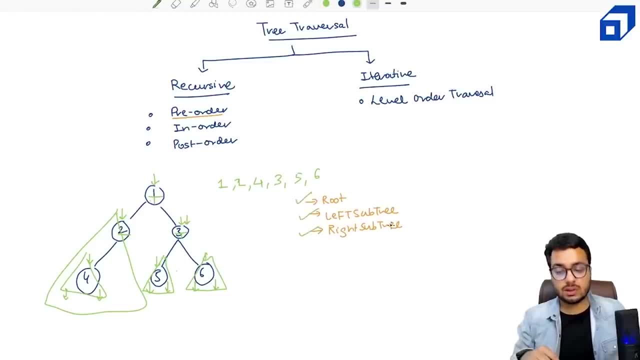 Been Printed, So Route Has Been Done, Left Of Three Has Been Done, Right Of Three Has Been Done, So This Whole Tree Has Been Printed. 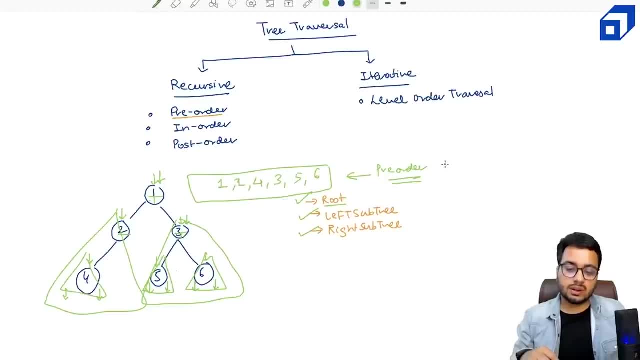 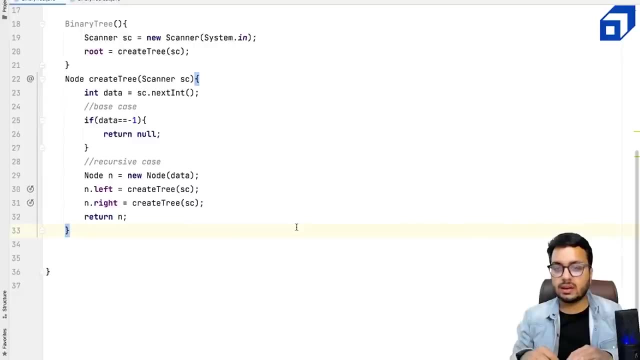 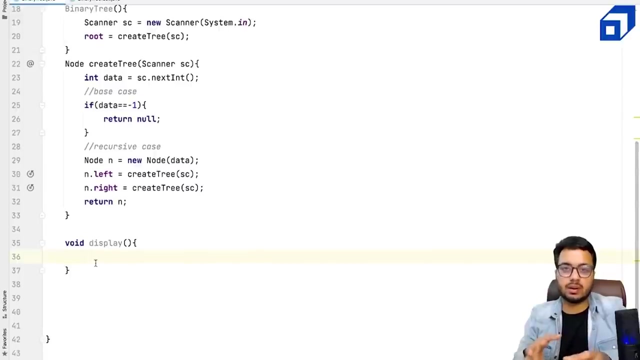 I Come To. This Will Be The Pre-order Output For This Tree Right Now. Let Us See This Thing In Our Code As Well. Let's. 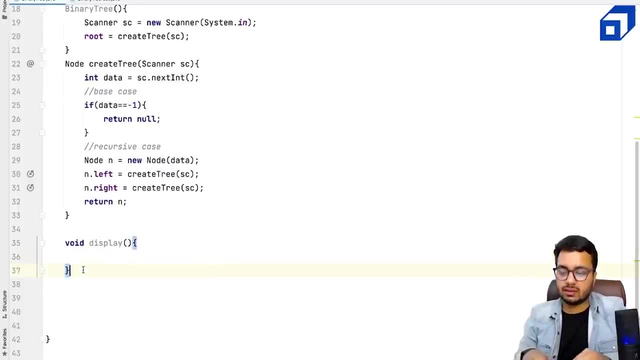 Write A Pre-order Print Method. Let's Avoid Pre-order. Avoid Pre-order Print. Now, This Is A Recursive Function, So I Have To Tell At What. 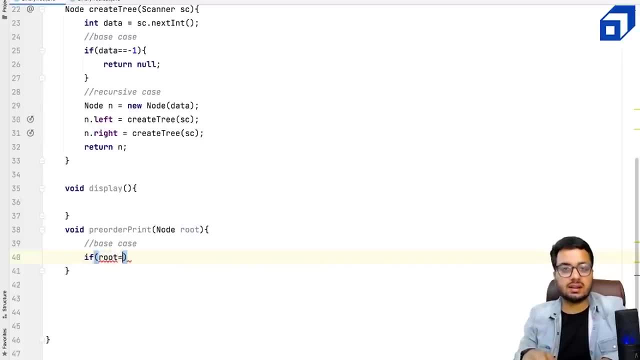 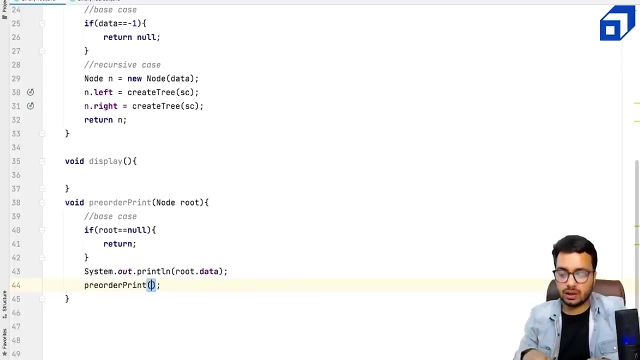 Node I'm Currently At, So I Will Simply Return. Otherwise What I Will Do: I Will Print The Root Data. Go And Print The Left. 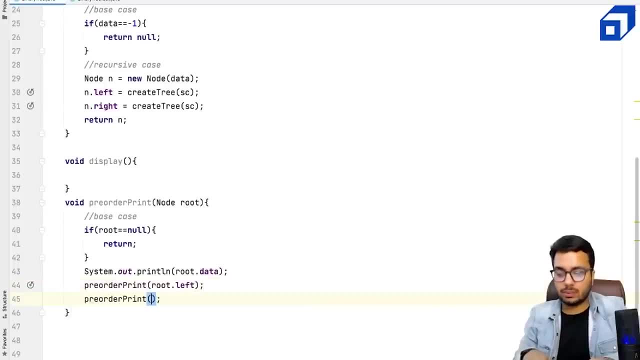 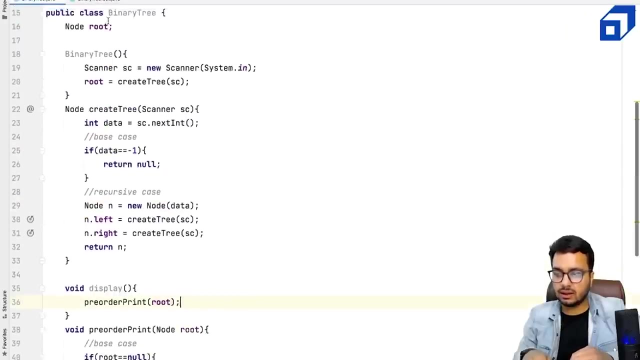 Subtree Recursively. So Pre-order Print Route Left, Then Pre-order Print Route The Root Of The. Now Let's Do One Thing, Let Us Test. 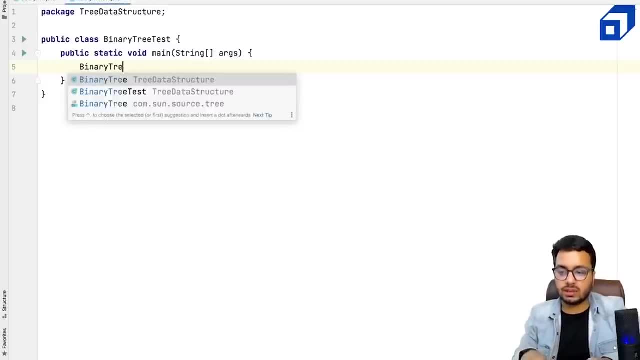 Our Binary Tree Because We Have The Create Method, We Have The Print Method. Now I Can Do Print. Now Think Of Any Tree That You 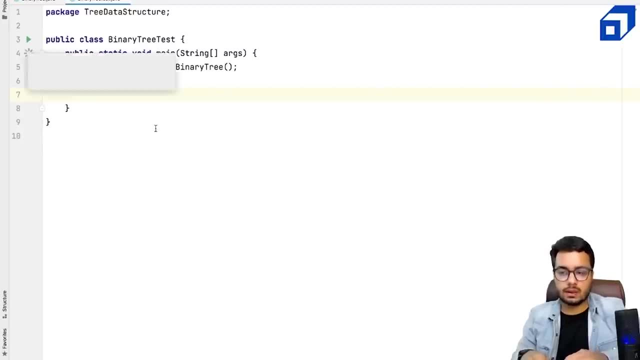 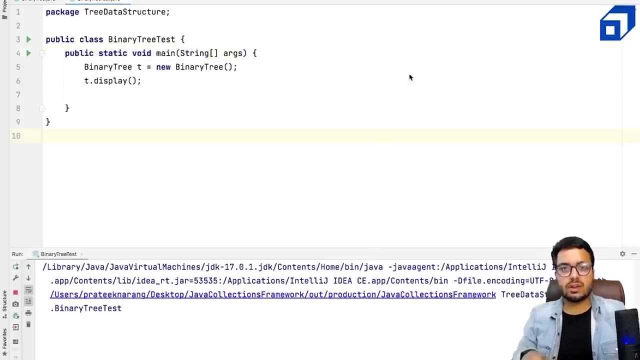 Want To Make. We Will Give It As A Input Here. Sorry, I Should Run This File Now. This Is Now How This Tree Will Be. 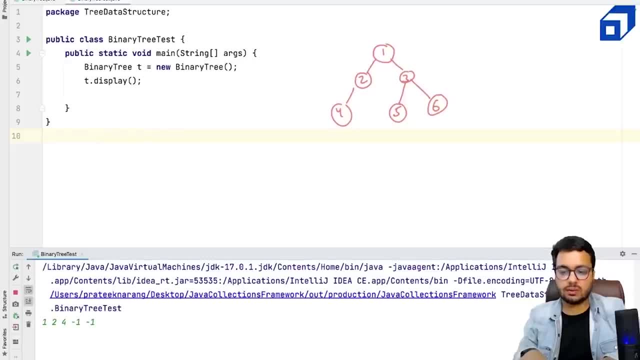 Given As Input. So You Will Input One, Then Two, Then Four, Then Left Of Four Minus One, Right Of Four Minus One Given And 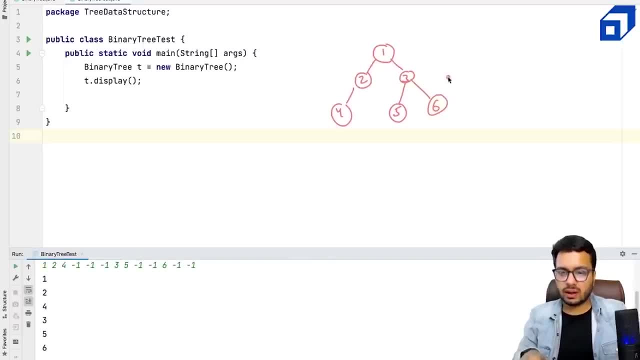 Now I'm Saying That Let Me Print This Tree. What I'm Getting? I'm Printing One, I Go Here, Then I Go To Two. Fine, 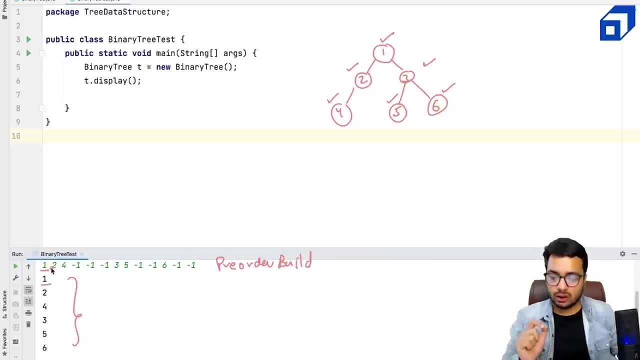 Then I Go One, One, Two, Two, Four, Four Minus One. I'm Not Printing Skip, Skip, Skip. Then Three, Five, Three, Five, Absolutely Correct Minus. 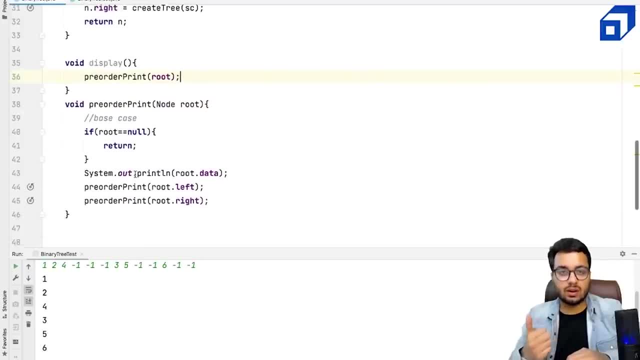 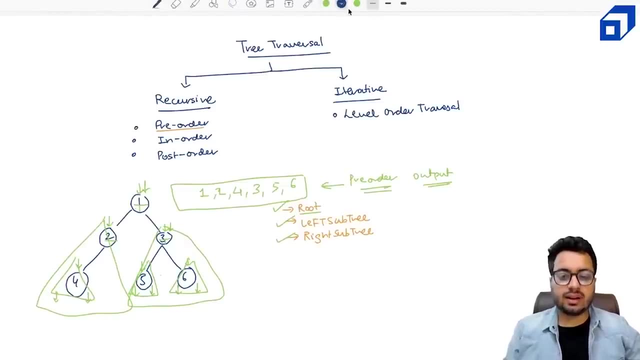 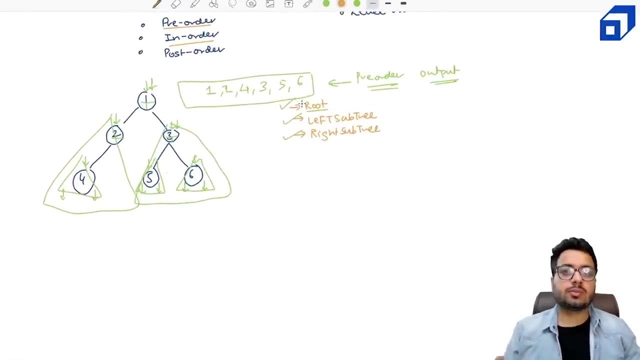 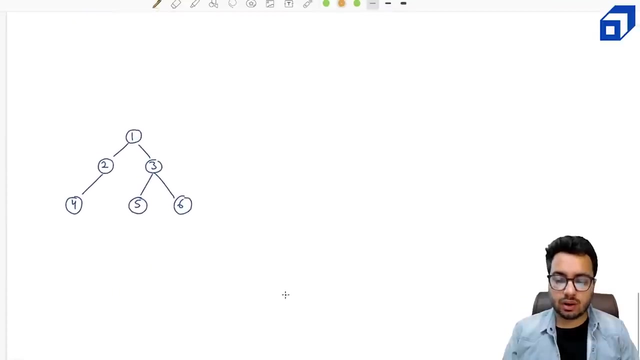 One. I'm Not Printing Six, Six Right Now. Let's Discuss The Next Type Of Recursive Printing That We Call As In Order Print. Okay, So. 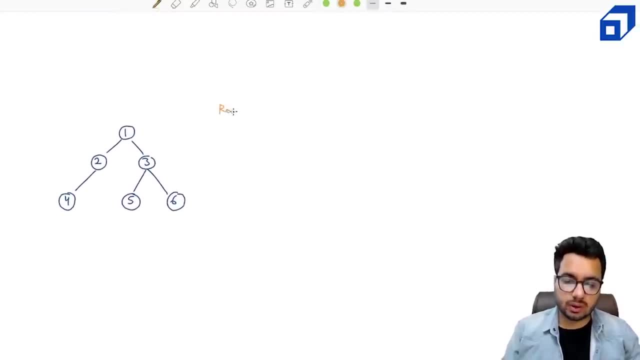 I Hope Pre-order Is Clear. Now We Are Moving To In Order Right Subtree. That Is What The In Order Printing Would Mean. Let Us 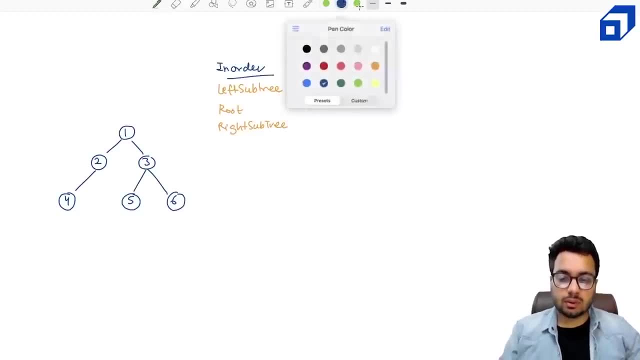 Drive In This Logic On Our Code And See What Do We Get In Order. Print The Left Subtree So That Means I Will Have. 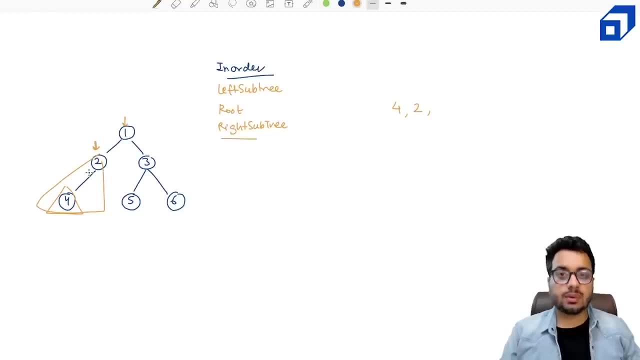 To Print For. So Four Will Be The First Output That I Will Get. Now. I Will Print The Left Subtree Before I Print Three. 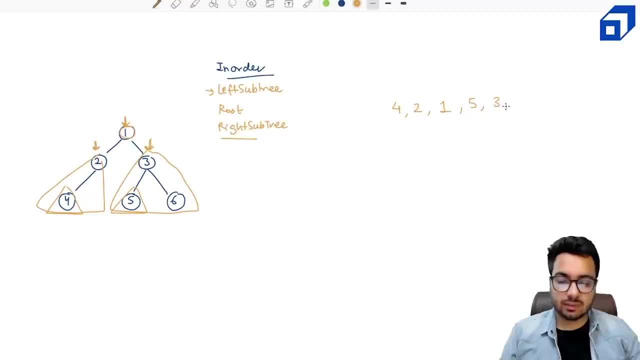 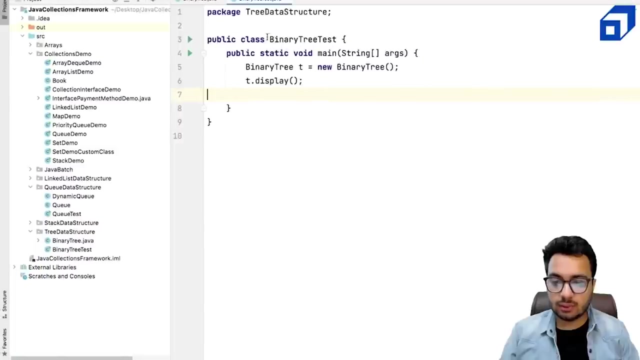 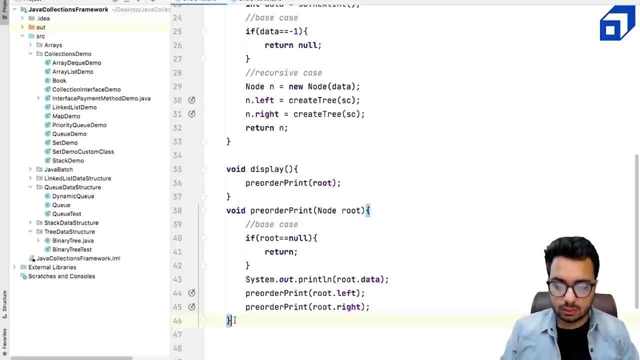 I Will Have To Print The Left Subtree, So Only One Node. I Will Print Five, Then I Can Print The Root Node, What I 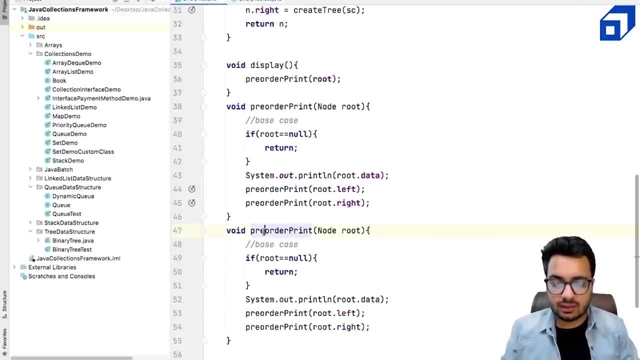 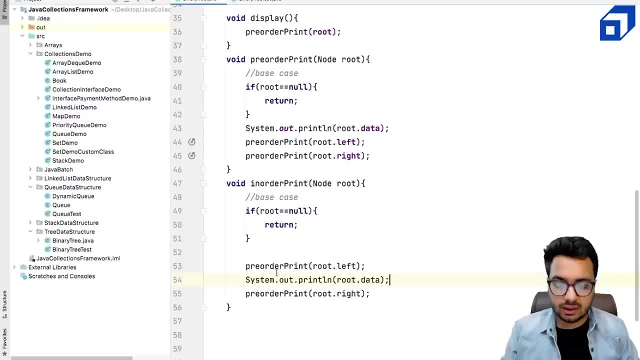 Will Do. I Will Create One More Method, Called As In Order Print. In This Case, The Root Will Be Printed In The Middle And This 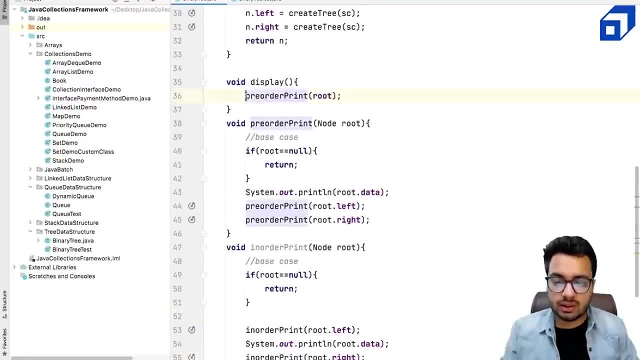 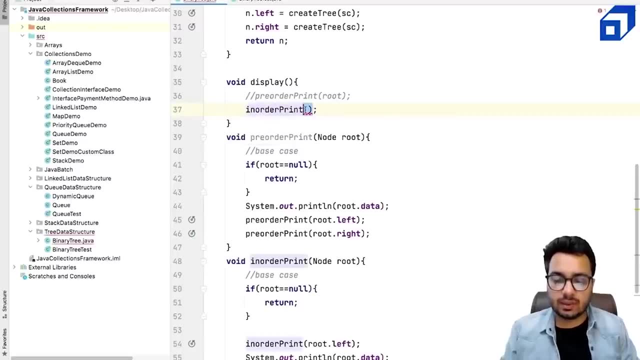 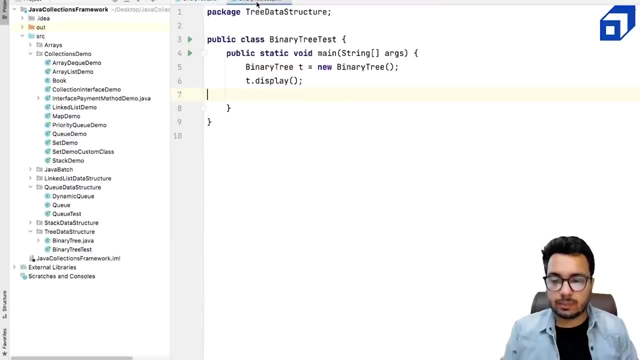 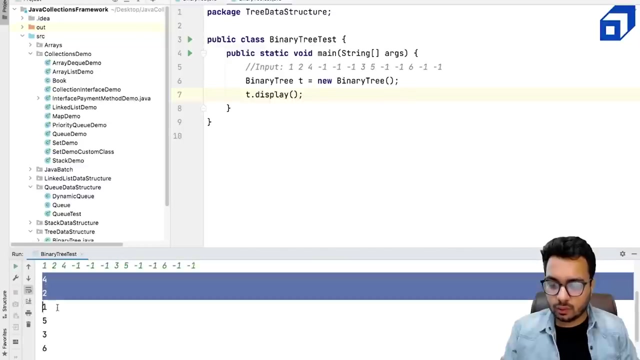 Call Will In The Display Method. Instead Of Calling Pre Order Print, Maybe Let's Just Call In Order Print This Time. I Want To Display. 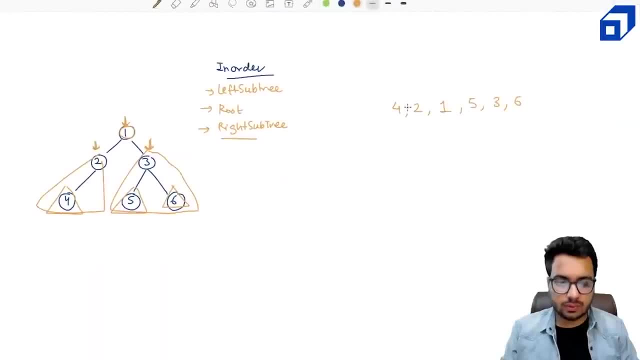 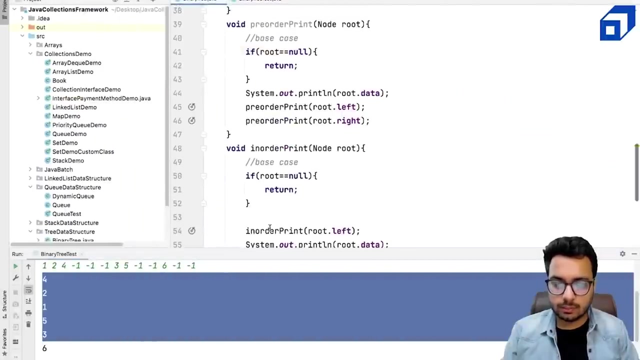 The Tree Using In Order Print. Now You Might Be Interested In Doing A Call Stack Analysis Of This Right. Let Us See How We Can. 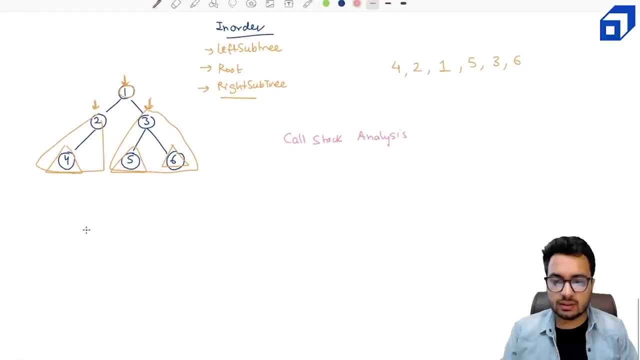 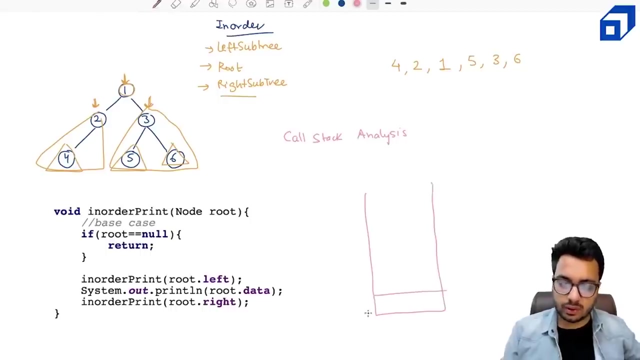 Do The All Stack Analysis As Well In The Beginning Of Calling. So The Call Stack Is Empty, So We Called In Order. Print Where The 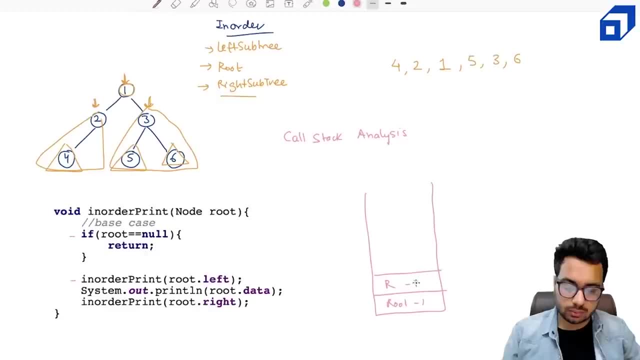 Route Node Is One. So I Say Route Is One, But I'm Not Again. I Make A Call On The Left When You Make A 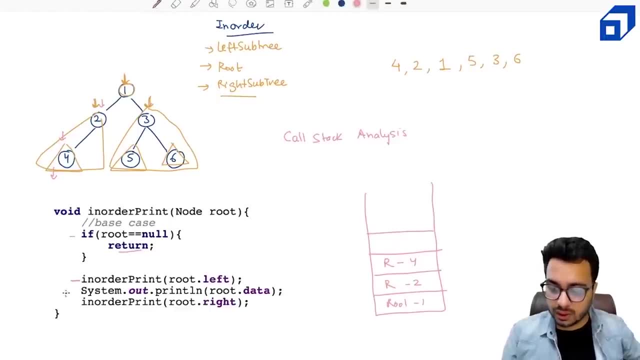 Call On The Left Of Four, You Actually Come Here. This Is Null. If This Is Null Again, You Make A Call To Null And You 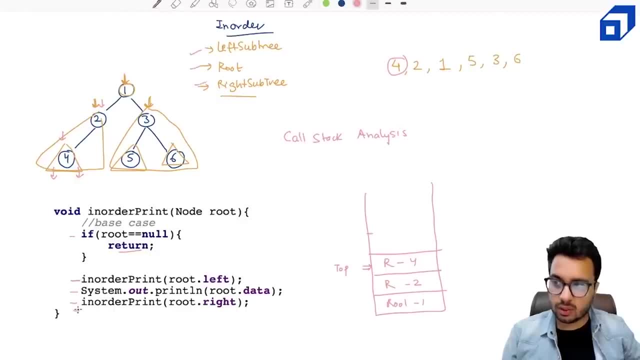 Return, So You Come Back Again. You Are Here For Four. You Have Done All The Three Things. Left Is: Yes. Have I Printed Root Data? 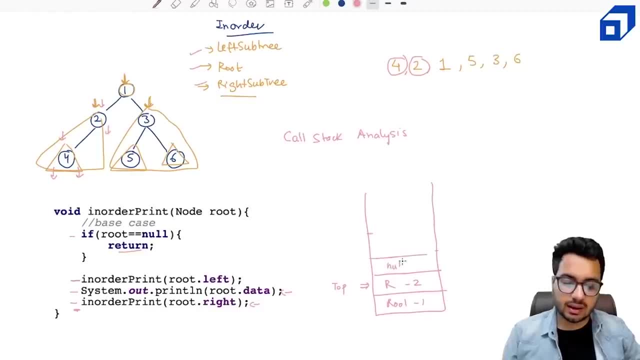 No, I Will Print It Now. Have I Printed The Right? No, So I Make A Call On The Right. I Make A, You Do A. 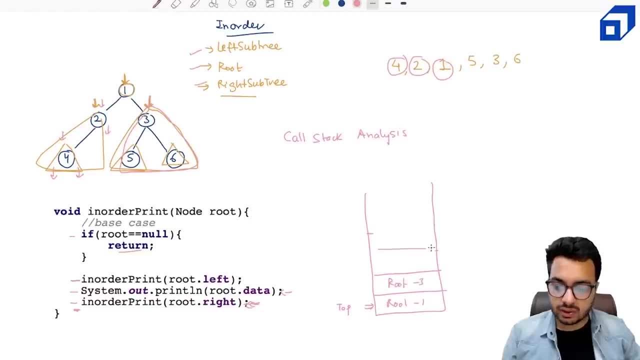 Similar Process. You Come At Three, So Root Is Three. Then You Make A Call On The Left. That Is: Root Is Five, Five Left Is: 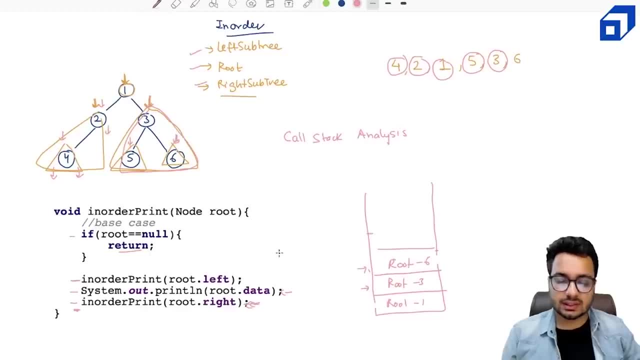 Here, You Went Here, Then You Came Here Six. Now Route Is Six Left And Right. They Are Null. So Six Will Get Printed, Right Is: 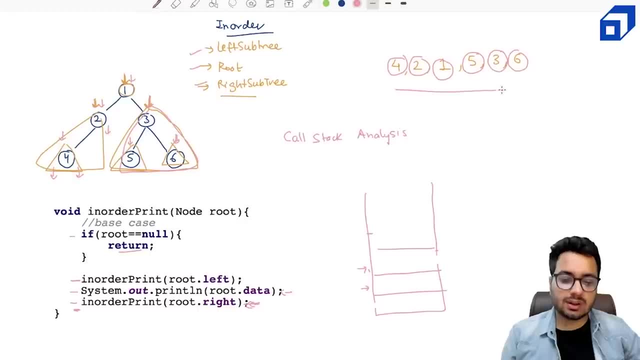 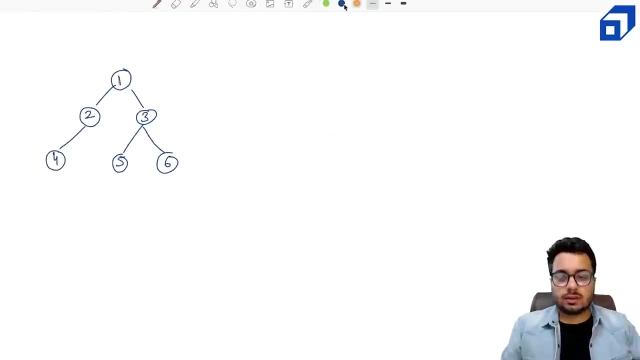 Null Right And Output That You Will Get Right. So I Hope You Have Understood The Inorder Traversal. Now Make A Bigger Tree And 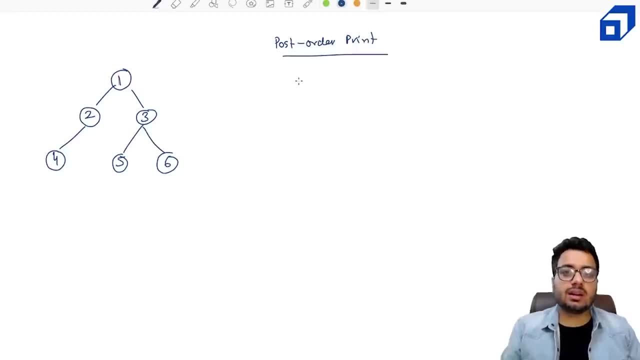 Try To Generate The Output For That Particular. Then We Print The Right Subtree, Recursively Of Course, And After Then We Print The Route. 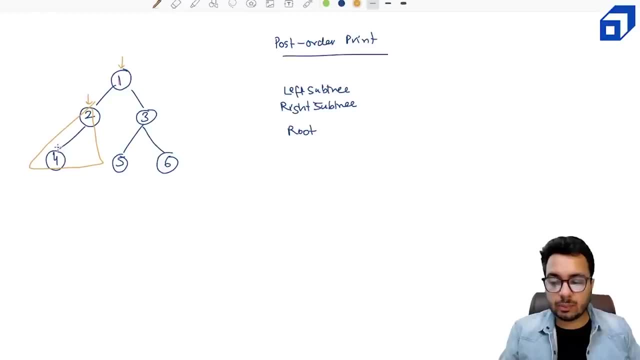 If This Is The Tree Once Again, What I Will Do. I Start With Then At One. I Have To Print Left, Which Is Done. I. 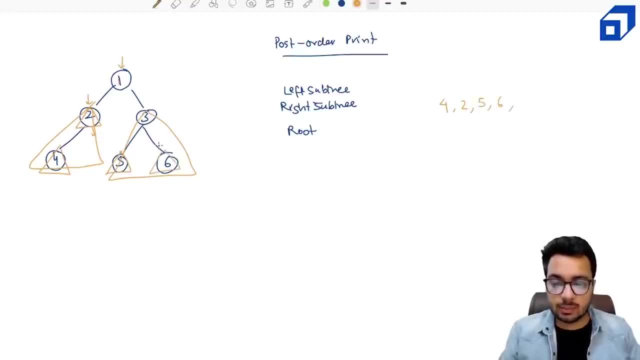 Have To Print Right Subtree And Then I Will Print Two, Three. I Will, Okay, Print Left Subtree. Now Let's Take A Look At 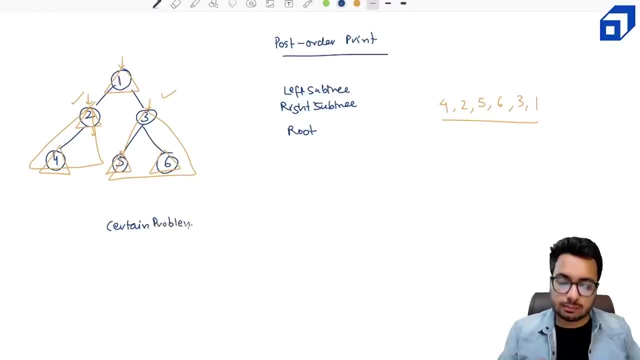 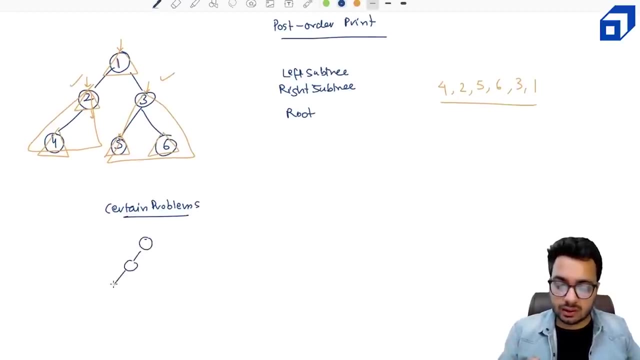 The Tree And The Output From The Left And Right Subtree, For Example, I Want To Calculate What Is The Height Of The Left Subtree. 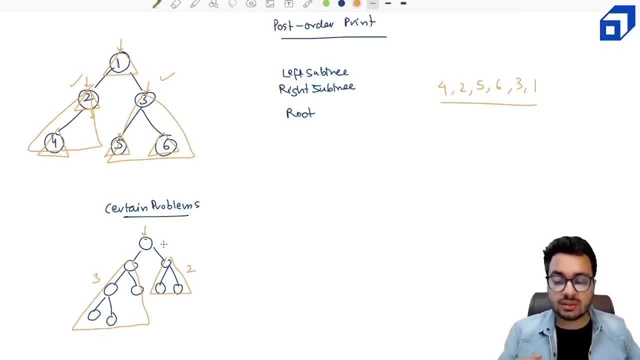 Let's Say This Height Is Three. What Is The Height Of The Right Subtree? This Height Is Two. And Can You Say Recursively At: 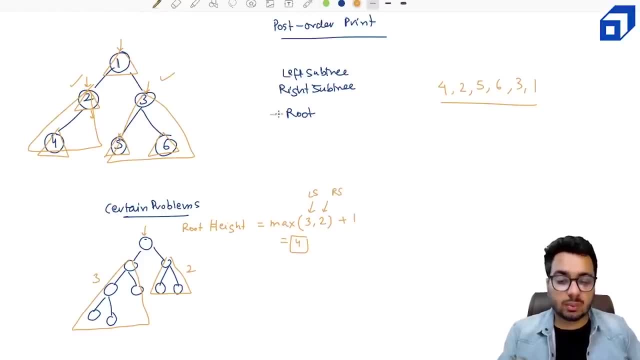 This Route To Claim Is In Order To Build The Answer At The Route Node. You Need The Answer For The Left Subtree And Right. 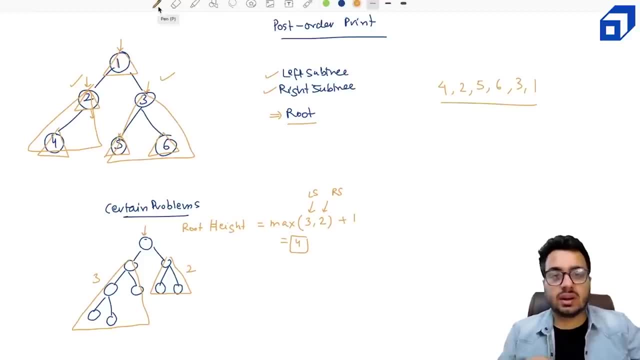 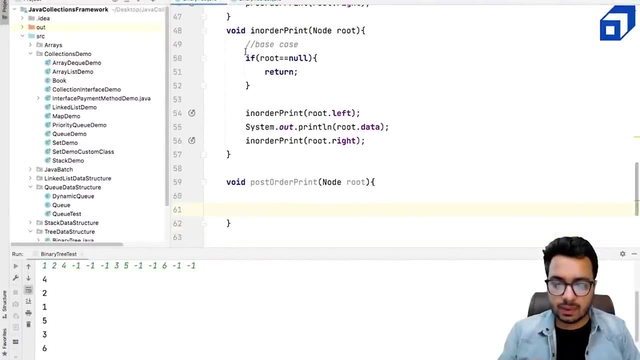 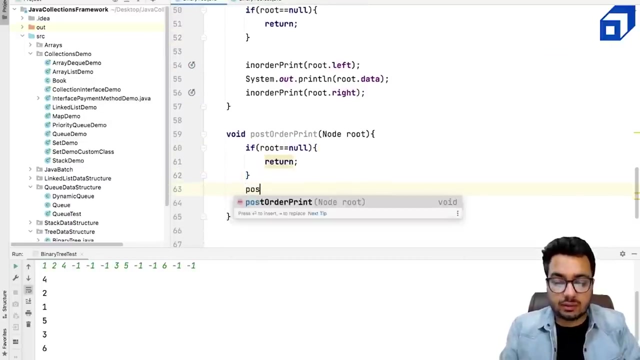 Subtree And Hence In Problems Like Code Is Very Easy, So I Am In The In This Class. If Route Is Null, I Will Return. 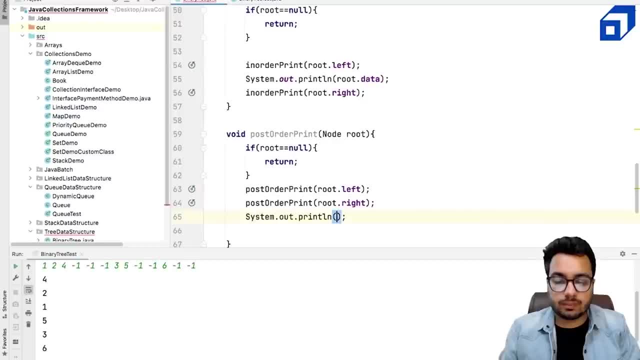 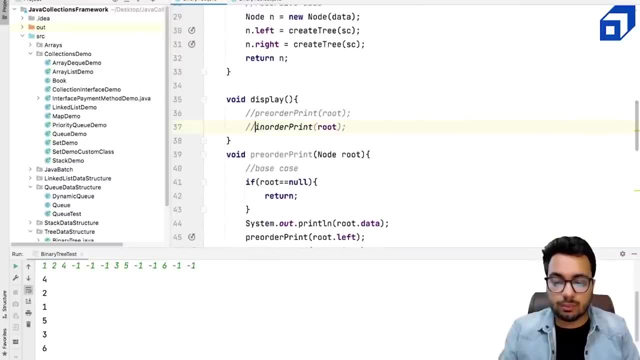 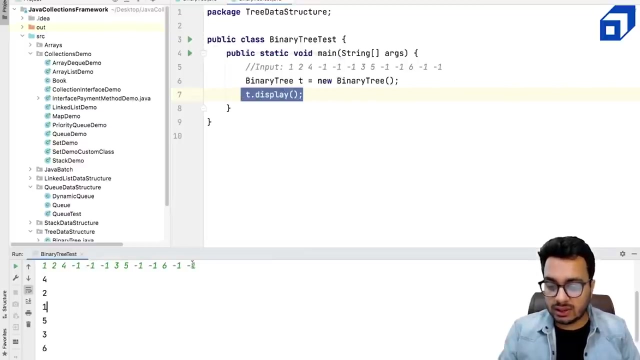 Then What I Will Do. I Will Go On The Call Post Order Print In Our Display Method, So I Can Just Pass The Route Here. 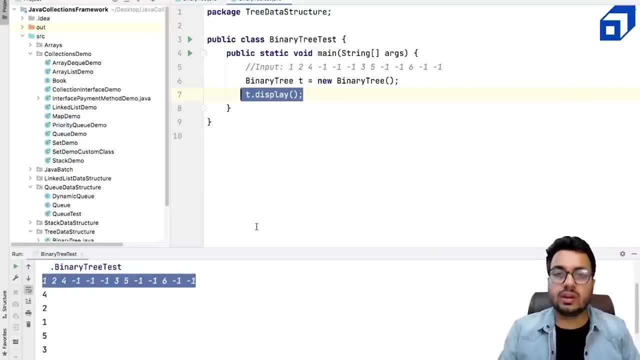 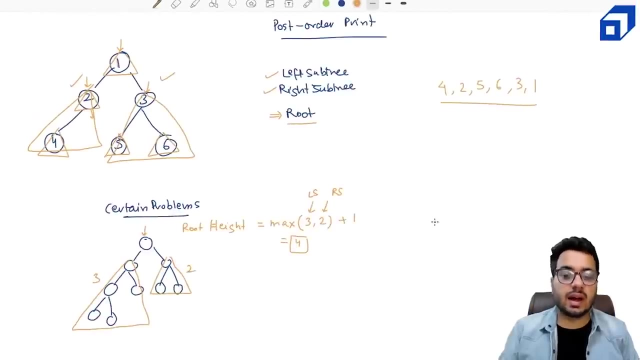 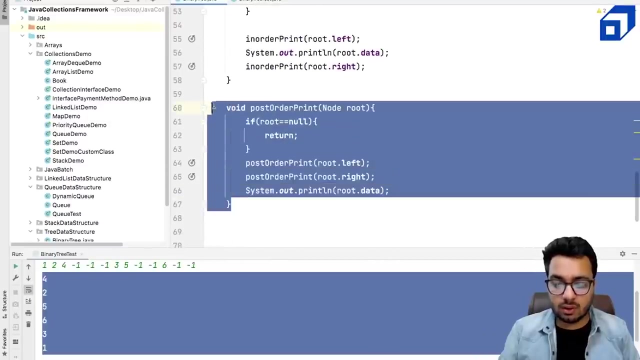 To T Dot Display. It's Calling The Post Order Print Method For The Route. As We Have Got Four, Two, Five, Six, Three, One Absolutely. 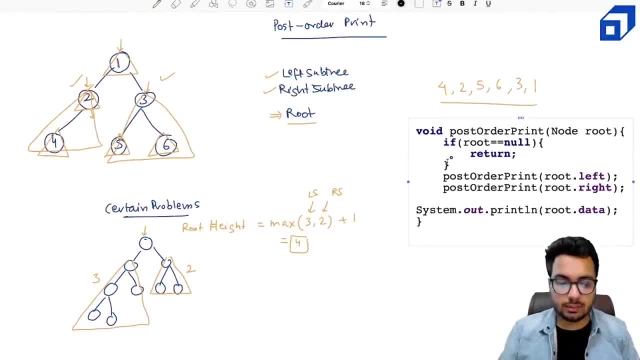 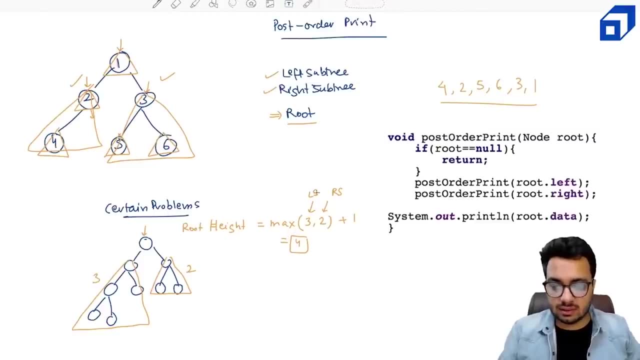 Yes, Let Us Do A Quick Call Stack Analysis Of This Method As Well. I'll Copy The Code And, As My Route, Note The Route. 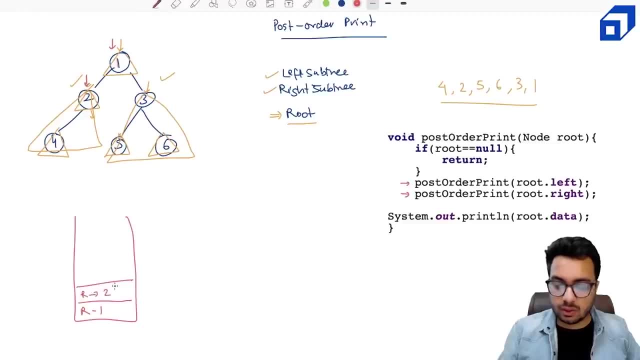 Is One, Nice, Okay, Make A Call On The Left. My Route Is Two. I Make A Call Here. Code Is Post. I Will Print Route. 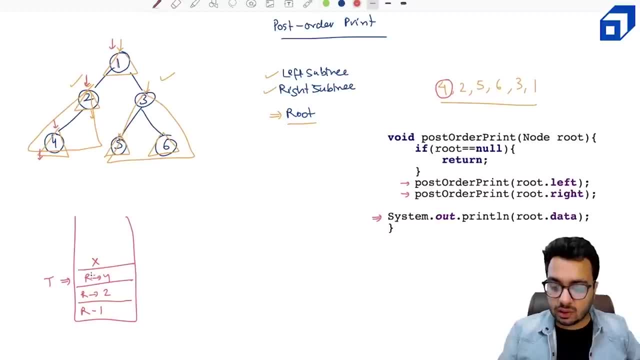 Dot Data. This Is The Top Of My Stack. I Will Print Four. Then If Four Is Gone From The Stack, What Is The New Print? 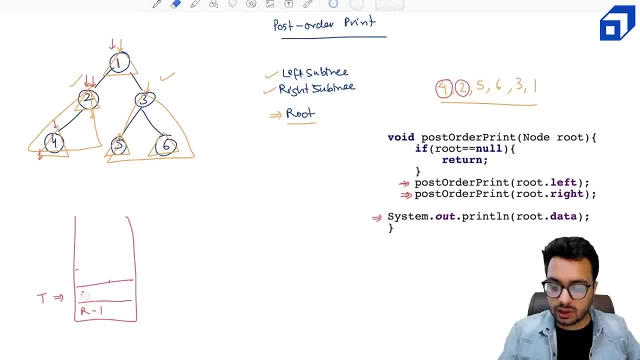 To A. Two Is Also Gone, We Are Done. One Is At The Top Of The Stack Now. At One I Said: Okay, Go, Left Which? 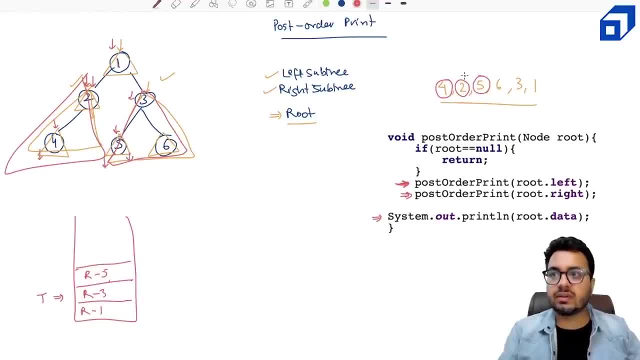 Is Already To Print Five, So You Will Get Five As The Next Output. Now, Once Five Is Gone, Your Bag Again At Three, He Says. 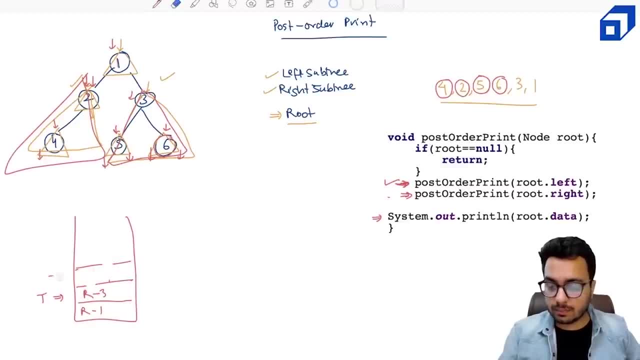 Okay, My Left Is Done, Right Is Done. I Will Print Root Data, So I Will Print. Three Is Also Gone From The Stack And Now. 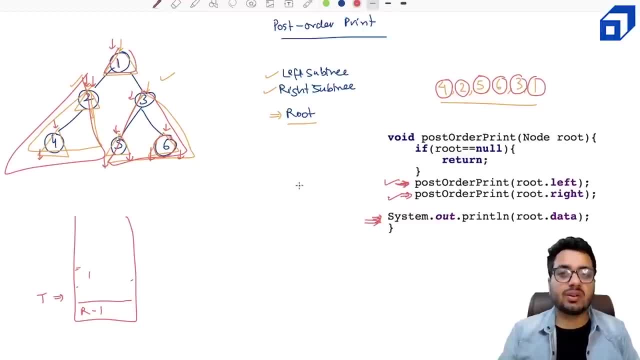 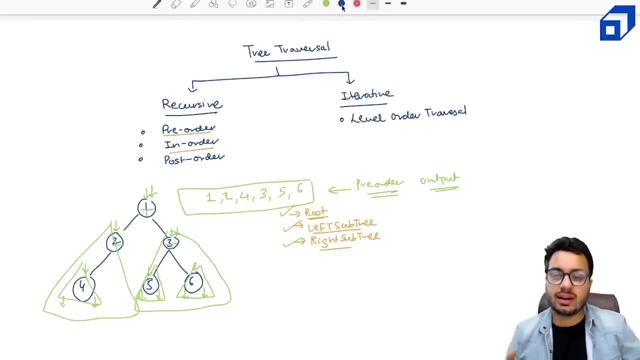 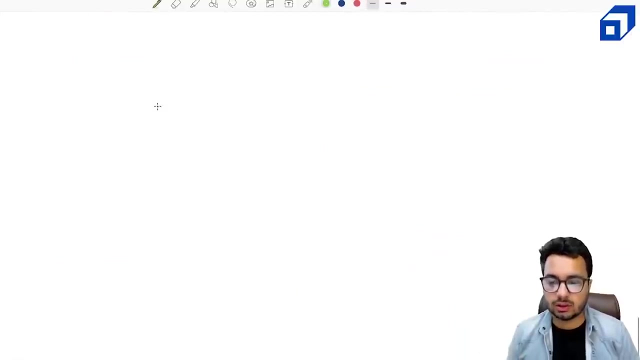 Top Is At One, So For One Left Is Done. Now Let Us Jump Into The Iterative Traversal, Which Is Also Known As Level Order. 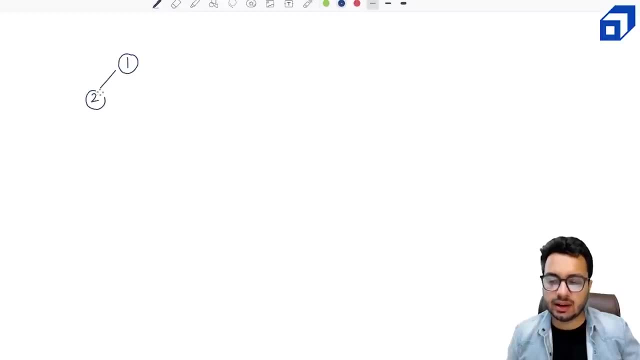 Traversal. Okay, So That Means We Won't Be Using Recursion. We Would Be Using Then We Are Going Here To All These Traversals. 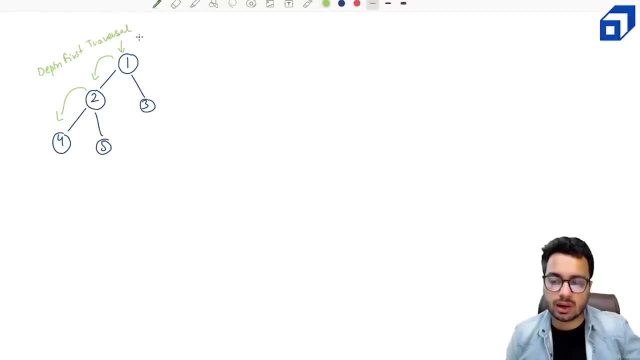 They Are Depth First Traversals. That Means You First Go Deeper Into The Tree And Then That's How You I Think Of Each Level. 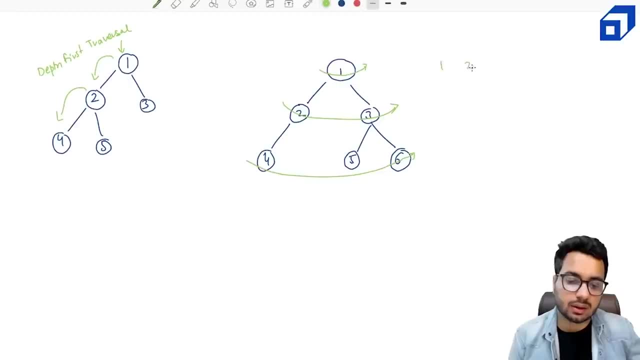 This Level, This Level, This Level Right. That Means I Can Expect An Output That Is One, Two, Three And Four, Five, Six, Right The Level. 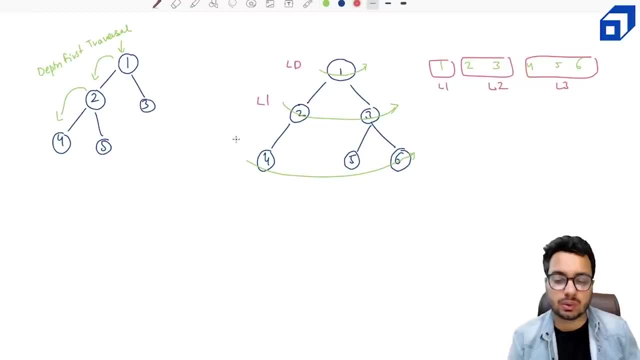 Zero, Level One. All The Nodes Are Distance One From The Root. Note: This Is Also Known As Bread First Reversal. Right Now, Let Us 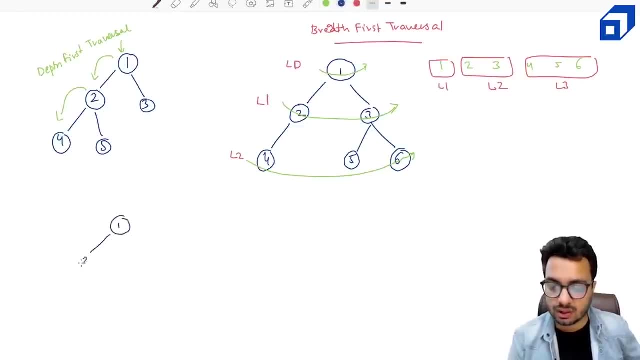 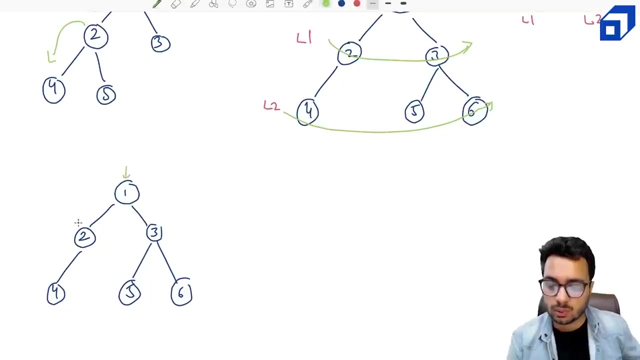 See How We Do This Tree Once Again. Now, If You Look Carefully, If You Start Doing Any Reversal, That Is A Recursive Reversal. 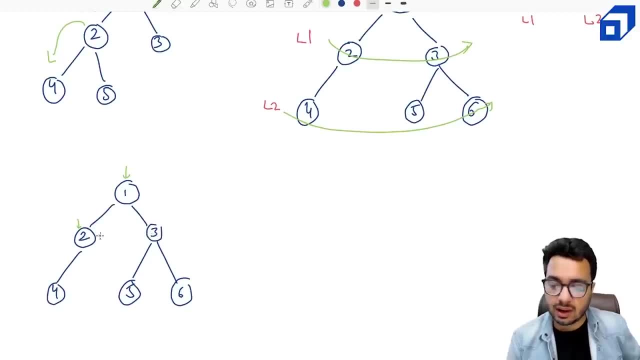 Right From One You Come To Do Right. We Cannot Go Back And Forth. Right. How This Is Achieved. This Is Achieved By Using 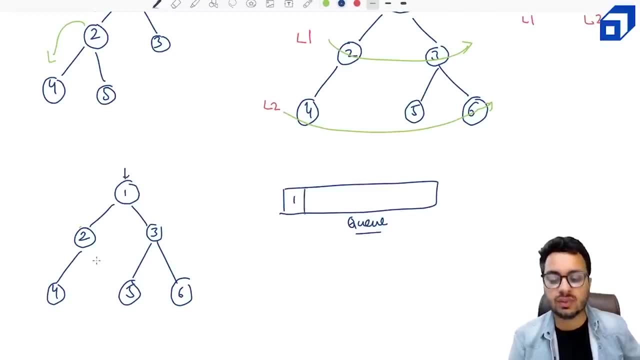 A Concept Of A Q Data Structure. Okay, What We Will Do, We Do And I Will Push The Children Of This Node Into The Cube. 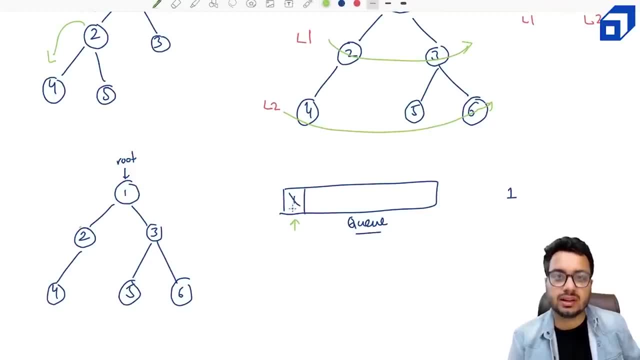 So I Will Print It. Output Will Be One. This Is Popped. And What Are The Children? So You Know, The Children Are Root Dot. 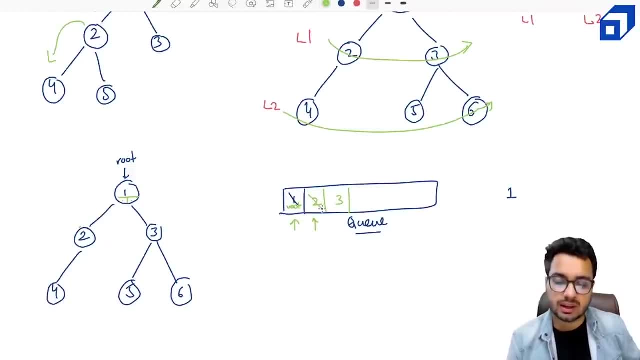 Left Root Dot Right. I Will Push The Reference Of Two And Three In The Cube Right. Next I Will Print It. Okay, One Is Done. 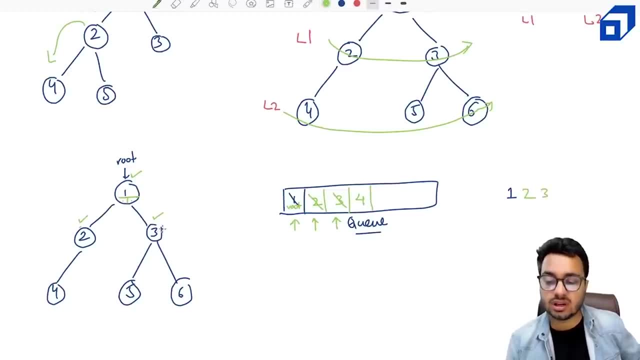 Two Is Done. The Next Node Is Coming Is Three. Right, I Will Pop It, I Will Print It And I Will Push Seven, Eight And 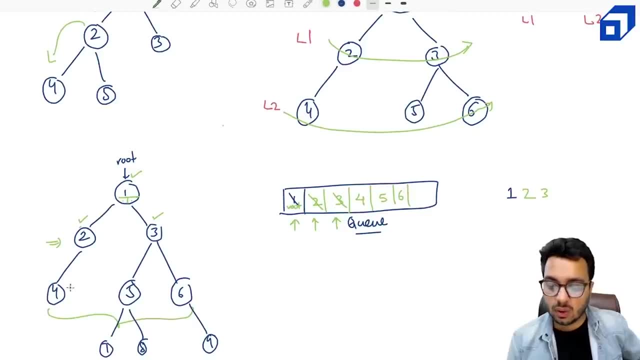 Nine, Right, So Let Us Just Extend This Example A Little Bit. Now. I Will Pop Four, I Will Print Four. This Will Be Removed. Four: 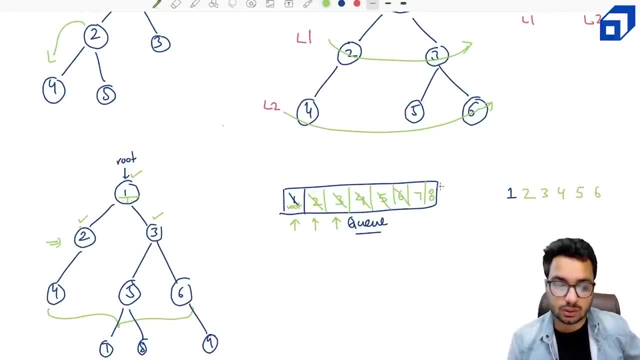 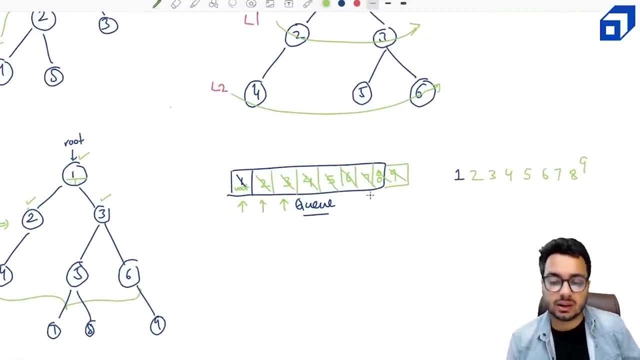 Does, And I Will Push The Children Of Six Into The Queue. So Nine Will Get Into The Queue. Next I Will Pop Seven. I Will. 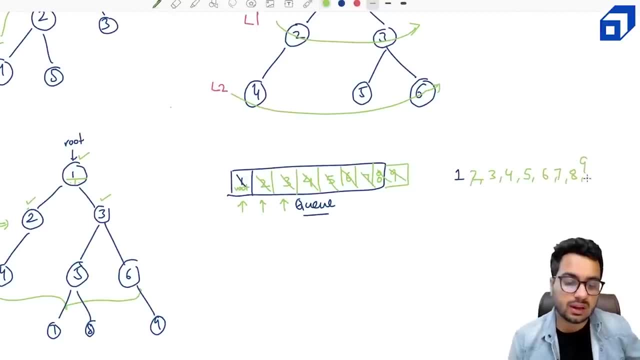 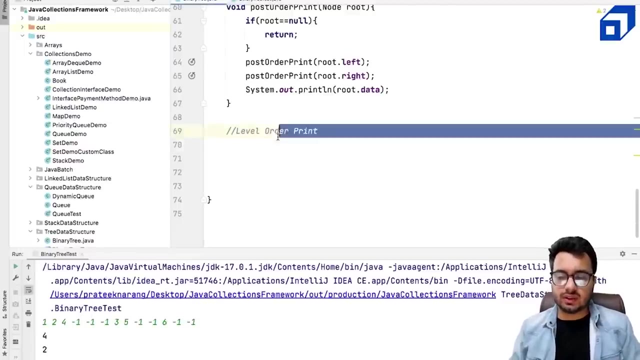 Print Seven And No Ordered Reversal. I Hope You Are Convinced That This Is The Correct Output For This Tree. Let Us Look At. 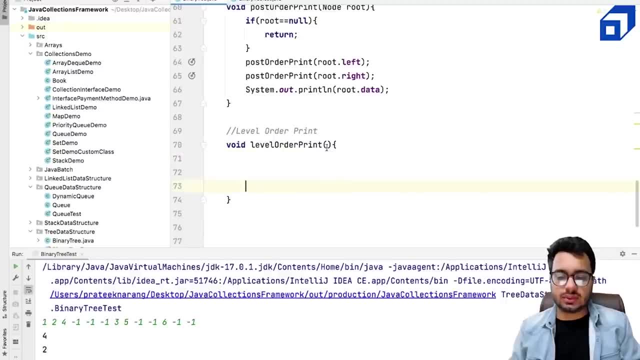 This Implementation In Our Code As Well. Let Us Look At The Queue Of Node, Called Queue. This Is Equal To New Linkless In Java. 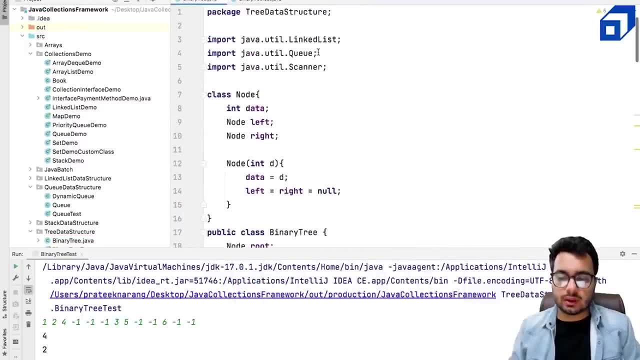 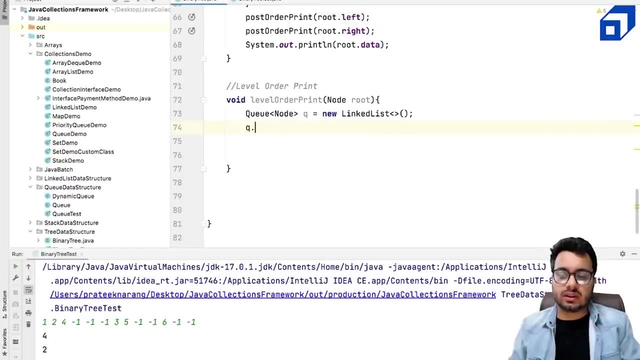 Queue Is A Interface And Linkless Is A Class That Implements The Methods. Offer, That Is Your Add Operation Right And I Can Offer Root. 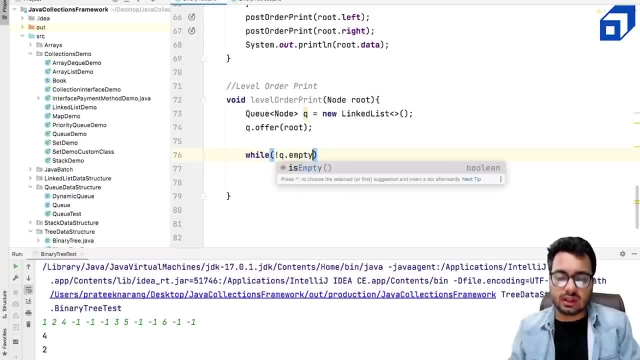 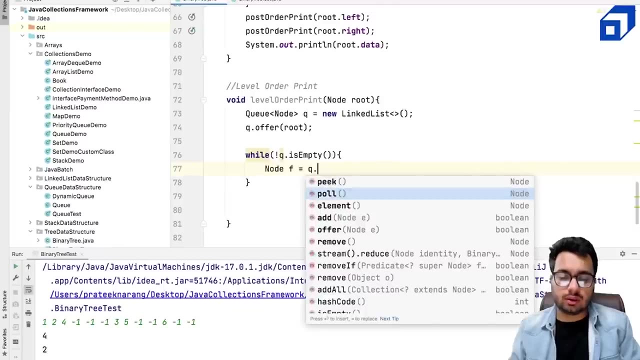 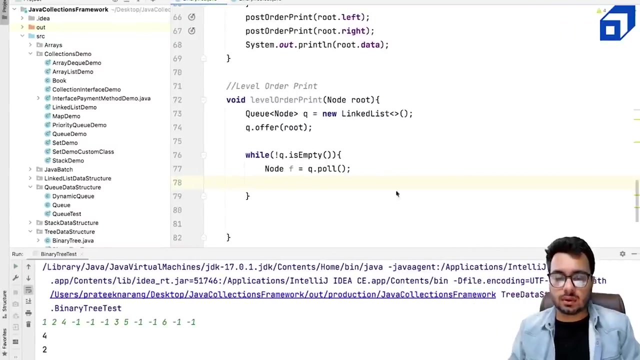 Inside The Queue. That Means I Can Add Queue Right. I Said You Will Do Some Work, All Right, So This Removes The First Note. Like 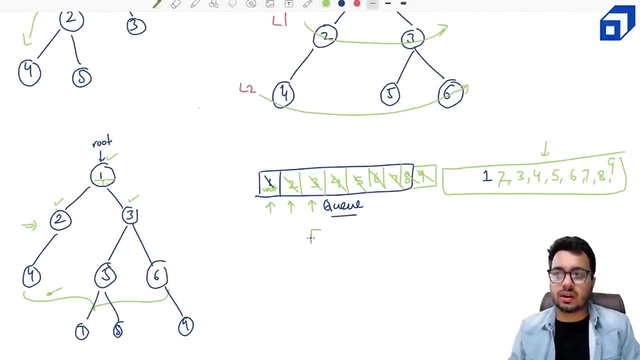 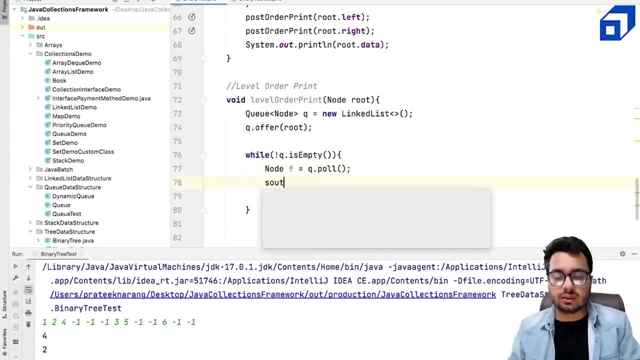 We Have Seen In The Diagram, We Are Always Removing The Node At The Front Of The Queue, Right. So F? Left Is Not Null I. 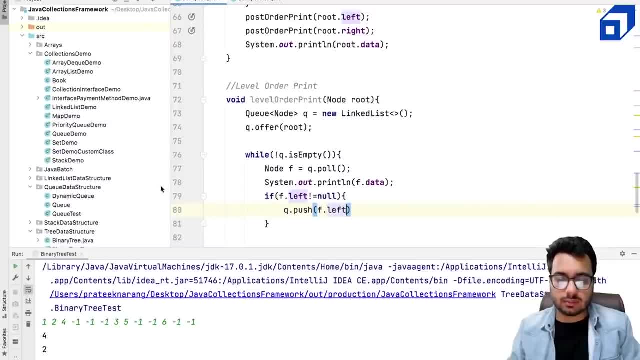 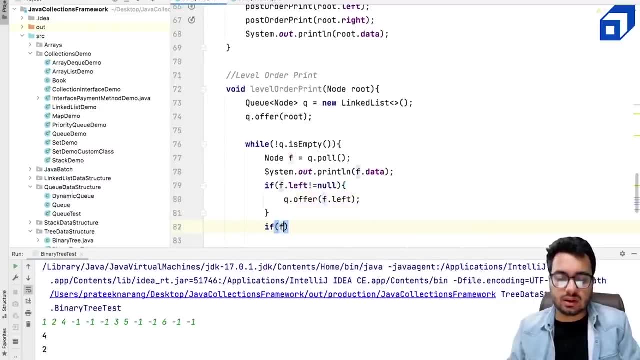 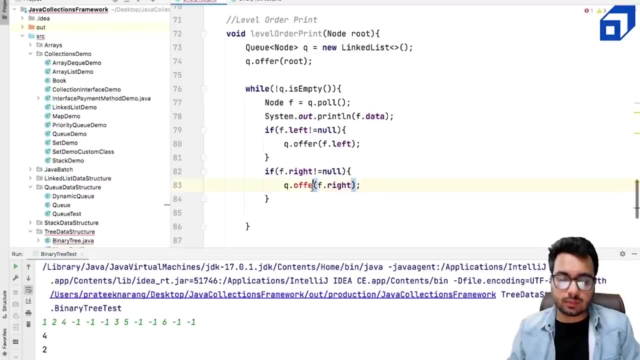 Will Say Queue, Push F Dot For The Queue, Offer F Dot Left, And If The Right Child Is Not Null Or If Is Filled, 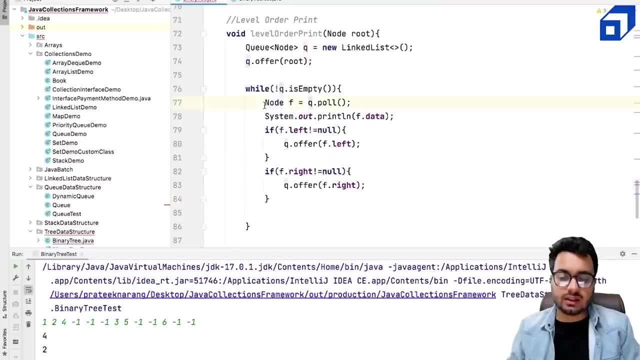 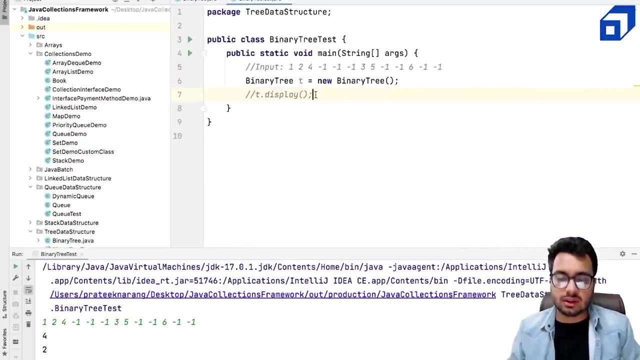 Using These If Conditions And It Is Getting Empty From The Front, Using This Whole Operation, Right, That's All, That Is The Code, And Now. 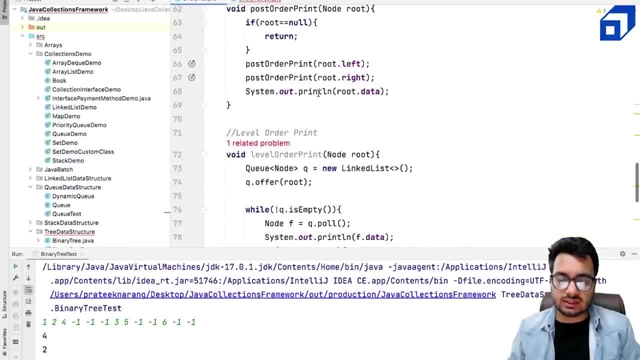 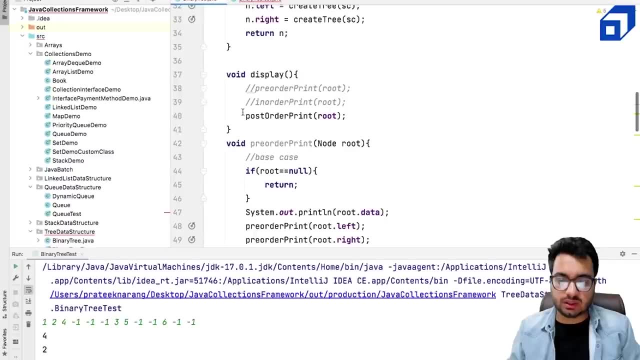 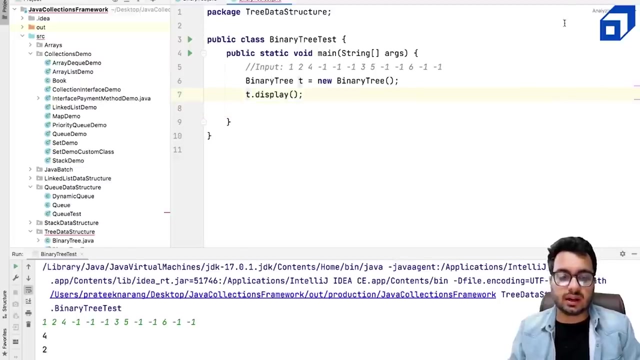 I Can, I Don't Want To Access It Outside, So If I'll Just Call It From The Display Method, Because We Are Testing The Functionality, 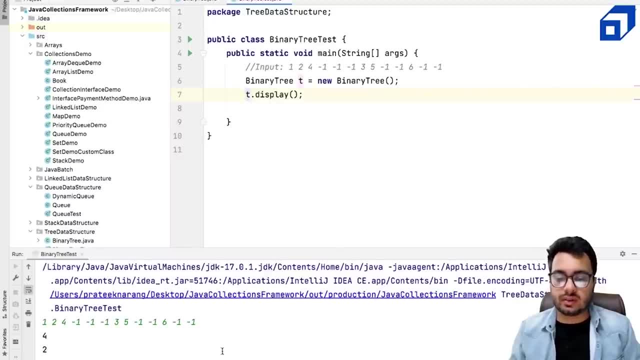 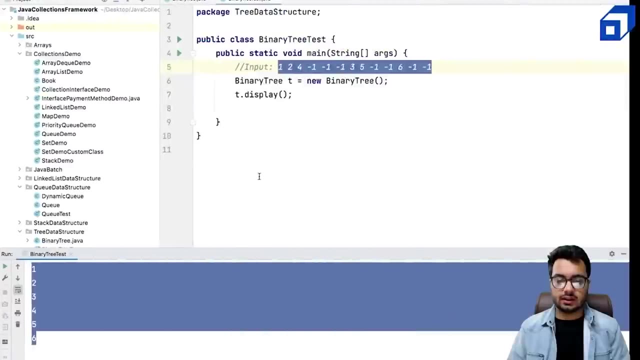 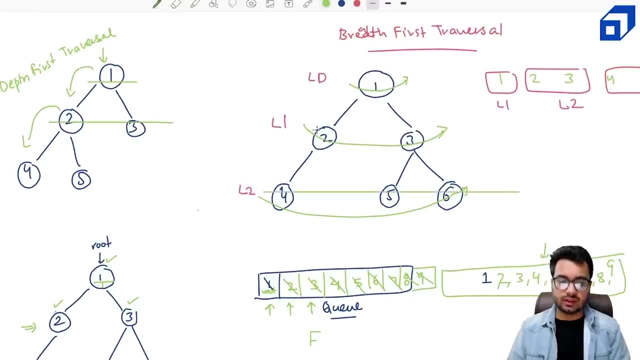 So I Can Say: Level Order Print. What Output Do We Get For The Given Tree? I'm Getting One, Two, Three, Four, Five, Six. Which? 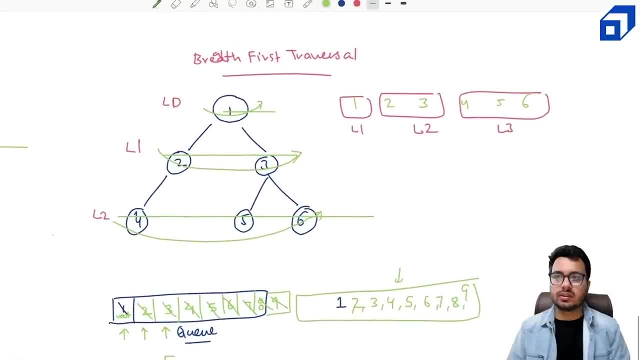 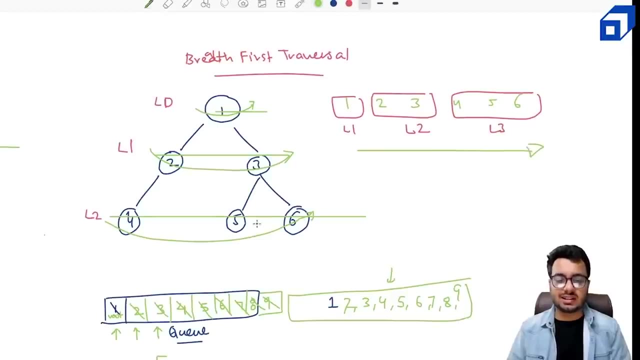 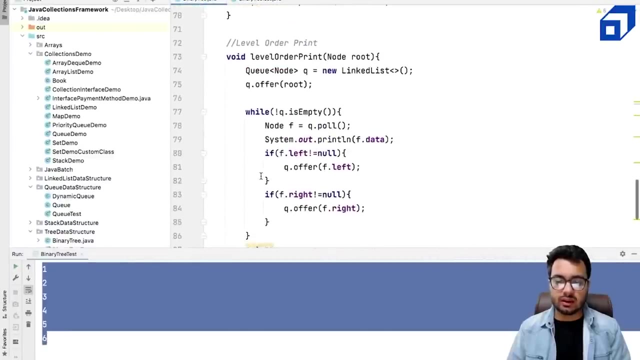 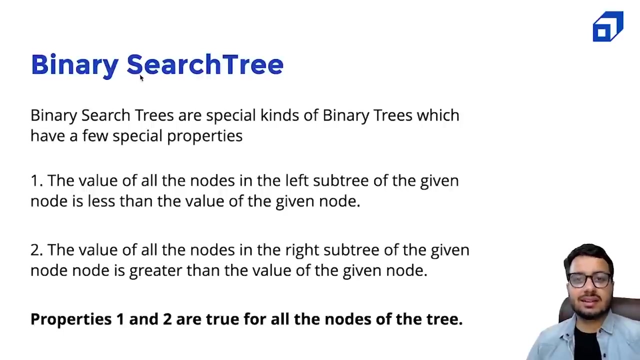 Is Correct And If You Look Carefully Here For This Tree, I'm Going To The Data Sector. The Code Is Very Simple And You Can. 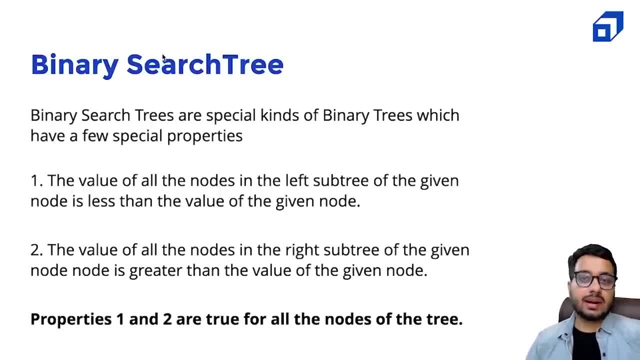 Also Do A Dry Run Of This Code At Your Own. Let Us Start Discussing Binary, That Is, By The Name Called Binary Search Tree. 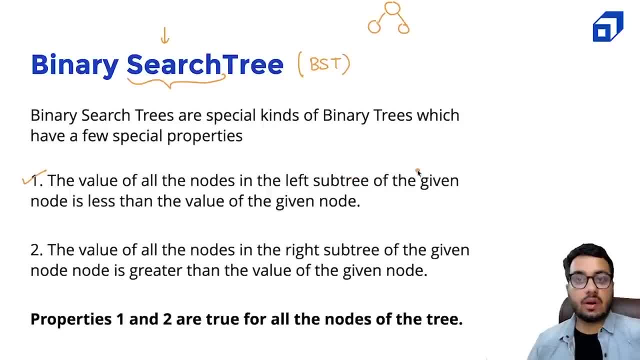 In Short, We Also Call It As BST. BST Is A Special Kind Of Binary Tree With The Following Properties: The Nodes Which Are In The 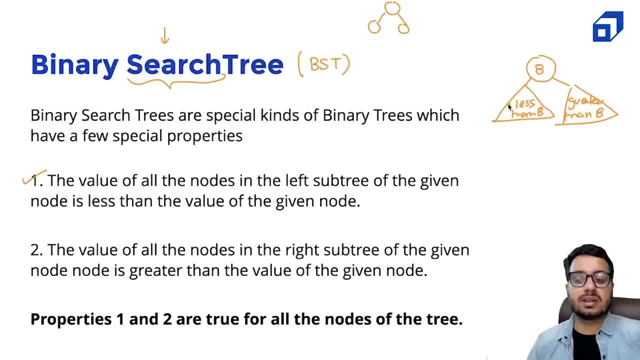 Right, They Must Be Greater Than It. This Is The BST Property Right Now. How This Makes Searching Easy For Example. You Are See An Example. 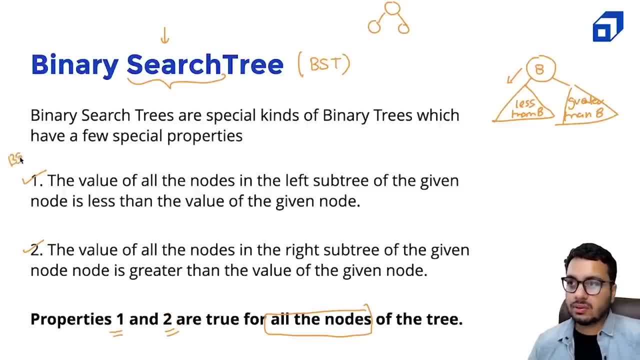 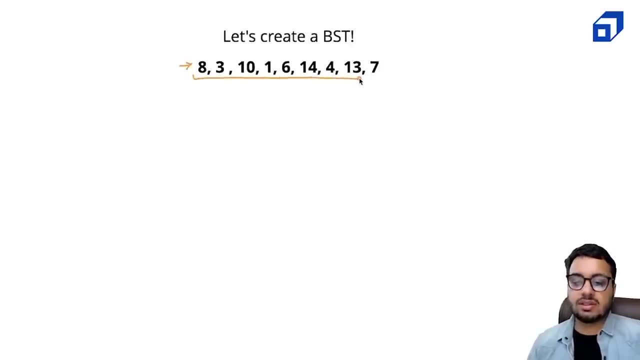 How Do We Construct Such A Tree Where Every Node Follows The BST Property? So This Call, This We Call As BST Property, Right Or? 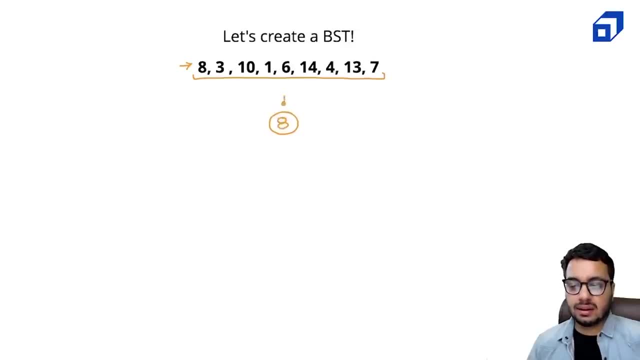 The Will Be The Root Node, Because My Tree Is Currently Null, So It Becomes The Root Right Now. Next Element That I'm Getting Is: 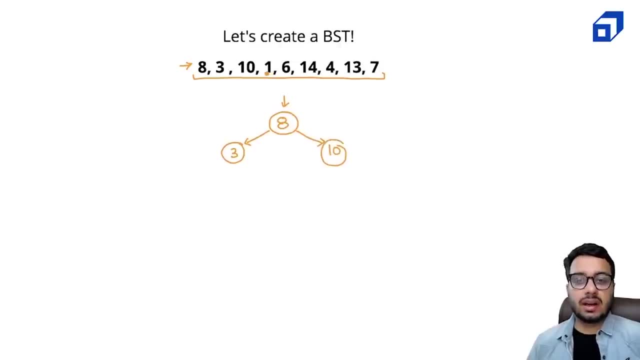 Three, Now Three I Know. So I Will Start From The Root Node. The One Is Less Than It. I Will Go Left. One Is Less. 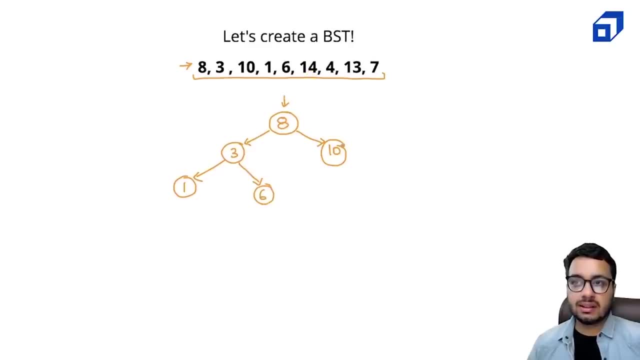 Than Three, So I Will Insert One Here. Then I Have Four. Four Is Less Than Eight. I Go Here. It Is Greater Than Three. I 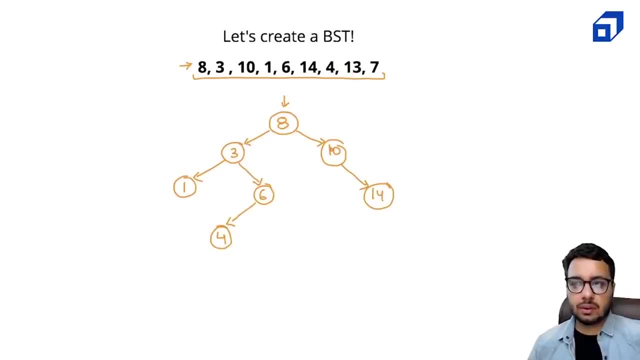 Go Here, But It Is Now Less Than Six, So I Finally I Have Seven, So Seven If I Start With Respect To Root Node, Less. 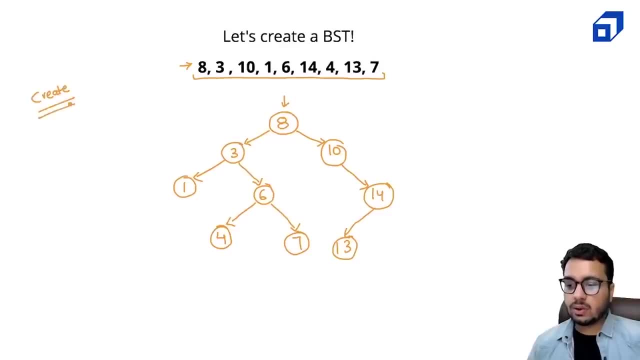 Than Eight, Go Here. Greater Than Three, Go Here. Greater Than Six, Go Here Three. Now Suppose, If This Tree Height Is H, And I Want. 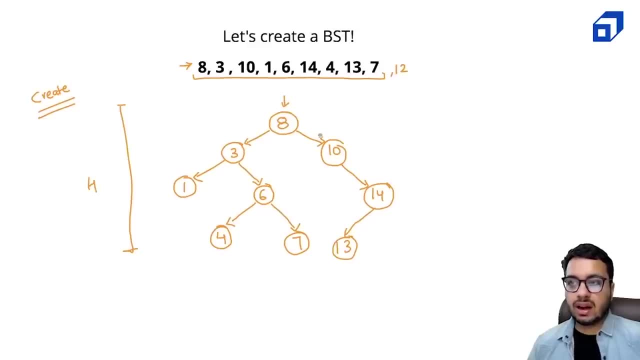 To Insert A Node. In The Worst Case, I Have To Travel One Branch, For Example. If This Is, How Well Will Be Inserted In. 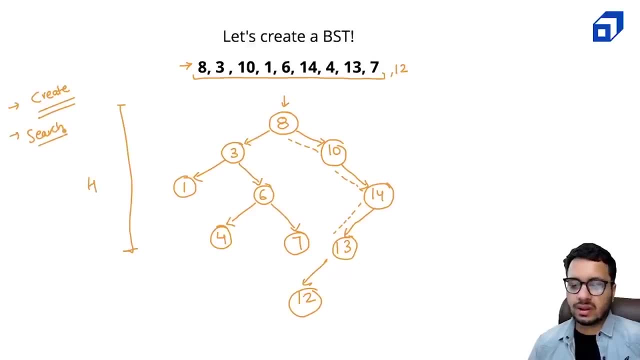 The Tree. Right Now, Let Us Talk About Searching. Okay, How Do I Search For A Given Now? For Example, I At Three If Seven Is. 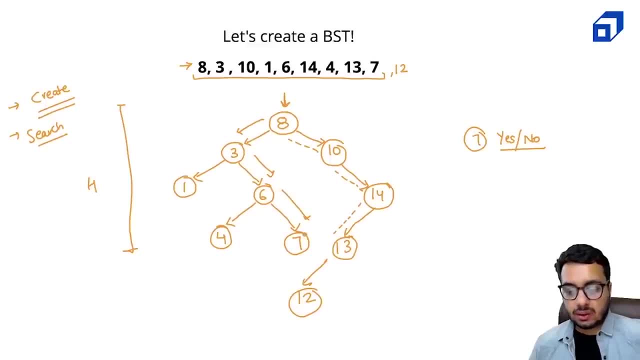 Present, It Must Be On The Right. So I Go Here At Six. If Seven Is Present, It Must Be On The Right. So One, Two. 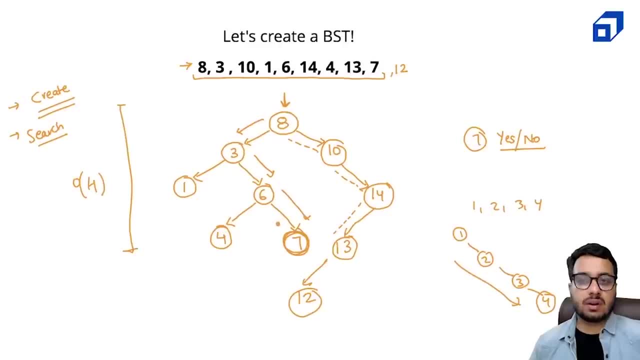 Three, Four Right. A Height Can Become An Also, So That Is Why I'm Not Seeing Order Of N, Or I'm Not Seeing Order Of. 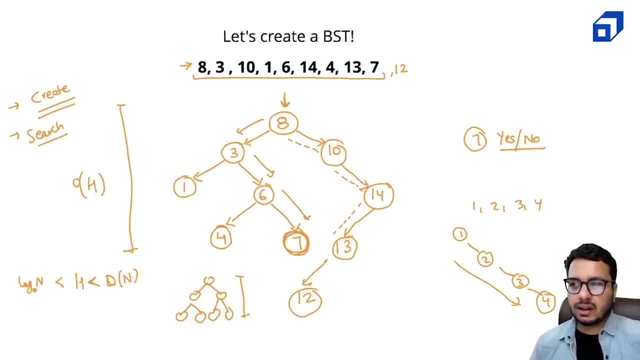 Login Right. So Height Will Be Greater Than Login, Greater Than Equal To Login, And It Will Be Less Than Equal To N. So Height Lies. 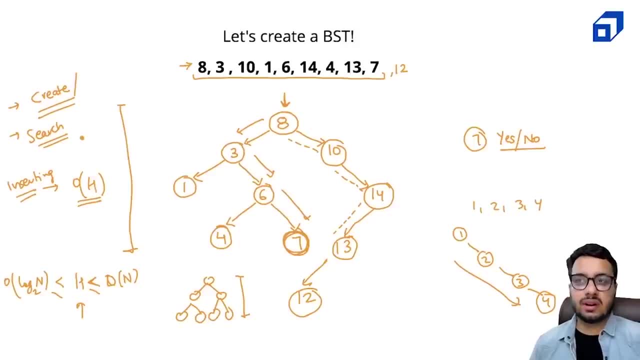 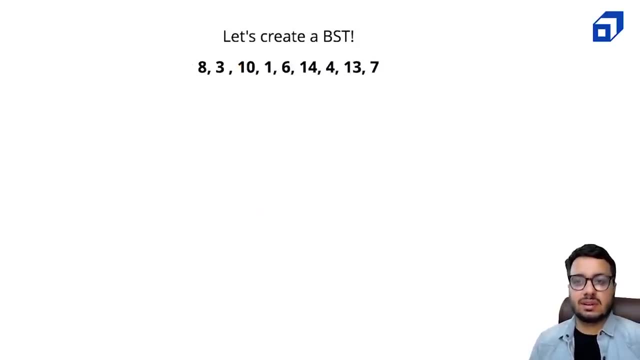 In This Range Right. So We Have Found The Fundamental Concept Behind Binary Search Tree, And Now Let Us Dive Into The Implementation Of It. Let 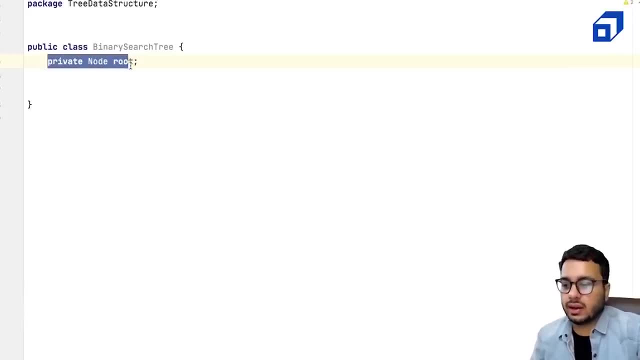 Us Start By Building A Binary Tree. Binary Start By Creating A Tree. Right, I Can Do. Okay, There Is A Binary Search Tree Contractor And 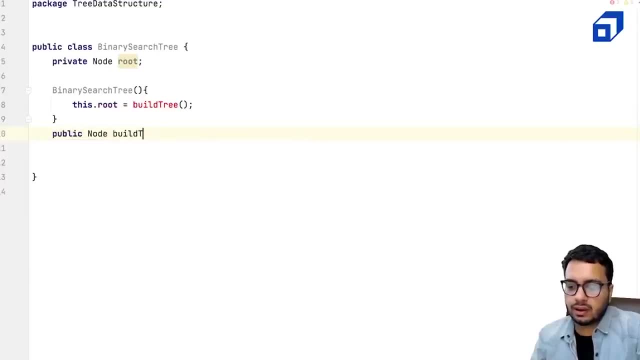 In This Case, I Can Do This Dot Root. This Is The Example That We Took. We Said: Okay, We Will Take These Notes And We 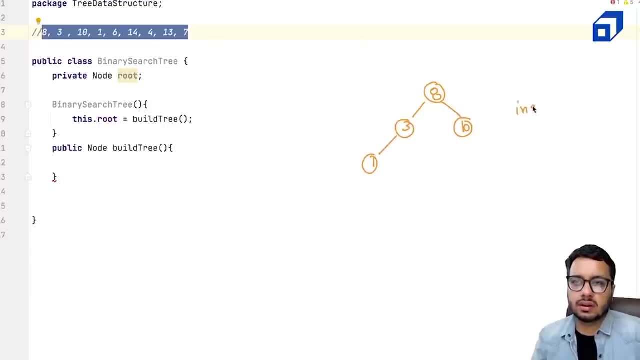 Will Insert Them Into The Tree One By One. So We Will Also Build It Minus One Right. So This Is One Way, Or You. 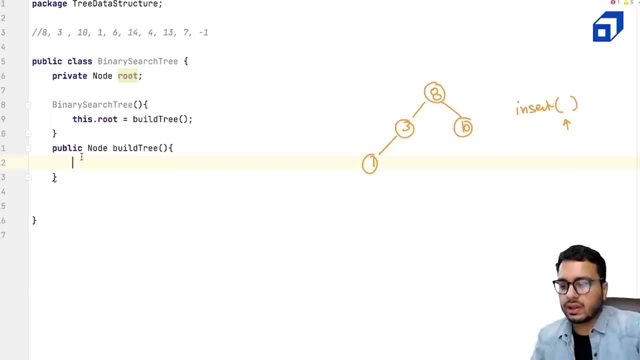 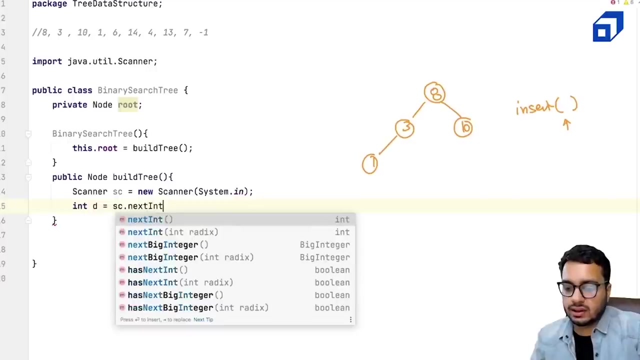 Can Ask How Many Notes You Want To Insert, And Then You Can Read And Numbers, Both Are, And Now I'm Going To Read Data. 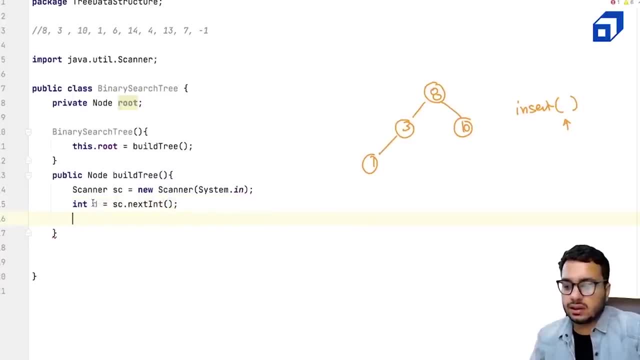 Right. So I Can Say: In Data This Is Equal To Next Int, While This Data Is Not Minus One. What I Need To Write? 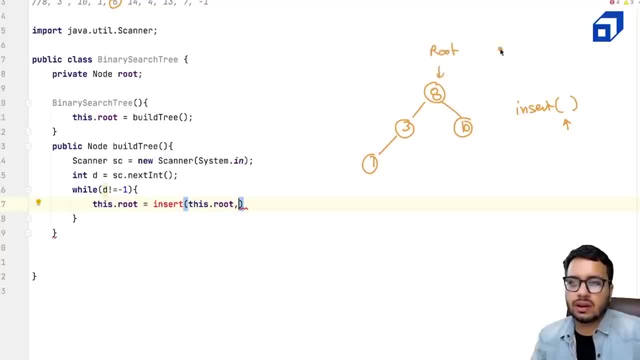 In Data, So I Can Write Data In Data. So I Can Write In Data To My Data. So I Can Write In Data In Data. 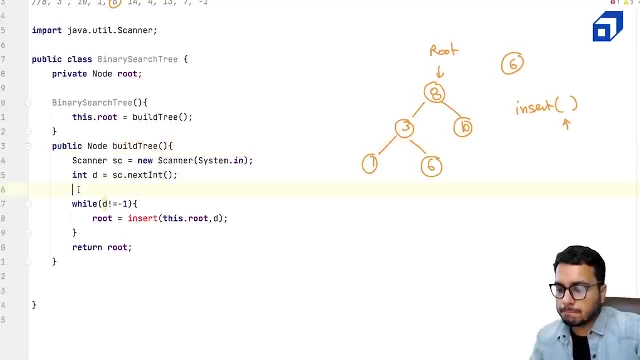 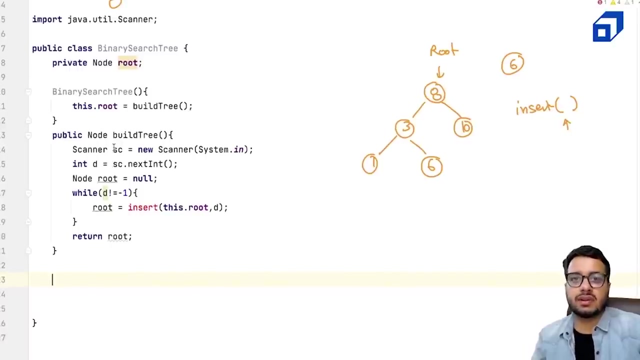 You Can Do It Like This As Well: Node Route Which Is Initially None. You Can Say It Like This As Well: I'm Finally Returning. 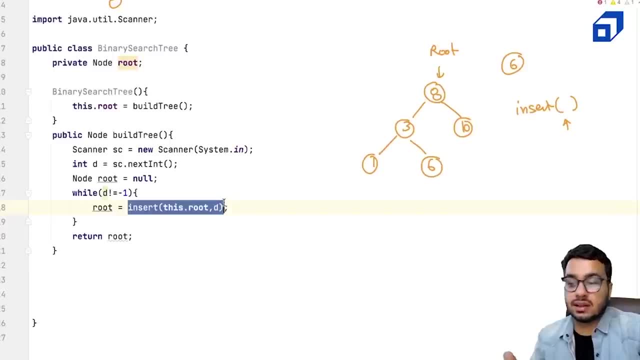 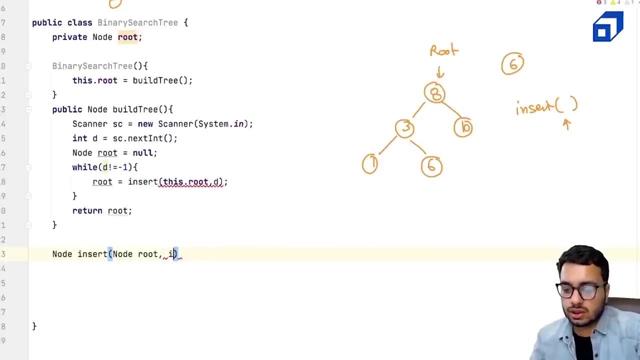 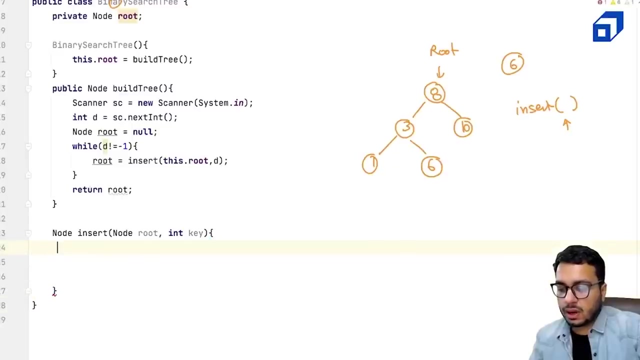 The Route Note. Which Is It? I Want To Say, Okay, Node Insert, I'm Going To Get Route Note Now. This Route Note Is In. 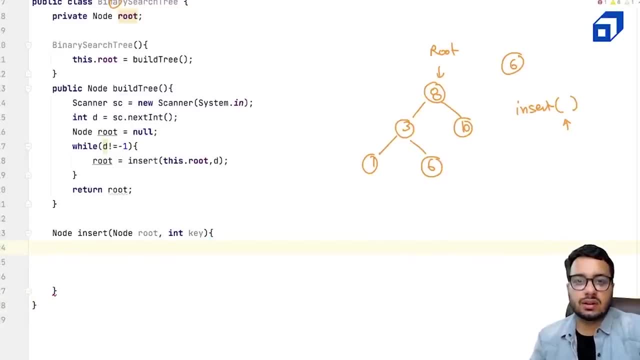 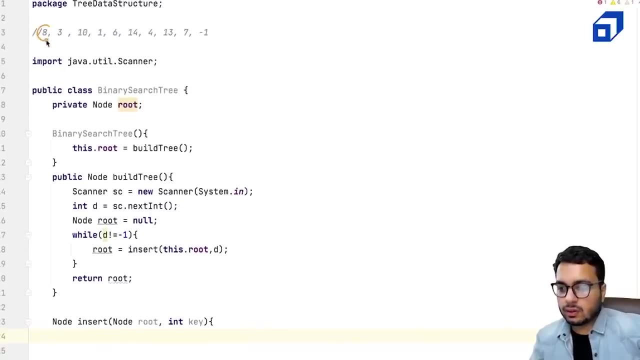 The Beginning. It Is This Route Note. But To Happen In The Starting, In The Starting You're Going To Insert It Route Is Null. So 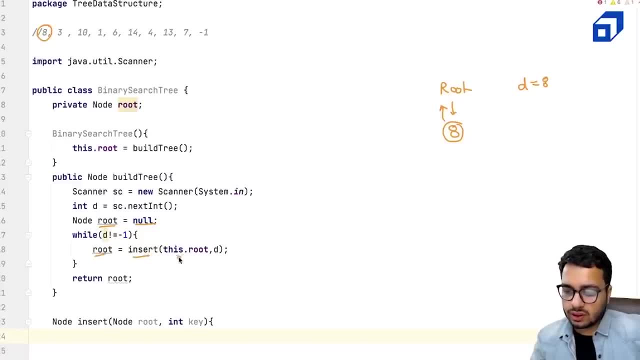 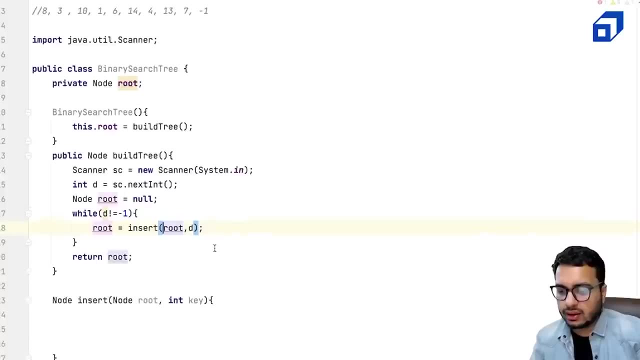 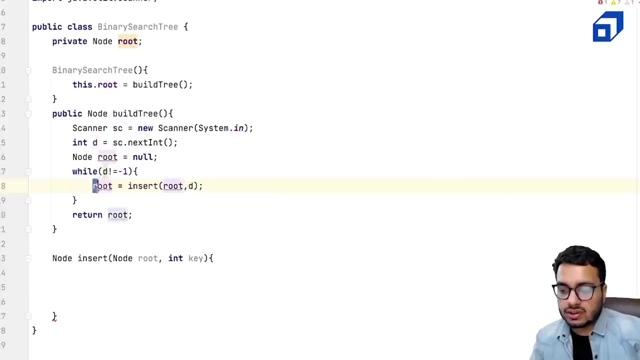 Here, The Route Is Null And The Data That You're Getting Is The Data Right. So What Is Going To Happen? You're Going To. 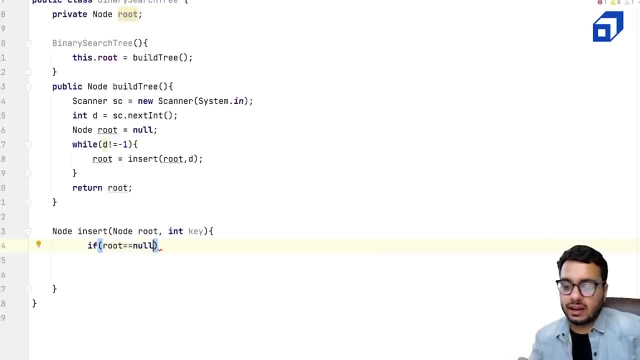 Say, Fine, I'm Inserting. I'm Inserting Something Into A Null Tree So You Can Say If Route To Create The Actual Route, Node Of 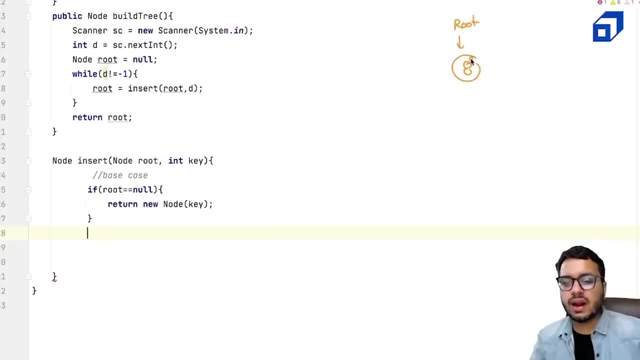 The Tree Right. But If This Is Not True, For Example, I've Inserted It. Now The Route Is Pointing Here Right, And Suppose I 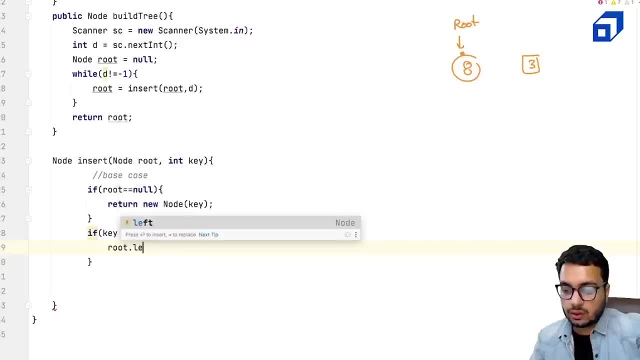 Should Go And Insert In The Left Subtree, Right, So I Can. So Okay, Route Left Now This Will Point. This Will Point To A. 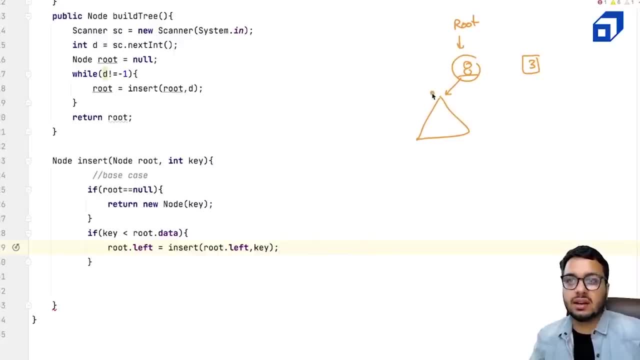 New Subtree In The Left Subtree Of It. So If You Hit This, What Will Happen? Your Route Will Come Here Again. You Will. 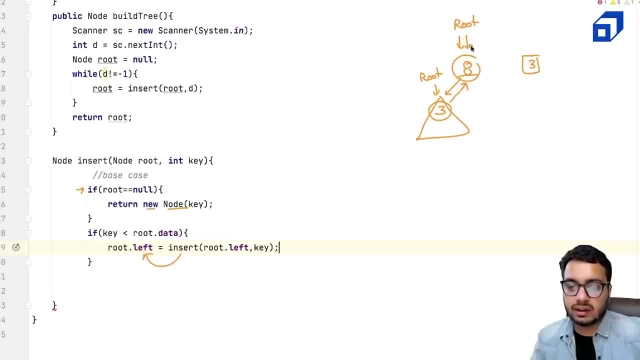 Observe That Route Is Null, So You Will Hit The Right Subtree. Okay, Let Me Finish The Code. I Will Do A Complete Dry Run. 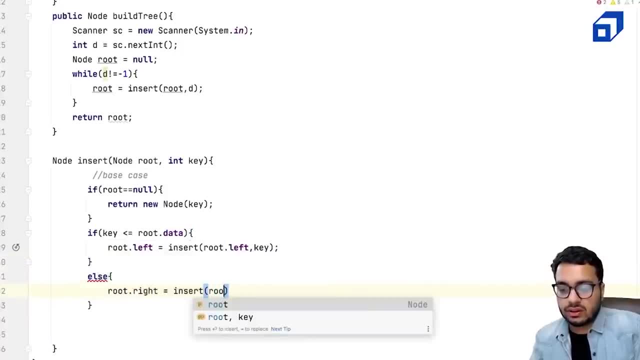 Okay, And The Complementary Case: Okay. We Can Make It Less Than The Route, Right, Okay. And Once It Is Done, What I Have To? 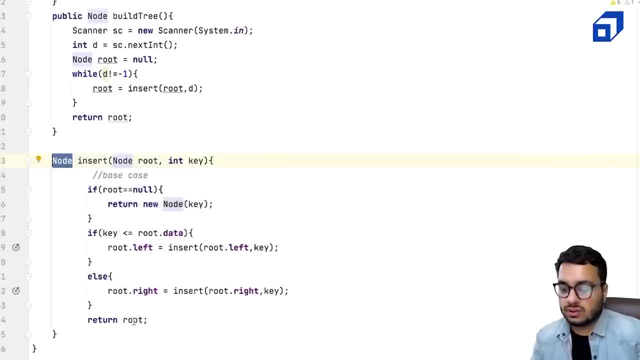 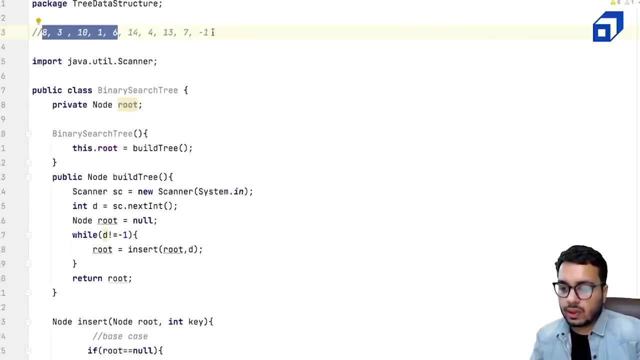 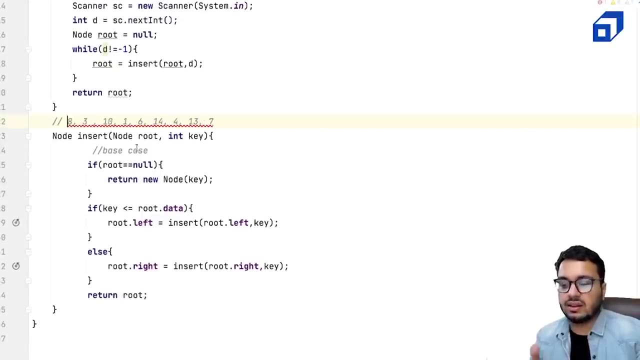 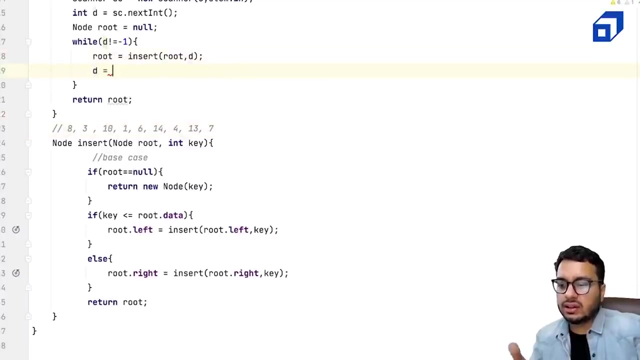 Say, Have To Say Return. Now, This Is Important Because Every Function Is Expecting That. Address This Example And I Will Dry Run This Function. 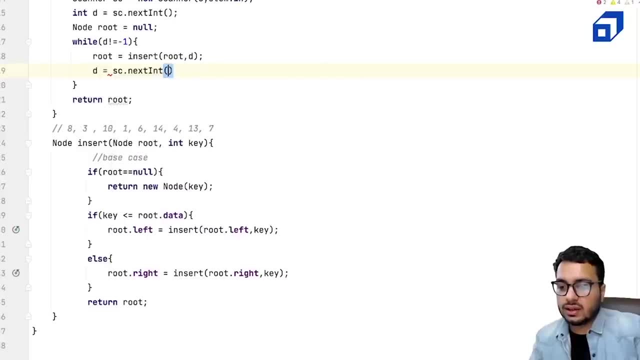 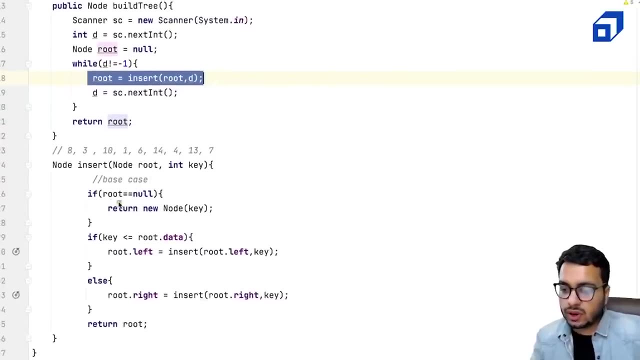 What Is Happening? Okay, I Think I Missed Out One Thing Here. I Will Have To Read The Data Again. New Note Of Key. So 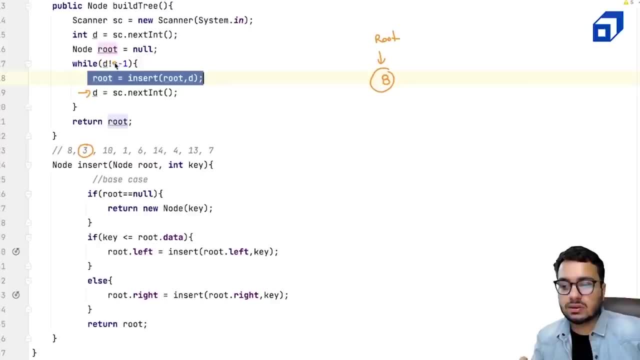 Insert Call Is Over. Next Time I'm Reading This Number Three: Using This Line Data Is Equal To Scanner Dot Extent Data Is Not Right. 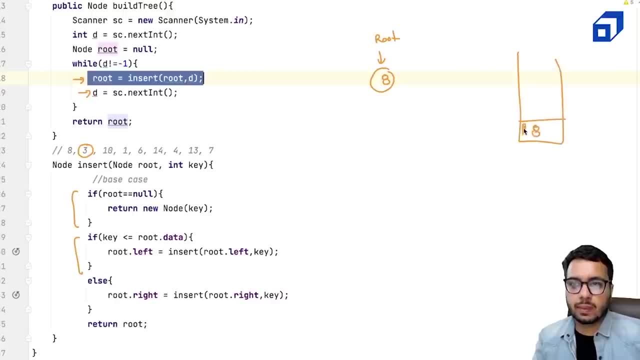 So I Will Draw This Call Stack As Well. So I Have Eight. So It Makes A Call On The Left. Left Is Null You Hit. 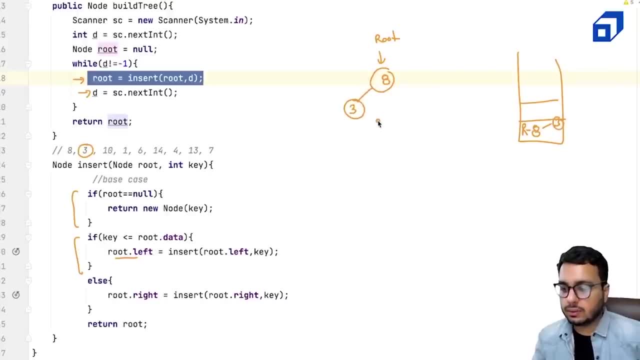 The Base Getting Connected Right. This Is Over. And Now From This Function, Call You Return Root, You Return Root, So You Basically Return The Address. 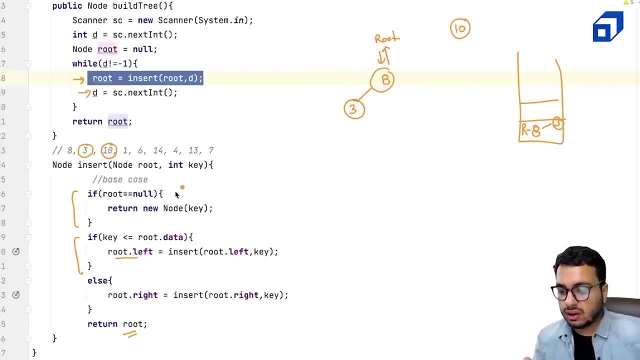 Of Eight Back Into The Root. So You Come Into The Else Block. You Say Root Right. This Is Equal To Insert Root Right Comma. 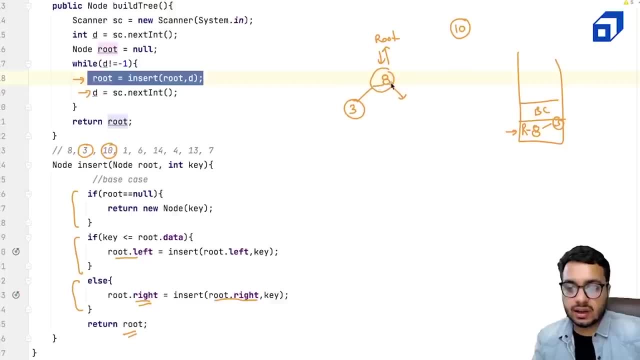 Key Root Right. This Is Null. That Means You This Case Is Over. Eight Is Connected With Ten And You Return Root. What Is The Root? 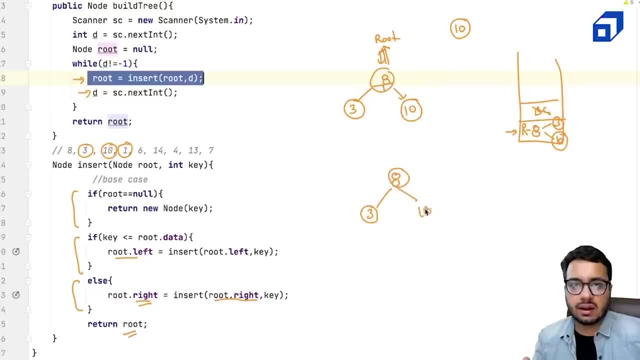 This Eight Is The Root Note, So You Return This Address Back. Insert One In My Left Subtree. It Makes A Call Here When You. 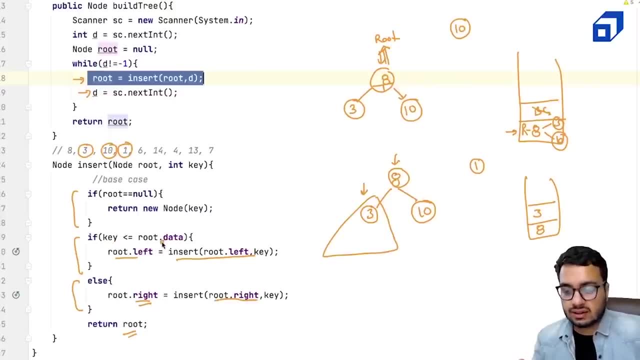 Reach Three, So Your Root Is Three And You Again, Compare, Is Three Is One, Less, That Is One. This One Is Updated In The Left. 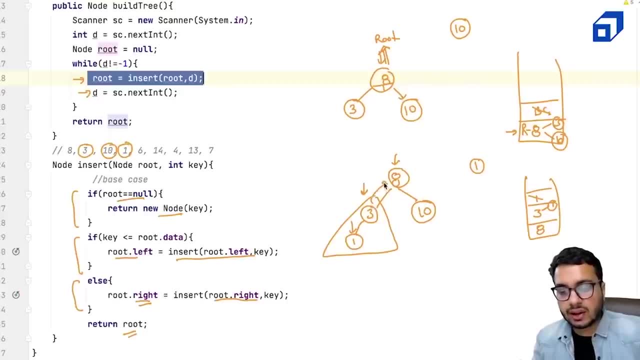 Of Three, So You Return One. One Gets Attached In The Left Of Three And Then You Say Return. So This Is Again Updated Earlier It. 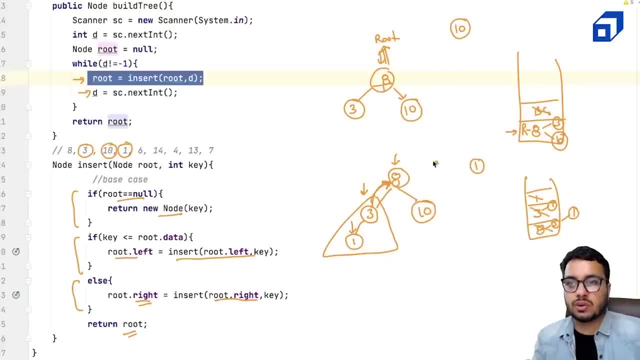 Was Storing The Address Of Three. Now Again It Is Storing The Address Of Three And Again You Say Okay From This Is Less Than. 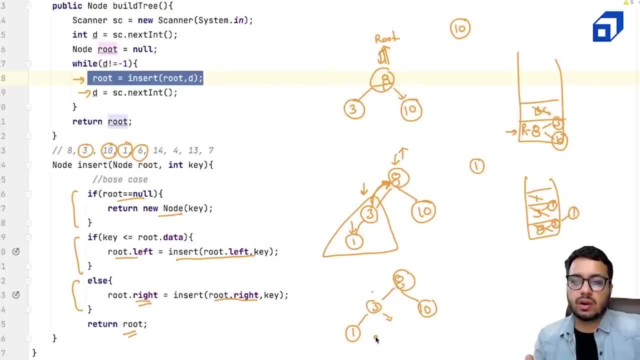 It. I Go Here. Six Is Greater Than Three. I Go Here Again. What Happens? This Is Null. So You Return A New Note. You. 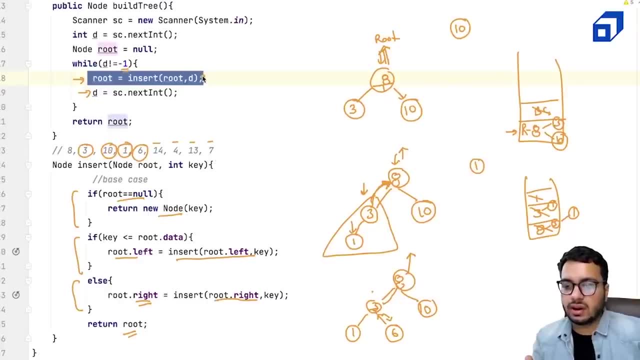 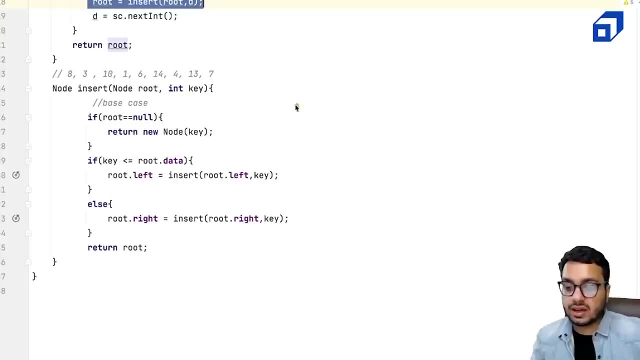 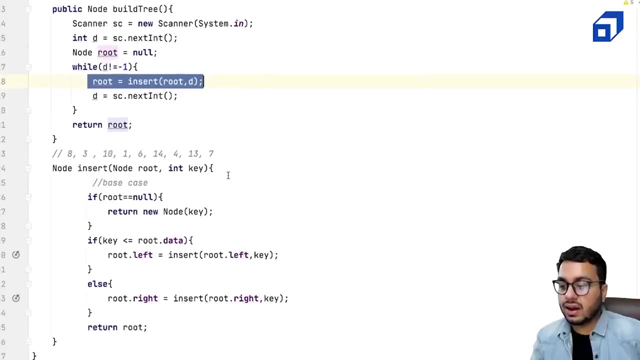 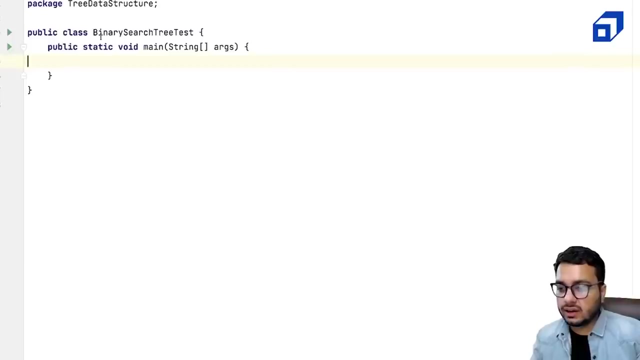 Create Until You Hit Minus One Into This Tree, Right? I Hope You Understood The Insert Method. The Insert Method Is Going To Take Order. 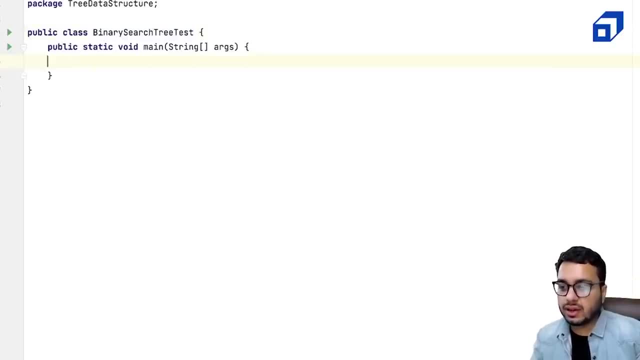 Of S Time To Insert A B S T Object Here. So I Have To Say Binary Search Tree B S T. This Is Equal To: 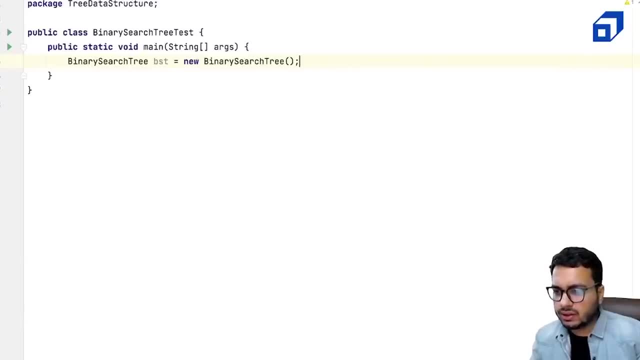 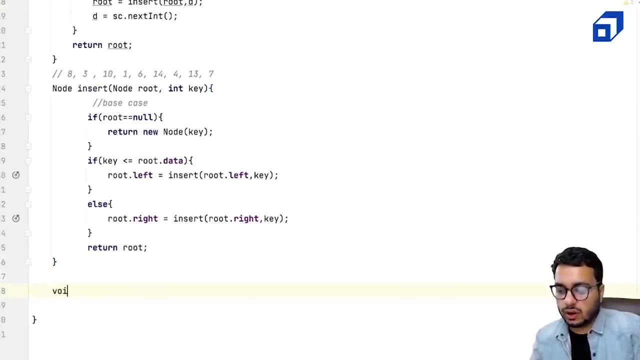 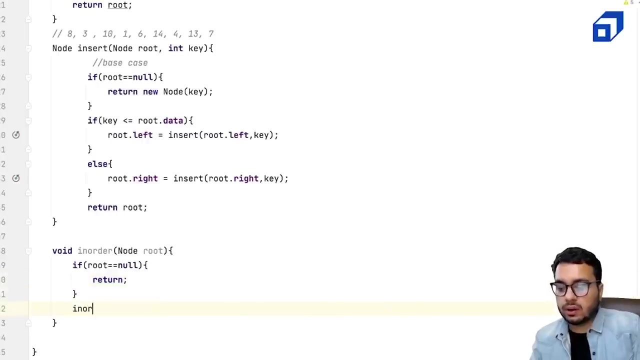 New Binary Search Tree. This Will Automatically Trigger The Inorder Print Of This Tree Right. So Void Inorder. I Can Say Node Root And Here 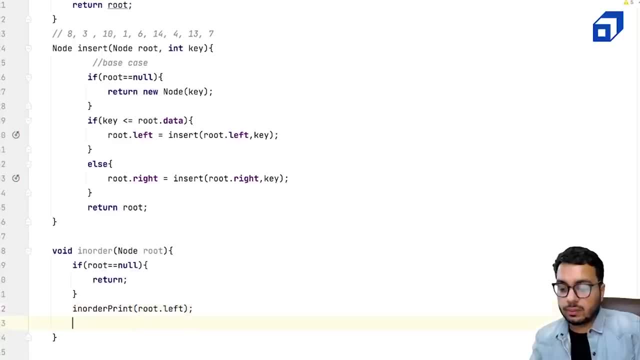 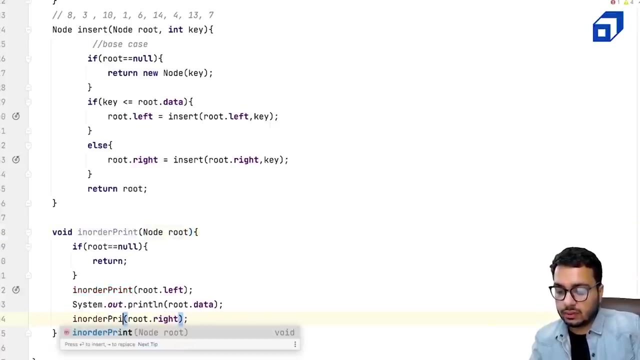 I Can, Okay, If Root Is Null To Nothing Otherwise, Do A Inorder Print, So Let's Call This As Inorder Print, Inorder Print, Okay. 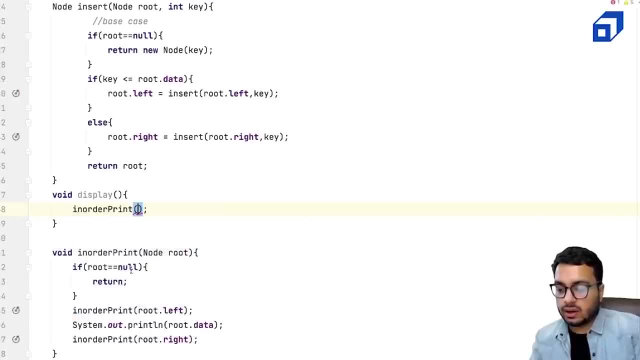 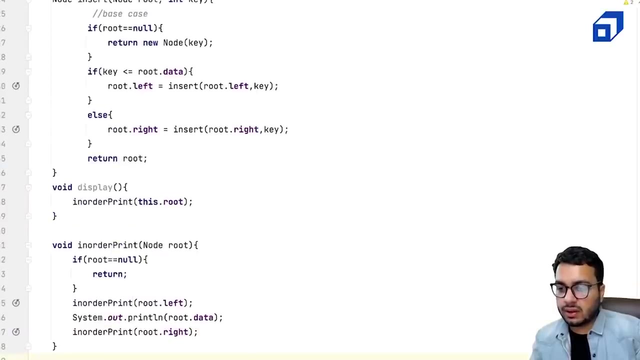 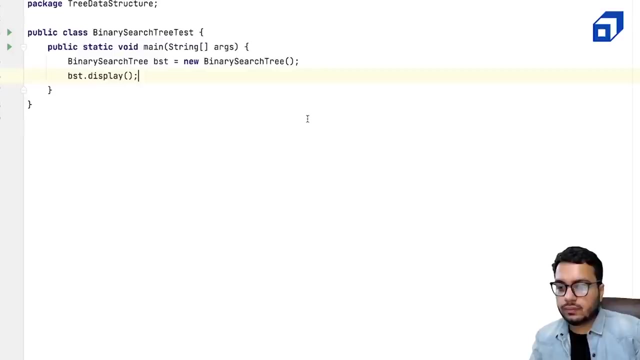 Let Me Create A Display Method From Where I Will Call The Inorder Print Method, So I Can To Create The BST And I Can. 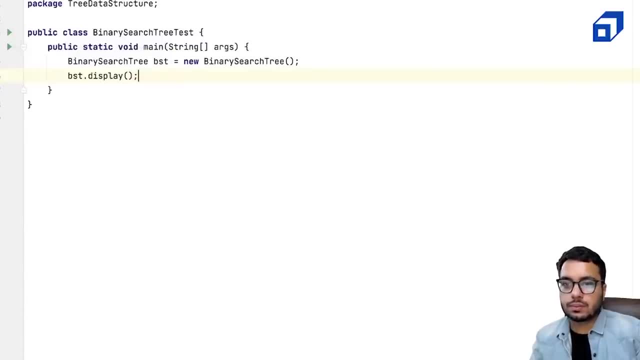 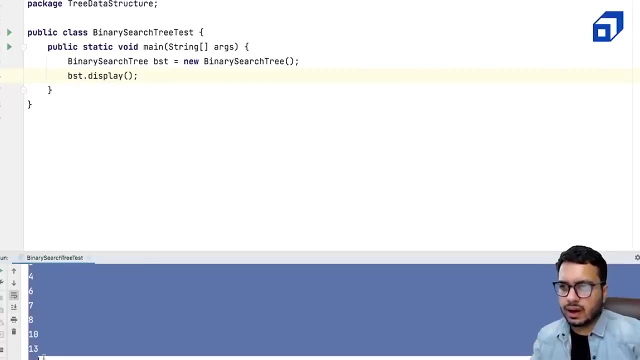 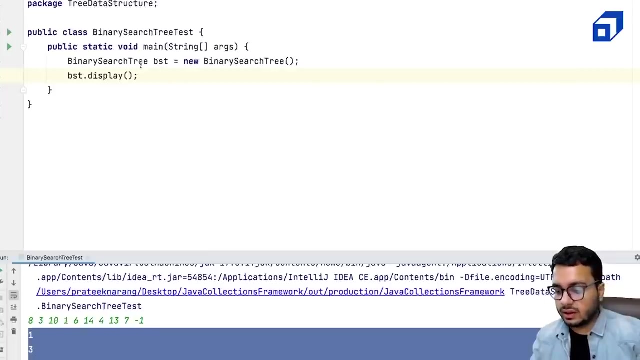 Say BST Display. Let Us Execute This Code. The Build Is Complete. It Is Waiting To Waiting For Us To Give Input, So Let Us Quickly. 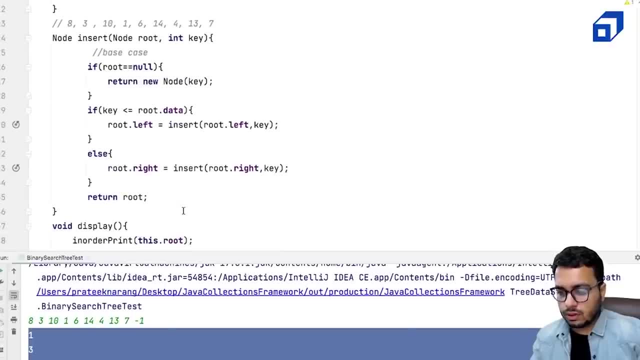 Create A Tree With These Numbers. So I Have Eight, I Have Three, I Have Ten, I Have One, I Have Six, I Have Fourteen. 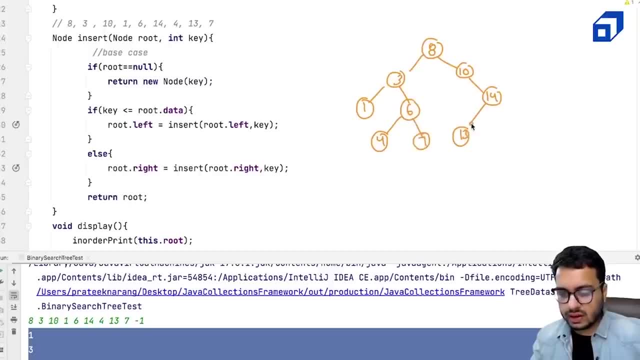 I Have Twelve, Fourteen, I Have Three, So One, Two, Three, Fourteen. One Three, One, Two, Four, Six. We Have Three Out, One, Two, Three. 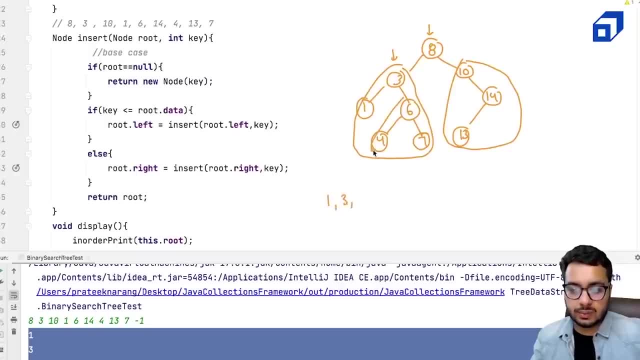 So We Have Two, Three, One left root, right, so you will print 4, 6, 7 and then you go back here for 8 left sub tree has been printed, so you print root and then you print right, so you come here at 10, you circle left. 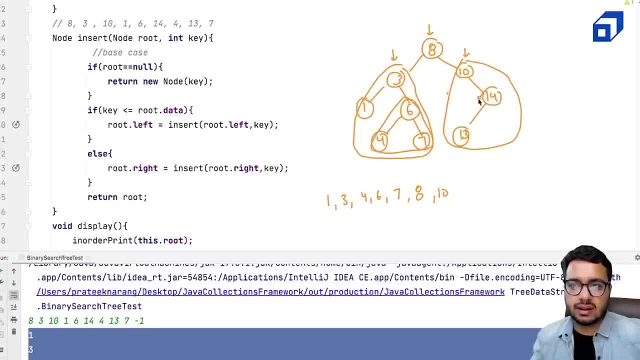 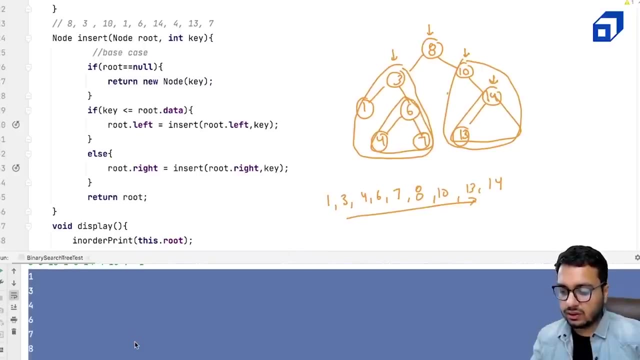 which is null, then root, which is 10, then the right sub tree. so again here, left root, right. so again you will print 13 and 14. so this is the expected output of in order traversal. let us verify: if it is correct, we are getting 1, 3, 4, 6, 7, 8, 10, 13, 14, which is absolutely correct, so that 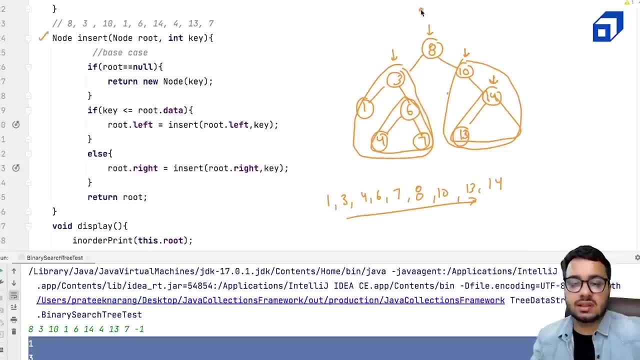 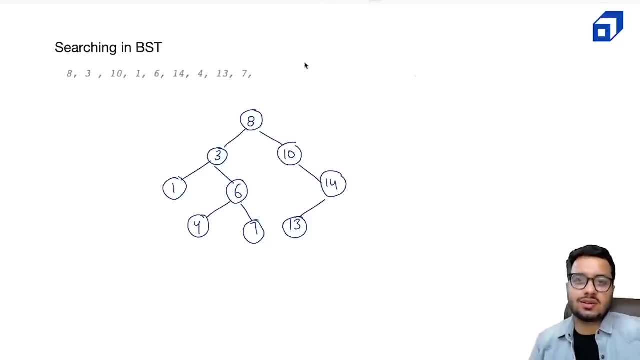 means our build tree and the insert methods. they are working perfectly fine, right? so i hope you have understood the insertion in a binary search tree. now let us talk about the search operation in a binary search tree. so, given this bst, i want to search for a particular node, for example: 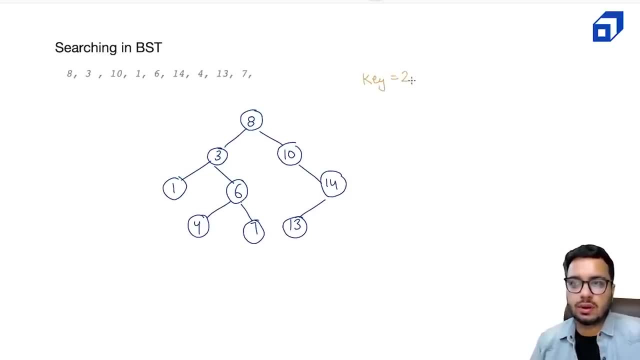 let's say i'm given that i'm searching for a key that is 2, how do i search for 2? right, so i will start from the root node. i will compare 8 with 2, so i will say, okay, 2 is less than 8, so i will go here, i will go left. 2 is also less than. 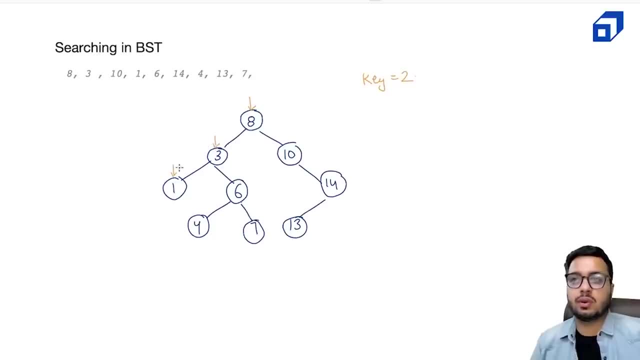 3. so i will go here and here i compare if 2 with 1. so what happens? if 2 is present, it must be on the right of 1. so i go here, so i go in the right of 1. but as i reach here i see that i am hitting. 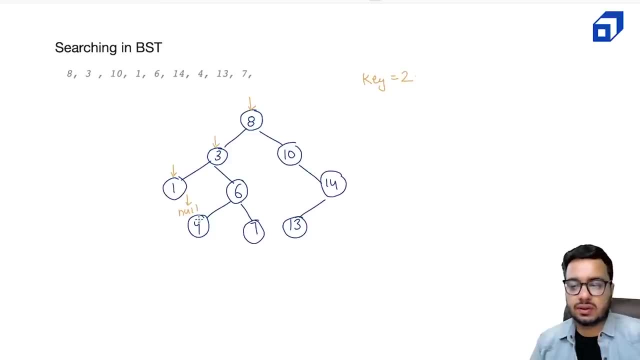 a null value, that means 2 is not present, right. so one of our case would be that if i hit a node that is null right, that means the given key is not present, so i can simply return false. that will be one kind of a base case, right? 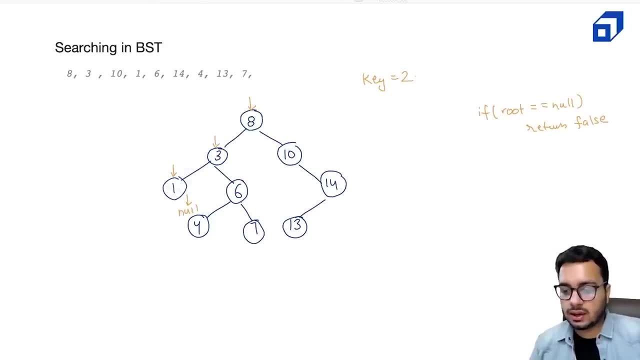 now suppose i am not searching for 2, but i am searching for, let's say, 7, right? so 7 is present here. let's see how we can do it now. if i compare 7 with 8, i know it is less than 8, so i will go left if i come to 3, right? so one of our case would be that if i hit a node, 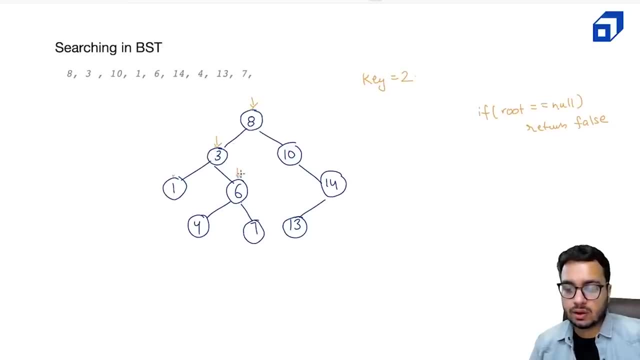 7 is greater than 3, so i will come towards right. and at 6, 7 is greater than 6, so i will again come towards right. so now i am hitting a node where my root data matches with key. so what should i return? of course i should return true. so if root data matches with my key, i would be returning. 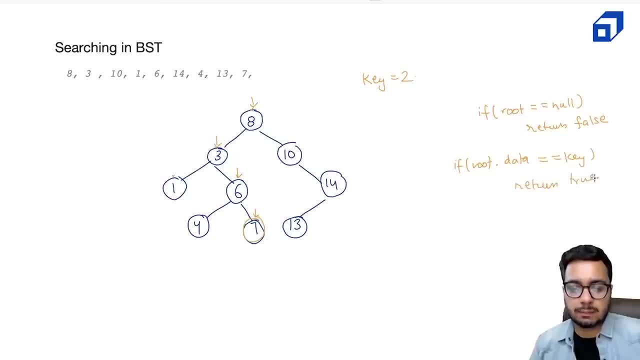 true from the method. right now, let us talk about a recursive case. if we are searching recursively, so what exactly we are doing right? so we are saying that, fine, i am going to compare root node with- uh, the given key. let's say the key is 7. so i am comparing 8 with 7 right now, if the key is, 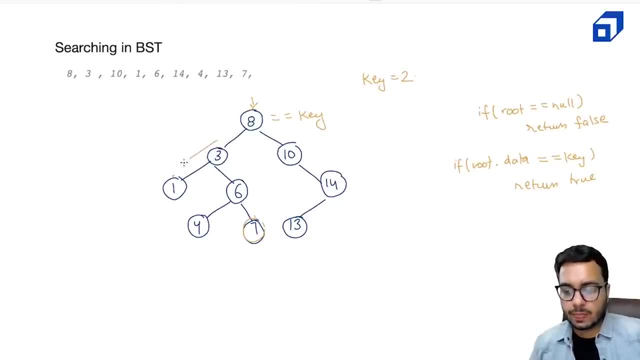 not matching. so what? i am saying that okay, if the key is lesser i will search in the left subtree. whatever is the answer of left subtree, i will return that answer. now, suppose the left subtree says true, that key is found, i will return true. but if the left subtree says false i will go and 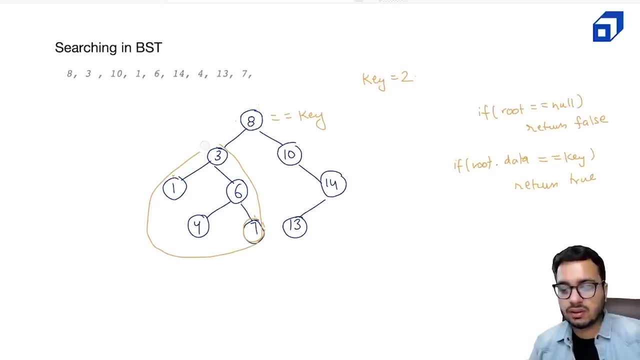 search you. I will not go and search in the right subtree. why? because i am already checking whether i should go left or i should go right. right, because if the key is less than or equal to, it will be present in the left subtree. if the key is greater than or equal to root node, it will be present in the right subtree. 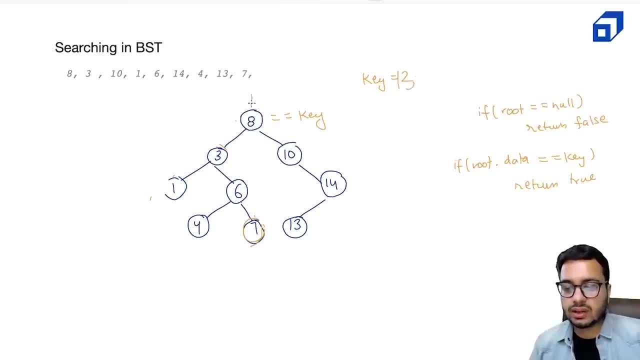 let us take an example of 13. right, so now 13 is greater. so i will not make a call in the left subtree, i will make a call in the right subtree price: okay, go and search in this tree now, at 10, 13 is greater. 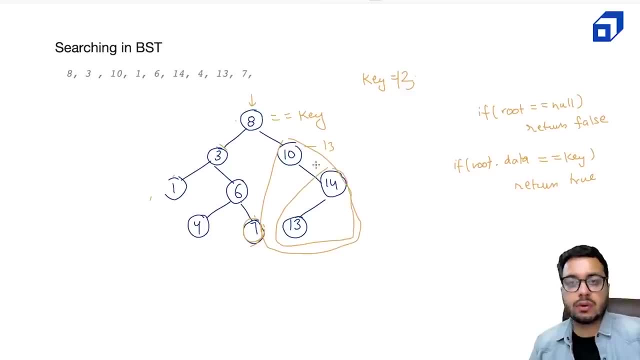 what i do? i say, okay, go and search in the right subtree. at 14, 13 is less than 14. so what do i do? i say, go and search in the left subtree. now, as i reach this node, i say, okay, this match is my key. 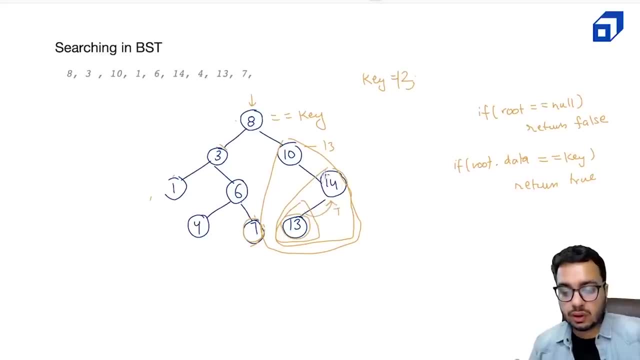 so what i will do: i will return true, this 14 will also return true, this 10 will also return true and this 8 will also return true. so this is how true will be propagated back right. so what i have to do if root data is. 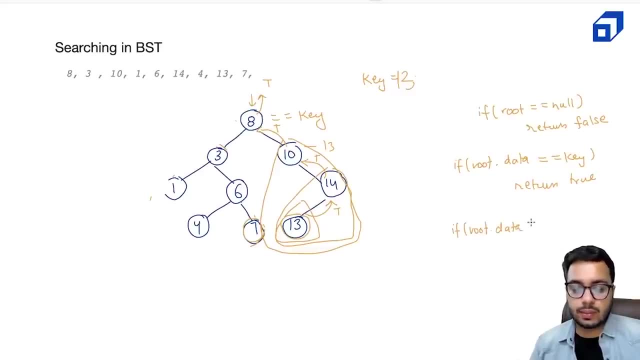 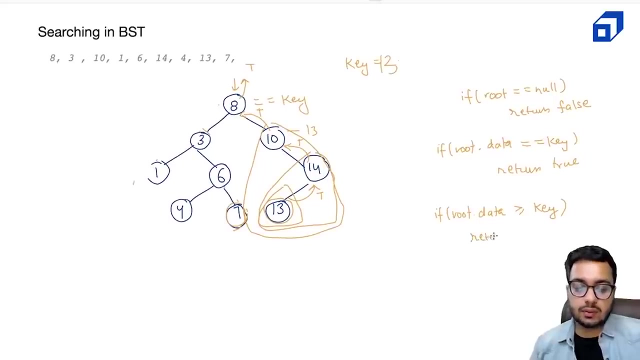 let's say root data is greater than equal to key right. so that means key is less than equal to root data. that means i will return the answer of the search method by calling the left subtree. so i will say, okay, return whatever has been returned by the left subtree for that key. so root dot left. 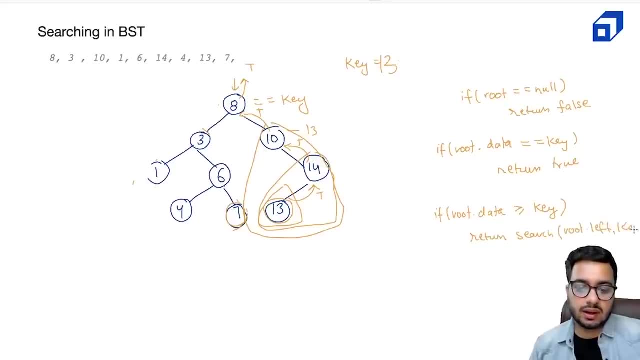 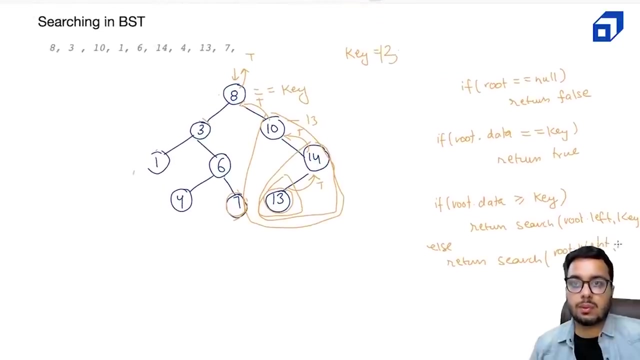 comma key right. otherwise i will say return. whatever has been returned by the left subtree has been returned by the search method, by calling it on the right tree. so root dot, right comma. so this will be my search method. now let us quickly write this method in our code as well. 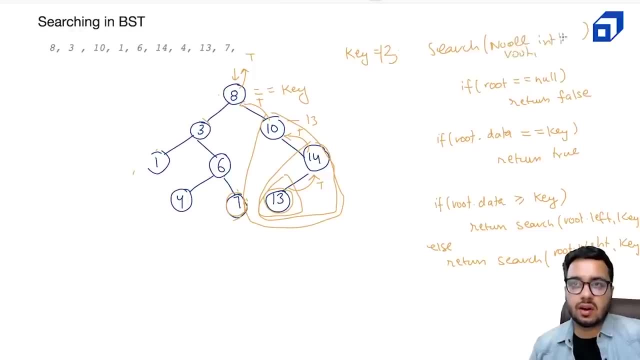 and then we will see whether this works correctly or not. it should, it should work, right. so this i'm writing it recursively. you can also write it iteratively, right? so the only thing that you to travel at max from the root node to one of the leaf nodes, in the worst case that means 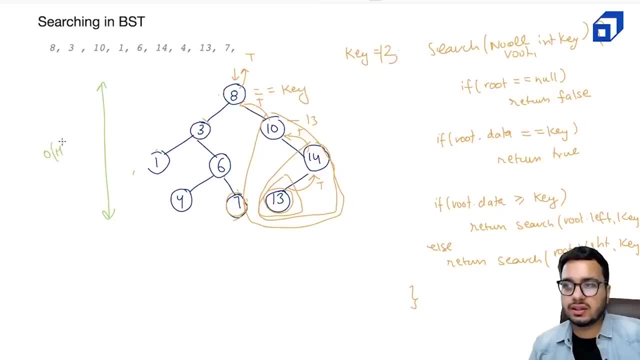 the complexity of this method will be order of h, where h can lie between n and log n, right. so in the best case scenario, when the tree is perfectly balanced, your height will be log n. in the worst case, if all the nodes are on one side, that is called as a skewed tree. 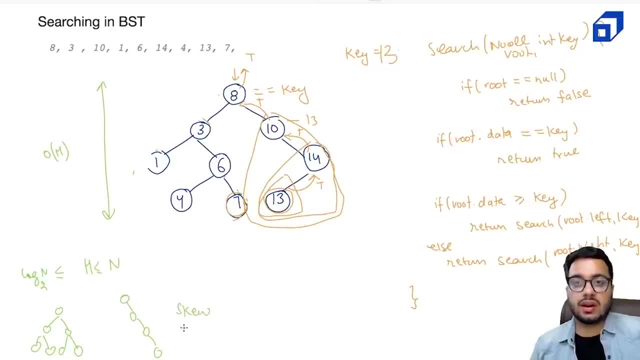 your complexity for search operation will be order of n. now, it is much better than binary tree, because in binary tree you have to search for across all the nodes, but here we know that we have to move in one direction, either left or right, but not both. okay, let us quickly. 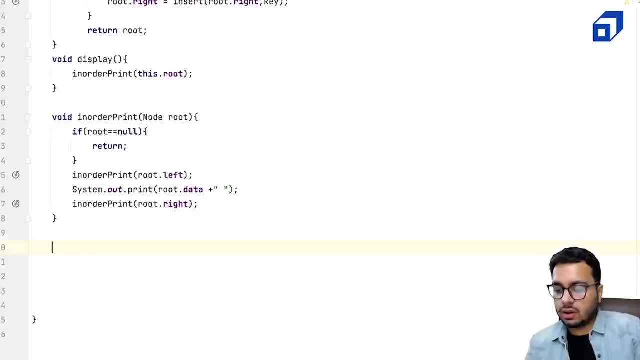 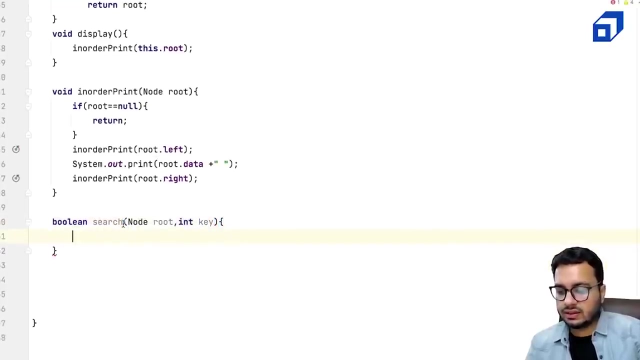 code it up and see. so let us write a method called search, so it will have a boolean return type, so i can say boolean search, i am going to get the root node and i am also going to get the key that i am searching for. okay, let's say this is some search function, right? so 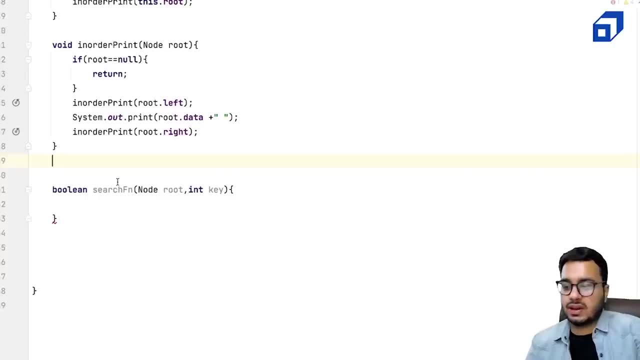 it's a recursive function, so i have to write a wrapper function as well. so i can say boolean search, where i am just getting the key, so it will return whatever has been returned by the search function, and here i will pass the root node and the key. now let us see how. 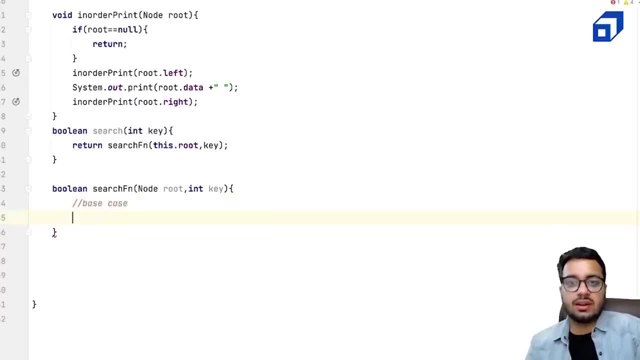 this can be done. so i discussed there will be two base case so you can stop. if your root is null, that means the key is not present. so i can say return false in that case. but if your root matches with the key, you can return true in. 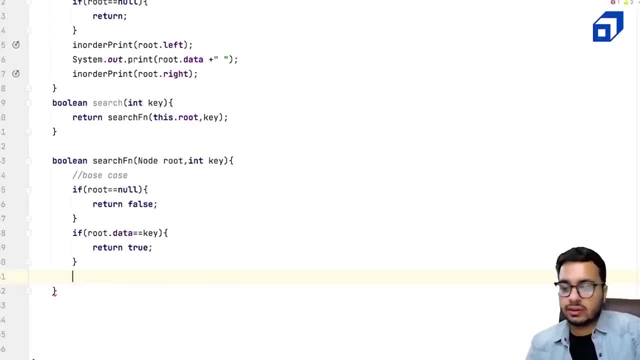 that case okay, otherwise i have to compare. okay. so i have to say: if root dot data is greater than equal to key, or you can say key is less than equal to root data, then you have to call the search function on the left. so i have to call the search function on the. 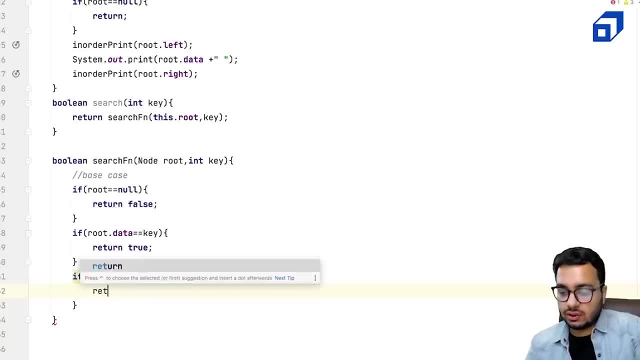 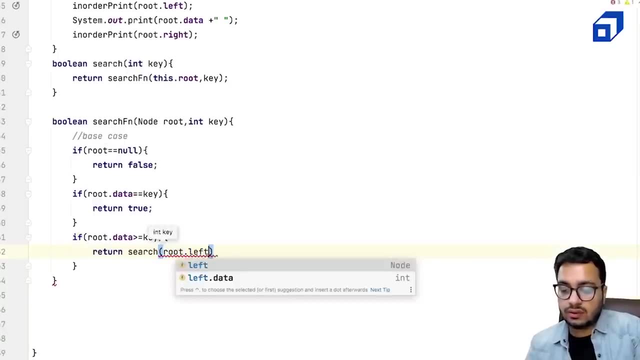 left and you have to return whatever that function is returning. so you return the output of the left subtree. so search in the left subtree that is root dot left comma key. else you can return the output of the right subtree. so root dot right, comma right. so this will. 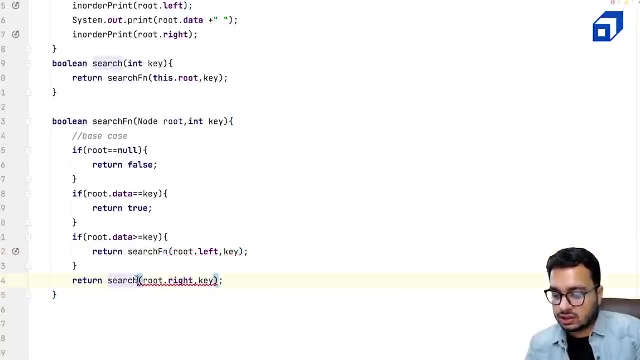 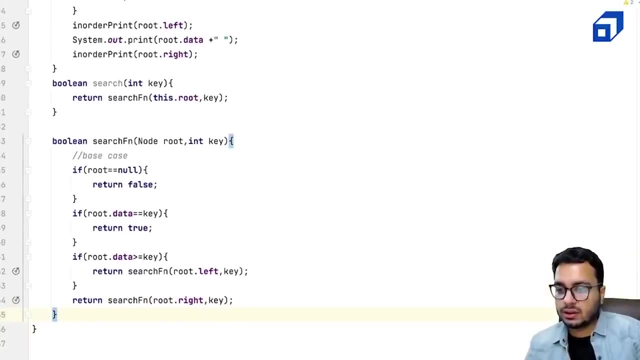 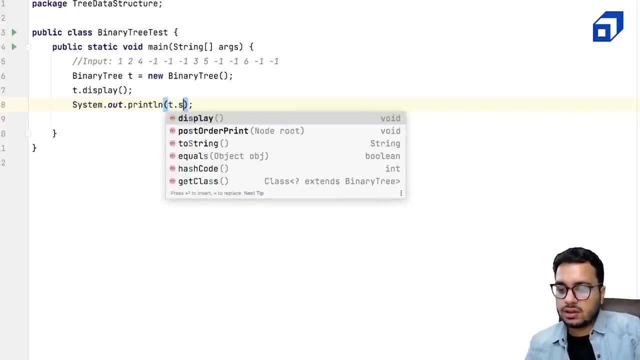 be your search function. recursive function is the search function. okay, so this looks good. so let us test our method. so here i can. okay uh s out t dot search. let's say i'm going to search for four. sorry, this is not uh the correct file. i have to do it in binary search tree: vst dot search. 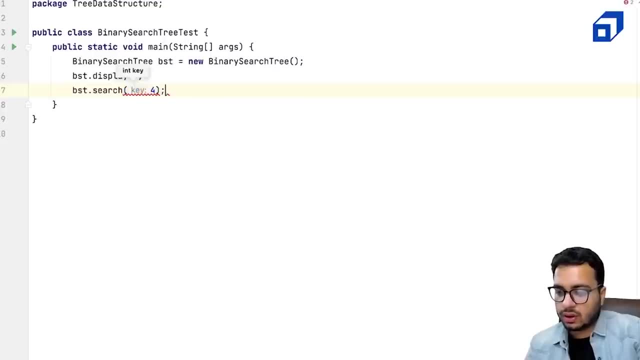 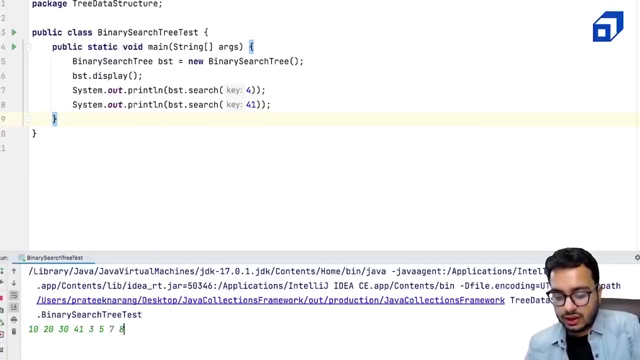 i can say: let's just search for four and bst dot search for. let's say 41, right, so i will s out output and same here. this looks good to go and let us run our code now. let us give some elements. let's say ten, twenty, thirty, forty one, three, five, six, eight. 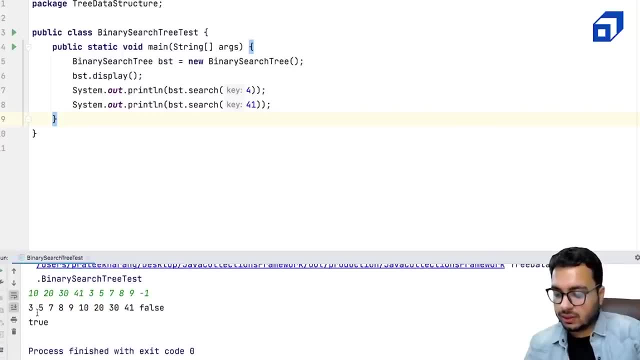 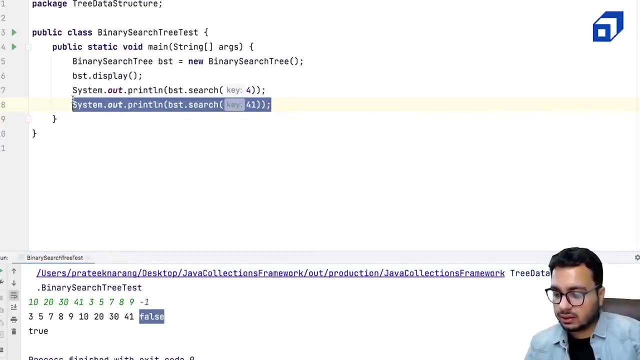 nine minus one, right, so this creates a tree. and for the value four, i'm getting an answer: false, that four is not present. and uh, for other values, i'm getting the tree, i'm getting. the tree is, uh, the forty one is present. the forty one is present here, right, and you can see in order. 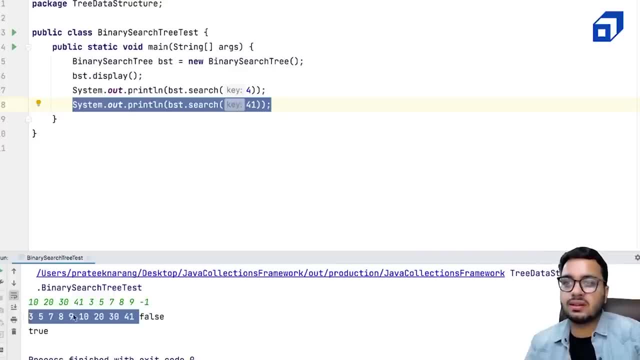 display is looking sorted and four is not present in this and forty one is present. okay, this is how the search method is working. i hope you understood the search method really well. next we will move on to deletion. let us discuss deletion in a case of a binary. 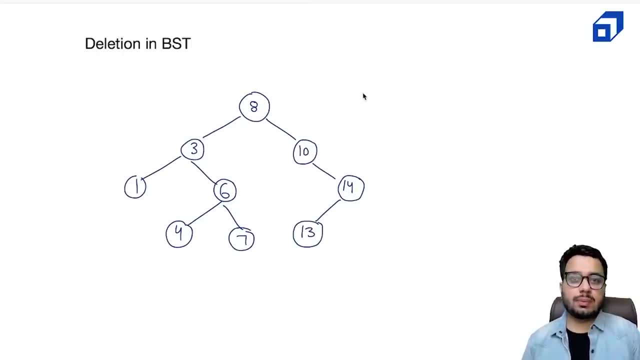 search tree. so deletion means that, okay, i've given a particular note and i want to remove that note. okay. for example, someone might say that, okay, let us delete thirteen, or let us delete three, or let us delete eight, right? so if you observe closely, there are three. 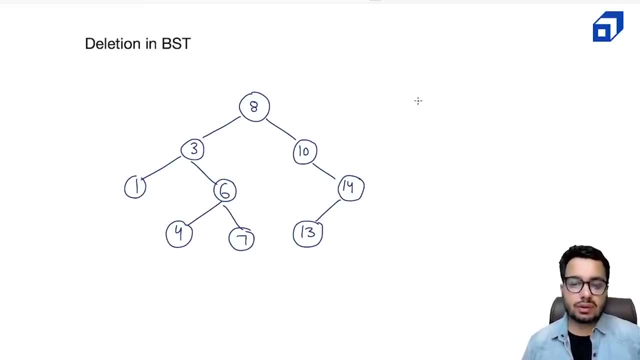 kinds of notes. okay, so there are nodes which have no children, also called as leaf nodes. there are nodes with zero children. deleting them is very easy. there are also nodes which have one child. deleting them is, uh, slightly more difficult. and there are nodes which have two children. they are even more tricky to delete. okay, for example, node like eight, if 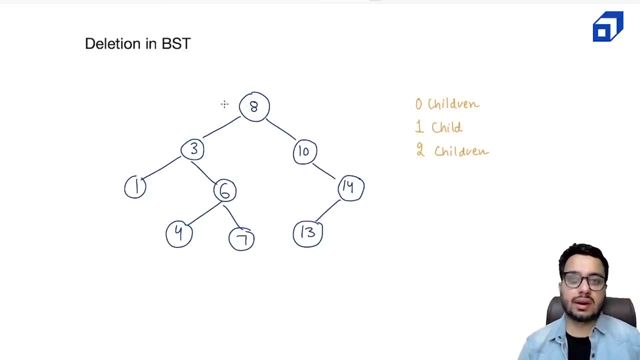 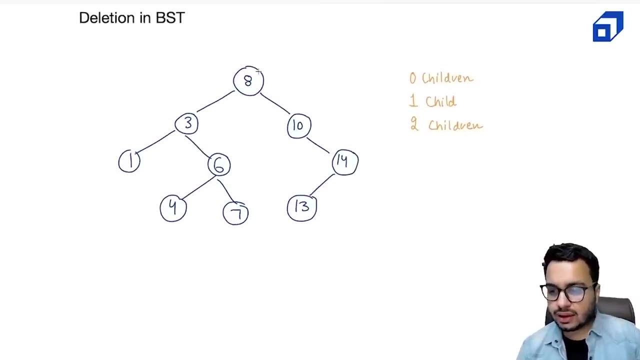 i want to delete this node, then how would my tree structure would look like? so we have to discuss all these scenarios now. right, let us start with scenario one and let me create a copy of this tree as well, so that i can use it right now. suppose i want to delete. 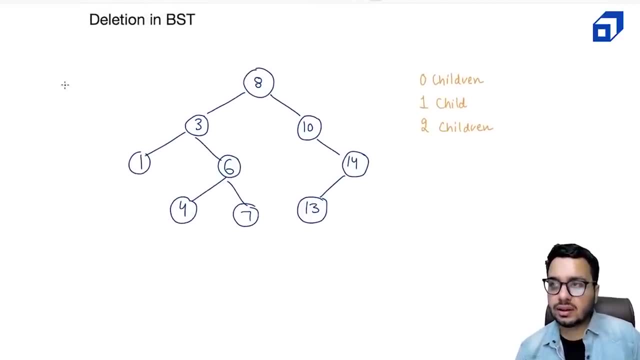 a node like four, or i want to delete seven, or i want to delete thirteen, so deleting it is very easy. so suppose let's say i want to delete, delete seven, right? so that is my case one, case number one. so in that case, what i need to do? first i need to search for seven. where is this seven located? right? so i need: 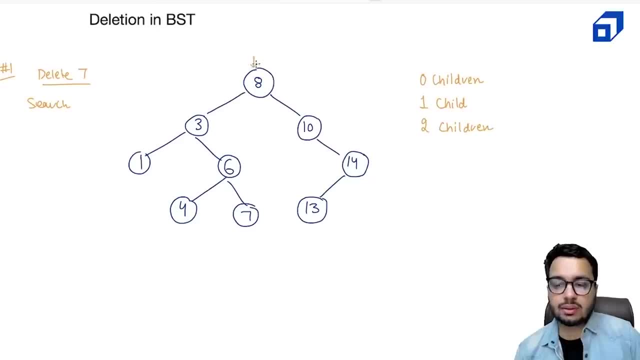 to reach that node. so i start from eight. i say, okay, seven must be on the left. so i go to three. so three says seven must be on the right. so i go here now. six says seven must be on. uh, right, so i go here right now. if i reach this node, what should i do? i would show. 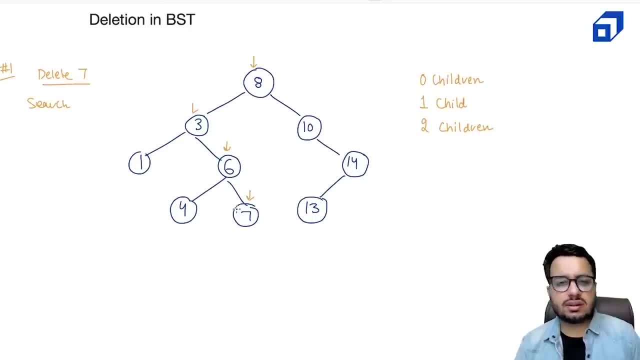 okay, fine, this is a node that i want to delete. i will somehow delete this node and i will return a value- null- to the parent. so basically what i will do: in every call i will try to change the tree. i will say: okay, in the right of six, i will attach a null value and this: 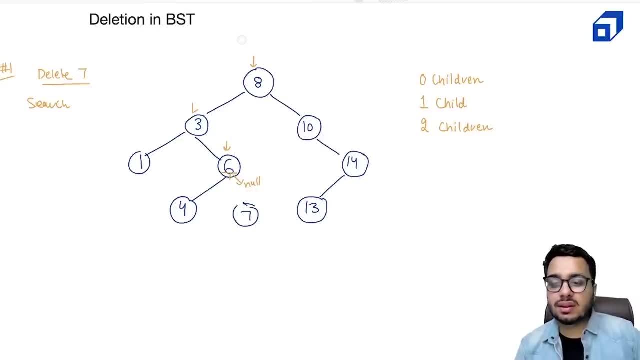 node is now referenced by no one, so that means this will be automatically garbage collected. okay, so garbage collector will come and it will get garbage collected because no one is referring to this node. okay, so garbage collection mechanism will clear out the memory occupied with by this node. so what? what i need to do is i need to reach this node and if this matches, 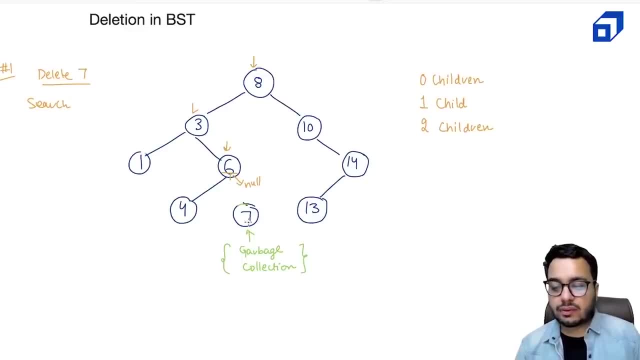 with the data that i am finding out, i have to return delete null. okay, so when i return null value, that will get updated in the right of six. okay, so i will also update. so that means, uh, the return type of the function will be of the type node. it will not be displayed. 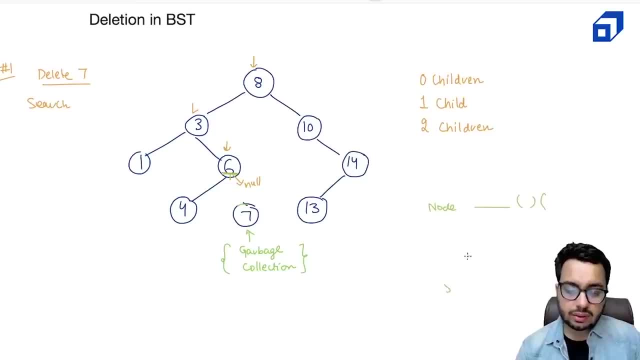 be a void function. so there will be a function and, as you can find root dot right, this is equal to some delete node and, uh, delete node returns a null value which gets attached in the right of six. okay, so this function is delete node, something like this. i will be doing so just to give you an. 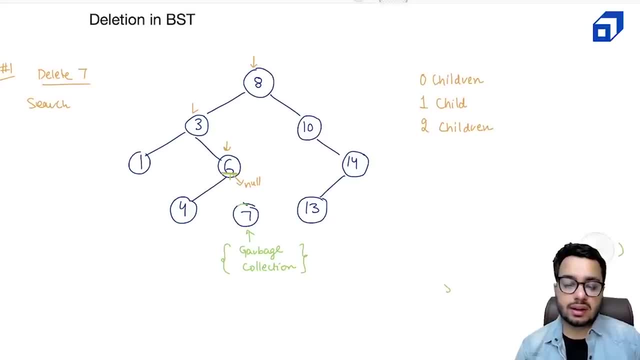 idea how it's going to work. so, basically, we are going to update the right reference in the parent. that is case number one. this is how it will be deleted. now let us write the code and see case number one, and then we will discuss case number two and case number three. 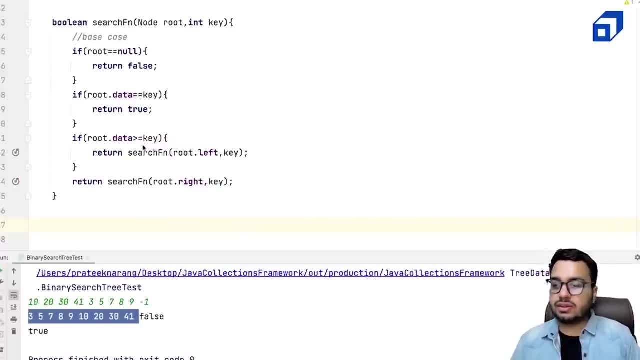 so i am in the uh file called binary search tree dot java, which we have written. now we are going to define a method called as node remove, and here we are going to accept the current root node and the key that we want to delete. right, of course there will. 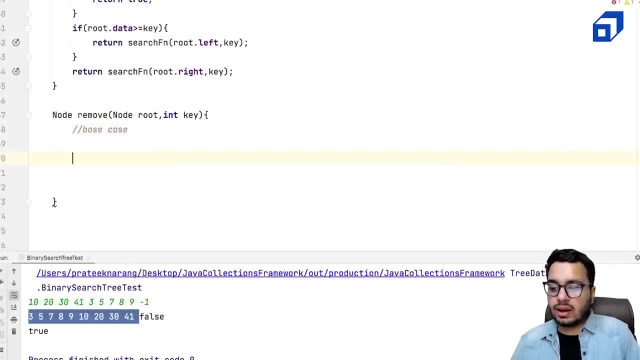 be some base cases, which we will see, okay, and there will be some recursive cases as well, right? so one thing that i told you that first we have to search for the node, okay, now, uh, three possibilities can happen. so if you are at eight and that the node that you are deleting, 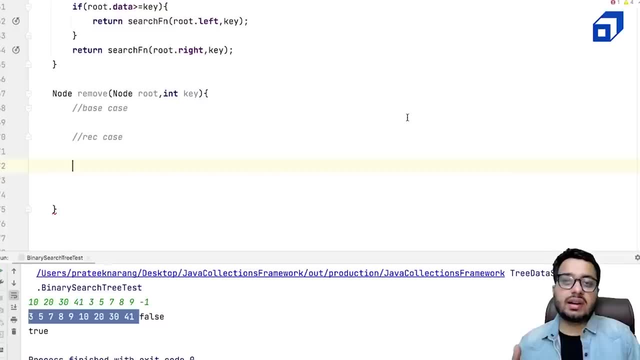 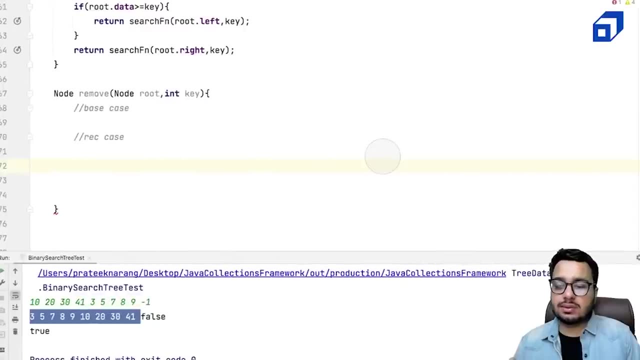 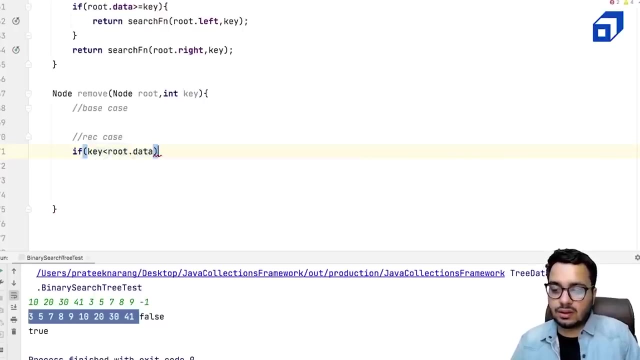 is also eight, then you can do work there. but if the data is lesser than eight, you have to go left. if the data is greater than eight, then you have to go right. so first let us do the searching part. so if the key that you are that you want to remove is less than root dot data, in that case you do not. 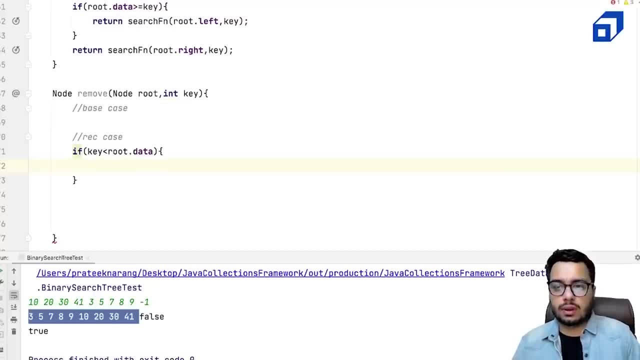 have to do anything at the current root node. what you need to do is make a recursive call in the left sub tree. for example, this is eight and i want to delete something which is five. a five is not present here. so what i will say? okay, i will say: go and remove five from the left sub. 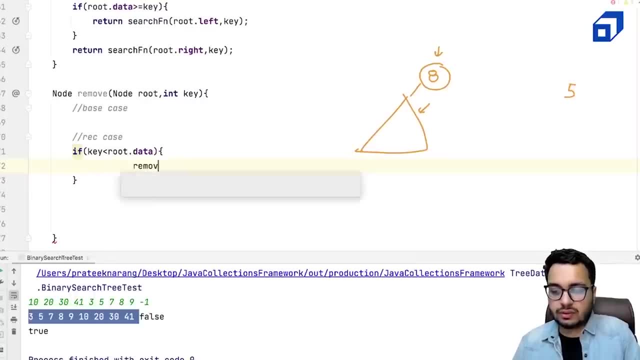 tree, the remove function will go and remove five from the left sub tree. so you say root, dot, left and key, go and go into this tree and remove it. now it is possible five might be present here here or five might be present here, we do not know right. so whatever it is, uh, after removing five, 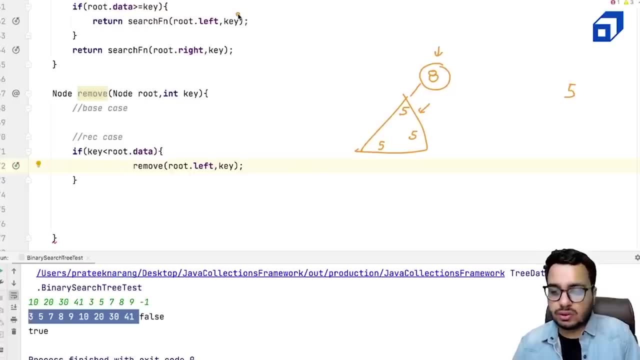 whatever is the new root of the tree, that will be given back to me. so i will say: okay, eight dot left, this is equal to remove. so i can say root dot left should be updated by the reference of the new left sub tree that i am going to get now. it is possible that 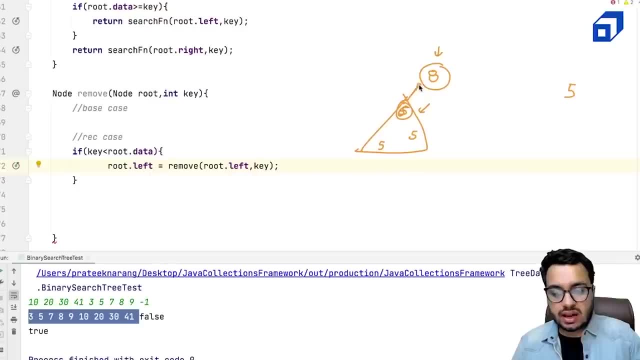 here the node was six and nothing changed. still, i will get the address of six back here, right? so that is something we have to do. the root dot left this is equal to remove. so i make a call in the left sub tree to remove it. so this is a recursive case, right, else it is also possible that key is. 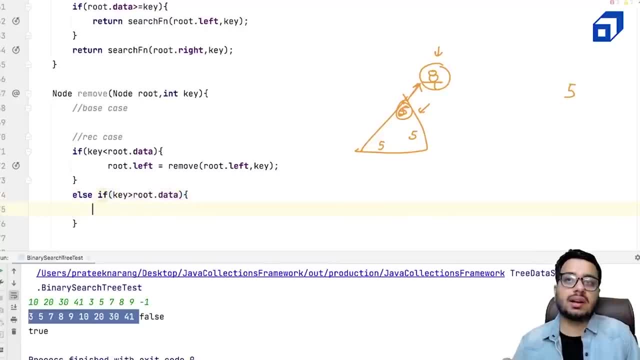 greater than root data. that means i have to do the same thing, but in the right sub tree, for example, i want to remove 10, i can say, okay, go and remove 10 from the right sub tree and whatever is the new tree, give the same thing to the new tree and then we can remove the tree from the right sub tree. 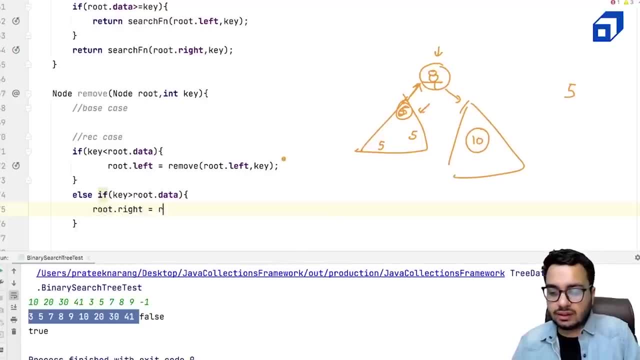 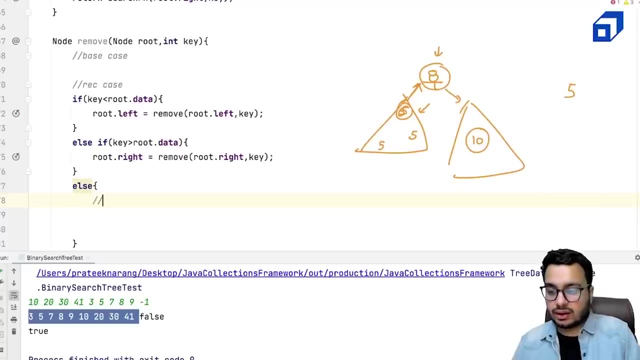 reference back to me, i can say: root dot right. this is equal to remove root dot right comma key right. else that means this is the node where i have to do the actual deletion. that means it is the case of equality right. so this is the node to be deleted now i i said there can be three cases. case 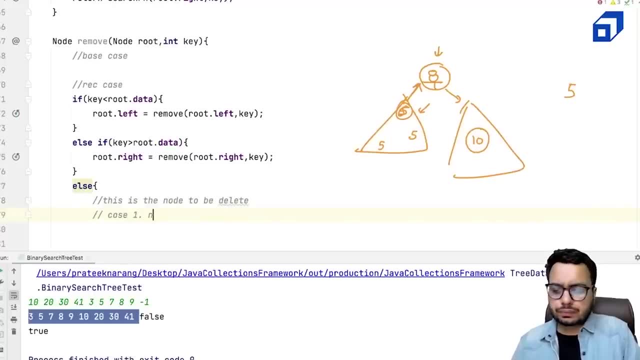 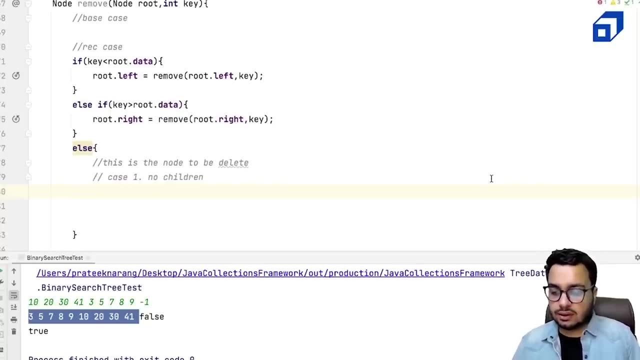 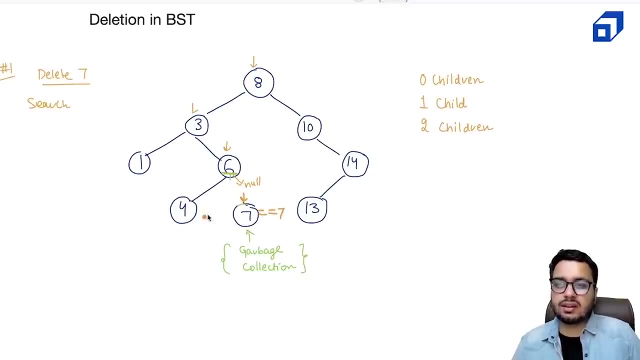 number one, that i have a node with no children. in that case, it is pretty easy that, for example, if you are talking about a node like this, uh, a node like seven, right, so if you have already traversed till this node and you want to delete this node, it matches seven. so what i can say 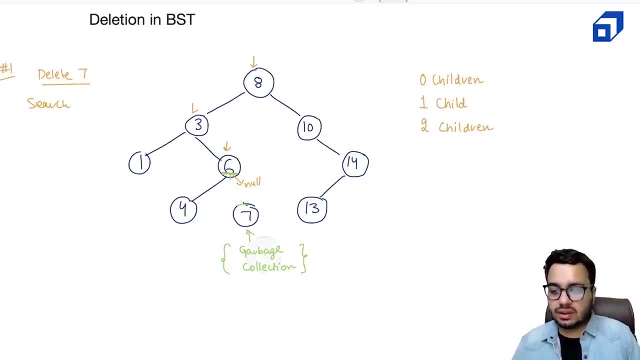 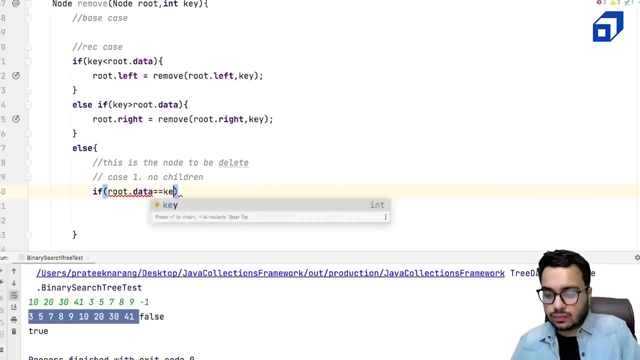 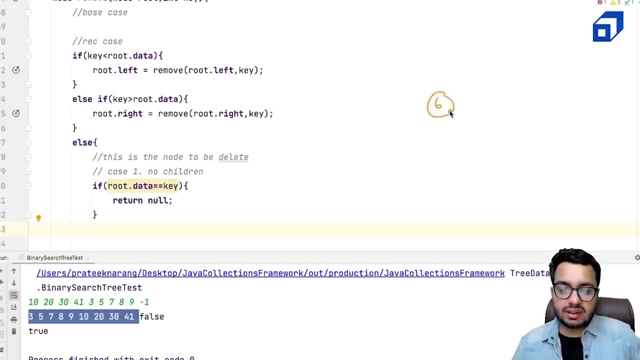 i can simply say return null. right, i can simply say return null. so i can say, if root dot data matches key, i can say return null. now this null will be attached in the uh back in the parent right. so if it was present in the left, the left value of the parent will become null. for example, six and seven right, so six made. 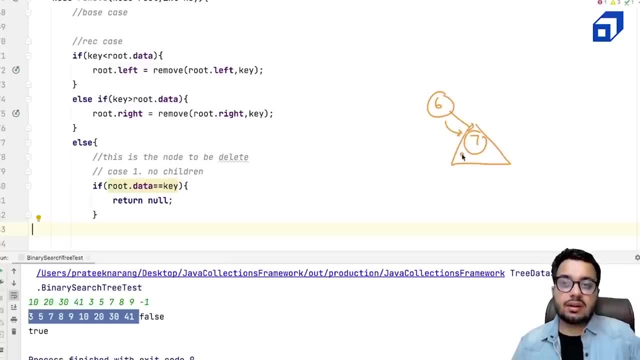 a call on the right that, okay, delete uh, the seven node from this subtree. now, seven is equal to seven. so i'm saying: return null, right, this null is returned. and root dot right called the remove function, which returned null. so this remove function returned null. so, eventually, what will happen? 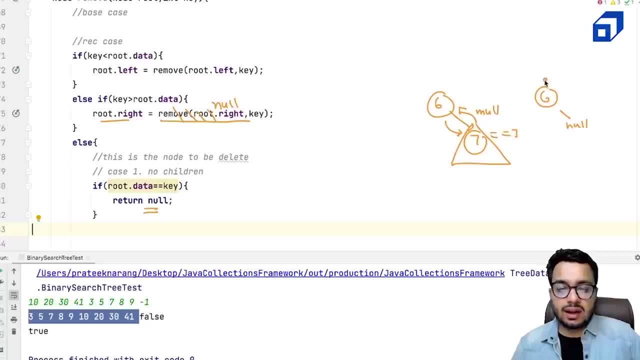 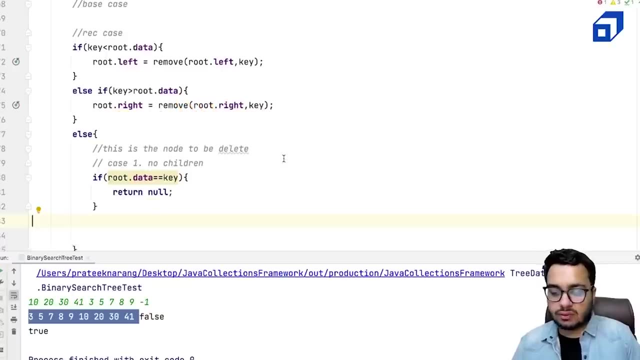 the right of six will start referring to null, and from six we will return the address of this subtree, which is nothing but this node itself, right? so finally, what what we have to return, we have to return root also, right, like if we are not returning null, that means if we are returning from. 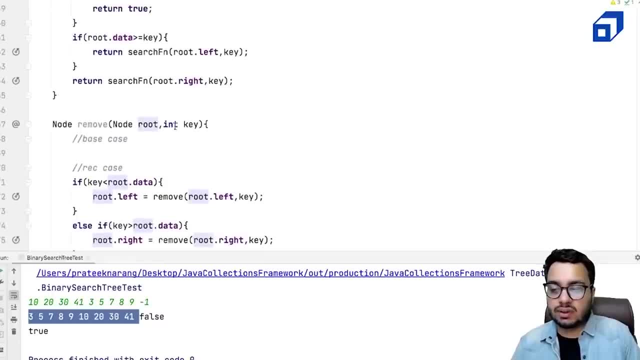 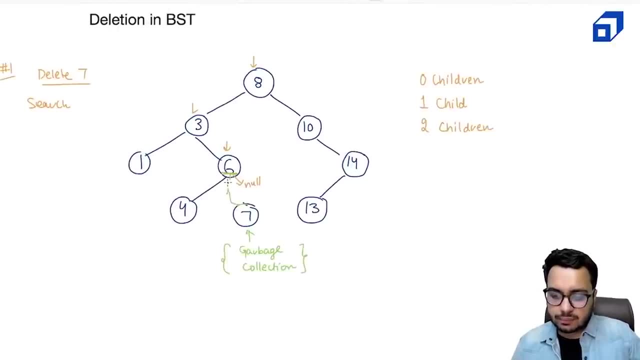 some other node, we have to return the same root that we were getting as input. so six will return null, and if we are returning from some other node we have to return this. so seven returns are null. okay, which gets attached here. six returns six. three returns three. eight returns eight. okay, this is how. 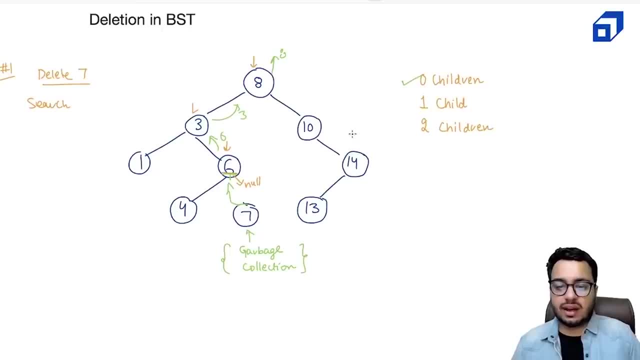 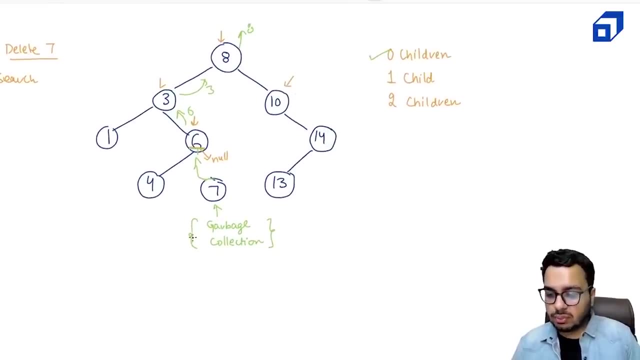 it's going to happen. so we have discussed the case with zero children. now let us discuss the case when we have one child right now. suppose i want to remove 10 right now. look at, look at this, i want to remove 10.. so let me draw this diagram again, right? 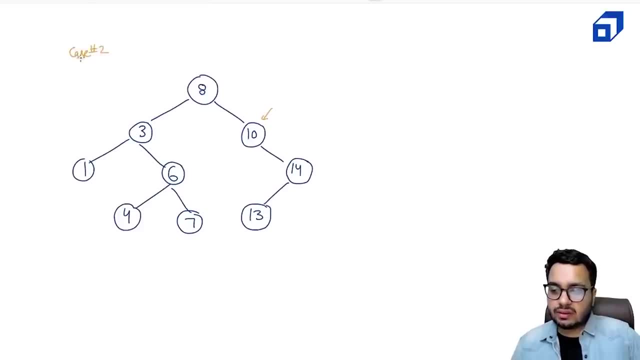 now this is case number two where i have one child right now. if you look carefully, if i want to remove 10, what should i do? right, so that simply means that it is a node which has either a left child or it has a right. check, right. if i want to remove 10, can i simply say that whatever is the left subtree or the right, 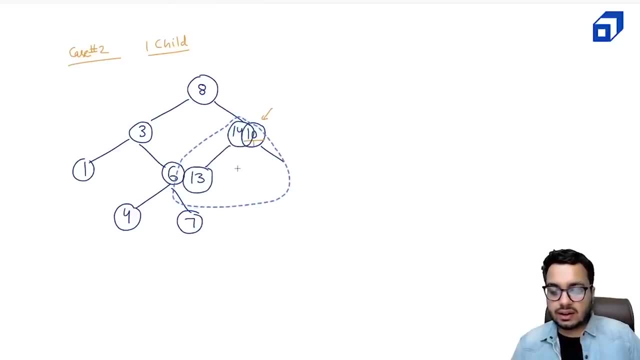 subtree of 10, this will get connected directly here and 10 will be removed. so if i simply remove 10, child will be connected here. is it correct? is it a BST? answer is yes. for 8, 14 is greater and for 13 is less than 14. so it is correctly placed, okay, what I am trying to say is, if you have 10, 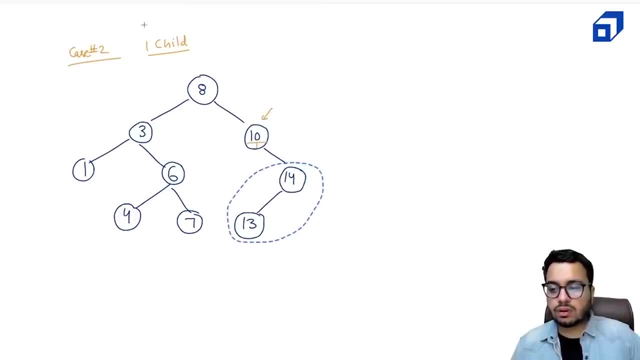 and if you want to remove 10, right, what? so you have to actually return the non null child of 10 back to 8. what is the null null child? so this is the right subtree, right? if you want to remove this node, you have to return the reference of this right subtree back to it. so 8 will point. 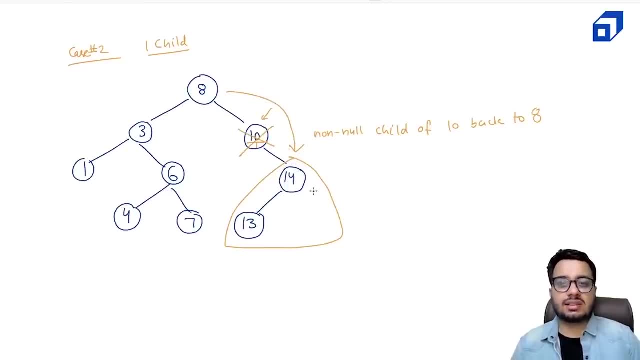 to 14 and the remaining subtree will get attached as it is. so nothing changes in the subtree. nothing changes in the subtree. okay, this is the point that I am trying to make, right? so how do you reach 10 by the search mechanism that we have already written, right? I want to delete 10, so 10 is greater. so I will come. 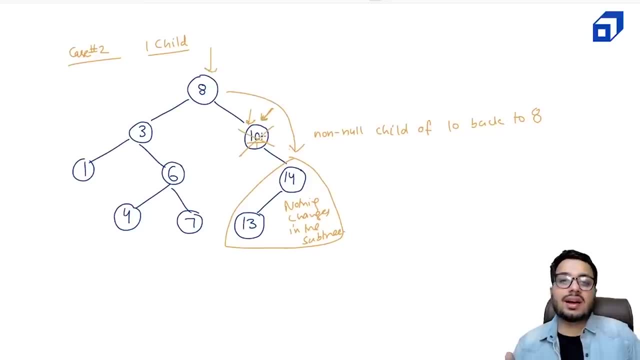 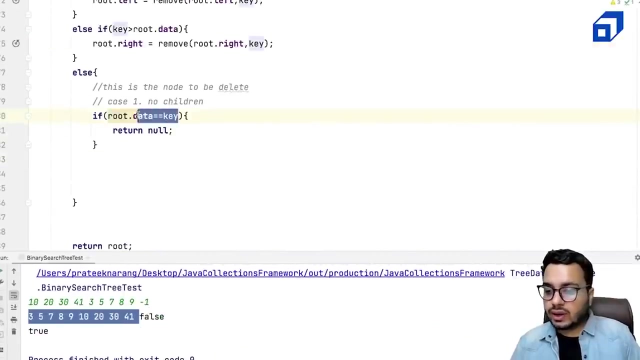 here now, at this node, 10 is equal to 10. what should I do? I will return the non null child of 10 back to the parent. this is what I have to do. now let us see how we can write it in the form of code. all right, okay, so I think I have. 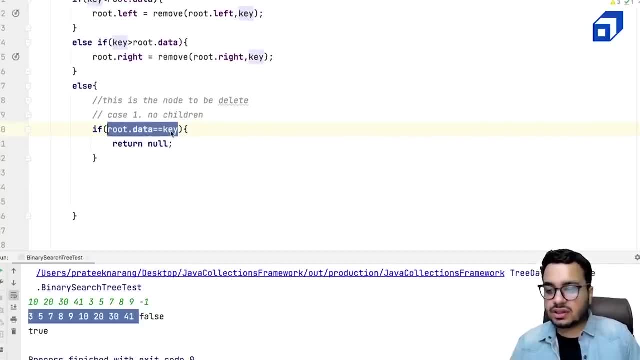 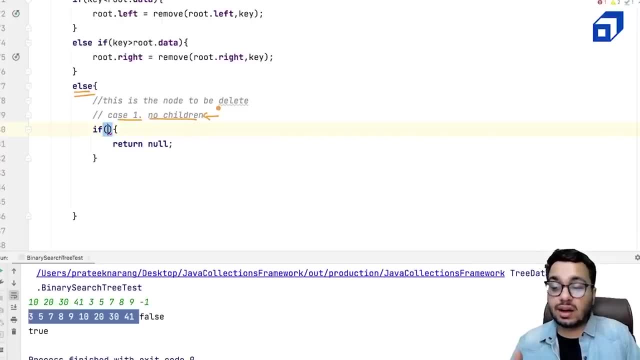 be both left and right of that node are null. okay, so I am fixing a small mistake here. root dot left is null and root dot right is also null. null would be small, small, so I can return null right. so root dot left is null and root dot right is also null. 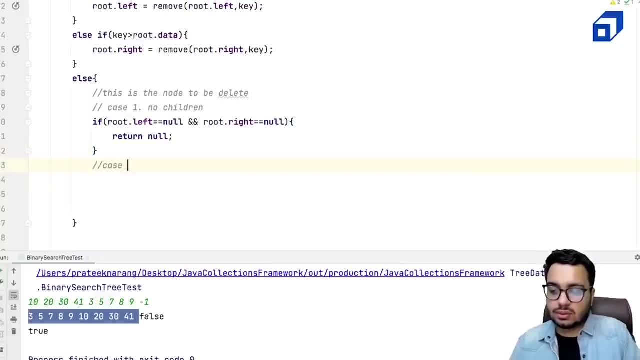 that means if it is a leaf node. okay, now let's talk about case two. that means exactly one of the child is not null. so else if root dot left is null, that means the left child is null and the right child is not null. in that case can I say I will return root dot right back to the 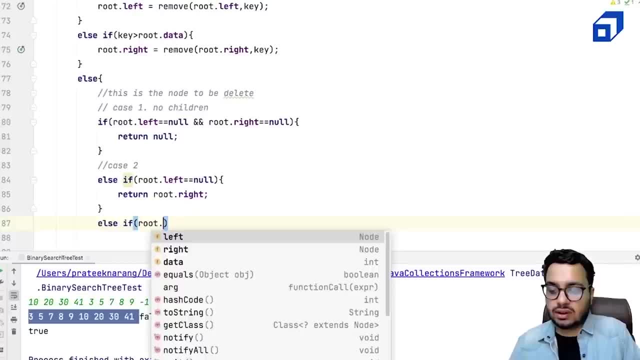 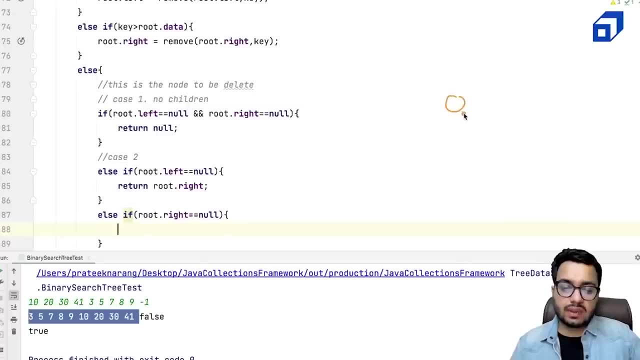 parent else. if it is the other way around, if root dot right is null, that means the right subtree does not exist. so we are at a node where the right subtree is null but the left subtree is existing, and I want to delete this node. so what I need to do? I need to return the address of the. 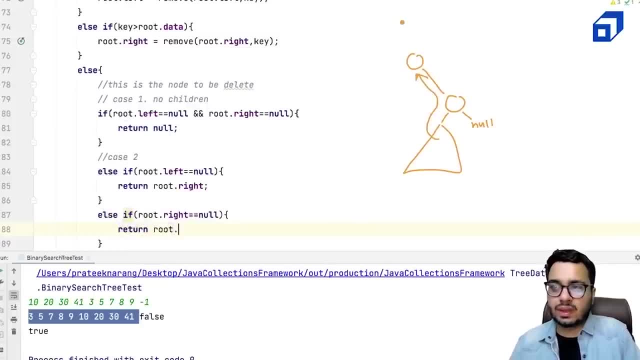 left subtree back to the parent so I can say return root dot left. now what's going to happen? this will get attached here, but do you really think that this node will be deleted? do you think this node will be deleted? the answer is yes. why? because who was storing the address of this node? 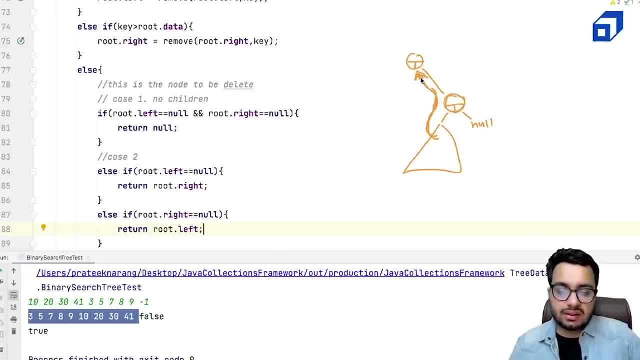 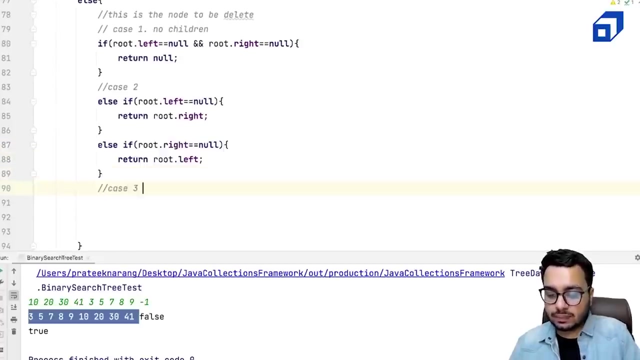 the address was being stored here. if this is updated, if this is updated, if the right of this root node is updated, then no one is referring to this node. that means, in a way, this object becomes eligible for garbage collection, so this will get deleted, right? so so this is what we need to do. now we have a third case, which is case three. 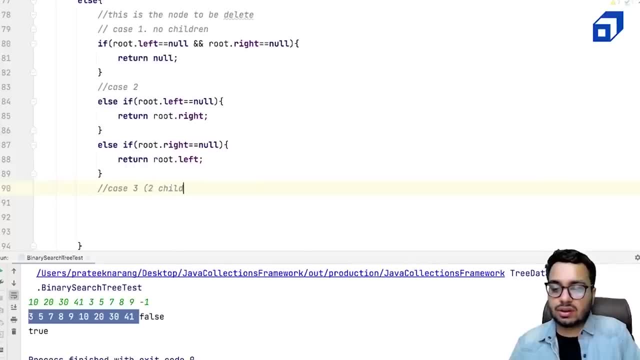 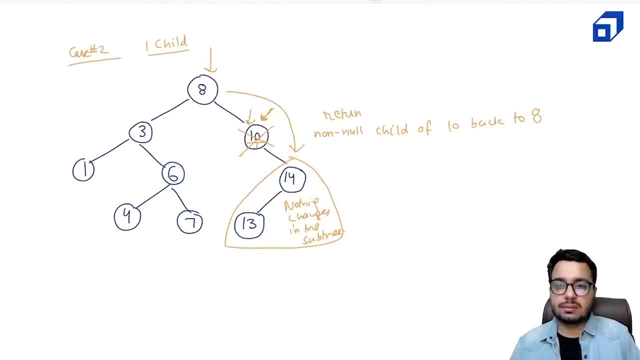 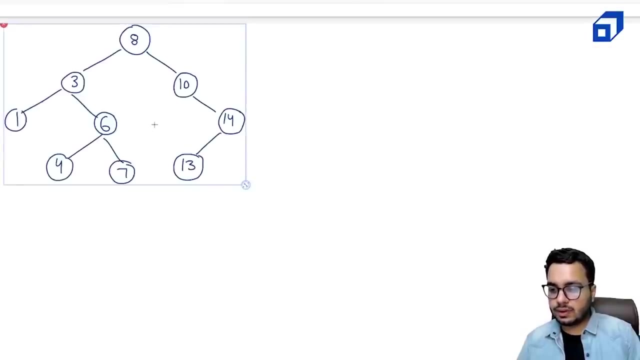 that means a node has two children. we need to delete a node with two children. so let us discuss how this case 3 will work. so let us discuss case number 3. this is the tree, and suppose i want to delete a node which has two children, so it can be anywhere. 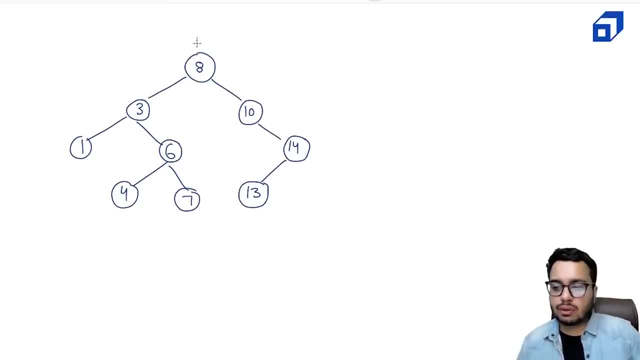 it can be any node which has two children. so let's say i want to delete it right now. if i directly delete it, this tree will be split into two parts, which i don't want. this tree should remain same, right, this tree should remain same. so what i can do is i need a way so that i do not disturb the. 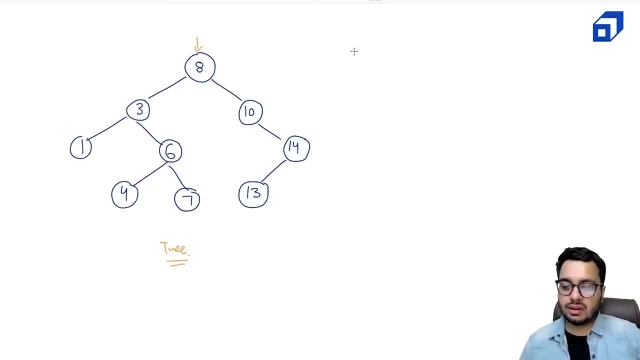 tree structure. a lot right. if i talk about in order to reversal of this tree, i get one, three, four, six, seven, eight, ten, uh, thirteen and fourteen, right. so this is what i get right. if i want to delete eight, the new root node should be either seven, okay, or it should be either. 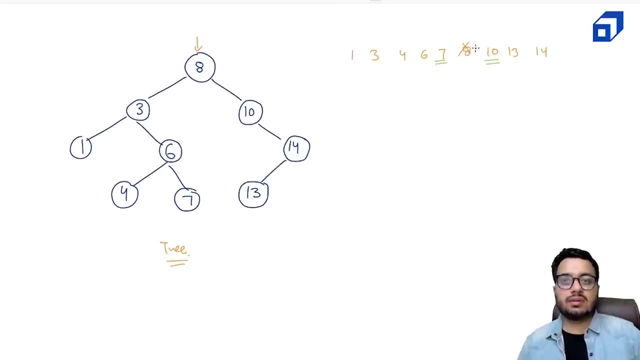 ten, so one of them should become the replacement of this node. right now how i'm going to do it so it can be the largest node in the left sub tree. that is option number one. right option one is: make the largest in the left sub tree as the root node. right option number two is: 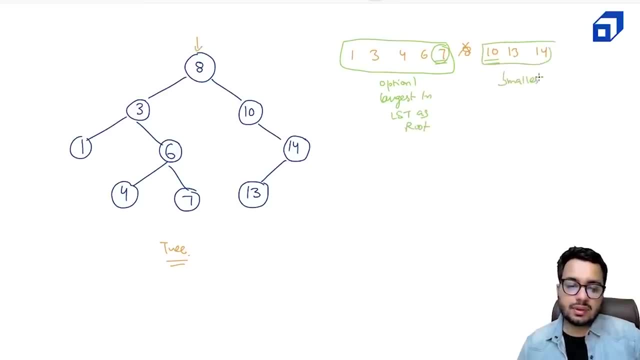 make the smallest in the right sub tree as the root node in the right sub tree as the root, so you can use any of these options. okay, so if i show you, if i make smallest in the largest in the left sub tree as the root node, in that case seven will be. 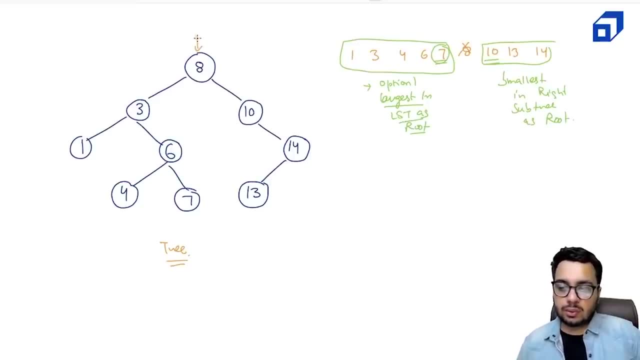 the root node. okay, now, how it is done. let us see now. suppose you have reached the node which you want to delete and it has two children, right, so you will. okay, i'm going to find out the largest node in the left tree. so how do you find the largest node in the left tree? you start from this: 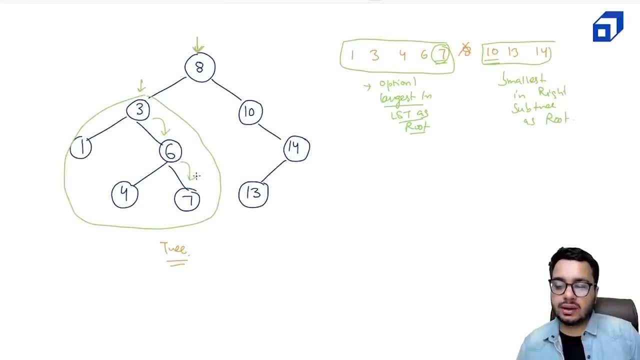 node and you try to keep on going right. you always go right and eventually, when you stop here because the right of this node is null, so you have to stop at this node, and you will have to say, okay, this is the largest node and i will put this node here right now. putting means i will copy the data, so you will copy. 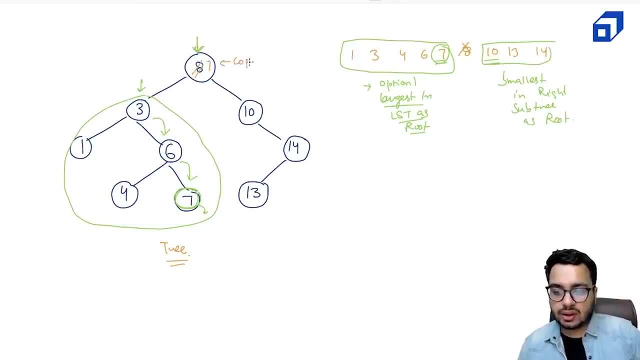 the data 7 here, so this data is copied, right. i'm not changing the node structure, i'm just copying the data. so 7 is copied here right now. if you copy 7 here, what you will observe? you will observe this: 7 is duplicate, right, this is present two times. this is duplicate right now. what i can do is 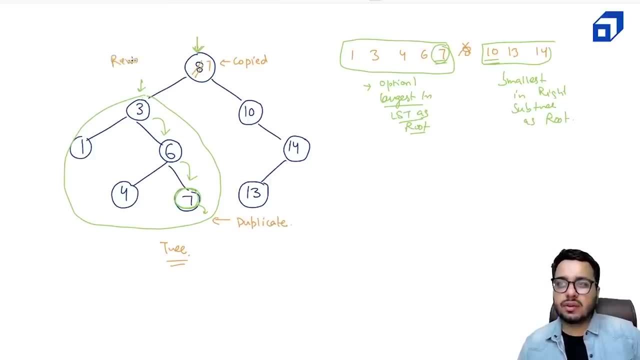 can i make a recursive call to remove 7 from this subtree, from this particular subtree? can? can it be done? the answer is yes. if i remove 7 from this tree, then my work will be done right now. if you look carefully now, 7 will be a node which has either: 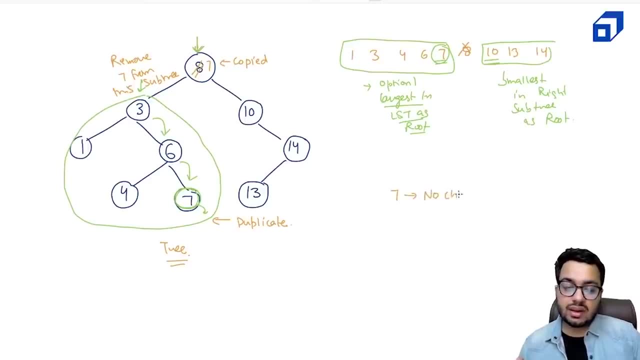 okay. it will have either no children, for example in this case, or if it is the largest node, it will not have any right child right. so 7 can have a left child can have a left subtree right. 7 can have a left subtree right. that means if i'm recursively removing 7 from this tree, 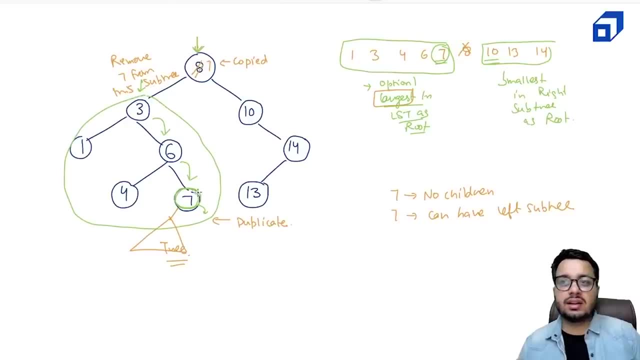 two. two things can happen. 7 does not have any child, so it will fall back to case number one, that a node with no children, so it can be easily removed. i can return a null here, right. or 7 has a left subtree. in that case that subtree can be returned here and it will be correct to attach it. 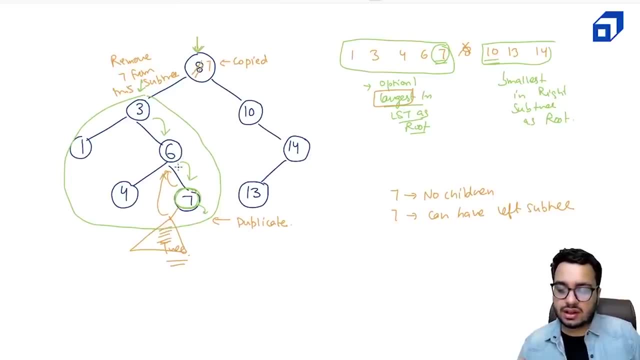 why? because all these nodes they are greater than 6 but they are less than 7.. they can be attached directly in the right of 6 right. so 7 still can be removed. so this: if this is the case, it will handled by case number one. if this is the case, it will be handled by case number two that node has. 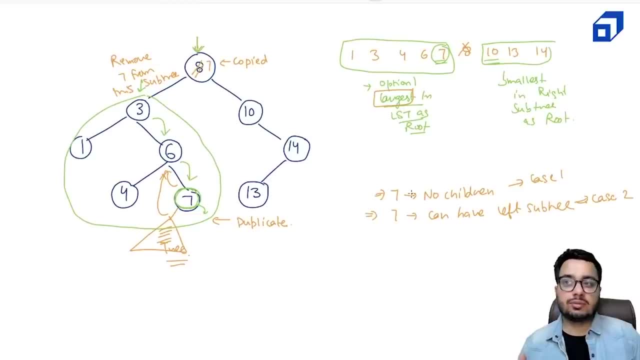 one left child or right child, but it it cannot have both. okay. so you can see, largest node can never have a right child, okay. similarly, the smallest node can never have a left child because it is a bst it. if it is a has a left child, then it is not the smallest right. so we 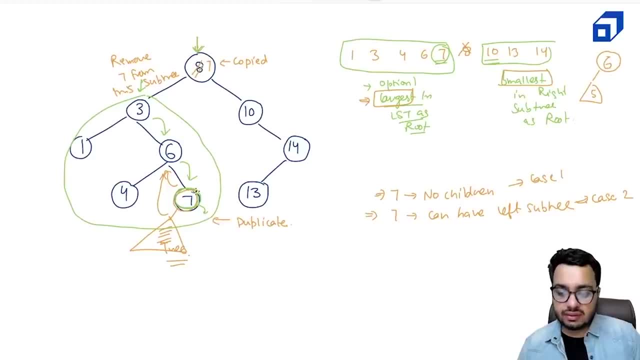 are going right until we don't find anything on the right. so 7 can be replaced. okay, so that means in this case, 7 is not having any left child. i want to remove this node. i will make a recursive call on this left subtree to remove 7. so 7 will be removed and this is how the tree structure would. 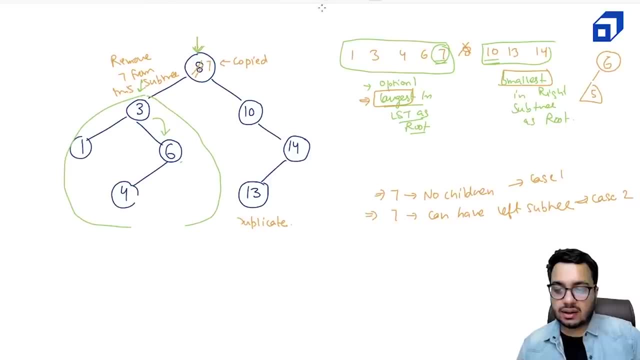 look like right, so i hope you are able to understand. new tree would look like this. it will be 7, 3, 1, 6, 4, and here i have 10, 14 and 13.. this is how the new tree would look like. if you talk about the inordered reversal, it will be 1, 3, 4, 6. 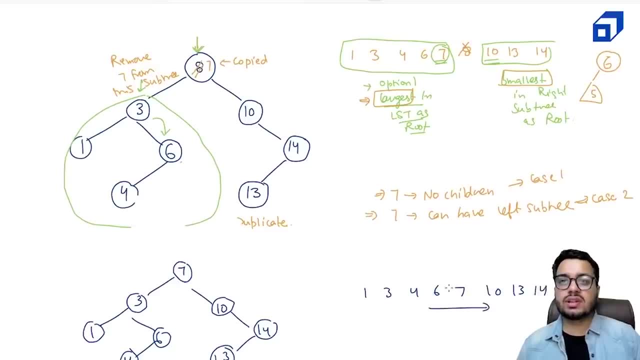 7, 10, 13, 14.. is it correct? of course it is correct. is 8 removed? yes, it is removed from this reversal. right now, let us locate in into the code how this can be actually done, right? so i have case 3, where 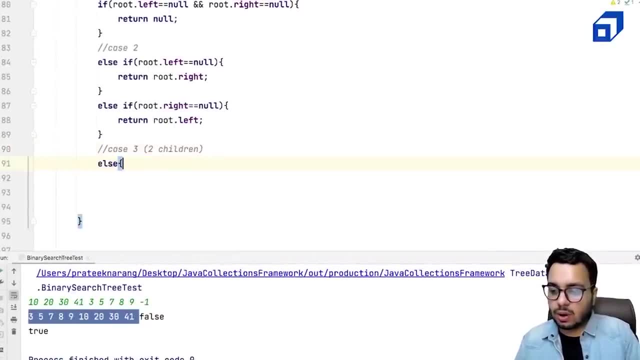 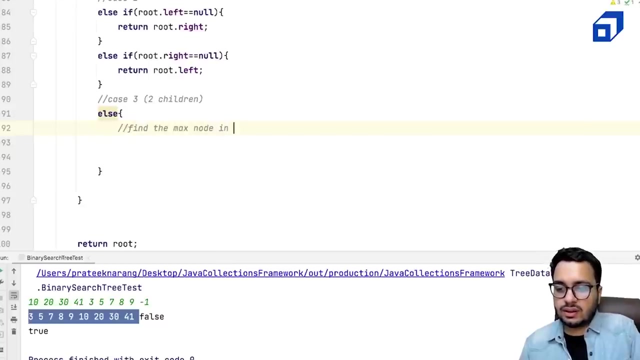 the node has two children, so this can be handled by the else block. so what we need to do we need to do is we need to find the max node in the left subtree. okay, so i can. okay, i will take a temp variable node: temp. this is equal to root dot left. so i can say: while temp dot right is not equal to. 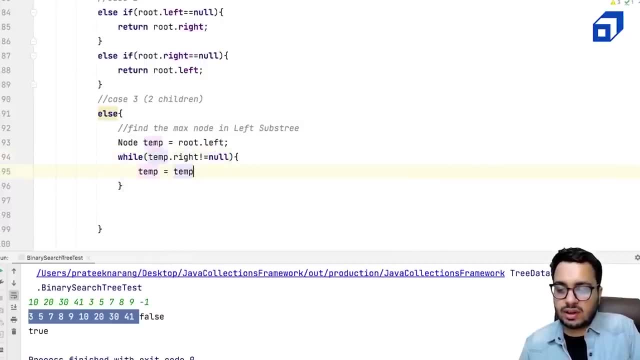 null. so i will move this temp towards right. so temp equal to m dot, right? so if you are confused, what we are doing now, suppose this is the tree. let's say i have five, six, seven and i have some nodes here as well. right, i'm saying: okay, i want. 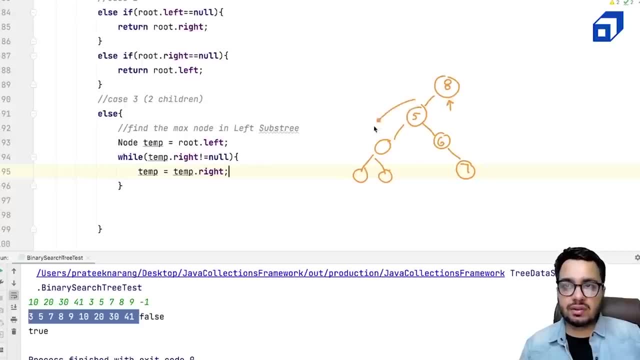 to find the largest in the left subtree. so i start a temp here. so temp dot right is not null. so temp goes here again. temp dot right is not null. temp goes here now. temp dot right is null. so what, what do i do? i stop. so even if it has a left subtree, temp will stop at seven right. 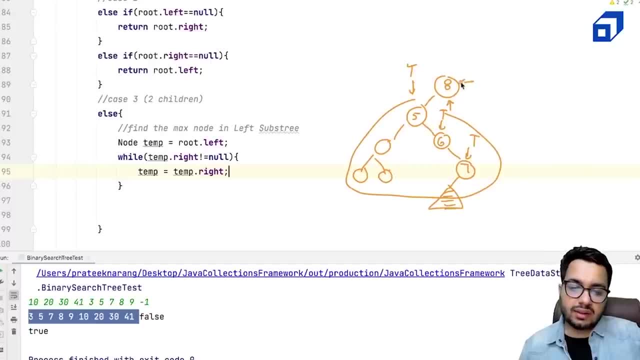 okay, so we found out the node. now what i need to do. i need to replace the data here so i can say: okay, fine, root dot data will be replaced by temp dot data, the data of the temp. i copy this 7 here right now what i need to do. i need to recursively delete the node 7 from the left subtree. can i call? 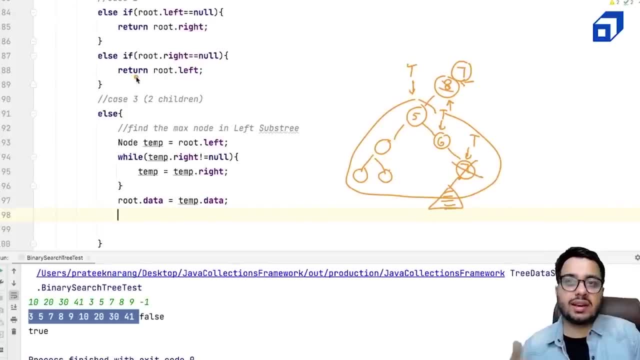 the remove function. yes, because it will either lead to case 2 or case 1, which i have handled right, so i can say: okay, fine, now my function is to remove the node with temp dot data from the left subtree so i can say: remove root dot left. the node is called temp dot data. i'm not, i don't want to. 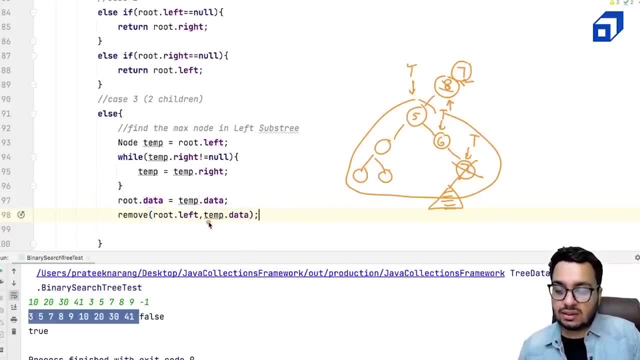 remove 8 now. i want to remove 7 now, so that is why the value is not key, but it is temp dot data. but after removing this, something will be updated right. so i am standing here, i'm making a function call on this left subtree, so this left subtree will tell me the updated uh address of the left. 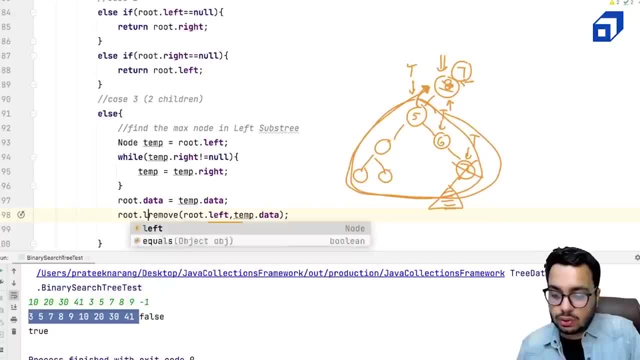 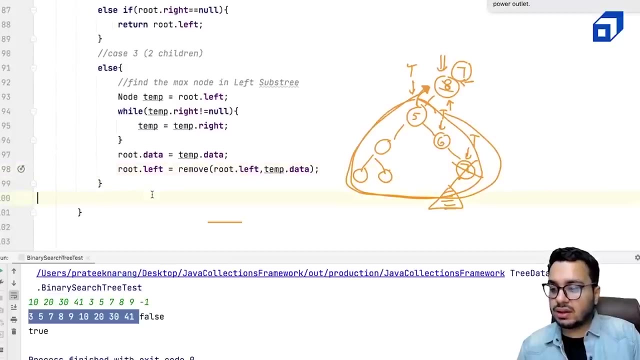 subtree or the updated reference. so i have to say: at root dot left, this is equal to remove right. so whatever uh is the tree after removing, please tell me it's a root dot left, this is equal to remove right. so once it is done, what should i do? i will simply return the address of the root. 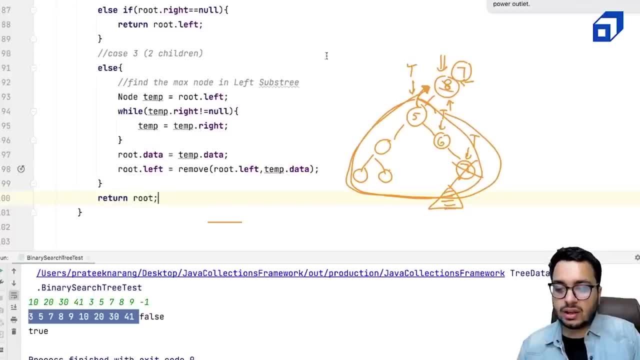 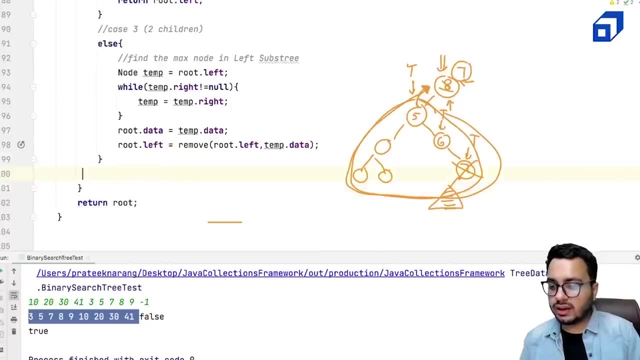 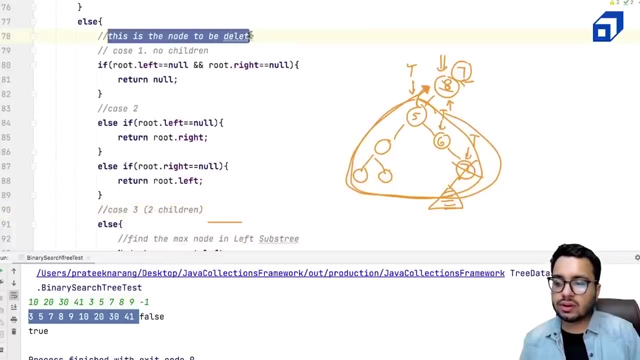 so this is something we will do, right, so i'll tell you quickly what is happening here, right? okay, return root: we have already done at the end, so, no, no need to do it here. so we have three cases: right, when we are at the node which is matching the given key that we need to delete. okay, we have. 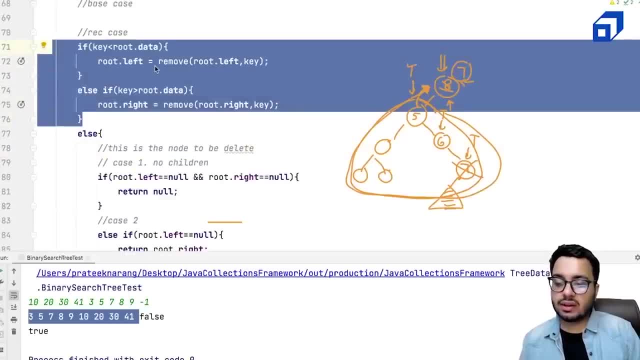 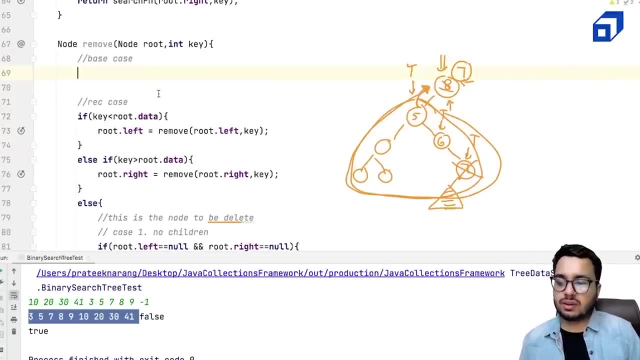 two recursive cases which are, uh, basically helping us to reach a node. okay, so there will be a base case also, right? the base case would be that if node is not present, so if node is not present, we might end up at the end of the node, and if node is not present, we might end up at the end of the node. 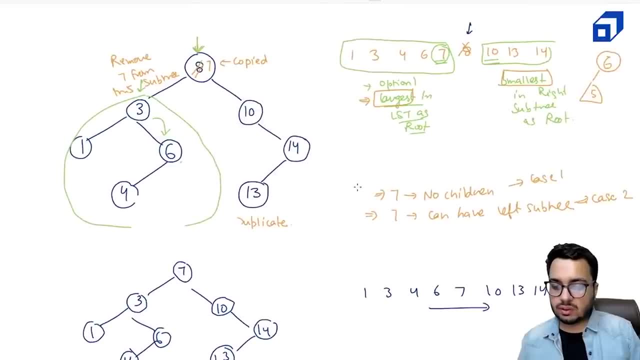 a value that is null, right? so i will show you what will be the base case. now, suppose i want to delete uh. let's say i want to delete uh 41 right now. i start with, let's say, 7. i say, okay, 41 is greater. i go to 10, it is greater, i go to 14.. now it says it must be on the right, so i go here. 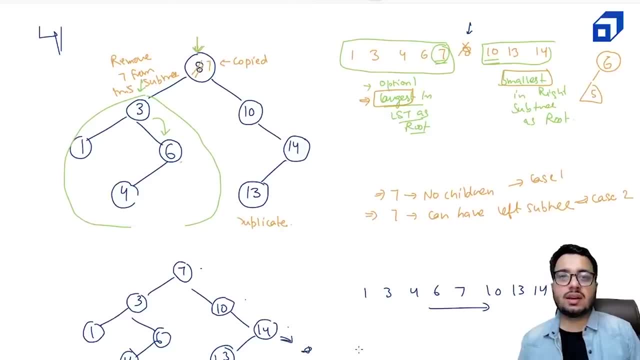 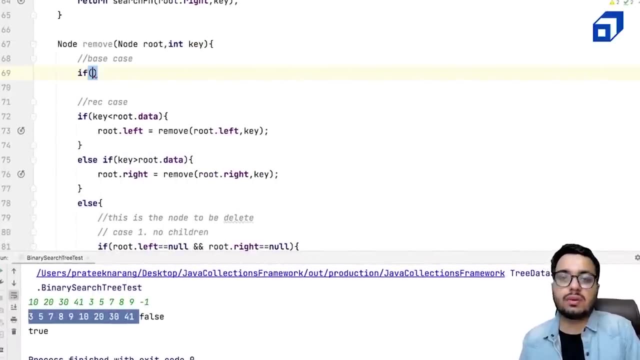 so basically, the right of 14 is null. if i reach a value that is null, that means the node is not present. so it is just like the search method where we were returning to the node false. here we will not do anything. so if root becomes null at a certain point, right, so i can. 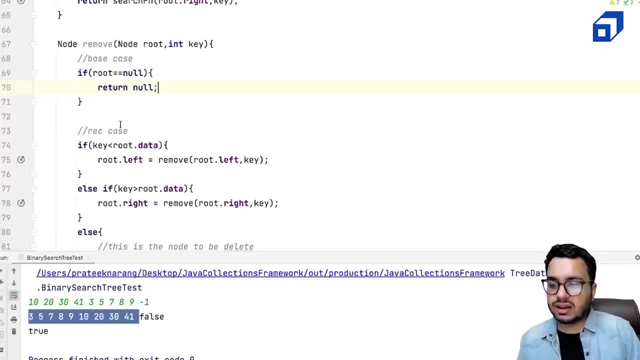 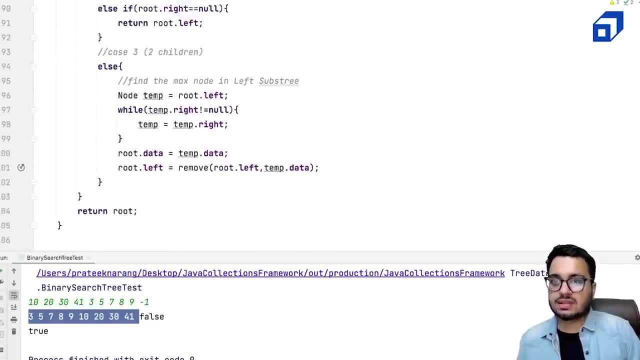 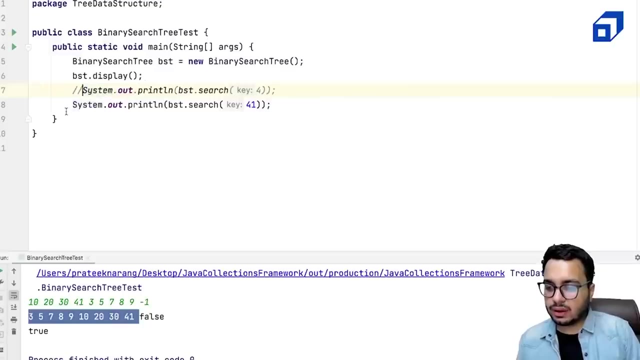 say, okay, i'm also going to return null, right? so this, i think, makes the code complete. now let us test our functionality by going to binary search tree test file. okay, so, okay, i was all doing searching earlier. now i can say, okay, uh, i will remove something and then i will display the tree. 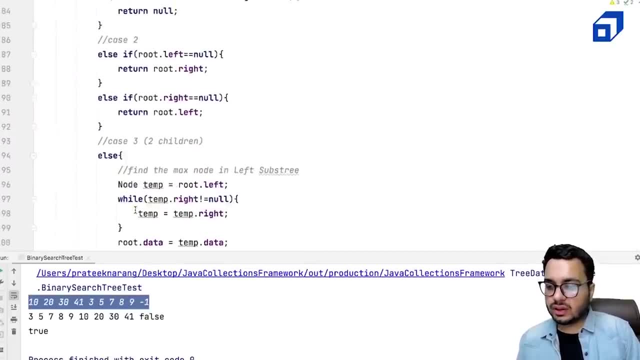 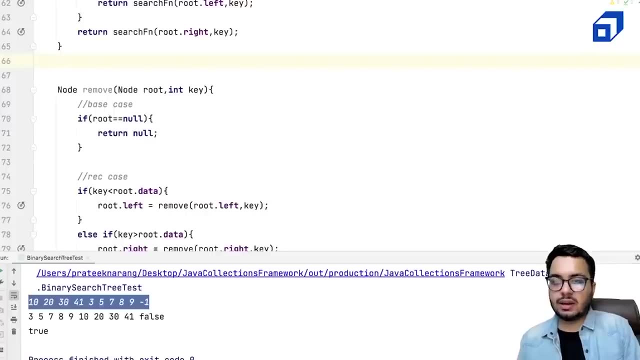 okay. one more thing we have to do is we cannot call the remove function directly because we have to supply the value of root, so we will create a wrapper function. let's say, node remove key let's or let's avoid remove key. this is the method, and here we will only accept the key right and from. 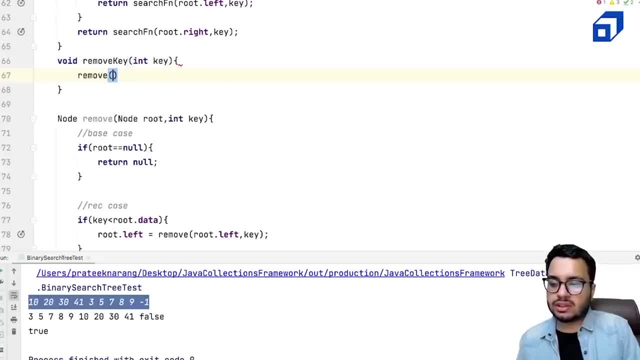 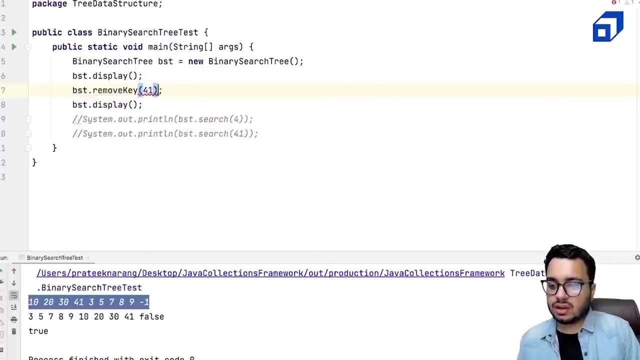 here we will say: okay, let us call the remove function, where we will give the actual root and the key here. so now from binary search tree test, we can say: okay, pst dot, remove key. and here i can give some key, let's say 41. now, if this is present, it will get removed. so i will give this value. 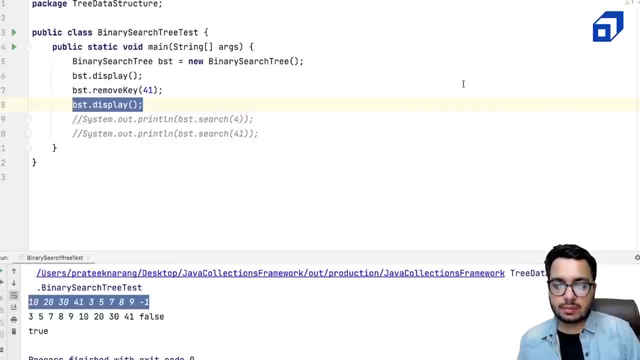 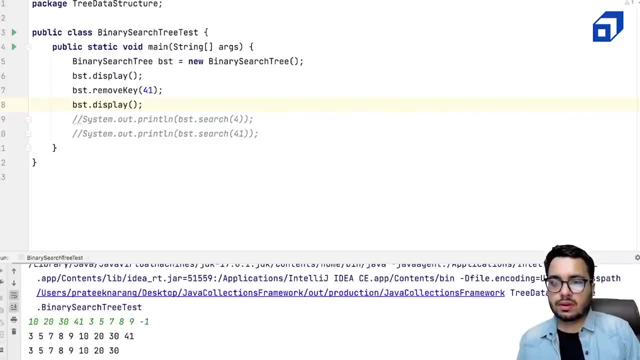 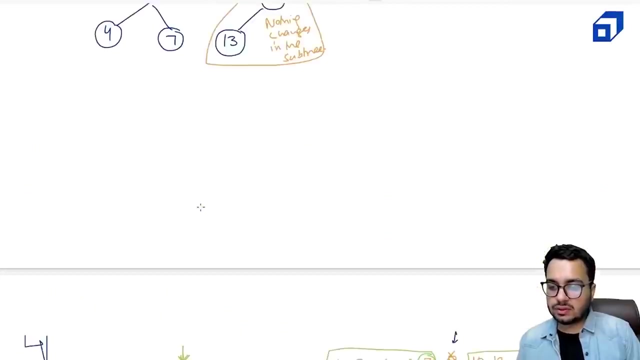 and let's say, i want to display this tree, so i have given this particular input, so this is the tree. before printing, before removing. then i removed 41 and this is the tree. right, we can experiment with this tree as well. that we had for this tree. uh, the input was: 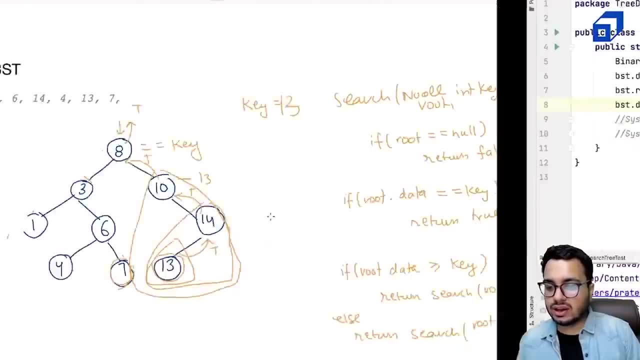 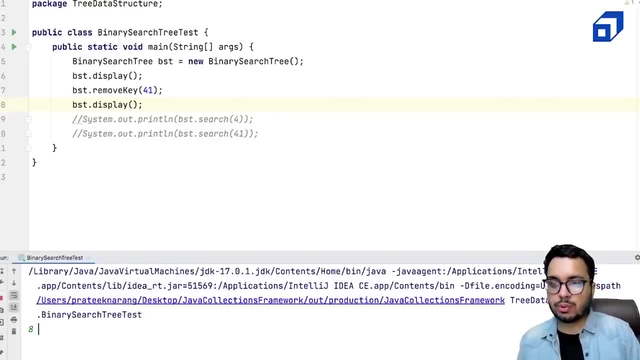 8, 3, 10, 1, 6, 14, 4, 13 and 7.. let us try to play with this tree as well, so i will quickly type the input. so this is the tree from the diagram, and from this tree, let's say i: 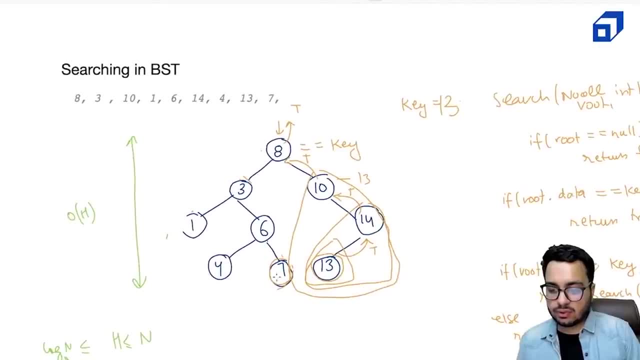 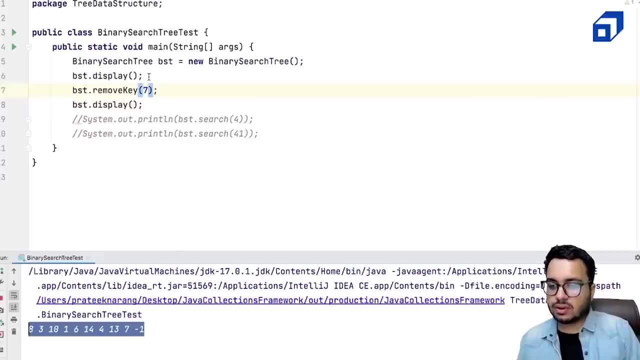 want to go with case 1, where i want to remove, let's say, 7.. i will give input as it says 7 or i can ask the user for the node to delete. okay, that that is also doable. i will just rerun this code and i want to delete 7 from this tree. 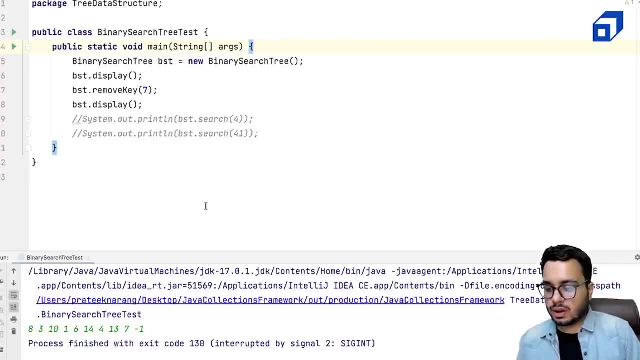 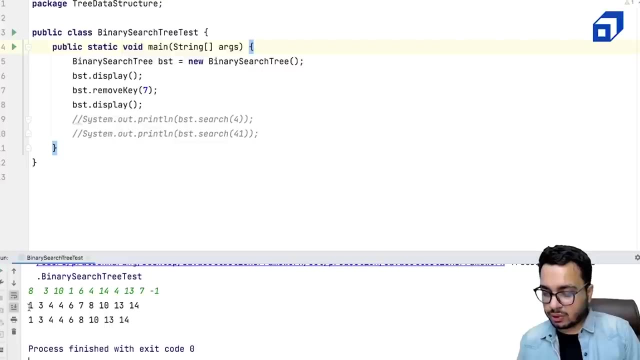 let's rerun it, okay. so let's say sorry, this is the wrong input we have given. all right, so this is the input we have given. and now from this input i have removed seven. so you can see the seven has been removed from this tree, right? so that means case one. 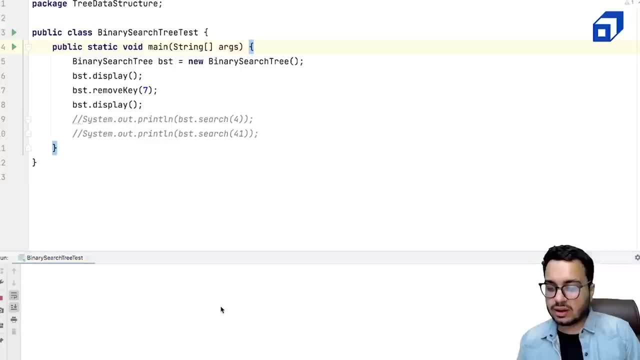 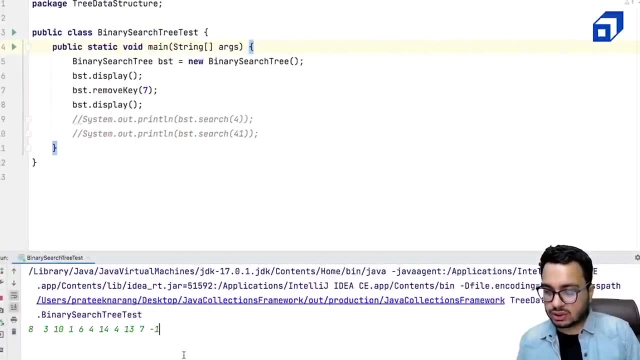 is working fine. now let us rerun this once again. and let us discuss case two, where i want to remove, let's say, 10.. so the same input goes, but i have to remove 10, so i have to rerun this code once again. i will stop it and i will rerun it. 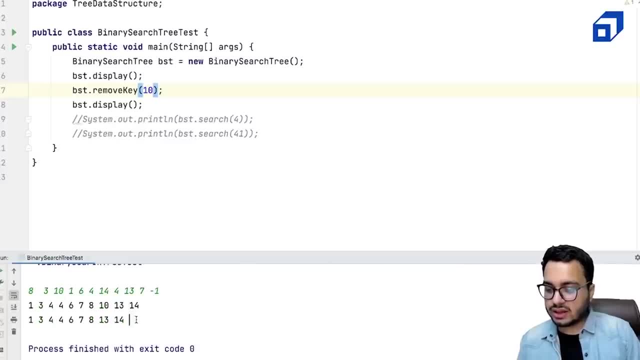 let's say i'm removing 10.. now from this code you can see 10 has been removed. that means it is working fine for case two as well case three. let's say i want to remove it, so i want to remove eight. i will rerun this code. 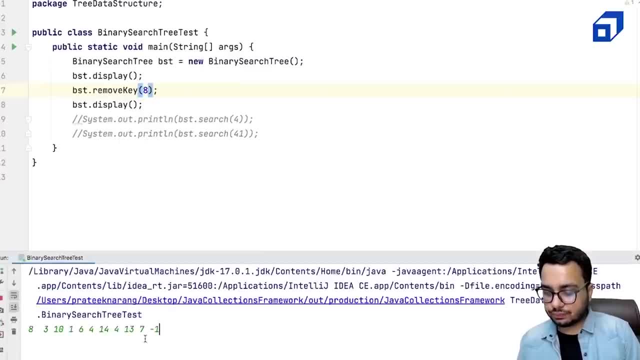 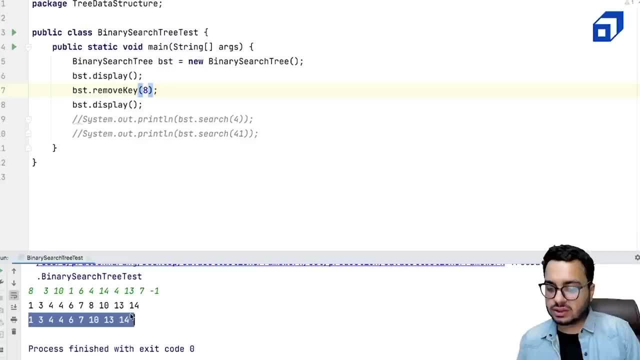 and let's see now, after removing it, you can see this is the in order traversal of the tree, which looks correct. okay, so in this code i have two fours, which is okay, but you can see eight is removed and eight was the root node of the tree. right, that means it is working fine for all the 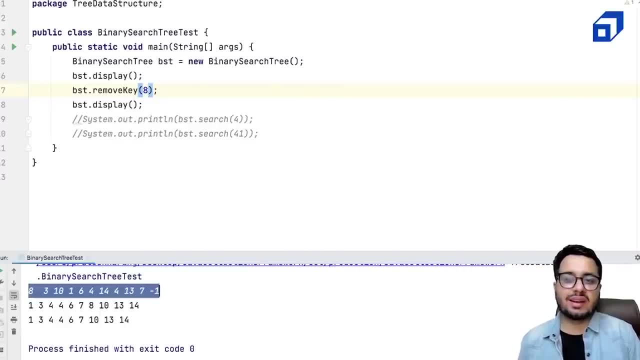 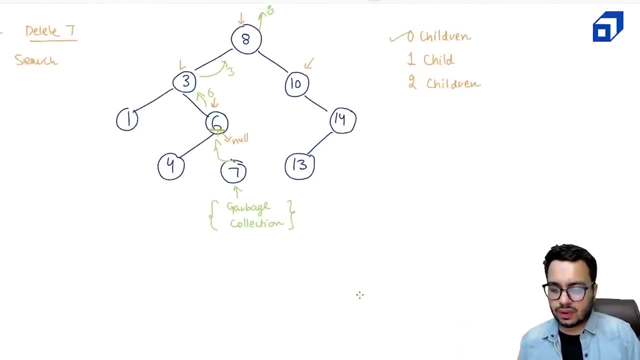 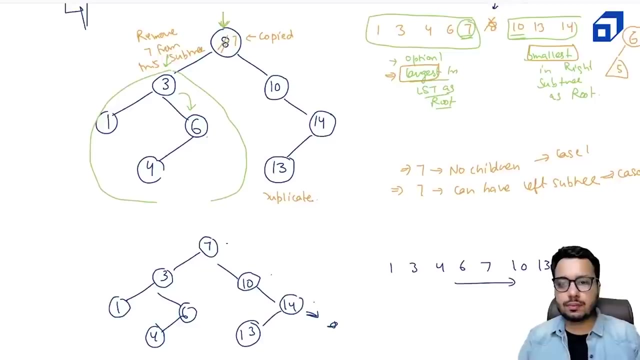 three cases. that's about how you remove a node from a binary search tree. okay, if you want a small dry run, we can do it once again. uh, let's say, now you're removing it, so as i discussed. so what are you doing? uh, you had seven here, right? so you say, okay, i want to remove eight, so i will. 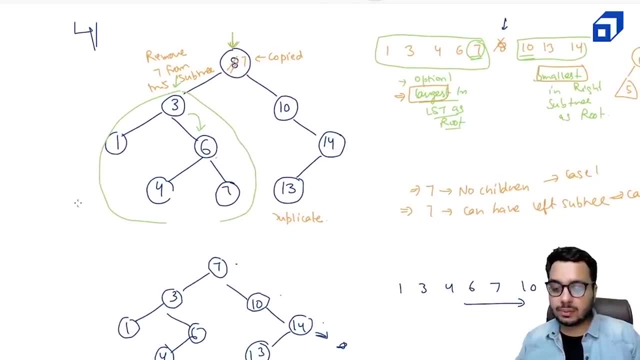 i will go in my right subtree, in the left subtree and i will try to iteratively find the largest node. so it says: okay, this is okay, temp is here. temp goes here right is not null, temp goes here right then as a root dot data. this is the current root where i want to delete. so i say root dot data. 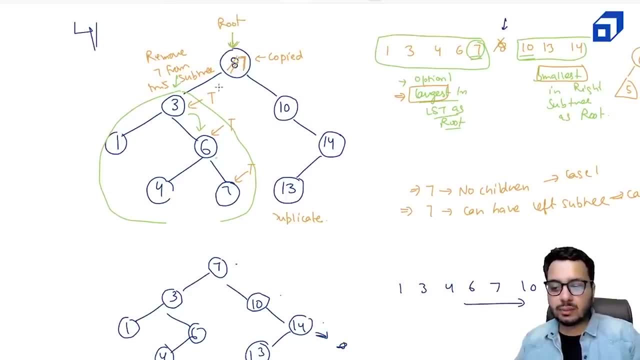 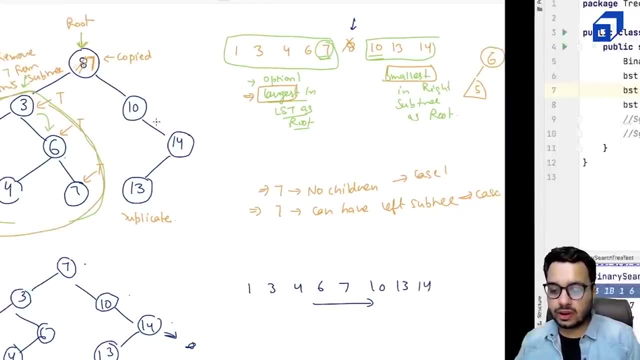 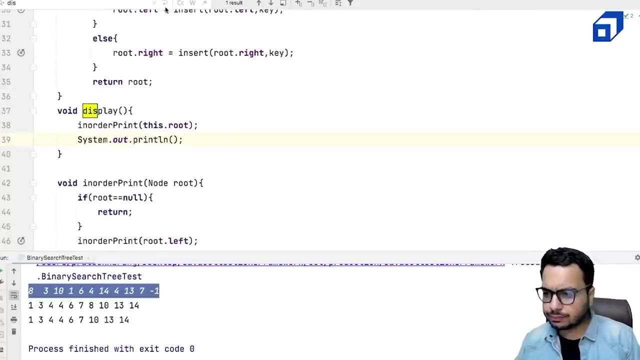 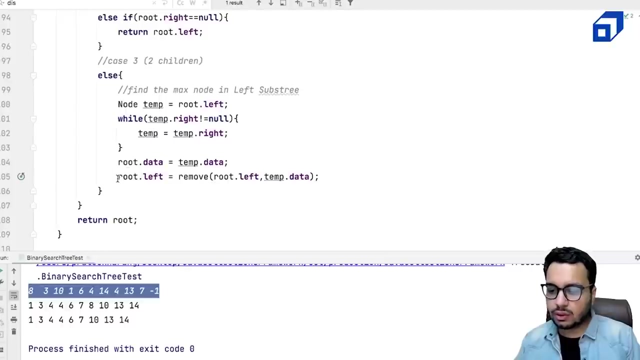 this is equal to temp dot data. so seven is copied here. then i make a recursive call on this is okay. root dot left, this is equal to remove. okay. uh, if i talk about in the code, i'm making this uh change here, uh, so i show you this is the remove function. so i'm saying: root dot left, this is equal to remove root. 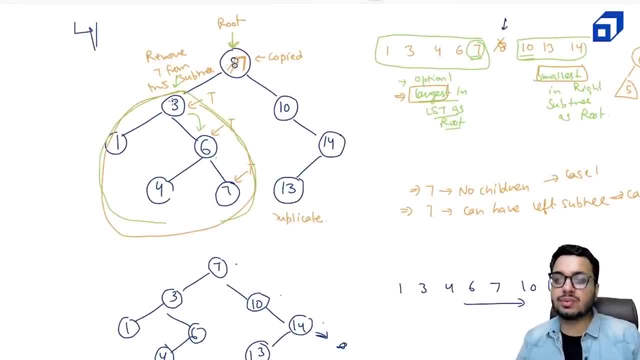 dot left and temp dot data. so i'm not saying remove it, i'm saying remove seven from this tree. right, because seven is now duplicate. so i guess i can say root dot left should point to a new tree in which seven is removed. so now i say seven, i want to remove seven from here. 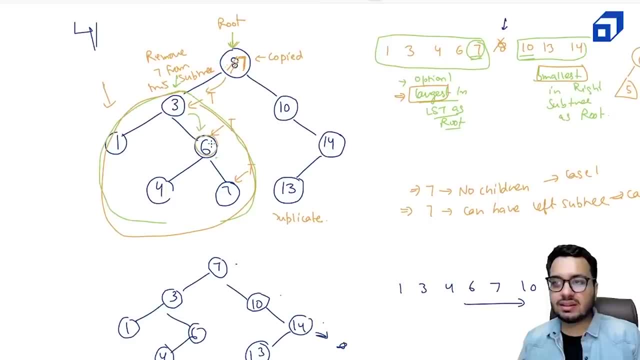 so seven is greater than three, i go here. seven is greater than six, i go here, so i reach finally seven. if i reach seven, i say return null. now six right is pointing to null and as a return root. so six is being returned. so three refers to six. this node is gone and from three as a return root. so 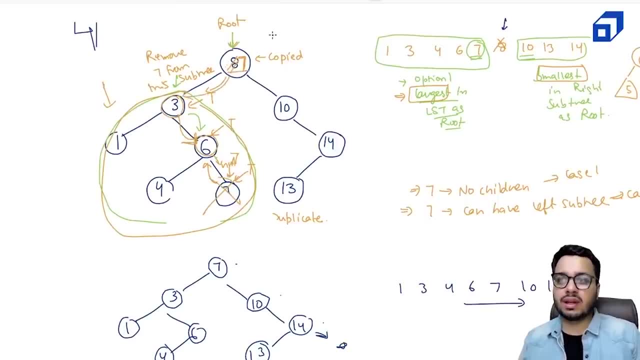 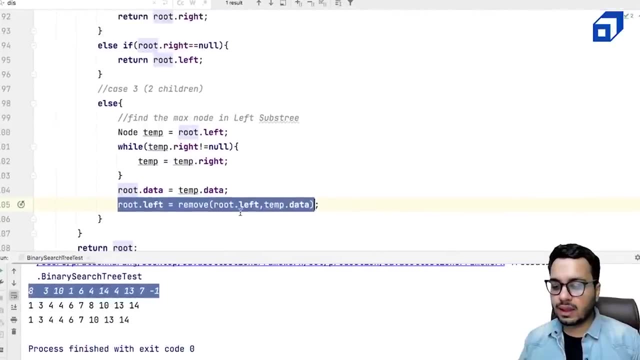 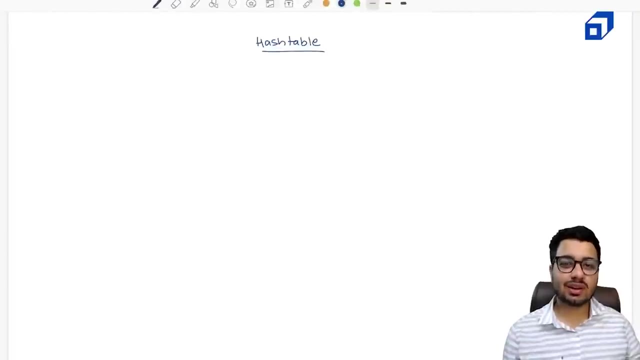 seven now refers to this three. so this is what is happening when i am doing a recursive call for deleting seven from this tree. i hope all those who had a doubt now it is clear and this is how removal in bst works. let us to understand what is a hash table and how it works. okay, so you might be already using. 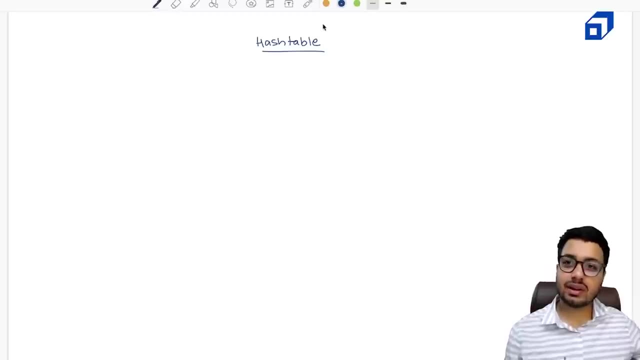 hash table a lot of times and it is known by different names in different languages. for example, in java it is called as hash map. in python it is called as dictionary. in c plus plus it is called as unordered map. right, so there are different names, but the internals of the data structure they are same in different languages. okay, so hash map. 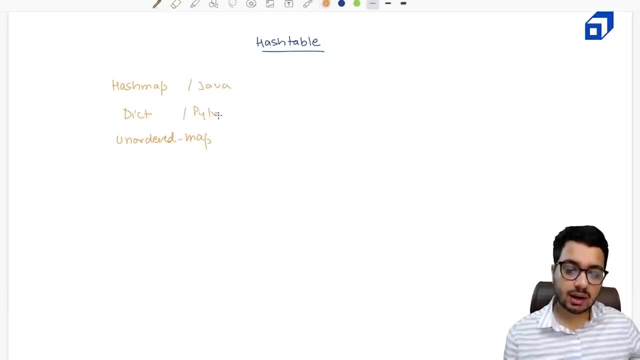 in java dictionary, in python and unordered map, in c plus plus and in, of course, in other languages as well. you have this data structure that is available, right? so the reason why we are going to study this data structure is it is very, very powerful, right, and it is used a lot, right, it is used a lot right. 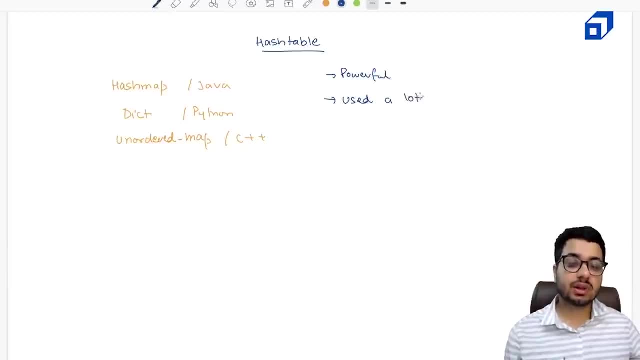 so when i'm saying it is used a lot, so not just business logic. so when you're dealing with your problem solving, when you're building real software, you would often require a hash map to store data in the form of key value pairs. okay, so it stores information. 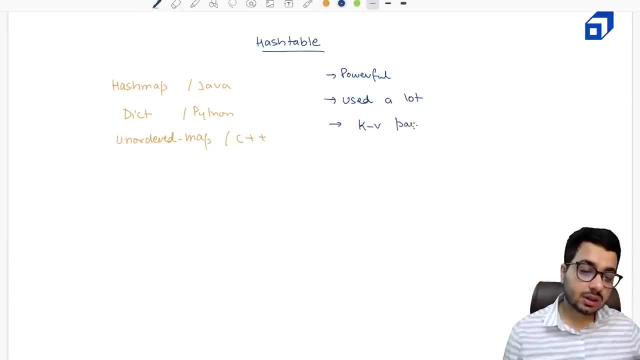 in the form of key and the value pairs. but not just that. we can also store key value pairs in the form of a list right. why it is powerful? because it allows us to do operations like insertion: i want to insert a key value pair, i want to look up for a particular key right and maybe i want to delete. 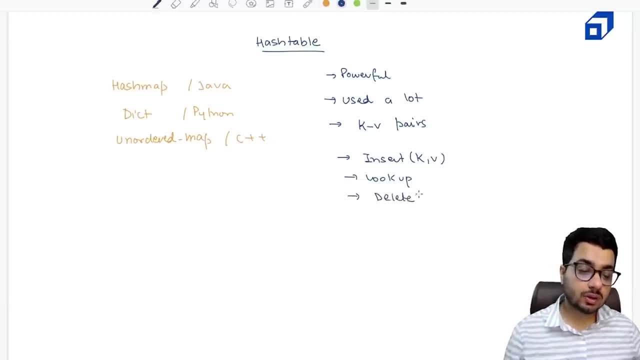 a particular key right, a key value pair. so i can just give: okay, this is the key, delete the corresponding value and the key. so delete the key value pair. given the key, lookup means the search right. i want to search for a particular key, if it is present or not, and if it is present, what is the 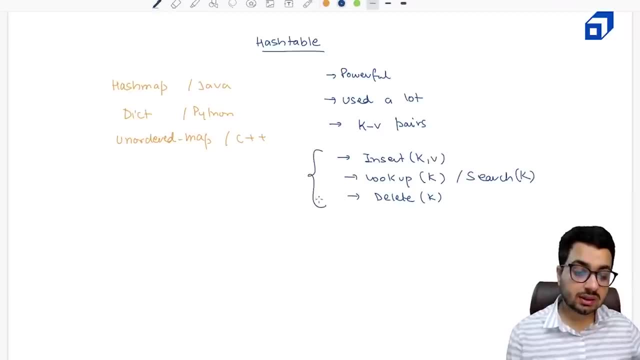 associated value with that particular key right. so these are the three important operations associated with the hash table right. and the good thing about these operations is why, uh, this is so popular or why this is so powerful? because these operations are performed on an average, in order one time. so order one on average, that means most of the times. 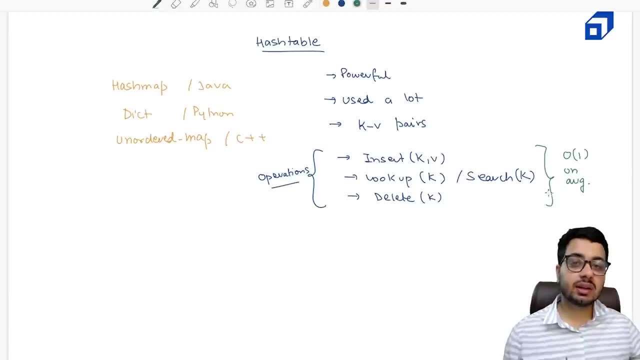 these operations will be performed in constant time. okay, so we will discuss the scenario when they are not performed in constant time. but you can say, okay, most of the practical scenarios, these operations would be performed in order one time by the hash table. right now let us discuss where this can be used. okay, so i discussed that it stores information in the. 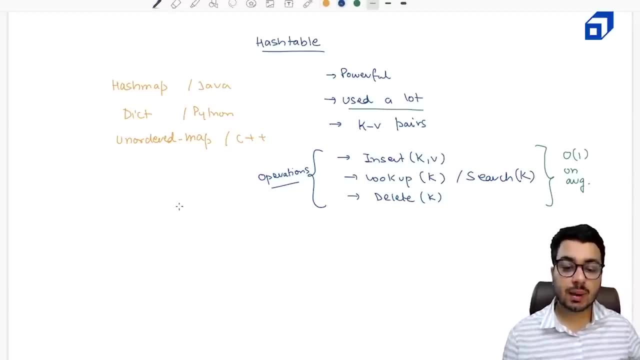 form of key value pairs. okay, suppose you are building a application for a restaurant and user item. a user of wants to order particular item, right. so user says, okay, i want to uh check if dosa is available and what is the price of the dosa. the restaurant owner might instantly: 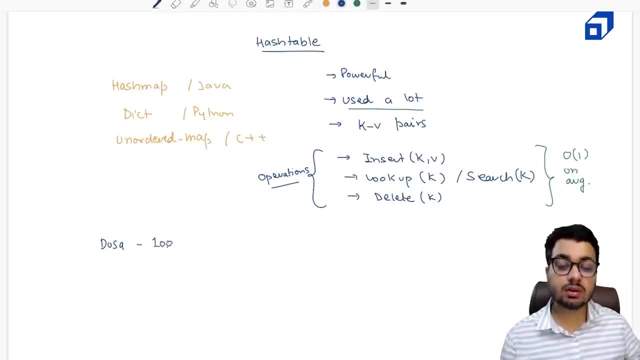 reply that, okay, the cost of the dosa is under right. so, given this key, you are telling the value in order one time. okay, maybe i want to order some uh coke. maybe this is priced at 50. maybe i want to order some noodles- right, this is cost costing maybe 70, right? so what can happen with? 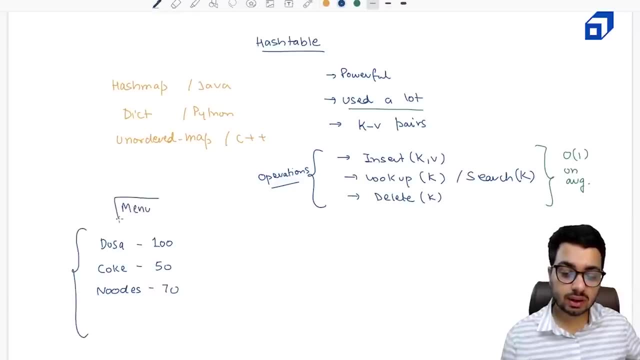 this menu. what are the operations we might be doing on a restaurant menu? right? so if we are building an online menu, we might be adding a key value pair. okay, a new item has been added. maybe a pizza has been added, so you will supply. okay, pizza has been added and it is. 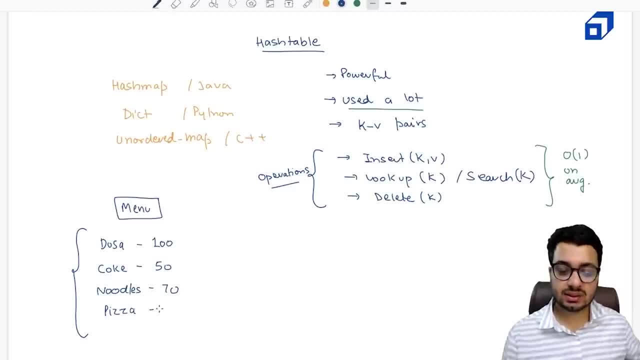 associated with some object, or in this case the. that object is nothing but an integer object only, right. so the cost of pizza is: is 250, right? so i can say i want to insert a new key value pair. that is doable. second is, i can look up now i can ask what is the price of the coke, so the 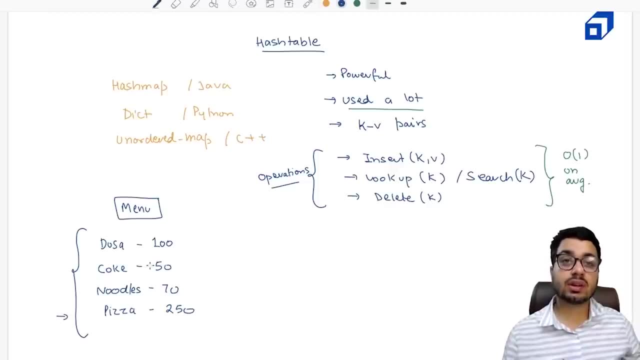 hash map will tell me in order one time: yes, the price of the coke is 50 rupees, then i can delete. i can say, okay, coke is not in the stock, delete coke. so it will be deleted from the table. so these are the three operations that we are going to be doing, in order one time. so first of all i want to 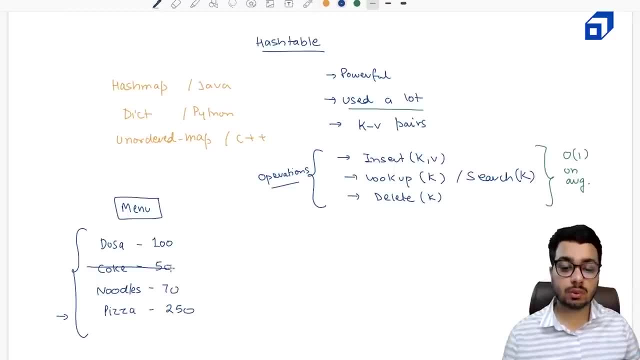 show you the operations that our hash table is going to support right now. of course, we saw that this can be used in business logic. when you are building an application, a hash map can be a useful data structure to use right, because it provides fast lookups, fast inserts and fast delete. 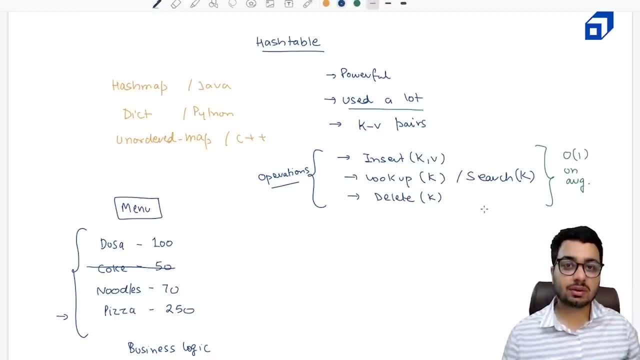 operations as well, right. but one major application is also in the language runtime, right? so whenever you are working with a language like java or c plus plus, you are going to be able to use this. you know, uh, you create certain variables. you say, create certain classes, so you say, okay, i am going. 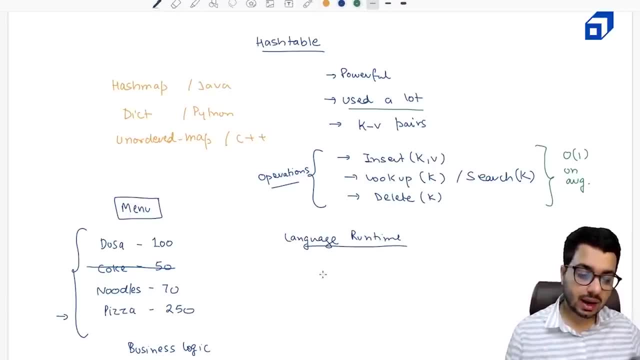 to create a variable uh index and i'm going to say this is 10, right, then it's okay. into y, this is 20, right. so what happened is how these uh variables are stored. so these variables are actually stored in the memory right. x is a bucket that is storing 10, y is a bucket that is storing 20, right. but when 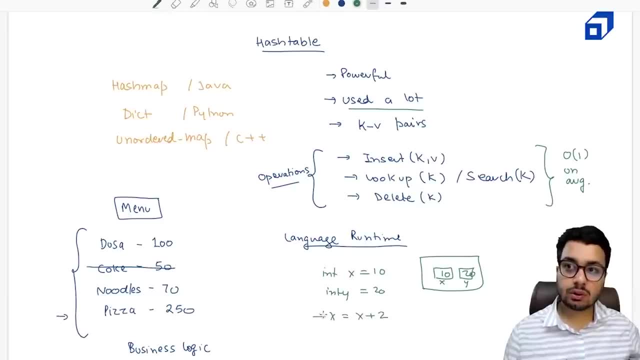 you want to say: okay, x is equal to x plus 2, right? so your compiler needs to know where is this x located so that it can go to that location and change that bucket. now suppose this bucket is at some address abc, right? let's say abc20, right? this is some address written in a hexadecimal. 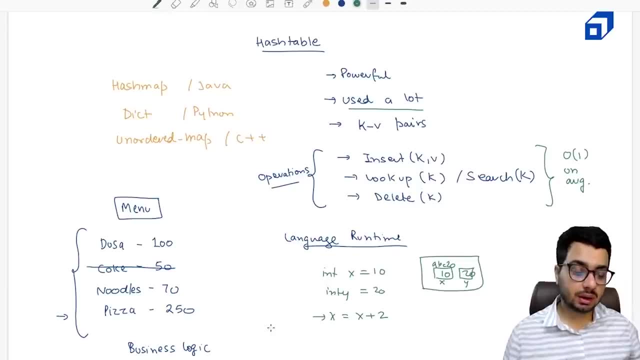 format. right, so the compiler maintains a symbol table for all the variables and the classes that you are going to, all the objects that you are going to create. so there is a symbol table, right, right, so this symbol table will tell that, okay, x is a bucket which is present at this location- abc20. 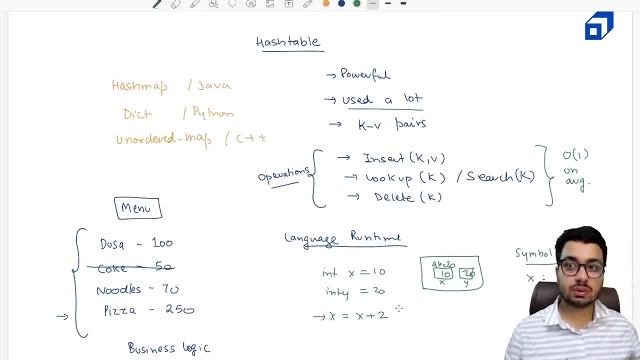 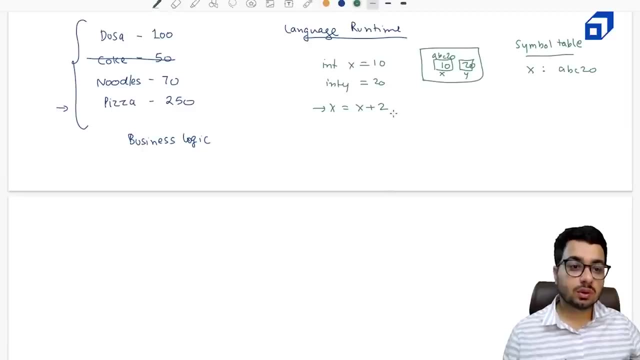 right now. when you do this operation, x is equal to x plus 2.. so i'll just scroll up a little bit. when you're doing this operation, x is equal to x plus 2, so the compiler will look at the symbol table. where is x located, it will go to that location and it will make the change right. 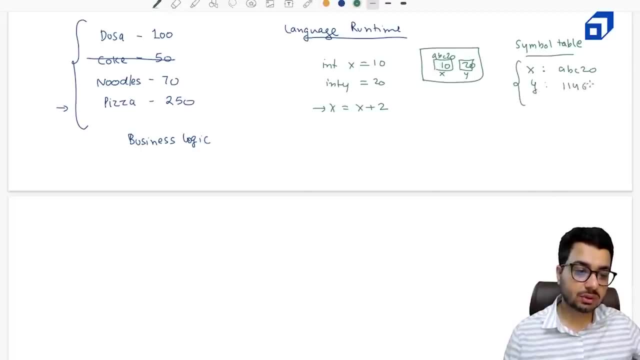 similarly, y is located at some location, maybe one one four six two right and maybe right. so one one four six two. this is some other location for y, so y will. it will again look up at the symbol table where is y located. it will go to this location and it will make the 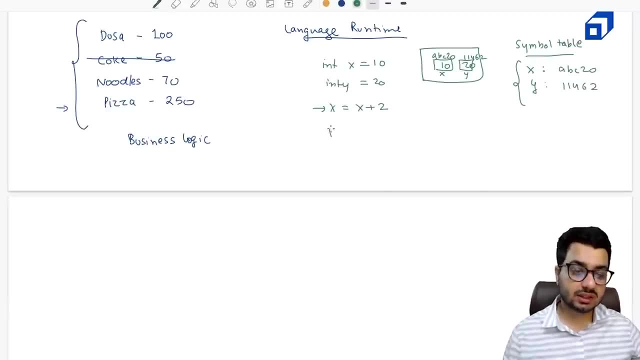 change in the wire right. similarly, if you create some objects, let's say dog d, this is equal to new dog. so this dog object is created at some location in the heap right. so similarly, your d will be mapped with some address. right now, what is your symbol table? a symbol table is also of a form of a. 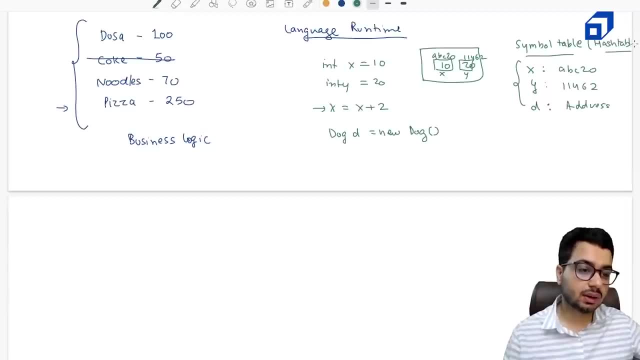 hash table right. it is also a form of a hash table right that your compiler is maintaining and it is called as symbol table right. similarly, when you have classes and objects right, so you say, okay, i want to create a new class called dog. dog has certain properties, right, let's say it has. 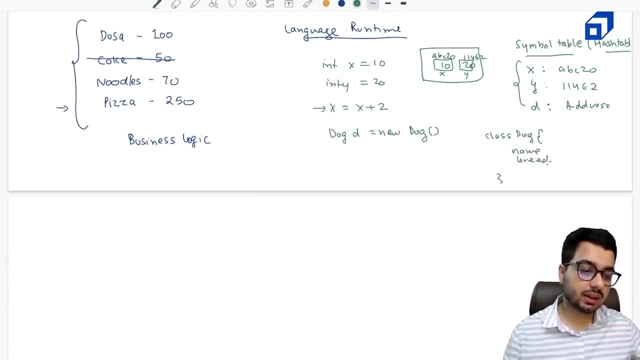 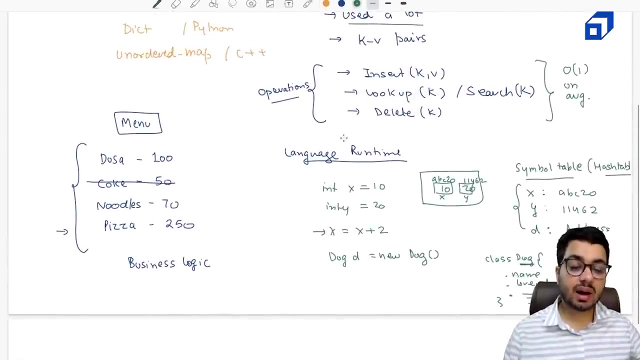 a certain name, it has a certain breed, it has a certain method, right? so what is happening? so you are also, you are able to map dog with various attributes and various methods, right? so all these features- right, they are powered by the language runtime, and language runtime might be- is actually using hash table internally, so that 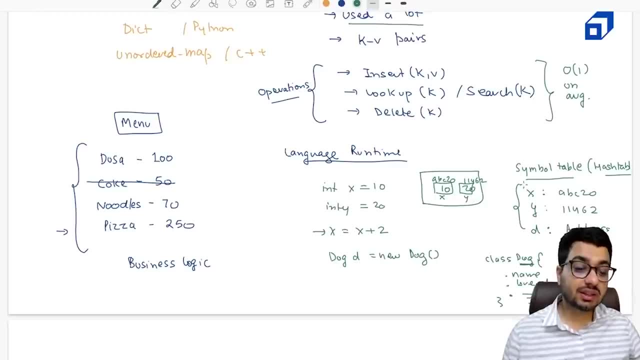 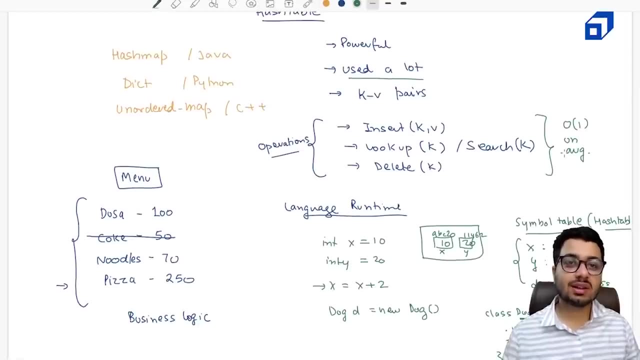 you can do lookups very, very fast. okay, if this functionality is slow, your language will become slow. so that is another application of hash table. it is used in the internals of the language, so i hope you got a good introduction to this video. thank you very much for watching and, if you like, the content. please like, share and subscribe and leave a comment down below also, comment below and, if you have any other, whenever you wish to add any more videos, make sure to leave a comment, nor comment down below, as it is very much appreciated. so i hope you have a good introduction. very, very. 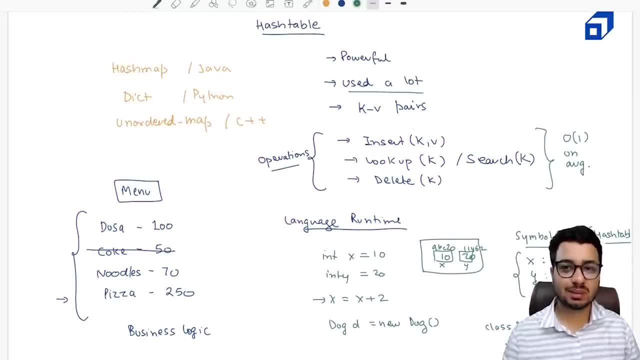 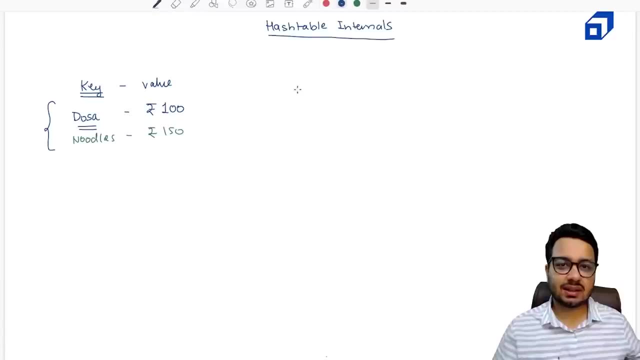 introduction about hash table. now we will jump into the internals of the hash table. so let us talk about hash table internals, right? so what is exactly a hash table from inside? basically it is nothing, but it's a container. okay, it's, it's like. in the simple form, it can be an array as well. 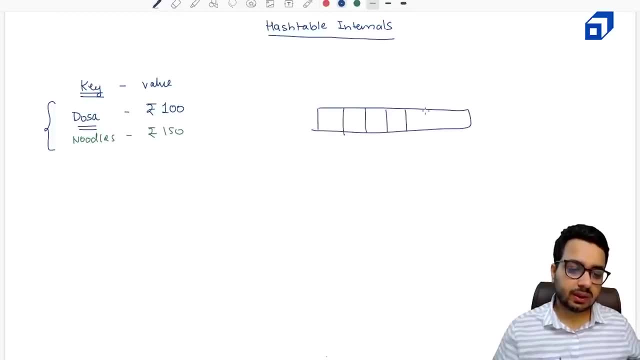 okay, of some size, right? so basically, whatever data we are given, we have to map this data with a certain index in this array, right? so suppose i'm getting dosa, right. so the first step of a hash table is that we have to hash the key value, right. we have to produce an integer location for a given 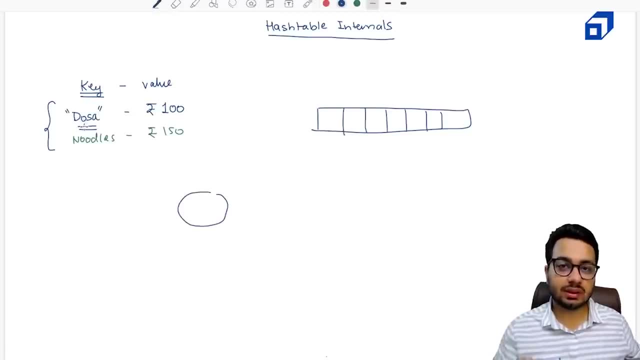 key now given key. in this case i'm taking it of the string type. but it can be any object, right? it can be student, it can be book. so for that particular type of object you need to tell the hash function how that integer value will be computed, right? so right now i'm assuming that 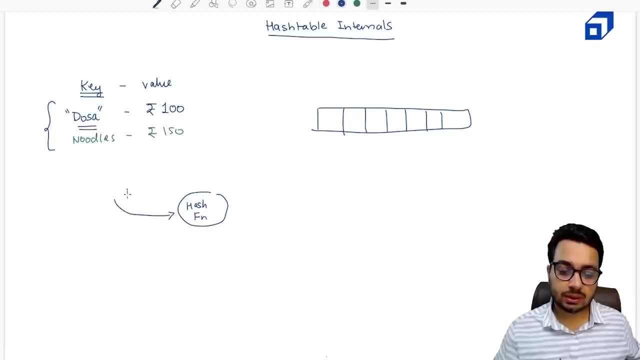 there is a hash function which is going to accept some key, let's say dosa, and it is going to produce an integer location, right? so maybe that integer location is zero, one, two, three, four, five, six and so on. right, maybe dosa will get stored here and the value will also get stored. 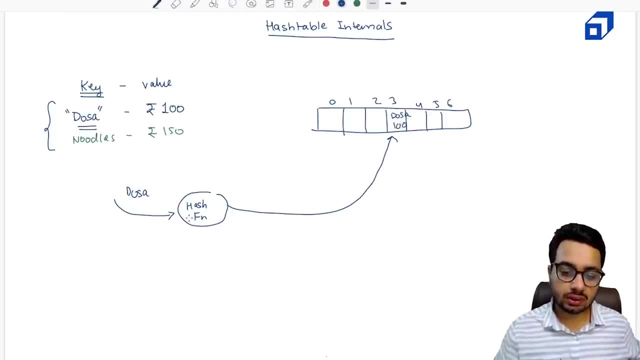 here, right, i got noodles, so noodles will go also go into this and maybe i get a location six. so maybe noodles get stored here and 150 gets stored here, right in the same location, right? so what is this hash function doing? hash function is taking input- a key, and it is producing a integer location. 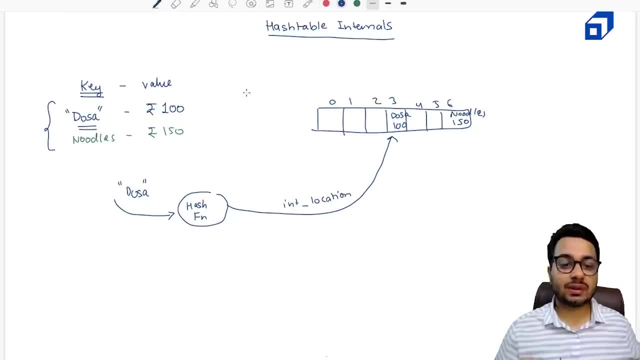 in the array. right now you might have some questions, right, how big this array should be, right if i have six keys? and if if i have six- uh, let's say six- size of the array right- and i have 12 keys, then of course i cannot store 12 keys in this area, right? so it's going to cause problems. so 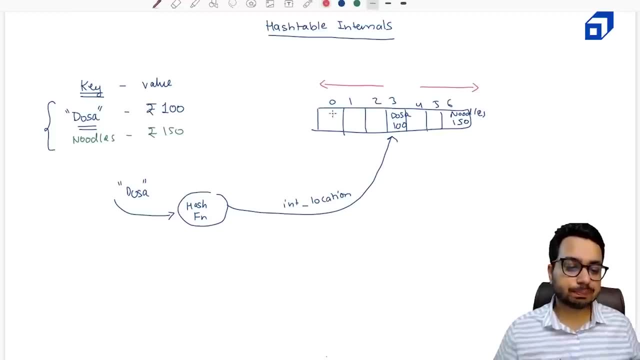 we will look at how to handle this very soon, right? this is not the completely correct implementation. we are going to discuss it step by step, right? so the idea of hash function is that it is going to use a unique integer location for every key, but it is also possible that for two different keys. 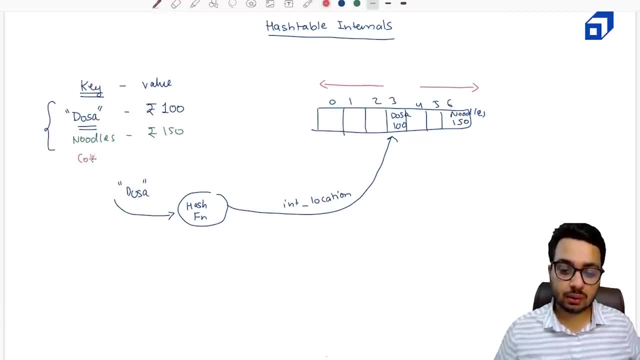 they get mapped with the same location. for example, if i get something like coke and this, since this is a mathematical function, it might compute similar location as well, right? so it might say: okay, coke should also go here, right. so this is called as a collision. we will discuss how do we. 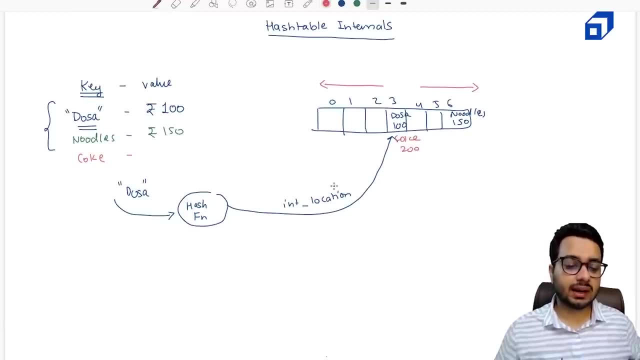 handle collision right, so maybe 200 something. but the idea is how big this array should be right. so one thing: we need to notice that this in: if it is producing an integer, then integer can take any value, right. so integer can be in the range maybe 0 to 10. it could be in the range 0 to 100, right, it could be even in the. 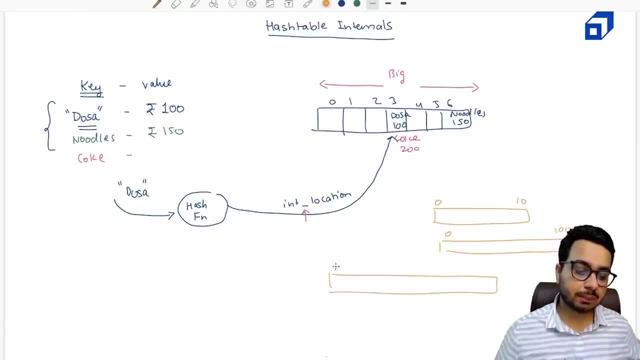 range of 0 to int max. right, so that means like, if i talk about every possible integer that can be generated, this range can be int max as well. right, but do i really need to create this big array? okay, int max is a proxy. there are almost 10 power, 9 elements. right, if i talk about how much space this array will take. 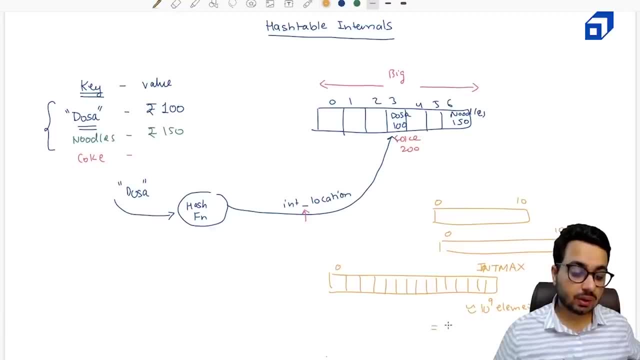 in the physical memory. this will come out around 16 gb, right? so will you need 16 gb of an array, right? or can you create this big array? the answer is definitely not. we cannot create this big array because this amount of continuous memory might not be. available. and secondly, suppose you have created this big array and you have created this huge array on your computer and you have a lot of memory data. you want to say a lot of memory data. we will include that to you and i'm going to make it even bigger than that. so it would be a lot. easier, and i'm not talking about 15 gb, right, but if you have a lot of memory data, there will be a lot of space to create these large arrays in this array. so I will be talking about how to create these numbers, right. so this is going to be important because we are going to have rough. 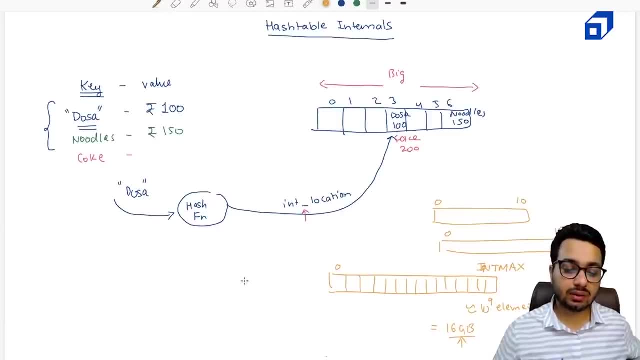 suppose you have created this big array and you have only 1000 keys in your key value pairs in your data set, right then you are allocating space for 10 power 9 elements and you just need space for 10 power 3 elements. that means you are doing lot of space wastage, which is not a good option. 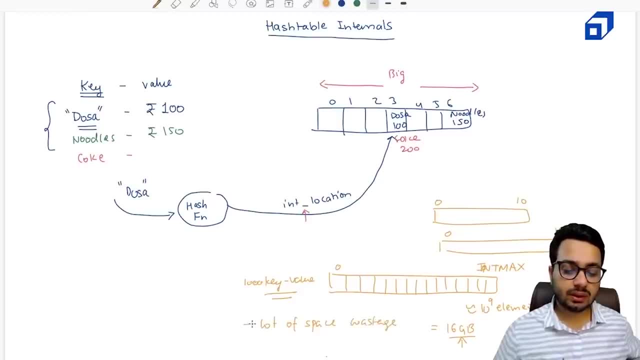 right then how big this array should be. it should be roughly of the order of number of keys that you are, you want to insert, right? so you, if you have an idea, okay, i want to insert somewhere around 1000 keys, then it is good enough. this array should have around 1000 buckets inside it. 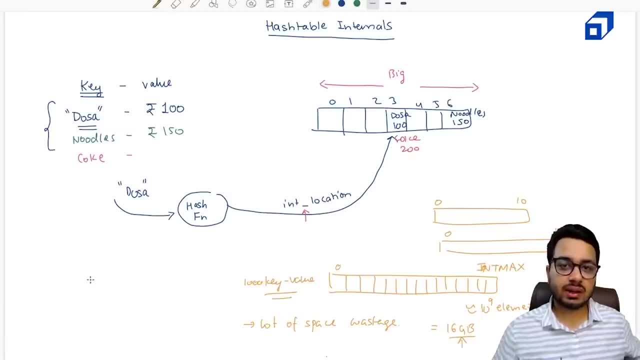 right? or if you want to insert maybe around 500 keys, it should be of the order this: much right, so what? i'm going to say? that table size should be of the order number of key value pairs that you're going to expect right now. it might happen that you expected 500 keys, but in practice, since the data, was dynamic, 700 keys would be of the order of number of keys that you are going to expect right now. it might happen that you expected 500 keys, but in practice, since the data was dynamic, 700 keys would be of the order of number of keys that you are going to expect, right, so we will also. 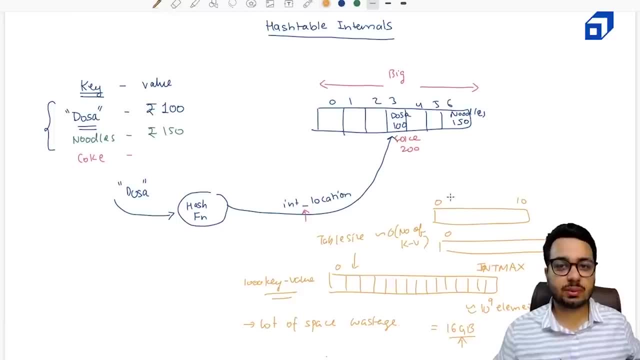 look at techniques to grow this table dynamically during the insertion process, right? so that is something we are going to study, right? what happens if there is a collision? how do we grow the table? how do we initialize the table? so all these concepts we are going to see next. so let's begin. 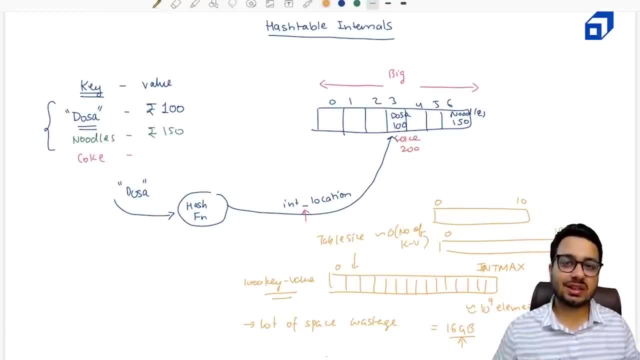 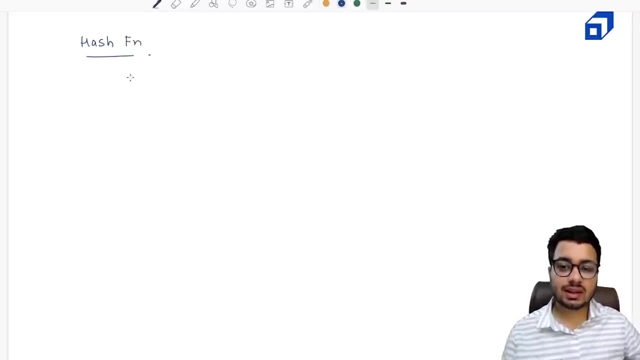 starting with the hash function, we will talk about insertion, searching and deletion in the hash table. so we are discussing hash function, right? so, as i discussed, hash function can accept a key. okay, input is a key. it can be of any, any. it can be any type of object. for our case, i'm just assuming. 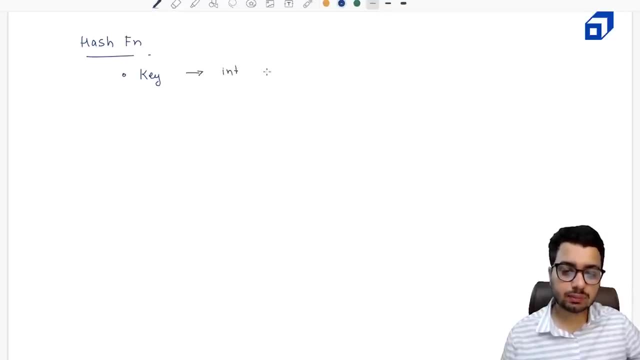 it to be a string and i want an integer value in some range. okay, in some range that is from 0 to n minus 1, where n is the size of the table, right? so n is the size of the table that i am implementing, right? so, for example, just to keep things simple, i am going to assume that i have a small table where 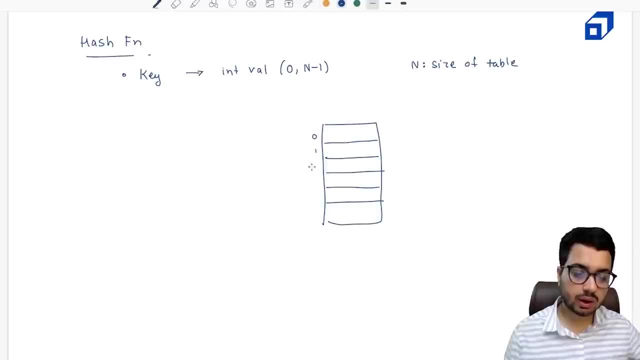 i have a huge library in the library sorø, where the i call it as table as well. so this are having a table size of 7. right now i have a hash function which knows how do i convert a given string into a numeric value. so suppose that if we want to convert a given string from text to a text, 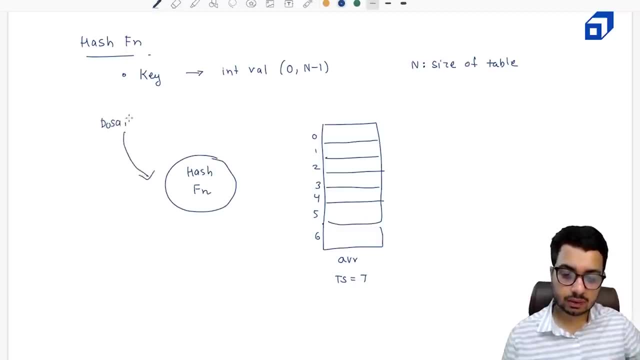 i'm getting a key like dosa, comma 100, right. the goal is to generate a integer, map it with an integer right and that value should not be random, it should be same always. so whenever you ask dosa, you have to tell me at what location this dosa is present, right? the goal is to convert this. 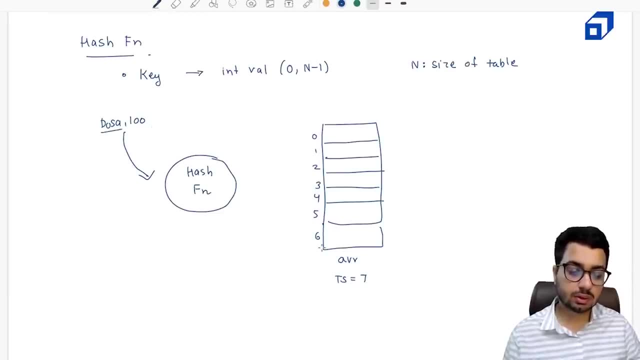 dosa into a number in the range 0 to 6. right? how do i do it? one simple way would be that i iterate over the ascii values of dosa, add them and since this addition will produce a number much larger than 7, okay, for example, your capital a, right it? i think it- has a ascii value of 65. b is 66, c is 67. 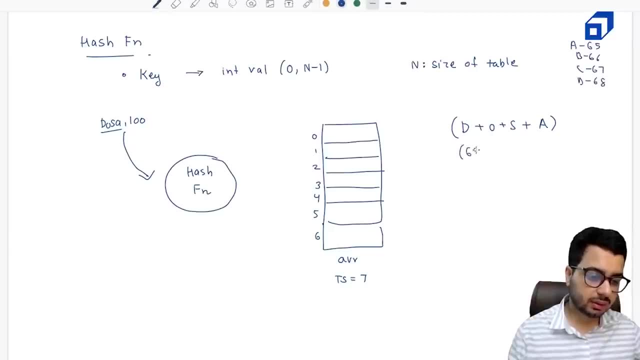 so d will be 68, right? so, similarly, here you will have certain values: 68 plus something plus something plus 65. this is going to produce a large integer, right? maybe of the order 200 to 300, right? but i want to map it in the range 0 to 6, right? what i will do? how do i reduce a bigger range which is some larger? 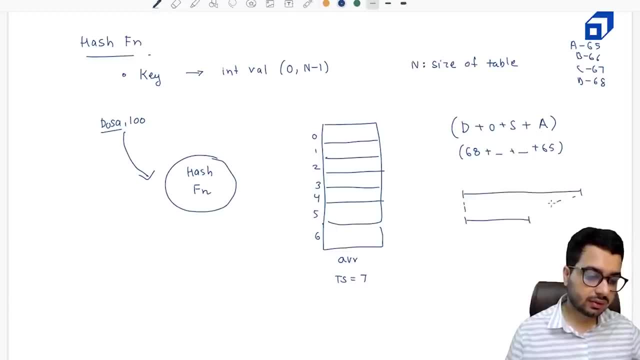 range into a smaller range. right, i can? okay, fine, this can be easily achieved by using a mod operator. so i can say mod with n, so i can take a mod with and so let us assume that this mod gives us an answer, that is 4.. 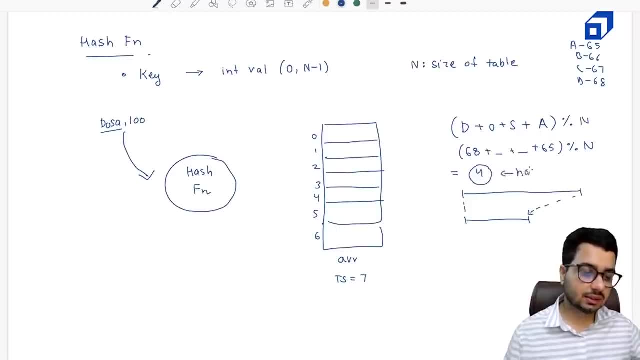 so that will be called as a hash index. okay, so basically the index on the table produced by hashing dash index is, let's say, 4.. so that means dosa will go at this particular index and this value will be stored at this place right now. the question is: what should i do? maybe i am getting 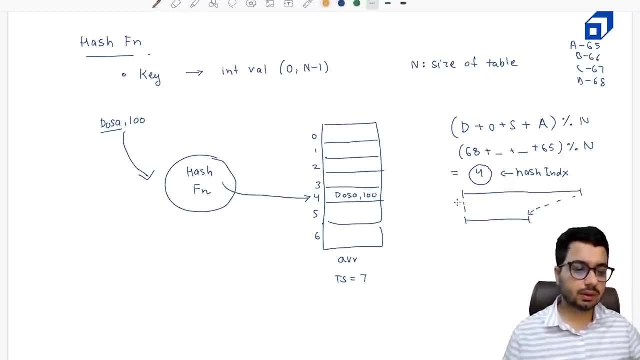 another key right in which the result is also four. right, the result is also four. so, can this happen? the answer is yes. so i can say: okay, i have maybe coke and maybe 150, right, i do not know. i add the letters of coke right and i take a mod with n. right now, mod with n can produce the same result for many. 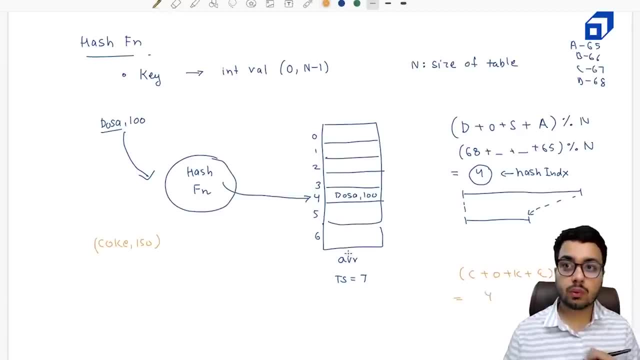 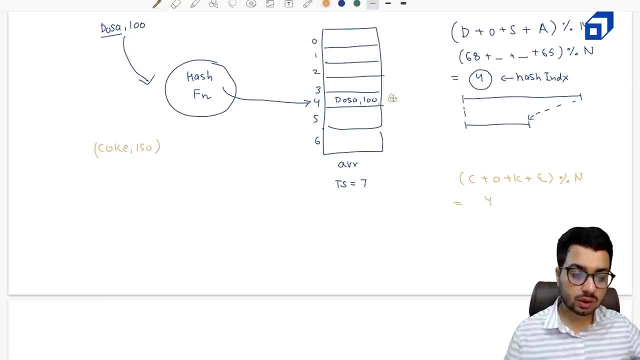 numbers, right, so maybe this also leads to four. what? what happened here? right? what happened here? so coke is also fighting for the same position. that means i also want to store coke here right now. this thing is called as a collision, right, we have space for only one key value pair, but 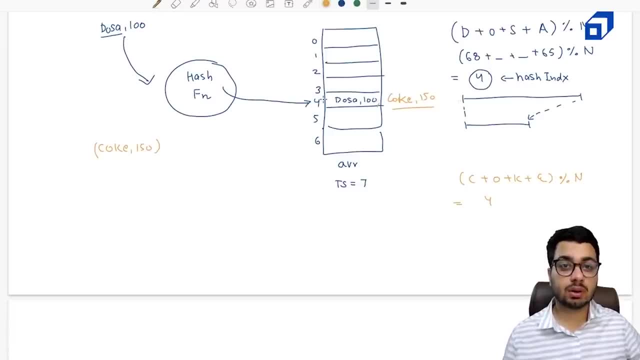 we want to store maybe two or more key value pairs at that particular location, right, so this is something called as a collision, right so what happens? right so what is a collision? so collision is a scenario in which, basically, two key value pairs, two or more key value pairs, they get mapped with the same bucket. 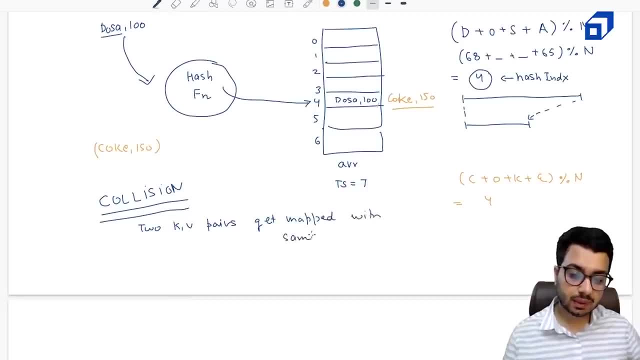 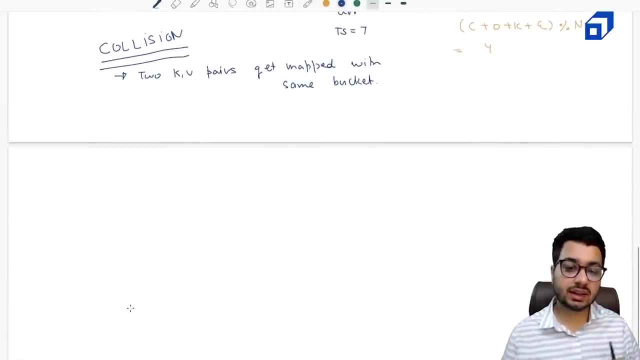 mapped with the same bucket. so this, what does this mean? right? can we avoid collisions? the answer is no. can we reduce collisions? the answer is yes. right, we will talk. talk about both the things, right? so, in order to reduce collisions, right, what we need to do is we. 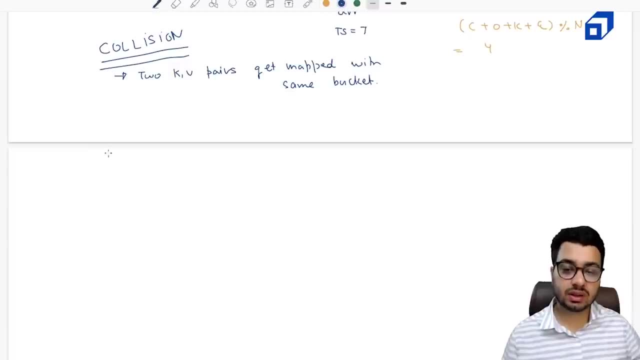 need is. we need a good hash function, so we will work on both the fronts. right, so collisions should be it. they cannot be avoided, right so how? irrespective of how good a hash function is, collisions cannot be avoided, but they need to be handled. right so cannot avoid collisions, right? 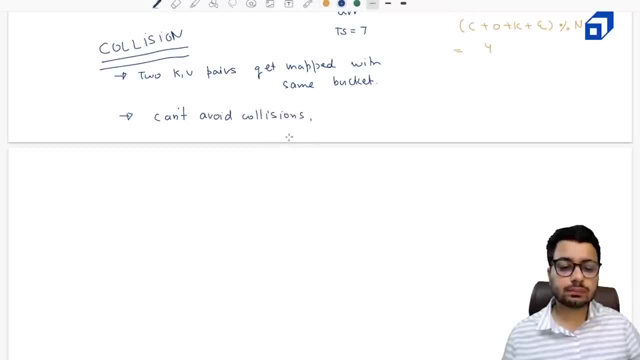 okay, but i can reduce the chances of collisions. but chances of collisions can be reduced by using a good hash function- right, but chances of collisions can be reduced using a good hash function- right, using a good hash function. now, how do we design a good hash function? we will discuss by taking an example of string right. 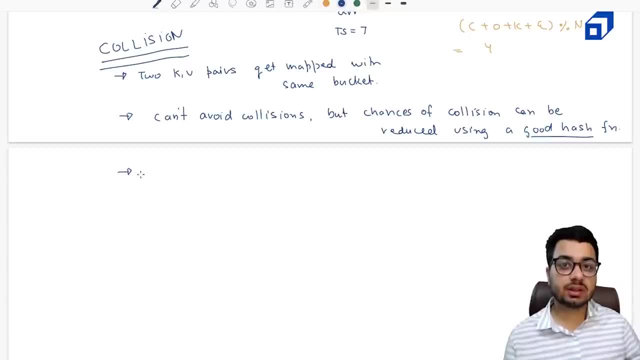 and secondly, since you cannot avoid collisions, so even if the collision is happening, you need a way to handle that collision right. they still need to be handled. so we need something called as a collision handling scheme, right collision handling scheme. this is something we will do, something we will discuss very shortly. right now, there are two important 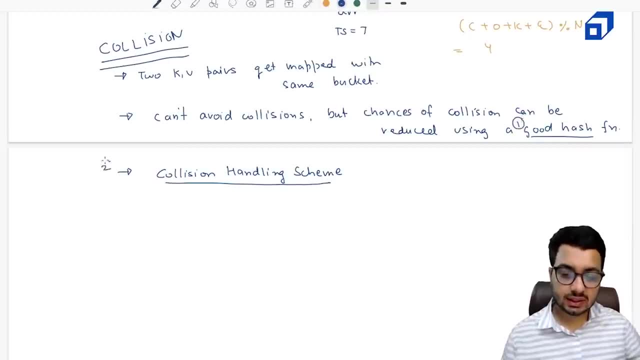 things here. one is: what is a good hash function? second is a good? second is we need a good collision handling scheme. so first, good hash function will reduce the chances of collisions, but they still can happen. so if the collision is still happening, we need to handle it using collision. 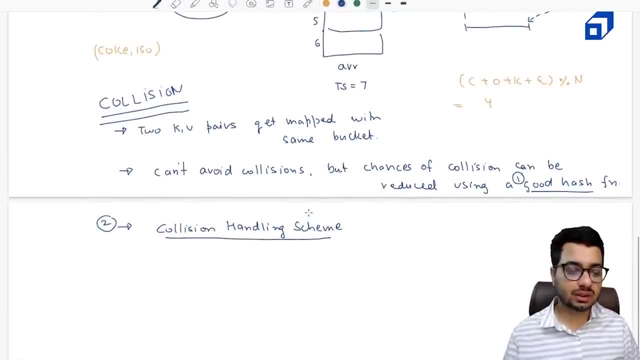 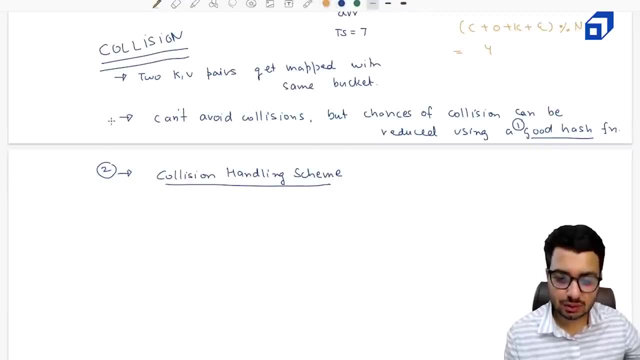 handling scheme. so let us discuss what is the? how do we design a good hash function and how do we handling scheme? next, let us discuss the properties of a good hash function. right, so I am going to discuss the properties of a good hash function, right? so, basically, a good hash function should. 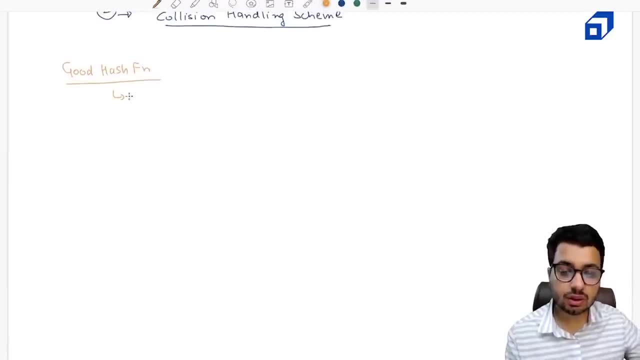 have two properties. first, it should ensure a more of a uniform distribution- okay, it should ensure more uniform distribution, right. and secondly, it should be fast to compute, right. so that means we do not spend a lot of time in computing the hash index itself, right, for example, in our case. 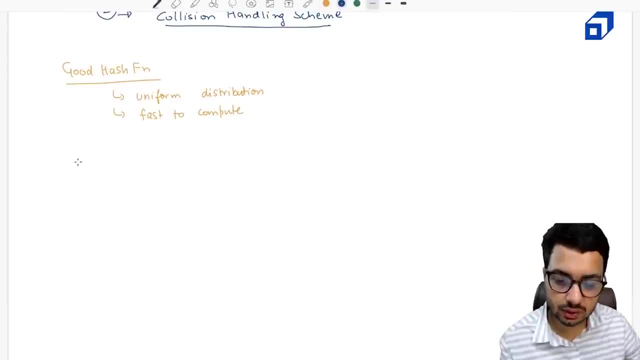 what we were taking. I will take examples of two hash functions. okay, so let's say example number one, in which I am simply adding the r square values and taking a mod with the table size. so I am saying, fine, I will add dosa d plus o plus s plus a and I will take a mod with the table size. right now is this: 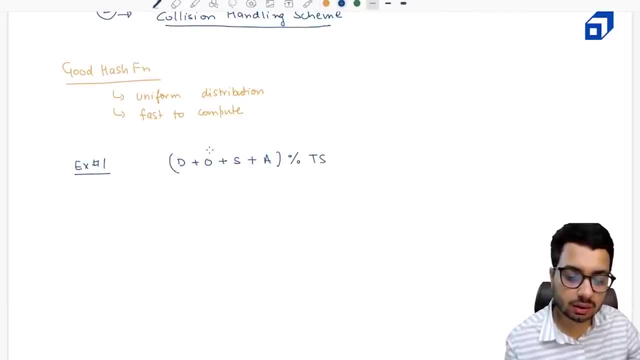 function fast to compute? yes, because I just need to iterate on the letters of the key right. so when, when I am talking about, I am going to insert many key value pairs. so what is n? n is the number of key value pairs? okay, so, key one: value one. key two: value two: right key three: value three. I want to. 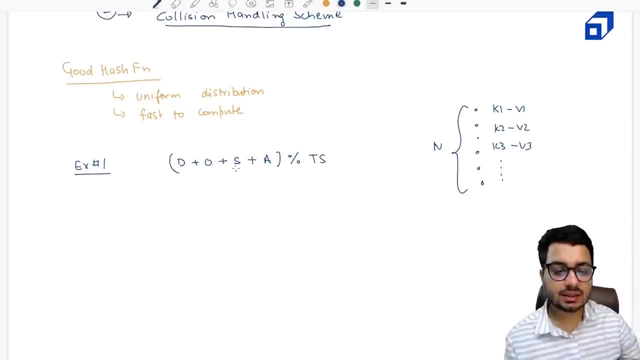 insert a number of key value pairs. okay, so I am going to insert a number of key value pairs. okay, you can see that I have inserted many key value pairs. so my hash index does not depend upon the value n, but it depends upon how big my key is. so in general, the key would be small length, so we can. 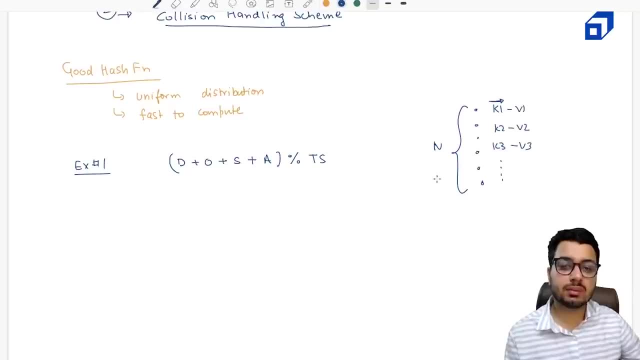 assume that, okay, if it is a name of a person and the phone number is the value, the key would be maybe maximum 50 characters or 100 characters. so, yes, in this case this is a fast hash function, right, but is this hash function is going to minimize the chances of collisions? maybe not right. 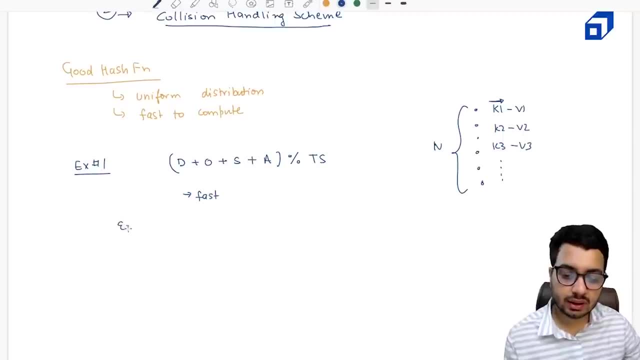 why? because if i talk about english language, right, in english lot of words they are anagrams. that means uh, lot of words have same set of letters in them. for example, let's say the word is tab, right, so it is made up of t, a and b and if you add you will get certain sum right. but if i talk about 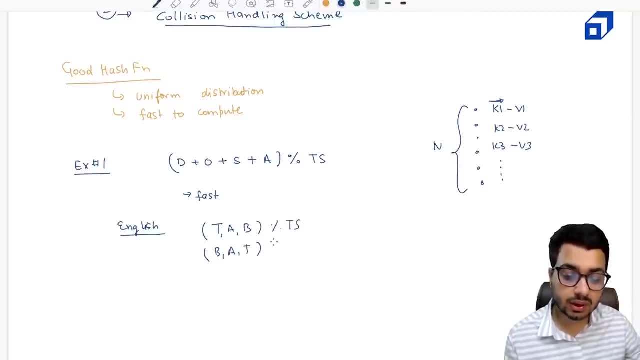 the word bat right. it is also made up of same letters, so in this case we are sure that these two are going to collide because our hash function is doing a very simple sum right. so in. maybe, of course, there could be other words also. maybe the word is mango right now. it is possible that. 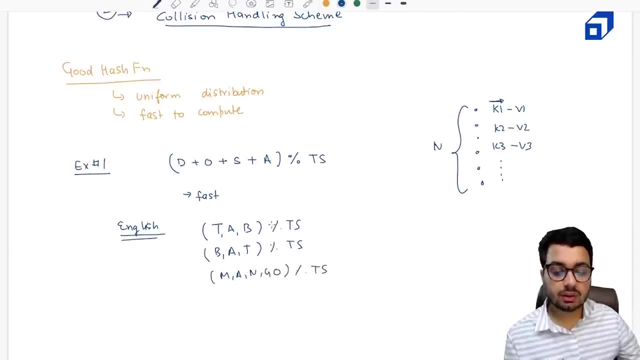 even if you do a mod with table size, you might end up at the same index, right? so we do not know. so in this case, it is of course difficult, uh, to tell whether the collision will happen or not, but it may still happen, right? but here we are sure that a collision will happen, right? so many words. 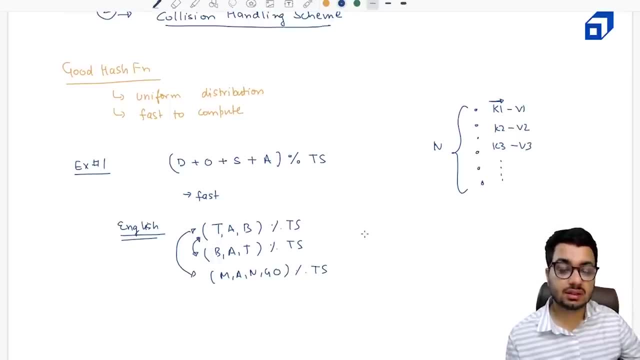 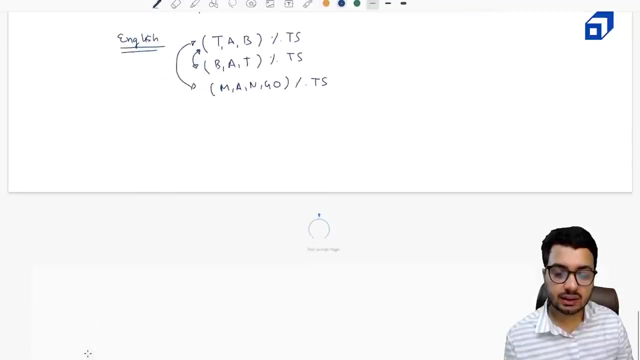 in english, they will have such a scenario, right? what we can do is, instead of doing a simple addition- right- we can do a weighted addition, right? so this is like a simple addition of rsk values we are doing right. so a better way would be that you do not do a simple addition. 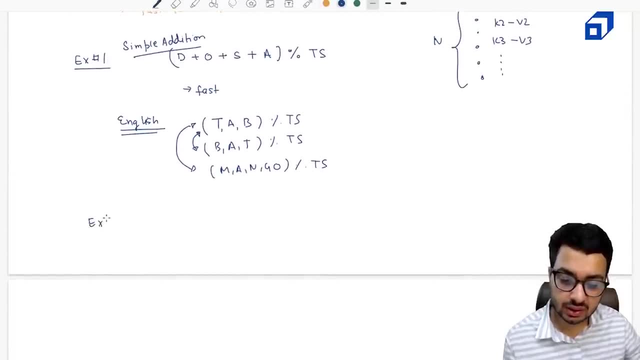 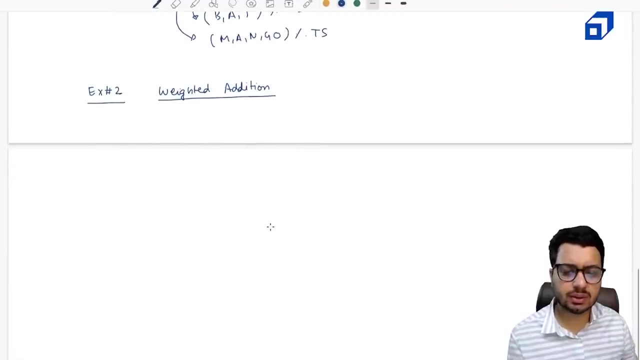 in your hash function, but you do a weighted addition, right? so example two of building a hash function would be that you do some weighted addition, right? so that means you are going to multiply each letters rsk value with some weight, right? so, for example, i choose a weight. maybe generally it is a prime number, right? so maybe i choose a weight as, let's say, 31. 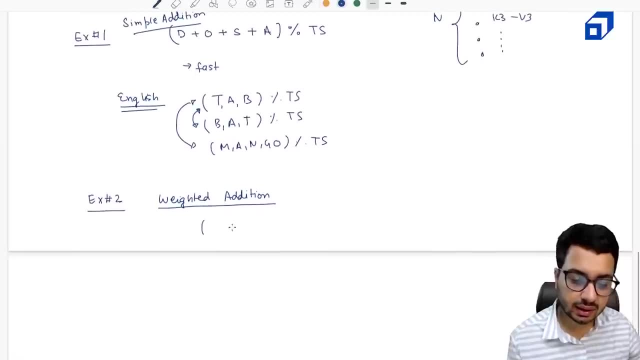 right, or 29 right what i can say. that fine, i will multiply dosa with powers of 2. so let's say the weight is 29, so 29 power 0, that is 1 into d plus 29 power 1 into o plus. 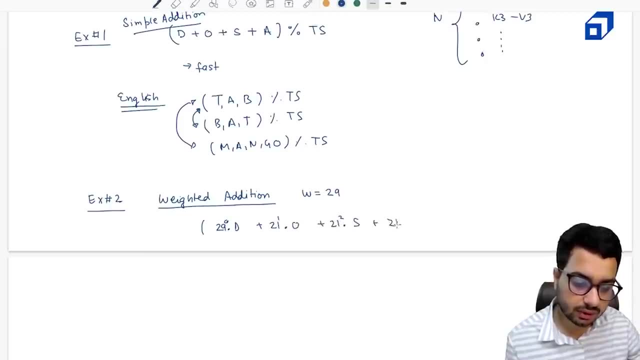 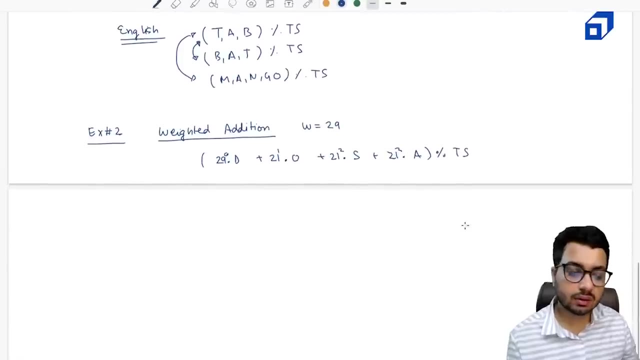 21 square into s, plus 21 square into a, and then i take a mod with table size, right? what i'm trying to claim is now: if you do it for bat and tab, it is less likely that you will have a collision, right? so i'm saying: you multiply, uh, 29, power 0, which is 1, this is 29 and this is 29 square right. 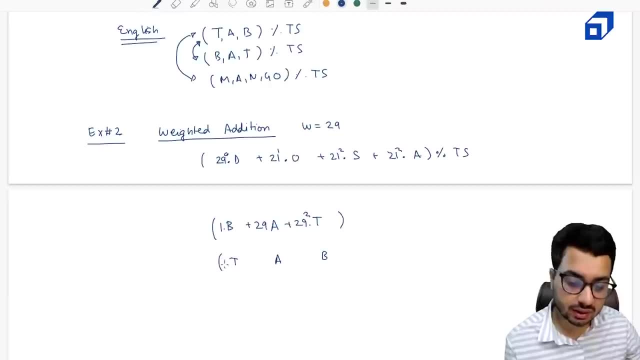 and then you like, it's a weighted addition. again, 1 plus 29 into a, plus 29 square into b and, of course, mod with the table size, mod with the table size right now. earlier we were sure that these two values are will surely collide. now we. 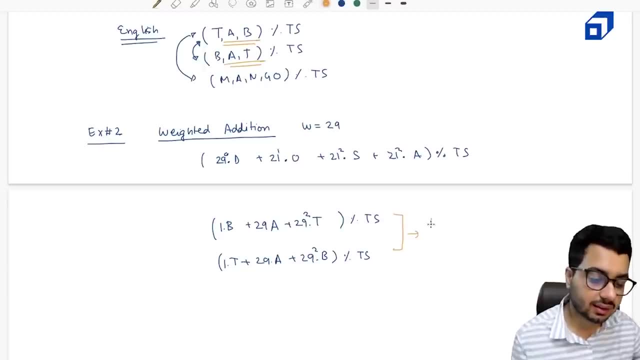 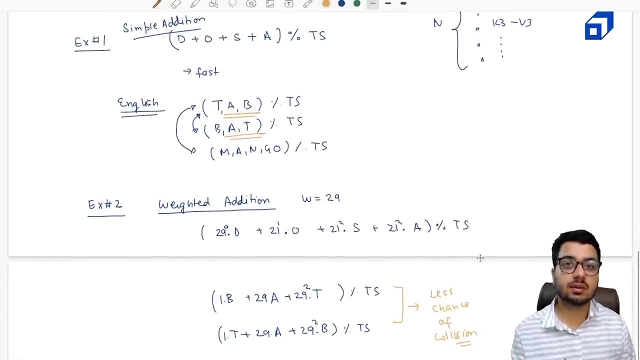 can. okay, the chances of the collisions are less. okay, so there is a less chance of collision, right? so these are the factors that you can keep in mind, that, okay, if i'm building a hash function, can i modify it some way so that it reduces the chances of collision and it is fast to compute, right? so here also, it is fast to compute. 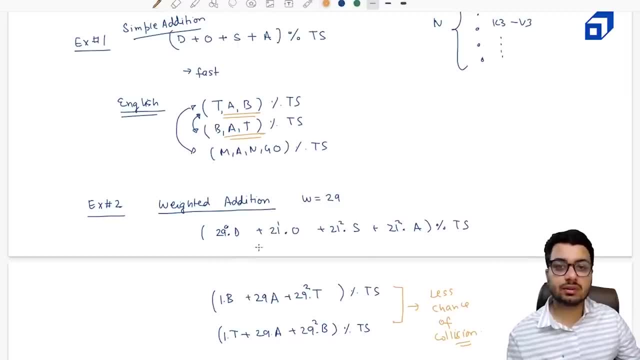 right. maybe if you have a string in which the length is too big, maybe you can restrict that. okay, i will consider only the first 10 letters of the string for this weighted addition. that can also be done, right? so that will even make the function a bit more faster, right? so if you are, 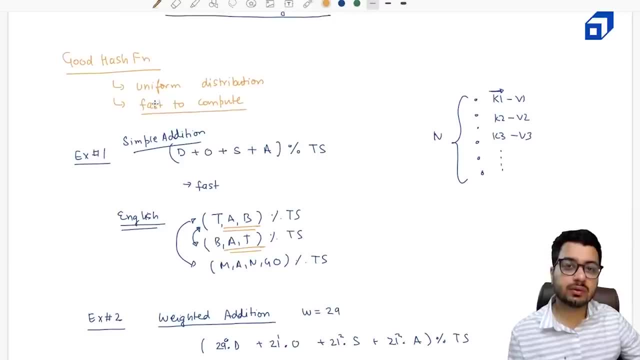 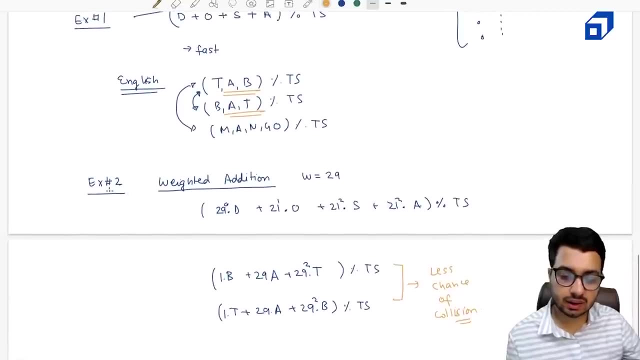 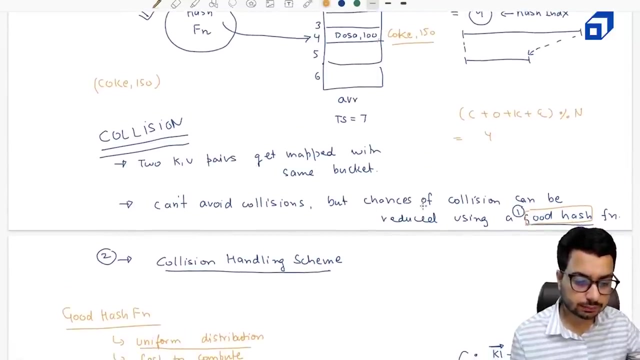 thinking that the keys are too, too long. you can restrict to maybe the first 10 letters or maybe something like that, right? So now we have a good hash function, which is the second one. second one is obviously better. we are doing weighted addition, so it is going to reduce, uh, the chances of collision, right, but a collisions. 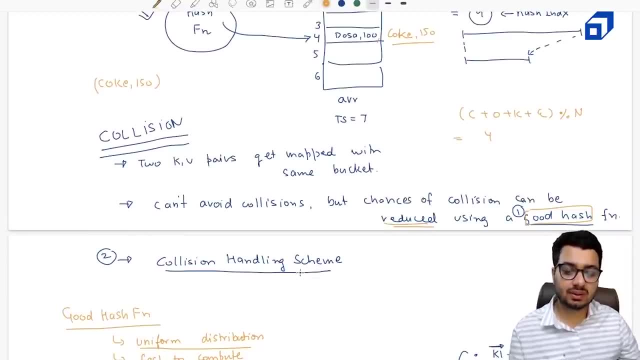 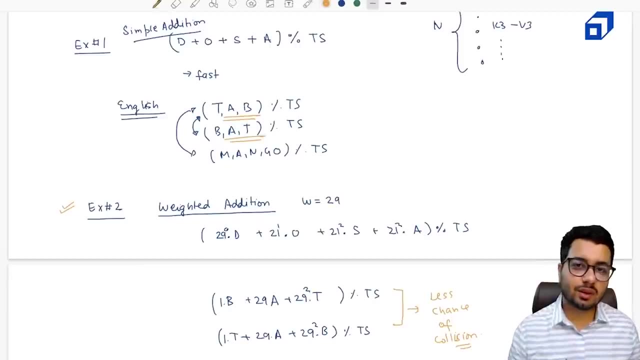 can still happen, right? so how do we handle if still a collision happens? so here comes a collision handling scheme, right? so let us discuss about collision handling scheme now. so you have seen how do we design a hash function. now we need to discuss how do we design a collision handling. 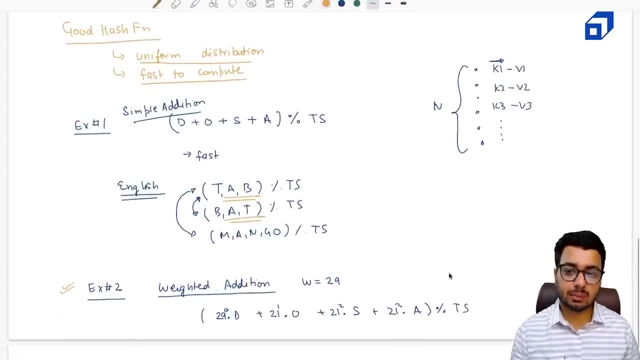 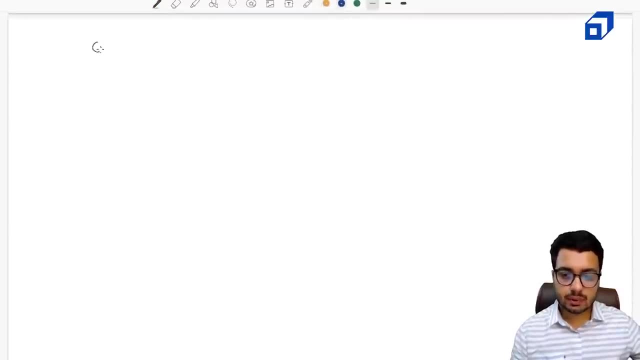 scheme right can still happen. we need to handle them right. so let us talk about how do we design a collision handling scheme right, collision handling scheme right. so there are actually multiple schemes, but I will particularly discuss one scheme right. so, in this case, what we can do, we can do something. 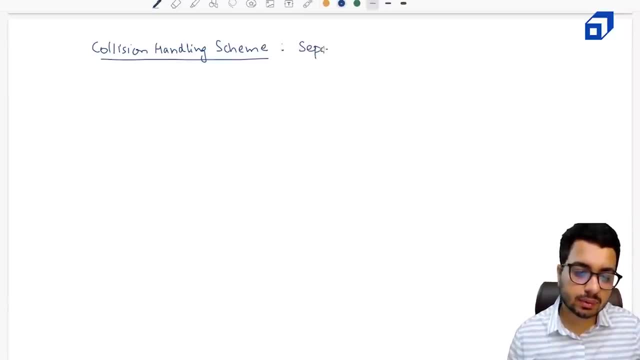 called as separate chaining, so we are going to discuss only one scheme. there are other probing techniques as well. right, so I will discuss separate chaining. right, so this is one of the most popularly and widely used schemes in implementing the hash table. right now, I'll just copy the diagram that we have seen earlier. this is the diagram, right, so let me just copy it. 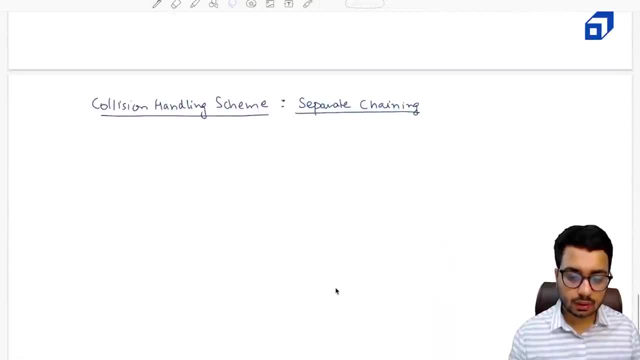 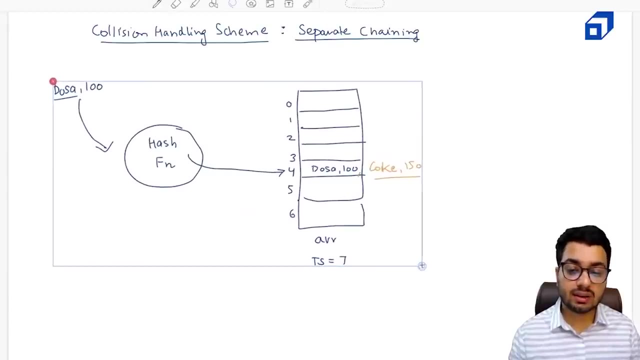 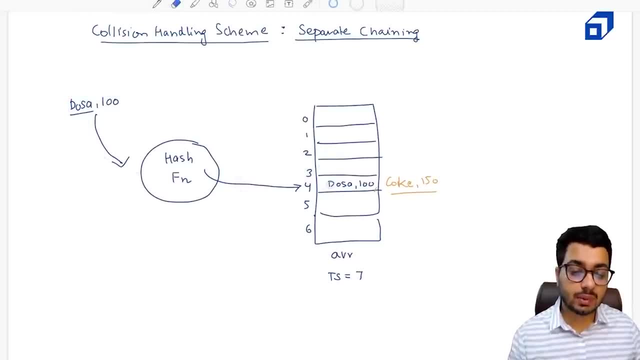 separate chaining. so suppose, if we got dosa and it gets get mapped with index 4, so what we will do will not store it directly inside this bucket, but instead, every time we get a particular bucket mapped with dosa, we will start a chain from there, right? so what? what is a chain? a chain? 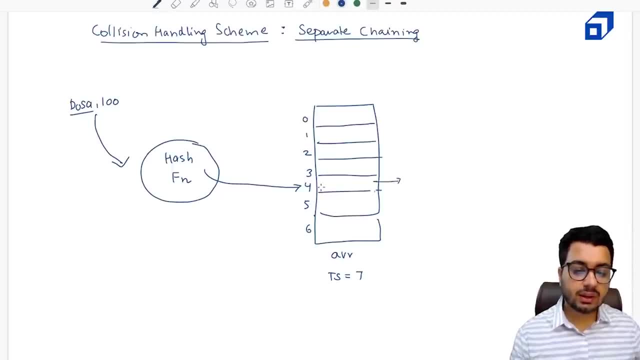 is like a linked list, so it's exactly a list, right? that means each bucket is actually going to hold the address of the first node of the list, right? so for, for example, I'm going to store dosa comma 100 here right now. suppose I got coke comma 150. the coke goes into the hash function and maybe 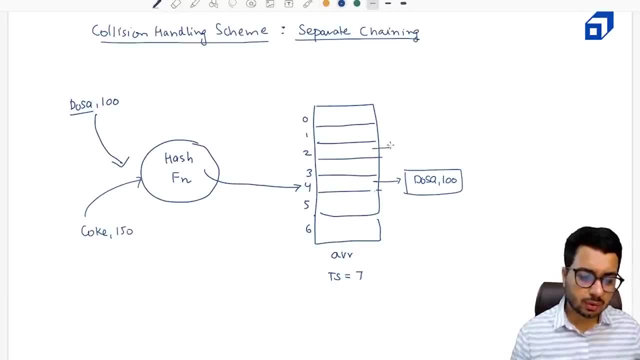 this time I get two, so I will start a chain from two and coke will go here, coke, comma 150. it will be stored here. right now suppose I got something like noodles, okay, and noodles is going to have a value, let's say 120.. now noodles, if it goes to the hash function, let us. 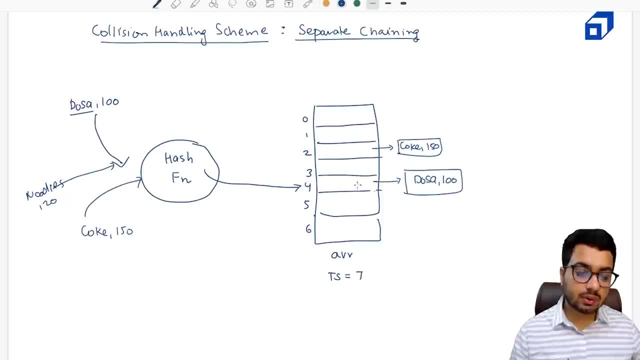 assume the hash function computes the index 4 right now, at index 4 we already have dosa. so what we will do? we will also try to store noodles at this index. how so we can. okay, we can add noodles to this linked list. now, suppose this is some address. let's say, this is uh, 150, this is 270. 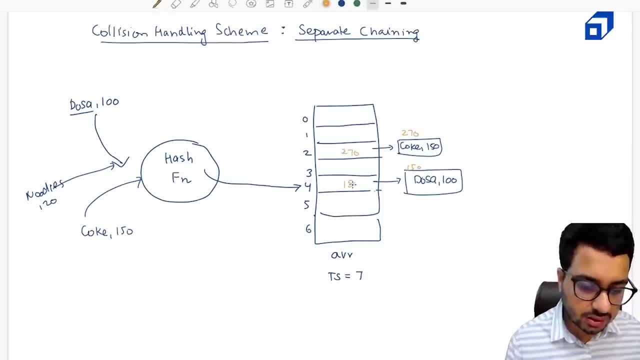 right. so this is storing 270. this is storing 150.. so each array bucket is actually storing the head of the linked list right now, how we can insert noodles in this chain in order one time. it's pretty easy. so you can say: okay, I will create a bucket called. 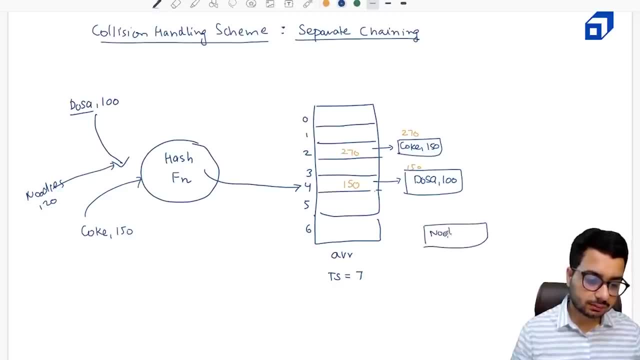 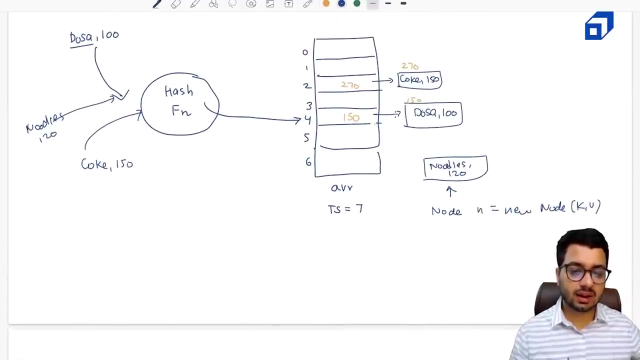 noodles. let's say this bucket is: uh, this node is created, so I'll create this node, and with the given key value pair: right, so it's a new node, with the given key value pair, right now. in this new node. what should I do? like? how do I add this node in this linked list? right, so I. 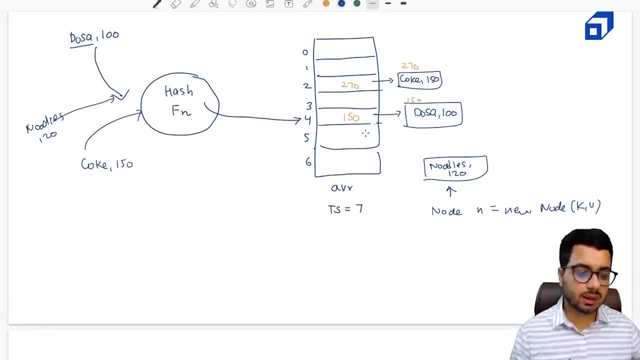 can: okay, this is some array, right, so. or this is some table, so I can say array of. and let us also compute the index so I can say index, where I want to store this is given by the hash function of the given key right, so I get to know the index also. so add this index. I need to store noodles. so one thing. 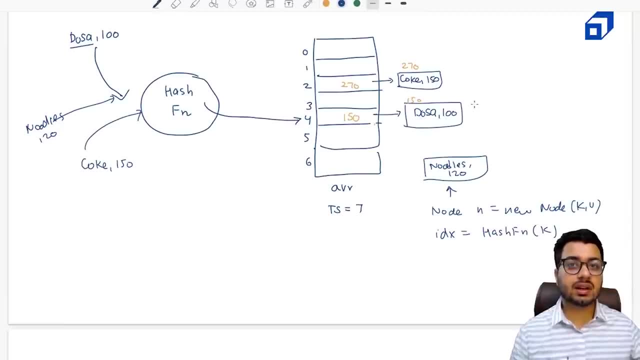 do is either i can insert at head or i can do insert at tail, since i'm not maintaining the tail of the linked list explicitly. but you can maintain. if you want, i can also do a direct insertion at the head right. so that means we can say, okay, uh, this node 4 will refer to noodles and 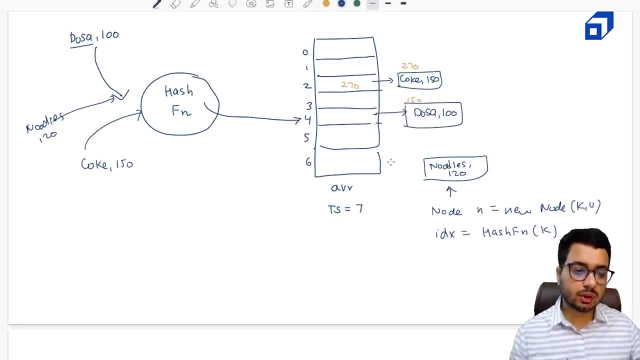 noodles will connect here. so right now this is connected here. so what i can do, i can ask noodles to connect with dosa, right, so i can say n dot next. so in every node i'm also going to have next field right, so that i can actually form a chain, just like a linked list. so every node is 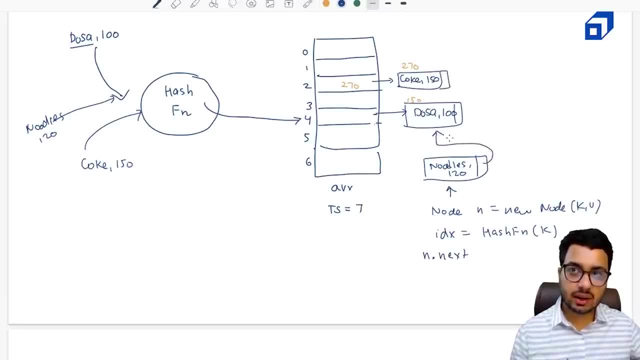 going to have a next field so i can say, okay, you should connect here right, so i can say n dot. next should be equal to array of index. area of index is storing 150, so that 150 will be copied here right, and now i can update area of index to point to this node so i can say area of. 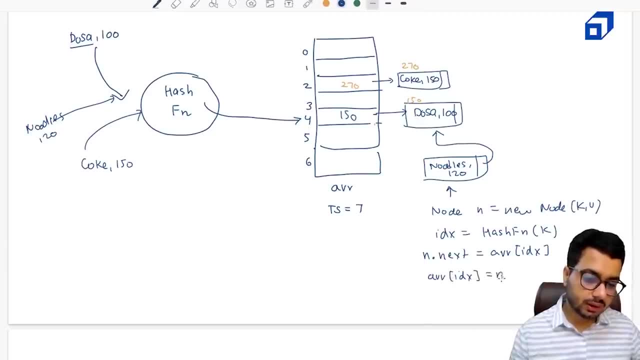 index should point to n. so basically, i'm changing this connection like this: n is what? whatever it is, this will be now referring to this node. if you look carefully, we have actually formed a chain right. so this is, let's say, this is some address. let's say 480, this is now. 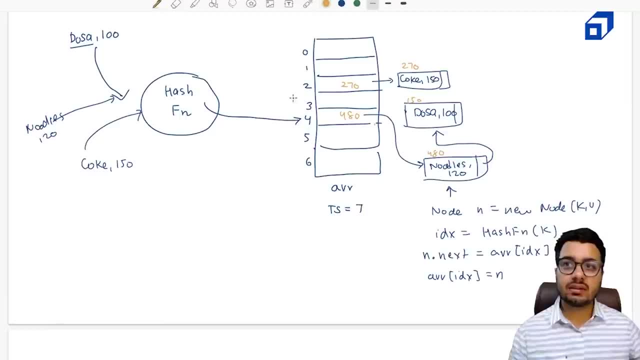 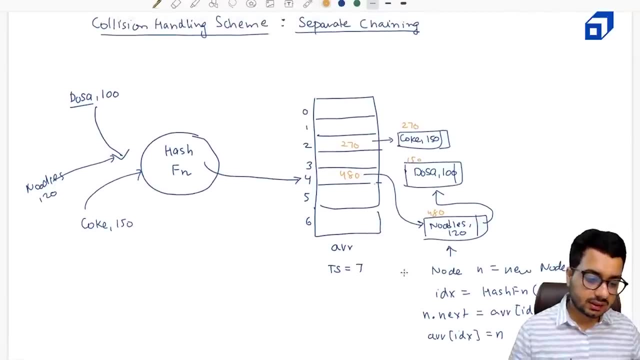 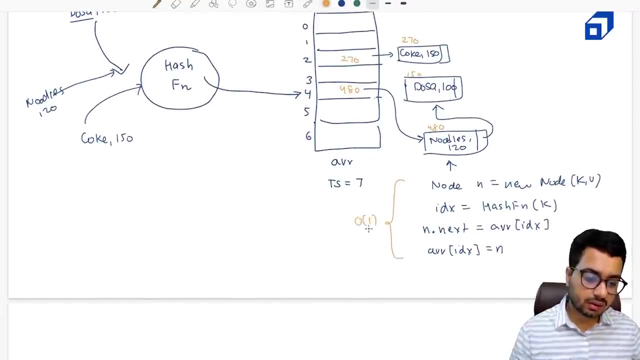 storing 480, right? so you can see we are actually forming a chain, right, we are actually forming a chain. so this is exactly how the insertion is going to work and this is the code to insert, right? do you think will it work in order one time? absolutely yes. this insertion will be always order one, right, because we are 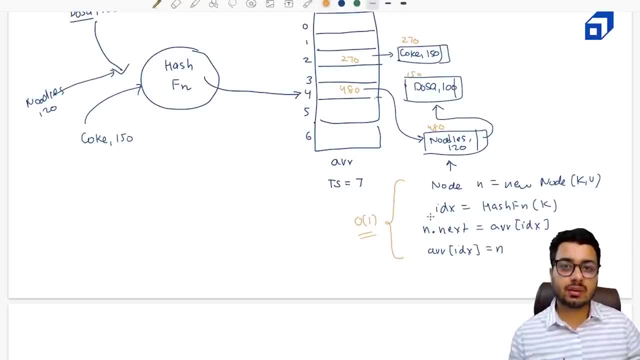 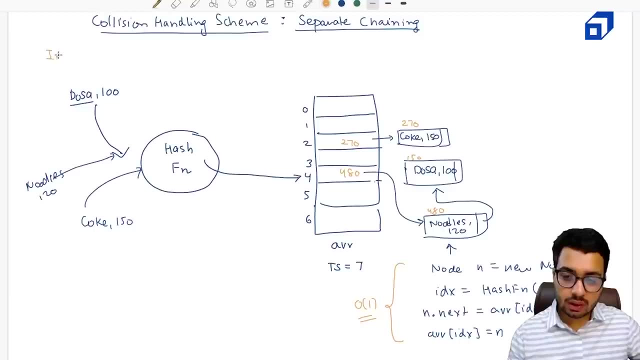 inserting something at the head of the linked list. irrespective of the chain length, the insertion will be always order one, right. so i hope you have understood insertion, but is it done? the answer is no. we are not yet complete right. we have to still discuss one more concept, but that concept i will discuss after discussing searching. okay, so this is: 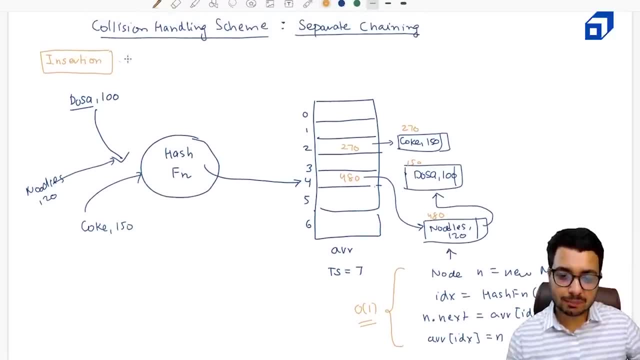 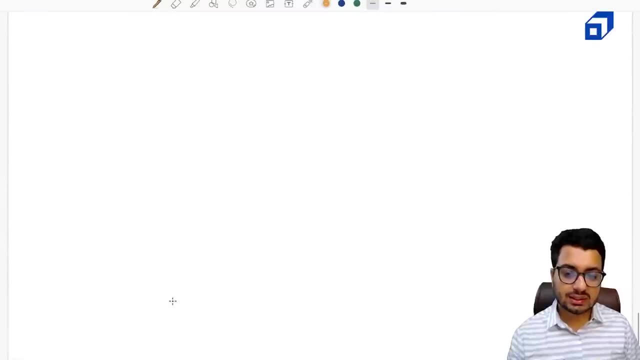 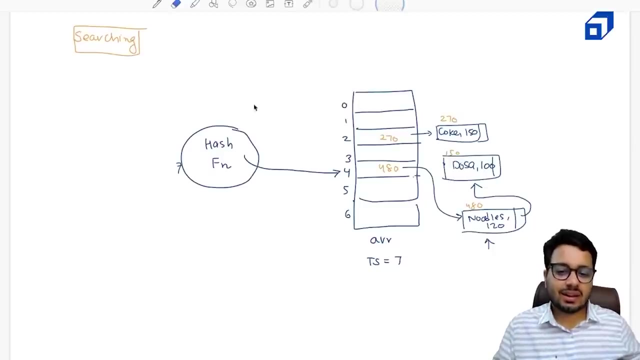 still not complete. so this is insertion part one, right? okay, so there is something more to the insertion that is going to come up. right, let us discuss searching, how we can actually search in such a scenario, right? so we are discussing searching now, right? so now, what is the purpose? 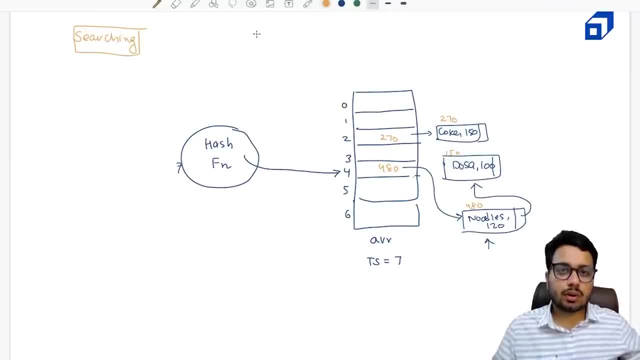 of searching. the purpose of the searching is that, given a key, i want to look up the search for the value of that particular key. right, if i ask? okay, i want to know what is the price of dosa, how i will find it. so, first of all, dosa is a key. this is given as input, so dosa will go to: 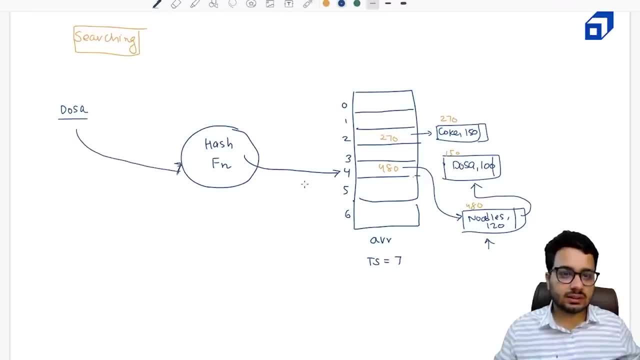 the hash function. the hash function will generate an index where this dosa can be present. in this case, hash function gives me an index 4.. that means now at index 4. i actually have a chain right, if i write it little more clearly. so this chain looks like this: 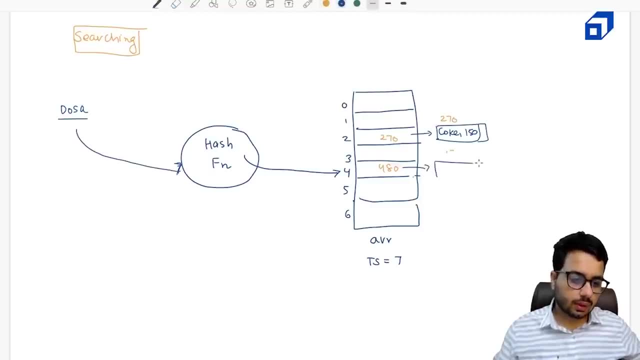 i have noodles and which is like 120, and i have dosa, which is part of the chain, and this price is 100, right, and of course the next is none. now i have to iterate on this chain to check if this chain can contain dosa or not. so if i iterate on this chain, 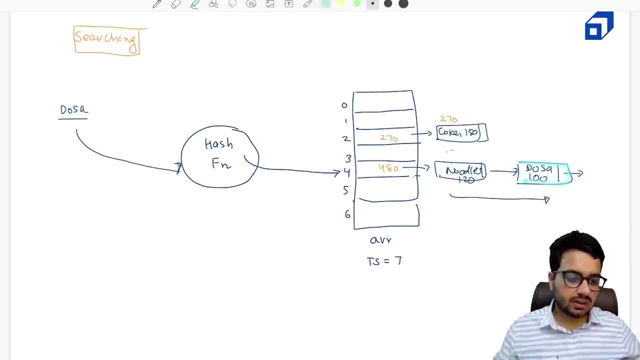 i will find a dosa at this particular position and once i find a dosa i can return the value that is 100. right, that is how searching is going to be performed. so we first find the bucket where the hash function is telling me: okay, in this bucket you have to check. 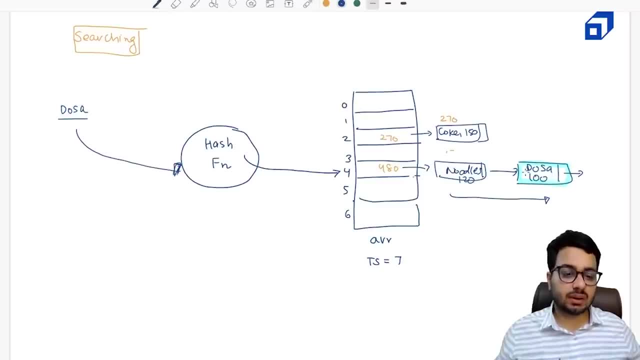 and in this chain, dosa can be present. dosa may not be present right now. you might ask: okay, if we have to iterate the chain, then what is the time? complexity of this operation. my answer is: it will be order of chain length. right, how do we figure out chain length? okay, can. 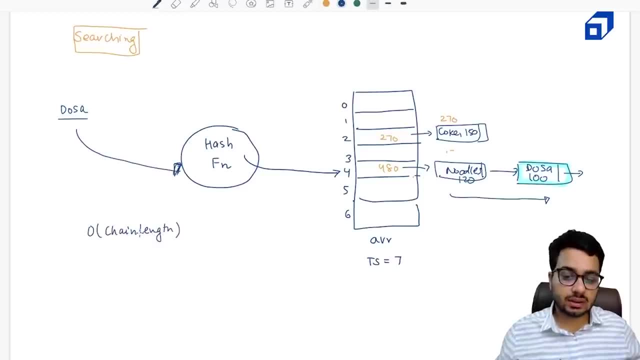 this chain length become very large? the answer is yes, it can become very large, right? so the key to successful search operation is that we have to ensure that this chain length is very small. okay, so we have to ensure that chain length is very small, right? maybe two to three nodes, or maybe. 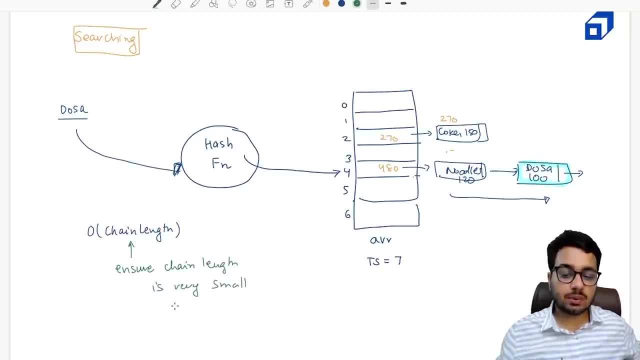 three to four nodes right, and this is achieved using a concept called as rehashing and load vector. so we will discuss this concept. ensure that the chain length is very small. so if the chain length is very small, we can say okay. on an average, this operation will be order one. maybe i say okay. 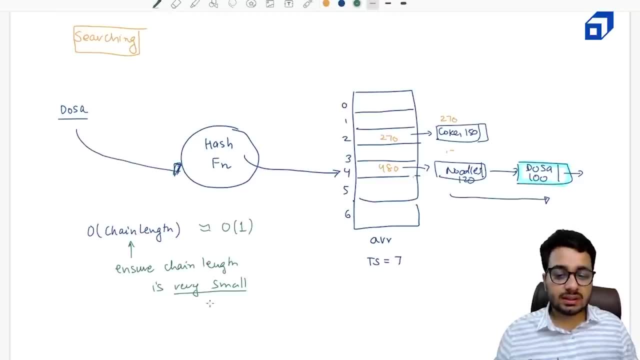 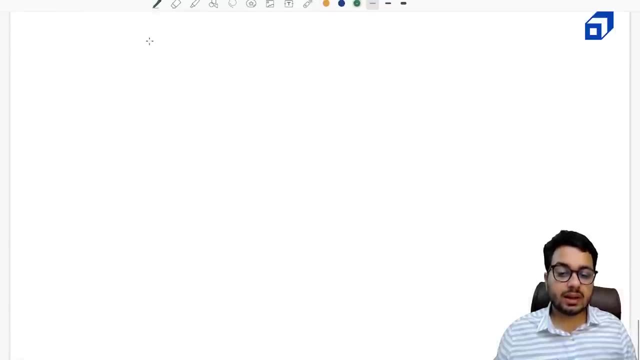 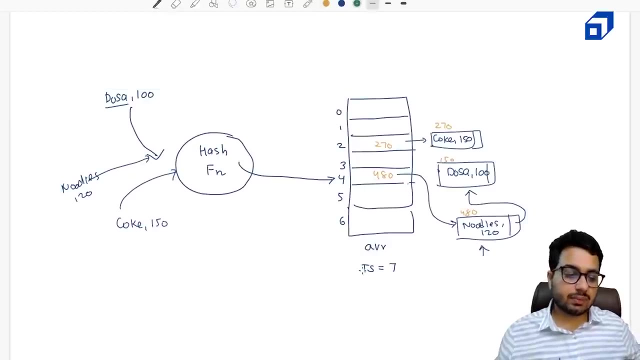 the chain will have only three nodes. two nodes, right. but now let us discuss how this chain length will be decided. right, how this chain length will be actually decided. right now, suppose i have a hash table where i have seven nodes, only, right, and i keep on inserting data, right, if i say okay? 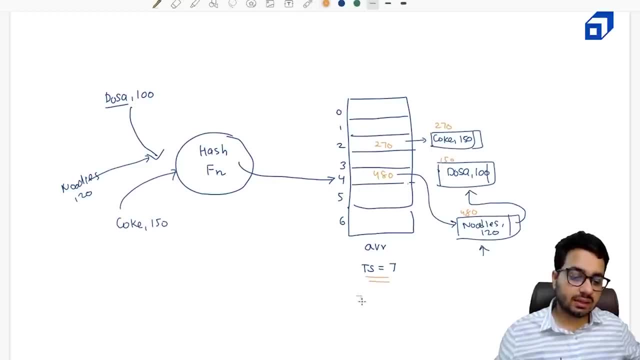 my table size is seven and i insert 70 key value pairs inside it. right, what will be the average chain length if i talk about the average chain length in this case, so i can say, okay, i have done 70 insertions, i cross seven buckets, so it will be 70 upon 7, that is 10.. 10 is a big number. 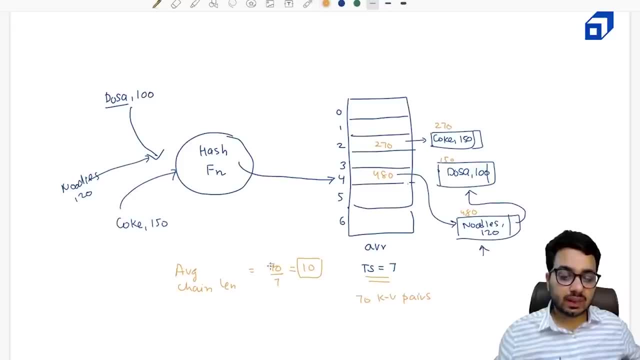 i do not want to keep this much chain length right. so this quantity that i have just written here, it is actually called as load factor. so load factor is a technical term for the average chain length. okay, so how do we compute load factor? so we say, okay, total number of key value pairs that have 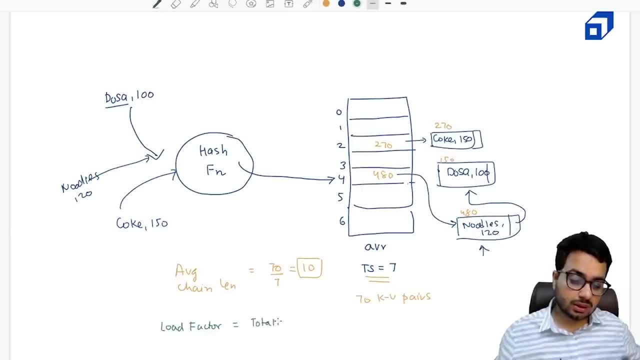 been inserted in into the hash table. so total key value pairs i have inserted upon my table size, or in other words can say current size, the number of key value pairs that have been inserted upon table size. that could be another way of writing it right, so i write this one. looks little more better to me. so in the 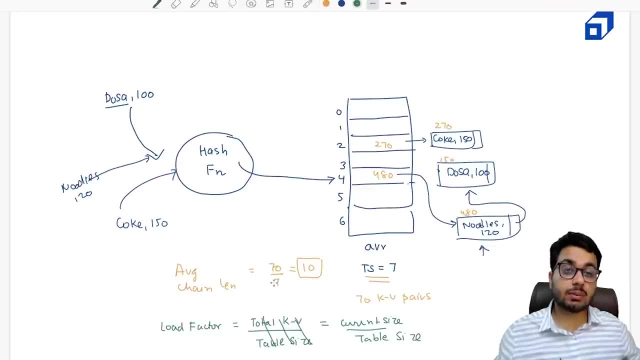 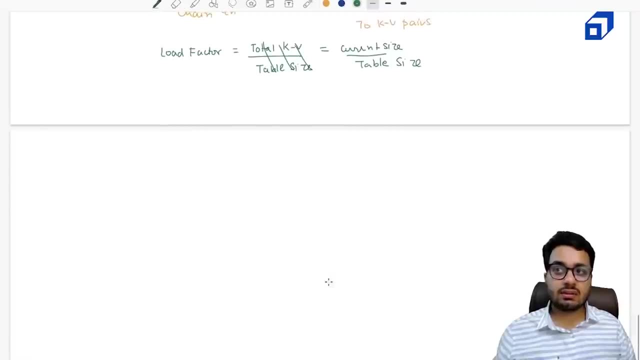 current scenario: if you have 70 key value pairs inserted in seven buckets, this is 10. it is actually huge. it's bad, right. so what do we need to ensure? we need to ensure that our load factor does not exceed a certain threshold, right? so in some languages it is one, in some languages it is. 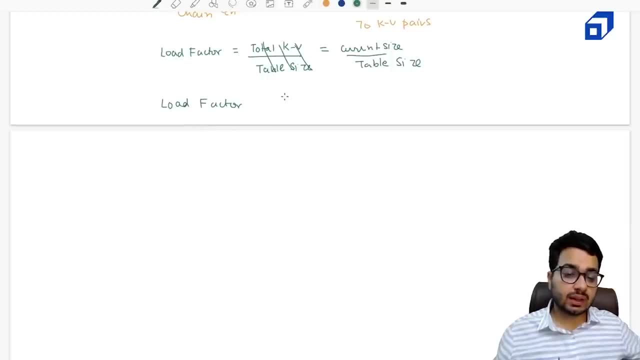 0.7. so, whatever is the case, we need to ensure that it does not exceed the threshold value of, let's say, 0.75. right now, what does it mean if i have, let's say, 10 buckets and i insert 7 key value pairs? so what will be the load factor? it will be 0.7. that means on an. 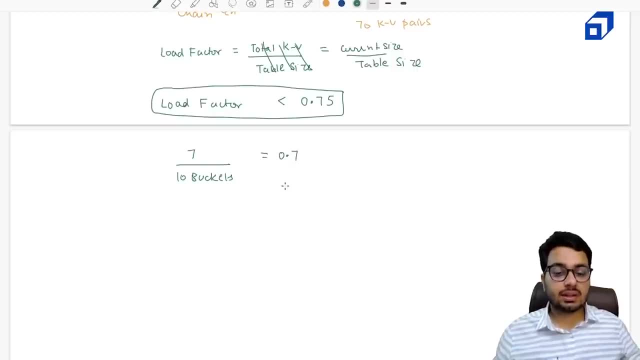 average, every chain has less than one node, right. so that also means that my table size will be slightly bigger than 0.7, and my table size expects to be bigger on average, rather than that van. our table size will be slightly bigger than every chain. i have less than one node, so by that i consider the daily load factor as less than one node, which means every chain has less than more. to first method. 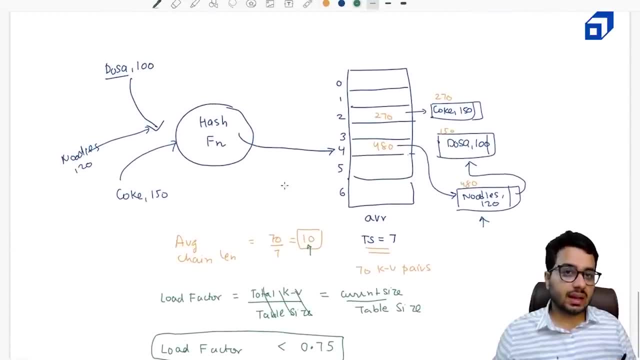 load factor value of 0.75, which means each of my multiple chains has less than one node, which means that my table sizeatu m number of keys i want to put. so if i want to put, let's say, 100 keys, then my table size 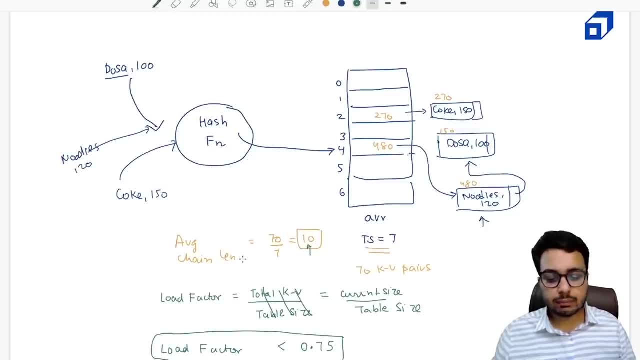 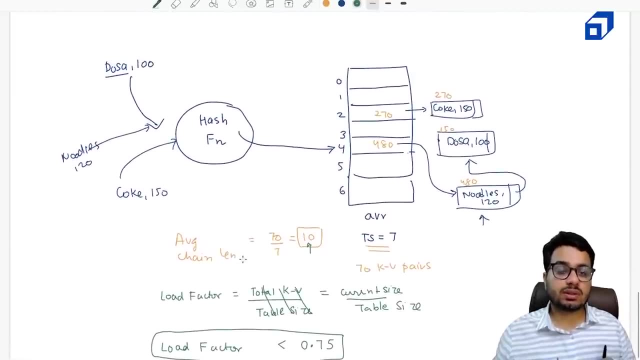 could be of the order 150, right? something of that sort. right, so that is something we need to ensure right now. how do we ensure that our table grows dynamically as the data in the table is increasing? right, one thing you can do is, if you have an idea, that, okay, i'm going to. 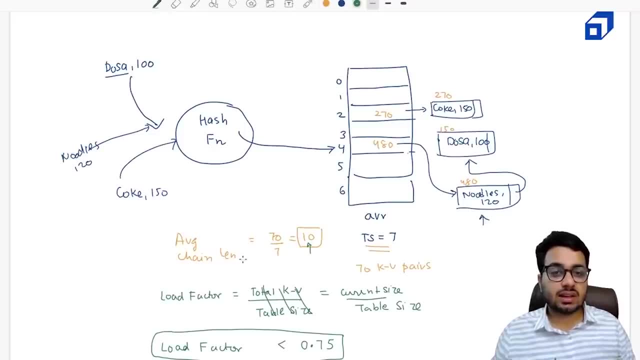 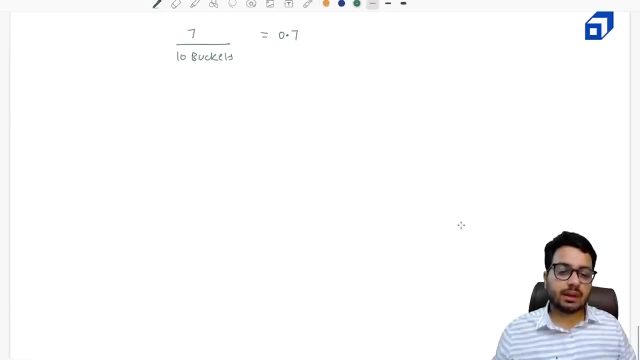 insert somewhere around 70 keys, you can initialize your table size um around 100, okay. so generally it is a prime number, right? so if it could be like 103, something of that sort, right? or 107, right? so you need to ensure that if it is a prime number, it it ensures a slightly better distribution, right. 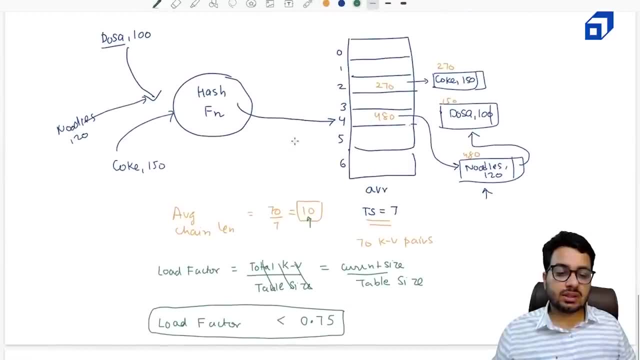 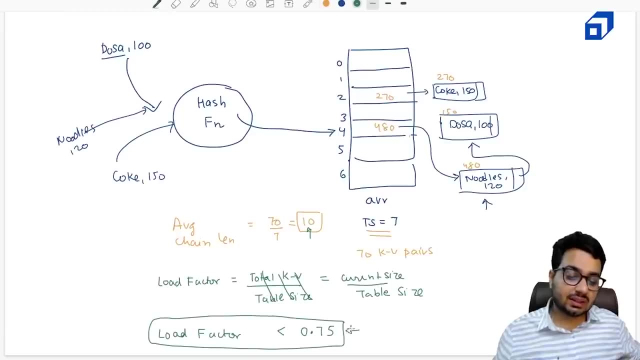 of the keys, right. so what i'm going to do, i'm going to do insertions and i'm going to show you how the load factor is going to change and what happens if the load factor exceeds the certain threshold. so, going back, i'm going to discuss. 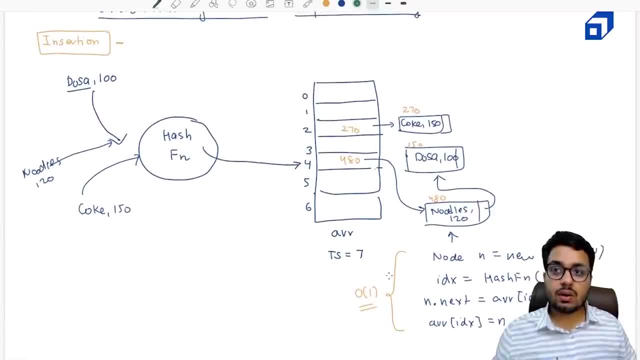 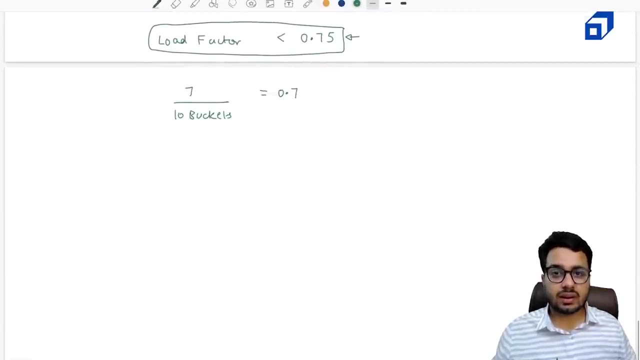 the insertion logic once again. and now, apart from doing the insertion in the chain, we will also discuss the concept of rehashing, and how do we increase the table size dynamically? let us talk about rehashing according to the load factor. let us talk about rehashing right, so rehashing. 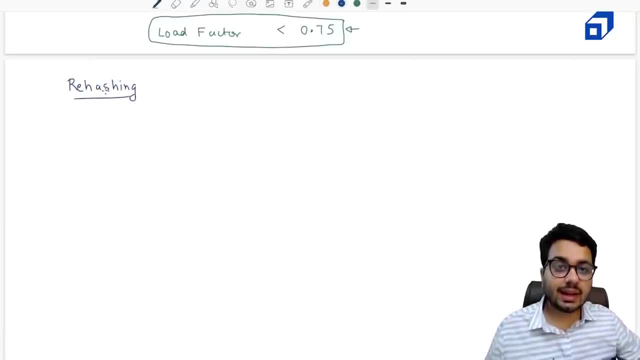 is a mechanism that is going to help us expand the table size and bring down the load factor. let us try to understand insertion and rehashing procedure with the example. okay, for example now suppose i have a table which is of size seven, zero, one, two, three, four, five, six. right now i'm going to insert certain key value pairs. 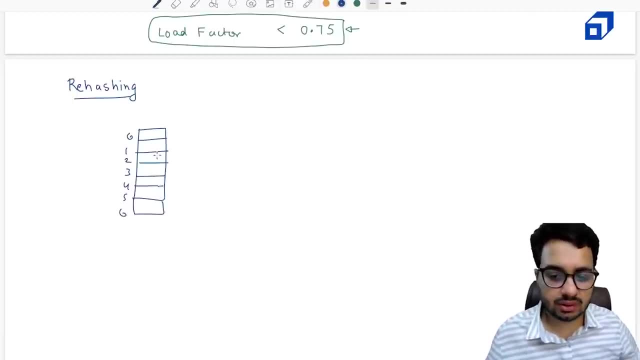 inside it and i will calculate the load factor during the insertion process. for example, i insert a right, so the locations are decided by the load factor, and i will calculate the load factor during the insertion process. for example, i insert a right, so the locations are decided by the load factor. 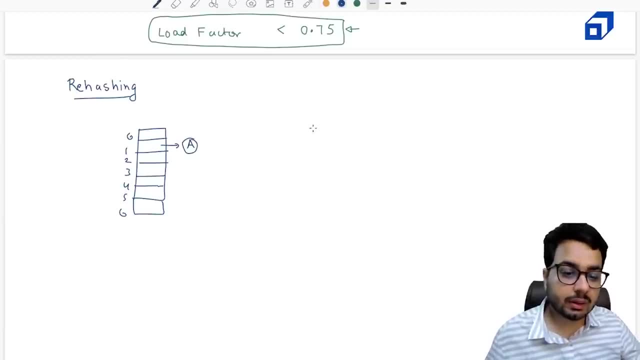 inside it by the hash index. so now the load factor will be 1 upon 7, which is 0.14, right, which is well below the threshold. okay, so our threshold is, let's say, 0.75, so it is below the threshold. i will not do anything. that means, on an average, every bucket has 0.114 elements inside it. 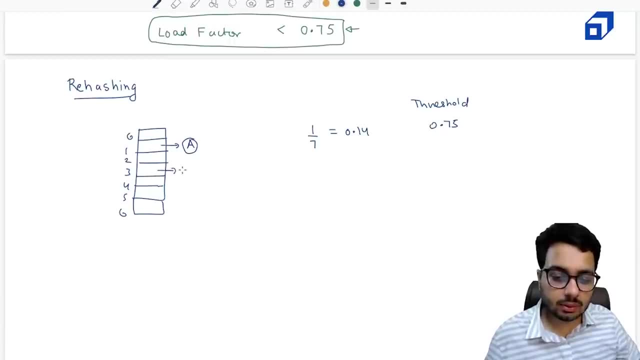 right, if i say okay, i will insert b, maybe it goes here. now my load factor is 2 by 7, which is about 0.28. right, then i insert c. maybe a collision happens and c goes here, but then on an average each bucket has now 0.42 elements, so it is 3 by 7. that is my load vector, right, and maybe i insert d. 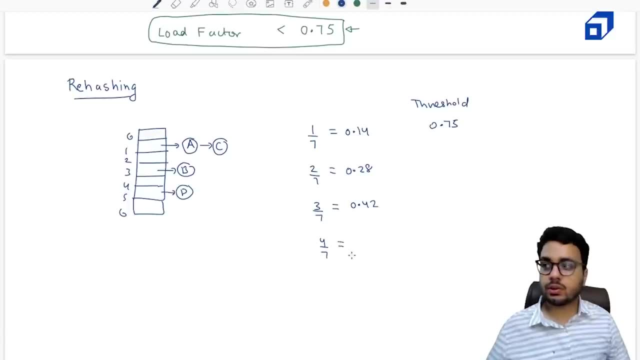 so it's going to be 4 by 7, right? so it's going to be around 0.56. right, so it's it's around 0.57 on the calculator. and similarly, if i insert, let's say e, maybe e goes here. so it is 5 by 7, it's going to be around 0.71. it is still below the threshold. then, if i insert the, 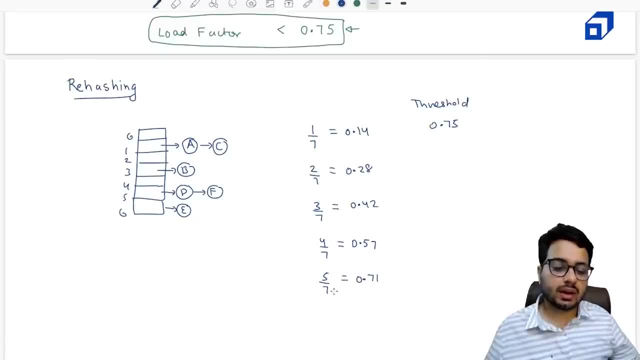 sixth element, maybe if it goes here and it collides right. so it's going to be 6 by 7, which is around 0.85. now, at this point, what do i see? i see that the load factor right has reached 0.85. that means it is close to 1. that means, on an average, every bucket has around 1.5. 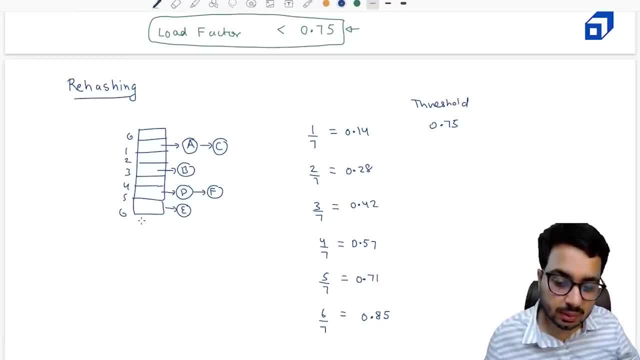 1 element each right. it is the time to grow the table, right. so what is the table? this is my table. i want to grow this table. i want to make it bigger, right? so what i will do? i will create a new table, or a new array, right, which is approximately double of the given size, right? so maybe this table size. 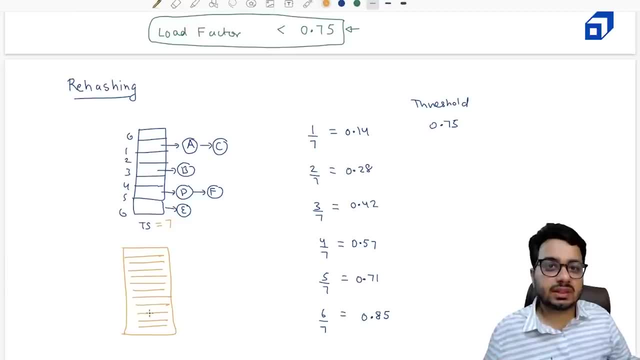 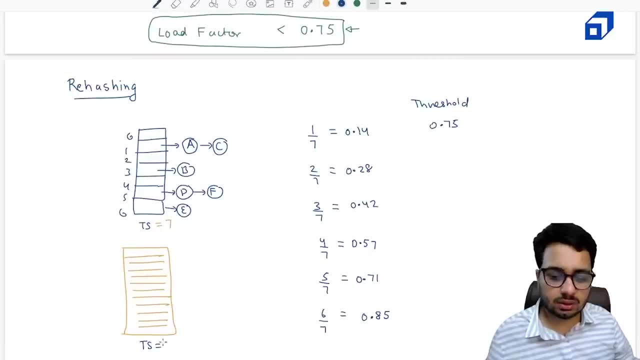 what is the nearest prime number close to 14? it could be 13 also. it could be 17 also. let's say, this is 17, right? so i'm taking the next biggest prime number right now. what i will do. this table is empty, right, this table is empty and my goal is to remove all the entries from this hash table. 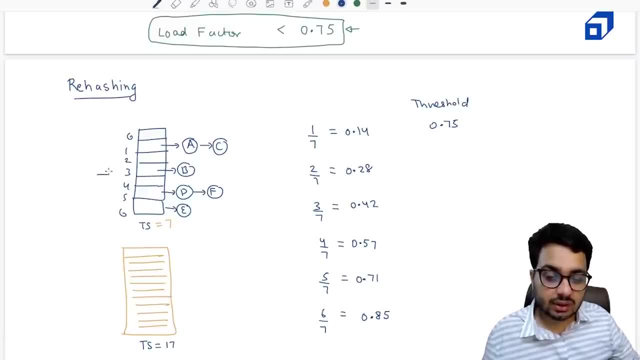 and put it into this hash table. now you might ask why can't we, uh, use this hash table right? the reason being, um, your table size has changed and your hash index that we saw right, so we saw it was a weighted sum. okay, it was a weighted sum of, um, the letters of the string. 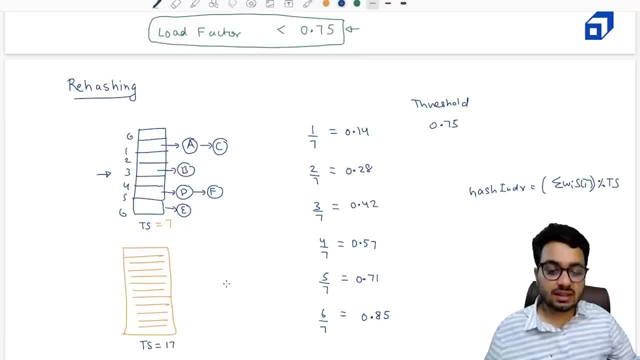 taken with taken mod with the table size. now table size has changed, so my hashing will also change. that means if i now insert a, earlier it was going at position one. it might go at certain some other position. so a might go here, c might go here, b might go here and d might go here. and since the 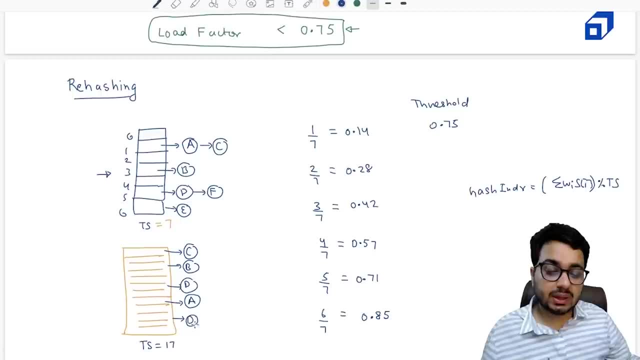 number of buckets they have increased. that means my distribution, uh, will also change, and it is possible that the number of collisions that are happening they might reduce. right, so what i have to do, i have to do rehashing. so this is what rehashing is. so we have created a table of size, double the capacity, right, and we we 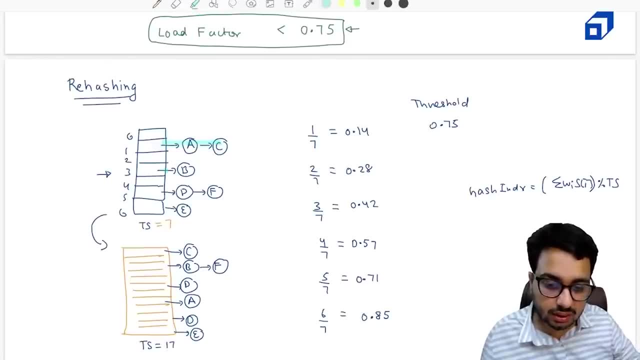 iterated over every chain in the original table, every node we added again into the hash table. once we are done what we will do, we will delete this from the memory. this will be cleared off and now my hash table is going to refer to this tip right now in this table, if i compute the load factor, okay, if i. 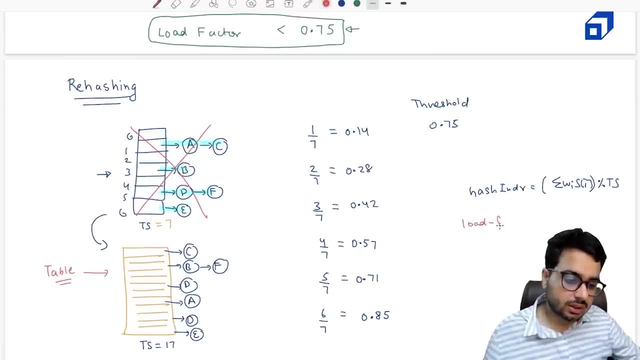 compute the load factor now, this will be much, much lower than 0.855, because it was now 6 by 7. now this will be 6 by 17.. so if i calculate this value 6 upon 17 broken Flower Is Первung. 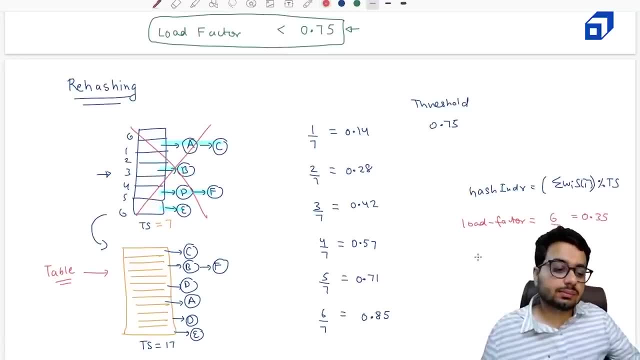 yeah, this value comes out to be 0.35, 0.35 light, so i can keep on adding more entries into this table right again. if, again, it exceeds the threshold, what i will do: i will execute rehashing once again right now. what i am trying to say is that this rehashing is a special mechanism that will be. 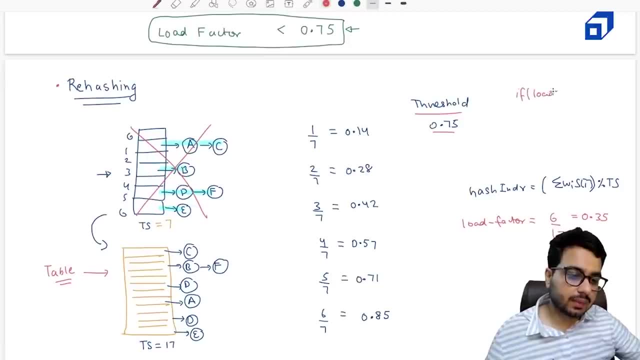 condition, like: if my load vector exceeds the certain threshold, i will have to call the rehash method from the insert function, right? so this is something i will show you in the code as well, right? but i hope you're understanding the reason of rehashing, right? what is importance of rehashing? 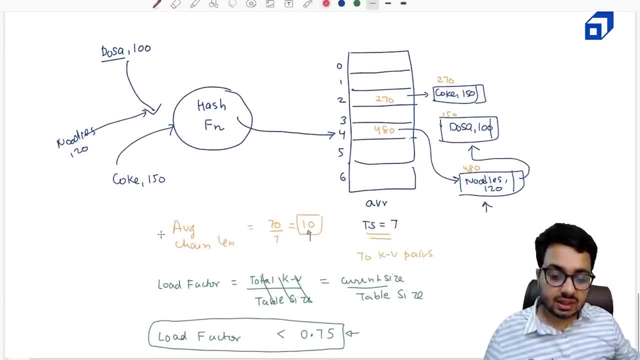 so if you have done rehashing right, can i say the average chain length will be always less than one. that means, on an average, no bucket has more than one node, right? so it might happen that some buckets may have zero nodes, some buckets might may have two or three nodes, but i'm going to say this: 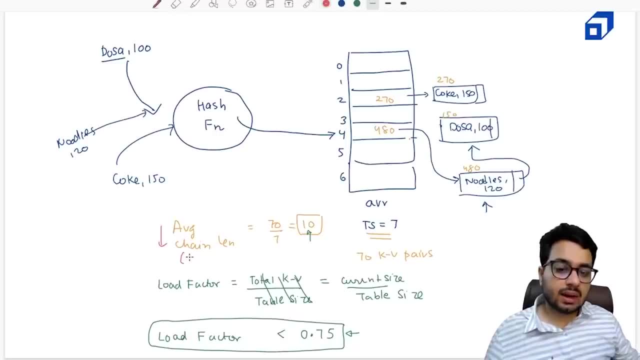 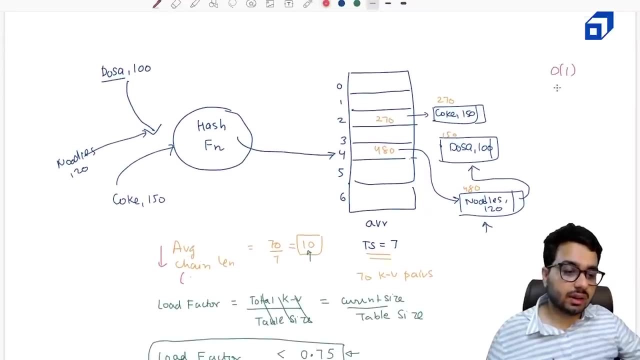 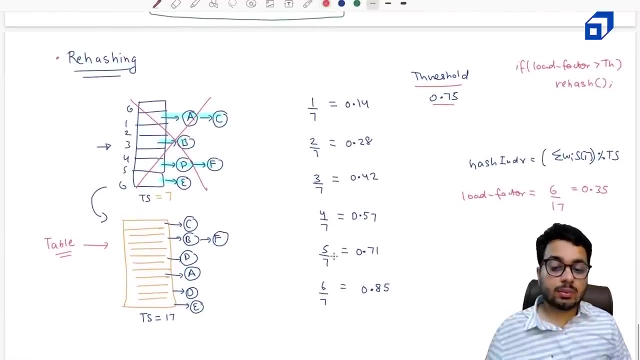 average chain length will be a very small number and it it is, it can be treated as constant. so that is why we say that our search is order one on average right, order one on average right. that is what what my search operation will be right now. another point: what is the? 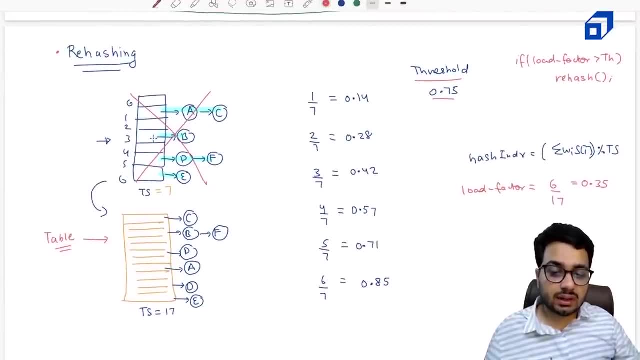 complexity of rehashing, right. so of course we have to iterate on the entire table and put all the keys into the new table. so it it is going to take order of n time, right then, how my insertion can be order of one. so if you look carefully, this rehashing is not happening again and again. so 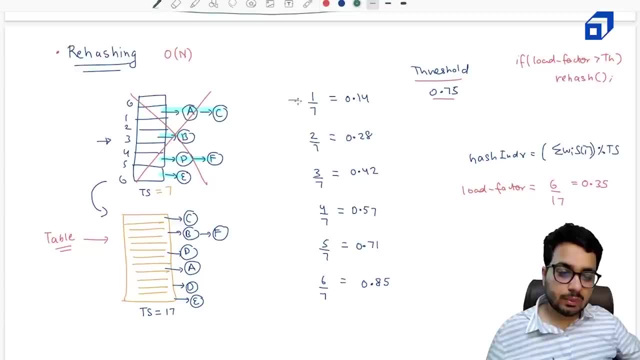 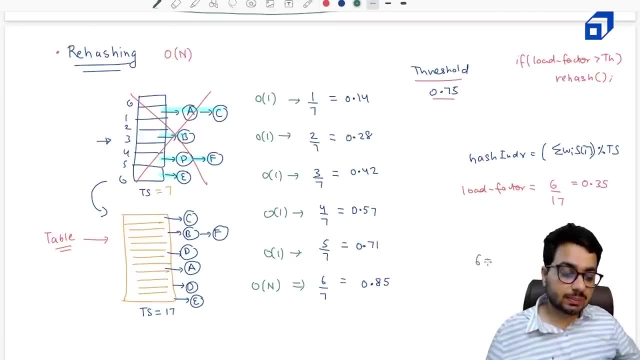 to hit order of n time right. so can i say that for six elements i spent it constant time, but for one element i spent order n time right. so if i talk about on average how much time i spent on each element, so again, if i take an average it it's like a worst case. right inserting six is like a worst. 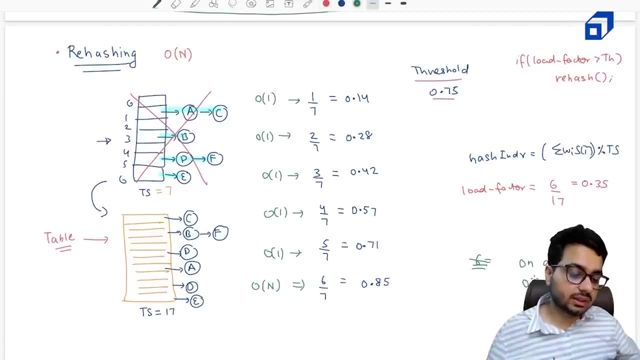 case, worst case: yes, it can go order of n, but on an average we are spending order of one time in doing an insertion. right, you might ask how can i bring down the time of rehashing? so if you know that, okay, i am going to insert about 500 keys. so you make sure in the beginning that your table 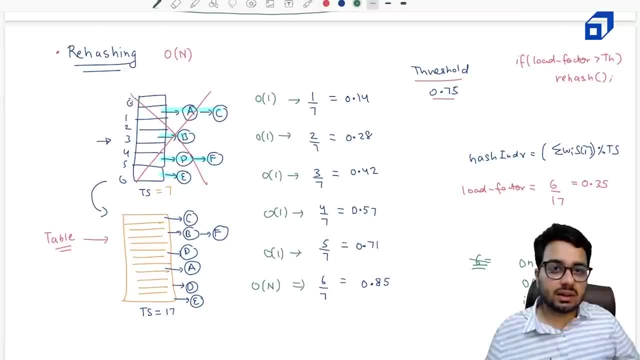 size is big enough so that rehashing is never triggered, okay, or it is triggered very, very rare, right? so the correct way to do it is initialize a large enough table. okay, it should not be too big, that you're using too much of memory, and so you have to make a balance between effective memory, memory. 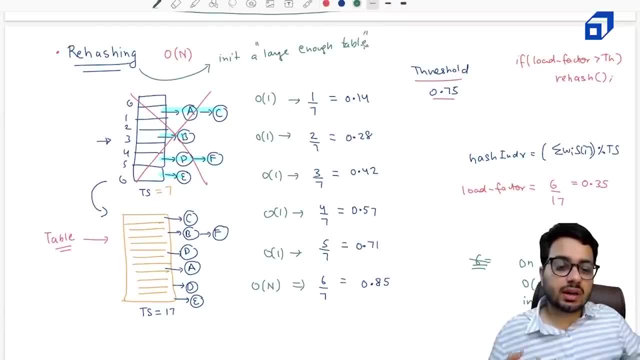 utilization. so you should know from the historic data, okay, how. how big table should be sufficient. so if you're storing phone contacts, you know in general people might have 500 to 1000 contacts, so you can initialize a table of the size around 1000, right? so it is just large enough, just large. 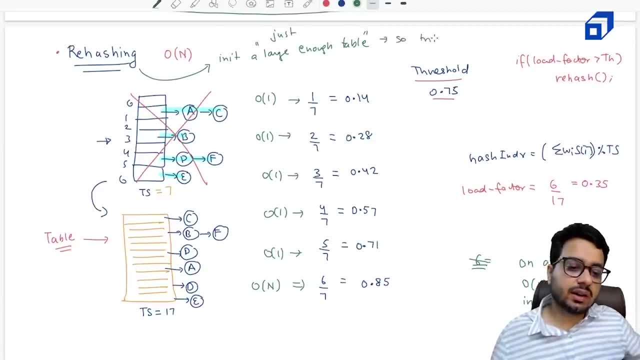 enough so that rehashing is never triggered, right, or it is triggered, maybe just once, right, it is never triggered, right. so this is something we can do right to make sure that almost every insertion is order one, right. so i hope you understood the concept of rehashing and i'll 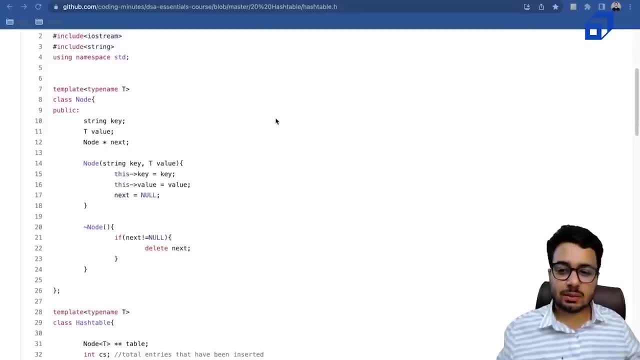 show you in the code as well. let us discuss the implementation of hash table. so i'm using c++, but you can also use java or any other language to map the same functionality in in your own language, right? so first of all, i discussed that hash table is a table and in this table i have 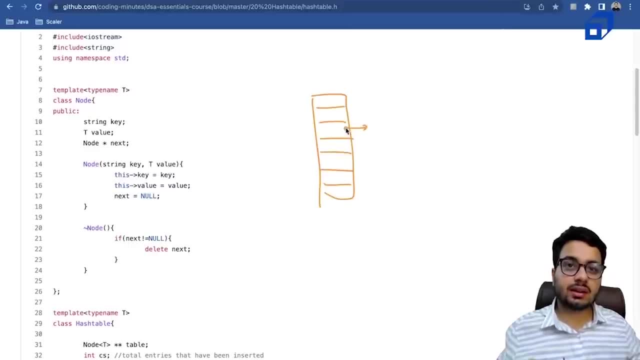 this table is going to contain the address of it. it is going to contain the head of the link list. so link list is made up of nodes, so node will store key, a value and the next field, right. so that is what i've defined in the node structure. so i'm using templated classes, so it's like generics. 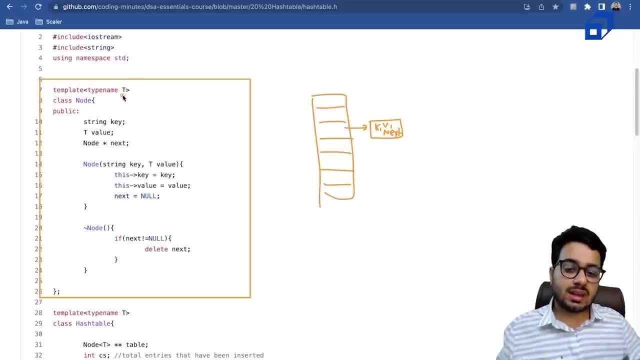 in java and templates in c++. these templates allow me to hold data of any t type in my node. right for keeping things simple, i'm assuming that my key is always a string, but it can be of other data types as well. for that also you need to use templated classes and you need to provide a way to convert that data type. 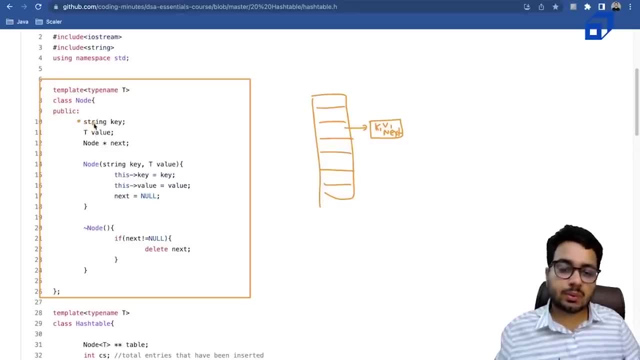 into a hash index value, right? so for now i'm dealing with strings only, but i'm saying the value can be of any type. it could be int, it could be string, it could be float, because we are not computing any hash on the value, we are just going to store that value as it is. and third thing is: 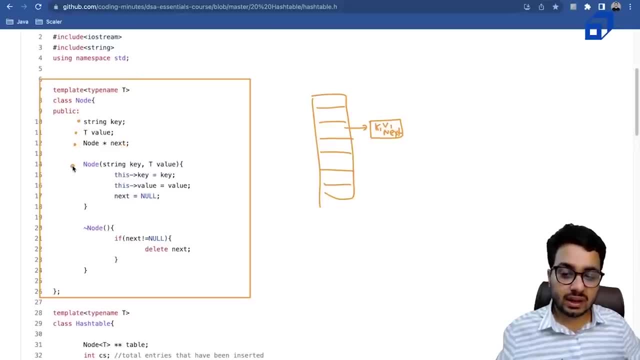 the next property, that is, of the node right. whenever i initialize the node, i set the value of key, i set the value, which is the value, and by default i set the next as now right, and this is my constructor. and if i want to delete a node, so this deletion will happen. if i am deleting a certain value or i'm doing, 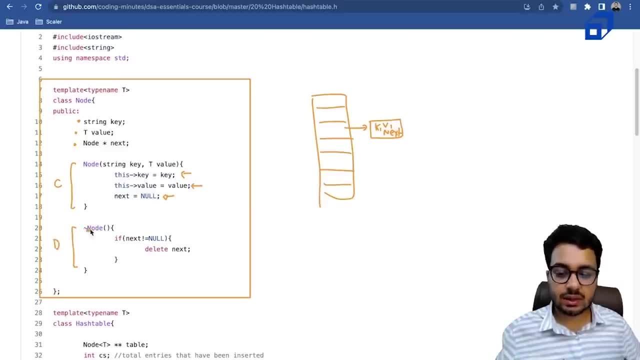 rehashing and i want to delete some data. right, this is actually a destructor which says that if next is not null, delete next. so basically it is a recursive way of deleting the node, right? so that means if i uh make a call at this point, it says, okay, if i'm going to delete this node and if the 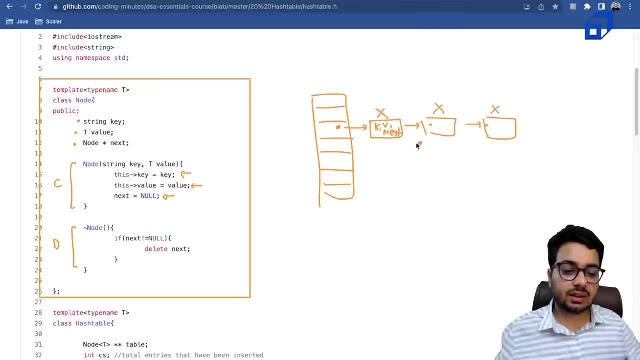 next is not null, first delete it. if the next is not null, first delete it. so it? it's a way in which i can delete the entire chain at once, right? so this is something, um, which you can also like. it's uh, it can be implemented in other way also, right? so you might not necessarily do the same thing. 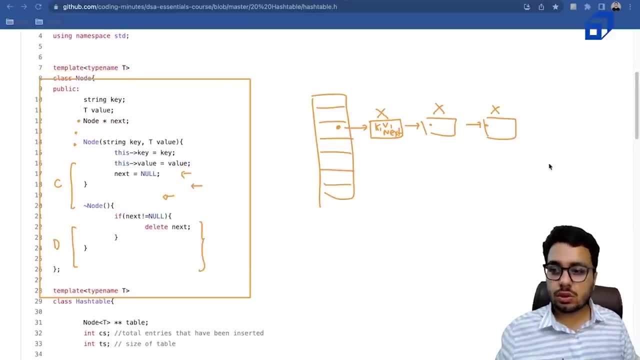 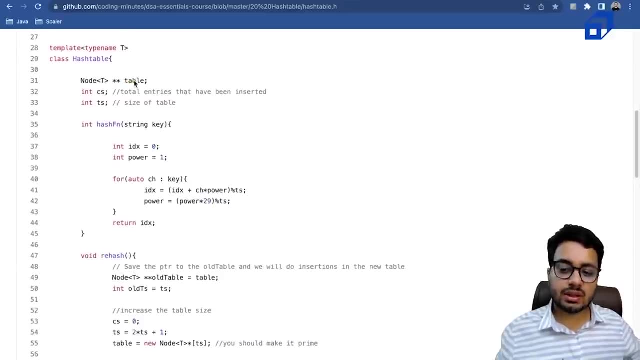 but in my case, i'm doing it, i will show, tell you why, right? so, uh, that is about the node constructor. and now let us come to the hash table class. right? what i have done, i am actually keeping a two dynamic array called table. so table is referring to an array, right? so you might ask why star? star, because, see, uh, each, each bucket in. 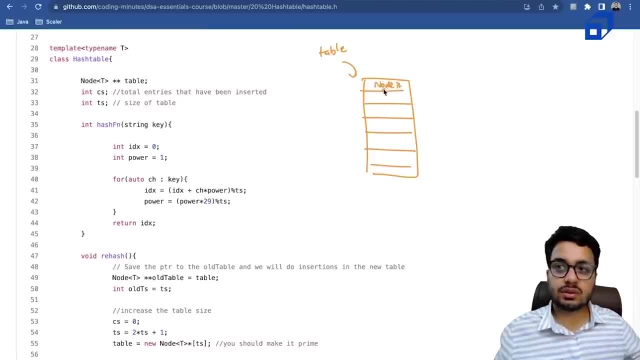 this array is going to hold an address of the node, so it is of the type node star. right. and what is table? table is a pointer to an array of pointers. right because each bucket is going to point to the head of the linked list, so each bucket is of the type node star, hence the type. 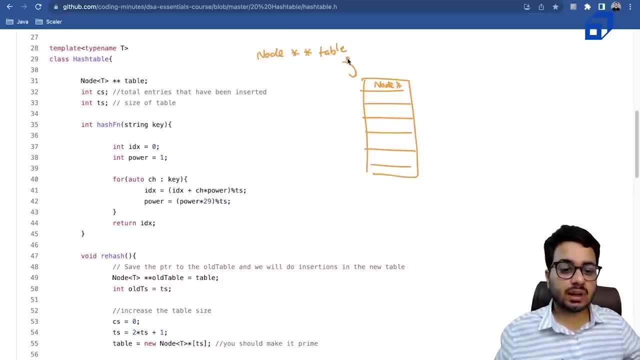 of the table is node star, star. right, it is going to be a dynamic array referring to an array of pointers. okay, so i have a table which is not initialized at the moment. i have current size, i have table size, so current size will be zero in the beginning. so i will show you. uh, the constructor for this. 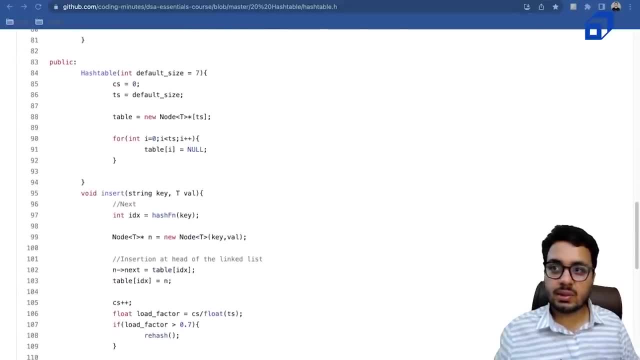 yeah, this is the constructor. so whenever a new hash table is created, right, so current size is set to zero. table size is set to default size. i'm taking a parameter with the default value of seven. so if user gives me, let's say, i want a table size of one zero seven, it will be one zero seven. but if 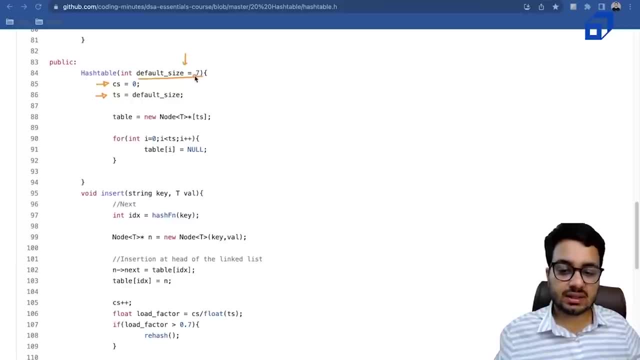 nothing is given by default. i'm taking it very small and it is seven, right, then i initialize my table array. so table is an array that points to an array of node star and this is of size, table size. so these many buckets i have initialized and by default, in every bucket i am putting a value null. 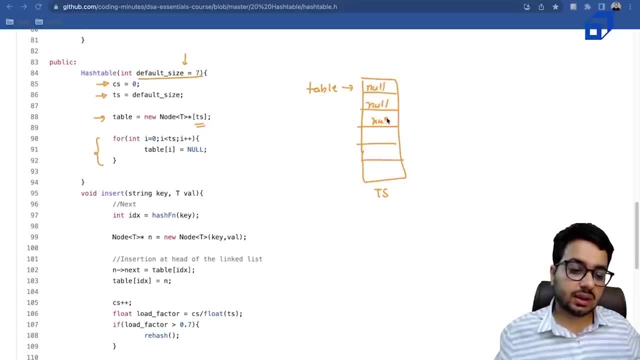 right? so this is null. this is null. this is null, right? so instead of having garbage, it is better to initialize everything with null. that is how that hash table has been initialized. i hope you don't have any doubts till now. now comes the interesting method that is insertion. 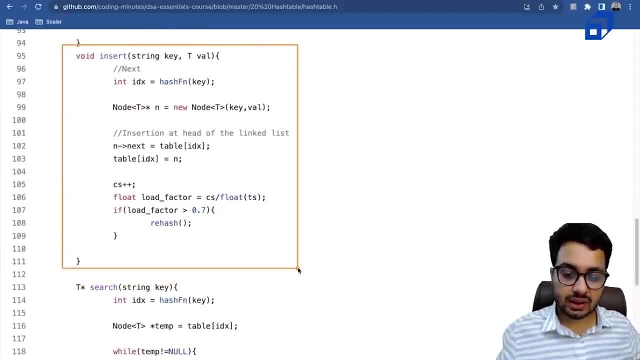 right now, if i want to insert something right, so i, my table is ready, so table is here, my hash function is also ready. okay, i'll show you the hash function. let's say i want to insert dosa, comma 100. what do i do? i will show you the hash function. let us understand the insert. so my key, that is: 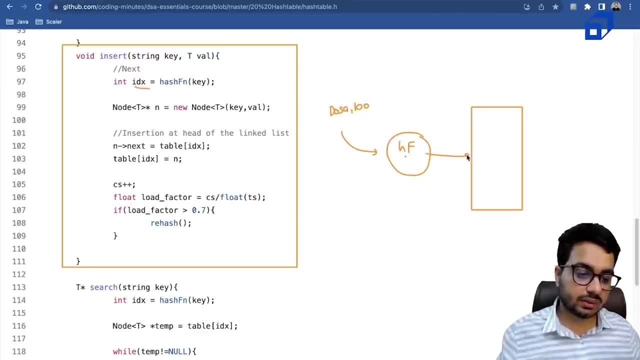 dosa. it goes through the hash function and i get an index. so maybe the index is four right at this index. what do i do? i will create a new node. so i say, okay, there is a new node called n, which is dosa, comma 100. in this line i do this: 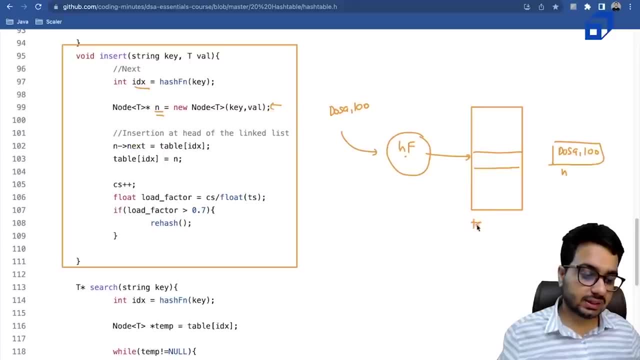 work. and i say n dot next, this is equal to table of index. so table and this is index. so n dot next will point to whatever this is pointing to. so it is currently pointing to null. the next starts pointing to null, right. then i say table of index is equal to n, so this index is going to hold the. 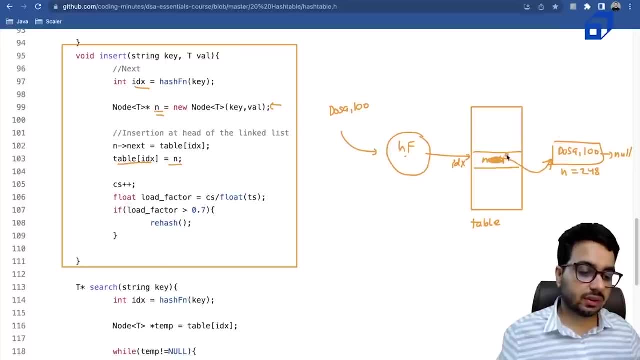 value n. so n is, let's say, 248. that is the index of index. so this index is going to hold the value n, so n is, let's say, 248, the address of this node. so it is going to store 2 for it, right? so this is how this node gets. 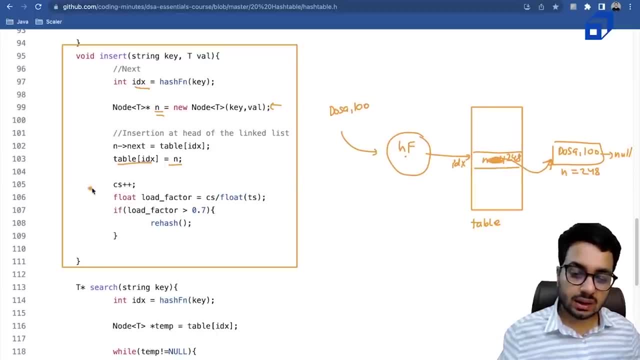 attached to the beginning of the table: current size plus plus. so current size becomes 1, then i compute load factor, so which is 1 upon 7.. is it greater than 0.7? the answer is no right. so if it becomes, then i will trigger rehash. i will show rehash method also right. so this is about the 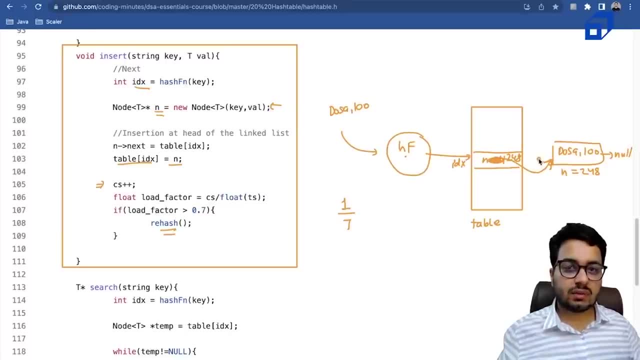 insert functionality right. so i hope you're getting it. let's say, i'm inserting one more node which at the index 4.. so i just want to insert one more node which at the index 4. so i just want to insert one more node which at the index 4. so i just want to insert one more node which at the index 4. so i just want. 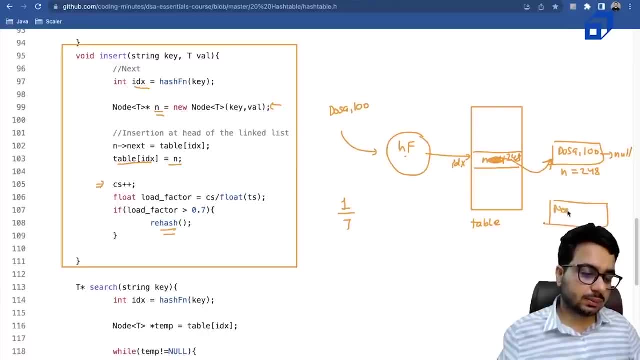 to show you how the chaining is going to work, let's say i inserted noodles and for noodles also i got an index 4.. so noodles, comma 120. i created a new node called n. right, then i said n dot next is equal to table of index. table of index is storing this value, so noodles starts pointing. 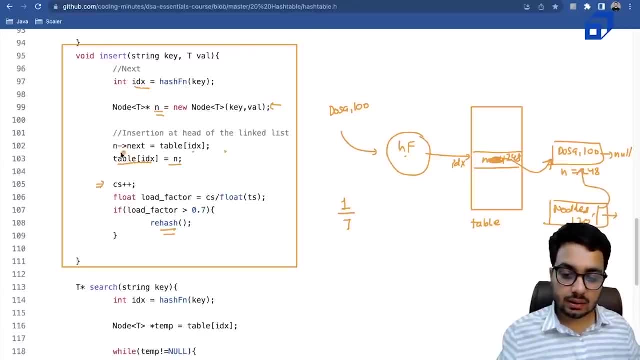 to this value, right, and table of index is equal to n, so this connection is broken and this starts pointing to this node, right. so you can see, in a way we are forming a chain in which noodles is being inserted at the head of the linked list, right. so this is nothing but insertion at the 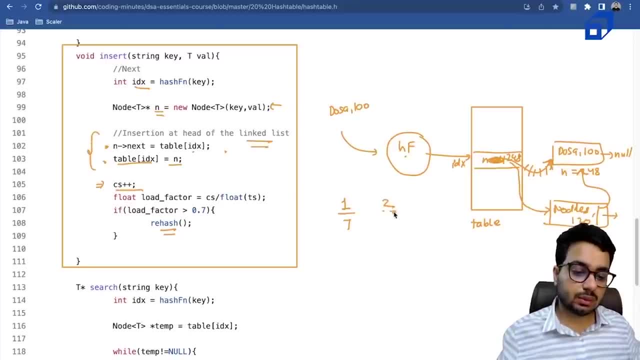 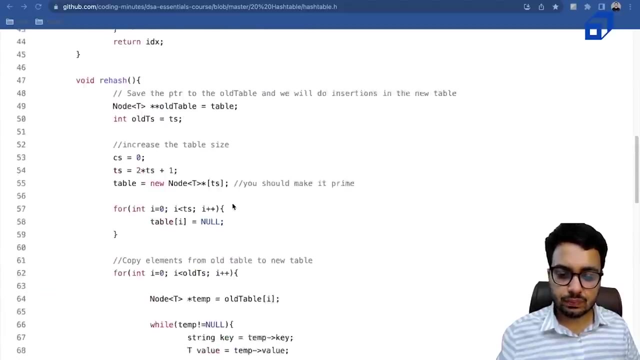 head of the linked list. current size plus plus. so current size is 2. load vector is 2 by 7, which is again less than 0.7. so hence i do not trigger rehash at this moment. right, so i hope you insert. you understood the insert method. next i want to show you the hash function that i've used here. 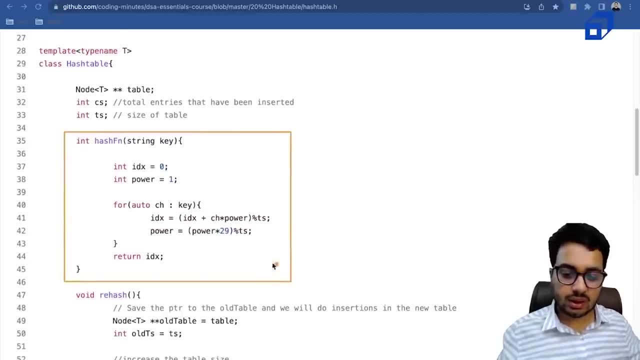 the hash function. i've made it as a private. so what i'm doing, i'm simply multiplying the numbers. let's say the word is dosa. what i'm doing, i'm iterating over this and i'm multiplying it with powers of 29, so it is one. so initially it is multiplied with one. then in the next iteration, 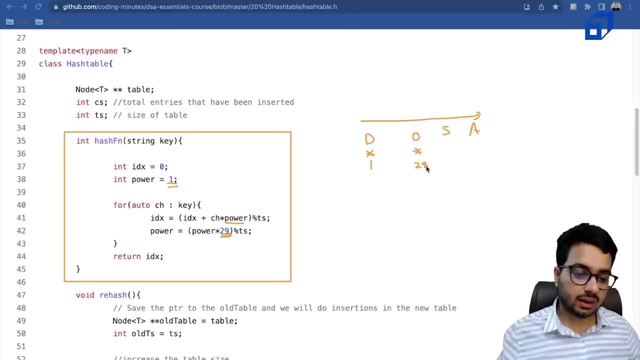 power becomes into 29, into 29. next time it becomes power becomes again power into 29, so it gets multiplied with 29 square and again it becomes 29 cube, right? so in order to avoid overflow, i'm doing the mod at each step, because if you take mod at the last, 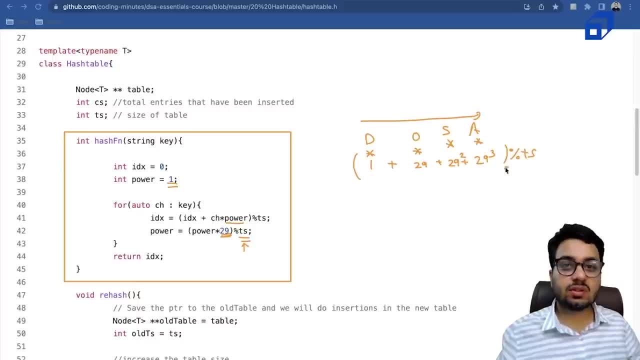 uh, or if you take mod at each step. you know this is the property of mod, so mod can be taken at each step as well. so this is a better thing to do because it helps us to avoid overflow. right, i'm taking a mod with power also and i'm taking the mod in the answer also, so i get an index. 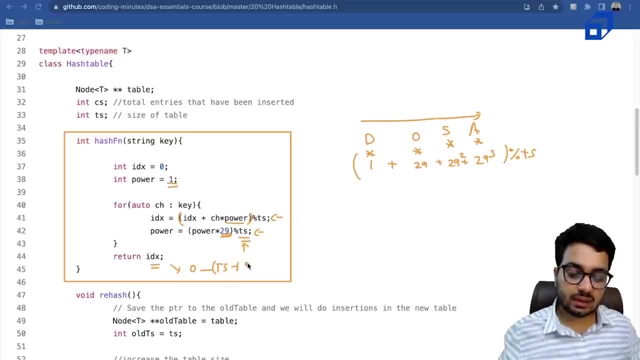 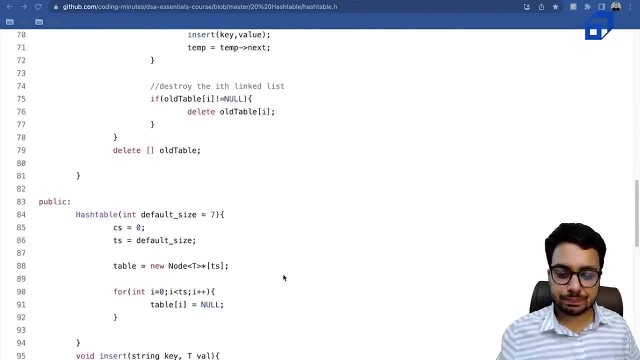 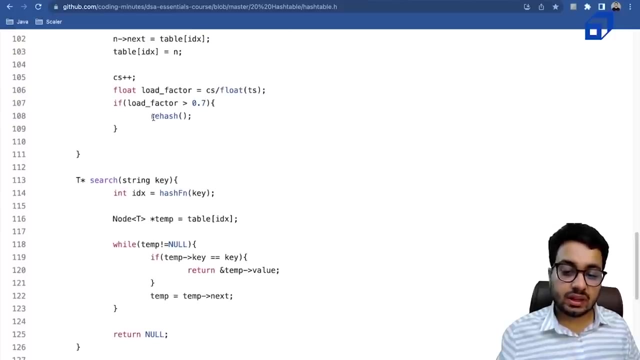 which is in the range zero to table size minus one, because i'm doing a mod with table size. so i hope start the hash function as well. right now, what i need to do is i need to understand the rehash method right. so if we understand the rehash method, our insertion will be complete. 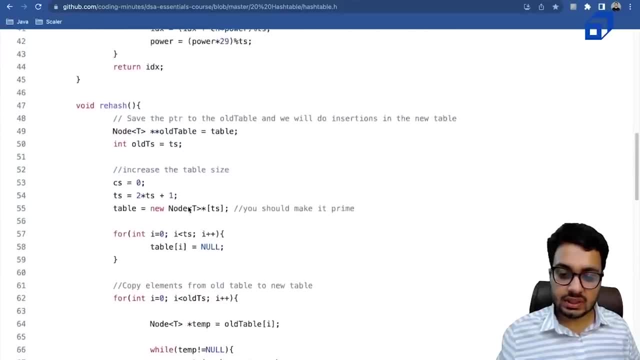 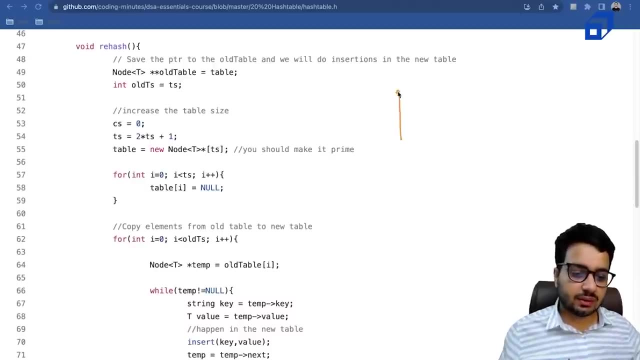 so i have written a rehash method as well, which is actually a private method as well. so what i'm doing in my rehash method? that suppose i have a old table like the actual table. in this i have inserted some keys. let's say a, b is there, c and d is there. what do? 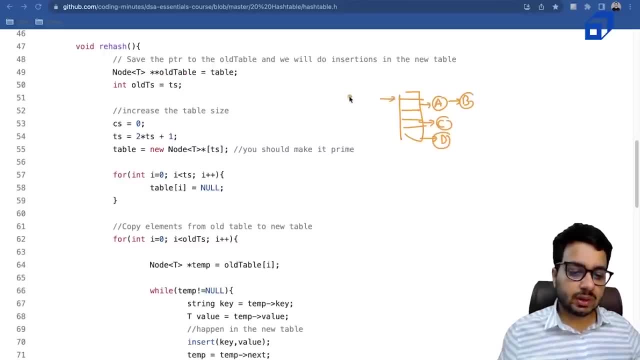 i do. i say, okay, old table is going to point to table. so this was my table. now old table is pointing to this table. i create a new table, okay, which is almost double of the previous size, plus one. i'm just making it as a odd number instead of making it as a prime number. 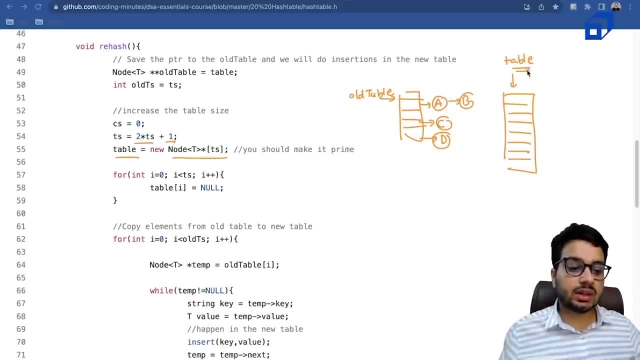 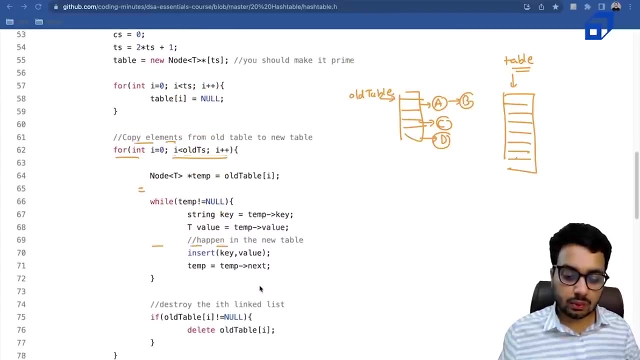 so i'm saying: this is my table now, which is also the data. member of the class, right? so? so what do i do? i initialize it with null, so all these values are set to null. and then what i do? i copy elements from the old table. so i iterate over the old table. and how do? 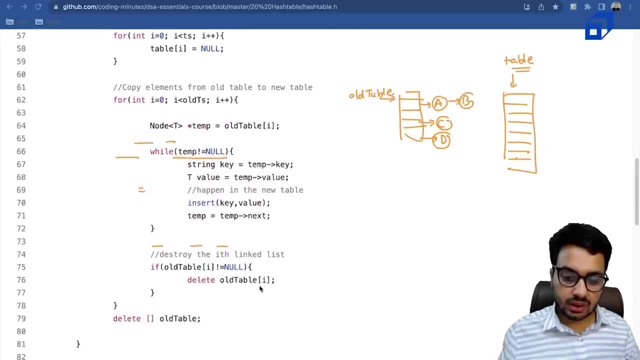 i do the work. let me show you. so i do it like this: i take a temp variable which is the ith row, so temp starts from here. okay, temp is referring to the head of the linked list and while temp is not null, so i iterate over the link list and i'll execute. flow to the loop. 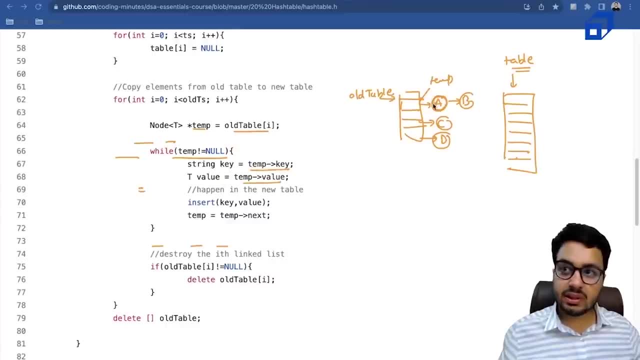 so that's super simple. so i do the rest of it and i'm going to do some stuff like reference: copy the key, i copy the value. so i say, okay, give me this key value pair and i call the insert method. so insert method. we know, by default it acts on the table, which is the data. member of. 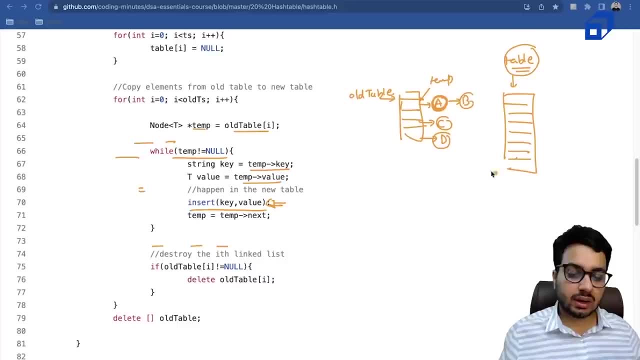 the class. so it is going to insert automatically in the new table right and temp goes as next. so temp comes to this node again. i copy b, i and insert it in the new table right. so once it is done i make a destructor call. if old table of i is not null, delete old table of i. so in java there. 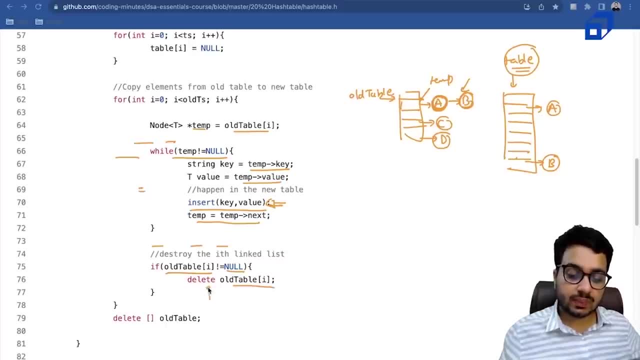 is a concept of garbage collection, but in c++ we have to use explicitly, we have to invoke the destruction of this, this entire linked list, by saying: delete old table of i. so i initiate a destructor call from here which makes a call to a is being, it being a recursive destructor. a makes. 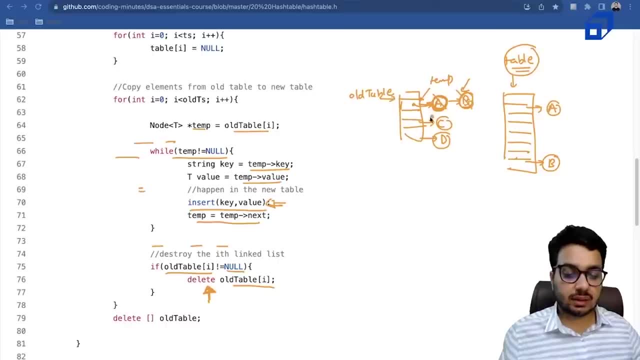 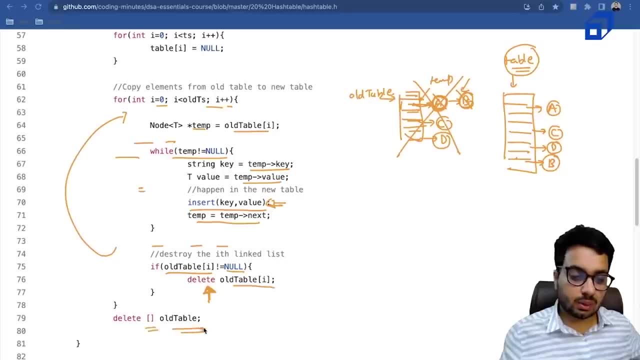 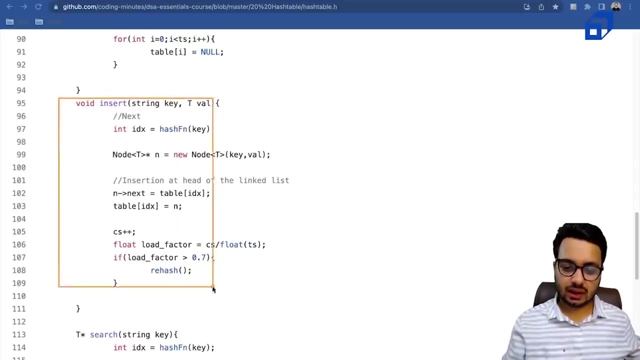 and finally i say okay, i want to delete the array. that is old table. so i also want to clear up this memory. so i say: delete old table. this old table is gone and since it is a local variable, this is also destroyed, right. so till now you have seen the insert functionality and we discussed that. uh, 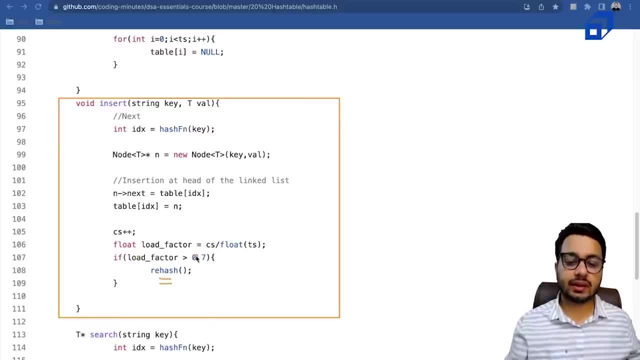 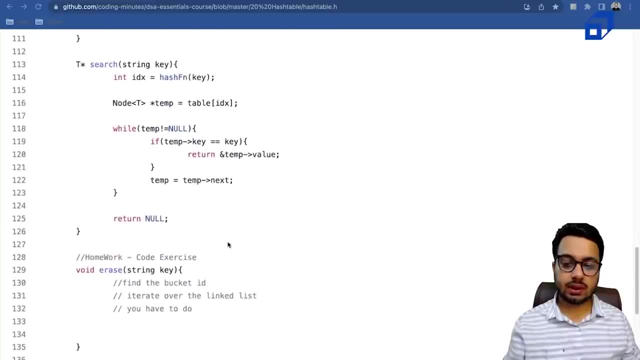 the function rehash will be triggered from the insert. whenever load factor exceeds the load factor, it's the threshold. okay, so we basically double the table size here. right now let us talk about searching a little bit. how do we actually do searching in a hash table? so searching is pretty. 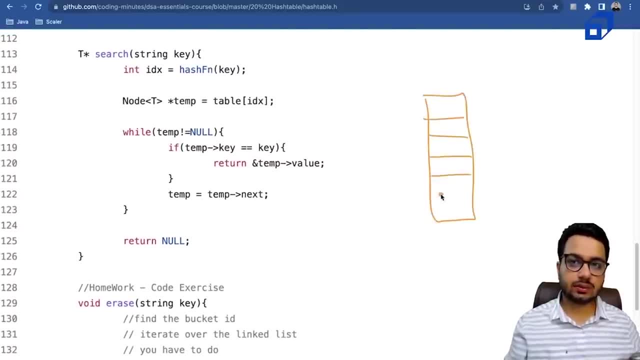 easy. so if you have a hash table right and you want to search for a certain key- let's say dosa, so that key will go through the hash function. the hash function will tell you the bucket. so maybe this is the index of the bucket and in this bucket there might be a chain in which dosa could be one. 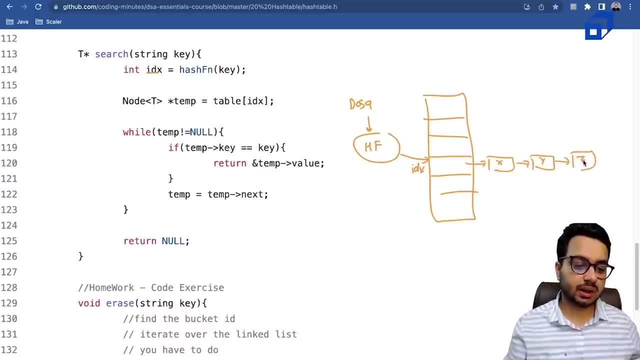 of the item, right? so maybe this is some x i, some y item, some red item, so you need to iterate on this chain linearly, right? so i start temp from this node, while temp is not null, while i do not hit the end of the chain. i compare is the key of 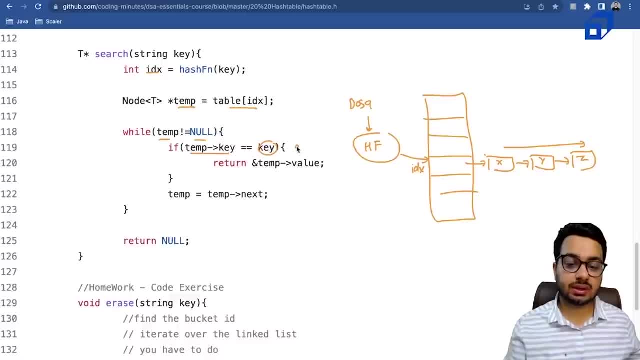 this node matches with the given key. if i'm that, i'm searching. so if that happens, i return the value. otherwise i go to the next node. if i hit end of the chain, that means i did not found the key, so i return null. in that case, right, this is how searching is done, right?